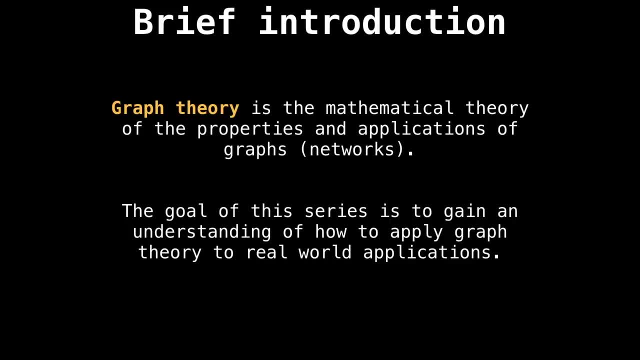 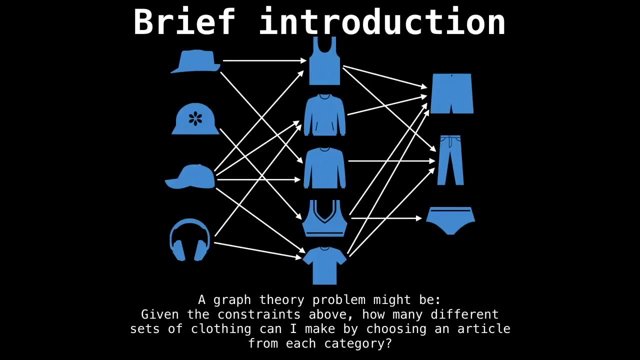 graphs, which common folk or non mathematical folks call networks. This is a very broad topic And my goal with this video series is to teach you how to apply graph theory to real world situations. graphs can be used to represent almost any problem which 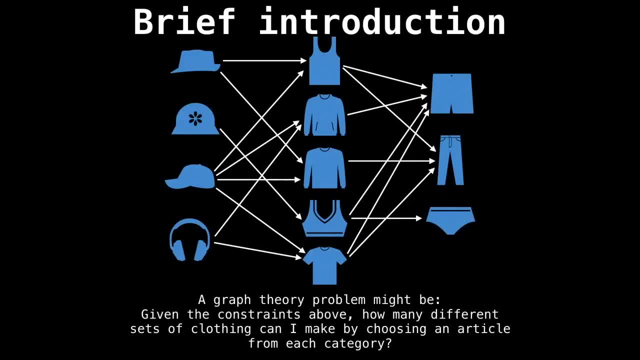 makes them so interesting because they pop up absolutely everywhere. A simple problem that can be phrased as a graph theory problem might be: given the constraints in this picture, how many different sets of clothes can I make, choosing an article from each category? Of course this could. 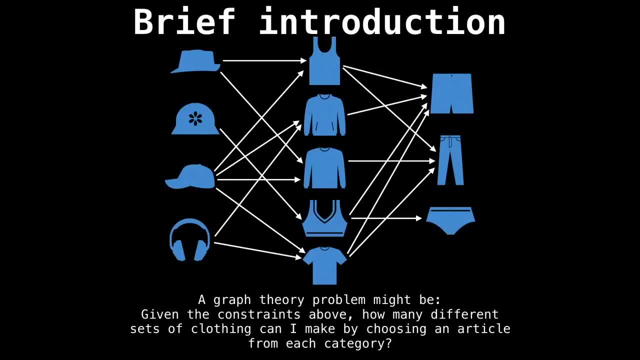 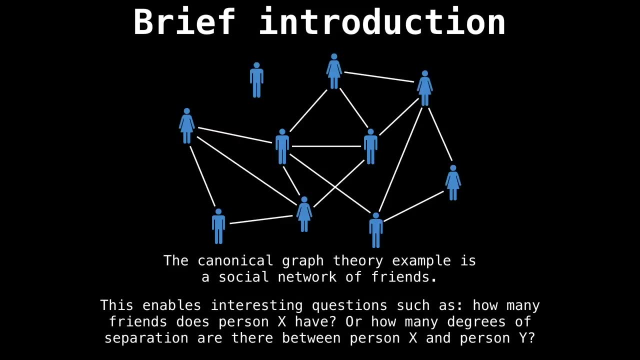 be phrased and solved using only mathematics. But the advantage to graph theory is that it allows us to visualize the problem Using nodes to represent an article of clothing and edges to represent relationships between them. Another canonical example of a graph theory problem is a social network of friends, a graph. 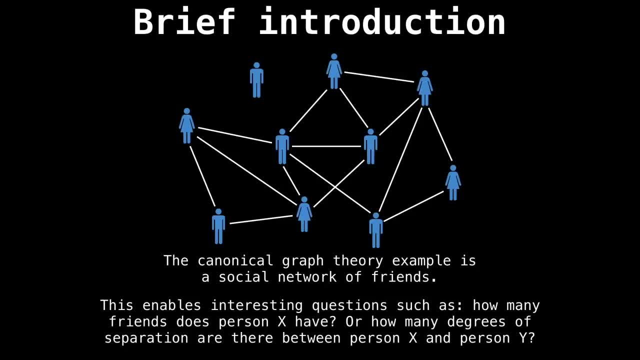 representation enables us to answer interesting questions, such as how many friends this person x have, Or how many degrees of separation are there between person x and person y? Now we have to talk about different types of graphs. Now we have to talk about different types of graphs, For example. 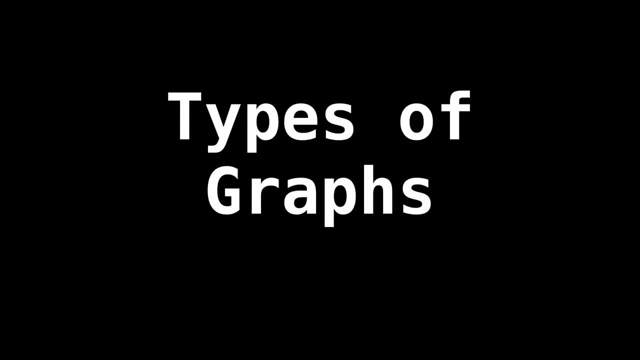 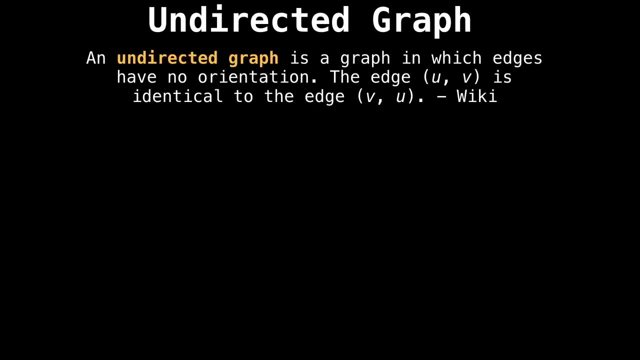 there are many different types of graph representations And it's really important- and I mean really important- to be able to recognize what type of graph you're working with and especially when you're programming and trying to solve a particular problem. This first type of graph is an undirected graph. It's the most simple kind of graph you'll encounter. 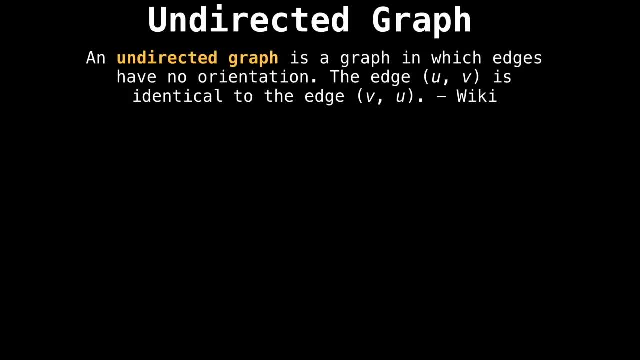 and it is where edges have no orientation, That is, if there's an edge from node u to node v, it is identical To the edge from v to u. For instance, in the following graph, nodes are cities and edges represent bi directional roads, Since if you drive from one city to another, you can always retrace. 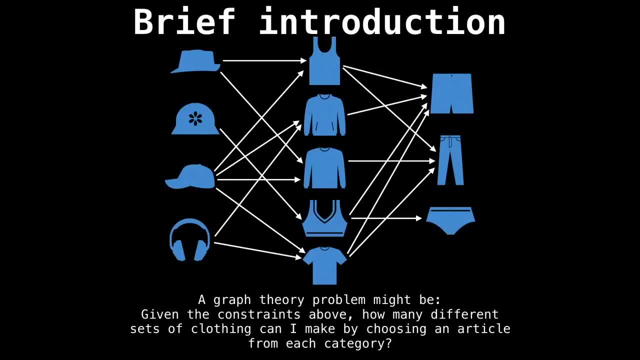 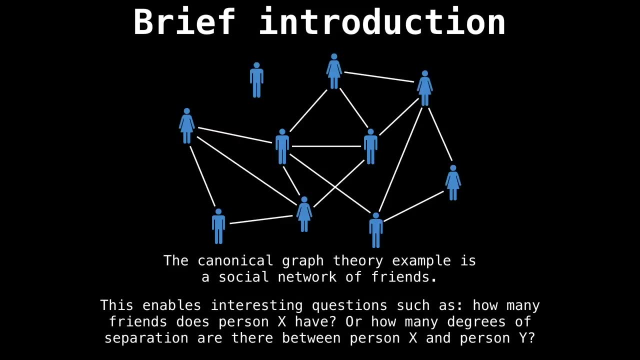 be phrased and solved using only mathematics. But the advantage to graph theory is that it allows us to visualize the problem Using nodes to represent an article of clothing and edges to represent relationships between them. Another canonical example of a graph theory problem is a social network of friends, a graph. 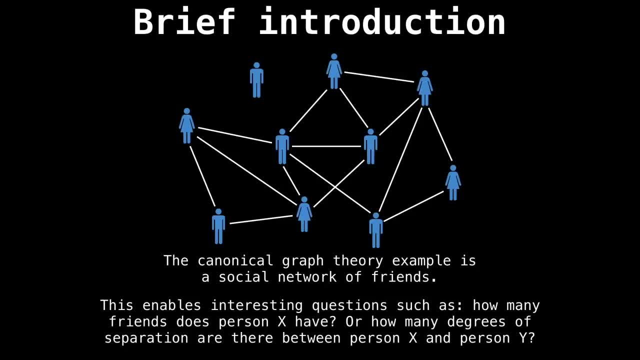 representation enables us to answer interesting questions, such as how many friends this person x have, Or how many degrees of separation are there between person x and person y? Now we have to talk about different types of graphs. Now we have to talk about different types of graphs, For example. 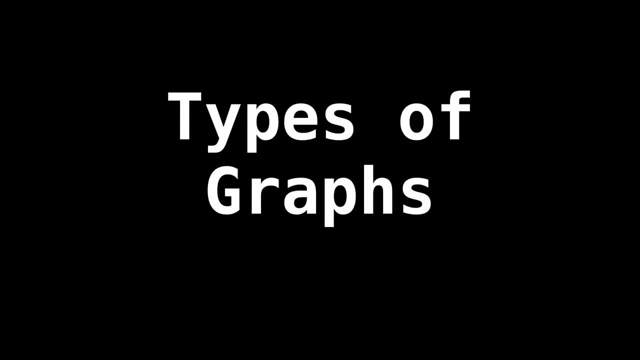 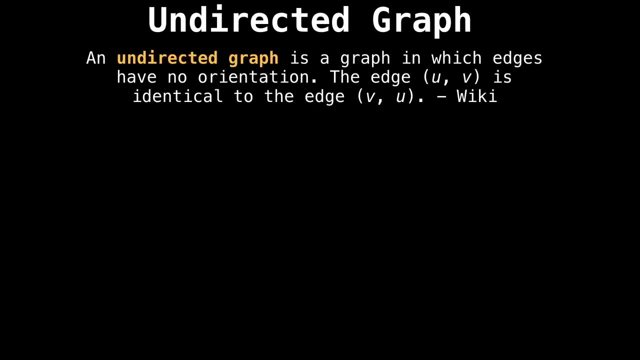 there are many different types of graph representations And it's really important- and I mean really important- to be able to recognize what type of graph you're working with and especially when you're programming and trying to solve a particular problem. This first type of graph is an undirected graph. It's the most simple kind of graph you'll encounter. 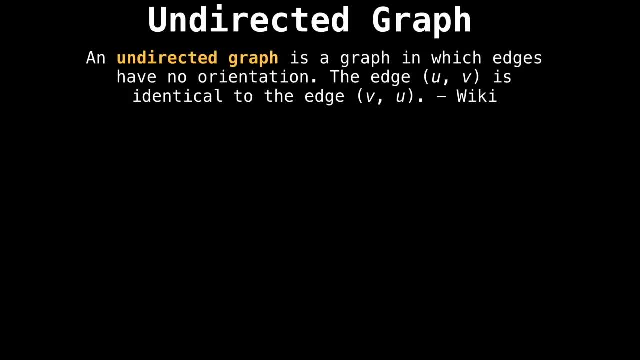 and it is where edges have no orientation, That is, if there's an edge from node u to node v, it is identical To the edge from v to u. For instance, in the following graph, nodes are cities and edges represent bi directional roads, Since if you drive from one city to another, you can always retrace. 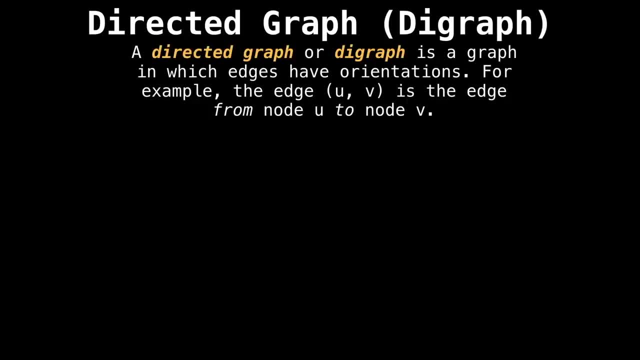 your steps by driving the other way. In contrast to undirected graphs, there are also directed graphs, sometimes called die graphs. In these graphs- you've guessed it- the edges are directed. So if we have an edge from u to v, then you can only go from node u to node v. 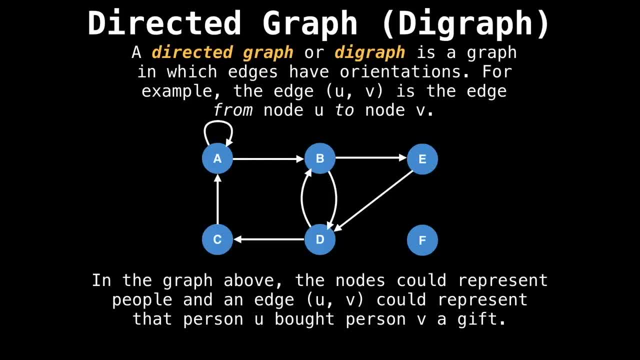 not the other way around. In this graph you can see that the edges are directed because of the arrowheads on the edges between nodes. This graph could represent people who bought each other gifts, So an incoming edge represents receiving a gift and an outgoing edge represents giving a gift. 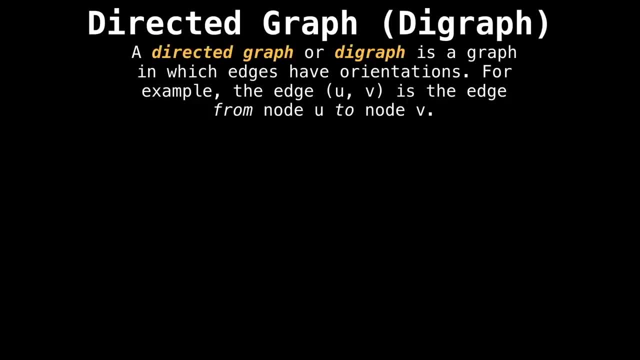 your steps by driving the other way. In contrast to undirected graphs, there are also directed graphs, sometimes called die graphs. In these graphs- you've guessed it- the edges are directed. So if we have an edge from u to v, then you can only go from node u to node v, not the other way. 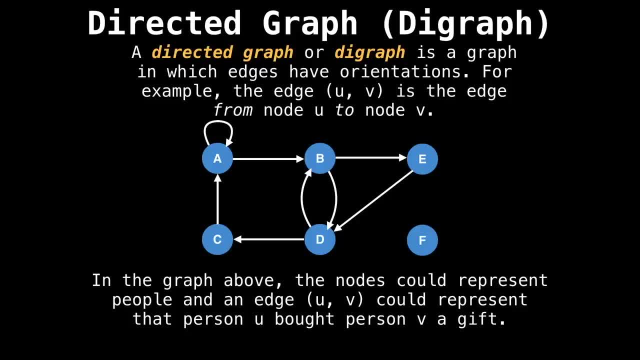 around In this graph. you can see that the edges are directed because of the arrowheads on the edges between nodes. This graph could represent people who bought each other gifts, So an incoming edge represents receiving a gift and an outgoing edge represents giving a gift. Therefore, person E in 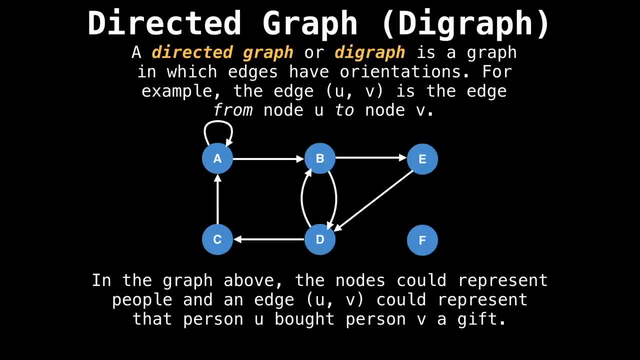 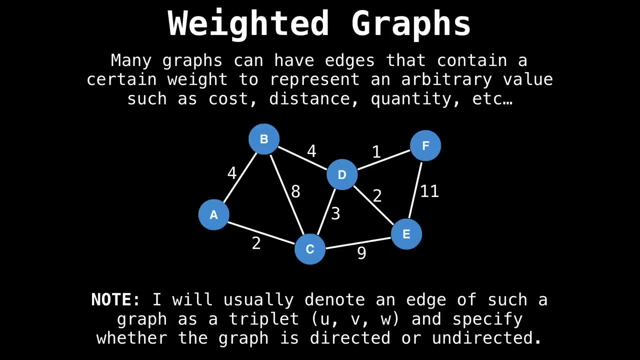 this graph, but person D gift, person A bought themselves and person B a gift and person F about nobody any gifts and received none. So far we've only seen unweighted graphs, but edges on graphs can contain weights to represent arbitrary values such as cost, distance, quantity, you name it. 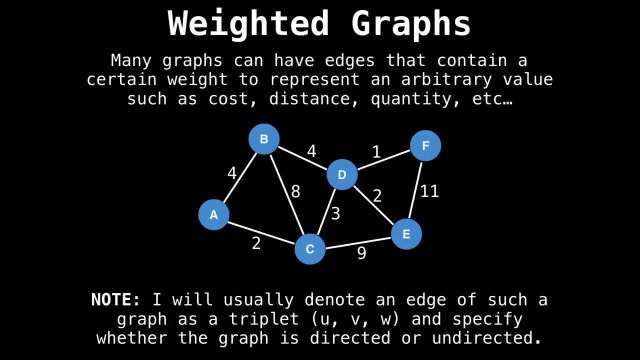 weighted graphs come in both directed and undirected flavors. As a side note, I will usually denote an edge of a graph as a triplet u vw to indicate where an edge is coming from, where it's going to and what its weight is, Of course, with this notation. 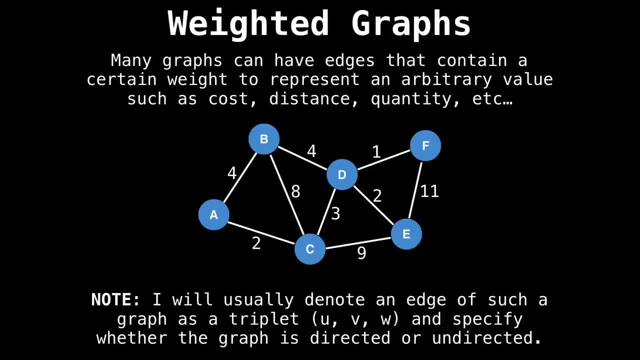 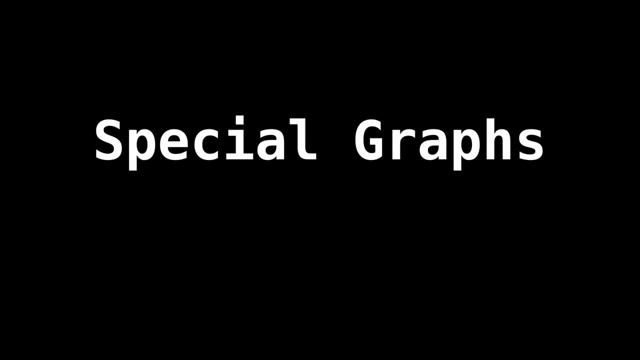 I also need to specify whether the graph is directed or undirected. Next up, I just want to have a quick chat about special types of graphs and graph theory. There are so many different types of graphs in graph theory. there are so many different types of graphs. 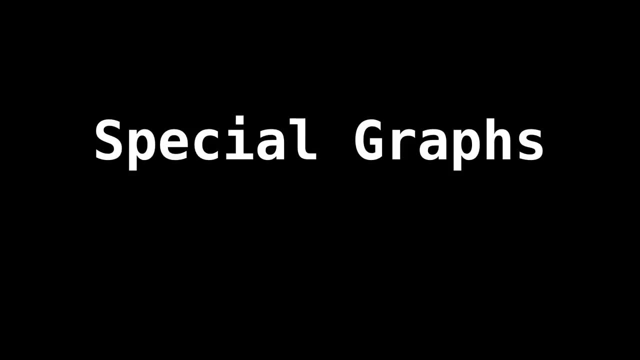 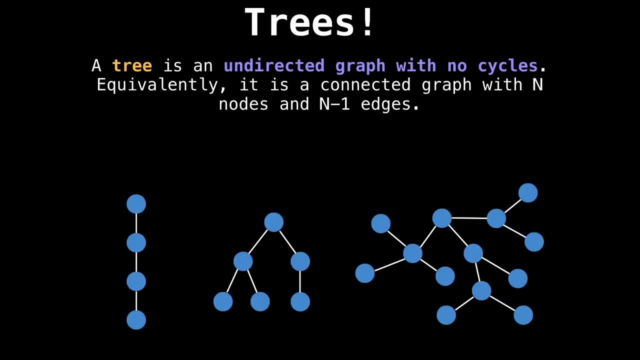 that I only had to select a few which will be most relevant for this upcoming video series. Most important type of special graph is definitely the tree. A tree is simply an undirected graph with no cycles. There are several equivalent definitions of a tree, such as a graph. 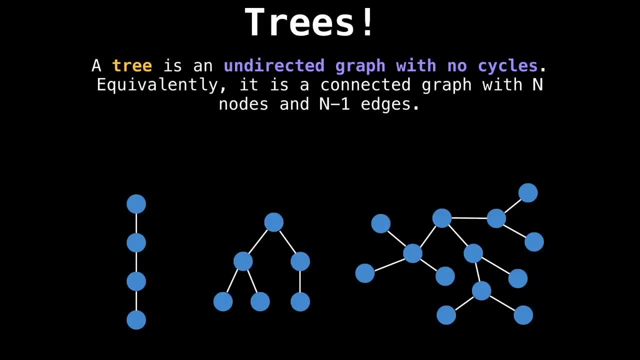 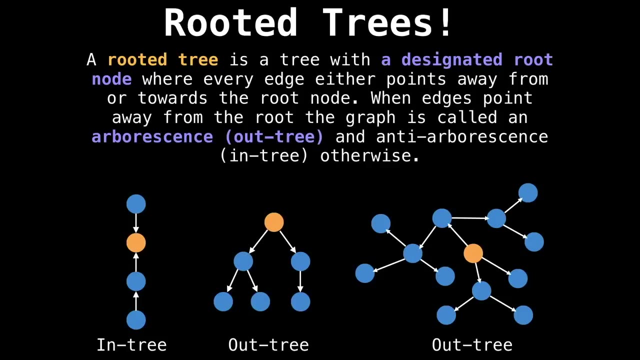 with n nodes and n minus one edges. All the graphs below are trees, Yes, even the left most ones, since it has no cycles. A related but totally different type of graph is a rooted tree. The distinction here is that a rooted tree has a designated 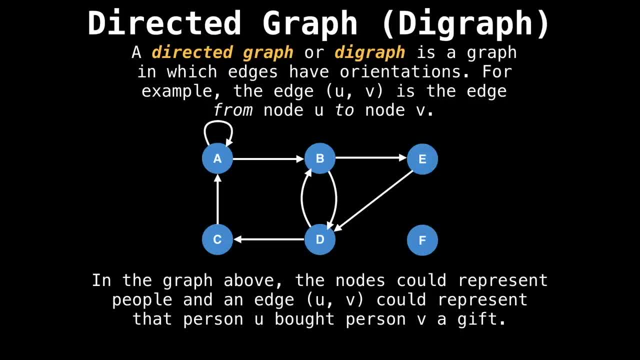 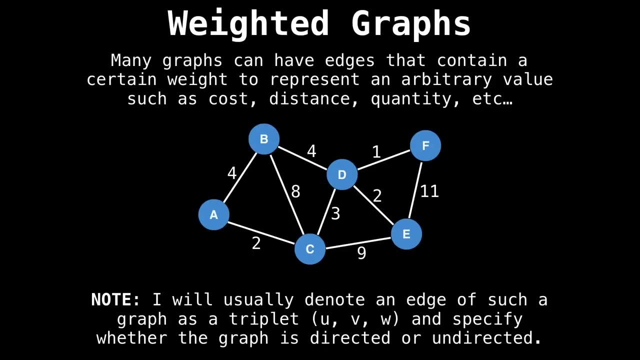 Therefore person e in this graph, but person D gift, person A bought themselves and person B gift and person F about nobody any gifts and received none. So far we've only seen unweighted graphs, but edges on graphs can contain weights to represent arbitrary values, such as cost, distance, quantity, you. 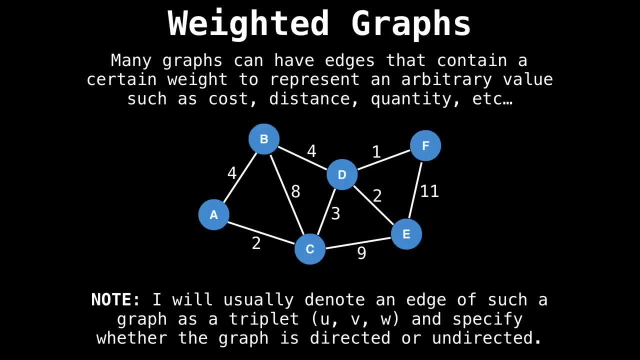 name it. weighted graphs come in both directed and undirected flavors. As a side note, I will usually denote an edge of a graph as a triplet u vw to indicate where an edge is coming from, where it's going to and what its weight is, Of course, with this notation, 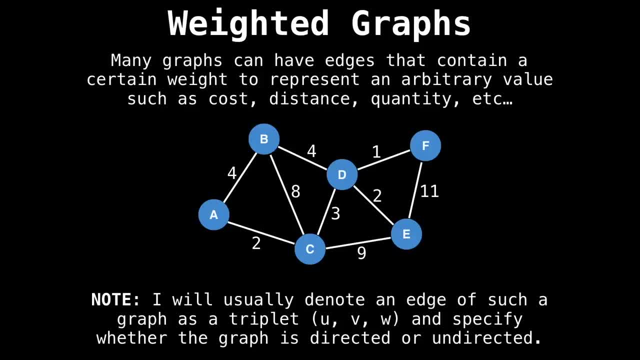 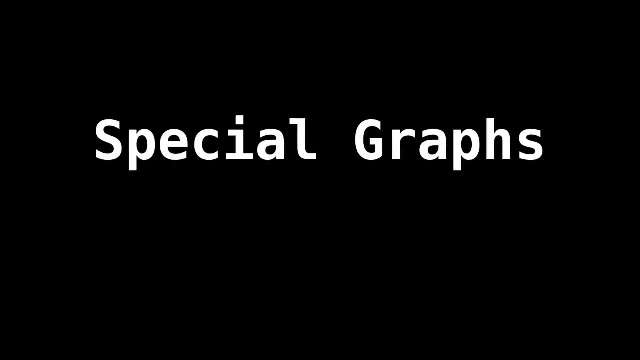 I also need to specify whether the graph is directed or undirected. Next up, I just want to have a quick chat about special types of graphs and graph theory. There are so many different types of graphs that I only had to select a few which will be most relevant for this. 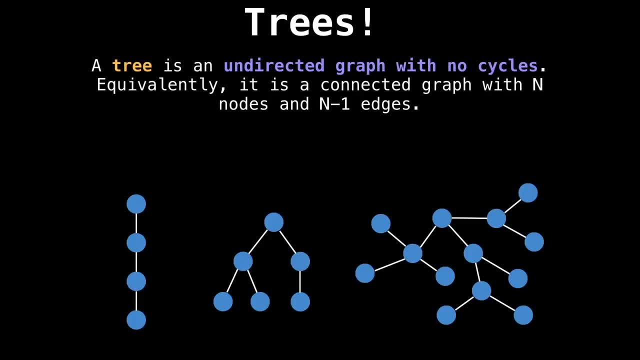 upcoming video series. Most important type of special graph is definitely the tree. A tree is simply an undirected graph with no cycles. There are several equivalent definitions of a tree, such as a graph with n nodes And n minus one edges. All the graphs below are trees. Yes, even the leftmost one, since 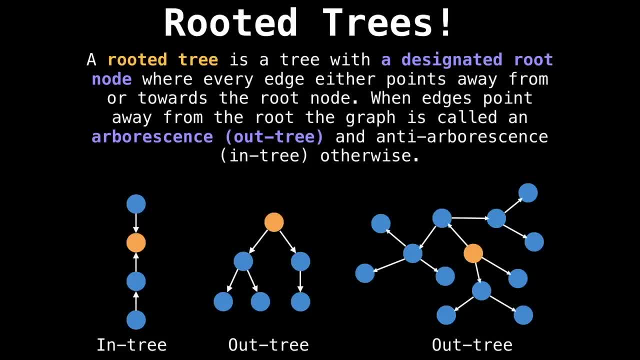 it has no cycles. A related but totally different type of graph is a rooted tree. The distinction here is that a rooted tree has a designated root node, where every edge either points away from or towards the root node. When edges point away from the root node, the graph is: 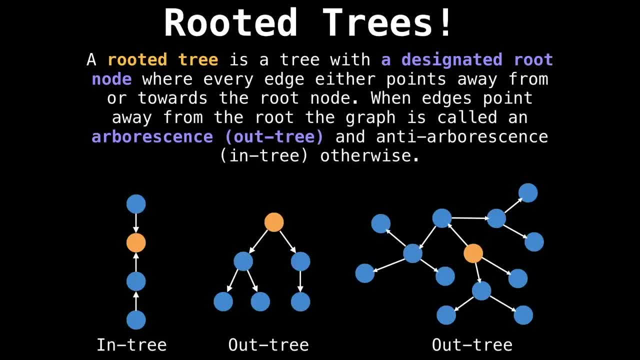 called n-1.. So the root node is a sign of the tree And then the tree is an aberrant or an out tree and an anti aberrant or entry. Otherwise, out trees are by far more common than entries. from what I observed, is also fairly common for people to refer to a rooted tree simply. 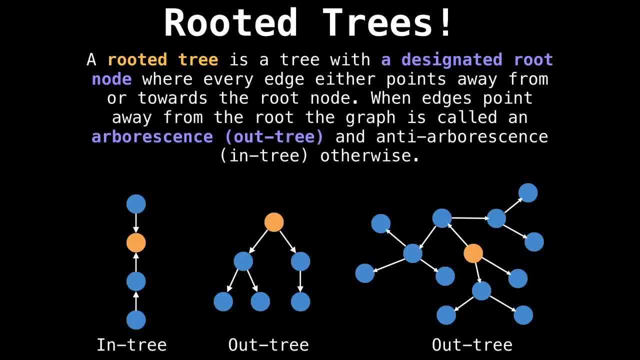 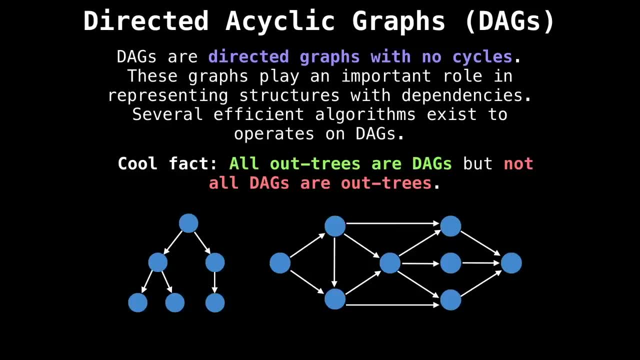 as a tree instead of an in or out tree, But there is an important distinction there. Next are directed acyclic graphs. These are graphs with directed edges and out trees, The selected- and no cycles. These graphs are very important and fairly common in computer science actually. 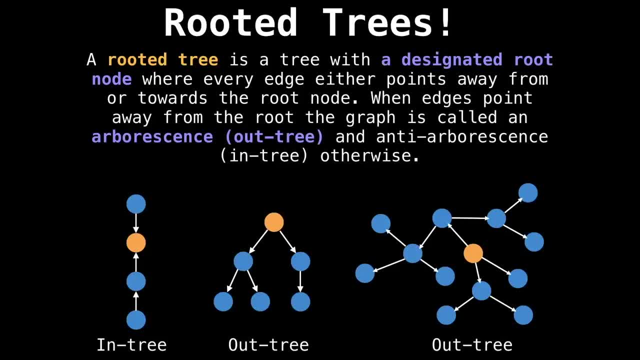 root node, where every edge either points away from or towards the root node. When edges point away from the root node, the graph is called an Android essence or an out retreat, and an anti fluorescence or hint of fluorescence. ике, a literalällen for graph, is called an abnormality or an. again, aber October 3,. 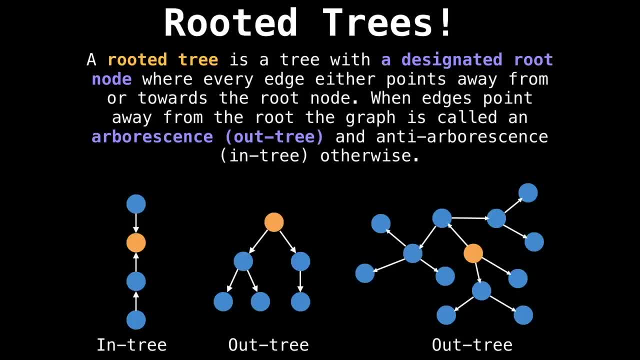 Präsident esperanz tego, who likes images of trees, each one as the multi милли информational value point. we could have some French and out tree, as we always would agency level SOL at an entry. Otherwise, out trees are by far more common than entries, From what I've observed. 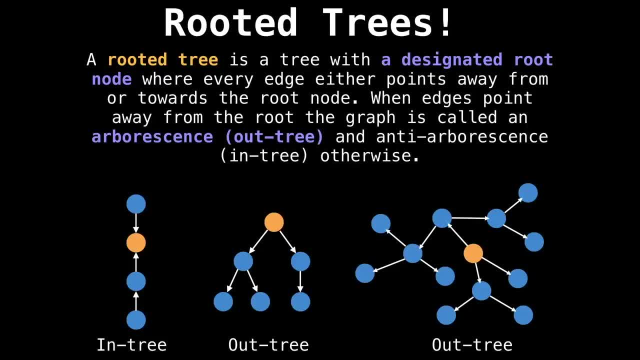 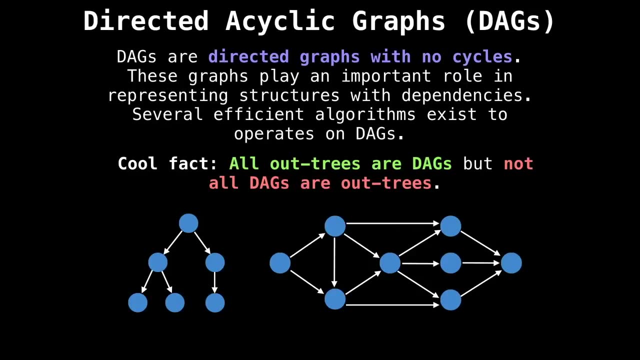 it is also fairly common for people to refer to a rooted tree simply as a tree instead of an in or out tree, But there is an important distinction there. Next are directed acyclic graphs. These are graphs with directed edges and no cycles. These graphs are very important and fairly common. 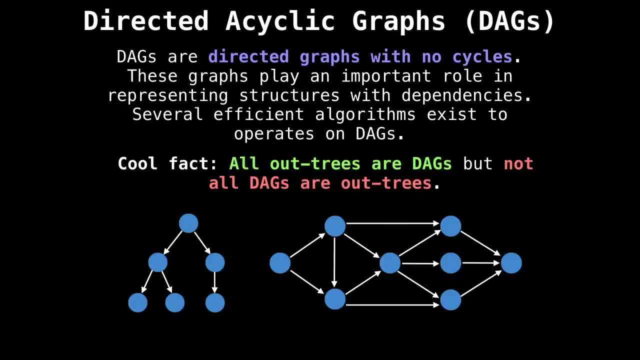 in computer science, actually, since they often represent structures with dependencies, such as a scheduler, a build system, a compiler maybe, or perhaps more relatable university class prerequisites. There are several efficient algorithms we'll be looking at to deal specifically with directed acyclic graphs, such as how to find the shortest path and produce a topological. 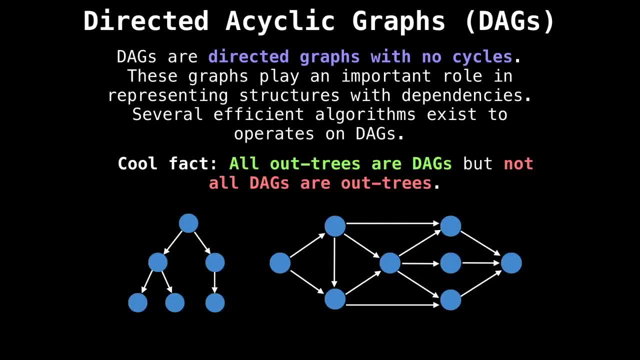 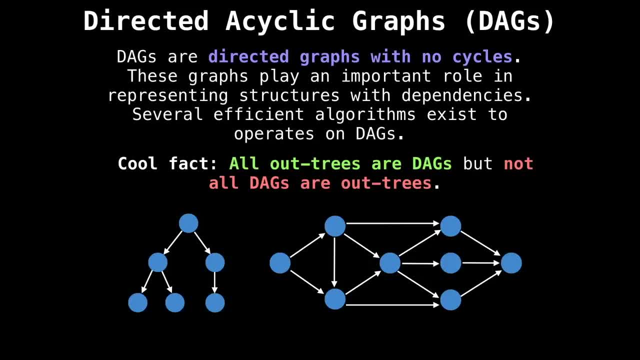 a graph, so you don't perform a task before first having completed all its dependencies. For example, a topological ordering of class prerequisites would tell you to take intro biology and intro chemistry before taking a class on, say, genomics. This next type of special graph is a 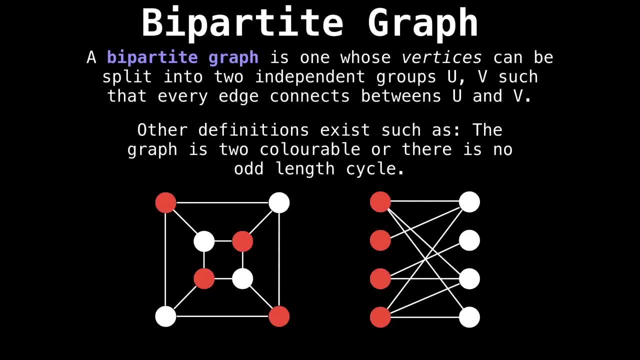 bipartite graph. It is one of the most common types of topological ordering of nodes in computer graphics. It is one whose vertices can be split into two independent groups, u and v, such that every edge connects between u and v. This is just a fancy way of saying that the graph is too colorable, or? 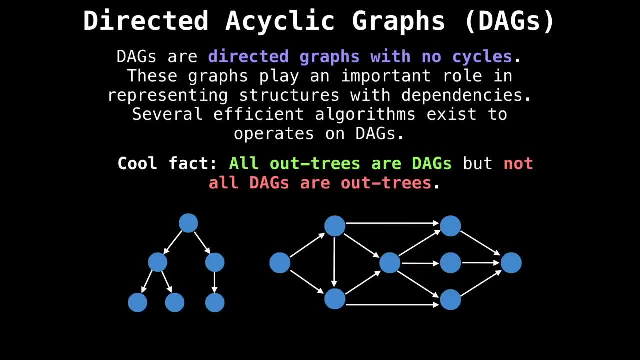 since they often represent structures with dependencies, such as a scheduler, a build system, a compiler maybe, or perhaps more relatable university class prerequisites. There are several efficient algorithms we'll be looking at to deal specifically with directed acyclic graphs, such as how to find the shortest path and produce a topological ordering of. 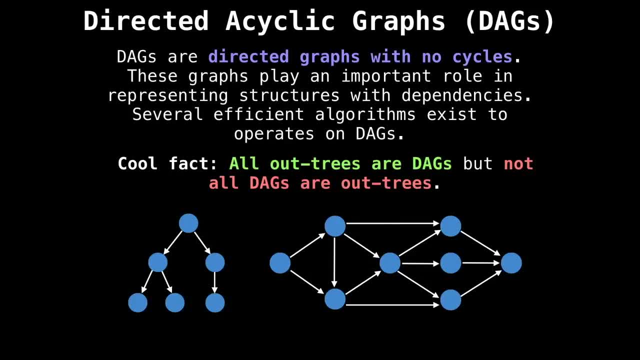 nodes. A topological ordering of nodes is an ordering of nodes that tells you how to process the nodes and the graph, so you don't perform a task before first having completed all its dependencies. For example, a topological ordering of class prerequisites would tell. 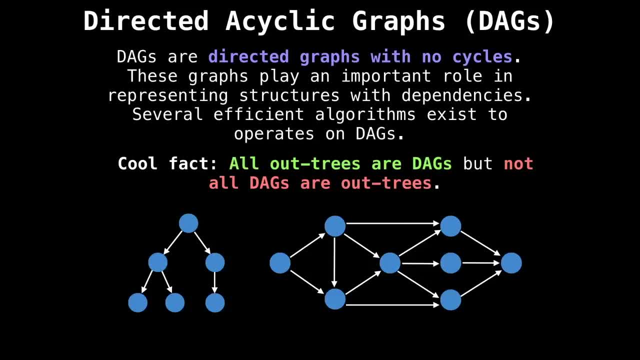 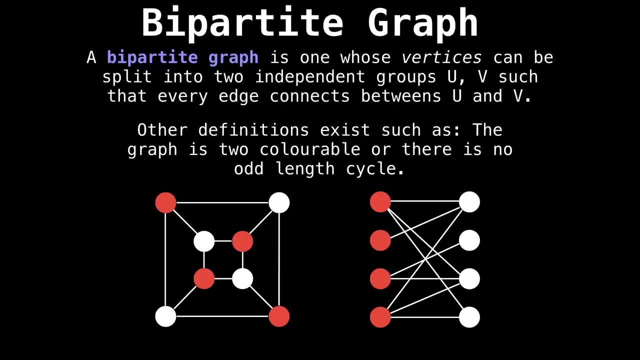 you to take intro biology and intro chemistry before taking a class on, say, the genomics. This next type of special graph is a bipartite graph. It is one whose vertices can be split into two independent groups, u and v, such that every edge connects between. 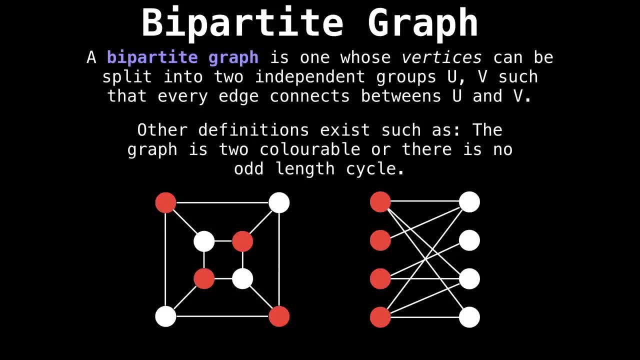 u and v. This is just a fancy way of saying that the graph is too colorable or that there are no odd length cycles and graph. Often a problem we like to ask is: what is the maximum matching we can create on a bipartite graph. Suppose white nodes are jobs and red nodes 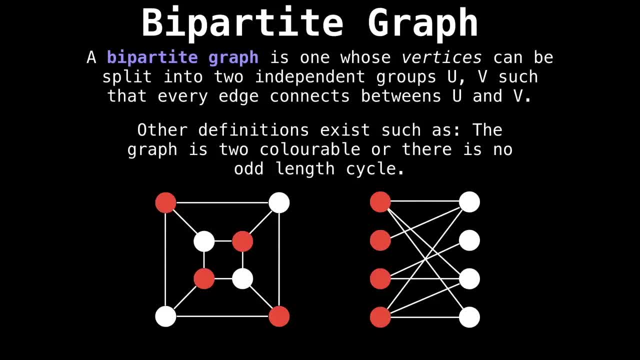 are people. then we can ask how many people can be matched to jobs. In this case, there are a lot of edges in each graph, So I think the answer for both is four, But in general it's not so easy If there are less edges, tougher constraints and more conflicts. bipartite graphs also. 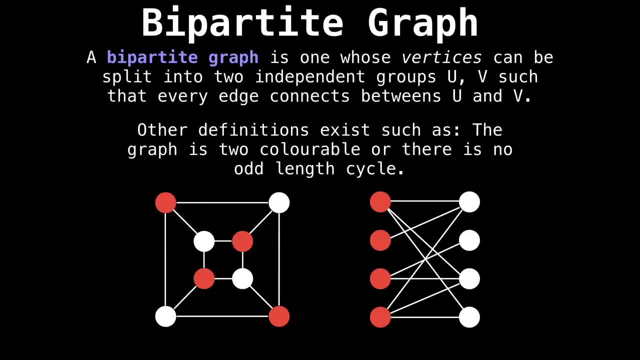 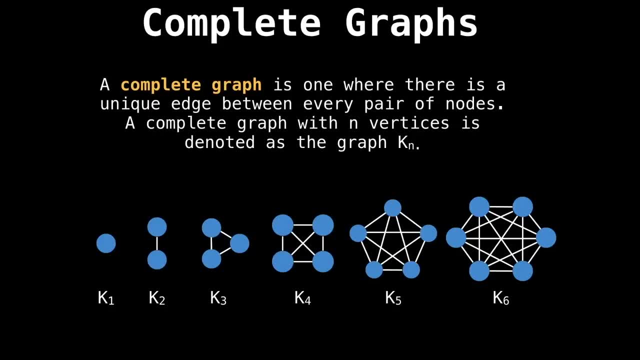 play a critical role in the field of network flow, which we will talk about later. This last type of graph is a complete graph, is one where there is a unique edge between every pair of nodes in the graph. A complete graph with n vertices is denoted as the graph k. 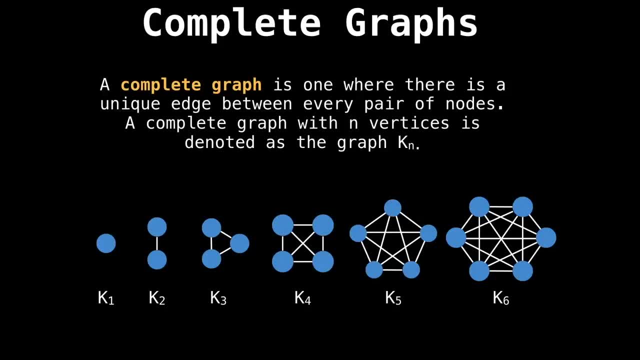 sub n. I have listed k one through k six on the bottom And you can easily see how this scales when we add more nodes. Complete graphs are often seen as the worst case possible graph you can possibly encounter because of how many edges there are. So if you want to test, 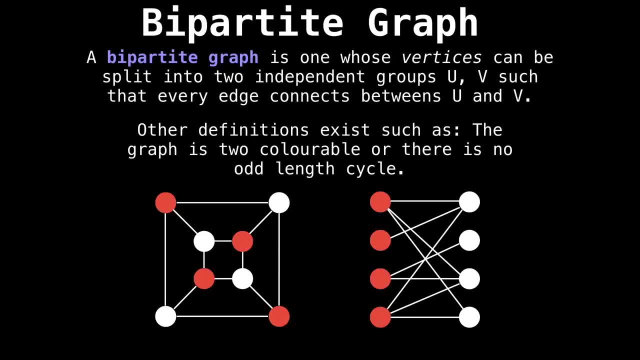 that there are no odd length cycles and graph. Often a problem we'd like to ask is: what is the maximum matching we can create on a bipartite graph? Suppose white nodes on a graph are jobs and red nodes are people. then we can ask how many people can be matched to jobs In this case. 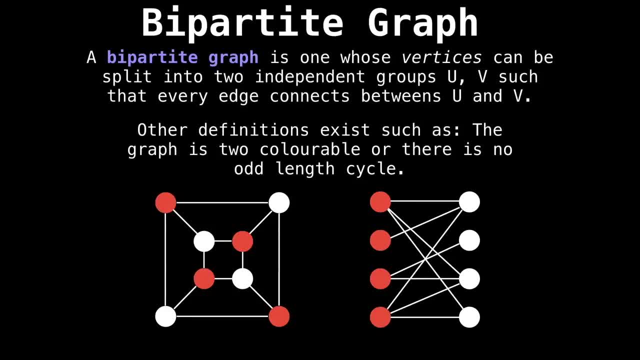 there are a lot of edges in each graph, So I think the answer for both is four, But in general it's not so easy if there are less edges, tougher constraints and more conflicts. bipartite graphs also play a critical role in the field of network flow, which we will talk about later. This last 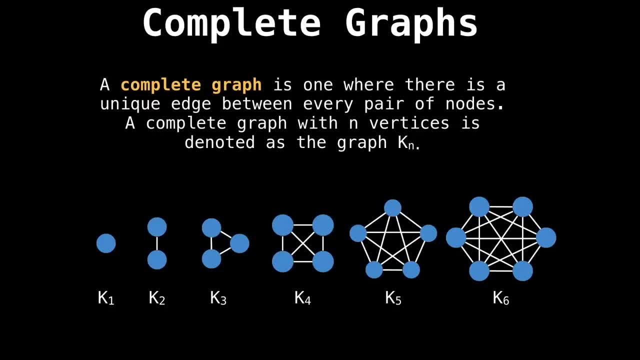 type of graph is called a network flow graph, And this is a graph that we're going to talk about in a little bit more detail in the next video, So let's get started. So a network flow graph is a graph. It is one where there is a unique edge between every pair of nodes in the graph: A complete. 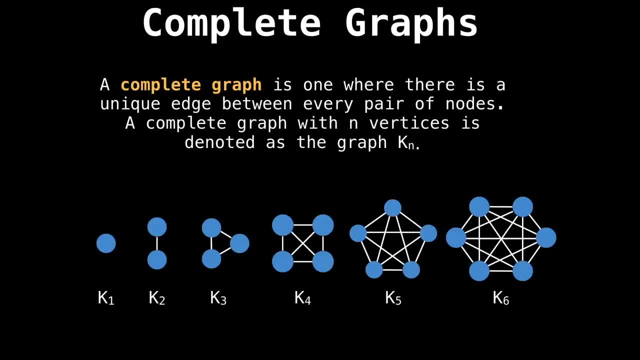 graph with n vertices is denoted as the graph k sub n. I have listed k one through k six on the bottom And you can easily see how this scales when we add more nodes. Complete graphs are often seen as the worst case possible graph you can possibly encounter. 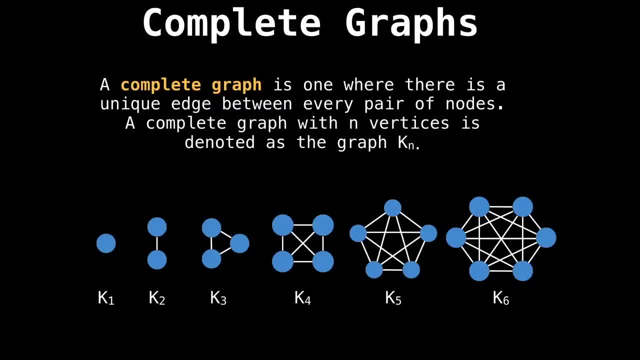 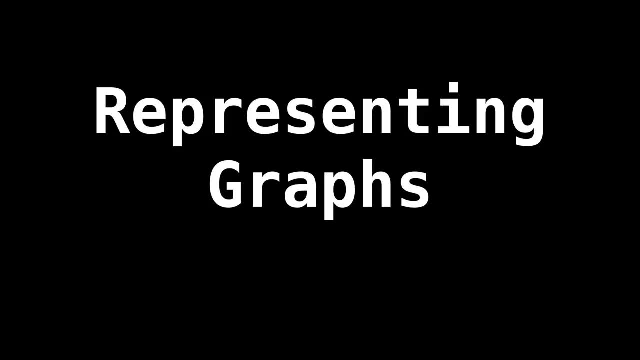 Because of how many edges there are. So if you want to test your algorithm for performance, a complete graph is an easy way to start. One thing we're going to have to be really cognizant about is how we're actually representing our graphs on the computer. This isn't just what type 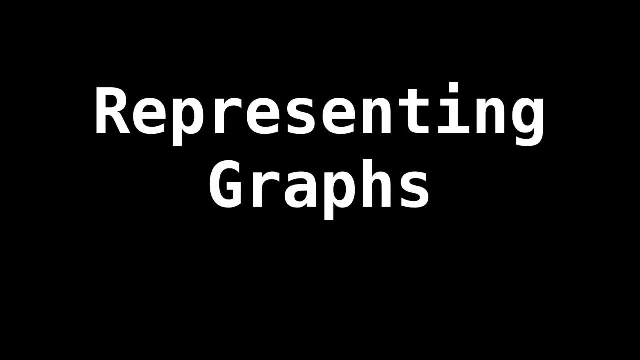 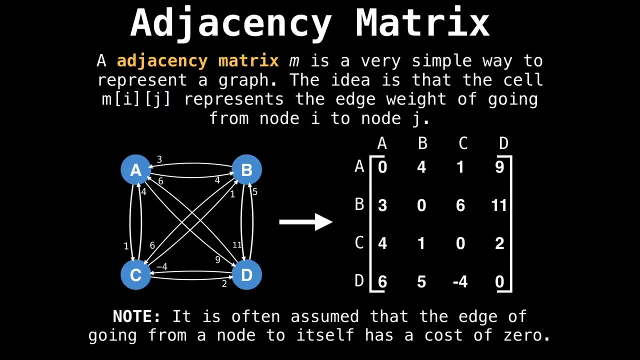 of graph it is, but what type of data structure it? but what type of data structure are we representing our graph with? And this can have a huge impact on performance. The simplest way is inside a 2d adjacency matrix. The idea is that the cell mi j represents 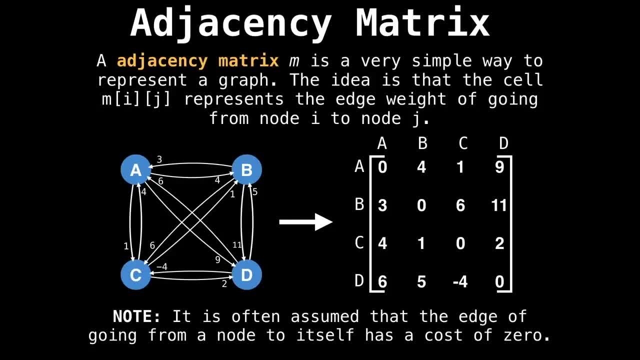 the edge weight of going from node i to node j. So in the graph below there are four nodes. So I create a four by four matrix and populate the graph with the edge weights. If you look at the edge weight from node c to node d, you'll see that it has an edge weight of 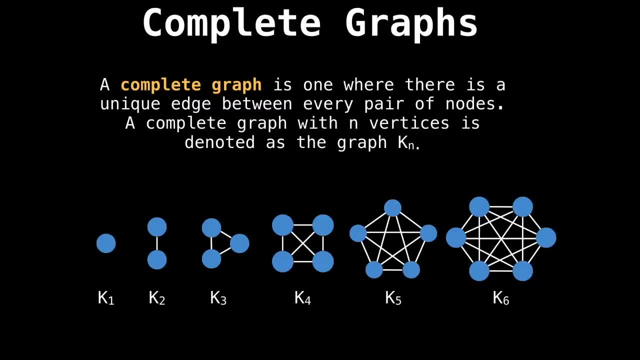 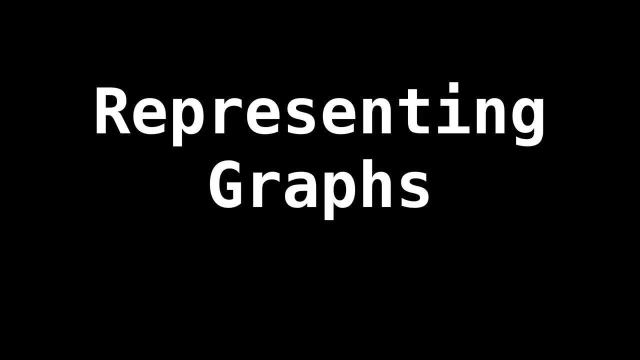 your algorithm for performance. a complete graph is an easy way to start. One thing we're going to have to be really cognizant about is how we're actually representing our graph. So we're going to have to be really cognizant about is how we're actually representing our graph. 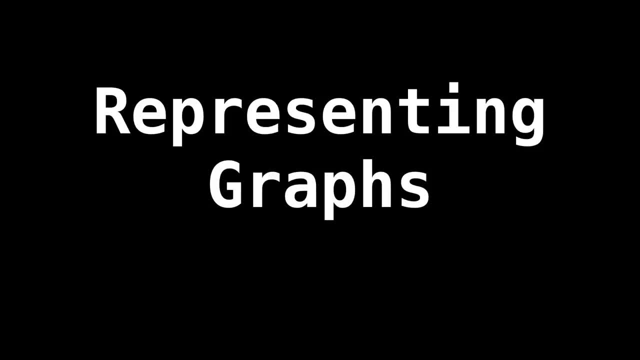 So we're going to have to be really cognizant about is how we're actually representing our graph on the computer. This isn't just what type of graph it is, but what type of data structure it. but what type of data structure are we representing our graph with? and this can have a huge impact. 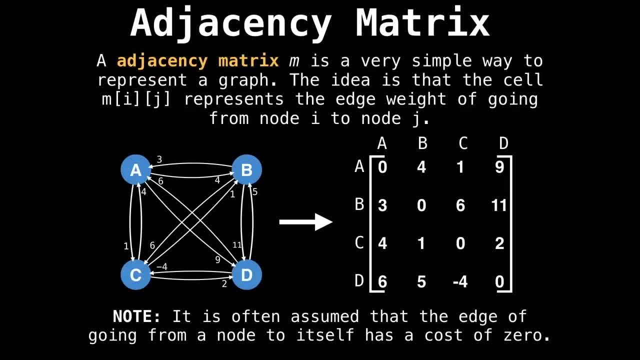 on performance. The simplest way is inside a 2d adjacency matrix. The idea is that the cell mi j represents the edge weight of going from node i to node j. So in the graph below there are four nodes. So I create a four by four matrix and populate the graph with the edge weights, If you look. 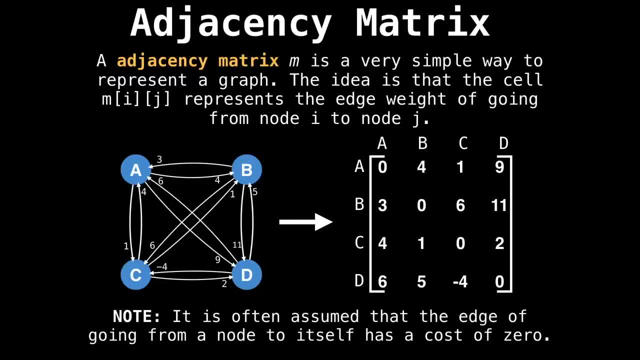 at the edge weight from node C to node D, you'll see that it has an edge weight of two. So in row three and column four of the matrix there is a value of two. Note that is often assumed that the edge of going from a node to itself has a cost of zero, which is why 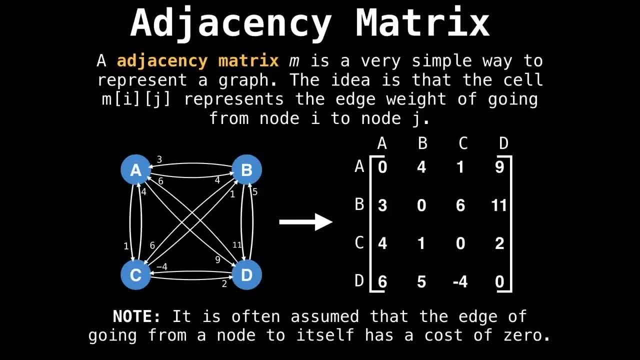 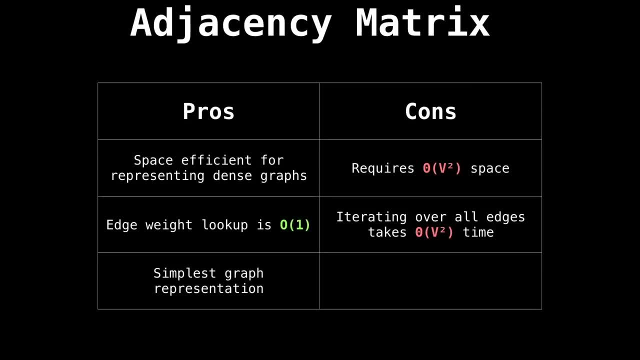 the diagonal of the matrix has all zero values. This matrix form has several advantages. First, that it's very space efficient for dense graphs, that is, graphs with a lot of edges. the edge weight lookup can be found in constant time, which is quite nice. And lastly, I would argue, 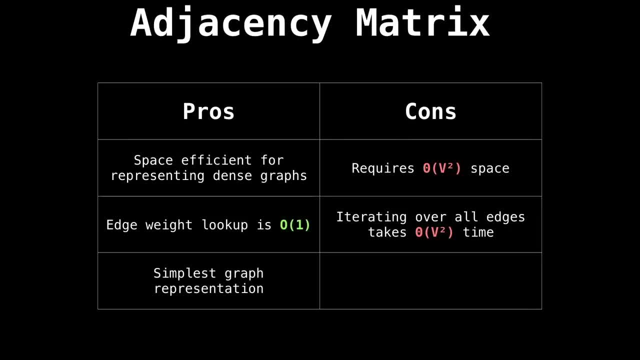 that it is the simplest form of graph representation you can have. On the downside, however, the main reason people don't go for the adjacency matrix as their first pick is because it requires v squared space, which is well a lot of space In practice. graphs with 10,000 nodes. 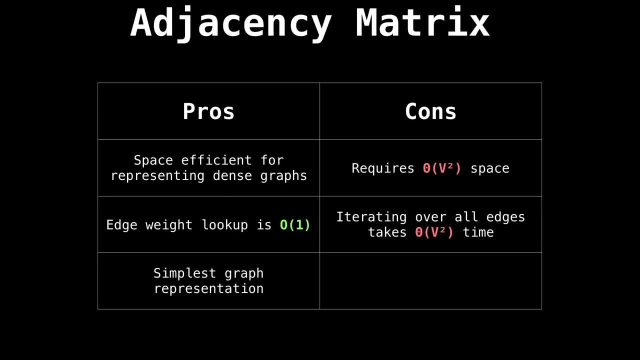 or more start to become infeasible very quickly. The other issue with adjacency matrix is that it requires v squared work to iterate over all the edges of your graph. This is fine for dense graphs with lots of edges, but it isn't so great for sparse graphs, since most 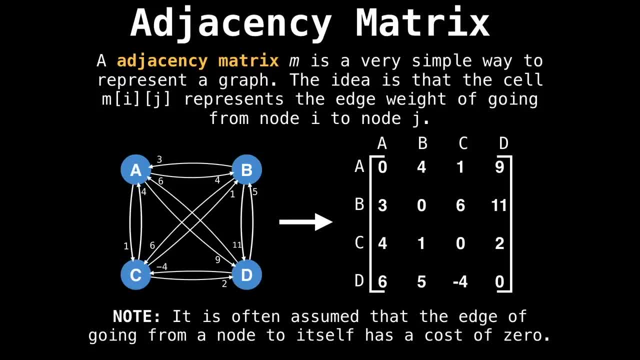 two. So in row three and column four of the matrix there is a value of two. Note that is often assumed that the edge of going from a node to itself has a cost of zero, which is why the diagonal of the matrix has all zero values. This matrix form has several. 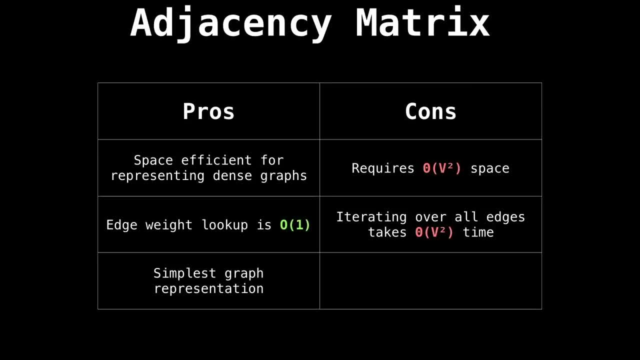 advantages. First, that is very space efficient For dense graphs, that is, graphs with a lot of edges. the edge weight lookup can be found in constant time, which is quite nice. And lastly, I would argue that it is the simplest. 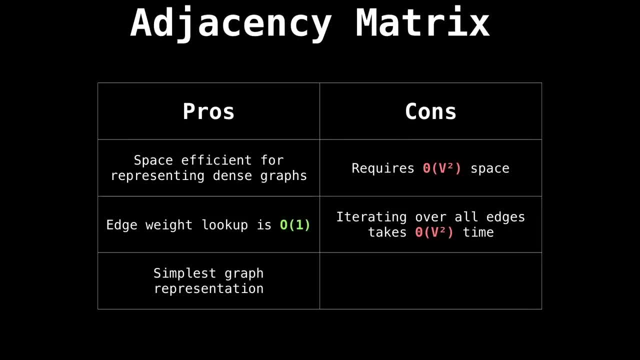 form of graph representation you can have. On the downside, however, the main reason people don't go for the adjacency matrix as their first pick is because it requires v squared space, which is well a lot of space. In practice, graphs with 10,000 nodes or more start to become infeasible. 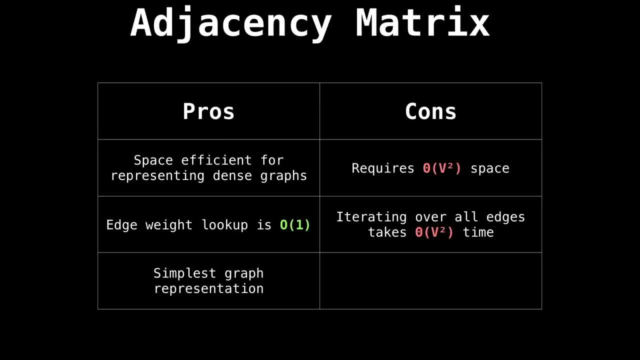 very quickly. The other issue with the adjacency matrix is that it requires v squared work to iterate over all the edges of your graph. This is fine for dense graphs with lots of edges, but it isn't so great for sparse graphs, since most cells will be empty. The main alternative. 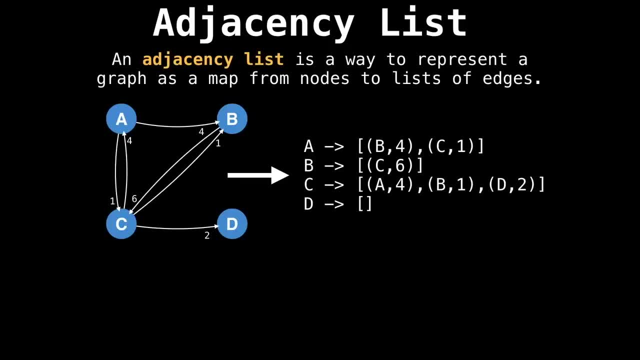 to the adjacency matrix. is the adjacency matrix. The adjacency matrix. is the adjacency matrix. is the adjacency matrix. is the adjacency list, which is a way to represent a graph as a map of nodes to list of edges. The idea is that each node tracks all of its outgoing edges, For example, node 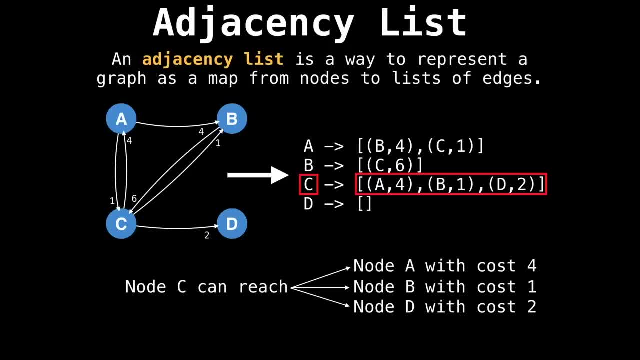 C has three outgoing edges. So the map entry for C will track the edge from C to A with cost for, the edge from C to B with cost one and edge from C to D with cost two. So the map entry for C will track the edge from C to B with cost two. Notice that in the list. 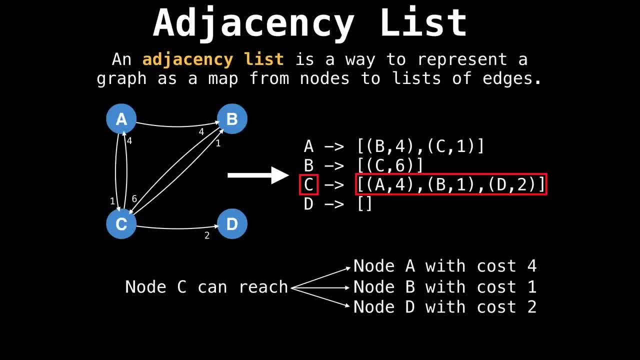 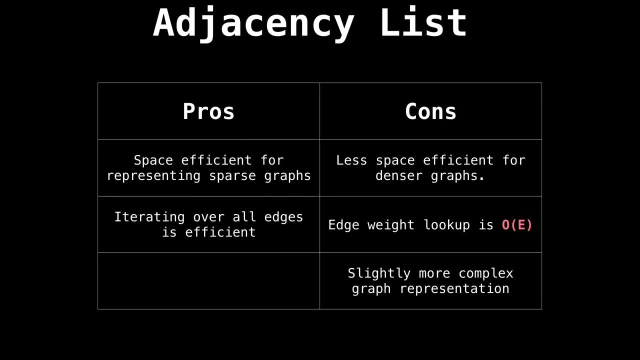 of edges. we only need to track two things: the node we're going to and the cost to get there. we don't need to keep track of where we came from, because that's already implicitly known. The nice thing about adjacency lists is that it is great for sparse graphs, because 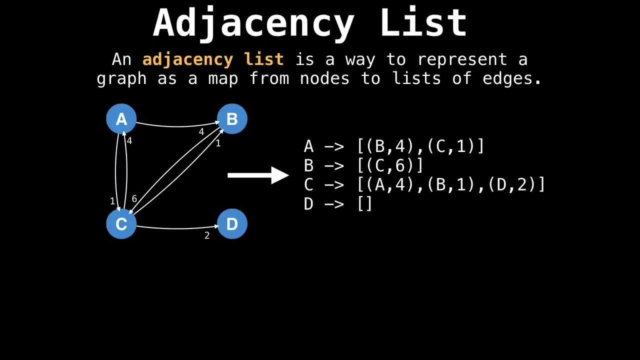 cells will be empty. The main alternative to the adjacency matrix is the adjacency list, which is a way to represent a graph as a map of nodes to list of edges. The idea is that each node tracks all of its outliers outgoing edges. For example, node C has three outgoing edges, So the map entry for C will. 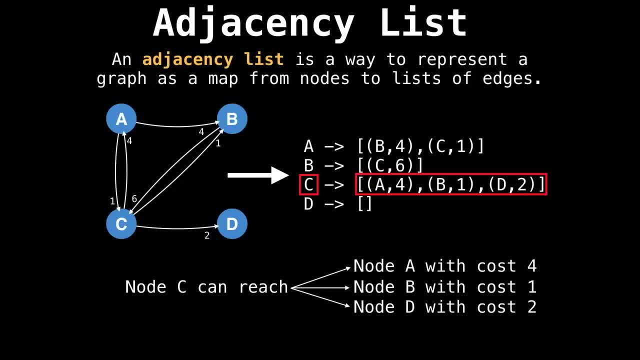 track the edge from seed a with costs for the edge from C to B with cost one, and edge from C to D With cost. to notice that in the list of edges we only need to track two things: the node we're going to and the cost to get there. 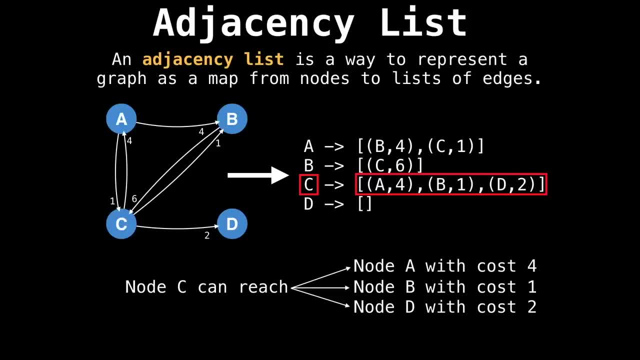 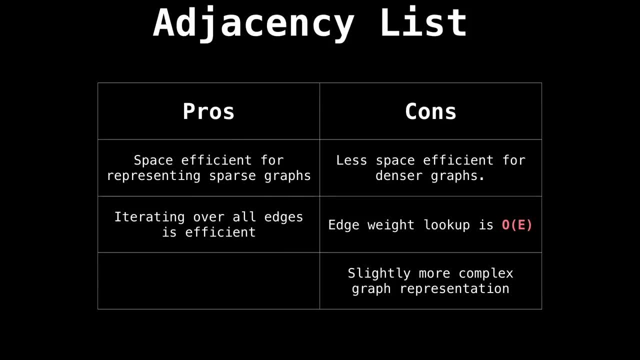 We keep track of where we came from, Because that's already implicitly known. The nice thing about adjacency lists is that it is great for sparse graphs, because it only tracks the edges that you have and doesn't allocate additional memory that you might not use, like. 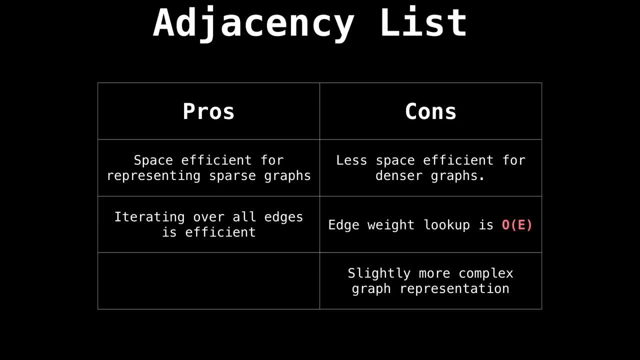 the adjacency matrix does. This also means it's efficient when iterating over all the edges. The main disadvantage to using an adjacency list is that it is less space efficient on denser graphs. Another subtle disadvantage is that it takes big O of E time to access. 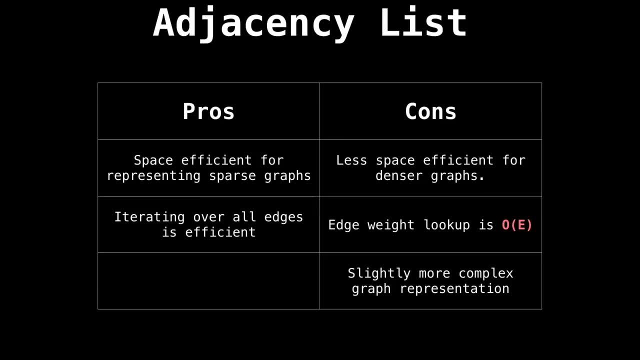 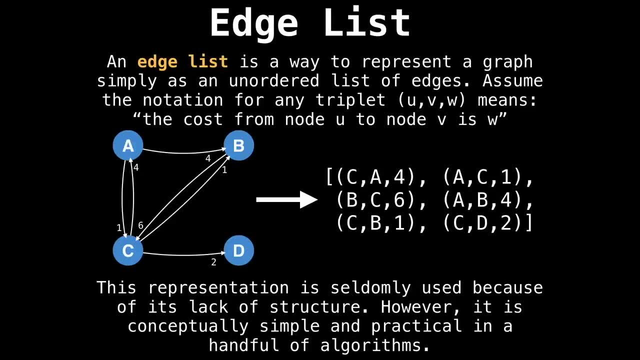 a specific edges wait, although in practice you rarely, or if ever, actually need to do this. The last representation I want to talk about is the edge list. An edge list is a way to represent a graph simply as a graph, as an unordered list of edges. Basically, it's exactly what it sounds like: a list of. 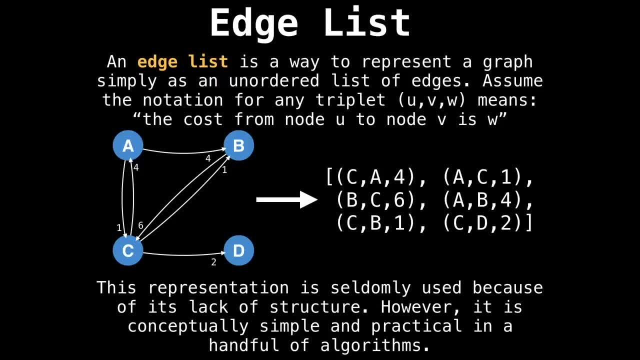 edges. Assume that the notation for any triplet u, v, w means the cost from node u to node v is w. So for this graph, the edge list is simply a list of six edges represented as those triplets. This representation is very simple. However, it lacks structure, and that's. 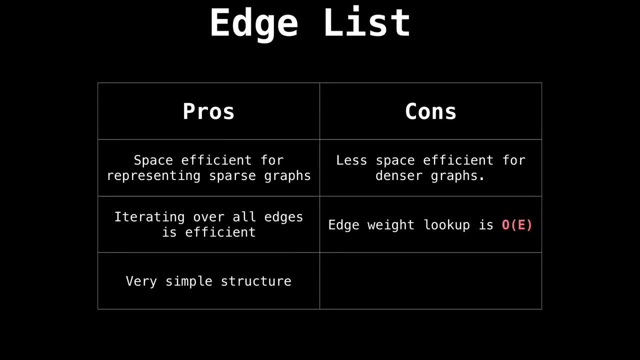 why it is seldomly used. Advantage to the edge list is as great for sparse graphs. iterating over all the edges is super easy and the structure is simple. The downside is that edge look up can be slow and you can run into memory issues on large graphs. Today I'm going to 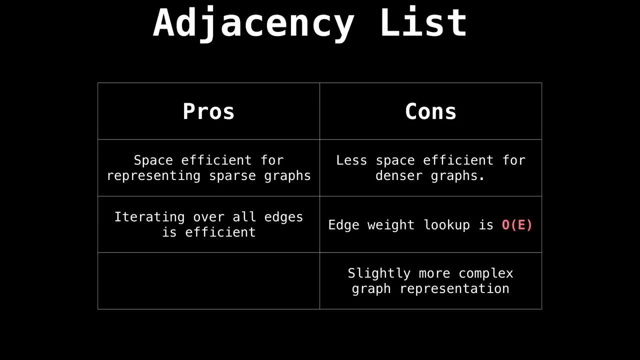 it only tracks the edges that you have and doesn't allocate additional memory that you might not use, Like the adjacency matrix does. This also means it's efficient when iterating over all the edges. The main disadvantage to using an adjacency list is that it is less space. 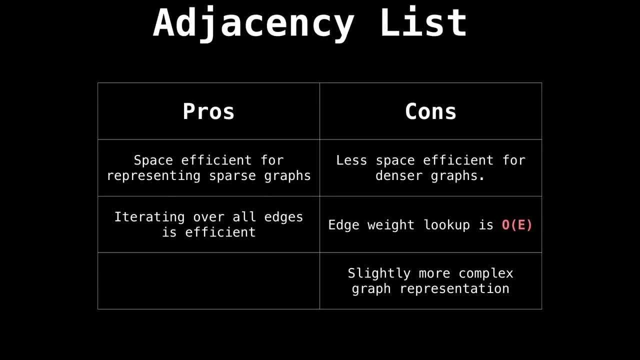 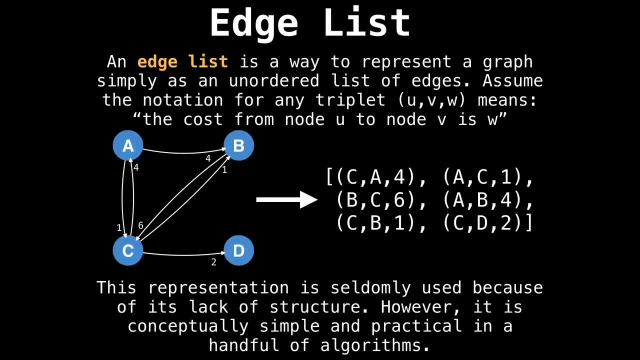 efficient on denser graphs. Another subtle disadvantage is that it takes big O of E time to access a specific edges weight, Although in practice you rarely, or if ever, actually need to do this. The last representative of the adjacency matrix is the adjacency matrix In this example. 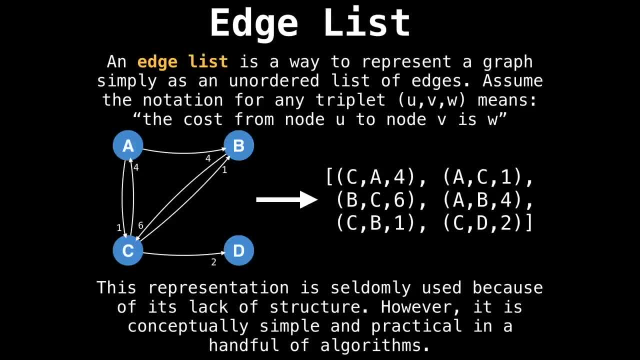 I want to talk about is the edge list. An edge list is a way to represent a graph simply as an unordered list of edges. Basically, it's exactly what it sounds like: a list of edges. Assume that the notation for any triplet u v, w means the cost from node u to node v. 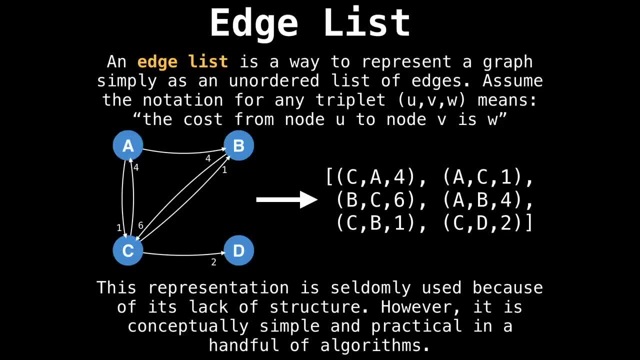 is w. So for this graph, the edge list is simply a list of six edges represented by those triplets. This representation is very simple. However, it lacks structure and that's why it is seldomly used. Advantage to the edge list is as great for sparse graphs, iterating. 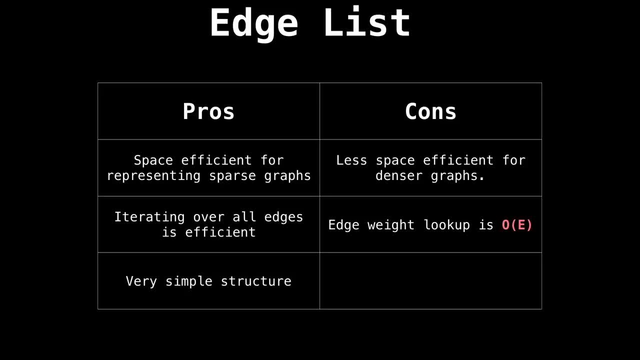 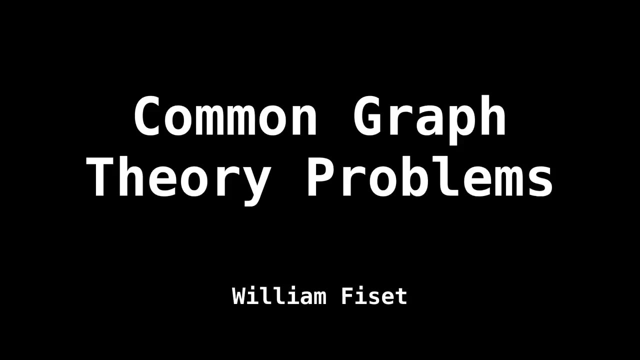 over all the edges is super easy and the structure is simple. The downside is that edge look up can be slow and you can run into memory issues on large graphs. Today I'm going to talk about common problems In graph theory. a lot of problems you will encounter can often be reduced to a famous 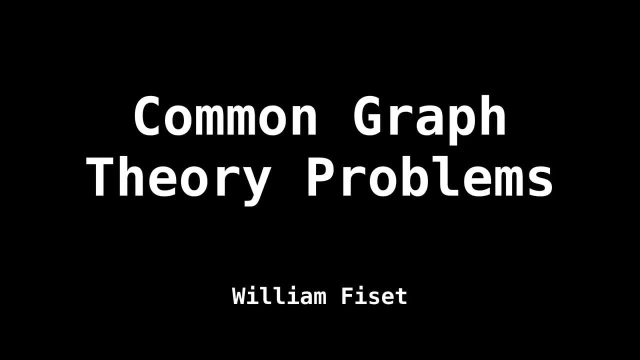 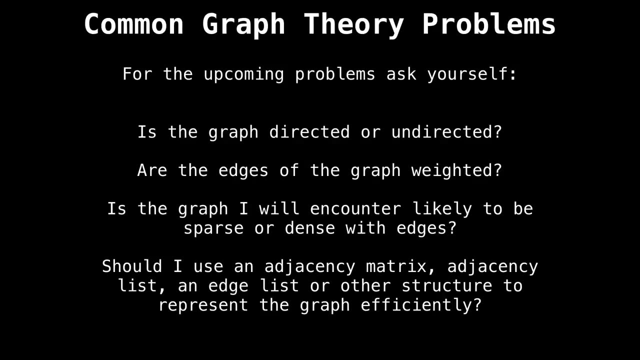 or a well known problem or some variant thereof, So it's important to be able to familiarize ourselves with common graph theory problems and their solutions Just before getting started. following off from what we learned in the last video about representing graphs, I want 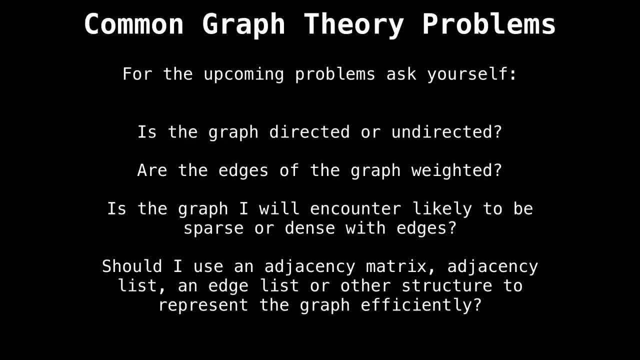 you to think about how you would store and represent the graphs in the upcoming problems I'm going to describe In particular. is the graph in the problem I'm describing directed or undirected? Are the edges of the graph weighted or unweighted? Is the common use case a graph that is likely to be sparse, or 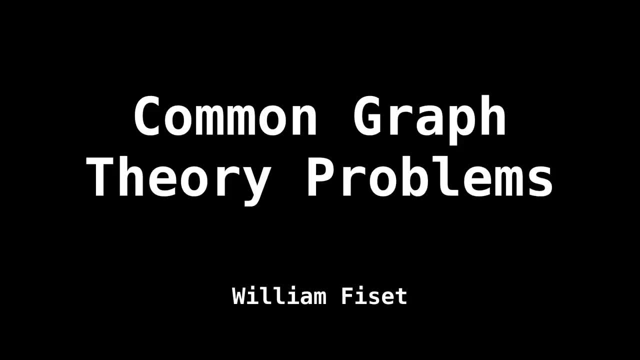 talk about common problems in graph theory. A lot of problems you will encounter can often be reduced to a famous or a well known problem or some variant thereof, So it's important to be able to familiarize ourselves with common graph theory problems and their solutions Just before getting started following off. 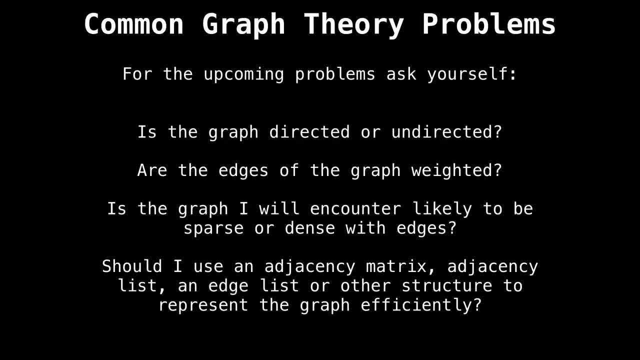 from what we learned in the last video about representing graphs, I want you to think about how you would store and represent the graphs in graph theory In particular. is the graph in the problem I'm describing directed or undirected? Are the edges of the graph weighted or unweighted? Is the common use case a graph that is likely? 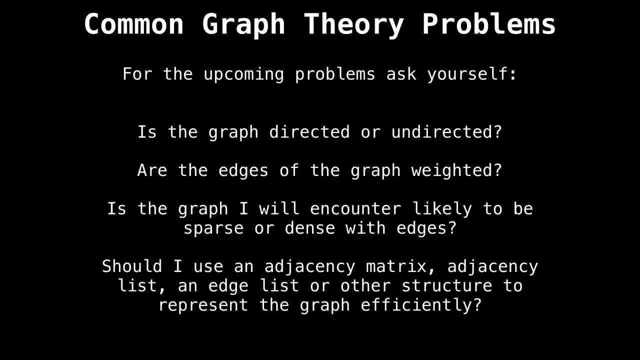 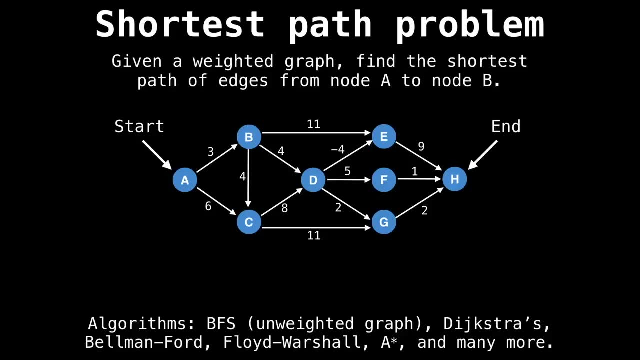 to be sparse or dense with edges? And lastly, should I use an adjacency matrix and adjacency list and edge lists or some other structure to represent my graph efficiently? So one of the most, if not the most, common problem in graph theory is the shortest path. 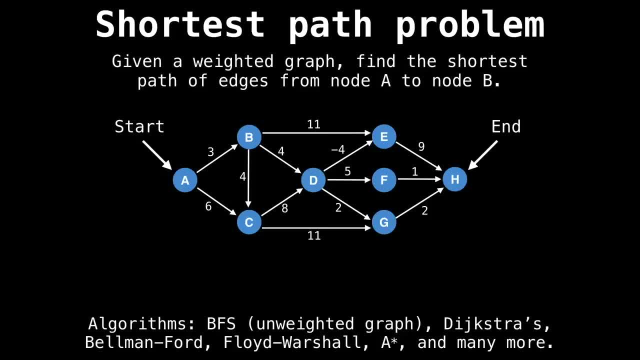 problem: Given a weighted graph, find the shortest path of edges from node A to node B. So if we pretend this graph represents a road system and we're at node A and want to get to node H, our shortest path algorithm should be able to find us a list of edges. 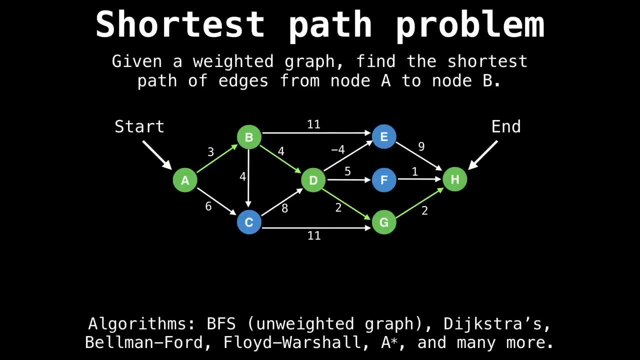 to follow that will lead us A to H with a minimal cost. Lucky for us, many algorithms exist to solve the shortest path problem, including a breadth. first search for unweighted graphs, Dijkstra's algorithm, Bellman Ford, a star, and many more. As simple as it sounds, connectivity is a big issue. 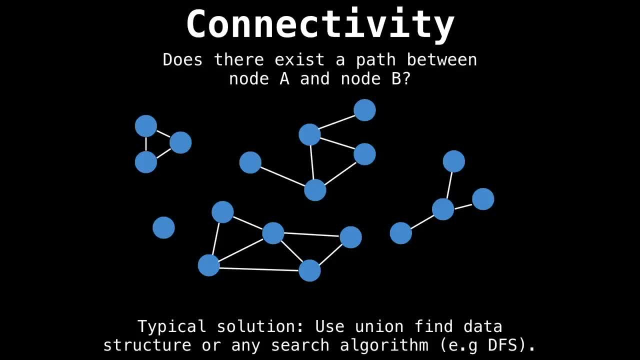 in graph theory The problem can also be simplified to: does there exist a path from node A to node B? In this scenario, we don't care about the minimum cost, we just want to know: can one node reach another node? A typical solution to this problem is to use a union, find data structure or do a very 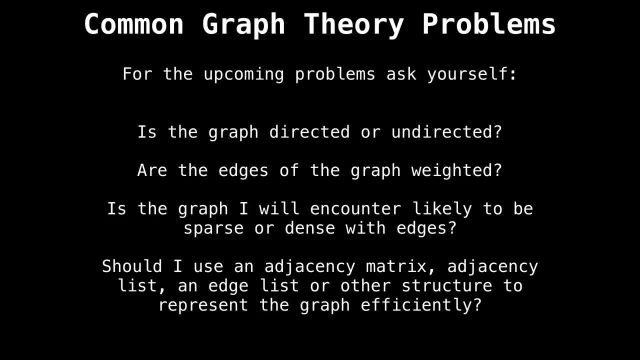 dense with edges. And lastly, should I use an adjacency matrix and adjacency list and edge lists or some other structure to represent? Okay, let's get started. So let's talk about how you could represent my graph efficiently. So one of the most, if 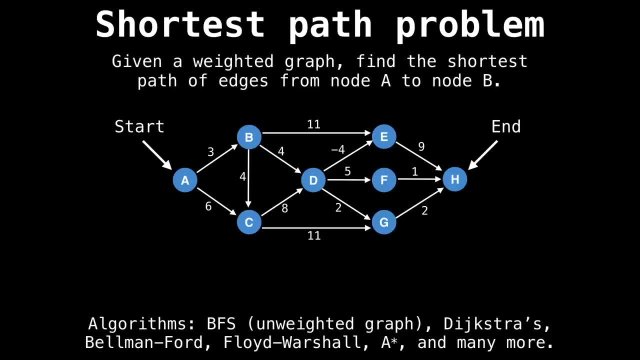 not. the most common problem in graph theory is the shortest path problem. Given a weighted graph, find the shortest path of edges from node A to node B. So if we pretend this graph represents a road system and we're at node A and want to get to node H, our shortest. 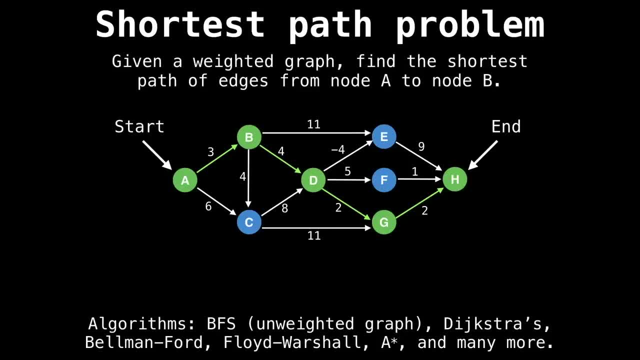 path algorithm should be able to find us a list of edges to find the shortest path algorithm. I'm going to run the graph here. so let's say we're at node A and we're at node A follow. that will lead us from A to H with minimal cost. Lucky for us, many algorithms. 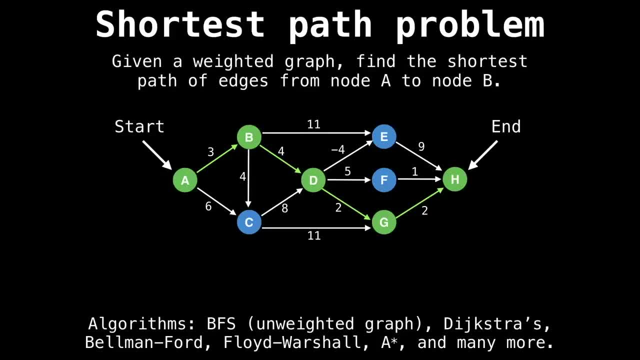 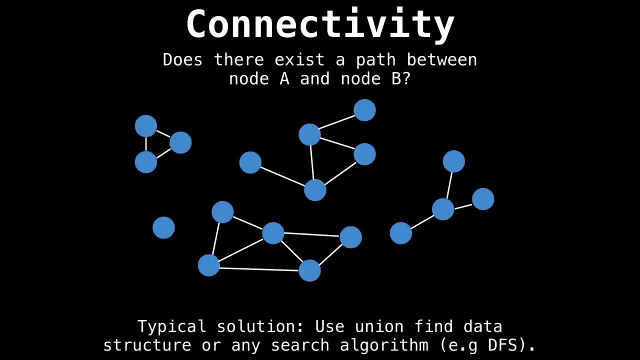 exist to solve the shortest path problem, including a breadth first search for unweighted graphs, Dijkstra's algorithm, Bellman Ford, a star and many more. As simple as it sounds, connectivity is a big issue in graph theory. The problem can also be simplified to does. 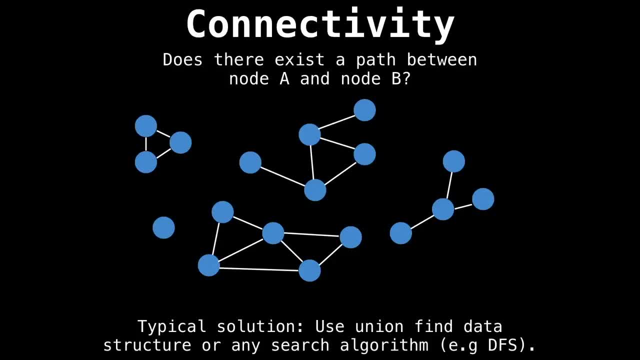 there exist a path from node A to node B. In this scenario, we don't care about the minimum cost, we just want to know can one node reach another node? A typical solution to this problem is to use a union find data structure or do a very basic search algorithm. 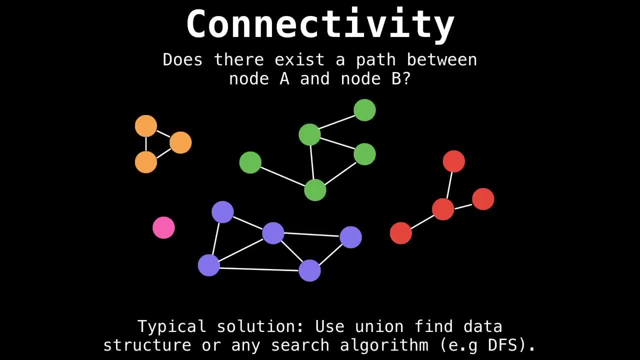 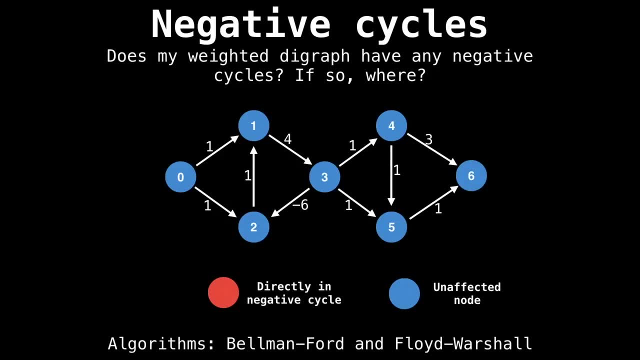 such as a depth first search or a breadth first search. Another common problem is detecting negative cycles in a directed graph. Sometimes we're dealing with graphs that have negative edge weights and we need to know if a negative cycle exists, Because if there does, it can throw everything off In 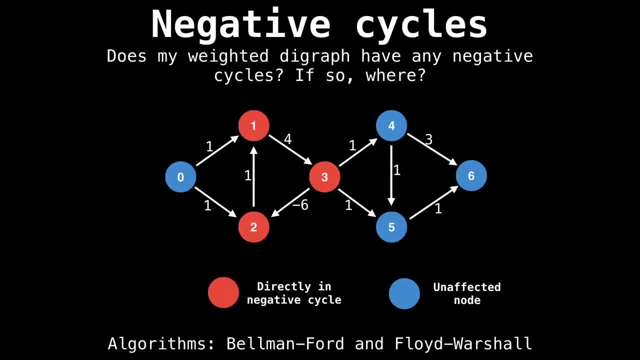 this graph, nodes one, two and three form a negative cycle, Because if you cycle through all the nodes, you end up with a cost of negative one. if you add up all the edge weights, In fact, you can cycle endlessly, getting smaller and smaller costs. 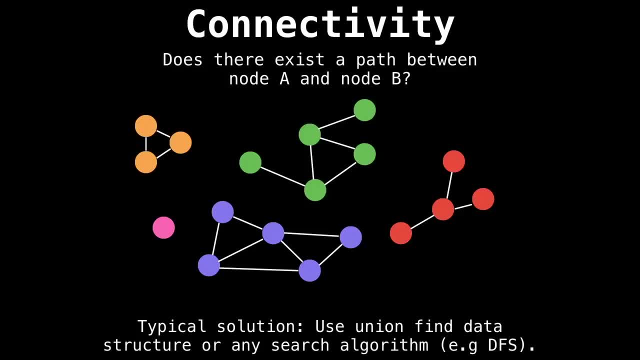 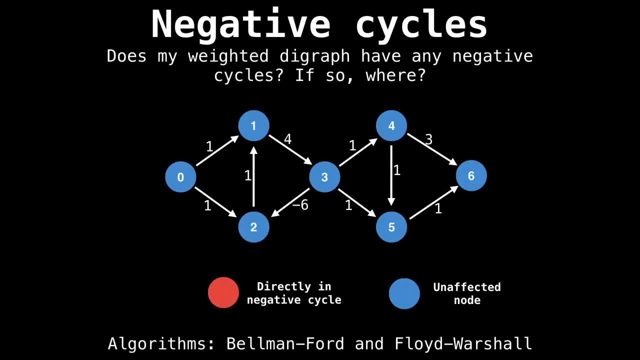 basic search algorithm, such as a depth first search or a breadth first search. Another common problem is detecting negative cycles in a directed graph. Sometimes we're dealing with graphs that have negative edge weights And we need to know if a negative cycle exists, Because if there does, it can throw everything. 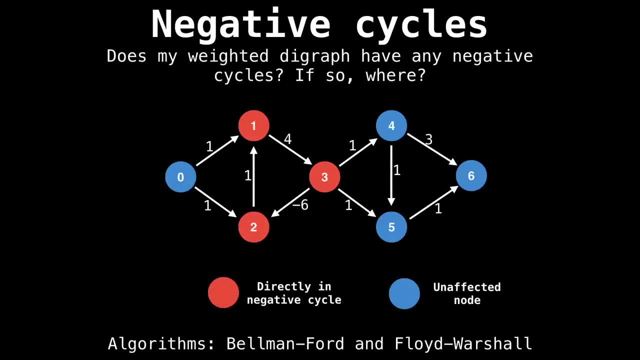 off. In this graph, nodes one, two and three form a negative cycle, Because if you cycle through all the nodes, you end up with a cost of negative one. if you add up all the edge weights, In fact, you can cycle endlessly, getting smaller and smaller costs In the 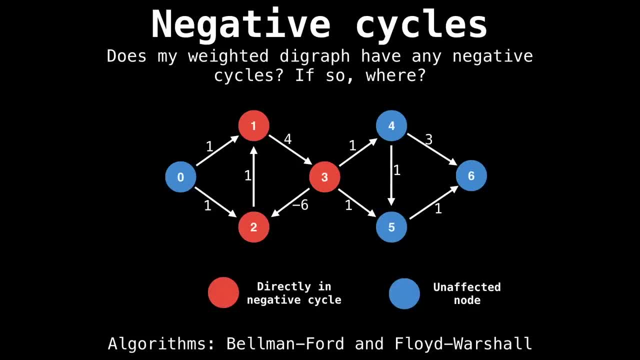 context of finding the shortest path, and negative cycle is The shortest path. A negative cycle is Like a trap that you can never escape. However, there are some contexts where negative cycles are beneficial. Suppose we're trading currencies across an exchange or multiple exchanges. 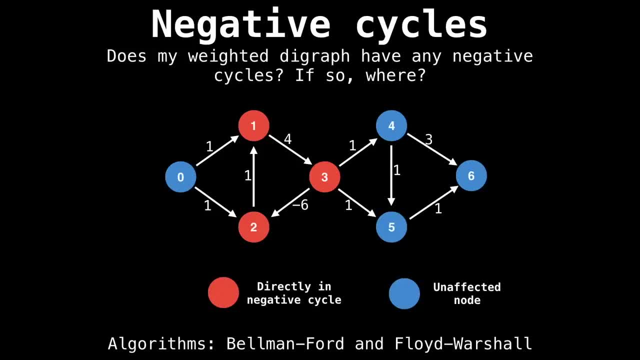 Currency prices try to remain consistent throughout the day across exchanges, such as trading USD to euros or Canadian to yen, But sometimes there are inconsistencies in the currency exchange prices. This makes it possible to do something called arbitrage And arbitrage, which cycles through multiple currencies exchanging one currency. 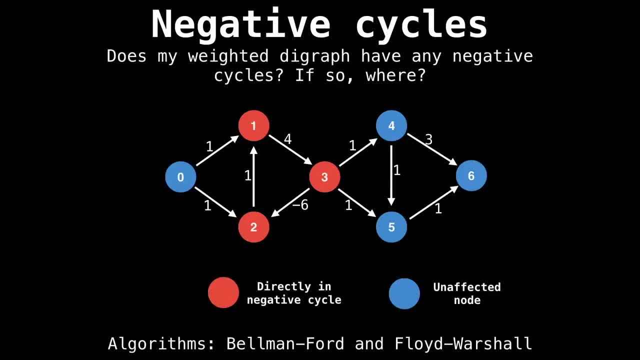 for another and coming back to the original currency with more money than you originally started at a risk free game. This is something we can use graph theory for, because it uses detecting negative cycles. There are two well known algorithms that can detect negative cycles, and those are Bellman Ford and Floyd to Warshall, Something that comes up now, and 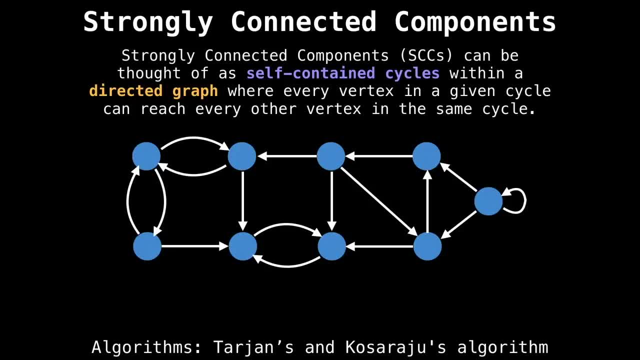 again Is Finding strongly connected components within a graph. This is analogous to finding connected components of an undirected graph, But for directed graphs. when looking at strongly connected components, we're looking for self contained cycles within the graph, where every vertex in a given cycle should be able to reach every other vertex in that same cycle. 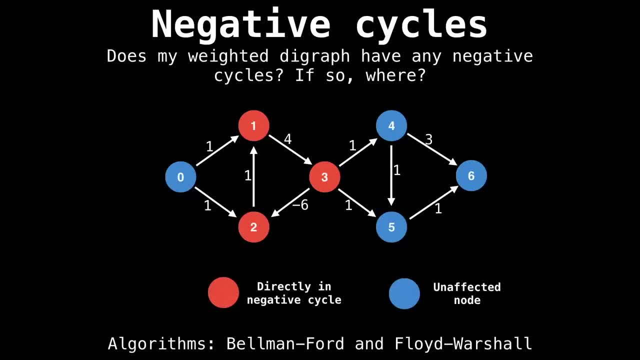 In the context of finding the shortest path, a negative cycle is like a trap that you can never escape. However, there are some contexts where negative cycles are beneficial. Suppose we're trading currencies across an exchange or multiple exchanges. currency prices try to remain consistent throughout the day across exchanges, such as trading USD to euros or 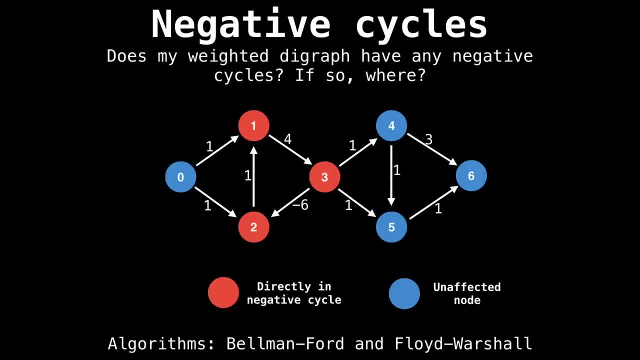 Canadian to yen. But sometimes there are inconsistencies between the two. For example, if you're trading USD to euros or Canadian to yen and you're trading USD to euros or Canadian to yen, you're trading USD to euros or Canadian to yen. You're probably trading the same. 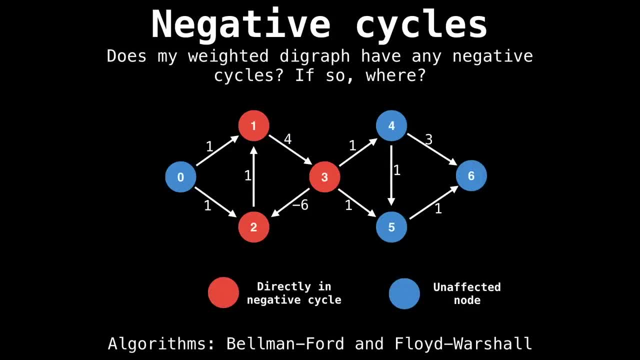 currency and the currency exchange prices. This makes it possible to do something called an arbitrage, which cycles through multiple currencies, exchanging one currency for another and coming back to the original currency with more money than you originally started, at a risk free gain. This is something we can use graph theory for, because it uses detecting. 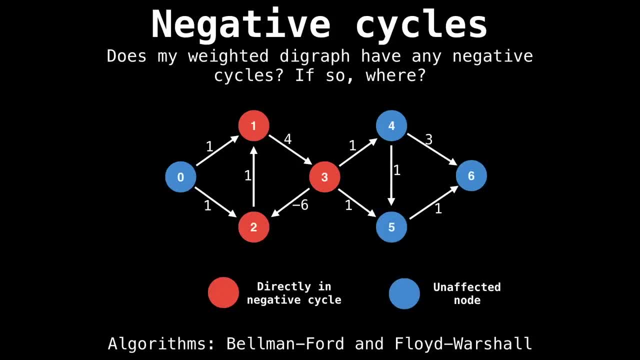 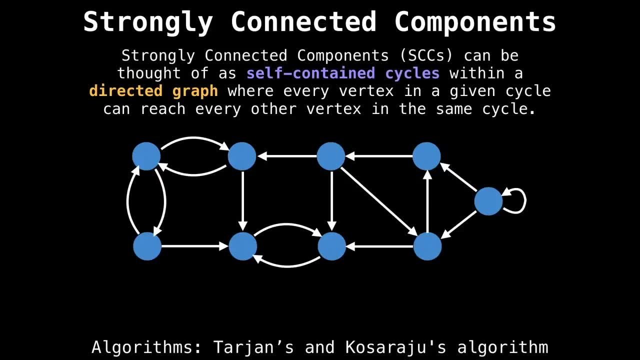 negative cycles. There are two well known algorithms that can detect negative cycles, and those are Bellman ford and florida to Warshall. Something that comes up now and again is finding strongly connected components within a graph. This is analogous to finding connected components of an undirected graph. 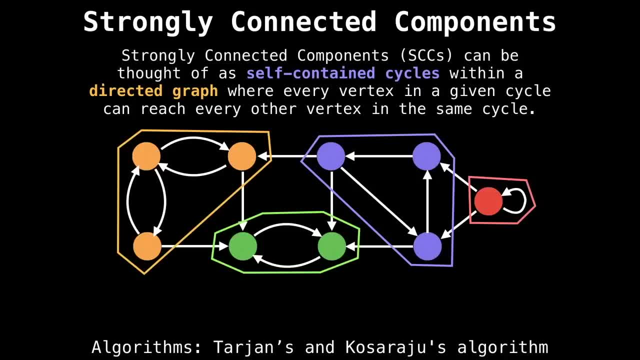 But for directed graphs. when looking at strongly connected components, we're looking for self contained cycles within the graph, where every vertex in a given cycle should be able to reach every other vertex in that same cycle. This is very useful in many algorithms and is usually an intermediate step, So it's important to know how to find these strongly connected. 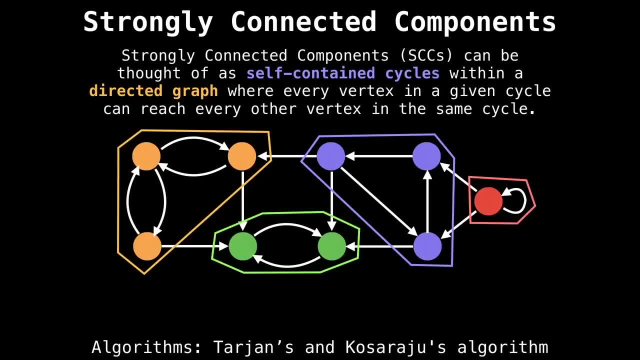 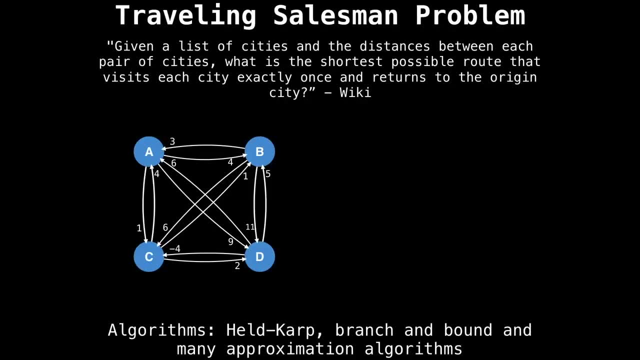 components, And there are many very elegant algorithms to do so, such as Tarzan's algorithm. you probably won't go through your computer science career without hearing about the traveling salesperson problem. The TSP problem is the problem of having a very elegant algorithm. 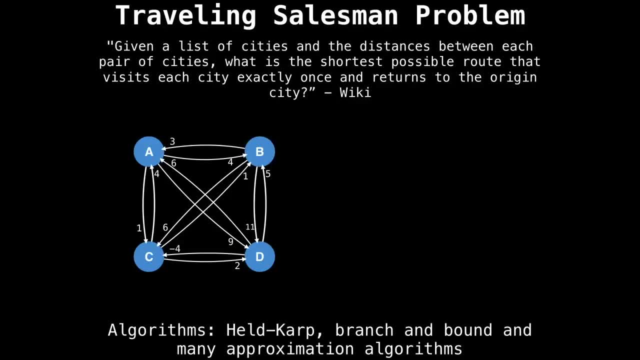 Having n cities and the distances between each of them, and finding the shortest path that visits each city and comes back to the original city at minimum cost. For example, if your graph is the one on the left, a possible TSP solution is the graph on the right, which. 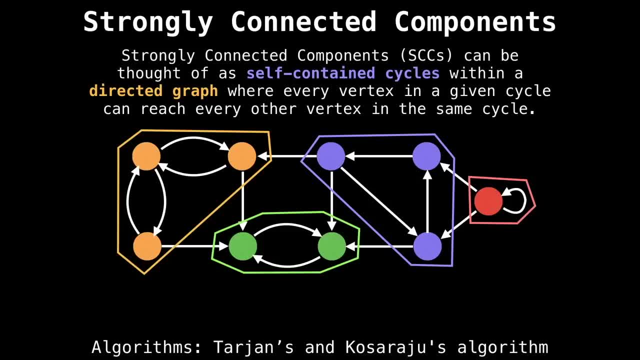 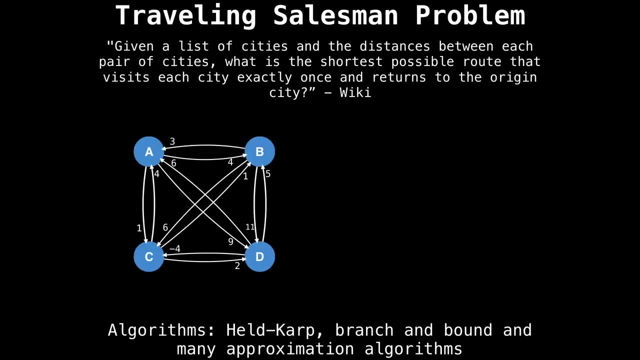 This is very useful in many algorithms and is usually an intermediate Step, So it's important to know how to find these strongly connected components, And there are many very elegant algorithms to do so, such as Tarzan's algorithm. You probably won't go through your computer science career without hearing about the traveling salesperson problem. 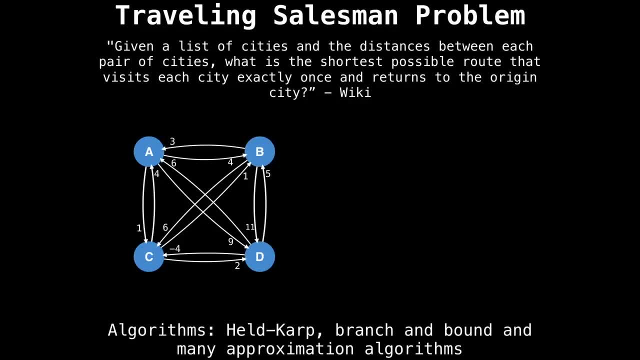 The TSP problem is the problem of having n cities and the distances between each of them and finding the shortest path that visits each city and comes back to the previous one. This problem comes back to the original city at minimum cost. For example, if your graph 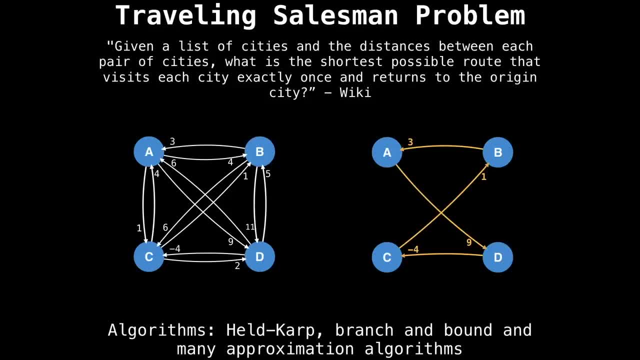 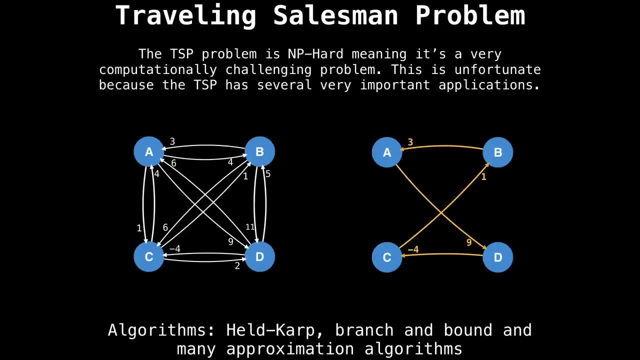 is the one on the left. a possible TSP solution is the graph on the right, which has a cost of nine. The TSP problem is NP hard, meaning it is computationally challenging problem. This is unfortunate because the TSP problem has several very important applications, Some: 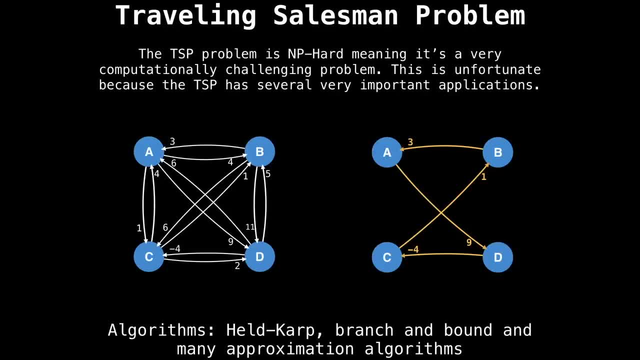 famous algorithms we can use to actually solve this problem. Then there are other algorithms that we can use to actually solve this problem. For example, this is the TSP and the. these are the various algorithms that we can use to actually solve problem. are the healed carp algorithm with dynamic programming doing some kind of branching? 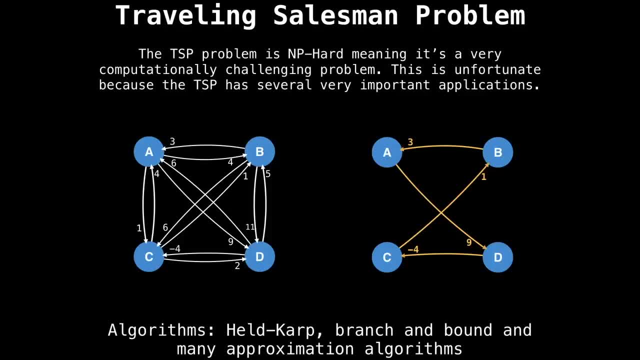 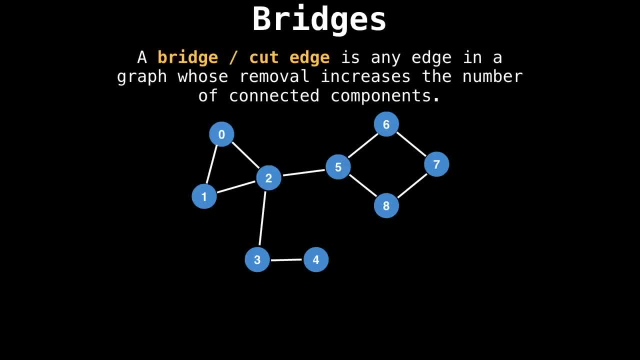 and bounding algorithm, Or you can use one of many, many approximation algorithms, such as the ant colony optimization. This next problem I want to talk about is finding bridges in a graph, which is something of a fascination to me. Bridges are edges which, if removed, 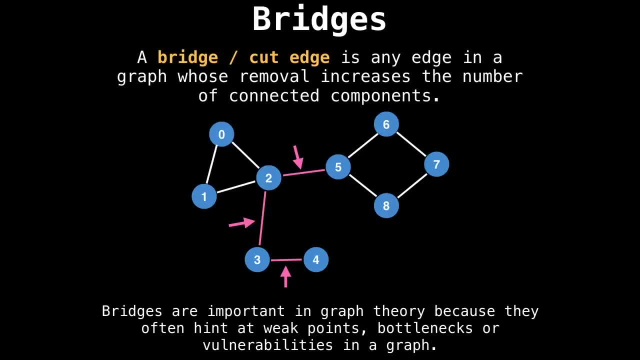 replace the number of connected components in a graph And this graph. the edges highlighted in pink, are bridges. Bridges are important in graph theory because they often hint at weak points, bottlenecks or vulnerabilities in a graph. Think of your graph as a telephone. 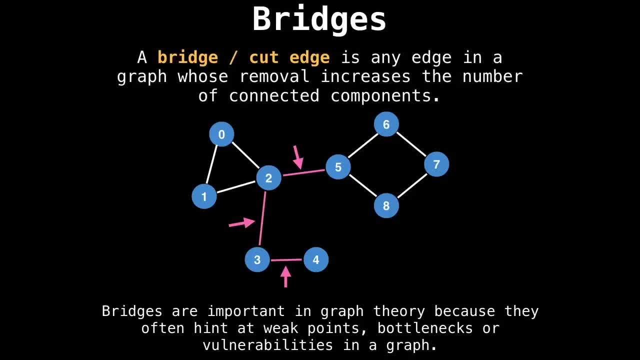 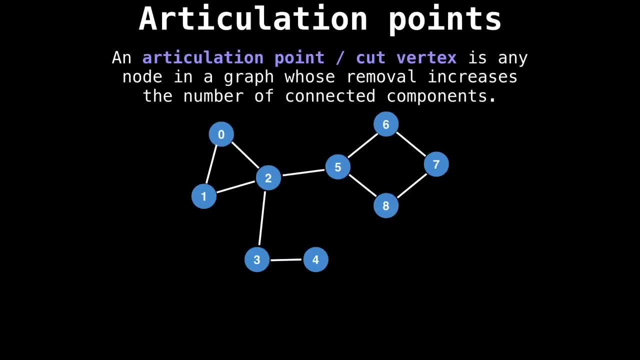 network or a set of bridges between islands. you can immediately see the usefulness of detecting bridges. related to bridges, but not the same, are articulation points, which are nodes that are connected to the graph, And then you can see that the number of connected components in the graph. In this same graph, you can see the three articulation points. 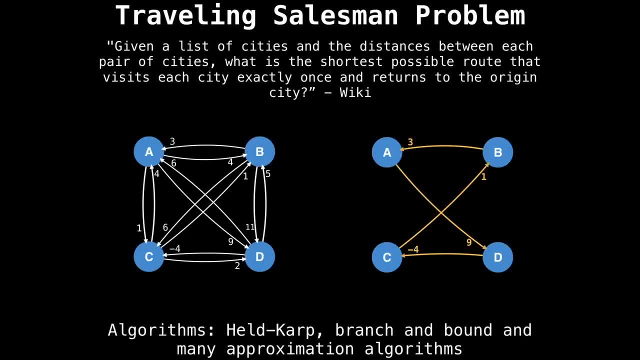 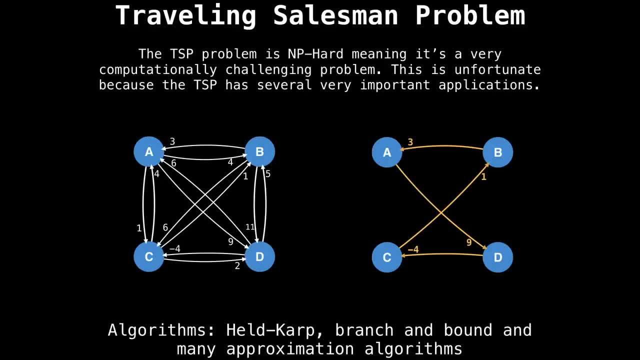 has a cost of nine. The TSP problem is NP hard, meaning it is computationally challenging problem. This is unfortunate because the TSP problem has several very important applications. Some famous algorithms we can use to actually solve this problem are the heeled carp algorithm with dynamic programming doing some kind. 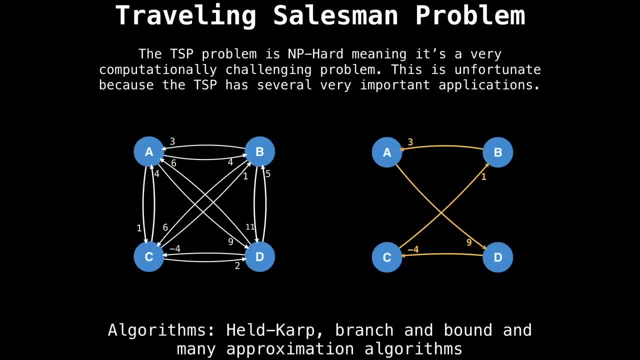 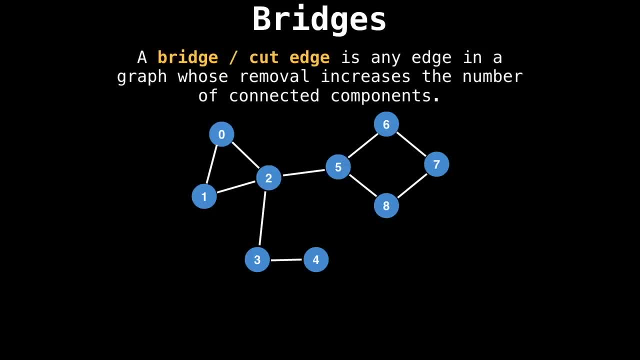 of branching and bounding algorithm, Or you can use one of many, many approximation algorithms, such as the ant colony optimization. This next problem I want to talk about is finding bridges in a graph, which is something of a fascination to me. Bridges are edges, and 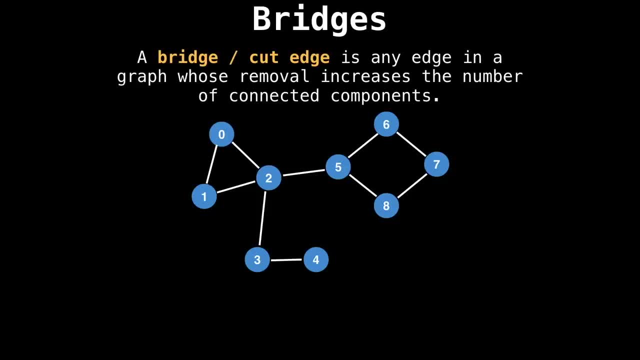 these are edges which, if removed, increase the number of connected components in a graph And this graph. the edges highlighted in pink are bridges. Bridges are important in graph theory because they often hint at weak points, bottlenecks or vulnerabilities in a graph. 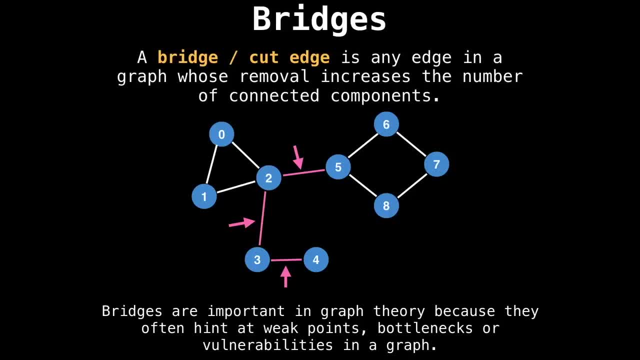 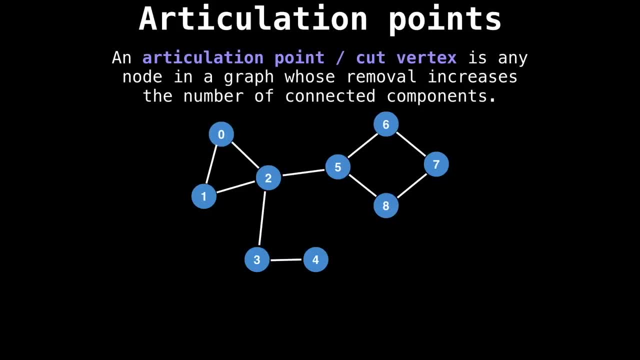 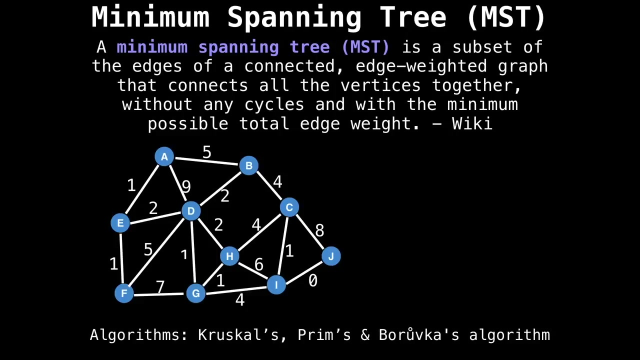 Think of your graph as a telephone network or a set of bridges between islands. you can immediately see the usefulness of detecting bridges related to bridges, but not the same. Our next problem is finding the minimum spanning tree of a graph. A minimum spanning tree is: 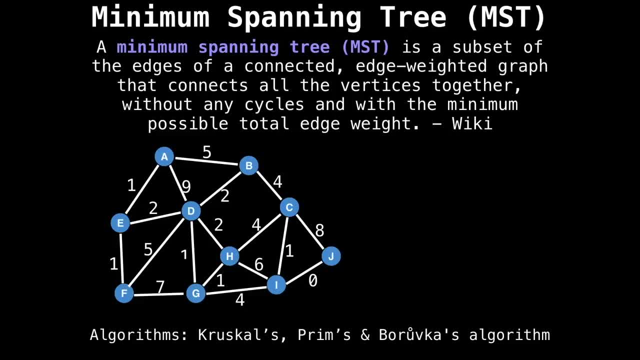 a subset of the edges that connects all the vertices together without any cycles and with minimal possible cost. So, in summary, it's a tree tree, meaning it has no cycles and it spans the graph at a minimal cost. Hence why we give it the name minimum spanning tree. For example, in the graph below, one of the possible 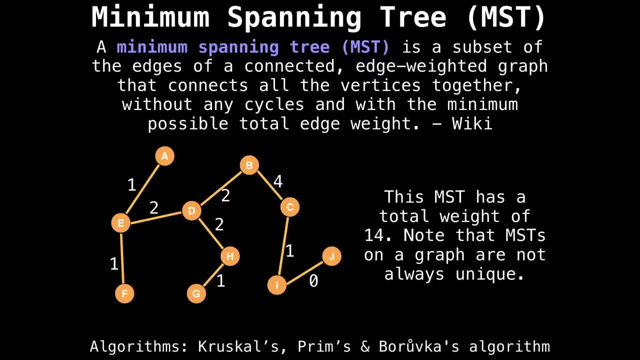 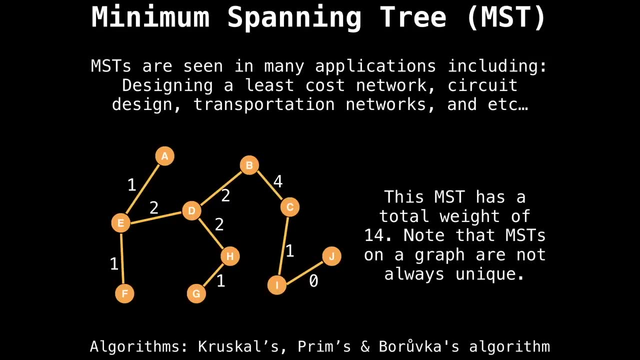 minimum spanning trees is this graph with a least cost of 12.. Note that all minimum spanning trees of a graph have the same minimal cost but are not necessarily identical. Minimum spanning trees are seen in lots of different applications in computer science, including designing a least cost network, circuit design, transportation networks, you name it. There's. 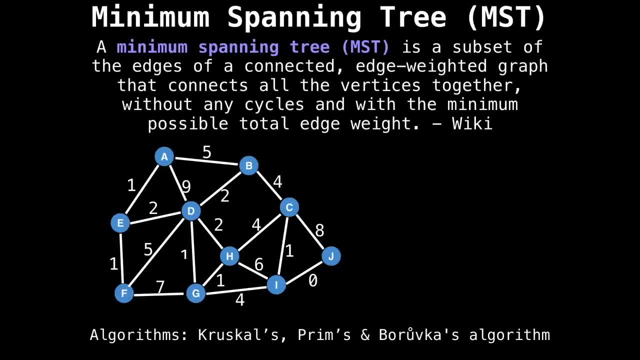 highlighted in pink. Next problem is finding the minimum spanning tree of a graph. a minimum spanning tree is a subset of the edges that connects all the vertices together without any cycles and with minimal possible cost. So, in summary, it's a tree, meaning it has. 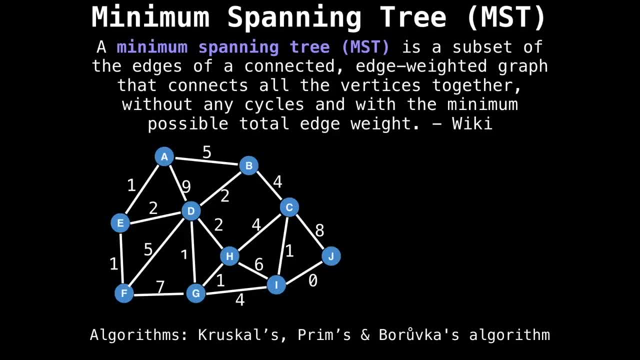 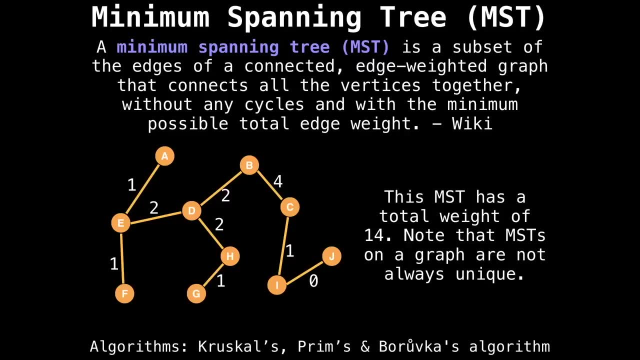 no cycles And it spans the graph at a minimal cost, Hence why we give it the name minimum spanning tree. For example, in the graph below, one of the possible minimum spanning trees is this graph with a least cost of 12.. Note that all minimum spanning trees of a graph have the same minimal. 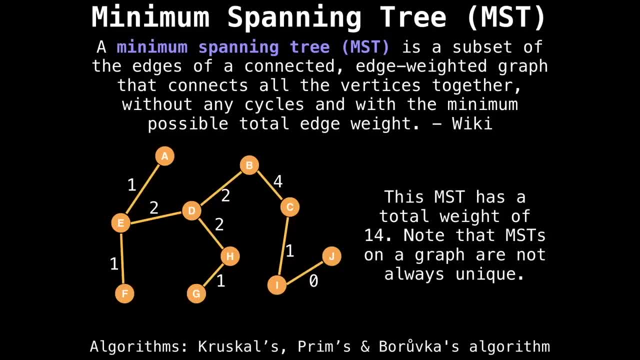 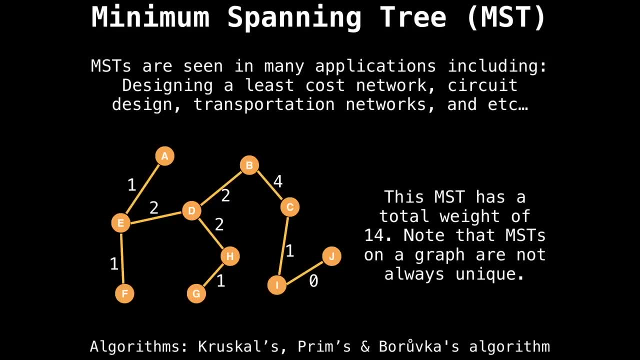 cost but are not necessarily identical. Minimum spanning trees are seen in lots of different applications in computer science, including designing a least cost network, circuit design, transportation networks, you name it. There's also several approximation algorithms which rely on minimum spanning trees, which is pretty interesting If you want to find a minimum spanning tree of a. 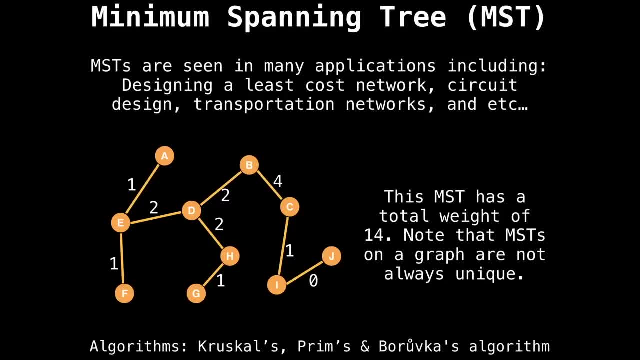 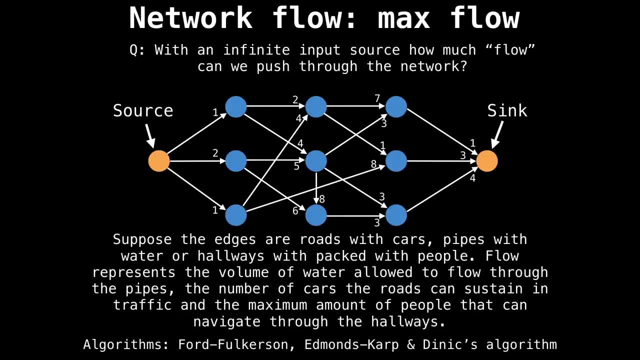 graph, I recommend using one of Kruskal's primes or bar of cars algorithm. This last problem, I think, is the most fascinating, and it is about finding the maximum flow through a special type of graph called a flow network. flow networks are networks where edge weights represent capacities. in some 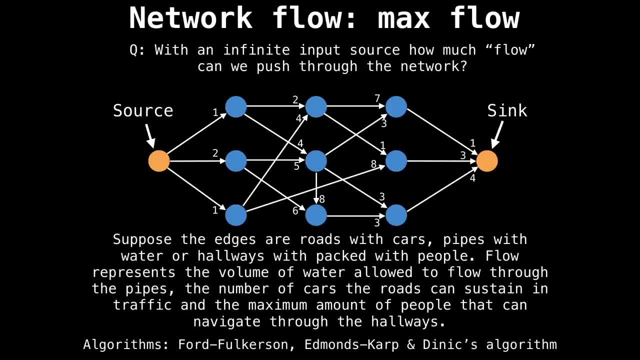 sense. capacities might be things like the maximum amount of cars that fit on a road, or the maximum amount of volume that can flow through a pipe, or even the number of boats a river can sustain without destroying the environment, And these types of flow networks we often find. 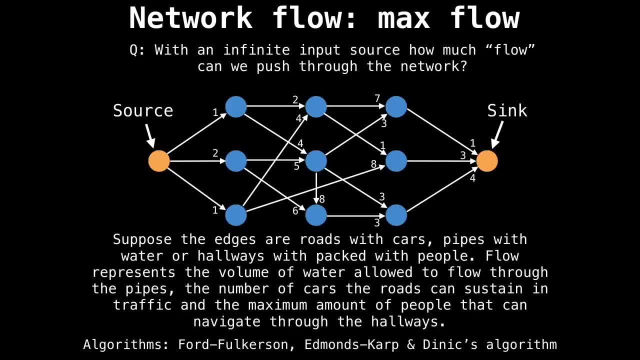 ourselves asking the question: with an infinite input source, that is, a cars, water, boats, whatever- how much flow can I push through the network, assuming we start at some source and try and make it to some sink node? This question is important because at some point there is bound to be a bottleneck. 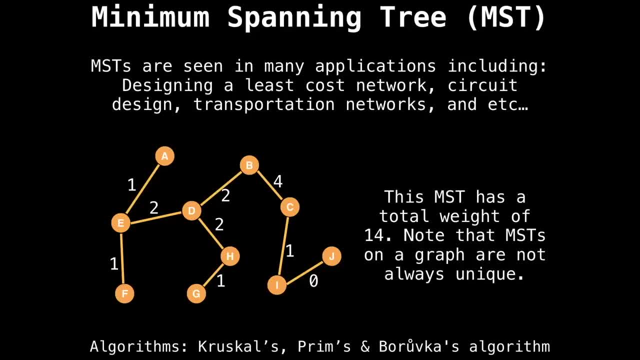 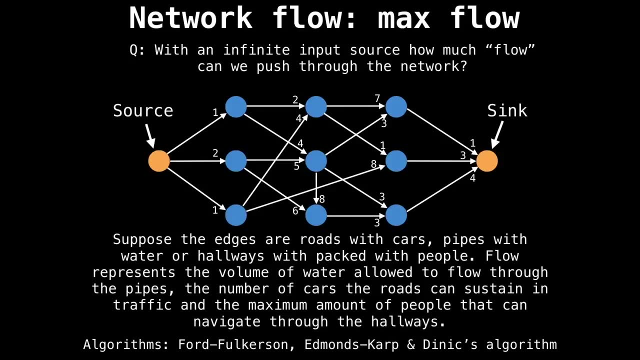 also several approximation algorithms which rely on minimum spanning trees, which is pretty interesting. If you want to find a minimum spanning tree of a graph, I recommend using one of Kruskal's, Primm's or Barovka's algorithm. This last problem, I think, is the most fascinating. 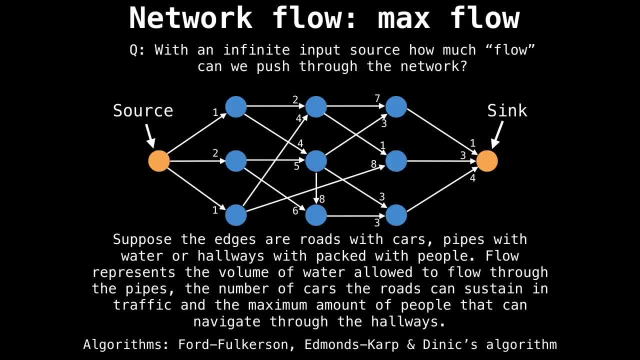 and it is about finding the maximum flow through a special type of graph called a flow network. Flow networks are networks where edge weights represent capacities. in some sense, Capacities might be things like the maximum amount of cars that fit on a road or the maximum amount. 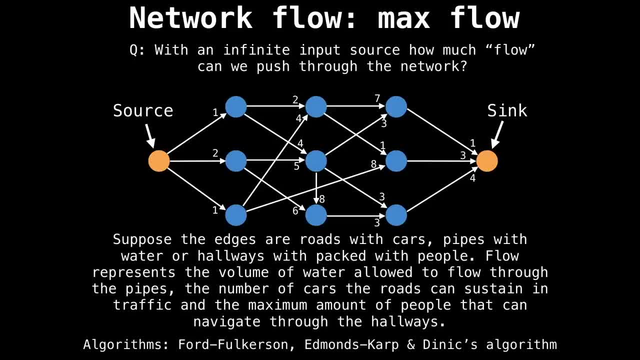 of volume that can flow through a pipe, or even the number of boats a river can sustain without destroying the environment And these types of flow networks. we often find ourselves asking the question: with an infinite input source, that is, a cars, water, boats, whatever- how much flow can I push through the network, Assuming 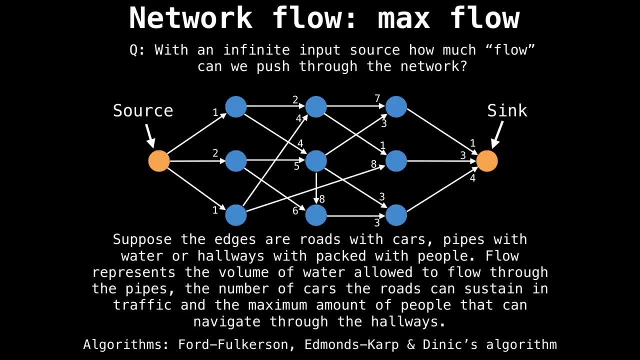 we start at some source and try and make it to some sync node. This question is important because at some point there is bound to be a bottleneck somewhere in our flow graph that limits the amount of stuff we can use. What about traffic? How much traffic that flows down the track and how much traffic? 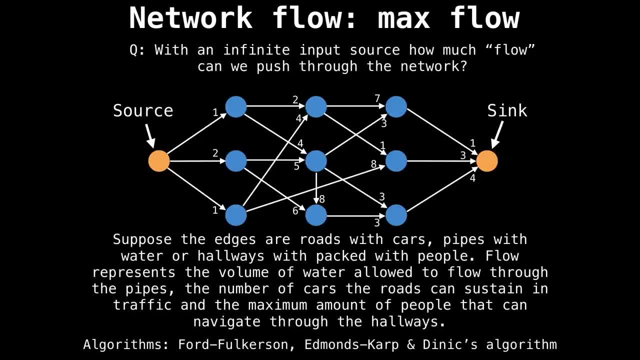 is there How many rows and how many tracks? And of course that is a dance. Now let's have traveling on the network, making it from point A to point B. the maximum flow would then represent things like the volume of water allowed to flow through the network of pipes. 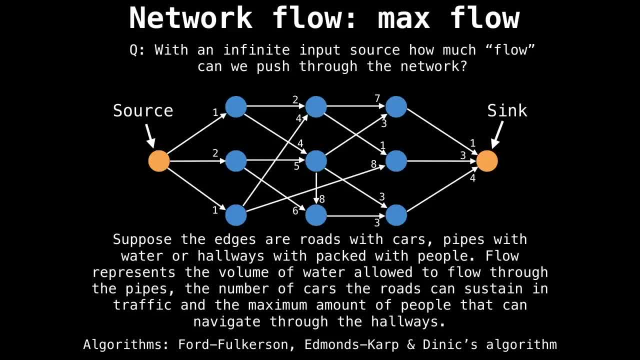 the number of cards the roads can sustain in traffic or the maximum amount of boats allowed on the river. With these maximum flow problems, we can identify the bottlenecks that slow down the whole network and fix the edges that have lower capacities. We're moving on to talking. 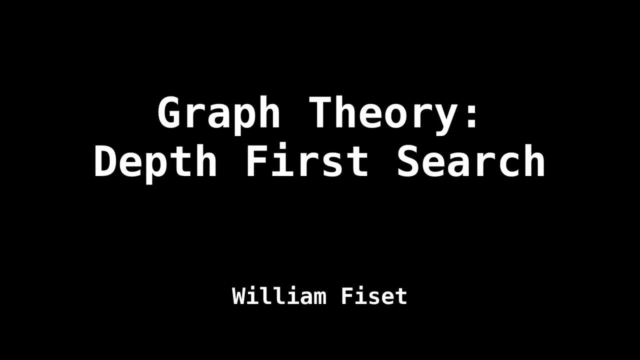 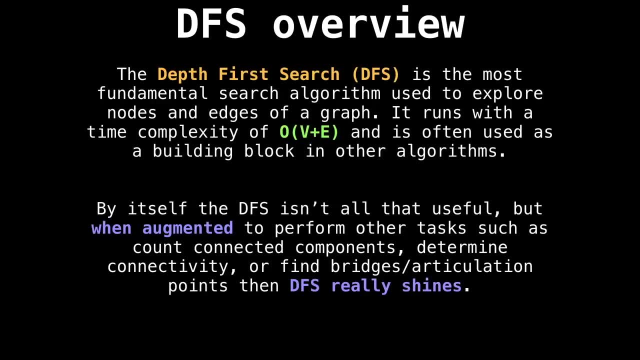 about the depth first search algorithm, which plays a central role in several graph theory algorithms. So what is a depth first search? a depth first search is a core algorithm in graph theory that allows you to explore nodes and edges of a graph, So it's a form of traversal. 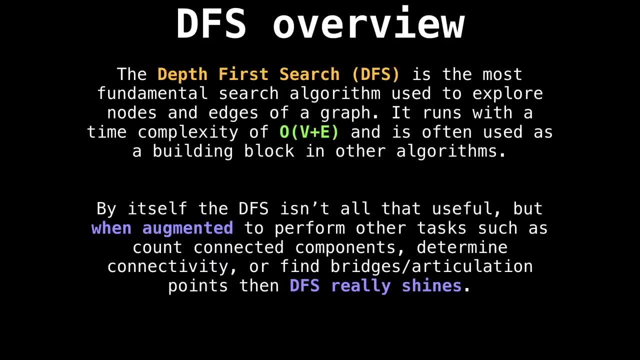 algorithm. The nice thing about a depth first search is that it's really easy to code And it runs in a time complexity of big O, of V plus E, that is, vertices plus edges, which is directly proportional to the size of your graph By. 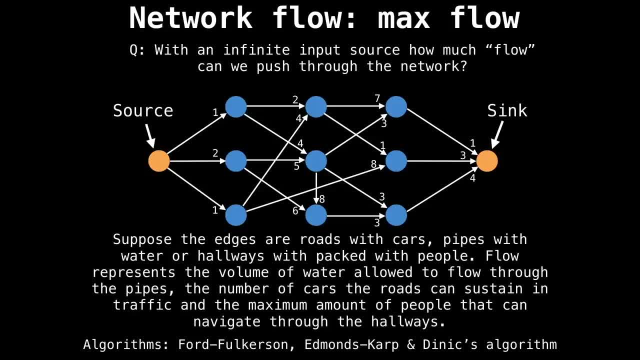 somewhere in our flow graph that limits the amount of stuff we can have traveling on the network, making it from point A to point B be the maximum flow with that, and represent things like the volume of water allowed to flow through the network of pipes, the number of cards the roads can sustain in traffic. 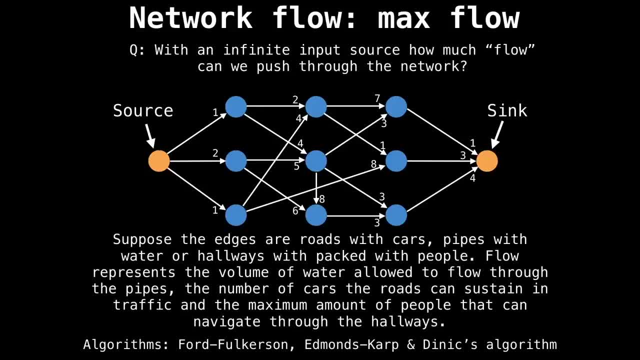 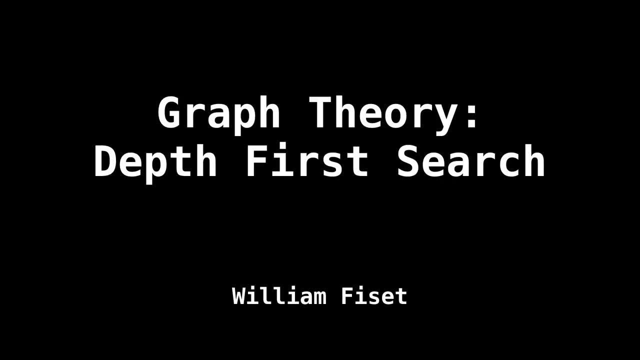 or the maximum amount of boats allowed on the river. With these maximum flow problems, we can identify the bottlenecks that slow down the whole network and fix the edges that have lower capacities. We're moving on to talking about the depth first search algorithm. 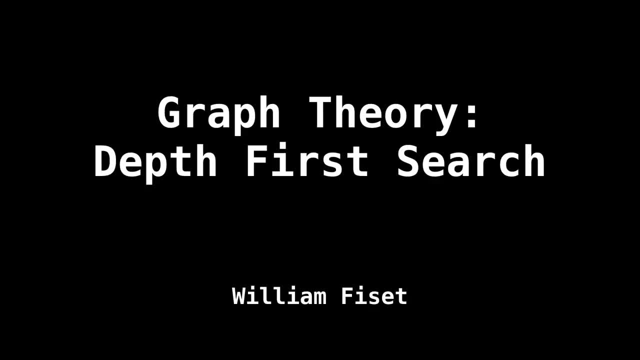 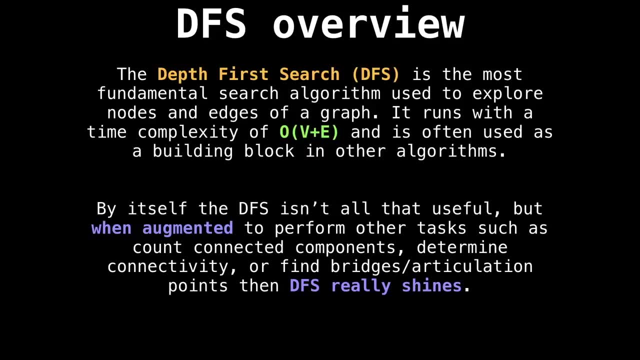 which plays a central role in several graph theory algorithms. So what is a depth first search? a depth first search is a core algorithm and graph theory that allows you to explore nodes and edges of a graph, So it's a form of traversal algorithm. The nice thing about 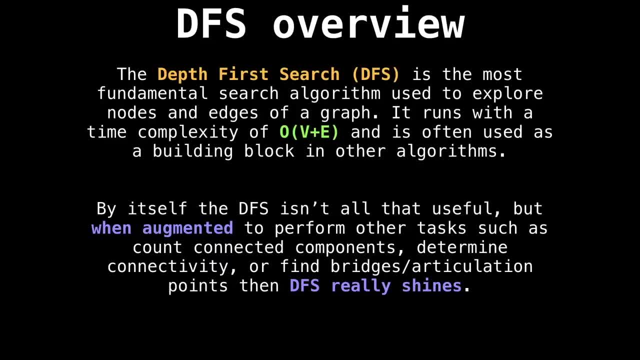 a depth first search is that it's really easy to code And it runs in a time complexity of big O, of V plus e, that is, vertices plus edges, which is directly proportional to the size of your graph. By itself, a depth first search isn't. 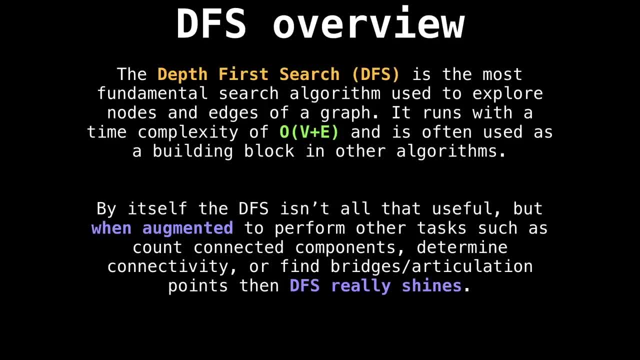 all that useful, But when augmented to perform other tasks such as count connected components, determine connectivity between nodes or find bridges and articulation points, the depth first search can be done. So just if you want to know how a depth first search works you. 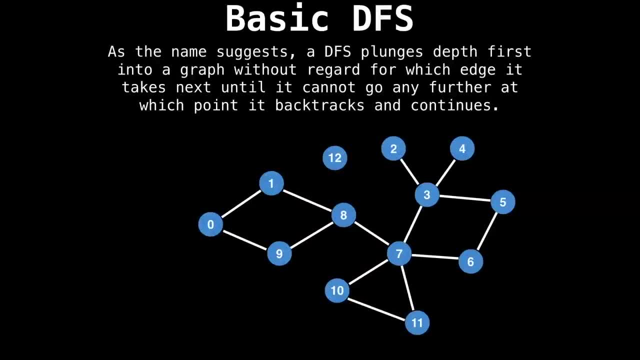 first search algorithm really shines. So let's look at an example. As the name suggests, a depth first search plunges depth first into a graph, without regard for which edge it selects next, until it cannot go any further, at which point it backtracks and continues its exploration. 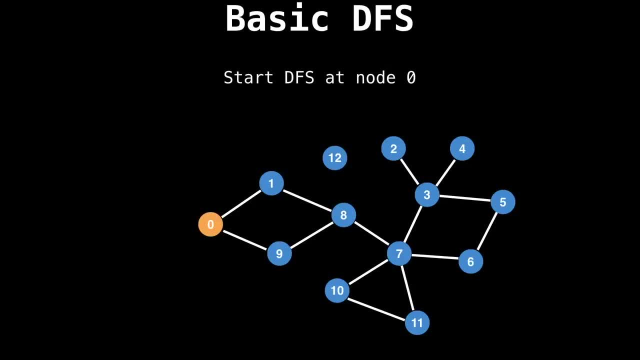 So a depth first search has to start on a node, And I'm going to start our depth first search on node zero. And now we arbitrarily pick a node to go to some from node zero, we're going to go to node nine. then, from node nine, we only have one choice, which. 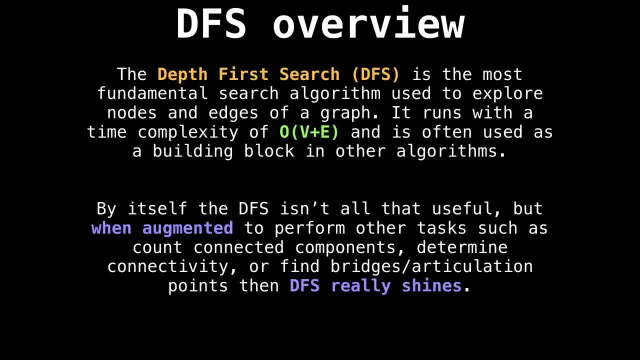 itself, a depth first search isn't all that useful, But when augmented to perform other tasks such as count connected components, determine connectivity between nodes or find both Bridges and articulation points, the depth first search algorithm really shines. So let's. 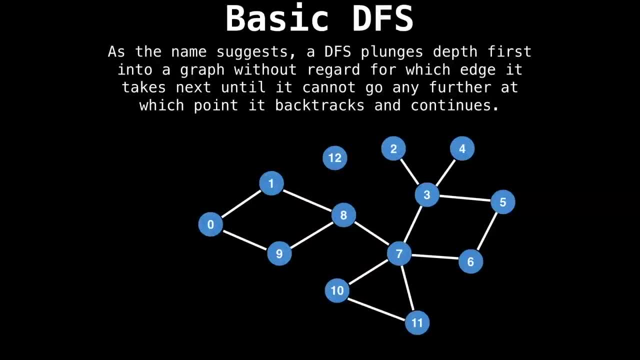 look at an example. As the name suggests, a depth first search plunges depth first into a graph, without regard for which edge it selects next, until it cannot go any further, at which point it backtracks and continues its exploration. So a depth first search has to start on a node. 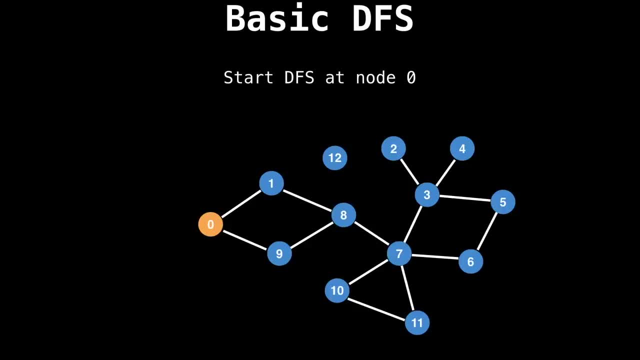 and I'm going to start our depth first search on node zero. And now we arbitrarily pick a node to go to some. from node zero, we're going to go to node nine. then, from node nine, we only have one choice, which is to go to node eight. at node eight, arbitrarily pick an. 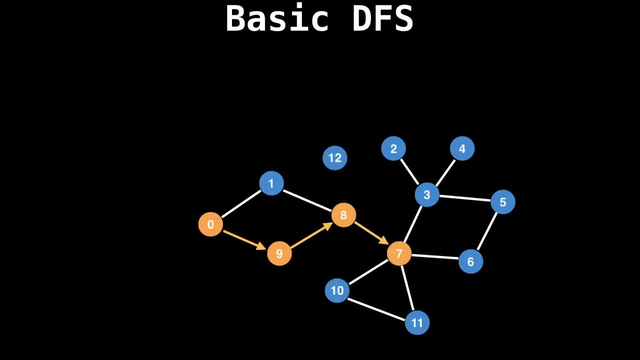 edge. So we're going to go outwards to node seven, node seven: we have plenty of edges to choose from, So let's go to node 10.. node 10 to node 11., 10., 10., 10.. 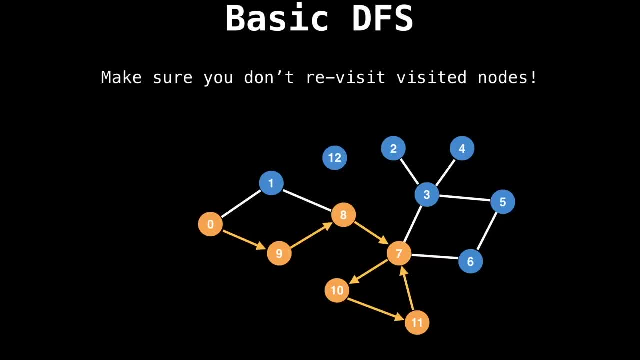 And 11 to seven. So we don't want to revisit already visited nodes or nodes that are currently being visited. So we have to backtrack. to indicate backtracking, I'm going to label edges and nodes as gray So backtrack all the way back to node seven. So we're not finished exploring. 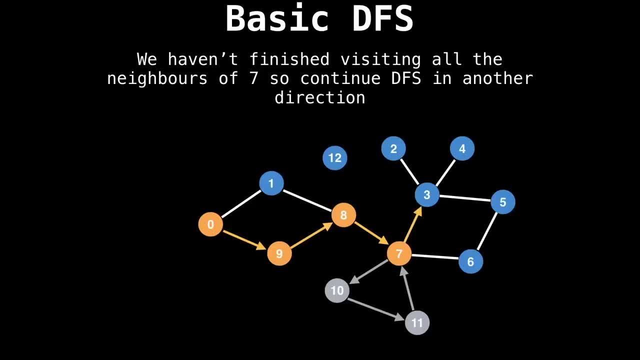 node seven because there are still edges to be picked. So I'm going to go to node three and node three. I'm going to go to node two. node two is a dead end, So we backtrack, then go to node four. node four is also a dead end. So 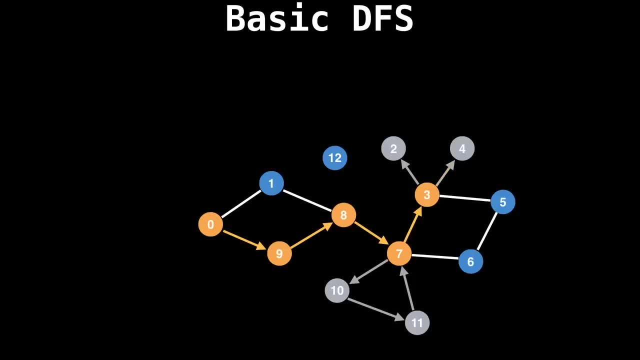 backtrack from node four back to node three, then pick node threes, last edge to go node 552, six and six to seven. can't go to seven because we're visiting seven currently. So backtrack all the way back to node seven, Back to node eight. From node eight. we still need to visit its last edge, which goes to. 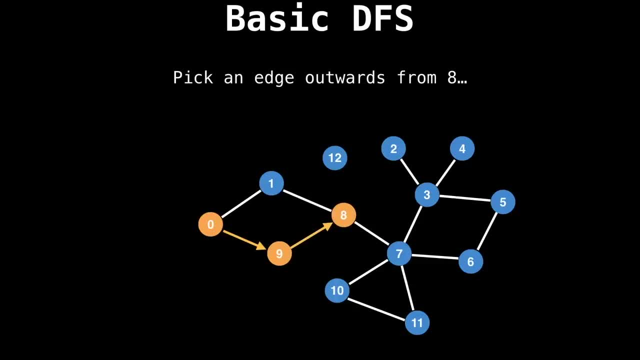 is to go to node eight. at node eight, arbitrarily pick an edge, So we're going to go outwards to node seven, node seven. we have plenty of edges to choose from, So let's go to node 10, node 10 to node 11, and 11 to seven. 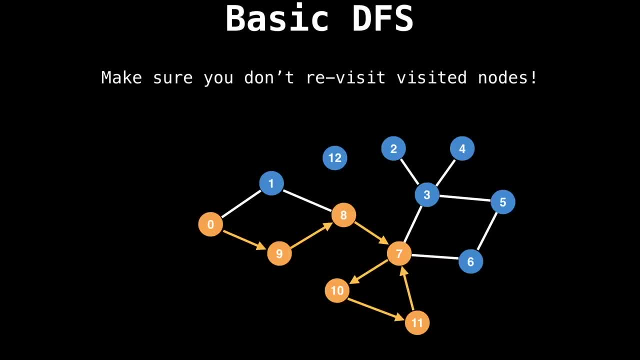 So we don't want to revisit already visited nodes or nodes that are currently being visited, So we have to backtrack. to indicate backtracking, I'm going to label edges and nodes as gray, So backtrack all the way back to node seven. So we're not finished exploring node seven. 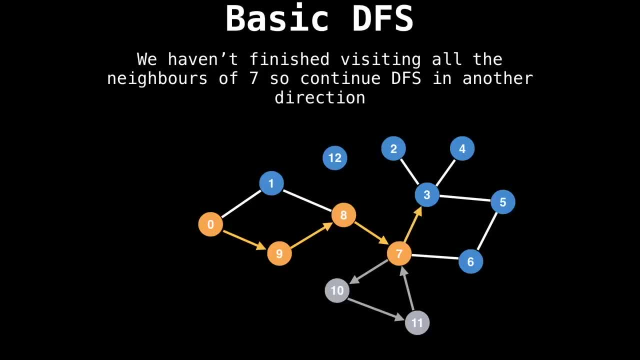 because there are still edges to be picked. So I'm going to go to node three And node three. I'm going to go to node two. node two is a dead end, So we backtrack, then go to node four. node four is also a dead end, So backtrack from node four back. 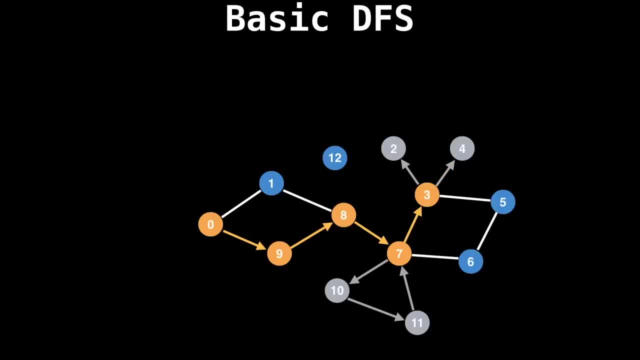 to node three, then pick node threes, last edge to go node 552, six and six to seven. can't go to seven because we're visiting seven currently, So backtrack all the way back to node eight From node eight. we're visiting seven, So backtrack all the way back to node eight from node eight. 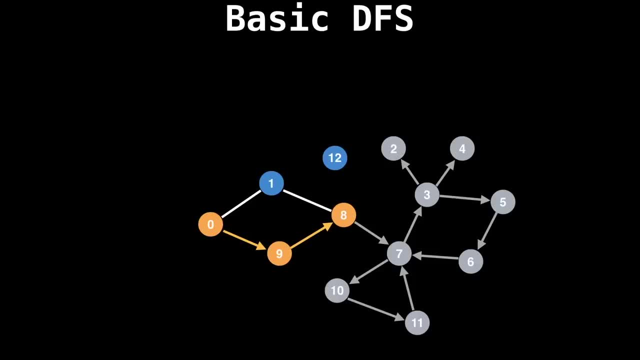 we still need to visit its last edge, which goes to node one, node one, back to node zero. we can't go to node zero because we're currently exploring it- then backtrack all the way to zero, which completes our depth first search traversal of this graph. So this was one particular depth. 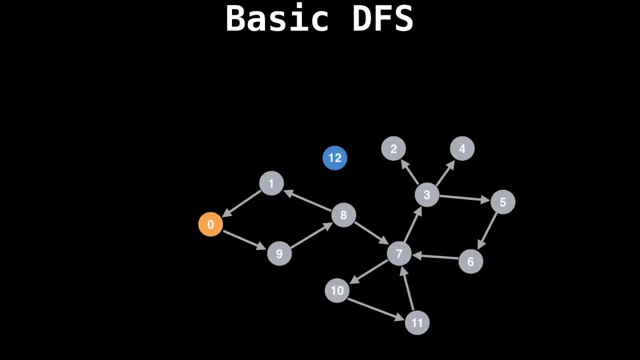 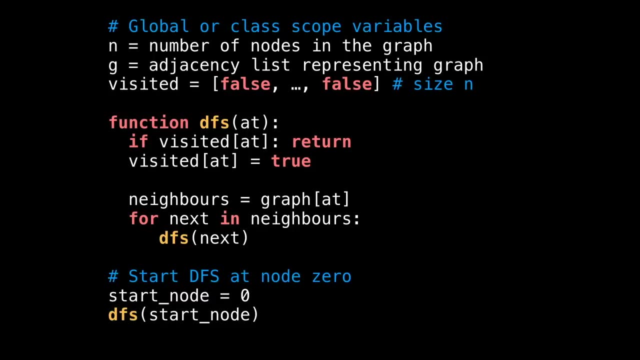 first search traversal, But, as you saw, it could have gone a lot of different ways. So now let's look at some pseudocode for this depth first search to get a deeper understanding of how it works. The first thing we'll need to do is initialize these three variables, which are: n. the number of nodes. 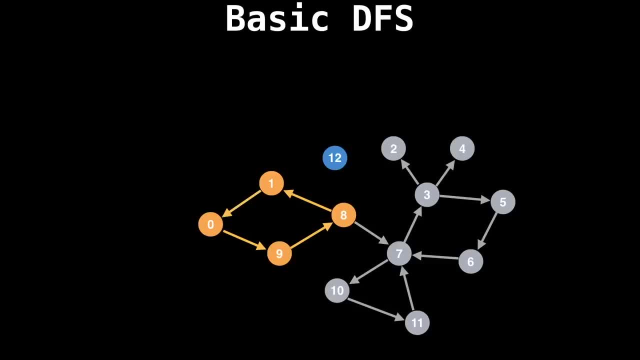 node one, node one back to node zero. we can't go to node zero because we're currently exploring it- then backtrack all the way to zero, which completes our depth first search traversal of this graph. So this was one particular depth first search traversal, But, as you saw, 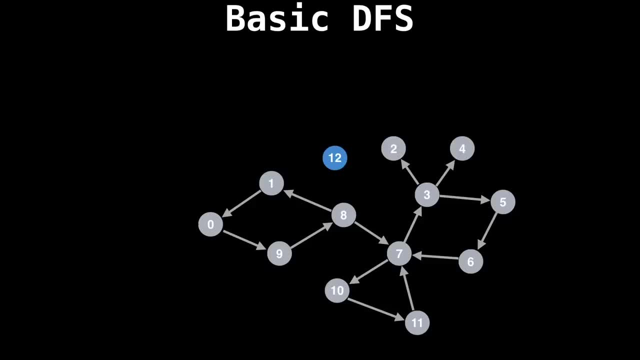 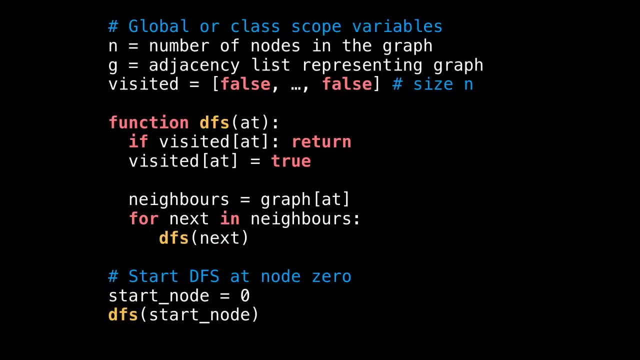 it could have gone A lot of different ways. So now let's look at some pseudocode for this depth first search to get a deeper understanding of how it works. The first thing we'll need to do is initialize these three variables, which are: n- the number of nodes in our graph, g- the adjacency list. 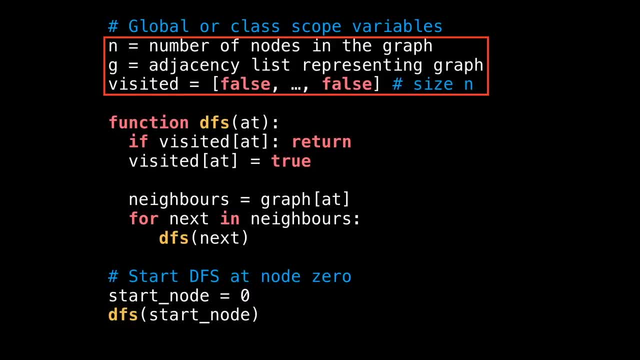 representing the graph and visited a Boolean array Containing true or false at index i, depending on whether or not node i has been visited. In the beginning, this array should have all false values because we have not visited any nodes in the graph. Once that is set up at the bottom, I define our starting node to: 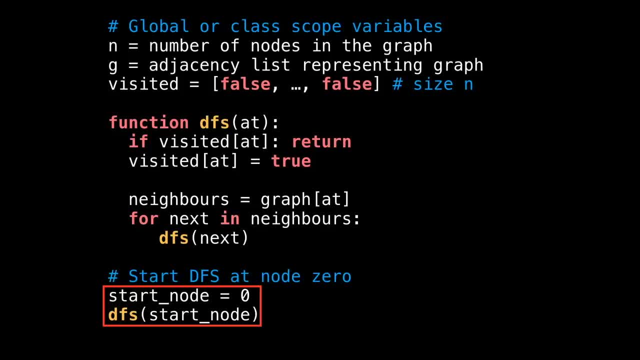 be node zero and then call the depth first search method to do the exploration. The depth first search itself has one argument: The current node. we're going to call it the depth first search method. This method is recursive. So I check the base case, which is whether 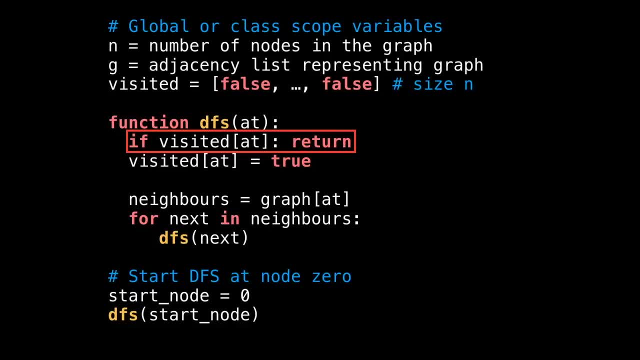 we have already visited this node. If so, we have no business here and can return. Otherwise, let's visit this node by marking it as true and exploring all of its neighbors. To explore all the neighbors of the node, reach into the adjacency list and pull out all the neighbors. 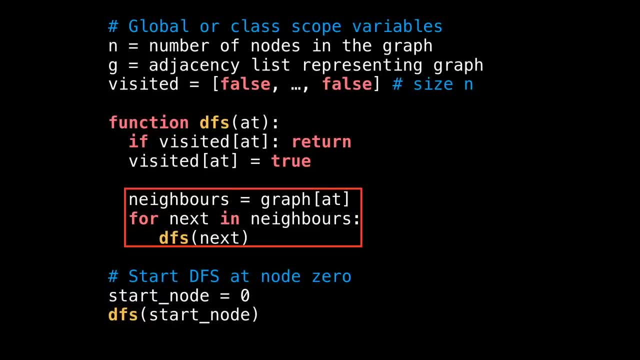 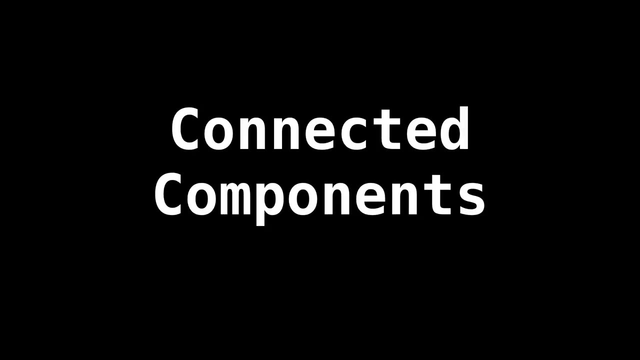 of this node And explore them depth first by looping over each and recursively calling the depth first search method. And that's all a depth first search really is in a nutshell. Let's look at another simple use case for depth first search. I want to discuss finding connected. 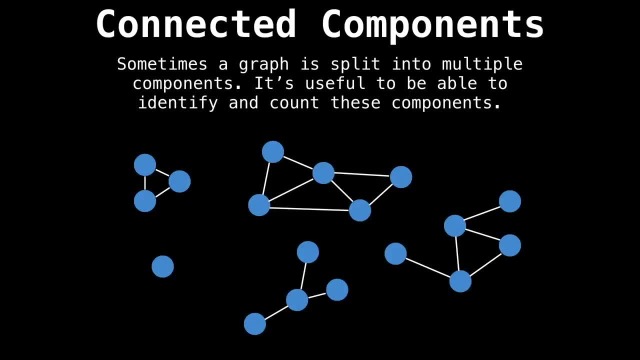 components in a graph. First, let's understand what we mean by connected component. Sometimes a graph is split into multiple disjoint components And it's useful to be able to identify and count these components. One way to identify these components might be to color them so we can tell them apart. But what does coloring? 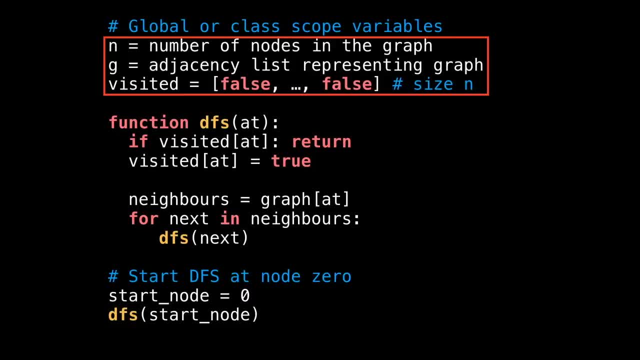 in our graph g- the adjacency list representing the graph, and visited a Boolean array containing true or false, And then we'll add the index i, depending on whether or not node i has been visited. In the beginning, this array should have all false values because we have not visited any nodes in the graph Once. 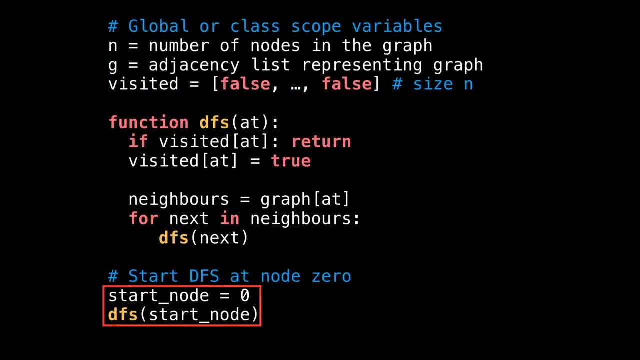 that is set up at the bottom. I define our starting node to be node zero and then call the depth first search method to do the exploration. The depth for search itself has one argument: the current node we are at, which I have a convenient 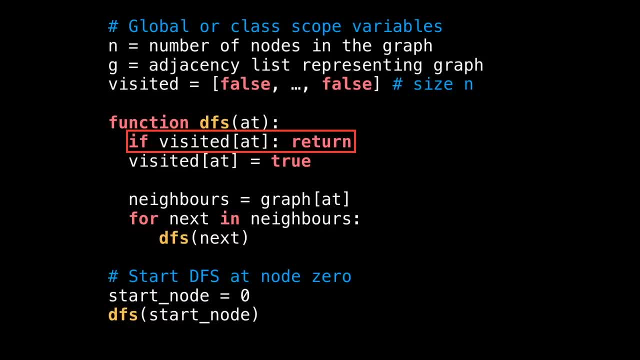 index. index index conveniently named at. this method is recursive, So I checked the base case, which is whether we have already visited this node. If so, we have no business here and can return. Otherwise, let's visit this node by marking it as true and exploring all of its neighbors To explore. 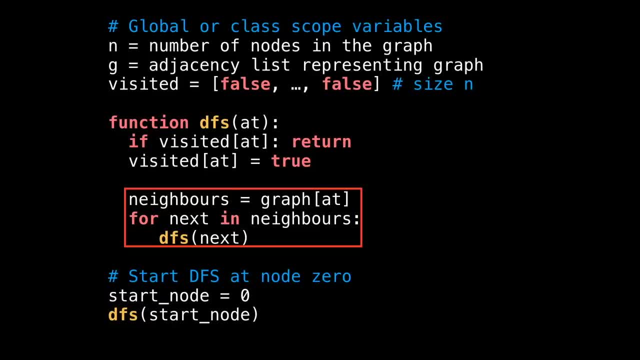 all the neighbors of the node. reach into the adjacency list and pull out all the neighbors of this node and explore them depth first by looping over each and recursively calling the depth first search method. And that's all. a depth first search really is in a nutshell. 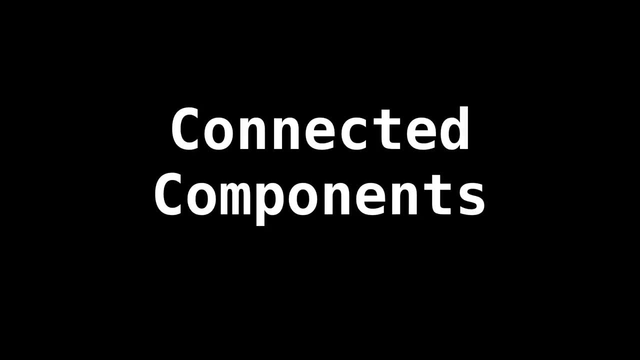 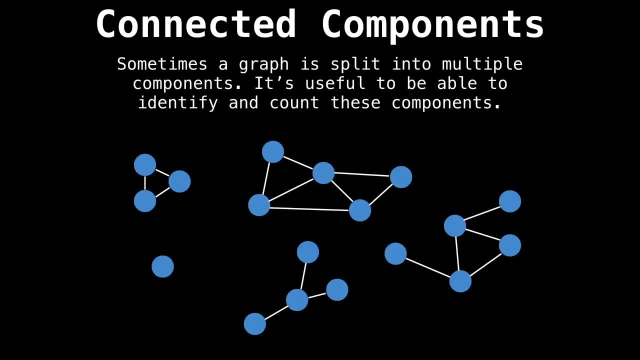 Let's look at another simple use case for depth first search. I want to discuss finding connected components in a graph. First, let's understand what we mean by connected component. Sometimes the graph is split into multiple disjoint components And it's useful to be able to identify and count these components. One way to identify: 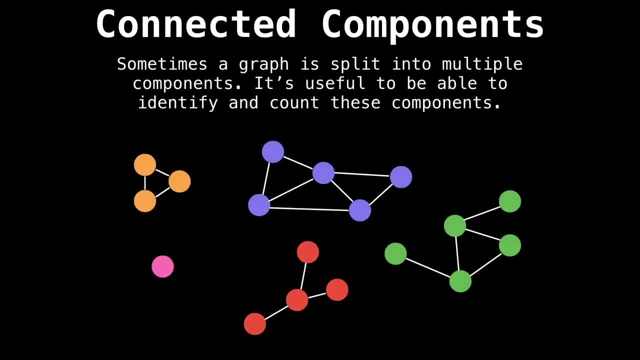 these components might be to color them so we can tell them apart. But what does coloring nodes really mean to a computer? Coloring nodes is equivalent to labeling each node in a component with the same ID value, For example, every node in the purple component. 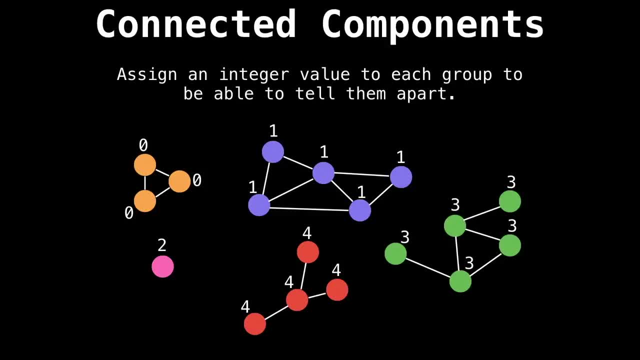 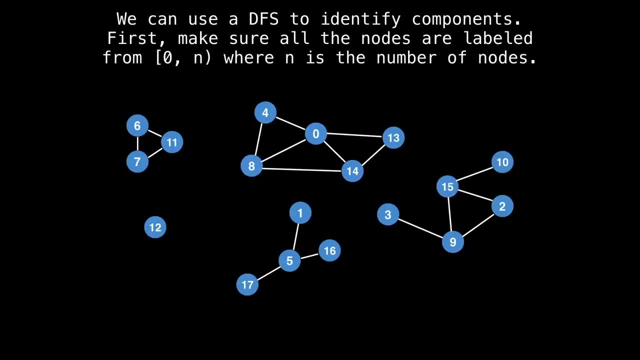 gets an idea of one, and every node in a green component gets an idea of one. so it's just ID of three. we can use a depth first search to identify components this way. First, make sure all the nodes are labeled from zero to n, non inclusive, where n is the number of nodes. 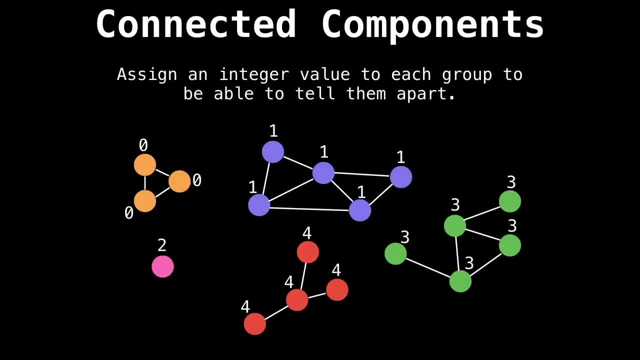 nodes really mean to a computer. coloring nodes is equivalent to labeling each node in a component with the same ID value. For example, every node and the purple component gets an ID of one And every node in the green component gets an ID. Oh Okay, that's great, That's. a perfect example. For example, each node in the purple component gets an ID of green. Here's a perfom to us ischez. In this case, the first instance would be the first one when thisse tactic will green At first 되고. is there a response outside the context to generate a query? 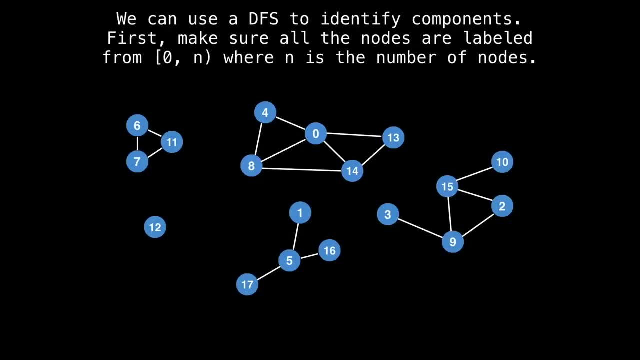 of three. we can use a depth first search to identify components this way: First, make sure all the nodes are labeled from zero to n, non inclusive, where n is the number of nodes. The basic algorithm is to start a depth first search at every node, except if that node 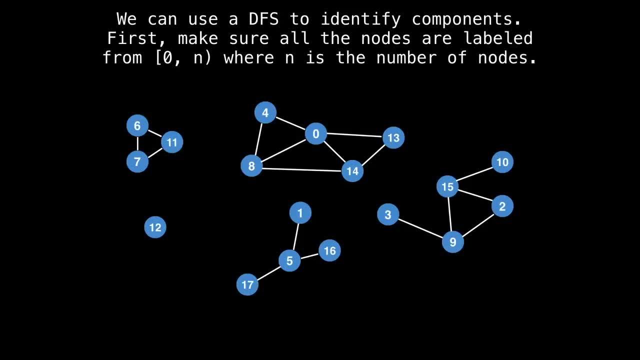 has already been visited and mark all reachable nodes as being part of the same component using the same ID. So if we start at node zero, then we do a depth first search here And then every node in this component gets an ID of zero. So go to eight given an ID. 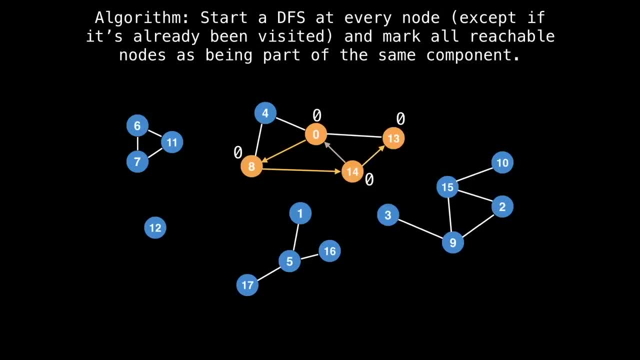 of 014 gets 013.. Also label it with a zero, then backtrack like you do a depth first search, then explore node four, give it an ID of zero and then finish exploring that component and then move on. So we would go on to the next node in order. So go to node one next, then node one, sorry. 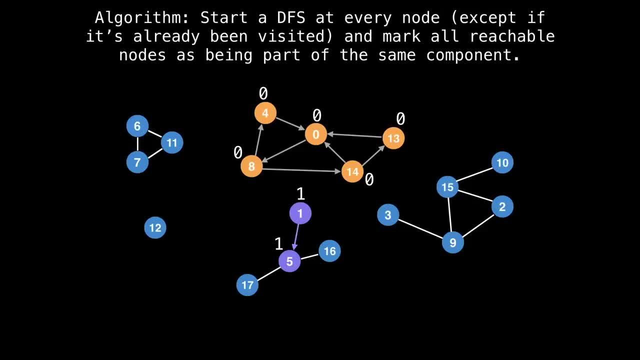 depth. first search there. So go node five. label it with a 15. goes to 17. label it with a one. backtrack, go to 16.. Also label it with a one. we're finished exploring this component. then we would go on to node two, wherever node two is, then explore that component. 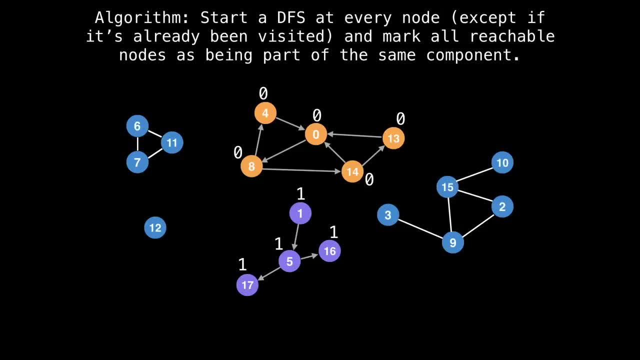 then node three, explore node three's component. Okay, Okay, unless node three has already been visited, and so on. So you do this for every component and eventually we get to label all the components And we use a depth first search to do that. 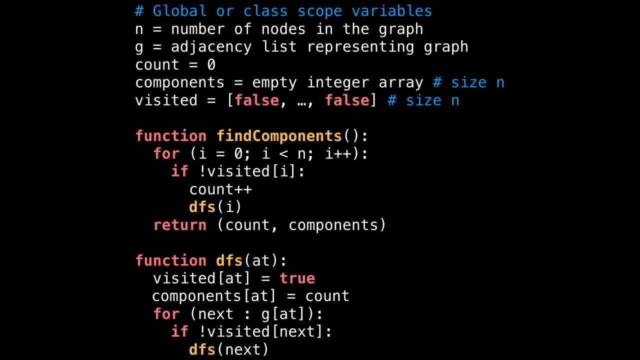 Awesome. So that's how we find connected components using a depth first search. Now let's look at some pseudocode for how we do this. First, we'll need a couple of things. We'll need everything from the previous code. we looked at So n, the number of nodes in our graph. 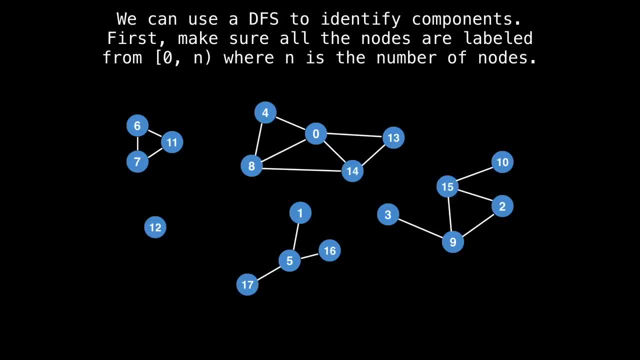 The basic algorithm is to start a depth first search at every node, except if that node has already been visited, and mark all reachable nodes as being part of the same component using the same ID. So if we start at node zero, then we do a depth first search here. 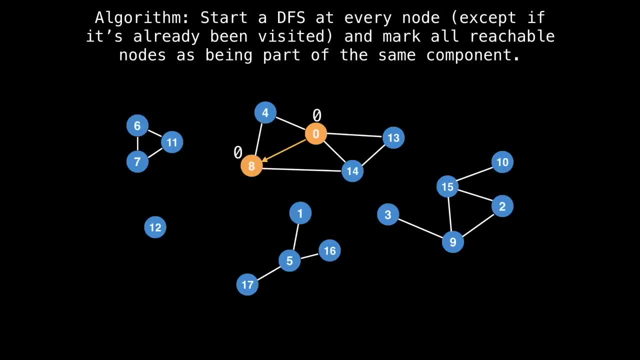 And then every node in this component gets an ID of zero. So go to eight: given an ID of 014, gets 013.. Also label it with a zero, then backtrack like you do a depth first search, then explore node four, give it an ID of zero and then finish exploring that component. and 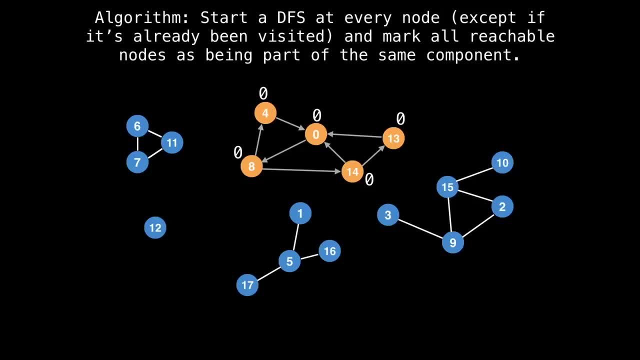 then move on To the next node in order. so go to node one. next then node one. sorry, depth, first search there. So go to node five. label it with a one. Five goes to 17,. label it with a one- backtrack, go to 16.. Also label it with a one, We're. finished exploring this component, then we would go on to Node Two, wherever node two is, then explore that component, then node three, explore node three, its component on base. le셨 Ос жив. It is still okay, in case we go on the bottom, on the bottom, on the. 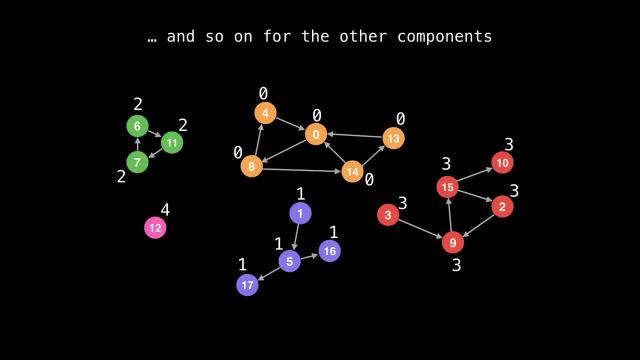 unless node three has already been visited, and so on. So you do this for every component and eventually we get to label all the components And we use a depth first search to do that. Awesome, So that's how we find connected components using a depth first search. Now let's look. 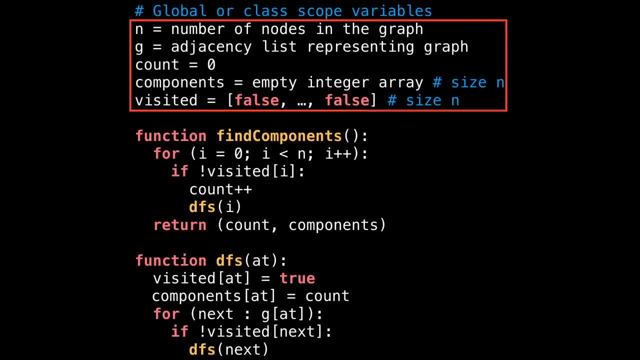 at some pseudocode for how we do this. First, we'll need a couple of things. We'll need everything from the previous code we looked at, So n, the number of nodes in our graph g, our adjacency list and our visited array. But additionally we'll also need a variable. 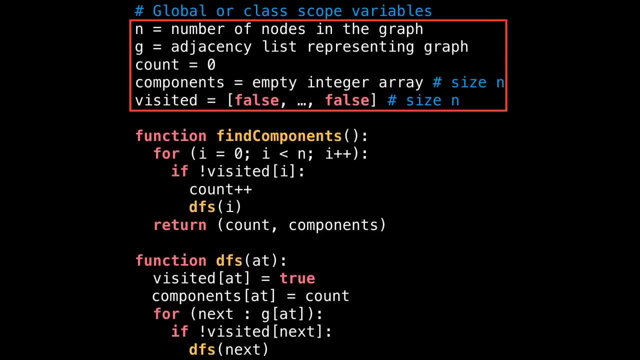 called count, that tracks the number of connected components and components. an integer array that holds the integer value of which component a node belongs to. Inside the find components method, we loop over every node and check if the current node has been visited or not, and then execute some logic. 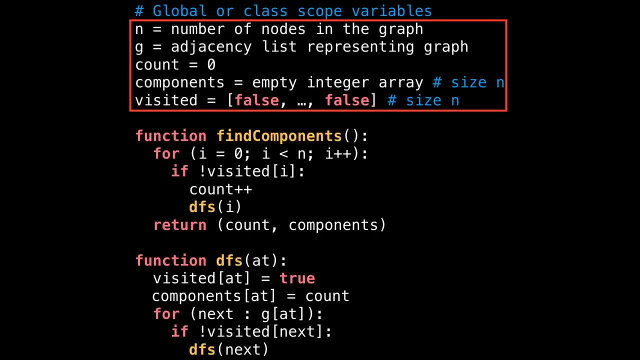 g, our adjacency list and our visited array. But additionally we'll also need a variable called count that tracks the number of connected components and components, an integer array that holds the integer value of which component a node belongs to. Inside the find components method, we loop over every node and check if the current node has been visited or not. 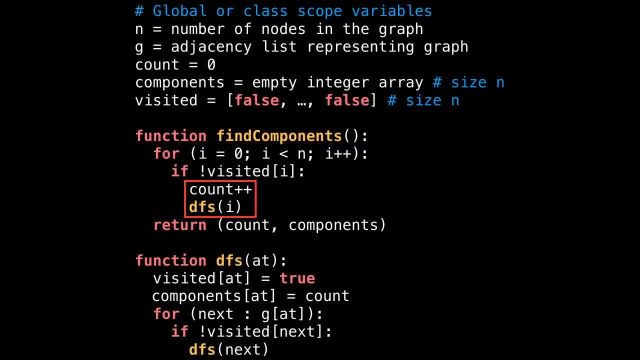 and then execute some logic. This depth first search will then give us a list of all the components that we need to find. So let's go ahead and do that. So let's go ahead and do. the depth first search Variant differs slightly from the previous in that we execute a depth first search for 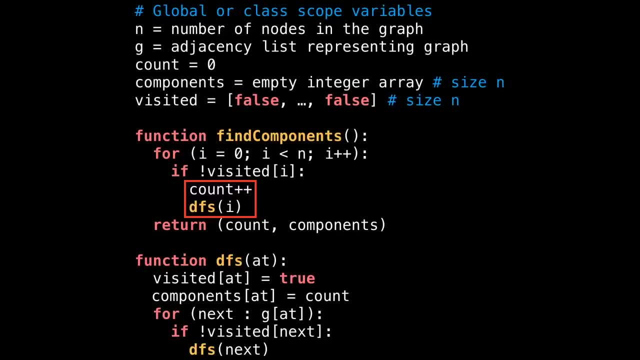 every unvisited node. when we actually do the depth first search, we visit nodes and mark them as visited, So we never revisit the same node more than once. we either skip over a node because it's been visited in this for loop or start a depth first search there. 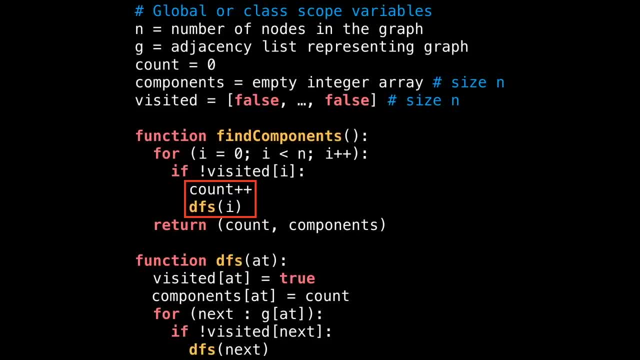 If we start a new depth first search, we increment the count variable to zero And then we can also increment the count variable and keep track of how many depth first searches we have done Inside the depth first search method itself. the two things we do are mark the 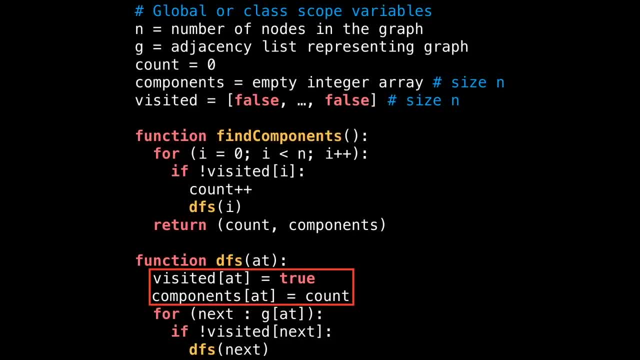 current node as visited and set the current node to be part of the component equal to the value of count. then simply iterate over every neighboring node that has not yet been visited and call the depth first search method to explore them as well Back inside the find. 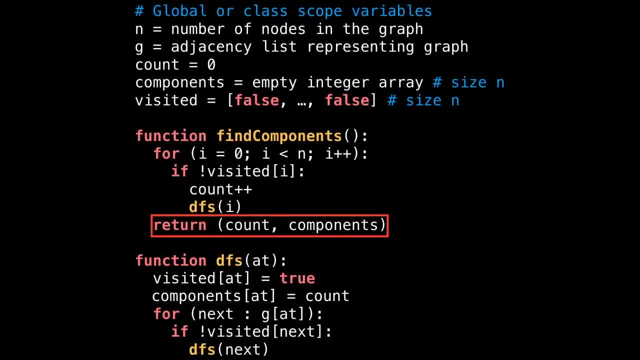 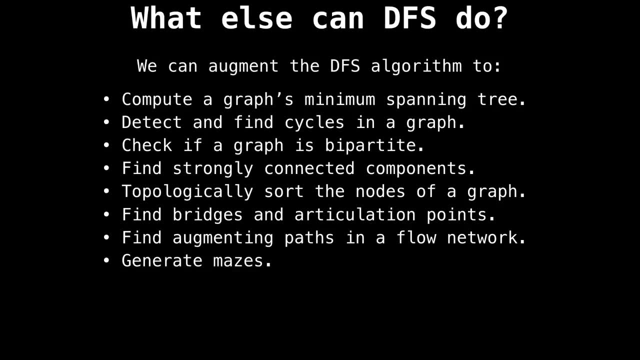 components method simply return the number of components And the components array that contains the information about which component each node belongs to. So we've covered two of the things. you can use a depth first search for doing a simple traversal and determining connected components. But we can augment a depth first. 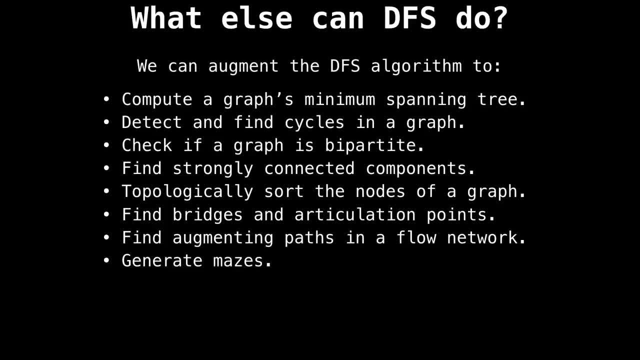 search to do so much more, such as computer graphs, minimum spanning tree detect and find cycles in a graph, check if a graph is bipartite, Find strongly connected components topologically, sort your graph, find bridges and articulation points, find augmenting paths in a flow network, generate mazes and many, many more applications. So 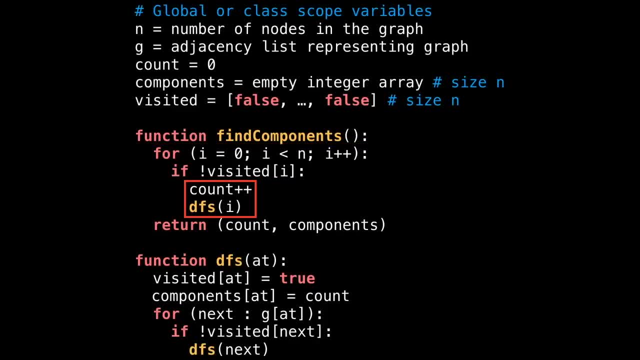 This depth first search will be used to find the component that is connected to the node. The depth first search variant differs slightly from the previous in that we execute a depth first search for every unvisited node. when we actually do the depth first search, we 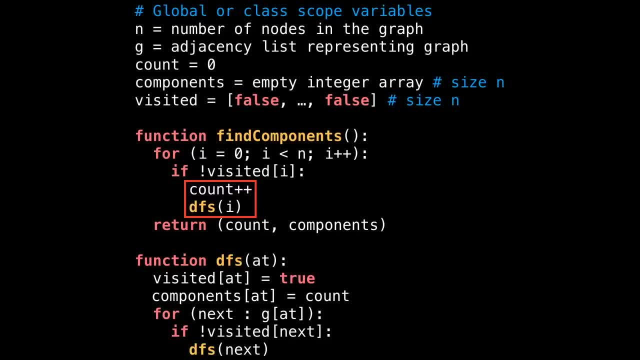 visit nodes and mark them as visited, So we never revisit the same node more than once. we either skip over a node because it's been visited in this for loop or start a depth first search there. If we start a new depth first search, we increment the count variable. 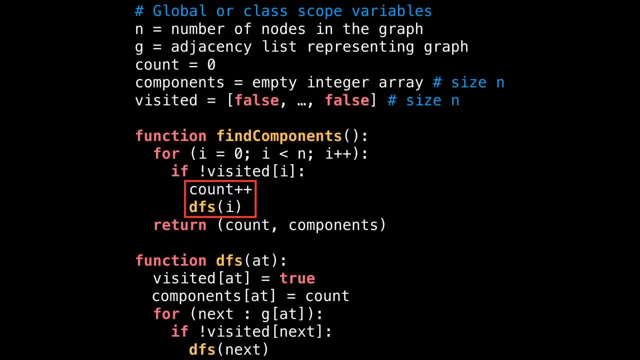 and keep track of how many depth first searches we have done. Inside the depth first search method itself. the two things we do are mark the current node as visited and set the current node to be part of the component equal to the value of count, then simply iterate over. 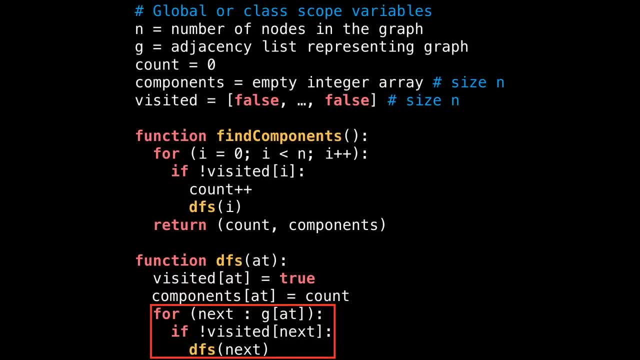 every neighboring node that has not yet been visited and call the depth first search method to explore them as well. Back inside the find components method, simply return the number of components and the components array that contains the information about which component each node belongs to. So we've 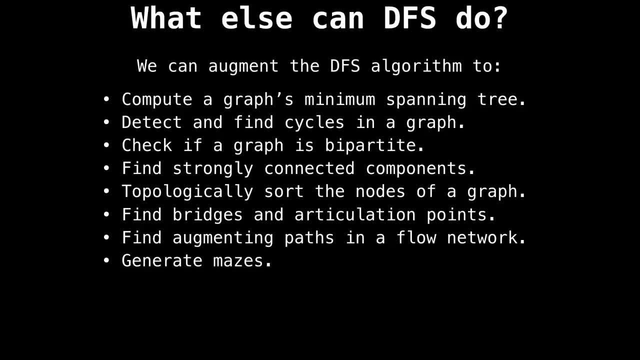 covered two of the things you can use a depth first search for doing a simple traversal and determining connected components. But we can augment a depth first search to do so much more, such as computer graphs, minimum spanning, tree detect and find cycles in a 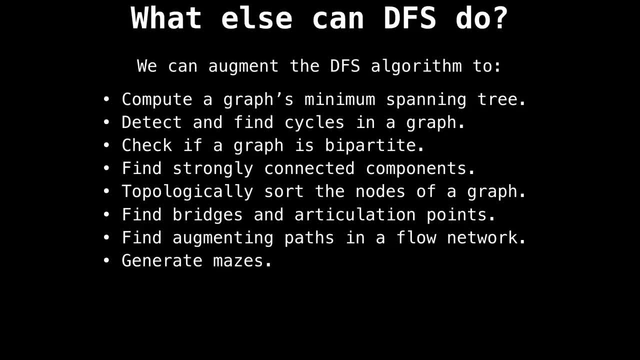 graph. check if a graph is bipartite. Find strongly connected components. topologically. sort your graph. find bridges and articulation points. find augmenting paths in a flow network, generate mazes and many, many more applications. So a depth first search is super versatile and can be extended to do a whole ton of things. 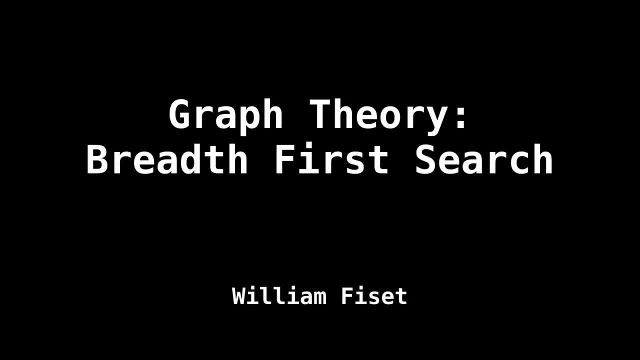 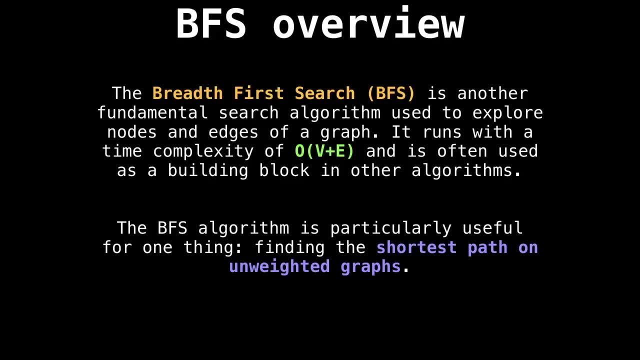 Today's topic is the breadth first search graph traversal algorithm. Alongside the depth first search, the breadth first search algorithm is another one of those fundamental search algorithms used to explore nodes and edges of a graph. It runs in a time complexity of big O of v. 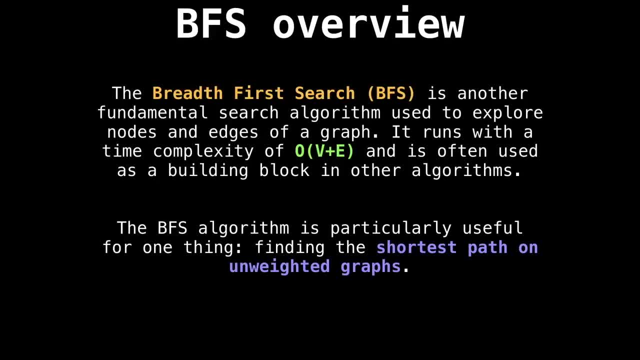 plus e, that is, vertices plus edges, and is often used as a building block in other algorithms. It differs from a depth first search in the way that it explores the graph. The breadth first search algorithm is particularly useful for one thing: finding the shortest path on. 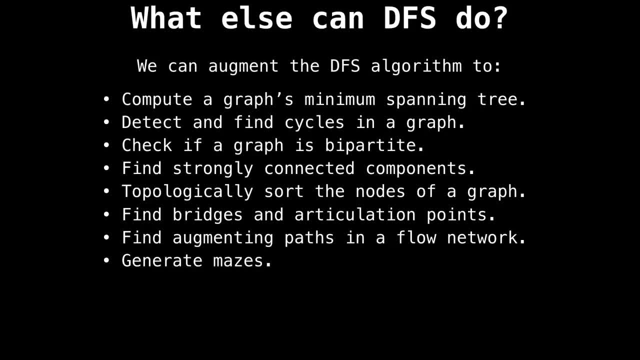 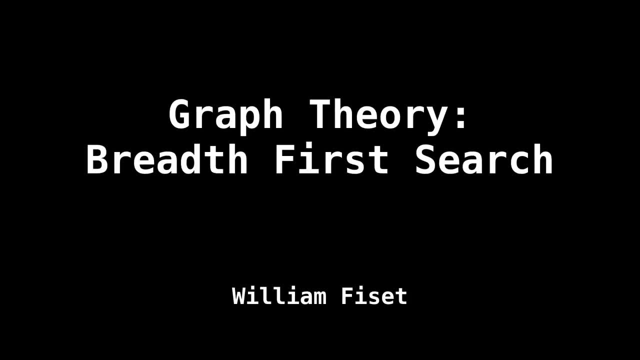 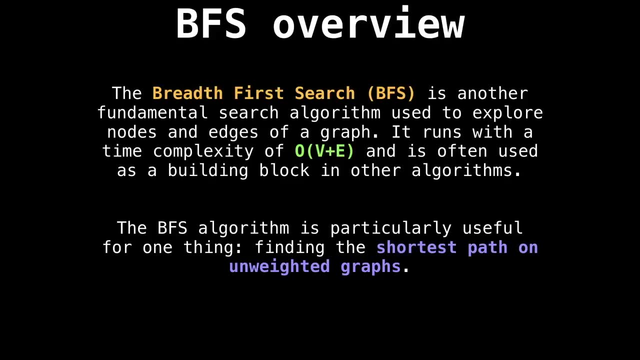 a depth first search is super versatile and can be extended to do a whole ton of things. Today's topic is the breadth first search graph traversal algorithm. Alongside the depth first search, the breadth first search algorithm is another one of those fundamental search. 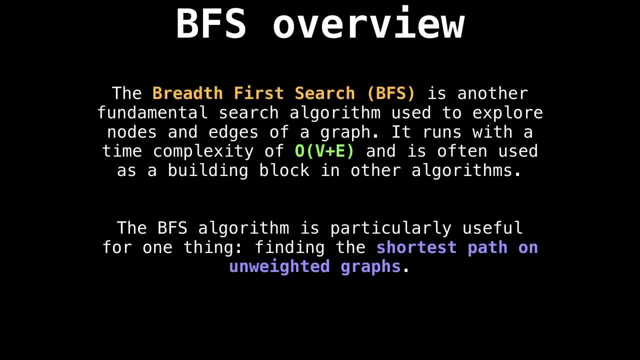 algorithms used to explore nodes and edges of a graph. It runs in a time complexity of big O, of v plus e, that is, vertices plus edges, and is often used as a building block in other algorithms. It differs from a depth first search in the way that it explores the graph, The breadth. 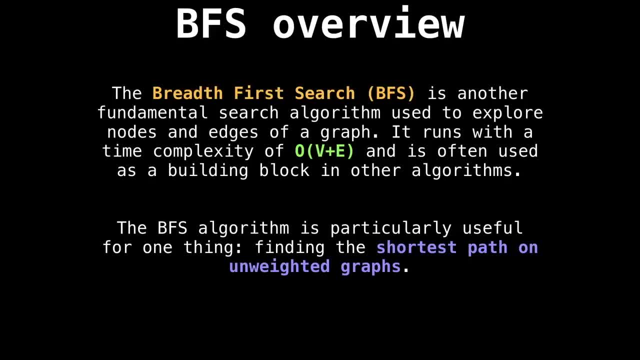 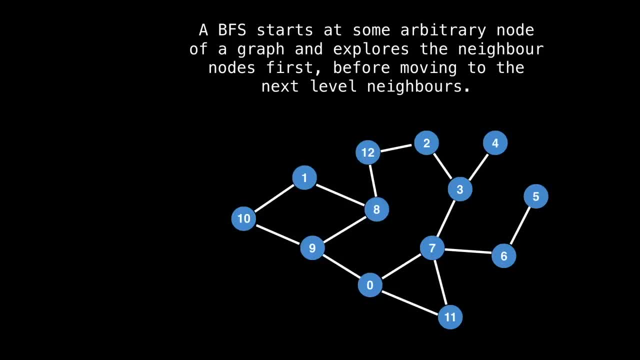 first search algorithm is particularly useful for one thing, finding the shortest path on an unweighted graph. A breadth first search starts at a node in the graph and explores its neighbor nodes first before moving on to explore the next level of neighbors. In a sense, a breadth first search explores nodes. 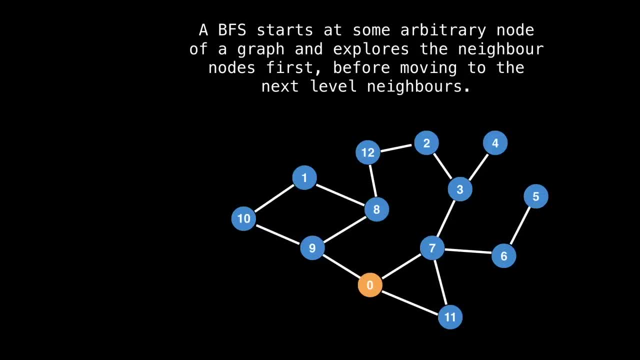 in layers. So if we start a breadth first search at zero, we would visit zero first, then visit all of zeros neighbors. then we would visit all of zeros neighbors- the nodes in yellow, before moving on to the next layer of nodes. then we would visit all their neighbors. 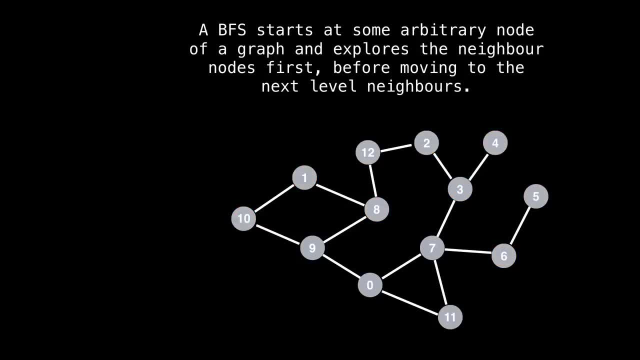 and so on. So, as you saw, a breadth first search explores a graph in a layered fashion. It does this by maintaining a queue of which node it should visit next. This is most easily seen with an example. Let's begin a breadth first search at node zero once more. So let's 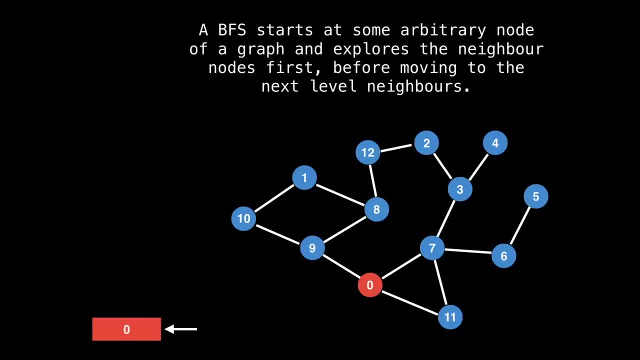 add zero to the queue on the left. I will denote the current node in red. So zero is the current node And we want to explore all of zeros, unvisited neighbors and add them to the queue. So we would add nine to the queue, seven to the queue and 11 to the queue. So zero has no. 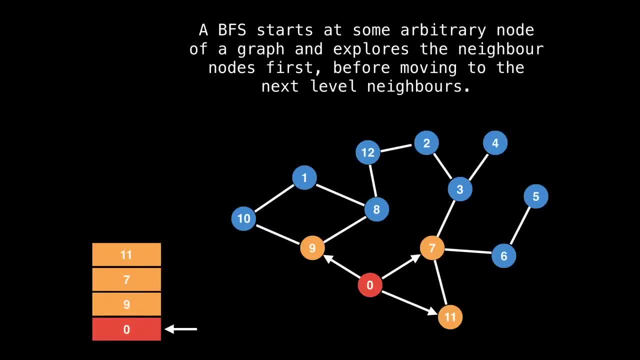 more unvisited neighbors, So we move on. So nine is next up in the queue. So we add all of nines unvisited neighbors to the queue, So that is 10 and eight. then there are no more neighbors of nine to visit, So we move on to the queue. 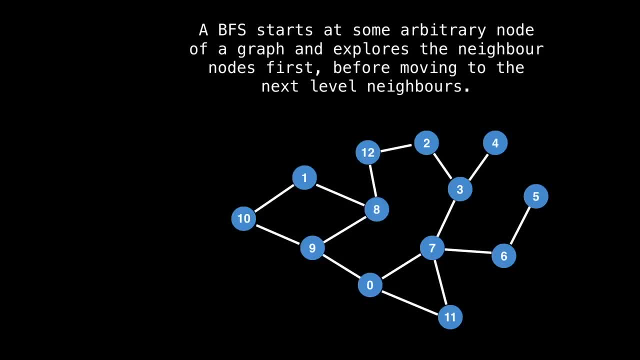 an unweighted graph, a breadth first search. The breadth first search starts at a node in the graph and explores its neighbor nodes first before moving on to explore the next level of neighbors. In a sense, a breadth first search explores nodes in layers. So if we start a breadth first search at zero, 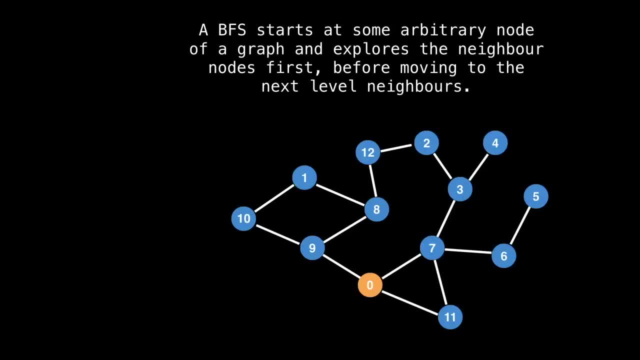 we would visit zero first, then visit all of zeros neighbors, then we would visit all of zeros neighbors- the nodes in yellow before moving on to the next layer of nodes- then we would visit all their neighbors, And so on. So, as you saw, a breadth first search explores a graph in a layered fashion. 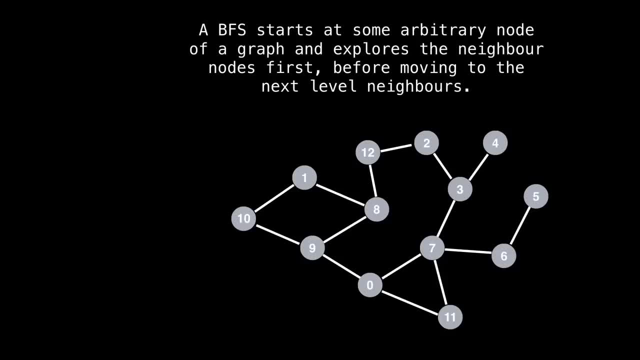 It does this by maintaining a queue of which node it should visit next. This is most easily seen with an example. Let's begin a breadth first. search at node zero once more. So let's add zero to the queue on the left. I will denote the current node in red. So zero is the current. 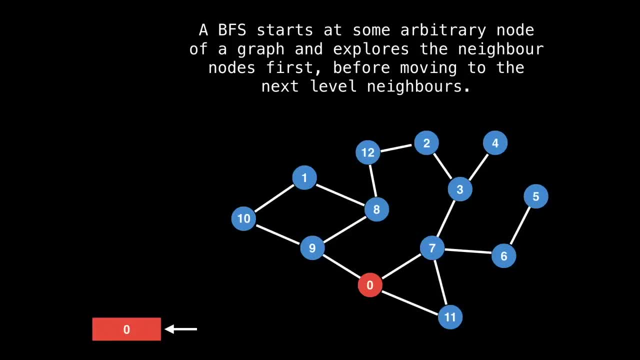 node And we want to explore all of zeros- unvisited neighbors- and add them to the queue. So we would add nine to the queue, seven to the queue and 11 to the queue. So zero has no more unvisited neighbors. So we move on. So nine is next up in the queue, So we add all. 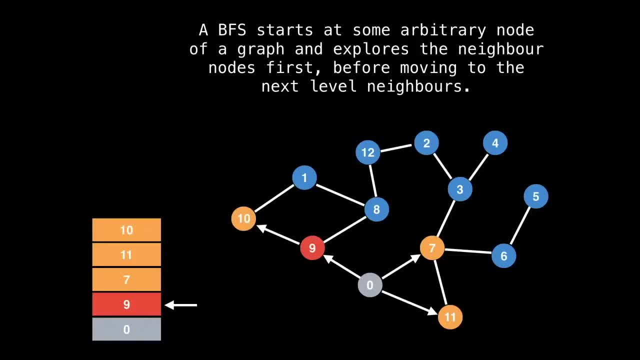 of nine's unvisited neighbors to the queue. So that is 10 and eight. then there are no more neighbors of nine to visit, So we move on to the next Now in our queue, which is seven. then we add all of seven's unvisited neighbors to the queue. 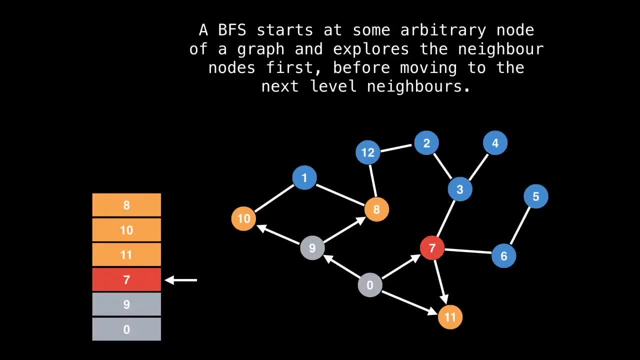 So we try and visit node 11.. But node 11 is already in the queue So we don't want to add it again, So we skip it. then we would add six to the queue and three to the queue, Then this process. 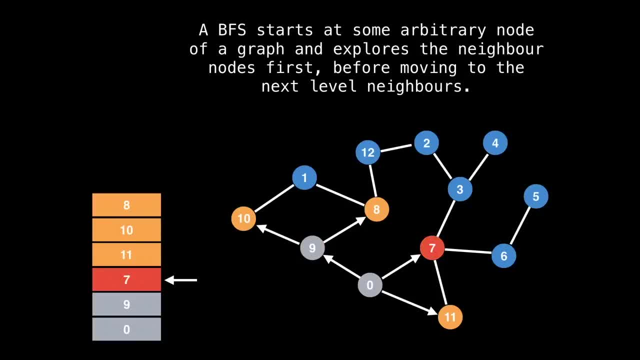 The next node in our queue, which is seven. then we add all of sevens unvisited neighbors to the queue, So we try and visit node 11.. But node 11 is already in the queue So we don't want to add it again, So we skip it. then we would add six to the queue and three. 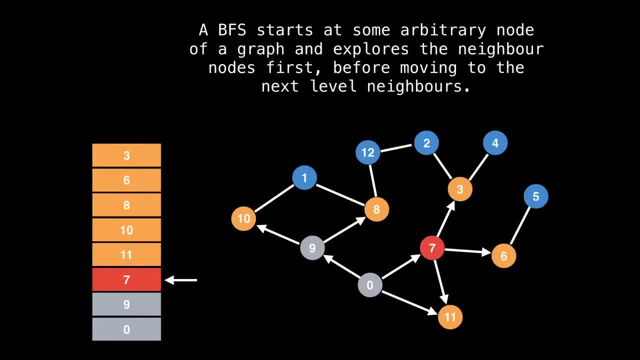 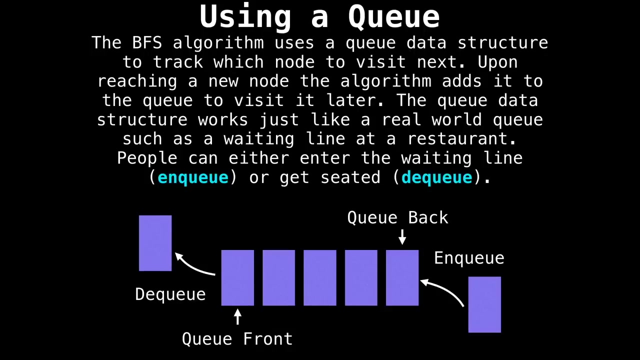 to the queue. Then this process goes on and on until we run out of nodes in the queue. So I will let the animation play. Okay, and that's how you do a breadth first search. in a nutshell, In the previous animation we relied on a queue to help us track which node we should visit next, Upon reaching a. new node. we can now add a new node to the queue. So we can add a new node to the queue And that's how you do a breadth first search. in a nutshell: In the previous animation we relied on a node to help us track which node we should visit next, And that's how. 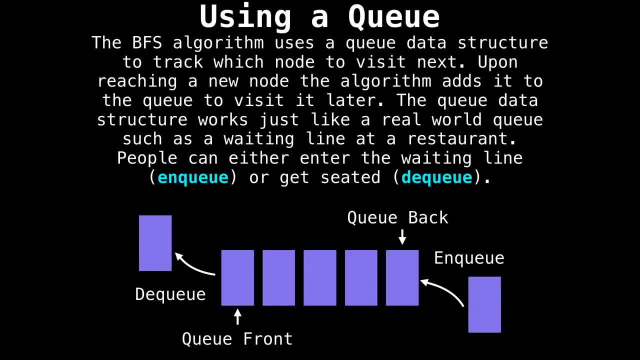 we do a breadth first search, in a nutshell, So we node. the algorithm adds it to the queue to visit it later. the queue data structure works like a real world queue, such as a waiting line in a restaurant. people can either enter. 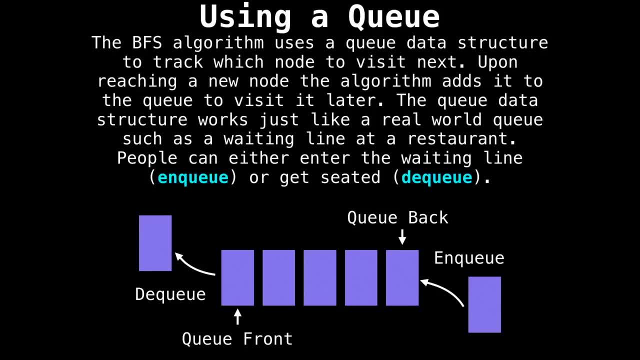 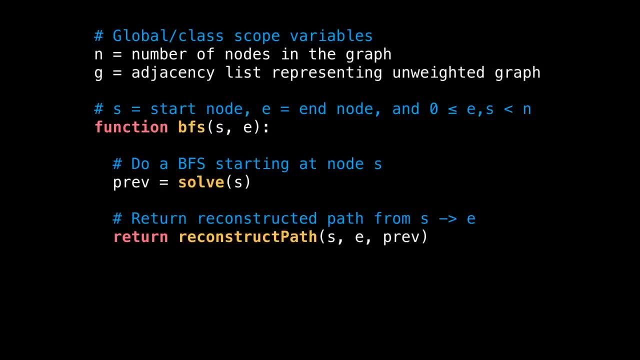 the waiting line, that is, get n queued or get seated d queued. Let's look at some pseudocode for the breadth first search. First things first. we'll need two variables: and the number of nodes in our graph, and G, the adjacency list representing our unweighted graph. This breadth first search. 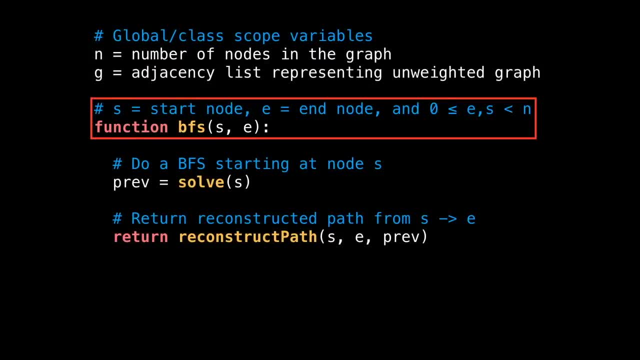 function takes two arguments: s and e, the start and end node indices of the search. The return value for this function is the shortest path of nodes from s to e. I've divided the function into two methods for simplicity. First, we solve the problem by executing the breadth. 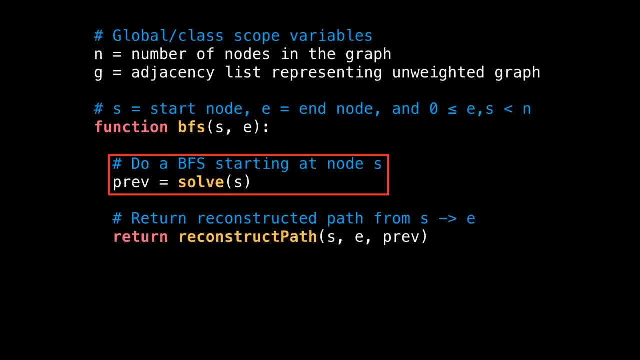 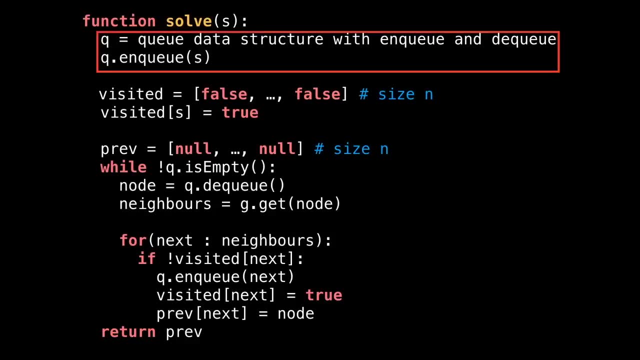 first search and then we reconstruct the path from s to e. So let's take a look at the solve method. So here we are inside the solve method. The first thing I do is initialize the queue data structure that we'll need and add the starting node to it. This queue should: 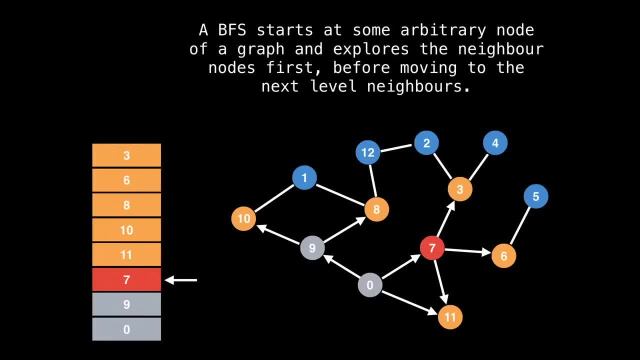 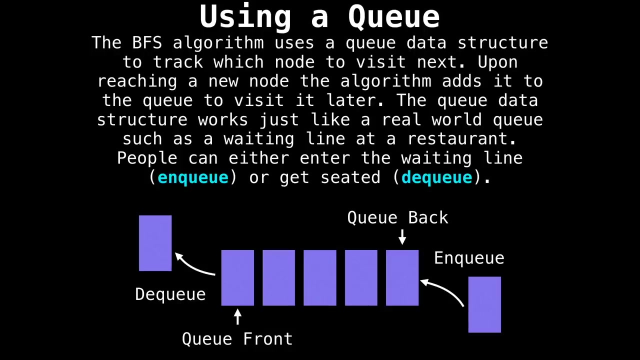 goes on and on until we run out of nodes in the queue. So I will let the animation play. And that's how you do a breadth first search. in a nutshell. In the previous animation we relied on a queue to help us track which node we should visit next, Upon reaching a 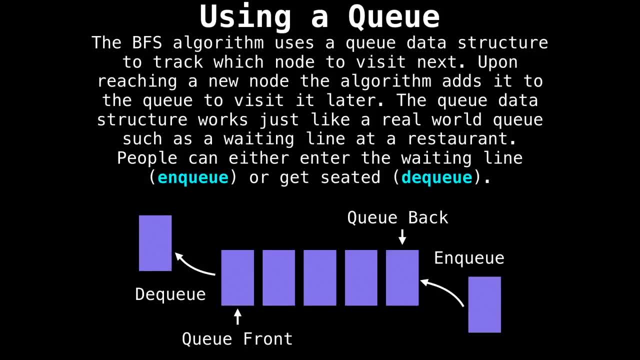 new node. the algorithm adds it to the queue to visit it later. the queue data structure works like a real world queue, such as a waiting line in a restaurant. people can either enter the waiting line- that is, get an queued- or get seated d queued. Let's look at some pseudocode for. 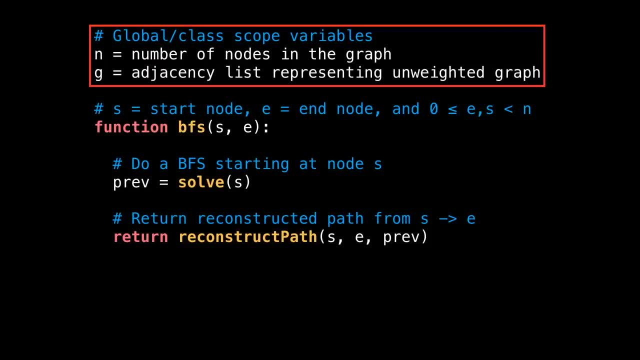 the breadth first search. First things first. we'll need two variables: and the number of nodes in our graph graph, and G, the adjacency list representing our unweighted graph. This breadth first search function takes two arguments: s and e, the start and end node, indices of the search, The return. 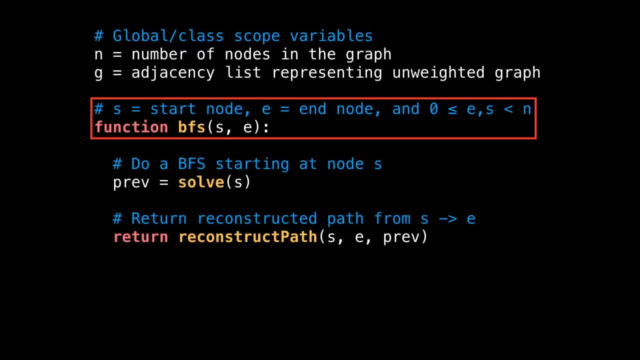 value for this function is the shortest path of nodes from s to e. I've divided the function into two methods for simplicity. First we solve the problem by executing the breadth first search and then we reconstruct the path from s to e. So let's take a look at. 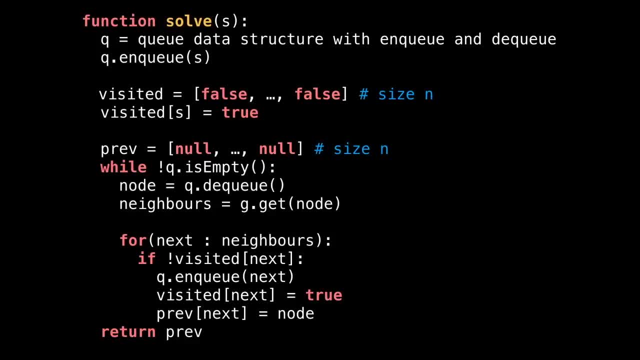 the solve method. So here we are. inside the solve method, The first thing I do is initialize the queue data structure that we'll need and add the starting node to it. This queue should support, at minimum, the NQ and DQ operations I just talked about. 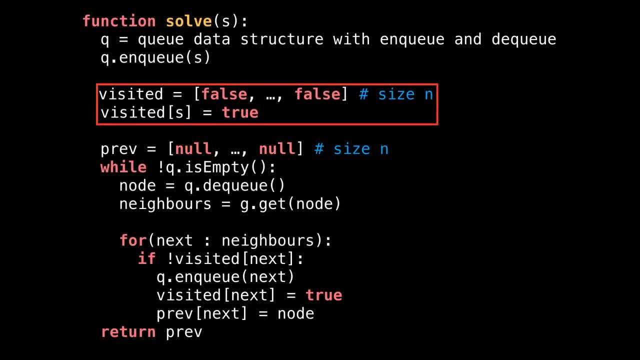 Then initialize a Boolean array with all false values and mark the starting node as visited. This array tracks whether or not node i has been visited. If the value at index i is true, then the node has either been visited or is being visited and is on the queue. And 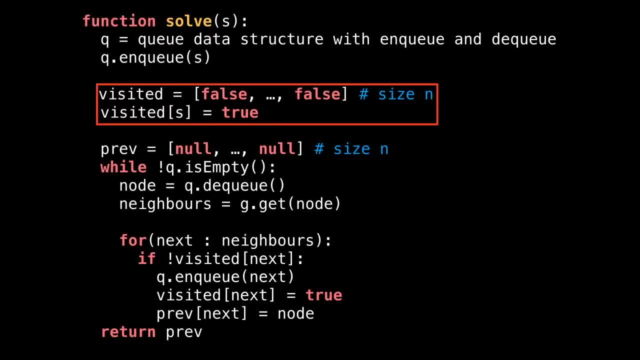 the animation. this corresponds to the gray and yellow nodes. The last thing we'll need is an array of nodes I called Prev, which will help us reconstruct the shortest path from the start to the end node. Initially, this array should be initialized with all null values. This array tracks who. 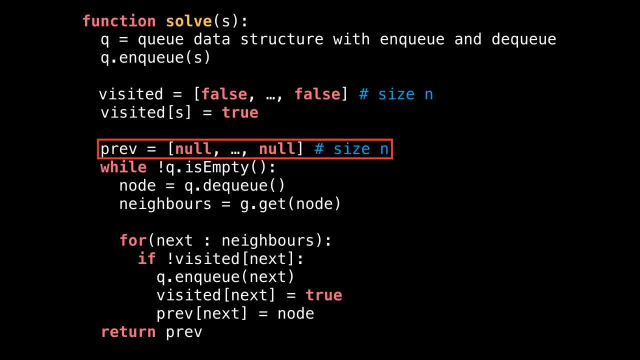 the parent of node i was, so we can reconstruct the path later. Let's loop while the queue is not empty and pull out the top node from the queue by issuing a DQ operation, then reach inside the adjacency list and get all the nodes that we need. 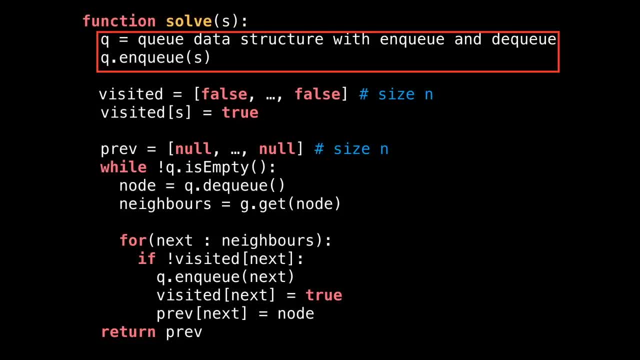 support at minimum the NQ and DQ operations I just talked about. Then initialize a Boolean array with all false values and mark the starting node as visited. This array tracks whether or not node i has been visited If the value at index 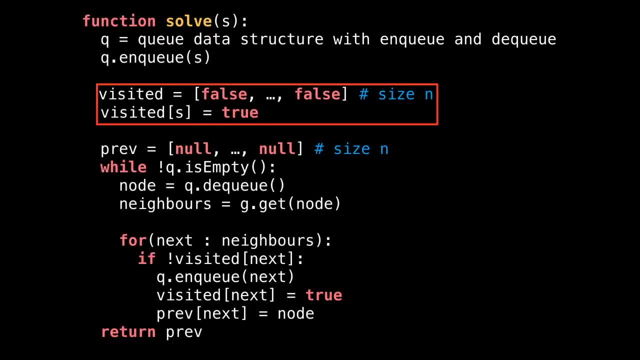 i is true, then the node has either been visited or is being visited and is on the queue And the animation. this corresponds to the gray and yellow nodes. The last thing we'll need is an array of nodes- I called Prev- which will help us reconstruct the shortest path from the start to the end. 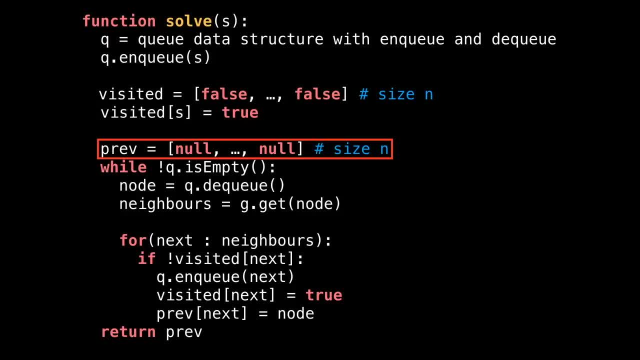 node. Initially, this array should be initialized with all null values. This array tracks who the parent of node i was, so we can reconstruct the path later. Let's loop while the queue is not empty and pull out the top node from the queue by issuing a DQ operation, then reach. 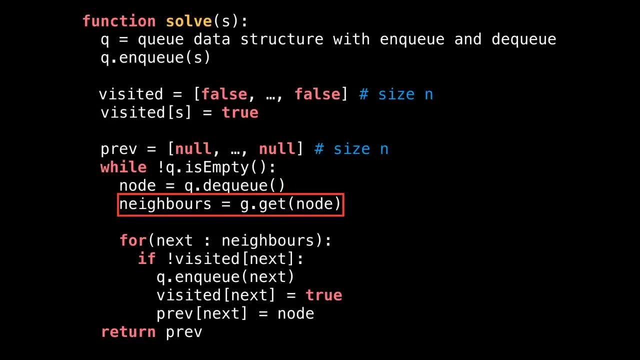 inside the adjacency list and get all the nodes that we need. Once we get all the neighbors of this node loop over each unvisited node. Once we find a next unvisited node and cue it to the queue market as visited and keep track of the parent. 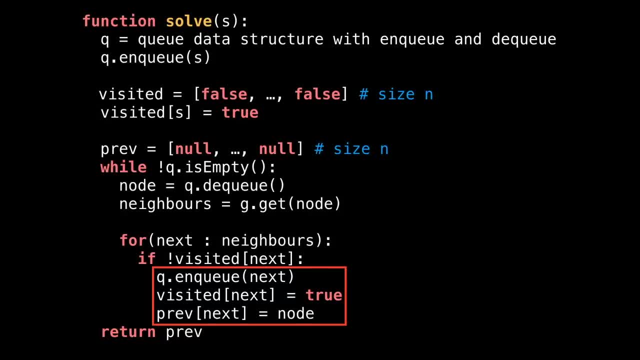 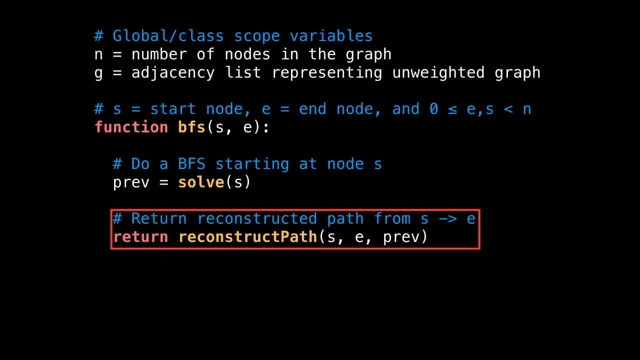 node of the next node in the Prev array. Once the queue is empty and our breadth first search is complete, simply return the Prev array Back inside the breadth first search method. take the output of the solve method And we're going to call it Prev. 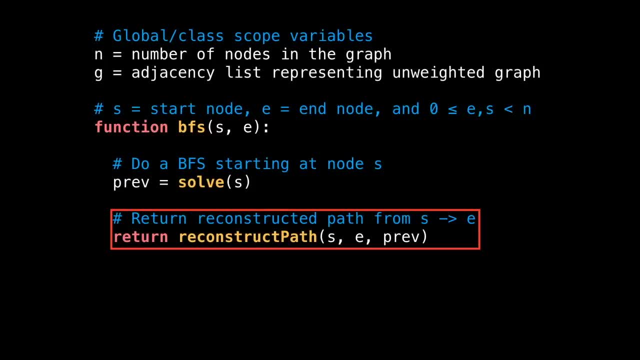 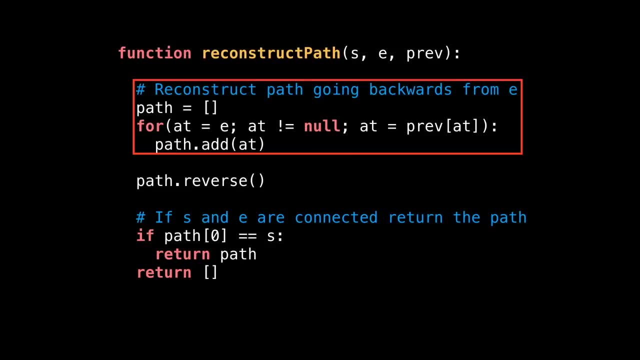 And we're going to call it Prev, And we're going to call it Prev method, which gave us the Prev array, and call the reconstruct path method. Here we are inside the reconstruct path method. The first thing we do is actually reconstruct the path by 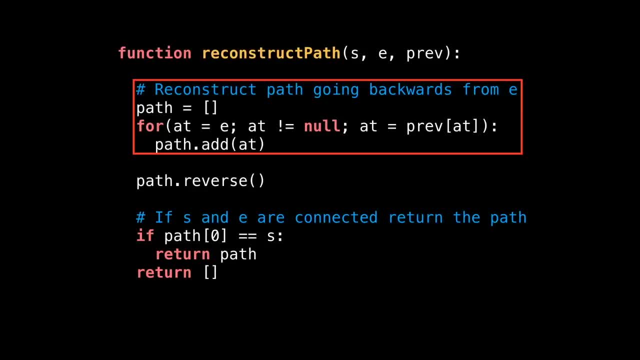 looping backwards from the end node and making our way back to the start node. That is assuming we can reach it. The reason the Prev array had to be initialized to all null values is because that is the way I'm checking whether or not the for loop should stop, Since we loop through the Prev array backwards, starting with the. 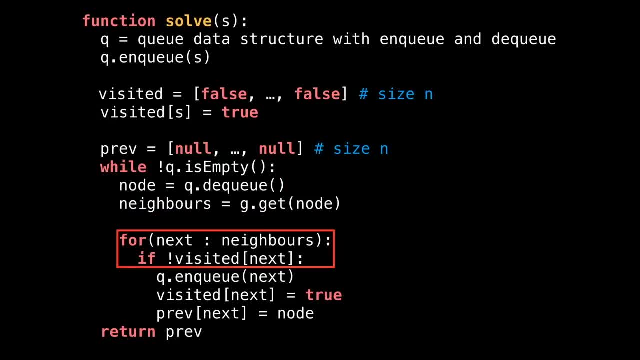 Once we get all the neighbors of this node loop over each unvisited node, Once we find a next unvisited node and cue it to the queue market as visited and keep track of the parent node of the next node in the Prev array Once the queue is empty and our breadth first. 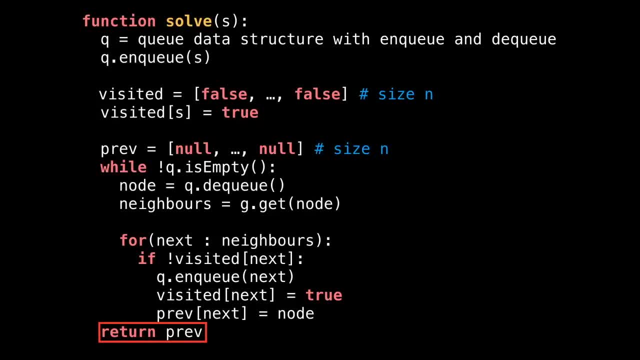 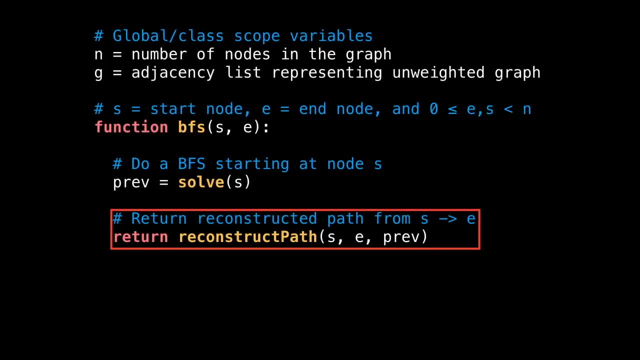 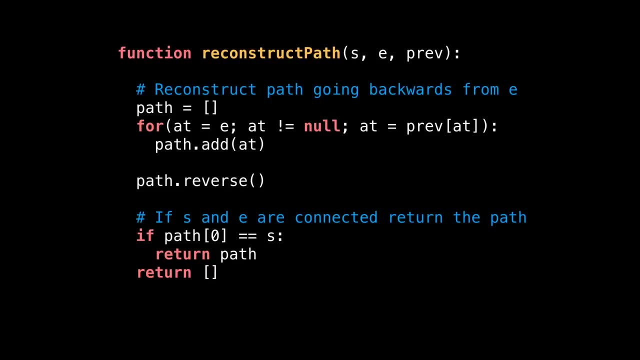 search is complete, simply return the Prev array Back inside the breadth. first search method. take the output of the solve method, Prev method, which gave us the Prev array, and call the reconstruct path method. Here we are inside the reconstruct path method. The first thing we do is actually reconstruct the path by 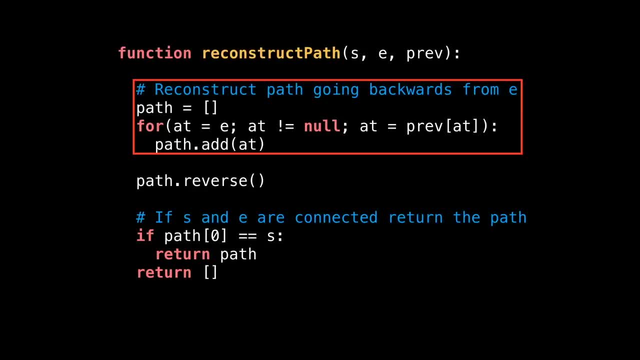 looping backwards from the end node and making our way back to the start node. That is assuming we can reach it. The reason the Prev array had to be initialized to all null values is because that is the way I'm checking whether or not the for loop should stop, Since we loop through the Prev array backwards. 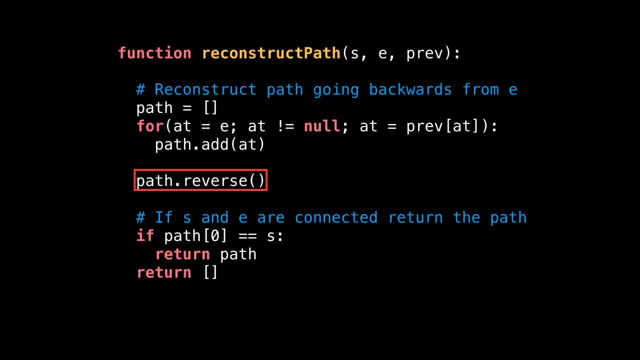 starting with the end node. we need to reverse the order of the nodes so that the path starts at the start node and ends at the end node. Last but not least, we actually have to make sure the path between nodes s and e exists. 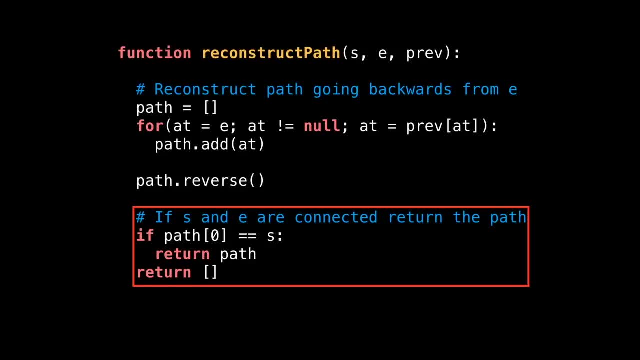 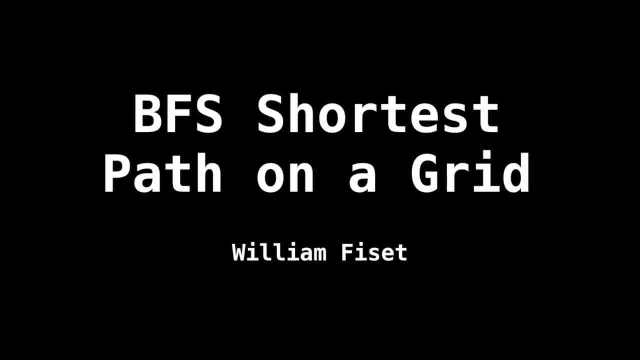 it might not be possible to reach node E from node s If the graph is disjoint. If this is the case, then simply return an empty path. Today we're going to talk about using a breadth first search to find the shortest path on a grid. This is going to be a really fun video. 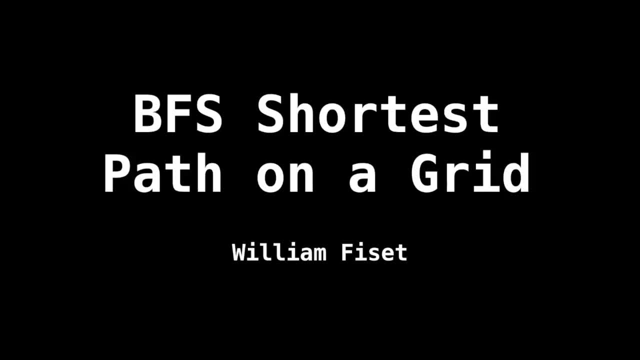 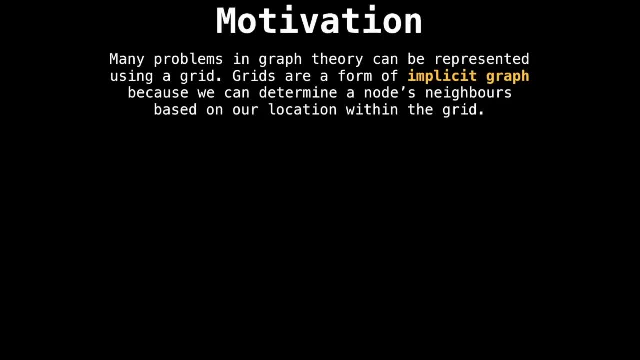 because we're going to solve a problem And I'm going to teach you a bunch of handy tricks when doing graph theory on grids. The motivation behind why we're learning about grids in this video is that a surprising number of problems can easily be represented using a grid which 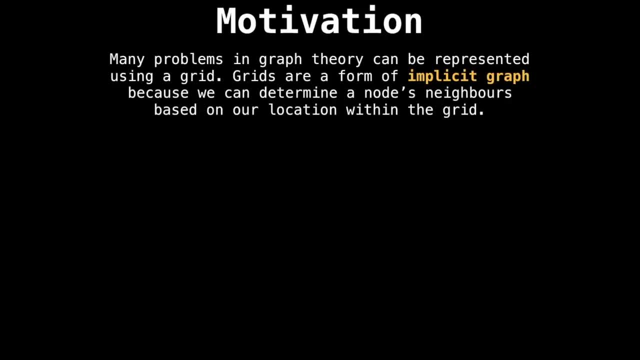 a lot of the times turns into a graph theory problem. Grids are interesting because they're a form of implicit graph, which means that we can determine a node's neighbors based on our location within the grid. For instance, finding a path through a maze is a form of. 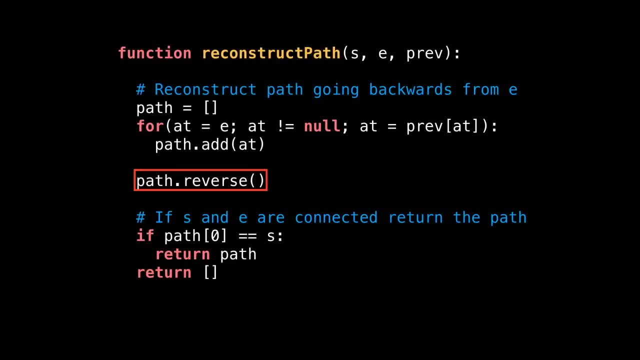 end node. we need to reverse the order of the nodes so that the path starts at the start node and ends at the end node. Last but not least, we actually have to make sure the path between nodes s and E exists. it might not be possible to reach node E from node s if 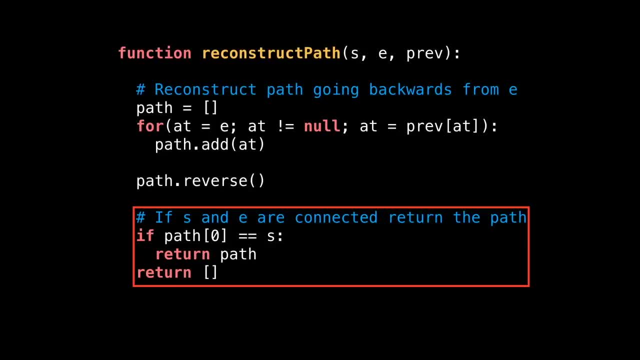 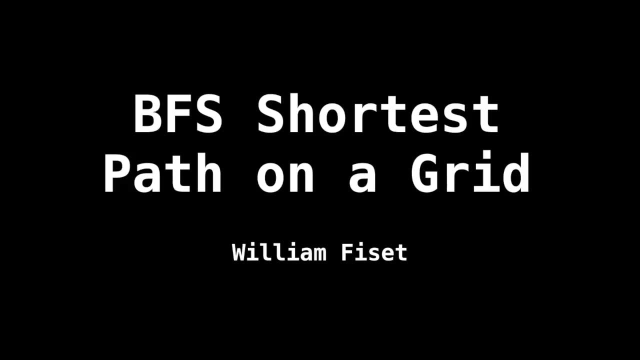 the graph is disjoint. If this is the case, then simply return an empty path. Today, we're going to talk about using a breadth first search to find the shortest path on a grid. This is going to be a really fun video, because we're going to solve a problem And I'm going to teach you a bunch of handy tricks when 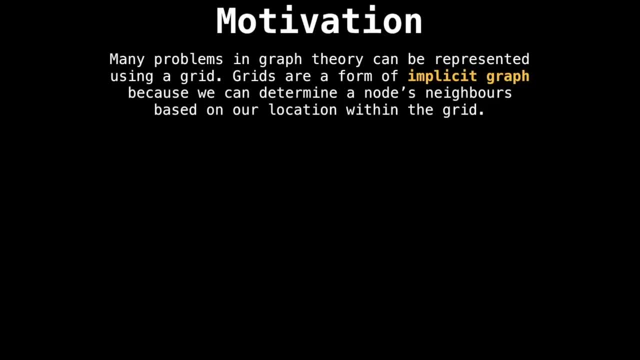 doing graph theory on grids. The motivation behind why we're learning about grids in this video is that a surprising number of problems can easily be represented using a grid, which a lot of the times turns into a graph theory problem. Grids are interesting because they're a form of implicit graph, which means that we can 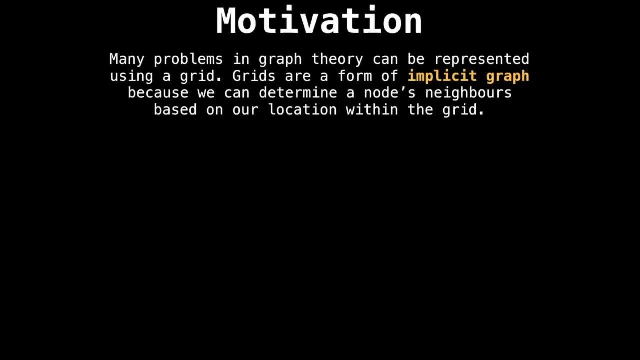 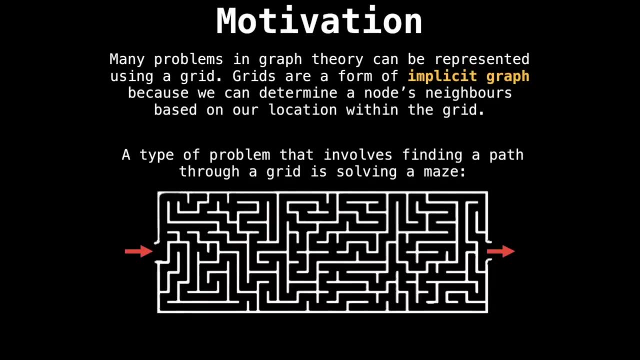 determine a node's neighbors based on our location within the grid. For instance, finding a path through a maze is a form of a grid problem. you're trying to get from one side of the maze through the other. Well, you need to find a path. it's a pathfinding problem. 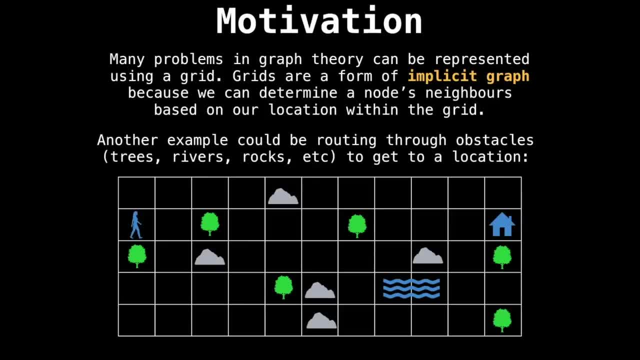 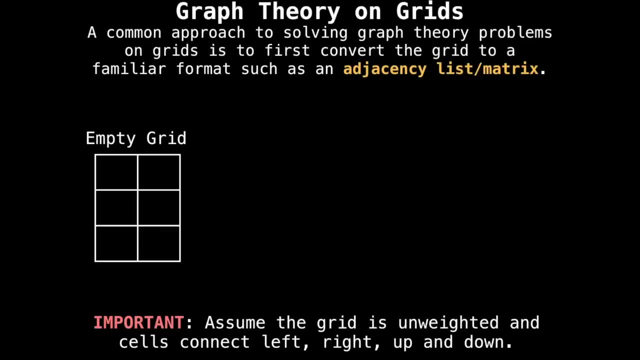 Or perhaps you're a person trying to navigate your way through obstacles such as trees, rivers and rocks to get to a particular location, And this can be modeled using a grid And in turn, we end up using graph theory to navigate around. A common approach to solving graph theory problems on grids is to first convert. 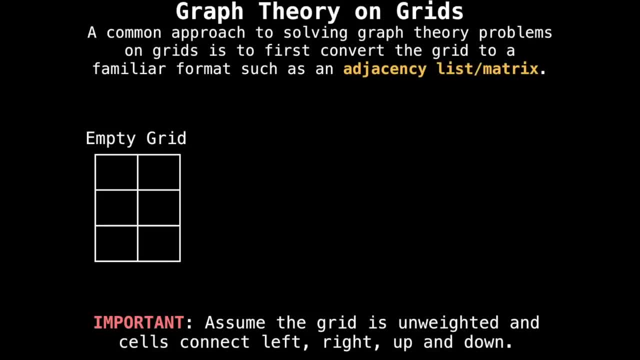 the grid to a familiar format such as an adjacency list or an adjacency matrix, so we can easily work with them. However, this isn't always the most efficient technique, but we'll get to that. Suppose we have a grid on the left and we want to represent it as both in the 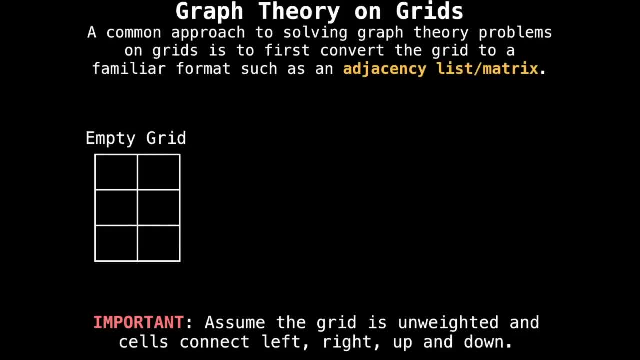 adjacency list and an adjacency matrix. What do we do first? first, you should label all the cells in the grid with the numbers zero through n, non inclusive, where n is the product of the number of rows and columns. So in this grid on the left there are six cells. So 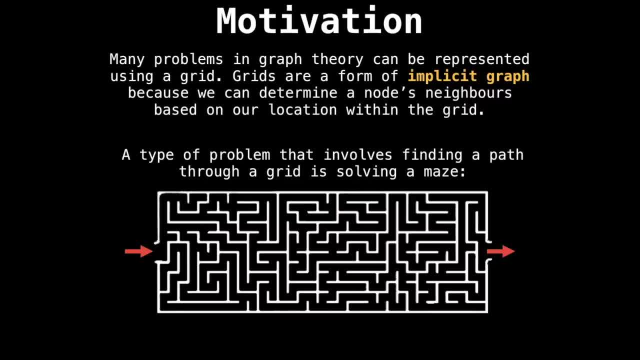 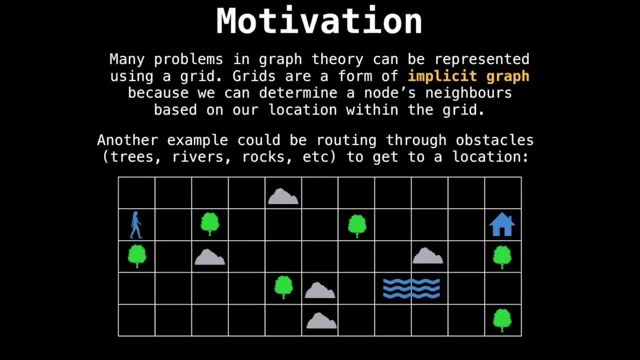 a grid problem. you're trying to get from one side of the maze through the other. Well, you need to find a path. it's a pathfinding problem. Or perhaps you're a person trying to navigate your way through obstacles Such as trees, rivers and rocks to get to a particular location, And this can be modeled. 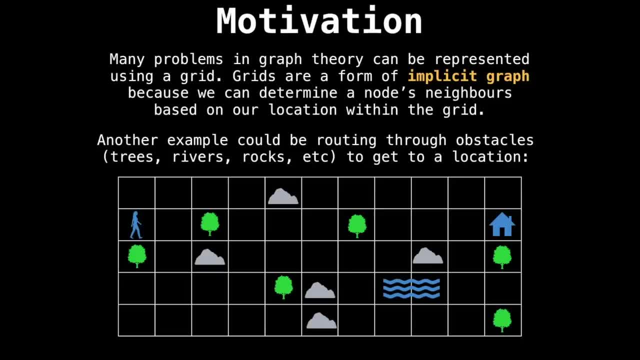 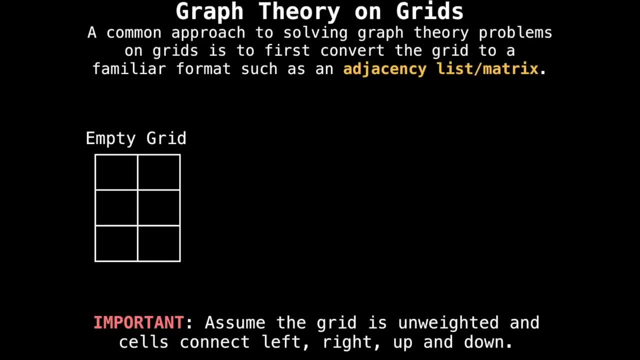 using a grid And in turn we end up using graph theory to navigate around. A common approach to solving graph theory problems on grids is to first convert the grid to a familiar format, such as an adjacency list or an adjacency matrix, so we can easily work. 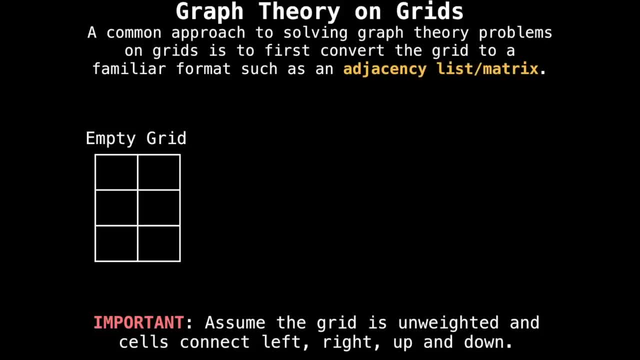 with them. However, this isn't always the most efficient technique, but we'll get to that. Suppose we have a grid on the left and we want to represent it as both an adjacency list and an adjacency matrix. What do we do first? first, you should label all the cells in the grid with the numbers. 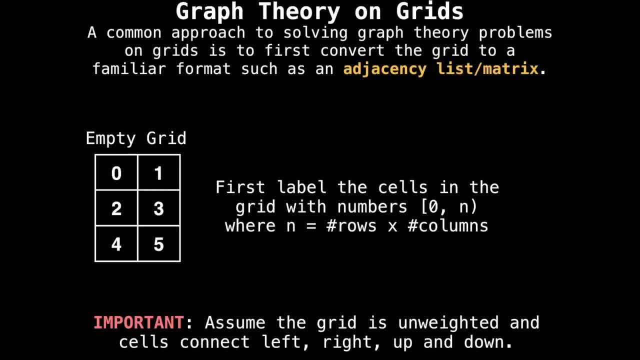 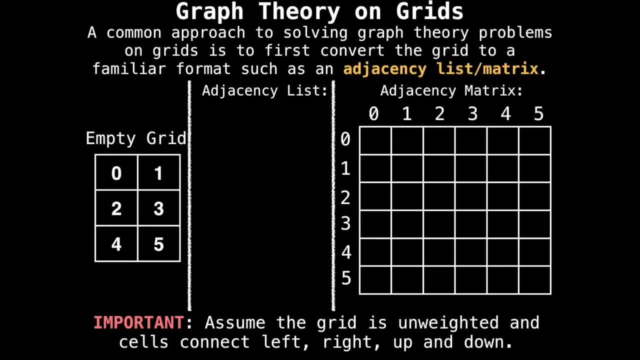 zero through n- non inclusive, where n is the product of the number of rows and columns. So in this grid on the left there are six cells, So I labeled each cell with the numbers zero through six non inclusive. Then we actually want to construct an adjacency list and an adjacency matrix based off this. 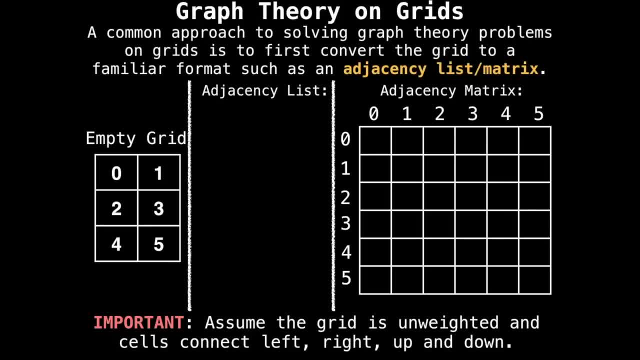 grid. the adjacency list doesn't require any setup because it's simply a map that we initialize, But the adjacency matrix requires us to initialize a matrix of size six by six to represent our graph. there are six rows and six columns in the new adjacency matrix because it's 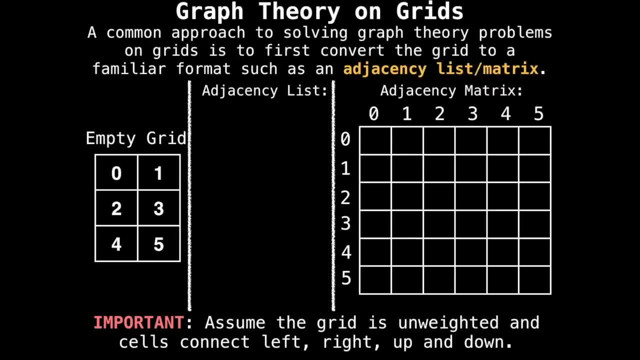 how many nodes there are in the grid we're trying to represent, Assuming edges are unweighted and cells connect left, right, up and down. node zero connects with node one and node two, which we reflect in the adjacency list and adjacency matrix on the right, then node 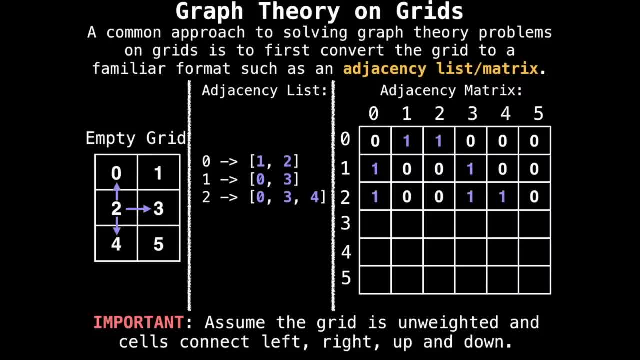 one connects to node zero and node three, node two to nodes zero, three and four, node three with nodes one, two and five and so on, And that's basically how you convert a grid to an adjacency list or an adjacency matrix. 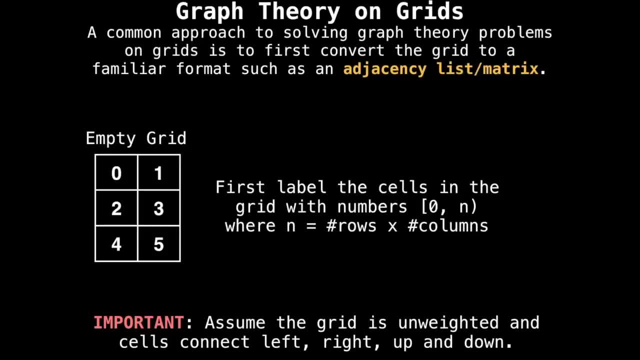 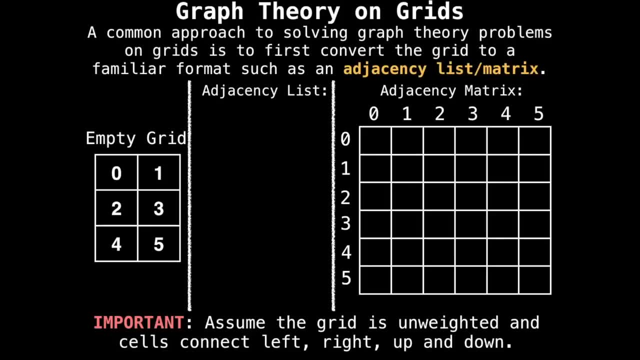 I labeled each cell with the numbers zero through six, non inclusive. then we actually want to construct an adjacency list and an adjacency matrix Based off this grid. the adjacency list doesn't require any setup because it's simply a map that we initialize, But the adjacency matrix requires us to initialize a matrix of size. 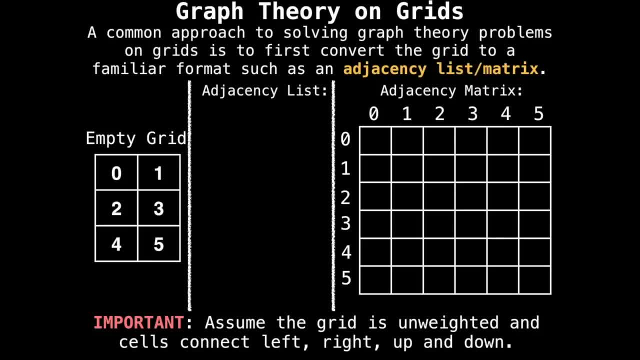 six by six to represent our graph. there are six rows and six columns in the new adjacency matrix because it's how many nodes there are in the grid we're trying to represent, Assuming edges are unweighted and cells connected left, right, up and down. node zero connects. 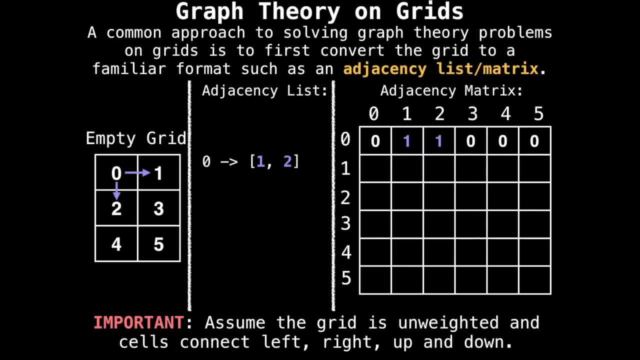 with node one and node two, which we reflect in the adjacency list and adjacency matrix on the right. then node one connects to node zero and node three, node two to nodes zero, three and four, node three with nodes one, two and five and so on, And that's basically. 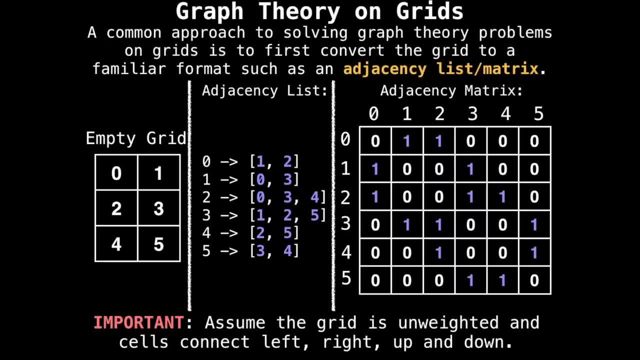 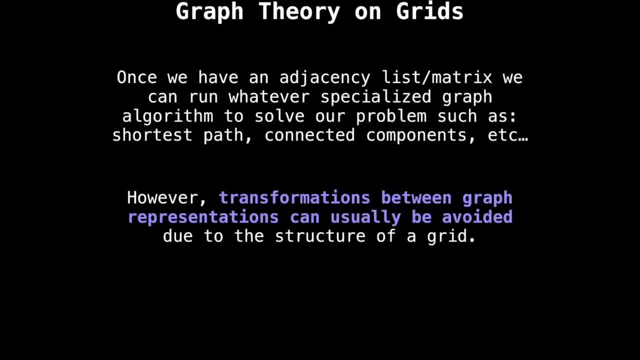 how you convert a grid to an adjacency matrix. Now let's talk a little bit about what we call an adjacency list or an adjacency matrix. Once we have an adjacency list or an adjacency matrix, we are able to easily run whatever specialized graph algorithm we need to solve our problems, such as finding the shortest. 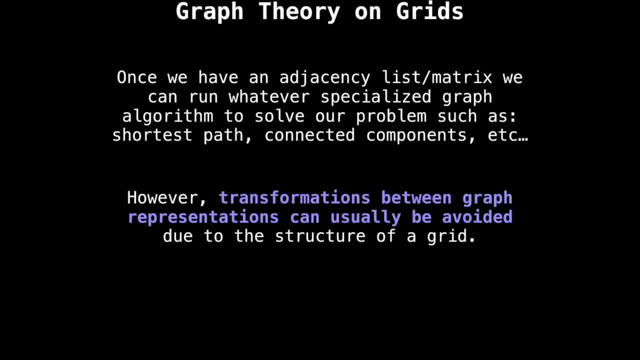 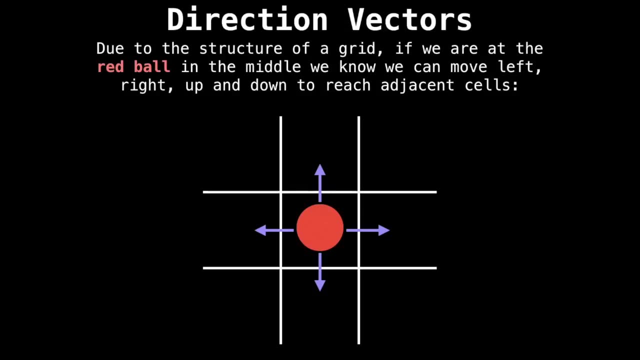 path, finding connected components, etc. However, transformations between graph representations can usually be avoided due to the structure and the nature of a grid. Let me explain. Suppose we're the red ball in the middle And we know we can move left, right, up and down to reach adjacent cells. Well, mathematically, 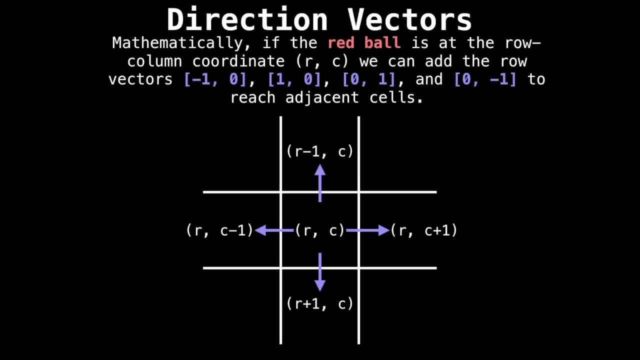 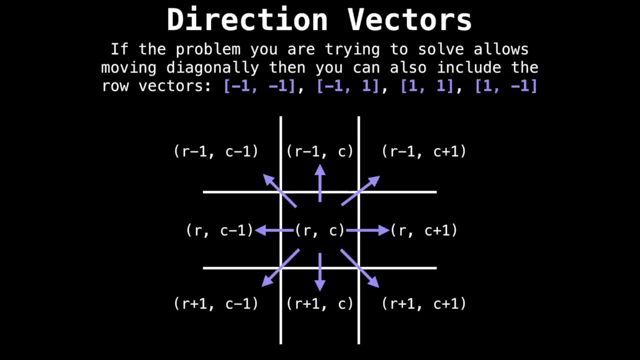 if we're the red ball at the row column coordinate r comma c, we can add the row vectors minus one, zero one comma zero, zero comma one and zero comma minus one to reach all the adjacent cells. If the problem you're trying to solve allows moving diagonally, then you: 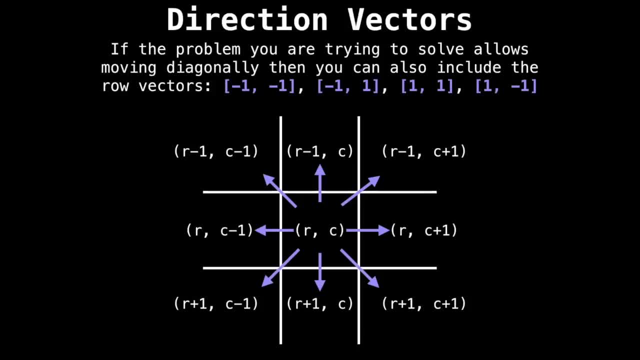 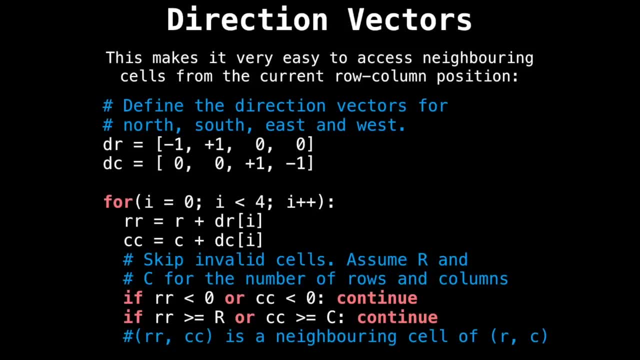 can also use the row vectors minus one minus one, minus 1111 and one minus one. Using row vectors makes it easy to access neighboring cells from the current row column position. First, define the direction vectors for north, south, east and west, broken down into their 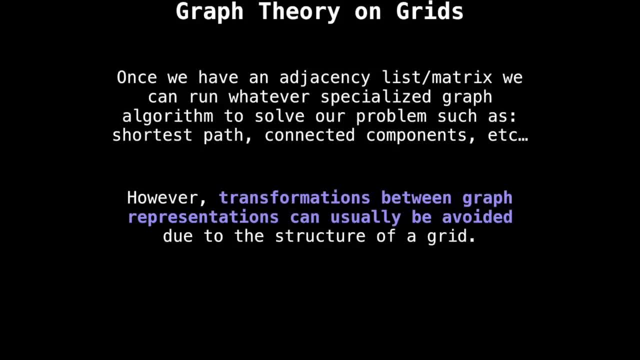 Once we have an adjacency list or an adjacency matrix, we are able to easily run whatever specialized graph algorithm we need to solve our problems, such as finding the shortest path, finding connected components, etc. However, transformations between graph representations can usually be avoided due to the structure and the nature of a grid. 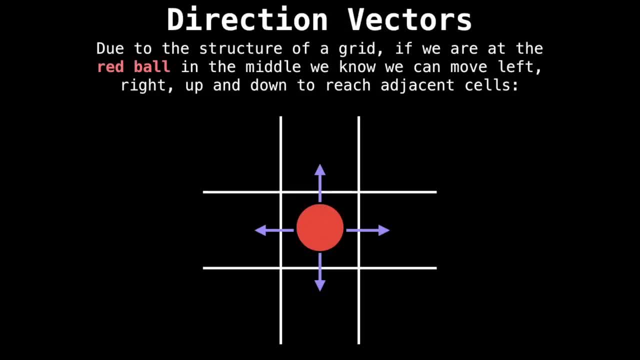 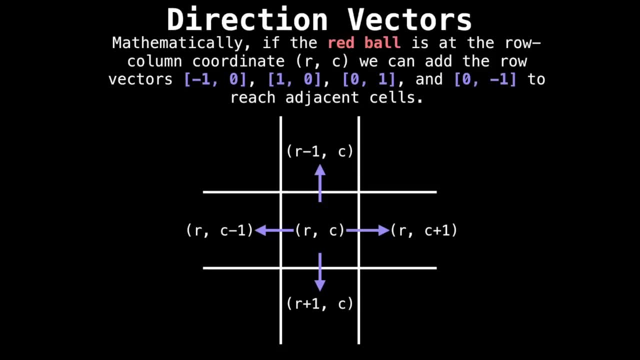 Let me explain. Suppose we're the red ball in the middle and we know we can move left, right, up and down to reach adjacent cells. Well, mathematically, if we're the red ball at the row, column, coordinate r, comma C, we can add the row vectors minus one, zero one. 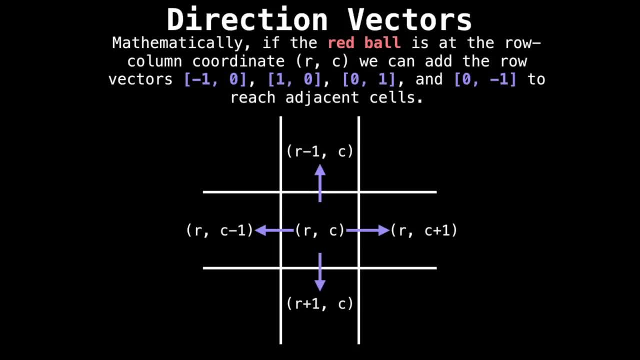 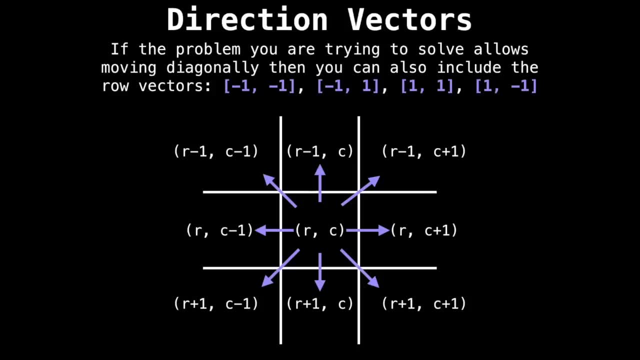 comma zero, zero comma one and zero comma minus one to reach all the adjacent cells. If the problem you're trying to solve allows moving diagonally, then you can also use the row vectors minus one minus one. minus 1111 and one minus one Using row vectors. 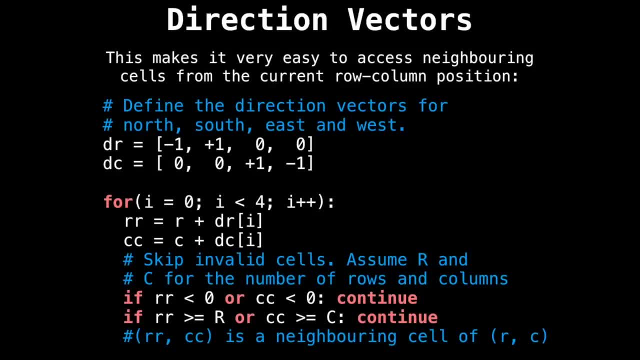 makes it easy to access neighboring cells from the current row column position. First, define the direction vectors for north, south, east and west, broken down into their row column components. Then what we want to do is loop over each direction vector and add it to the current position. here I iterate, I from. 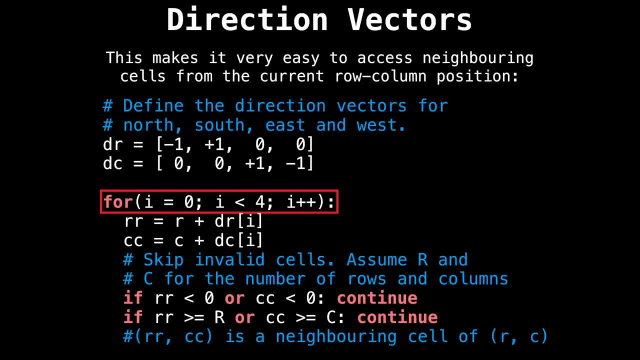 zero to four, non inclusive, because we only have four directions. then add the row direction to the current row to make our the variable representing the new row. and then add the column direction to the current column to make CC the new column position, So the new. 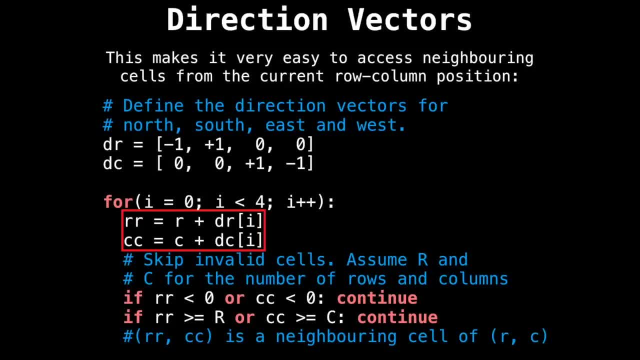 position on the grid. our comma CC is an adjacent cell. However, it might not be an adjacent cell if we're on the border of the grid and the new position is out of bounds. So we check that the new coordinate is within our grid. 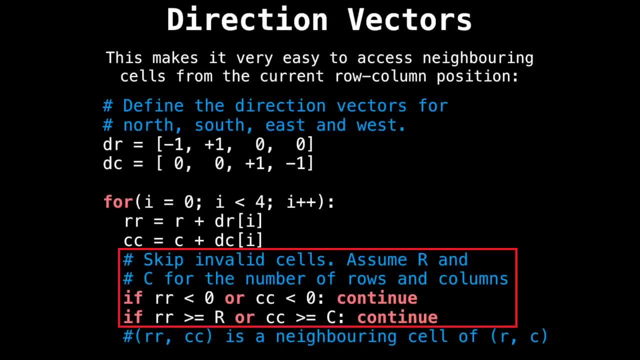 by making sure that the new row column position is greater than or equal to zero and doesn't exceed the number of rows and columns of our grid respectively. So if those two checks pass, then we know that the new position r, r comma CC is the. 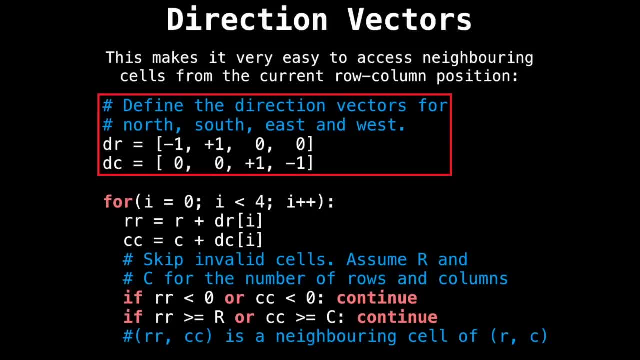 row column components, Then what we want to do is loop over each direction vector and add it to the current position. Here I iterate I from zero to four, non inclusive, because we only have four directions. then add the row direction to the current row to make our the variable representing the new. 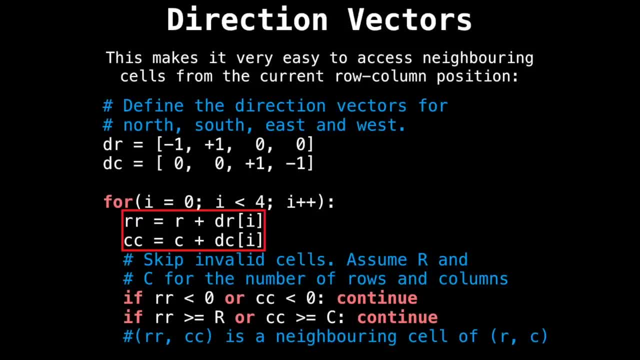 row and then add the column direction to the current column to make CC the new column position. So the new position on the grid, our comma CC, is an adjacent cell. However, it might not be an adjacent cell If we're on the border of the grid and the new position is out of bounds. So we check. 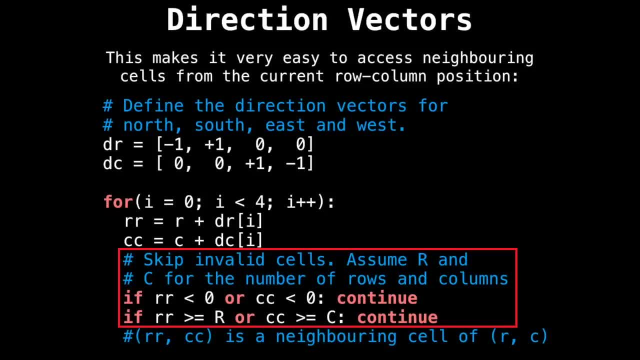 that the new coordinate is within our grid by making sure that the new row column position is greater than or equal to zero and doesn't exceed the number of rows and columns of our grid respectively. So if those two checks pass, then we know that the new position 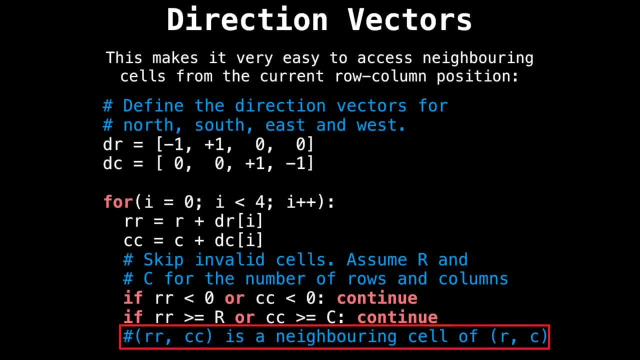 are r comma CC is a neighboring cell of our current position, where the red line is, the red ball was r comma C. So in summary, this technique is really nice, really easy to code and actually naturally extends to higher dimensions. So let's solve a shortest path. 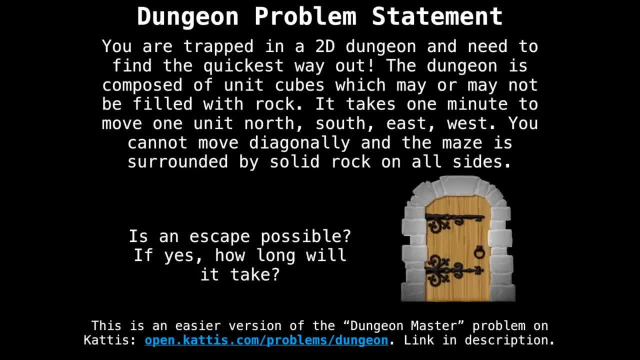 problem on a grid using the direct should vector technique we just learned about. So here's an abridged problem statement that you might encounter during an interview or in a programming competition, And it goes as follows: Suppose you're trapped inside a 2d dungeon and need 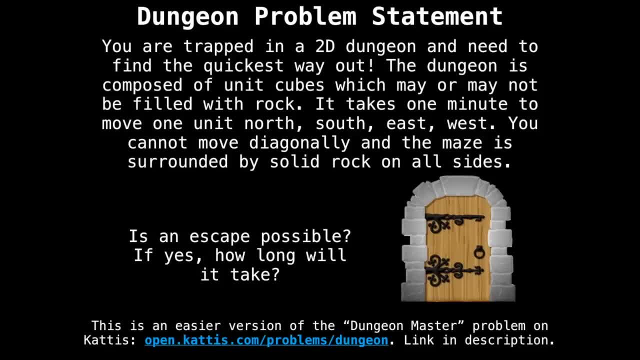 to find the quickest way out. The dungeon is composed of unit cubes which may or may not be filled with a rock. it takes one minute to move one unit north, south, east or west. you cannot move diagonally and the maze is surrounded by solid rock on all sides. This 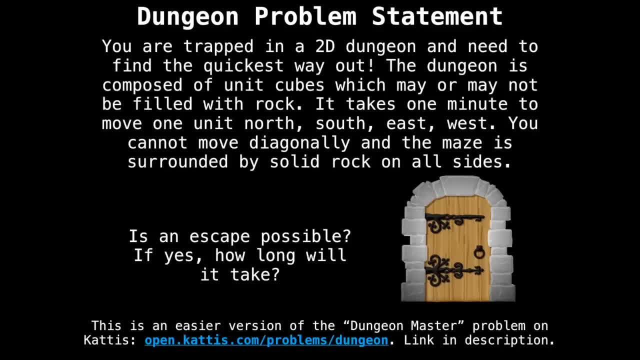 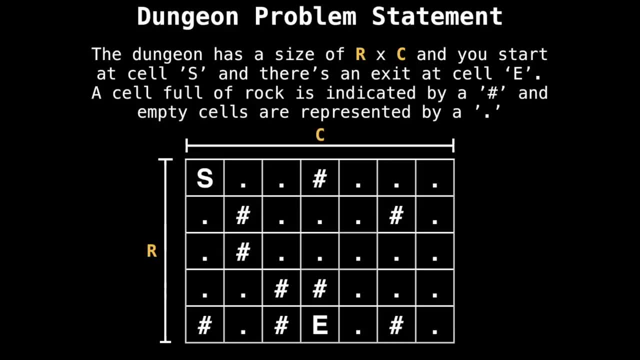 problem statement is an easier version of the problem: dungeon master on the caddis online judge: See the problem link in the description. The dungeon is a grid of size are by C and you start at the node with an s character and there's an exit at the cell with an E. 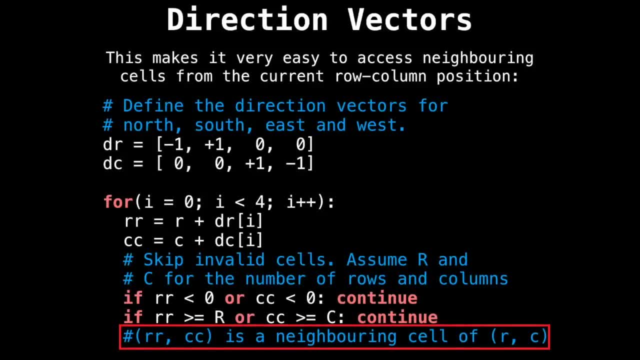 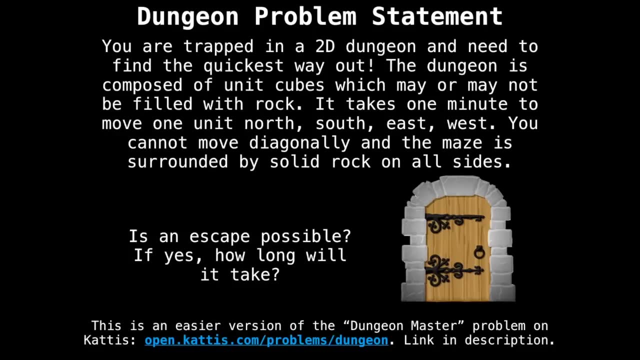 is a neighboring cell of our current position where the red ball was r comma C. So, in summary, this technique is really nice, really easy to code and actually naturally extends to higher dimensions. So let's solve a shortest path problem on a grid using the direction: 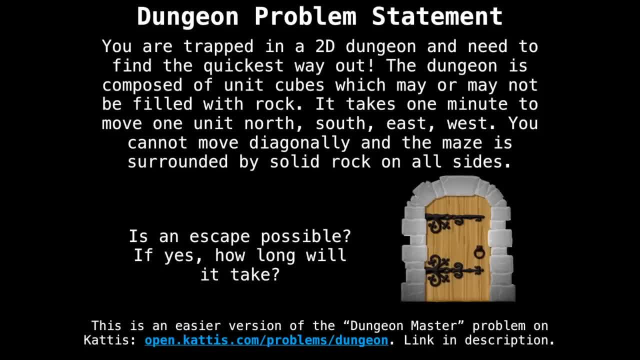 vector technique we just learned about. So here's an abridged problem statement that you might encounter during an interview or in a programming competition, And it goes as follows: Suppose you're trapped inside a 2d dungeon and need to find the quickest way out. The dungeon is composed of unit cubes which may or may not be filled with a rock. 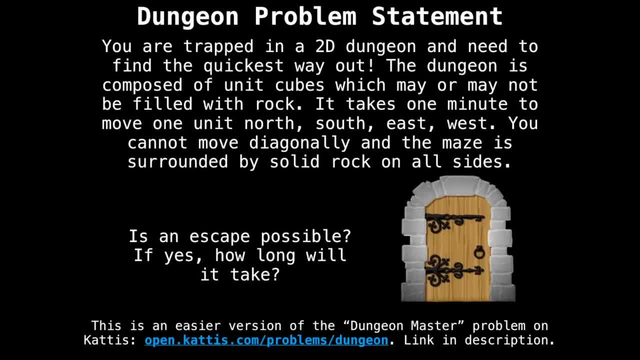 It takes one minute to move one unit north, south, east or west. You cannot move diagonally and the maze is surrounded by solid rock on all sides. This problem statement is an easier version of the problem statement. So here's an example of a problem statement. So you 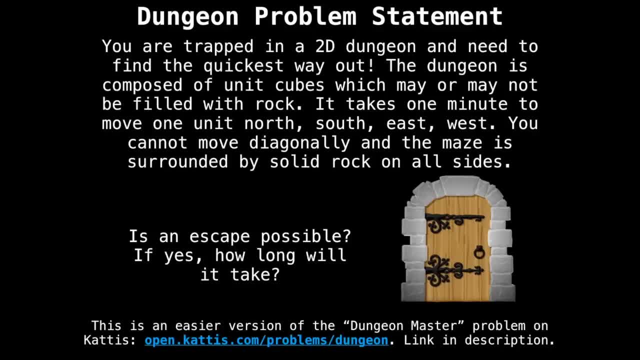 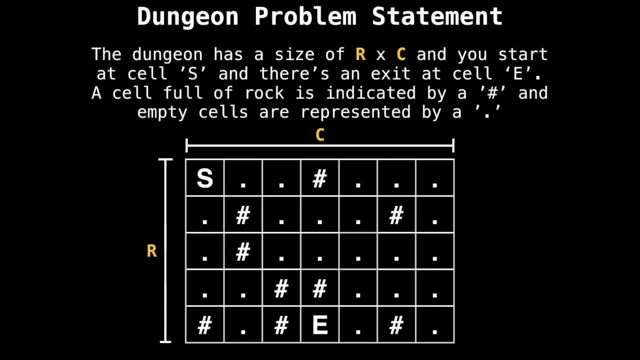 can see that the dungeon is a grid of size R by C And you start at the node with an S character And there's an exit at the cell with an E. a cell full of rock is indicated by a pound sign or a hashtag, And empty cells are represented using a dot And this particular. 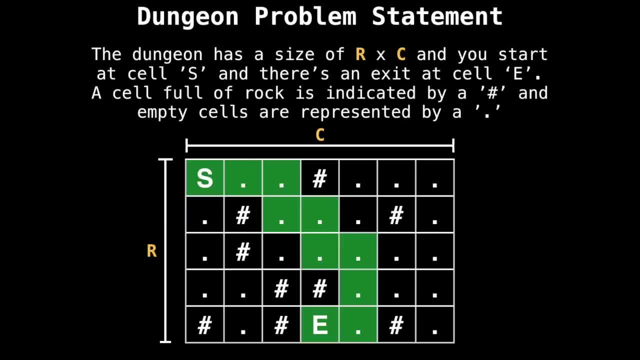 setup. it's possible to escape the dungeon using this particular route highlighted in green. Remember that we want the shortest path to escape dungeon, not just any path. Our approach is going to be to do a breadth first search from the start node until we 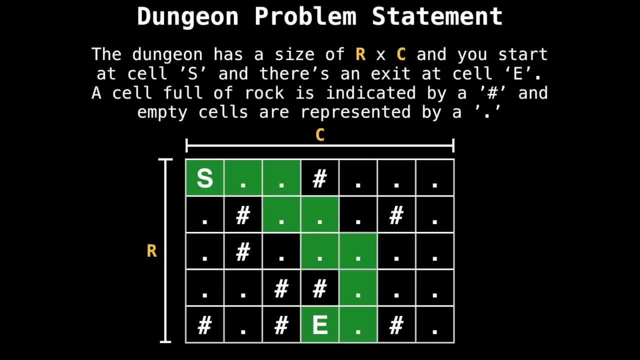 reach the end node and count the number of cells we traverse during that process. However, it might not be possible to exit the dungeon if we cannot reach the exit, So we'll have to be mindful of that. So, like in any breadth, first search. 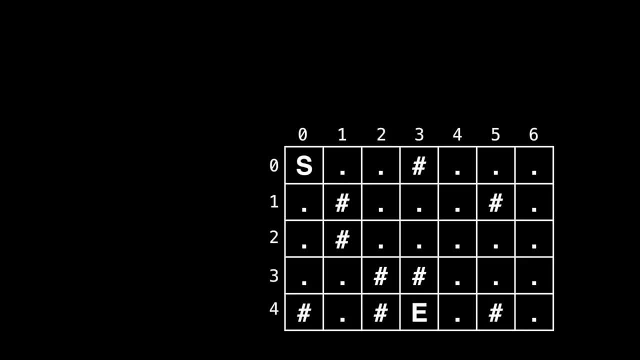 We need to start by visiting our start node and adding it to queue. Assuming we've already found the coordinate of our starting node within the grid, we can add it to the queue. Then we visit the adjacent unvisited neighbors and add them to the queue as well And continue. 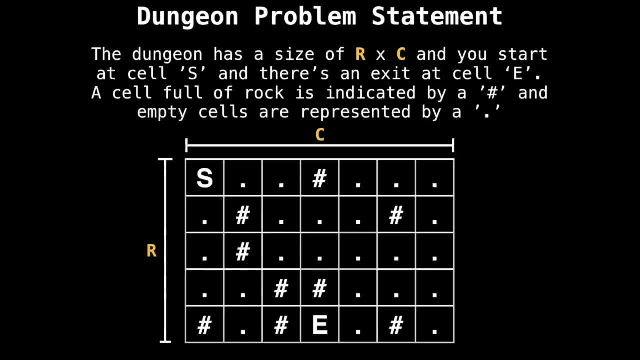 a cell full of rock is indicated by a pound sign or a hashtag, and empty cells are represented using a dot and this particular setup, it's possible to escape the dungeon using this particular rock. So the General rule is that the region of the dungeon has to be a star. 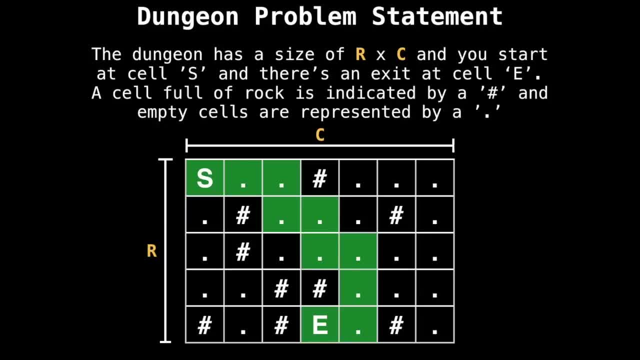 So if we are able to go down to number one and the number of cells that we have in the route highlighted in green, Remember that we want the shortest path to escape dungeon, not just any path. Our approach is going to be to do a breadth first, search from the start. 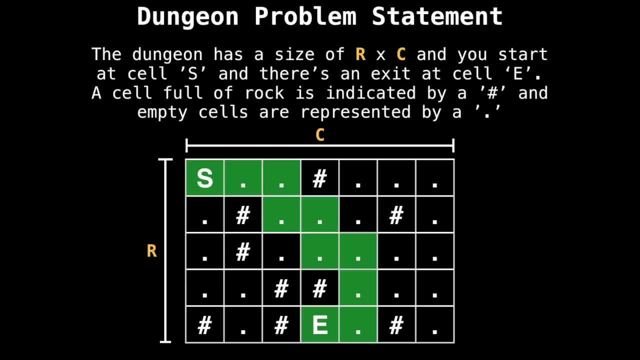 node until we reach the end node and count the number of cells we traverse during that process. However, it might not be possible to exit the dungeon if we cannot reach the exit, So we'll have to be mindful of that. So, like in any breadth, first search, we need 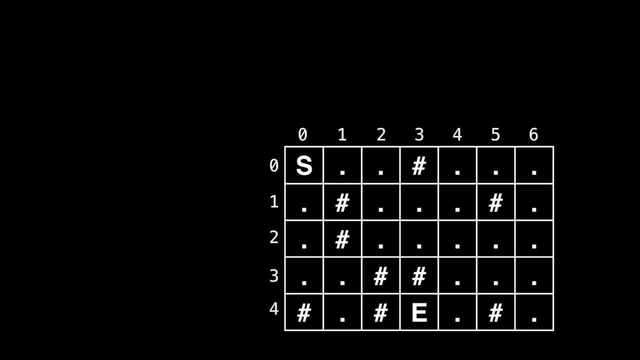 to start by visiting our start node and adding it to queue. Assuming we've already found the coordinate of our starting node within the grid, we can add it to the queue. then we visit the adjacent unvisited neighbors and add them to the queue as well And continue. 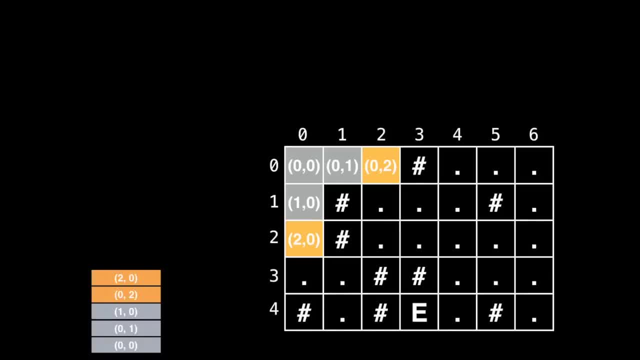 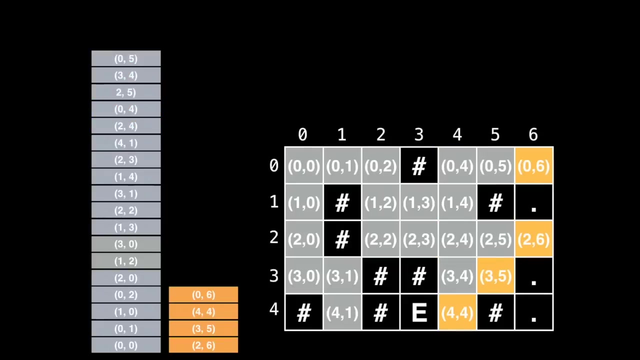 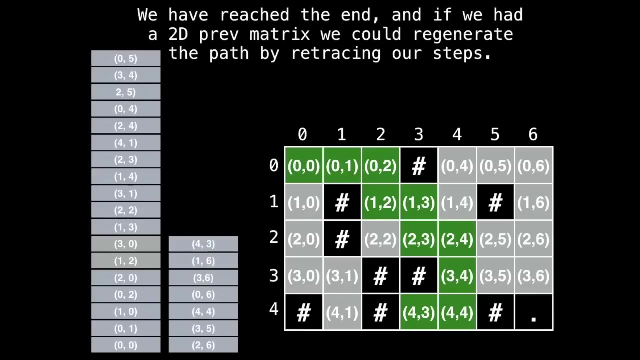 this process, all the while avoiding adding rock cells to the queue. So I'll let the animation play And meanwhile try and predict which cells will be visited next. Alright, after we find our end cell, we know how many steps it takes to get from the start. 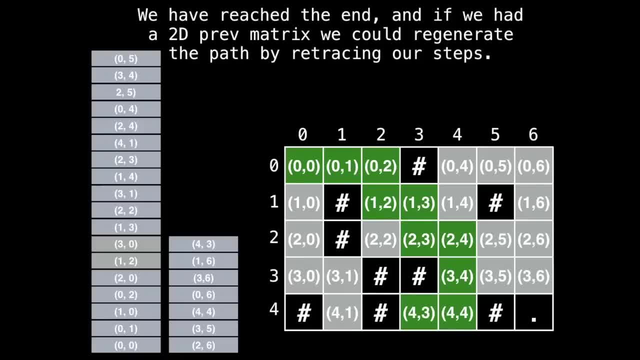 to the end. notice that we didn't even visit all the cells in the grid. the bottom right cell is still unvisited, So it's possible that we're not going to be able to visit all the cells that we terminate early If you're interested in actually finding the path itself. 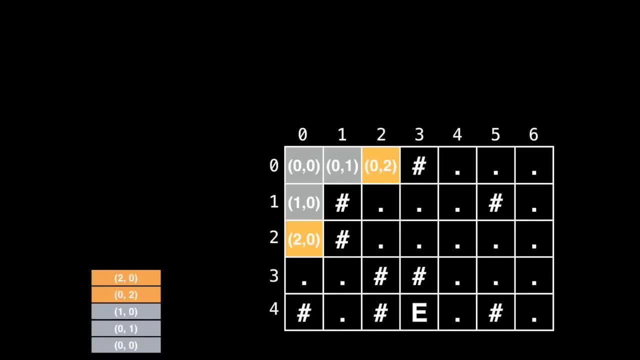 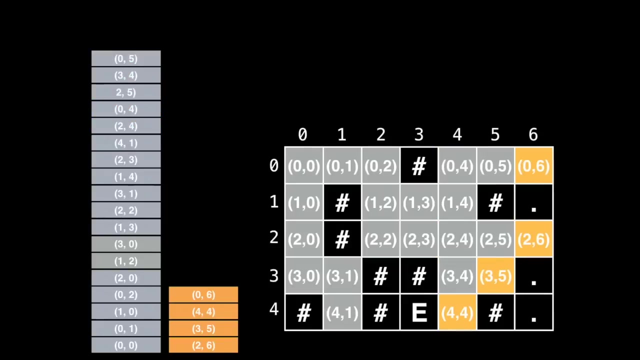 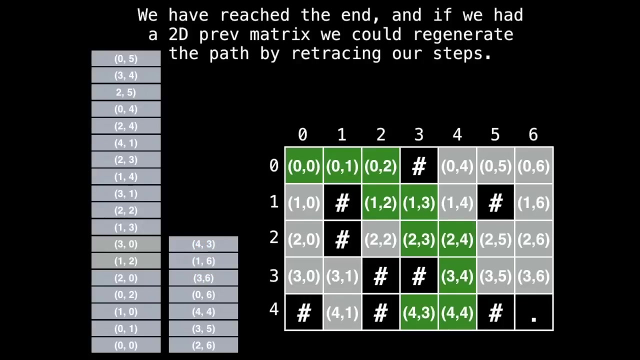 this process, all the while avoiding adding rock cells to the queue. So I'll let the animation play And meanwhile try and predict which cells will be visited next. All right, after we find our end cell, we know how many steps it takes to get from the. 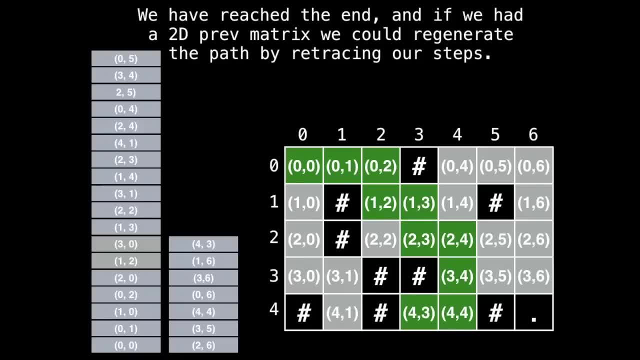 start to the end. notice that we didn't even visit all the cells in the grid. the bottom right cell is still unvisited, So it's possible to unvisit all the cells within the grid. So let's go ahead and do that. All right after we find our end cell. we know how many steps it takes to get from the start to the end. we know how many steps it takes to find those cells within the grid. And if we are at our first start, we know thatanna cleaning tells us that the內 cell. 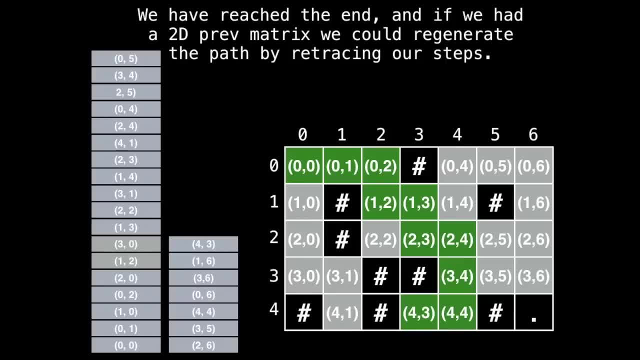 is not necessary And once again we pass on our first start node And every time the inner dry cell is left behind we know how many steps we have to find to get in the state of our second patient And for that we recall if we need to grade our next step, edge cells. we said in all 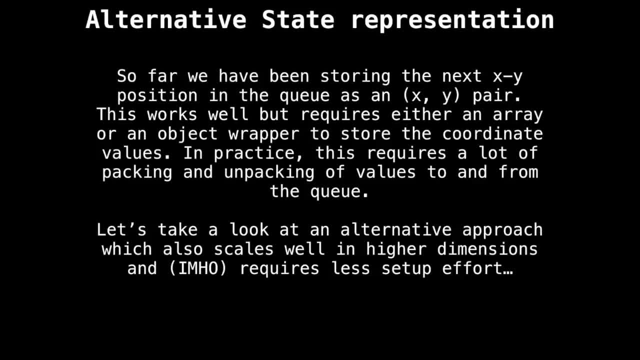 that we had al Emba. So, empty souls and 87 m 이름. we still and already think to move on from here. Let's save our rest of our team And then let's tell tactic with rabbit. We'll use our builder And then we'll apply a little bit of csq in our pivot engine. 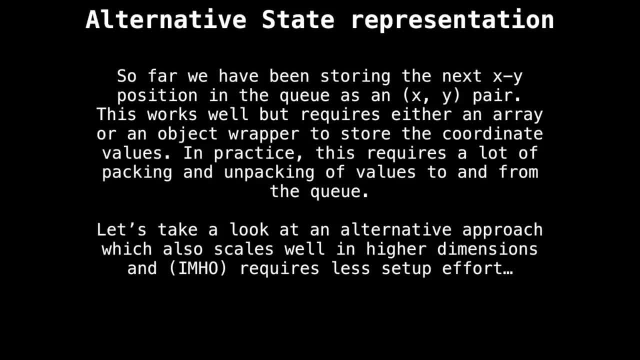 In fact, in case the class is still connected, I'm going to soaked food. these RPM cells x- y position in the queue as an x- y pair. This works well, but requires an array or an object wrapper to store the coordinate values. In practice this can require a lot of packing. 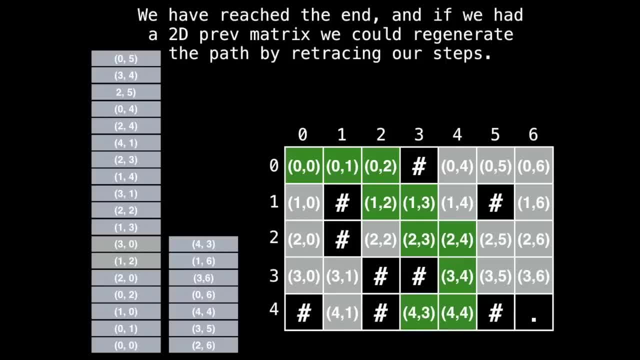 rather than just the number of steps that takes to escape the dungeon. then you'll need to keep track of the previously visited node for each node. Go and rewatch the last video if you need a refresher on how to do that. I want to talk a little bit about the way. 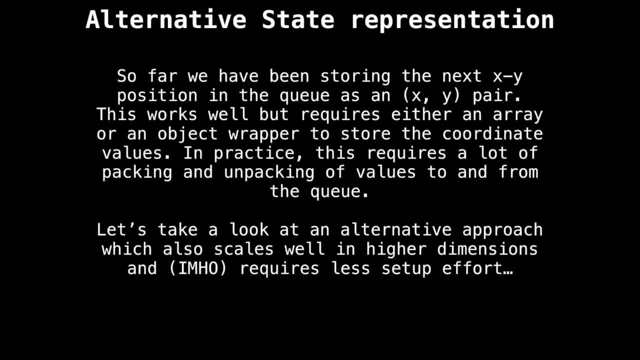 we're representing states in our breadth first search. So far we have been storing the next x y position In the queue as an x y pair. This works well but requires an array or an object wrapper to store the coordinate values. In practice this can require a lot of packing and unpacking. 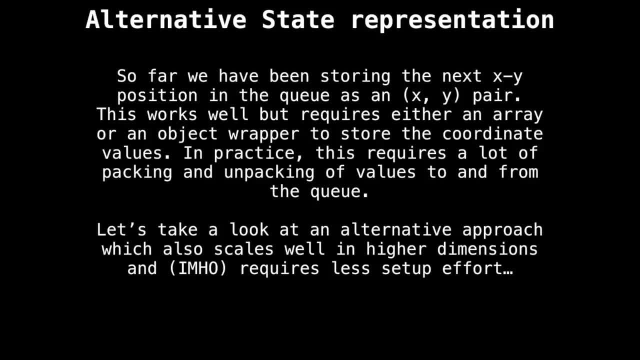 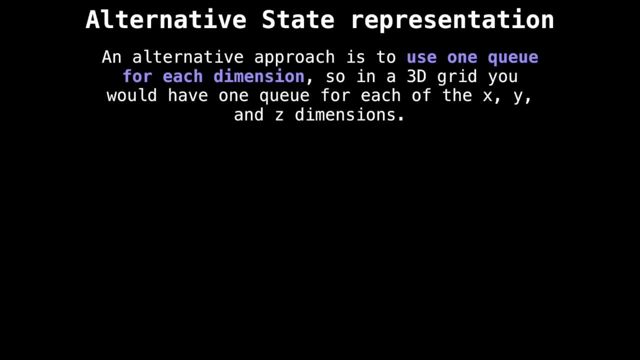 of values to and from our queue. Let's look at an alternative approach which also scales well in higher dimensions and, in my opinion, requires less setup and effort. So the alternative approach I'm suggesting is to use one queue for each dimension. So in a three dimensional grid you would have 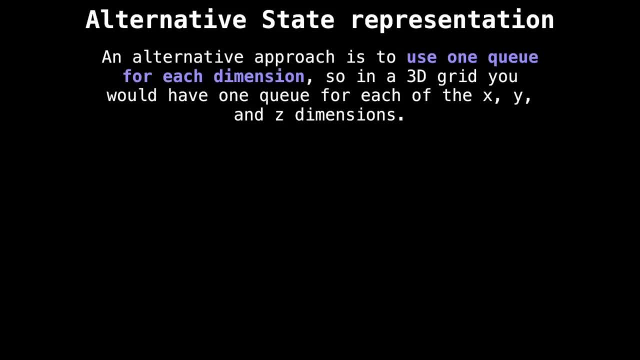 one queue for each of the x, y and z dimensions. Suppose we're in queuing the coordinate x one, y one, z one, then we would simply place each coordinate in their respective cues. So the x coordinate goes in the x q, the y goes in its own y q, and so on As we need. 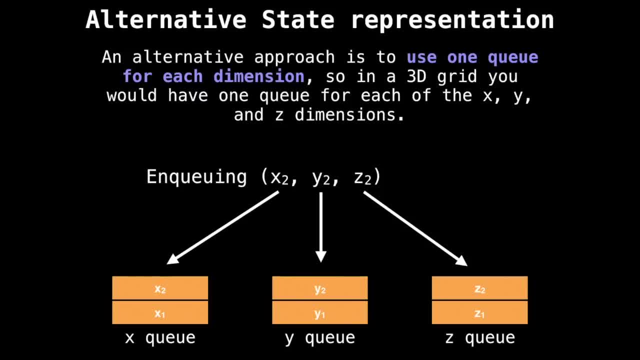 to keep in queuing different positions, So we simply keep filling up these cues this way. This contrasts the approach of simply having one queue with each of the components packed away inside an object. The one thing we have to be mindful about, however, is that when we either end keyword the queue elements. 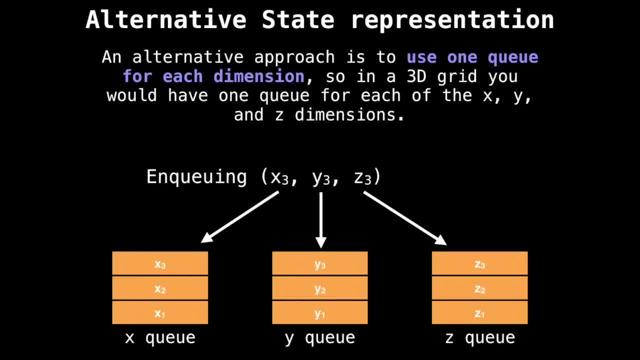 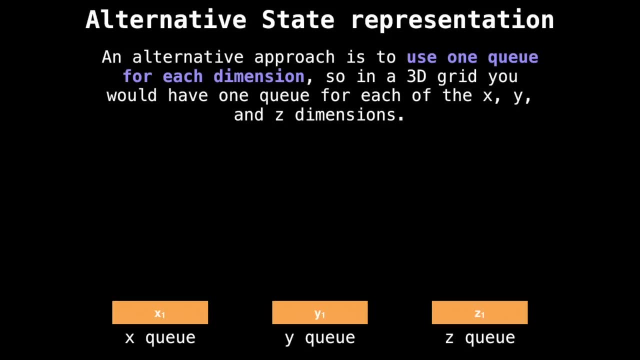 you need to end queue and dequeue elements from each of the queues all at the same time. So when I dequeue or pull elements from the queue, I need to remove it from the queue So I can pull an element from each of these queues. I prefer this representation when. 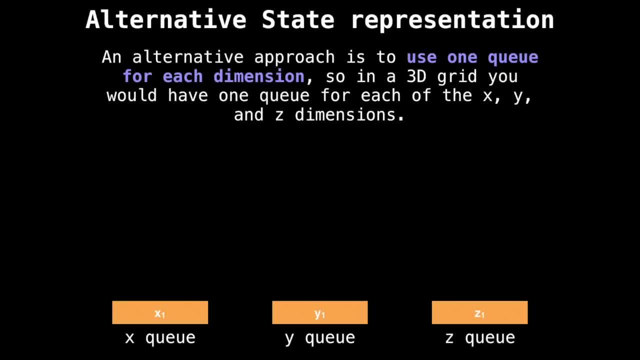 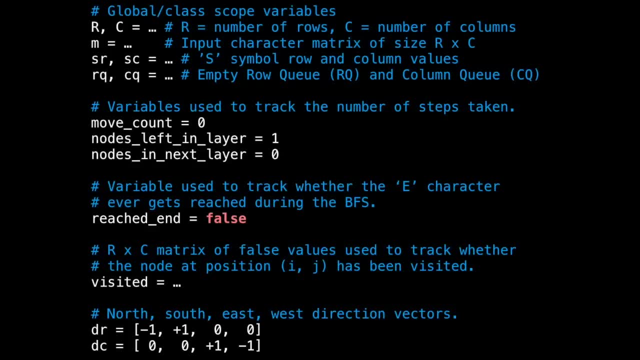 working with multi dimensional coordinates, which is why I want to share it. try it out and see if it works for you. So now that we have all the knowledge we need, we can solve the dungeon problem. Let's look at some pseudocode. Assume that I have already read in the input. 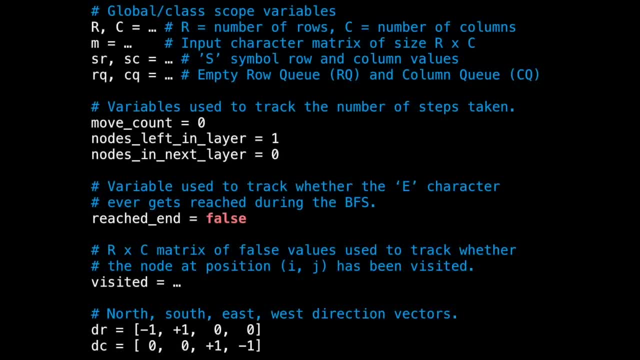 matrix into memory and did some pre processing to find the coordinate of the starting node. So let's see if we can find the coordinate of the starting node. So let's do that. So first of all we need to find the coordinate of the starting node. The first two variables: 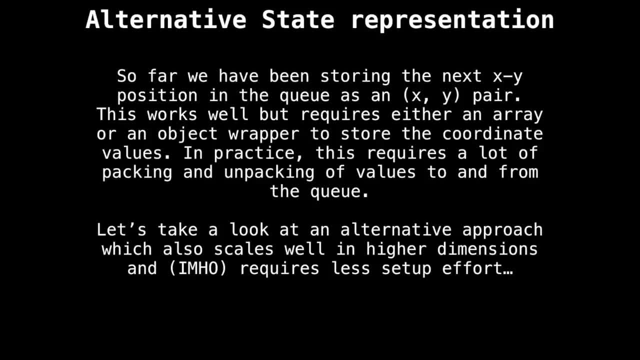 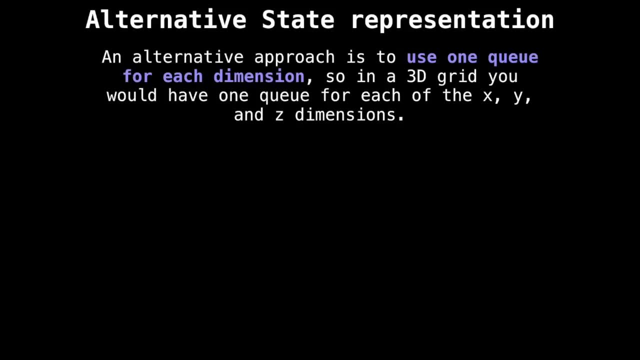 and unpacking of values to and from our queue. Let's look at an alternative approach which also scales well in higher dimensions and, in my opinion, requires less setup and effort. So the alternative approach I'm suggesting is to use one queue for each dimension. So 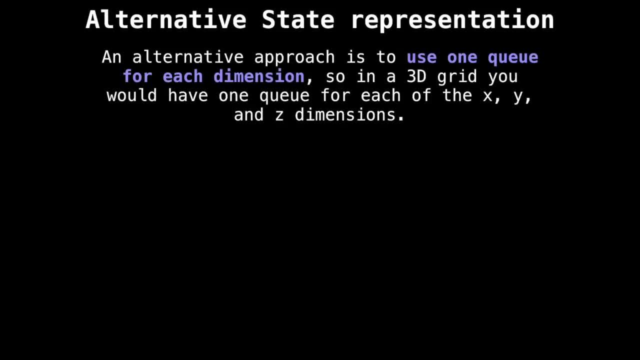 in a three dimensional grid, you would have one queue for each of the x, y and z dimensions. Suppose we're in queuing the coordinate x one, y one, z one, then we would simply place each coordinate in their respective queues. So the x coordinate goes in, the x, q, the y. 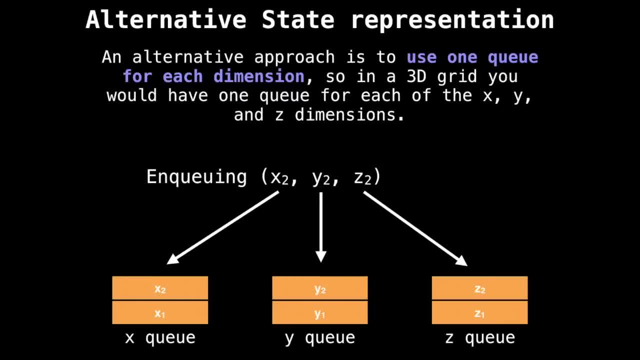 goes in its own: y, q and so on. As we need to keep in queuing different positions, we simply keep filling up these queues this way. This contrasts the approach of simply having one queue with each of the components packed away inside an object. The one thing we have to be mindful about, however, is that 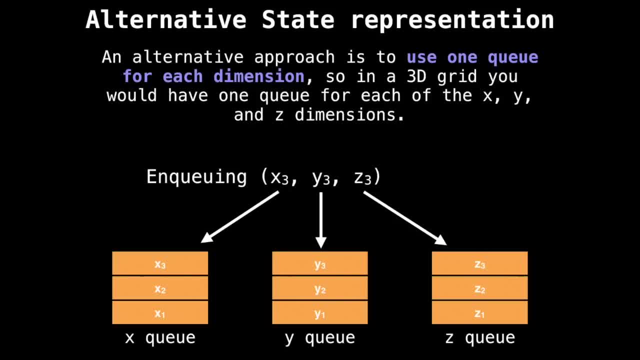 when we either end keyword the D Q elements- you need to end queue- and D Q elements from each of the queues all at the same time. So when I D Q elements from each of the queues all at the same time. so when I D Q elements. 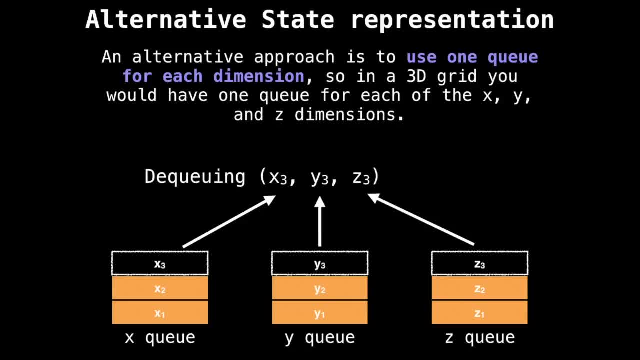 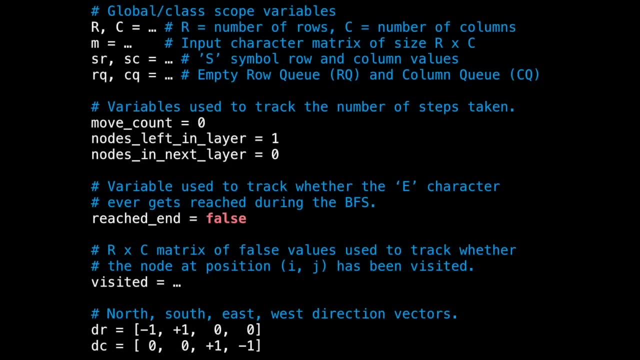 queue or pull elements from the queue. I need to remove an element from each of these queues. I prefer this representation when working with multi dimensional coordinates, which is why I want to share it, try it out and see if it works for you. So, now that we have, 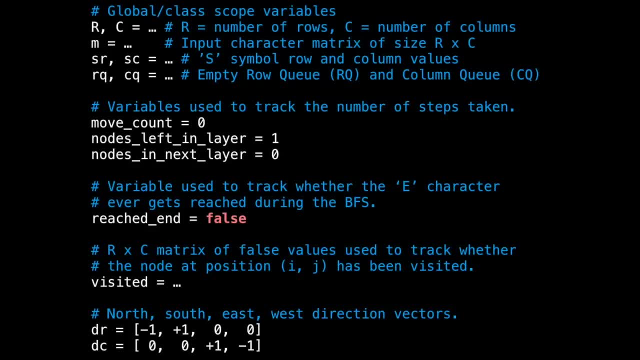 all the knowledge we need, we can solve the dungeon problem. Let's look at some pseudocode. Assume that I have already read in the input matrix into memory and did some pre processing to find the coordinate of the starting node, The first two variables are the constants. 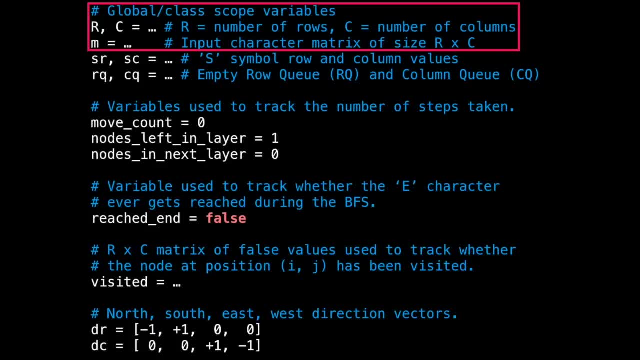 are and see the number of rows and columns in the input matrix. Following this is m, the input character matrix of size r by C. Next are two variables: s, r and s. see the row column position of the starting node. We'll need this to start our breadth. first search. 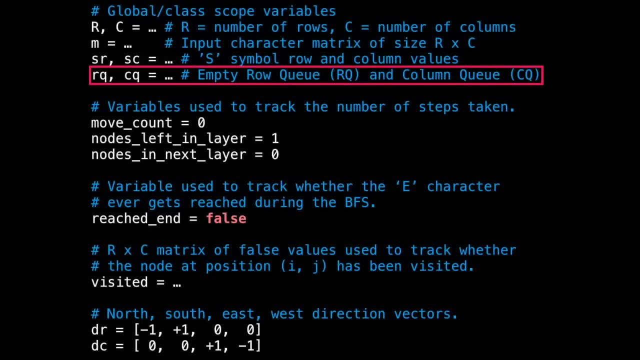 RQ and CQ are two queued data. These data structures that represent the row queue and the column queue will be n queuing and de queuing elements from during the breadth first search. This next set of variables is to keep track of the number of steps taken to reach the exit. move count will actually. 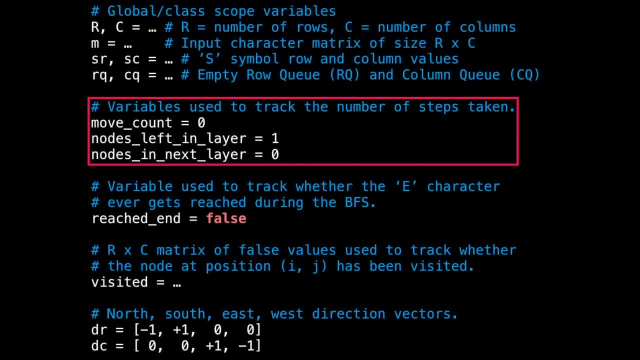 track the number of steps taken. nodes left in layer tracks how many nodes we need to de cube before taking a step. and nodes in next layer tracks how many nodes we actually added in the breadth first search expansion so that we can update nodes left in layer. 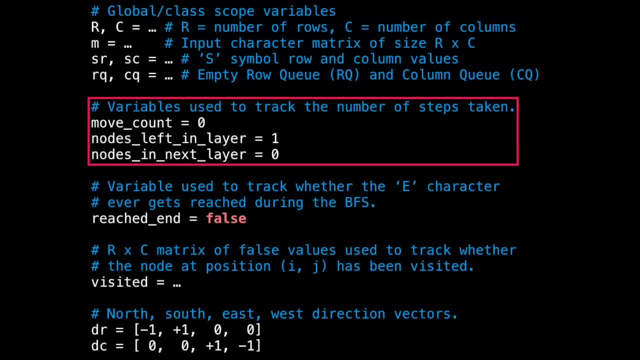 accordingly In the next iteration. this will make more sense soon reached and tracks whether or not we have reached the end cell marked with an E. we're also going to make use of a visited matrix the same size as the input grid to track whether or not a cell has been. 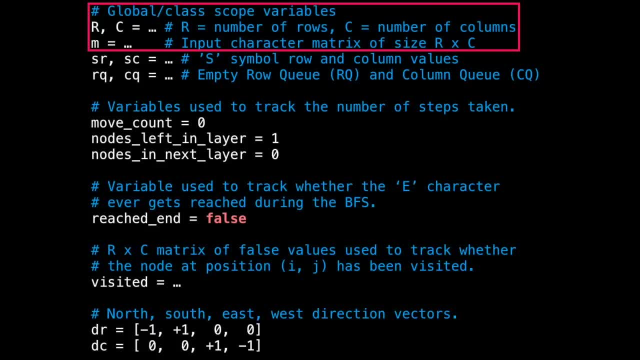 are. the constants are, and see the number of rows and columns in the input matrix. Following this is m, the input character matrix of size r by C. Next are two variables, s r and s c, the row, column position of the starting node. We'll need this to start our breadth. 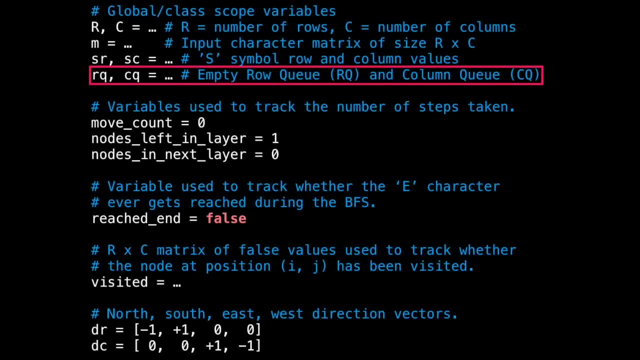 first search. our q and cq are two q data structures that represent the row q and the column q will be n queuing and de queuing elements from during the breadth first search. This next set of variables is to keep track of the number of steps taken to reach the 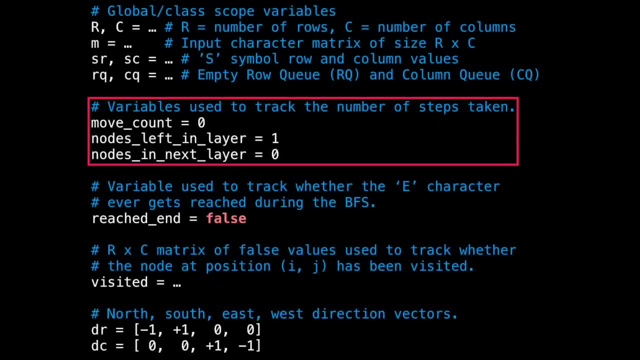 exit move count will actually track the number of steps taken. nodes left in layer tracks how many nodes we need to de cube before taking a step and nodes in next layer tracks how many nodes we added in the breadth first search expansion So that we can update nodes left in layer accordingly In the next iteration. this will 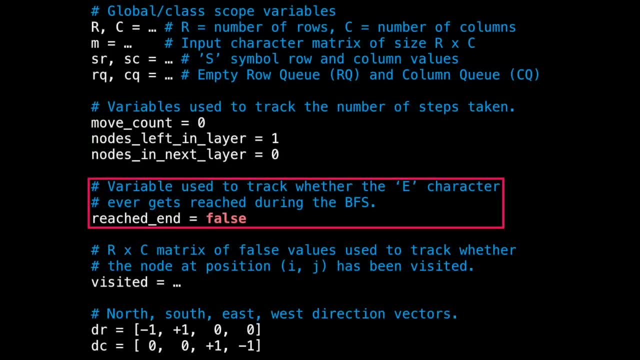 make more sense soon reached and tracks whether or not we have reached the end cell marked with an E. we're also going to make use of a visited matrix the same size as the input grid to track whether or not a cell has been visited, since we do not want to visit a cell. 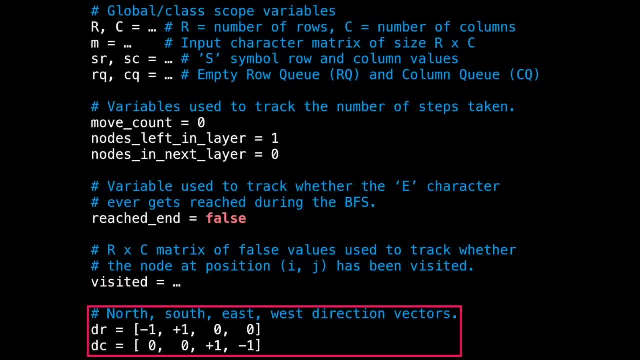 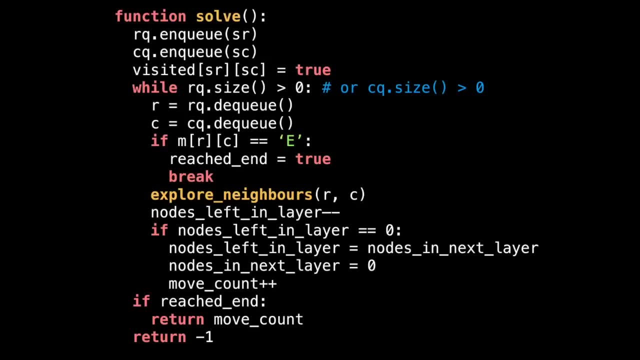 multiple times And, lastly, I defined the north, south, east and west direction. So we're going to use the start cell as the start cell and the end cell as the end cell To solve the dungeon problem. this is all the code we'll need to execute our breadth. 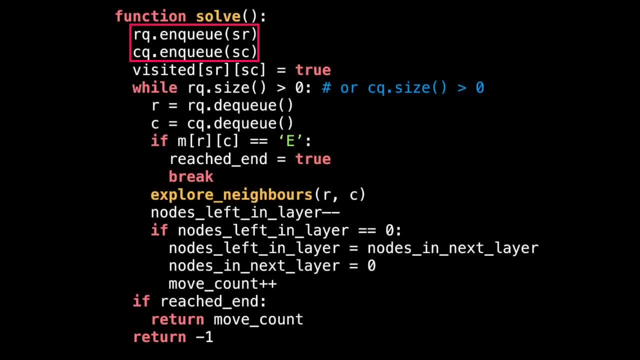 first search and reach the exit. The first thing I do is add the start cells row and column values to the row q and column q. Then don't forget to mark the start cell as visited, because we don't want to go there again. We're not done our breadth. first search until both. 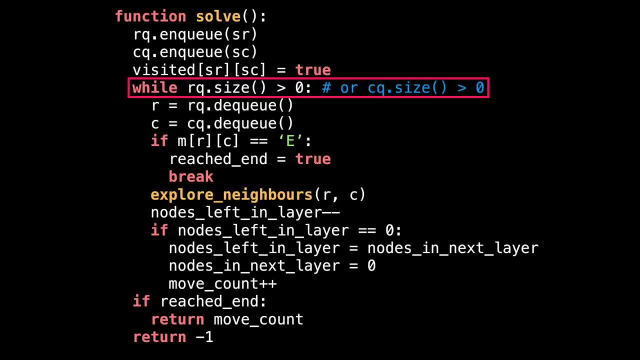 of our queues are empty. I checked: the size of the row q is greater than zero, So we're good to go. But you can also check that the size of the column q is greater than zero, since their sizes should always be in sync. Then, since I know, the queues aren't empty. 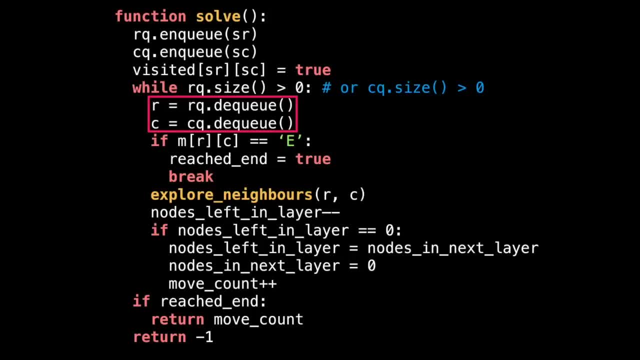 I can dequeue the current position from the queues as the row position R and the column position C. Then I check if we've reached the dungeon exit by checking if the current character in the grid is an E. if it is, then mark that we've reached the exit and break. 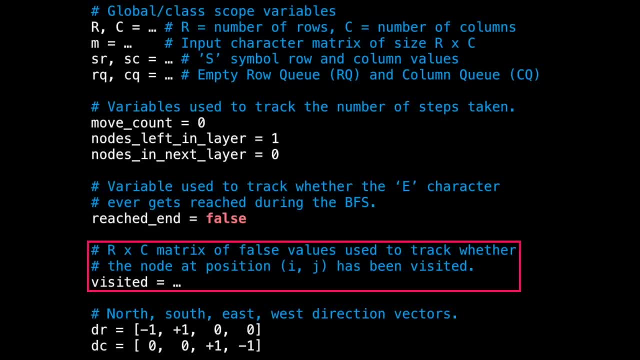 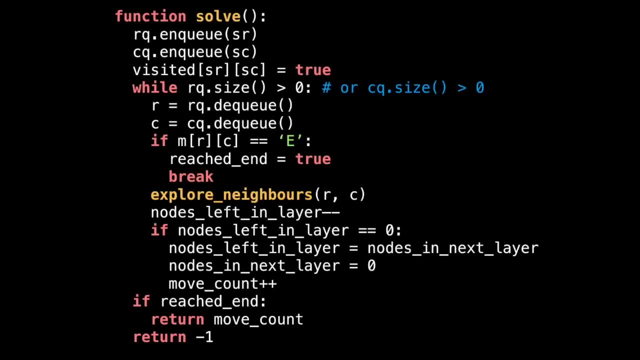 visited, since we do not want to visit a cell multiple times. And lastly, I defined the the north, south, east and west direction vectors To solve the dungeon problem. this is all. the code will need to execute our breadth first, search and reach the exit, The first. 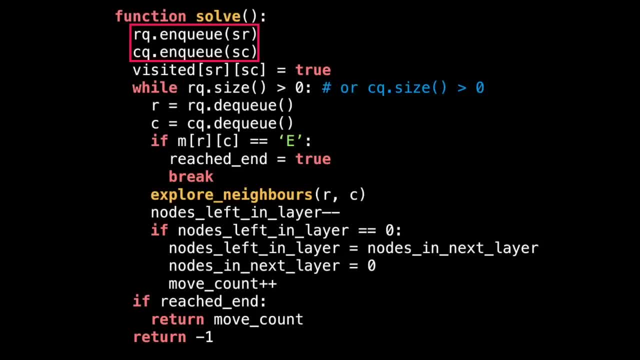 thing I do is add the start cells, row and column values to the row queue and column queue. Then don't forget to mark the start cell as visited, because we don't want to go there again. We're not done our breadth. first search until both of our queues are empty. 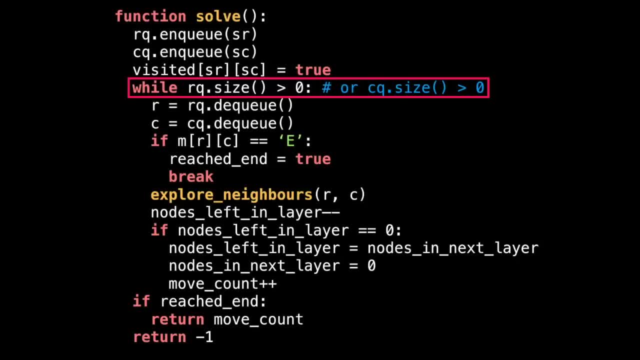 I checked, the size of the row queue is greater than zero, But you can also check that the size of the column queue is greater than zero, since their sizes should always be in sync. Then, since I know the queues aren't empty, I can dequeue the current position from the 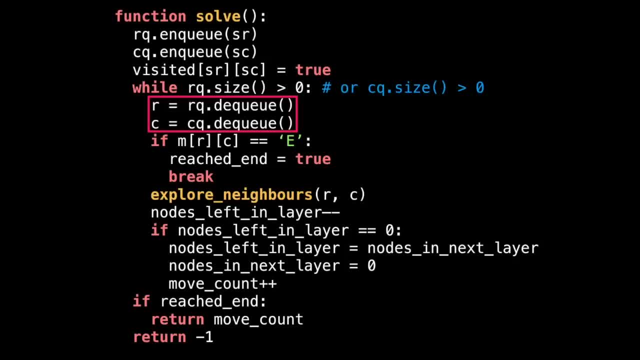 queues. as the row position are and the column position C, then I check if we've reached the dungeon exit by checking if the current character in the grid is an E. if it is, then mark that we've reached the exit and break out early. Otherwise we're not done exploring and we 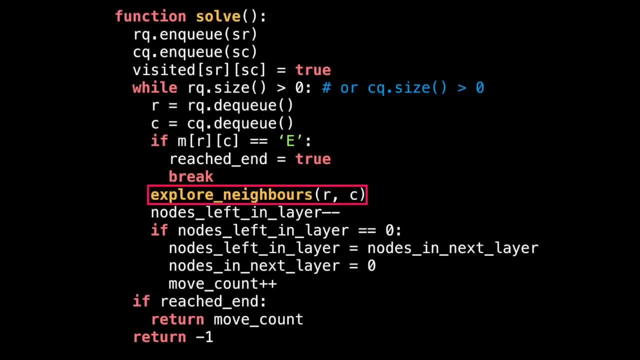 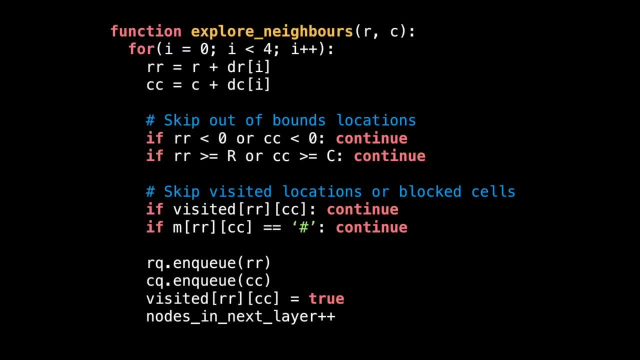 want to add all valid neighbors of the current node to the queue. I wrote a function called explore neighbors that'll do just that. Let's have a look. Here we are inside the explore neighbors method. This is where we'll be using the direction vector technique we learned. 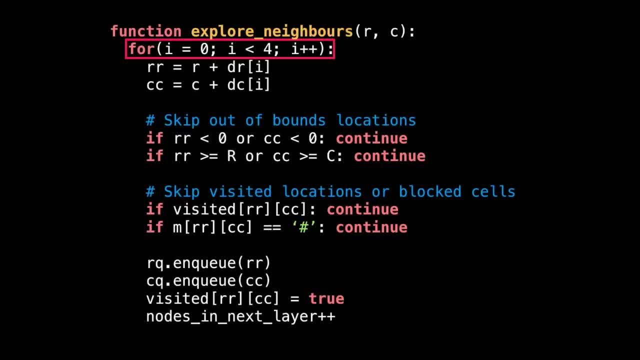 about earlier. Since cells have four directions, we care about north, south east, south east, south east and west. I loop I from zero to four, non inclusive. compute the new coordinate r, r, comma, CC by adding the direction vector to the current position. make sure the new 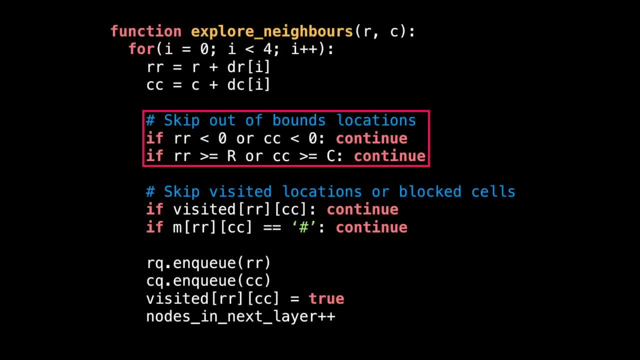 position is actually within the grid, because we could end up with positions like zero comma minus one, which is out of bounds. Even if the new position is within the grid, that does not guarantee that is a valid position. The position might already have been visited. 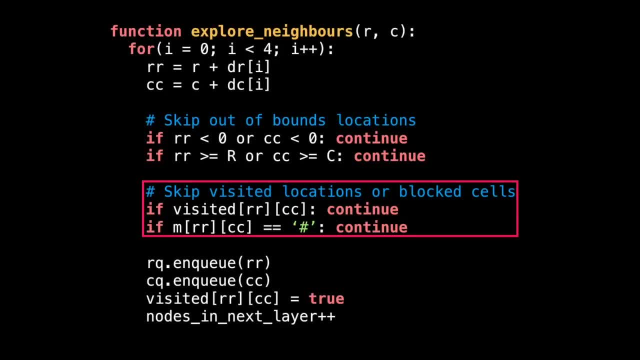 previously, or it could be a blocked off cell, such as a cell that isn't traversable and full of rock. If both of those conditions aren't true, then we can enqueue the new position to visit it later. When enqueuing a new position we are going to visit, make sure to mark it. 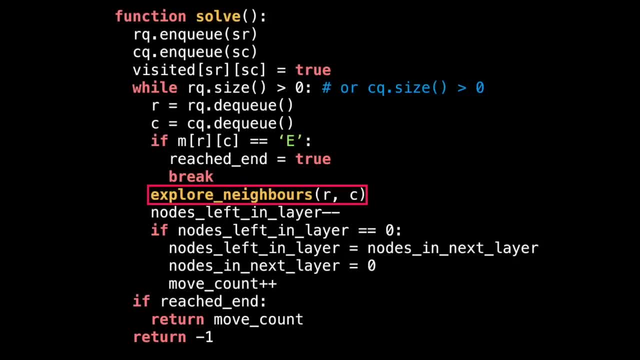 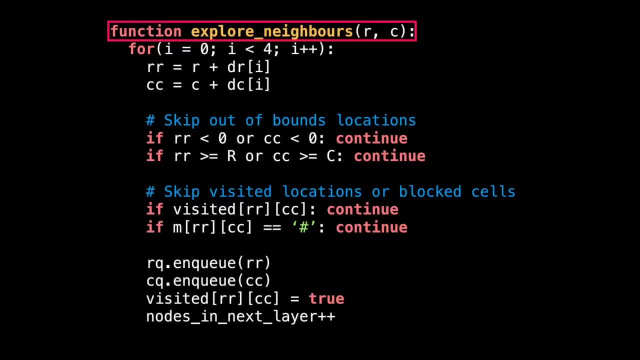 out early. Since we're not done exploring and we want to add all valid neighbors of the current node to the queue, I wrote a function called explore neighbors that'll do just that. Let's have a look. Here we are inside the explore neighbors method. This is where we'll be using. 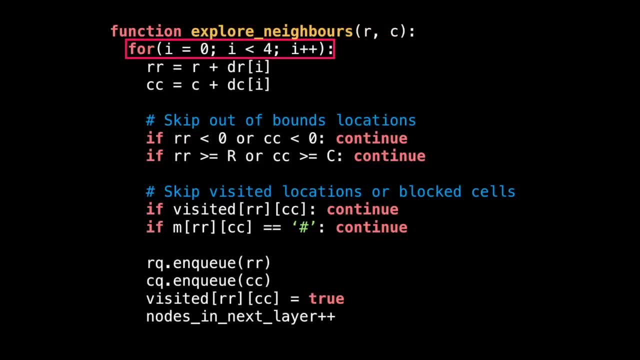 the direction vector technique we learned about earlier. Since cells have four directions, we care about north, south, east and west. I loop I from zero to four, not included. So we're going to use the direction vector technique to add the direction vector to the 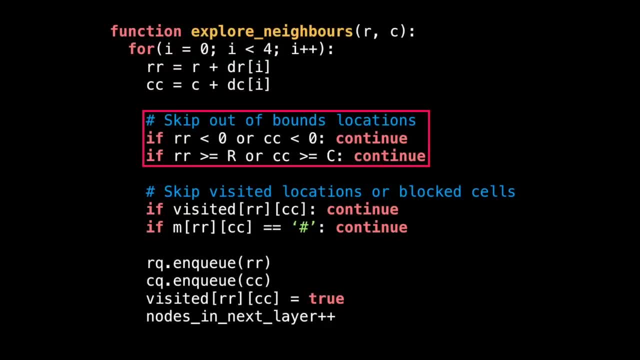 current position. Make sure the new position is actually within the grid, because we could end up with positions like zero comma minus one, which is out of bounds. Even if the new position is within the grid, that does not guarantee that is a valid position. The position: 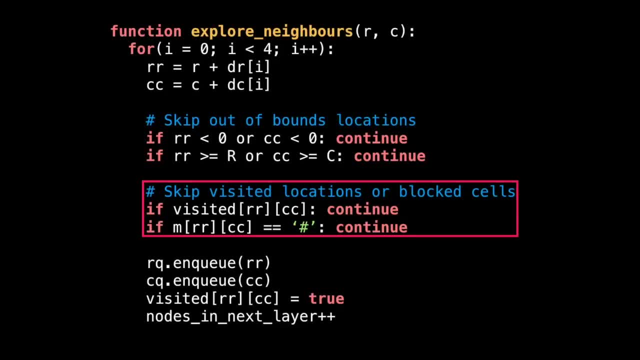 might already have been visited previously, or it could be a blocked off cell, such as a cell that isn't traverses first and full of rock. If both of those conditions aren't true, then we can enqueue the new position to visit it later, When end q n a new position. 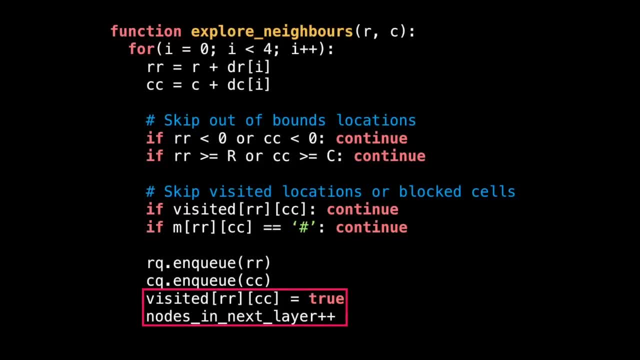 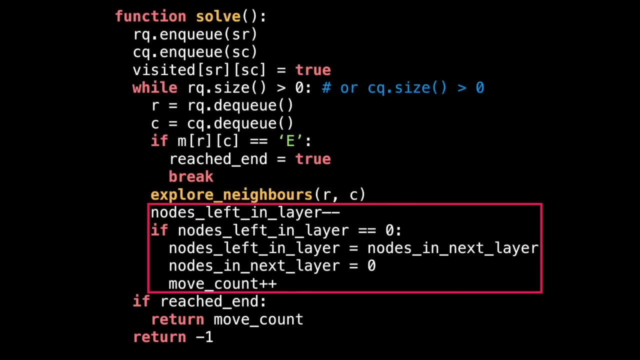 we are going to visit. make sure to mark it as visited now so that it doesn't get added to the queue multiple times in the future. Also, increment the number of nodes in the next layer which will be needing shortly. This nextos block of code is used to track the number of steps we took getting to the dungeon exit. 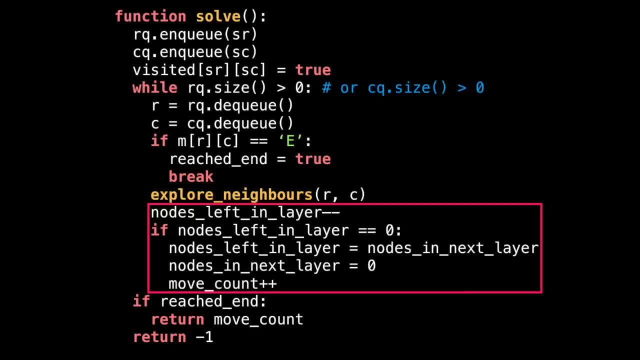 Every time we finish a layer of nodes, we increment the number of steps taken. we know how many nodes are in each layer because we kept track of that in the explore neighbors method. When the number of nodes on the current layer reaches zero, we know to increment the. 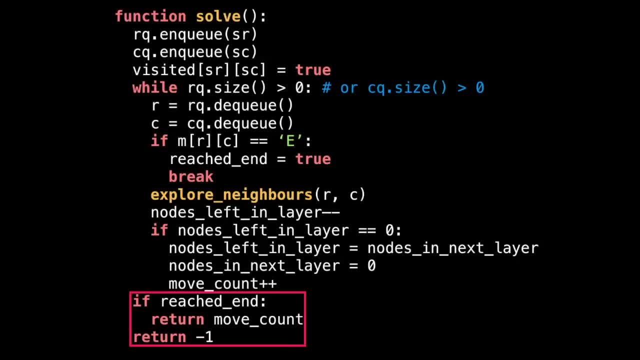 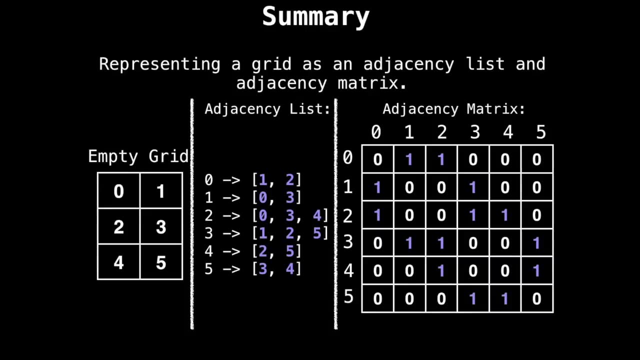 move count. At the end, if we are able to reach the exit, we return the move count. Otherwise, we return minus one to indicate that the dungeon exit was not reached. So, in summary, things we learned in this video are how to represent a grid as an adjacency. 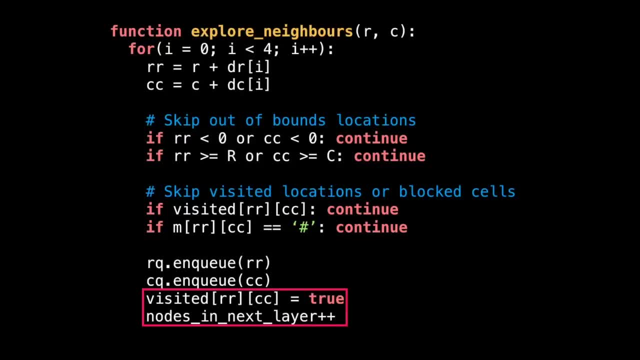 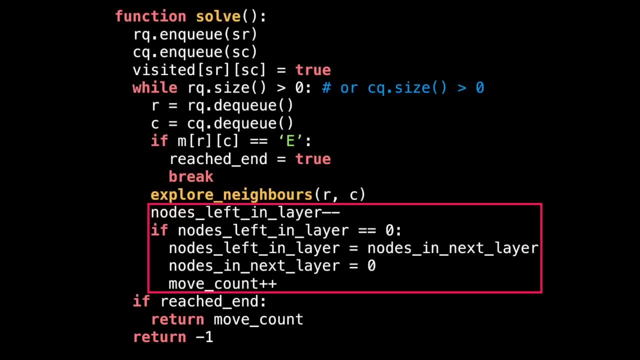 as visited now, so that it doesn't get added to the queue multiple times in the future. Also, increment the number of nodes in the next layer which will be needing shortly. This next block of code is used to track the number of steps we took. 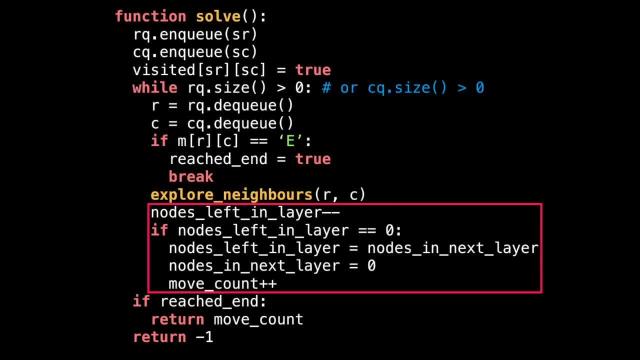 getting to the dungeon exit. Every time we finish a layer of nodes, we increment the number of steps taken. we know how many nodes are in each layer because we kept track of that in the explore neighbors method. When the number of nodes on the current layer reaches, 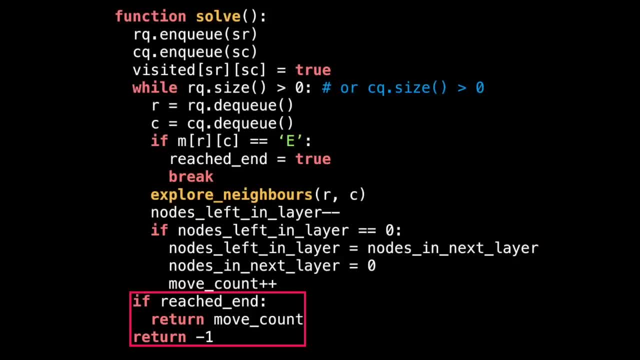 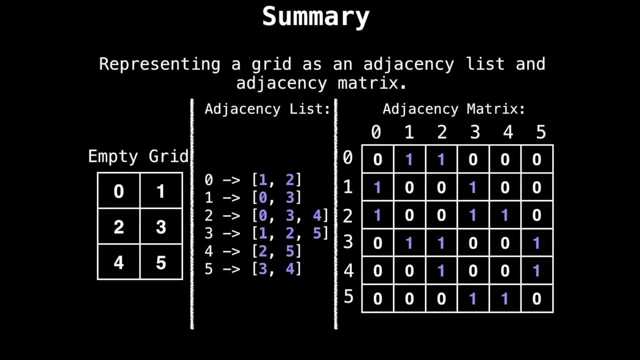 zero. we know to increment the move count At the end. if we are able to reach the exit, we return the move count. Otherwise we return minus one to indicate that the dungeon exit was not reached. So, in summary, things we learned in this video. 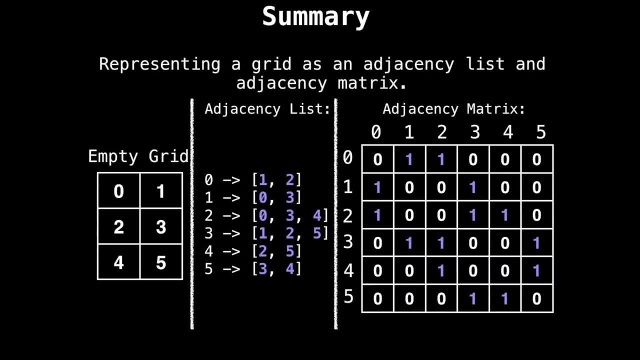 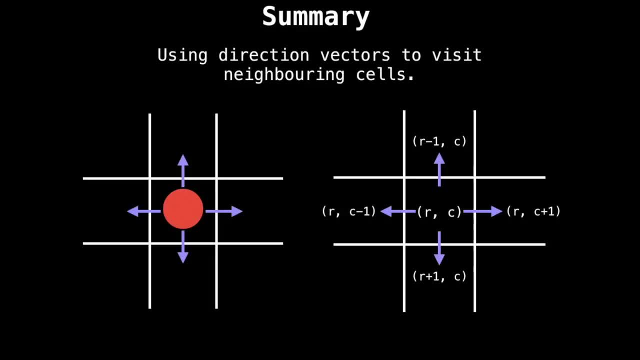 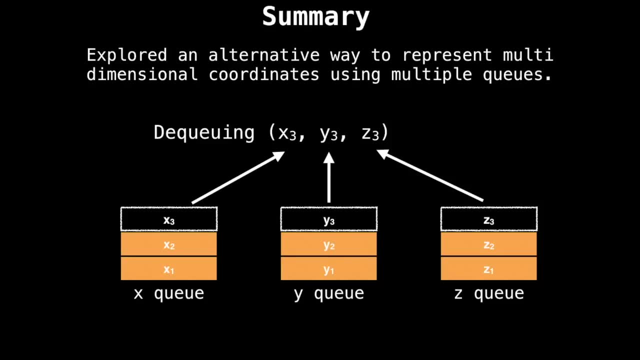 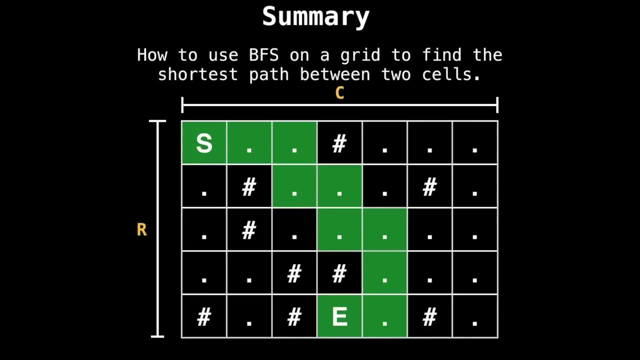 are how to represent a grid as an adjacency list and an adjacency matrix, how to use direction vectors to visit neighboring cells, We explored an alternative way of representing multi dimensional coordinates with multiple cues And, lastly, we looked at how to use a breadth. first search on a grid to find the shortest path between two cells. Today's topic: 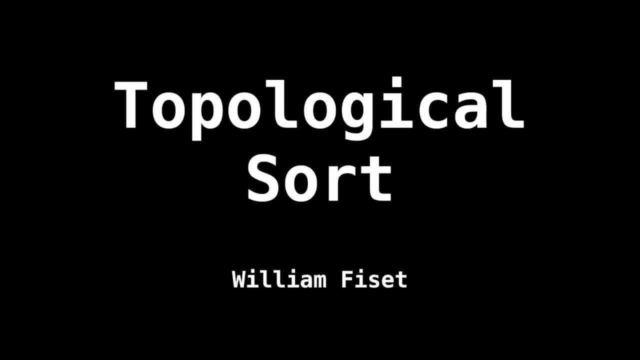 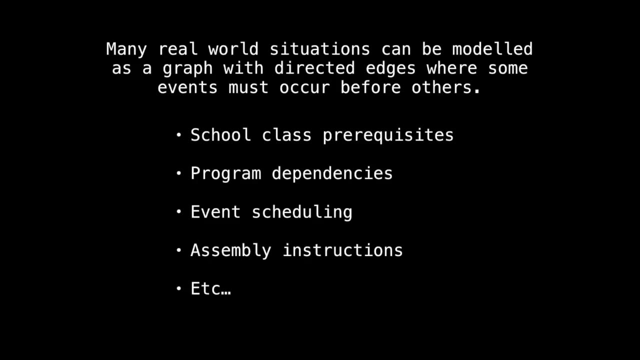 is topological sort, also called top sort for short. we're going to discuss what is top sort, where it's used and how to find a topological ordering with some animation. The motivation for top sort is that many real world situations can be modeled as a graph of nodes and directed edges, where 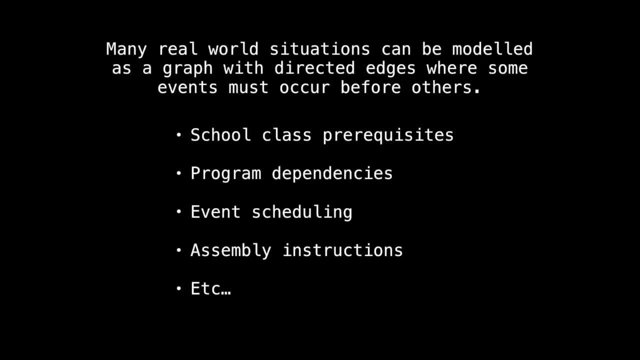 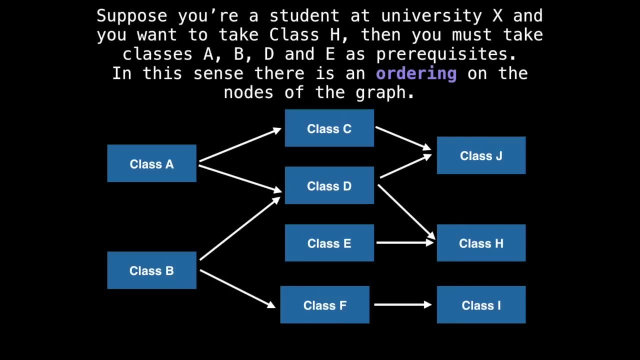 some events have to occur before others. Some simple examples include school class prerequisites, program dependencies, event scheduling, assembly instruction ordering and much, much more. Let's begin with an example. Suppose you're a university student and you really want to take class H. 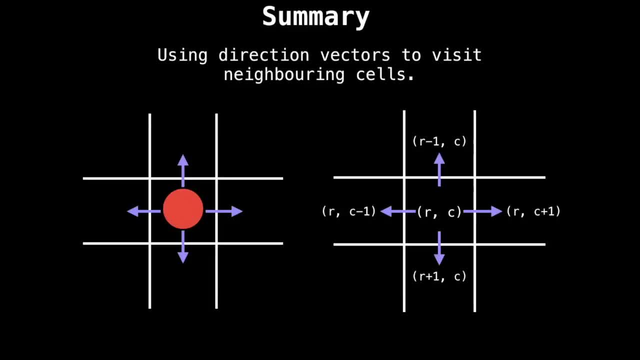 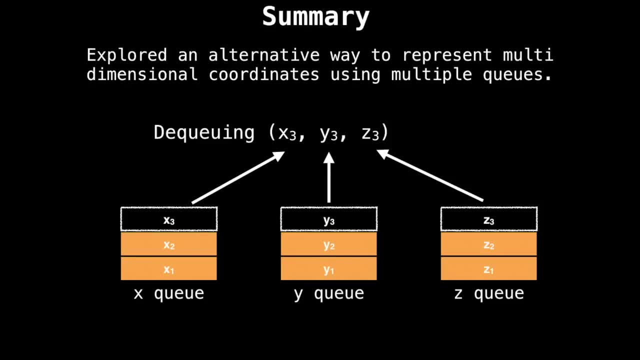 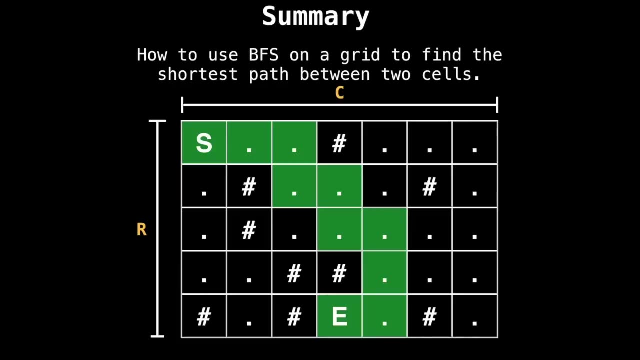 list and an adjacency matrix, how to use direction vectors to visit neighboring cells, We explored an alternative way of representing multi dimensional coordinates with multiple queues And, lastly, we looked at how to use a breadth. first search on a grid to find the shortest. 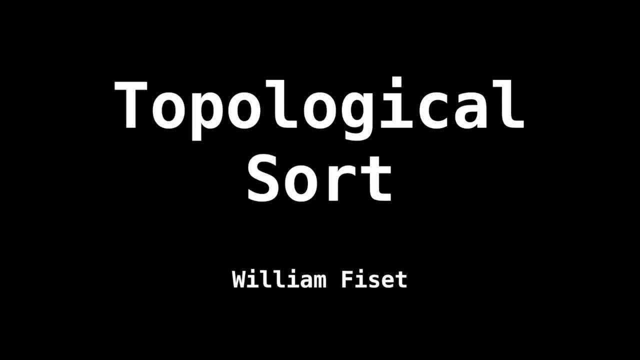 path between two cells. Today's topic is topological sort, also called top sort for short. we're going to discuss what is top sort, where it's used and how to find a topological ordering with some animation. The motivation for top sort is that many real world situations can. 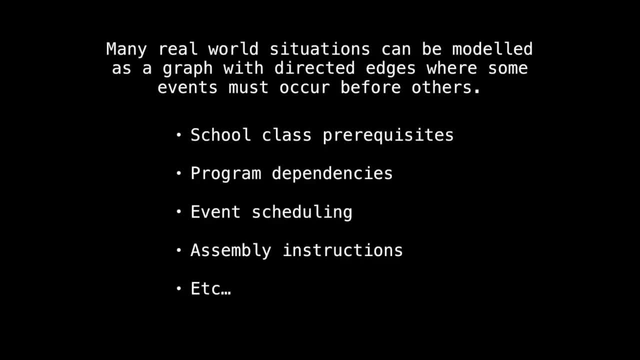 be modeled as graph. Top sort is a graph of nodes and directed edges where some events have to occur before others. Some simple examples include school class prerequisites, program dependencies, event scheduling, assembly instruction ordering and much, much more. Let's begin. 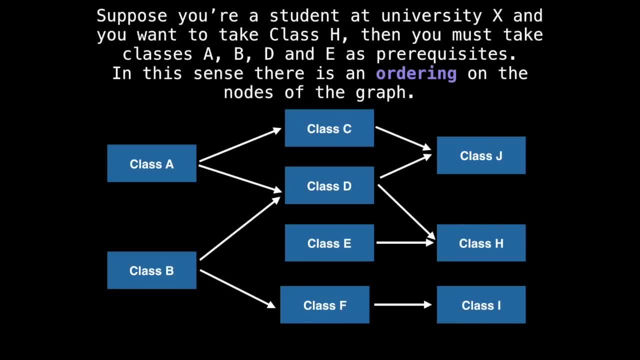 with an example. Suppose you're a university student and you really want to take class H. Well, before you can enroll in class H, you must first take classes D and E. But before taking class D, you must also take classes A and B, which have no prerequisites. So in some sense there appears to be an ordering. 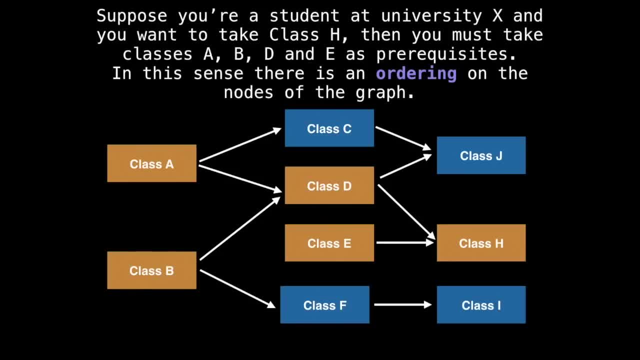 on the nodes of the graph. If we needed to take all the classes, the top sort algorithm would be capable of telling us the order in which we should enroll in classes, such that we never enroll in a course which we do not have prerequisites for Another canonical. 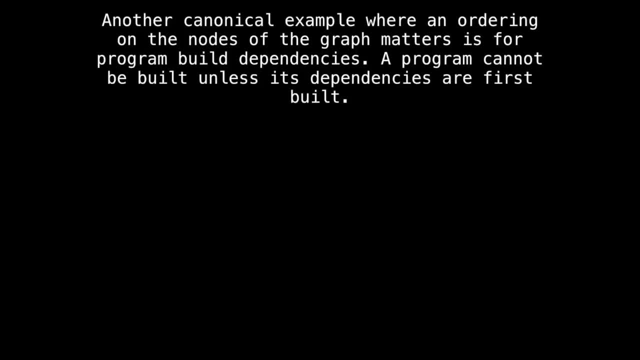 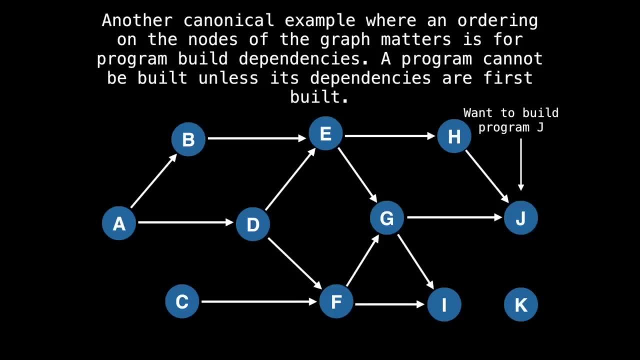 example of an application of top sort is for program build dependencies. A program cannot be built unless all its dependencies are first built. For example, consider this graph where each node represents a program and the edges represent that one program depends on the other to run. Well, if we're trying to build program J on the right hand side, then we 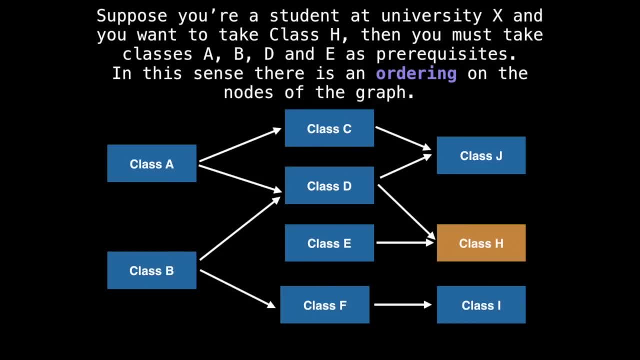 Well, before you can enroll in class H, you must first take classes D and E. But before taking class D you must also take classes A and B, which have no prerequisites. So in some sense there appears to be an ordering on the nodes of the graph. If we needed to, 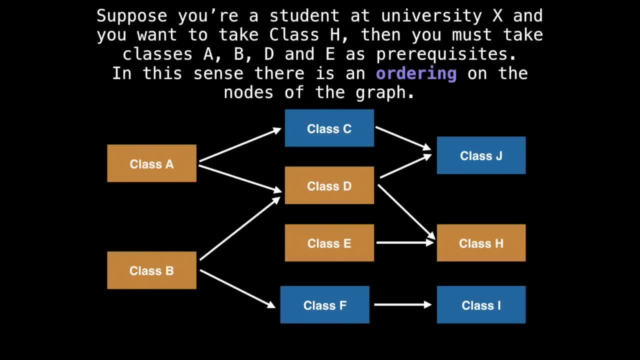 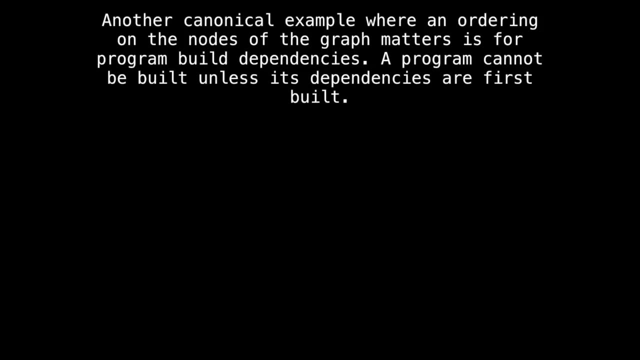 take all the classes, the top sort algorithm would be capable of telling us which nodes we should enroll in, unless the order in which we should enroll in classes, such that we never enroll in a course which we do not have prerequisites for. Another canonical example of an application: 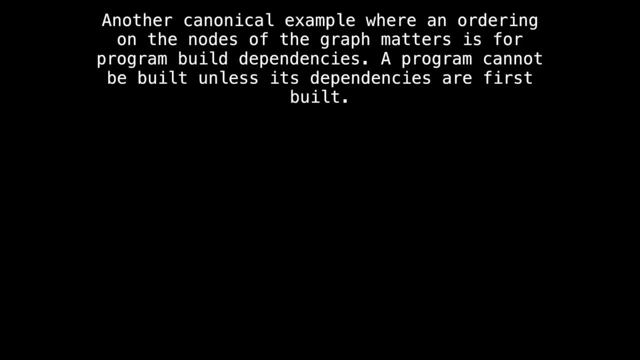 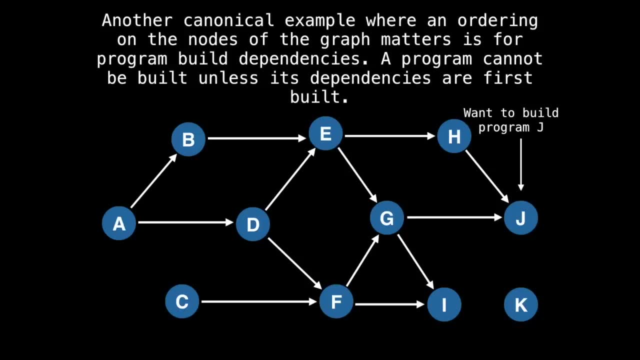 of top sort is for program build dependencies. A program cannot be built unless all its dependencies are first built. For example, consider this graph, where each node represents a program, but it would IP move into another component, a program, And the edges represent that one program depends on another to run. Well if 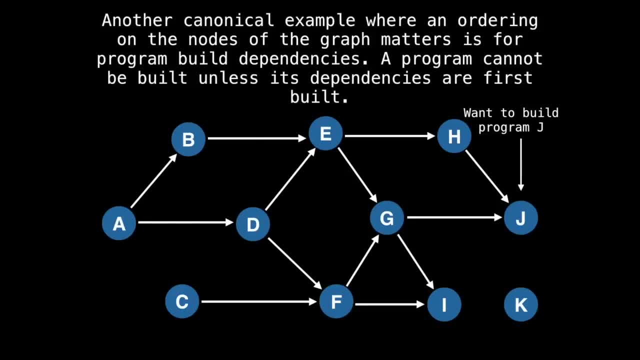 we're trying to build a program J on the right hand side, then we must first build program H and G, But to build those we also need. E and F, But to build those we also need, and so on. The idea is to first build the programs without dependencies and then move. 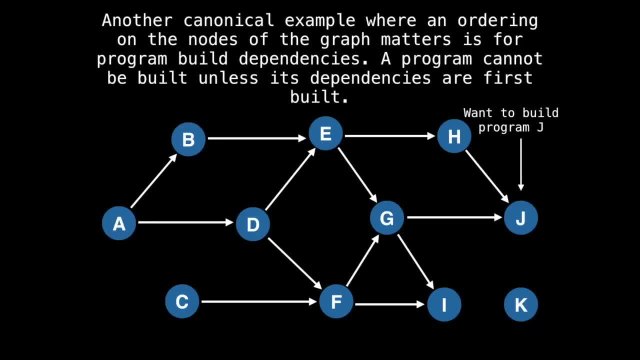 onwards from there. How do we find a valid ordering in which to build all the programs? Well, this is where TopSort comes into play. One possible ordering might be to start by building a, then building C, B, D, F, E, G, H and then J. Notice that there are unused. 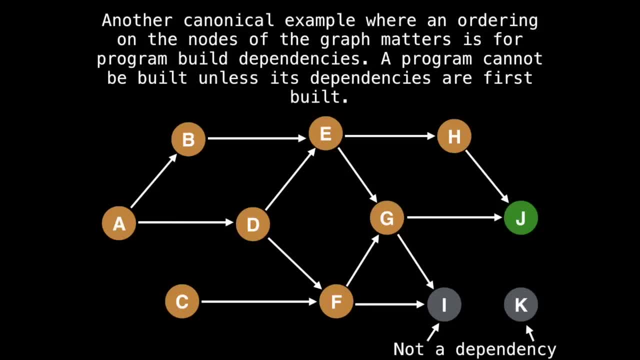 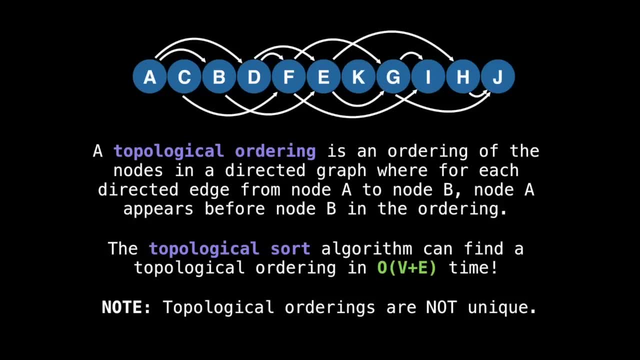 dependencies in this case, And that will happen from time to time, which is fine. But if we build a program J on the right hand side, then we must first build a program J on the left hand side, which is fine. So, in conclusion, TopSort is an algorithm which will give us 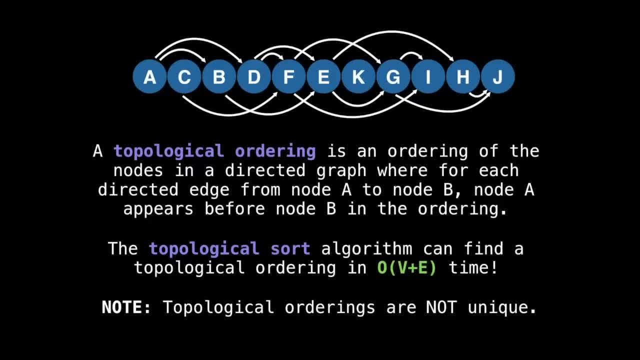 a topological ordering on a directed graph. A topological ordering is an ordering of nodes for which each edge from node A to node B, node A appears before node B in the ordering. If it helps, this is just a fancy way of saying that we can align all the nodes in the same. 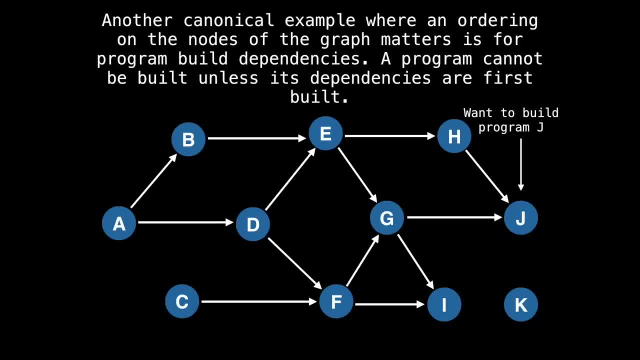 must first build program H and G, But to build those we also need. E and F, But to build those we also need, and so on. The idea is to first build the programs without dependencies and then move onwards from there. How do we find a valid ordering in which to build all the? 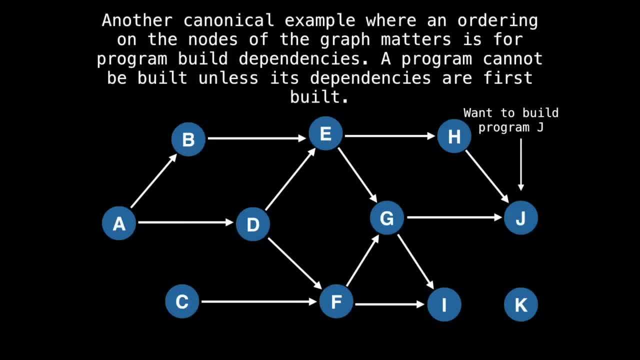 programs. Well, this is where top sort comes into play. One possible ordering might be to start by building a, then building C, B, D, F, E, G, H and then J. Notice that there are unused dependencies in this case, And that will happen. 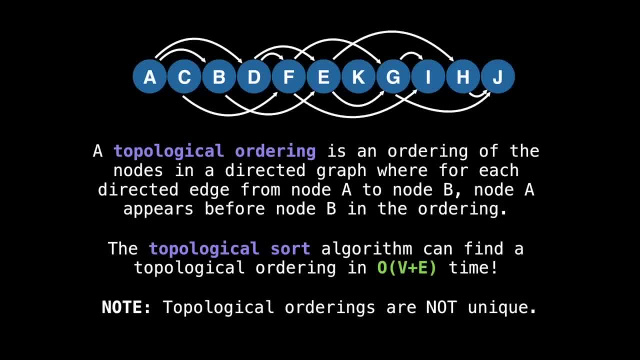 from time to time, which is fine. So, in conclusion, top sort is an algorithm which will give us a topological ordering on a directed graph. A topological ordering is an ordering of nodes for which each edge from node A to node B, node A, appears before node B in the ordering, If it helps. 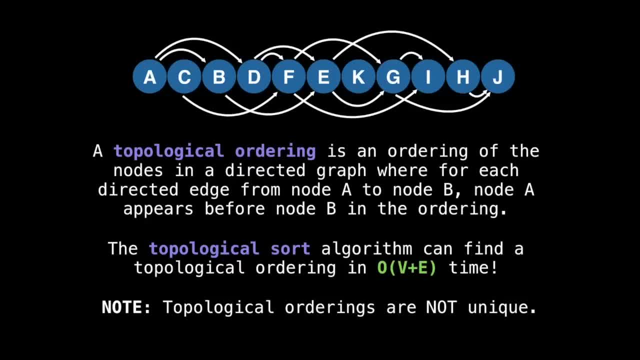 this is just a fancy way of saying that we can align all the nodes in a line and have all the edges pointing to the right. An important note to make is that topological ordering is not unique. As you can imagine, there are multiple valid ways to enroll in courses. 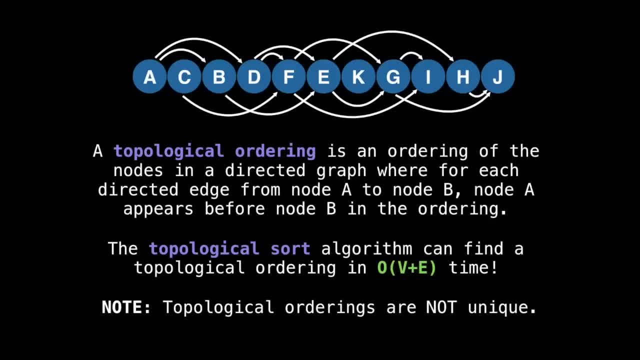 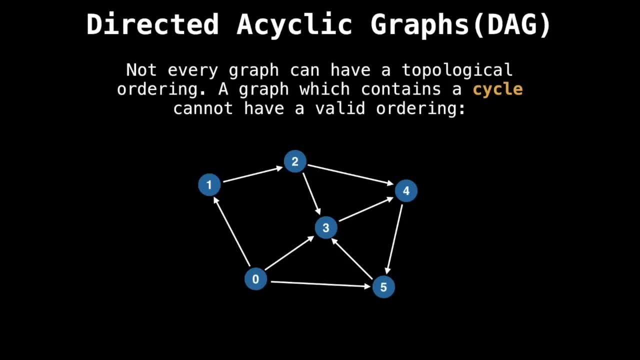 such that you can still graduate or to compile a program and its dependencies in a different order than you previously did. Sadly, not every type of graph has a topological ordering. For example, any graph with a directed cycle cannot have a valid ordering. Well, think. 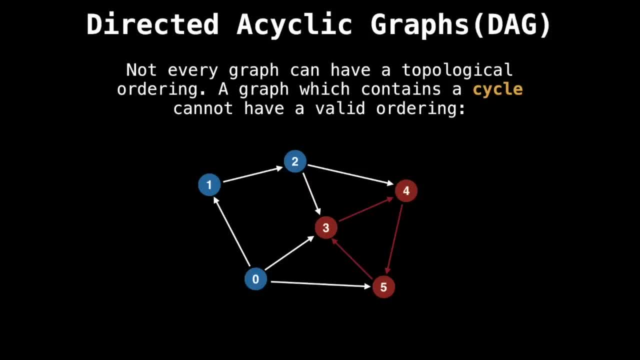 of why this might be true. There cannot be an order if there is a cyclic dependency. Since there is nowhere to start, every node in a cycle depends on another. So any graph with a directed cycle is therefore forbidden, The only graphs that have valid topological 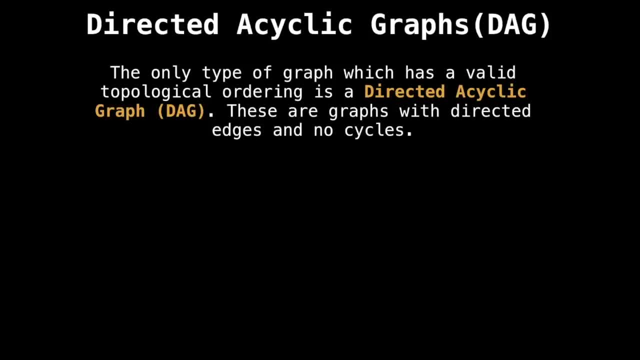 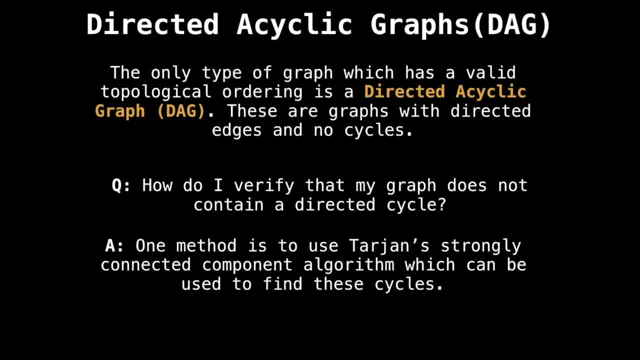 orderings are called directed acyclic graphs, That is, graphs with directed edges and no cycles. So a natural question to ask is: how do I verify that my graph does not contain a directed cycle? One method is to use tarjans, strongly connected component algorithm, which 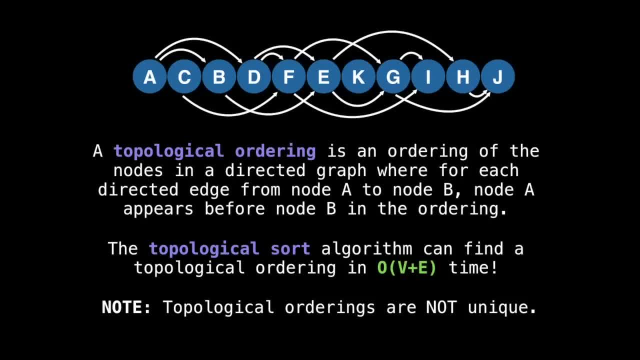 way, All the nodes in a line and have all the edges pointing to the right. An important note to make is that topological orderings are not unique. As you can imagine, there are multiple valid ways to enroll in courses such that you can still graduate or to compile. 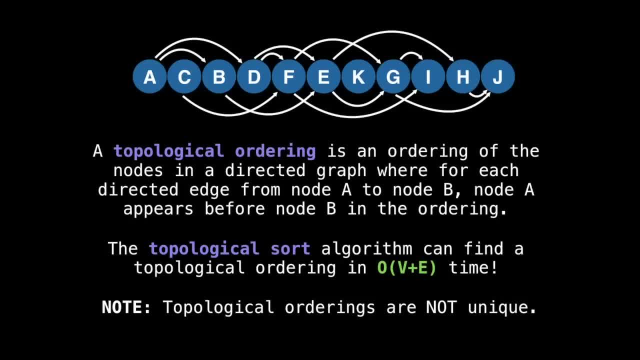 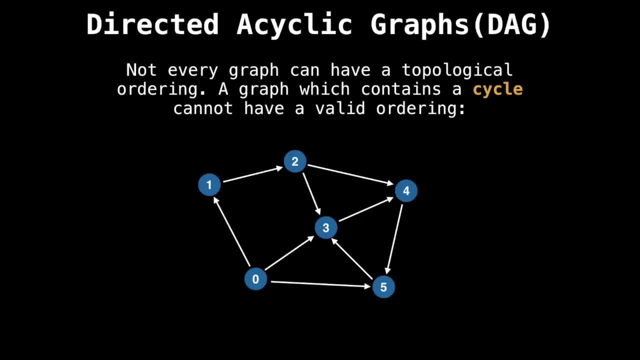 a program and its dependencies in a different order than you previously did. Sadly, not every type of graph has a topological ordering, So let's take a look at the topological ordering. The topological orderings are defined by the following. For example, any graph with a directed cycle cannot have a valid ordering. 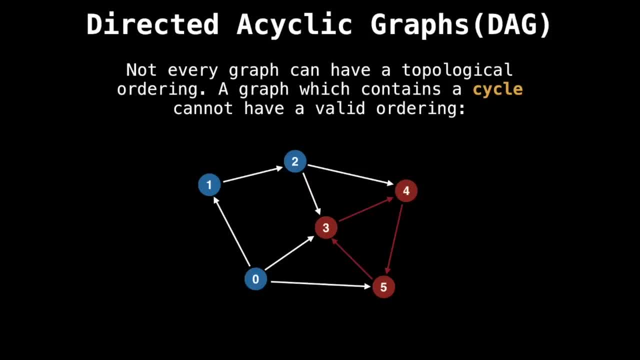 Well, think of why this might be true. There cannot be an order if there is a cyclic dependency, Since there is nowhere to start. every node in a cycle depends on another. So any graph with a directed cycle is therefore forbidden, The only graphs that have valid topological 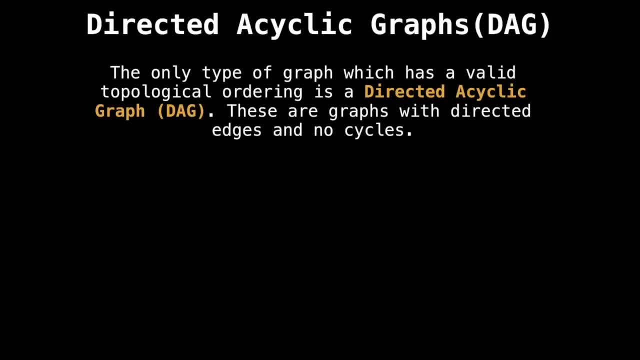 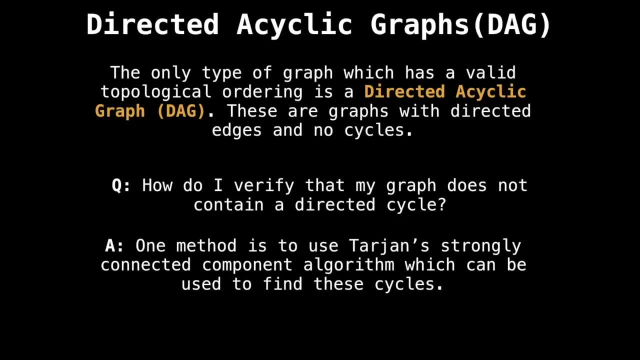 orderings are called directed acyclic graphs, that is, graphs with directed edges and no cycles. So a natural question to ask is: how do I verify that my graph does not contain a directed cycle? One method is to use tarjans, strongly connected component algorithm, which 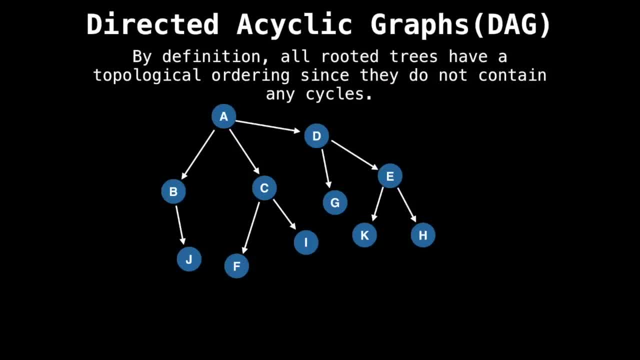 can detect these cycles. Another neat thing definitely worth mentioning is that the topological orderings of every tree have a topological ordering, since, by definition, trees do not have any cycles. An easy way to find a topological ordering with trees is to iteratively pick. 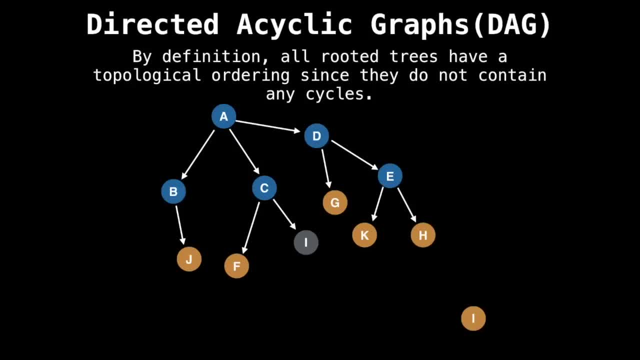 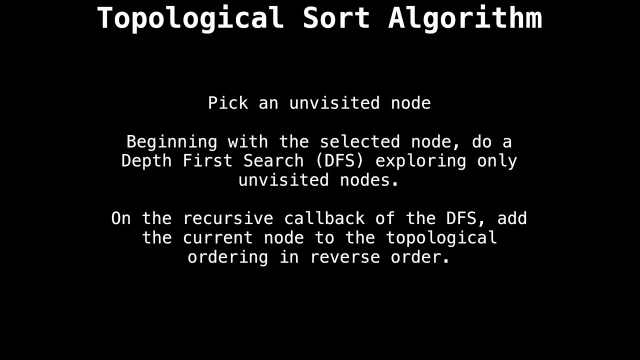 off the leaf nodes. It is like you're cherry picking from the bottom. it doesn't matter the order you do it. Once the root of a subtree has all grayed out children, then it becomes variable. This procedure continues until there are no more nodes left. So we know how. 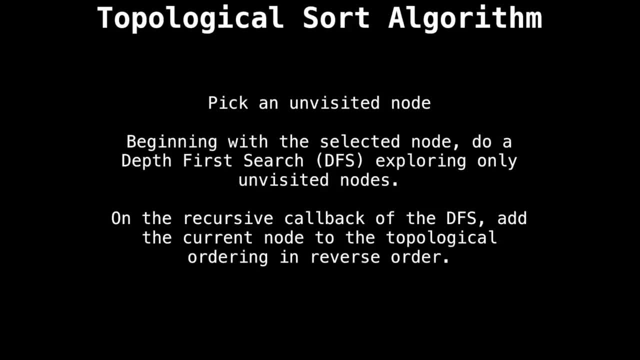 it works for trees. But how about general directed acyclic graphs? Well, the algorithm is also simple. Just repeat the following steps. First, find an unvisited node, it doesn't matter which. from this node, do a depth. first search: 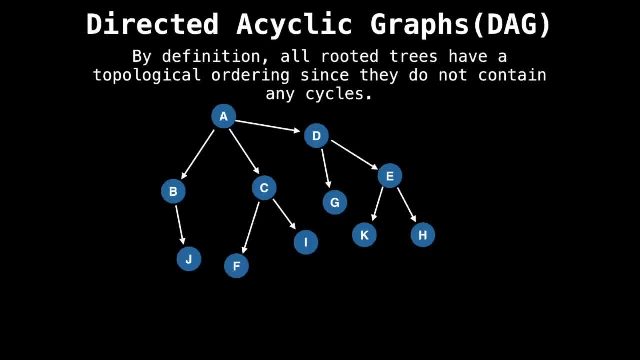 can detect these cycles. Another neat thing definitely worth mentioning is that every tree has a topological ordering, Since, by definition, trees do not have any cycles. An easy way to find a topological ordering with trees is to iteratively pick off the leaf nodes. It is like you're cherry picking from the bottom. it doesn't matter the order. 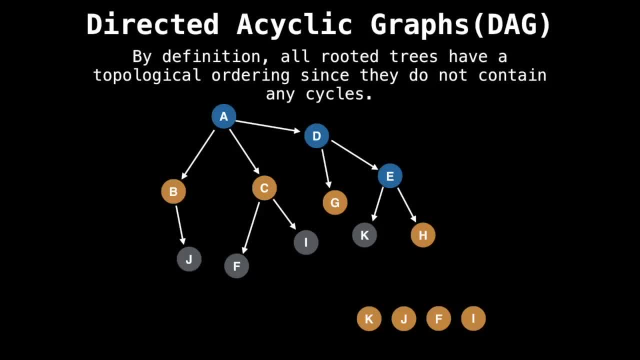 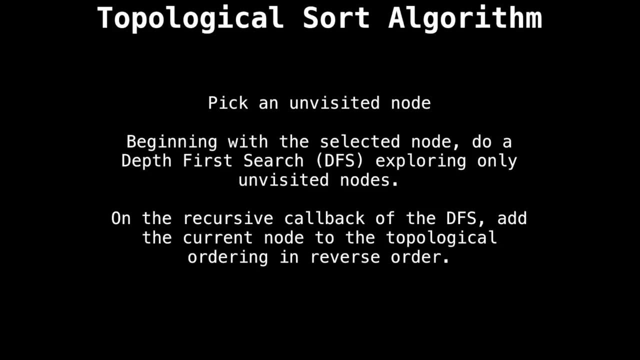 you do it Once the root of a subtree has all grayed out children, then it becomes available. This procedure continues until there are no more nodes left. So we know how it works with trees. But how about general directed acyclic graphs? Well, 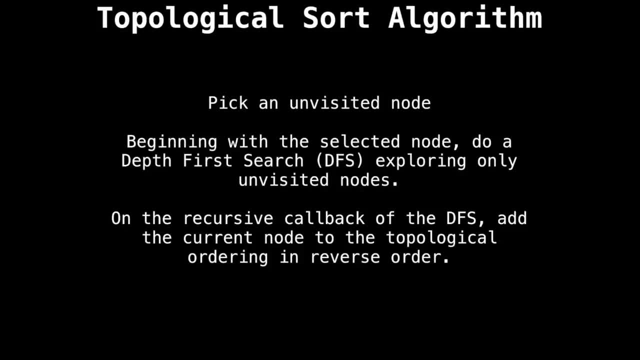 the algorithm is also simple. just repeat the following steps. First, find an unvisited node- it doesn't matter which from this node do a depth. first search, exploring only reachable unvisited nodes. On the recursive callback, add the current node to the top And then 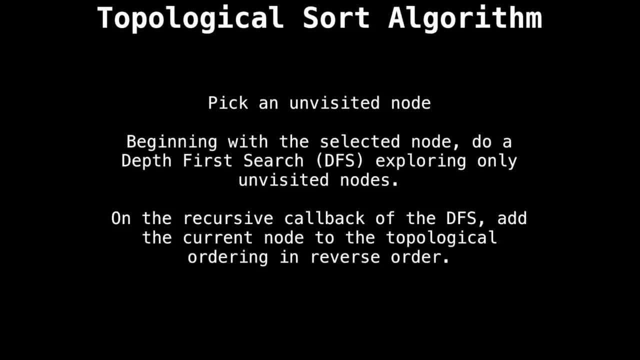 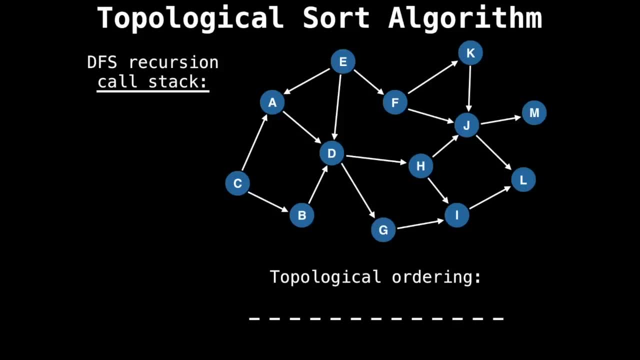 add a topological ordering in reverse order And that's it. Let's do an example and things will become much clearer. Here's a directed acyclic graph that we want to find one of many topological orderings for. As the algorithm executes, I'll be keeping track of the call. 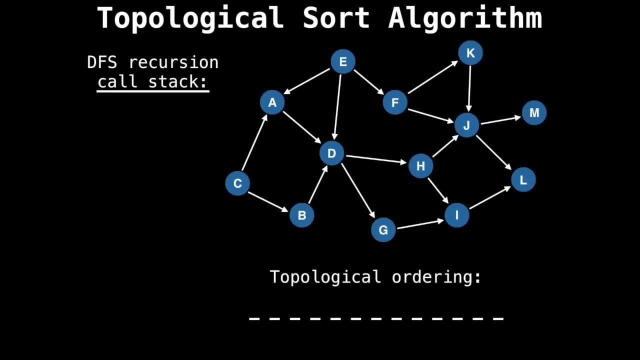 stack on the left hand side And in case you're curious, I will also be posting the current topological ordering at the bottom bottom of the screen. The first step is going to be to pick an unvisited node. I'm going to pick node h arbitrarily. Now we do a depth first search out towards from H and all possible. 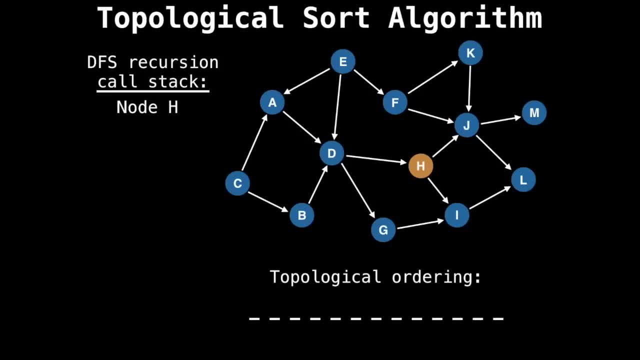 directions, exploring where we can, Let's go to node j. Now that I'm at node j, I'm going to keep exploring, And so let's go to M. Now that we're at M, we're going to go to M. there's nowhere left to go, So we backtrack and add M as last element to the topological. 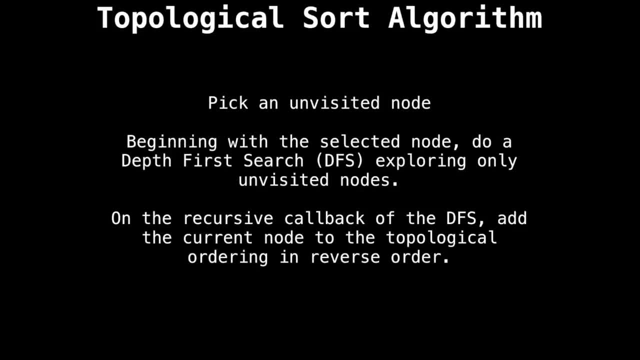 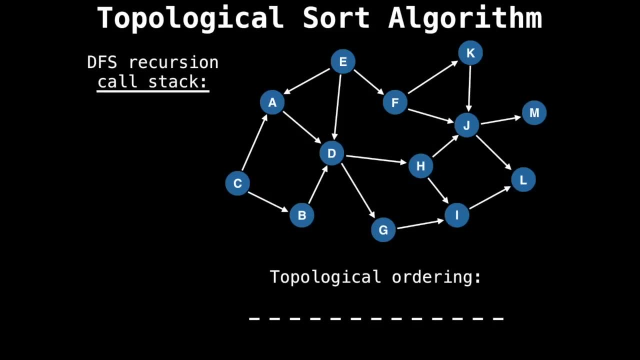 Exploring only reachable unvisited nodes. on the recursive callback, add the current node to the topological ordering in reverse order And that's it. Let's do an example and things will become much clearer. Here's a directed acyclic graph that we want to find. 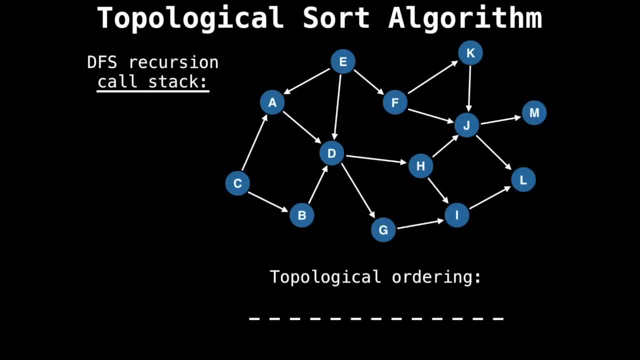 one of many topological orderings, for, As the algorithm executes, I'll be keeping track of the call stack on the left hand side And, in case you're curious, I will also be posting the current topological ordering at the bottom of the screen. The first step is going to be to pick an unvisited node. I'm 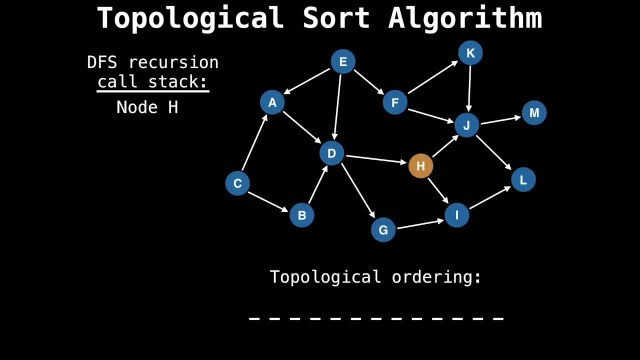 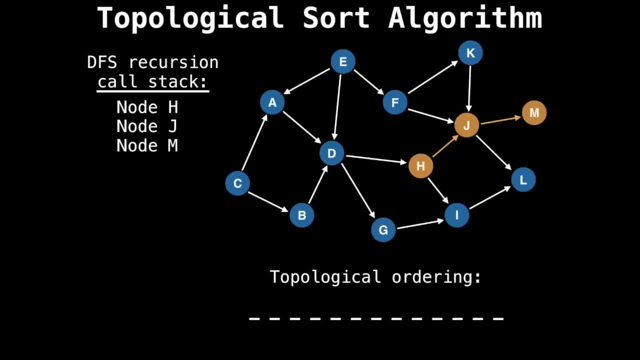 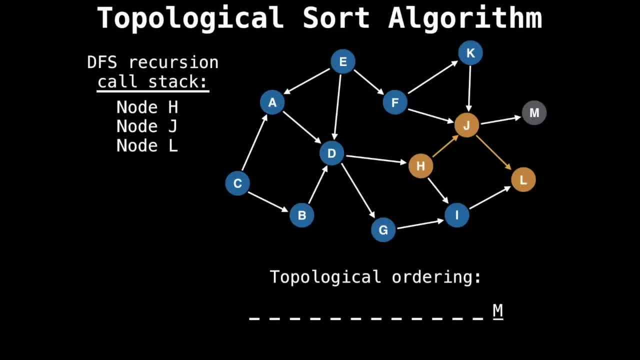 we still need to explore L. Now we're at L Now backtrack because there's nowhere left to go. Also backtrack because there's nowhere left to go. Also backtrack because there's nowhere left to go. So backtrack again and add it to the ordering. Notice that the stacked frames Again I popped off. 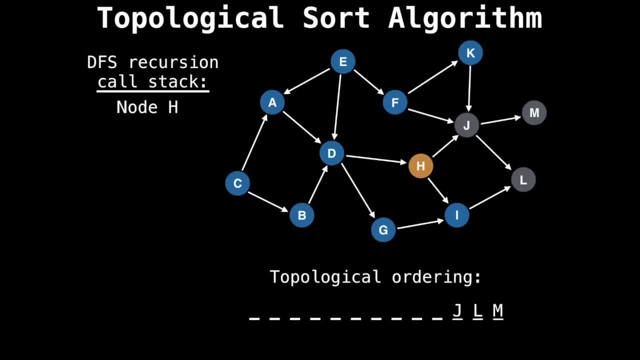 the call stack, as I request. Now we're at H and we still need to visit node I. So now we're at node I and from node AI we try and visit node L, But then we figure out that node l is already visited. 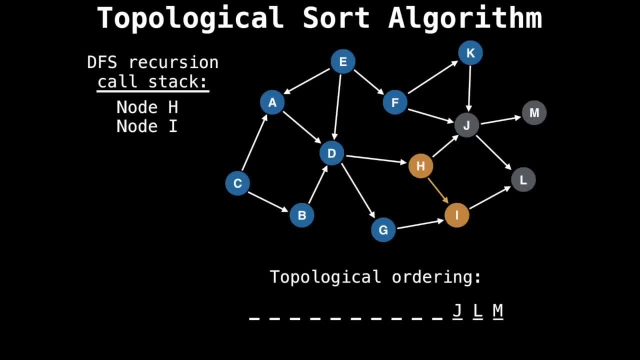 So we don't go there. Backtrack, backtrack again, add AI to the ordering and mark it as explored And finally we're back at h. As you saw, selecting a random unvisited node made us visit a subsection of the graph. We continue this process until 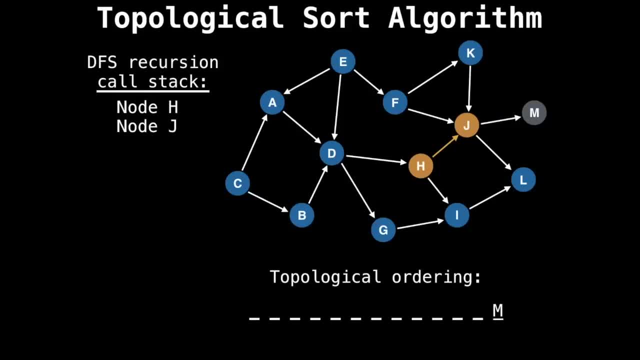 ordering: Still at J. we still need to explore L. Now. we're at L, Now backtrack because there's nowhere left to go. Also backtrack at J and add it to the ordering. Notice that the stack frames are getting popped off the call stack as I recurse. 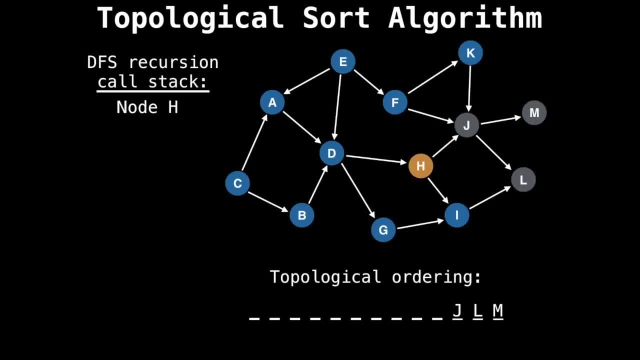 Now we're at h and we still need to visit node i. So now we're at node i and from node i we try and visit node l, But then we figure out that node l is already visited, So we don't go there. Backtrack, backtrack again. add i to the ordering and mark it as explored. 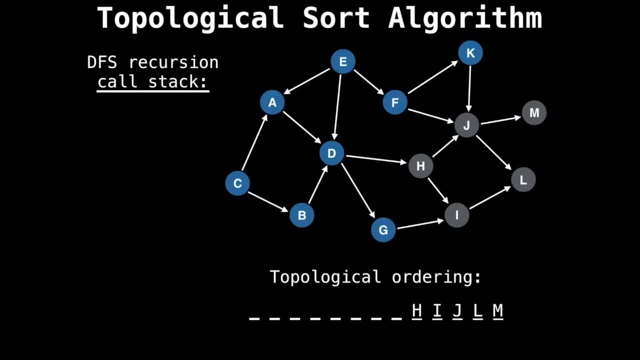 And finally we're back at h. As you saw, selecting a random unvisited node visited node made us visit a subsection of the graph. We continue this process until all nodes are visited. The next node I'm going to randomly pick is going to be node E In. 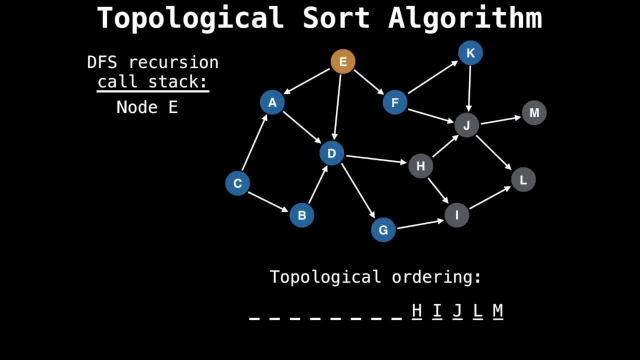 the interest of time and simplicity, I will let the animation run and you can follow along. Note that if you try and predict the next few values and topological ordering, you may not get the same values as me, Because topological orderings are not unique. However, this does. 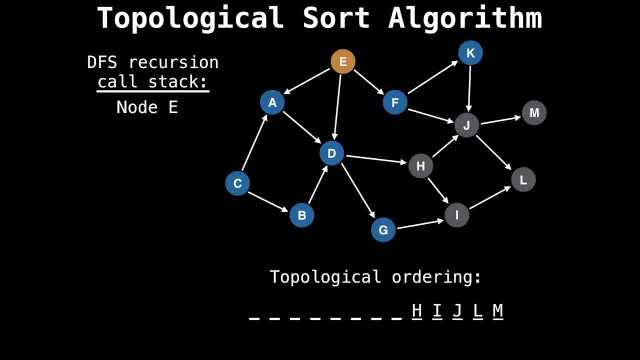 not mean you are incorrect. Alright, I will let the animation play and try and follow along. So that's it for that subsection of the graph. The next node I'm going to pick is going to be node C to visit. So we start at node C and explore this subsection of the graph. 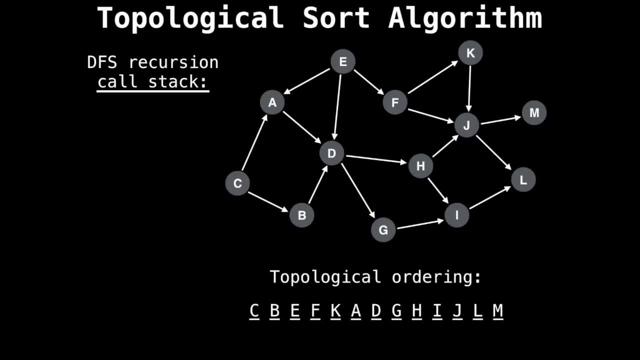 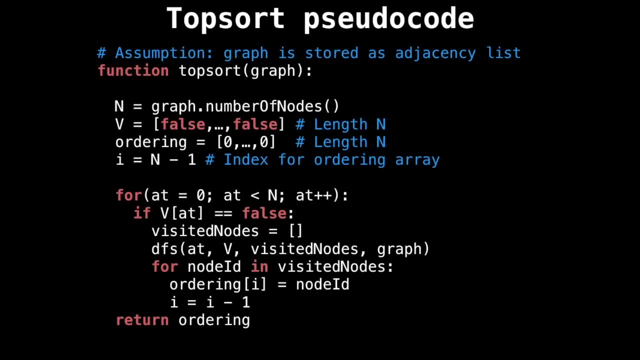 Now that all nodes are visited, we have a valid topological order. So now that we understand how the algorithm works, what does the code actually look like? Here's some pseudocode for top sort. Let's walk through it real quick. The first thing: 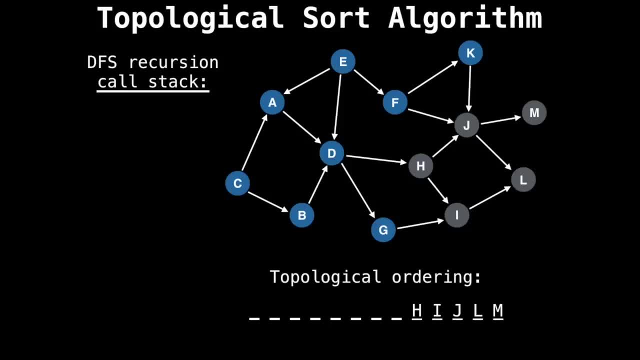 all nodes are visited. The next node I'm going to randomly pick is going to be node E. In the interest of time and simplicity, I will let the animation run and you can follow along. Note that if you try and predict the next few values and topological ordering, you may. 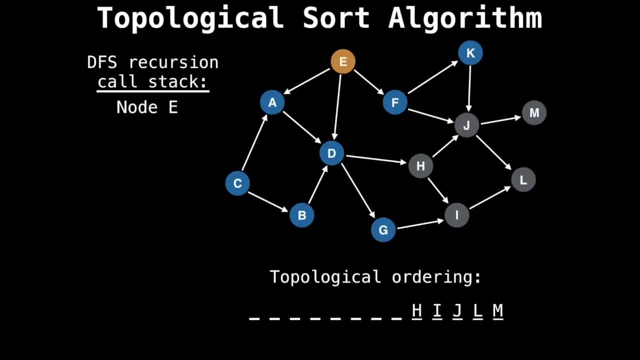 not get the same values as me Because topological orderings are not unique. However, this does not mean you are incorrect. Alright, I will let the animation play and try and follow along. So that's it for that subsection of the graph. The next node I'm going to pick is going to: 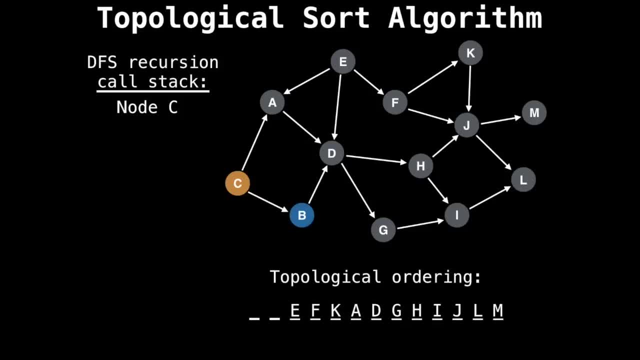 be node C to visit. So we start at node C and explore this subsection of the graph. Now that all nodes are visited, we have a valid topological ordering at the bottom of the screen. So now that we understand how the algorithm works, what does the code actually? 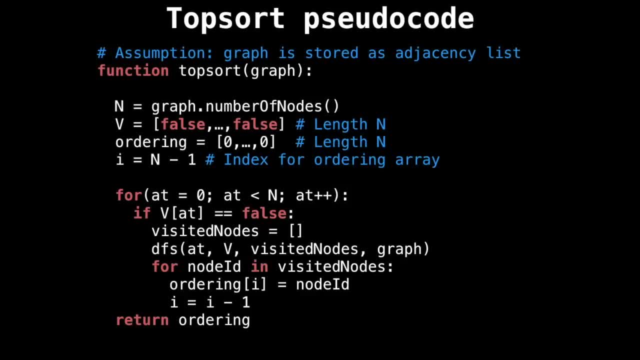 look like. Here's some pseudocode for top sort. Let's walk through it real quick. The first thing I do is I get the number of nodes from the graph, which I assume is passed in as an adjacency list from the function. Then I declare an array called v, short for the. number of nodes that are visited. So I get the number of nodes from the graph, which I assume is passed in as an adjacency list from the function. Then I declare an array called v short for the number of nodes that are visited. So now that we understand how. 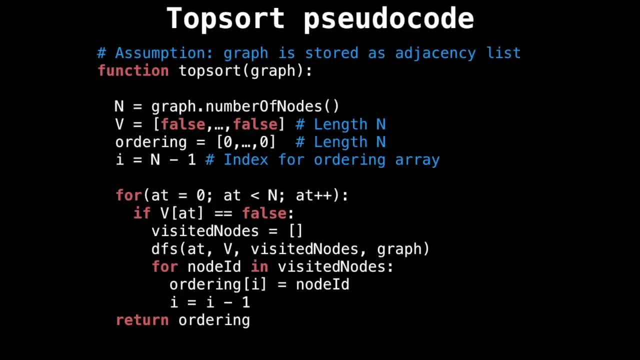 the algorithm works. let's explore this subsection of the graph. Here's some pseudocode for this subsection of the graph. Here's some pseudocode for visited, which tracks whether a node has been visited or not. The next array, called orderings, is the result that 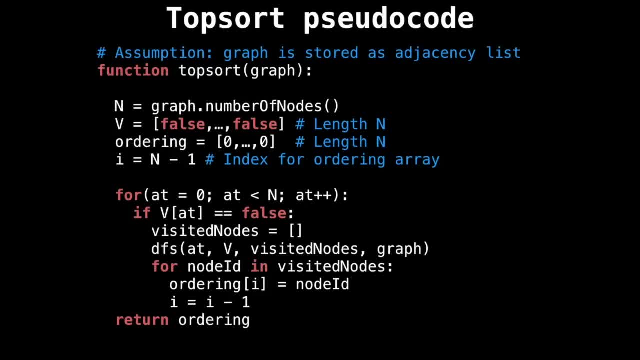 will be returning from this function. This is equivalent to the ordering at the bottom of the screen in the last slides. Associated with the orderings array is the index i, which tracks the insertion position of the next element in the topological ordering, As you. 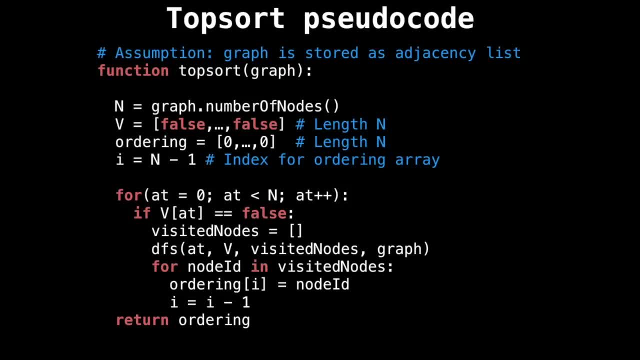 I do is I get the number of nodes from the graph which I assume is passed in as an adjacency list from the function. Then I declare an array called V, short for visited, which tracks whether a node has been visited or not. Alright, so now that we have the number of nodes from the graph which I assume is passed, 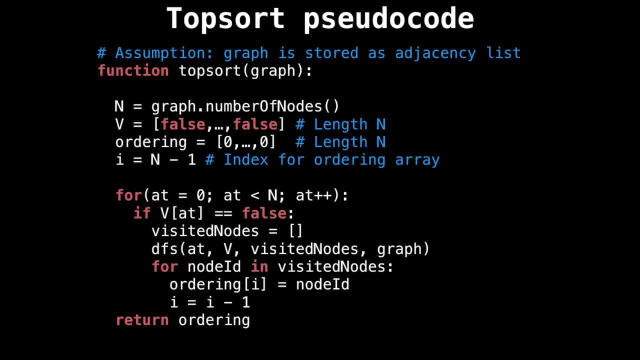 in as an adjacency list from the function. then I declare an array called V, short for visited, which tracks whether a node has been visited or not. The next array, called orderings, is the result that will be returning from this function. 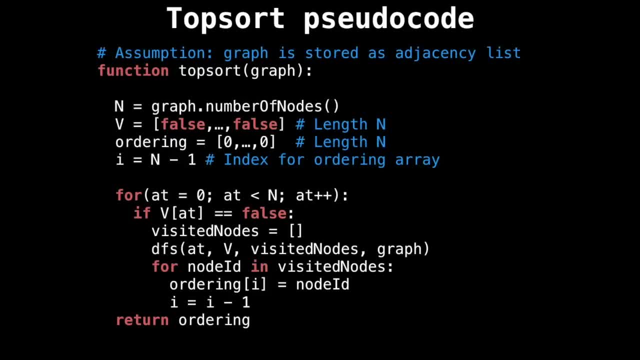 This is equivalent to the ordering at the bottom of the screen in the last slides. Associated with the orderings array is the index i, which tracks the insertion position of the next element in the topological ordering. As you have been seeing in the slides, we insert elements backwards, which is why i 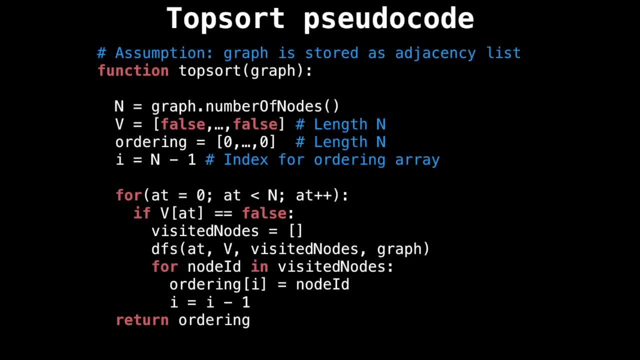 starts at n. Next we're ready to enter a for loop to iterate over all the nodes in our graph. The loop variable called at tracks the id of the node we're currently processing. I then check if we're on a visited node, because those are the only ones we care about. 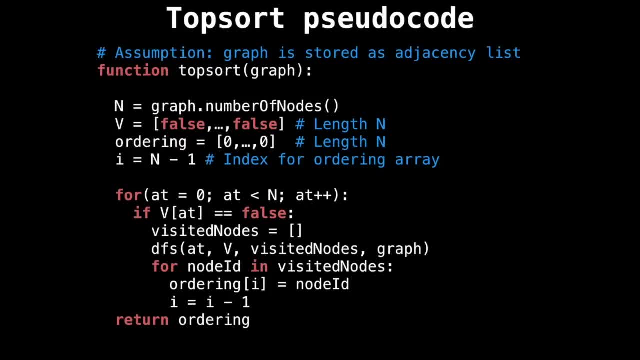 Then I start a depth first search. notice that before I do, I initialize an array called visited nodes which I pass into the depth first search method to add the nodes as we find them. Then, after that's done, after the depth first search is finished, I look at the nodes we 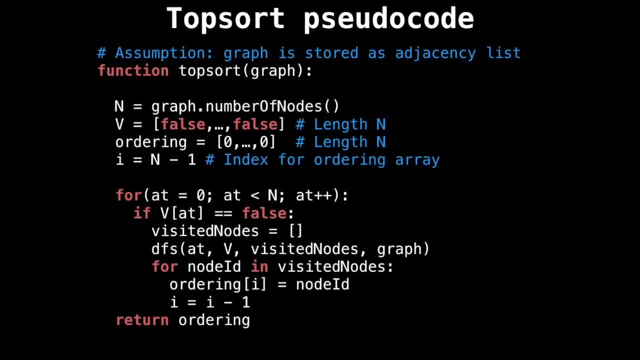 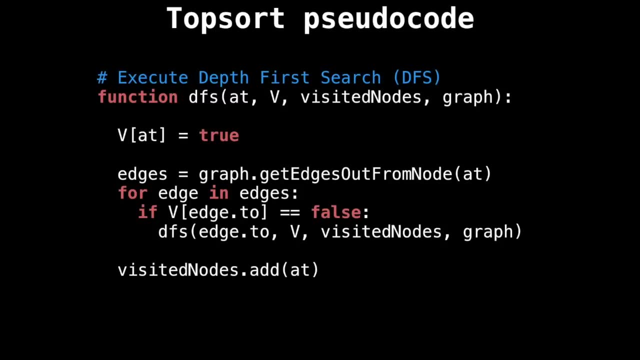 found in our visited nodes array and then add them to the ordering. Now the last bit we need to look at is the depth first search method itself. depth first search method is very simple. All I do is I mark the node we're currently at to be visited. then, for each edge going outwards from the node we're 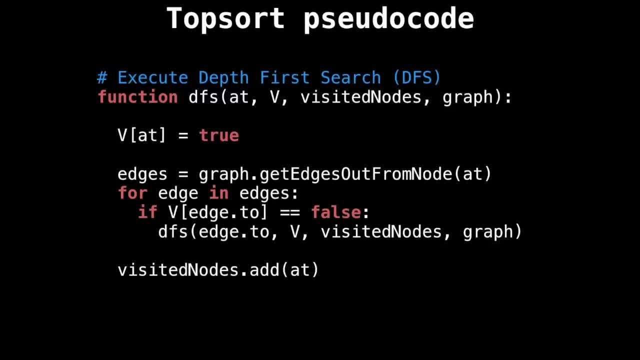 at I make sure the destination node is unvisited, then call the method again, but this time on the destination node, On the callback when the method returns. this is when we're stuck and need to backtrack. so this is where I add the current node. 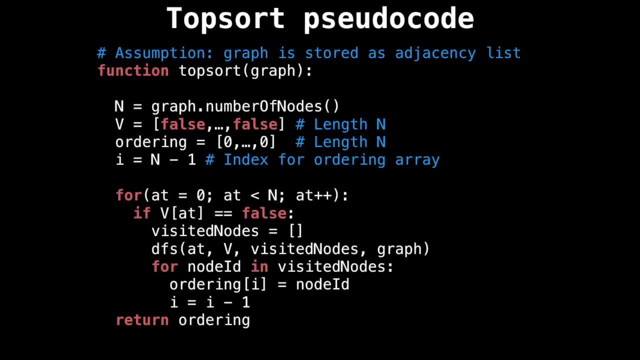 have been seeing, this is the index i which tracks the insertion position of the next element in the topological ordering. As you have been seeing, this is the index i which tracks the MansionType first element and then the correct answer comes: River beer. 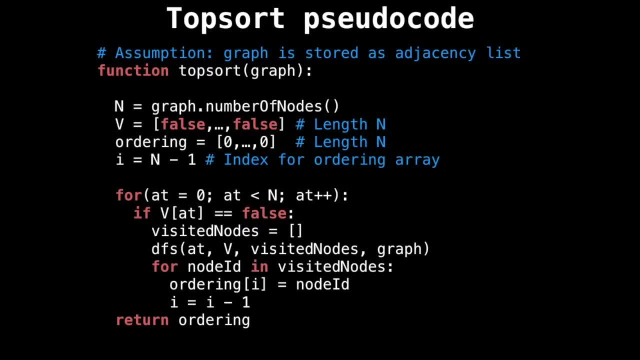 and peas. The index i- or the problem here- has the Iím function in the first line of the graph. If we want an index, we have to remember to insert input at id a. then let's add input at amGrad RuggerY, which is the exact Sci Doctor failed setting. Also, it is 홀. 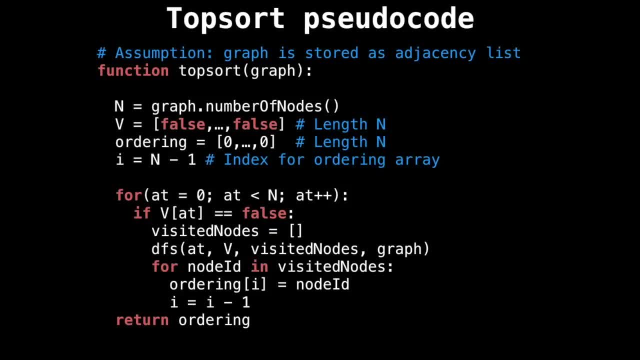 已經 consegue entry into eine Solideach, Die Z matte element comedy開心. We need to do one more thing now After Lee. here a few things could be a little bit tricky, but the typical logic is that an initial order will be issued later in the original component expected at the NAG property. 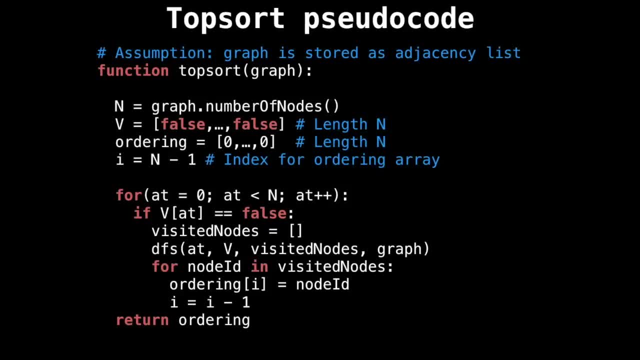 If you're interested, let me know if you implemented it. later on processing I then check if we're on a visited node, because those are the only ones we care about. Then I started depth first search. notice that before I do I initialize an array. 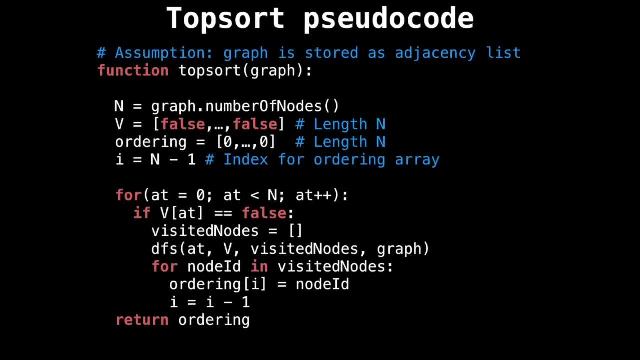 called visited nodes, which I pass into the depth first search method to add nodes as we find them. Then, after that's done, after the depth first search is finished, I look at the nodes we found in our visited nodes array and then add them to the ordering. Now. 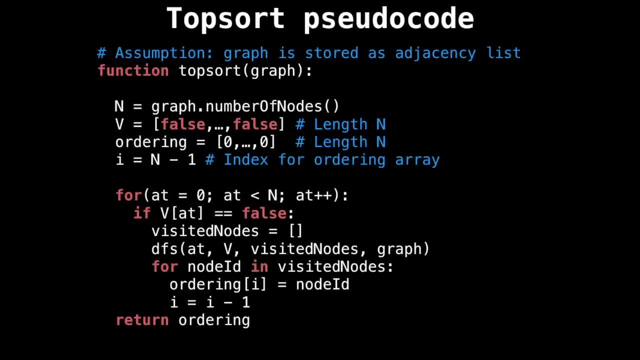 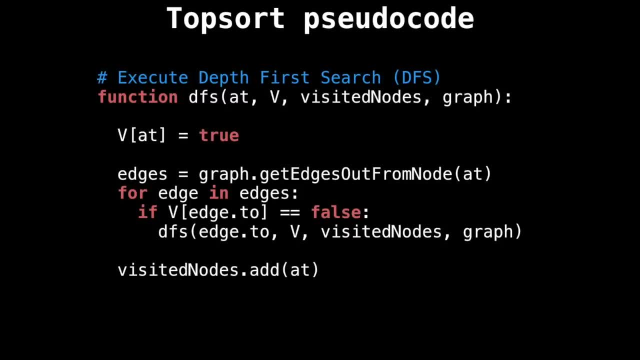 the last bit we need to look at is the depth first search method itself. The depth first search method is very simple. All I do is I mark the node we're currently at to be visited. Then, for each edge going outwards from the node we're at, I make sure the destination node is unvisited. 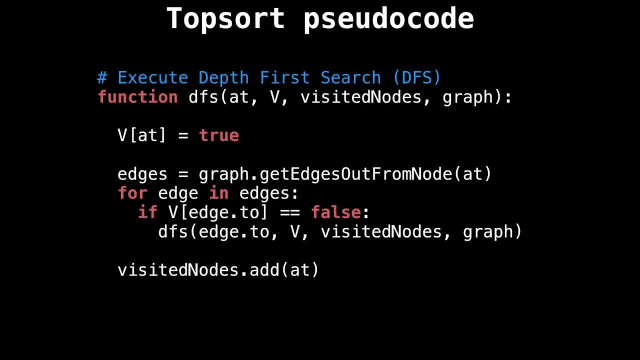 then call the method again, but this time on the destination node, On the callback when the method returns. this is when we're stuck and need to backtrack. So this is where I add the current node to the visited nodes array, which is essentially the output for. 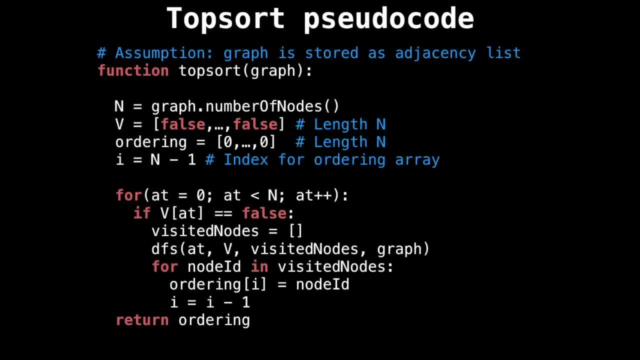 this method Back to the top sort method. Now that we understand how the top sort algorithm works, there's a neat optimization we can do to improve the performance in terms of both time and space. Notice that every time we enter the inner if statement block, we need to allocate memory for an array that. 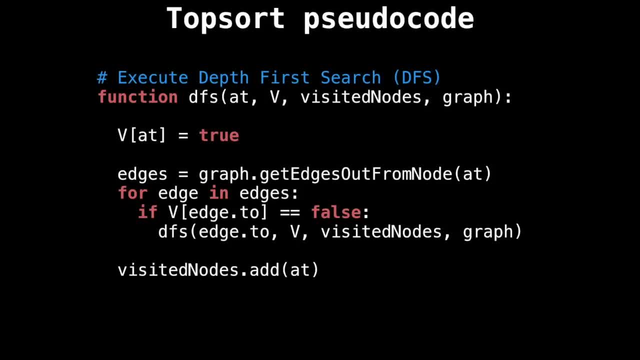 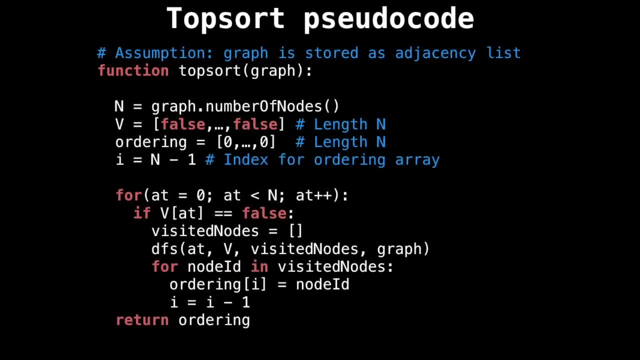 to the visited nodes array, which is essentially the output for this method. Back to the top sort method. Now that we understand how the top sort algorithm works, there's a neat optimization we can do to improve the performance in terms of both time and space. Notice that. 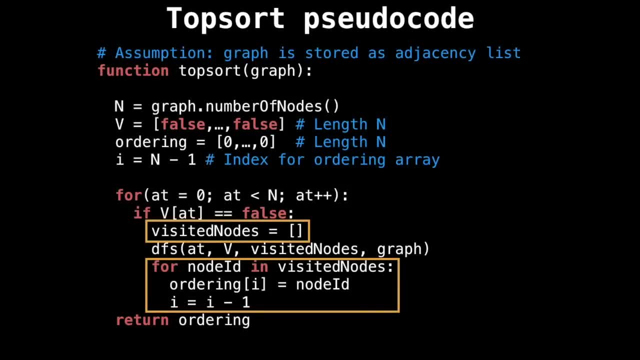 every time we enter the inner if statement block we need to allocate memory for an array. that array is filled with node IDs and then we iterate over them to place them inside the orderings array. But how about we just directly insert found node inside the orderings array instead? 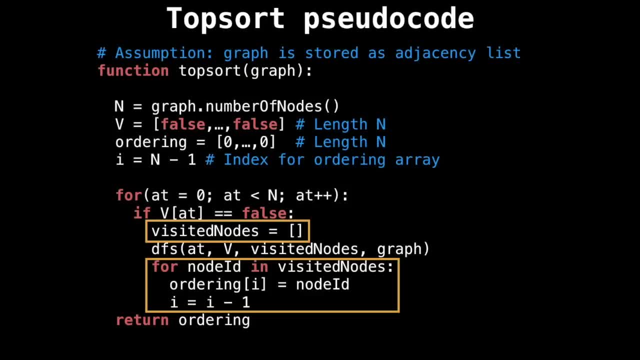 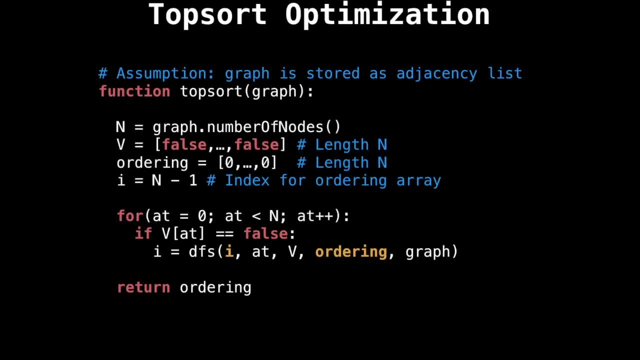 of allocating memory and doing this additional work. Well, that's exactly what we're going to do Here. I got rid of the unnecessary array and modify the depth first search method to return the next valid insertion position in the orderings array. Now we need to power. 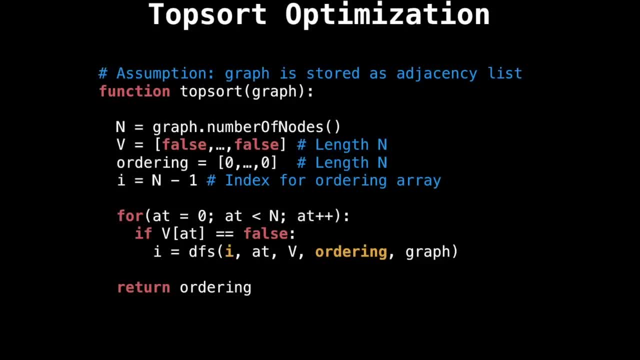 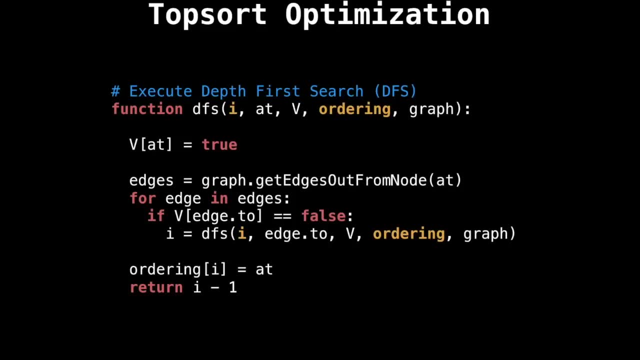 in the index i and the orderings array so that it can be filled directly inside the depth first search method, Inside the new depth first search method. one thing that changed is that now we have a return value and we're passing in some additional variables. 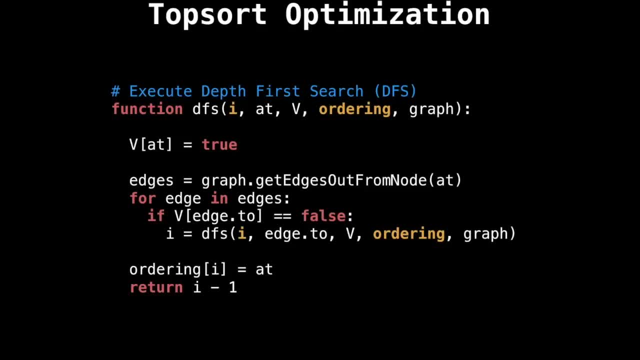 Notice that instead of adding the current node to the visitor nodes array, as we were doing before, now, we simply insert that node directly inside the orderings array. The orderings array is no longer an index i, but an index i minus one. So related to the topic of topological 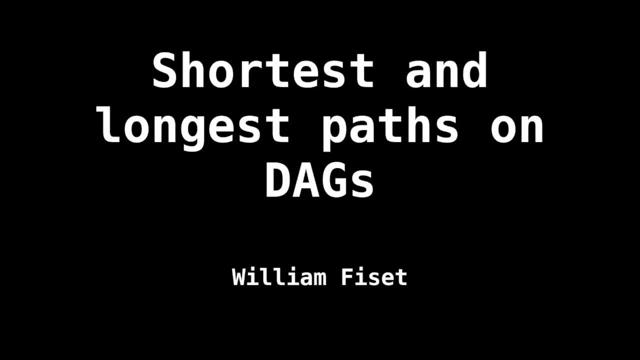 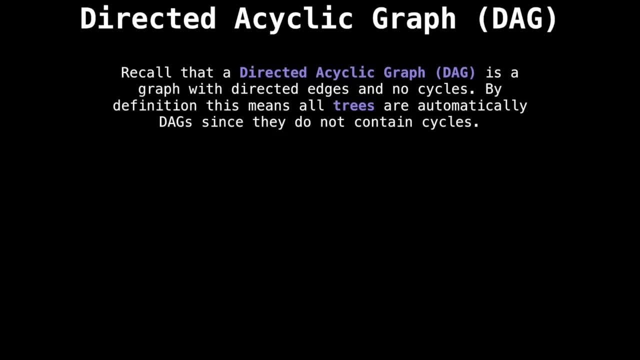 orderings is the topic of shortest and longest paths. on directed acyclic graphs, Recall that a directed acyclic graph is a graph with directed edges and no cycles. By definition, this means that all trees are automatically directed acyclic graphs since they do not contain any cycles. Here is a. 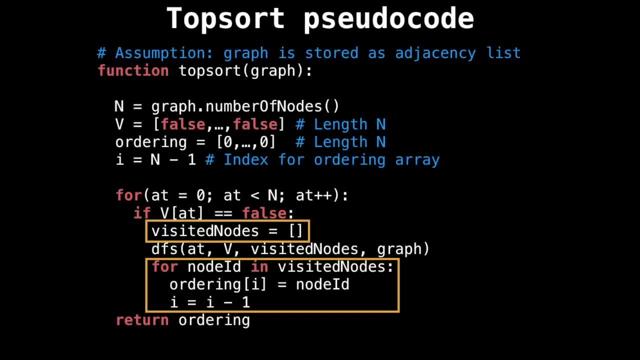 array gets filled with node IDs and then we iterate over them to place them inside the orderings array. But how about we just directly insert found node? then we add the node inside the orderings array, instead of allocating memory and doing this additional. 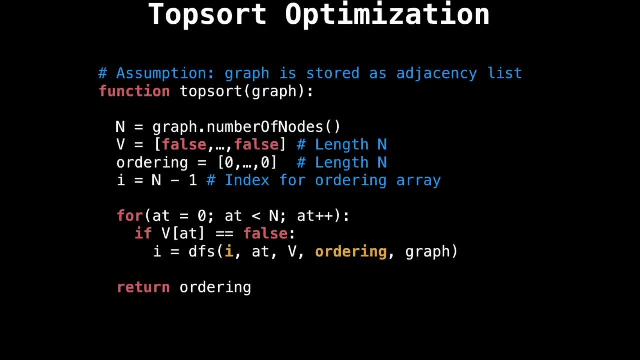 work. Well, that's exactly what we're going to do Here. I got rid of the unnecessary array and modify the depth. first search method to return the next valid insertion position in the orderings array. Now we need to pass in the index i and the orderings array. so 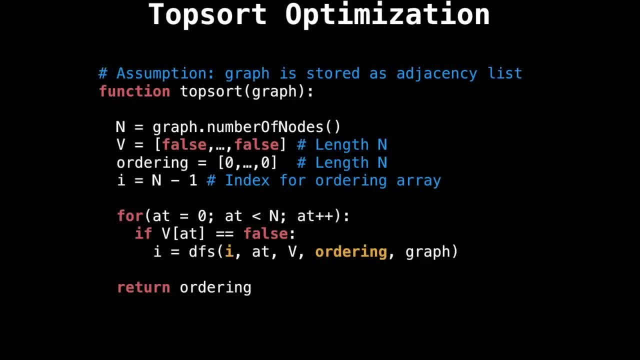 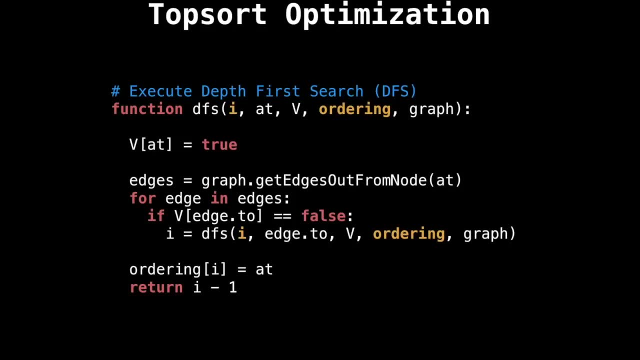 that it can be filled directly inside the depth first search method, Inside the new depth first search method. one thing that changed is that now we have a return value and we're passing in some additional variables. Notice that instead of adding the current node to the visitor nodes array, as we were doing before now, we simply insert that node. 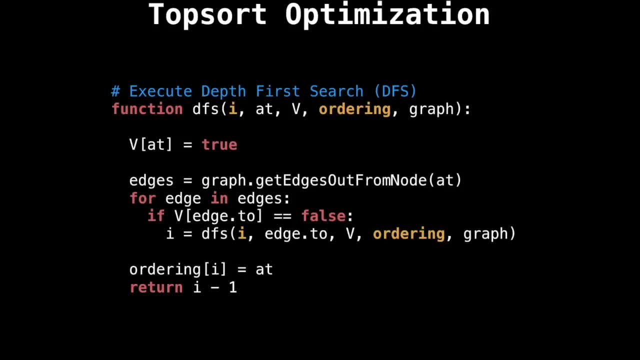 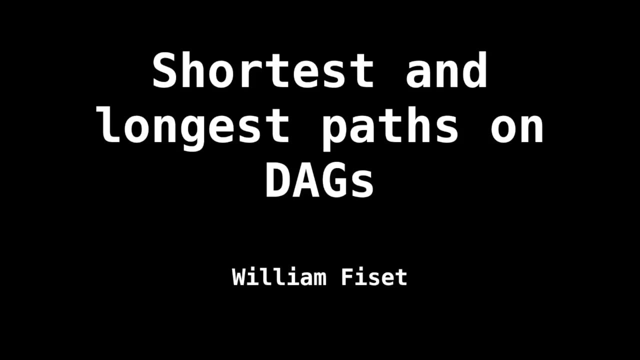 directly inside the orderings array. The last thing to do is to return i minus one, because the index of the current insertion position is no longer the current insertion position, No longer index i, but index i minus one, So related to the topic of topological orderings. 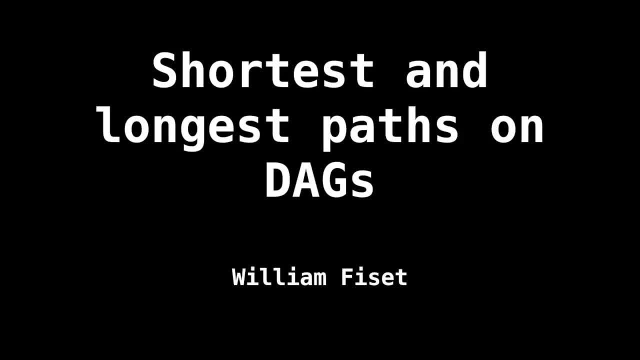 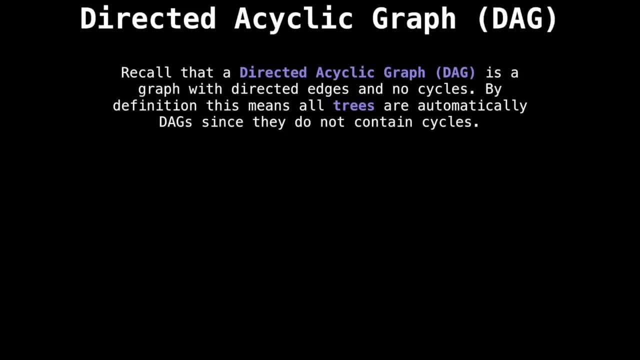 is the topic of shortest and longest paths. on directed acyclic graphs, Recall that a directed acyclic graph is a graph with directed edges and no cycles. By definition, this means that all trees are automatic Directed acyclic graphs, since they do not contain any cycles. Here is a graph. My question: 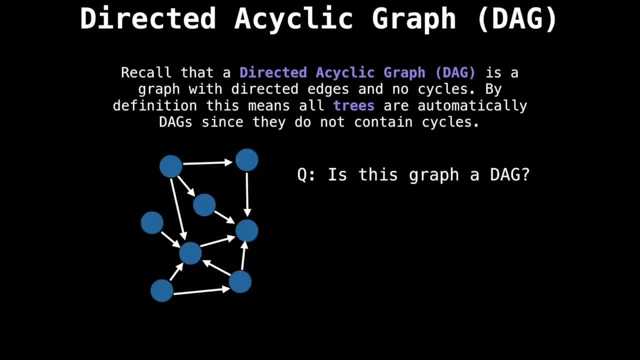 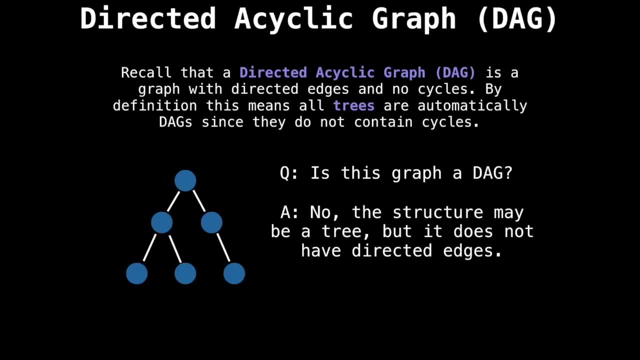 to you is: is this graph a directed acyclic graph? And the answer is yes, But what about this structure? I'll give you a moment to think about it. The answer is no, because this graph has undirected edges as opposed to directed edges. 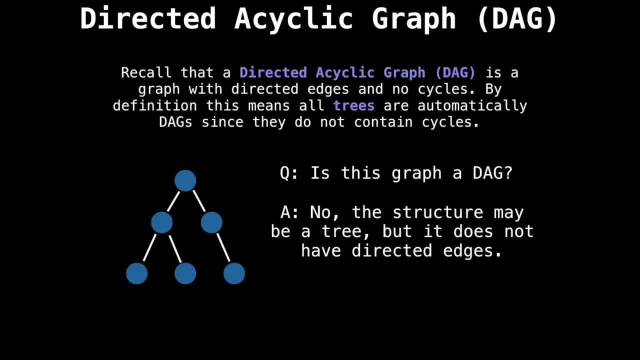 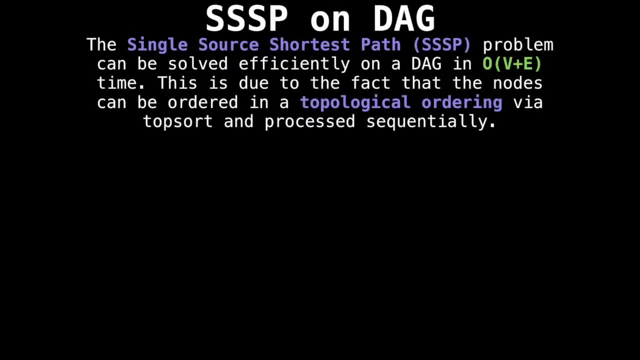 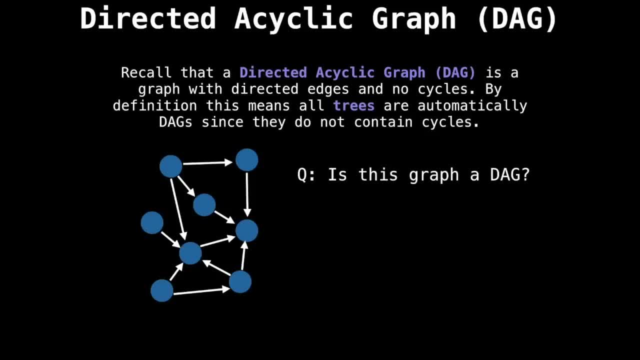 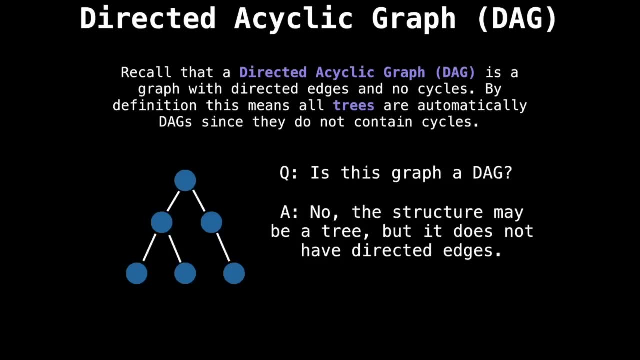 graph. My question to you is: is this graph a directed acyclic graph? And the answer is yes, But what about this structure? I'll give you a moment to think about it. The answer is no, because this graph has undirected edges as opposed to directed edges. The graph 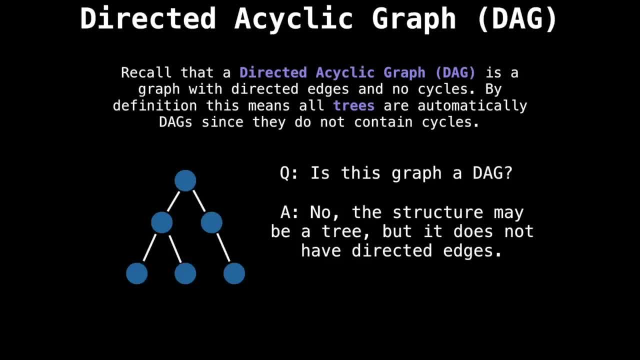 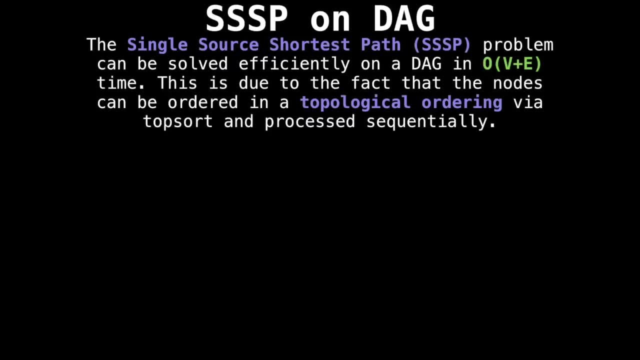 may be a tree, but directed edges are a requirement for a directed acyclic graph. What's really great about working with directed acyclic graphs is that the single source shortest path problem can be solved very efficiently, In fact, in linear time. The next fastest single source shortest path algorithm is dexterous algorithm, which may 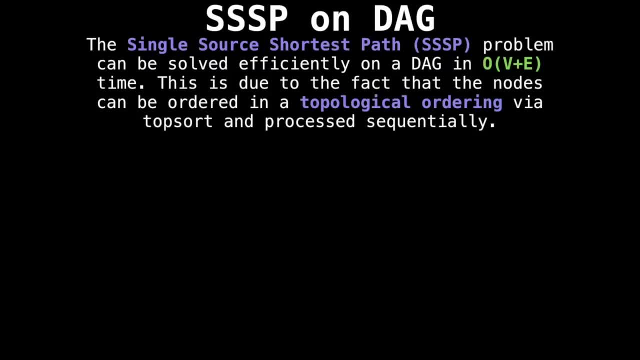 not work if there are negative edge weights. This algorithm I'm about to show you is faster and doesn't care about positive or negative edge weights. The essence of the algorithm is that it finds a topological ordering on the graph using the top sort algorithm. we 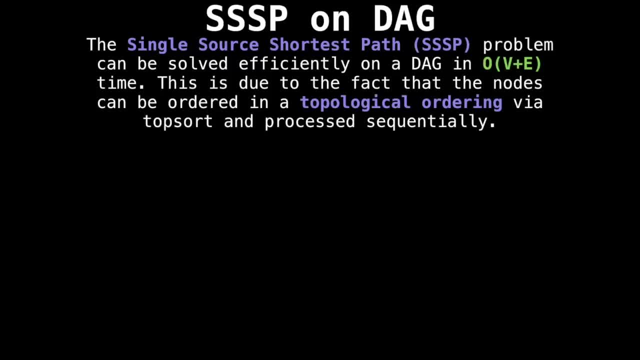 saw in the last video and processes each node. This algorithm is used sequentially to get the shortest path by relaxing each edge. as it is seen, Relaxing edge simply means updating to a better value if a shorter path can be obtained using the current edge. Suppose this is the graph we're working with, you can verify? 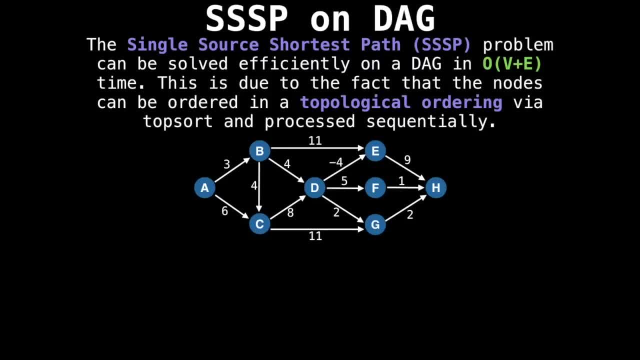 that it is, in fact, a directed acyclic graph. What we wish to do is find the shortest path from node A to all other nodes in the graph. In order to do this, the first thing we'll want to do is generate a topological ordering of the nodes of this graph using the top sort. 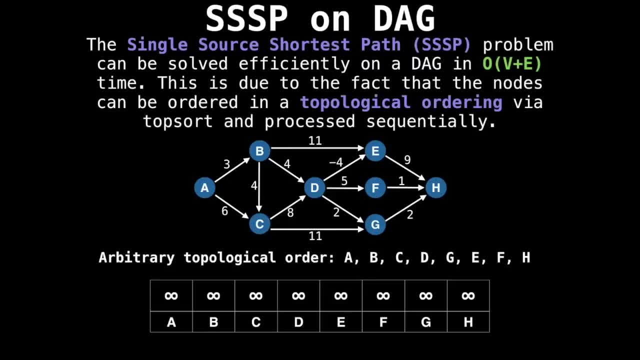 algorithm. Below I have selected an arbitrary topological ordering, which is the order we will process the nodes in this graph. I'm also displaying the current best distance to each node at the bottom of the screen. This is the first step of the algorithm is to set the distance to the starting node to 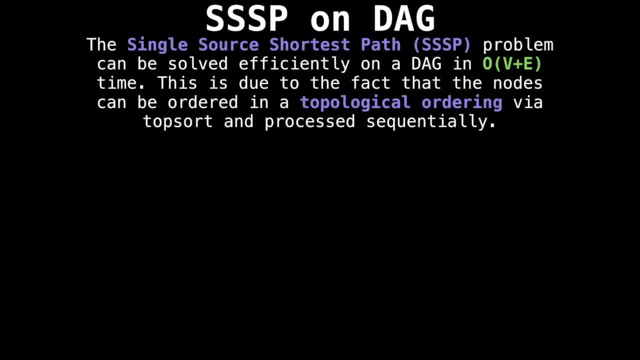 What's really great about working with directed acyclic graphs is that the single source shortest path problem can be solved very efficiently. In fact, in linear time. the next fastest single source shortest path algorithm is Dexter's algorithm, which may not work if there are 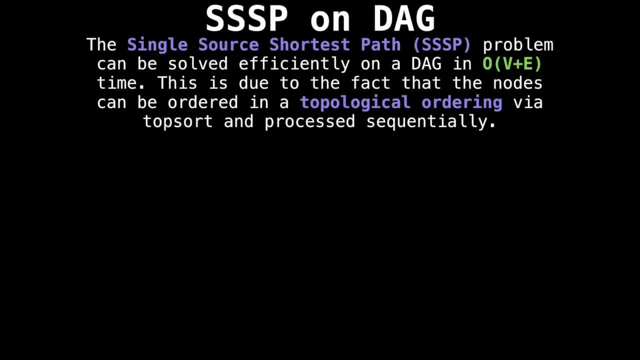 negative edge weights. This algorithm I'm about to show you is faster and doesn't care about positive or negative edge weights. The essence of the algorithm is that it finds a topological ordering on the graph using the top sort algorithm we saw in the last. 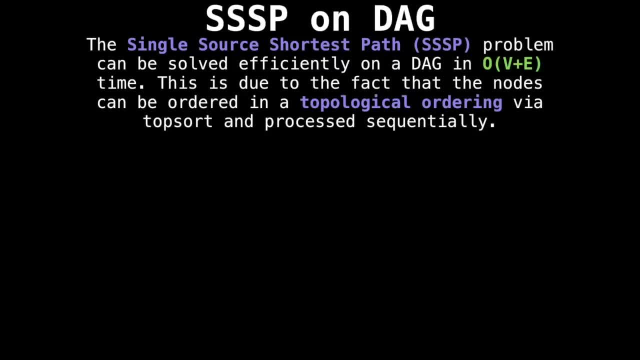 video and processes each node sequentially to get the shortest path by relaxing each edge. as it is seen, Relaxing an edge simply means updating to a better value if a shorter path can be obtained using the current edge. Suppose this is the graph we're working with. 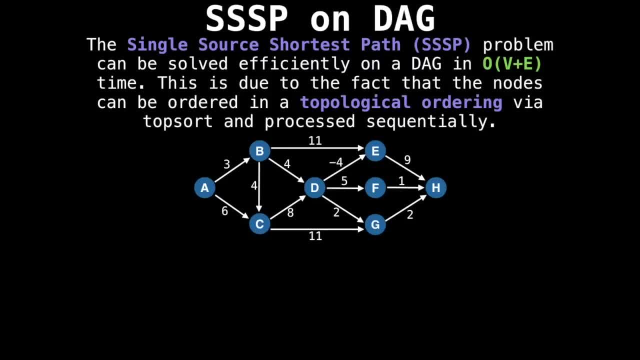 you can verify that it is, in fact a directed acyclic graph. What we wish to do is find the shortest path from node A to all other nodes in the graph. In order to do this, the first thing we'll want to do is generate a topological ordering of the 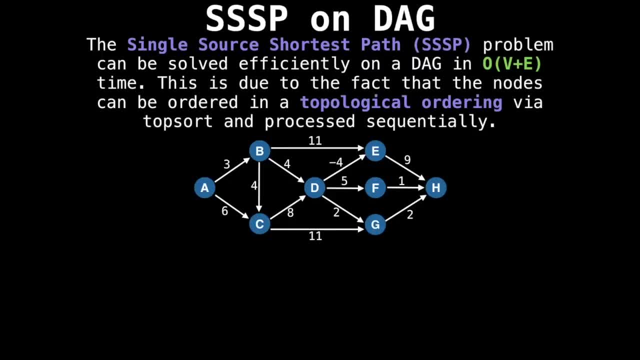 nodes of this graph using the top sort algorithm. Below I have selected an arbitrary topological ordering, which is the order we will process the nodes in this graph. I'm also displaying the current best distance to each node at the bottom of the screen, which are all currently. 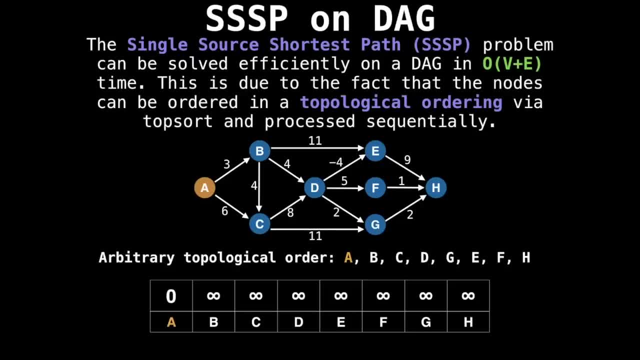 set to infinity. The first step of the algorithm is to set the distance to the starting node to be zero. In this case, since a is the starting node, its initial distance is zero because we're already there From a we want to visit. 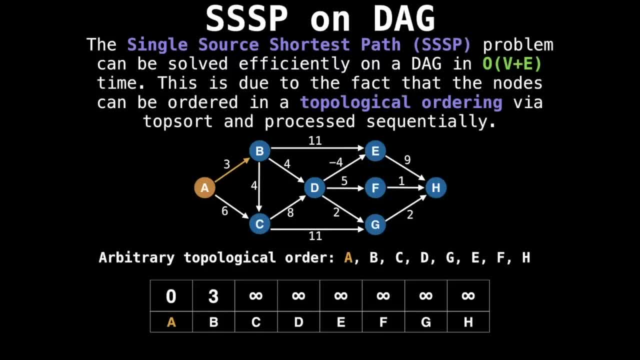 all reachable nodes, starting with node B, and update the value to be if it is better than what was already there. This is the edge relaxation step of the algorithm. we noticed that a value of three is better than infinity, So we update the best value of B to be three, then the 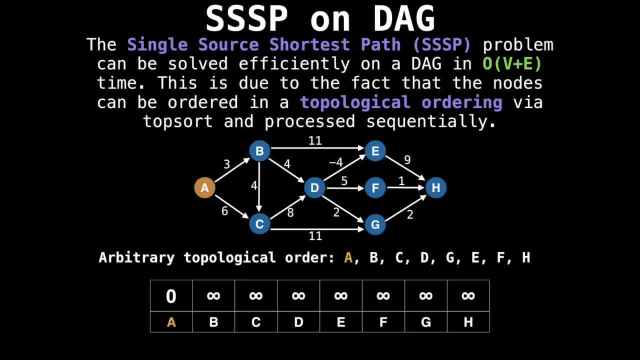 be zero. In this case, since a is the starting node, its initial distance is zero because we're already there From a. we want to visit all reachable nodes, starting with node B, and update the value to be if it is better than what was already there. This is the A. 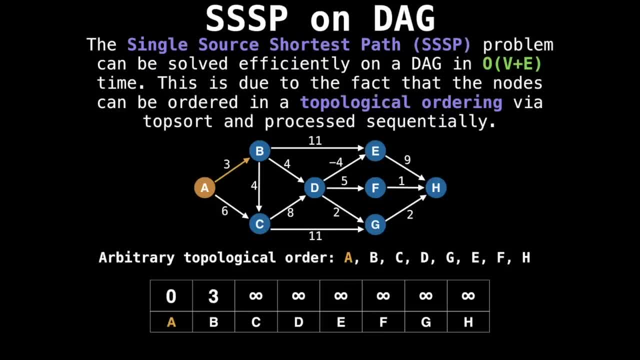 edge relaxation step of the algorithm, we noticed that a value of three is better than infinity, so we update the best value of B to be three, then the best value to see to be six, And now we've explored all of a's edges and want to move on to the next node. 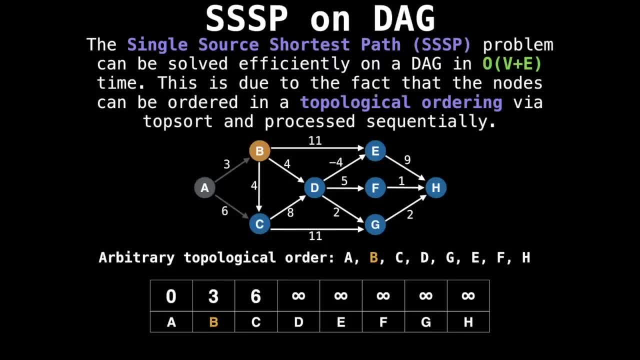 in our topological ordering, which is B, and explore all of its edges. So the first edge brings us to node he. we update its best value to 14. Because the best value at node B was three plus the edge weight to get to E was 11. For a total of 14.. Notice that edges get grayed out as they. 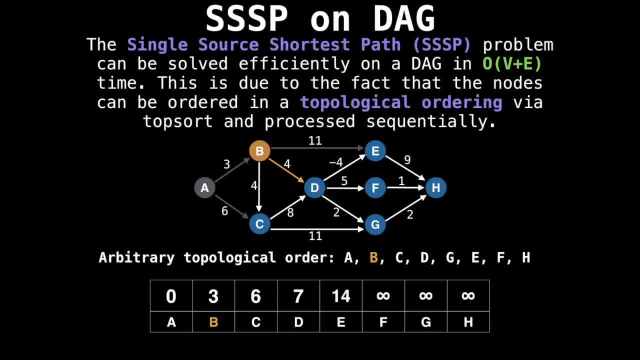 are being processed. Next, we update the best value to D, to be seven. Now we've reached the first instance, where it is best not to update the value of the destination node, since a better path already exists to where we want to update. Now we move on to the next. 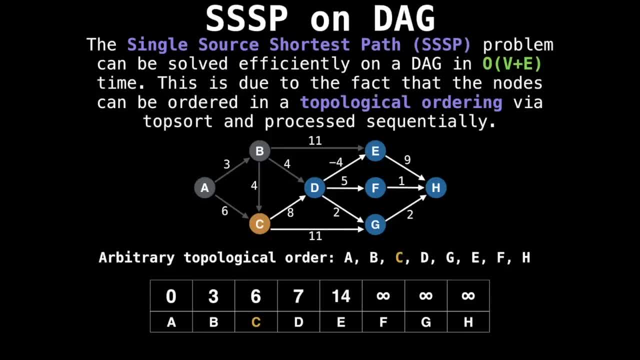 known or topological ordering, and keep repeating the same steps where we explore all the nodes, try and relax each edge and then move on to the next node in the topological ordering. If we repeatedly do this, the array at the bottom of the screen- 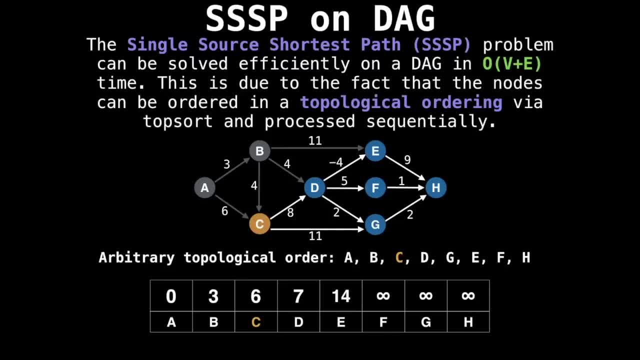 will contain the shortest path from node A to each node. I will let the animation play And you can try and determine the shortest path to all the remaining nodes which have not yet been processed. Okay, we're done processing all the nodes and know the shortest distance to every node. Let's 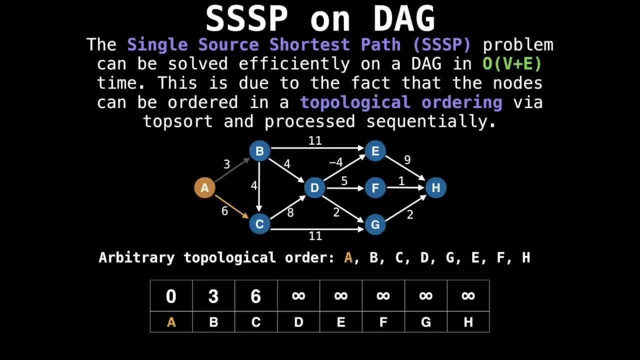 best value to see to be six. And now we've explored all of A's edges and want to move on to the next node in our topological ordering, which is B, and explore all of its edges. So the first edge brings us to node E and we update its best value to 14.. Because the best 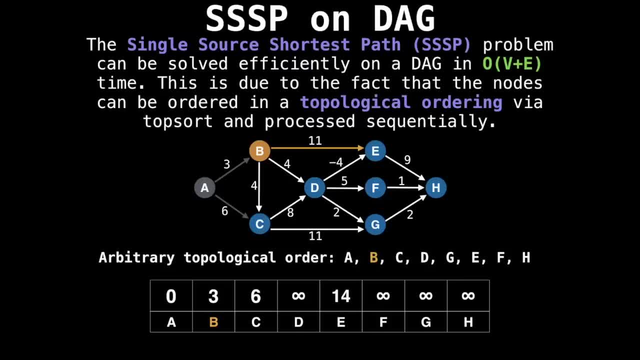 value at node B is 14.. So we update the best value at node B. and we update: the best value at node B was three plus the edge weight to get to E was 11 for a total of 14.. Notice that edges get grayed out As they are being processed. Next, we update the best value. 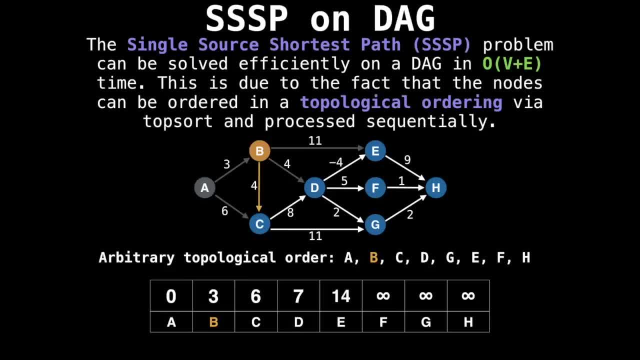 to D to be seven. Now we've reached the first instance, where it is best not to update the value of the destination node Since a better path already exists. we can set the best value to D. And now we move on to the next node in our topological ordering and keep repeating. 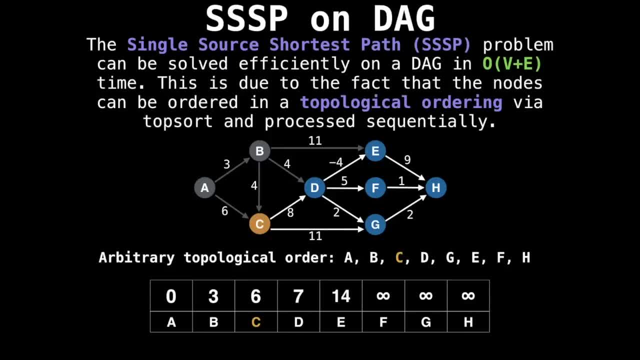 the same steps where we explore all the nodes, try and relax each edge and then move on to the next node in the topological ordering. If we repeatedly do this, the array at the bottom of the screen will contain the shortest path from node A to each node. I will let 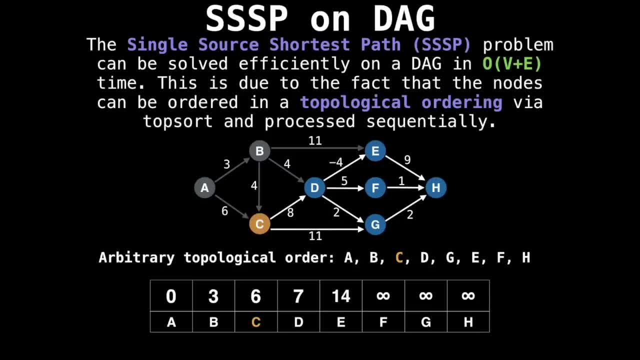 the animation play And you can try and determine the shortest path to all the remaining nodes which have not yet been processed. Okay, we're done processing all the nodes and know the shortest distance to every node. So let's verify our algorithm computer the correct values by finding the shortest path. 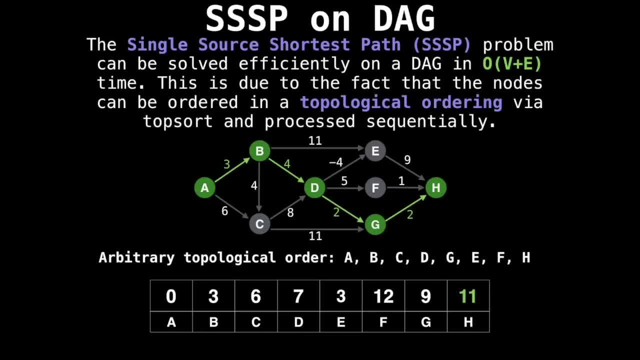 to node H. Indeed, if we look at the path and sum up the values along the edges, you will find that they do indeed sum up to 11, Which is the shortest path in our array. for node h, There's a similar problem to the shortest path problem, which is finding the longest. 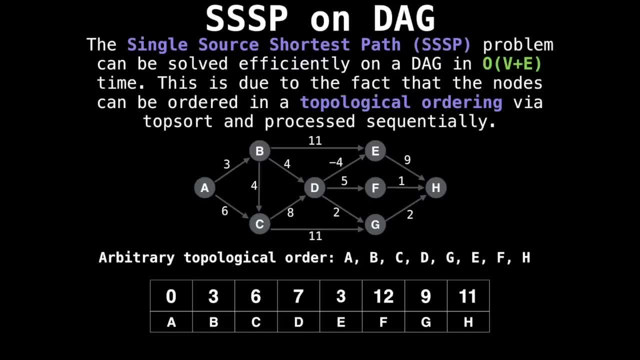 verify our algorithm computer the correct values by finding the shortest path to node H. Indeed, if we look at the path and sum up the values along the edges, you will find that they do indeed sum up to 11, which is the shortest path in our array for node A. 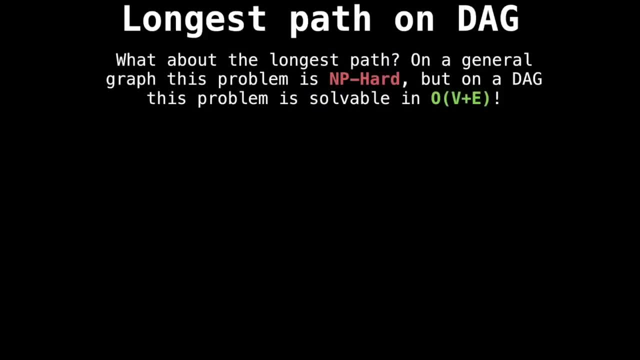 There's a similar problem to the shortest path problem, which is finding the longest path in the graph. This problem is actually NP hard on general graphs, but can actually be solved in linear time on a directed acyclic graph. The trick is going to be to multiply each edge by minus one: find the. 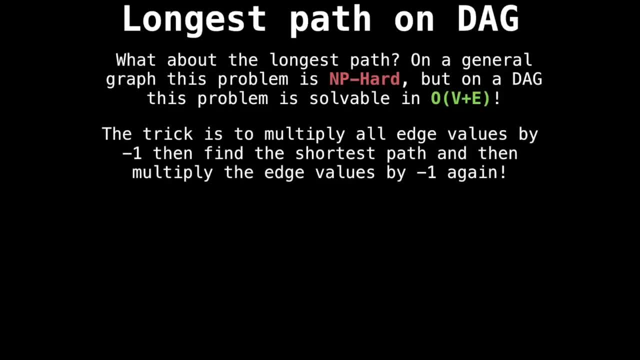 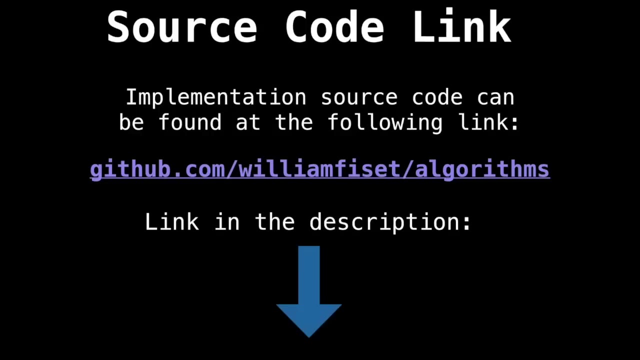 shortest path and then multiply all the edge values by minus one. again, Take the previous graph. we had to find the longest path. simply negate all the edges, then find the shortest path and multiply the answer by minus one, And there you go. That's all you need to do. Okay, now let's have a. 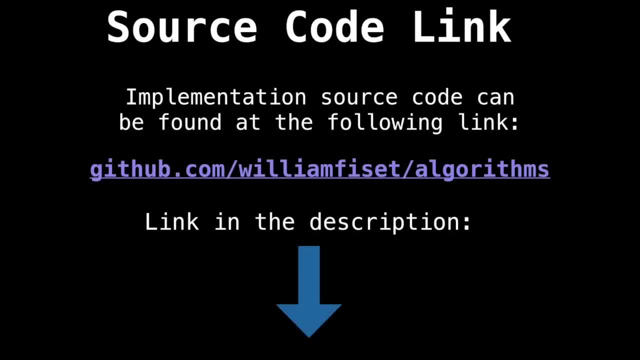 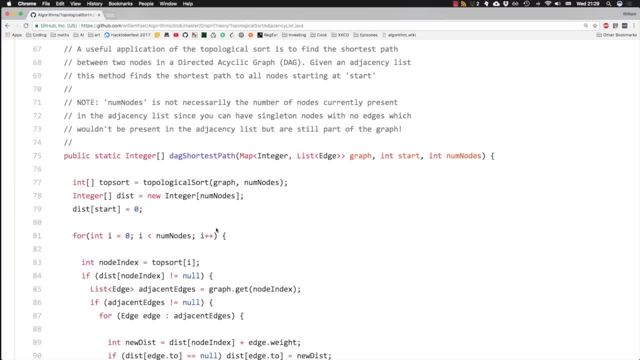 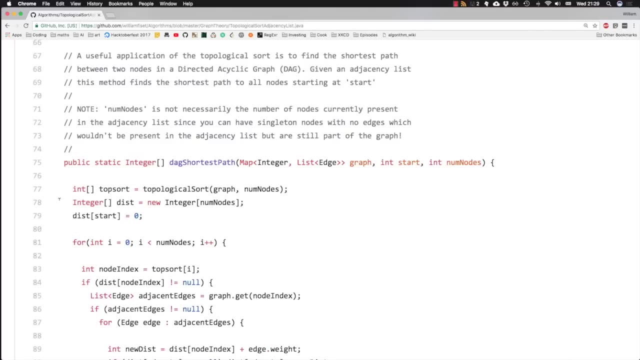 look at some source code. you can find the code I'm about to show you on GitHub at githubcom. slash willie infuse that slash algorithms. Here I am on GitHub and we're looking at some code for the shortest path on a directed acyclic graph. Here's our method: directed basic graph, shortest path and it. 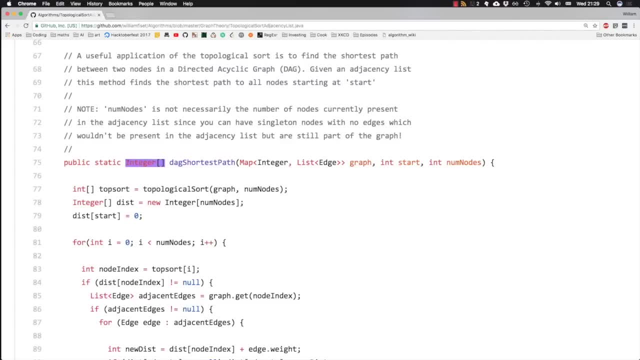 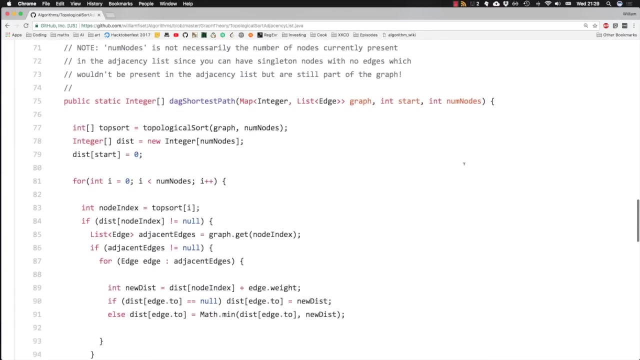 returns the distance to each node, stored in an integer array for some starting node And as input we give it the graph we're working with as an adjacency list, Of course, the starting node and lastly the number of nodes in our graph. So what we do is find the topological ordering for our nodes. I. 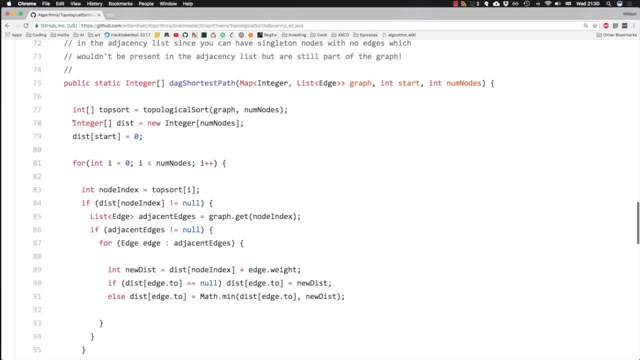 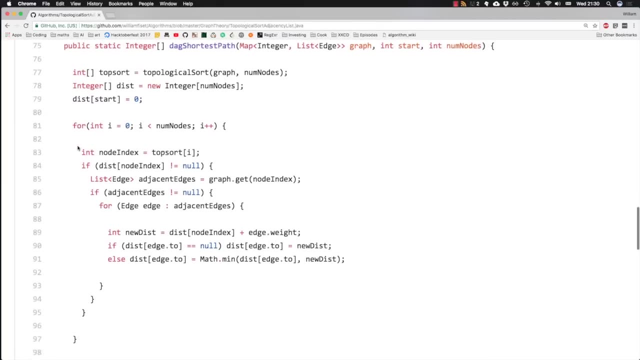 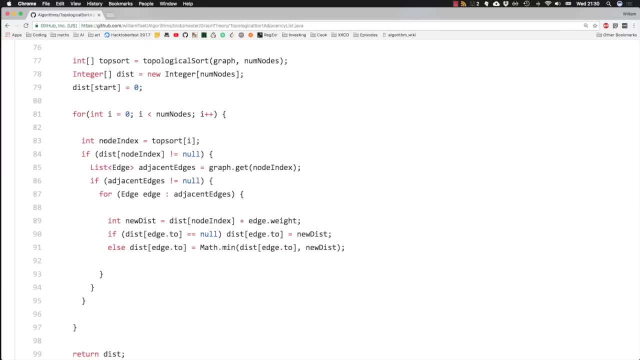 covered this last video- then initialize our distance array and then set the starting nodes distance to be zero And all we do is we loop through each node, starting at the first node, looking at what our node index is for top sort. So this is. 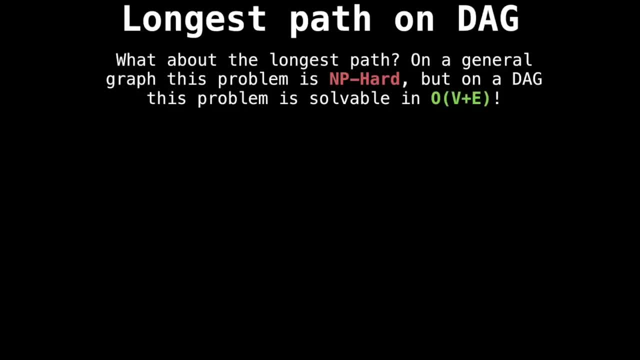 path in the graph. This problem is actually NP hard on general graphs, but can actually be solved in linear time on a directed acyclic graph. The trick is going to be to multiply each edge by minus one, find the shortest path and then multiply all the edge values. 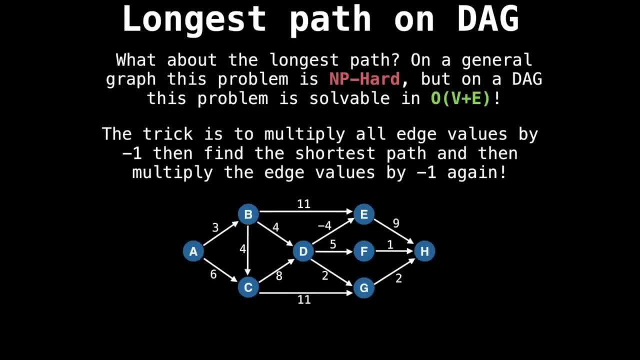 by minus one. again, Take the previous graph. we had to find the longest path. simply negate all the edges, then find the shortest path and multiply the answer by minus one, And there you go. That's all you need to do. Okay, now let's have a look at some sources. So 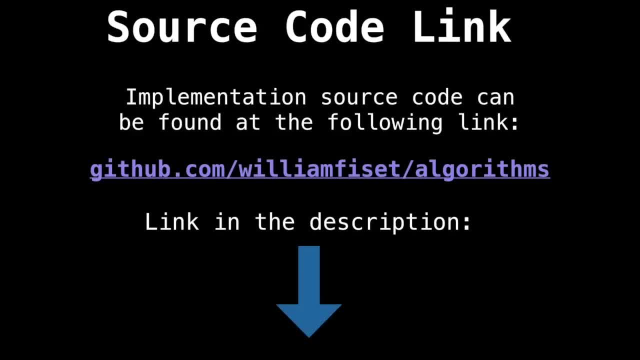 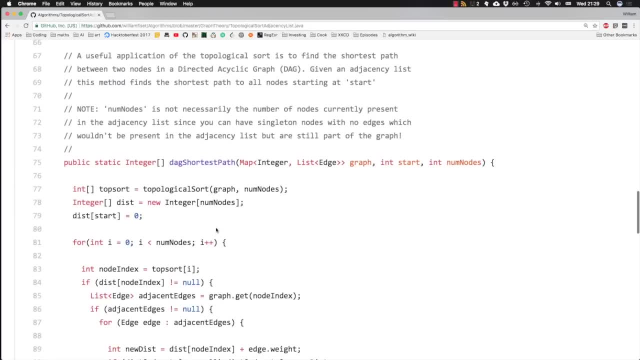 your source code. you can find the code I'm about to show you on GitHub at githubcom. Slash- William fuzett slash algorithms. Here I am on GitHub and we're looking at some code for the shortest path on a directed acyclic graph. Here's our method: directed basic graph. 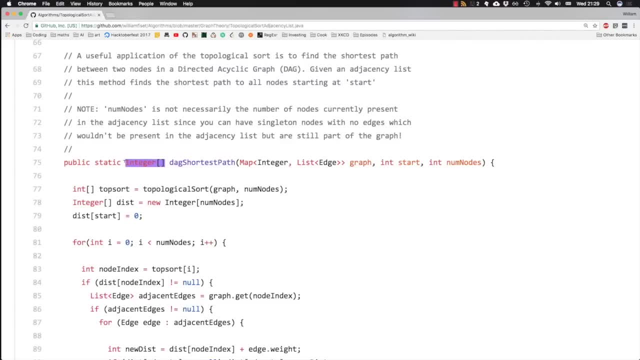 shortest path and it returns the distance to each note sorted in infrastructure integer array for some starting node And as input we give it the graph we're working with as an adjacency list, Of course, the starting node and lastly the number of nodes. 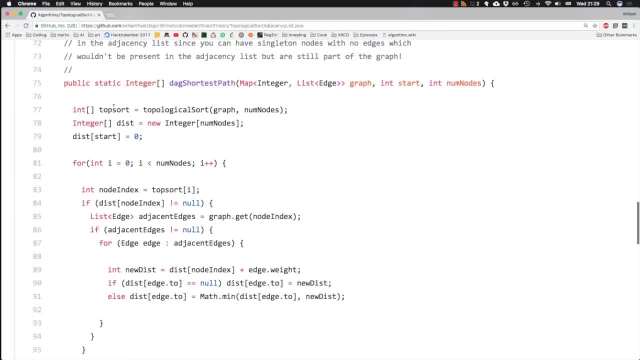 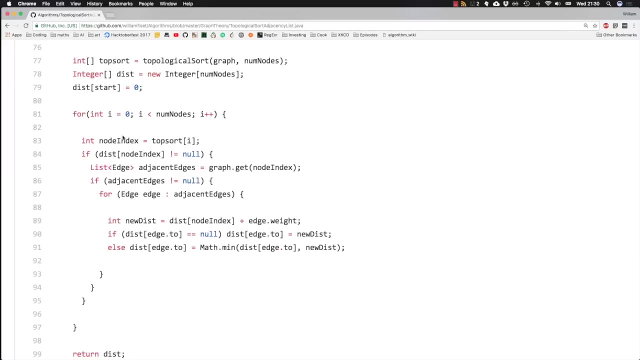 in our graph. So what we do is find the topological ordering for our nodes- I covered this last video- then initialize our distance array and then set the starting nodes distance to be zero, And all we do is we loop through each node, starting at the first node looking. 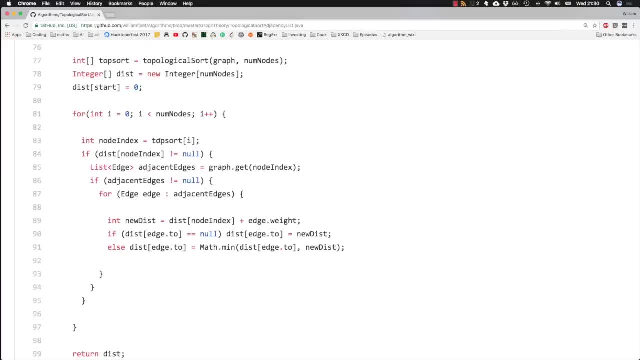 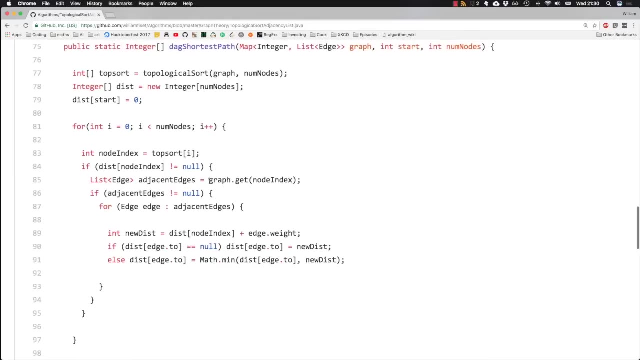 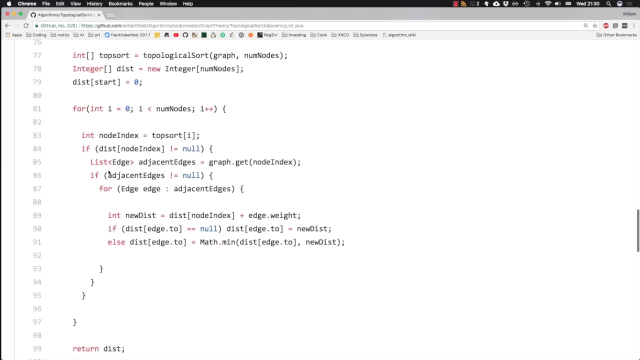 at what our node index is for top sort. So this is the first node we need to visit And then check if that node is not equal to null And then grab all the edges For that node. So we reach in our graph and then pull out all the edges for the node index. 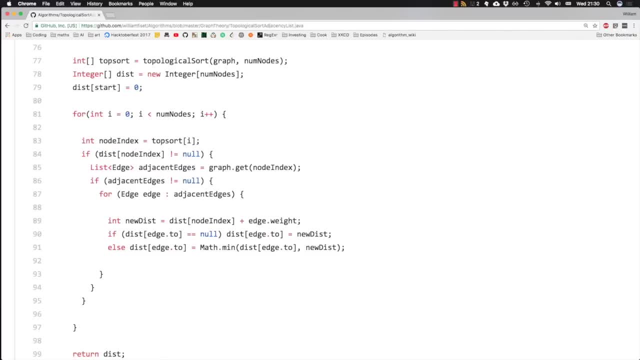 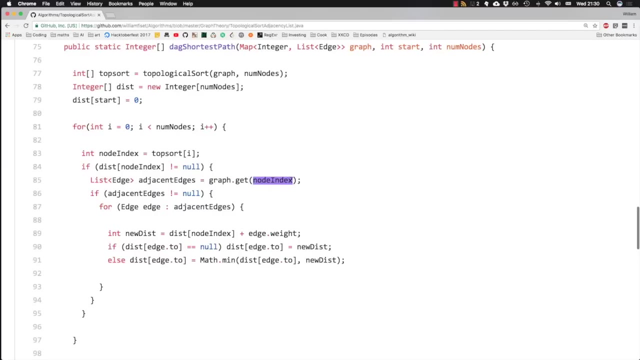 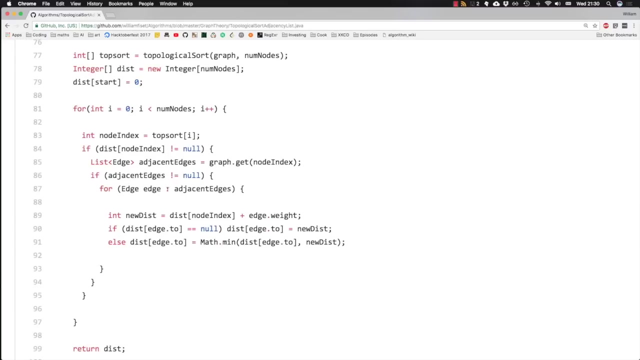 the first node we need to visit And then check if that node is not equal to null and then grab all the edges for that node. So we reach in our graph and then pull out all the edges for the node index. Give original values of internal and absolut�로 there. 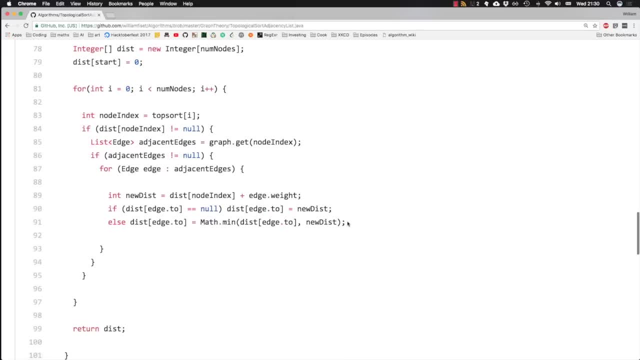 And now we're gonna make sure there actually are some edges, And then for each edge in the edges that we got, which were the adjacent edges, then all we do is the relaxation step, which is just this: So we compute the new distance. 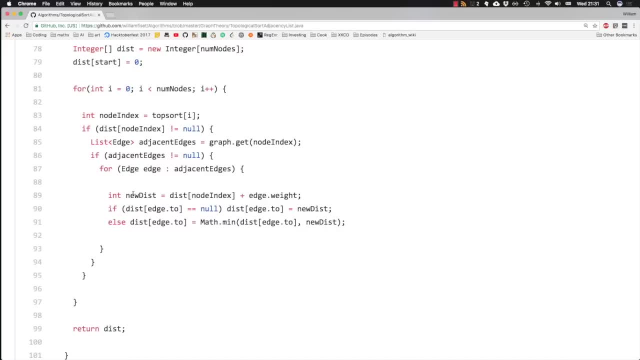 we were trying to improve upon. then we check: okay, has there ever been a distance set to where we want to go? This is basically the equivalent of infinity- And if so, then we just want to give the new distance. Otherwise, we're going to take the minimum of the distance that's already there. 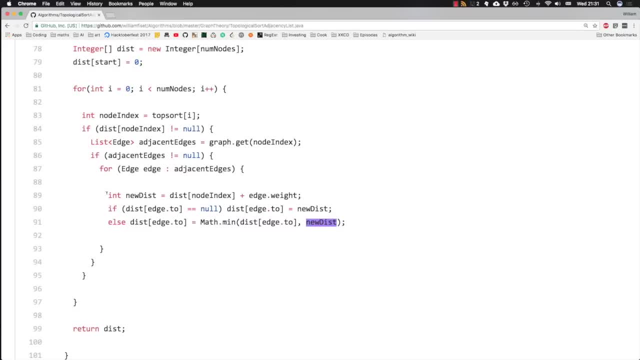 and our new competing distance, which is this over here. And then we just do this over and over again, processing nodes in topological order, because we're pulling them out of the top sort array And at the end we just return that distance array And we can get the distance. 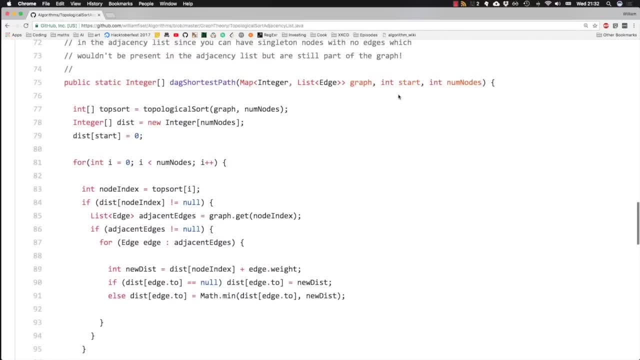 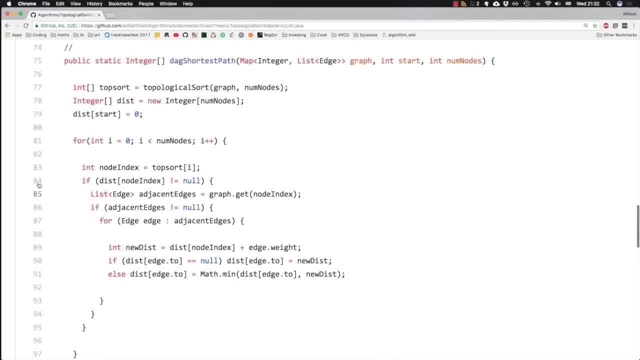 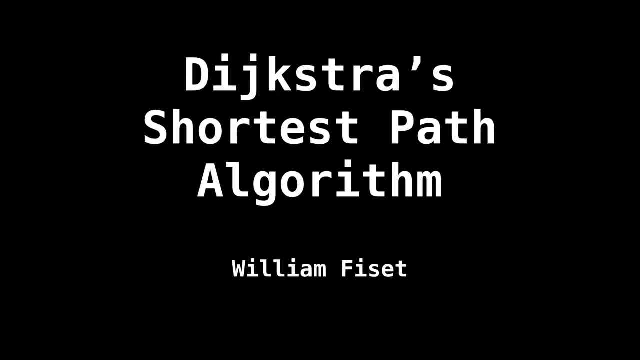 from our starting node to any other node in the graph. just through a lookup in this array And, guys, this is super simple algorithm And that's all there is to shortest paths on directed, basically, graphs. Today we're going to tackle Dykstra: shortest path algorithm. 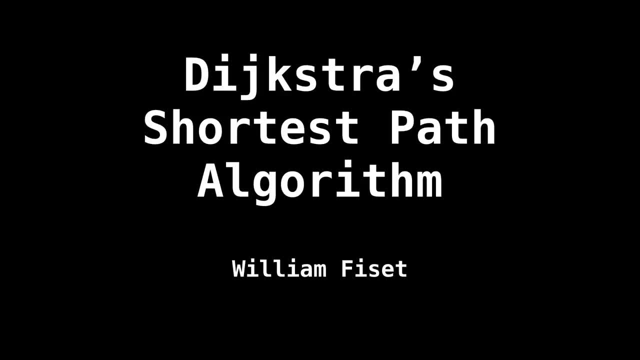 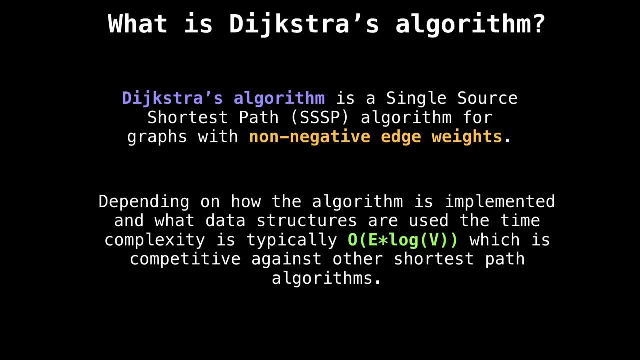 This is one of the most important algorithms in graph theory for finding the shortest path on a graph. So without further ado, let's dive right in. The first thing to mention about Dykstra is algorithm is that it is a single source: shortest path algorithm. 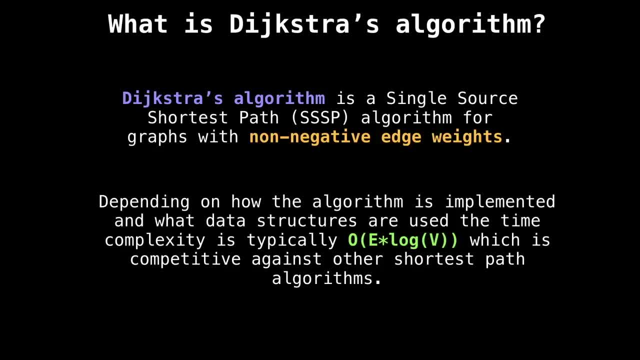 This means that at the beginning of the algorithm you need to specify a starting node to indicate a relative starting point for the algorithm. Once you specify the starting node and execute the algorithm, Dykstra's can tell you the shortest path between that node and all other. 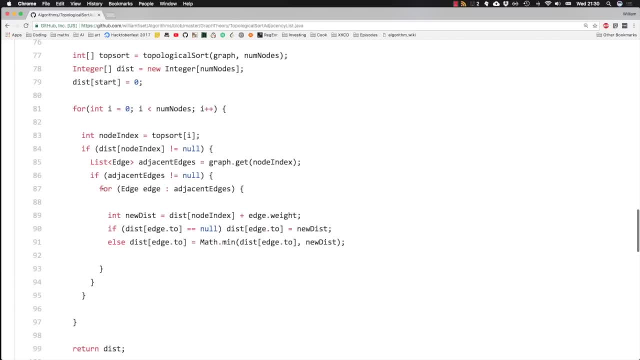 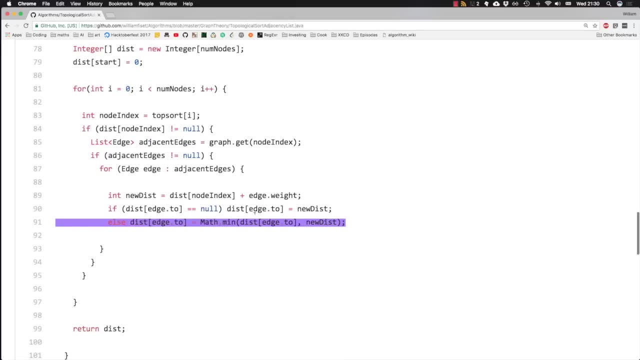 Make sure there actually are some edges, And then, for each edge in the edges that we got, which were the adjacent edges, then all we do is the relaxation step, which is just this, So we compute the new distance. So this is the distance to the node. 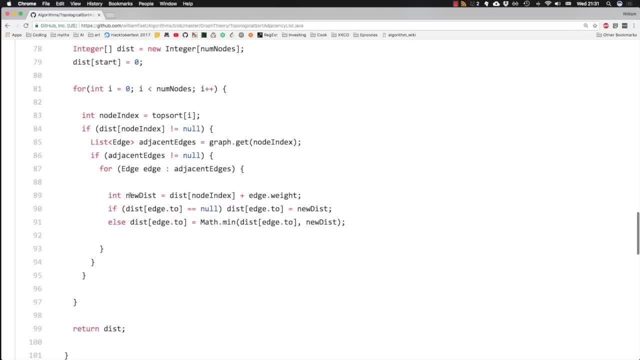 we're currently at plus the edge weight. So this is like the competing distance, the distance we were trying to improve upon. then we check: okay, has there ever been a distance set to where we want to go? This is basically the equivalent of infinity, And if so, then we: 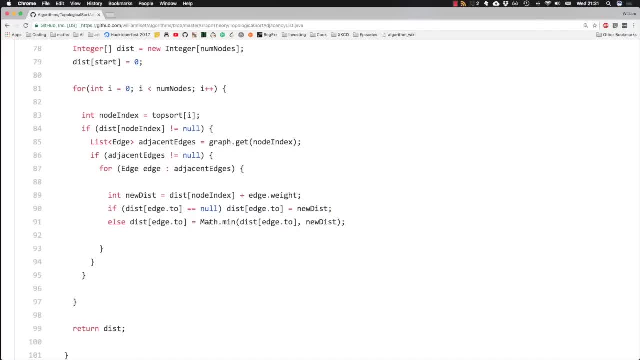 just want to give the new distance, Otherwise we're going to take the minimum of the distance that's already there And our new competing distance, which is this over here. And then we just do this over and over again, processing nodes and topological order, because we're pulling them out of the 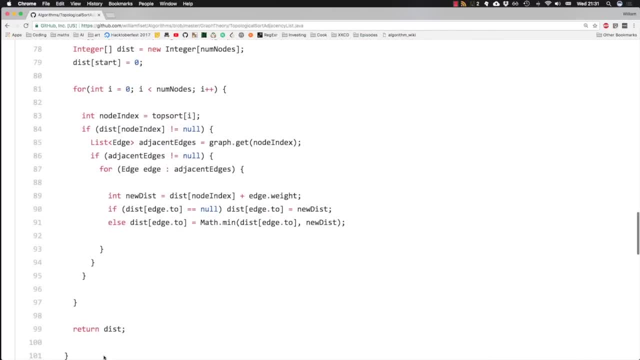 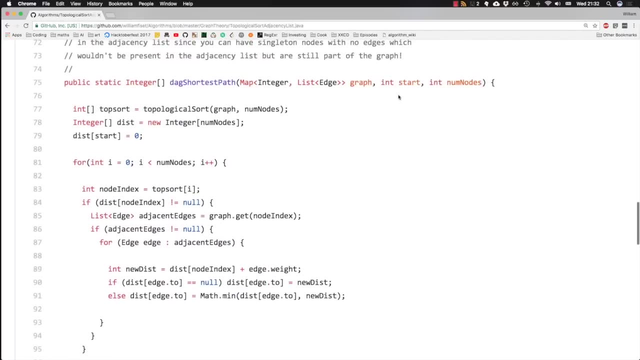 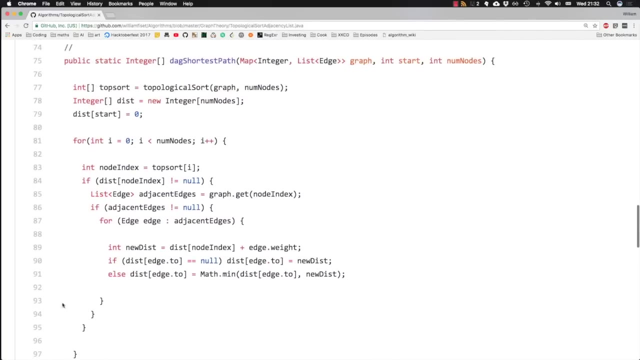 top sort array And at the end we just return that distance array And we can get the distance from our starting node to any other node in the graph just through a lookup. And this is the same thing we did with our previous array. And, guys, this is super simple algorithm. 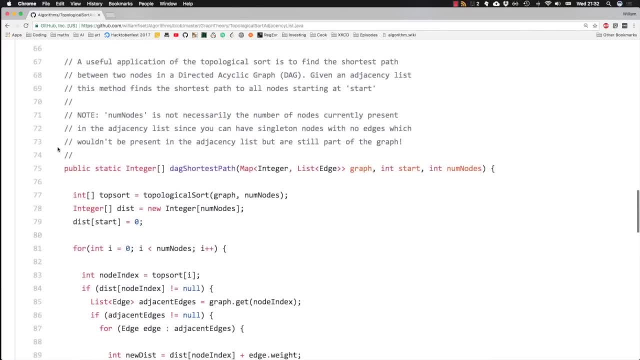 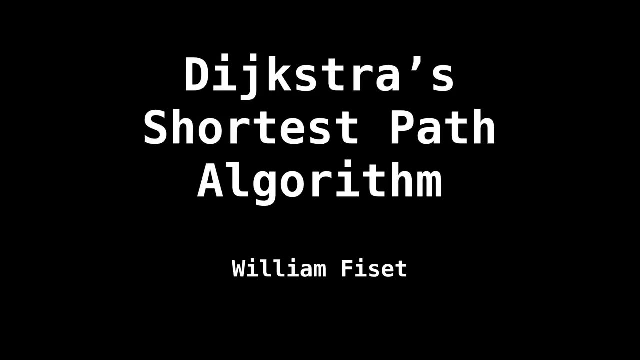 And that's all there is to shortest paths on directed, basically, graphs. Today we're going to tackle Dykstra: shortest path algorithm. This is one of the most important algorithms in graph theory for finding the shortest path on a graph. So, without further ado, let's. 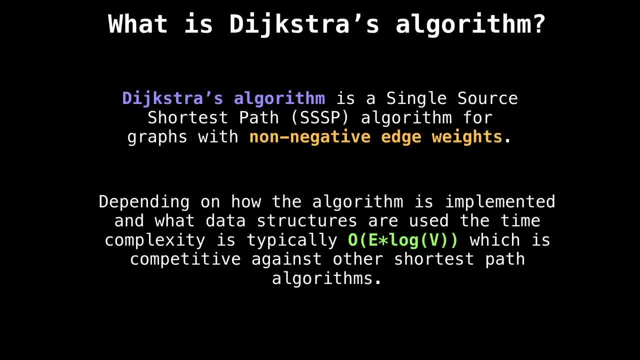 dive right in. The first thing to mention about Dykstra is algorithm is that it is a single source, The shortest path algorithm for graphs. This means that at the beginning of the algorithm you need to specify a starting node to indicate a relative starting point for the algorithm. 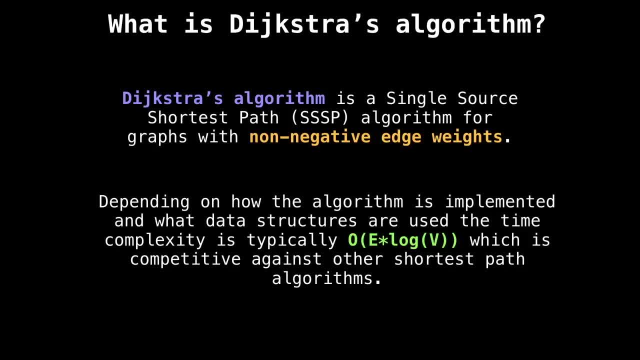 Once you specify the starting node and execute the algorithm, Dykstra's can tell you the shortest path between that node and all other nodes in your graph, which is pretty sweet. So, depending on how you implement your Dykstra's and what data structures you use, the time 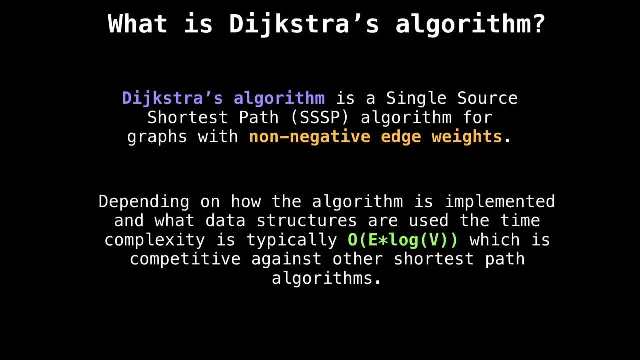 nodes in your graph, which is pretty sweet. So, depending on how you implement your Dykstra's and what data structures you use, the time complexity is big O of E log V, which is fairly competitive against other shortest path algorithms we see around. However, before we go crazy trying to find shortest paths on various graphs, 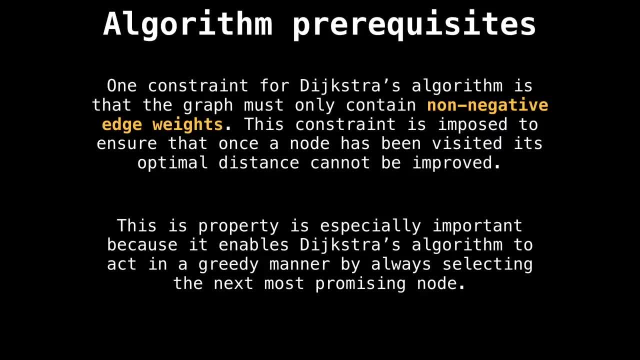 you need to know which graphs we are allowed to run Dykstra's algorithm on. the one main constraint for Dykstra's is that all edges of the graph need to have a non negative edge weight. This constraint is imposed to ensure that once a node has been visited, it will 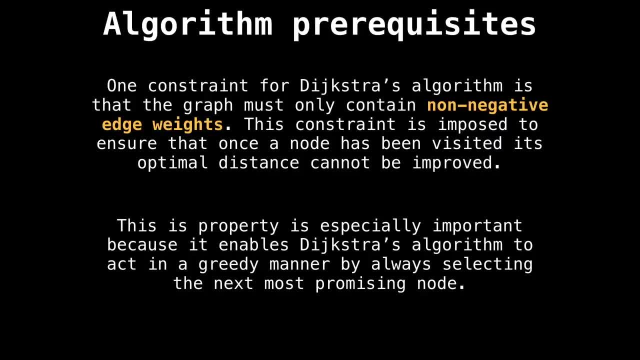 have a negative edge weight. Its optimal distance from the starting node cannot be improved any further by finding a shorter path by taking an edge with a negative weight. This property is especially important because it enables Dykstra's algorithm to act in a greedy manner by always selecting 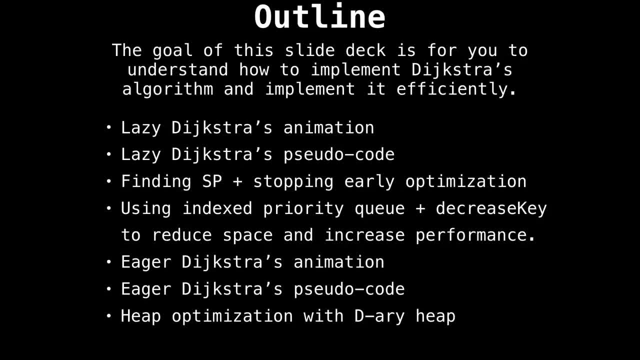 the next most promising node For this slide deck. my goal is to help you understand how implement Dykstra's algorithm and also how to implement it very efficiently. We're going to start by looking at the lazy implementation, because it's by far the most. 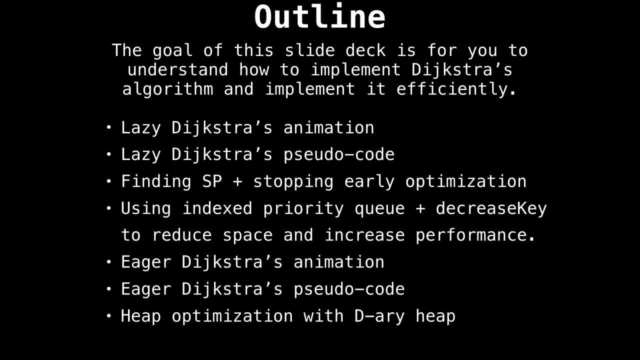 common. and then we'll look at the eager implementation of Dykstra's algorithm, which uses an indexed priority queue alongside the decrease key operation. And lastly, I want to briefly mention how we can use other types of heaps, in particular the da re heap, to further boost performance. 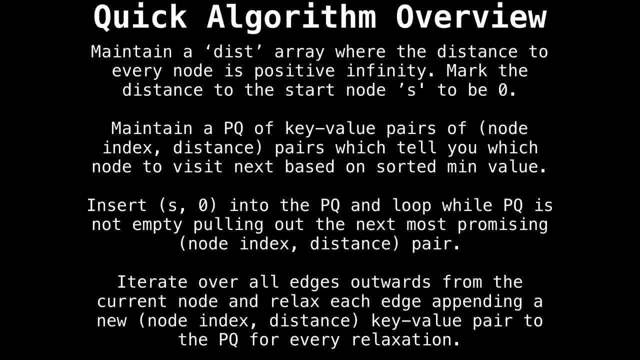 of the algorithm at a high level. These are the steps required in executing Dykstra's algorithm. Note that there are two bits information we'll need. The first is an array called dist that keeps track of the shortest distance to every node from the start node. Initially, this 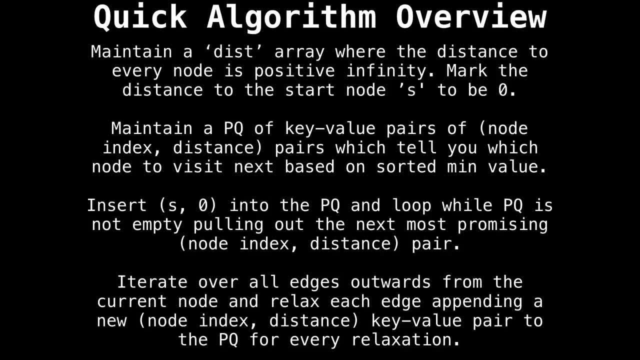 array can be populated with a value of positive infinity, except for the index of the starting node, which should be initialized to zero. Additionally, we'll also need to maintain a priority queue of key value pairs. The key value pairs will be: node index. This will 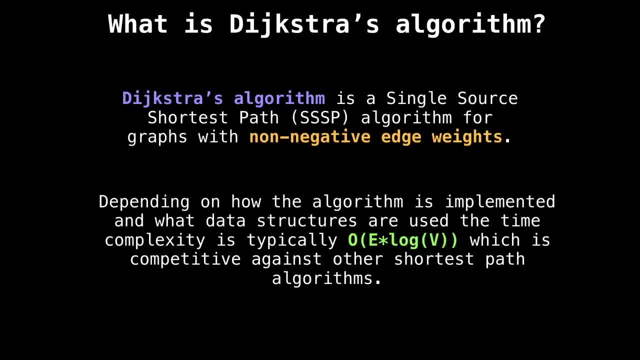 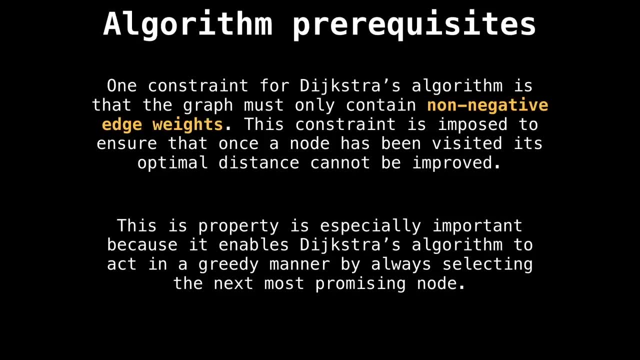 complexity is different. Dykstra's algorithm is typically big O of E log V, which is fairly competitive against other shortest path algorithms we see around. However, before we go crazy trying to find shortest paths on various graphs, you need to know which graphs we are allowed to run. 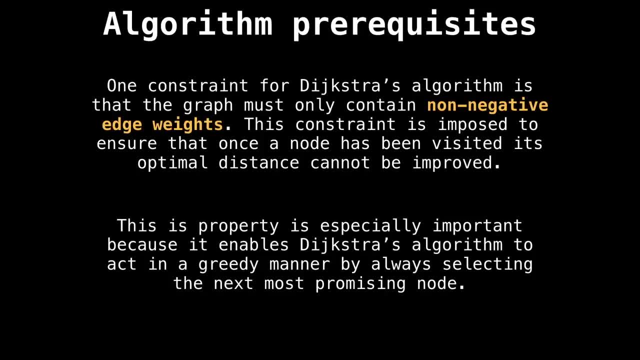 Dexter's algorithm on the one main constraint for Dykstra's is that all edges of the graph need to have a non negative edge weight. This constraint is imposed to ensure that, once a node has been visited, its optimal distance from the starting node cannot be improved. 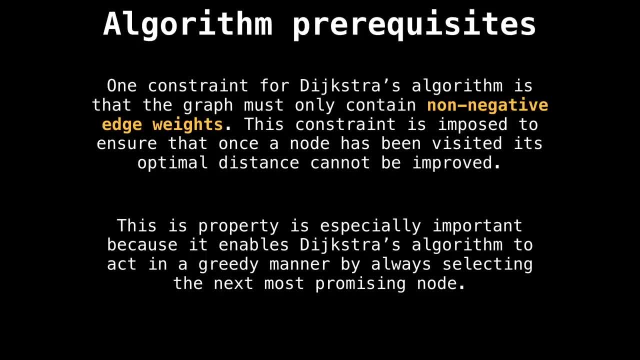 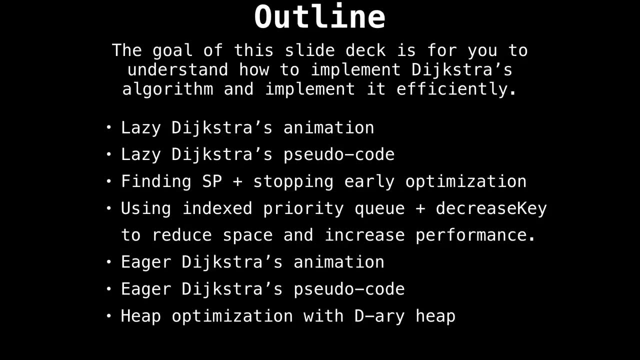 any further by finding a shorter path, by taking an edge with a negative weight. This property is especially important because it enables Dykstra's algorithm to act in a greedy manner by always selecting the next most promising node For this slide deck. my goal is to help. 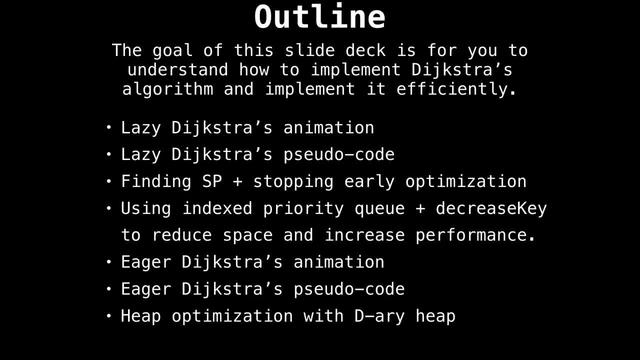 you understand how to implement Dykstra's algorithm and also how to implement it very efficiently. We're going to start by looking at the lazy implementation, because it's by far the most common, and then we'll look at the eager implementation of Dykstra's algorithm, which uses an index. 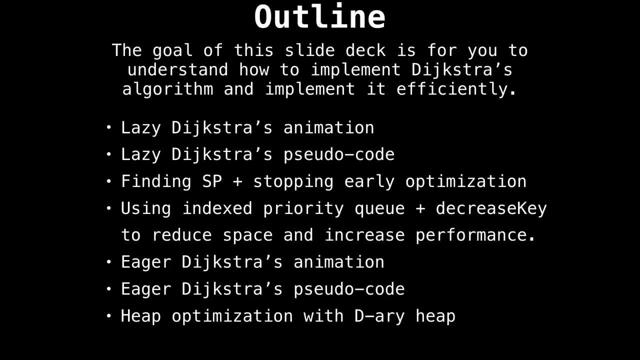 priority queue alongside the decrease key operation. And lastly, I want to briefly mention how we can use other types of heaps, in particular the da re heap, to further boost performance of the algorithm At a high level. these are the steps required in executing Dykstra's. 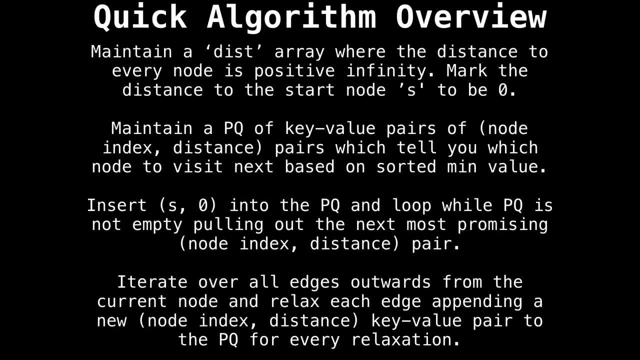 algorithm. Note that there are two bits information we'll need. The first is an array called dist that keeps track of the shortest distance to every node from the start node. Initially, this array can be populated with a value of positive infinity, except for the index of the starting. 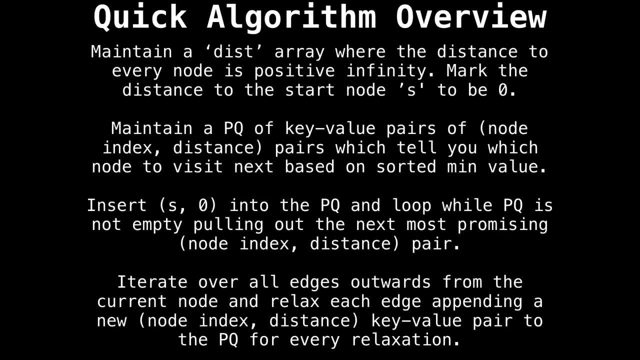 node, which should be initialized to zero. Additionally, we'll also need to maintain a priority queue of key value pairs. the key value pairs will be node index distance pairs, which tell us which node to visit next, based on a minimum sorted value. 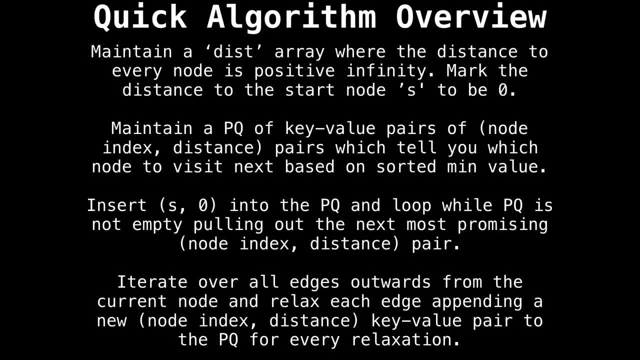 At the start of the algorithm. we will begin by inserting the key value pair s comma zero into the priority queue. then we'll loop while the priority queue is not empty, pulling out the next most promising node: index distance pair. as we go After that, for each node, we 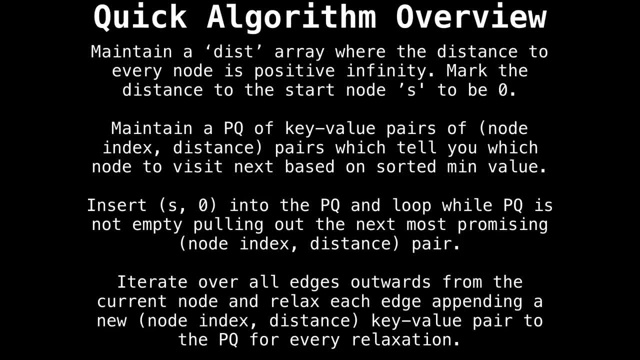 be the index of the next distance pairs which tell us which node to visit next, based on a minimum sorted value. at the start of the algorithm we will begin by inserting the key value pair s comma zero into the priority queue. then we'll loop while a priority queue. 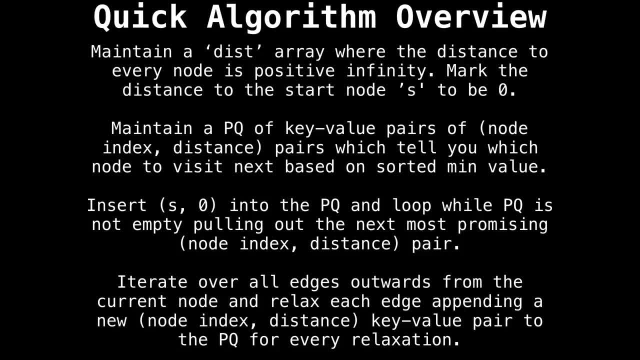 is not empty, pulling out the next most promising node index distance pair. as we go After that, for each node we visit, we will want to iterate over all the outwards edges and relax each edge, pending a new node index distance key value parent to the priority queue upon every successful 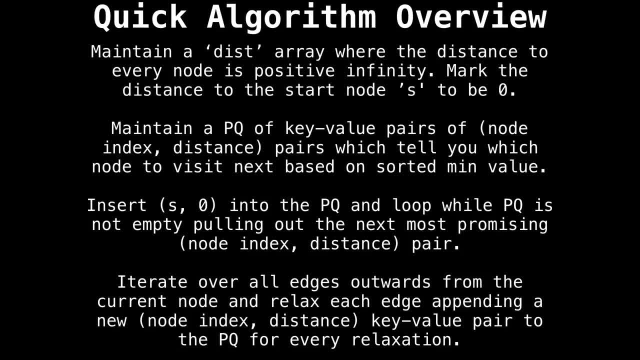 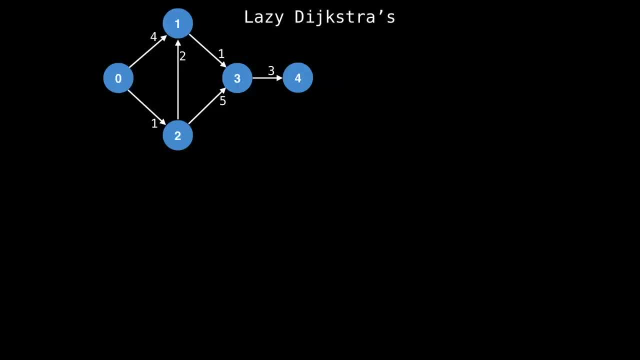 relaxation. We do this until our priority queue is empty, at which point the shortest distance to each node will be stored in the dist array we are maintaining. So that explanation may have sounded a little bit abstract. Now let's look at an example with some animation. 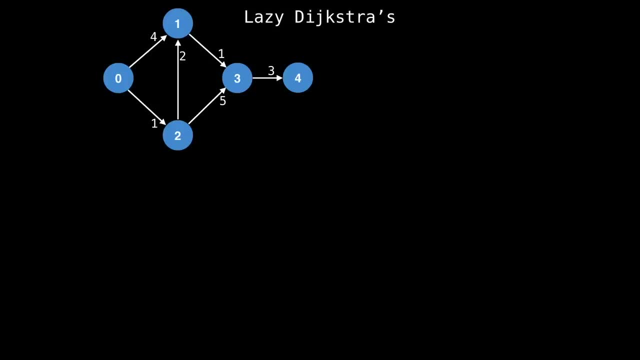 to put all the pieces together In all these examples. assume node zero is always the starting node, although any node is perfectly fine. boxed in red is the distance array. I will be using it to track the optimal distance from the Start node to every node in the graph. 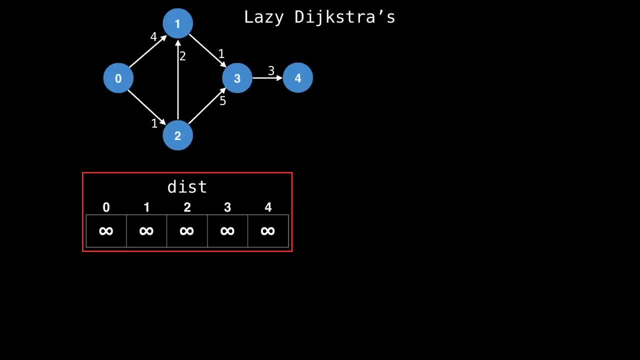 In the beginning the distance to every node is initialized to have the value of positive infinity, since we assume that every node is unreachable. Here we can see that the distance to every node is a positive infinity value. You have, If at the end of the algorithm there's still a value of infinity at a certain index, then 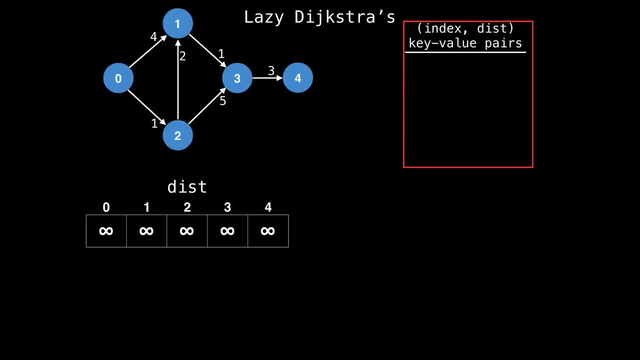 we know that that node is unreachable. On the right I will be maintaining key value pairs corresponding to a nodes index and the best distance to get to that node. This priority queue will tell us which node we should visit next, based on which key value pair has the 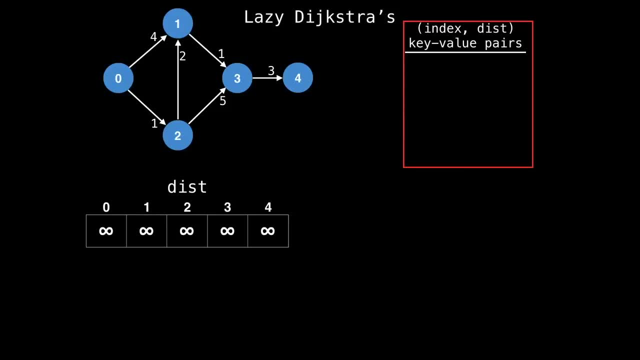 lowest value. Internally, priority queues are usually implemented as heaps, but I'm not going to show that visualization here. To start with, assign a distance of zero to the start nodes index, which is index zero in the distance array. Also insert the key. 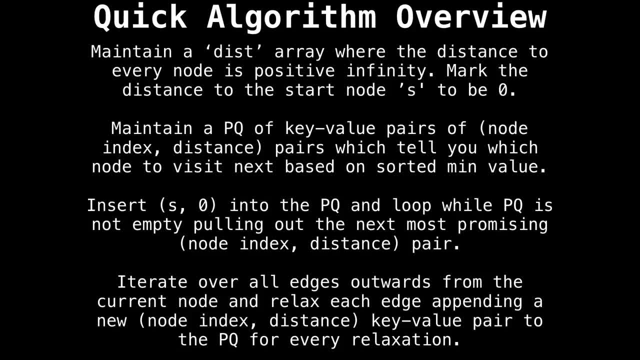 visit, we will want to iterate over all the outwards edges and relax each edge a pair pending a new node index distance key value pair to the priority queue Upon every successful relaxation. we do this until our priority queue is empty, at which point the shortest 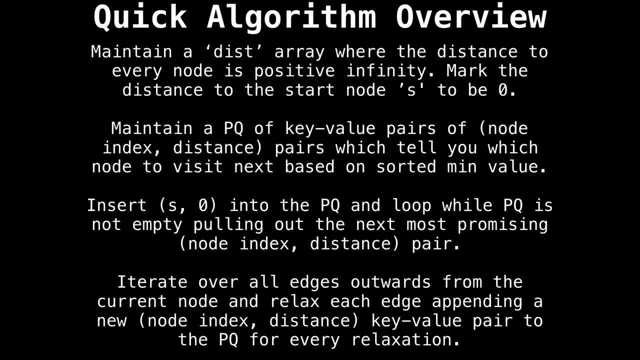 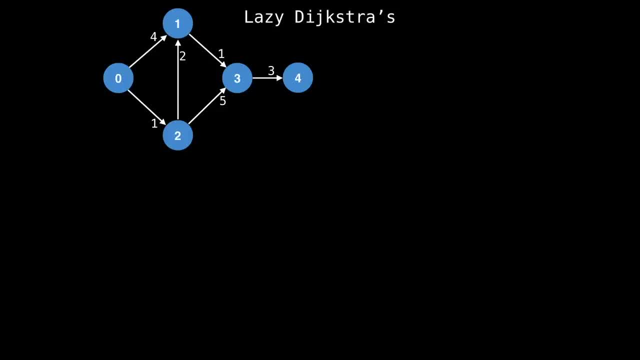 distance to each node will be stored in the dist array we are maintaining. So that explanation may have sounded a little bit abstract. Now let's look at an example with some animation to put all the pieces together. In all these examples, assume node zero is equal to zero. 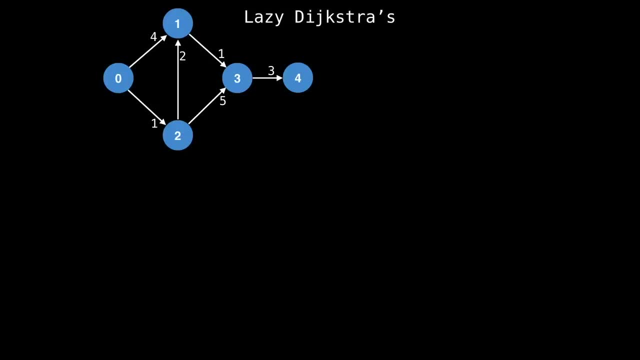 zero is always the starting node, although any node is perfectly fine. boxed in red is the distance array. I will be using it to track the optimal distance from the start node to every node in the graph. In the beginning, the distance to every node is initialized. 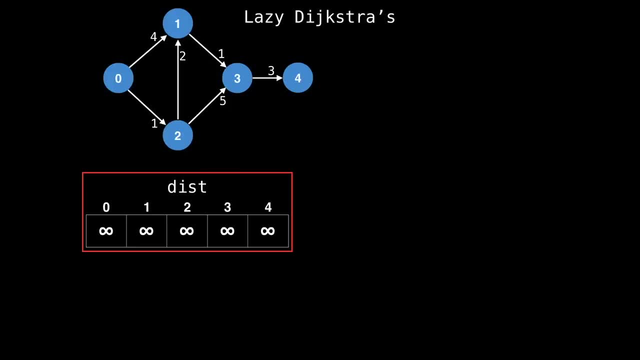 to have the value of positive infinity, since we assume that every node is unreachable. If, at the end of the algorithm, there's still a value of infinity at a certain index, then we know that that node is unreachable. On the right, I will be maintaining key value. 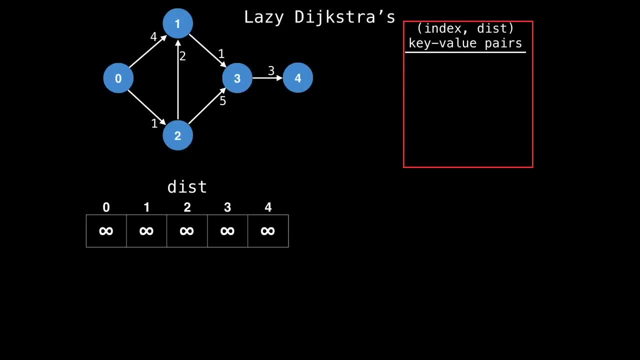 pairs corresponding to a nodes index and the best distance to get to that node. This priority queue will tell us which node we should visit next, based on which key value pair has the lowest value. Internally, priority queues are usually implemented as heaps, but I'm 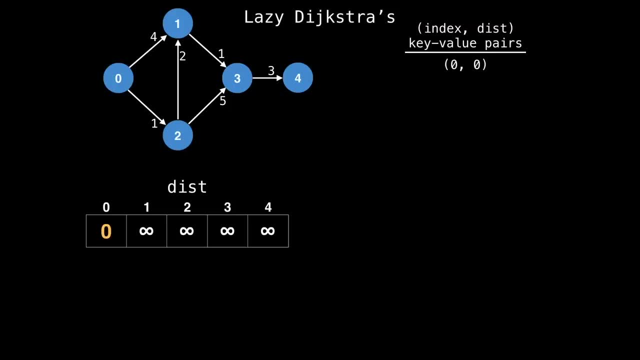 not going to show that visualization here. To start with, assign a distance of zero to the start nodes in index, which is index zero in the distance array. Also, insert the key value pair zero, comma zero into the priority queue to indicate that we intend on visiting node zero with. 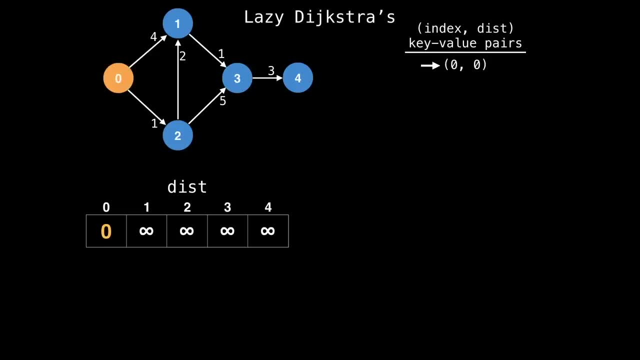 a best distance of zero. then the algorithm actually starts and we look inside the priority queue for the first time and we discover that we should visit node zero. From node zero we can visit node one by using the edge, with a cost of four. This gives us a best distance. 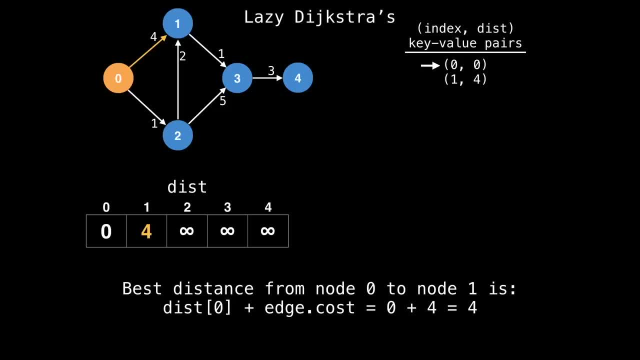 of four, so we can update the best distance from infinity to four In the dist array. also add this information to the priority queue. Next we can visit node two from node zero, just like the last node, we can update the optimal distance to. 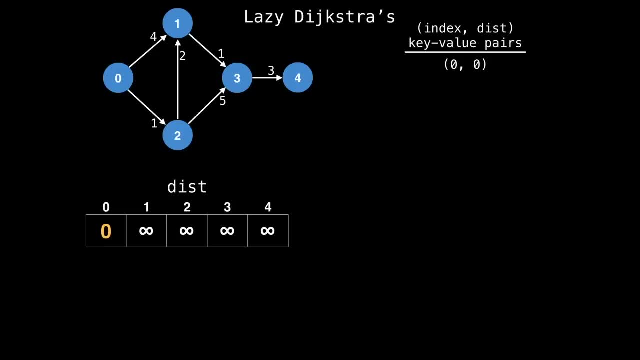 value, pair zero, comma zero into the priority queue to indicate that we intend on visiting node zero with a best distance of zero. then the algorithm actually starts and we look inside the priority queue for the first time and we discover that we should visit node zero. From node zero we can visit node one by using: 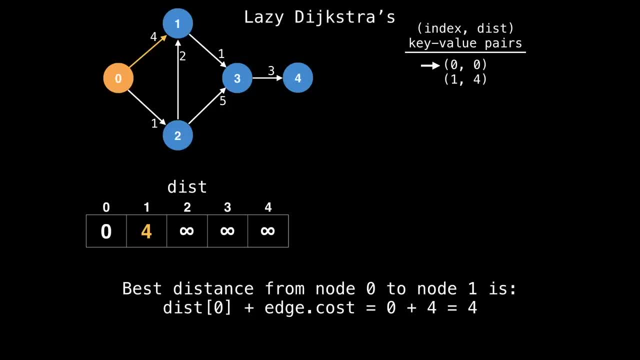 the edit edge with a cost of four. this gives us a best distance of four, So we can update the best distance from infinity to four in the dist array. Also, add this information to the priority queue. Next we can visit node two from node zero, just like the last node. we 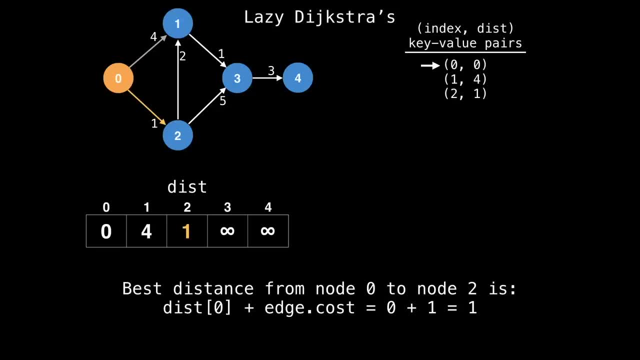 can update the optimal distance to reach node two from infinity to one. Additionally, add that node two is reachable with a distance of one to the priority queue. So that concludes visiting all the edges for node zero. to decide which node we should visit, 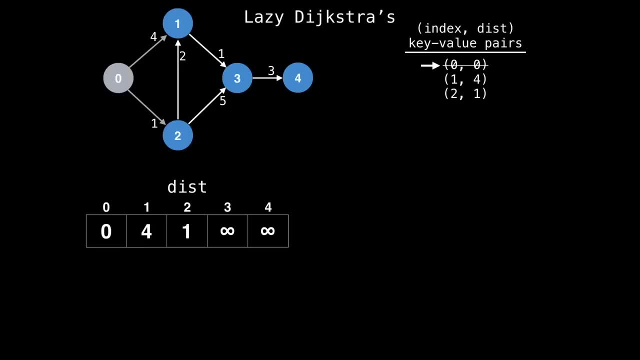 Next, Dijkstra's always selects the next most promising node in the priority queue. To do this, simply pull the next best key value pair from the priority queue. node two is the next most promising node because it has a distance of one from the start node, while 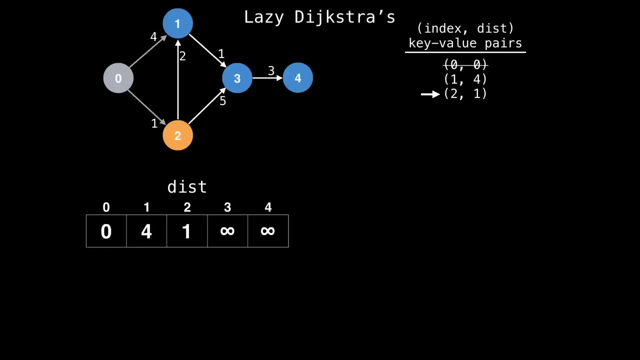 node one has a greater value of four From node two. if we take the upwards edge we can improve the best distance to node one by taking the current best distance from node two, which is one plus the edge cost of four, edge cost of two to get to node one for a total cost of three. this is better than the. 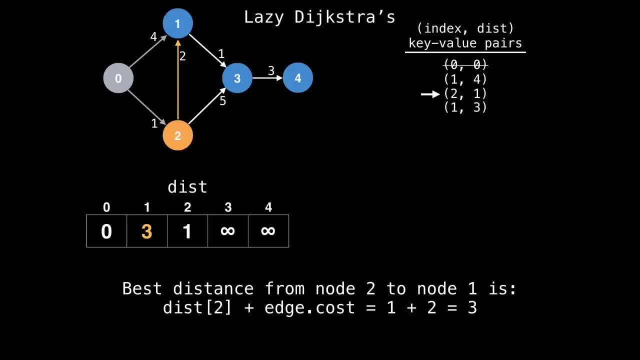 previous value of four. For every time we find a better distance like this, we insert that information into the priority queue. then we improve the best distance to node three to be six. The next most promising node is node one. we can improve the best distance. 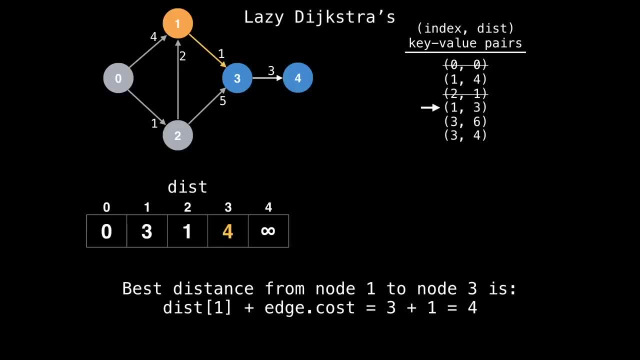 to node three by taking the edge from node one to node three, with a cost of one. The next most promising node is node one, with value four, but we have already found a better route to get to node one, since the dist array at index one has a value of three. Therefore, 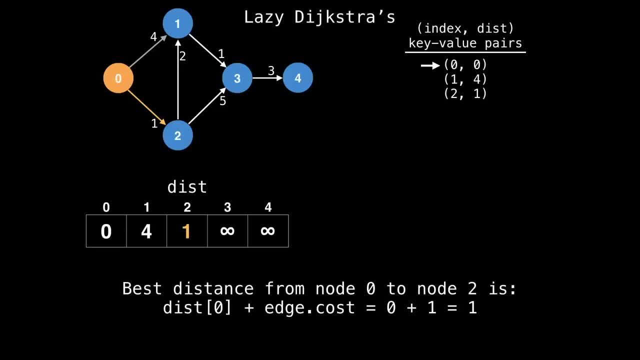 reach node two from infinity to one. Additionally, add that node two is reachable with a distance of one to the priority queue. So that concludes visiting all the edges for node zero. to decide which node we should visit next, dexterous always selects the next most promising node. 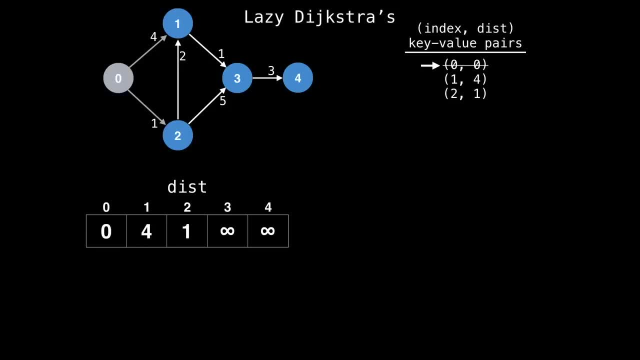 in the priority queue. To do this, simply pull the next best key value pair from the priority queue. node two is the next most promising node because it has a distance of one from the start node, while node one has a greater value of four From node two if we take the upwards edge. 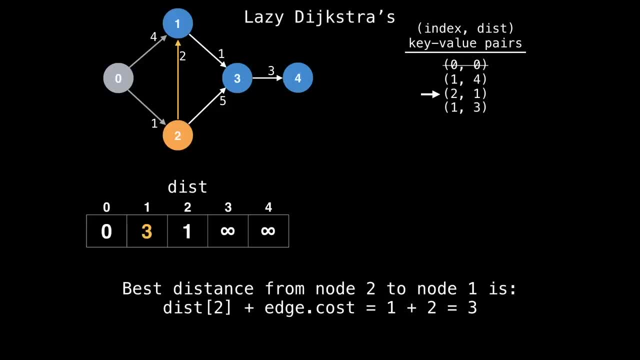 we can improve the best distance to node one by taking the current best distance from node two, which is one plus the edge cost of two to get to node one, for a total cost of three. This is better than the previous value of four. For every time we find a better distance like this, we insert that information into the. 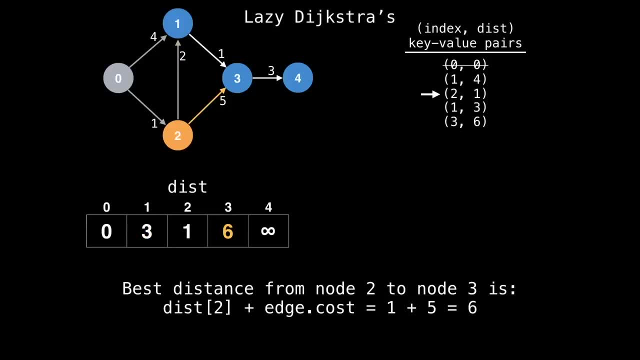 priority queue. then we improve the best distance to node three to be six. The next most promising node is node one. we can improve the best distance to node three by taking the edge from node one to node three with a cost of one. The next most promising node is node 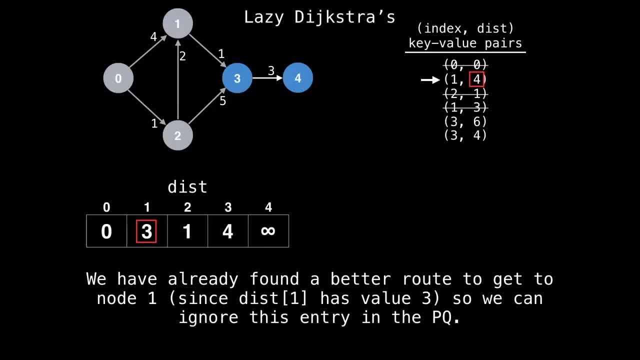 one with value four. But we have already found a better route to get to node one, since the dist array at index one has a value of three. Therefore, we can ignore this entry in the priority queue. Having these duplicate key entries in the priority queue is what constitutes to making this implementation. 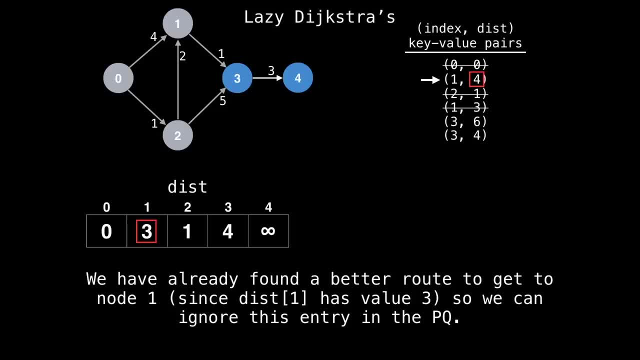 of Dijkstra is the lazy implementation, because we lazily delete outdated key value pairs. Next up is node three. Update the best distance to node four to be six. We already found a better route to node three, So skip this entry in the party queue. Finally, 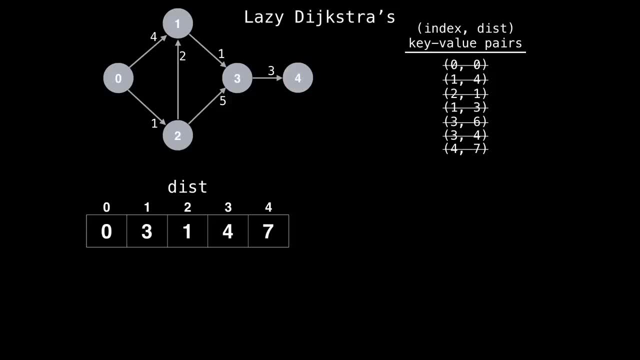 visit node four. And that's all for the lazy implementation of Dijkstra. There are only a few moving parts, But in large the only things to really keep track of is the distance array, which contains the best distance so far from the start node to every other node. 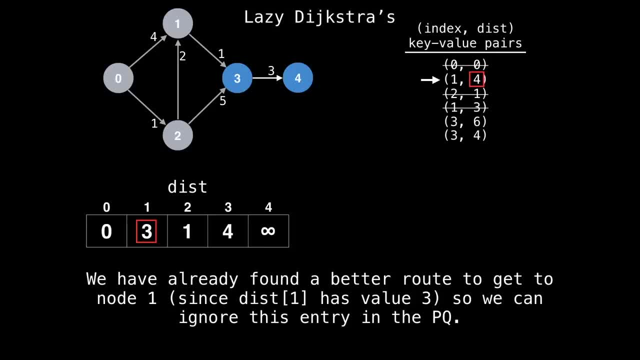 we can ignore this entry in the priority queue. Having these duplicate key entries in the priority queue is what constitutes to making this implementation of Dijkstra's the lazy implementation, because we lazily delete outdated key value. Next up is node three. update the best distance to node four to be seven. We already found. 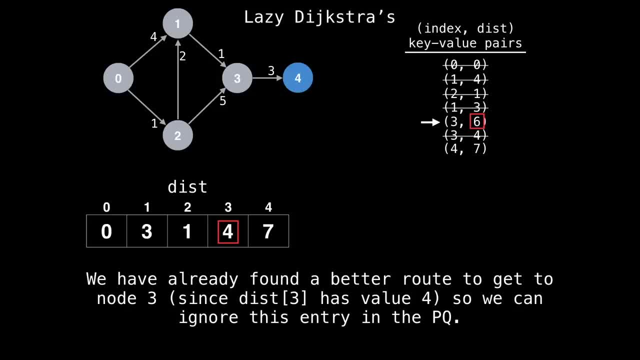 a better route to node three, So skip this entry in the priority queue. Finally, visit node four, And that's all for the lazy implementation of Dijkstra's. there are only a few moving parts, But in large, the only things to really keep track of is the distance array. And finally, 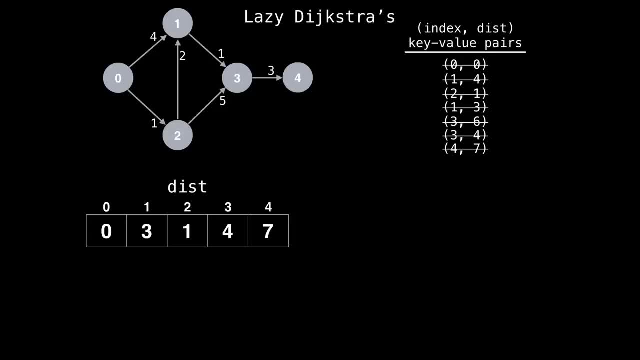 the distance array, which contains the best distance so far from the start node to every other node, and the priority queue, which tells us which node we should visit next, based on the best value found so far. Let's look at some pseudocode for how this works. I'll be 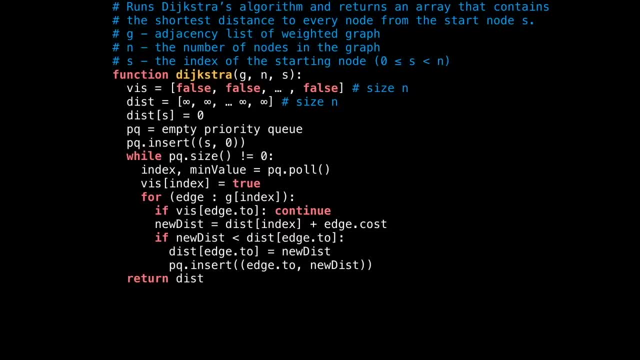 covering the real source code in the next video For those interested. This pseudocode runs Dijkstra's algorithm from a start node and returns the distance array, which tells us the shortest distance To every node in the graph. However, it will not tell you which sequence of edges to follow. 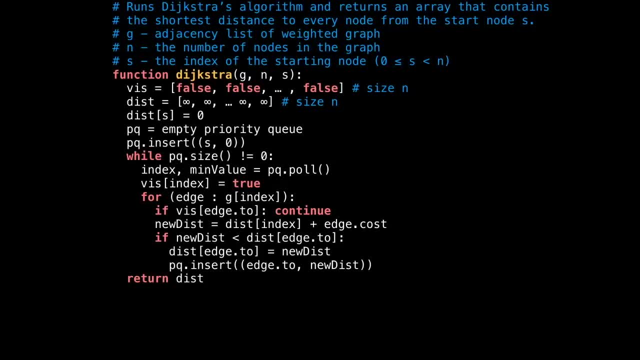 to achieve that optimal distance. This is something that we will need to maintain some additional information for which I will cover as well. So, in terms of the variables we'll need in the function definition, I specify three things. First is G the adjacency list. 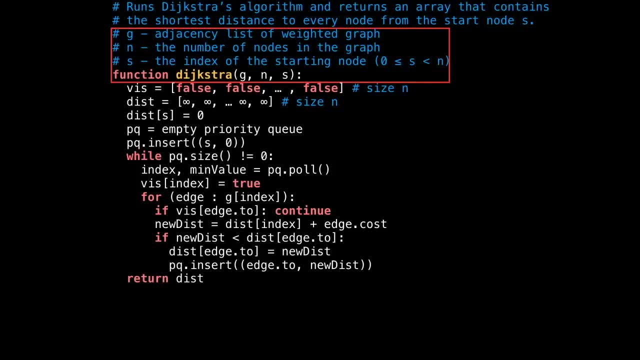 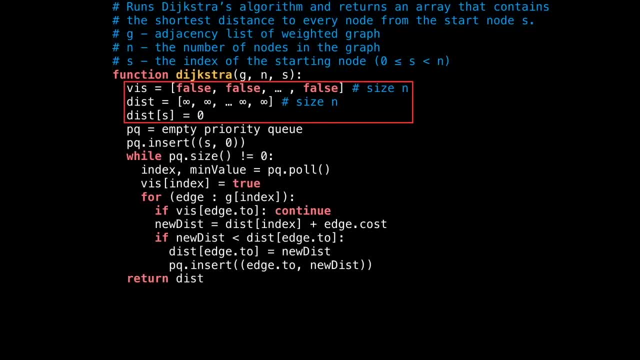 the graph and s the index of the number of nodes in the graph and s the initialized amento, Instead of any an array named id. I always use this bracket when I do any of the atomic operations. The first one we need is the public decor вообще, which returns the number of nodes in the 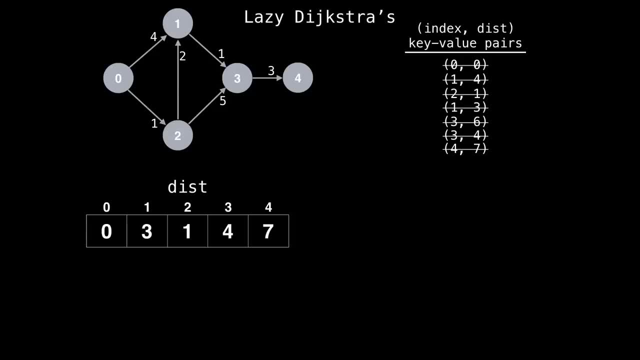 and the priority queue. In that case, we'll look at the value of the run sequence of the first node and the second node to the next. The next step is to use the Dijkstra algorithm to measure the distance between the two nodes in the graph. For this, we'll use the Dijkstra algorithm to run the sequence of nodes in the graph. We'll use the Dijkstra algorithm to measure the distance between the two nodes and the priority queue, which tells us which node we should visit next, based on the best value. 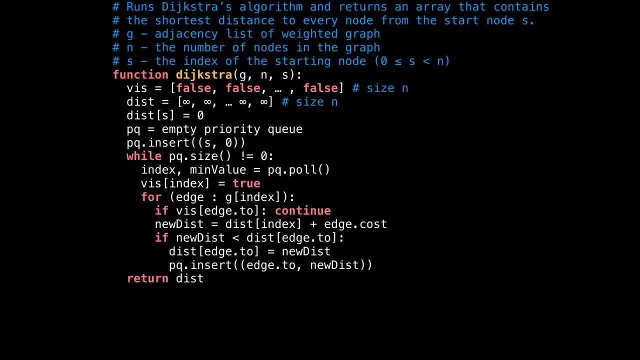 found So far. let's look at some pseudocode for how this works. I'll be covering the real source code in the next video For those interested. this pseudocode runs Dijkstra's algorithm from a start node and returns the distance array, which tells us the shortest distance to every node in the. 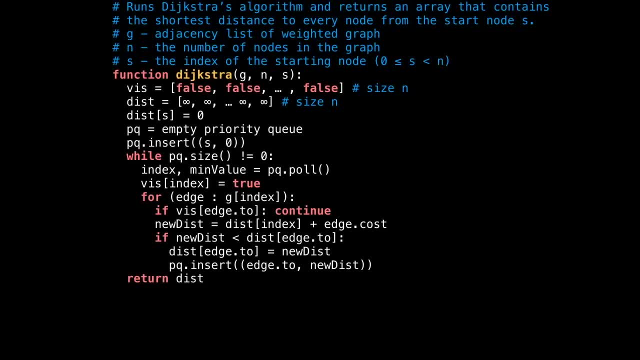 graph. However, it will not tell you which sequence of nodes in the graph will be the shortest, not tell you which sequence of edges to follow to achieve that optimal distance. This is something that we will need to maintain some additional information, for which I will cover. 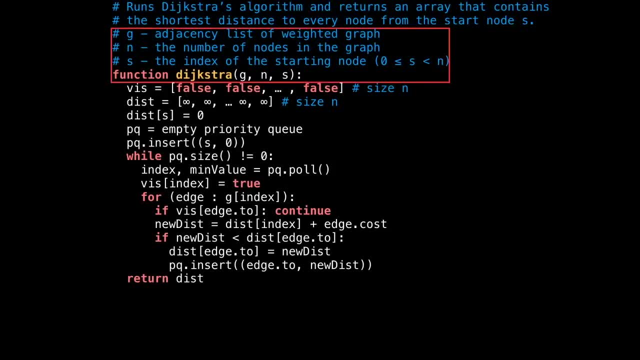 as well. So in terms of the variables we'll need in the function definition, I specify three things: First is G the adjacency list of the weighted graph and the number of nodes in the graph, and s the index of the start node inside the function. I begin by initializing. 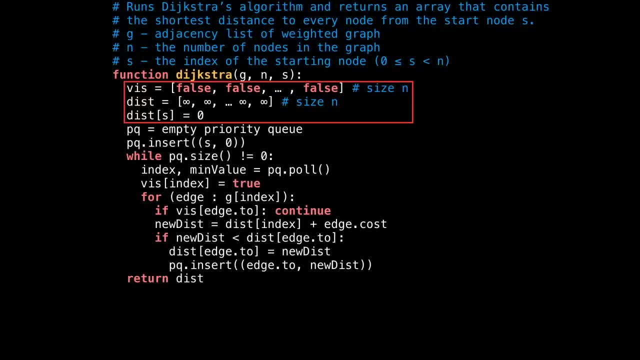 two arrays to keep track of the information we'll need. first is a Boolean array- I called vi s short for visited, which tracks whether node i has been visited or not. then I initialize dist, the distance array, which will be the output of the function. make sure you fill. 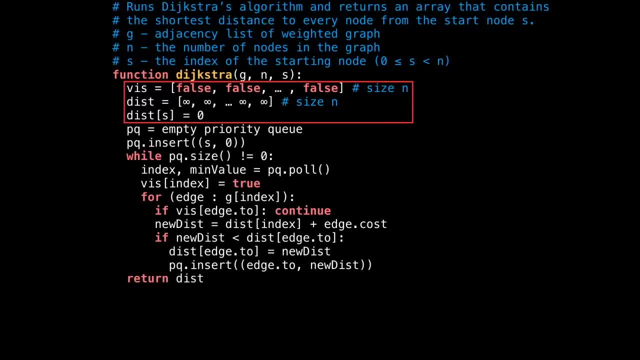 the distance array with positive infinity, except for the start node, which should be set to zero. After this, initialize a priority queue that will store the node index: best distance pairs sorted by minimum distance. you should be able to use the built in priority queue in whatever programming. 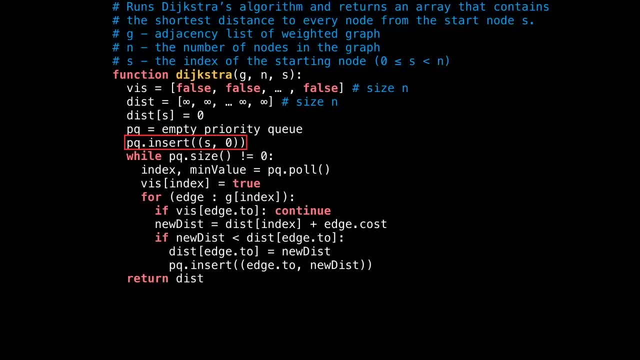 language you're using. Remember to insert the start nodes index, paired with the distance of zero, into the priority queue to kickstart the algorithm. If you're wondering why there are two sets of brackets, that's because the pair s comma zero is meant to represent a. 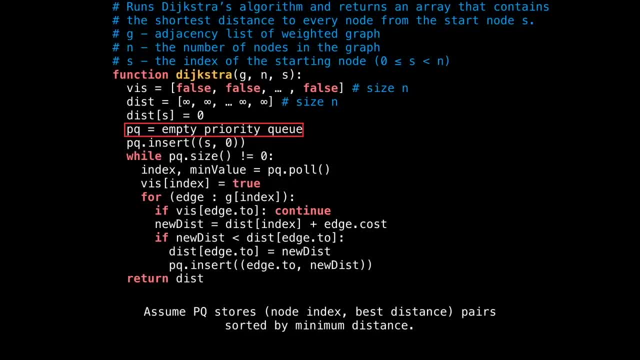 for the node index: best distance pairs sorted by minimum distance. you should be able to use the built in priority queue in whatever programming language you're using. Remember to insert the start nodes index paired with the distance of zero into the priority queue to kickstart the algorithm. If you're wondering why there are two sets of brackets, that's: 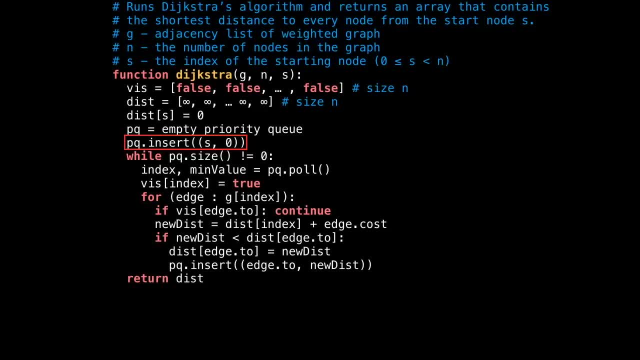 because the pair s comma zero is meant to represent a tuple or an object with two values: a key and a value. So, while the priority queue is not empty, remove the next most promising index, minimum distance pair, and mark that node as visited. then loop over all the neighbors. 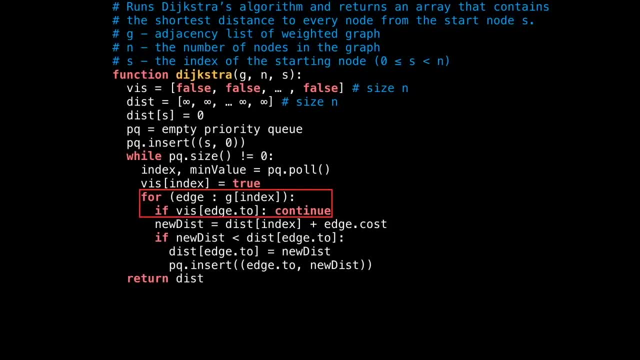 of the current node and skip visited neighbors so that we don't visit them again. then simply perform the edge relaxation operation. First, compute the distance to the new node, which is calculated by adding the best distance from the start node to the current node, which. 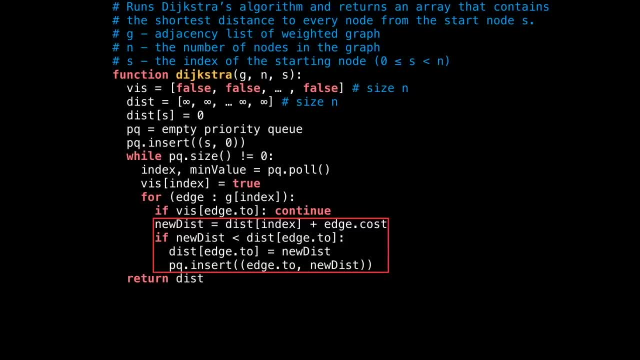 is found: the distance array plus the edge cost of getting to the next node. Once you know that, compare it against the best distance for the next node and update the value. if it's better. then finally insert a new key value pair inside the priority queue. So we visit that node in the future. So in practice, 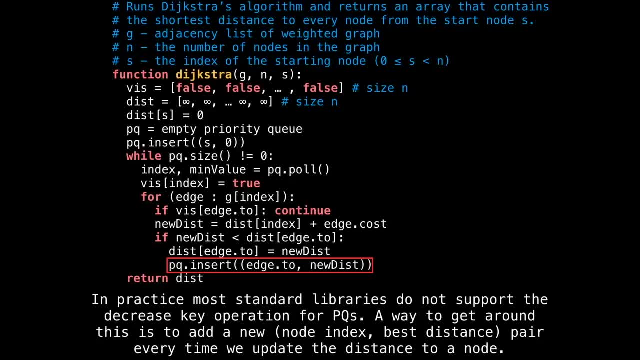 most standard priority queues do not support a decrease key operation. for the built in priority queue, you can think of a decrease key operation as an operation which updates the value of a key in the priority queue. A way to get around this is to add a new node index: best distance pair. every time we need to update the distance. 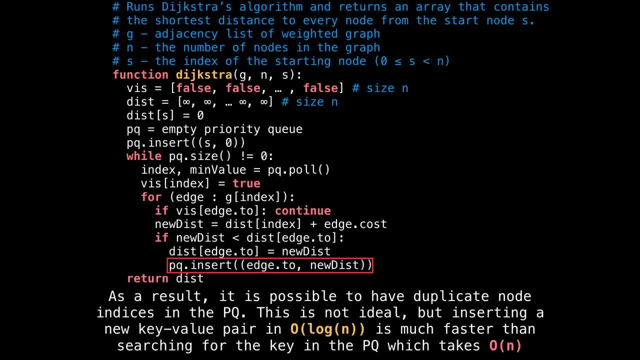 to a node. As a result, it's possible that we have duplicate node indices and the priority queue, like we saw in the animation. this is not ideal, But inserting a new key value pair in logarithmic time is much faster than searching for the key we want to update in the priority. 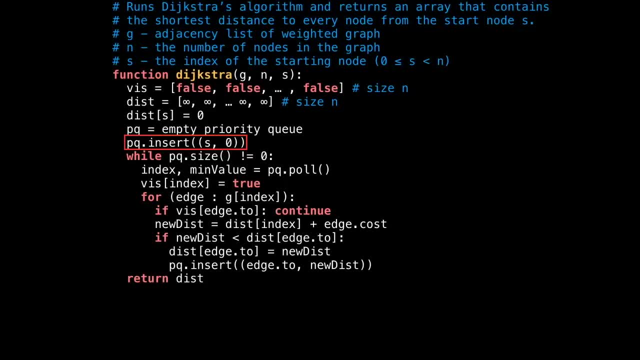 tuple or an object with two values: a key and a value. So, while the priority queue is not empty, remove the next most promising index, Minimum distance pair, and mark that node as visited. then loop over all the neighbors of the current node and skip visited neighbors so that we don't visit them again then simply. 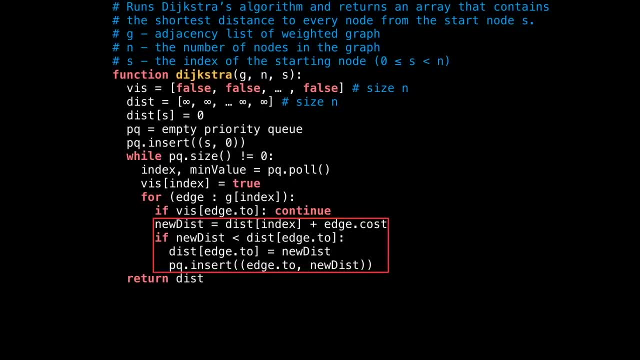 perform the edge relaxation operation, First compute the distance to the new node, which is calculated by adding the best distance from the start node to the current node, which is found the distance array plus the edge cost of getting to the next node. Once you 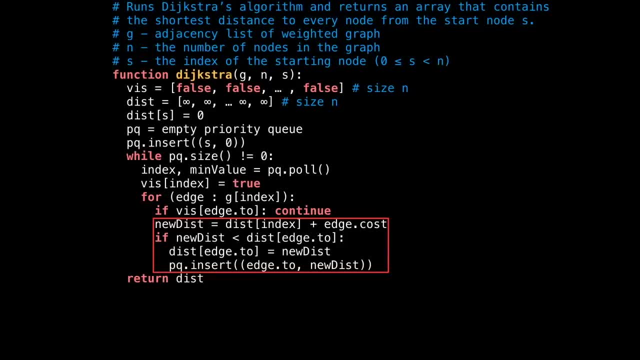 know that, compare it against the best distance for the next node. you should be able to get the best distance from the start node to the next node. Once you know that, compare it against the best distance for the next node And update the value if it's better, then finally insert a new key value pair inside. 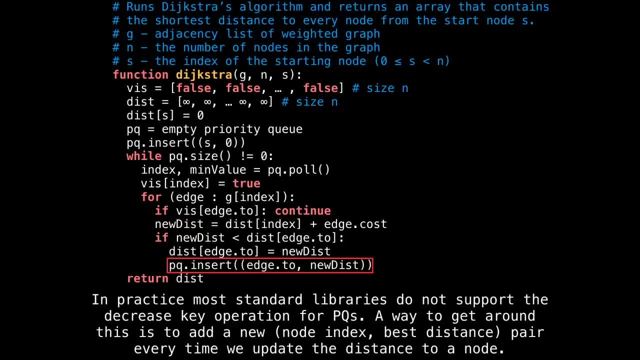 the priority queue. So we visit that node in the future. So in practice most standard priority queues do not support a decrease key operation. for the built in priority queue, you can think of a decrease key operation as an operation which updates the value of 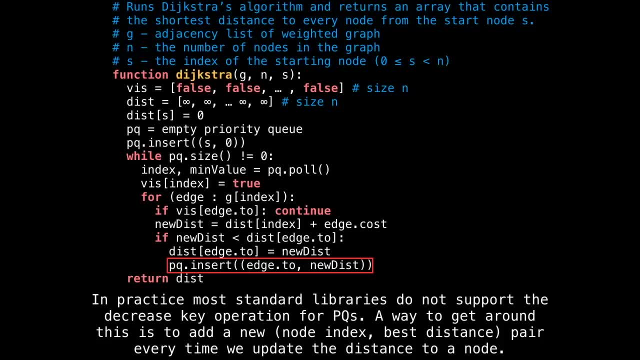 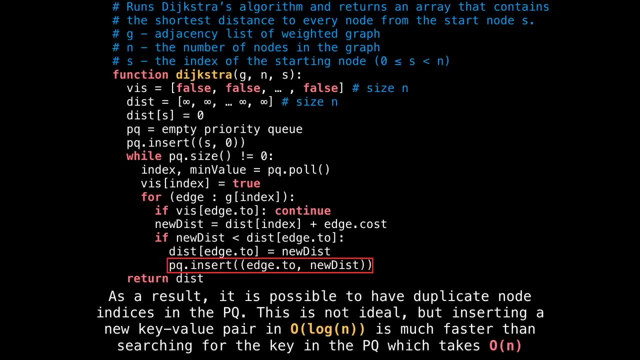 a key and the priority queue. A way to get around this is to add a new node index- best distance pair. every time we need to update the distance to a node. As a result, it's possible that we have duplicate node indices in the priority queue, like we. 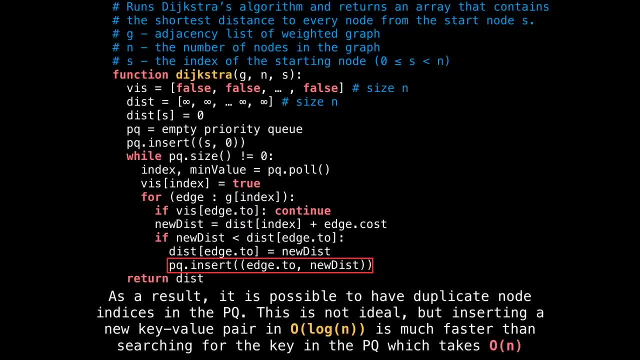 saw in the animation. This is not ideal, but inserting a new key value pair in logarithmic time is much faster than searching for the key we want to update in the priority queue, which actually takes linear time. Yes, searching for a key in a priority queue takes linear. 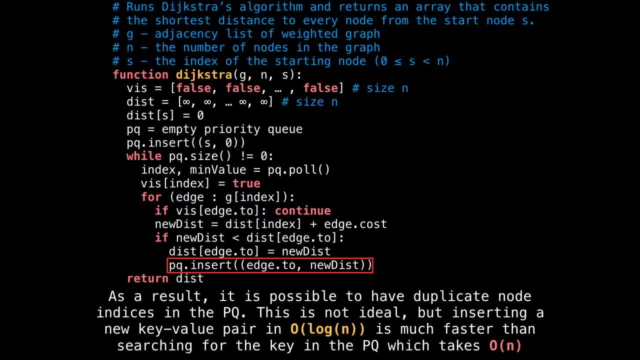 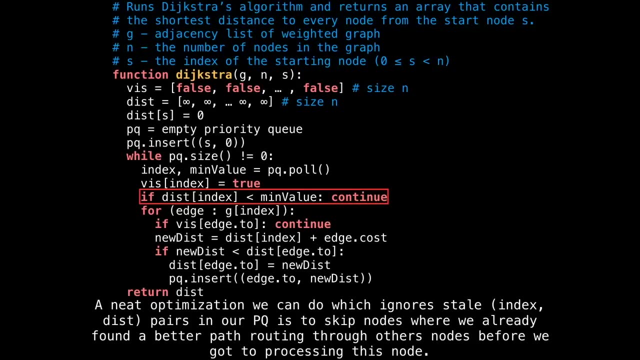 time because the heap is sorted by the keys values, not the keys themselves So effectively. it's like searching In an unordered list for a particular element. A neat optimization we can do which ignores stale, outdated index min distance pairs in our priority queue, is to skip them immediately. 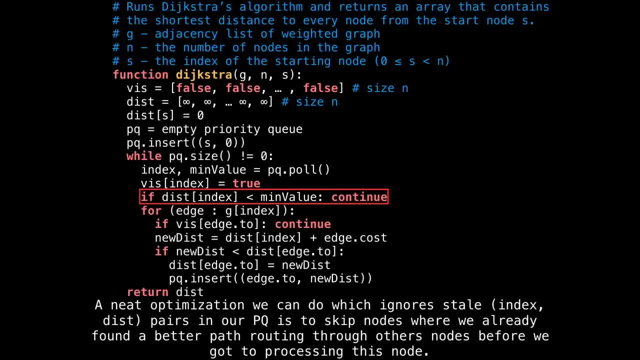 As we pull them from the priority queue. We can do this by checking if the value in the distance array is better than the value in the priority queue, And if it is, then we know we have already found a better Power path routing through other nodes. before we got to processing this note, I'll let that 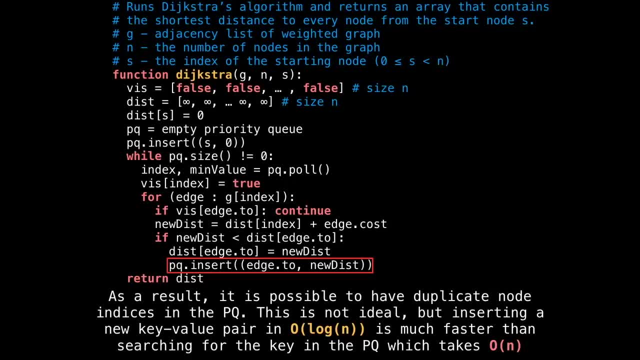 queue, which actually takes linear time. Yes, searching for a key in a priority queue takes linear time Because the heap is saving, which means the prior queue is also very efficient because the heap is sorted by the keys values, not the keys themselves, So effectively it's. 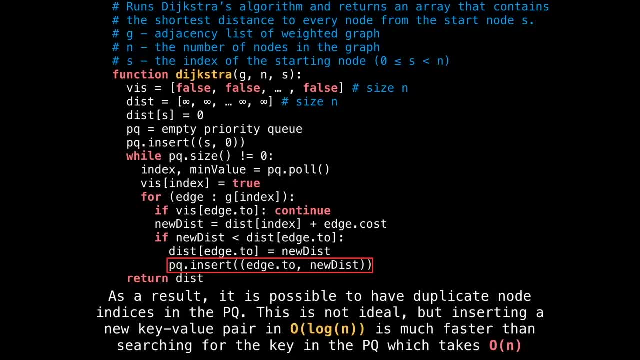 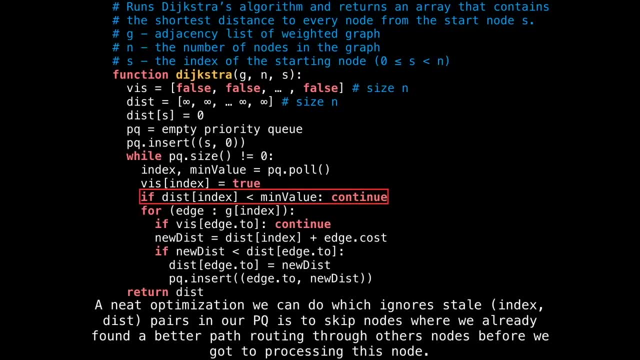 like searching in an unordered list for a particular element. A neat optimization we can do which ignores stale, outdated index min distance pairs in our priority queue, is to skip them immediately As we pull them from the priority queue. We can do this by checking if the value in the distance array is better than the value in the priority queue. 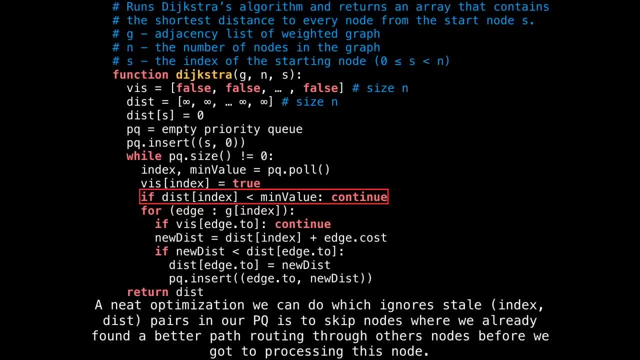 And if it is, then we know we have already found a better path, routing through other nodes before we got to processing this note. I'll let that sink in for a little bit, But this is definitely a neat optimization. you'll want to keep around. Now I want to talk about 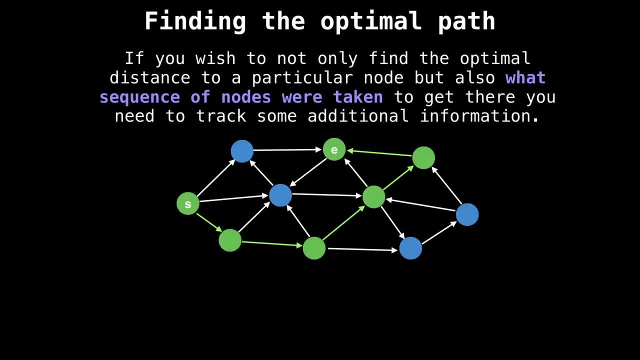 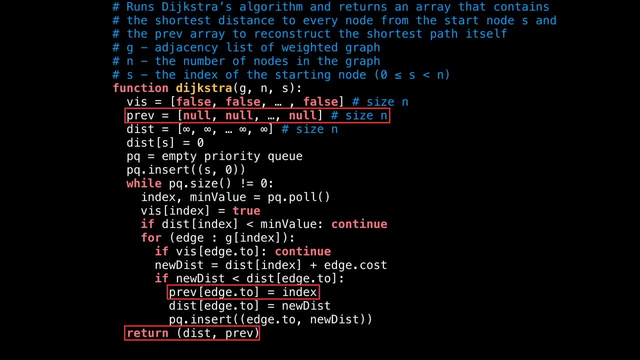 finding the shortest path itself, and not just the shortest distance to get there. To do that, we'll need to keep track of some additional information. In particular, we'll want to keep track of the index of the previous node we took to get to the current node. The way to do this is to maintain a previous array. 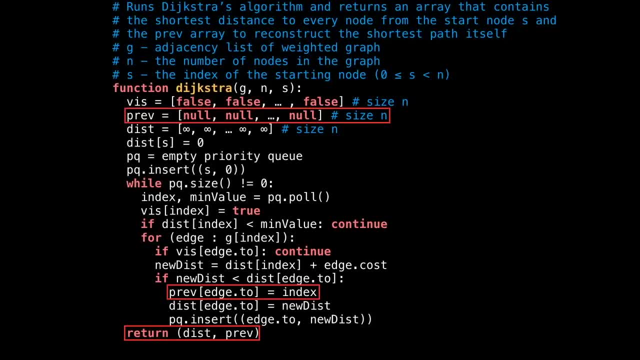 I call Prev In this slide. this array tracks the index of the node you took to get to node I. initially, the previous array should be filled with a sentinel value, such as null or minus one, But as you perform edge relaxation operations, you want to update the index of. 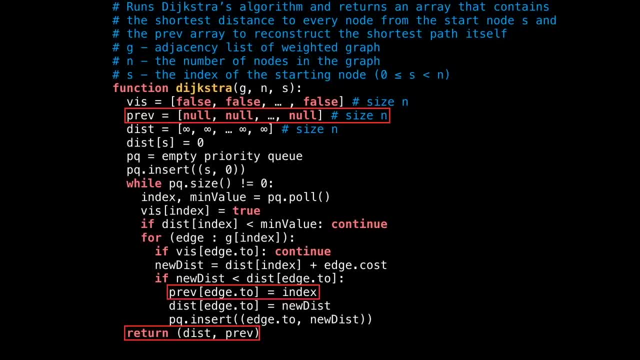 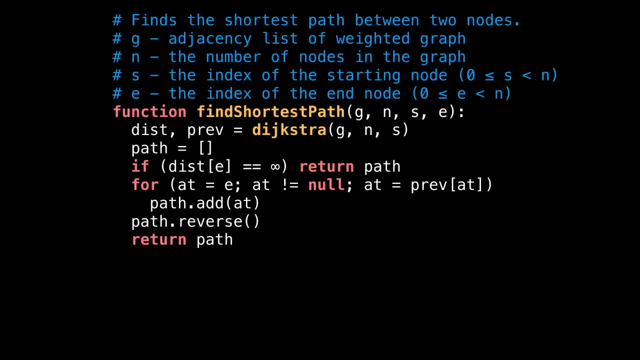 the previous array to say that the node you're going to came from the node you're currently at, then, at the end, instead of returning the distance array, also return the previous array, which we will use soon In another method of perhaps called find shortest path. 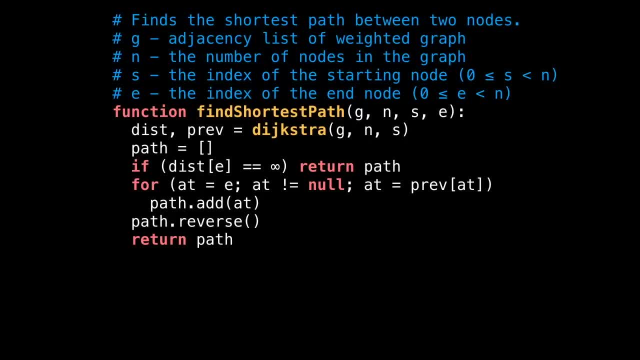 provide all the same arguments with the addition of the end node index and execute Dijkstra's to obtain the distance array and the previous array. With these two bits of information we can reconstruct the previous array and the previous array. So let's go ahead and 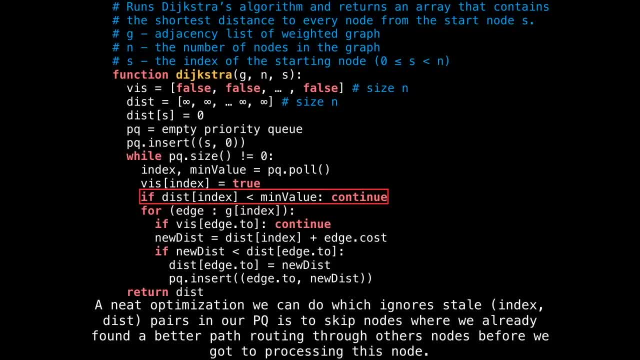 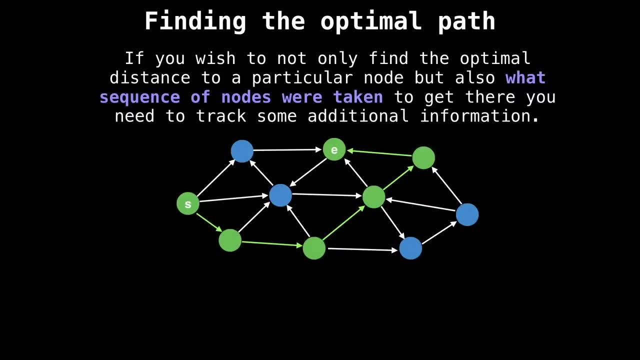 sink in for a little bit, But this is definitely a neat optimization you'll want to keep around. Now I want to talk about finding the shortest path itself, and not just the shortest distance to get there. To do that, we'll need to keep track of some additional information, In particular. 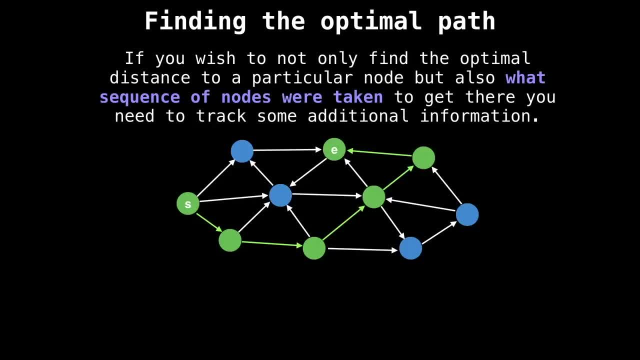 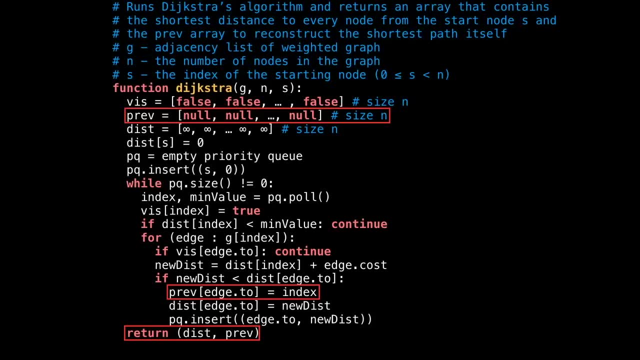 we'll want to keep track of the index of the previous node we took to get to the current node. The way to do this is to maintain a previous array. I call Prev In this slide. this array tracks the index of the node you took to get to node i Initially, the previous array. 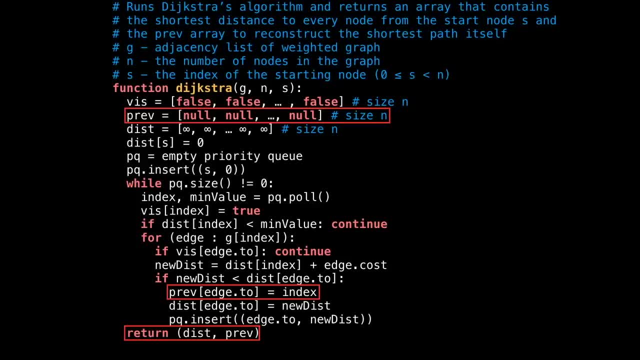 should be filled with a sentinel value such as null or minus one. But as you perform edge relaxation operations, you want to update the previous array to say that the node you're going to came from the node you're currently at. then, at the end, instead of returning, 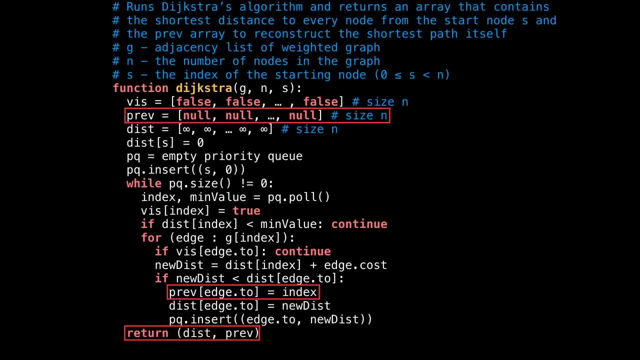 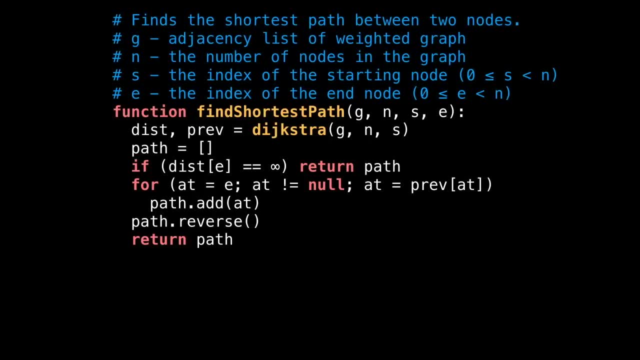 the distance array, also return the previous array, which we will use soon In another method, perhaps called find shortest path, provide all the same arguments with the addition of the end node index and execute Dijkstra's to obtain the distance array and the previous. 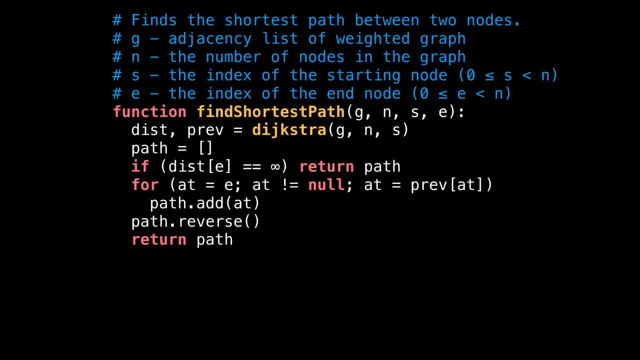 array. With these two bits of information we can reconstruct the shortest path. First check that the end node is reachable by checking that its value in the distance array is not infinity. Then start at the end node and loop backwards through the previous array until you make. 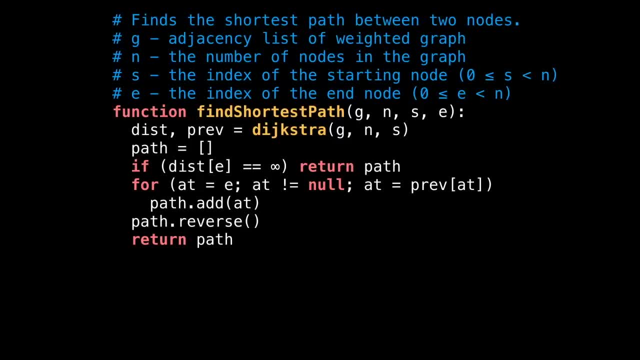 it back to the start node. You know you made it back to the start node when the value of null is reached, since the start node does not have a parent node index, from which came from the resulting path of node indices to follow for the shortest path from the start. 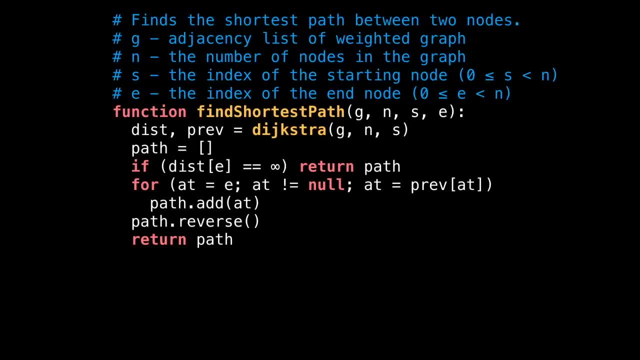 construct the shortest path. First check that the end node is reachable by checking that its value in the distance array is not infinity. then start at the end node and loop backwards through the previous array until you make it back to the start node. You know. 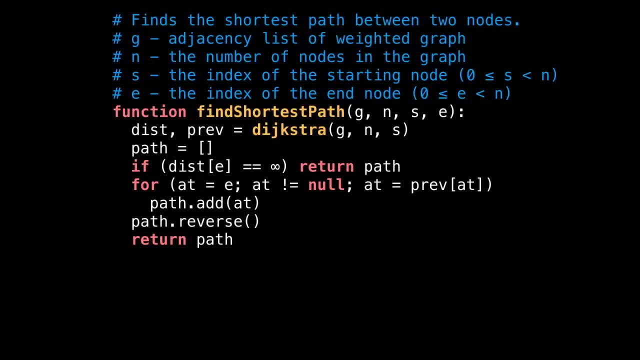 you made it back to the start node when the value of null is reached, since the start node does not have a parent node index, from which came from the resulting path of node indices to follow for the shortest path from the start node to the end node will be in reverse order 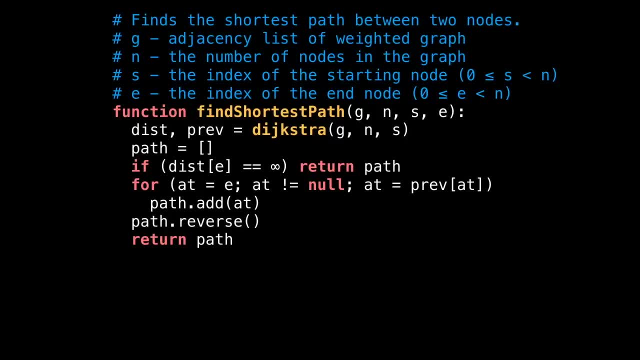 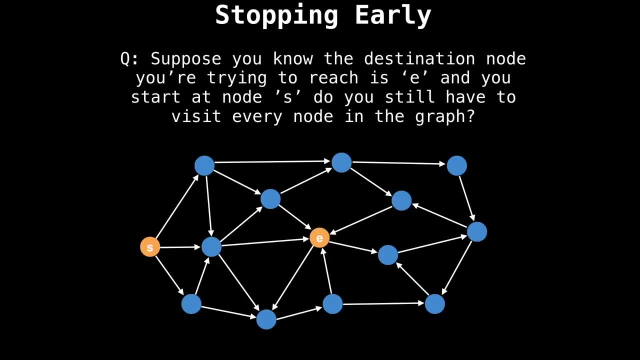 because we've already done that in the previous array, So let's go ahead and check that out. We started at the end node and worked backwards. Therefore, we want to make sure we reverse this array before returning the result. Now I want to talk about a few optimizations. we 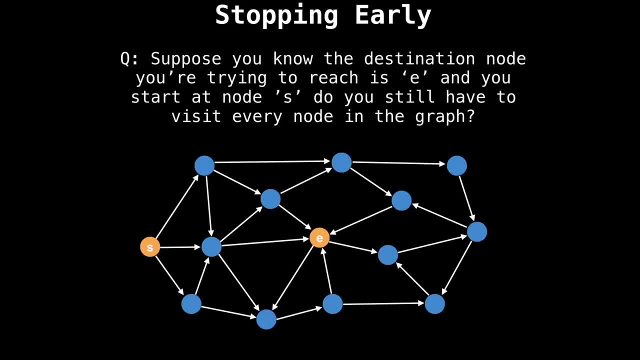 can use to make Dijkstra's algorithm more efficient. Sometimes we know the index of our destination node and don't necessarily need to know the optimal distance to every node in the graph, just that one particular node. So the question is, do we still have? 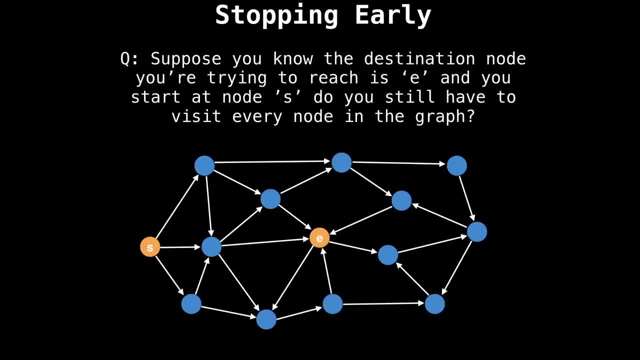 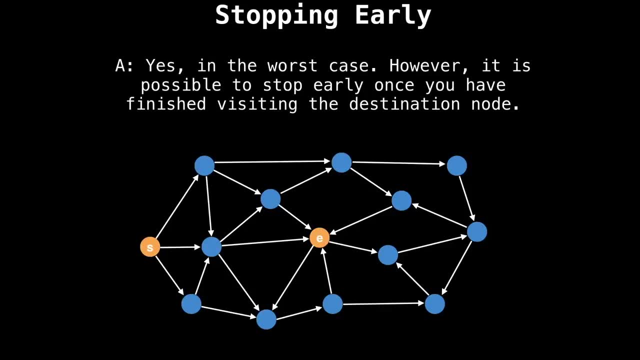 to visit every node in the graph Just to figure out the distance of that one particular node we want to get to? The answer is yes, we do, but only in the worst case, which, depending on your graph, can be somewhat rare. The key realization we'll need to make is that it is possible to stop early once. 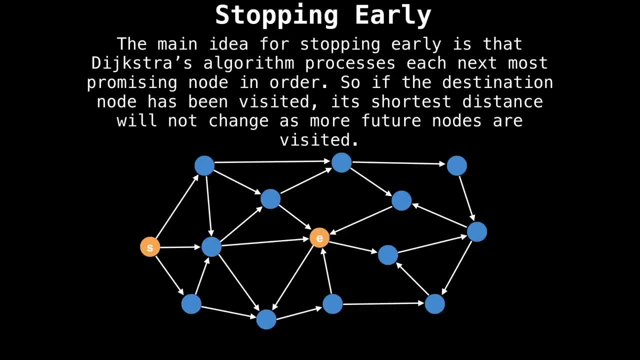 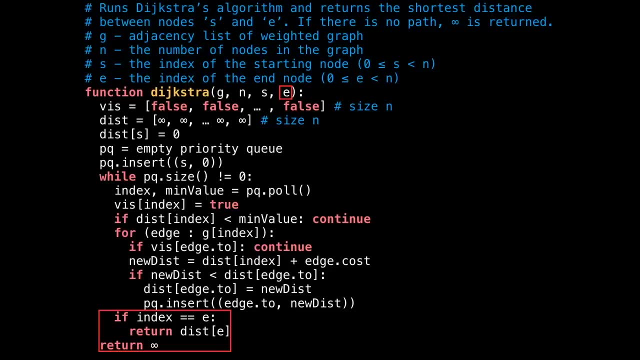 we have finished visiting the destination node. The main idea for stopping early is that Dijkstra's algorithm processes each next most promising node in order. So if the destination node has already been visited, its shortest distance will not change as more future nodes are visited. In terms of code, 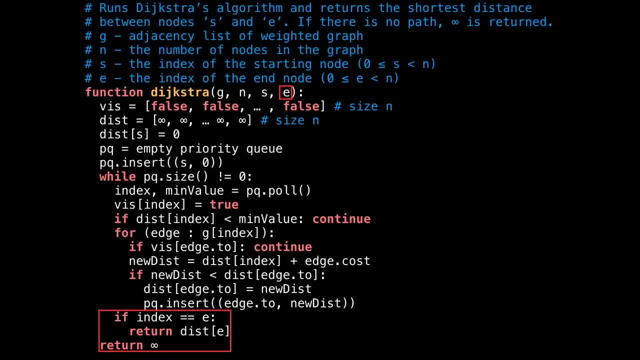 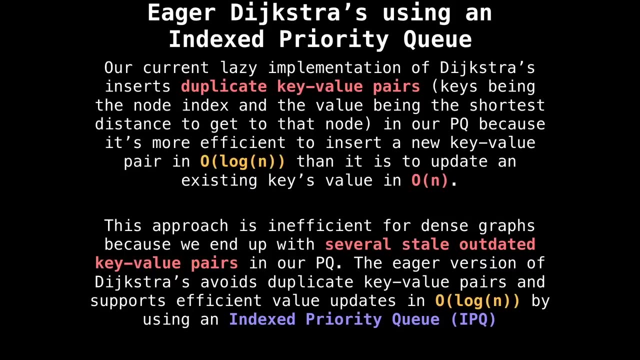 all we have to do to stop early is check if the current node index is the end node and return early. This can prove to be a very substantial speed up depending on how early you encounter the end node while processing the graph. Our current implementation of Dijkstra's 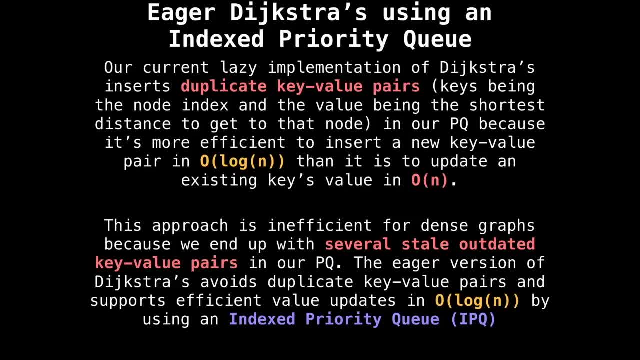 is what we call the lazy implementation, because it inserts duplicate key value pairs and the lazily deletes them. This is done because it's more efficient to insert a new key value pair in logarithmic time into the priority queue than it is to update an existing keys. 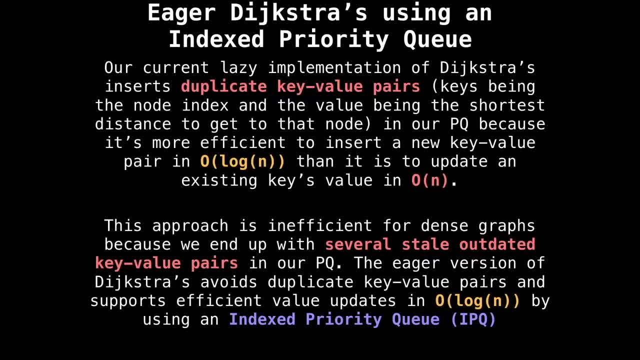 value in linear time. The lazy approach works, but it is inefficient for dense graphs because we end up with all these stale, outdated key value pairs in our party queue. The eager version of Dijkstra's aims to solve this by avoiding duplicate key value pairs and supporting 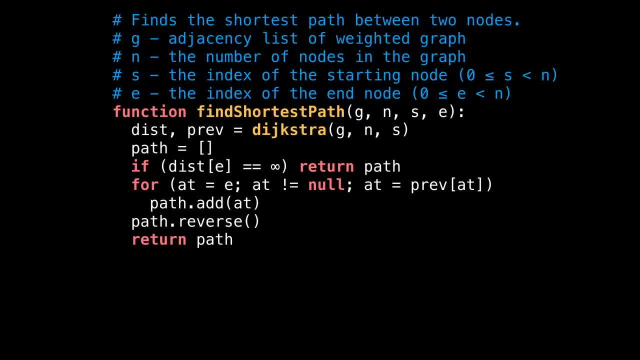 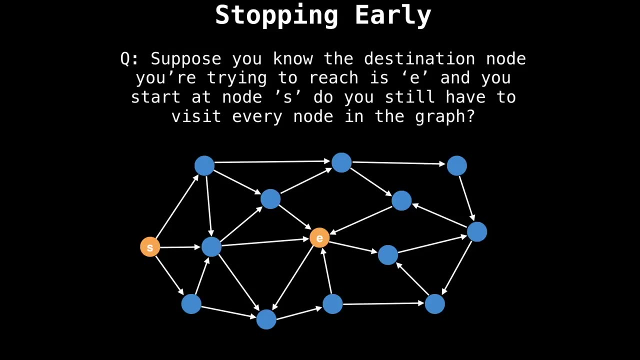 node to the end node will be in reverse order because we started at the end node and worked backwards. Therefore, we want to make sure we reverse this array before returning the result. Now I want to talk about a few optimizations we can use to make Dijkstra's algorithm more. 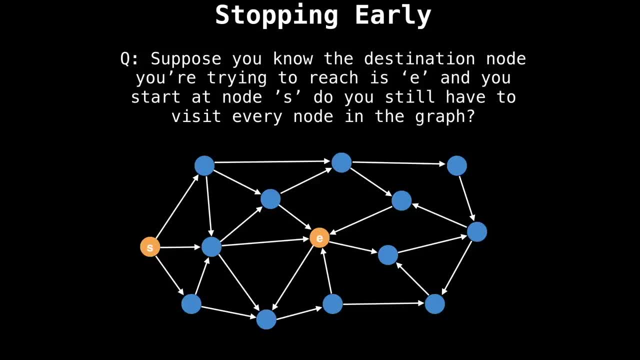 efficient. Sometimes we know the index of our destination node and don't necessarily need to know the optimal distance to every node in the graph, just that one particular node. So the question is, do we still have to visit every node in the graph just to figure? 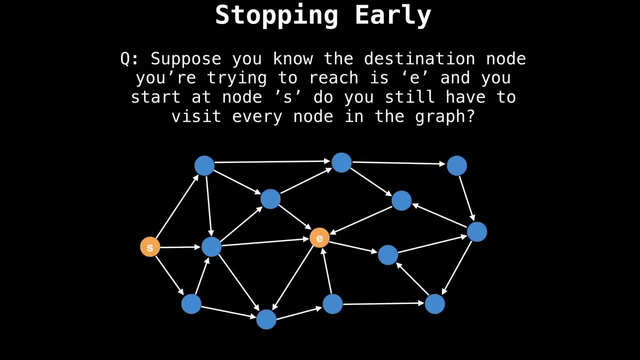 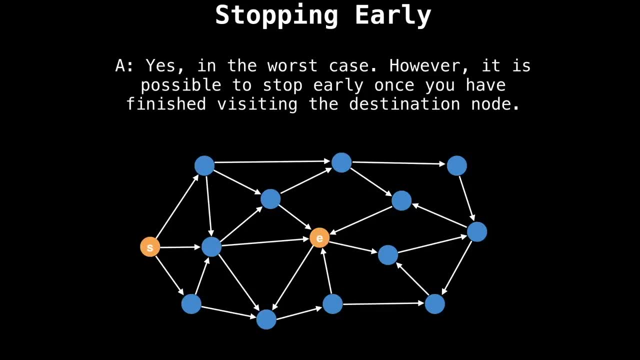 out the distance of that one particular node we want to get to? The answer is yes, we do, But only in the worst case, Which, depending on your graph, can be somewhat rare. the key realization we'll need to make is that it is possible to stop early once we have finished visiting the destination. 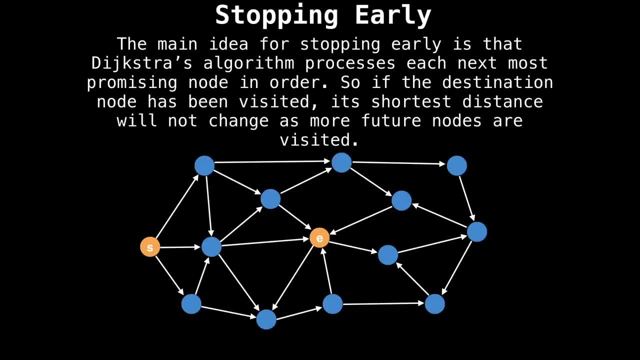 node. The main idea for stopping early is that Dijkstra's algorithm processes each next most promising node in order. So if the destination node has already been visited, its shortest distance will not change as more future nodes are visited. In terms of code, all we have 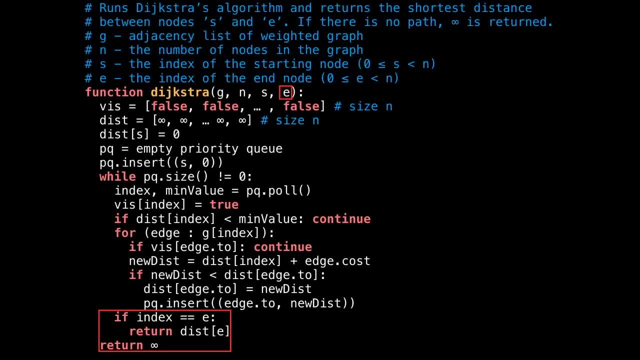 to do to stop early is check if the key realization is correct. If the key realization is correct, then we can stop early once we have finished visiting the destination node- The key realization is that the current node index is the end node- and return early. This can prove to 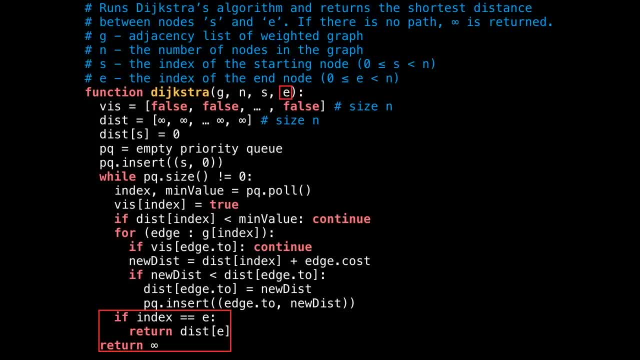 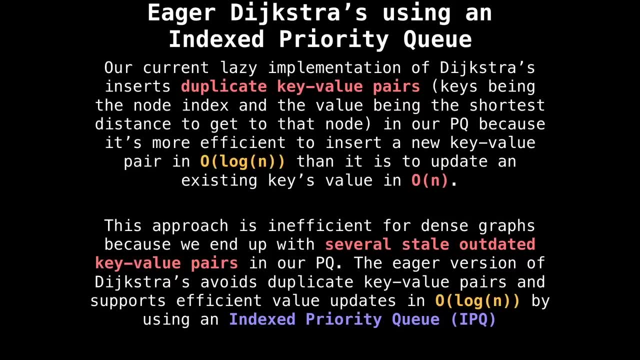 be a very substantial speed up, depending on how early you encounter the end node while processing the graph. Our current implementation of Dijkstra's is what we call the lazy implementation, because it inserts duplicate key value pairs and lazily deletes them. This is done because 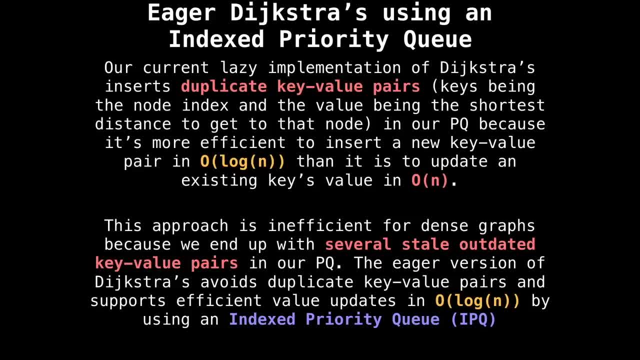 it's more efficient to insert a new key value pair in logarithmic time into the priority queue than it is to update an existing key's value in linear time. The lazy approach works, but it is inefficient for dense graphs because we end up with all these stale, outdated key. 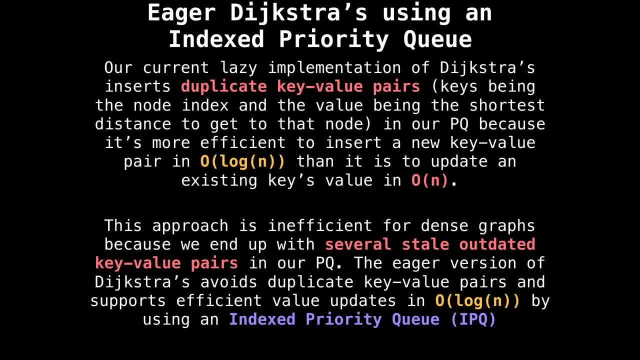 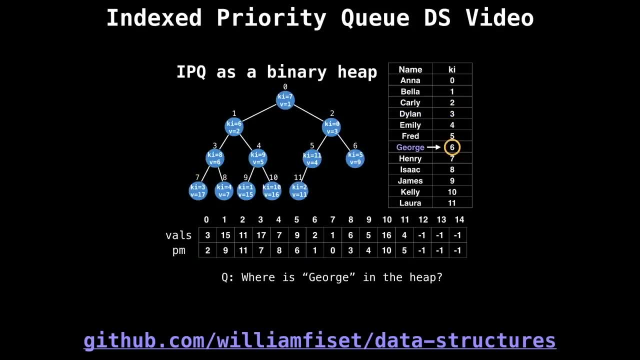 value pairs in our priority queue. The eager version of Dijkstra's aims to solve this by avoiding duplicate key value pairs and supporting efficient value updates in logarithmic time using an indexed priority queue. An index priority queue is a priority queue variant which allows access to key value pairs within the priority queue in constant time and updates. 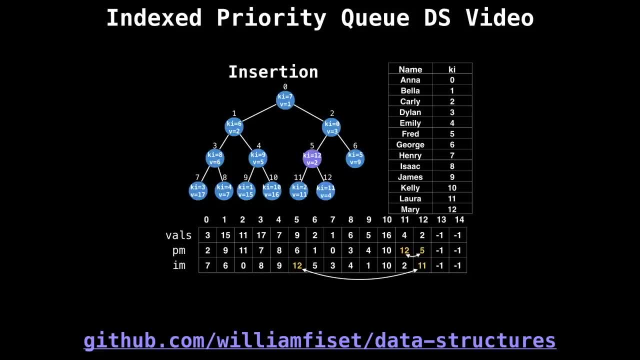 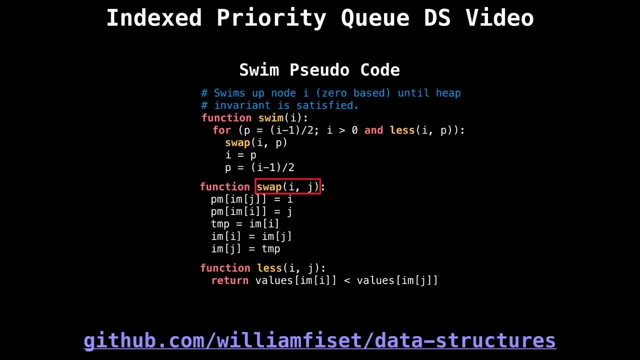 in the log time if you're using a binary heap. This type of priority queue is extremely useful in many applications and I highly recommend you watch my video on the index priority queue to become enlightened. I'll make sure to leave a link in the description, But in the meantime, 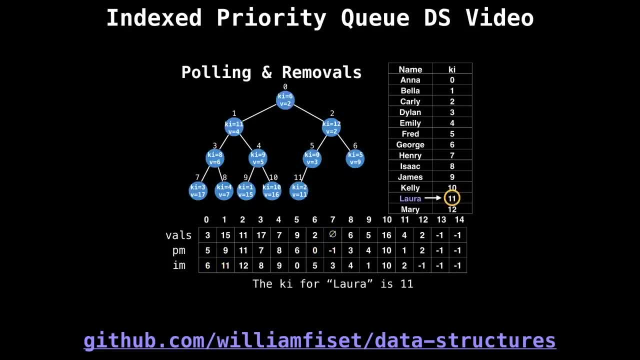 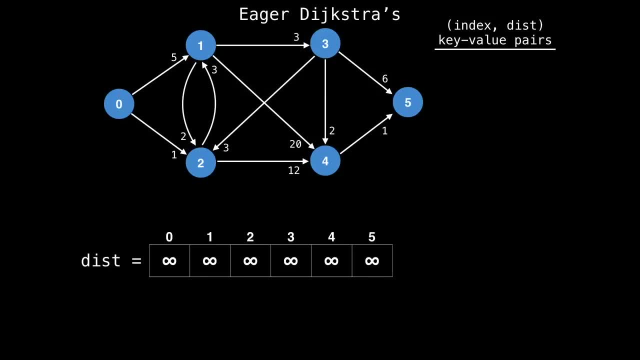 we'll just assume that we have access to an indexed priority queue. Now we're going to take a look at the eager version of Dijkstra's algorithm, where we don't have duplicate keys in the priority queue. So, to start with, assign a distance of zero to the start node at index zero in the distance array. Also insert the. 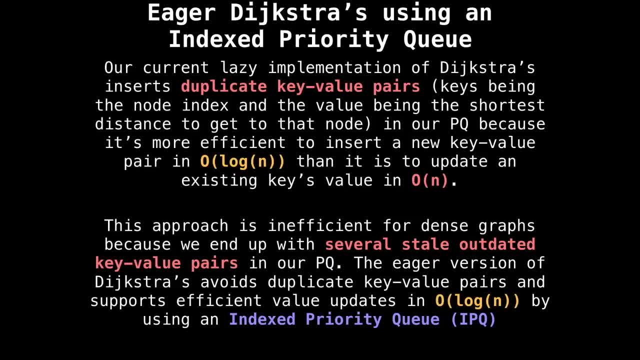 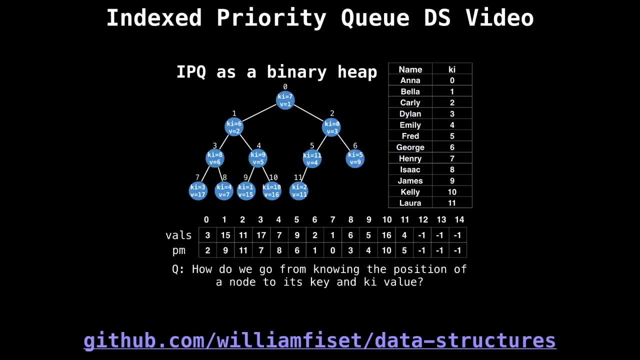 efficient value updates In logarithmic time using an indexed priority queue. An index priority queue is a priority queue variant which allows access to key value pairs within the priority queue in constant time and updates in the log time. if you're using a binary heap, This type of priority 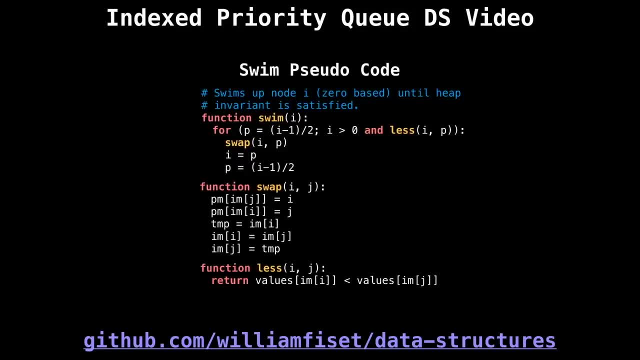 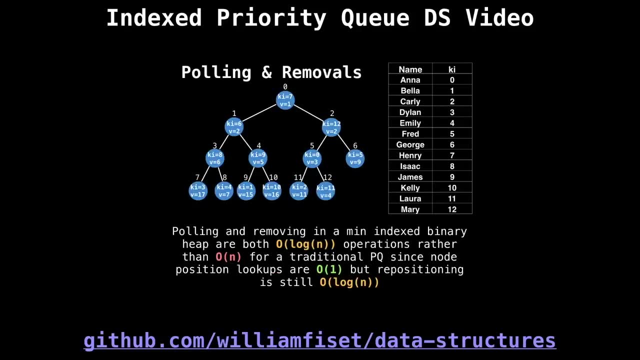 queue is extremely useful in many applications and I highly recommend you watch my video on the index priority queue to become enlightened. I'll make sure to leave a link in the description below, But in the meantime we'll just assume that we have access to an indexed priority. 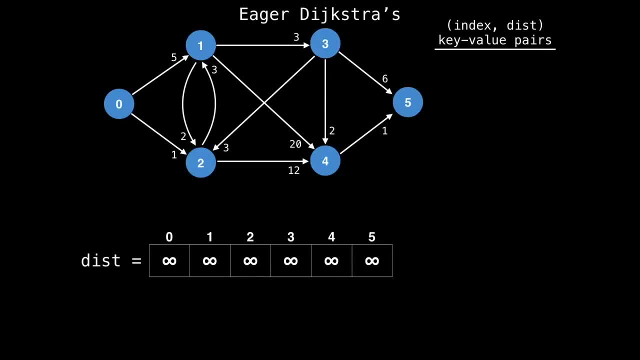 queue. Now we're going to take a look at the eager version of Dijkstra's algorithm, where we don't have duplicate keys and priority queue. So to start with, assign a distance of zero to the start node at index zero in the distance array. Also insert the key value. 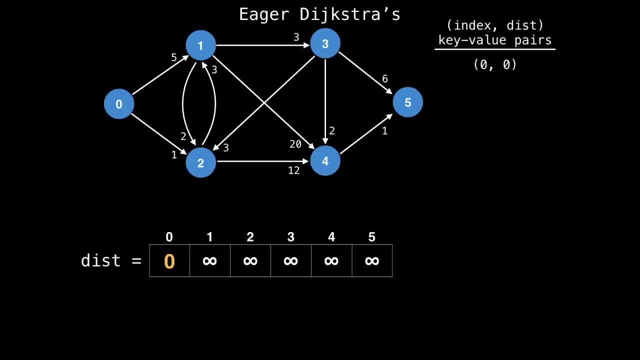 pair zero comma zero into the priority queue to indicate that we intend on visiting node zero with the best distance of zero. Then the algorithm starts and we look inside the priority queue First time and we discover we should visit node zero. From node zero we can visit node. 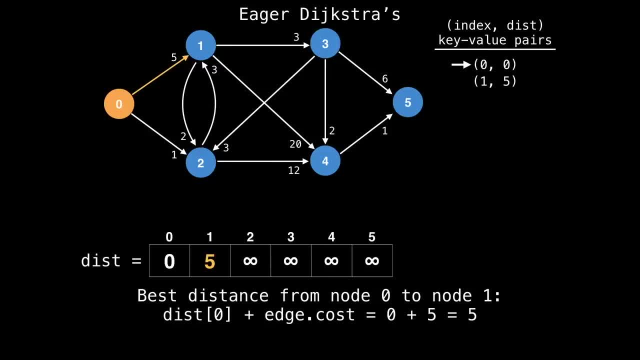 one by taking the edge with cost five. this gives us the best distance of five. So we update the best distance from infinity to five in the distance array. Also add this information to the priority queue. Next we can visit node two from node zero, just like. 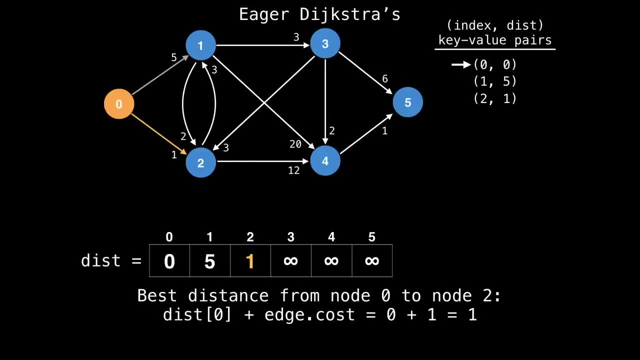 the last node. we can update the optimal distance to reach node two from infinity to one. Additionally, add node two to the priority queue with a distance of one. That concludes visiting all the edges for node zero. To decide which node to visit next, 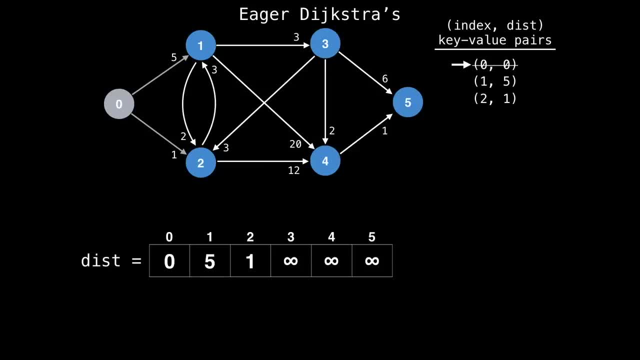 Dijkstra selects the next most promising node in the priority queue. So pull the next best key value pair from the priority queue. No two is that next most promising node because it has a distance of one from the start node, which is better than five From node two. 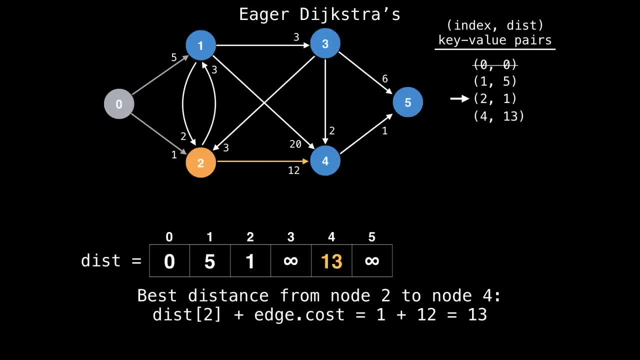 we can take the sideways edge to improve the best distance to note for it to be 13.. And then we can add the best distance to node four, to be 13.. And then we can add the best distance to node one by taking the current best distance from node two, which is one. 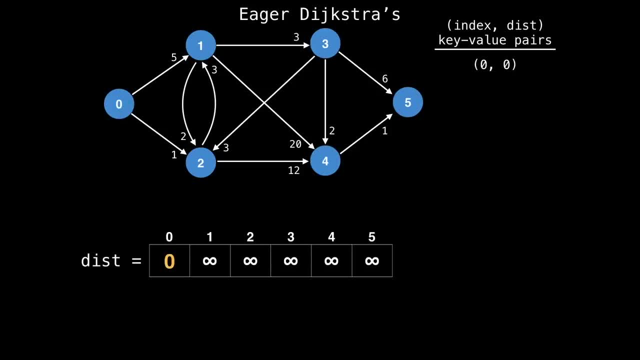 key value pair zero, comma zero into the priority queue to indicate that we intend on visiting node zero with the best distance of zero. then the algorithm starts and we look inside the priority queue for the first time And we discover we should visit node zero From. 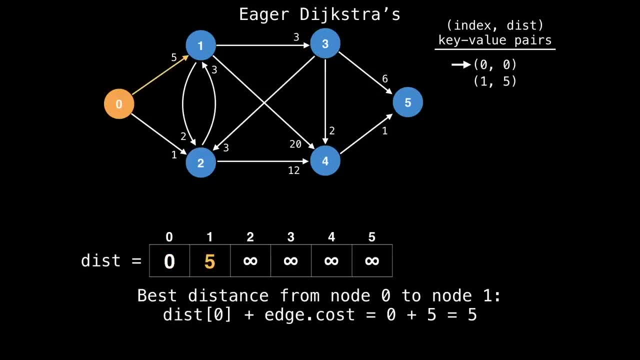 node zero. we can visit node one by taking the edge with cost five, And then we can also update the best distance of five. This gives us a best distance of five. So we update the best distance from infinity to five and the distance array Also. add this information. 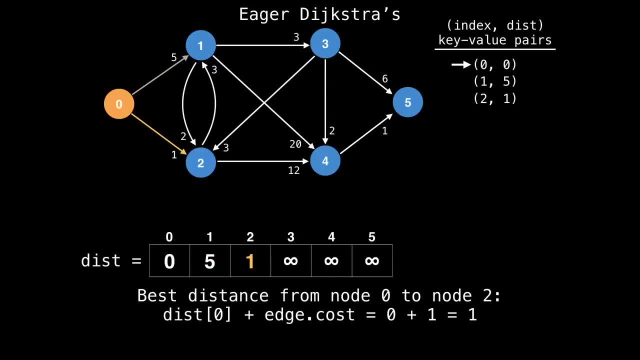 to the priority queue. Next we can visit node two from node zero, just like the last node. we can update the optimal distance to reach node two from infinity to one. Additionally add node two to the priority queue with a distance of one. That concludes visiting all. 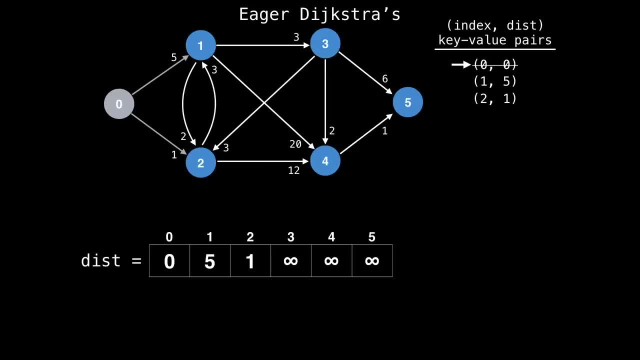 the edges for node zero. To decide which node to visit next, make sure to select the next most promising node in the priority queue. So pull the next best key value pair from the priority queue. No two is that next most promising node because it has a distance of one from the start node, which is better than five From node two. 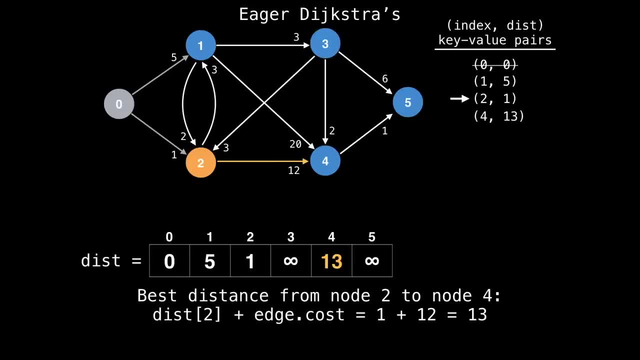 we can take the sideways edge to improve the best distance to node four, to be 13.. By taking the current best distance from node two, which is one, plus the edge cost of 12, to get to node four, for a total cost of 13.. 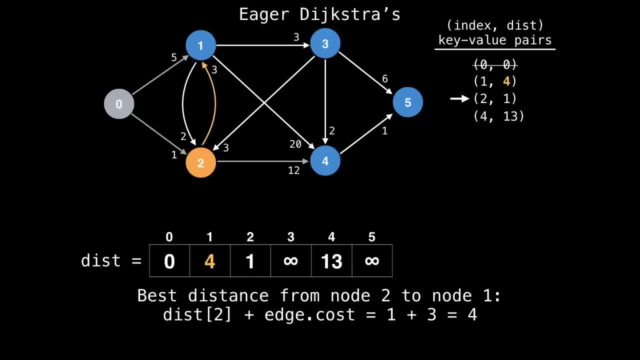 We can update the best distance to node one by taking the upwards edge from node two. Notice that I did not insert a new key value pair with a value of one comma four inside the priority queue, but rather simply updated the existing value in the priority queue from. 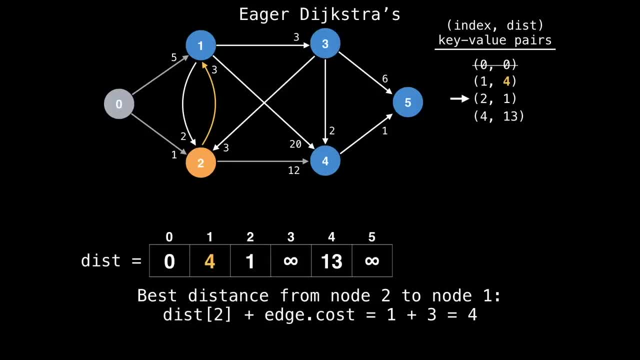 five to four. This is the main difference between the lazy and the eager version. The next most promising node is node one. When taking the downwards edge from node one to node two, we discover that node two has already been visited, So we cannot improve its already best distance. we also cannot 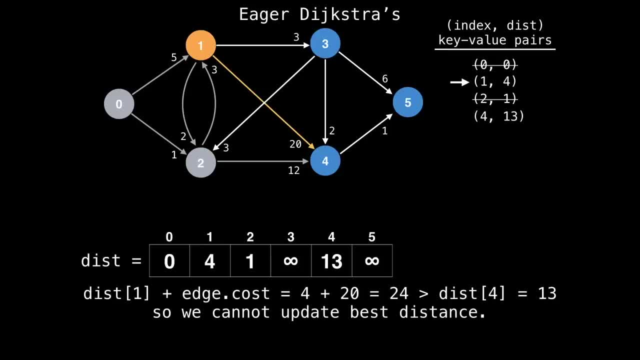 improve the best distance node forward by taking the diagonal downwards edge, since the total cost of 24 outweighs the best distance of 13,, which is already known for that node. However, we can improve the best distance, node three, by taking the edge from node one. 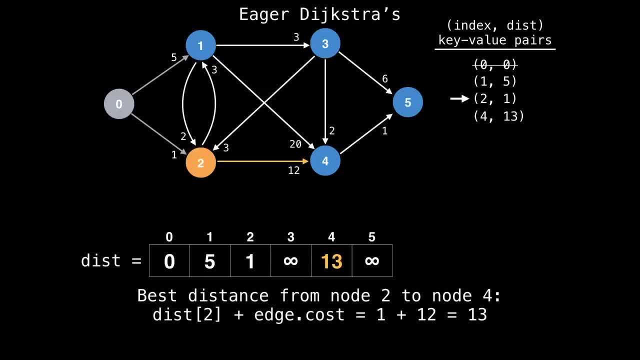 plus the edge cost of 12 to get to node four for a total cost of 13.. We can update the best distance to node one by taking the upwards edge from node two. Notice that I did not insert a new key value pair with a value of one comma four inside the priority queue. 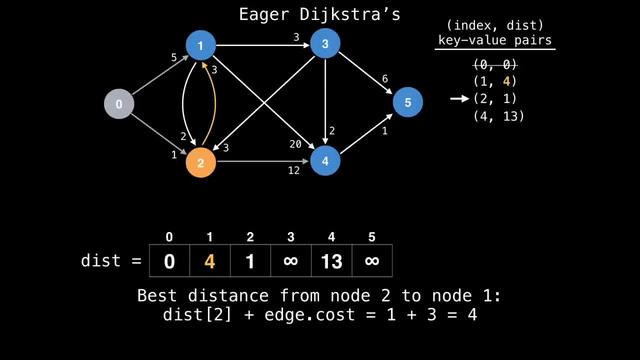 but rather simply updated the existing value in the priority queue from five to four. This is the main difference between the two values. I think this graph shows the Pittsburgh farm, or is the next-most promising node, is node one. when taking the downwards edge from node one to 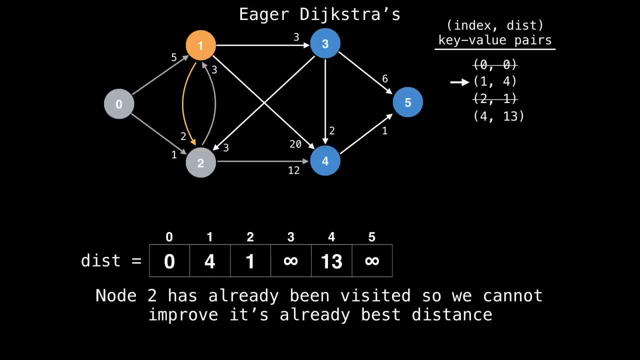 node two would discover that no two has already been visited, So we cannot improve its already best distance. We also cannot improve the best distance, node four, by taking the diagonal downwards edge, since the total cost of 24 outweighs the best distance of 13.. Of course, 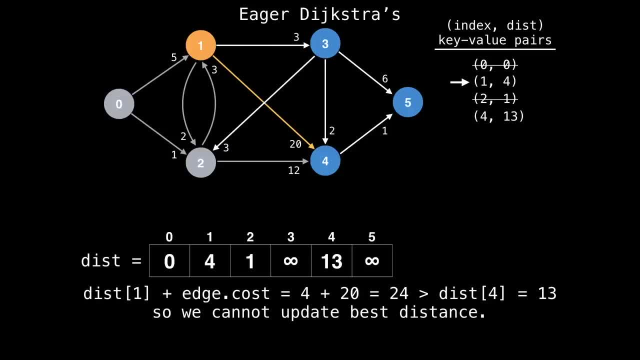 by ending the first power step, by ending the value of 23.. The second tore will go through. the two are the most promisingwd node again, aunque this is actually from our last time here. as of highwayalia node two, 你们 see that the power damage is not significant because there is no super-stonte range temperature. 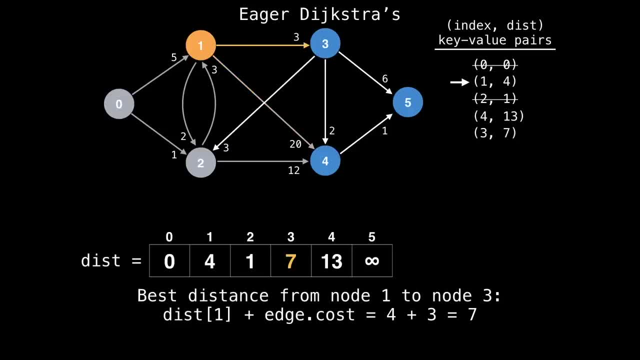 On the depends on the journey 13,, which is already known for that note. However, we can improve the best distance, node three, by taking the edge from node one to node three with a cost of three. I'll let the animation play And, as it does, try and predict what the next move for the algorithm. 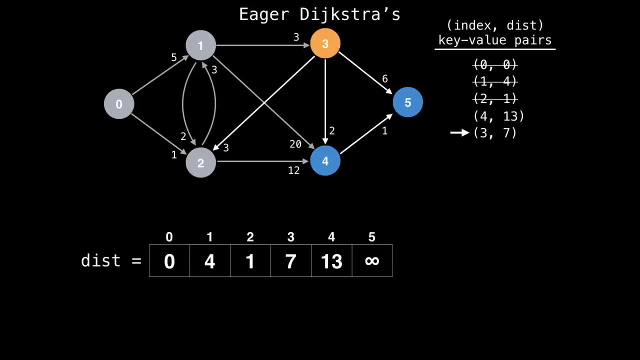 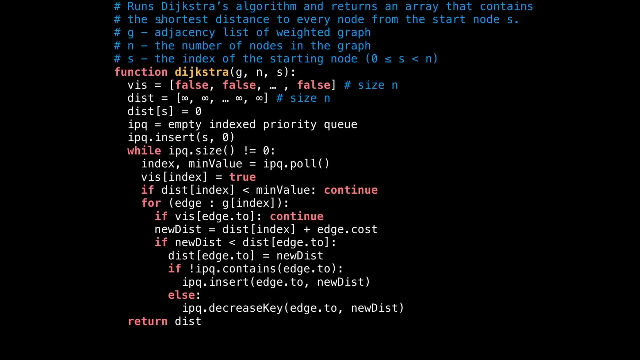 will be. So that's the eager version of Dijkstra's algorithm, which I would say is the more proper way of implementing Dijkstra's algorithm. Now let's look at some pseudocode and see what needs to change. First, notice that we're using. 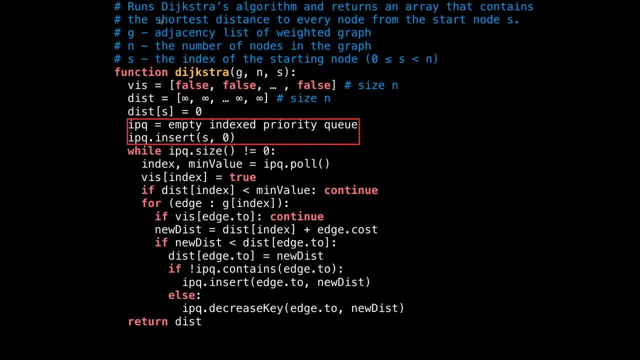 an indexed priority queue instead of a regular priority queue. Also, notice that we no longer need to wrap our key value pairs as tuples in an object, because index party queues have first class support for key value pairs as opposed to a priority queue, which you would. 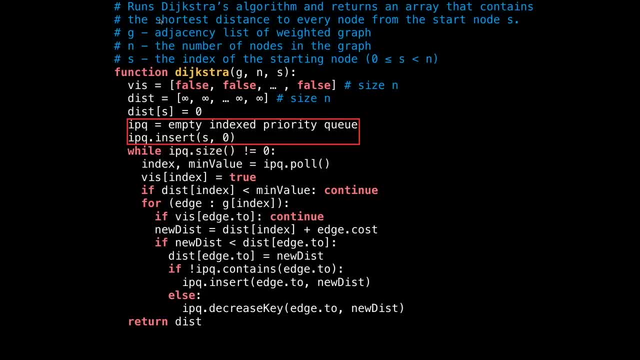 find in your programming languages standard library. The other thing that needs to change is how we insert key value pairs into the priority queue. If the key or node index does not yet exist in the indexes priority queue inserted, otherwise, invoke the decrease key operation to update. 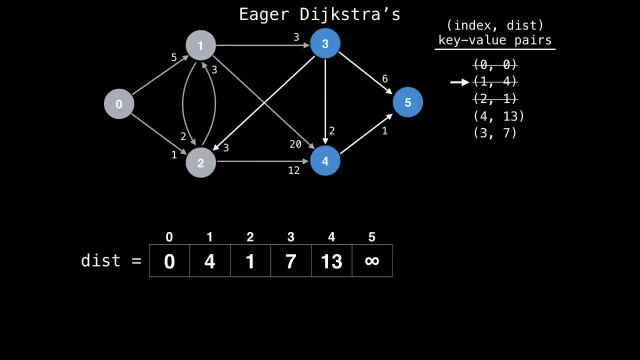 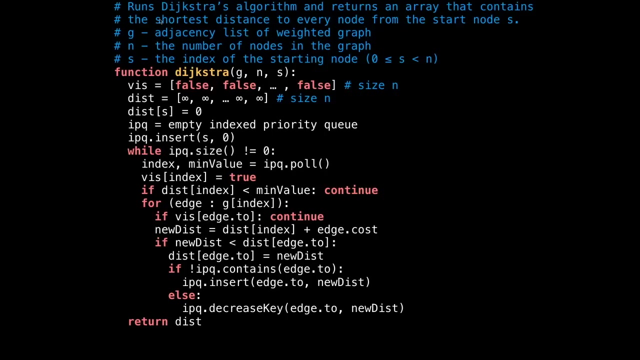 to node three with a cost of three. I'll let the animation play And, as it does, try and predict what the next move for the algorithm will be. So that's the eager version of dixtra's algorithm, which I would say is the more proper way of. 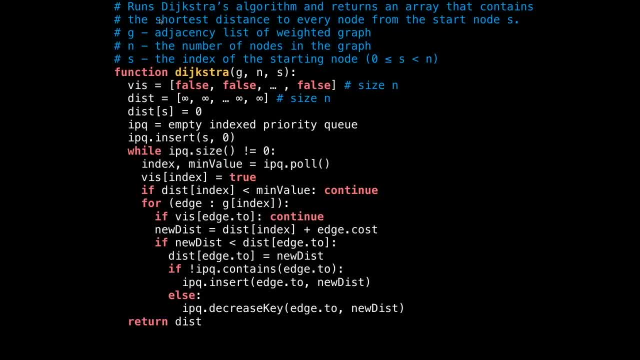 implementing dixtra's algorithm. Now let's look at some pseudocode and see what needs to change. First, notice that we're using an indexed priority queue instead of a regular priority queue. Also, notice that we no longer need to wrap our key value pairs as tuples. 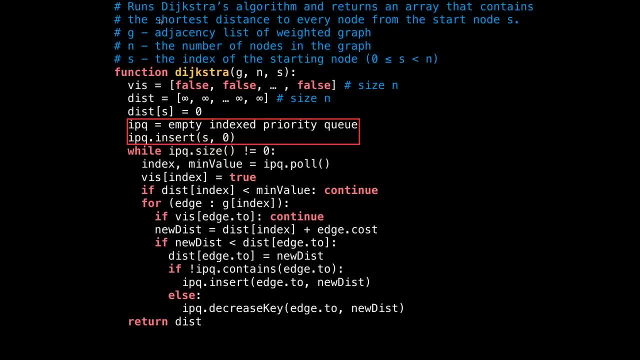 in an object, because indexed priority queues have first class support for key value pairs as opposed to regular priority queue. There are two different ways to do this. First, to a priority queue, which you would find in your programming languages standard library. The other thing that needs to change is how we insert key value pairs into the party queue. 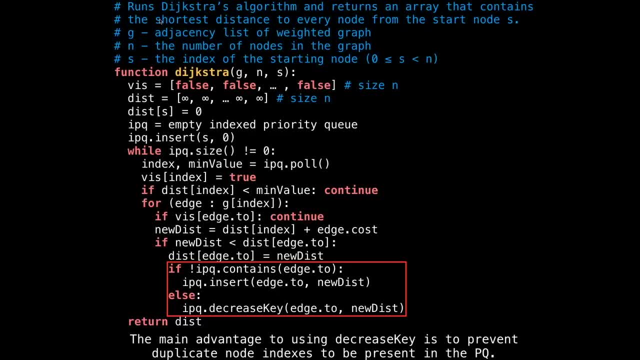 If the key or node index does not yet exist in the index party queue, insert it. Otherwise, invoke the decrease key operation to update the best distance to that node and party queue. The operation is called decrease key instead of update because it only updates the value. 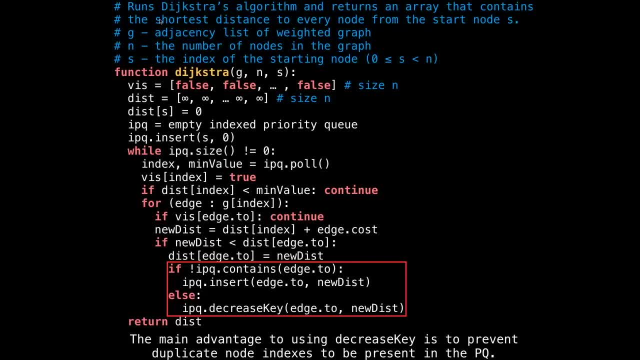 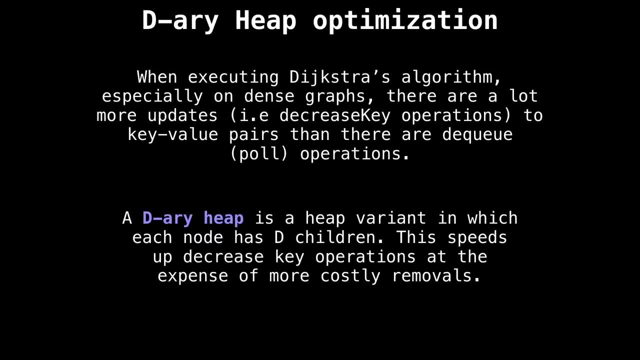 if it is strictly less than the current value in the party queue. Alright, we've looked at several Dijkstra optimizations already, But there's one key last optimization I want to talk about, And that is improving the heap we're using Currently. 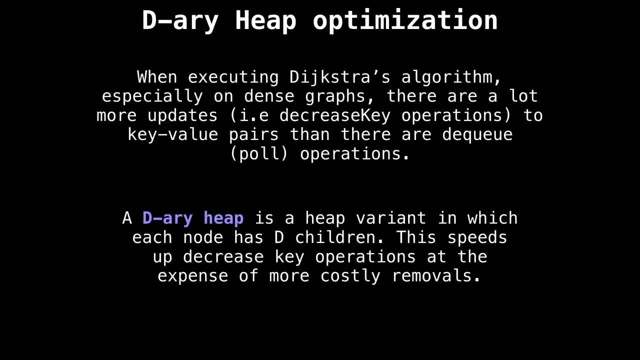 we're probably using an indexed binary heap for our priority queue, But we can do better. The thing to notice is that when executing Dijkstra, there are a lot more update operations, especially on dense graphs, than there are removal operations. A dairy heap is a heap. 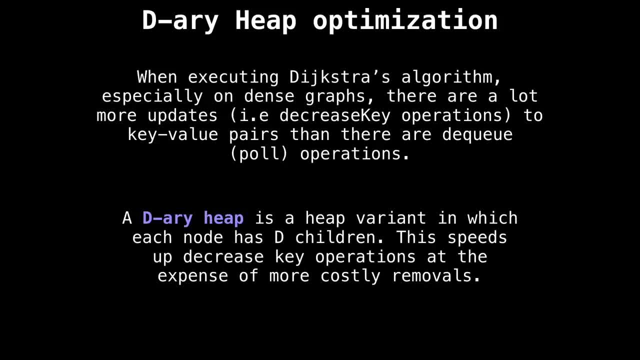 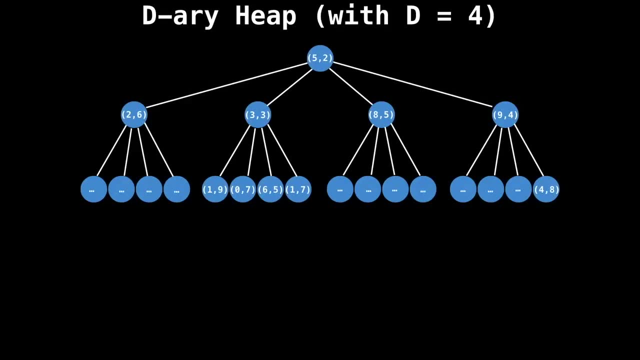 variant in which each node has at most D children instead of two. This speeds up the decrease key operation at the expense of more costly removals. So if we look at an example real quick, this is a dairy heap with D equals four. Suppose we want to perform an update. 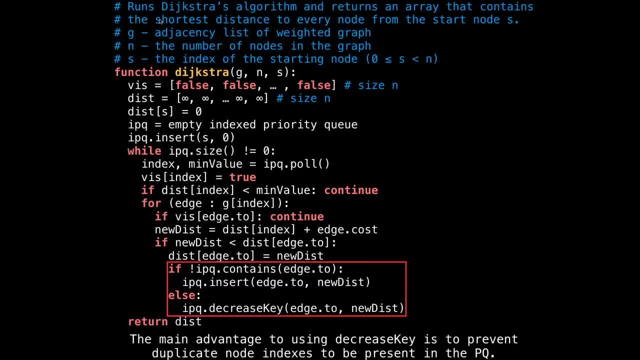 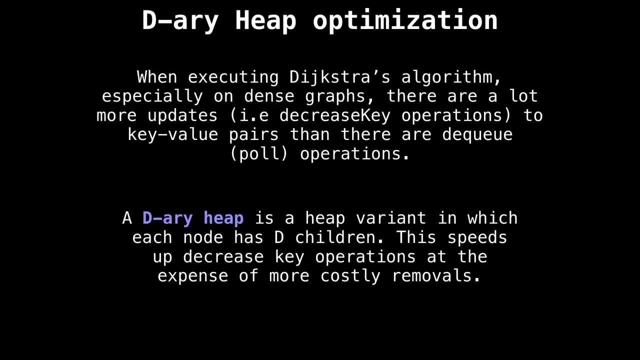 the best distance to that node in priority queue. The operation is called decrease key instead of update, because it only updates the value if it is strictly less than the current value in the trading queue. Alright, we've looked at several Dijkstra optimizations already. 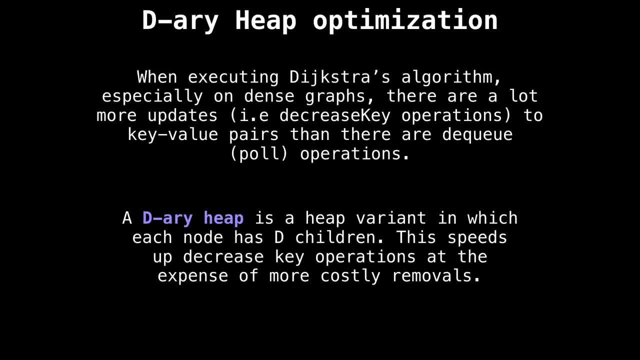 But there's one key last optimization I want to talk about, And that is improving the heap we're using. Currently, we're probably using an indexed binary heap for our priority queue, But we can do better. The thing to notice is that when executing Dijkstra, there are 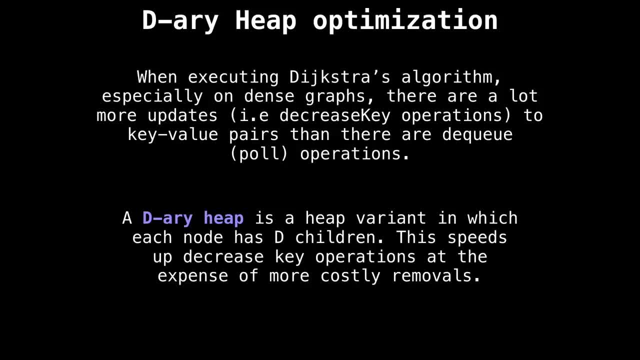 a lot more update operations, especially on dense graphs. then there are removal operations. A diary heap is a heap variant in which each node has at most D children instead of two. this speeds up the decrease key operation at the expense of more costly removals. So 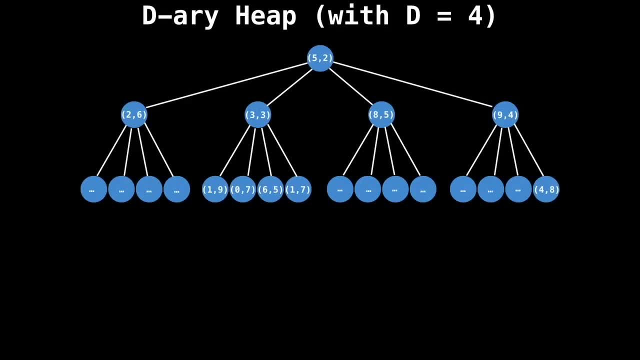 if we look at an example real quick, this is a dairy heap with D equals four. suppose we want to perform an update operation. say we want to perform decrease key for node at index six with a value of five. So if we want to perform a decrease key for node at index six with a value of five, we 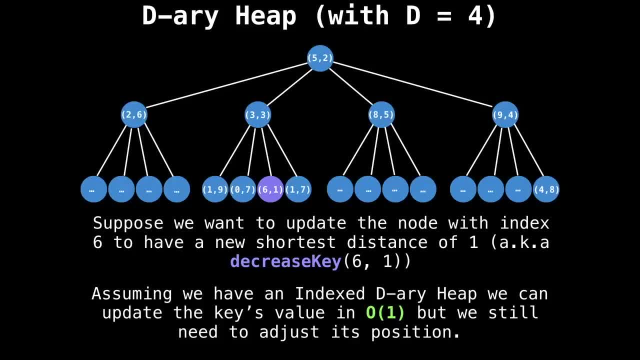 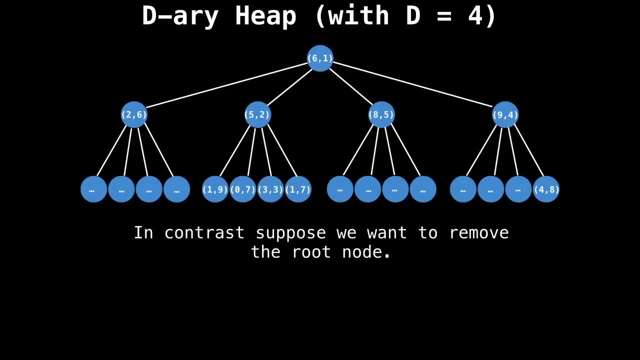 value of one, then we can do the update, And then we reposition the key value pair inside the heap, So we bubble it up, and we bubble it up again, and now it's in the correct position. So that only took a total of two operations, While in contrast, suppose, we want to remove. 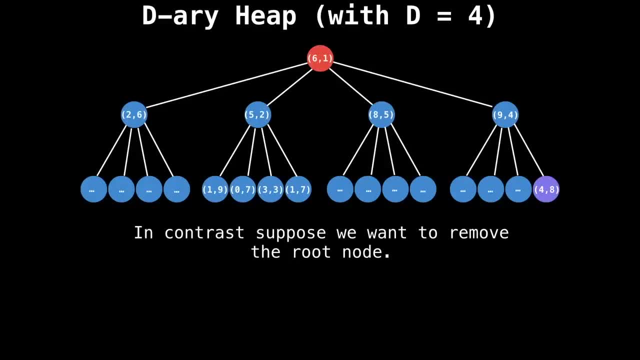 the root node, then we swap it with the bottom right node And then we need to reposition the purple node so that it's in position. So we need to look at all the children, find the one with the least value and swap it. And the purple node is still not in its correct. 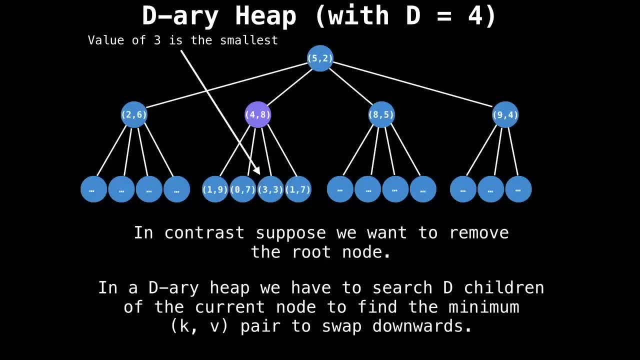 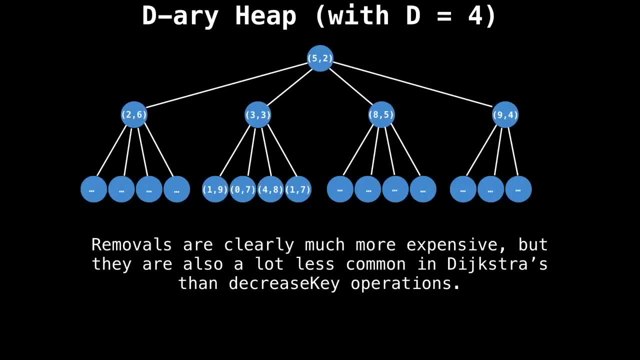 position. So again we need to look at all the children, find the one the smallest value and swap it. So that took a total of eight operations, which is clearly more expensive. But remember there are a lot more decreased key operations and Dijkstra's than there are. 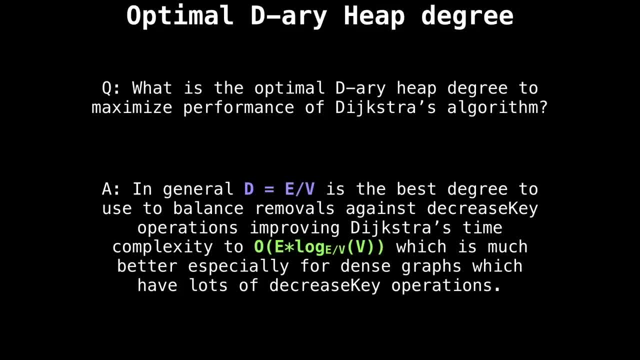 removals, So this might be beneficial. Okay, so let's go ahead and do that. So let's go ahead and do that. So let's go ahead and look at all the. So the question then becomes: what is the optimal dairy heap degree? I should 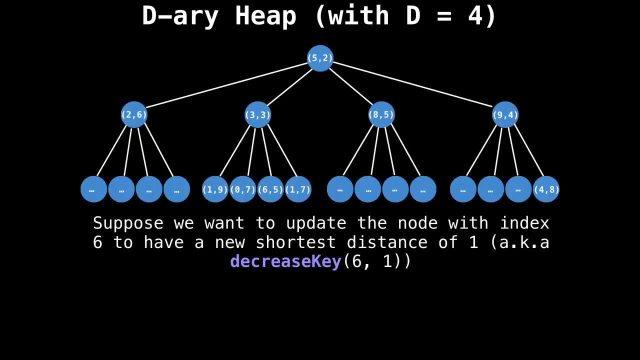 operation. Say we want to perform decrease key for node at index six with a value of one, then we can do the update And then we reposition the key value pair inside the heap. So we bubble it up, and we bubble it up again And now it's in the correct position. So that only took a total of two. 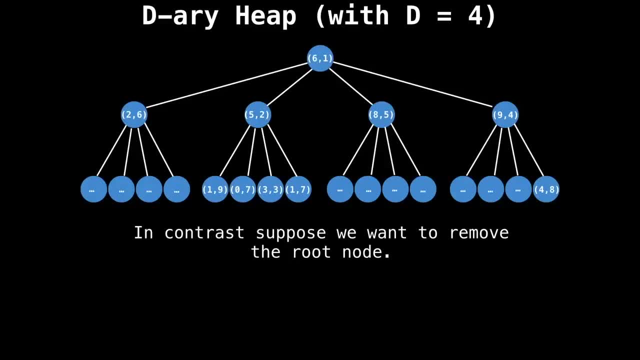 operations, While, in contrast, suppose we want to remove the root node, then we swap it with the bottom right node, And then we need to reposition the heap, We need to reposition the purple node so that it's in position. So we need to look at all. 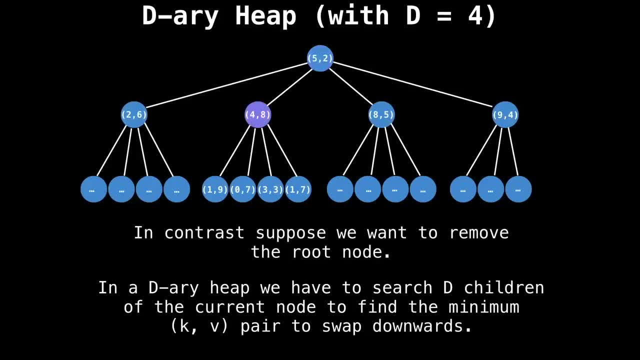 the children, find the one with the least value and swap it. And the purple node is still not in its correct position. So again we need to look at all the children, find the one with the smallest value and swap it. So that took a total of eight operations. 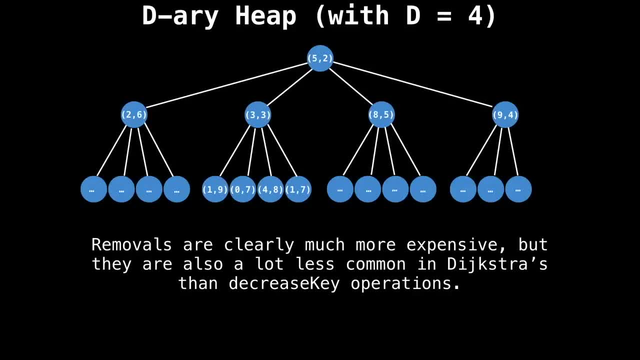 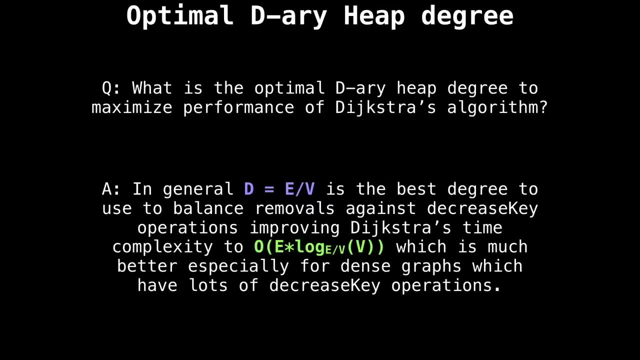 which is clearly more expensive. But remember, there are a lot more decrease key operations and Dijkstra's than there are removals, So this might be beneficial Overall. So the question then becomes: what is the optimal dairy heap degree I should use to maximize the performance of Dijkstra's algorithm? And the answer in general, is that 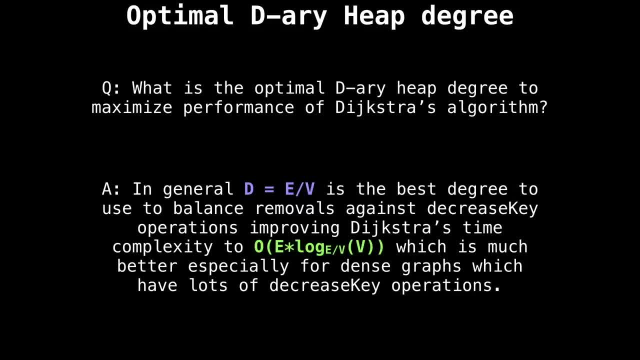 the value of D should be equal to the number of edges divided by the number of nodes. This is the best degree to use to balance removals against decrease key operations. In turn, this improves Dijkstra's time complexity to be a big O. 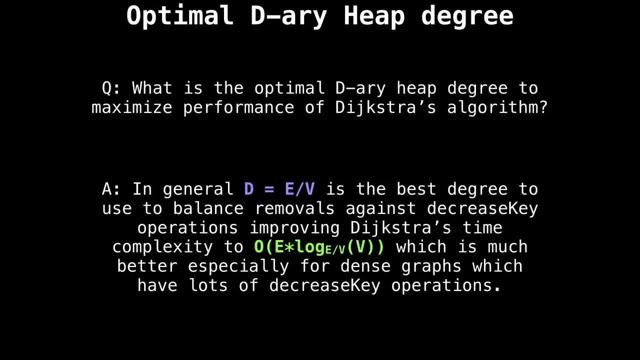 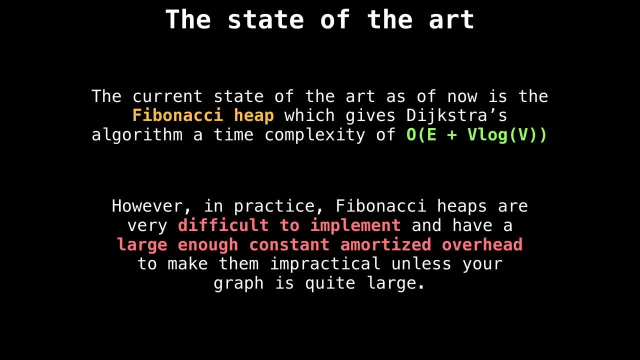 Of e times log base e divided by v of v, which is better, especially for dense graphs which have a lot of decrease key operations. The last thing I want to mention is the current state of the art when it comes to choosing the right heat for Dijkstra's algorithm, And 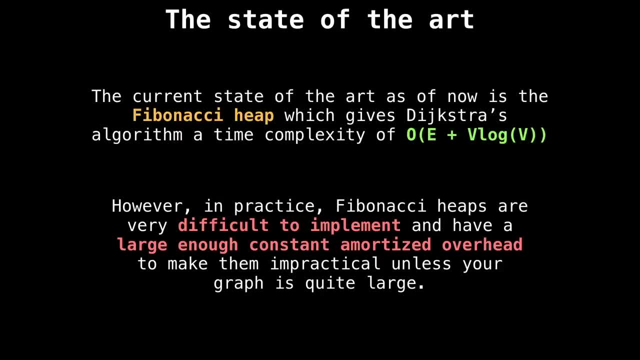 right now, the best heap we know of is the Fibonacci heap, which gives Dijkstra's algorithm, believe it or not, a time complexity of big O, of E plus v log v, which is extremely fast. However, in practice the Fibonacci heap is very difficult to implement and also has a large constant amortized overhead. 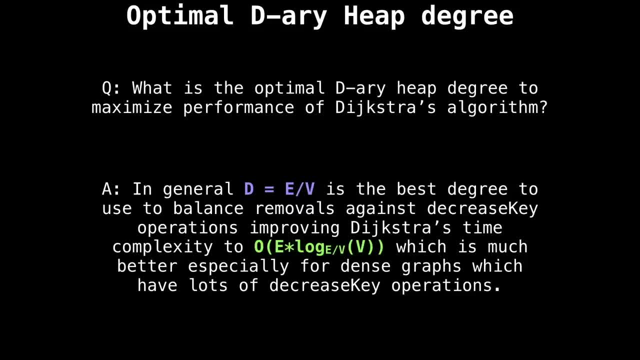 use to maximize the performance of dice's algorithm And the answer in general is that the value of D should be equal to the number of edges divided by the number of nodes. this is the best degree to use to balance removals against decrease key operations In turn. 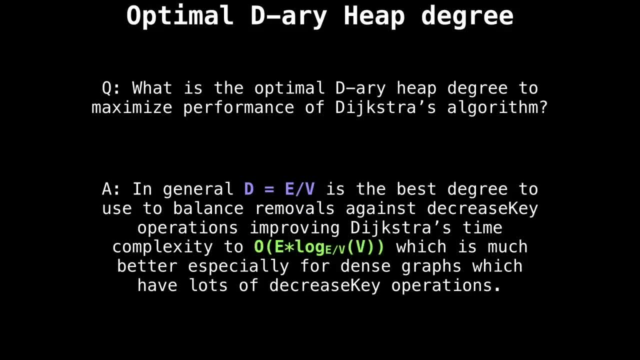 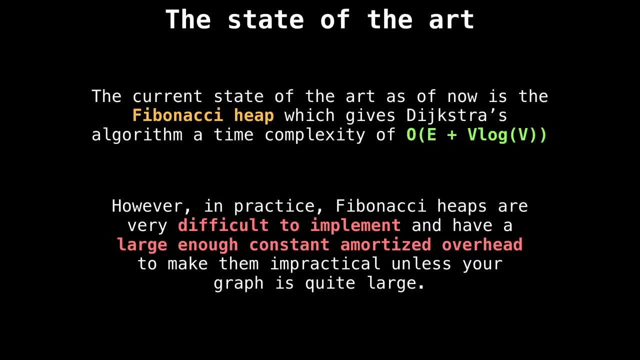 this improves Dijkstra's time complexity to be a big O of e times log base e divided by v of v, which is better, especially for dense graphs which have a lot of decreased key operations. The last thing I want to mention is the current. 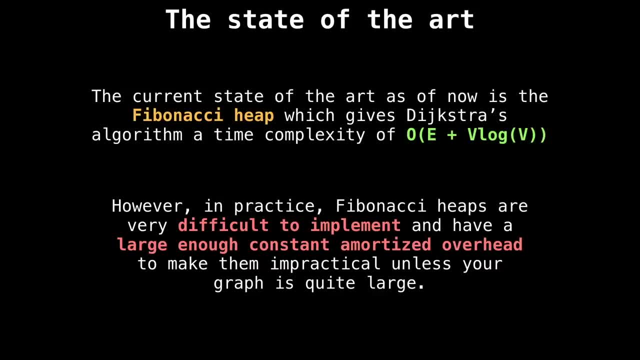 state of the art when it comes to choosing the right heat for Dijkstra's algorithm. And right now, the best heap we know of is the Fibonacci heap, which gives Dijkstra's algorithm, believe it or not, a time. complexity of big O of E plus v, log v, which is extremely fast. 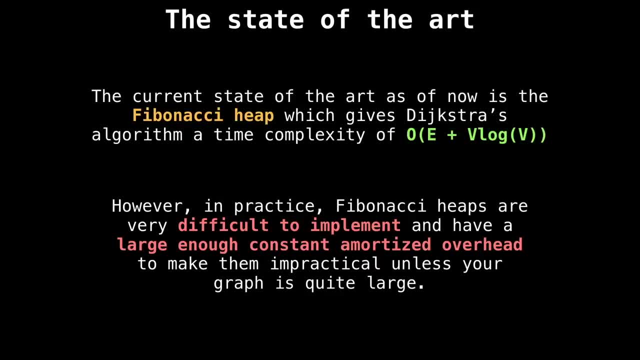 However, in practice, the Fibonacci heap is very difficult to implement and also has a large constant amortized overhead, So it makes them slightly impractical in practice because your graph has to be very large for you to see the benefit. I have yet to implement. 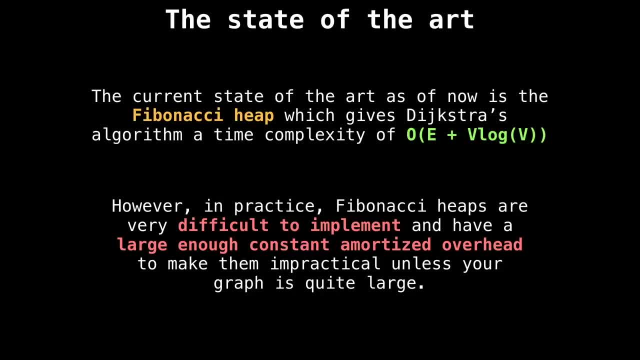 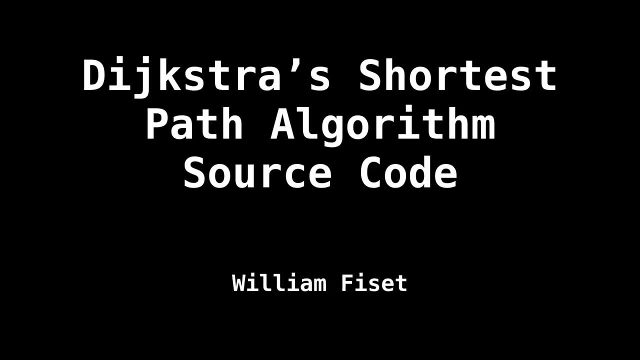 one of these, So I cannot say whether they're that good, But this is just what I've read from other sources. Today we're going to have a look at some source code for Dijkstra's shortest path algorithm. All right, here we are in. 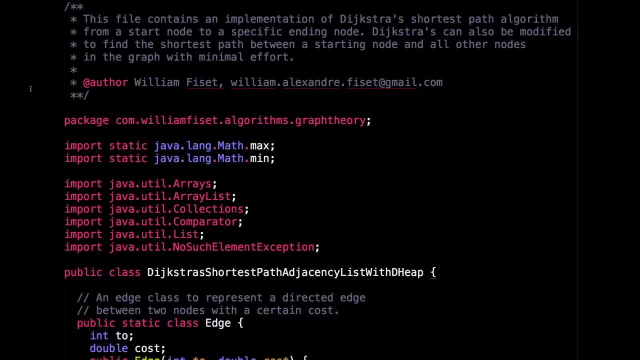 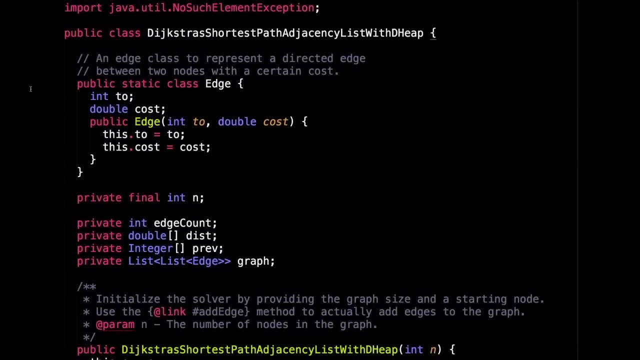 the source code for Dijkstra's shortest path algorithm implemented in the Java programming language. Let's have a quick run through. So in this class I define an edge class which represents a directed edge. you'll notice that this directed edge has a certain coefficient. 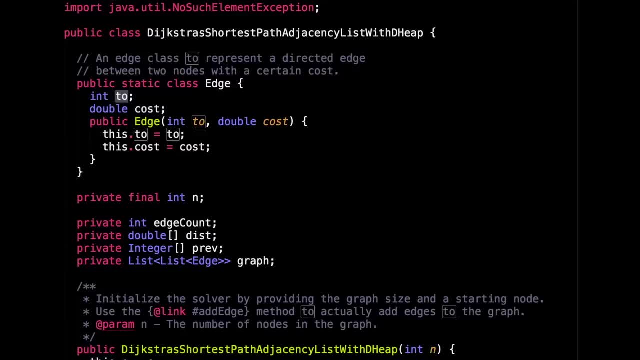 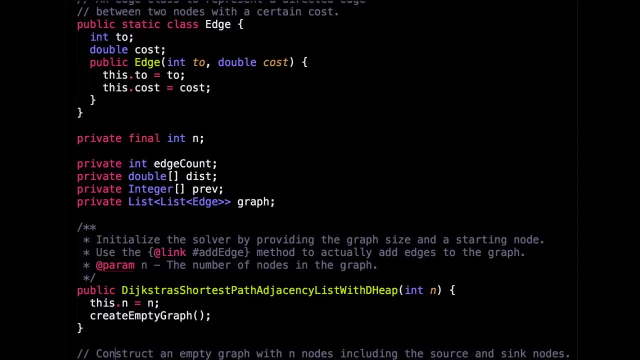 a cost of taking this edge And it also has a destination node which I call to. the node which this edge comes from will be implicitly represented in our adjacency list, So we don't need to take care of that. So when you go and create an instance of this class, you 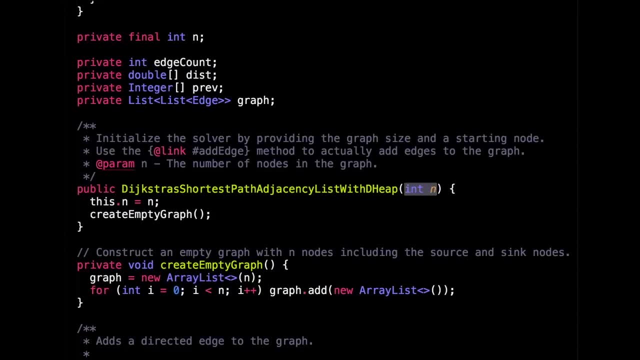 need to specify the number of nodes that are going to be in this graph, And that's the variable n. Once you know the number of nodes in your graph, you can get the number of nodes that are going to be in this graph, And that's the variable. 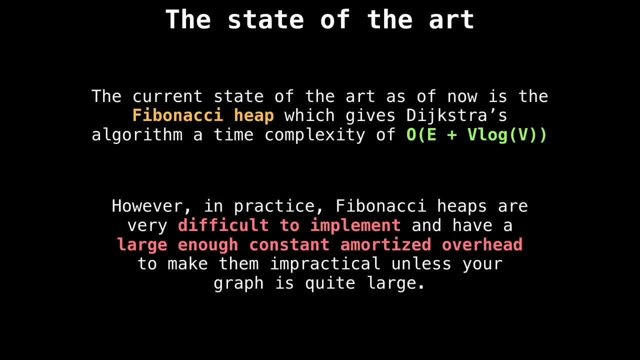 So it makes them slightly impractical in practice, because your graph has to be very large for you to see the benefit. I have yet to implement one of these, So I cannot say whether they're that good, But this is just what I've read. 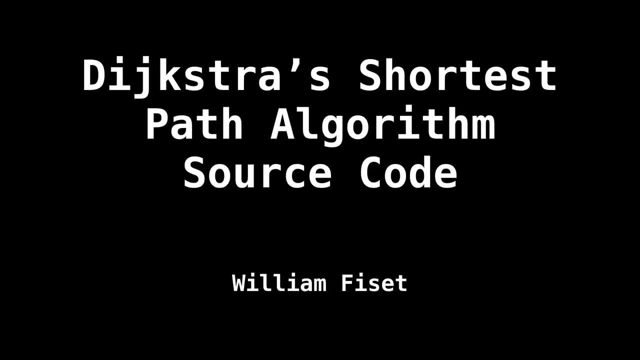 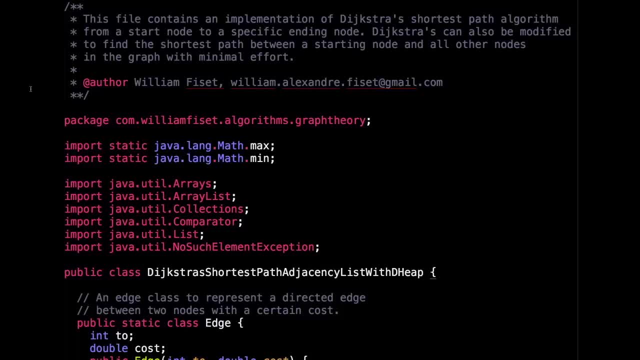 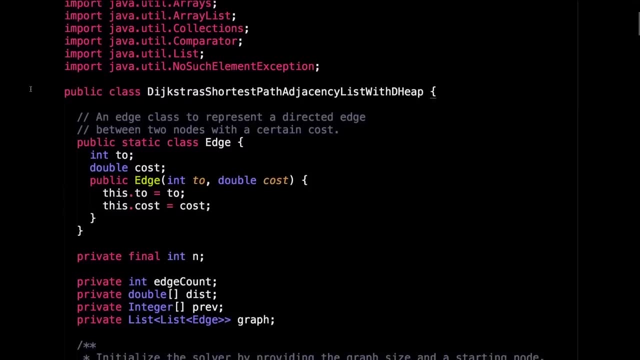 read from other sources. Today we're going to have a look at some source code for Dijkstra's shortest path algorithm. All right, here we are in the source code for Dijkstra shortest path algorithm implemented in the Java programming language. Let's have a quick run through. 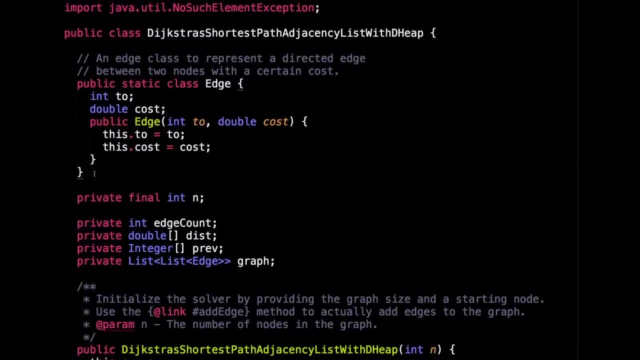 So in this class I define an edge class which represents a directed edge. you'll notice that this directed edge has a certain cost of taking this edge And it also has a destination node which I call to. the node which this edge comes from will be implicitly represented. 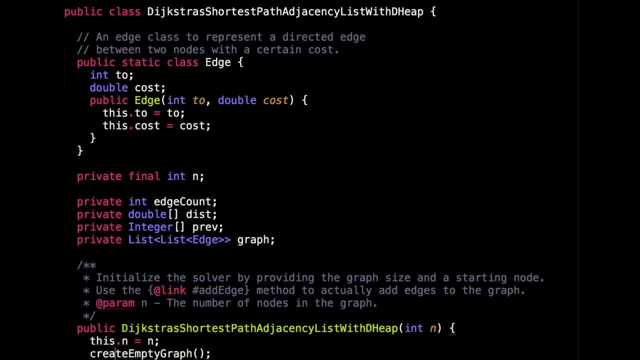 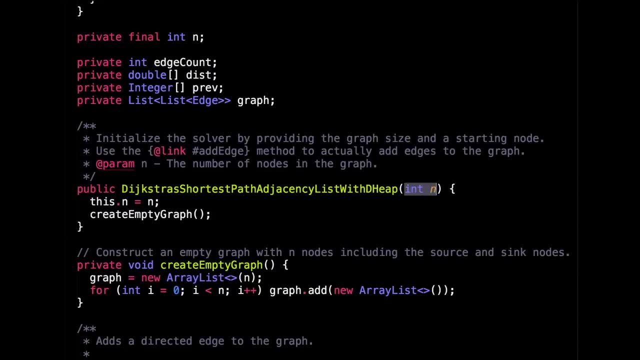 in our adjacency list, So we don't need to take care of that. So when you go and create an instance of this class, you need to specify the number of nodes that are going to be in this graph, And that's the variable. 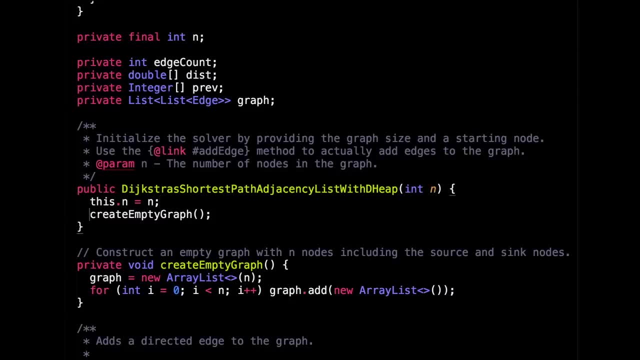 Okay, n. once you know the number of nodes in your graph, you can go ahead and create an empty graph. this simply initializes our adjacency lists. So, as you see here, I create an empty array list with n nodes And then for each position in the list I create another list. 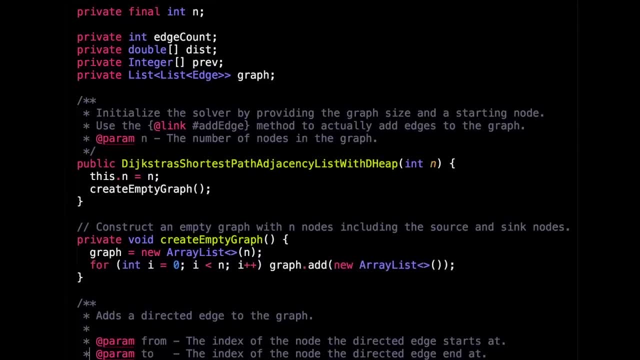 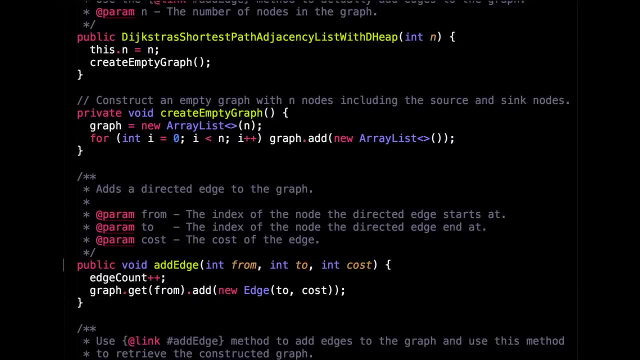 So this is just an empty decency list. this will help us add edges to our graph, which you can do by by calling this add edge method. So when you want to add an edge to the graph, you specify the node the edge starts at, the node the edge ends at and the cost of taking that edge. 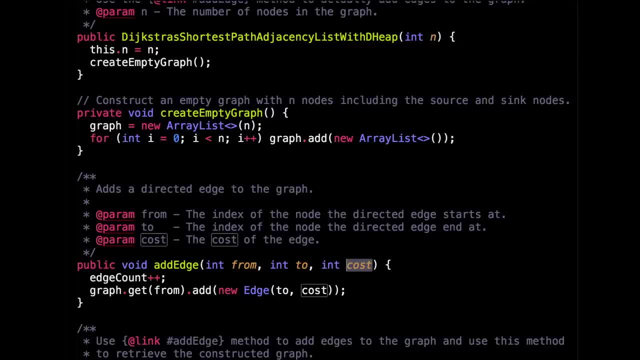 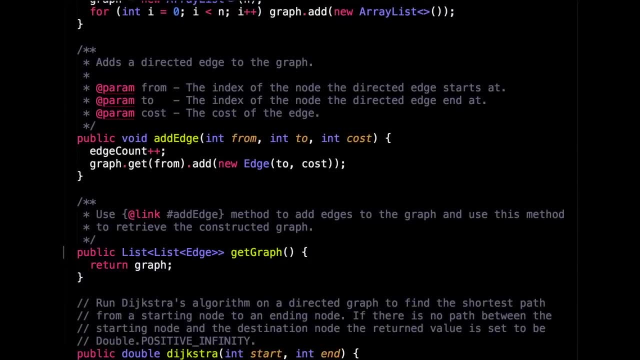 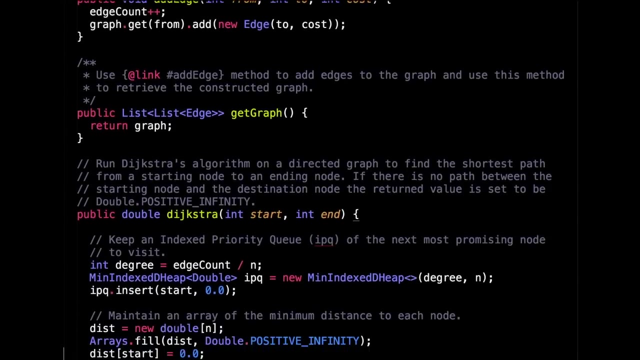 remember that the cost of taking edge cannot be a negative value. All right, and then there's the, just this convenience method to retrieve the constructed graph. if ever you want to have a look at that, then here comes the interesting method which actually executes the edge. once you know the number of nodes in your graph, you can get the number of nodes that are going to be in this graph, And that's the variable n. Once you know the number of nodes in your graph, you can get the number of nodes that are going to be in this graph, And that's the variable n. So 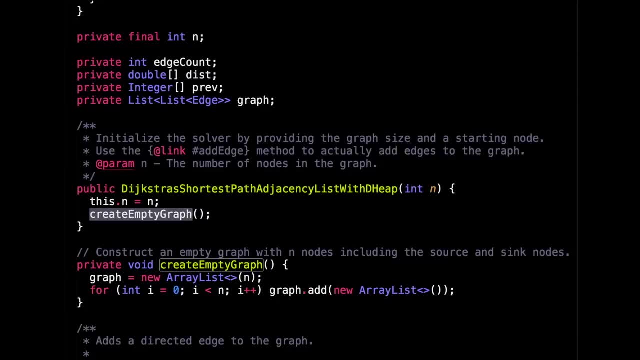 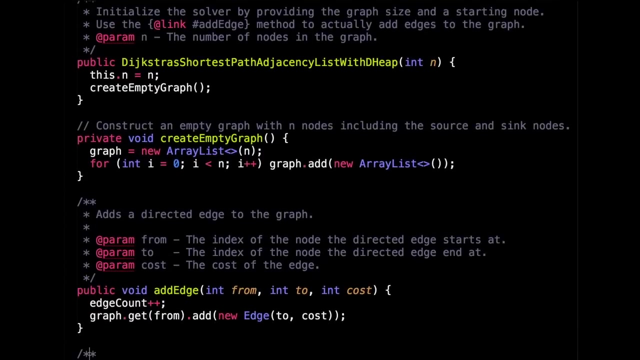 when you go ahead and create an empty graph, this simply initializes our adjacency lists. So, as you see here, I create an empty array list with n nodes And then for each position in the list, I create another list. So this is just an empty decency list. this will help us add edges to our 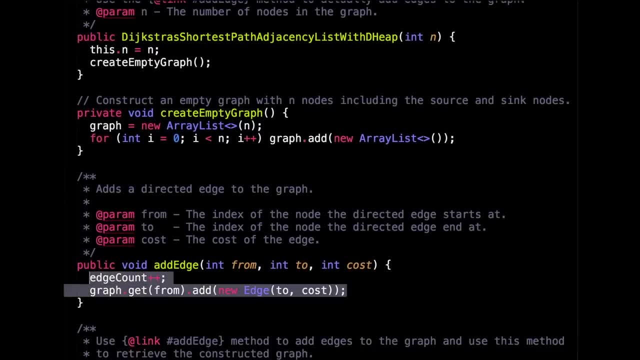 graph, which you can do by calling this add edge method. So when you want to add edges, you can add an edge to the graph. you specify the node the edge starts at, the node the edge ends at and the cost of taking that edge. remember that the cost of taking edge cannot be a negative value. 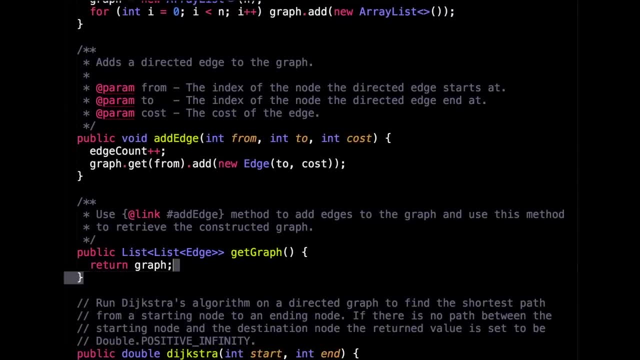 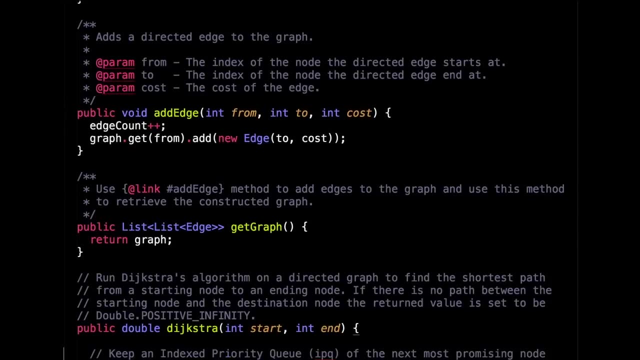 All right. and then there's the- just this convenience method to retrieve the constructed graph. if ever you want to have a look at that, then here comes the interesting method which actually executes Dijkstra shortest path algorithm. So in this case, we're going to use the shortest. 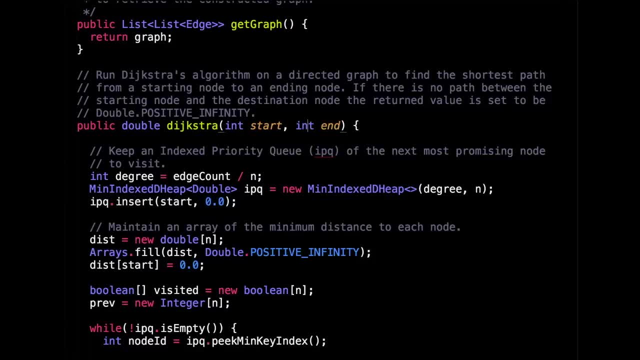 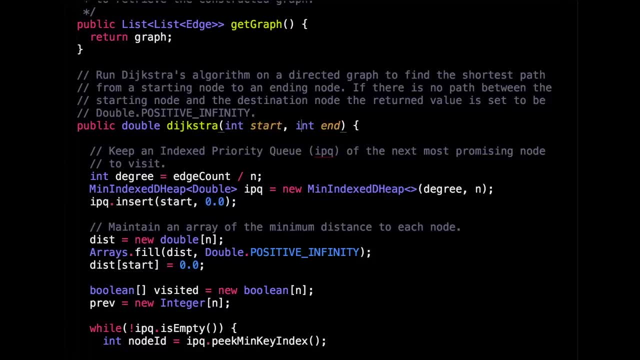 implementation. I provide a start node and the end node. this means we're going to try and go from a starting node index to an end node index. note that we can also modify Dijkstra is to give us the shortest distance to every node, not just a specific end node. So there is a way we can just. 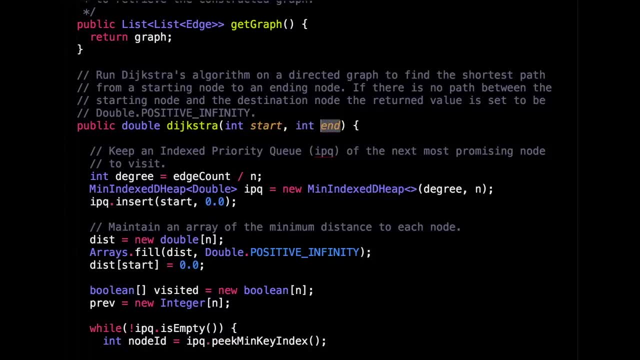 remove this parameter. we don't really need it. But providing the end node allows us to do a small optimization, which is to stop early If we know we've reached that end node. so let's keep it in for now. So in the slides in the last: 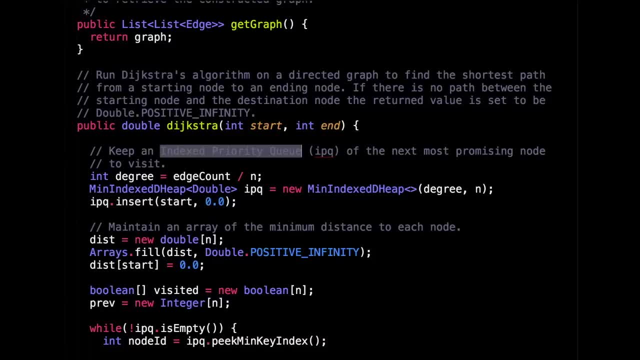 video. I mentioned that we can use an indexed priority queue to speed up Dijkstra's algorithm, And this is exactly what I'm doing below. I have an implementation of a min indexed diary heap which allows us to avoid duplicate nodes in our priority queue. I won't be going over the details. 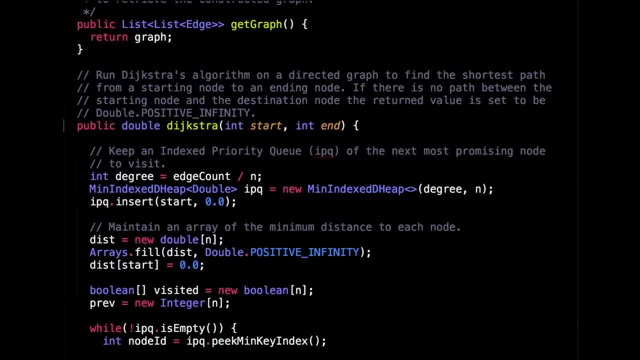 which executes Dijkstra shortest path algorithm. So in this implementation I provide a start node and the end node. this means we're going to try and go from a starting node index to an end node index. note that we can also modify Dijkstra's to give us the shortest distance. 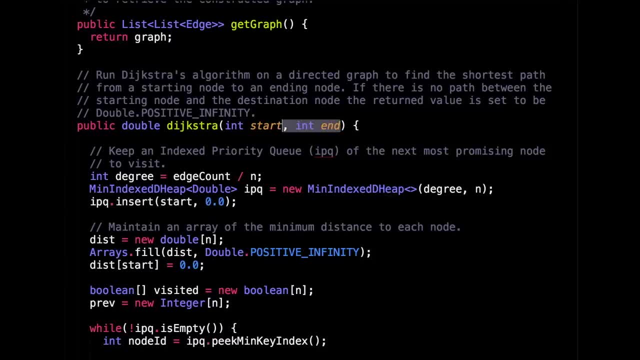 to every node, not just a specific end node. So there is a way we can just remove this parameter. we don't really need it, But providing the end node allows us to do a small optimization, which is to stop early if we know we've reached that end node. So 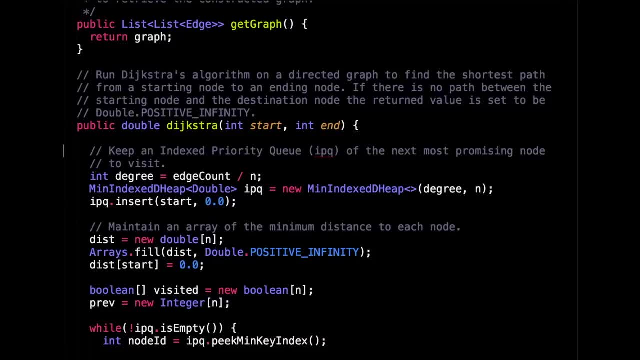 let's keep it in for now. So in the slides in the last video, I mentioned that we can use an indexed priority queue to speed up Dijkstra's algorithm, And this is exactly what I'm doing below. I have an implementation of a min indexed diary heap which allows 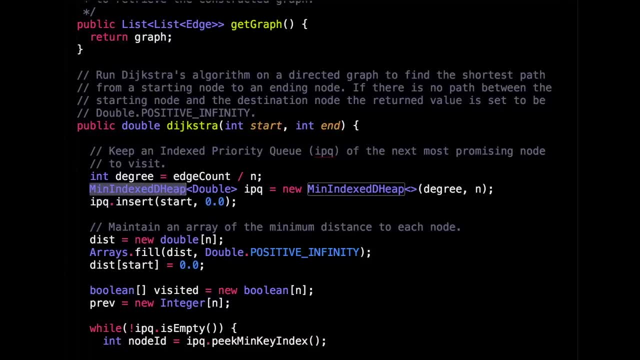 us to avoid duplicate nodes in our priority queue. I won't be going over the details of the min indexed diary heap per se, because I already have another video on that In my data structure series. I'll make sure to have a link to that in case you. 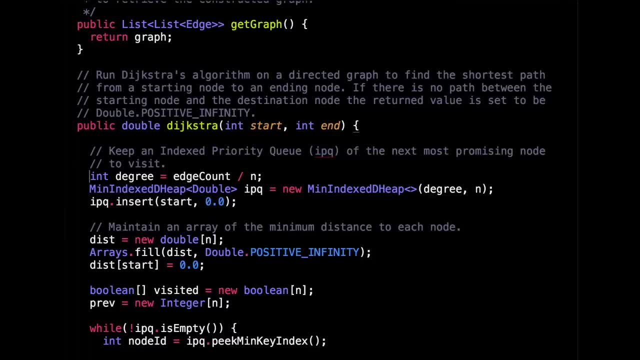 want to check it out But to construct a min indexed diary heap, I compute the degree of how many children each node should have in the heap by dividing the edge count by the number of nodes And finally inserting that the optimal distance to the start node at 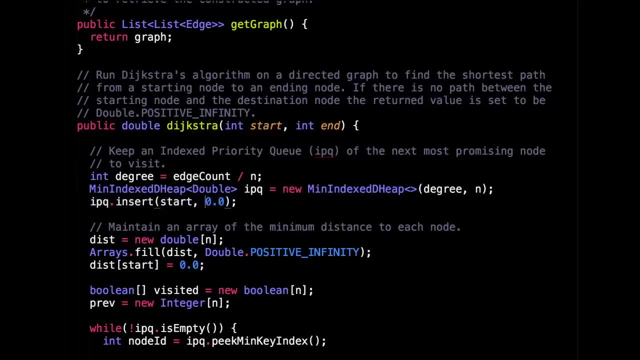 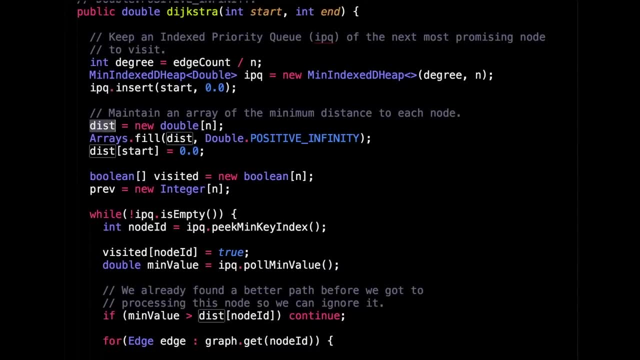 the beginning of the initial node. So now I can actually just say that I've got the value of zero, which makes sense. then I just initialize a few arrays. So this is the distance array which is going to keep track of the minimum distance to each node. So initially I fill that with. 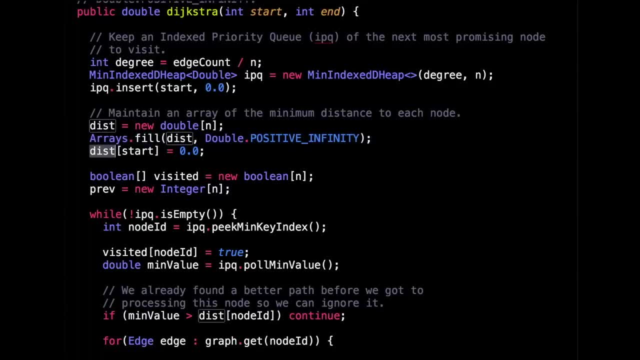 a value of positive infinity, and I set that the optimal distance to the start node has a value of zero, perfect. And then these are just two supporting arrays that track whether node I has been visited, And this prep array is going to be used to reconstruct the shortest path should. 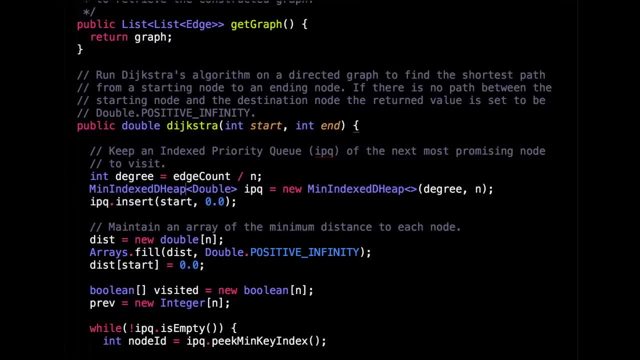 of the min indexed diary heap say, because I already have another video on that in my data structure series. I'll make sure to have a link to that in case you want to check it out. But to construct a min indexed diary heap I compute. 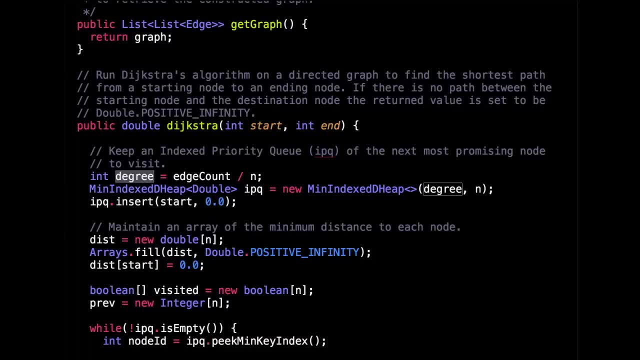 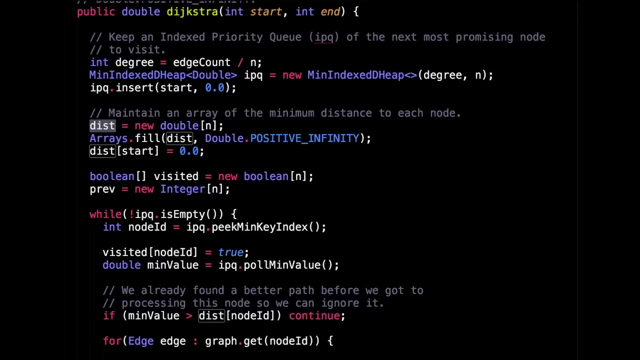 the degree of how many children each node should have in the heap by dividing the edge count by the number of nodes And finally inserting that the optimal distance to the start node at the beginning of the algorithm has a distance of zero, which makes sense. then I just initialize a few arrays, So this is the distance array which is going to keep. 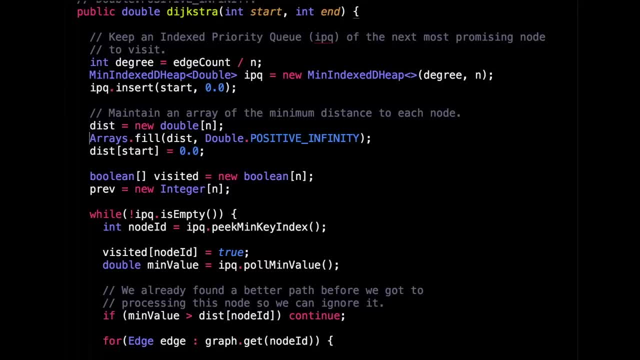 track of the minimum distance to each node. So initially I fill that with a value of positive infinity and I set that optimal distance to the start. node has a value of zero, perfect. And then these are just two supporting arrays that track whether node i has been visited, And this prep array is a value of zero. And then we can. 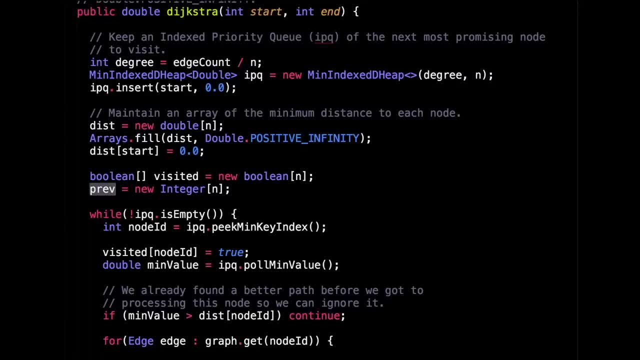 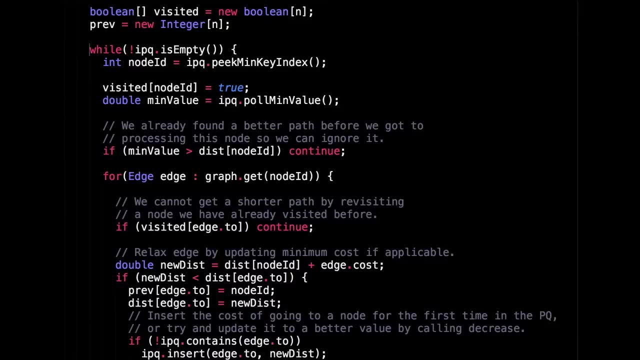 add a value of negative infinity, which is going to be used to reconstruct the shortest path, should we ever need to? All right, let's look at this while loop, which contains the bulk of the Dijkstra algorithm implementation. So, while the priority queue is not empty, we're going to first get the ID of the node with the shortest distance And we're 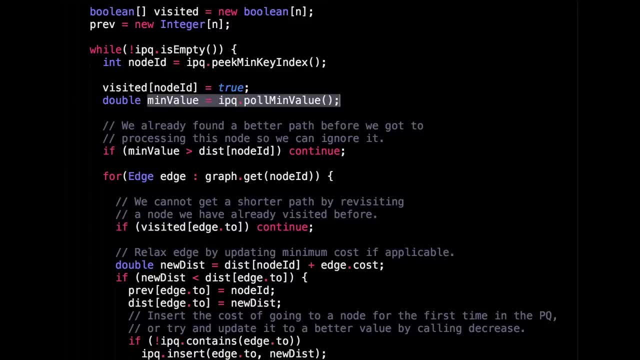 also going to get the minimum value associated with that node. So, while we're So, while we're So, while we're at it, we're going to mark that this node is visited so that we don't visit it again in the future. this line right here. 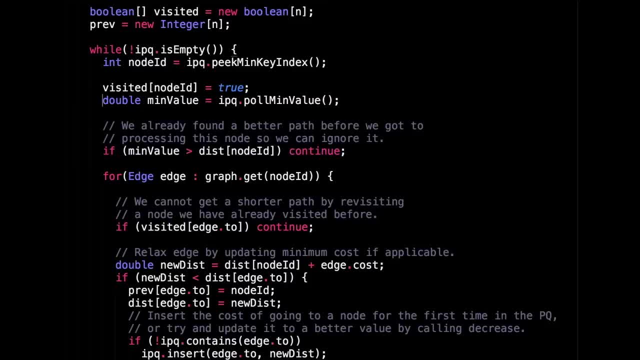 which says that the min value- if the minimum value we got from the priority queue is greater than the already optimal distance and the distance array for the node we currently pulled out of the queue, then we can continue. this is because we already found a better path routing through another set of nodes before we got to processing. 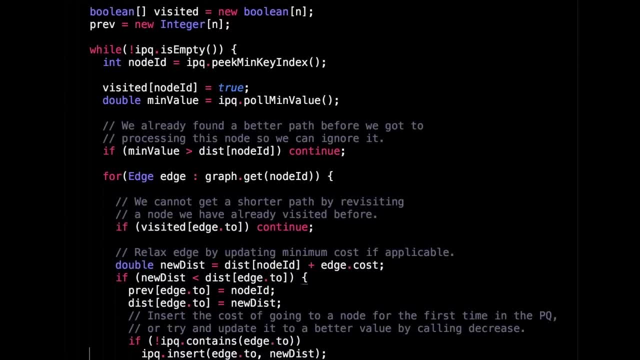 we ever need to. Alright, let's look at this while loop, which contains the bulk of the Dijkstra algorithm implementation. So, while the priority queue is not empty, we're going to first get the ID of the node with the shortest distance And we're also going to get the 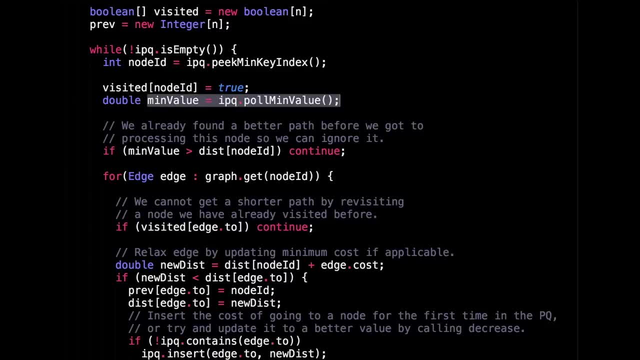 minimum value associated with that node. So while we're at it, we're going to mark that this node is visited so that we don't visit it again in the future. This line right here which says that the min value, if the minimum value we got from the priority queue is greater. 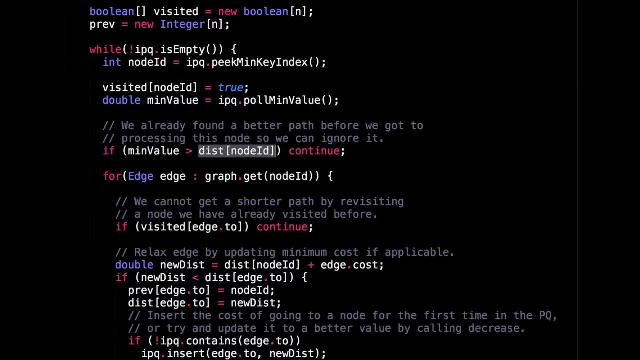 than the already optimal distance and the distance array for the node we currently pulled out of the queue, then we can continue. this is because we already found a better path or routing through another set of nodes before we got to processing this node, which is fine. 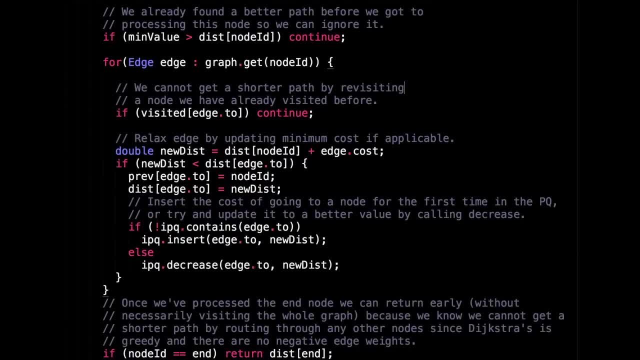 The next thing we want to do is get all the edges going outwards from this node So we can reach into our adjacency list and get all the edges coming out of the current node. then we check if the node this edge wants to go to has already been visited. then we 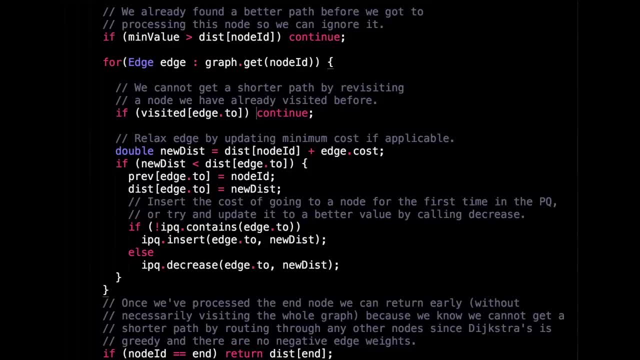 can skip that, we don't want to revisit an already visited node. And then we compute the new distance of going up from the current node to the destination node. And we do this by reaching into the distance array, grabbing the already optimal distance for that node and adding the edge costs. then we try and relax the edge. So 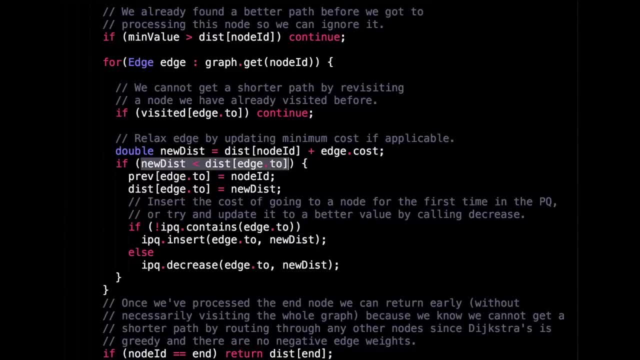 we check if the new distance is better than the distance already in the distance array at the node. we want to go to Remember that originally all the indices in the distance array positive infinity. So the first time we visit any node this condition will always be true. 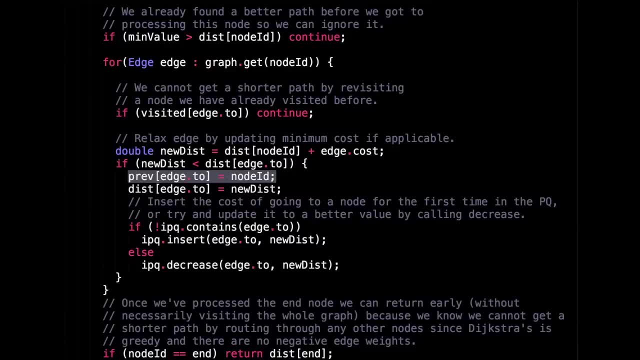 then we just do some housekeeping stuff. So mark that the optimal distance to get to a certain node came from the current node we're at and also update the distance array to have the new optimal distance. then we update our index priority queue. We do this by inserting: 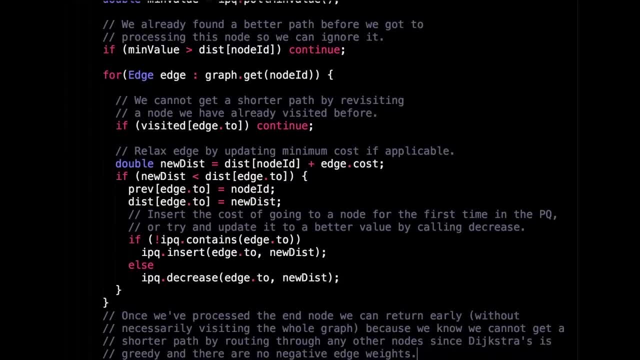 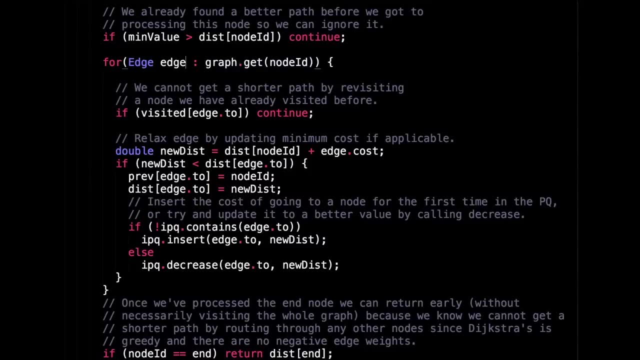 this node, which is fine. the next thing we want to do is get all the edges going outwards from this node So we can reach into our adjacency list and get all the edges coming out of the current node. then we check if the node this edge wants to go to has already. 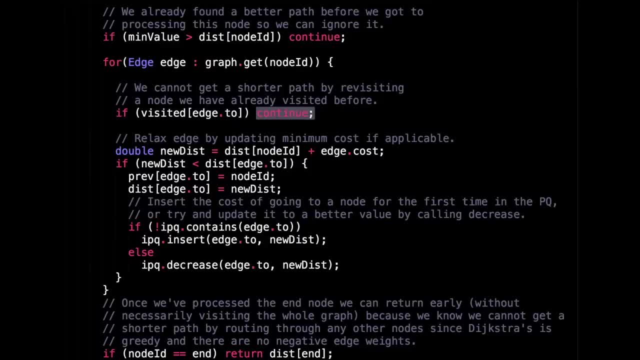 been visited, then we can skip that. we don't want to revisit an already visited node. then we compute the new distance of going from the current node to the destination node, And we do this by reaching into the distance array, grabbing the already optimal distance. 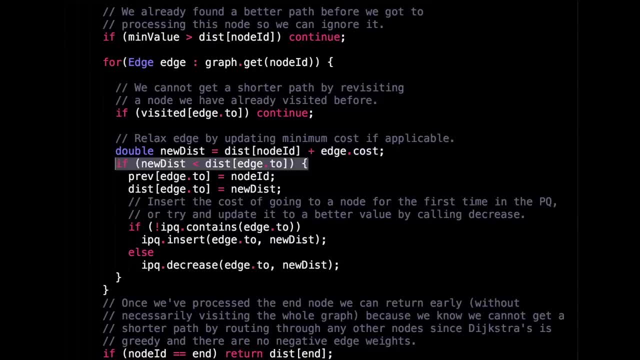 for that node and adding the edge costs, then we try and relax the edge. So we check if the new distance is better than the distance already in the distance array at the node. we want to go to Remember that originally all the indices in the distance 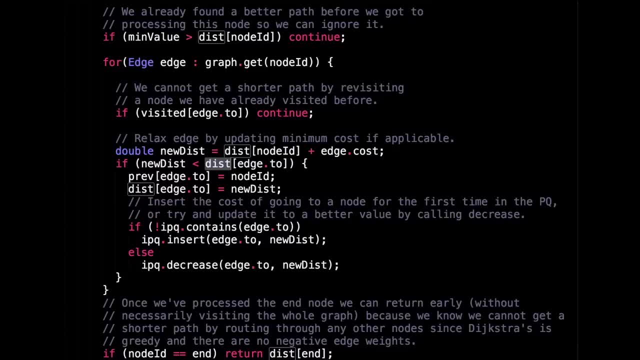 array are set to positive infinity. So the first time we visit any node this condition will always be true. then we just do some housekeeping stuff. So mark that the optimal distance to get to a certain node came from the current node we're at and also update the distance array to have the new optimal distance. then we update our index. 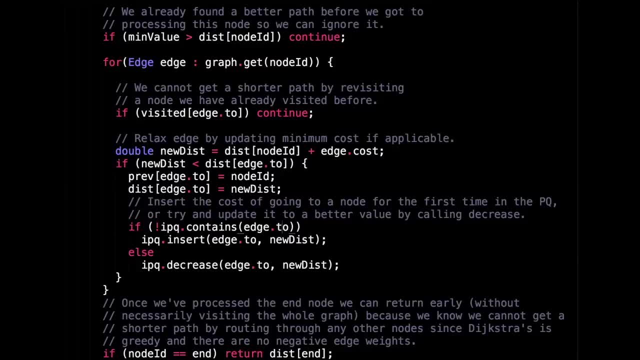 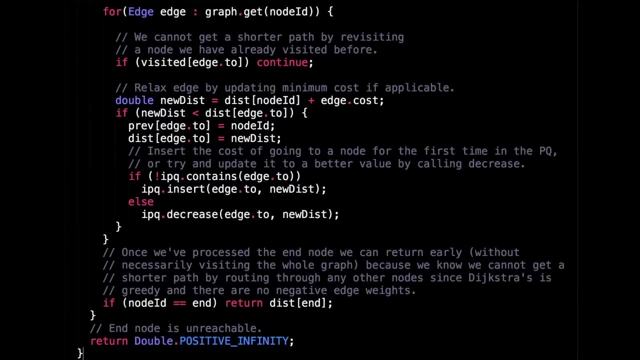 priority queue. We do this by inserting the cost of going to a node for the first time, or we try and employ a decrease key operation to update the current best distance to that node to be even better. Then after that loop we can check if we've reached our end node And if 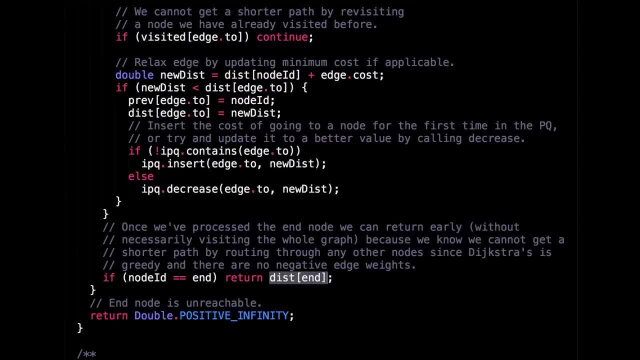 we have, we can return the optimal distance to it. So this is the optimization of returning early. Otherwise, if we've reached the end of the algorithm and the while loop has terminated and the priority queue is empty, then return positive infinity. 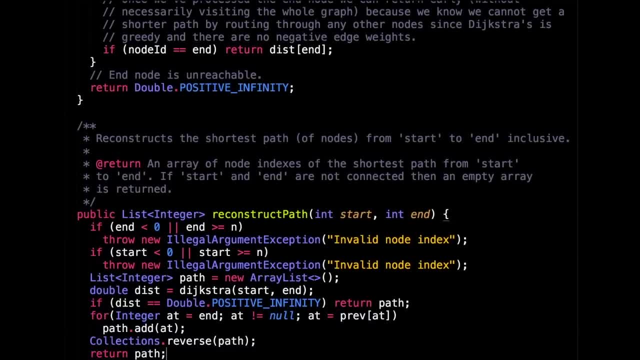 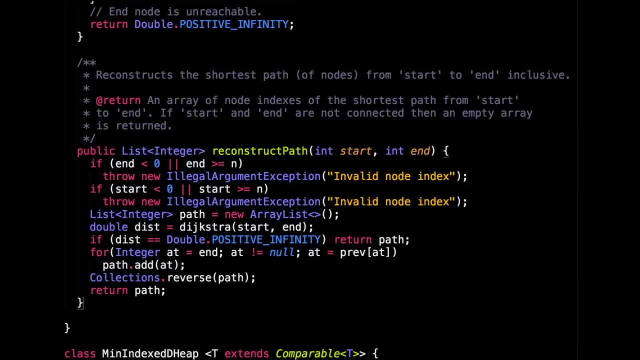 the rest of this class contains the reconstruct path method. in the event that you wanted to actually reconstruct the shortest path from the start node to the end node- And this is pretty straightforward- Simply give it the start node you want to start at the end node index. then run Dijkstra's algorithm: make sure that the end node is actually reachable from the start. 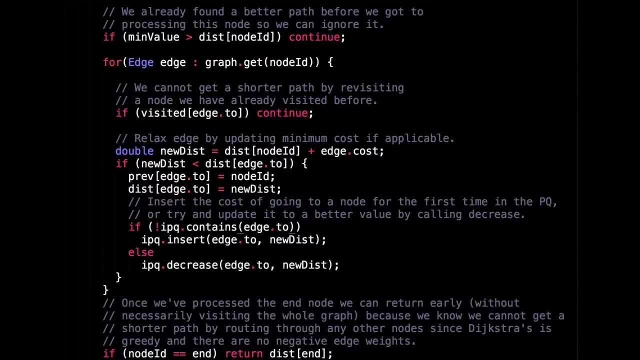 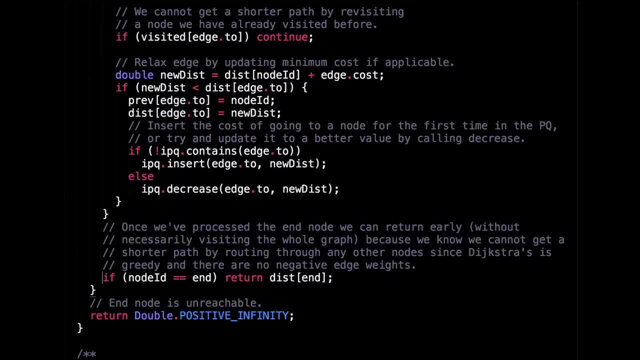 the cost of going to a node for the first time, or we try and employ a decrease key operation to update the current best distance to that node to be even better. Then after that loop we can check if we've reached our end node And if we have, we can return the. 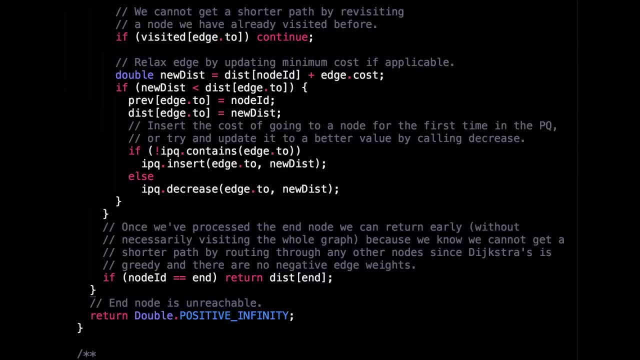 optimal distance to it. So this is the optimization of returning early. Otherwise, if we've reached the end of the algorithm and the while loop has terminated and the priority queue is empty, then return positive infinity. The rest of this class contains the reconstruct path method in the 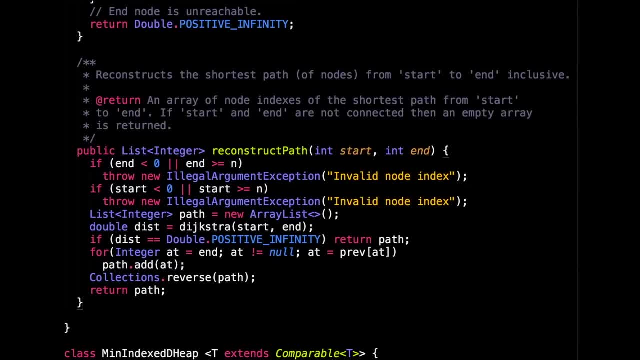 event that you wanted to actually reconstruct the shortest path from the start node to the end node, And this is pretty straightforward: Simply give it the start node you want to start at the end node index, then run Dijkstra's algorithm, make sure that the end node is the one that you want to start at, And then you can run. 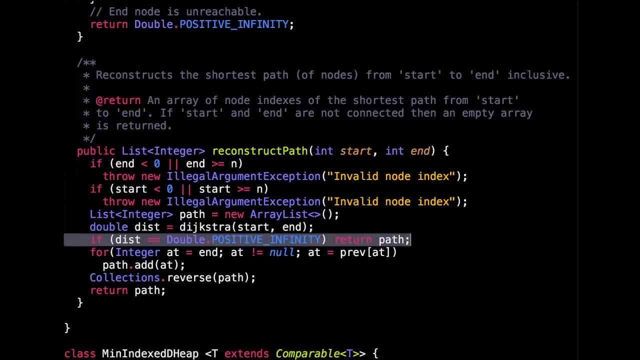 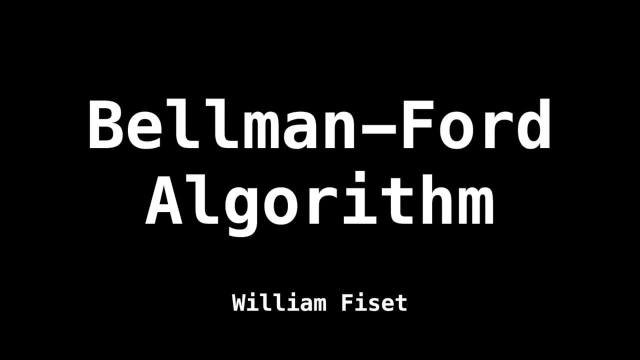 Dijkstra's algorithm make sure that the end node is actually reachable from the start node, then simply loop through the previous array and reverse the path and return it. as simple as that Of all the shortest path algorithms in graph theory, Bellman Ford is definitely. 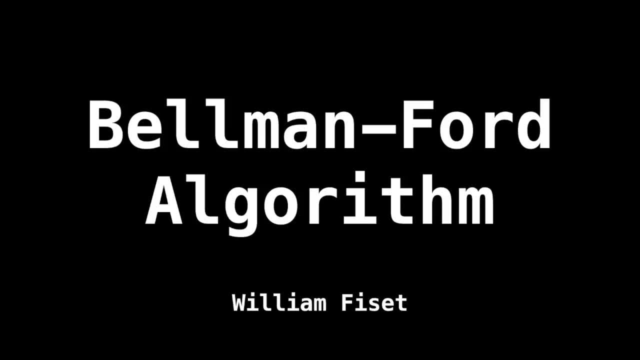 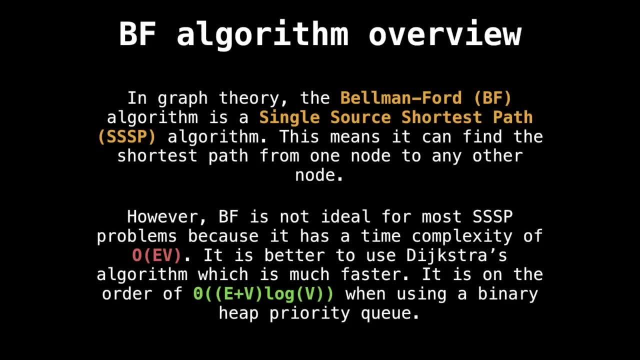 one of the simplest, Yet I struggled as an undergrad student trying to learn this algorithm, which is part of the reason I'm making this video. So what is the Bellman Ford algorithm? In short, it's a single source shortest path algorithm. This means that it can find the 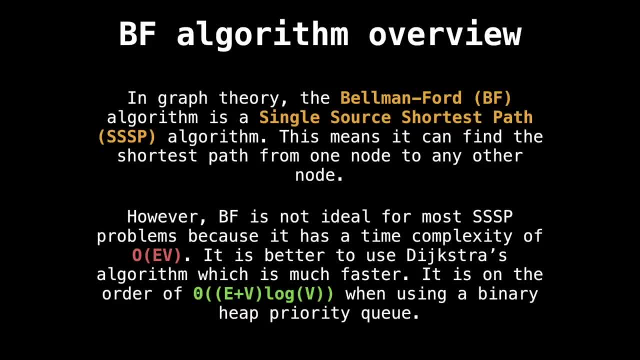 shortest path from a starting node to all other nodes in the graph. As you can imagine, this is very useful. However, Bellman Ford is not ideal for single source shortest path algorithms because it has a much worse time complexity than Dijkstra's algorithm In practice. 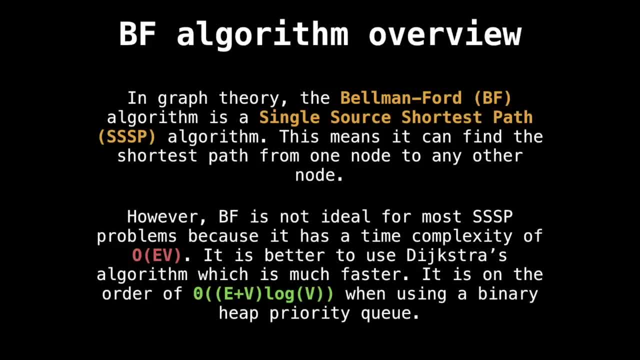 Bellman Ford runs in a time complexity proportionality. It's proportional to the product of the number of edges and the number of vertices, While Dijkstra can do much better at around big O of E plus v, log v with a binary heap. So when? 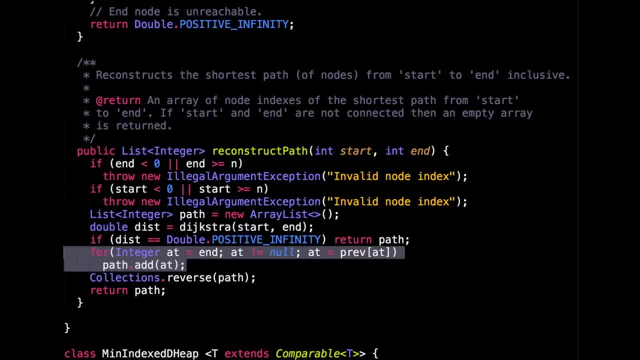 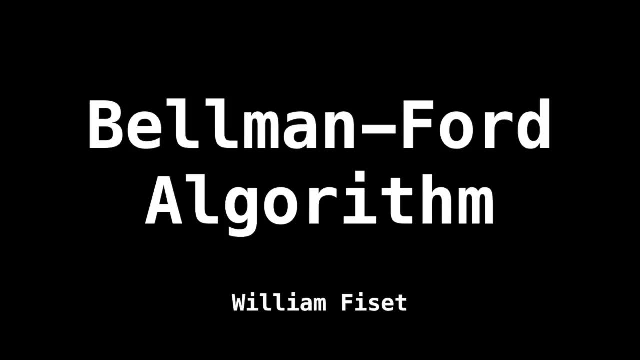 node, then simply loop through the previous array And reverse the path and return it. as simple as that. Of all the shortest path algorithms in graph theory, Bellman ford is definitely one of the simplest, Yet I struggled as an undergrad student trying to learn this algorithm, which is part of the 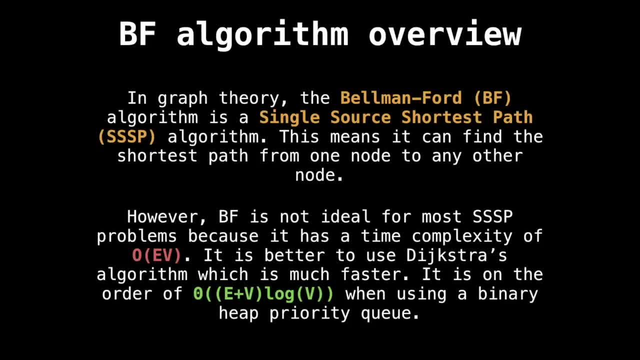 reason I'm making this video. So what is the Bellman ford algorithm? In short, it's a single source shortest path algorithm. This means that it can find the shortest path from a starting node to all other nodes on the graph. As you can imagine, this is very useful. However, Bellman 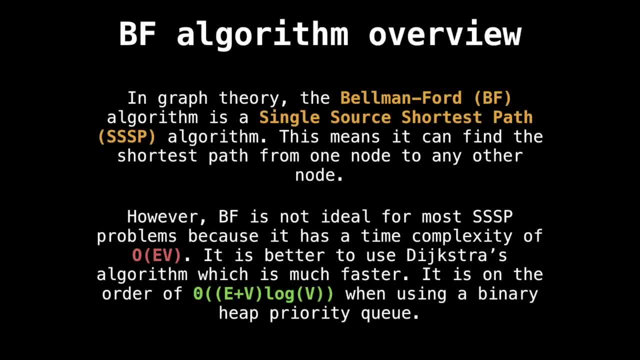 Ford is not ideal for single source shortest path algorithms because it has a much worse time complexity than Dijkstra's algorithm. In practice, Bellman Ford runs in a time complexity proportional to the product of the number of edges and the number of vertices, While 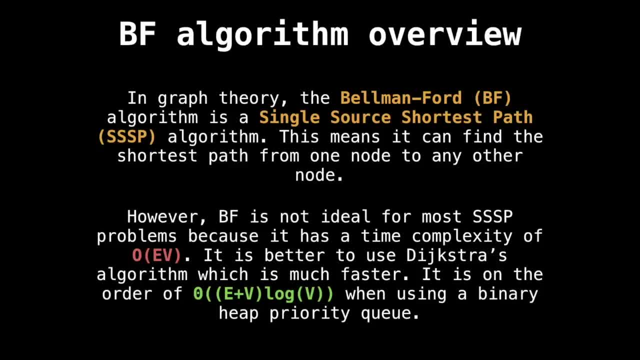 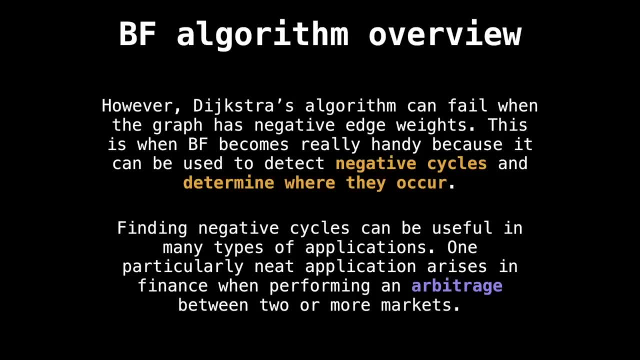 Dijkstra can do much better at around big O of E plus v, log v with a binary heap. So when would we ever use the Bellman Ford algorithm? The answer is when Dijkstra's fails, And this can happen when the graph has negative edge weights. When a graph has negative edge weights, 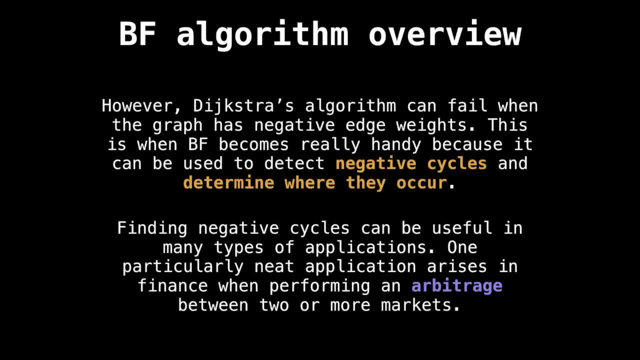 it is possible that a negative cycle can manifest itself, And when it does, it is of critical importance that we are able to detect it. If this happens and we're using Dijkstra's to find the shortest path, we'll get stuck in an infinite loop, because the algorithm will keep finding better. 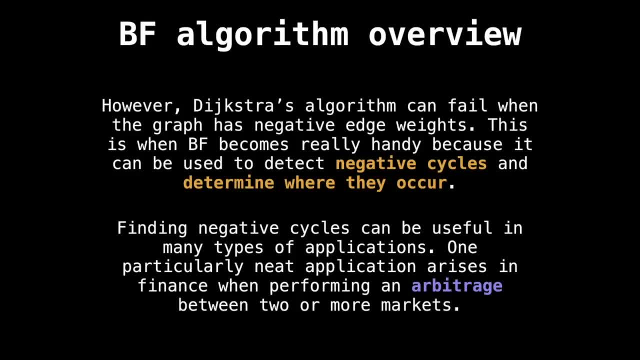 and better paths. A neat application of Bellman Ford and negative cycles is in finance and economics on performing an arbitrage between two or more markets. I'm not an expert, but this is when prices between different markets are such that you can cycle through each market. 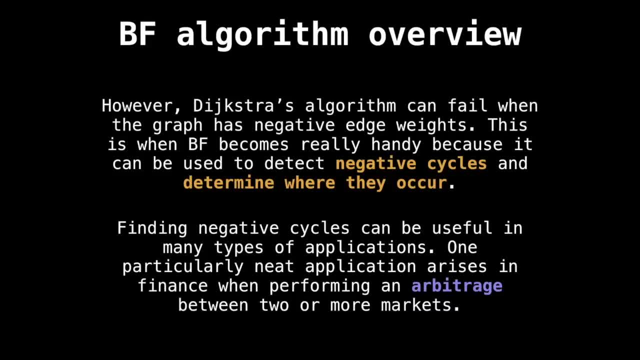 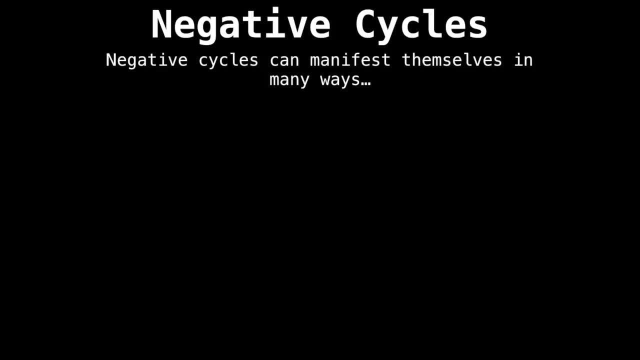 with a secure security, such as a stock or currency, and end up with more profit than you originally started, with essentially getting risk free gains. Let's look at how negative cycles can arise. because this seems important. Here is a graph I made with directed edges. some of 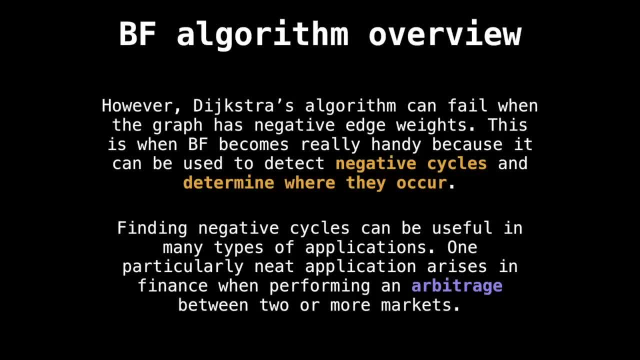 would we ever use the Bellman Ford algorithm? The answer is when Dijkstra's fails, And this can happen when the graph has negative edge weights. When a graph has negative edge weights, it is possible that a negative cycle can manifest itself, And when it does, it is of critical importance that we are able to. 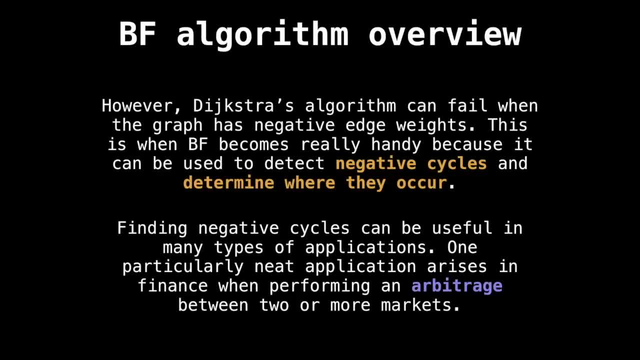 detect it. If this happens and we're using Dijkstra's to find the shortest path, we'll get stuck in an infinite loop because the algorithm will keep finding better and better paths. A neat application of Bellman Ford and negative cycles is in finance and economics. 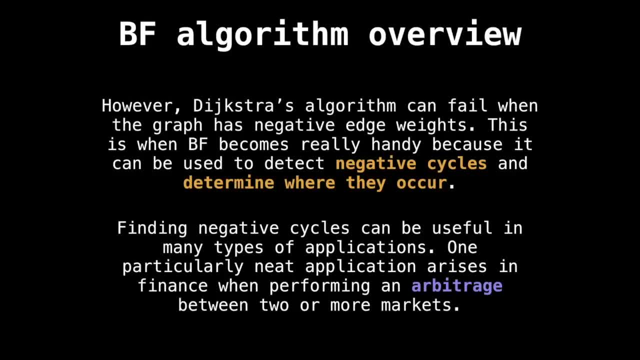 on performing an arbitrage between two or more markets. I'm not an expert, but this is an example of an arbitrage between two or more markets, So let's take a look at the graph. The graph shows that the prices between different markets are such that you can cycle through. 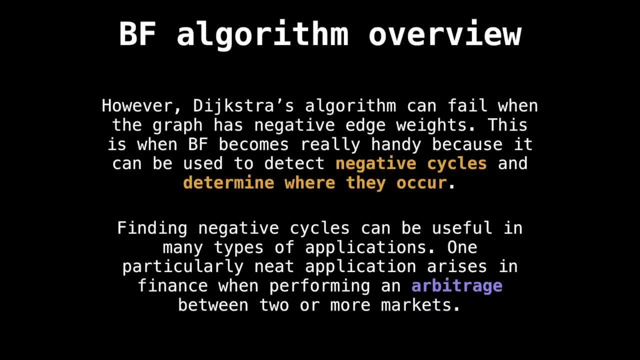 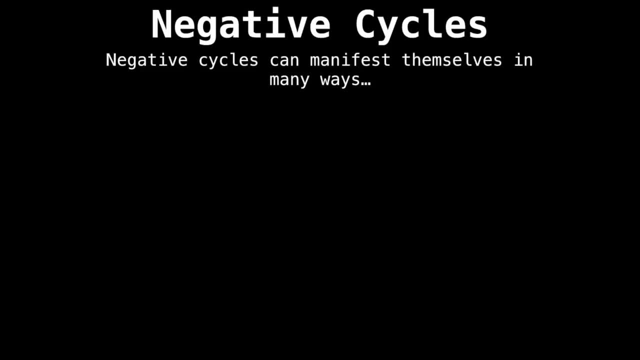 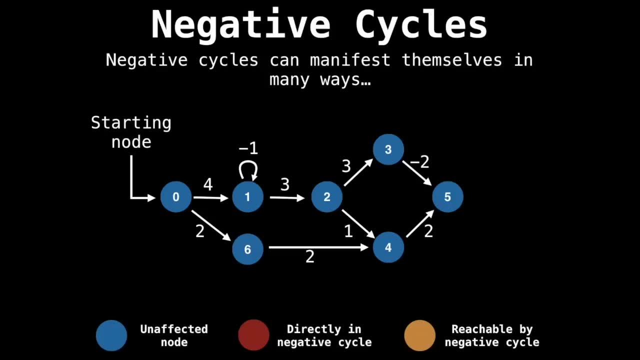 each market with a security, such as a stock or currency, and end up with more profit than you originally started, with essentially getting risk free gains. Let's look at how negative cycles can arise. because this seems important, Here is a graph I made with directed edges: 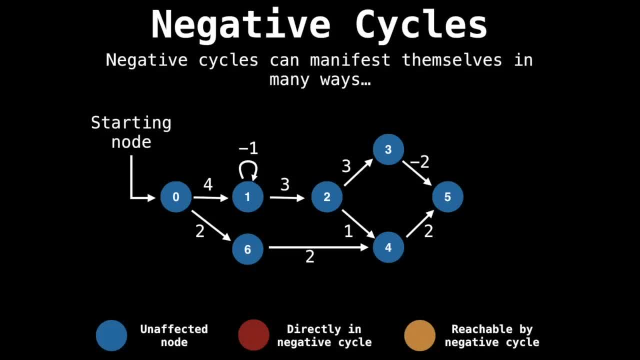 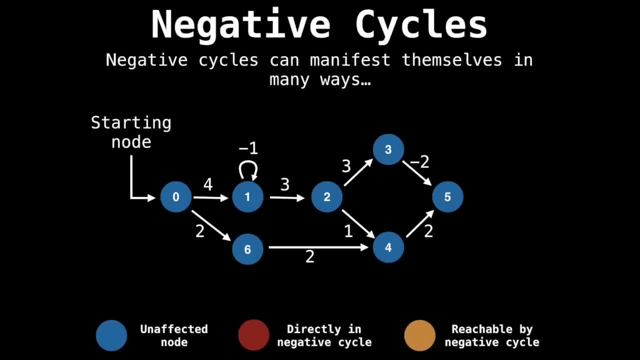 source: shortest path context. But right now we are only interested in detecting negative cycles. I will label blue nodes as regular nodes, red nodes as nodes directly involved in the negative cycle and yellow nodes as those reachable by a negative cycle One way. 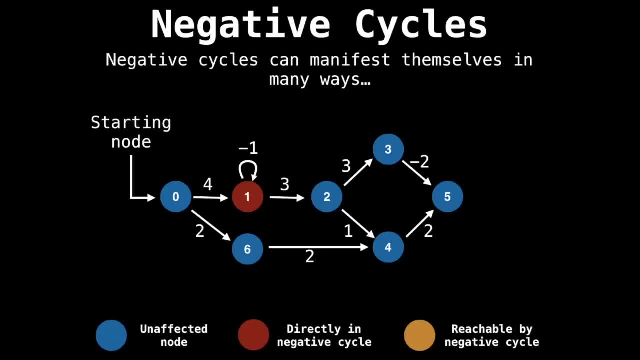 negative cycle cycles can emerge is through negative self loops. What happens is that once we reach a self loop, we can stay in that loop for a near infinite amount of time before exiting. As a result, everywhere reachable by the cycle has a best cost of negative infinity, which 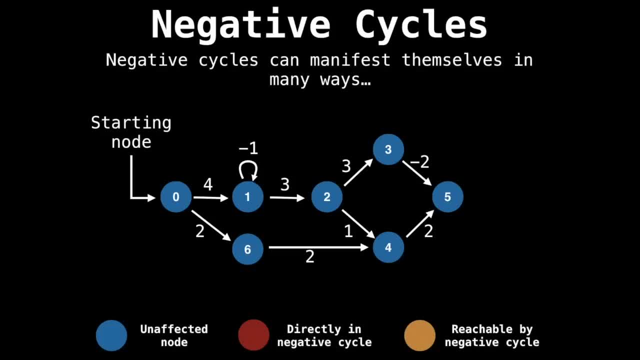 which are negative. I've labeled our starting node to be node zero And our goal would be to find the distance from zero to every other node in a single source- shortest path context. But right now we are only interested in detecting negative cycles. I will label blue nodes as regular nodes, red nodes as 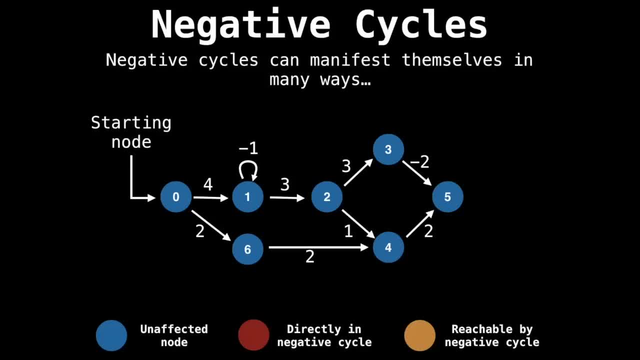 nodes directly involved in a negative cycle and yellow nodes as those reachable by a negative cycle. One way negative cycles can emerge is through negative self loops. What happens is that once we reach a self loop, we can stay in that loop for a near infinite amount. 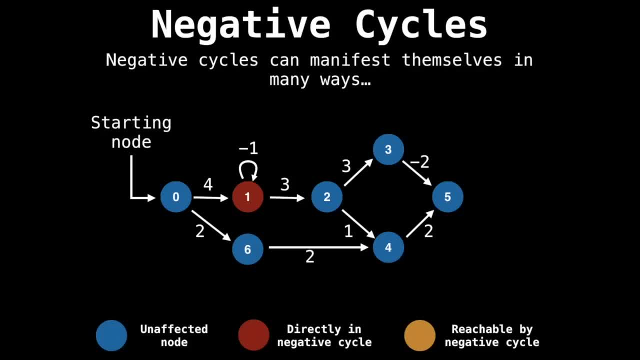 of time before exiting. As a result, everywhere reachable by the cycle has a best cost of negative infinity which, depending on your problem, may either be good or bad. In this graph, nodes 234 and five are all reachable by node one, So they all have a best cost of negative. 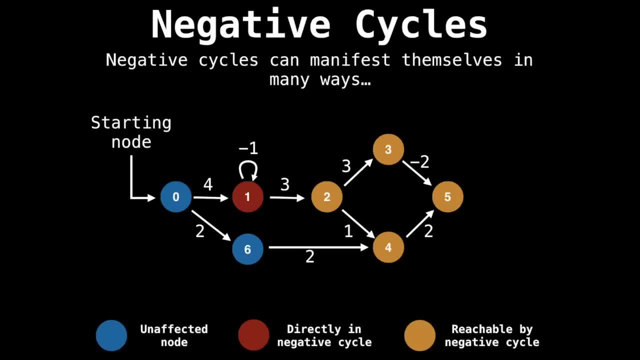 infinity. With regards to the single source shortest path problem, Let's look at another example. In this graph, a negative cycle manifests itself, but not as the result of a negative self loop, Instead through a cycle of nodes whose net gain is less than zero, If you add. 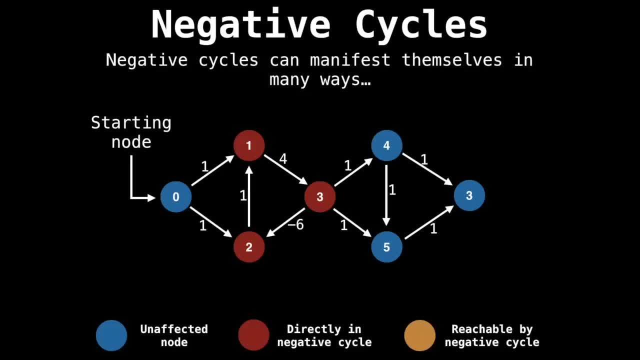 up the edge values one, four and minus six attached to the nose 12 and three, the net change is minus one. If we look at where the cycle can reach, we can see that the entire right side of the graph is affected, So hardly any nodes are safe from this negative cycle. Now let's 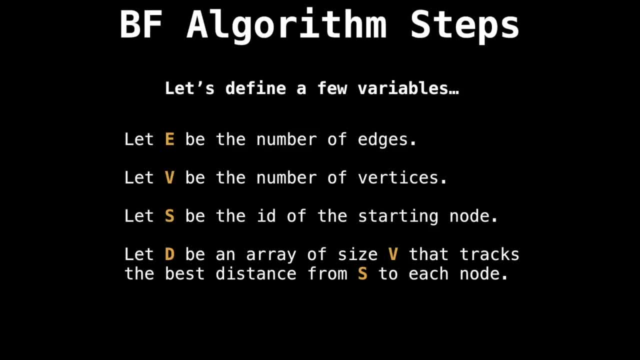 look at the actual steps involved in the Bellman Ford algorithm. First, we'll need to define a few variables. Let e be the number of edges in the graph, Let v be the number of vertices, Let s be the ID of the starting node- In this case s is short for start- And lastly, let d be an array. 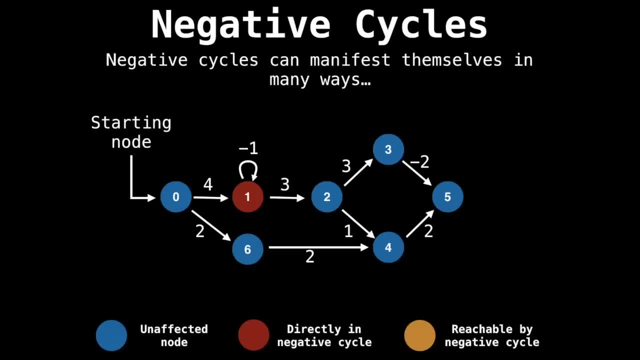 depending on your problem, may either be good or bad. In this graph, nodes 234 and five are all reachable by node one, So they all have a best cost of negative infinity. with regards to the single source shortest path problem, Let's look at another example In 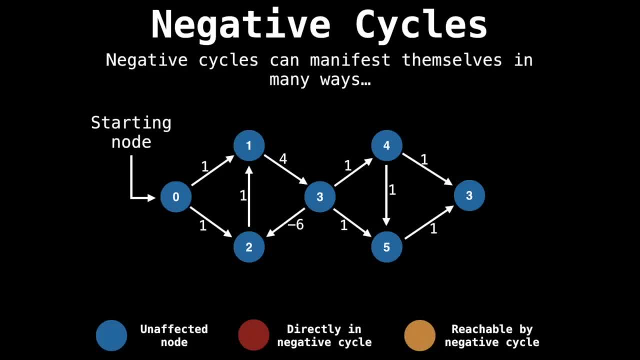 this graph, a negative cycle manifests itself, but not as the result of a negative self loop, Instead through a cycle of nodes whose net gain is less than zero. If you add up the edge values one, four and minus six, you get a negative self loop. If you add up the edge values one, four and minus. 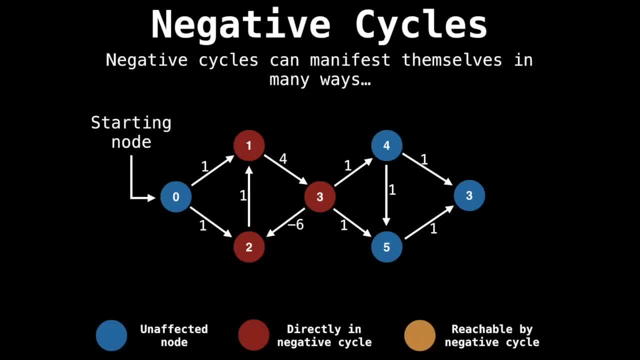 six. you get a negative self loop Instead through a cycle of nodes whose net gain is less than zero. if you add up the edge values one, four and minus six to the node's one, two and three, the net change is minus one. If we look at where the cycle can reach, we 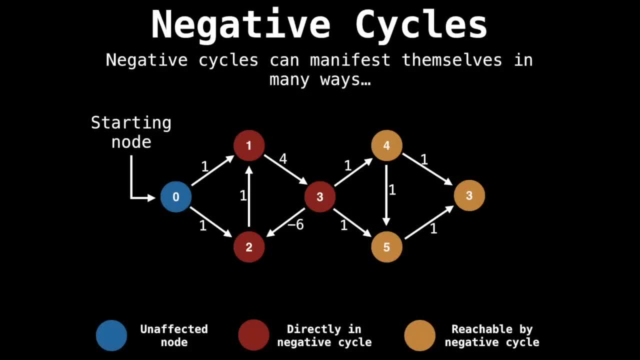 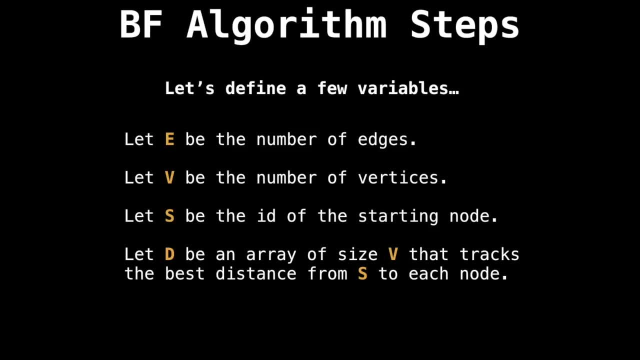 can see that the entire right side of the graph is affected, So hardly any nodes are safe from this negative cycle. Now let's look at the actual steps involved in the Bellman ford algorithm. First, we'll need to define a few variables. let e be the number of edges. 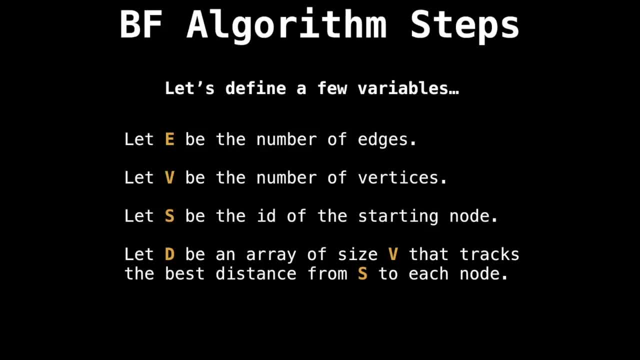 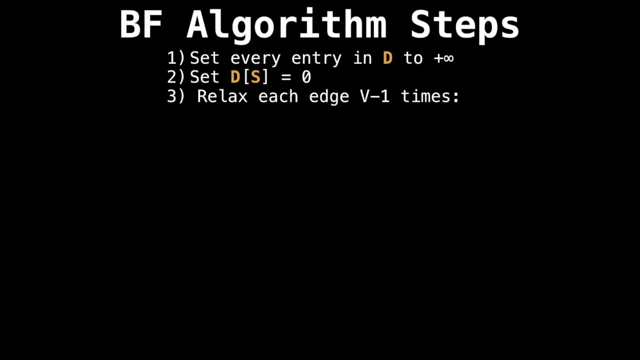 and grab restaurant graph. Let v be the number of vertices, Let s be the ID of the starting node- In this case, s is short for start- And lastly, let D be an array of size v that tracks the best distance from s to each node. The first thing we'll want to do is set every entry in D to: 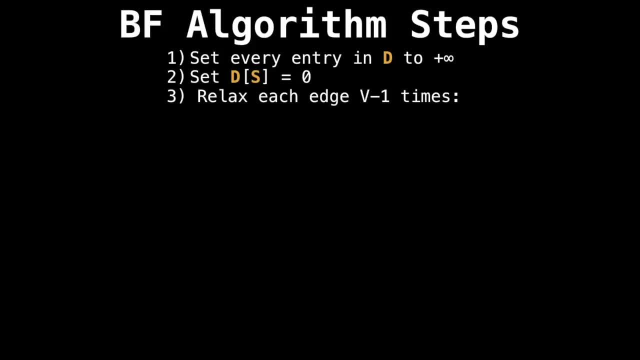 positive infinity. This is because the distance to each node is initially unknown and we have no idea how far each node is. Next, we'll want to set the distance to the starting node to be zero, because we're already there. The last part of the algorithm is to relax each 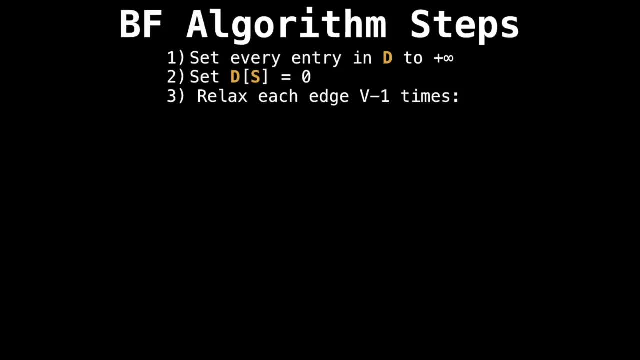 edge of v minus one times. Relaxing an edge simply means taking an edge and trying to update the value from where the edge starts to where it ends. Okay, so we're done with the first part of the algorithm. Now let's move on to the second. 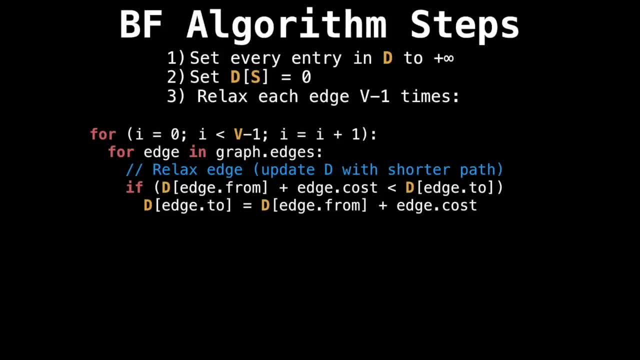 part of the algorithm. Let's go back to the first part of the algorithm and look at the first part of the algorithm In terms of code. this is all we need to do. We loop v minus one times. then for each edge, we relax the edge In the relaxing step. what we do is we look at the 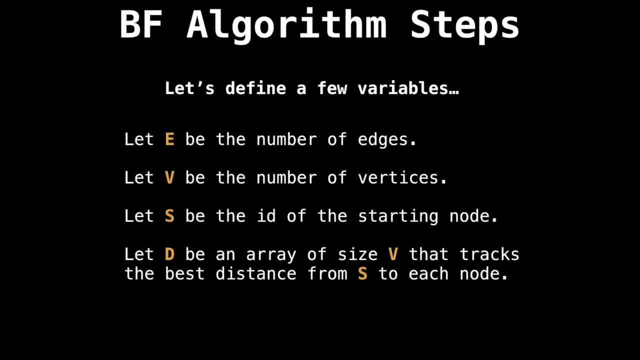 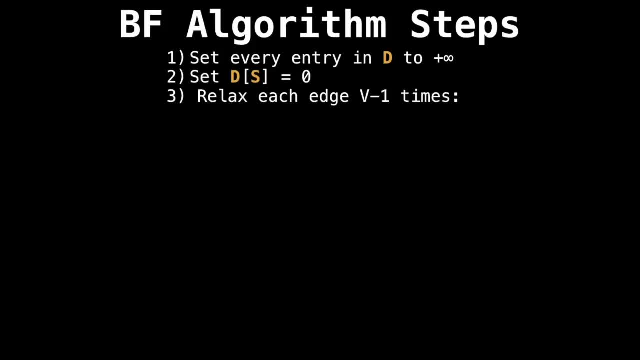 of size v that tracks the best distance from s to each node. The first thing we'll want to do is set every entry in D to positive infinity. This is because the distance to each node is initially unknown and we have no idea how far each node is. 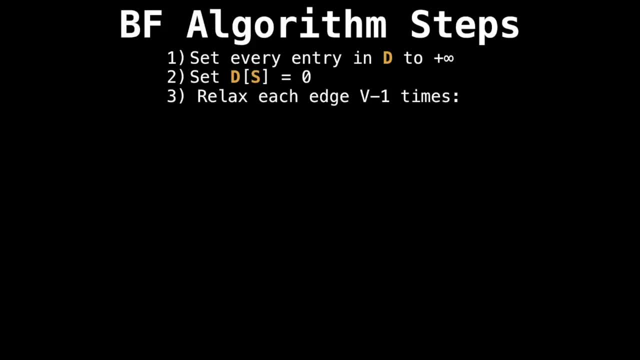 Next, we'll want to set the distance to the starting node to be zero, because we're already there. The last part of the algorithm is to relax each edge v minus one times. Relaxing an edge simply means taking an edge and trying to update the value from where the edge starts. 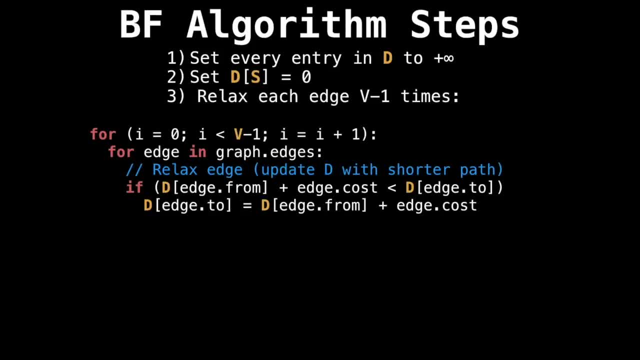 to where it ends In terms of code. this is all we need to do. We loop v minus one times, then for each edge, we relax the edge. So we're going to do a loop v minus one times, then for each edge, we relax the edge. 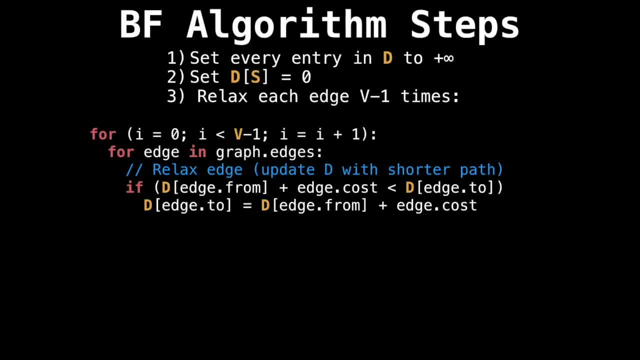 In the relaxing step. what we do is we look at the value of where the edge starts, add the edge cost and see if that's better than where we're trying to go And, if so, update with the shorter path value To actually detect negative cycles. we don't do anything too. 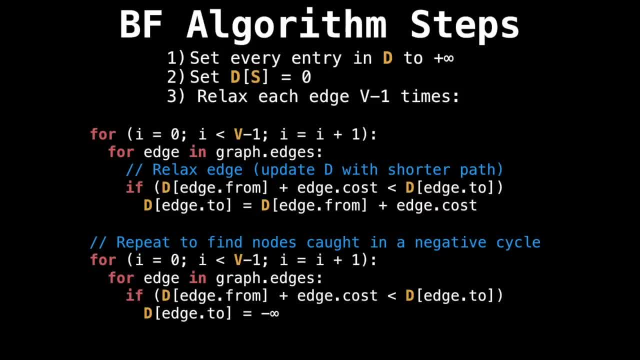 special. All we do is run the algorithm a second time. What we're doing in the second pass is checking for any nodes that update to a better value than the known best value, And if they do, then they're part of a negative cycle And we want to mark that node as having. 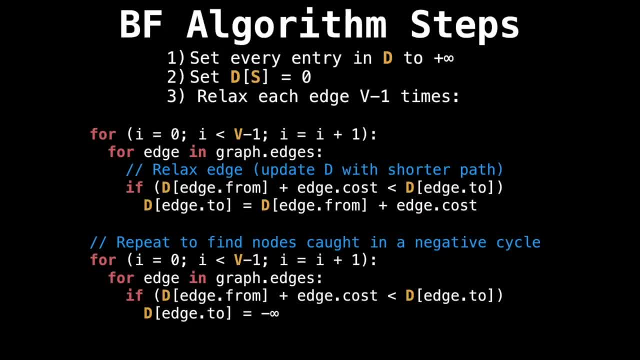 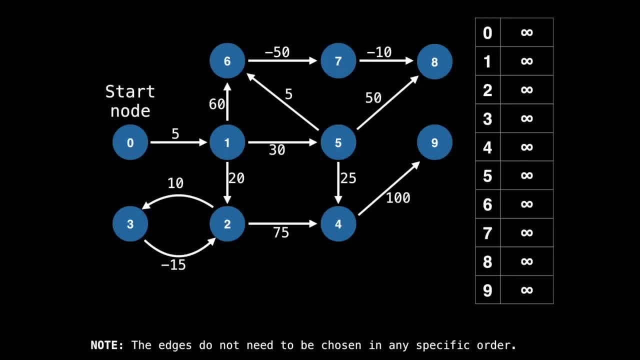 a cost of negative infinity. Let's look at a full example. Here is a graph I made. Again, we will start at node zero and find the shortest path to every other node. On the right I have illustrated the distance array D. Watch the values in this array change as the algorithm. 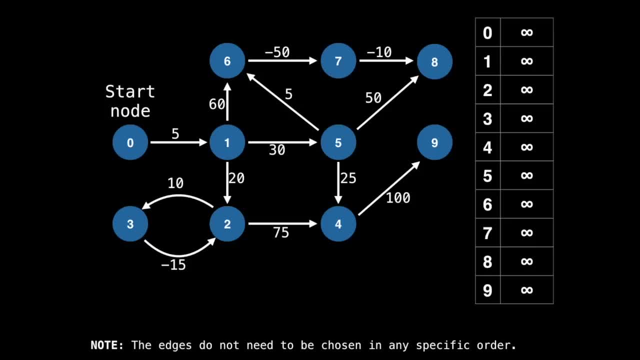 executes. Right now, all the values in the array are set to positive infinity, as per the first step of the algorithm. In the second step we set the starting nodes value to zero. Now the algorithm starts and we are on the first iteration where we attempt to relax each edge. 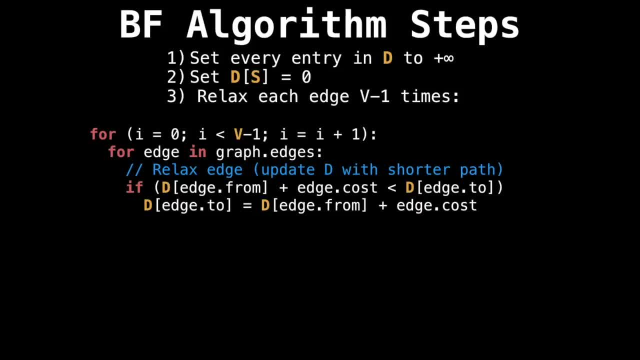 value of where the edge starts, add the edge cost and see if that's better than where we're trying to go And if so, update with the shorter path value To actually detect negative cycles. we don't do anything too special. All we do is run the value of v minus one times And we're 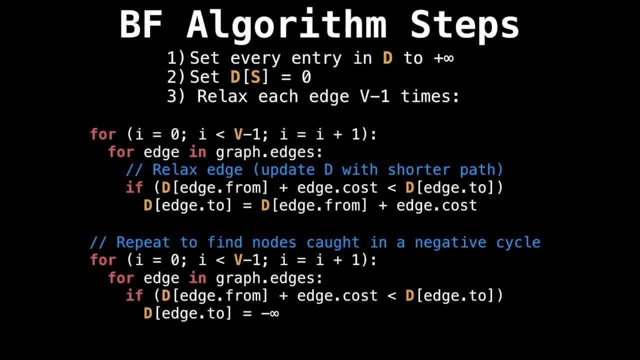 going to run the algorithm a second time. What we're doing in the second pass is checking for any nodes that update to a better value than the known best value, And if they do, then they're part of a negative cycle And we want to mark that node as having a cost. 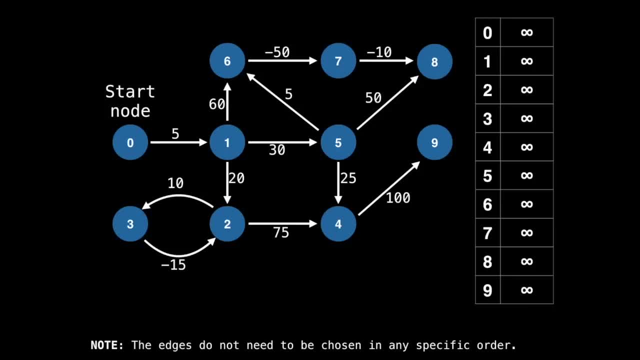 of negative infinity. Let's look at a full example. Here is a graph I made. Again, we will start at node zero and find the shortest path to every edge. On the right I have illustrated the distance array D. Watch the values in this array change. 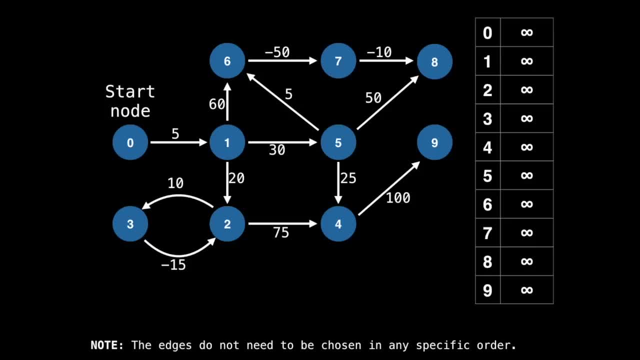 as the algorithm executes Right now, all the values in the array are set to positive infinity, as per the first step of the algorithm. In the second step we set the starting nodes value to zero. Now the algorithm starts and we are on the first iteration where we attempt. 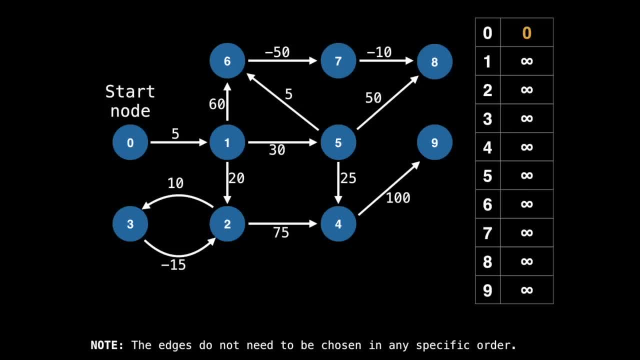 to relax each edge, But before we do that, we want to make sure that we have all the values in the array Before we continue. I have an important note at the bottom of the screen which says that the edges do not need to be processed in any particular order. I may process the edges. 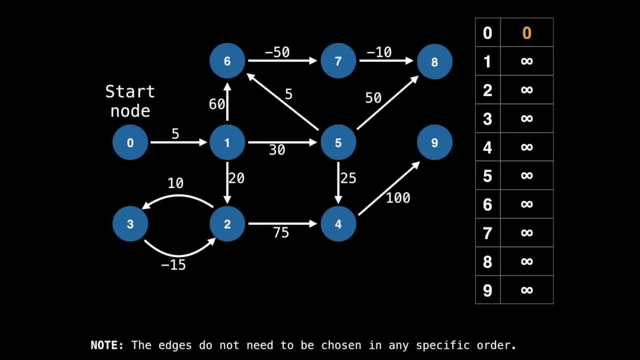 with one ordering and you process them with another ordering and we may not end up with the same values on each iteration, But we will get the same result in the distance array. at the very end I will highlight the edge currently being processed in orange and update. 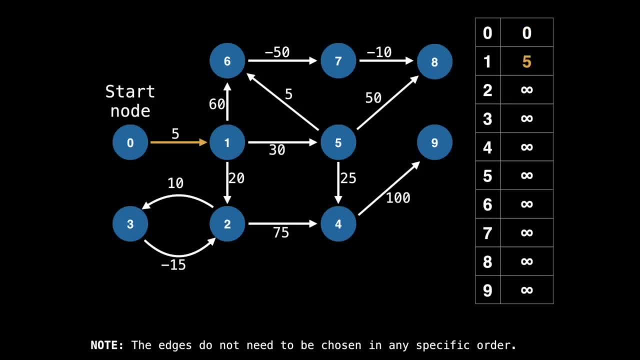 the distance array. Now we want to be able to see the edges in the same order as the distance array whenever appropriate. Right now, the best value to node one is five, because a distance of five is better than a distance of positive infinity. then node two gets its. 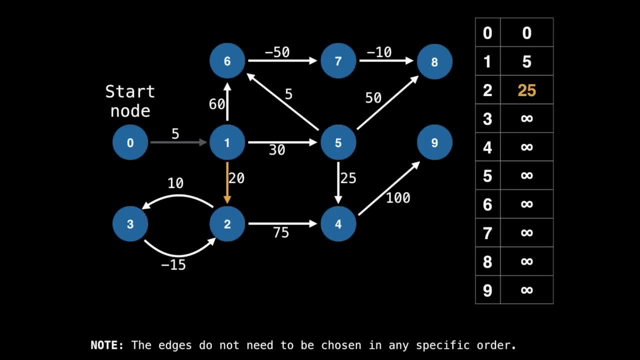 value updated to 25.. Because node one had a value of five from the last term and the edge from node one to node two is 20, for a total of 25.. Then a similar thing happens to node five and node six as well. By the way, an edge is dark gray if it has already. 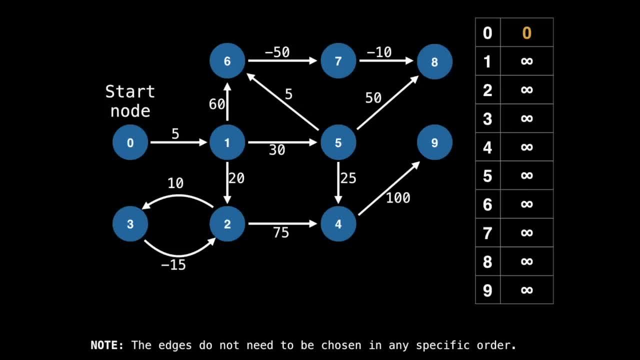 But before we continue, I have an important note at the bottom of the screen which says that the edges do not need to be processed in any particular order. I may process the edges with one ordering and you process them with another ordering, and we may not end up with the same values on each iteration, But we will get the same. 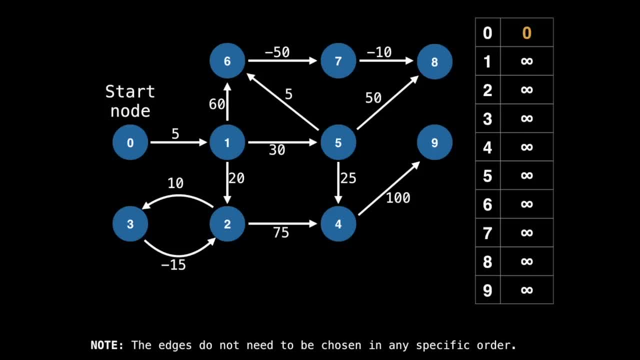 result in the distance array. At the very end I will highlight the edge currently being processed in orange and update the distance array whenever appropriate. Right now, the best value to node one is five, Because a distance of five is better than a distance of five. 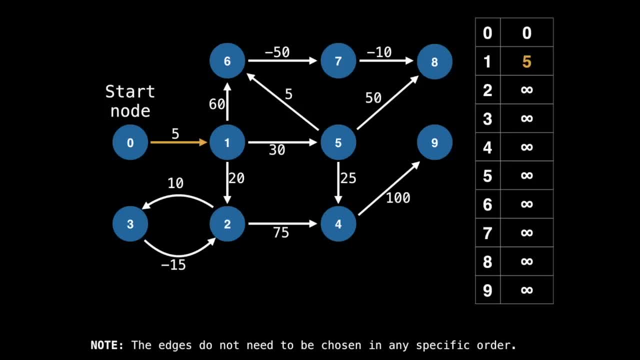 So I'm going to set the distance of five as negative infinity Rather than a distance of positive infinity. then node two gets its value updated to 25.. Because node one had a value of five from the last term and the edge from node one. 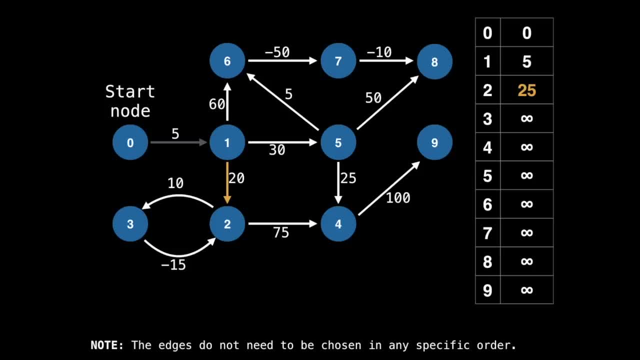 to node two is 20, for a total of 25.. Then a similar thing happens to node five and node six as well. By the way, an edge is dark gray if it has already been processed in this iteration. Next up, node three gets its value updated from infinity to 35. Because the best value 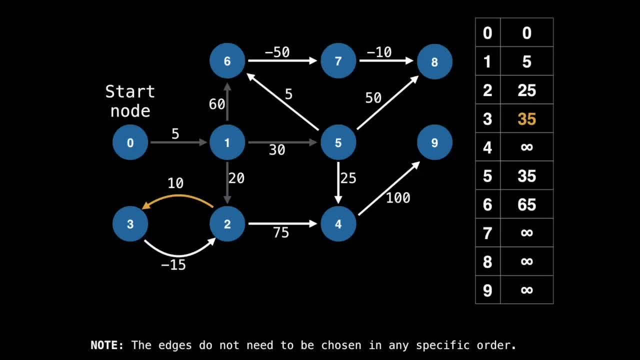 in node two so far as 25, plus the edge cost of 10 is 35. Then the edge from two to four updates to a best value of 100.. Up next is an interesting edge because it was able to update node twos best value from. 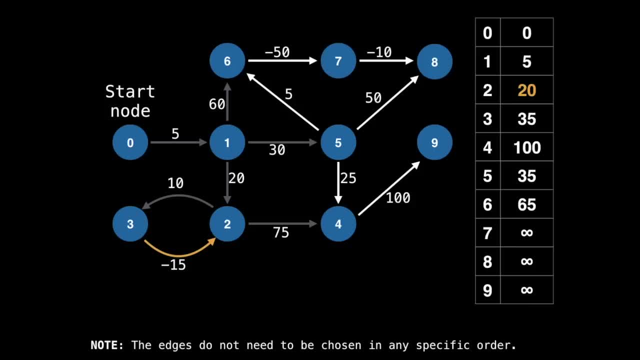 25 to 20.. By taking the value in node three, which is currently 35, adding a weight of minus 15 and giving us a better value of 20.. So this is all the algorithm does, processes each edge, performing relaxation operations. I'll let the animation play for the rest of this iteration. 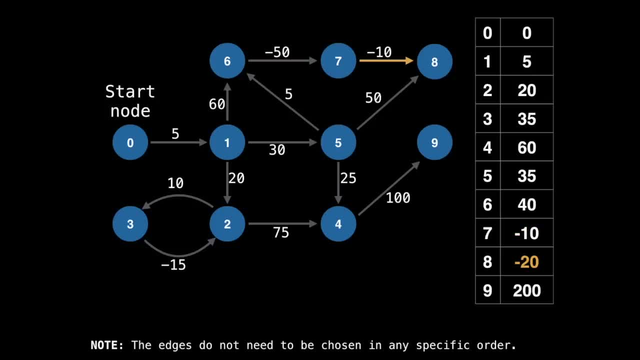 So iteration one is over and there are eight more iterations to go. But for simplicity I'll just play one more iteration to give you an idea of how the algorithm works. We reset all the edges and start processing the edges again. you'll notice that a lot less. 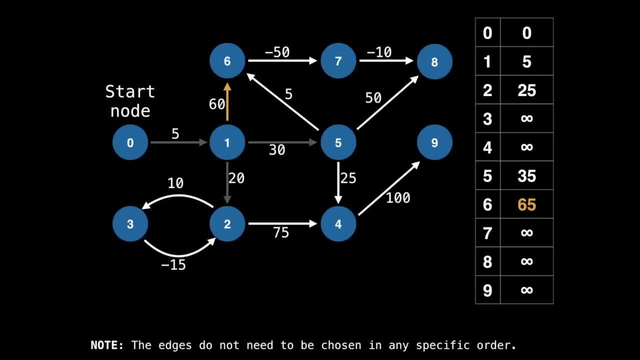 been processed in this iteration. Next up, node three gets its value updated from infinity to 35.. Because the best value in node two so far is 25.. Plus the edge cost of 10 is 35.. Then the edge from two to four updates to a best value of 100. 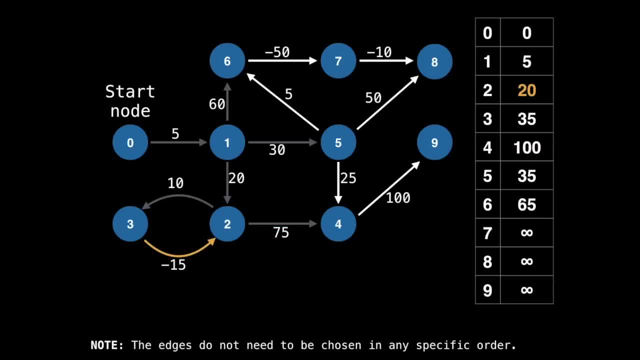 Up next is an interesting edge, because it was able to update node twos best value from 25 to 20.. By taking the value in node three, which is currently 35, adding a weight of minus 15 and giving us a better value of 20.. So this is all the algorithm does, a process. 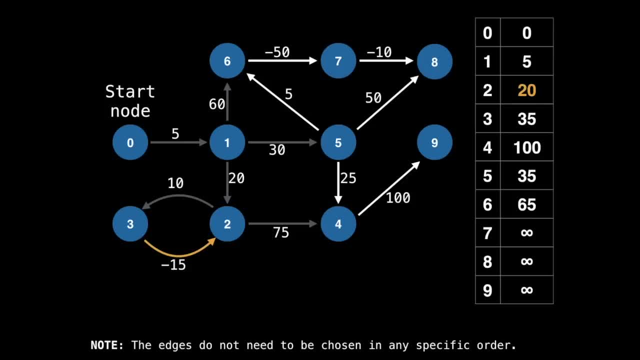 of practicing each edge, performing relaxation operations. I'll let the animation play for the rest of this iteration. So iteration one is over and there are eight more iterations to go. But for simplicity, I'm going to go ahead and add another iteration. So I'm going 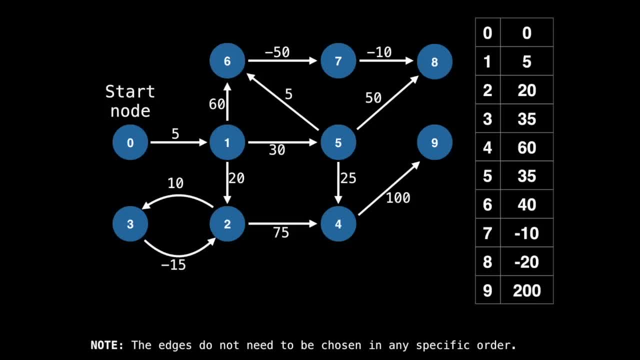 to go ahead and add another iteration. So I'm going to go ahead and add another iteration For simplicity. I'll just play one more iteration to give you an idea of how the algorithm works. We reset all the edges and start processing the edges again. you'll notice that a lot. 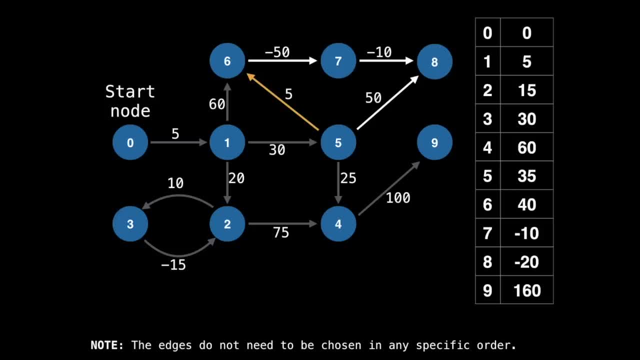 less updating happens in the distance array this round, particularly because I unintentionally selected the edges to be processed in a more or less optimal way. So that's the end of the second iteration. If we fast forward to the second iteration, we can see that we've 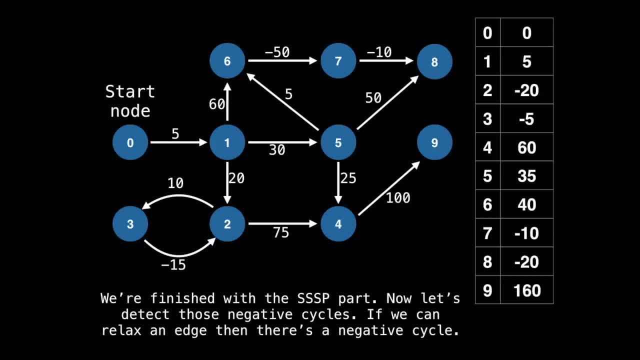 got two edges And if we fast forward to the end, here's the resulting distance array. However, we're not done. we still need to find the negative cycles. Let's execute the algorithm a second time, Same procedure as usual, just relax each edge. But when we are, 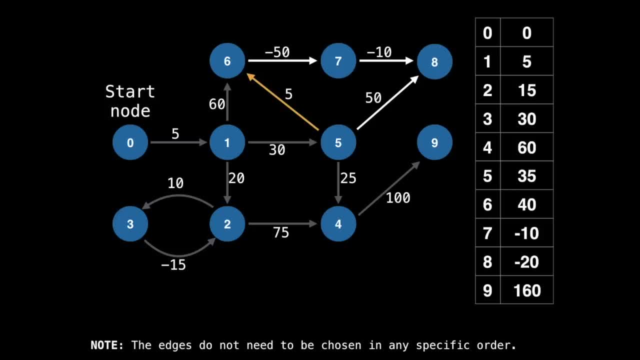 updating happens in the distance array this round, Particularly because I unintentionally selected the edges to be processed in a more or less optimal way. So that's the end of the second iteration. If we fast forward to the end, here's the resulting distance array. However, we're not done. we still need to find the 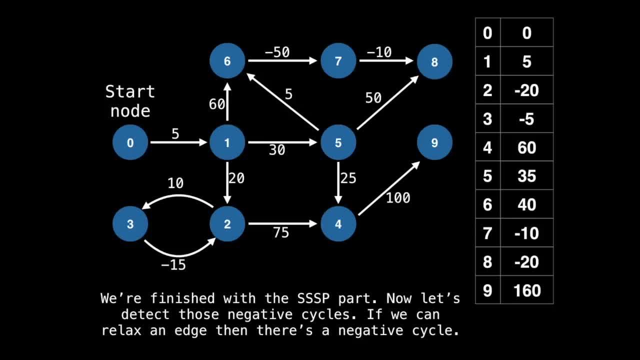 negative cycles, Let's execute the algorithm a second time. Same procedure as usual. just relax each edge. But when we are able to relax an edge, update the nodes value to negative infinity. instead, Let's process some edges until something interesting happens. So it appears that when we went from node two to 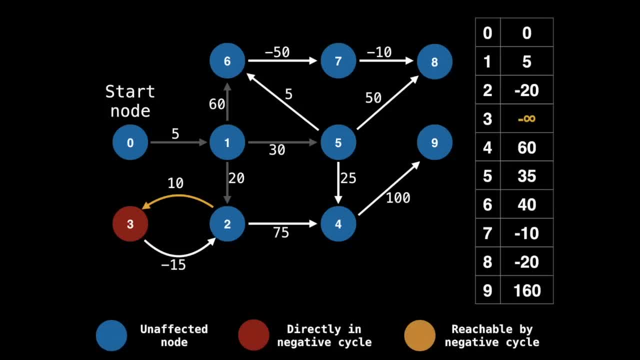 node three. we are able to relax the edge and obtain a better value for node three than was previously there. So node three is part of some negative cycle. Therefore I will mark it as red. Similarly, node four is connected to a negative cycle, although indirectly in the distance. 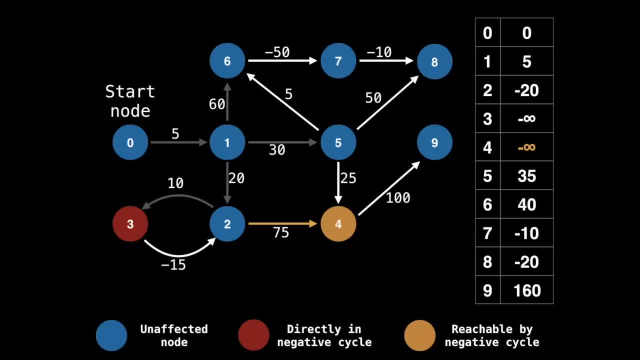 table. I do not distinguish between nodes which are reachable by a negative cycle and those which are primarily involved in one, So there's no way to tell them apart. Feel free to add some logic in the Bellman ford algorithm if you need to make this distinction. 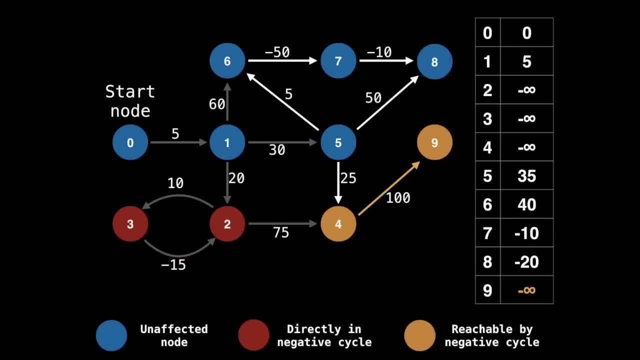 Continuing on, new two is also trapped in the cycle, And the last node also affected by the cycle is node nine on the right. Let's finish up with this iteration by processing the rest of the edges. So that's it for the first iteration. there are another eight iterations to perform In. 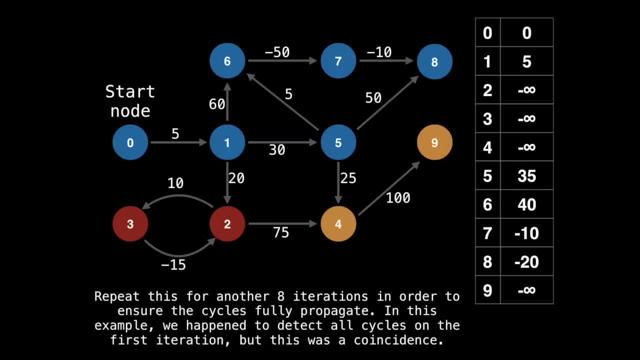 this example, we happen to detect all cycles on the first iteration, But this was a coincidence, though. In general, you really need another eight iterations. This is because you want the negative cycle minus infinity values to propagate throughout the graph. The propagation is highly dependent. 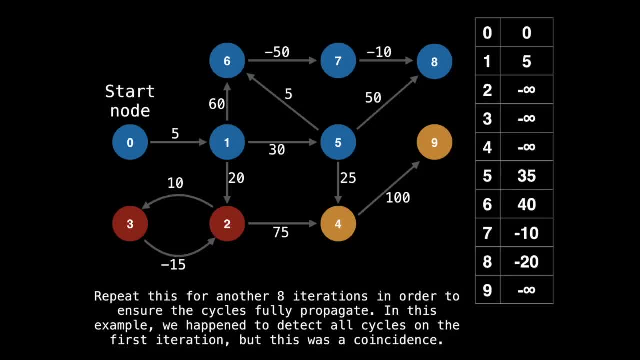 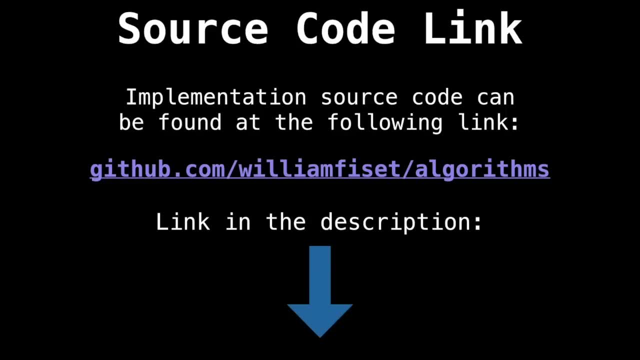 on the order in which the edges are being processed, But having v minus one iterations ensures that this propagation occurs correctly. All right, now I want to have a look at some source code. you can find a link in the description below, Or you can go to githubcom And you. 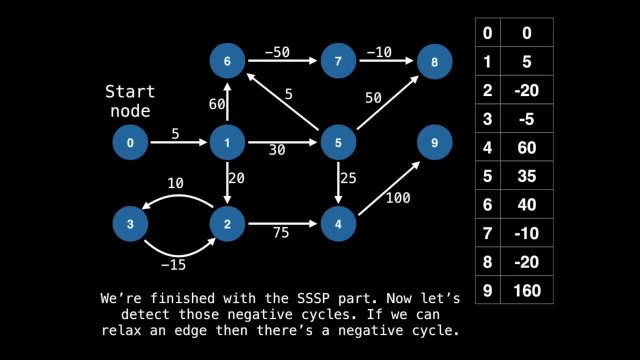 able to relax an edge, update the nodes value to negative infinity. instead, Let's process some edges until something interesting happens. So it appears that when we went from node two to node three, we are able to relax the edge and obtain a better value for node three than was previously there. So node three 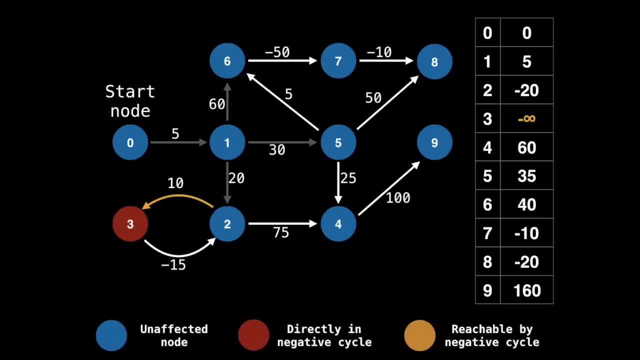 is part of some negative cycle. Therefore I will mark it as red. Similarly, node four is connected to a negative cycle, although indirectly. in the distance table I do not distinguish between nodes which are reachable. So node three is connected to a negative cycle and node four is connected to a negative cycle. 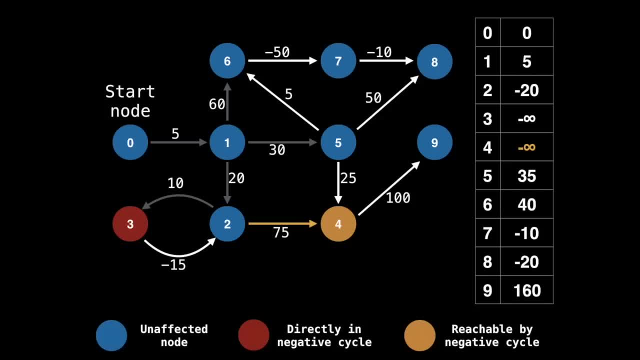 So there's no way to tell them apart. Feel free to add some logic in the Bellman Ford algorithm if you need to make this distinction. Continuing on, node two is also trapped in the cycle, And the last node also affected by the cycle is node nine on the right. Let's 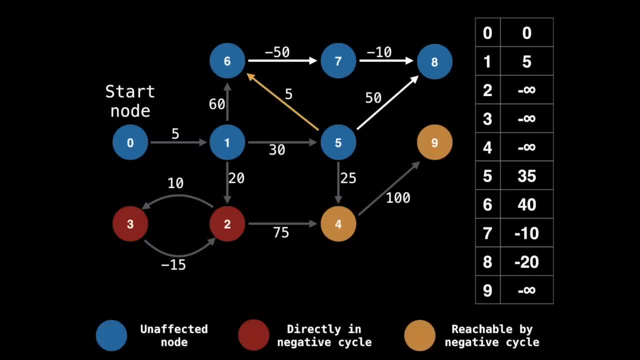 finish up with this iteration by processing the rest of the edges. So that's it for the first iteration. there are another eight iterations to perform. In this example we happen to detect all cycles on the first iteration, But this was a coincidence. 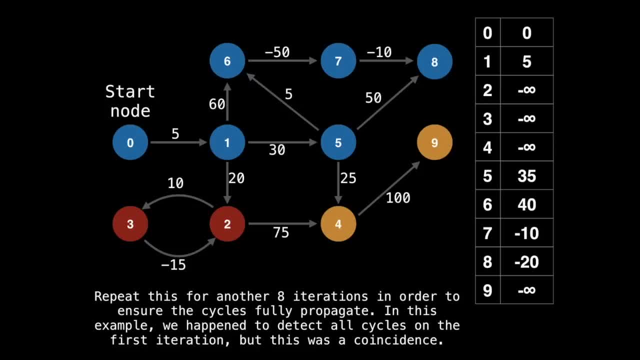 In general, you really need another eight iterations. This is because you want the negative cycle minus infinity values to propagate throughout the graph. The propagation is highly dependent on the order in which the edges are being processed, But having v minus one iterations ensures that this propagation occurs correctly. All right, now I want to have a look at some. 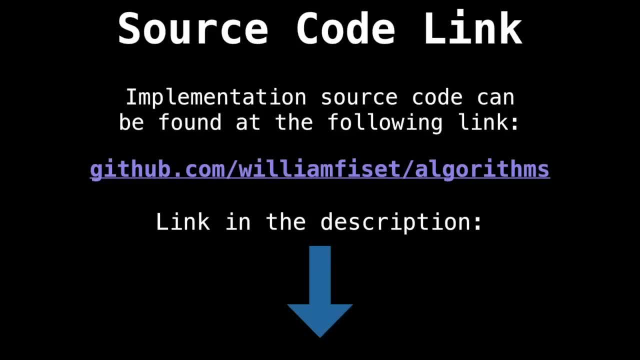 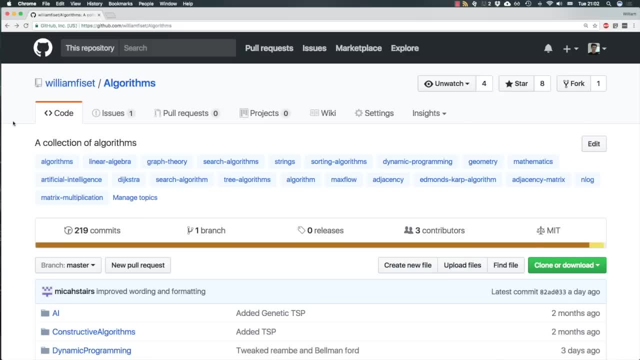 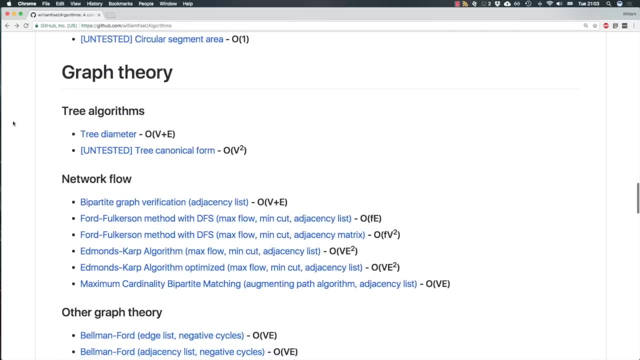 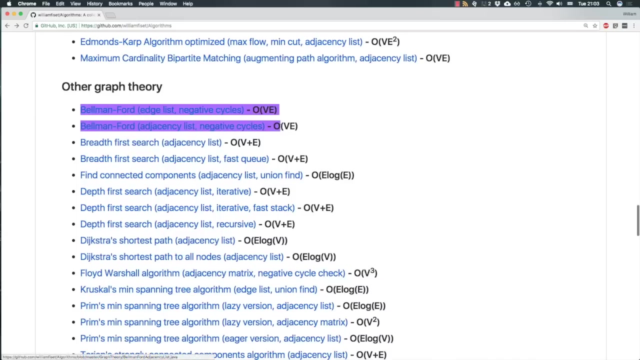 source code. you can find a link in the description below Or you can go to githubcom. slash William physio slash algorithms. Here we are on GitHub in my algorithms repository Now. if you scroll down and look for Belman Ford under the graph theory section, you can see that currently there are two different. 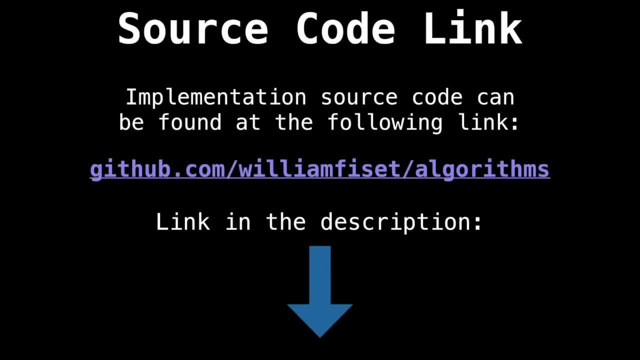 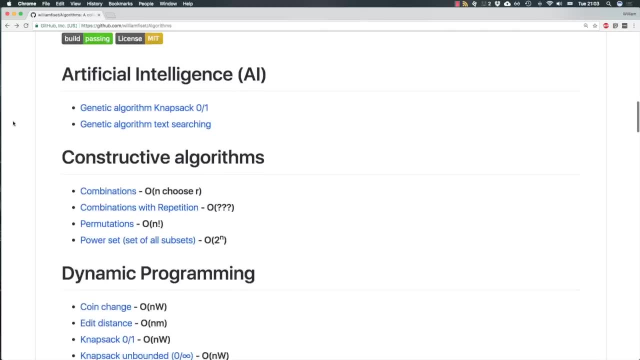 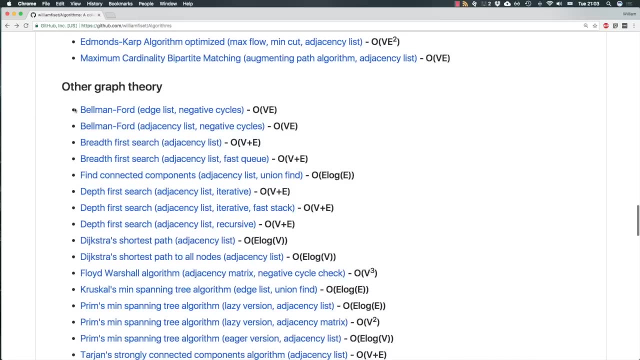 can also go to githubcom: slash William physio slash algorithms. Here we are on GitHub in my algorithms repository. Now. if you scroll down and look for Bellman Ford under the graph theory section, you can see that currently there are two different implementations: one: 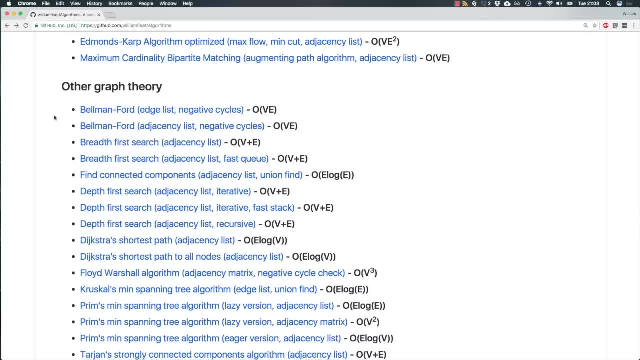 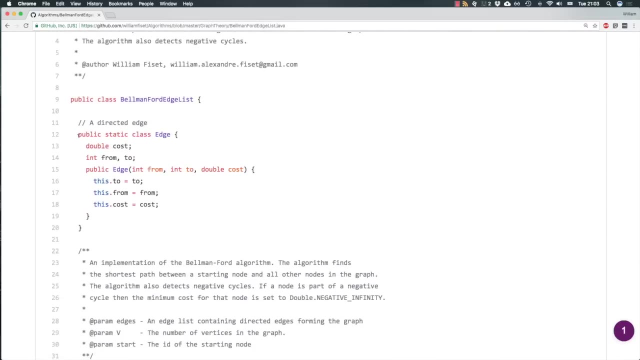 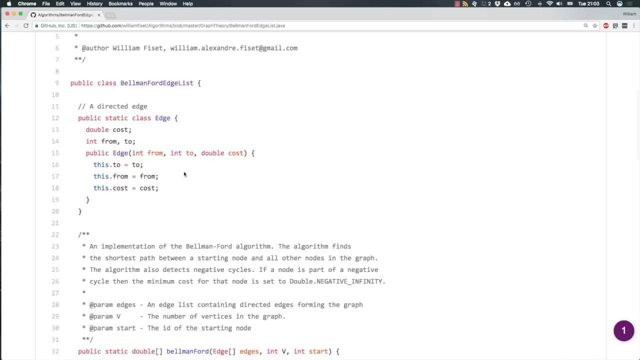 for graph represented as an edge list, another one for a graph represented as an adjacency list. Today we'll have a look at the edge list implementation. So in the edge list implementation, first thing I do is I define a directed edge, And a directed edge simply consists of an. 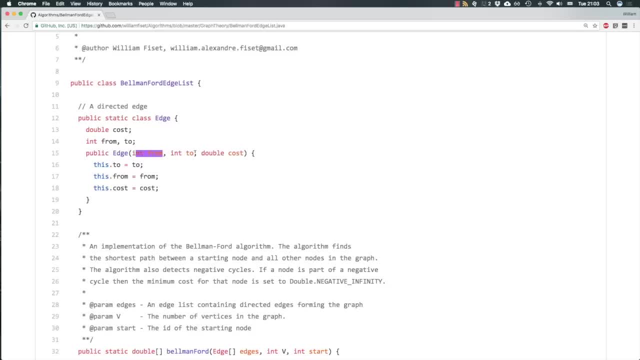 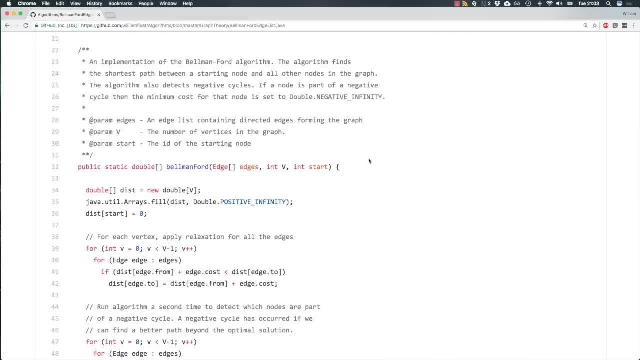 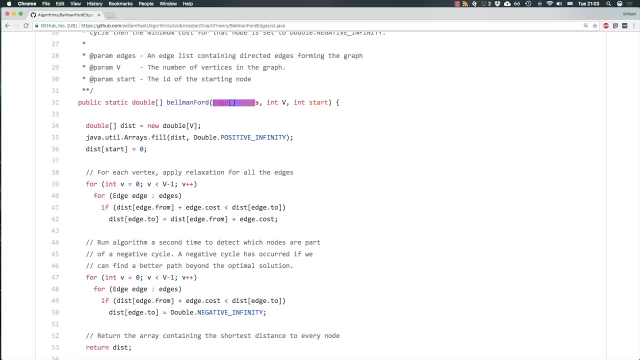 edge that goes from a node to a node with a certain cost. Next, let's have a look at the actual algorithm itself. So for Bellman Ford, what we need is, well, a graph. So since this is an edge list, we just pass in all the edges. I'll also need the number of vertices in 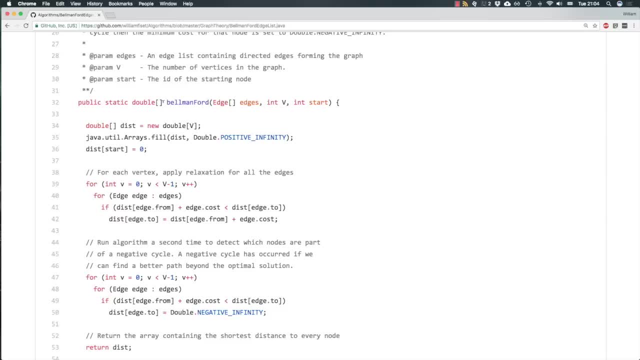 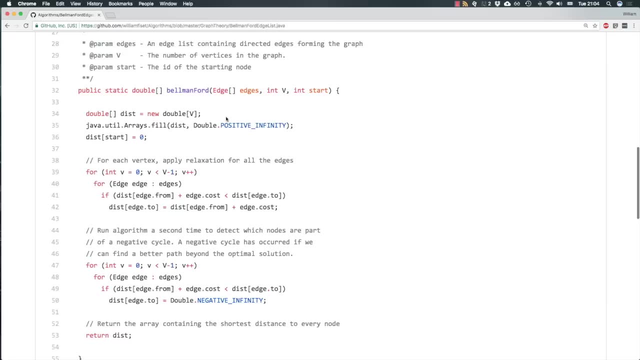 the graph and some starting node, And what we're returning is that distance array. Alright, so let's initialize the distance array and then populate it with this special array. So I'm going to use this special value, double dot positive infinity, then set dist of start. 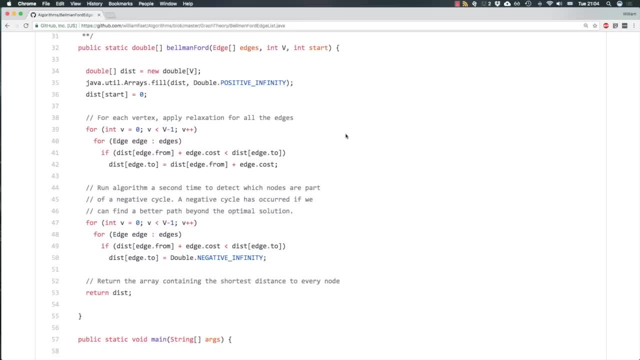 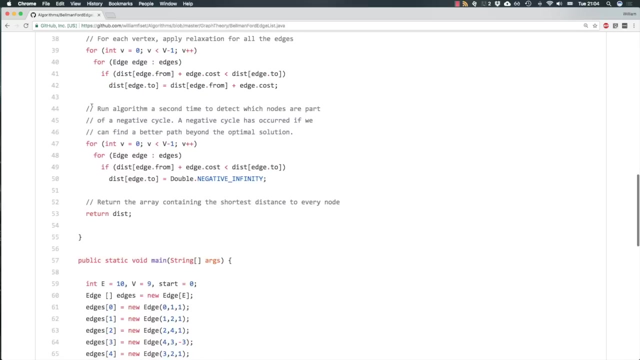 to be zero And then, just as the pseudocode said, just loop v minus one time. then, for each edge, just relax the edge. So that's what we're doing And here Now. this second pass of the algorithm is to detect negative cycles. 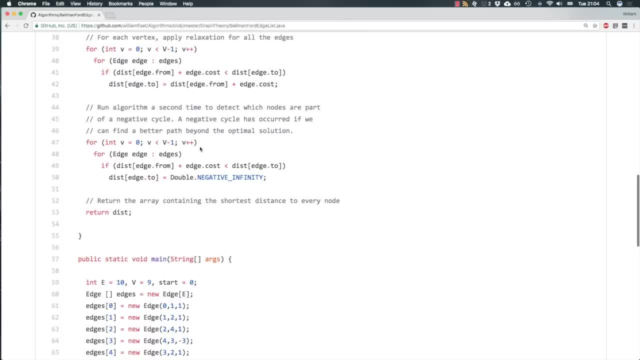 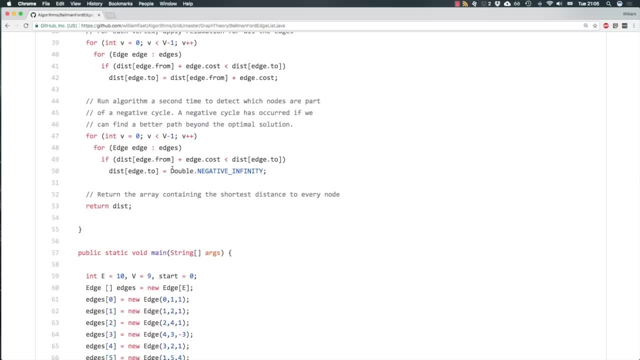 So run the algorithm a second time. So loop v minus one times for each edge, relax the edge, But this time, instead of updating the edge to a better value, we set the value to double dot negative infinity, And this is a special value defined in Java that represents 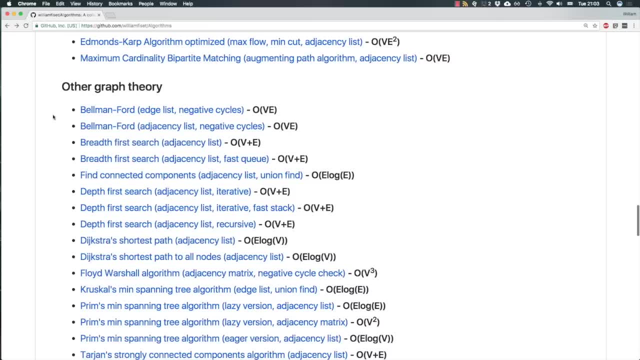 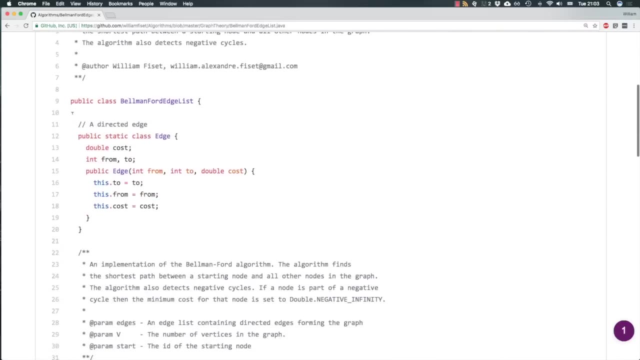 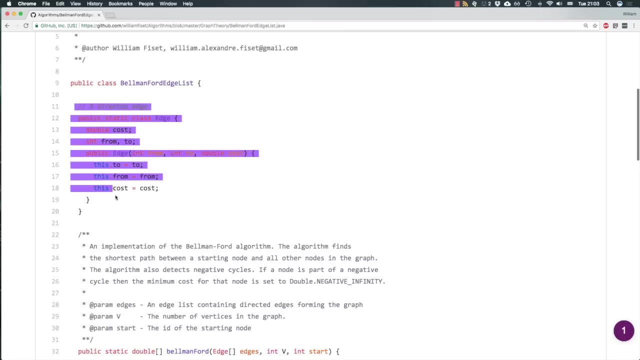 implementations: one for graph represented as an edge list, another one for a graph represented as an adjacency list. Today we'll have a look at the edge list implementation. So, in the edge list implementation, first thing I do is I define a directed edge, And a directed edge simply consists of an edge that goes from a node. 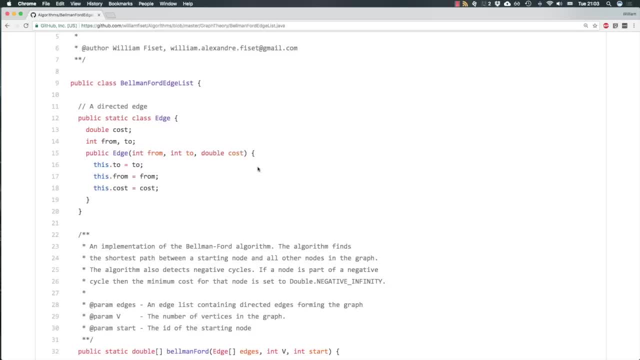 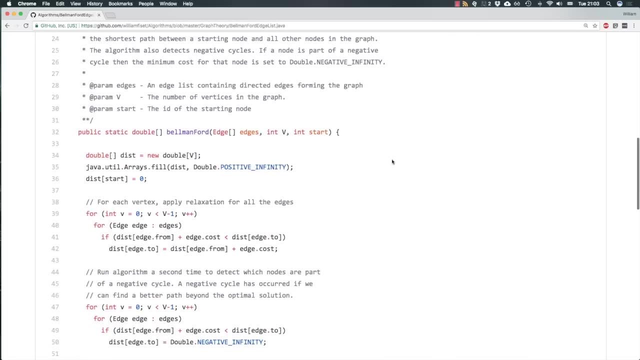 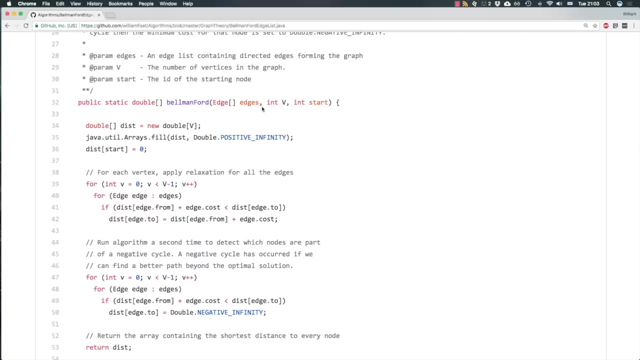 to a node with a certain cost. Next, let's have a look at the actual algorithm itself. So for Bellman Ford, what we need is, well, a graph. So since this is an edge list, we just pass in all the edges. I'll also need the number of vertices in the graph and some 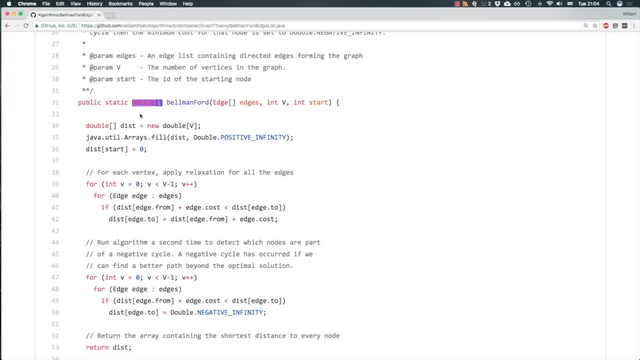 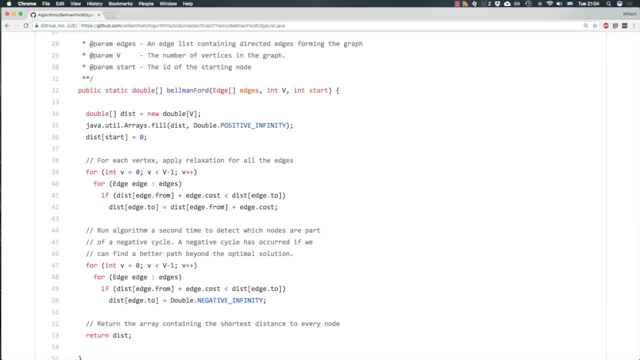 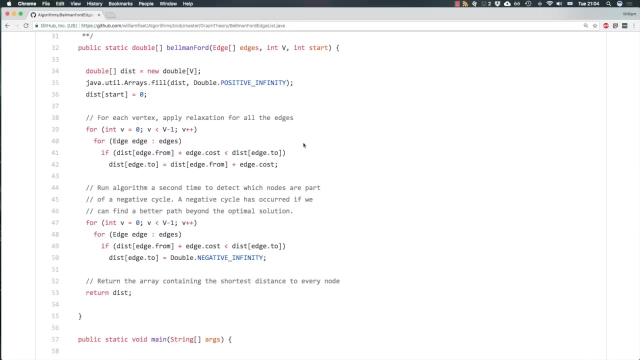 starting node, And what we're returning is that distance array. Alright, so let's initialize the distance array and then populate it with this special value, double dot, positive infinity, then set dist of start to be zero. And then just notice, as the pseudocode said, just loop v minus one time, then for each edge, just. 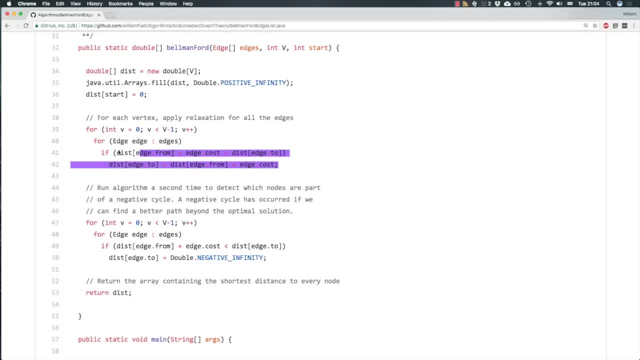 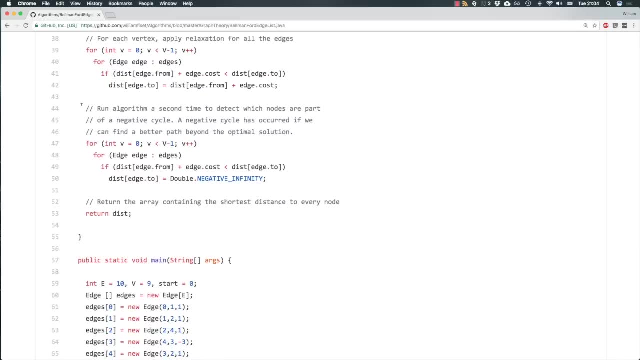 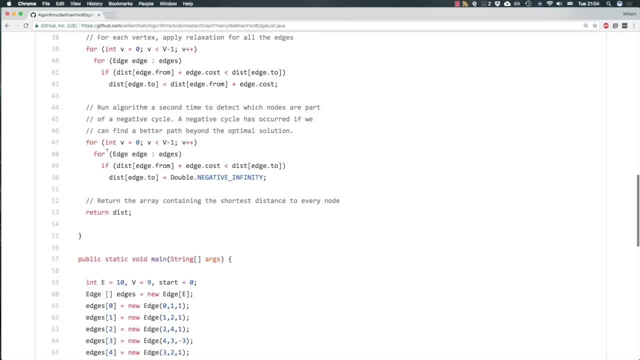 relax the edge. So that's what we're doing. And here Now. this second pass of the algorithm is to detect negative cycles. So run the algorithm a second time. so loop v minus one times for each edge. relax the edge, But this time instead of updating the edge to a better state. 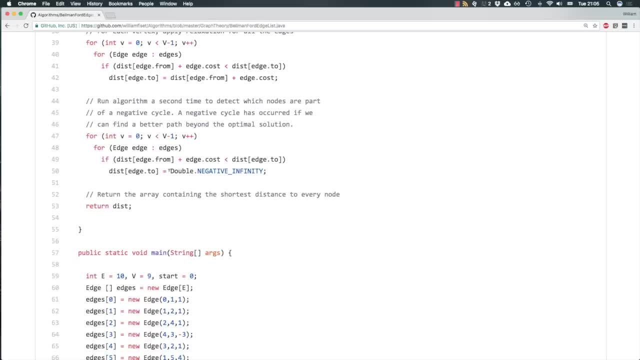 let's say a zero, then we're doing the same things again, the same way. value: we set the value to double dot negative infinity, And this is a special value defined in Java that represents negative infinity, And no matter what value you add to double. 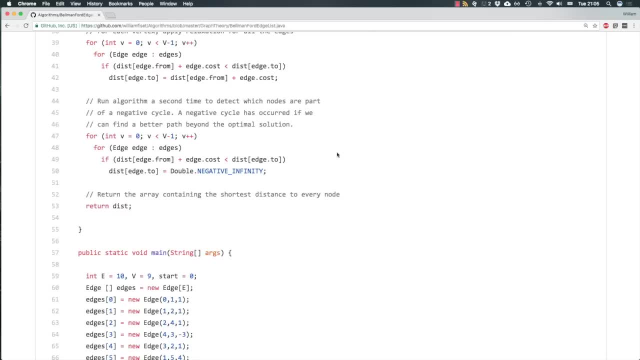 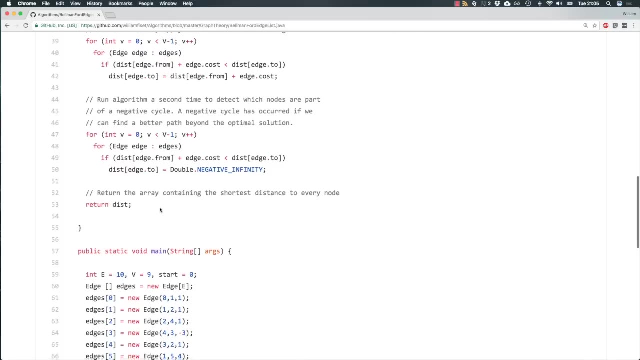 dot negative infinity, it will still be negative infinity Unless you add double dot positive infinity, then I think, gives you double dot, not a number or something like that, And that's the entire algorithm. then we just return the distance array And if you look in the 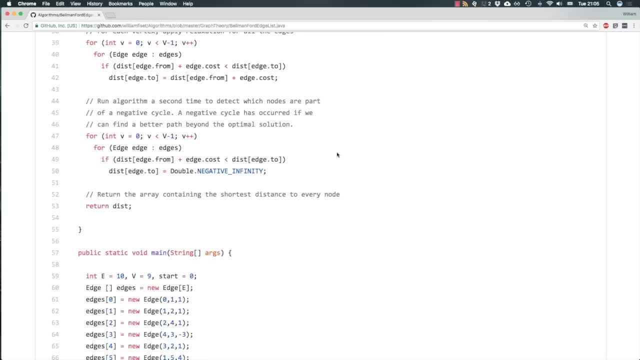 negative infinity And no matter what value you add to double dot negative infinity, it will still be negative infinity. Unless you add double dot positive infinity, then, I think, gives you double dot, not a number or something like that, And that's the entire algorithm. then we just return the distance. 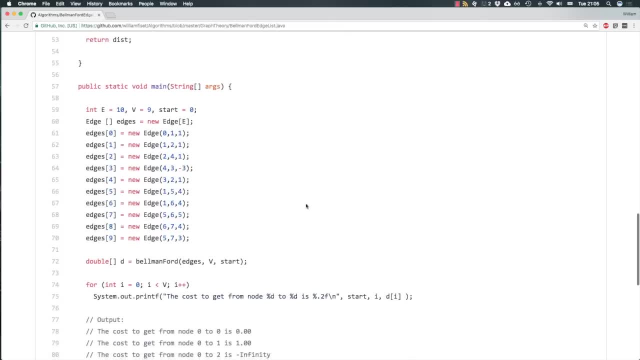 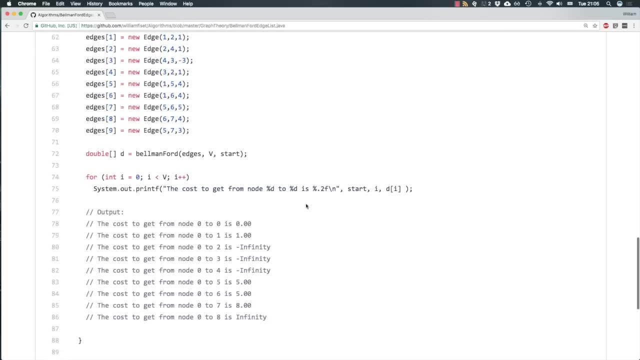 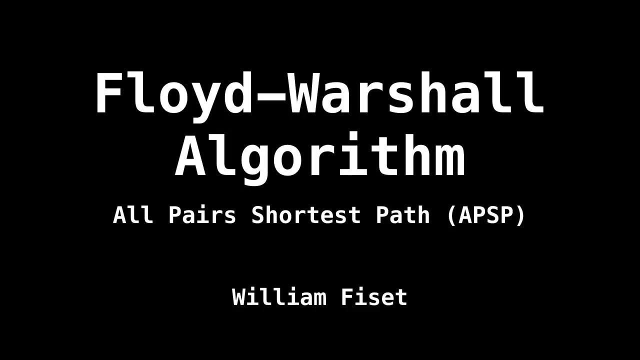 array And if you look in the main method, it shows you how to actually create a graph: add some edges and then run Bellman forward and find the distance from a starting node to all other nodes in the graph, And that is Bellman forward. 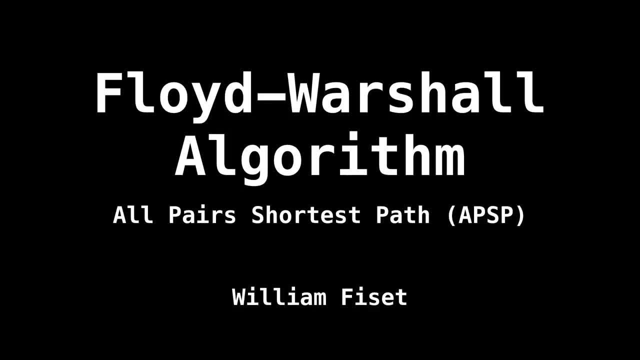 Now let's move on to the next topic is the Floyd Warshall all pairs- shortest path algorithm. we will be covering how the algorithm works, how to reconstruct shortest paths, the handling of negative cycles, followed by some code. So let's get started In graph theory, the 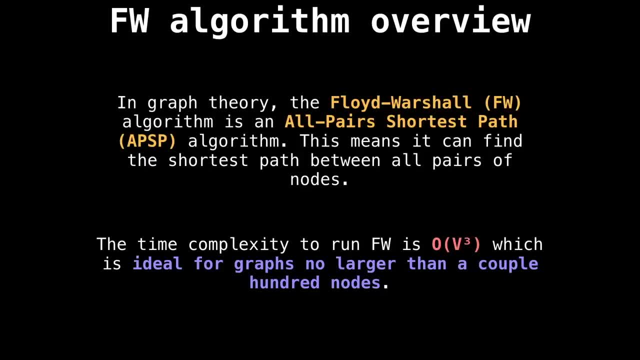 Ford Warshall algorithm is an all pairs shortest path algorithm. This means it can find the shortest path between all pairs of nodes. This is very important for many applications across several fields. The time complexity to run for the Warshall is big. O of v cubed, v being the number of. 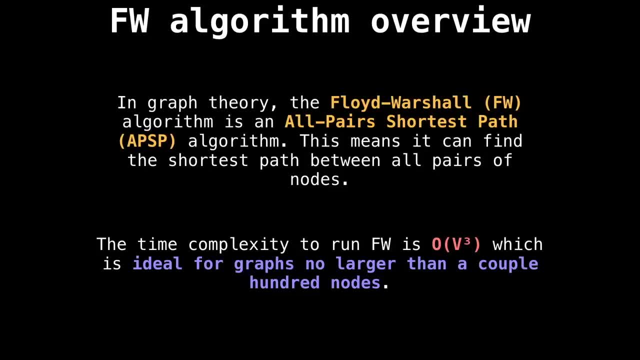 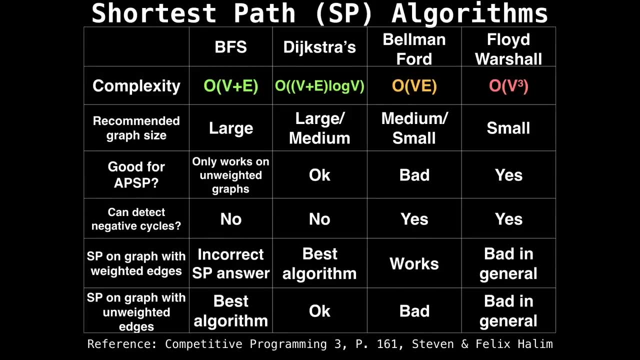 vertices in a graph. This makes the algorithm ideal for graphs with no more than a couple 100 nodes. Before we dive too deeply into the Ford Warshall algorithm, I want to address when you should and should not use this algorithm. This table gives information about various 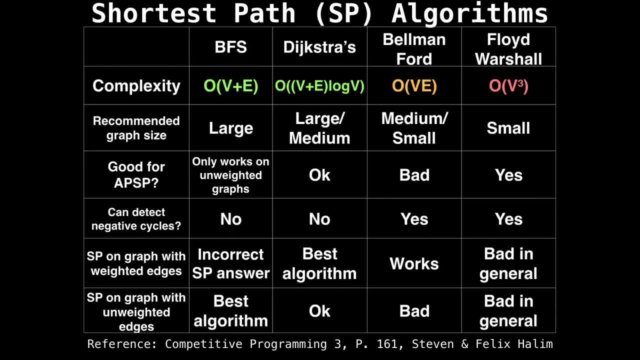 types of graphs and or constraints In the leftmost column and the performance or outcome of common shortest path algorithms. For example, you can see in the second row that a breadth first search and Dykstra's can handle large graphs with lots of nodes, while Bellman Ford and Florida Warshall not so much. I suggest 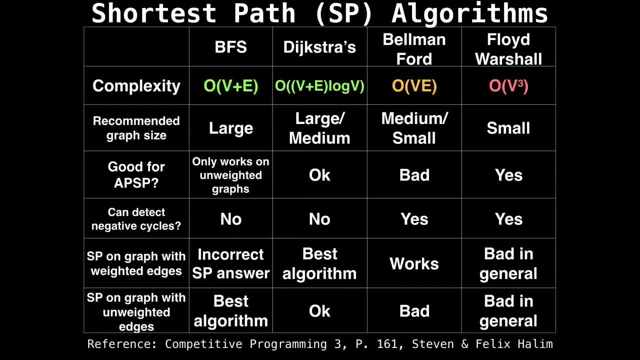 you pause the video and really go through this table and make sure you understand why each cell has the value it does. What I want to highlight is the number of nodes that are present in the graph. The number of nodes that are present in the graph is the rightmost. 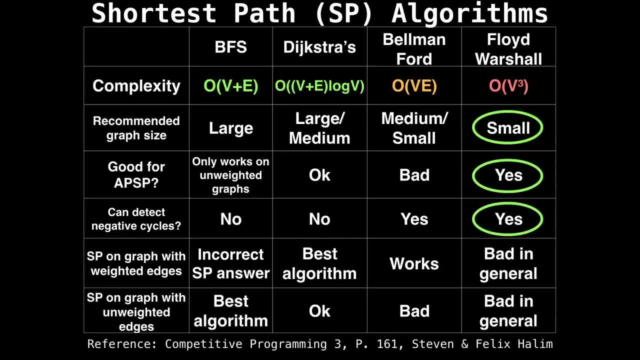 column, Since we're talking about the Floyd Warshall algorithm. the Floyd Warshall algorithm really shines in three places, And those are on small graphs: solving the all pairs, shortest path problem and detecting negative cycles. You can use the algorithm for other tasks. 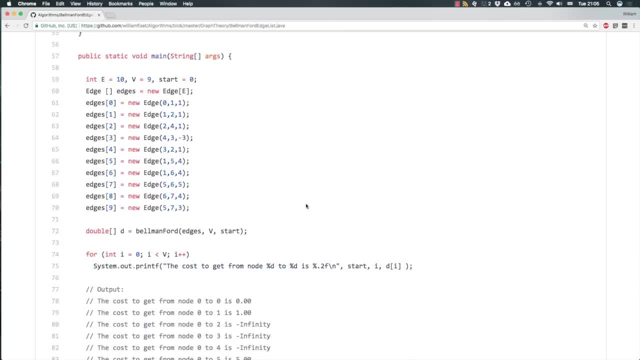 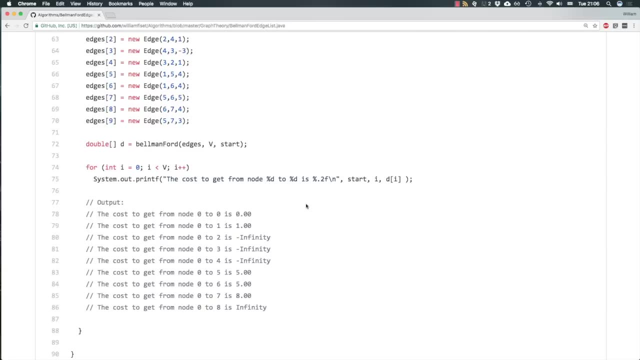 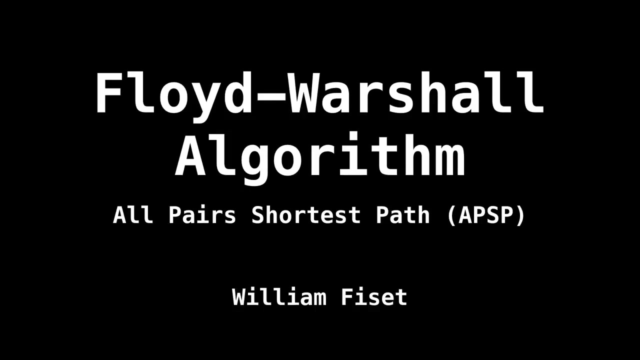 main method. it shows you how to actually create a graph, add some edges and then run Bellman Ford and find the distance from a starting node to all other nodes in the graph. And that is Bellman Ford, And today's topic is the Floyd Warshall. all pairs shortest. 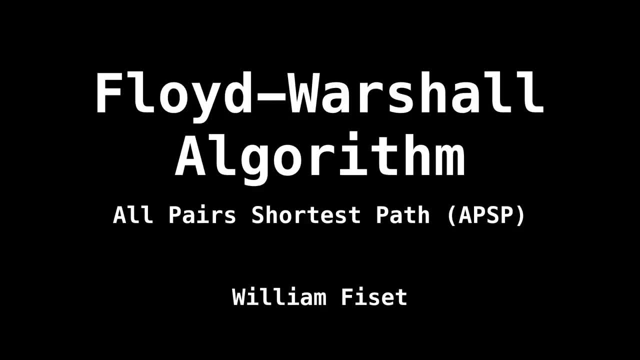 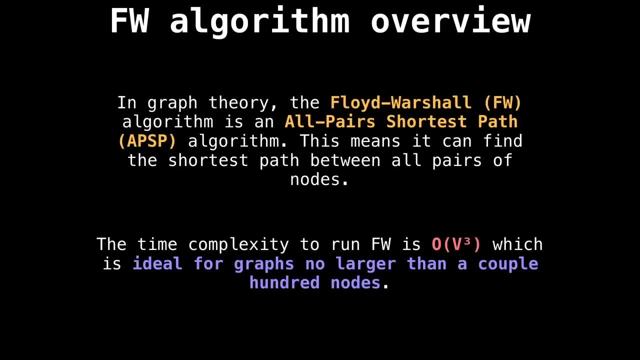 path algorithm. we will be covering how the algorithm works, how to reconstruct shortest path paths, the handling of negative cycles, followed by some code. So let's get started. In graph theory, the Ford Warshall algorithm is an all pairs shortest path algorithm. This means: 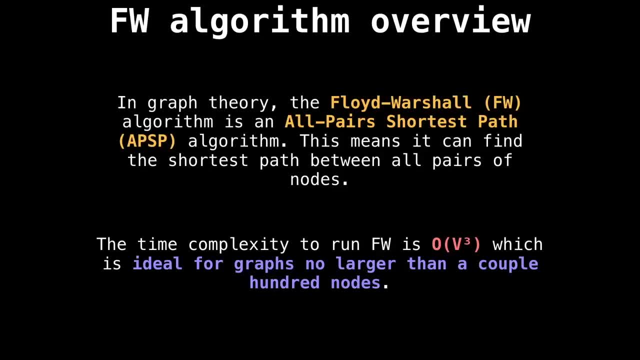 it can find the shortest path between all pairs of nodes. This is very important for many applications across several fields. The time complexity to run for the Warshall is big. O of v cubed, or v being the number of vertices in a graph. 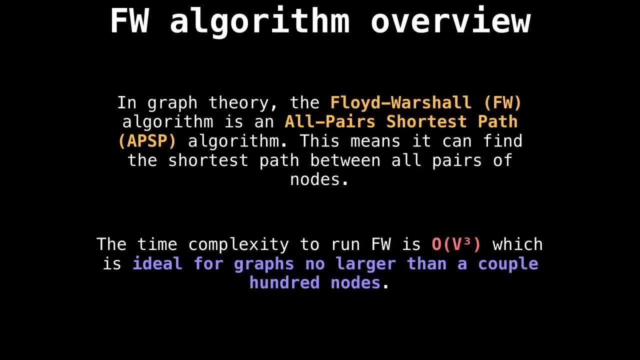 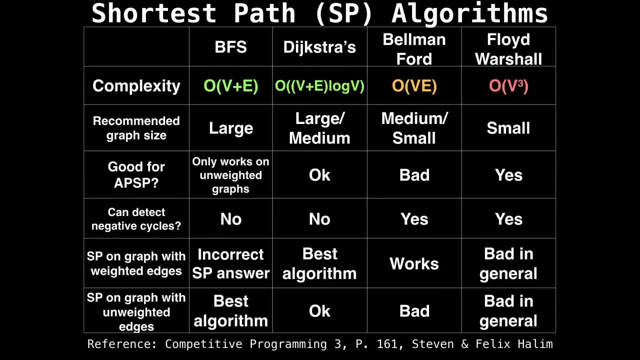 This makes the algorithm ideal for graphs with no more than a couple 100 nodes. Before we dive too deeply into the Ford Warshall algorithm, I want to address when you should and should not use this algorithm. This table gives information about various types of graphs and or constraints. 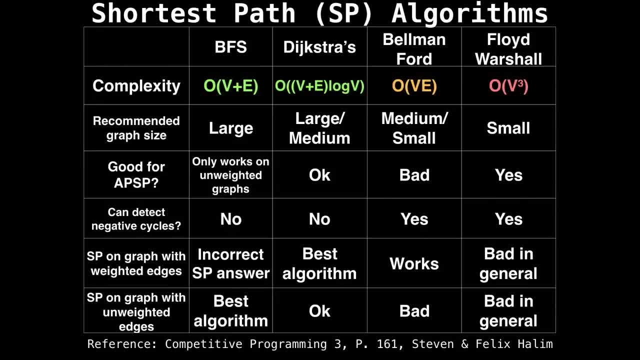 in the leftmost column and the performance or outcome of common shortest path algorithms. For example, you can see in the second row we have the shortest path algorithm and the second row that a breadth first search and Dykstra's can handle large graphs with lots. 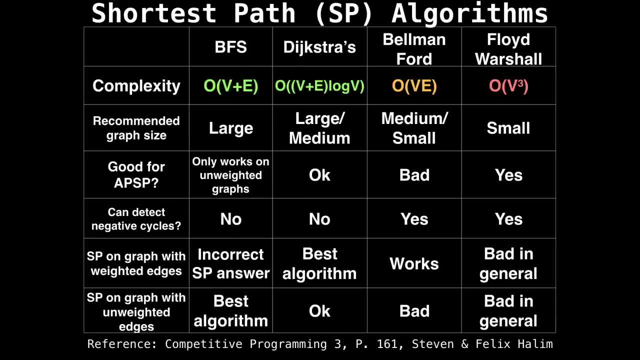 of nodes, while Bellman Ford and Ford Warshall not so much. I suggest you pause the video and really go through this table and make sure you understand why each cell has a value it does. What I want to highlight is the rightmost column, since we're talking about the Floyd. 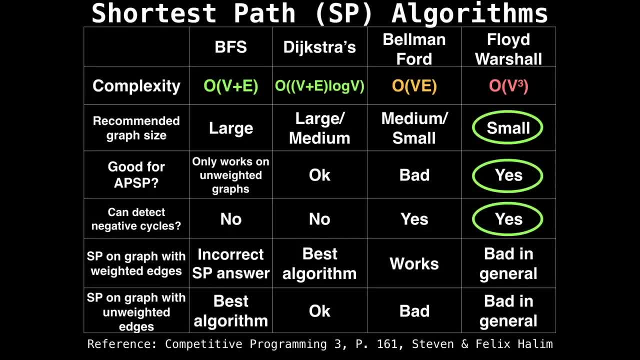 Warshall algorithm. the Ford Warshall algorithm really shines in three places, And those are on small graphs: solving the all pair shortest path problem and detecting negative cycles. You can use the algorithm for other tasks, but there are likely better algorithms out there. With Ford Warshall, the optimal way to represent our graph is with a two dimensional. 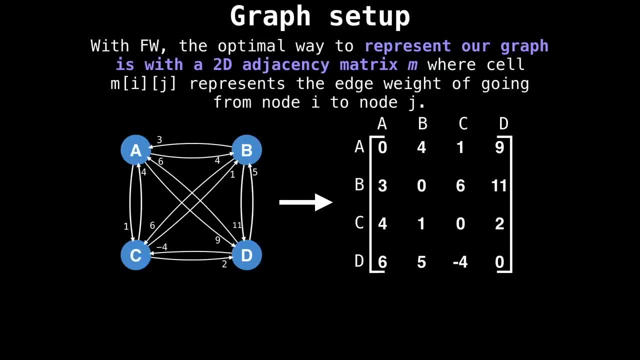 but there are likely better algorithms out there. With Floyd Warshall, the optimal way to represent our graph is with a two dimensional adjacency matrix, which I will denote as the letter m. The cell m, i, j represents the edge weight of going from node i to node j. So 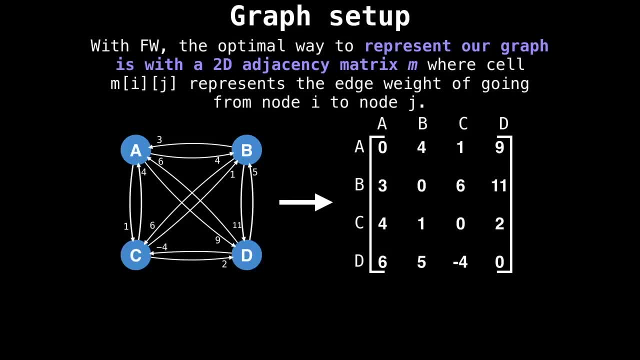 in the image below. I transformed the graph with nodes a, b, c and d into an adjacency matrix on the right. An important note I should mention is that I assume that the distance from a node to itself is zero, which is usually the case. This is why the diagonal 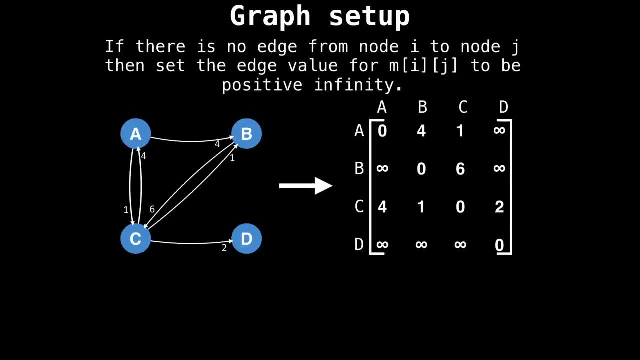 has all zero values. When there is no edge between nodes I and j, set the value in the matrix from im IJ to be positive infinity. this indicates that two nodes are not directly connected to each other. A very important note to make is that if your programming language 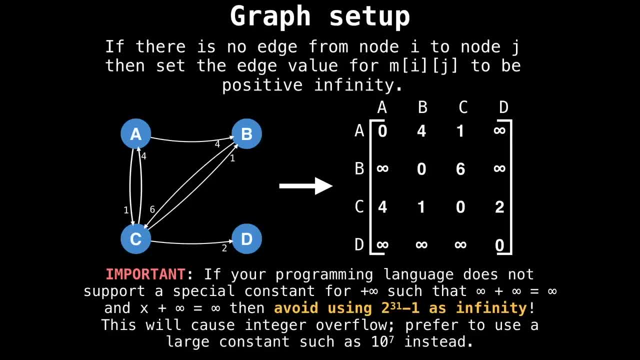 doesn't support a special constant in its standard library for positive infinity, such that plus infinity equals infinity and infinity plus x equals infinity, then you should avoid using two to the power of 31 minus one as infinity. If you do so, then you will likely. 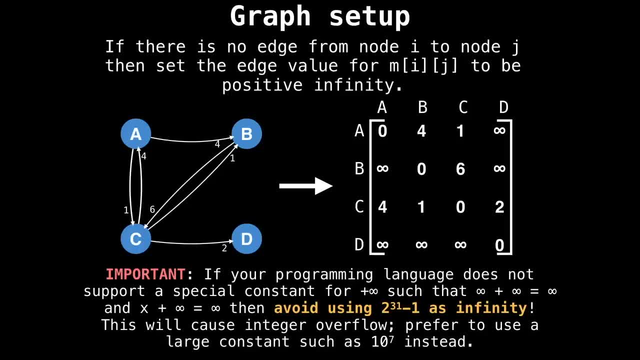 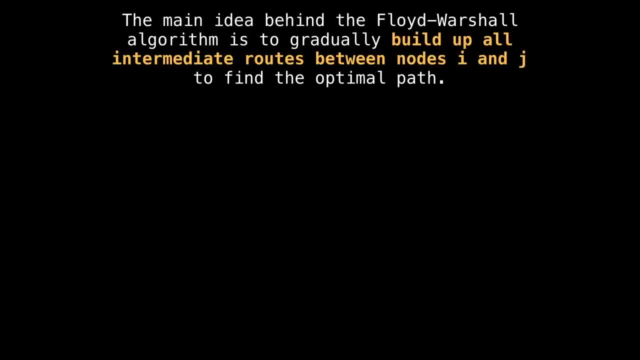 get integer overflow, simply use a large constant instead. as we will see, the main idea behind the Florida Warshall algorithm builds off the notion that you want to compute all intermediate routes between two nodes to find the optimal path. Suppose our adjacency matrix tells us. 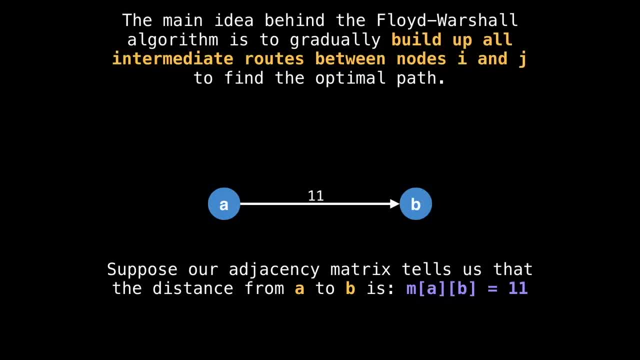 the distance from a node A to a node B is 11.. Now suppose there exists a third node, C. if the distance from A to C and then C to B is less than the distance from A to B, then it is better to go through node C. Again, the goal is to consider all. 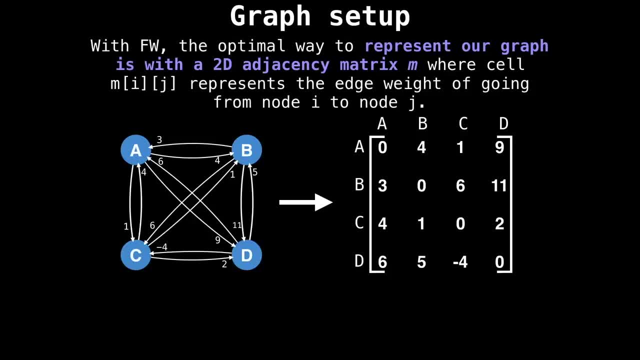 adjacency matrix, which I will denote as the letter m. the cell m, i, j represents the edge weight of going from node i to node j. So in the image below I transform the graph with nodes A, B, C and D into an adjacency. 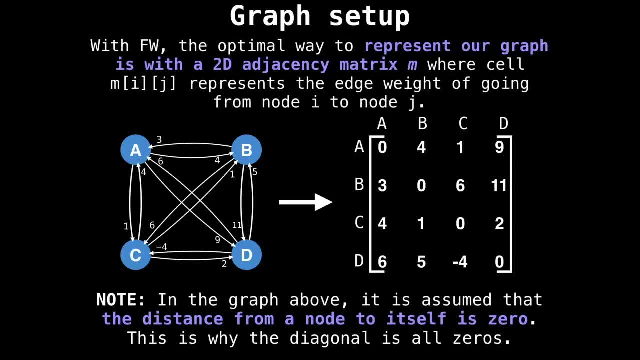 matrix on the right. An important note I should mention is that I assume that the distance from a node to itself is zero, which is usually the case. This is why the diagonal has all zero values When there is no edge between nodes i and j. 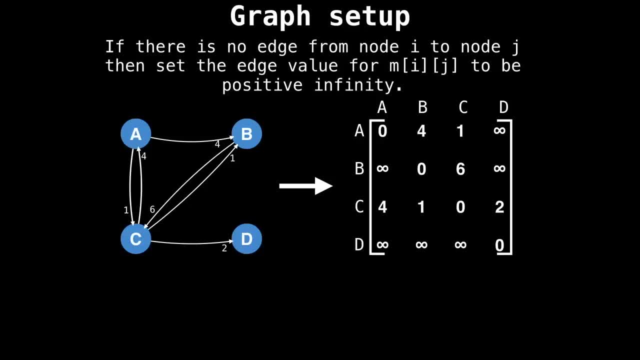 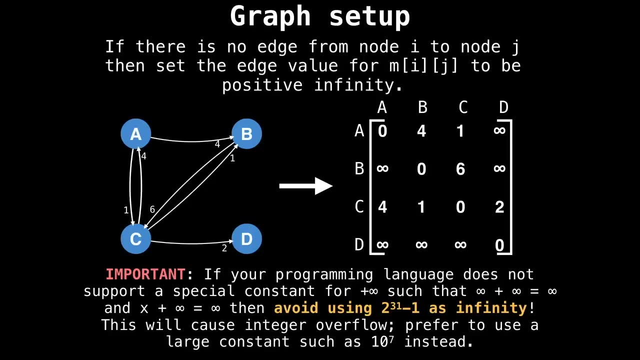 Set the value in the matrix from m i j to be positive infinity. This indicates that two nodes are not directly connected to each other. A very important note to make is that if your programming language doesn't support a special constant in its standard library for positive infinity, such that infinity plus infinity equals infinity and infinity, 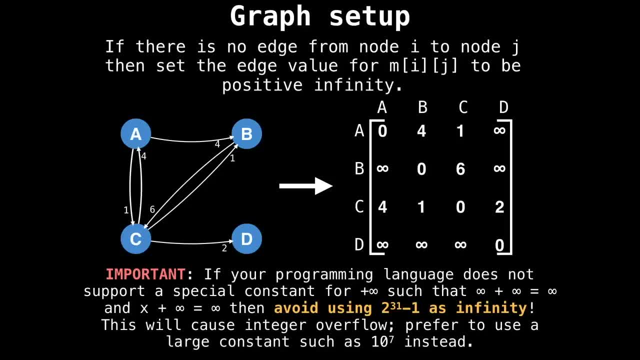 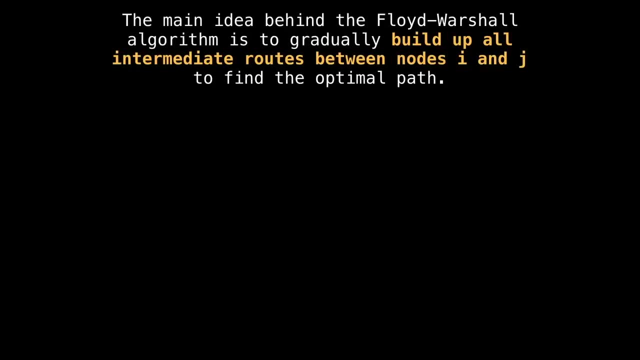 plus x equals infinity, then you should avoid using two to the power of 31.. minus one as infinity. If you do so, then you will likely get integer overflow. simply use a large constant instead, As we will see, the main idea behind the Florida Warshall. 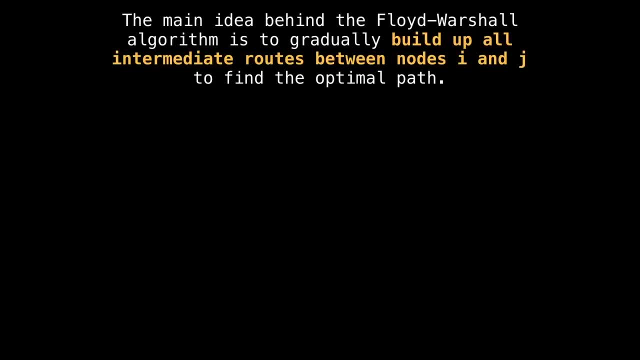 algorithm builds off the notion that you want to compute all intermediate routes between two nodes to find the optimal path. Suppose our adjacency matrix tells us the distance from a node a to a node B is 11. Now suppose there exists a third node, C. if the distance from A to C and then C to 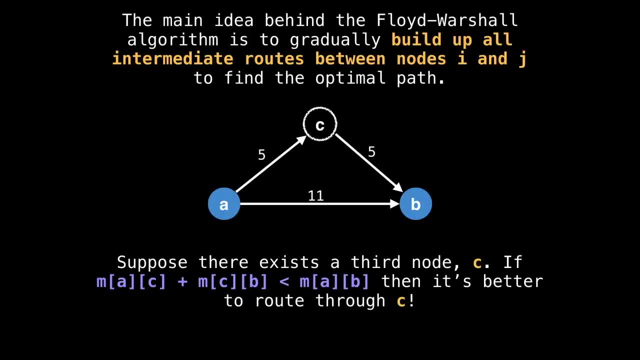 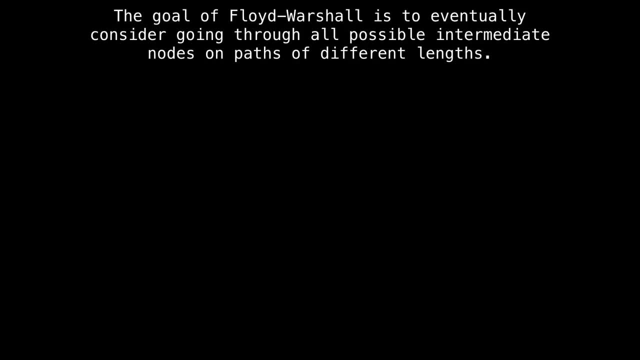 B is less than the distance from A to B, then it is better to go through node C. Again, the goal is to consider all possible intermediate paths between triplets of nodes. This means we can have something like this: where the optimal path from A to B is first, we can. 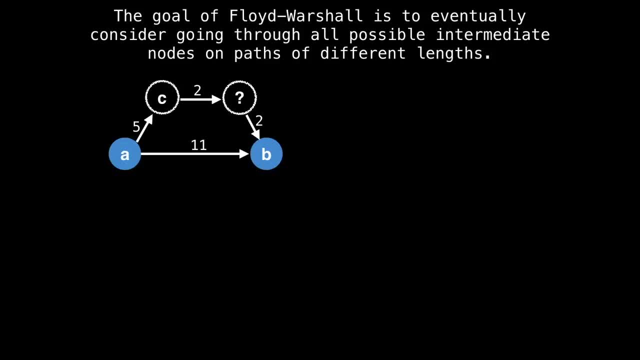 go to C, then go from C to B, But in the process we actually route through another node, which I labeled with a question mark, because we've already computed the optimal path from C to B and I know that it involves an intermediate node. Similarly, we can get 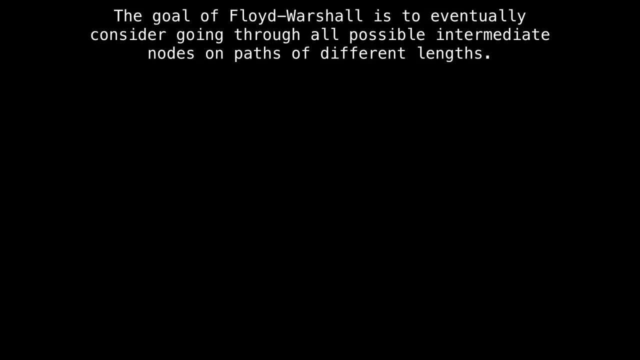 C to B is less than the distance from A to B, then it is better to go through node C. Again, the goal is to consider all possible intermediate paths between triplets of nodes. This means we can have something like this, where the optimal path from A to B is first going to see, then going from C. 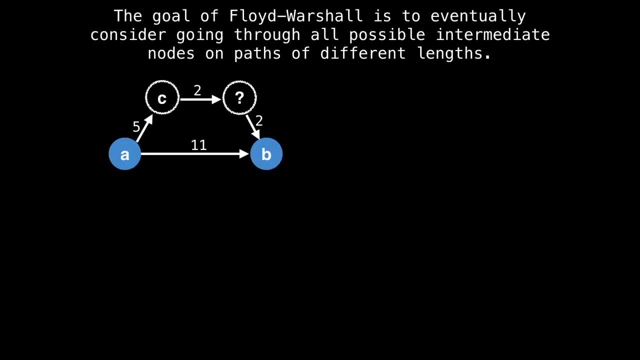 to B, But in the process we actually route through another node, which I labeled with a question mark, because we've already computed the optimal path from C to B And I know that it involves an intermediate node. Similarly, we can get longer paths between triplets of. 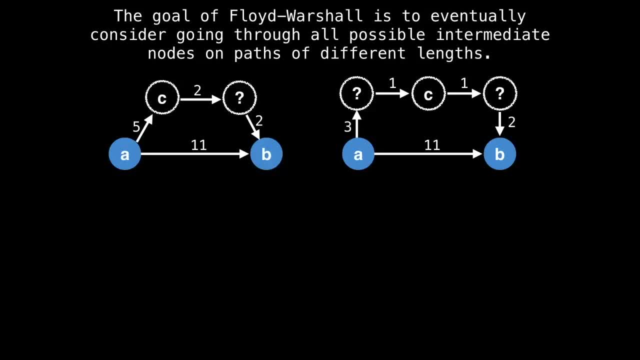 nodes. We can get longer paths with more intermediate nodes between A and C and C and B with a smaller cost. We are also not just limited to one intermediate node in between A and C and C and B. we can have several, like in the graph below. Now the question comes up: how do we? 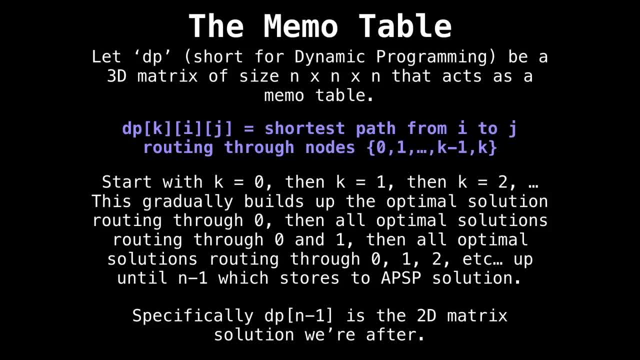 actually compute all intermediate paths? The answer is: we will use dynamic programming to cache previous optimal solutions. Let dp be a three dimensional matrix of size n by n by n, which acts as our memo table. we're going to say that the cell dp at k i j in our table gives us the shortest path. 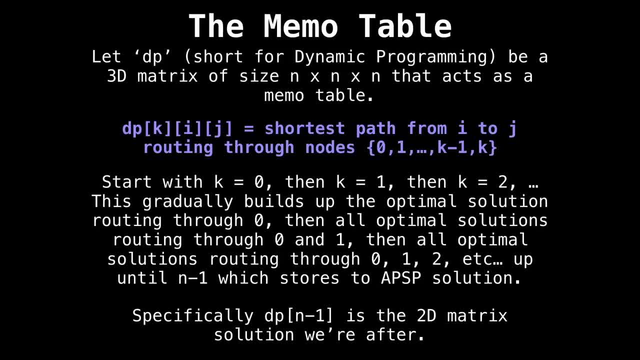 from node i to node j, routing through nodes zero, through k. What we'll do is start by computing: k equals zero, then k equals one, Then k equals two, and so on. This gradually builds up the optimal solution: routing through zero, then all optimal solutions routing through zero and one, then all optimal solutions routing. 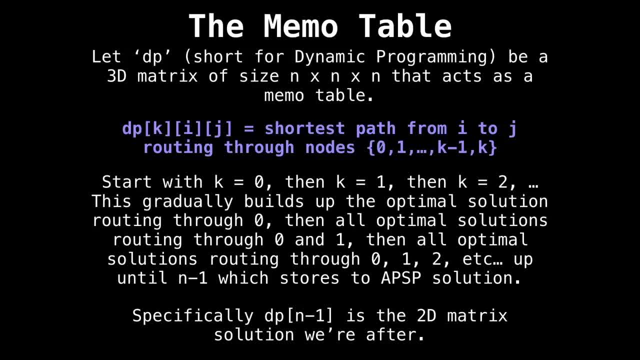 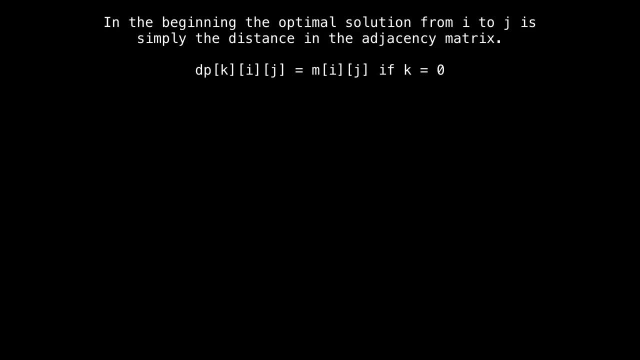 through zero, one and two and etc. Up until we covered all nodes, at which point we have solved the all pairs shortest path problem. Let's talk a bit more about how to populate the dp table. In the beginning, the optimal solution from: 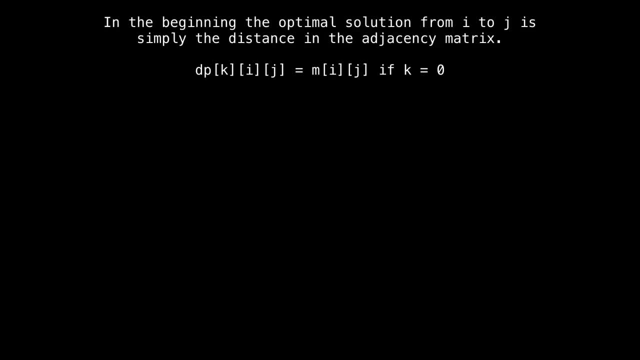 i to j Is simply the distance given to us in the adjacency matrix. So when k equals zero, dp of k i- j is equal to m i j, the value of the edge from i to j. Otherwise, in general, dp k i- j can be summed up with the following recurrence relation. I'm going to break it. 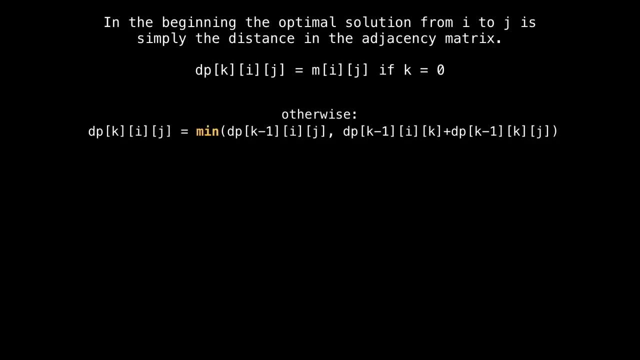 down so that we can understand all its components, Because this may look scary to some people. The left hand side of the recurrence simply says: reuse the best distance so far from i to j, routing through nodes zero to k minus one. it's important to note that the solution 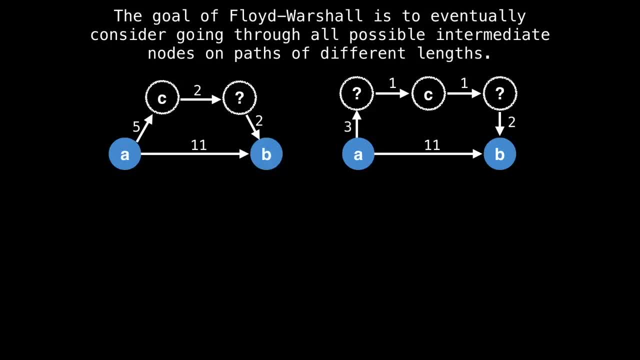 longer paths with more intermediate nodes, between A and C and C and B, with a smaller cost. We are also not just limited to one intermediate node, but we can also have a path that is smaller than the first intermediate node. So, for example, if we looked at the first 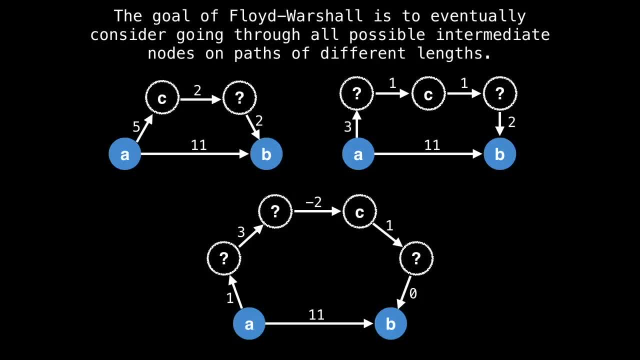 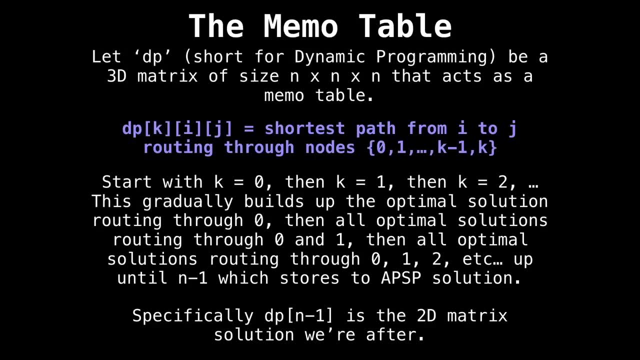 intermediate node in between A and C and C and B. we can have several like in the graph below. Now the question comes up: how do we actually compute all intermediate paths? The answer is: we will use dynamic programming to cache previous optimal solutions. Let dp. 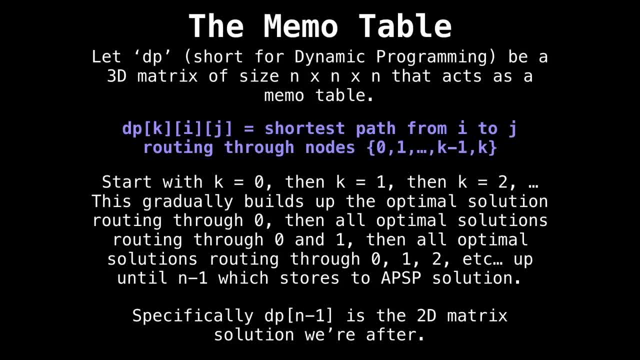 be a three dimensional matrix of size n by n by n, which acts as our memo table. we're going to say that the cell DP at K, i, j in our table gives us the shortest path from node i to node j, routing through nodes zero, through k. what we'll do is start by computing. 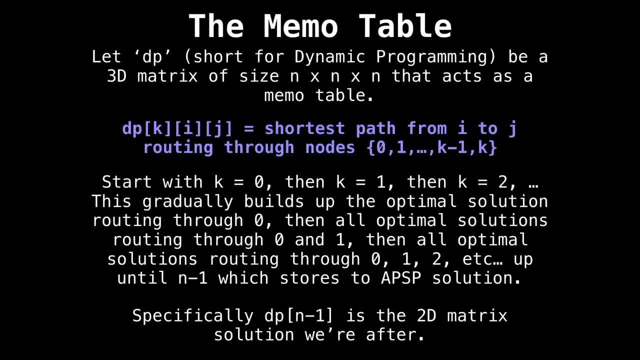 k equals zero, then k equals one, then k equals two, and so on. This gradually builds up the optimal solution routing through zero, then all optimal solutions routing through zero and one, then all optimal solutions relating through zero, one and two, and etc. Up until we covered all nodes, at which point we have 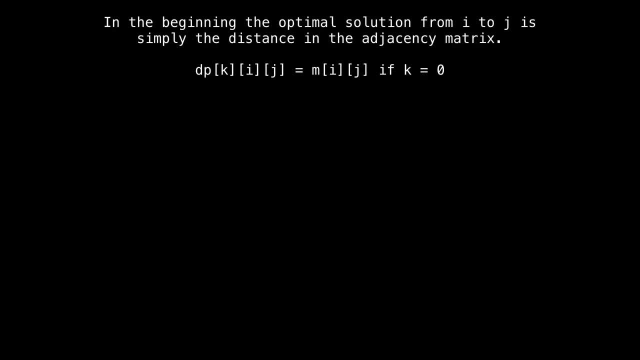 solved the all pairs shortest path problem. Let's talk a bit more about how to populate the DP table. In the beginning, the optimal solution from i to j is simply the distance given to us in the adjacency matrix. So when k equals zero, dp of K ij is equal to m ij. 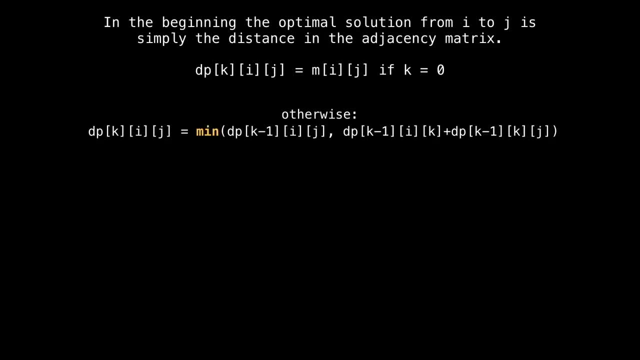 the value of the edge from i to j. Otherwise, in general, dp, K, i, j can be summed up with the following recurrence relation. I'm going to break it down so that we can understand all its components, Because this may look scary to some people. 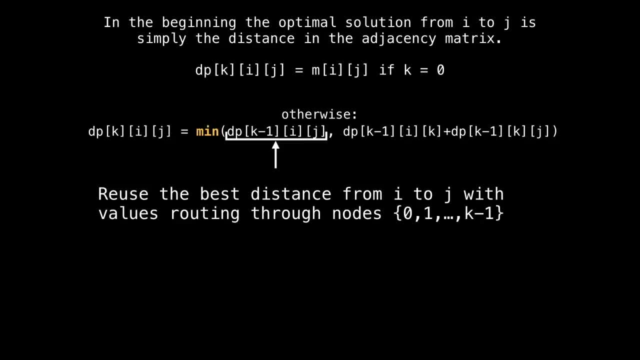 The left hand side. Next, let's look at the right hand side and make sure that we have hand side of the recurrence simply says: reuse the best distance so far from i to j routing through nodes zero to k minus one. It's important to note that the solution using nodes zero. 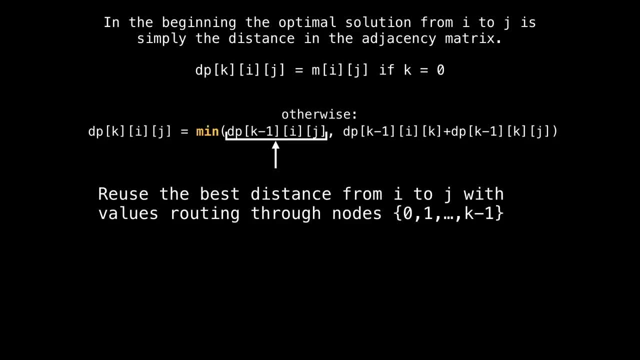 using nodes zero to k minus one is a partial solution. it is not the whole picture. This is part of the dynamic programming aspect of the Floyd Warshall algorithm. The right hand side of the recurrence finds the best distance from it. The right hand side of the recurrence finds the best distance from it. So in this case, 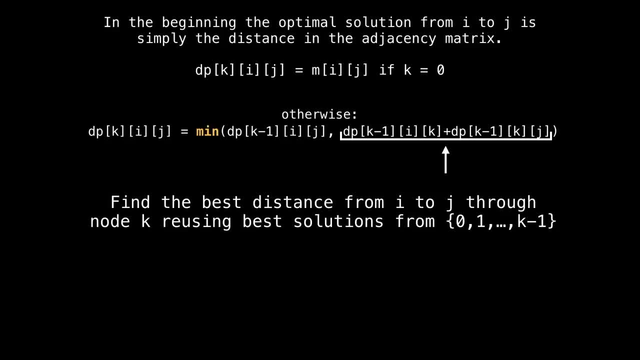 i j is equal to m i j. The left hand side of the recurrence simply says: reuse the best to j, but routing through node k reusing the best solutions from zero to k minus one. If we analyze the right side of the min function in English, it basically says: go from i to 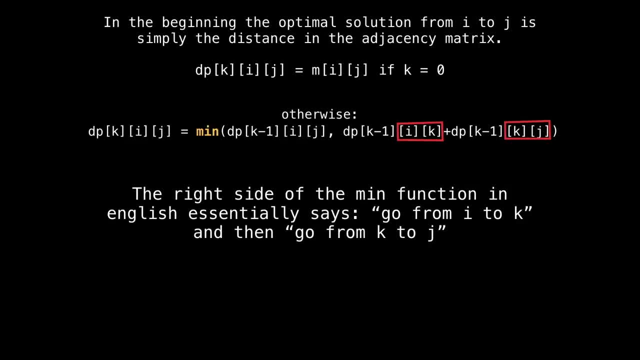 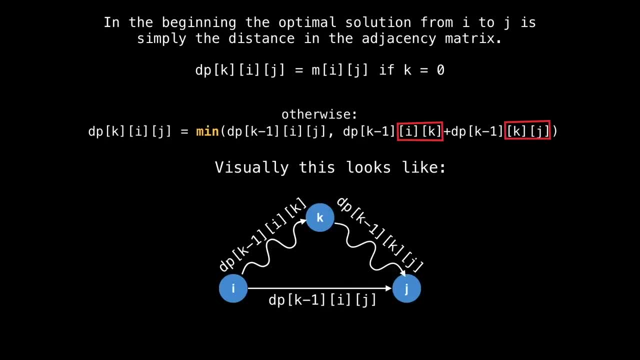 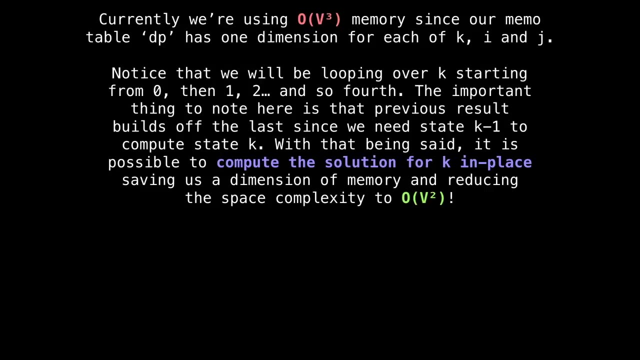 k, then go from k to j. Visually, this is what it looks like. You start at I, route through some nodes, get to k and then from k route back to j. Currently, our algorithm uses big O of v cubed memory, Since our memo table dp has one dimension for each of k, i and 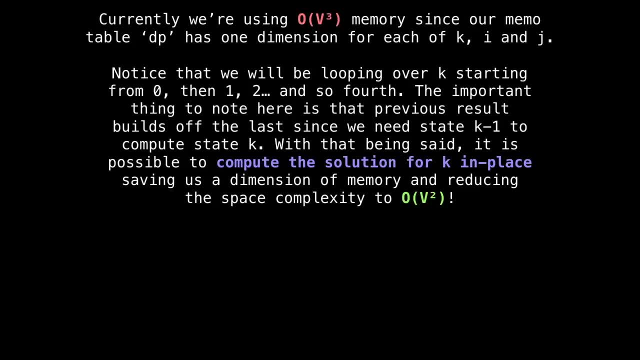 j. This isn't particularly great. Notice that we will be looping over k, starting from zero, then one, then two and so forth. The important thing to note here is that probably the most important thing to note here is that we're going to be looping over. 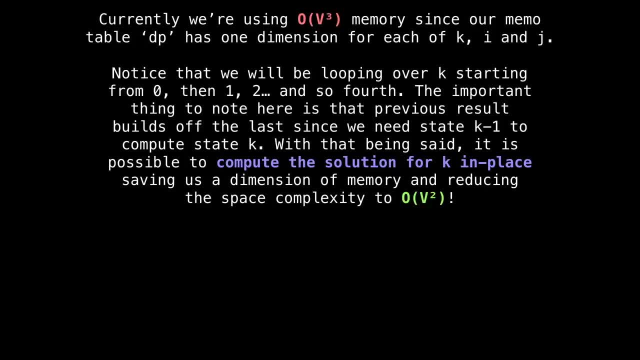 k starting from zero, then one, then two and so forth. The important thing to note here is that. probably the most important thing to note here is that probably previous results build off the last, since we need the state of k minus one to compute state k. That 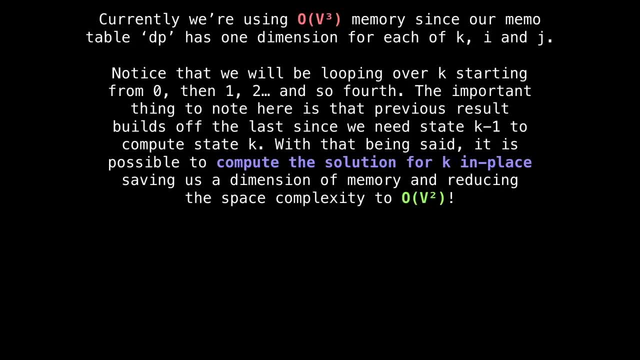 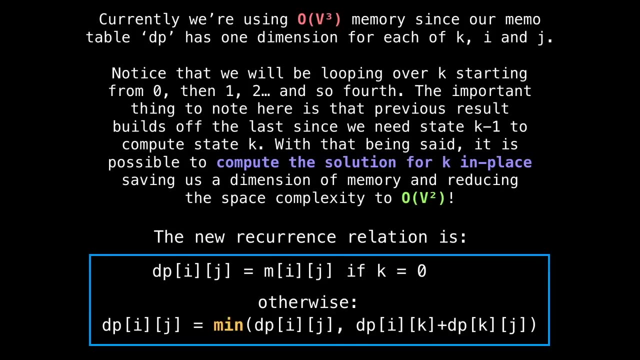 being said, it is possible to compute the solution for k in place, saving us a dimension of memory and reducing the space complexity to big O of v squared. Now we have a new recurrence relation which no longer involves the k dimension. This has been replaced by the fact that the 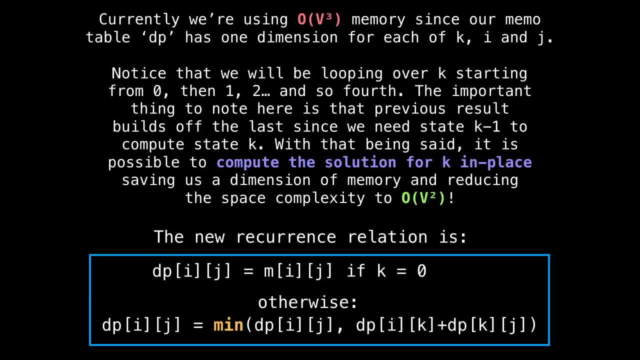 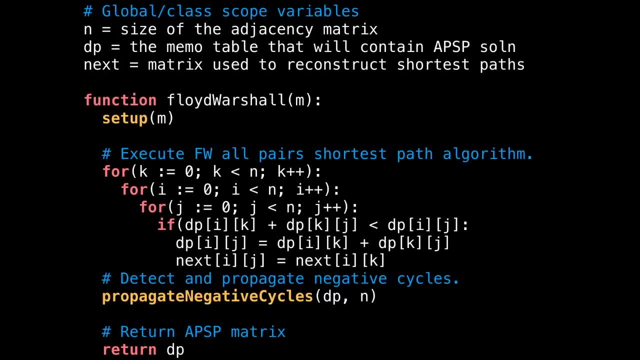 that we're computing the k plus one solution in place inside our matrix. Okay, that's all the theory we need. For now, let's get our hands dirty and look at some pseudocode. Below is the function that actually solves the Florida Warshall algorithm, or rather executes the 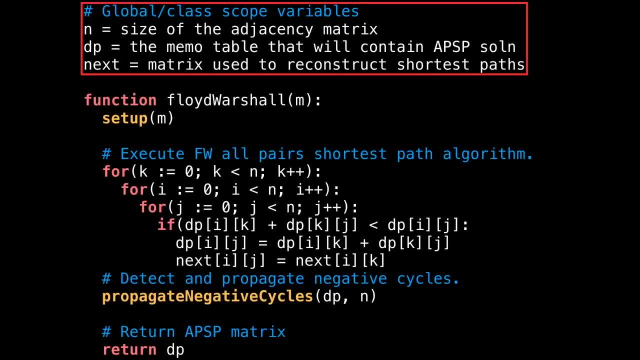 Florida Warshall algorithm. But before we get into that, let's look at some of the variables I have defined in the global or class scope which I will be using throughout these functions. The first variable is the number of nodes in our graph. then is the 2d memo table that 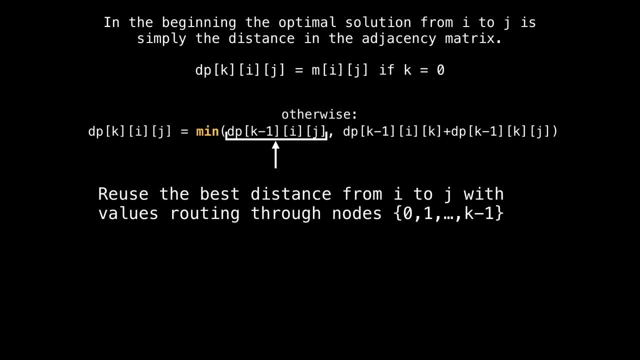 to k minus one is a partial solution. It is not the whole picture. This is part of the dynamic programming aspect of the Floyd Warshall algorithm. The right hand side of the recurrence finds the best distance from i to j, but routing through node k, reusing the best solutions. 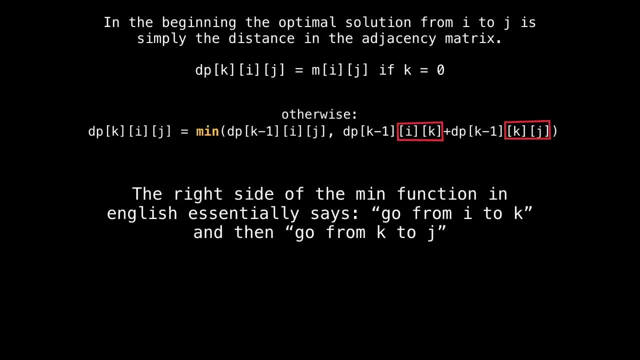 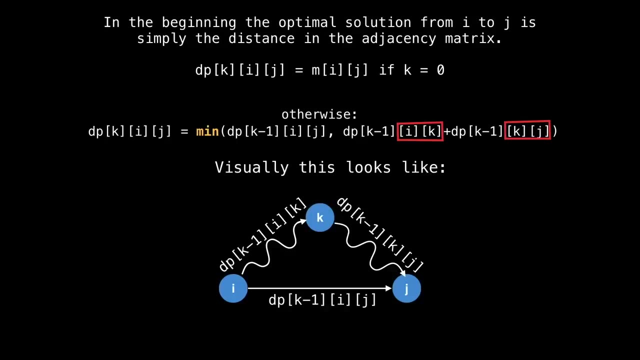 from zero to k minus one. If we analyze the right side of the min function in English it basically says: go from itk, then go from k to j. Visually this is what it looks like You start at. I wrap through some nodes, get to k and then from k route back to j And 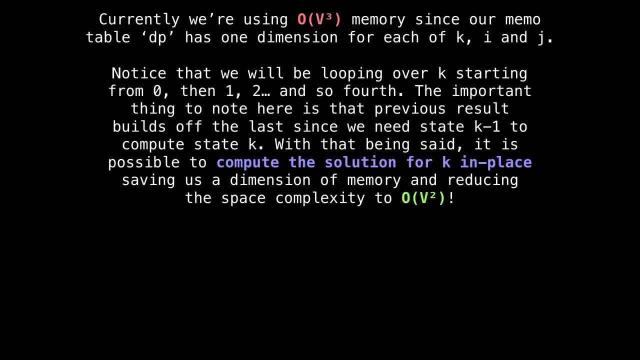 Currently, our algorithm uses big O of v cubed memory. Since our memo table dp has one dimension for each of k, i and j, This isn't particularly great. Notice that we will be looping over k starting from zero, then one, then two and so forth. The important thing to note. 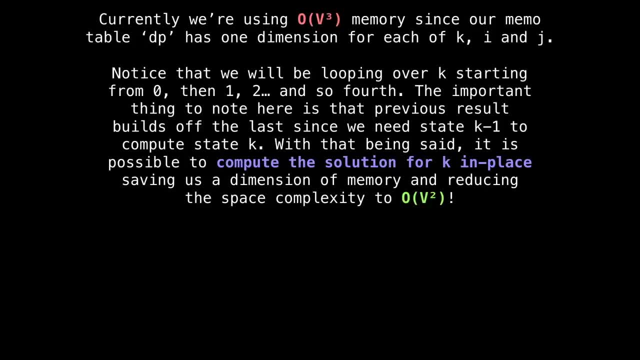 here is that previous results build off the last, since we need the state of k minus one to compute state k. That being said, it is possible to compute the solution for k in place, saving us a dimension of memory and reducing the space complexity to big O of 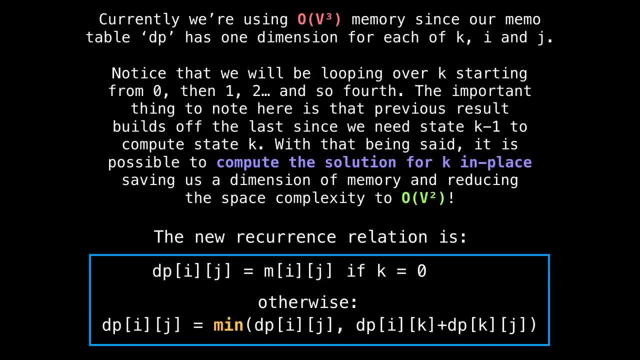 v squared. Now we have a new recurrence relation which no longer involves the k dimension. This has been used in the previous example. we can compute the solution for k in place. This has been replaced by the fact that we're computing the k plus one solution in place. 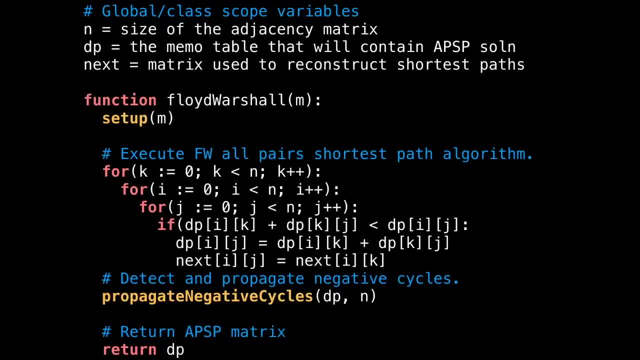 inside our matrix. Okay, that's all the theory we need. for now, let's get our hands dirty and look at some pseudocode. Below is the function that actually solves the Florida Warshall algorithm, or rather executes the Florida Warshall algorithm. But before we, 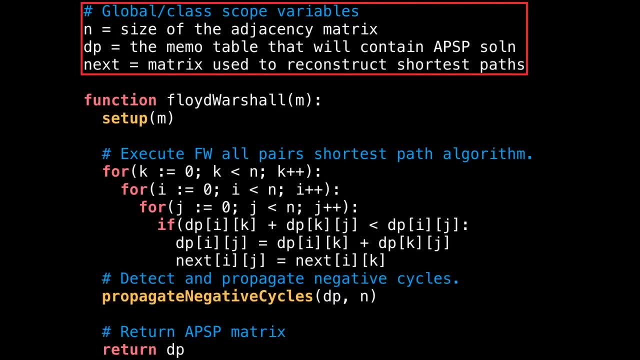 get into that. let's look at some of the variables I have defined in the global or class scope, which I will be using throughout these functions. The first variable is the number of nodes in our graph. then is the 2d memo table that will contain our all pair. 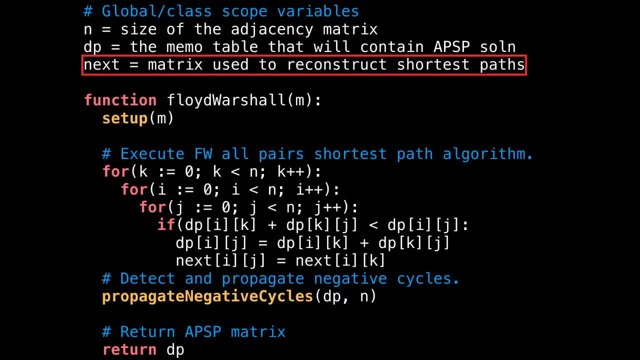 will contain our all pair shortest path solution. Last is the next 2d table that we will use to reconstruct our shortest paths. Now, moving on to the Floyd Warshall function, you see that it takes one parameter. This is the table that we have defined in the global or class scope, which I will be 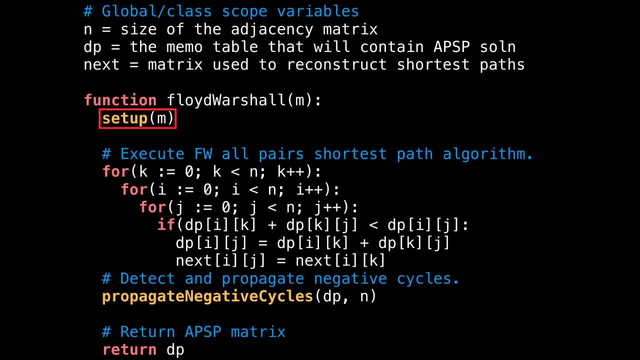 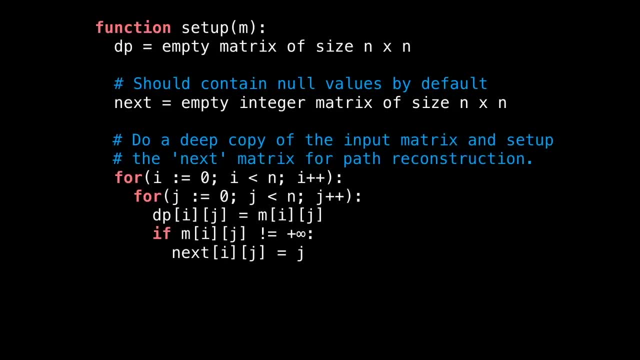 using in the global or class scope. Next is the 2d adjacency matrix representing our graph. The first thing I do in the method is called the setup function, So let's take a look at that real quick. So here we are, inside the setup function. The first thing I do is I: 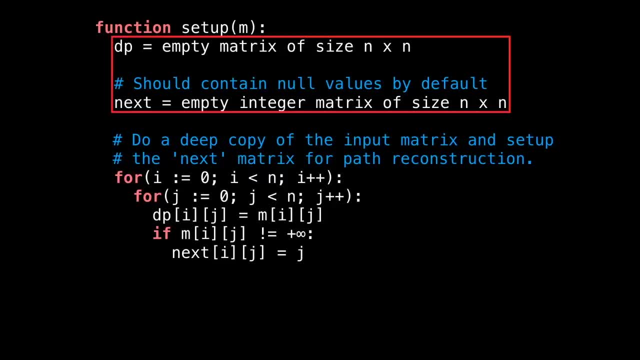 allocate memory for our tables. the DP matrix should have the same type as the input adjacency matrix. What I mean by this is, if your edges in your input matrix are represented as real numbers, then your DP matrix should also hold real numbers. The next matrix will contain indexes of nodes to reconstruct the shortest paths found from. 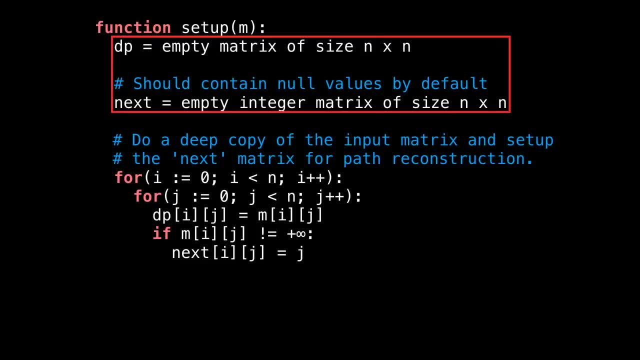 running the Floyd Warshall algorithm, it is important that initially this matrix be populated with null values Inside the for loops. all I do is copy the input matrix into the DP matrix. Think of this as the base case, or rather the k equals zero case For the next. 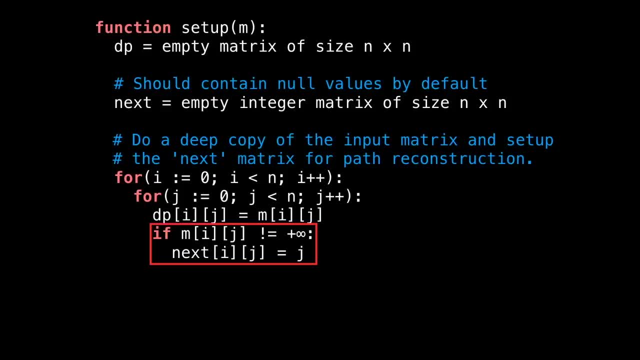 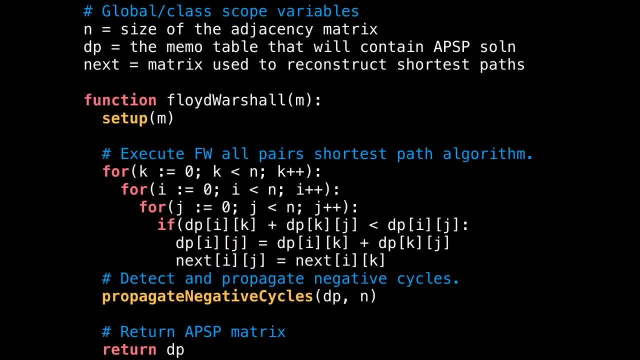 matrix. if the distance from i to j is not positive infinity, then the next node you want to go to from node i is node j by default. Now we're back inside the Floyd to Warshall function In here after the setup loop over k on the exterior loop. it's important that 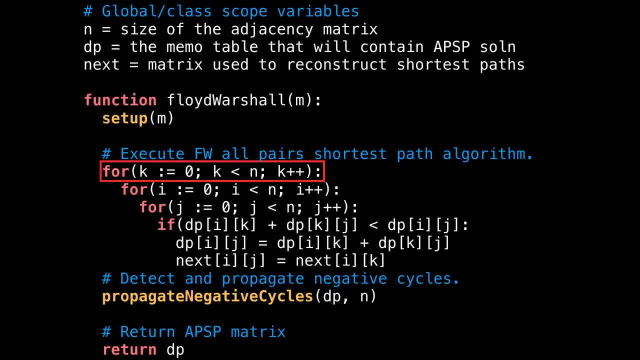 k is on the exterior loop, Since we want to gradually build up the best solutions for k equals zero, then k equals one, then k equals two, and so on, Followed by this loop over all pairs of nodes i and j inside the main body actually tests. 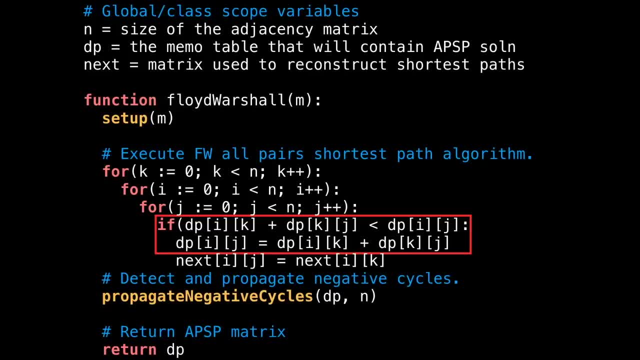 for our condition to improve the shortest path from i to j going through k and update the value at dp i j if there's a better route through K. Also inside here, update the next array at ij to point to the next index at next ik. 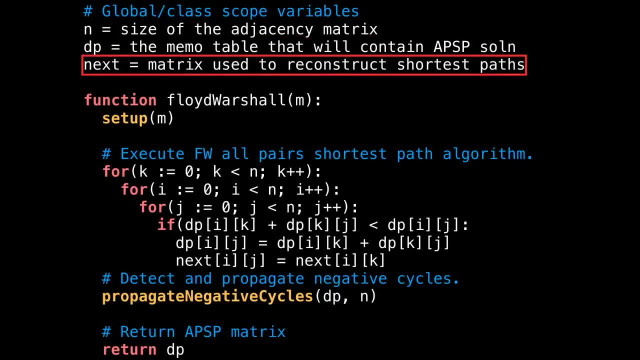 shortest path solution. Last is the next 2d table that we will use to reconstruct our shortest paths. Now, moving on to the Floyd Warshall function, you see that it takes one parameter. This is the 2d adjacency matrix, representing the number of nodes in our graph. 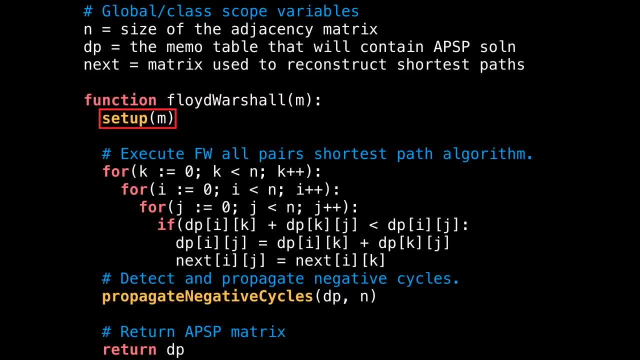 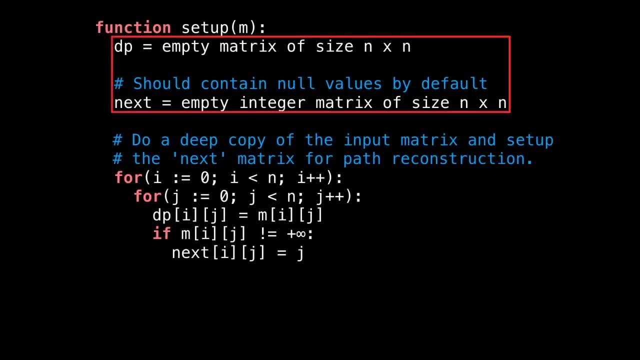 The first thing I do in the method is call the setup function. So let's take a look at that real quick. So here we are inside the setup function. The first thing I do is I allocate memory for our tables. the DP matrix should have the same type as the input adjacency. 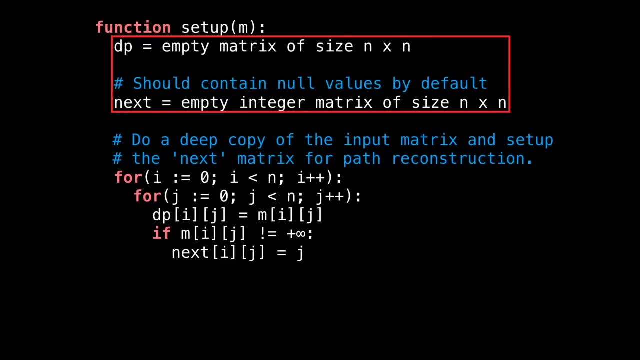 matrix. What I mean by this is if your edges in your input matrix are represented as real numbers, then your DP matrix should also hold real numbers. The next matrix should also hold real numbers. The next matrix should also hold real numbers. The next matrix will contain indexes of nodes to reconstruct the shortest paths found from. 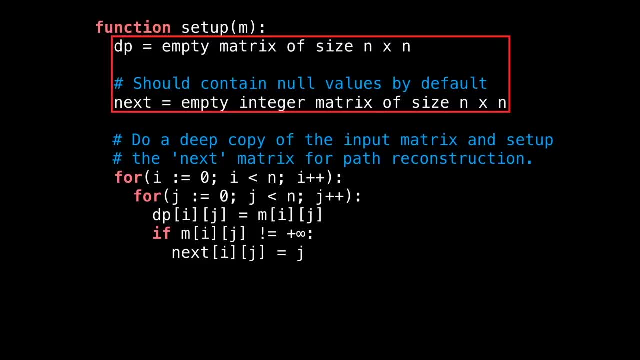 running the Floyd Warshall algorithm, It is important that initially this matrix be populated with null values Inside the for loops. all I do is copy the input matrix into the DP matrix. Think of this as the base case, or rather the k equals zero case For the next. 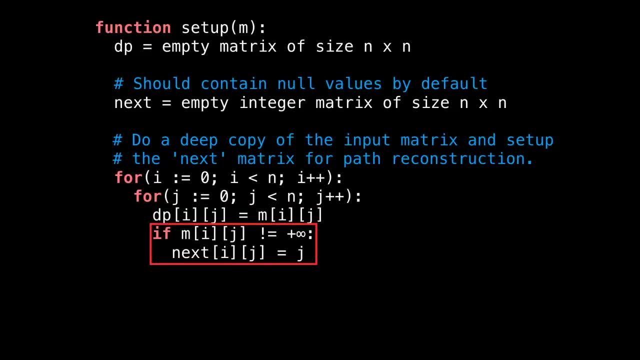 matrix. if the distance from i to j is 0, then the input matrix should be 0.. The input matrix should be 0.. If the distance from i to j is not positive infinity, then the next node you want to go to from node i is node j by default. Now we're back inside the Floyd. 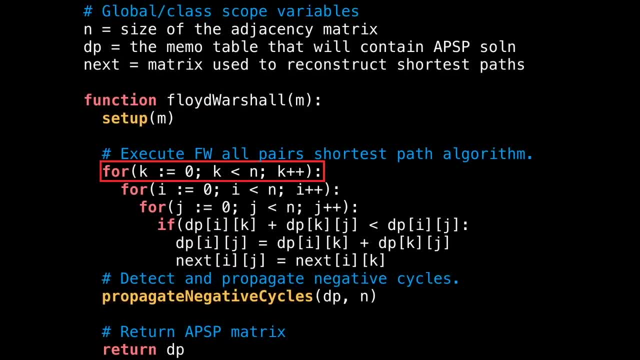 Warshall function In here after the setup loop over k on the exterior loop. it's important that k is on the exterior loop since we want to gradually build up the best solutions for k equals zero, then k equals one, then k equals two, and so on. 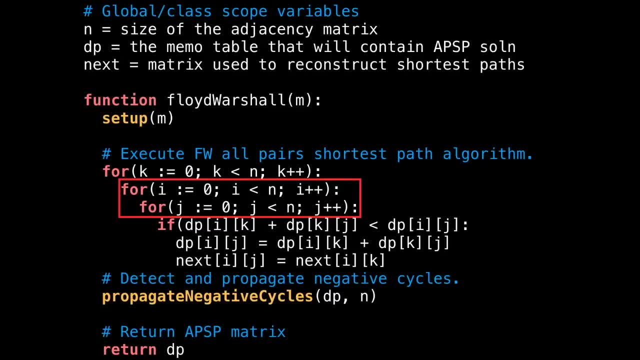 Followed by this loop over all pairs of nodes i and j Inside the main body. actually test for our condition to improve the shortest path from i to j going through k and update the value at dpi j if there's a better route through k, Also inside here, update the next. 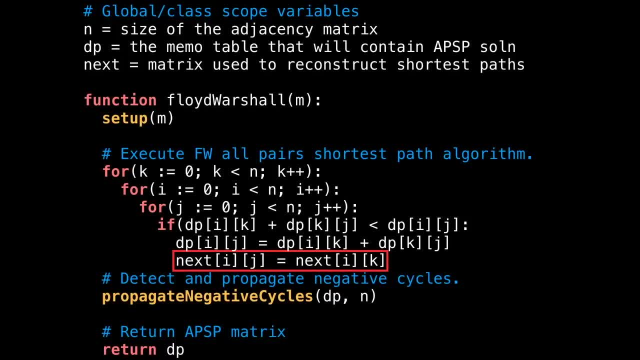 array at I j to point to the next index at next I k. The last thing I want to do is to detect and propagate negative cycles. This is an optional step if you know that negative cycles will not manifest themselves within your graph, Although I still recommend. 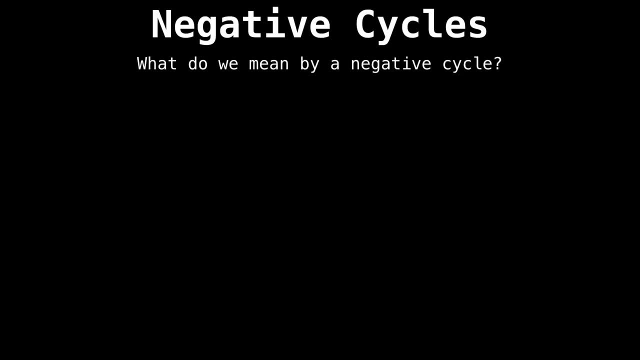 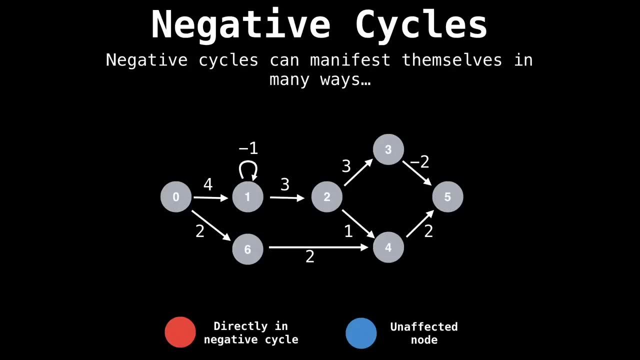 you keep this function around. But before we get too far, I want to discuss negative cycles and what they entail, because it isn't entirely obvious. So consider the following graph. There are basically two types of node to consider here: nodes directly involved in negative cycles and nodes unaffected by negative cycles. This red node is the cause. 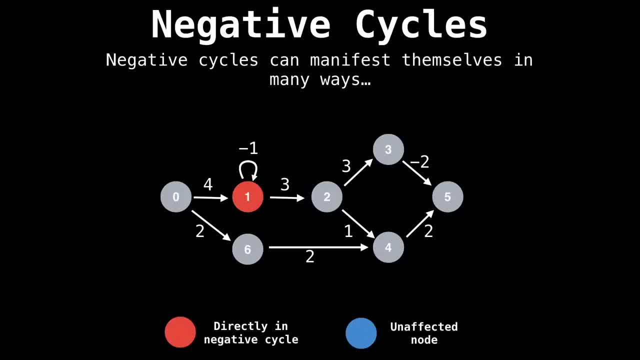 of a negative cycle because it can endlessly loop on itself and obtain smaller and smaller costs. While these blue nodes are not directly in a negative cycle, This, however, doesn't mean they're not necessarily safe from negative cycles, as we will see. 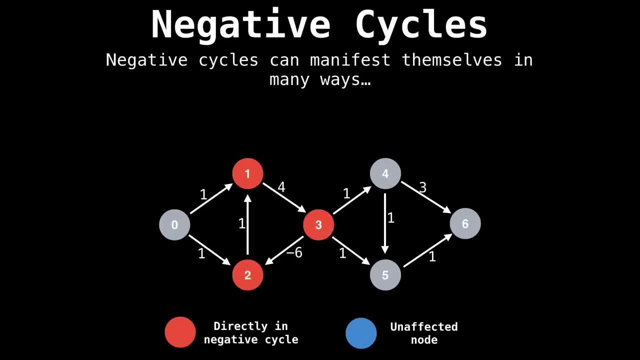 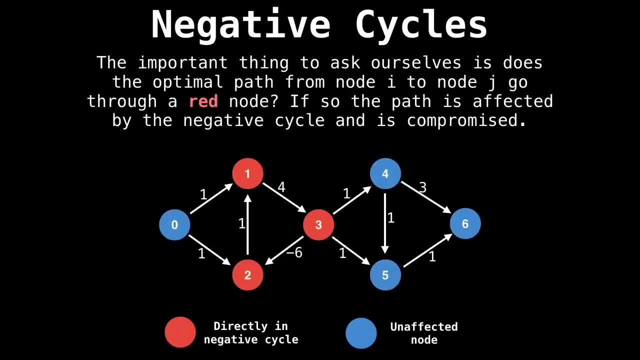 Negative cycles can also manifest themselves as groups of nodes working together, like the following. So an important thing to ask ourselves is: does the optimal path from node i to node j go through a red node? If so, the path is affected by the negative cycle. 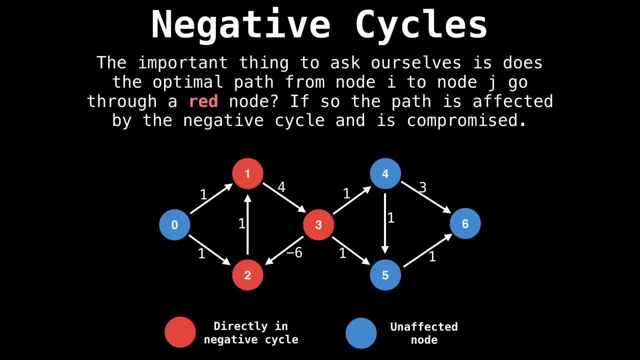 and is compromised. For example, the shortest path from zero to five is negative infinity, Because I can go from zero to node two and indefinitely loop in the negative cycle consisting of nodes 12 and three, obtaining better and better costs before eventually going to five. 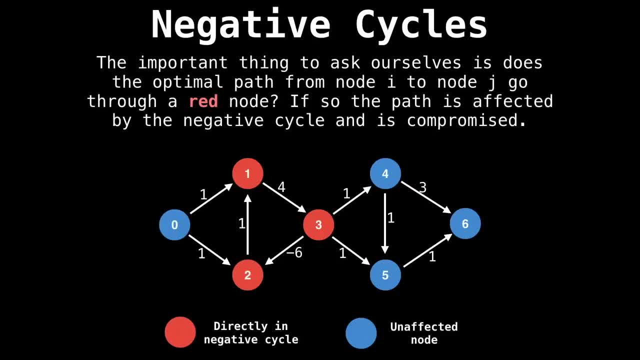 This is a consequence of traversing a red node on the way to five. Some shortest paths, however, avoid red nodes altogether. Consider the shortest path from four to six. This doesn't involve any red nodes. However, the shortest path from zero to five is negative infinity. 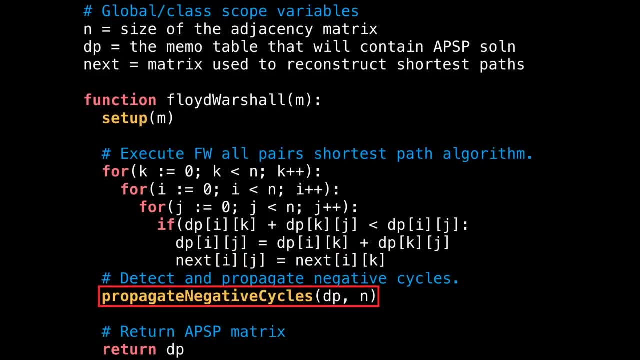 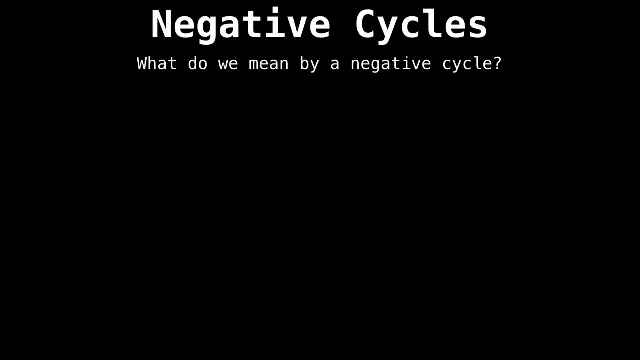 The last thing I want to do is to detect and propagate negative cycles. This is an optional step if you know that negative cycles will not manifest themselves within your graph, Although I still recommend you keep this function around. But before we get too far, I want to discuss. 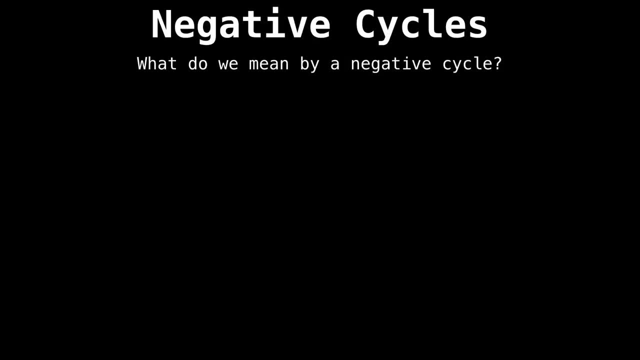 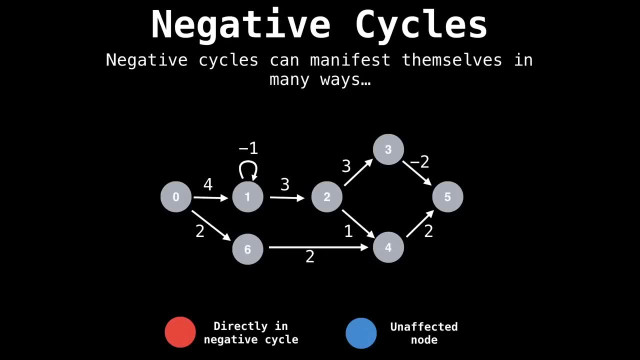 negative cycles and what they entail, because it isn't entirely obvious. So consider the following graph. There are basically two types of node to consider here: nodes directly involved in negative cycles and nodes unaffected by negative cycles. This red node is the cause of a negative cycle because it can endlessly loop on itself and obtain smaller and smaller. 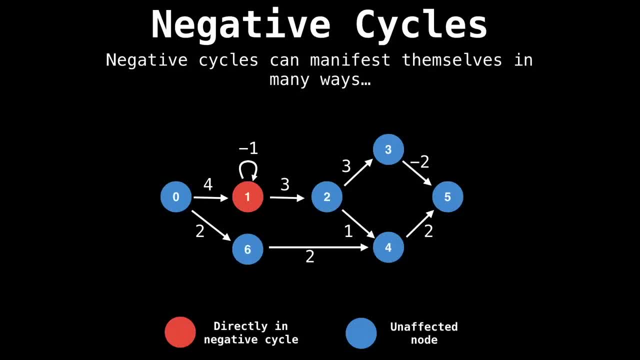 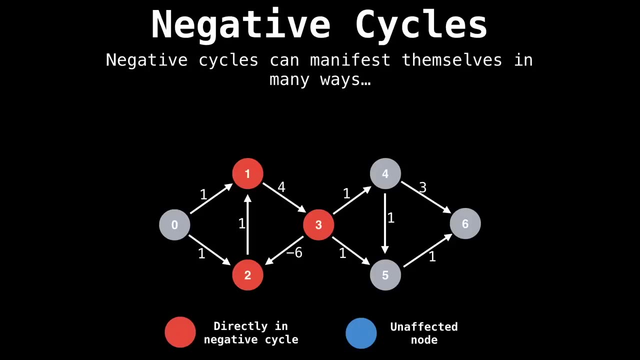 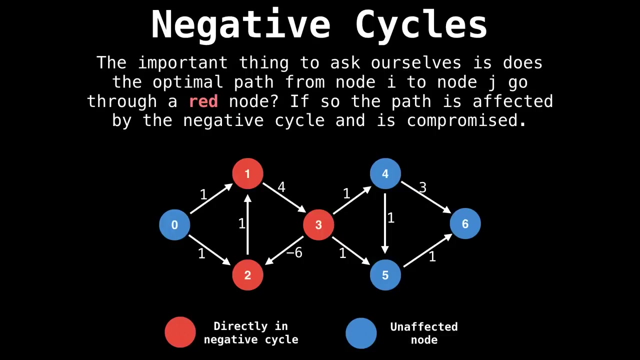 costs. While these blue nodes are not directly in a negative cycle, This, however, doesn't mean they're not necessarily safe from negative cycles. As we will see, negative cycles can also manifest themselves as groups of nodes working together, like the following. So an important thing to ask ourselves is: does the optimal path? 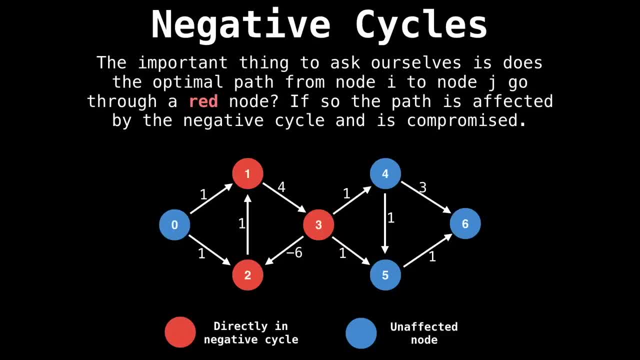 from node i to node j go through a red node. If so, the path is affected by the negative cycle and is compromised. For example, the shortest path from zero to five is negative. If so, the path is affected by the negative infinity, because I can go from zero to node. 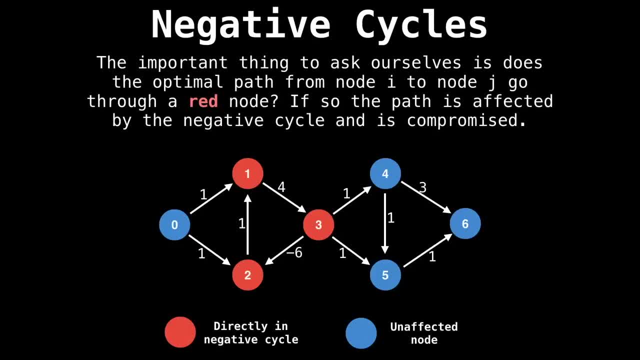 two and indefinitely loop in the negative cycle consisting of nodes one, two and three, obtaining better and better costs before eventually going to five. This is a consequence of traversing a red node on the way to five. Some shortest paths, however, avoid red nodes altogether. 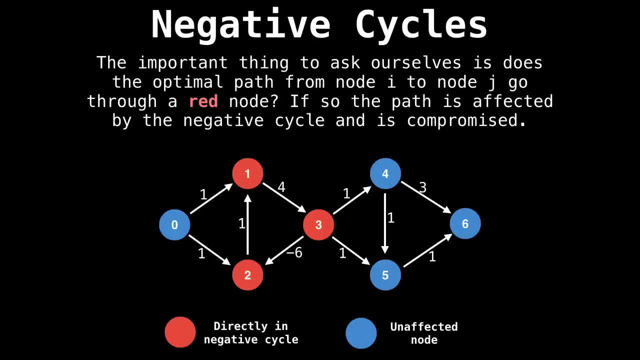 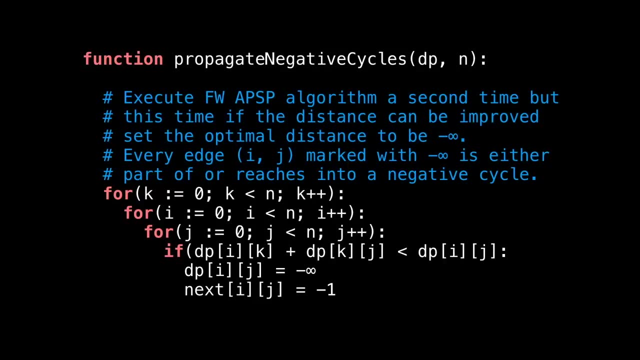 Consider the shortest path from four to six. This doesn't involve any red nodes, So we can safely conclude that the shortest path from four to six is indeed two. So to identify whether or not the optimal path from i to j is affected by a negative cycle, rerun the Floyd to Warshall algorithm second time. if 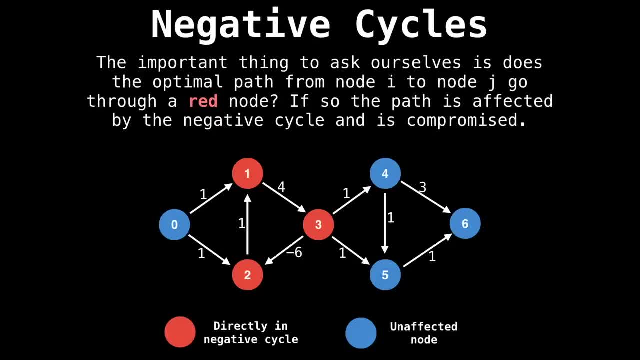 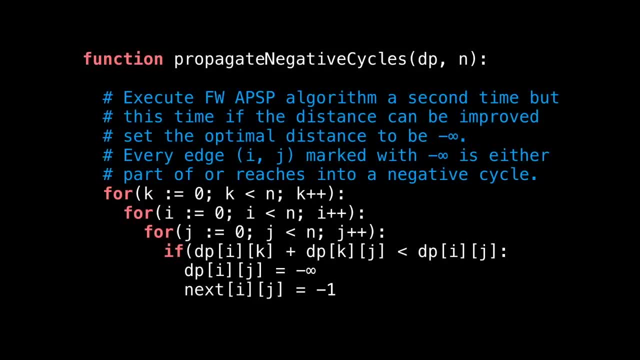 So we can safely conclude that the shortest path from four to six is indeed two. So to identify whether or not the optimal path from i to j is affected by a negative cycle, rerun the Floyd to Warshall algorithm second time, if the best distance is better than the already. 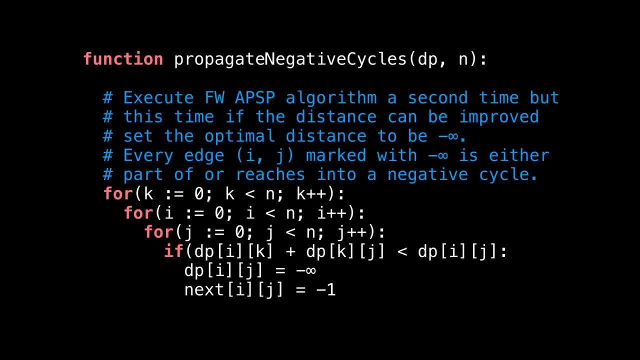 known best distance stored in our table dp. then set the value in the matrix from i to j to be negative infinity. Also mark the index at i- j in the next matrix with a minus one to indicate that the path is affected by a negative cycle. We will use this shortly. 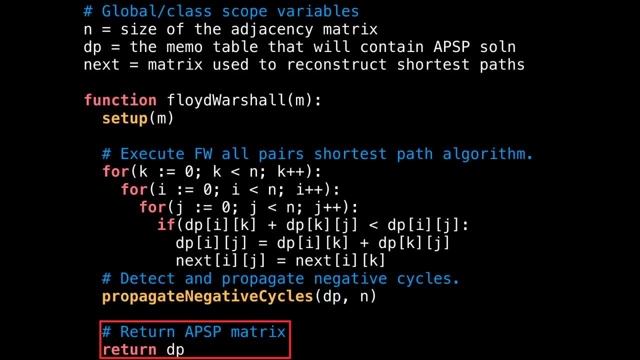 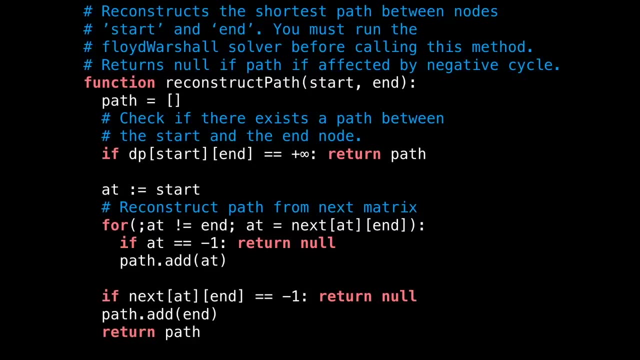 Back in the fluid to Warshall function. all we need to do is return the matrix dp, which contains the shortest distance from any node to any other node. This is the solution to the all pairs shortest path problem. The last thing I want to cover is how to reconstruct the shortest path between any 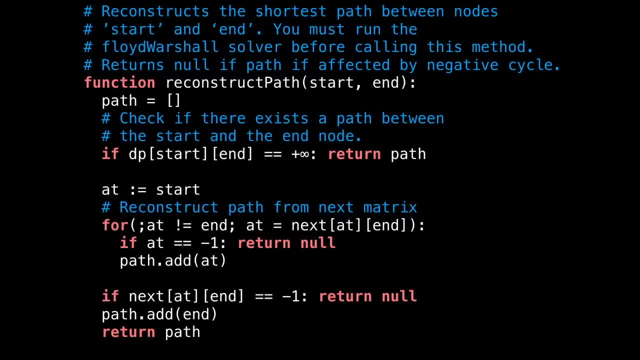 two pairs of nodes. This method returns the shortest path between the start and end nodes specified, or null. if there is a negative cycle, First check the distance between the start and end nodes. is positive infinity? If so, then return an empty path. Then to reconstruct. 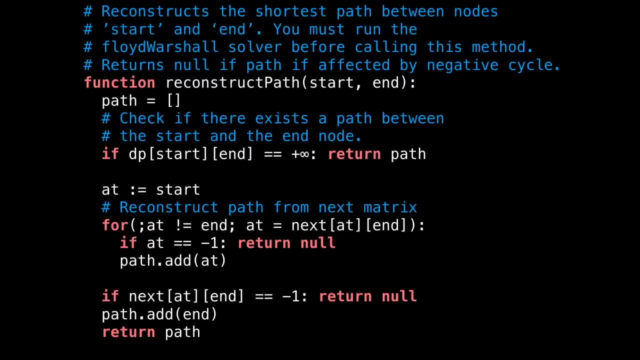 the path. I create a variable called at to track the current node, And then I loop through the next array adding the current node to the path. as I go During this process, I check if the current node has the value minus one. if it does, then this means that the optimal 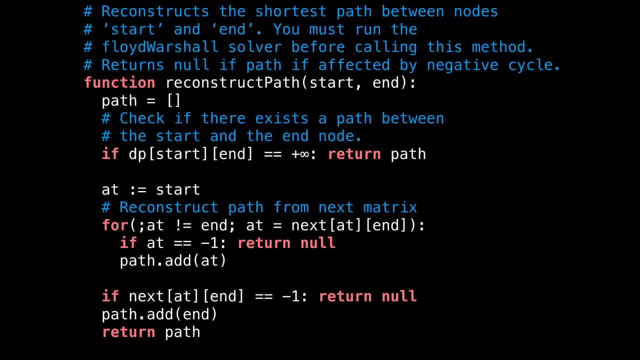 path encountered a red node and is trapped in a negative cycle, So return null. notice that, in reality, this method has three key return values: an empty path, which means that the start and end nodes are not connected. A null value, meaning a negative cycle was encountered. And lastly, a non empty path of node indices. 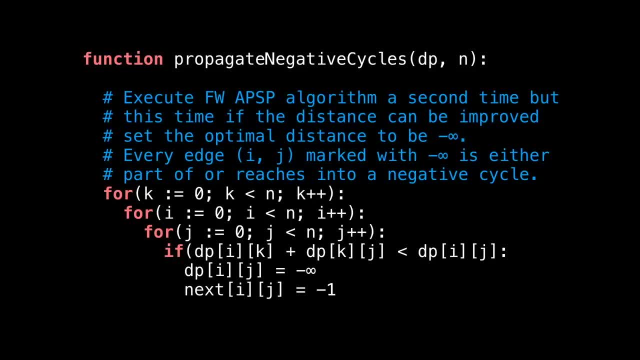 the best distance is better than the already known best distance stored in our table dp. then set the value in the matrix from i to j to be negative infinity. Also mark the index at i- j in the next matrix with a minus one to indicate that the path is affected by a negative cycle. We will use this shortly. 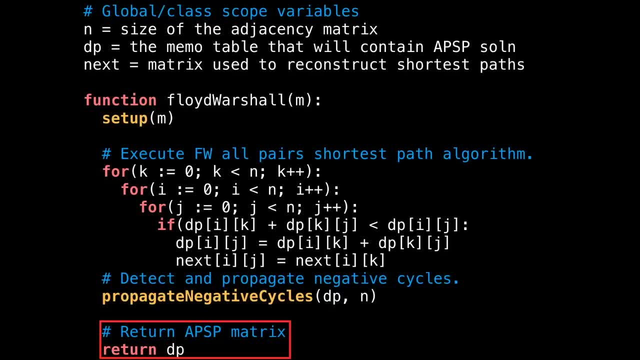 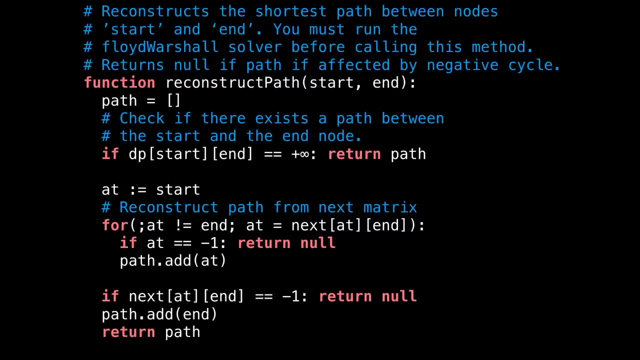 Back in the fluid to Warshall function. all we need to do is return the matrix dp, which contains the shortest distance from any node to any other node. This is the solution to the all pairs shortest path problem. The last thing I want to cover is how to reconstruct the shortest path between any 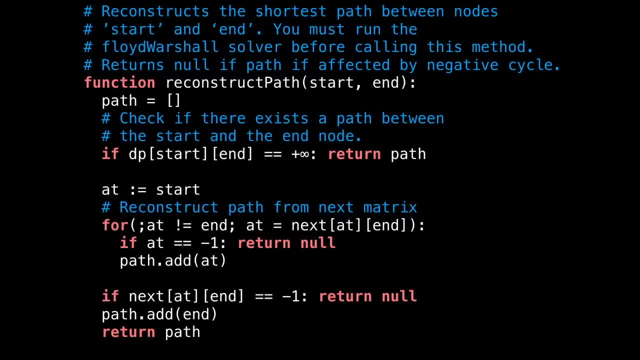 two pairs of nodes. This method returns the shortest path between the start and end nodes specified, or null. if there is a negative cycle, First check the distance between the start and end nodes. is positive infinity? If so, then return an empty path. Then to reconstruct. 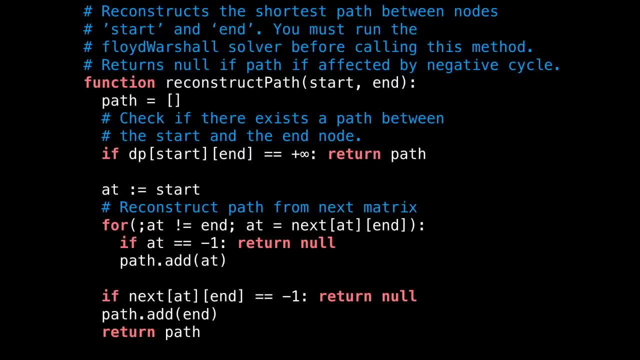 the path. I create a variable called at to track the current node, And then I loop through the next array adding the current node to the path. as I go During this process, I check if the current node has the value minus one. if it does, then this means that the optimal 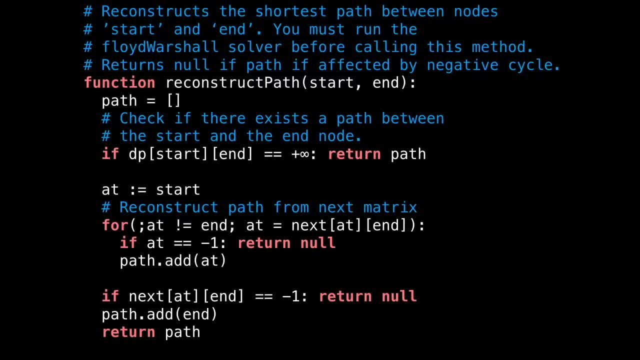 path encountered a red node and is trapped in a negative cycle, So return null. notice that, in reality, this method has three key return values: an empty path, which means that the start and end nodes are not connected. A null value, meaning a negative cycle was encountered. And lastly, a non empty path of node indices. 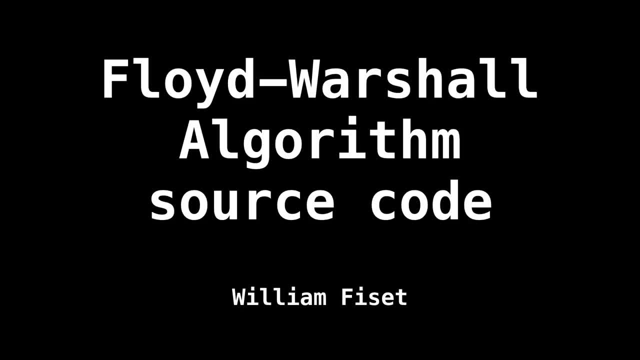 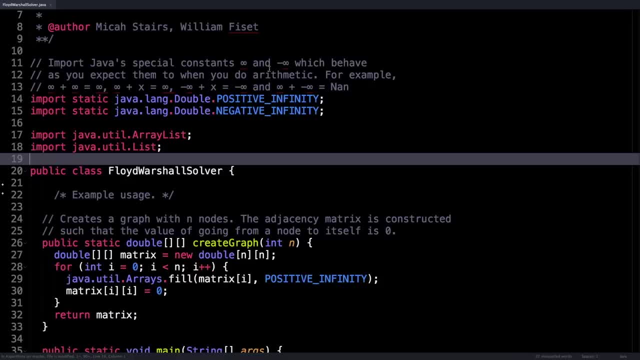 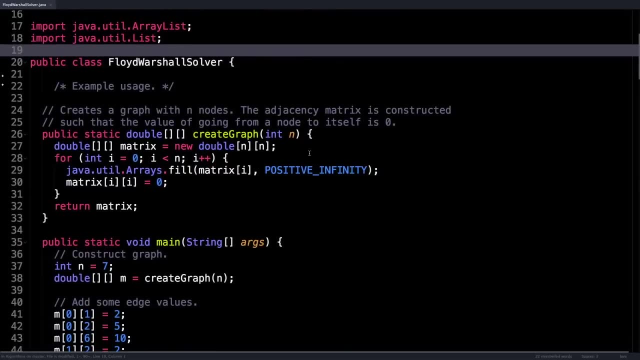 to mean an actual shortest path was found. Today we're going to be looking at some source code for the Floyd to Warshall all pairs shortest path algorithm. Here we are in the source code for the Ford to Warshall algorithm. So let's get started. Let's start by looking. 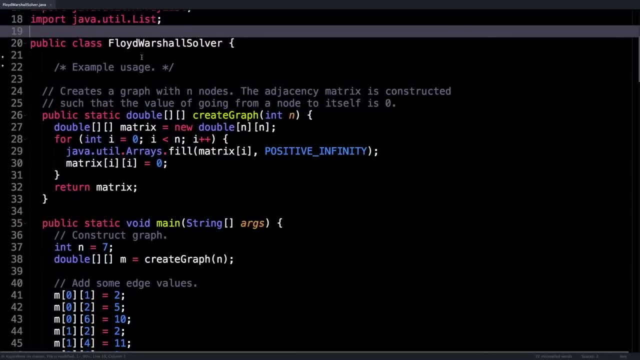 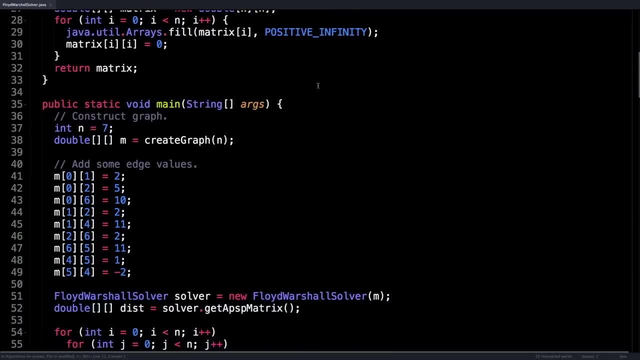 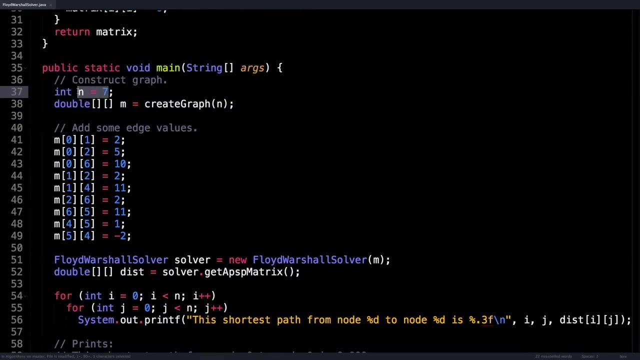 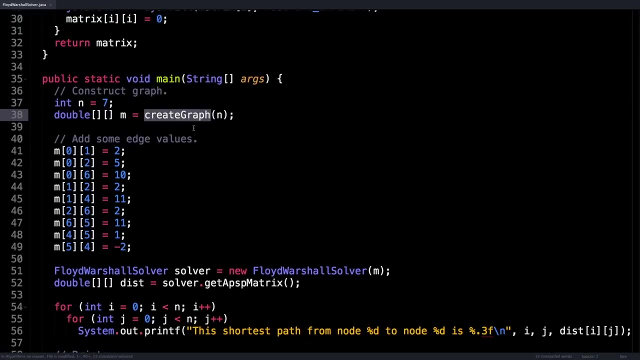 at an example of how to use this Floyd Warshall solver class to actually find all pairs shortest path. So here in the main method, the first thing I do is I actually initialize a graph with n nodes where n is set to seven And I create our adjacency matrix by calling the create graph method. And if we look at 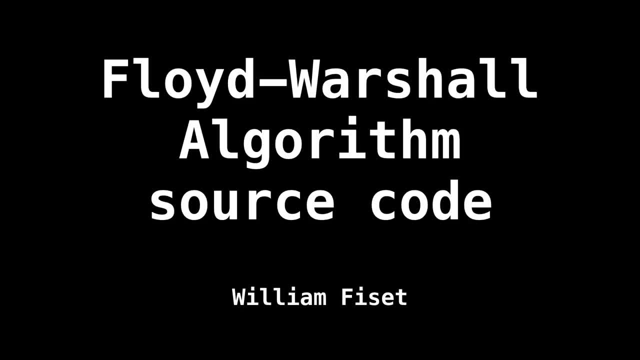 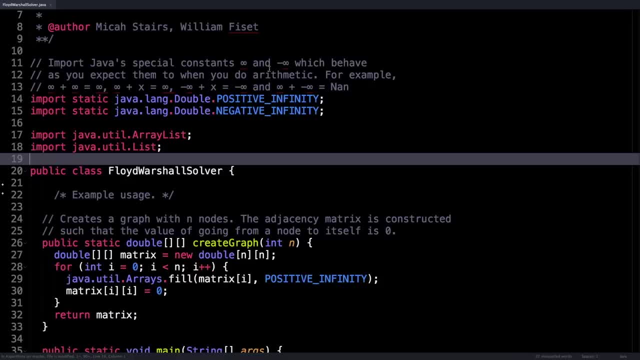 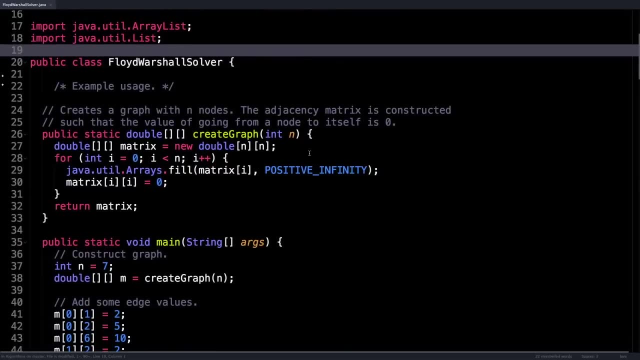 to mean an actual shortest path was found. Today we're going to be looking at some source code for the Floyd to Warshall all pairs shortest path algorithm. Here we are in the source code for the Ford to Warshall algorithm. So let's get started. Let's start by looking. 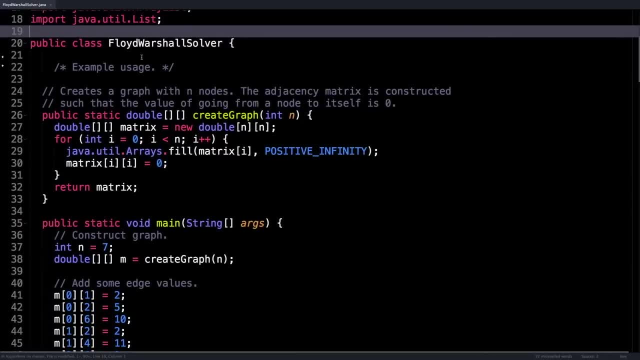 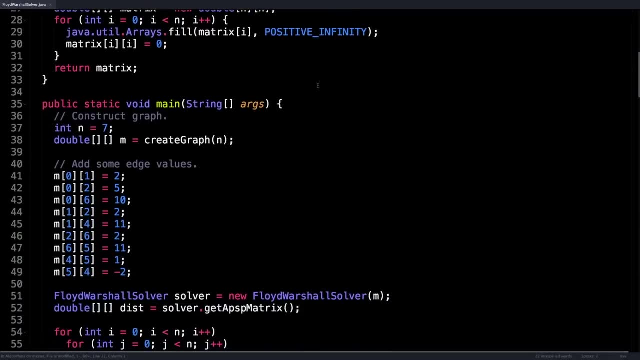 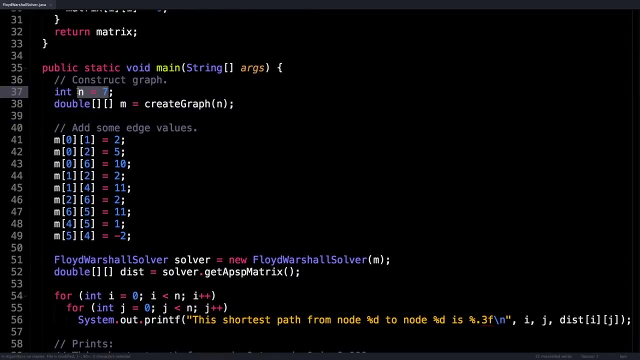 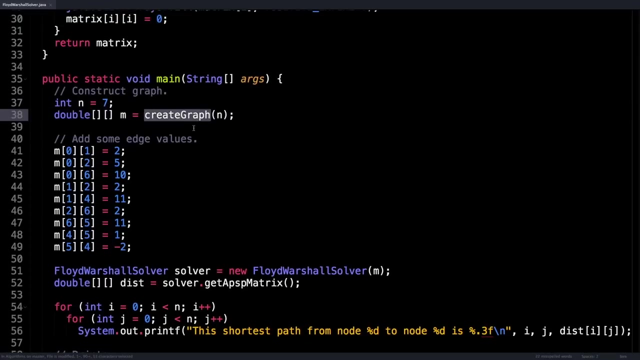 at an example of how to use this Floyd Warshall solver class to actually find all pairs shortest path. So here in the main method, the first thing I do is I actually initialize a graph with n nodes where n is set to seven And I create our adjacency matrix by calling the create graph method. And if we look at 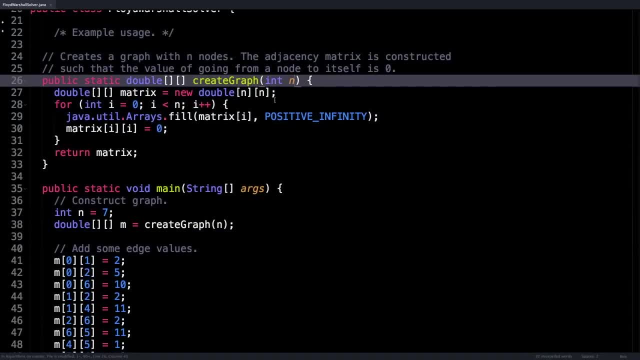 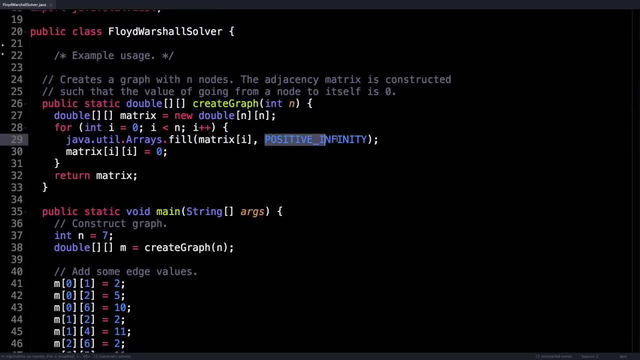 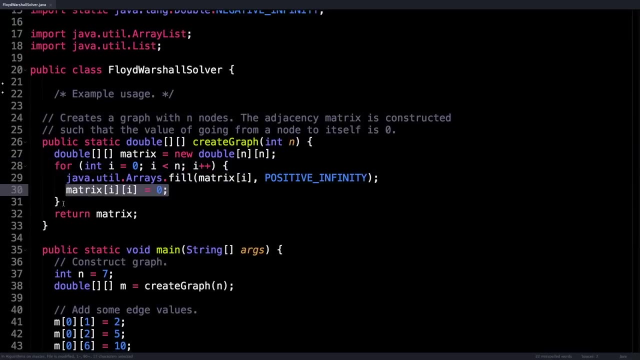 up here. this is the create graph method, And all it does is it initializes a matrix of size n by n, it fills the matrix with the special constant positive infinity And it also sets the diagonal to have all zero nodes by default, because I assume that this is the behavior you want. 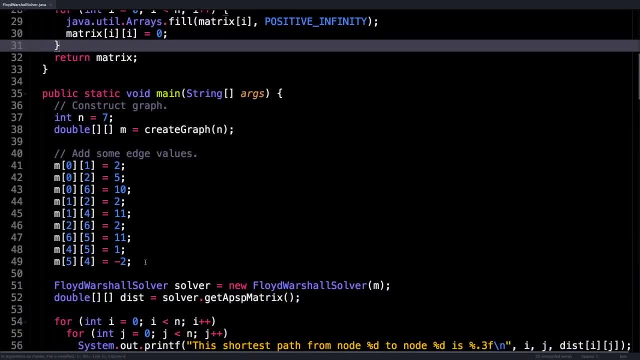 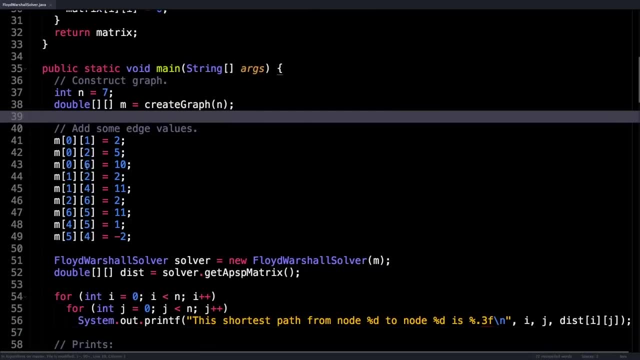 If it's not, then that's not an issue, because you can just override it when you add some edge values to your adjacency matrix. Alright, so we created a matrix, we added some edge weights, And then what we're going to do is we're going to create a matrix called the. 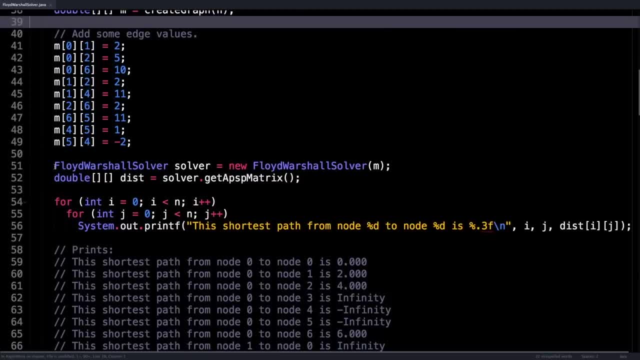 edge weights, And then what we're going to do is we're going to create a matrix called the edge weights, And then what we're going to do is we're going to create a matrix called the adj js matrix, And so what you'll want to do is create an instance of the solver and 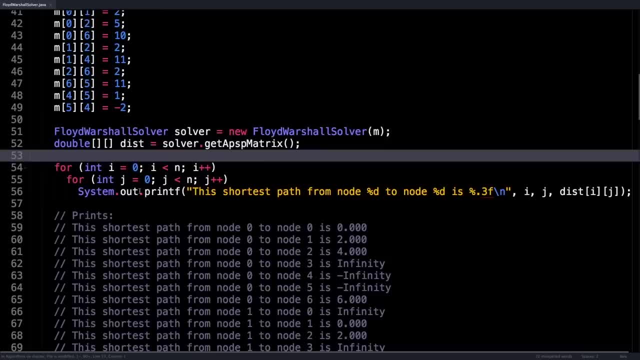 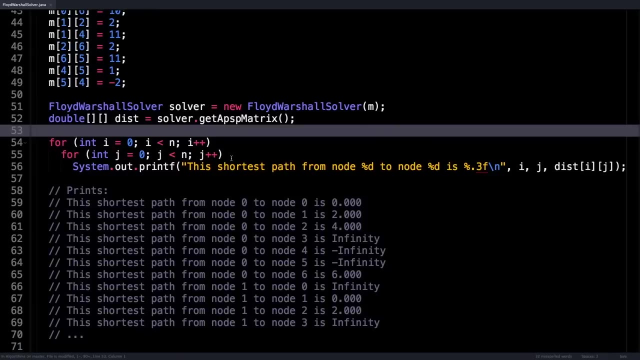 give it our adj js matrix And then call the get all appare shortest path matrix function, which will return the all paragraphs path matrix as a matrix called dist for distance. And then here all I do is I loop over all pairs of nodes, iN, j, and I print with the 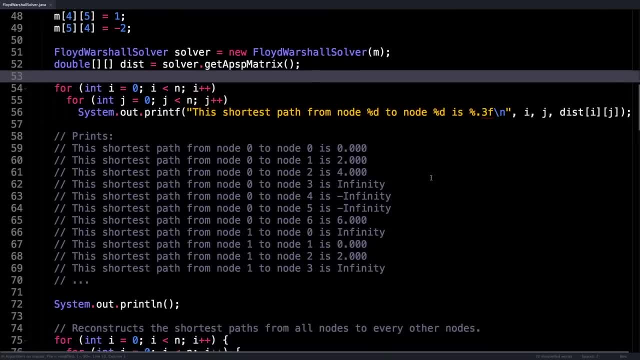 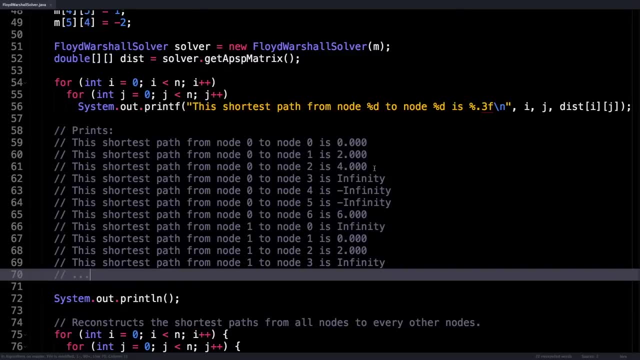 shortest path from node i to J is. Here's a sample of of what that looks like. So there can be roughly three different kinds of outcomes. we get a concrete shortest path. there does not exist a path between the two nodes. that'd be infinity. 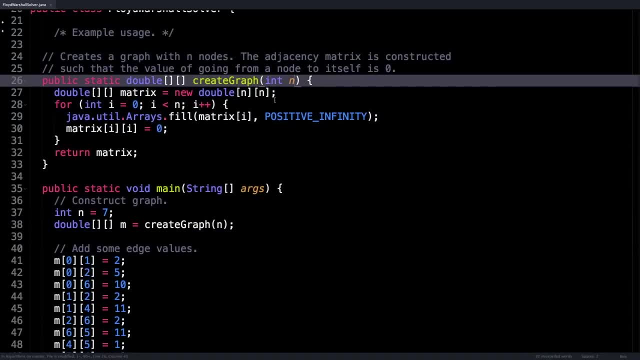 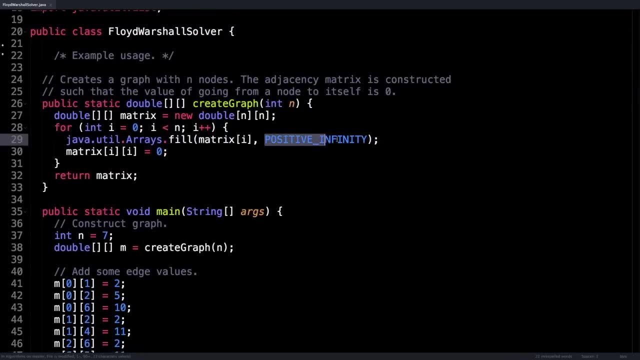 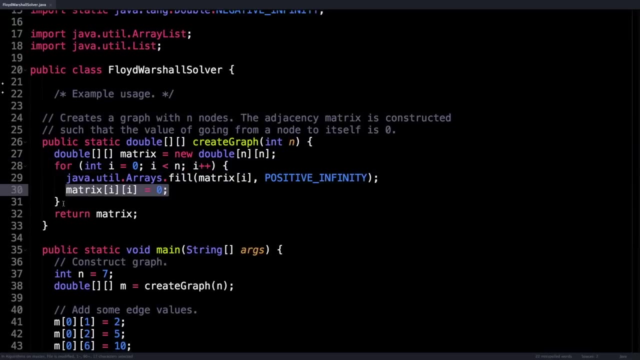 up here. this is the create graph method, And all it does is it initializes a matrix of size n by n, it fills the matrix with the special constant positive infinity And it also sets the diagonal to have all zero nodes by default, because I assume that this is the behavior you want. 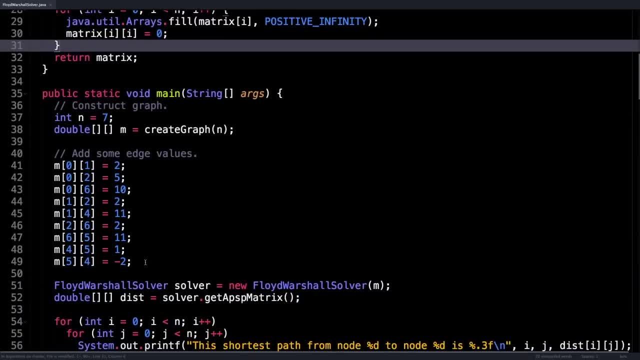 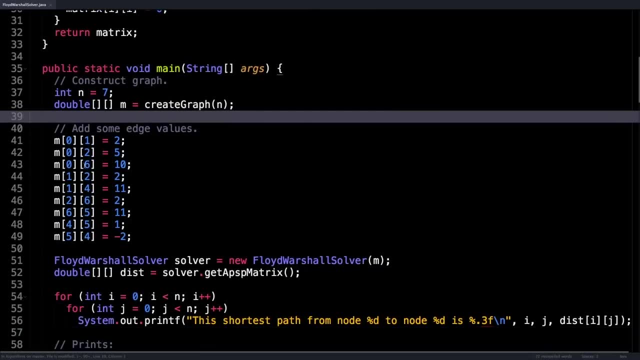 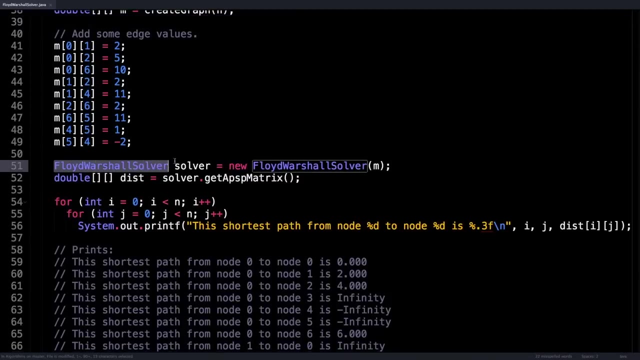 If it's not, then that's not an issue, because you can just override it when you add some edge values to your adjacency matrix. Alright, so we created a matrix, we added some edge weights, And then what you'll want to do is create an instance of the solver, give it our adjacency matrix. 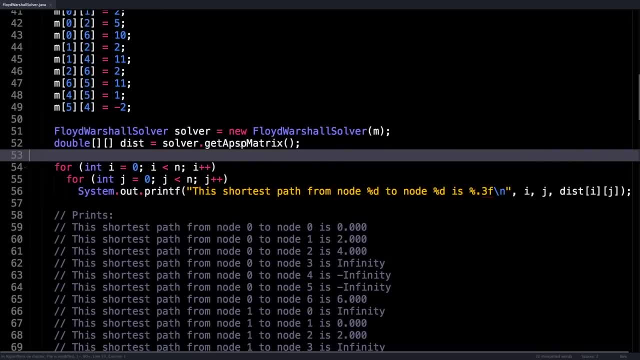 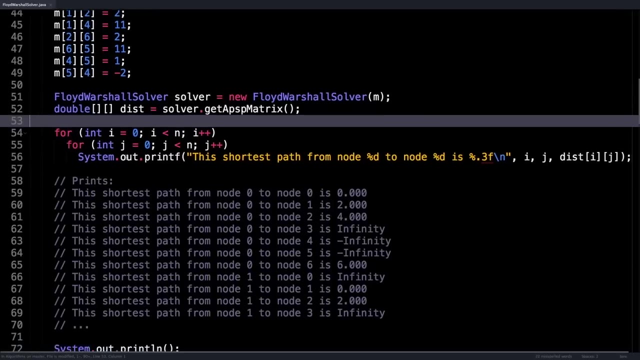 and then call the get all pair shortest path matrix function, which will return the all pair shortest path matrix as a matrix called dist for distance. And then here all I do is I loop over all pairs of nodes i and j, and I print with the shortest path from node. 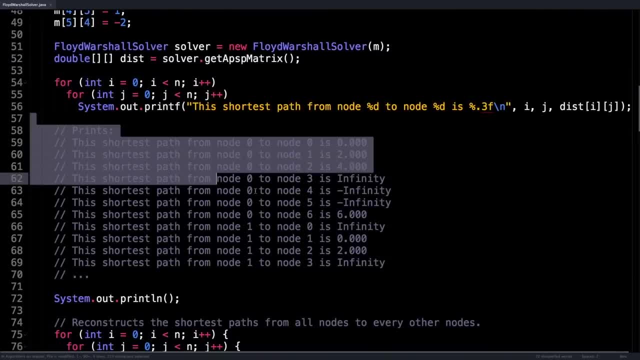 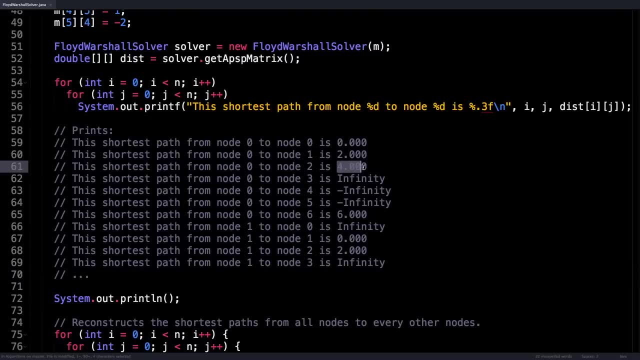 i to j is. here's a sample output of what that looks like. So there can be roughly three different kinds of outcomes. we get a concrete shortest path. there does not exist a path between the two nodes- that'd be infinity- and we encounter a negative cycle, So that 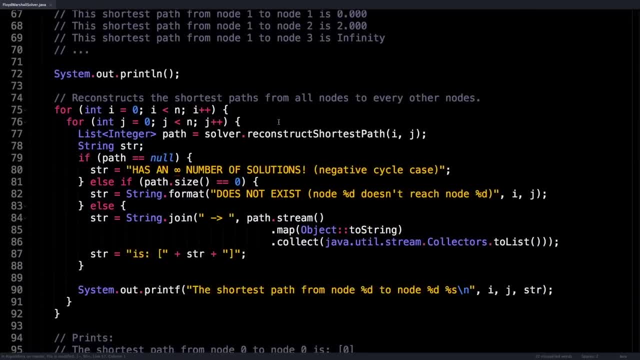 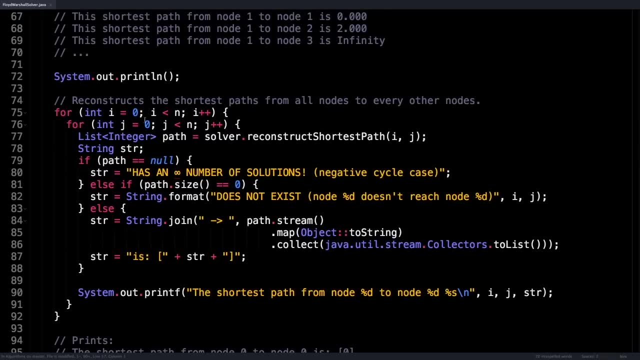 is negative infinity. Similarly, if we want to reconstruct the paths, this is how we're going to do it. Don't be scared by any of this. it's just text Being printed on the screen. So here I want to reconstruct the shortest path between all. 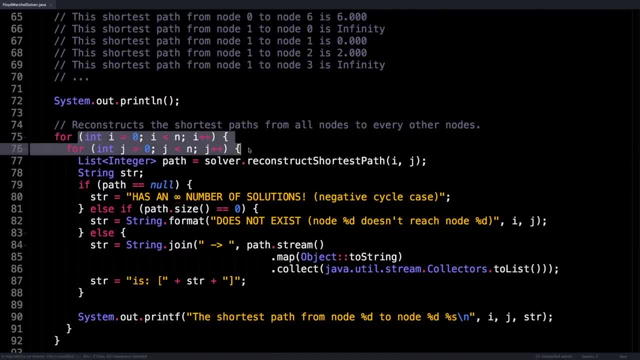 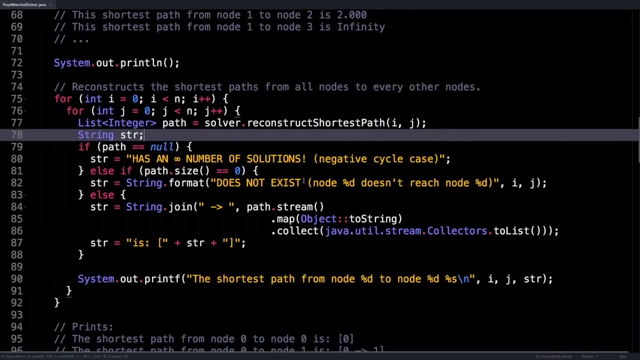 pairs of nodes. So I loop through all pairs of nodes i and j And then on the solver again I call reconstruct shortest path from i to j And that returns a list of nodes. And here I just print three different options, depending on when I get back. If the path 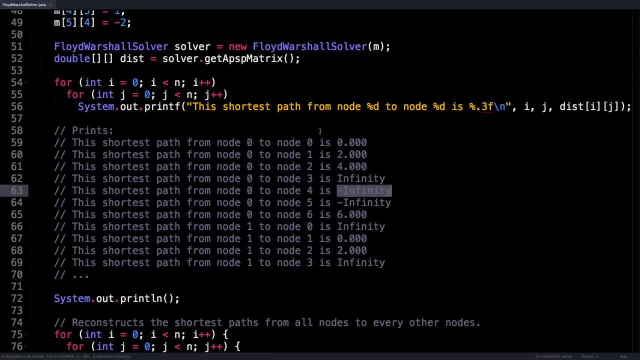 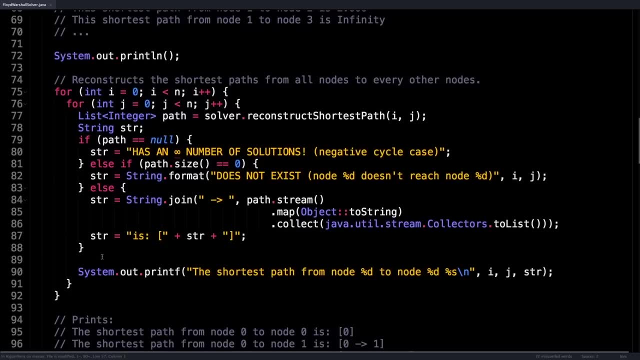 and we encounter a negative cycle. So that is negative infinity. Similarly, if we want to reconstruct the paths, this is how we're going to do it. Don't be scared by any of this. it's just text being printed on the screen. So here I want to reconstruct the 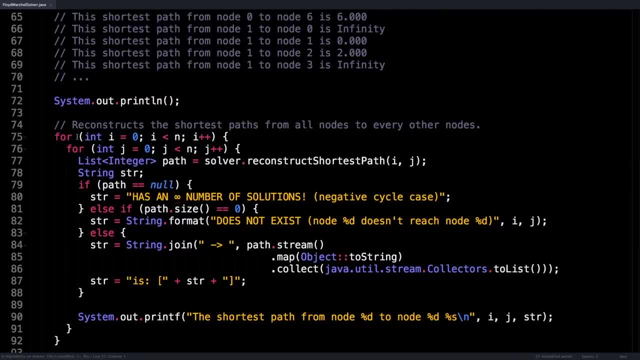 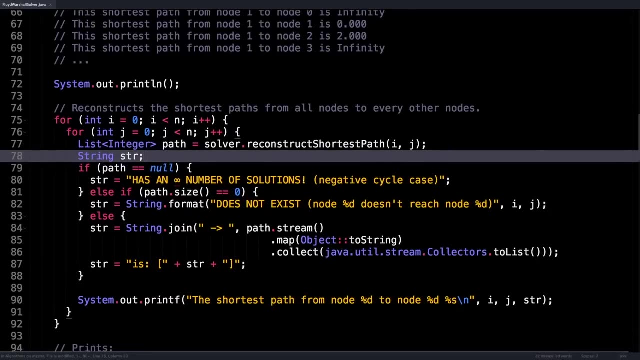 shortest path between all pairs of nodes. So I loop through all pairs of nodes, i and j, And then on the solver again I call reconstruct shortest path from i to j, And that returns a list of nodes. And here I just print three different options, depending on when I get. 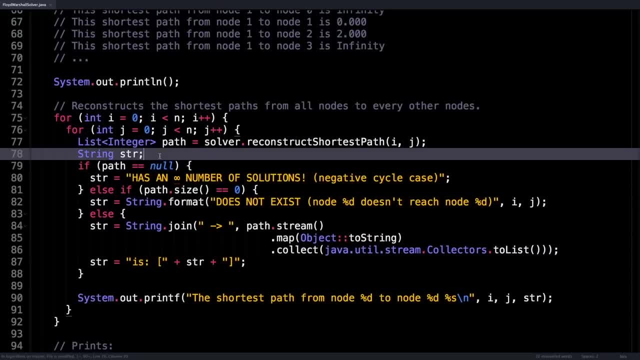 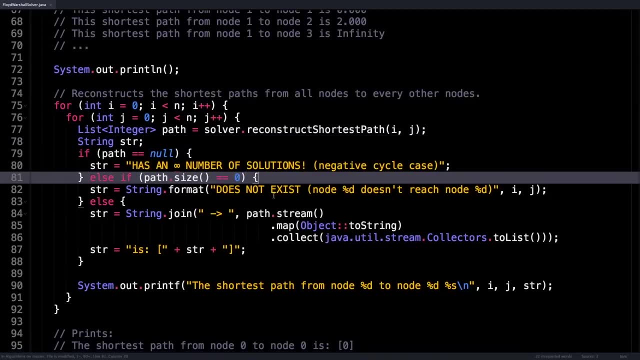 back. If the path is null, then there does not exist, or rather, sorry, there exists an infinite number of solutions. If the path has zero length, then there is no path, And if there is no length, there is no solution, And otherwise I just do a pretty formatting. 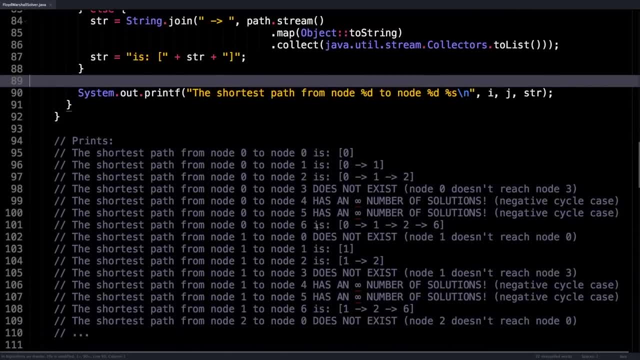 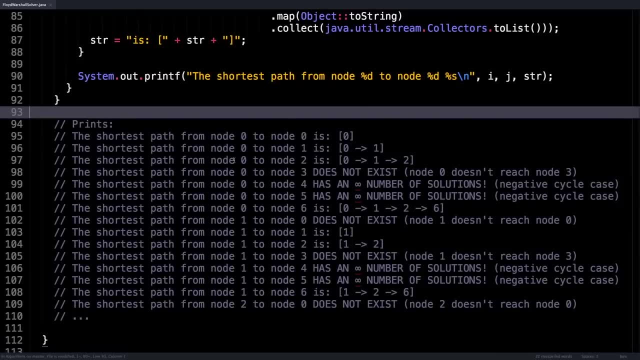 of the output. And this is what that would look like. So just prints what the path would be between all pairs of nodes. So, for instance, the shortest path from node two or node zero to node two in our graph goes through nodes 01 and two. And it does it, just prints all. 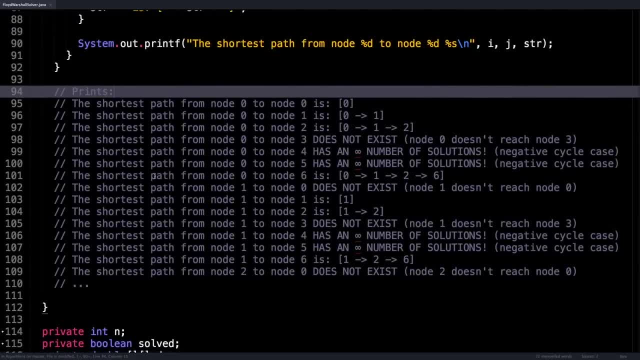 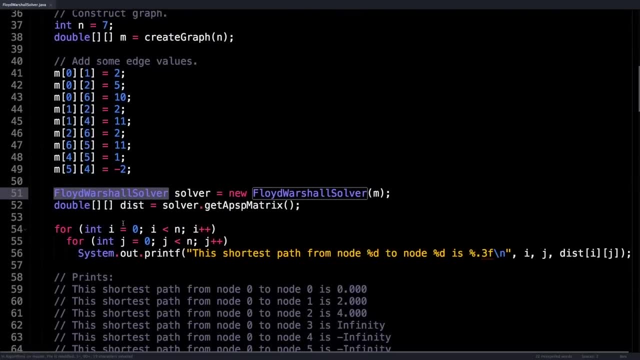 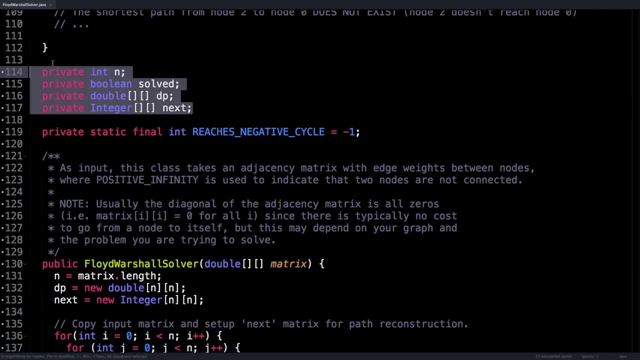 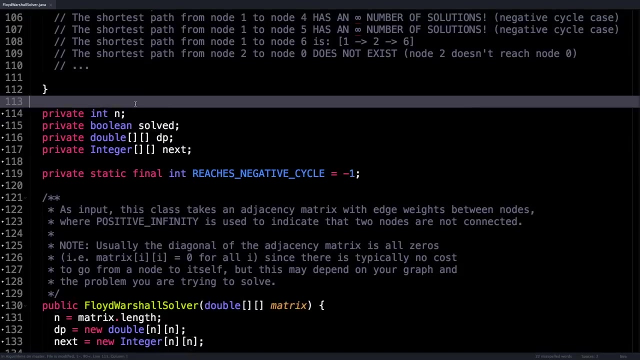 this information for all nodes. Okay, so what is this Floyd to Warshall solver actually doing? and that's what we're going to look at right now. So inside that class we have four instance variables and the number of nodes in our adjacency matrix, a Boolean value called solved, which just tracks whether 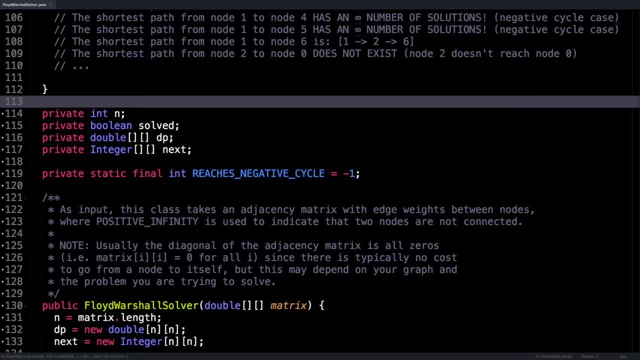 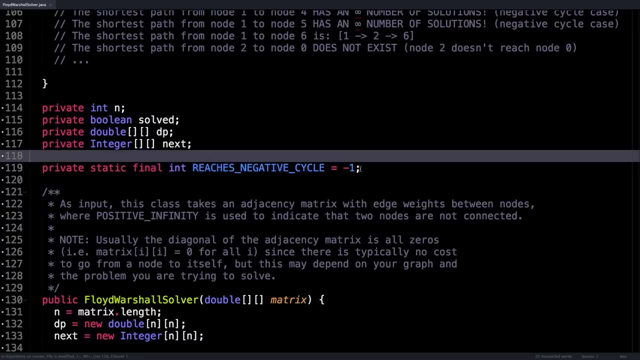 we've solved the all pairs: shortest path problem or not, Our DP matrix And a next matrix which is used to reconstruct the paths. And oh, there's also this constant, which I just initialize, minus one, so we can identify when we've reached negative cycles. 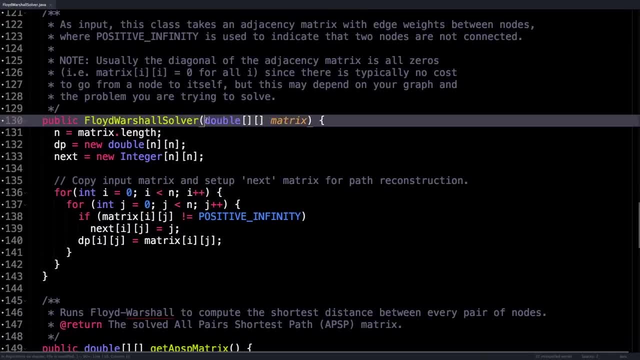 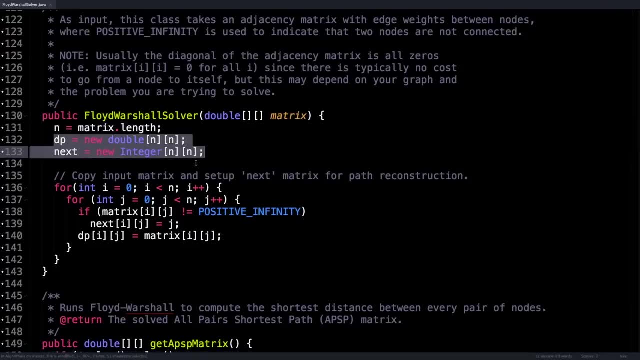 Okay. so, looking at the constructor again, you just pass in the input adjacency matrix And then I do some initialization, So simply allocate memory for our matrix. And then I do some initialization, And then I do some initialization, So simply allocate memory. 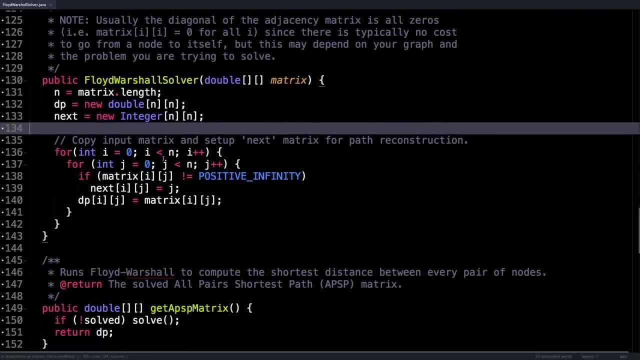 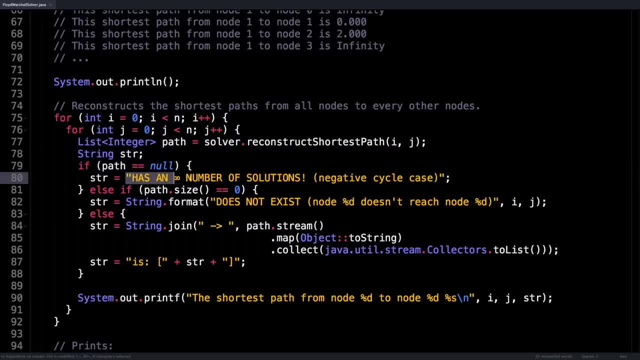 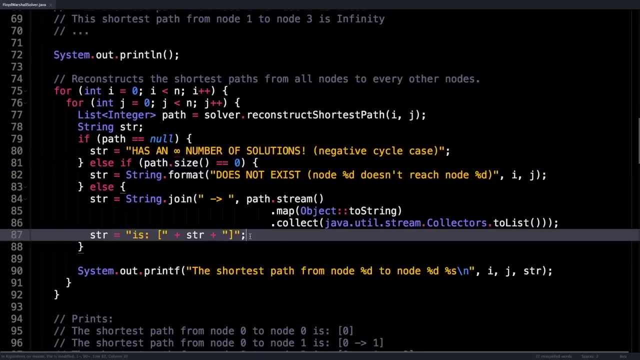 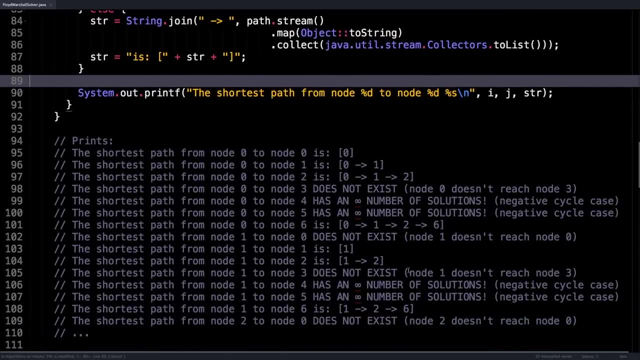 is null, then there does not exist, or rather, sorry, there exists- an infinity, And then I can just print a number of solutions. If the path has zero length, there is no solution, And otherwise I just do a pretty formatting of the output, And this is what that would. 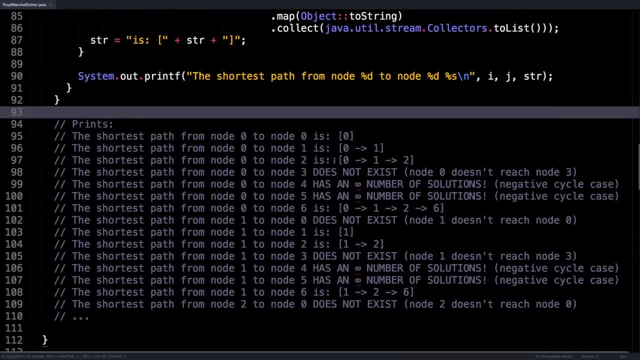 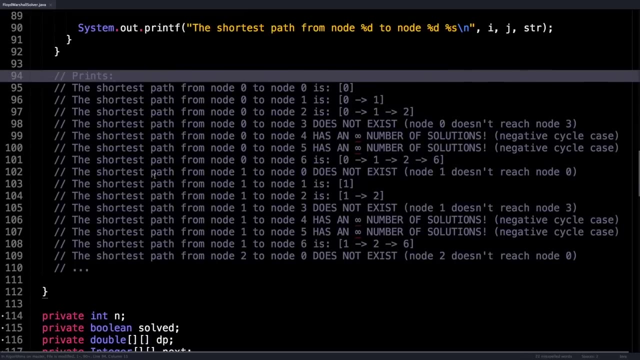 look like, So just prints what the path would be between all pairs of nodes. So, for instance, the shortest path from node two or node zero to node two in our graph goes through nodes zero, one and two, And it just prints all this information for all nodes in our graph, which is really useful. 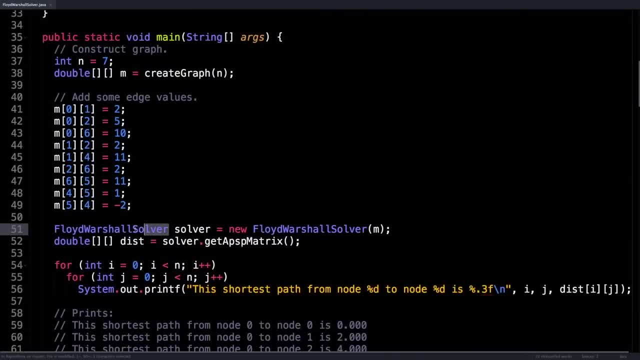 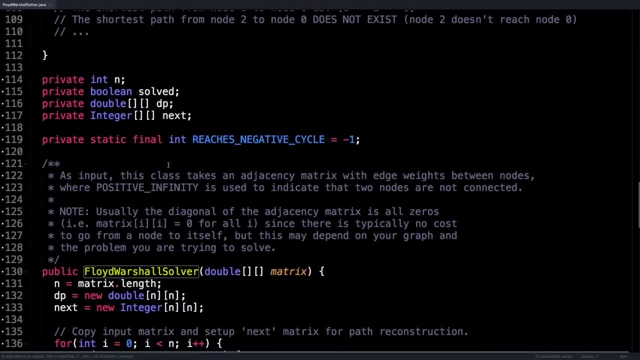 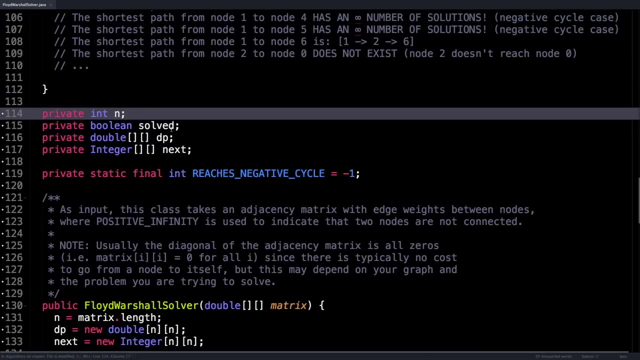 Okay, so what is this Floyd to Warshall solver actually doing? And that's what we're going to look at right now. So inside that class we have four instance variables and the number of nodes in our adjacency matrix, a Boolean value called solved, which just tracks whether we've solved the all pair. 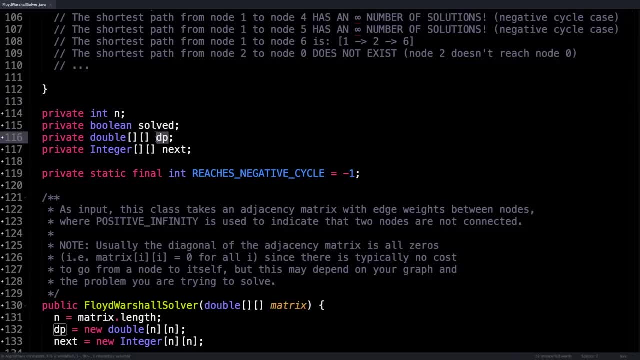 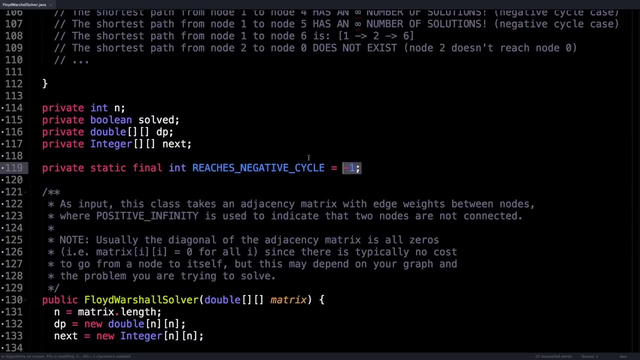 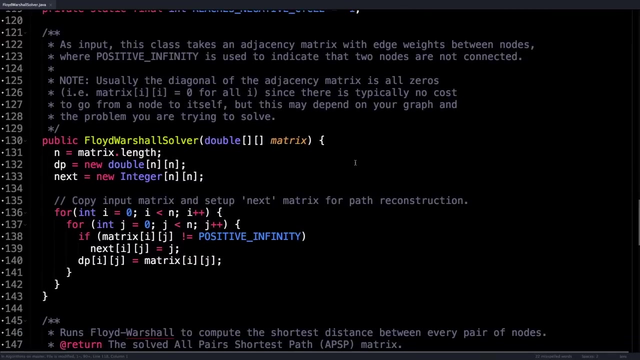 shortest path problem or not? our DP matrix and a next matrix which is used to reconstruct the paths. And oh, there's also this constant which I just initialize to minus one, so we can identify when we've reached negative cycles. Okay, so looking at the constructor again. 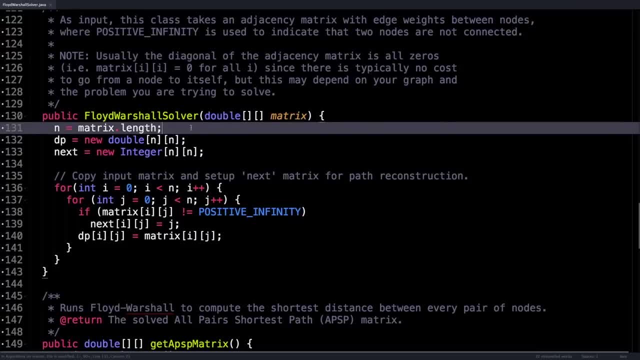 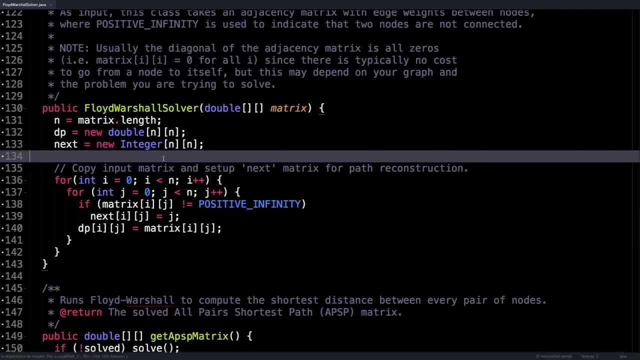 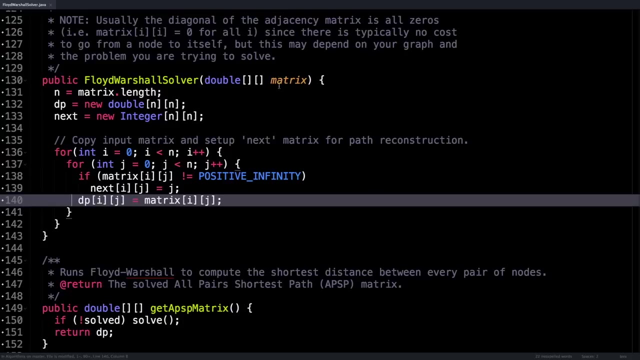 you just pass in the input adjacency matrix And then I do some initialization. So simply allocate memory for our matrices that we're going to need and then populate the DP matrix with whatever is given to us for our input And also make sure to initialize. 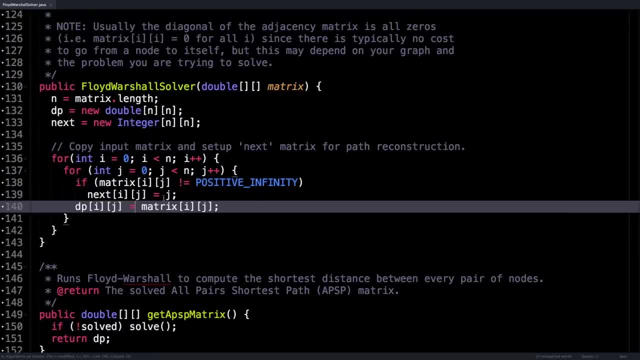 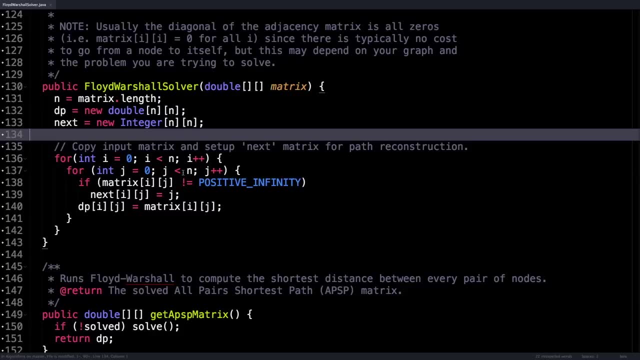 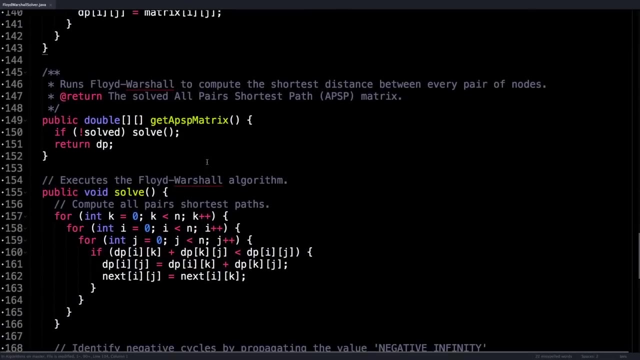 the next matrix to contain j as the next value, going from i to j, And that's all you need to do for the setup, Nothing too complicated. Let's look at some of the methods that are provided in this class. The first one is get. 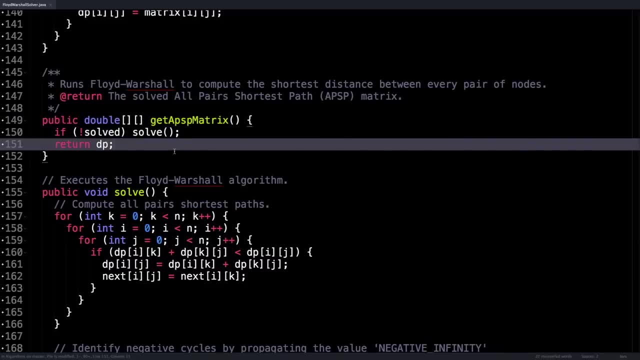 All Pairs Shortest Path matrix, which is the first method we called, And what that does is it looks if we've solved the all-pairs shortest path problem already and if not, it calls the solver. The reason I do this is so that if we want to get the all-pairs shortest path matrix, 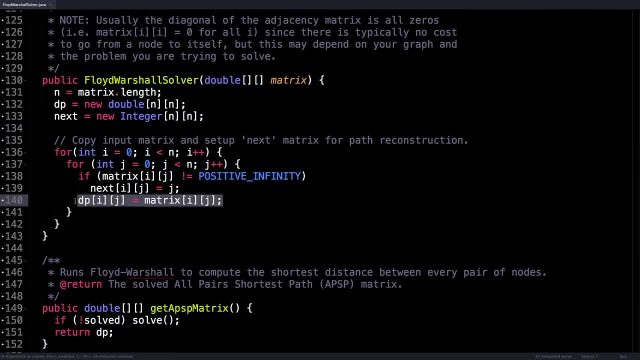 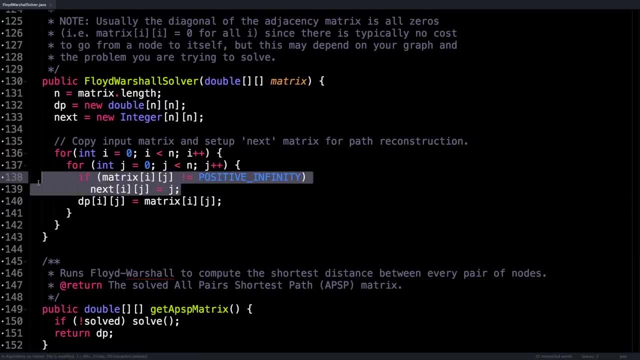 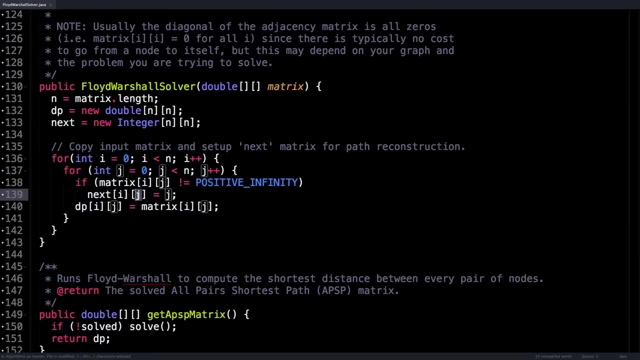 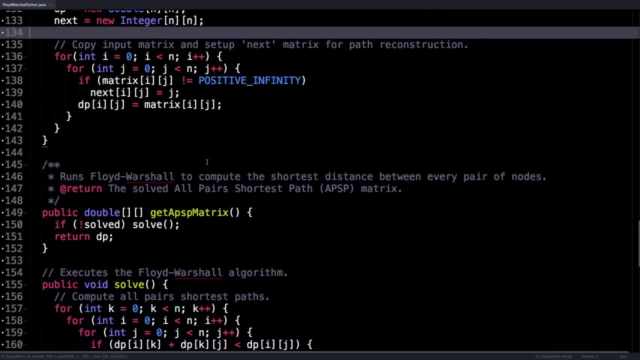 the DP matrix with whatever is given to us for our input and also make sure to initialize the next matrix to contain j as the next value, going from i to j. And that's all you need to do for the setup, Nothing too complicated. Let's look at some of the methods that are. 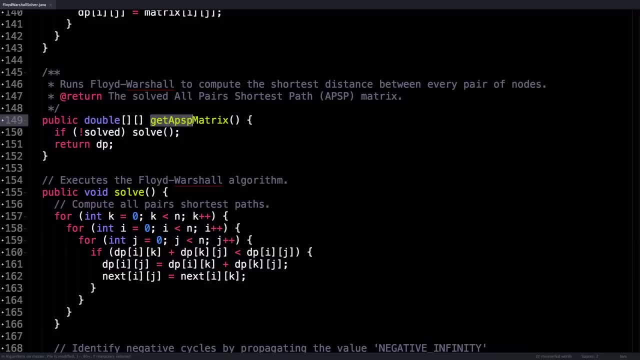 provided in this class. The first one is get all pairs shortest path matrix, which is the first method we called, And what that does is it looks if we've solved the all pairs shortest path problem already And if not, it calls the solver. The reason I do this: 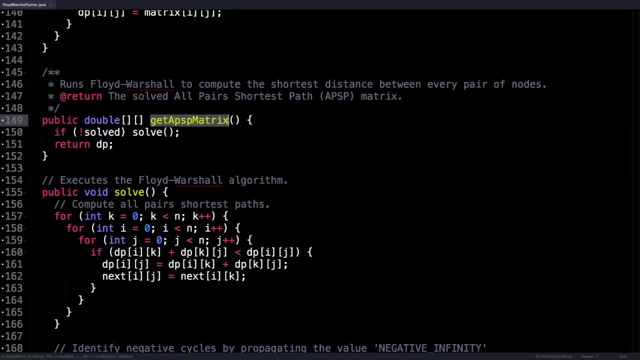 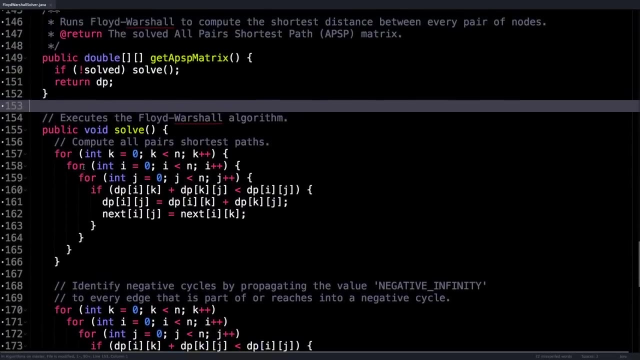 is so that if we want to get the all pairs shortest path matrix multiple times, that we don't run the solve method several times. So the solve method is what actually solves, or rather executes, the Floyd to Warshall algorithm. And here's what we're going to do to compute. 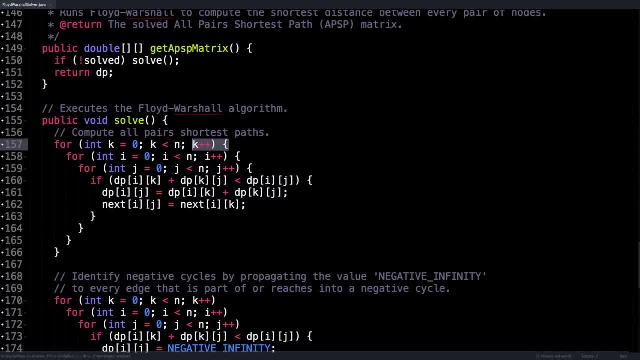 all pairs of shortest paths. First we iterate through k on the exterior loop And then we loop through all pairs of nodes and then we check for our condition. So if the path of going from i to k and then k back to j is less than the path from i to j, then update. 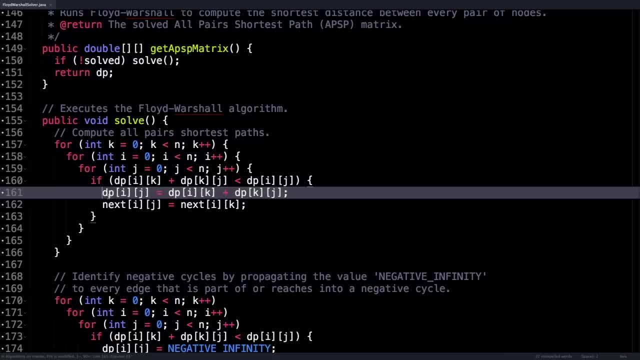 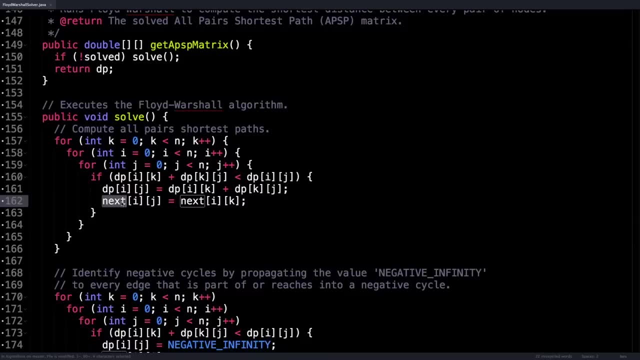 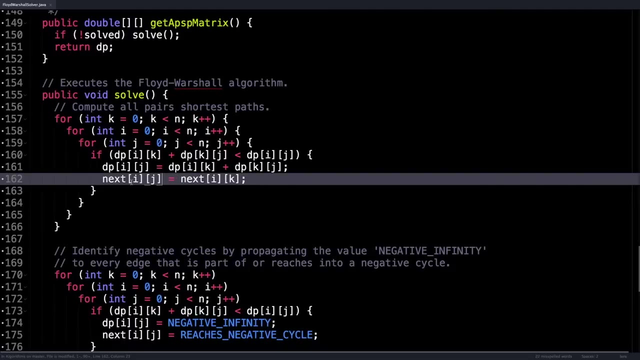 the value of i to j to route through that node k And while doing this also update the next matrix so that we can reconstruct the path later on. So it is now shorter to go through i to k, then i to j. So update the indices for i j. 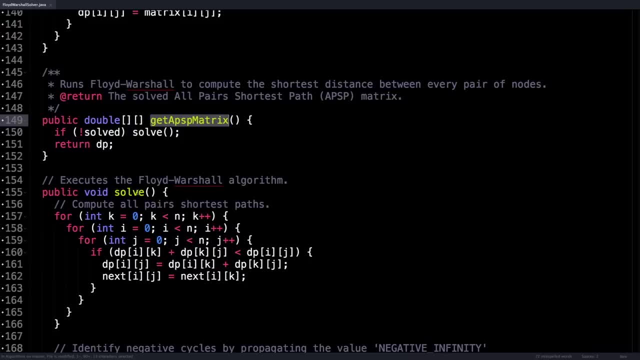 multiple times that we don't run the solve method. Okay, so first of all, I want to run the solve method, which is going to tell me how many pairs are gone. The first method I'm going to call the solve method, Because it's such a. 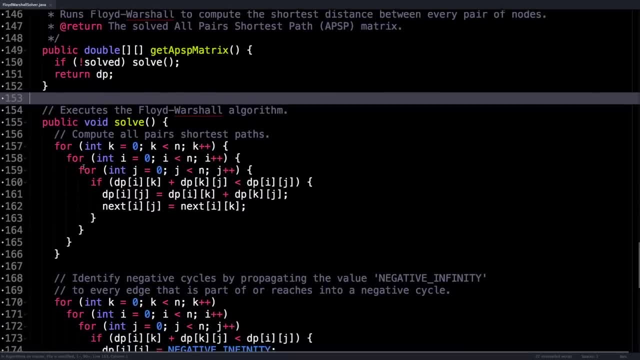 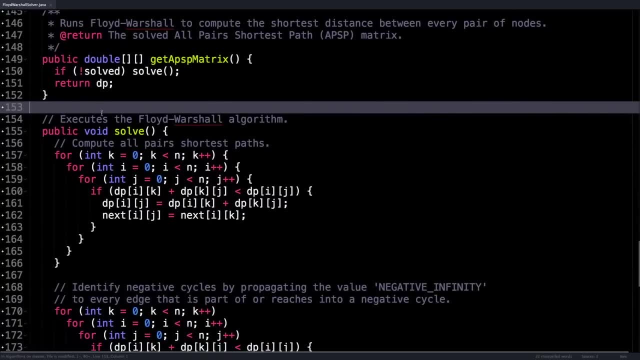 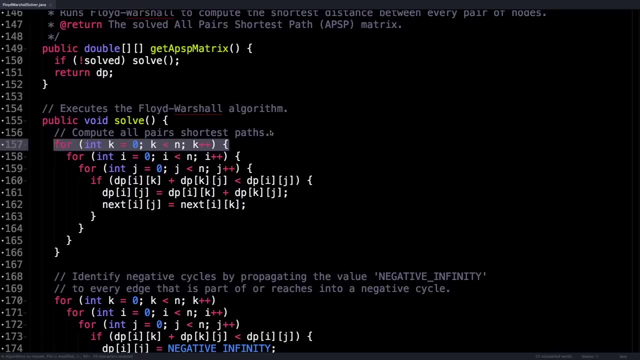 method several times. So the solve method is what actually solves, or rather executes, the Floyd to Warshall algorithm. And here's what we're going to do. to compute all pairs of shortest paths, First we iterate through k on the exterior loop And then we loop through. 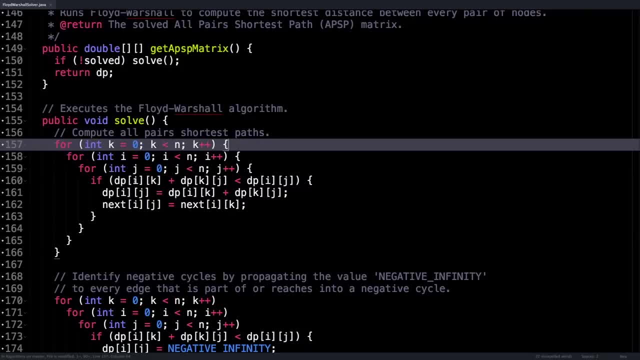 all pairs of nodes and then we check for our condition. So if the path going from i to k and then k back to j is less than the path from i to j, then update the value of i to j to route through that node k And while doing this also update the next matrix. so 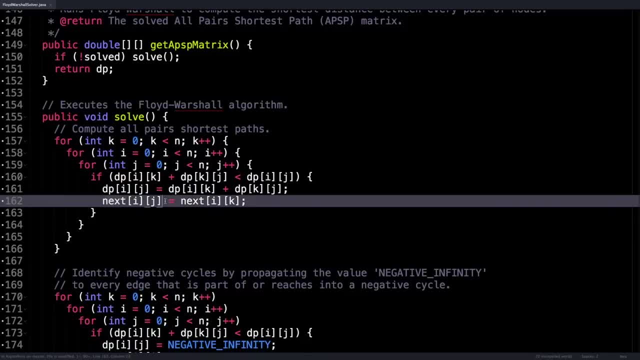 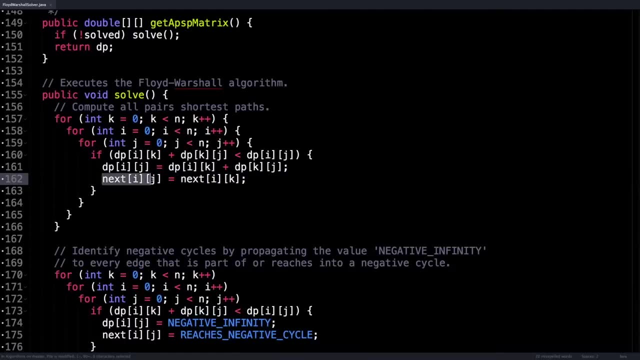 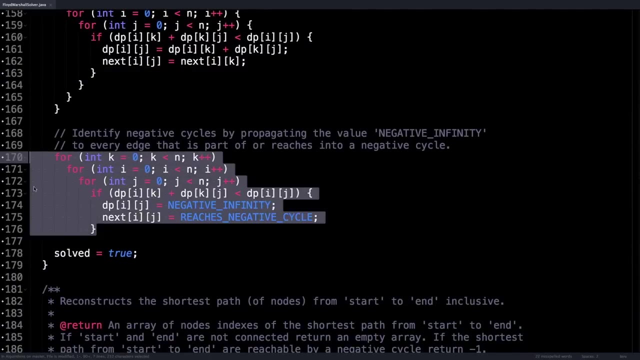 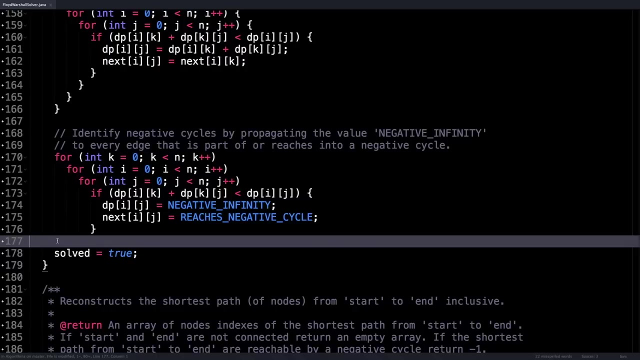 that we can reconstruct the path later on. So it is now shorter to go through i to k than i to j, So update the indices for ij. Okay. this next loop is if you want to identify negative cycles. identifying negative cycles means that we need to propagate the value of negative infinity throughout our graph. 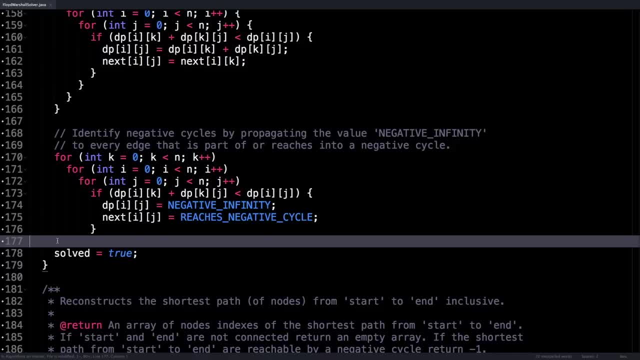 for every part of the graph that reaches a negative cycle. So, basically, if we can improve upon the already optimal solution, then we know that we're reaching a negative cycle somehow And that that that particular edge is compromised. So, simply, market with negative infinity. That is again. 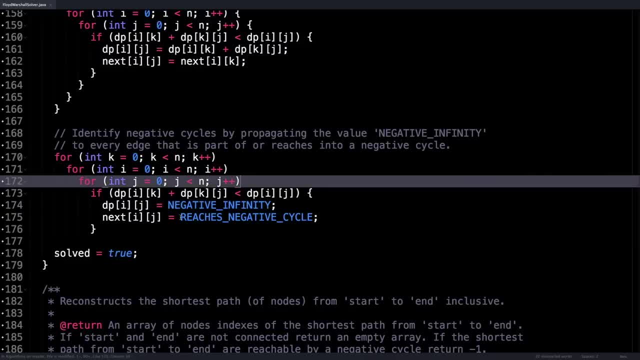 one of the special constants provided by Java. Similarly, update the next matrix to also mark the node as being contaminated by a negative cycle. But since next stores integer values, we can't give it the value negative infinity, which is a double, So give it the value minus. 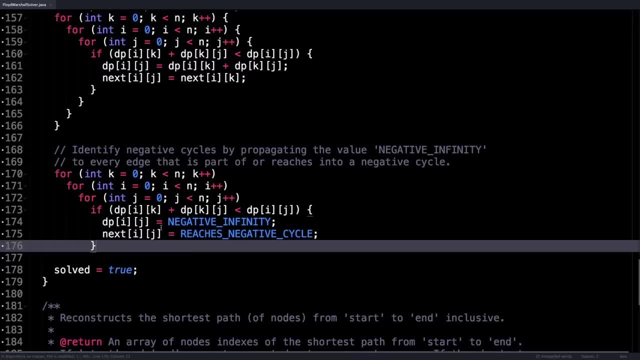 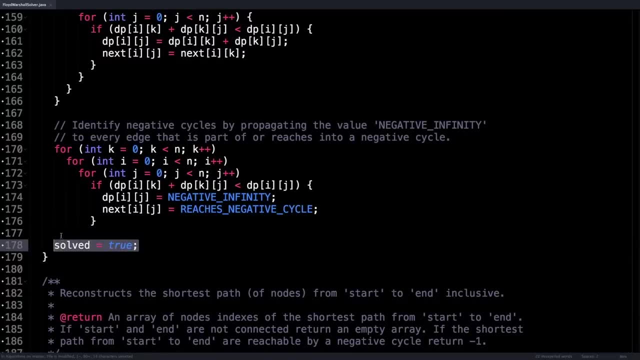 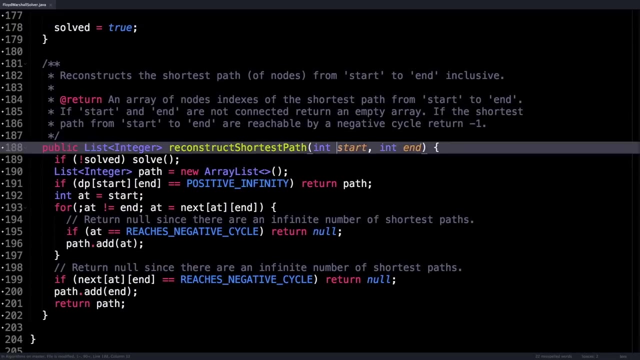 one stored in reaches. And once that is done, we have fully executed the Floyd Warshall algorithm And we can mark our Boolean value of solved as true. Now, if we look at reconstructing the shortest path from the start node to some ending node, what we want to do is- if we haven't done so already- 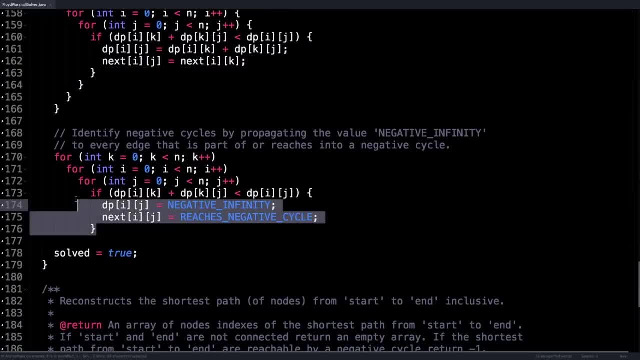 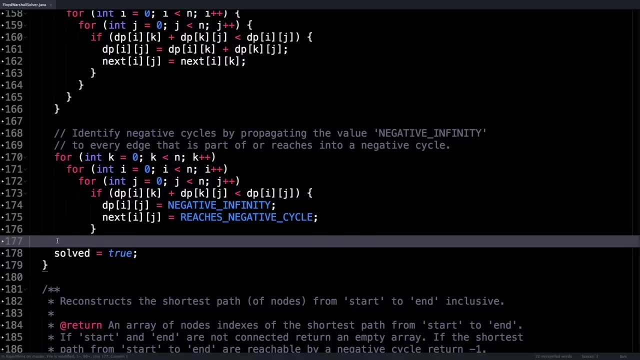 This next loop is if you want to identify negative cycles. identifying negative cycles means that we need to propagate the value of negative infinity throughout our graph for every part of the graph that reaches a negative cycle. So, basically, if we can improve upon the already optimal solution, then we know that we're reaching a negative cycle. 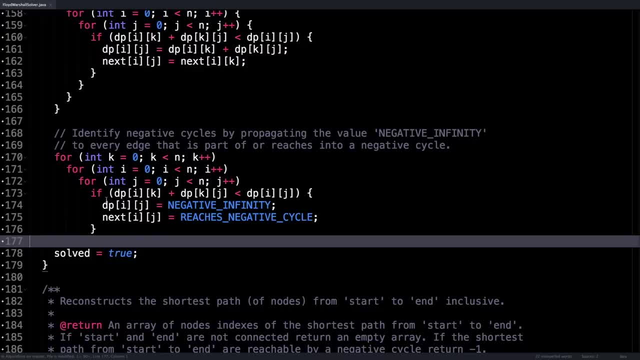 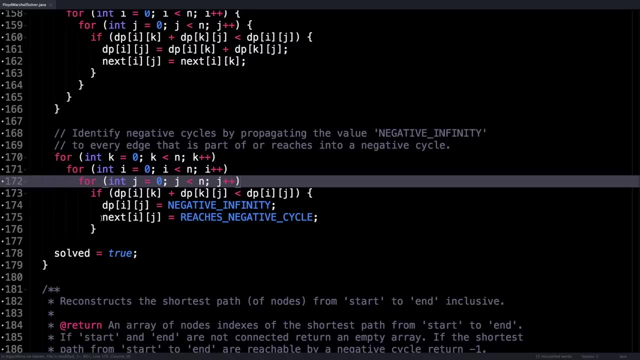 somehow, And that that particular edge is compromised. So simply, market with negative infinity. That is again one of the special constants provided by Java. Similarly, update the next matrix to also mark the node as being contaminated by a negative cycle, But since next stores. 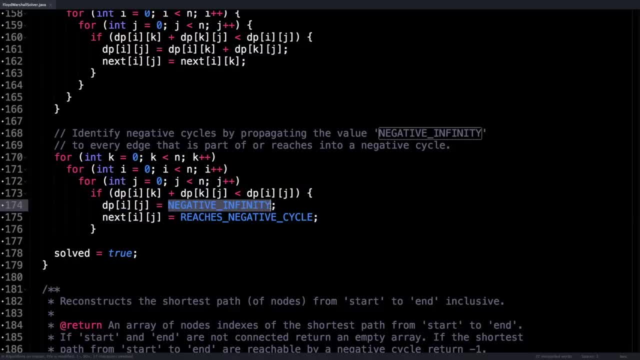 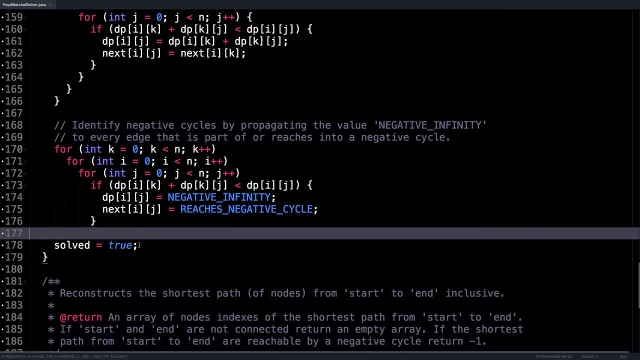 integer values. we can't give it the value negative infinity, which is a double, So give it the value minus one. stored in in reaches a negative cycle And once that is done, we have fully executed the Floyd Warshall algorithm And we can mark our Boolean value of solved as true. Now, if we look at 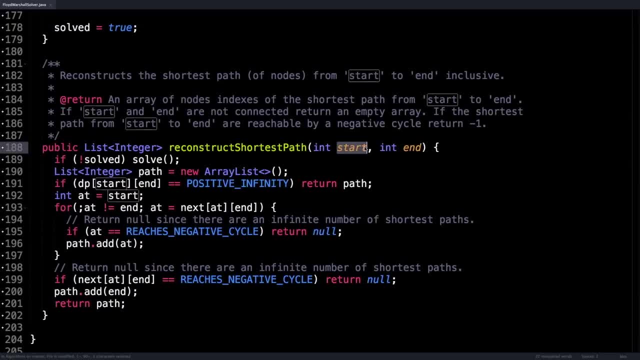 reconstructing the shortest path from the start node to some ending node. what we want to do is, if we haven't done so already, run the solver and then initialize a value called path to an empty array list. look at if it's even possible to reach the end node from the 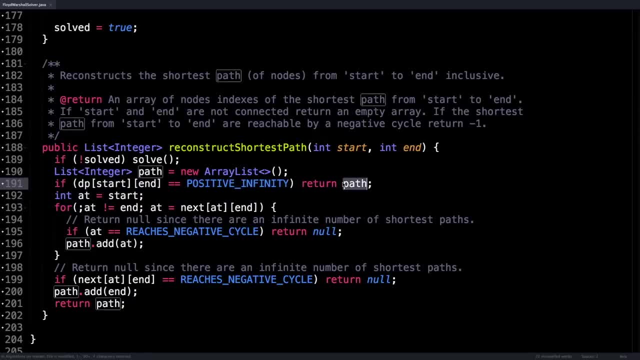 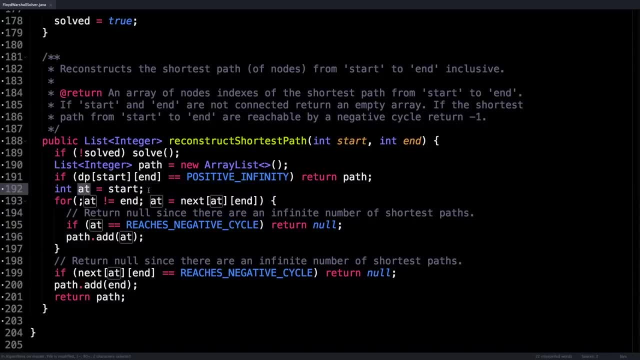 start node And if it's not return an empty path, otherwise populate the path with the current node, which I know denoted as at, and, for each current node, check if we reach into a negative cycle And if we do return null because the best value or, sorry, the 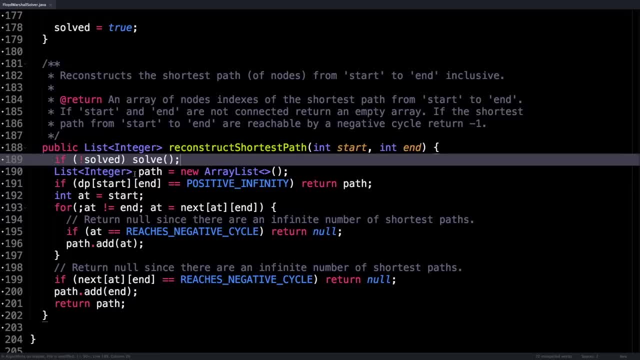 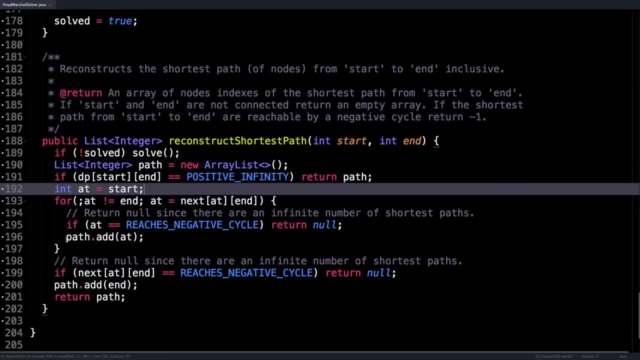 run the solver and then initialize a value called path to an empty array list. Look at this: If it's even possible to reach the end node from the start node and if it's not, return an empty path, otherwise populate the path with the current node, which I know denoted. 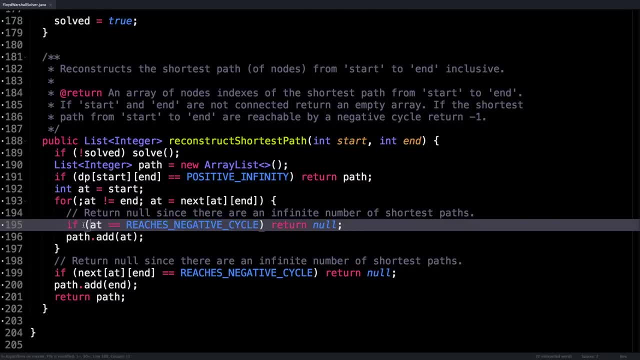 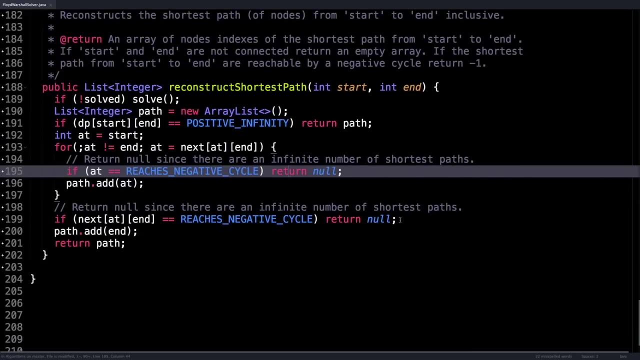 as at and for each current node, check if we reach into a negative cycle And if we do return null because the best value or, sorry, the shortest path doesn't exist, because there are an infinite number of shortest paths, And also make sure to check the edge case where the last node is part of an infinite. 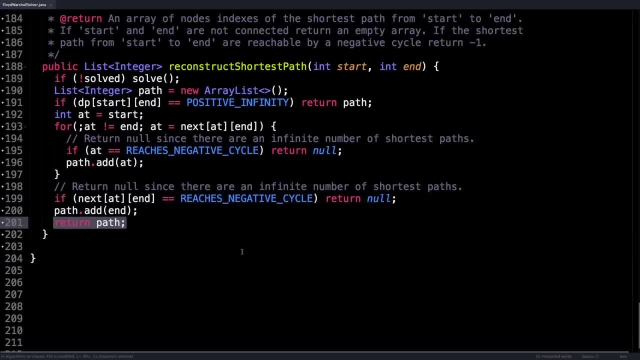 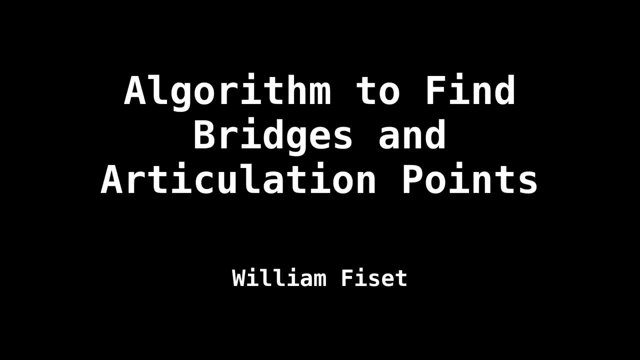 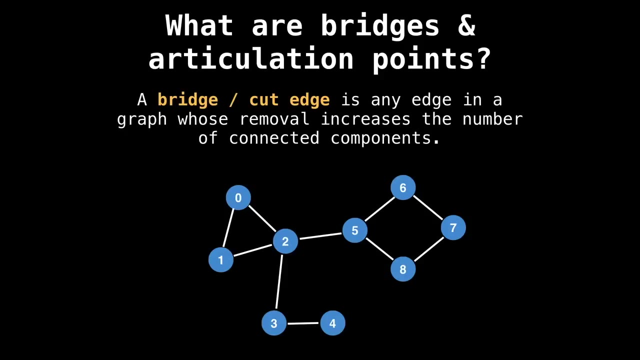 loop And simply return the shortest path. Today we're going to talk about how to develop an algorithm to find bridges and articulation points in an undirected graph from a computer science perspective. For starters, let's talk about what a bridge is in a graph: Bridges- 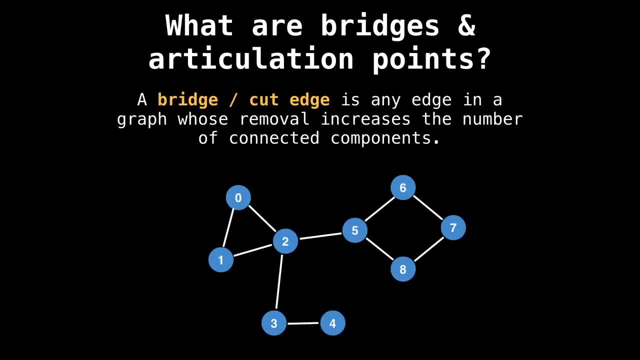 are sometimes also called cut edges. Essentially, if you have a graph which is a connected component, a bridge is an edge which, if removed, increases the number of connected components in the graph. The name bridge makes sense because if you think about connected components, 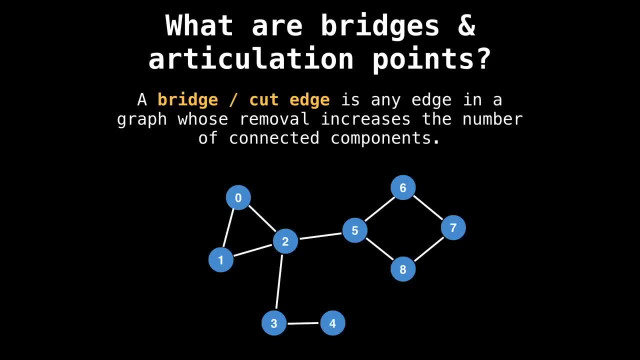 as islands, then a bridge is what separates them. So, for example, in this graph below there would be three possible bridges, Which are those edges in pink, because if you remove any of them, the graph is divided into two components. And articulation point, also called a cut vertex, is very similar. 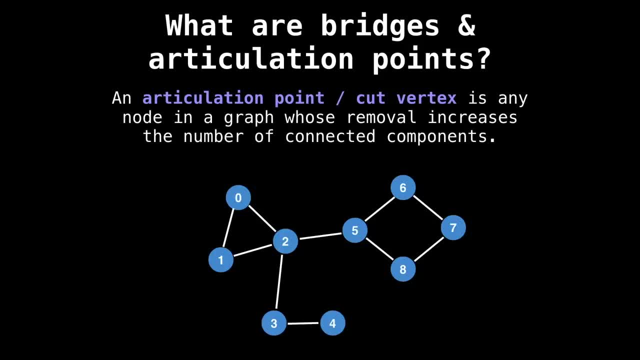 to a bridge, in that the criteria for being an articulation point is that it needs to be any node whose removal will increase the number of connected components. As an example, on this graph, there would be three articulation points since removing any of these vertices. 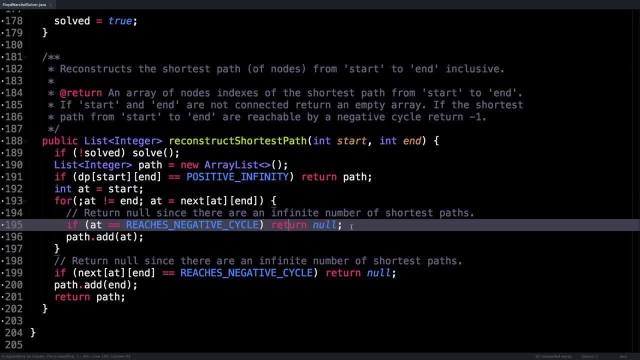 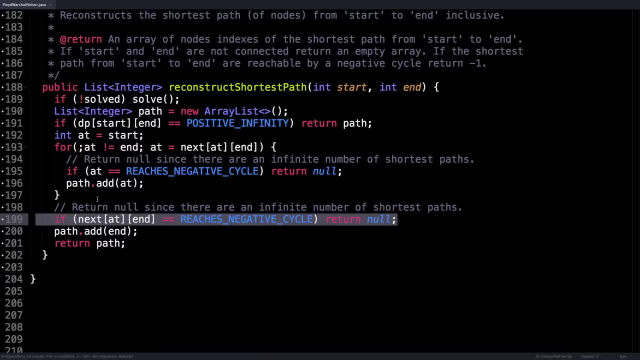 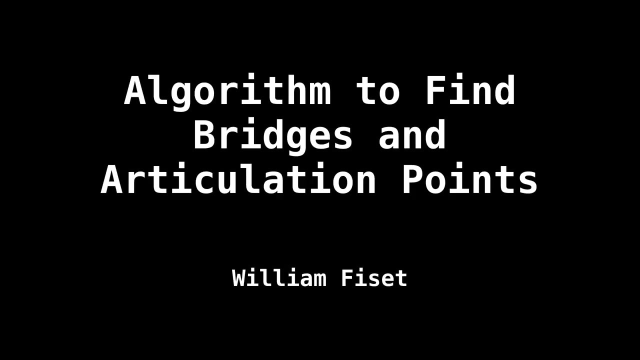 shortest path doesn't exist, because there are an infinite number of shortest paths. And also make sure to check the edge case, where the last node is part of an infinite loop, And simply return the shortest path. Today, we're going to talk about how to develop an algorithm. 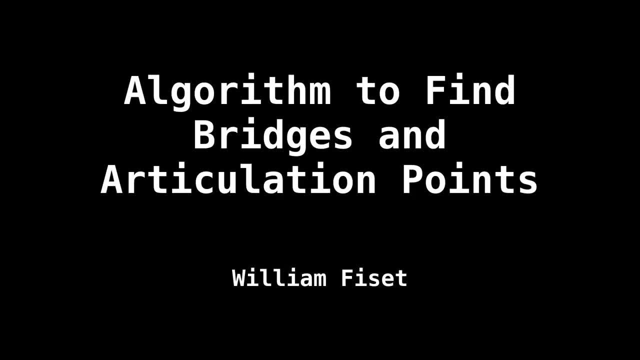 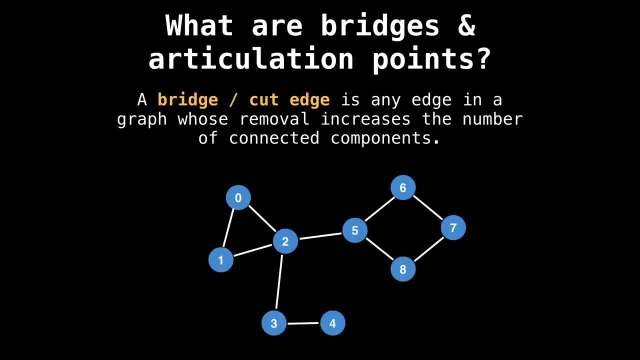 to find bridges and articulation points in an undirected graph from a computer science perspective. For starters, let's talk about what a bridge is In a graph. bridges are sometimes also called cut edges. Essentially, if you have a graph which is a connected component, a bridge is an edge which, if removed, increases the number. 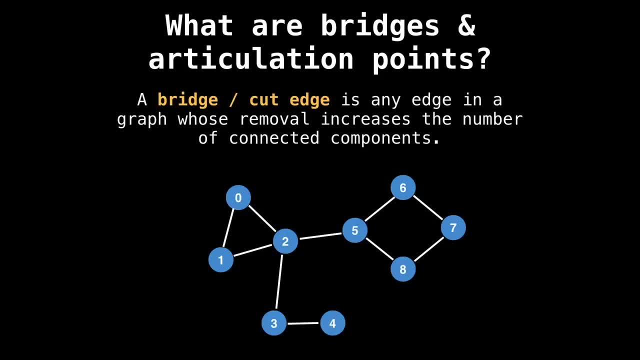 of connected components in the graph. The name bridge makes sense because if you think about connected components as islands, then a bridge is what separates them. So, for example, in this graph below there would be three possible bridges, which are those edges in pink, because if you remove 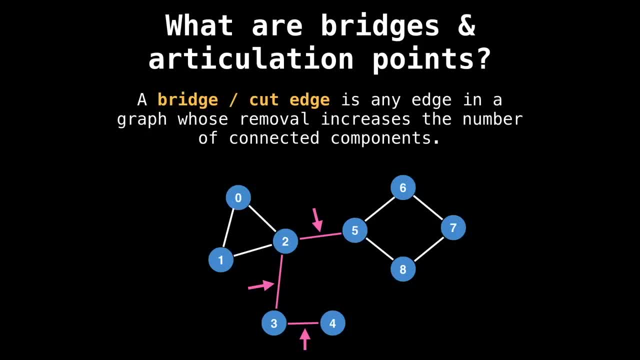 any of them, the graph is divided into two components, And articulation point, also called a cut vertex, is very similar to a bridge in that the criteria for being an articulation point is that it needs to be any node whose removal will increase the number of connected. 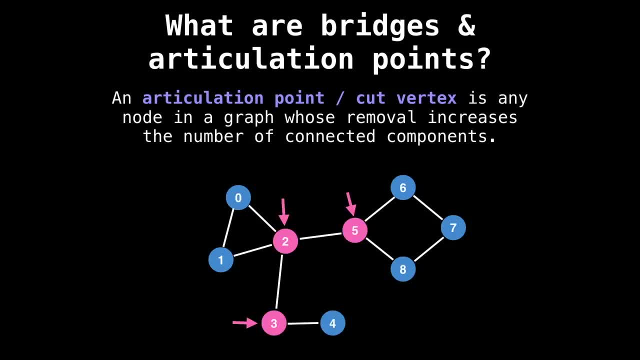 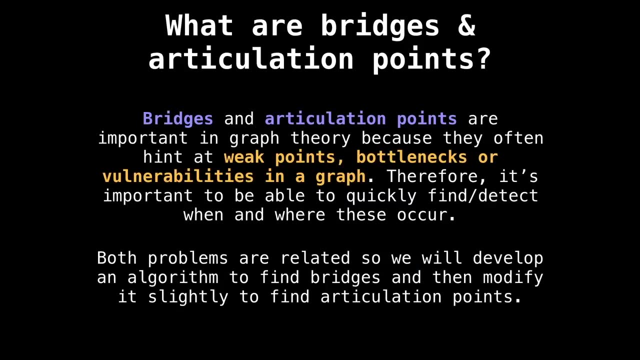 components. As an example, on this graph there would be three articulation points, since removing any of these vertices will divide the graph in two. As we start to think more about bridges and articulation points, we realize how important they are in graph theory, In real world situations. 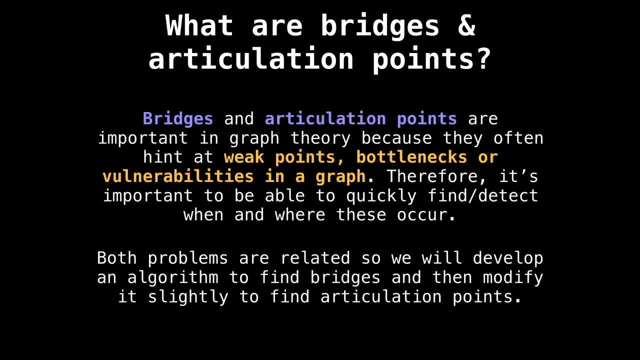 bridges and articulation points often hint at bottlenecks Or vulnerabilities or weak points in a graph. Therefore, it's important to be able to quickly find and detect where these occur. We'll begin by investigating how to find bridges and then slightly modify that algorithm to also find articulation points In the simplest way. 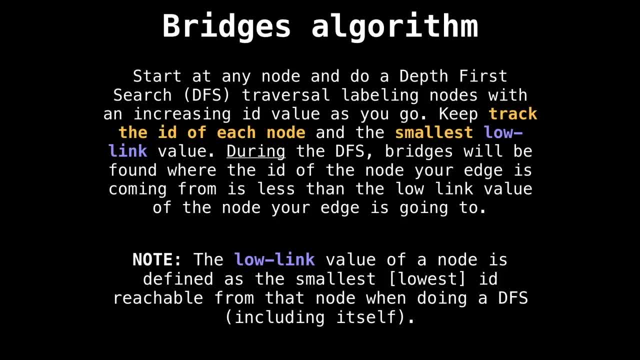 I can explain it. this is the algorithm we'll be following to find bridges. We'll start by creating a bridge in an undirected graph. First, start at any node in the graph and begin doing a depth. first, search, traversal, labeling nodes with an increasing ID as you. 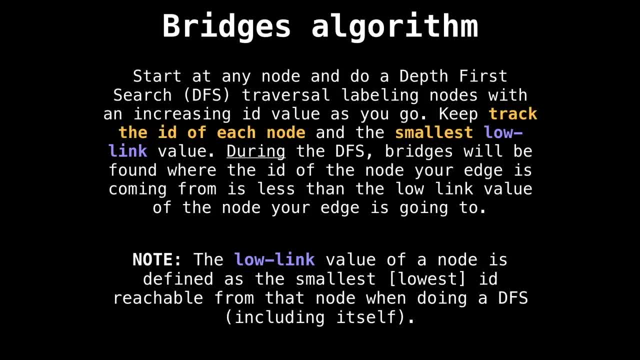 encounter them. During the traversal, you will need to keep track of two variables. The first is the nodes ID, which I just mentioned, and the other is the nodes low link value. During the depth first search, bridges will be found where the ID of the node your edge. 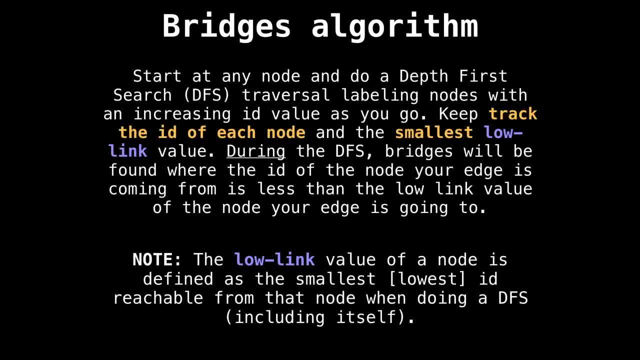 is coming from Is less than the low link value of the node the edge is going to. the low link value of a node is defined as the smallest node ID reachable from the node you're currently at when doing the depth first search, including the ID of the node itself. This is an interesting 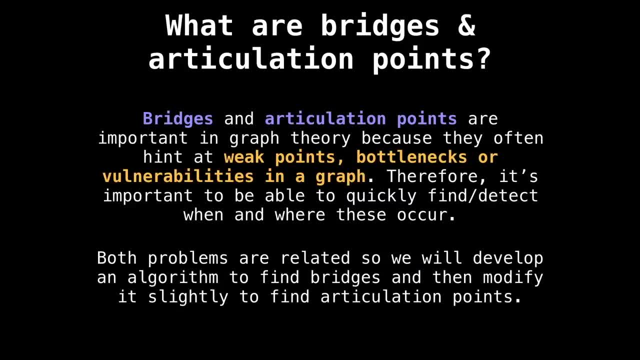 will divide the graph in two. As we start to think more about bridges and articulation points, we realize how important they are in graph theory. In real world situations, bridges and articulation points often hint at bottlenecks or vulnerabilities or weak. 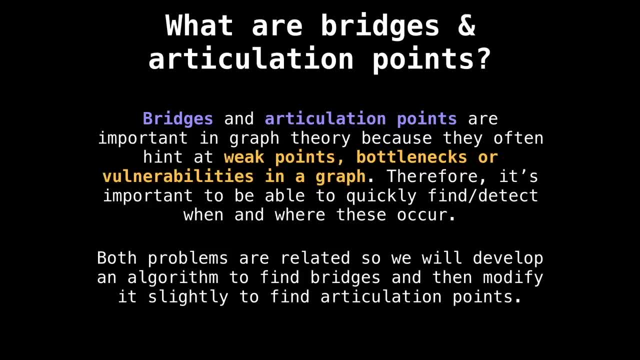 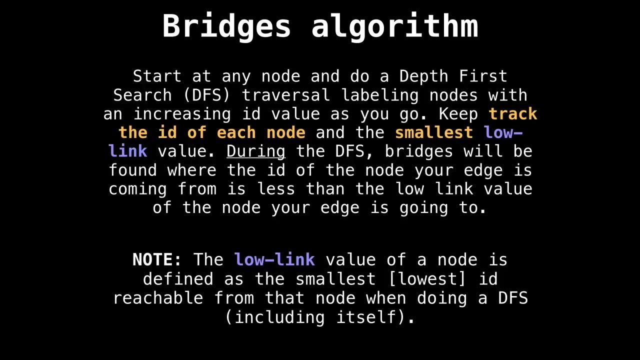 points in a graph. Therefore, it's important to be able to quickly find and detect where these occur. We'll begin by investigating how to find bridges and then slightly modify that algorithm to also find articulation points. In the simplest way I can explain it, this is the algorithm we'll 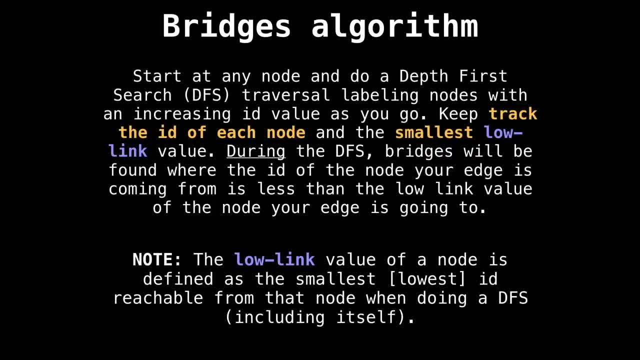 be following. to find bridges in an undirected graph, First start at any of these bridges. Then start at any node in the graph and begin doing a depth first search, traversal labeling nodes with an increasing ID as you encounter them During the traversal. you will need 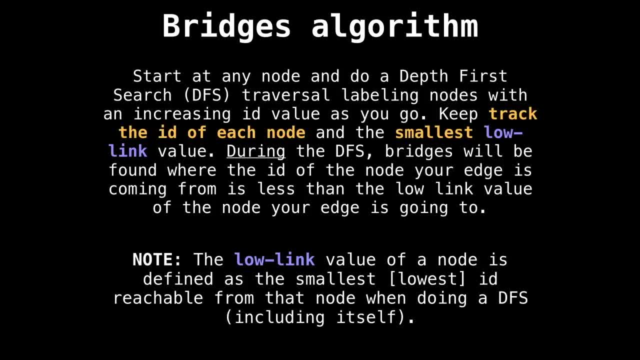 to keep track of two variables. The first is the nodes ID, which I just mentioned, and the other is the nodes low link value. During the depth first search, bridges will be found where the ID of the node your edge is coming from is less than the low link value of the 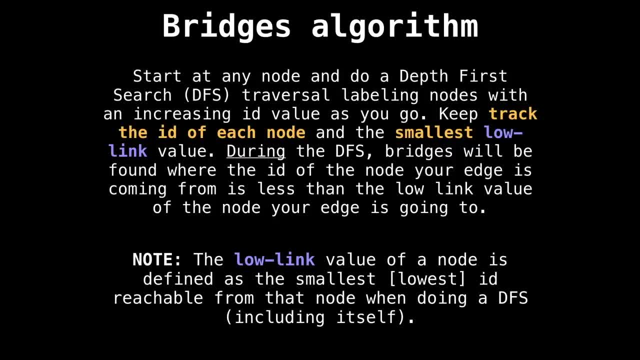 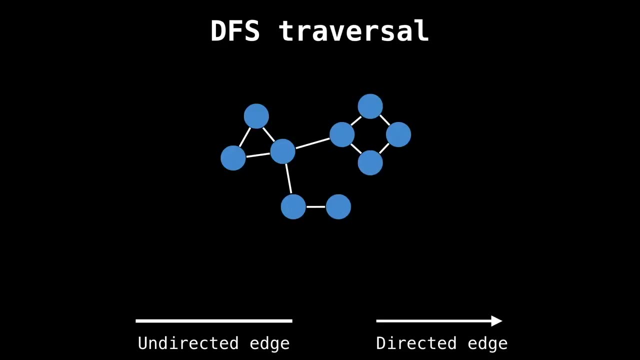 node. The low link value of a node is defined as the smallest node ID reachable from the node you're currently at when doing the depth first search, including the ID of the node itself. This is an interesting concept. we'll get back to later. For now, let's look at an example. 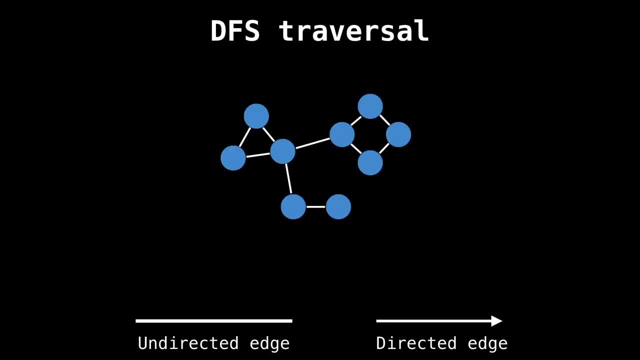 Suppose we have the following graph: we've been looking at And we want to find out where all the bridges are, Let's begin our depth first search on the node at the top left corner. As we do our depth first search, we're going to label each node with a unique ID, which. 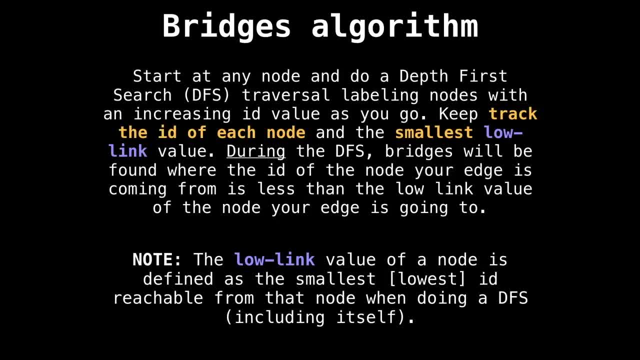 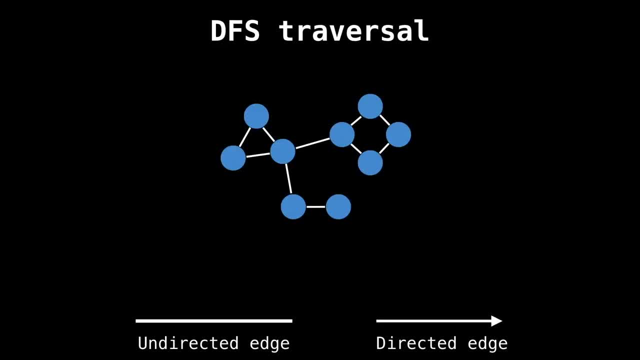 concept we'll get back to later. For now, let's look at an example. Suppose we have the following graph We've been looking at and we want to find out where all the bridges are. let's begin our depth first. search on the node at the top left corner, As we do. our depth first. 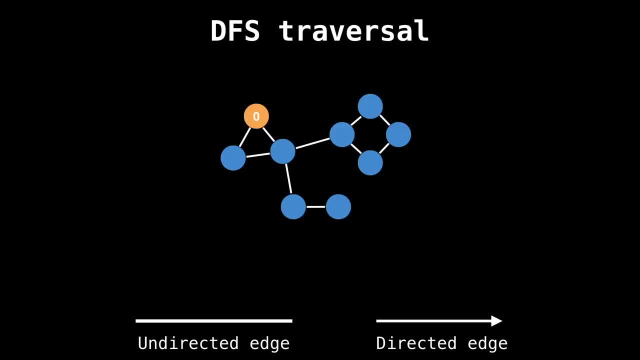 search. we're going to label each node with a unique ID which I will place inside the node. I will also mark nodes which are visited as yellow and the nodes which are blue as unvisited. So let's finish off our depth first search. 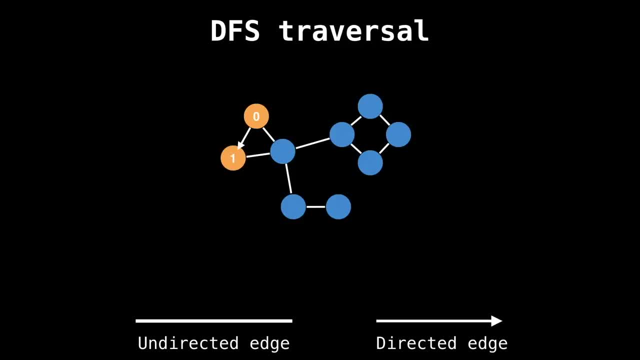 So explore all nodes, transforming undirected edges into directed ones and marking off edges or nodes rather as visited. So that would conclude our depth first search. I want to take a moment to think about what all the low link values are. For example, the value of a node is defined as the smallest ID reachable from that node. 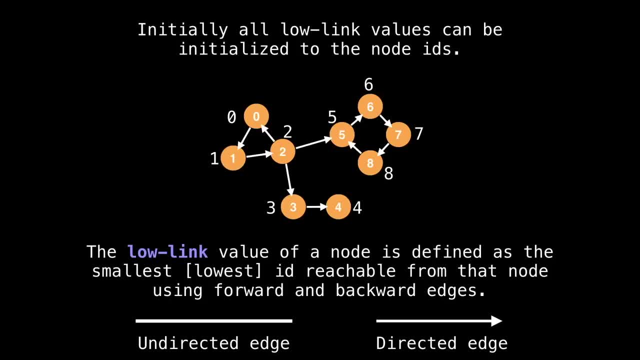 For now, initialize all low link values to be equal to each nodes ID. I place a low link value of each node on the exterior of that node. If you inspect node one, you will notice that its low link value should be zero because there exists a path of edges going from node. 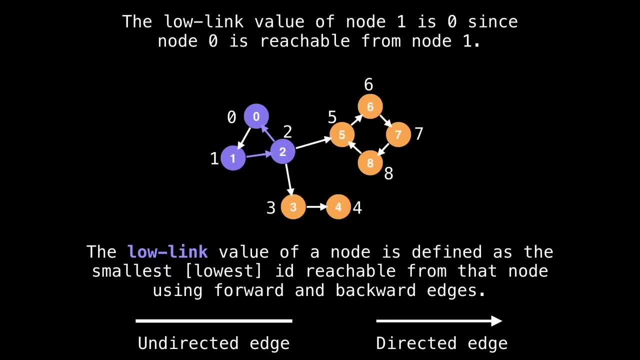 one to node zero and node zero has an ID of zero, So we can update node ones low link value to zero. Similarly, node twos low link value should also be zero, because node two to node zero There exists a path. However, nodes three, four and five are already at their optimal. 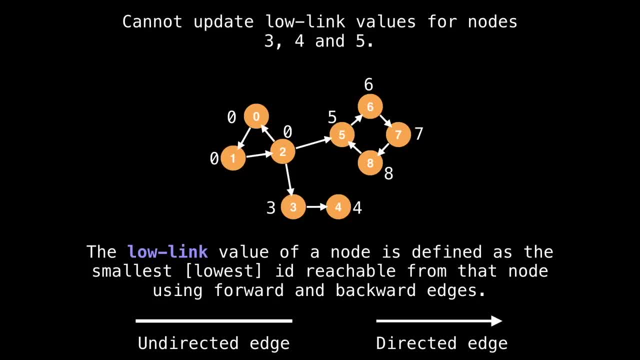 low link value because there's no other node they can reach with a lower ID. However, node six is low link value can be updated to five, since there is a path from node six to node five Via these sequence of nodes. So let's take a look at our depth. first search. 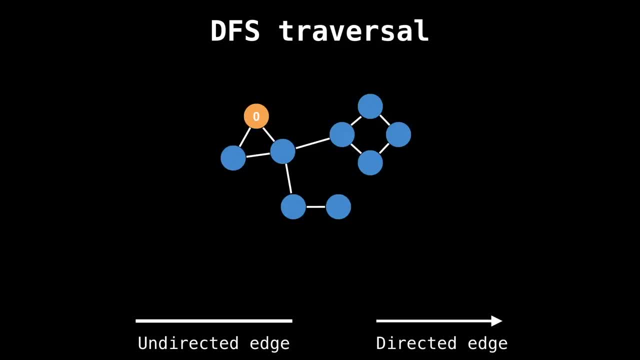 I will place inside the node. I will also mark nodes which are visited as yellow and the nodes which are blue as unvisited. So let's finish off our depth first search. So explore all nodes, Forming undirected edges into directed ones and marking off edges or nodes rather as visited. 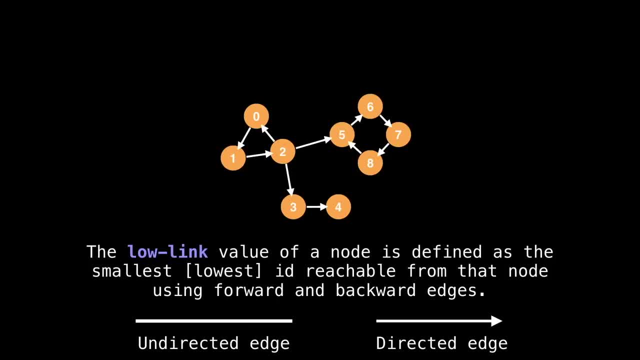 So that would conclude our depth first search. I want to take a moment to think about what all the low link values would be for these nodes. As a result reminder, the low link value of a node is defined as the smallest ID reachable from. 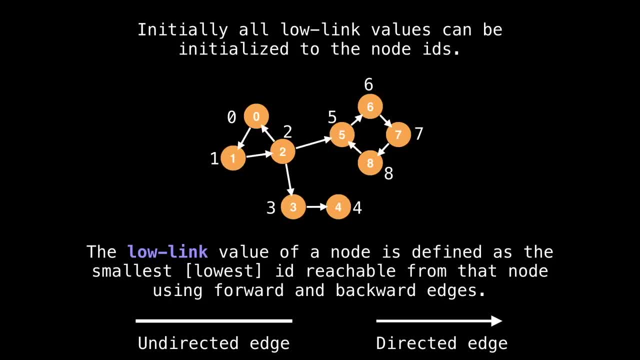 that node. For now, initialize all low link values to be equal to each nodes ID. I place the low link value of each node on the exterior of that node. If you inspect node one, you will notice that it's low link value should be zero because 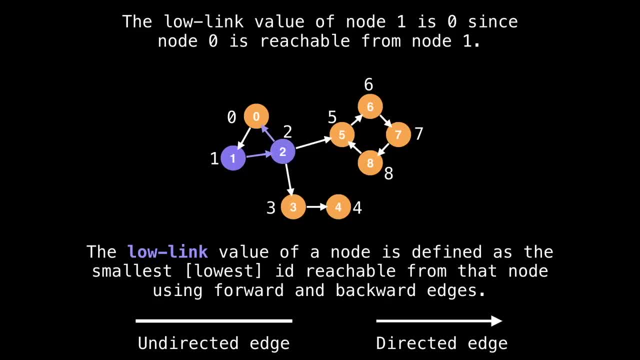 there exists a path of edges going from node one to node zero, and node zero has an ID of zero, So we can update node one's low link value to zero. Similarly, node twos low link value should also be zero, because node two to node zero, there exists a path, However. 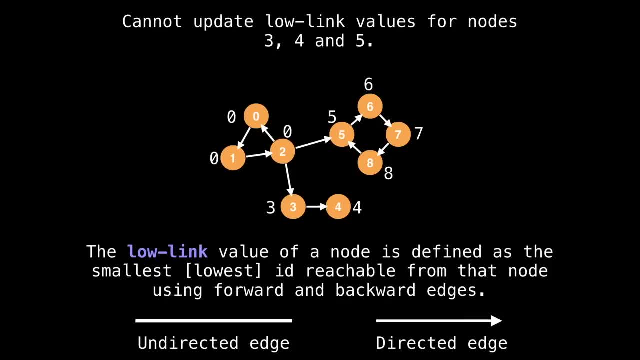 nodes three, four and five are already at their optimal low link value because there's no other node they can reach with a lower ID. However, node six is low link value can be updated to five since there is a path from node six to node five via these sequence of edges And we can also update 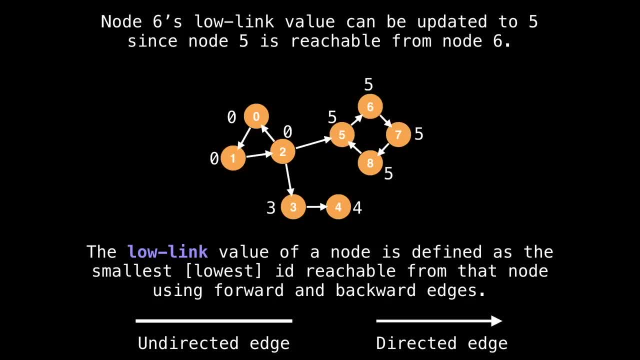 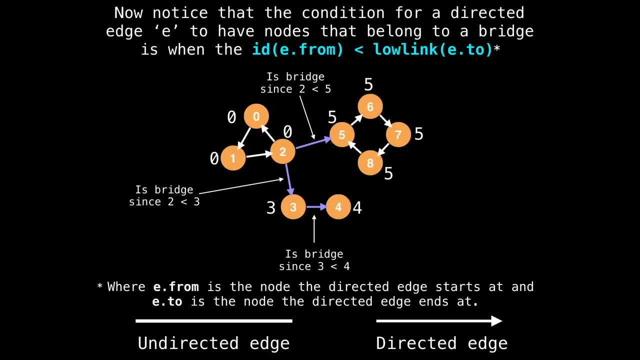 node seven and eight, low link value by the same logic. So, in general, when we look at all the directed edges we have traversed, the ones which form bridges in our graph are the ones where the ID of the node you started. that is, less than the low link value of the 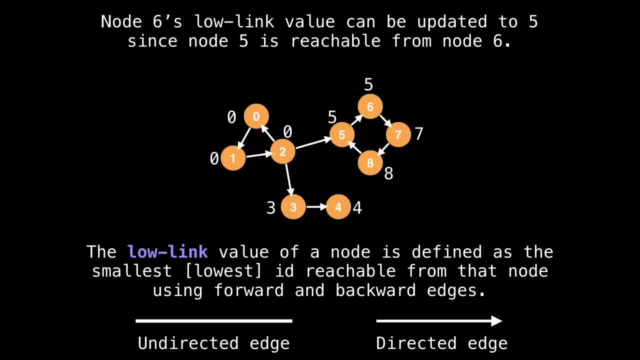 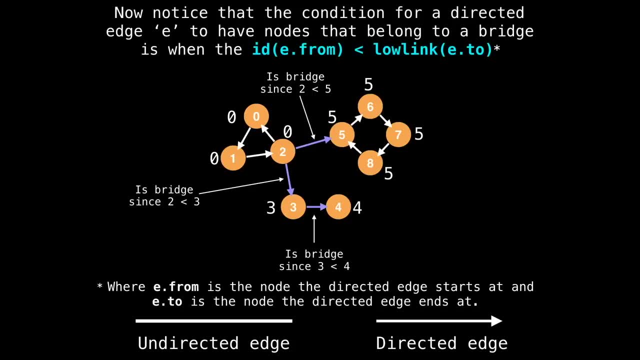 So let's take a look at our depth, first search Edges, And we can also update node seven and eight, low link value, by the same logic. So in general, when we look at all the directed edges, we have traversed, the ones which form: 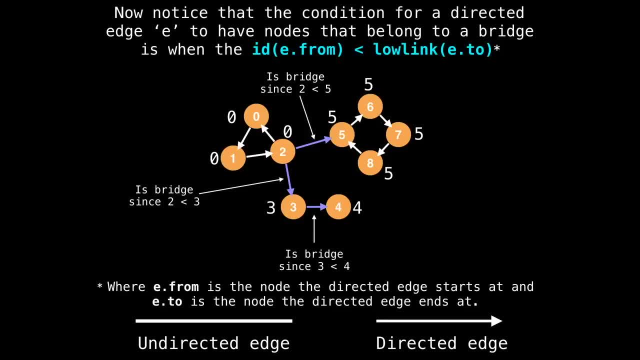 bridges in our graph are the ones where the ID of the node you started, that is less than the low link value of the node. you're going to take a moment to think about why this is true. Let's of where these bridges actually occur. In each instance, the idea of the node where 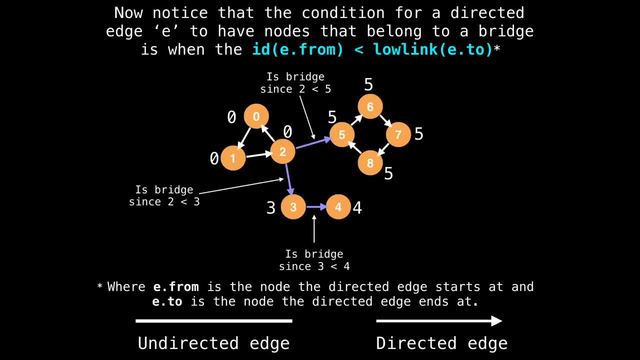 the directed edge started at is less than the loading value of the node. it's going to rephrasing that in another way. It means there was no edge connecting back to the start of the component, which is really the definition of what a bridge is. Otherwise, if there wasn't, 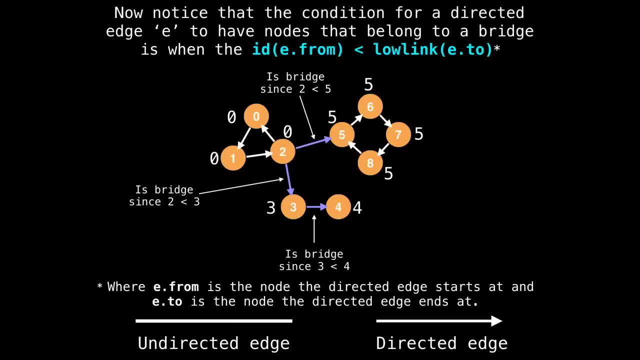 edge connecting backwards to the start of the component. the loading value of where the edge is pointing to would be at least as low as the ID of the node you started at, because it would be reachable, For example, if I have an edge from node eight to node. 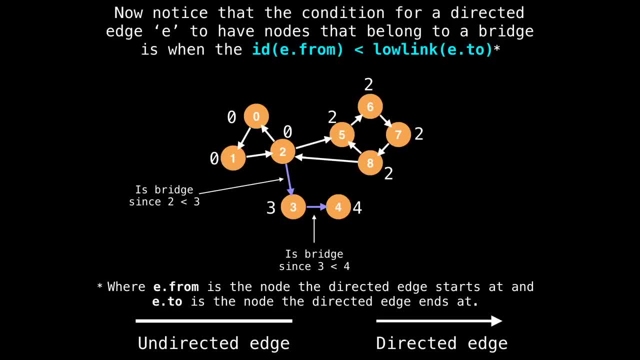 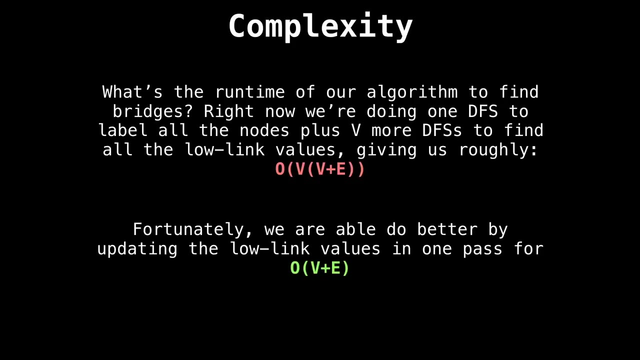 two. suddenly, the edge from node two to node five is no longer a bridge, because the loading value on node five got updated to two and our bridge property, highlighted in teal, no longer holds. Let's take an aside and think of the time complexity of the algorithm I just presented. 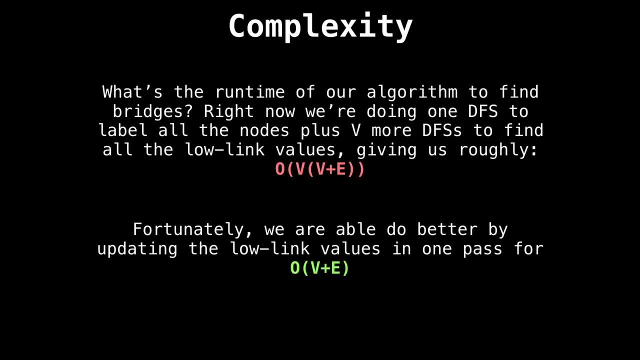 Right now we're doing a depth first search to label all the nodes plus v. more depth first searches to find all the low length values for roughly v times v plus v plus v plus e. in the worst case, if you're really pessimistic and careless about your programming. 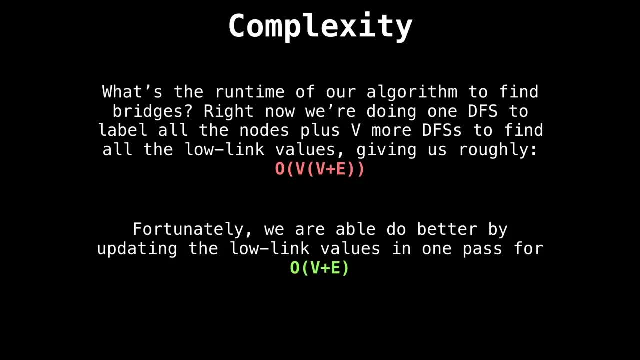 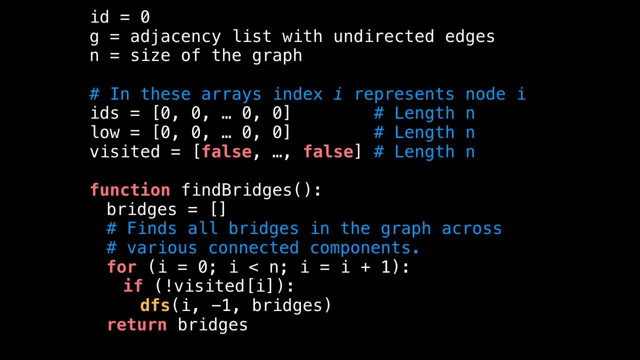 Luckily, however, we can do much better than this and instead update all the loading values in one pass for a linear time- complexity- Let's look at some pseudocode on how to do this- and linear time. I'll show you some actual code in the video that follows. You might. 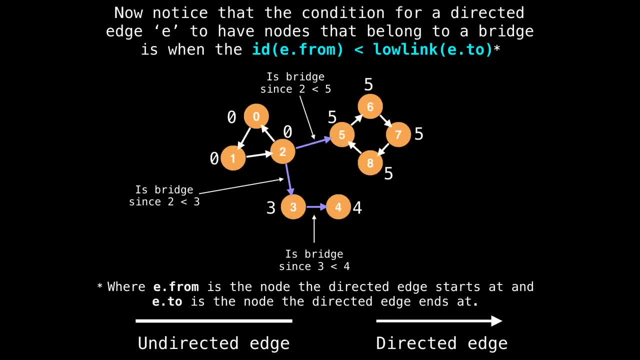 node. you're going to take a moment to think about why this is true. Let's look at where these bridges actually occur. In each instance, the ID of the node where the directed edge started at is less than the low link value of the node. it's going to rephrasing that in another way. It means 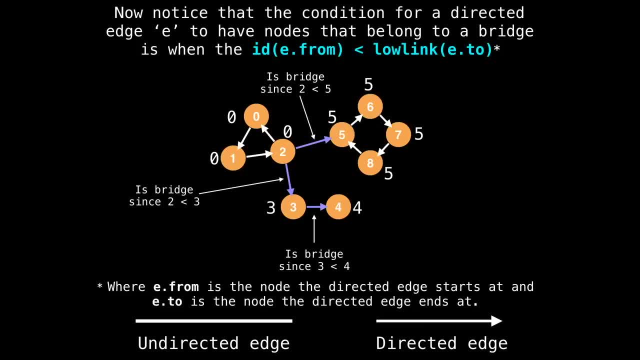 there was no edge connecting back to the start of the component, which is really the definition of what a bridge is. Otherwise, if there was an edge connecting backwards to the start of the component, the low link value of where the edge is pointing to would be at least as low as the ID of the 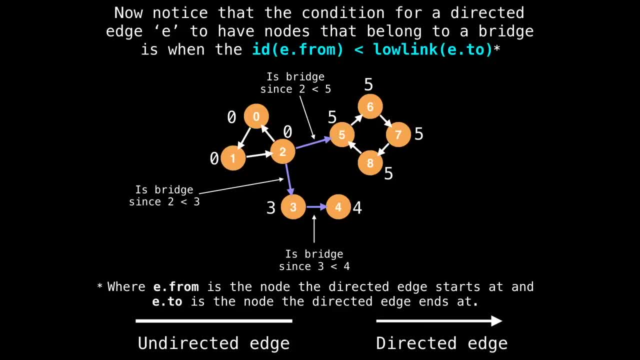 node. you started that because it would be reachable. For example, if I have an edge from node eight to node two, suddenly the edge from node two to node five is no longer a bridge, because the low link value on node five got updated to two And our bridge, our. 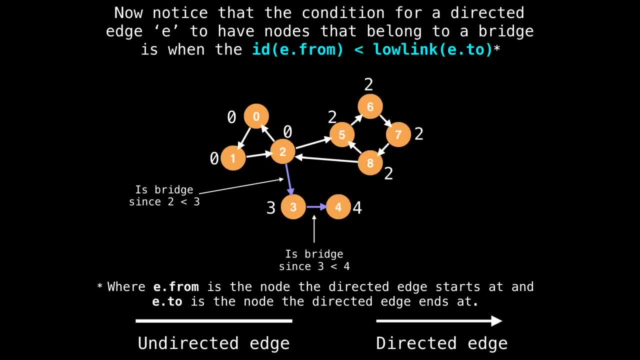 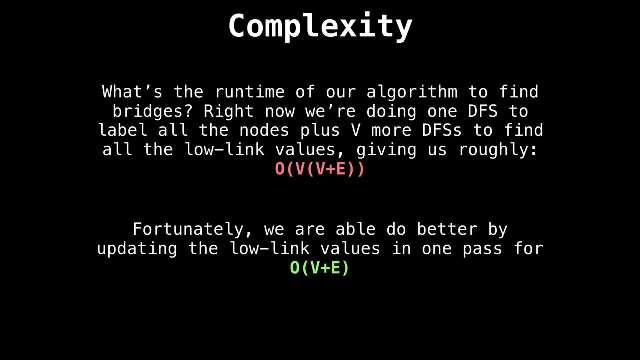 property highlighted in teal no longer holds. Let's take an aside and think of the time complexity of the algorithm I just presented. Right now we're doing a depth first search to label all the nodes plus v. more depth first searches to find all the low length values. 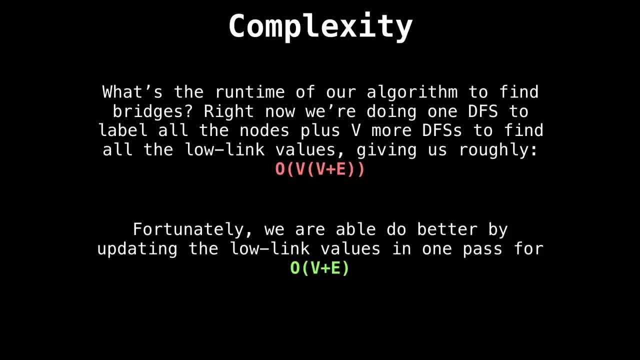 for roughly v times- v plus e in the worst case- if you're really pessimistic and careless about your programming. Luckily, however, we can do much better than this and instead update all the loading values in one pass for a linear time complexity. Let's look at. 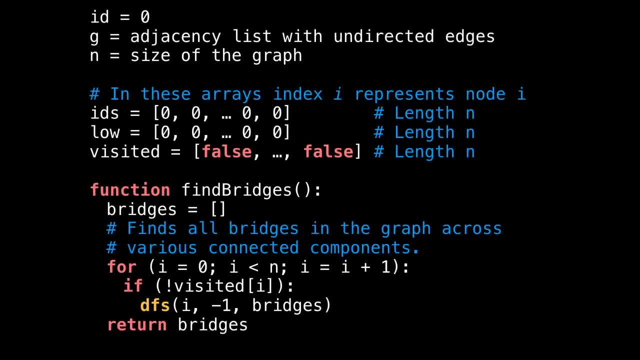 some pseudocode on how to do this in linear time. I'll show you some actual code in the video that follows, But let's get started. In the global, or class scope, I define three variables. The first is ID, which I use to label each. 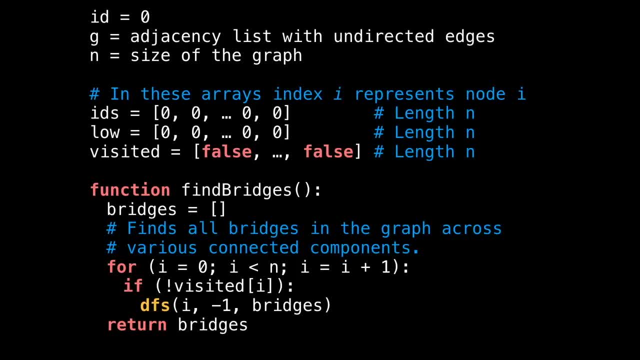 those. But let's get started. In the global or class scope, I define three variables. The first is ID, which I use to label each node with a unique ID number. Then I have an undirected graph, G. The last is n, which is the number of nodes in the graph Following. 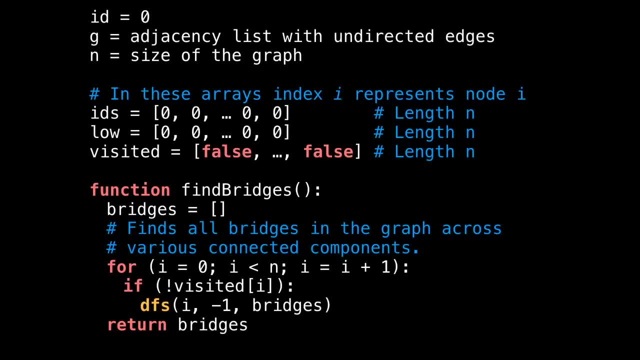 the top level variables are three arrays which track information about each node in the graph. index i in each of these arrays represents node i in the graph. So the first array tracks the ID of node i. The second array tracks the low link value of node i. 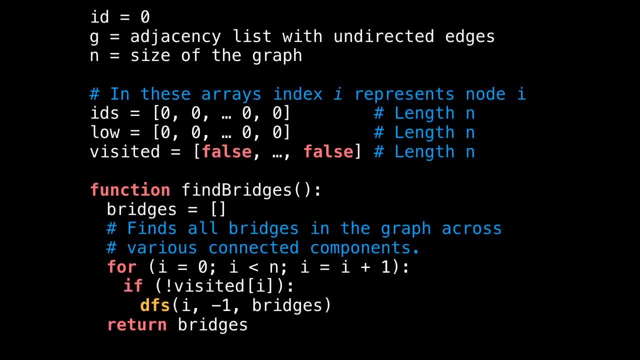 And the visitor array keeps track of whether or not we have visited node. i. Moving on, the fine bridges function is what a actually finds the bridges In the method I iterate over all the nodes which have not yet been visited by our depth first search. This is to ensure that we find all the bridges. 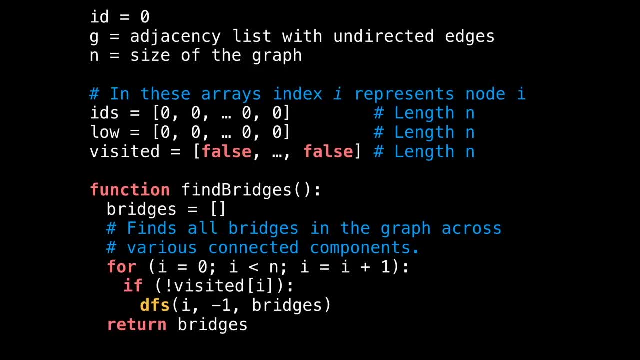 in our graph, even if our graph consists of multiple connected components. Let's dive into the depth. first, search method, which is where the real work is happening. The first argument is the current node you're at, which is node i. then is the parent node, which I set to minus one because there is no previous node. And last, 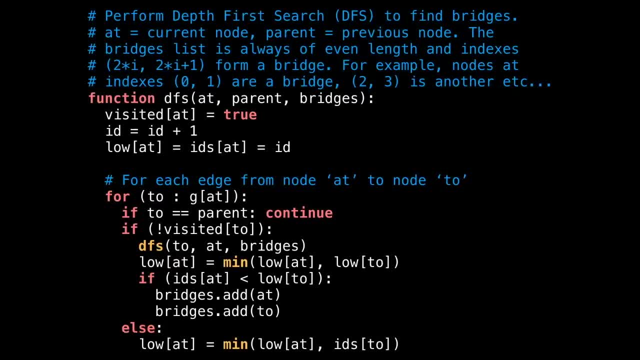 is the bridges array which we are populating. So here we are in the depth. first search method itself. The arguments to the method are just as I described them to you. The first variable is: at which is the current node ID. then comes parent, the previous node ID and the 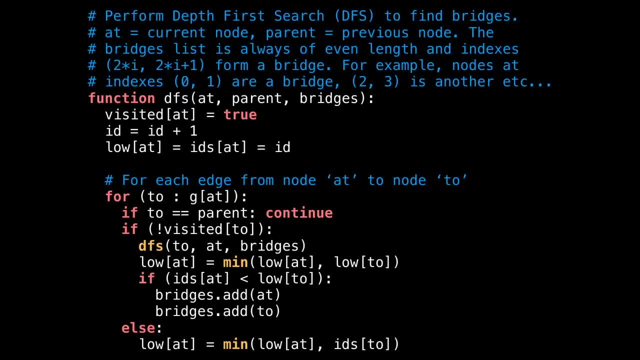 array bridges which stores pairs of nodes which form bridges in a flat array. In the first three lines of the method I simply do some housekeeping stuff, which is mark the current node as visited, increment the ID value variable and assign the current node. 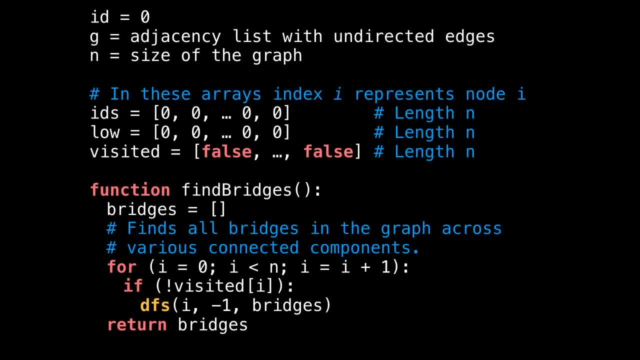 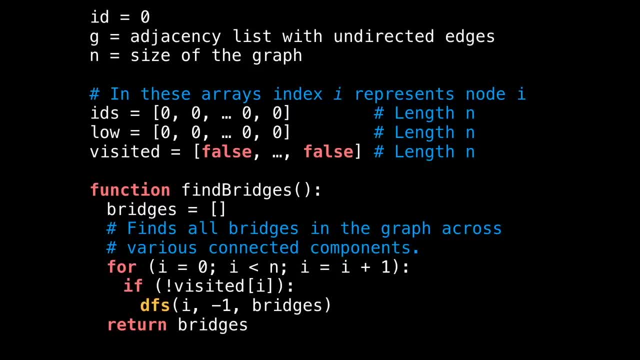 following the top level variables are three arrays which track information about each node in the graph. Index i in each of these arrays represents node i in the graph. So the first array tracks the ID of node i. The second array tracks the low link value of 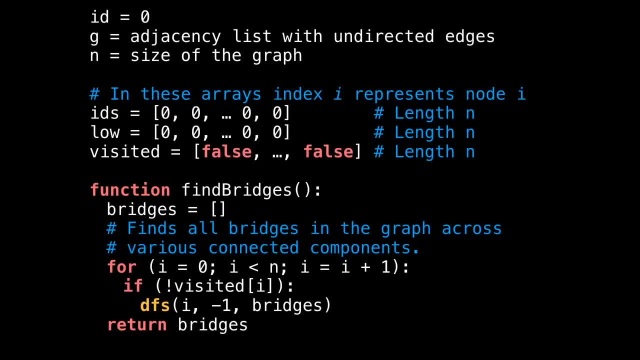 node i and the visitor array keeps track of whether or not we have visited node i. Moving on the fine bridges function is what actually does the job. So in this case I'm going to actually find the bridges In the method I iterate over all the nodes which have not. 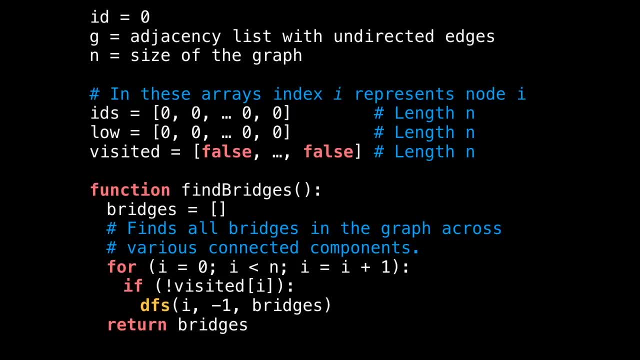 yet been visited by our depth first search. This is to ensure that we find all the bridges in our graph, even if our graph consists of multiple connected components. Let's dive into the depth first search method, which is where the real work is happening. The first: 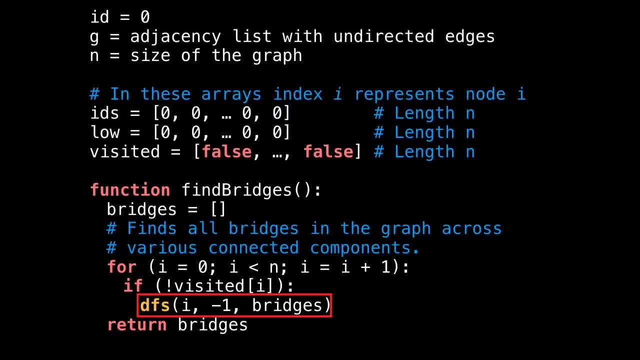 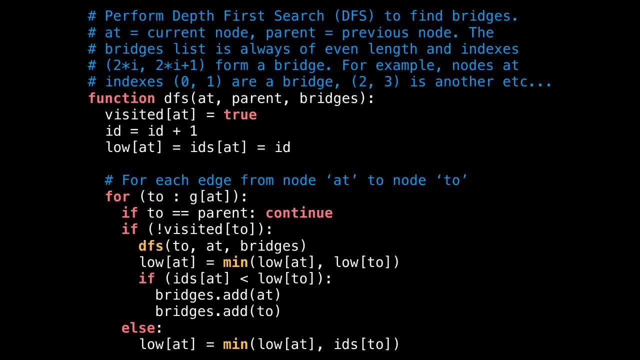 argument is the current node you're at, which is node i, then is the current node i, And then is the parent node, which I set to minus one because there is no previous node, And last is the bridges array which we are populating. So here we are in the depth. first search method. 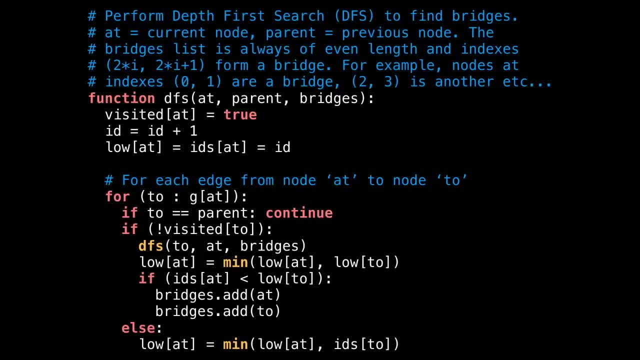 itself. The arguments to the method are just as I described them to you. The first variable is: at which is the current node ID. then comes parent, the previous node ID and the array array bridges, which stores pairs of nodes which form bridges in a flat array, In the 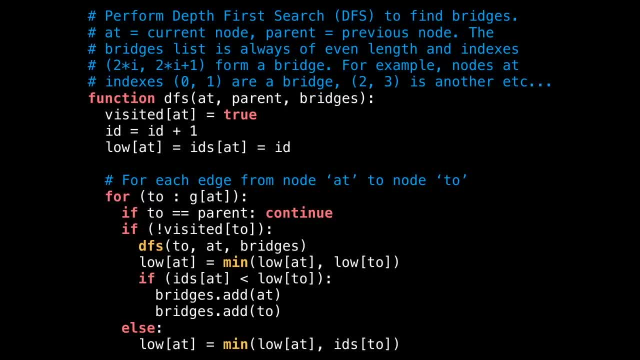 first three lines of the method. I simply do some housekeeping stuff, which is mark the current node as visited, increment the ID value variable and assign the current node to have a default ID and low link value. Then we get into the actual depth. first search: 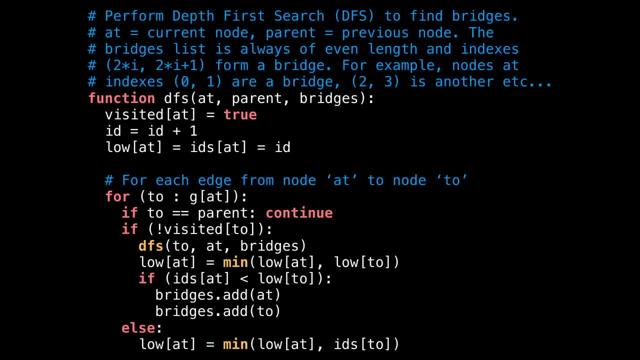 to have a default ID and low link value. Then we get into the actual depth, first search traversal bit. So we iterate over each edge from the node we're at and attempt to go to each node, which I've labeled two. Since this is an undirected graph, there is bound to be an edge that directly returns. 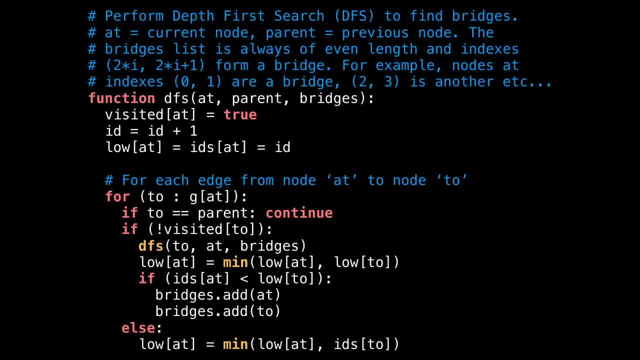 to the node we were just previously at, which is the parent node, which we want to avoid doing. so we continue on those cases. If the next node we're going to is not visited, we're going to have a default ID. Then we recursively call the depth first, search method, The two 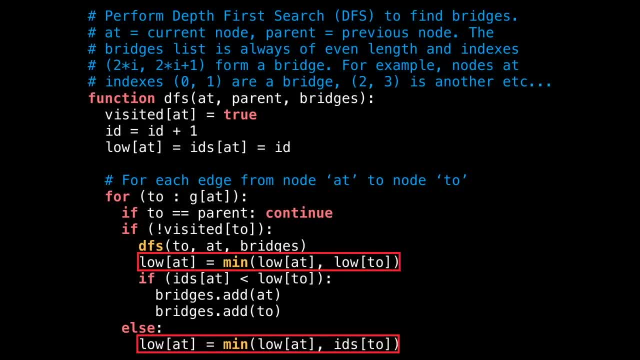 key lines in this method are the min functions, which differ ever so slightly. The first one happens on the callback and is what propagates the low link values, While the second one is when you try to visit an already visited node which has a chance of having a lower. 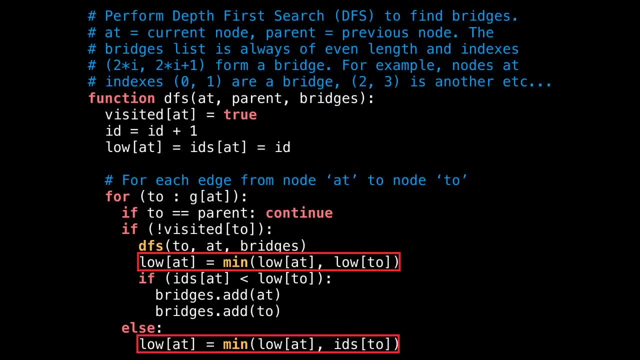 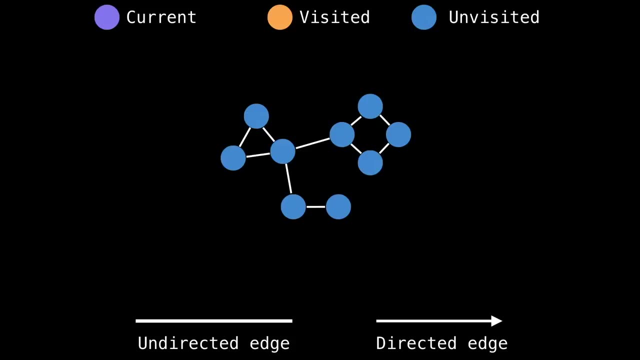 ID than your current low link value. Okay, then the last bit just checks if our bridge condition is met and appends a pair of node IDs to the bridges array. All right, now let's look at an example of all this in action. 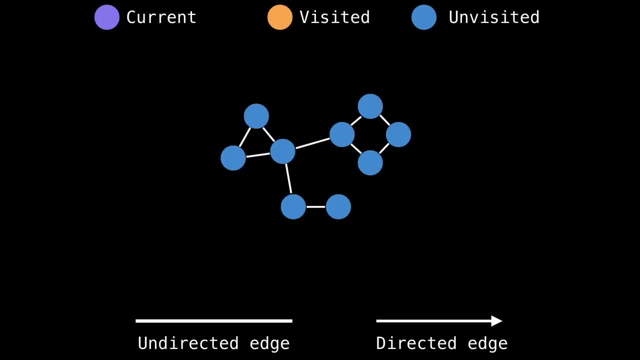 Suppose we have the following graph again and we start our depth first search somewhere, Let's start at node zero and explore from there. Okay, so now is the first instance of something interesting happening. We're trying to visit an already visited node, Since node two is able to reach node zero from where it is. 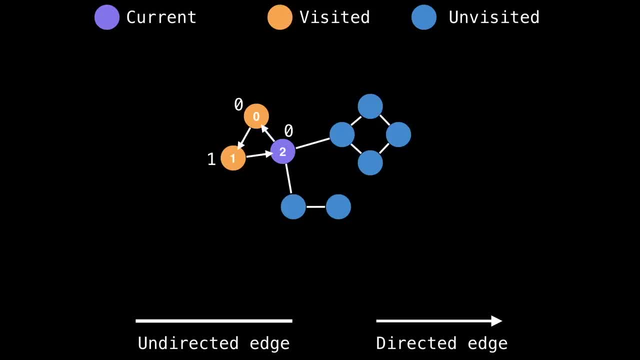 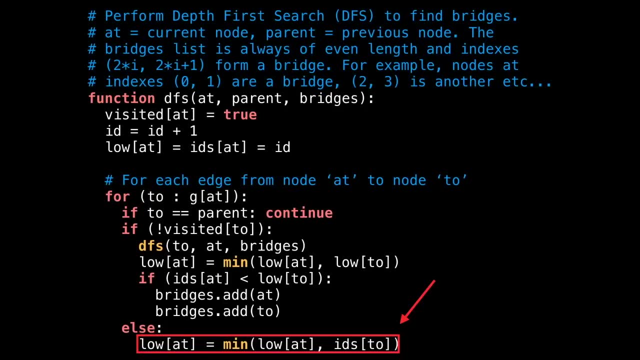 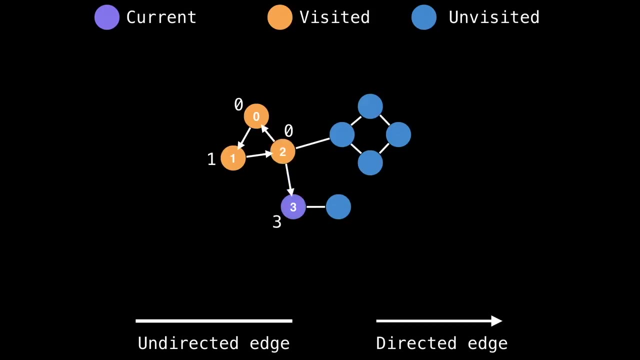 we can update its low link value. And that was the second min statement executing, Continuing on our depth: first search, which takes us downward, Okay, and now we get to explore the other branch we have not visited Again. we have an edge. 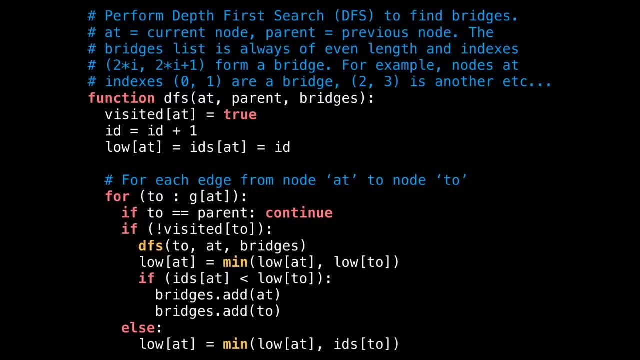 traversal bit. So we iterate over each net edge from the node we're at and attempt to go to each node which I've labeled to, Since this is an undirected graph. there is bound to be an edge that directly returns to the node we were just previously at, which is the parent node, which we want to avoid doing. 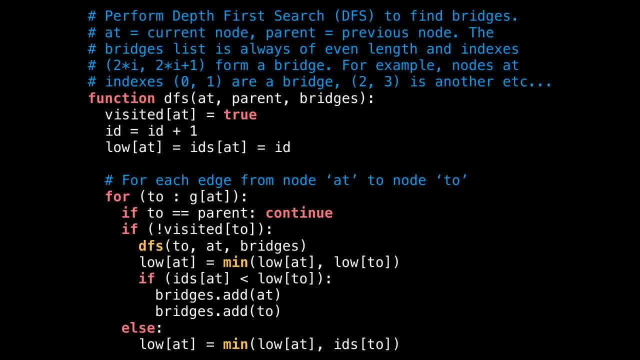 So we continue on those cases. If the next node we're going to is not visited, then we recursively call the depth first search method. The two key lines in this method are the min functions, which differ ever so slightly. The first one happens on the callback and 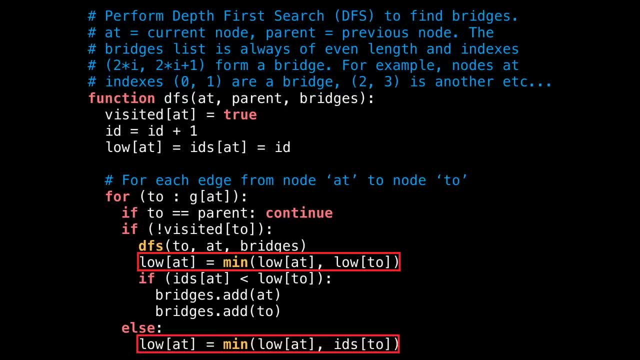 is what propagates the low link values, While the second one is when you try to visit an already visited node which has a chance of having a lower ID than your current low link value. So then the last bit just checks if our bridge condition is met and appends a pair of node. 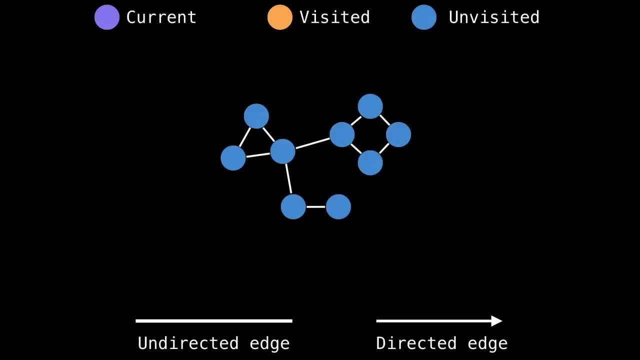 IDs to the bridges array. All right, now let's look at an example of all this in action. Suppose we have the following graph again and we start our depth first search somewhere. Let's start at node zero and explore from there. Okay, 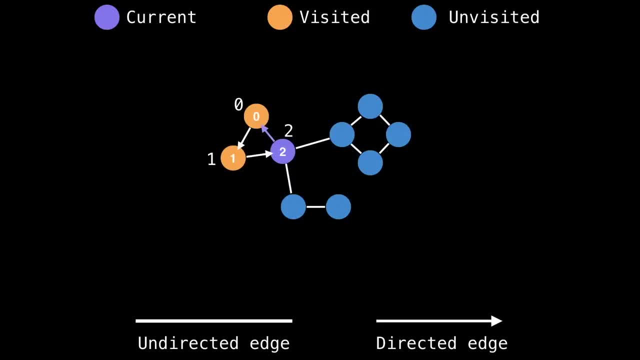 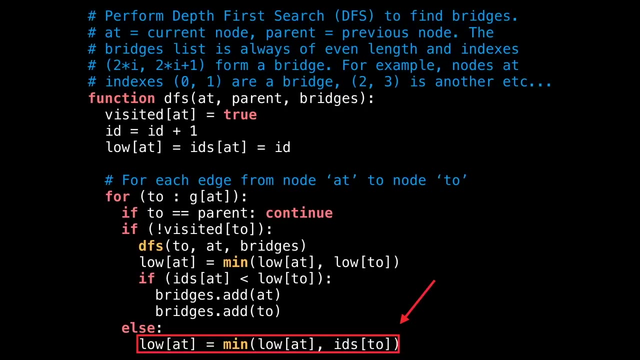 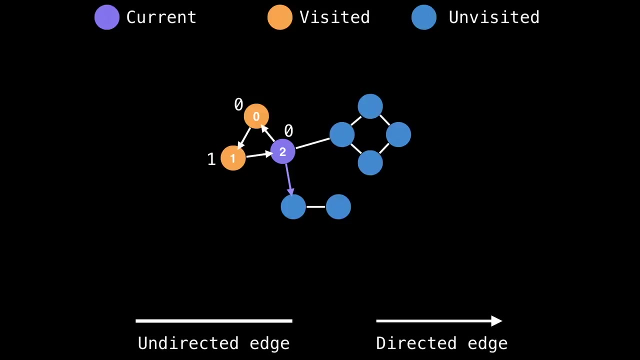 so now is the first instance of something interesting happening. We're trying to visit an already visited node. Since node two is able to reach node zero from where it is, we can update its low link value. And that was the second min statement. executing Continuing. 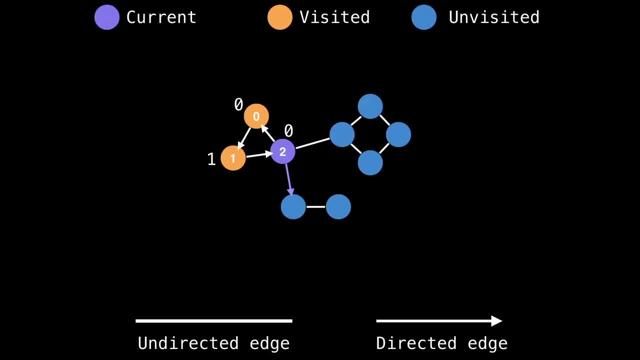 on our depth first search which takes us downward, And now we get to explore the other branch we have not visited Again. we have an edge which reaches out to find a node with a lower ID, So we need to update our low link value. 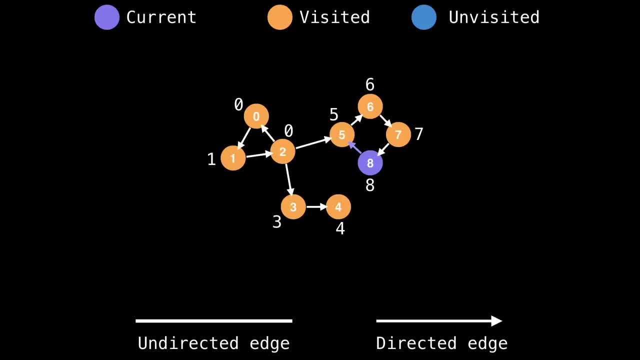 which reaches out to find a node with a lower ID. So we need to update our low link value for the current node, which is node eight. Now we can update node seven's low link value to five On the callback All back of the depth first search method. This is an instance of the first min function. 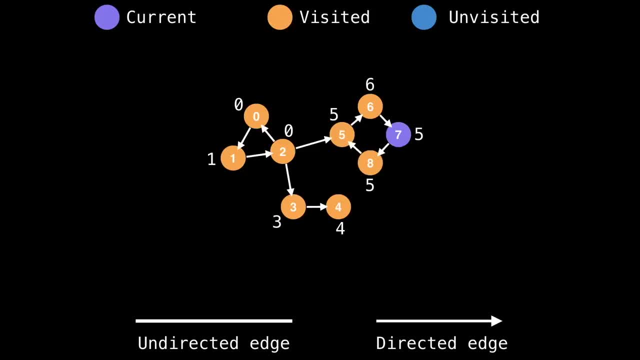 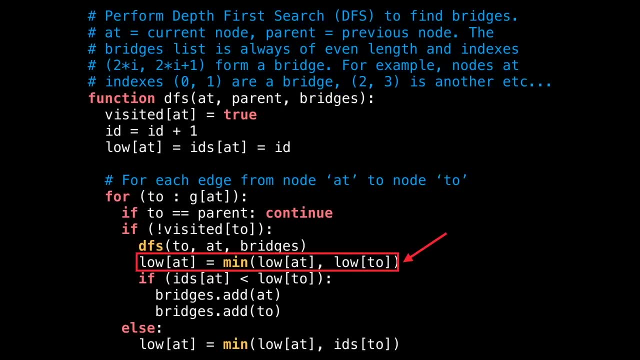 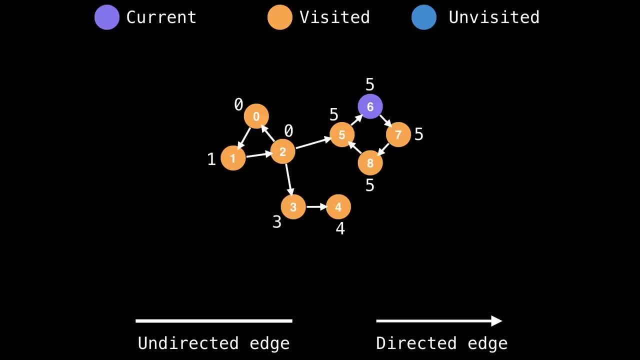 actually doing something. Just to put everything into context, The red box is a line which was just invoked And now that statement we just saw it gets executed for every node on the callback, all the way back to the root node. Okay, and now we have the same result as before, But we did it with just one pass, So again. 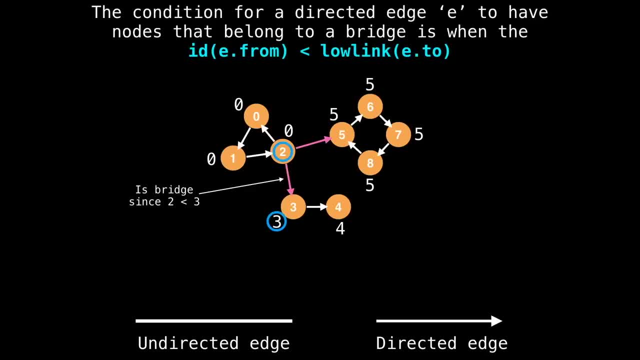 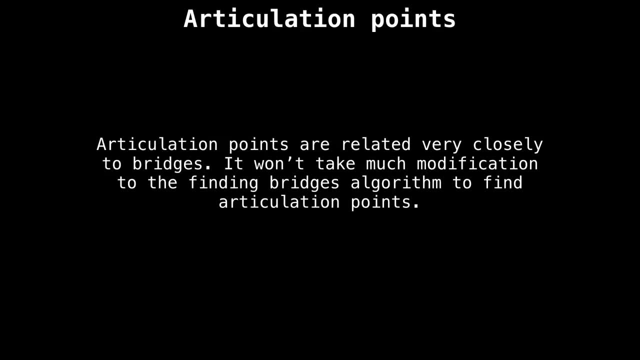 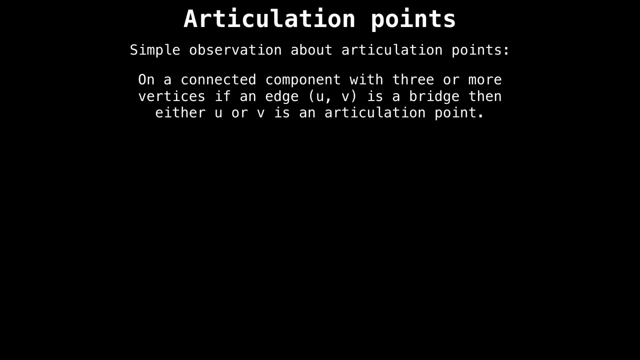 here are all the bridges that we found Perfect. Now let's move away from bridges and start discussing how we can find articulation points by modifying the allegory algorithm for bridges. A first simple observation we can make about articulation points is that: 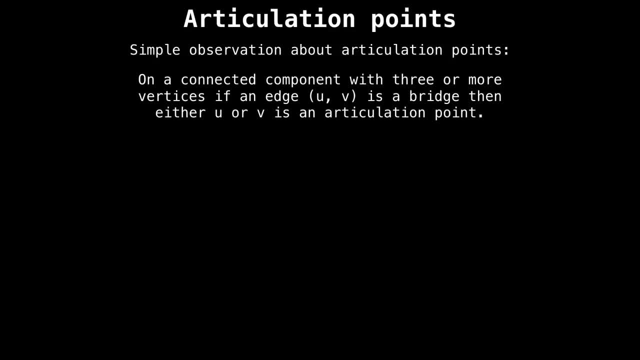 on a connected component with three or more vertices. if an edge UV is a bridge, then either U or V is an articulation point. This is a good starting point because it allows us to easily find where articulation points occur, For example: 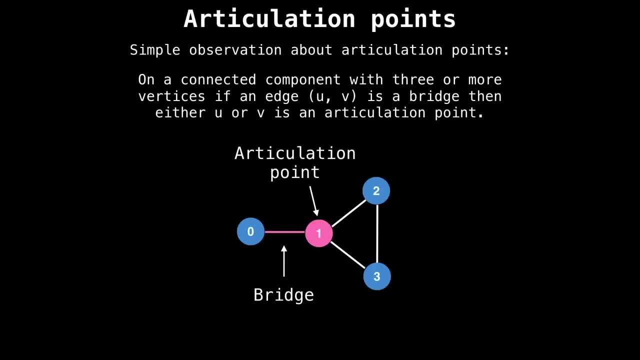 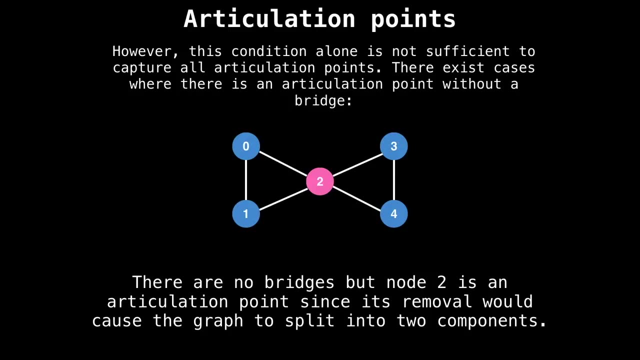 consider the following graph, you will notice that there is a bridge between nodes zero and one, meaning that either node zero or node one is an articulation point. Unfortunately, this condition is not sufficient to capture all articulation points. There exists cases. 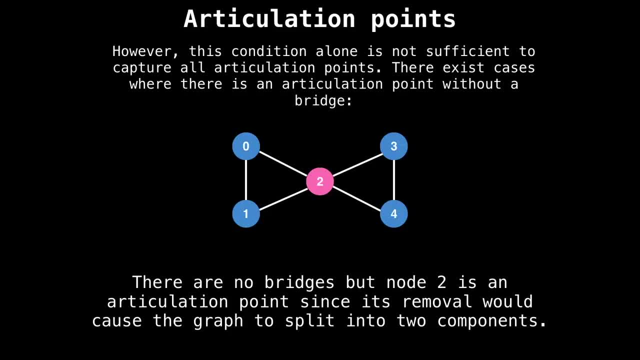 where there is an articulation point but there is no bridge nearby. For example, in the following graph, node two is an articulation point because its removal would cause the graph to split into two components. So the new question is: when do these cases occur? And the short answer: 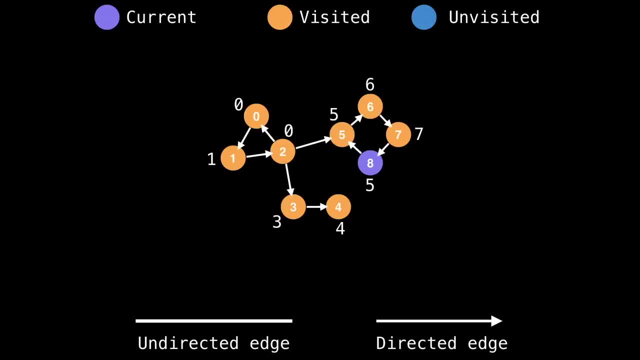 for the current node, which is node eight, Now we can update node seven's loading value to five on the callback And for that we're going to use the method And we're going to use the method of the depth first search method. This is an instance of the first min function actually doing something. 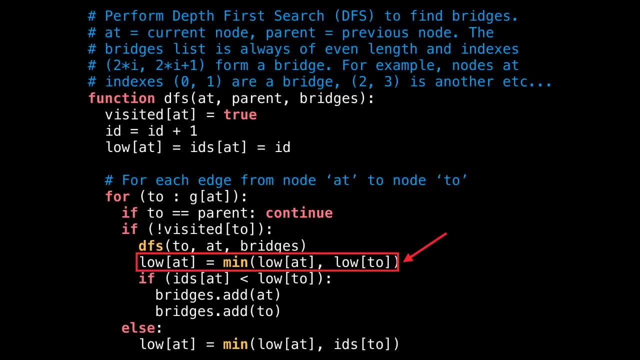 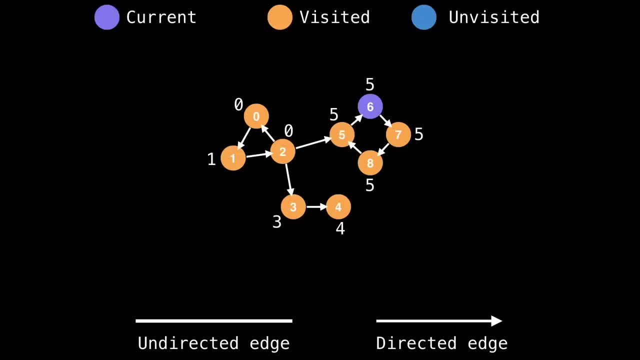 Just to put everything into context, The red box is the line which was just in the vote, And now that statement we just saw gets executed for every node on the callback, all the way back to the root node. Okay, And now we have the same result as before, but we did it with just one pass, So again, 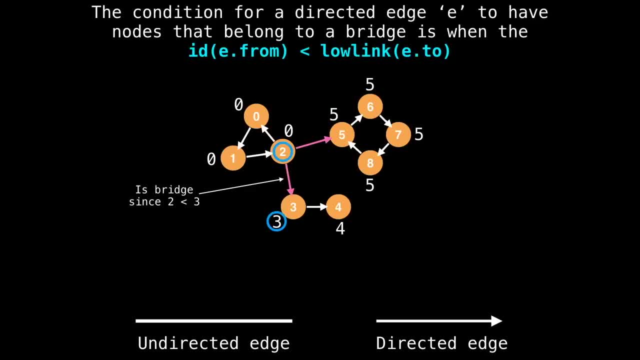 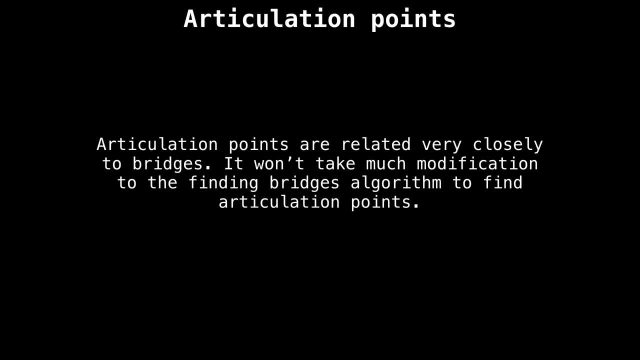 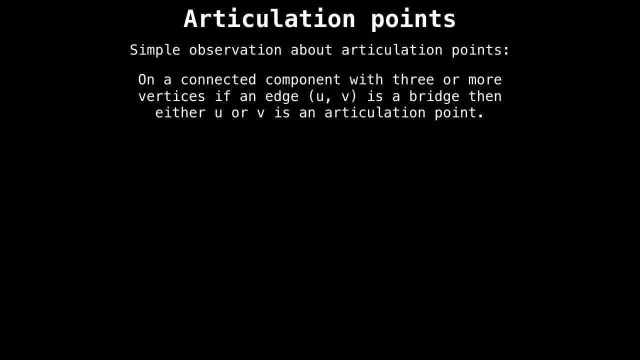 here are all the bridges that we found Perfect. Now let's move away from bridges and start discussing how we can find articulation points by modifying the algorithm for bridges. A first simple observation we can make about articulation points is that on a connected 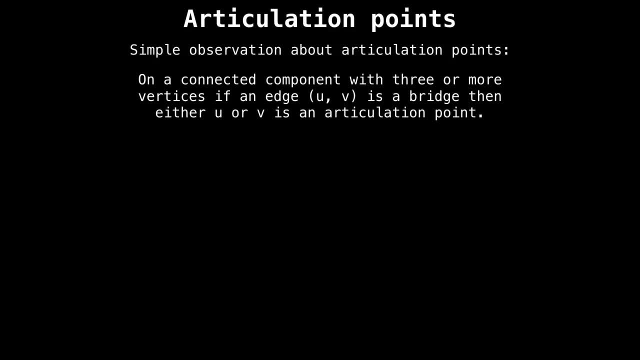 component with three or more vertices. if an edge UV is a bridge, then either U or V is an articulation point. This is a good starting point because it allows us to easily find where articulation points occur. For example, consider the following graph: you will notice. 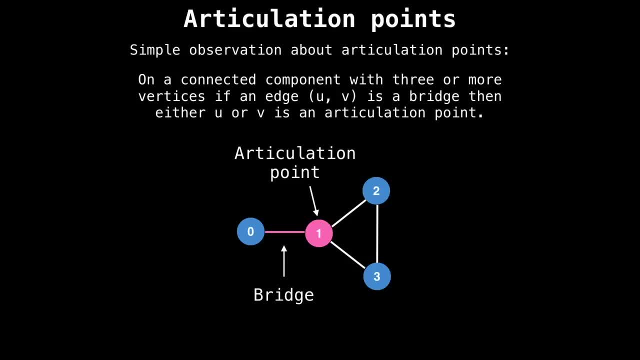 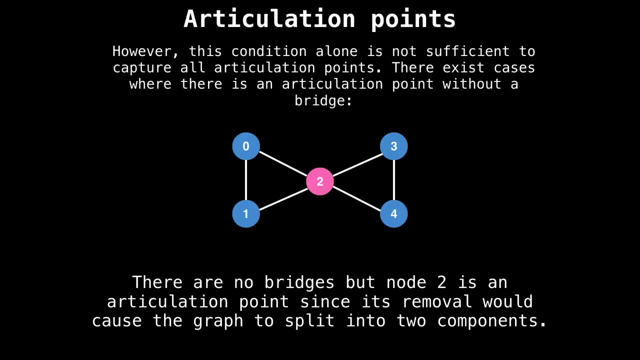 that there is a bridge between nodes zero and one, meaning that either node zero or node one is an articulation point. Unfortunately, this condition is not sufficient to capture all articulation points. There exists cases where there is an articulation point, but 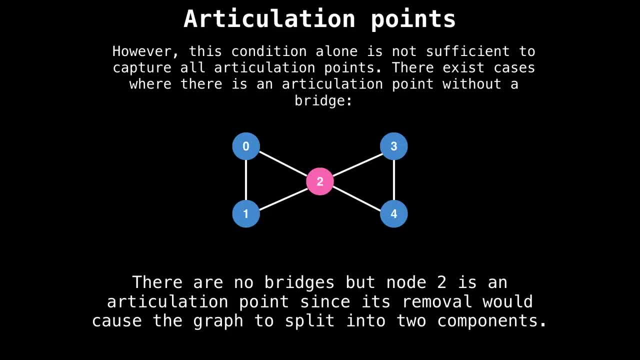 there is no bridge nearby. For example, in the following graph, node two is an articulation point, because its removal would cause the graph to split into two components. So the new question is: when do these cases occur? And the short answer is that it has to do. 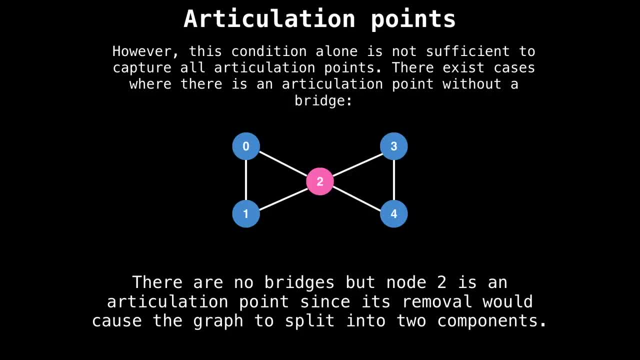 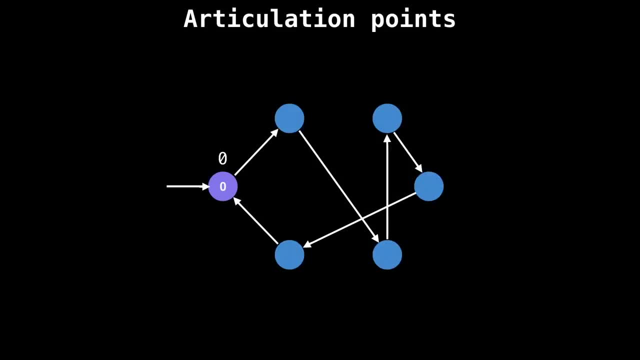 is that it has to do with cycles in the graph. To understand why, let's look at an example. Suppose you're traversing a graph and eventually you somehow arrive at node zero Initially. suppose you're traversing a graph and eventually you somehow arrive at node zero Eventually. 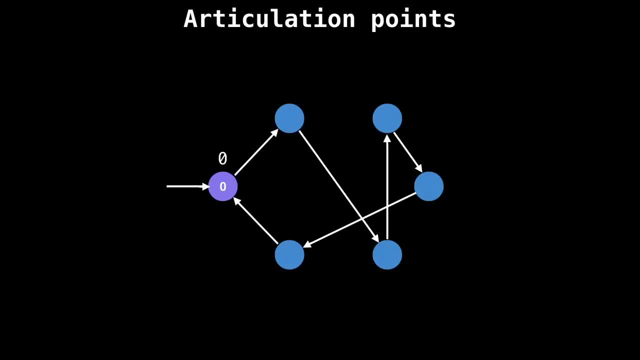 you're traversing a graph and eventually you somehow arrive at node zero. Eventually you're traversing a graph and eventually you somehow arrive at node zero. And, like in any depth first search, you would continue on to explore the graph And eventually, if you 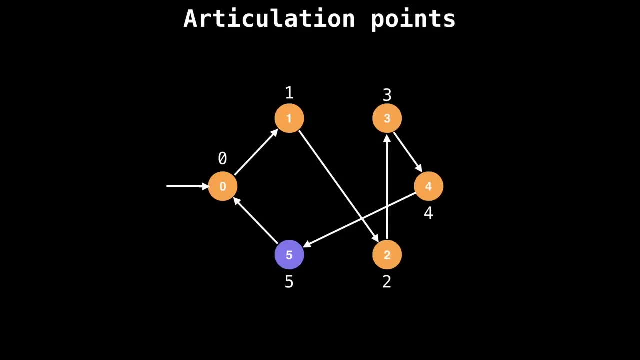 ever re encountered the node that started the cycle with an edge. its ID gets propagated throughout the cycle during the callbacks of the depth first search. This is the case because we are reassigning the new low link value to equal the min of the current value. 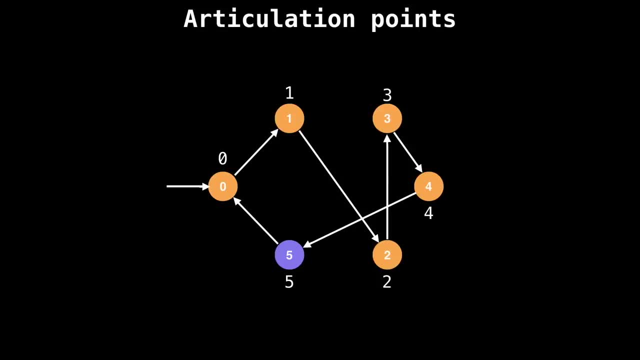 If we're able to identify the value that's being associated with the node, then we can current loading value and the ID of the node we were just visiting. You see now that node five has a loading value of zero acquired from the ID of node zero. This gets spread. 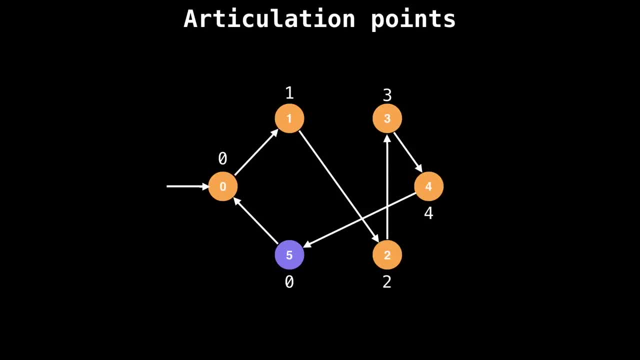 or propagated, as I like to say, throughout the cycle. Now, what you'll notice is that the ID of the node you started- that is equal to the loading value of where it's going to- this indicates that there is a cycle. What is key here is that: the presence of a cycle. 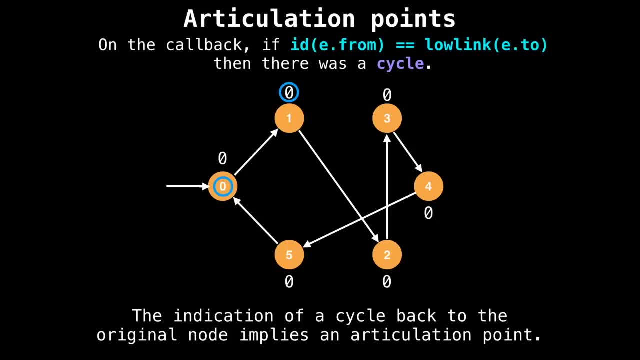 implies that the node is an articulation point. This is because a cycle in a graph corresponds to a strongly connected component and removing the node which started the cycle, who is also connected to another component, We'll sever the graph in two. However, there's just one exception to this, And this is when 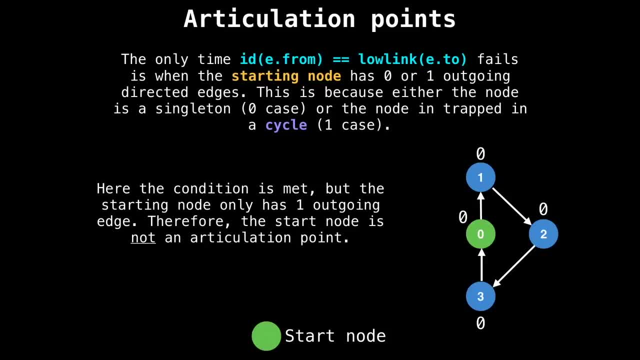 the starting node you choose has either no outgoing edges or, as part of a cycle, and only has one outgoing edge. This is because either the node is a singleton, a standalone node, that is the case with zero outgoing edges, or the node is trapped in a cycle where 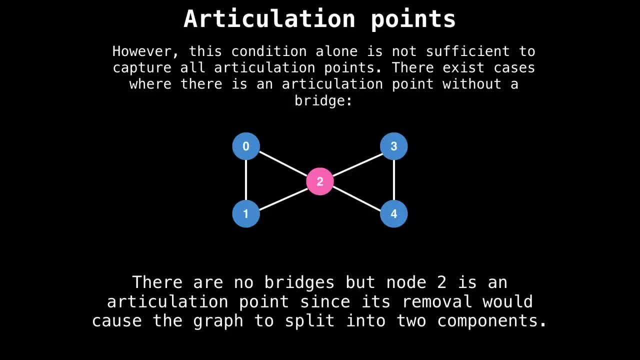 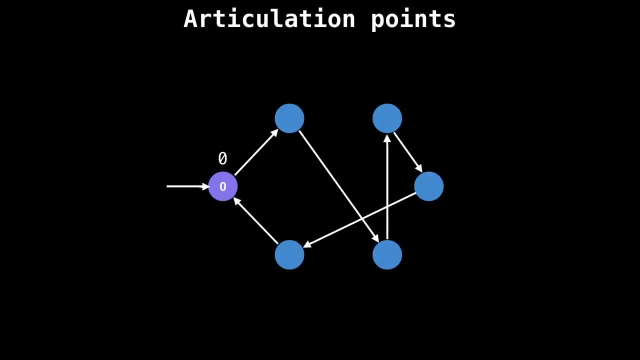 with cycles in the graph. To understand why, let's look at an example. Suppose you're traversing a graph And eventually you see, somehow arrive at node zero. Initially suppose no, zero has a loading value also of zero And like in any depth first search, you would continue on to explore the graph And eventually 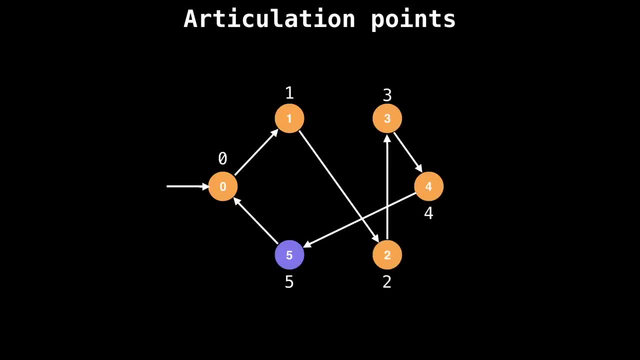 if you ever reencounter the node that started the cycle with an edge, its ID gets propagated throughout the cycle during the callbacks of the depth first search. This is the case because we're reassigning the new loading value to equal the min of the current loading value. 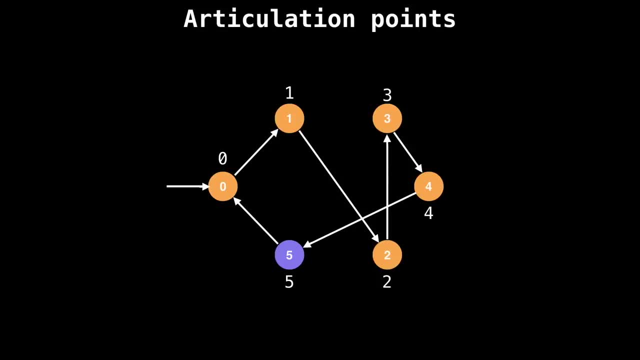 and the ID of the node we were just visiting. You see now that node five has a loading value of zero, acquired from the ID of node zero. This gets spread, or propagated, as I like to say, throughout the cycle. Now what you'll notice is that the ID of the node you started that is equal to the low. 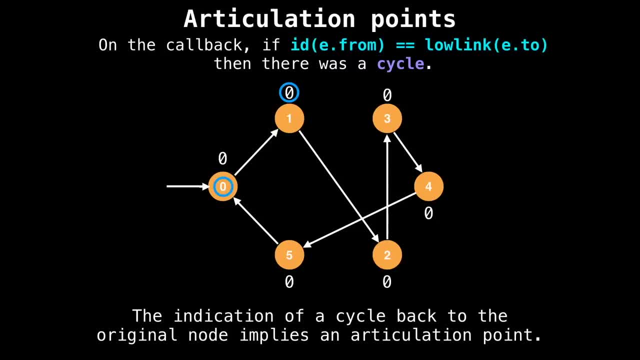 link value of where it's going to. this indicates that there is a cycle. What is key here is that the presence of a cycle implies that the node is an articulation point. This is because a cycle in a graph corresponds to a strongly connected component, and removing 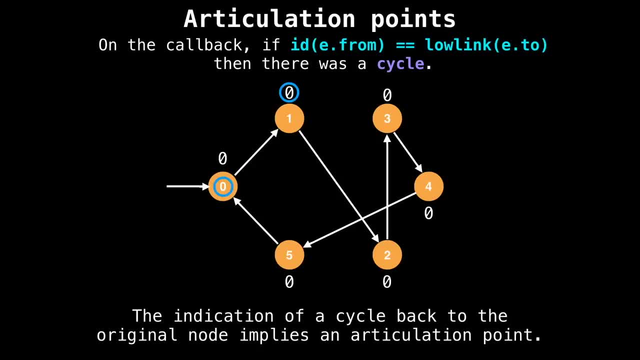 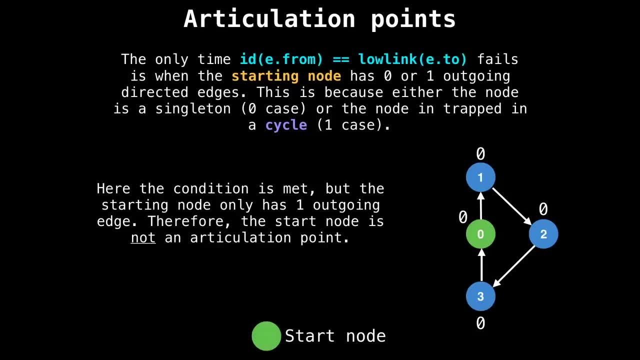 the node which started the cycle, who is also an articulation point. This is because the node that is also connected to another component will sever the graph in two. However, there's just one exception to this, And this is when the starting node you choose has either no, 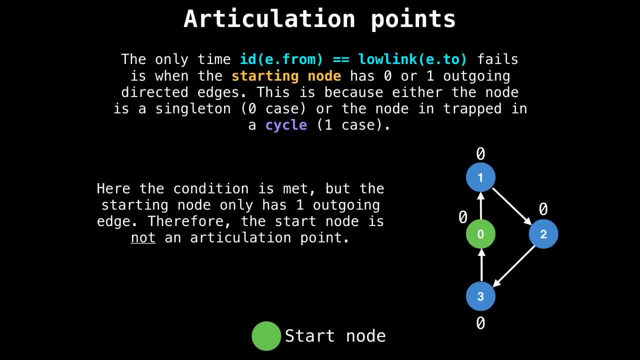 outgoing edges or as part of a cycle and only has one outgoing edge. This is because either the node is a singleton, a standalone node- that is the case with zero outgoing edges- or the node is trapped in a cycle where it only has one outgoing edge. To be an articulation point, you need to have 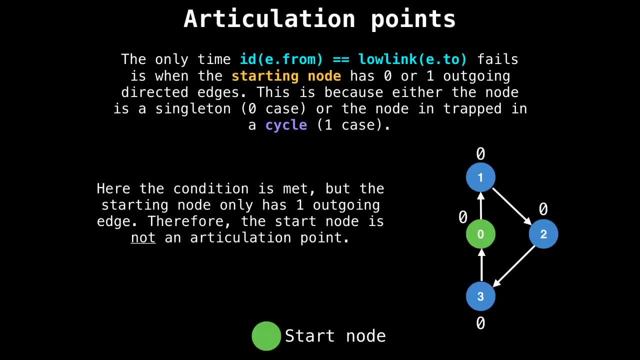 it only has one outgoing edge. To be an articulation point, you need to have more than one outgoing edge. For example, in the graph on the right, we start at node zero, the green node, and is not an articulation point, despite our condition of the ID equaling the loading value. However, as soon as we 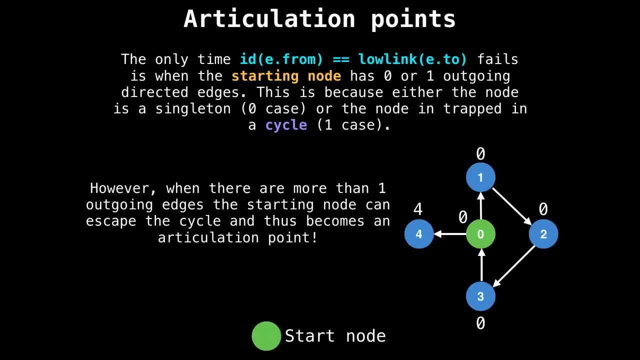 add another edge to our starting node. it becomes an articulation point. So this is something to watch out for and is unique to the starting node. Let's now take a quick look at the changes we need to do to our finding bridges algorithm to find: 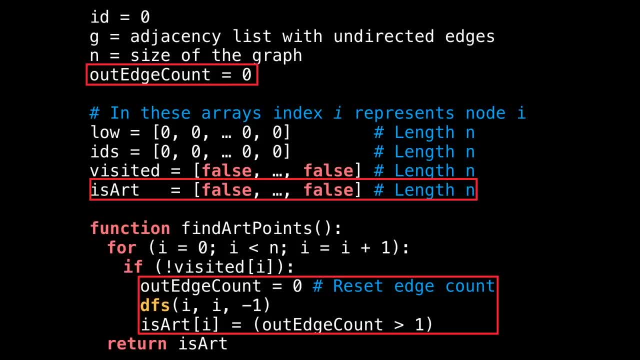 articulation points. To begin with, we'll need a way to track the number of outcoming edges The starting node has. so I define a new variable called out edge count. Next, I define a Boolean array, called is art, which has true or false, depending on whether or not node i is an articulation point. Ultimately, 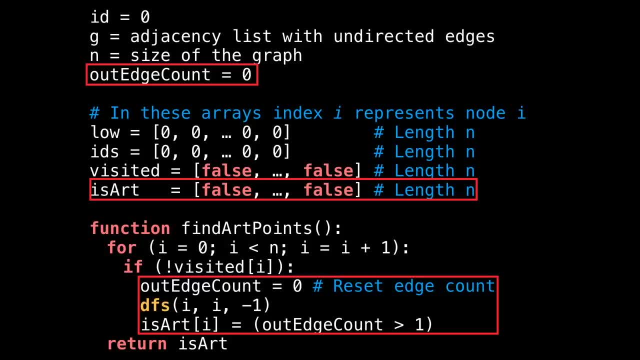 this will be the return value of the find art points function. In the body of the find art points function I reset the edge count variable for every connected component And, after the depth first search, mark the starting node I as either an articulation point or 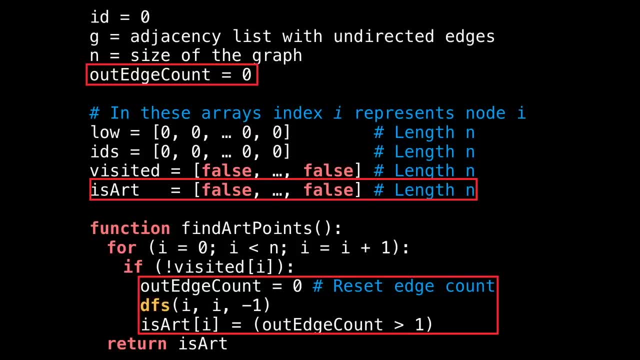 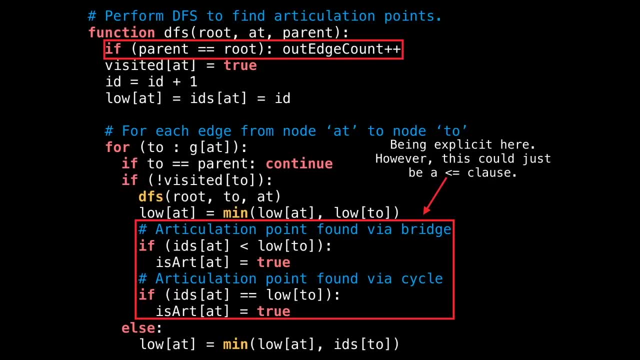 not based on how many outcoming edges were found Inside the depth first search method. all I added was an if statement to increment the number of outcoming edges from the starting node. Besides that, I added the equals case to track articulation points found via cycles and kept the less than case to find articulation. 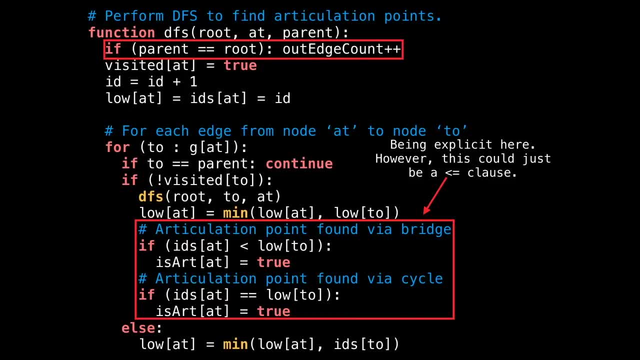 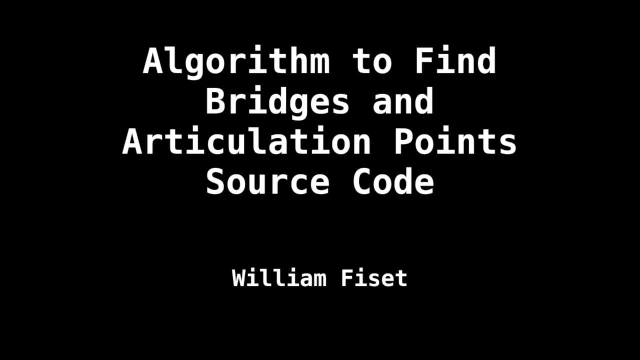 points found via bridges. In a real implementation, you can merge these two if statements into a single clause. However, I want to distinguish finding articulation points from bridges via those from cycles. In today's video, we're going to look at the algorithm to find articulation points and 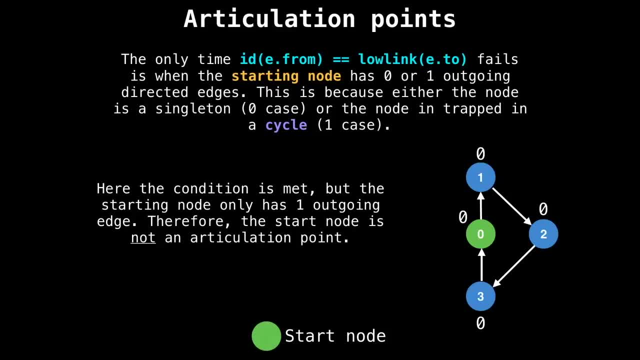 more than one outgoing edge. For example, in the graph on the right, we start at node zero, the green node, and is not an articulation point, despite our condition of the ID equaling the low link value. However, as soon as we add another edge to our starting node, it 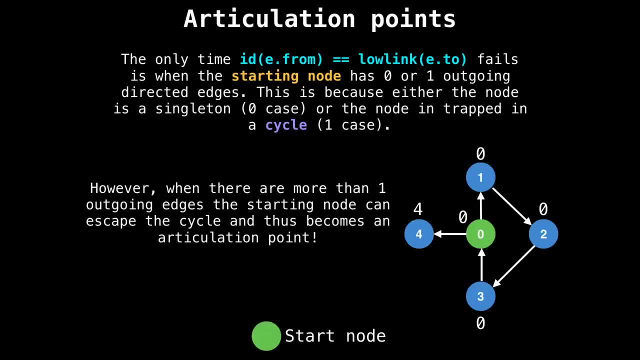 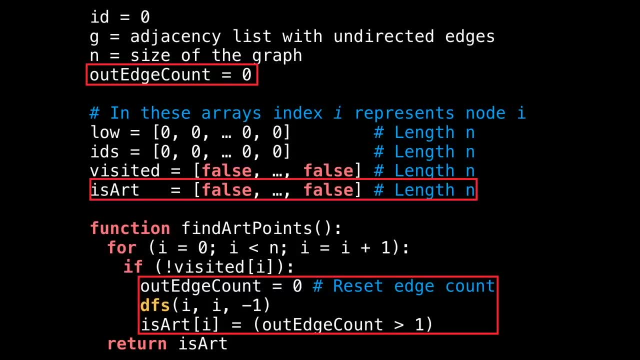 becomes an articulation point. So this is something to watch out for and is unique to the starting node. Let's now take a quick look at the changes we need to do to our finding bridges algorithm to find articulation points. To begin with, we'll need a way to track the 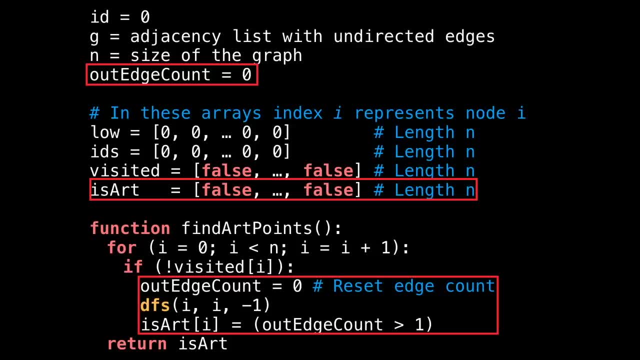 number of outcoming edges The starting node has. so I define a new variable called out edge count. Next I define a Boolean array called is art, which has true or false depending on whether or not node I is an articulation point. Ultimately, this will be the return value of the find art points function In. 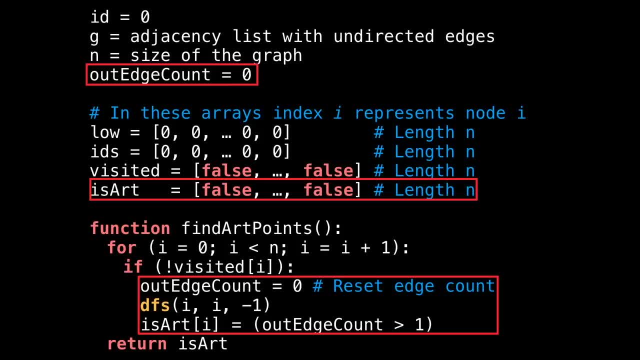 the body of the find art points function. I reset the edge count variable for every connected component And, after the depth first search, mark the starting node I as either an articulation point or not, Based on how many outcoming edges were found Inside the depth first search method. all I added. 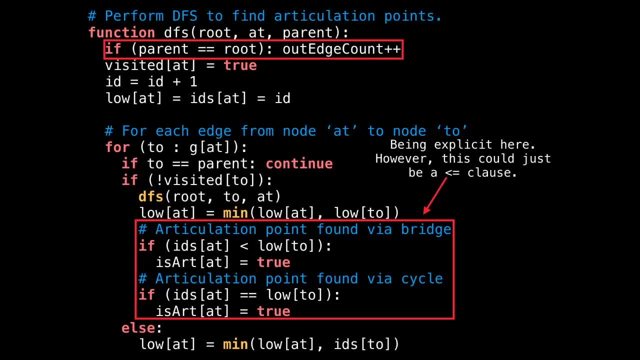 was an if statement to increment the number of outcoming edges from the starting node. Besides that, I added the equals case to track articulation points found via cycles and kept the less than case to find articulation points found via bridges In a real implementation. 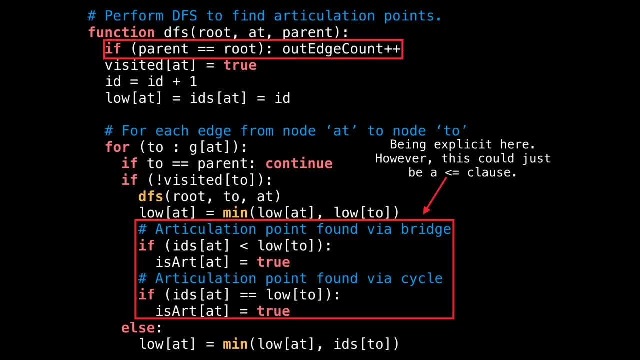 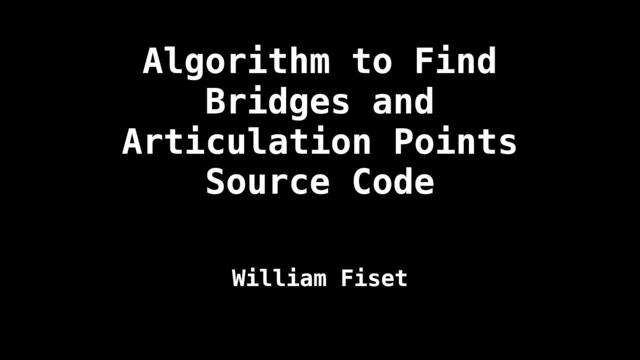 you can merge these two if statements into a single clause. However, I want to distinguish finding articulation points from bridges via those from cycles. In today's video, we're going to look at the algorithm to find articulation points and bridges, but this time with actual source. 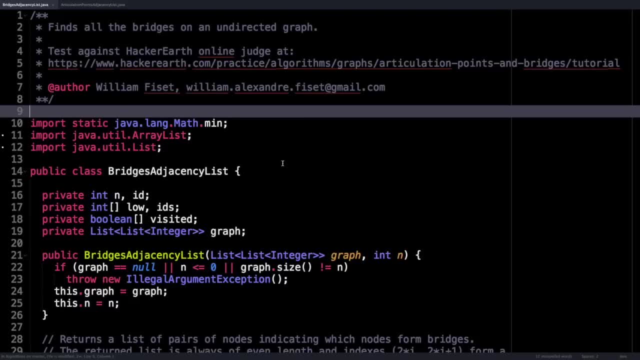 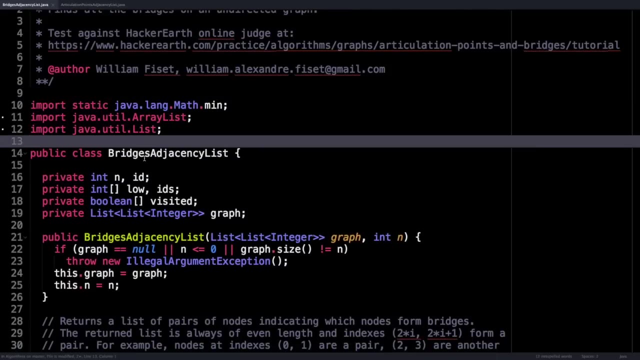 code. All right, here we are in the source code: find bridges. we'll look at the source code to find articulation points shortly. So this source code is written in the Java programming language And here I have a class which will find all the bridges in an undirected graph stored. 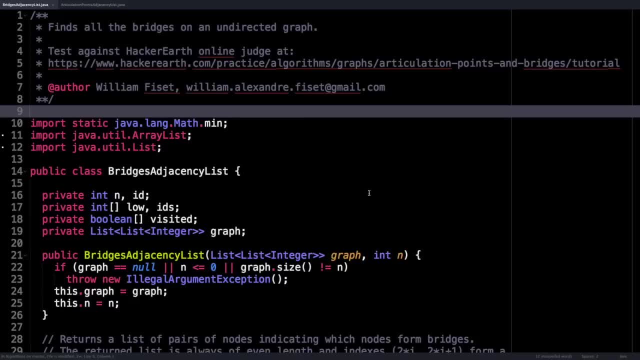 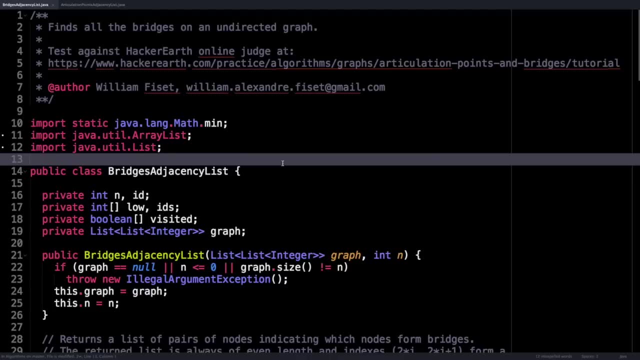 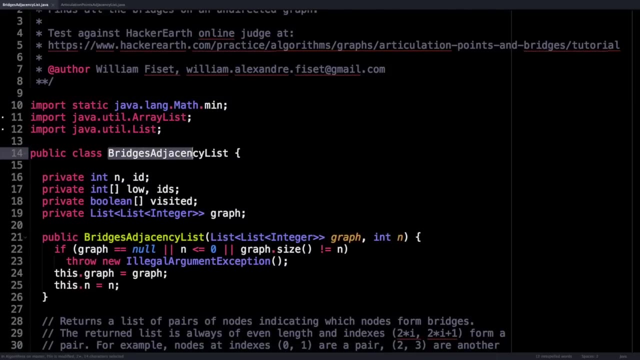 bridges, but this time with actual source code. All right, here we are in the source code: find bridges. we'll look at the source code to find articulation points shortly. So this source code is written in the Java programming language And in this class, which will find all the bridges in an undirected graph stored as an adjacency. 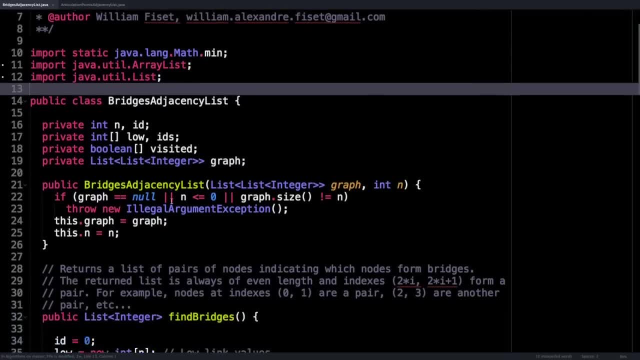 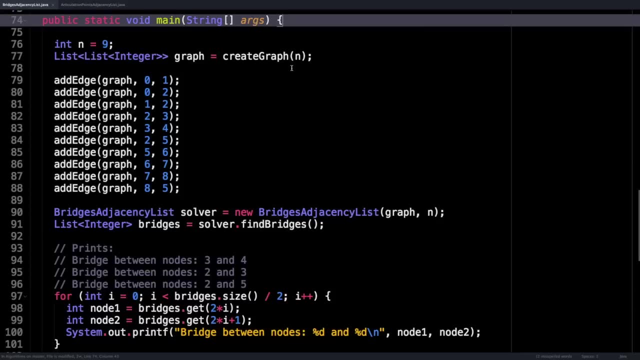 list. But before I get into the details of the code, I actually want to show you how the code works and how you're supposed to use it. So this is the main method that will set up the graph. But before we even do that, I'm just going to scroll down here and look. 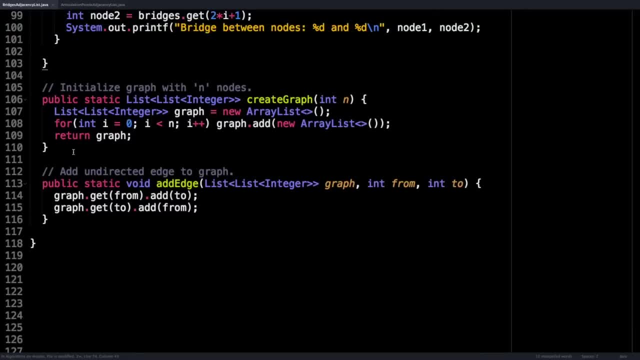 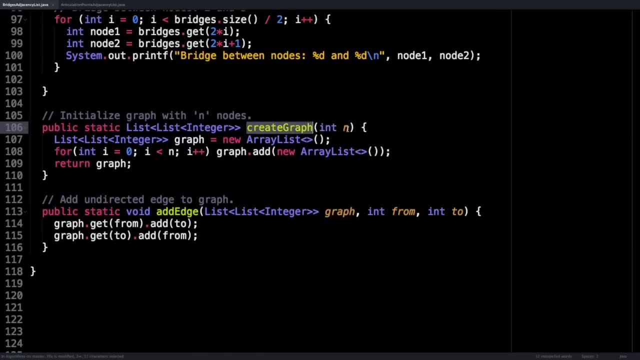 at some of the methods used to actually create the graph and make something useful. So this first method: we'll create a graph with n nodes. So I create a list of lists of type integer, which is basically an adjacency list with directed edges. So all I do is I create 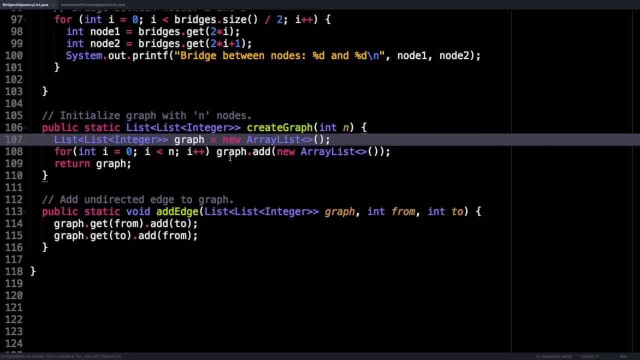 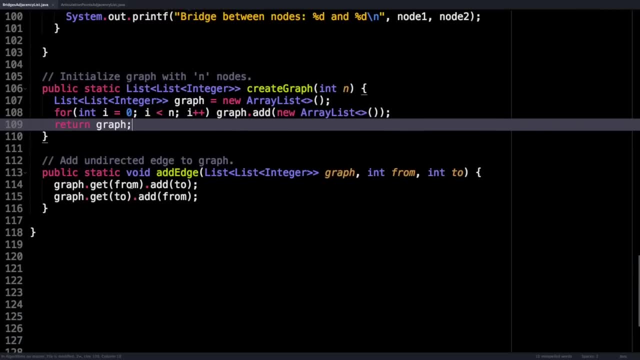 a new array list and then fill that list of lists with empty lists and then return the graph. That's our graph for now And then later on. what we'll do is we'll call this add edges method to add directed edges into the graph. So you see, first we add an edge from a node to 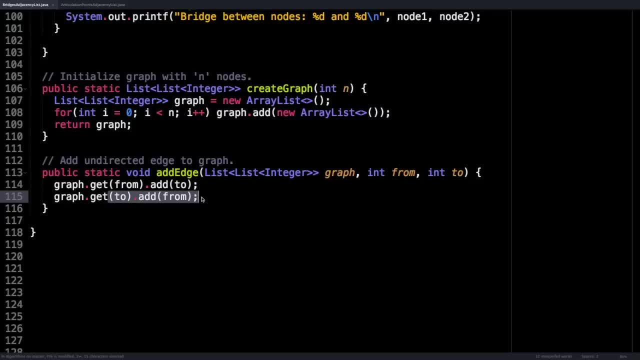 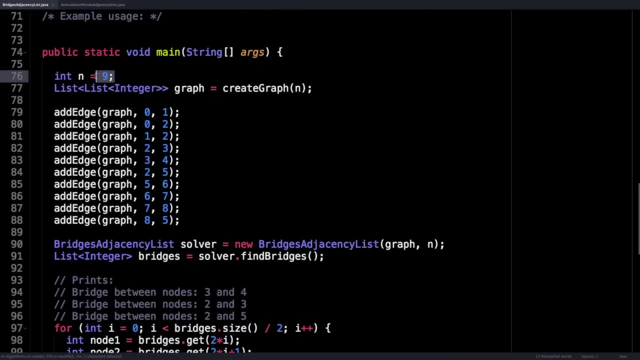 a node and then to that node, From that node. The naming is a little confusing- from into. I use from to mean the, the node the edge starts at, and to to be the node the edges going to. So in this example I have a graph with nine. 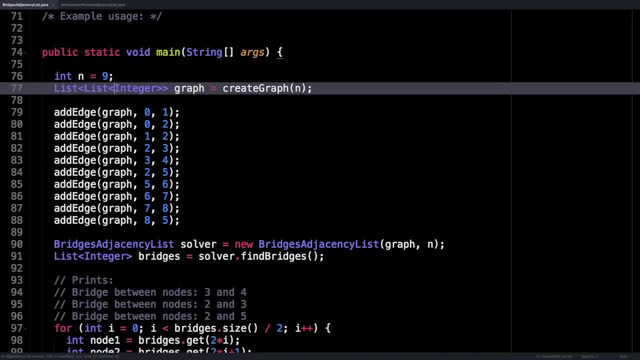 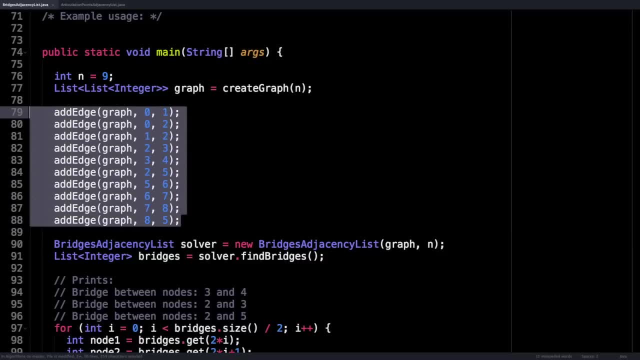 nodes. So I initialize n to be nine, then I create the graph and then add all my edges. you will notice that this graph is actually the graph from the slides in the last video. And then what we're going to do is we're going to pass this graph and the number of nodes. 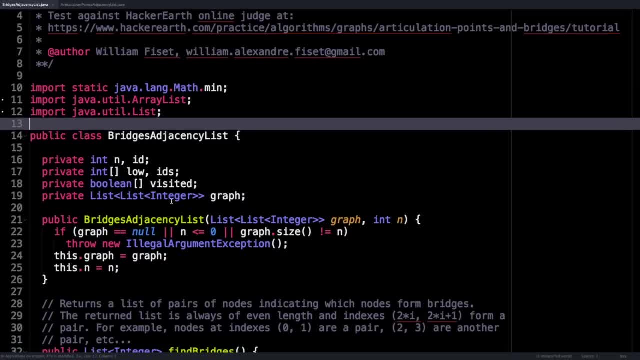 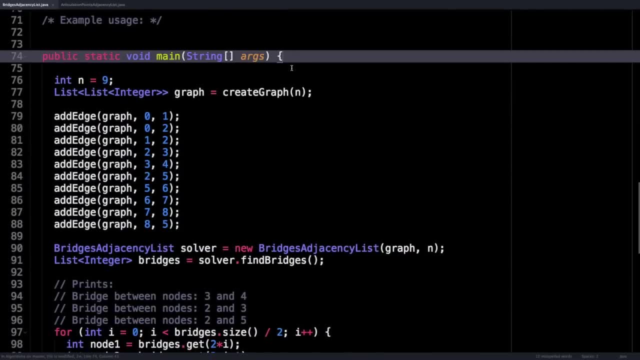 as an adjacency list. But before I get into the details of the code, I actually want to show you how the code works and how you're supposed to use it. So this is the main method that will set up the graph. But before we even do that, I'm just going to scroll down. 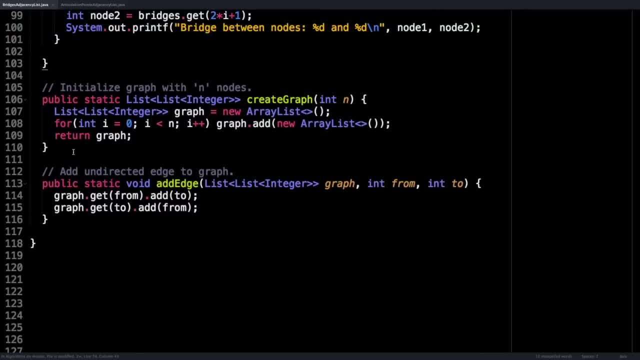 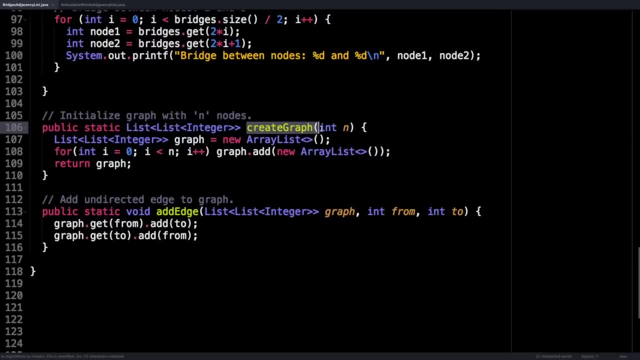 here and look at some of the methods used to actually create the graph and make something useful. So this first method will create a graph with n nodes. So I create a list of lists of type integer, which is basically an adjacency list with directed edges. So 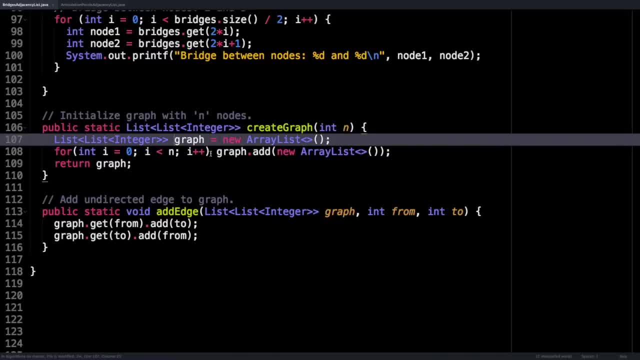 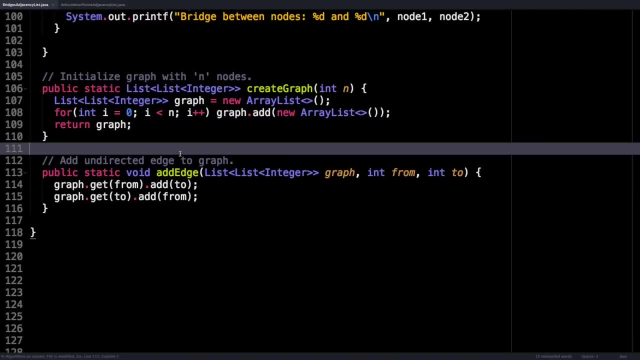 all I do is I create a new array list and then fill that list of lists with empty lists and then return the graph. That's our graph for now And then later on. what we'll do is we'll call this add edges method to add directed edges into the graph. So you see. 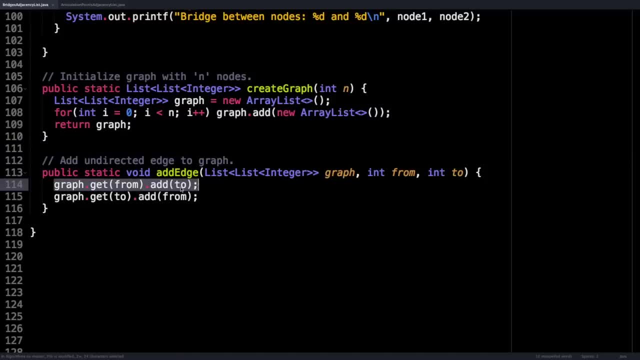 first we add an edge from a node to a node and then to that node, From that node. The naming is a little confusing: from into- I use from to mean the, the node the edge starts at, and to to be the node. Yeah, just going to. 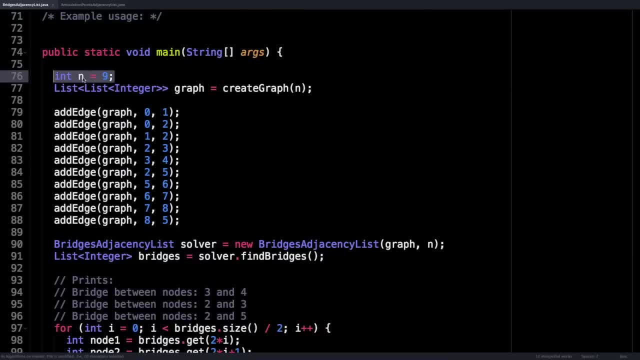 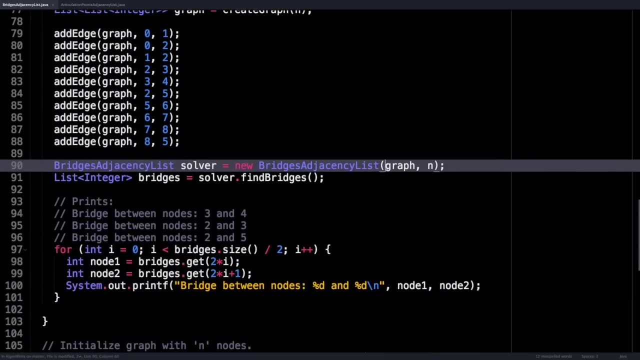 So in this example, I have a graph with nine nodes, so I initialize n to be nine, then I create the graph and then add all my edges. you will notice that this graph is actually the graph from the slides in the last video. And then what we're going to do is we're going to pass this graph. 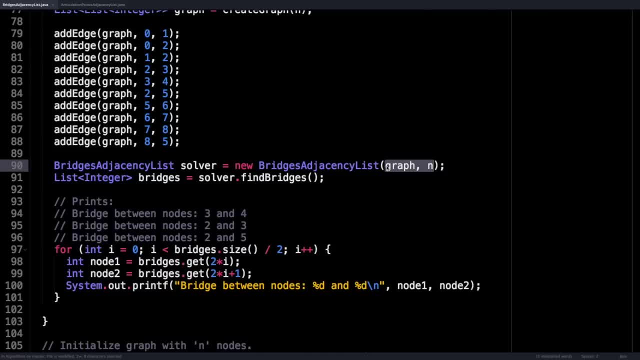 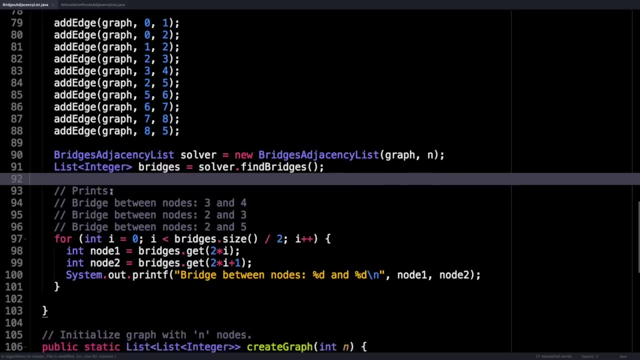 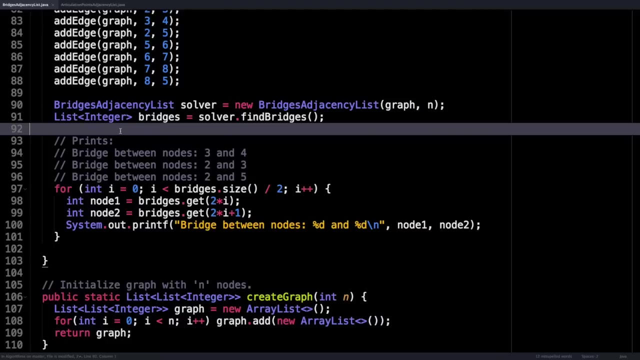 and the number of nodes into the class above, which is going to be our solver, And then the solver is going to be able to find all the bridges and return all the bridges as a list of integers. Then, once you have this list of bridges, bridges are going to be stored as pairs, So every 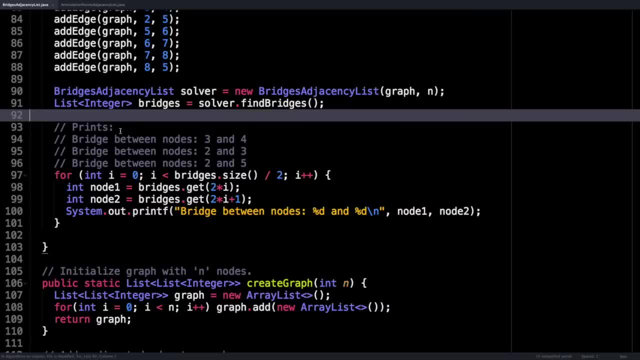 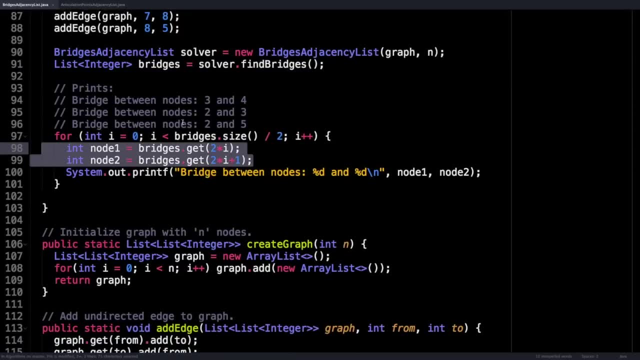 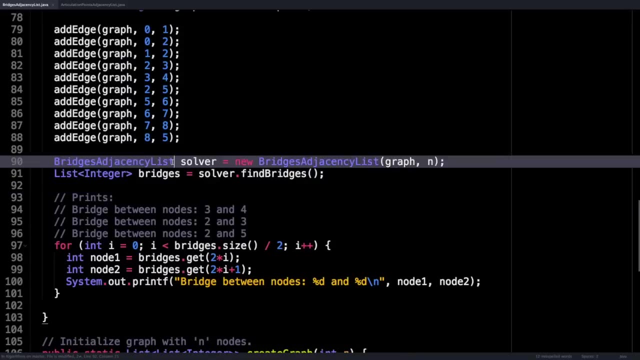 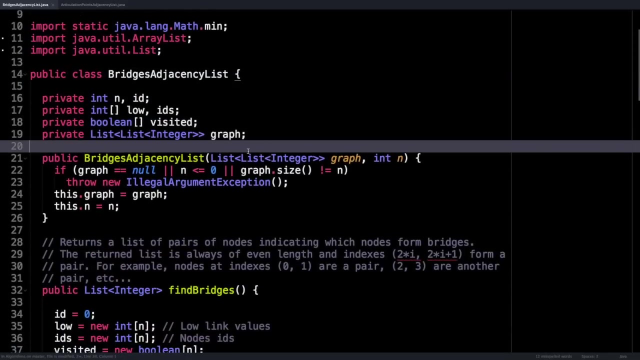 two integers that are adjacent in And pairs are going to be bridges, So I pull those out and I print them, And this is the result you would expect for this graph. Alright, great. Now you're wondering: how does the magic happen in here? So let's scroll up to the constructor And actually let's. 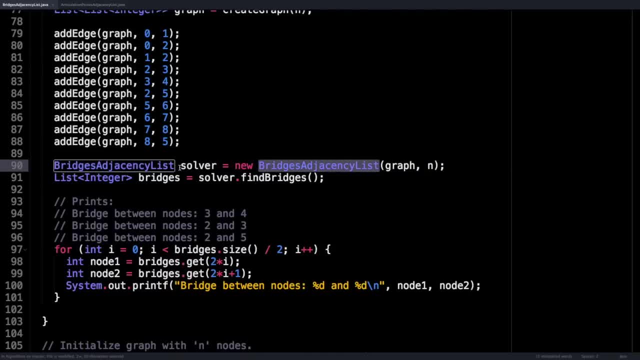 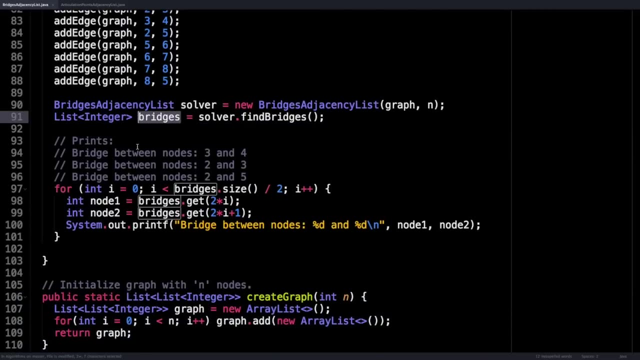 into the class above, which is going to be our solver, And then the solver is going to be able to find all the bridges and return all the bridges as a list of integers. Then, once you have this list of bridges, bridges are going to be stored as pairs, So every 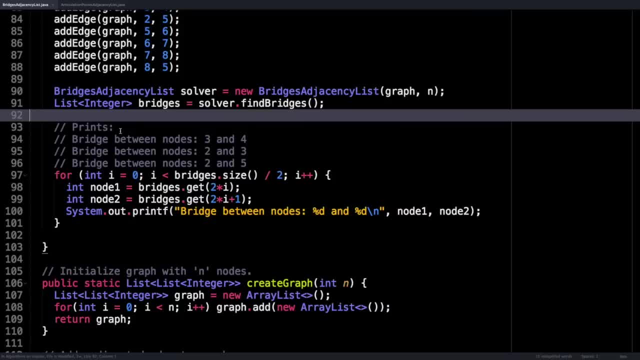 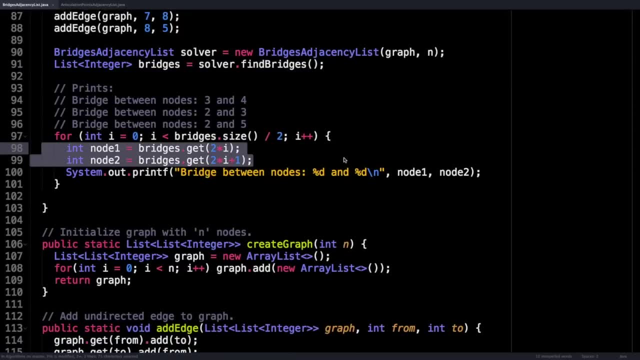 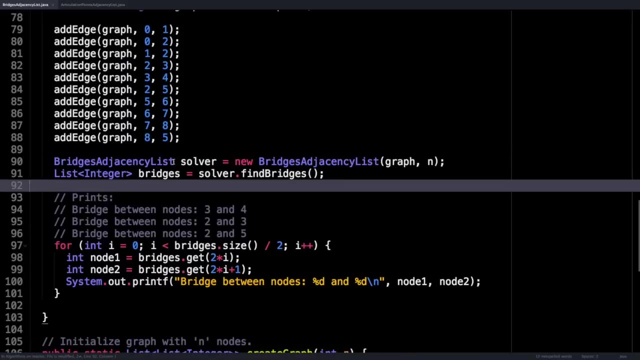 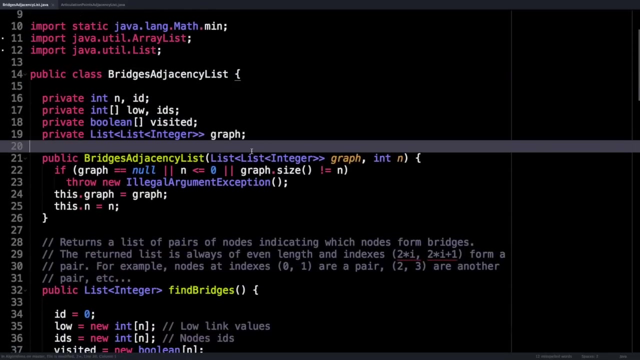 two integers that are adjacent in pairs are going to be bridges, So I pull those out and I print them, And this is the result, And this is what you would expect for this graph. All right, great. Now you're wondering: how does the magic happen in here? So let's scroll up to the constructor And actually 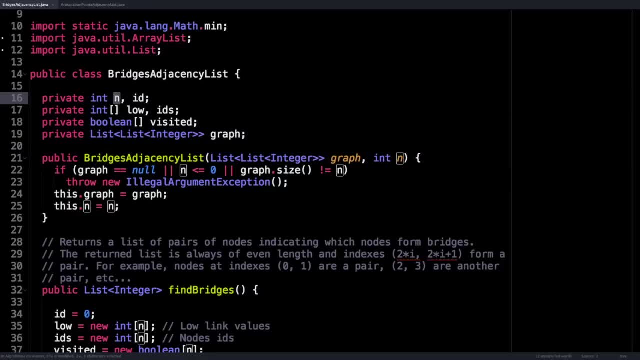 let's look at the instance variables. So we have n, which is the number of nodes in the graph, ID, which is that ID number to label each node. So we're going to give each node a unique ID And we need to keep track of. well, what was the last ID? Then I have a 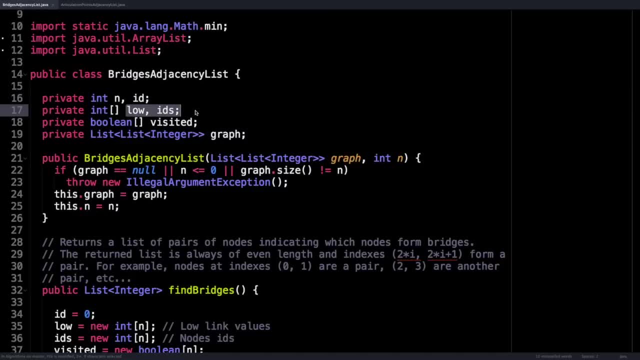 two arrays which track information about the nodes- So low is for the low link values and IDs is to track the ID of each node. we gave a node with the ID variable, then just a Boolean array to track whether or not the node was visited And finally the graph. 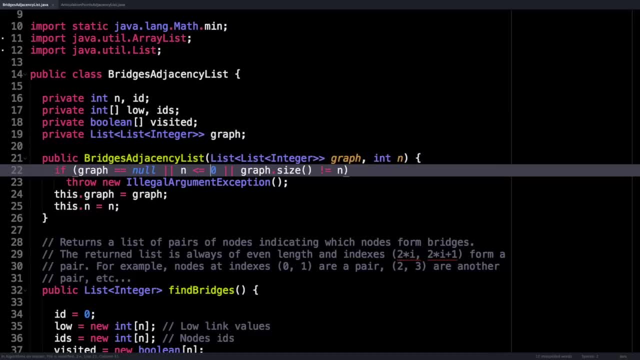 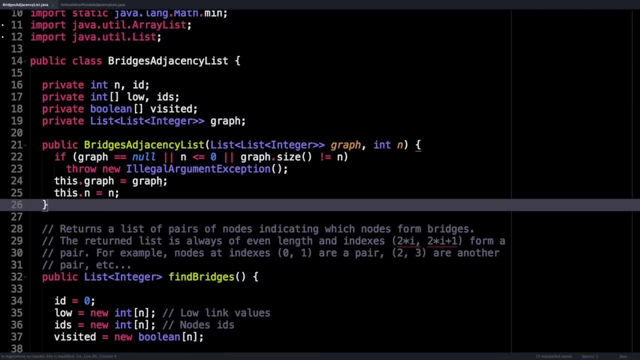 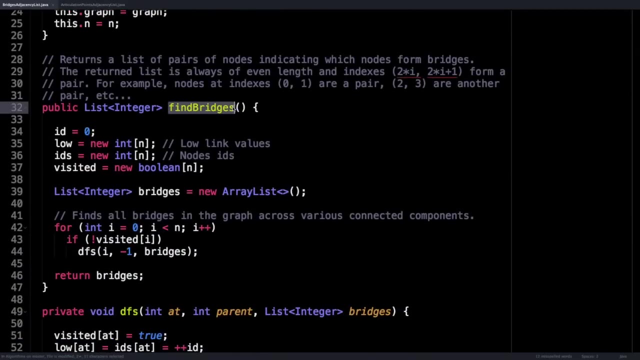 So in the constructor of course, get the graph and the number of nodes. it checks some conditions to make sure the graph is legit. Okay, so now we've constructed the object or the solver object, And the method we're interested in is find the bridges. So the fine bridges just initializes all our variables. 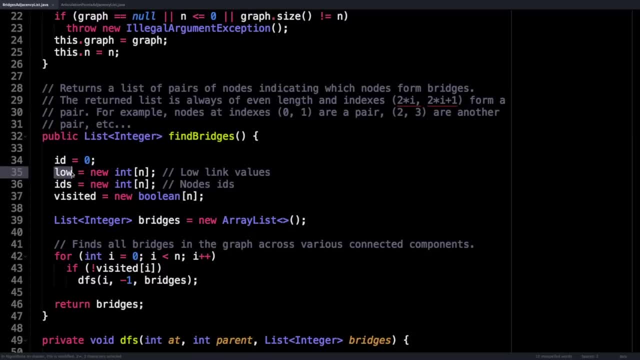 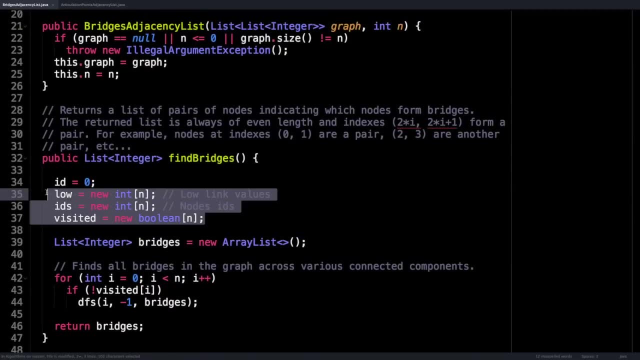 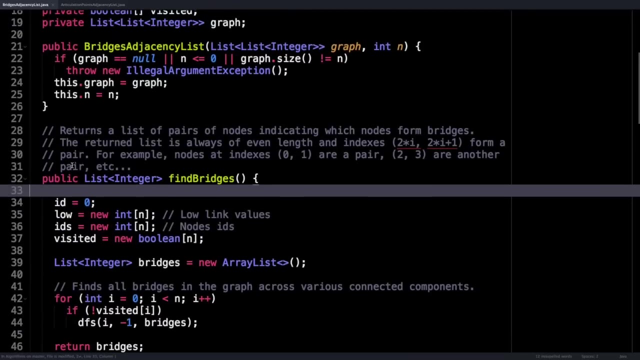 So set ID to be zero, initialize or allocate some memory for the low link values and the ID values and the visited array. It's good practice not to do this work into the constructor, Just because if you're just creating a bunch of these objects but never use them, you 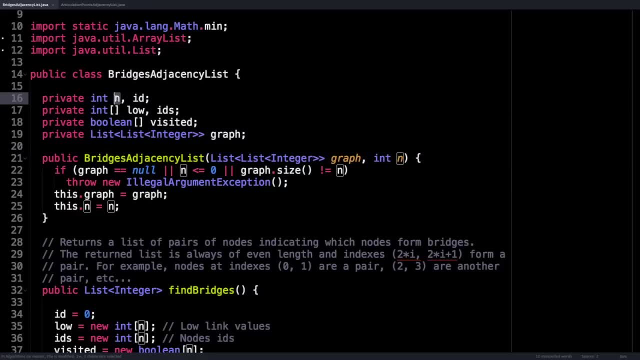 look at the instance variables. So we have n, which is the number of nodes in the graph, ID, which is that ID number to label each node. So we're going to give each node a unique ID And we need to keep track of. well, what was the last ID? then I have two arrays which 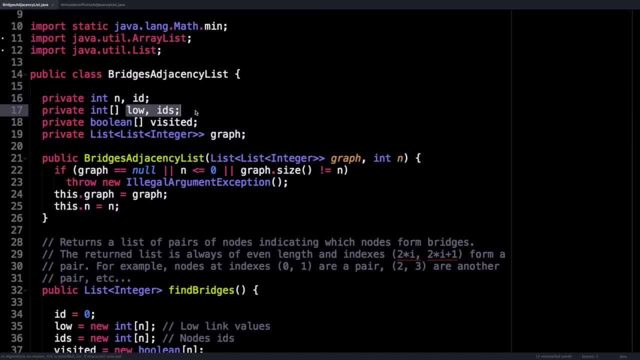 track information about the nodes. So low is for the low link values and IDs is to track the ID of each node. we give a node with the ID variable, then just a Boolean array to track whether or not the node was visited And finally the graph. So in the constructor of course, get the 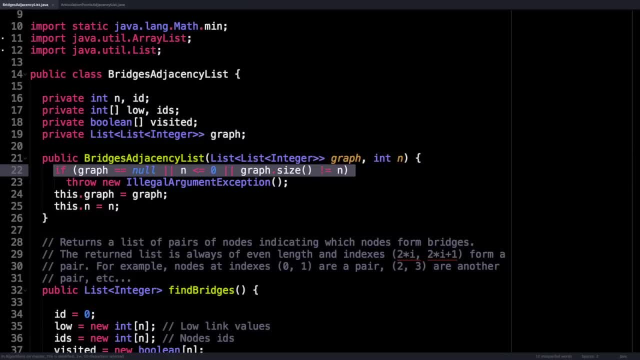 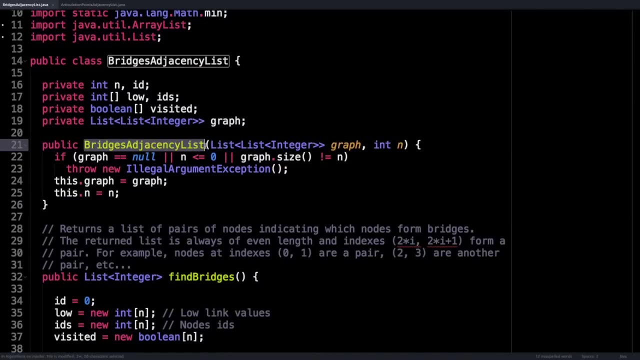 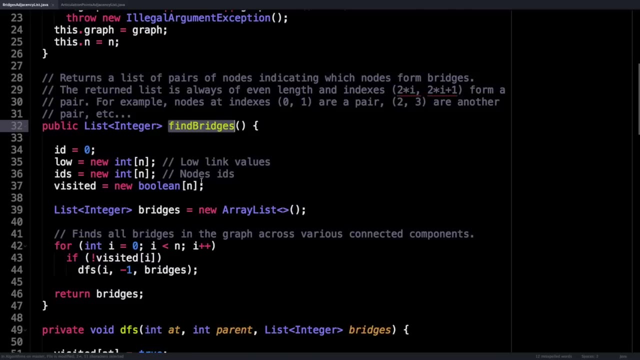 graph and the number of nodes. it checks some conditions to make sure the graph is legit. Okay, so now we've constructed the object or the solver object, And the method we're interested in is find bridges. So the fine bridges just initializes all our variables. 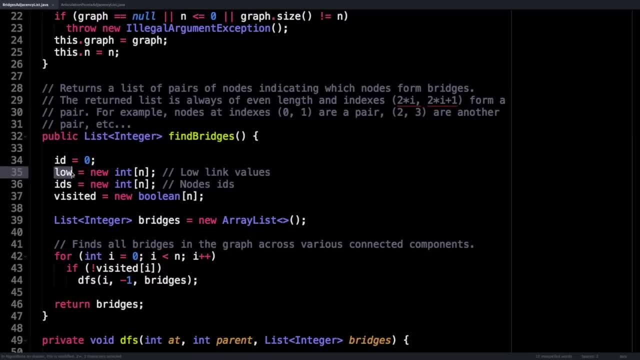 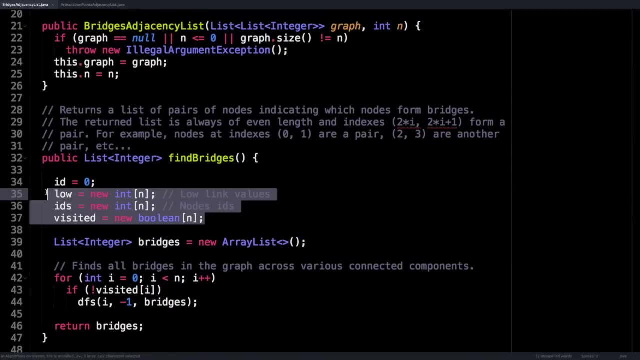 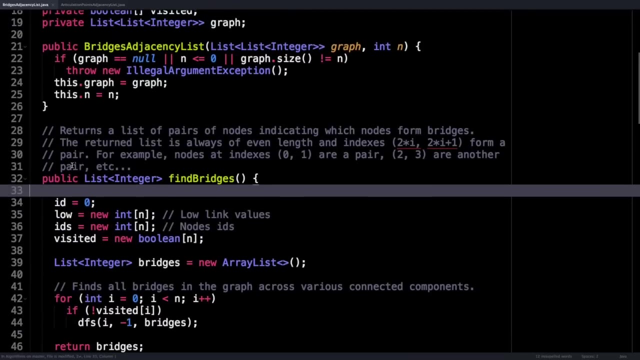 So set ID to be zero, initialize or allocate some memory for the low link values and the ID values and the visited array. It's good practice not to do this work into the constructor, Just because if you're just creating a bunch of these objects but never use them, you might surprise the person initializing. 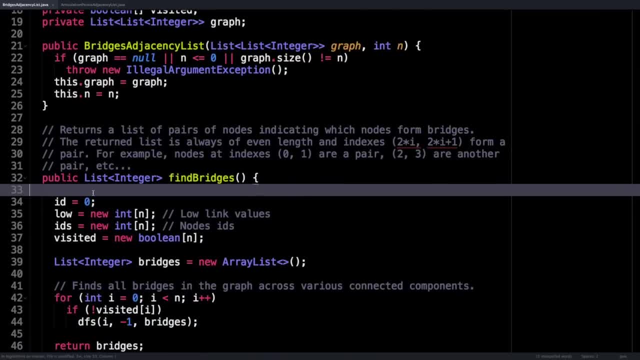 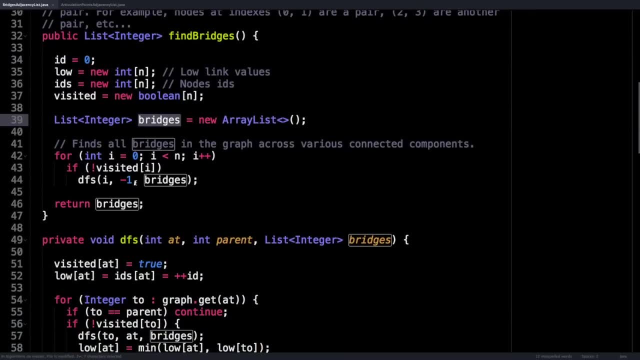 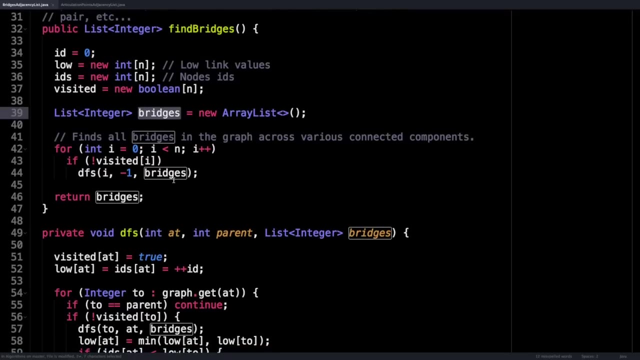 the object why they're having so much memory usage, then initialize the bridges array to be initially empty And then we pass that into the depth first search method. it gets populated and then returned afterwards. So for each node or node ID, right now loop through all the nodes And if that node hasn't, 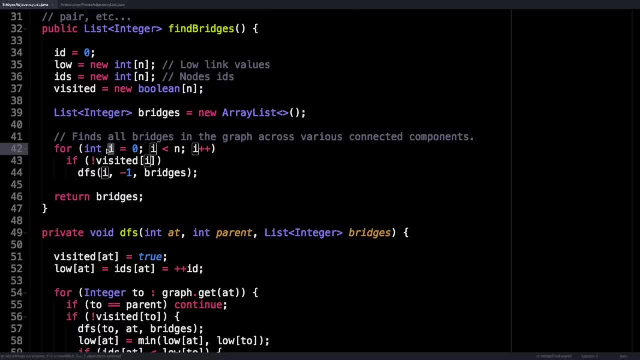 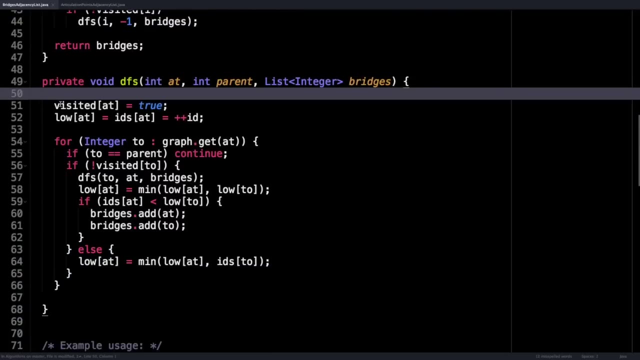 been visited yet start a depth first search on that node And call depth first search method with is the first argument, So the current node minus one for the parent, and then pass in the bridges array. So some housekeeping stuff like any usual depth first search: visit the node And then what we're. 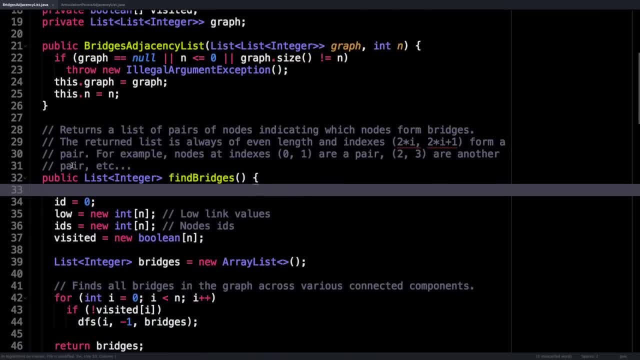 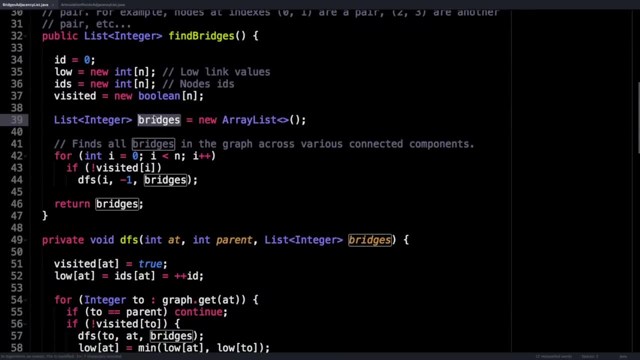 might surprise the person initializing the object why they're having so much memory usage. then initialize the bridges array to be initially empty And then we pass that into the depth first search method. it gets populated and then returned afterwards. So for each node. 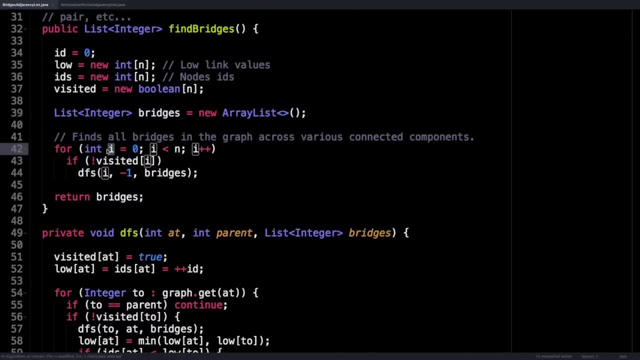 or node ID. right now, group through all the nodes And if that node hasn't been visited yet, start a depth first search on that node And called depth first search method. with is the first argument, So the current node minus one for the parent, and then pass in the bridges array, So some. 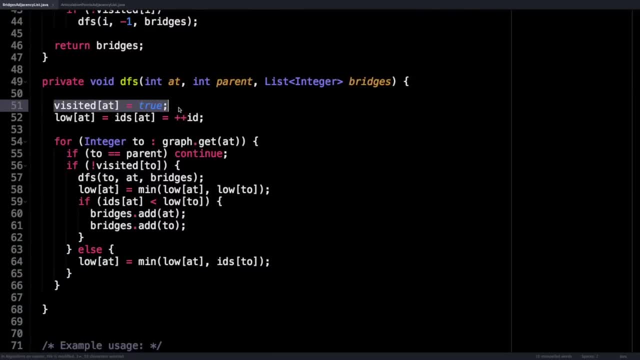 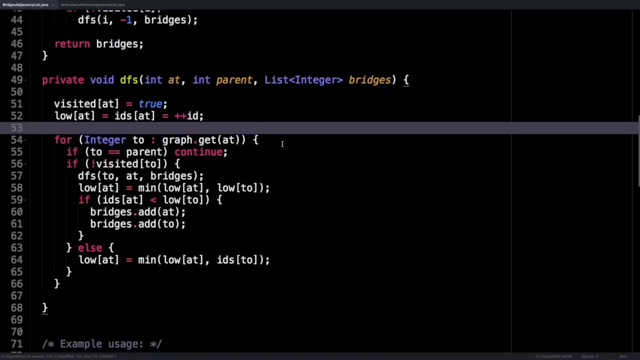 housekeeping stuff like any usual depth first search, visit the node And then what we're going to do is we're going to initialize the loading value and the ID of that node And we're going to do the current node to just be a unique ID which we increment. All right, 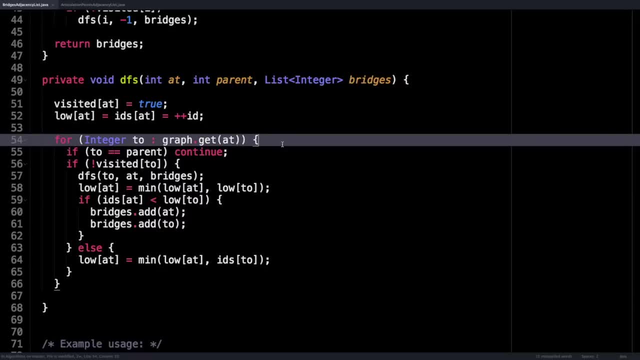 Then we visit from, from the current node, all the nodes we can reach and skip, skip the node that we were just at. So that is the parent node. So we don't want to do our depth first search and then immediately return to the node we just visited. So continue on those. 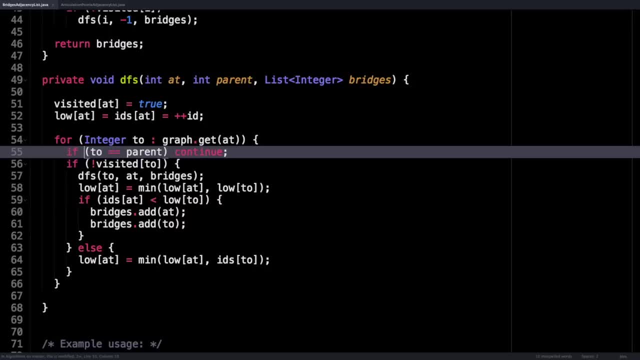 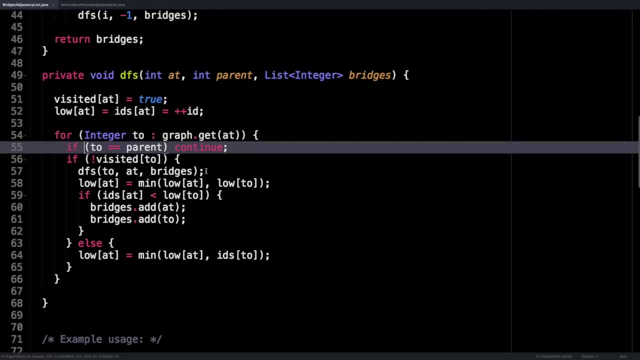 cases, And we have to do this because we have an undirected node graph, remember. So if you haven't visited the node yet, then recursively call our depth first search method and keep probing While if you have, if you're trying to visit a node, you've 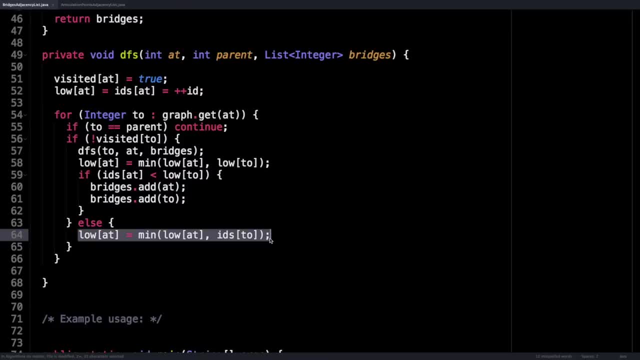 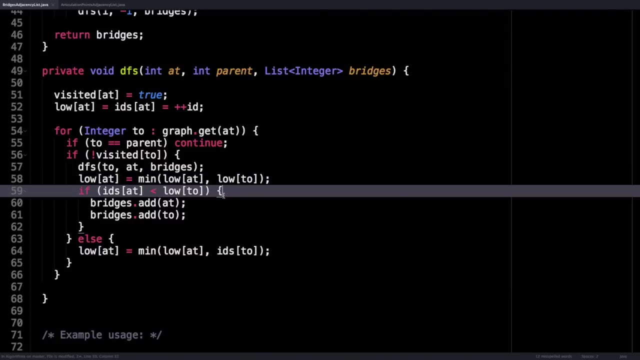 already visited, then you want to take the minimum of the current low link value and the ID of the node you're going to. Otherwise, on the callback of depth first search method is the other low link min statement, which differs from this one slightly in that we have- we're taking the minimum. 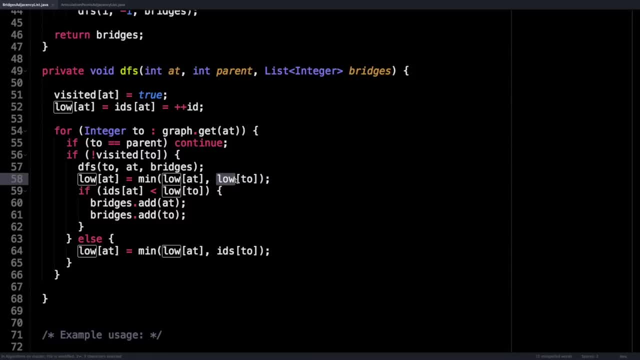 now not of the ID of the node but the low link of the other node And, as we saw in the slides, the condition for bridge is if the ID of the node we're at is less than the low link of the node we're going to. this means we have a bridge, and removing that bridge will cause the number of. 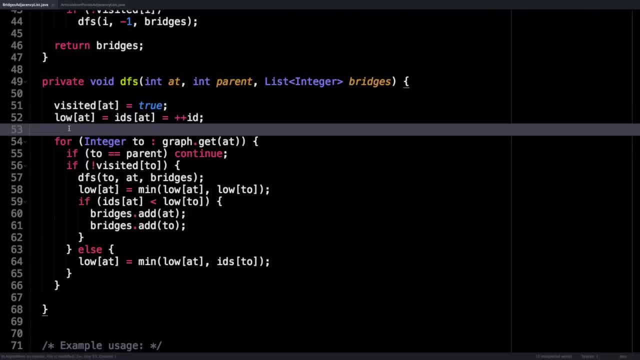 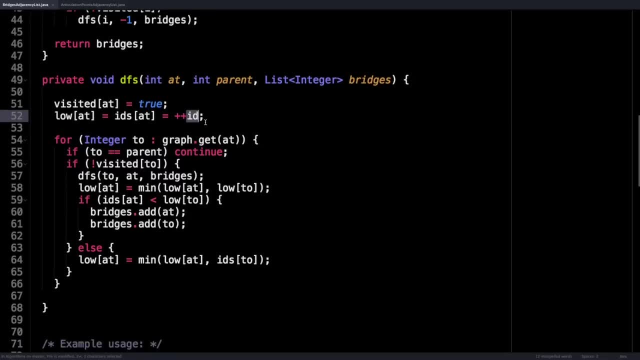 going to do is we're going to initialize the loading value and the ID of that node to just be a unique ID which we increment. All right, then we visit from, from the current node, all the nodes we can reach and skip, skip the node that we were just at. 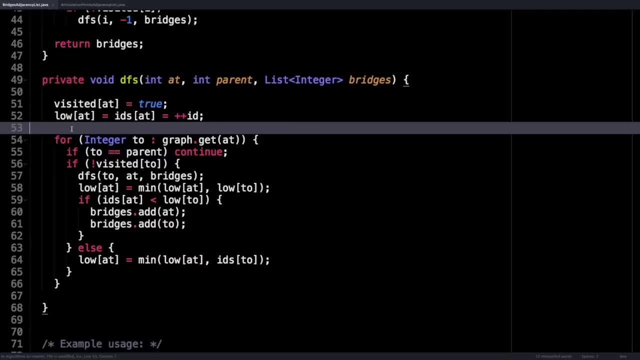 So that is the parent node. So we don't want to do our depth, first search and then immediately return to the node we just visited. So continue on those cases. And we have to do this because we have an undirected graph, remember. So if you haven't visited the node yet, then 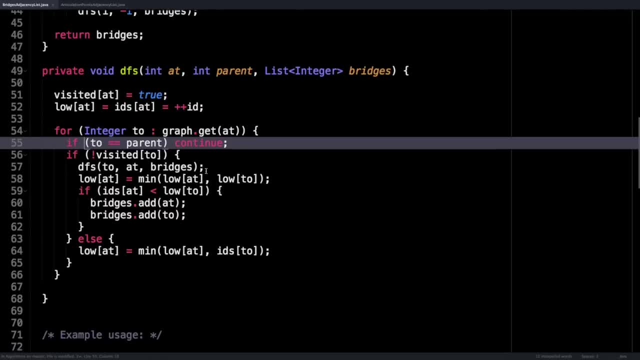 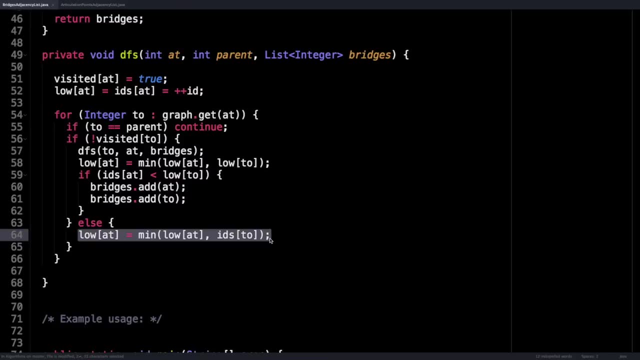 recursively call our depth first search method and keep probing While, if you have, if you're trying to visit a node you've already visited, then you want to take the minimum of the current loading value And the ID of that node, And then you want to take the minimum of the current. 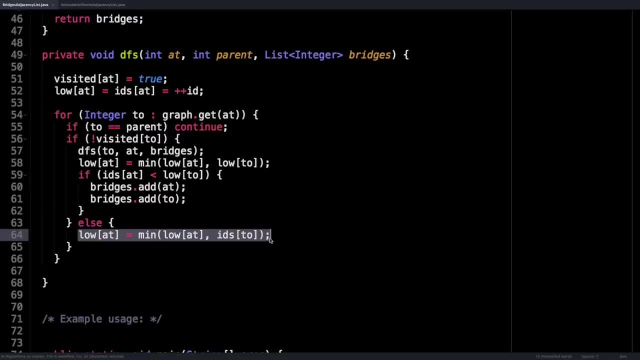 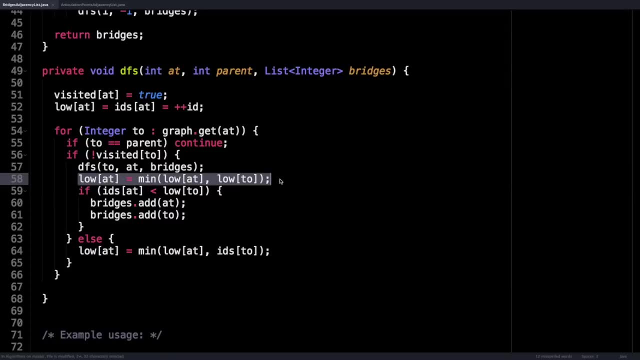 loading value And the ID of the node you're going to. Otherwise, on the callback of depth, first search method is the other low length command statement, which differs from this one slightly in that we have- we're taking the minimum now, not of the ID of the node, but the low link. 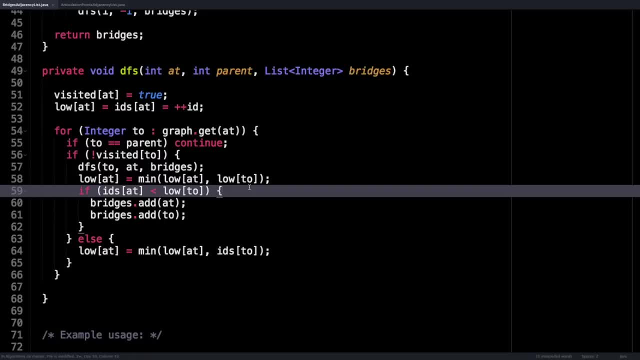 of the other node And, as we saw on the slides, the condition for bridge is if the ID of the node we're at is less than the low link of the node. So we're going to. this means we have a bridge, and removing that bridge will cause the number of 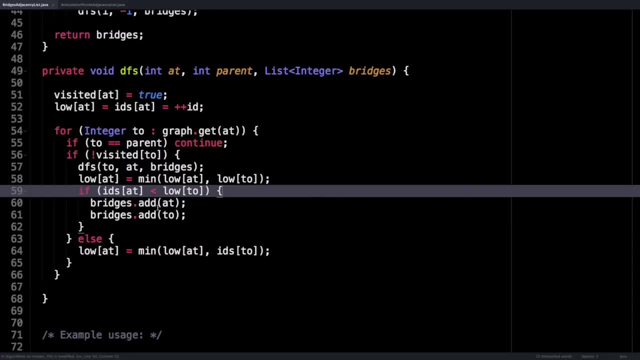 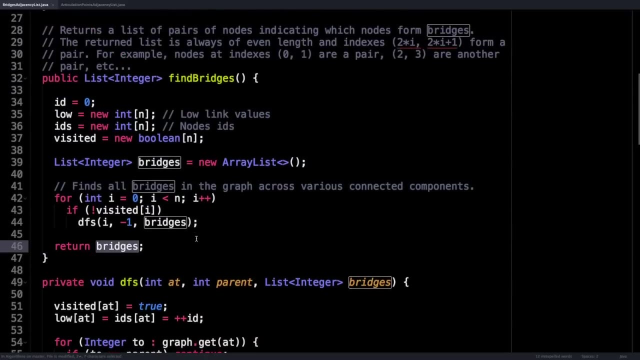 connected components to increase. So append both at and to which are the node IDs of the the bridge and put them in the bridges array and fill that up and then eventually return that down here. So that is all for bridges. Now let's look at articulation points, which 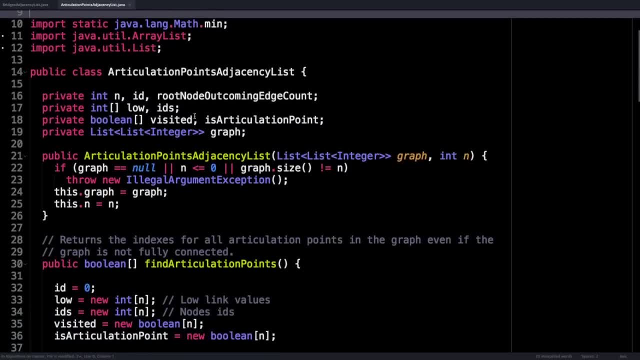 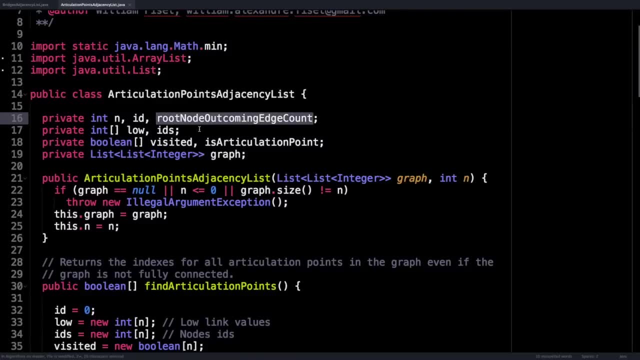 is really almost the same algorithm. So if we look at this, the only thing that's really different is we have a variable to track the number of outcoming edges from the start node, or what I call the root node in this script, And other than that, differences are that we have another Boolean array. 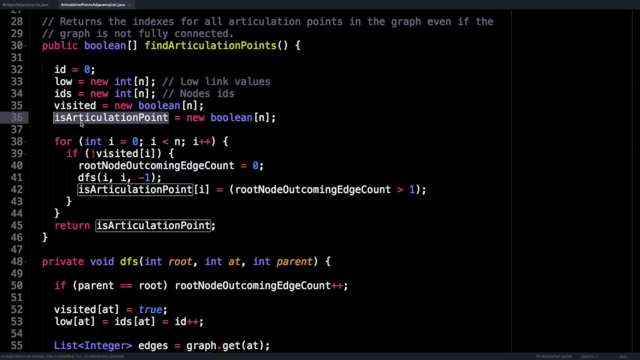 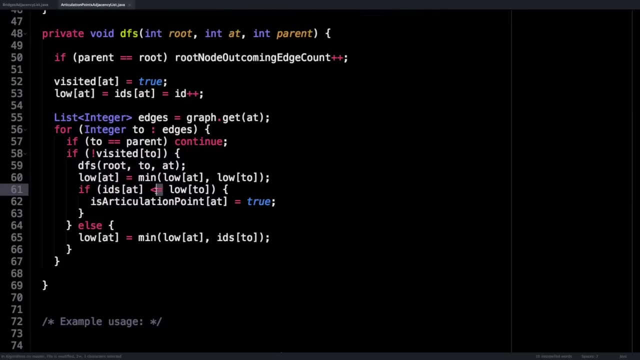 called is articulation point instead of the bridges array to track bridges, And that we have to reset the number of upcoming edges for every depth first search. we do That makes sense. What else is different? Oh, yes, we have a less than or less than or equal to, as opposed to. 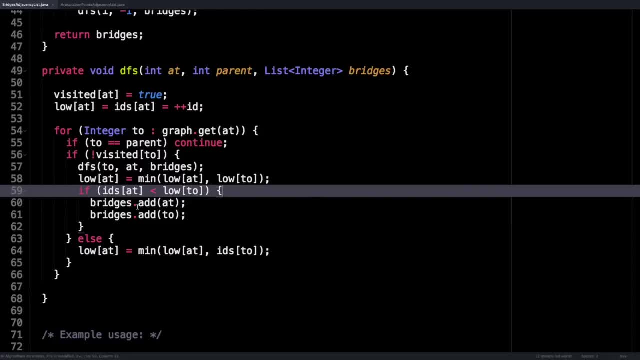 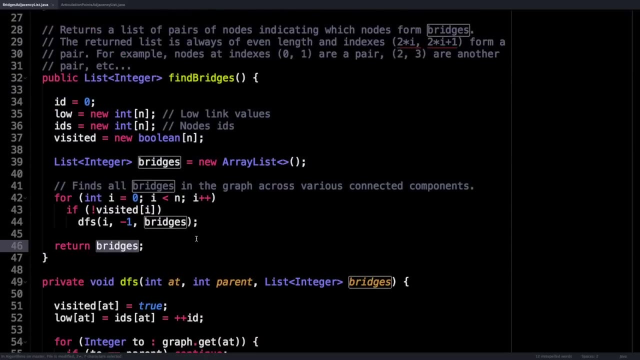 connected components to increase. So append both at and two, which are the node IDs of the the bridge, and put them in the bridges array and fill that up and then eventually return that down here. So that is all for bridges. Now let's look at: 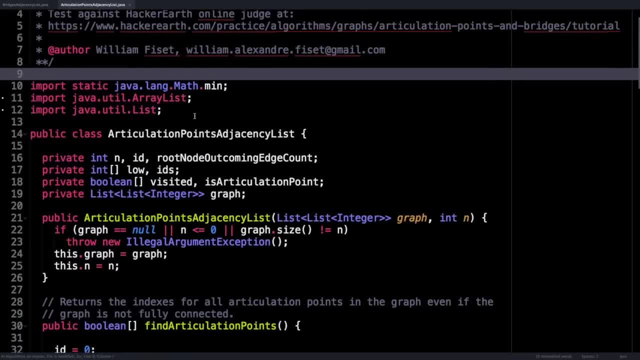 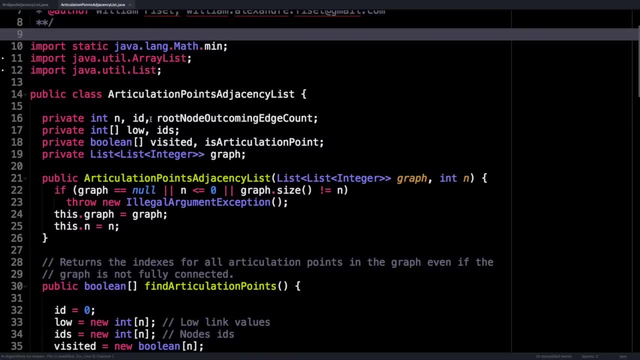 articulation points, which is really almost the same algorithm. So if we look at this, the only thing that's really different is we have a variable to track the number of Outcoming edges from the start node, or what I call the root node, in this script. And other than that, differences. 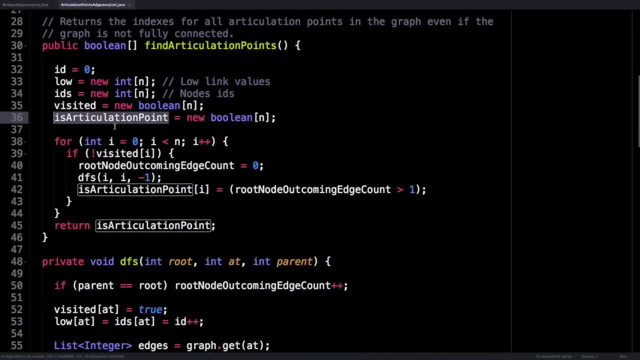 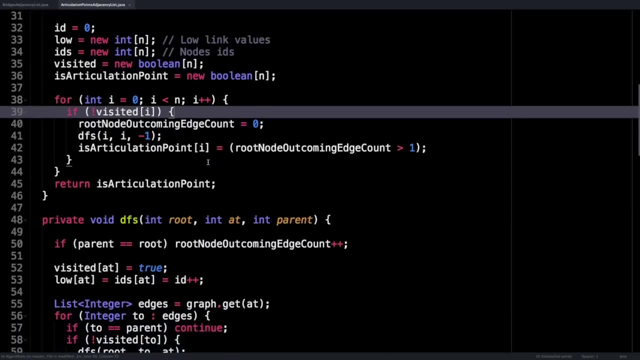 are that we have another Boolean array called is articulation point instead of the bridges array to track bridges, and that we have to reset the number of upcoming edges for every depth first search. we do That makes sense. What else is different? Oh, yes, we have a. 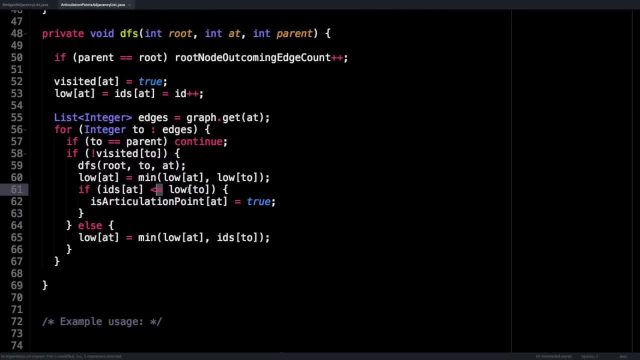 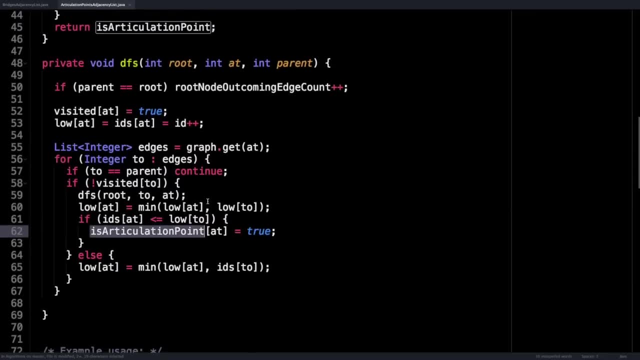 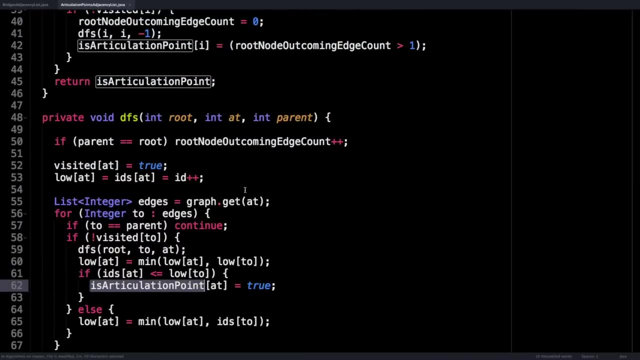 less than or less than or equal to- as opposed to just less than, to track cycles as well and mark off those as articulation points, And I think those are the major differences, If I didn't forget anything, between articulation points and bridges. 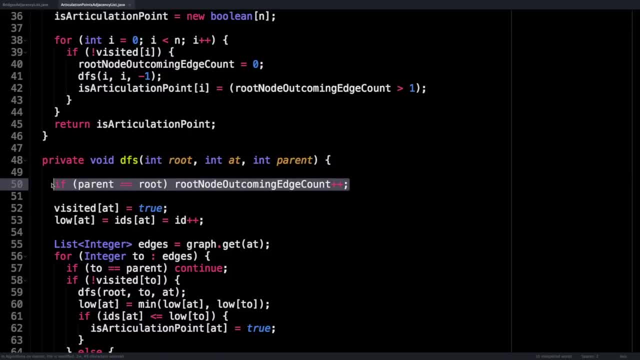 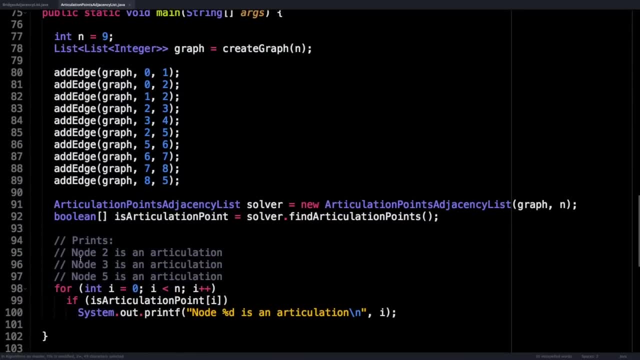 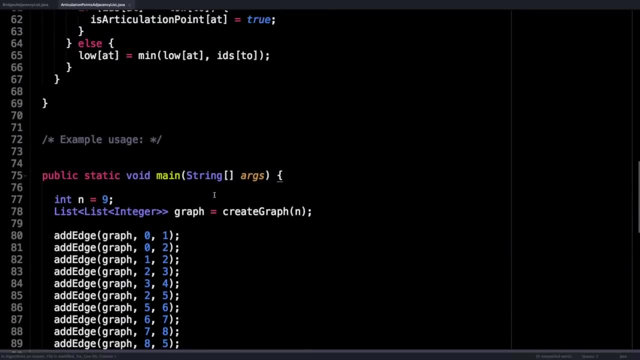 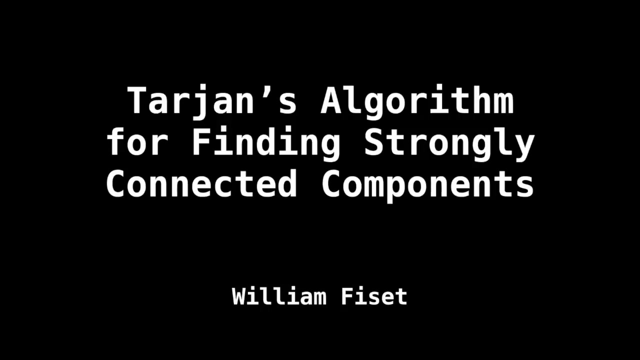 of course, we have to count the number of upcoming edges from the root. That's pretty important, And here's the same graph as before, But instead of printing bridges, it prints articulation points. So some very subtle differences between finding articulation points and bridges, but still very important ones. Today I want to talk about a fascinating topic And 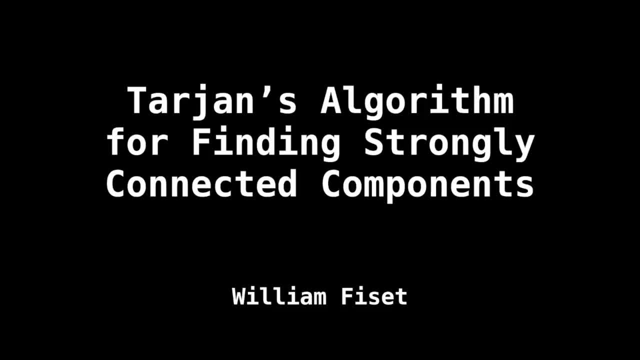 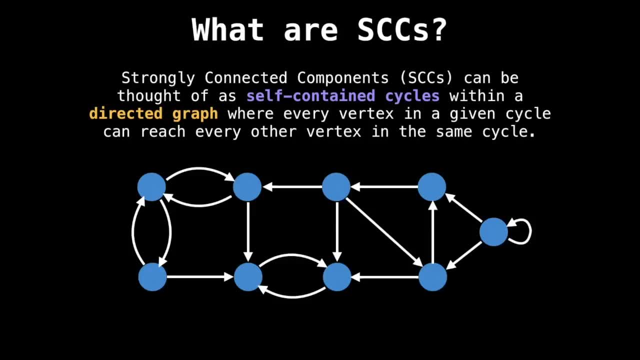 that is, strongly connected components and how we can use Tarzan's algorithm to find them. So what are strongly connected components or s CCS? I like to think of them as self contained cycles within a directed graph where, for every vertex in a given cycle, you can reach every other. 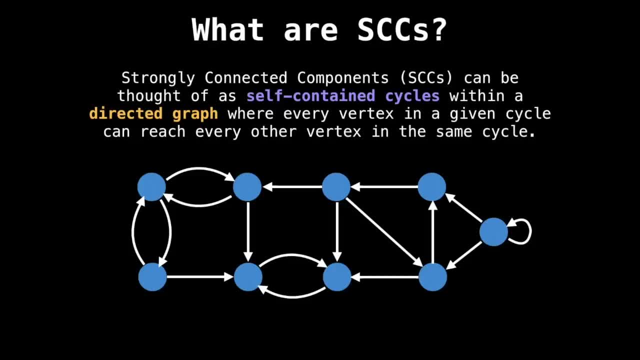 vertex in the same cycle. For example, in the graph below there are four strongly connected components. I've outlined them here in different colors. If you inspect each strongly connected component, you'll notice that each has its own self contained cycle And that for each component 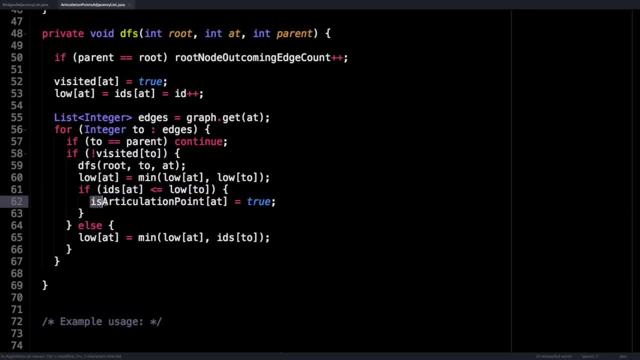 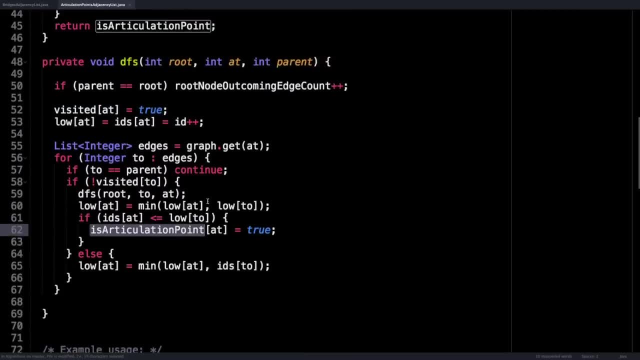 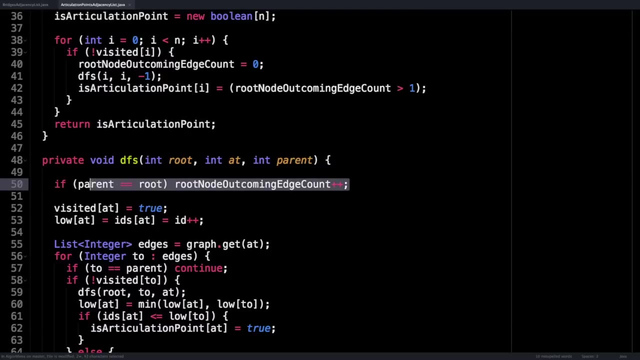 just less than to track cycles as well and mark off those as articulation points, And I think those are the major differences, If I didn't forget anything, between articulation points and bridges. of course, we have to count the number of outcoming edges from the 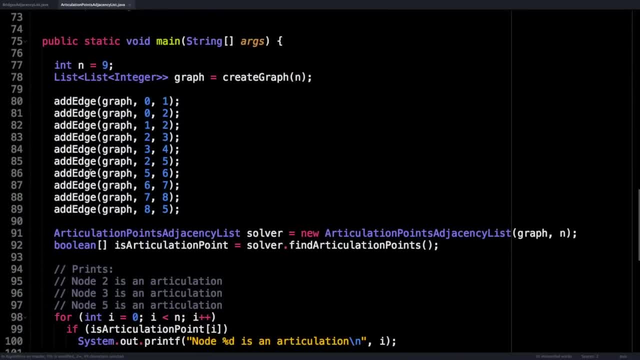 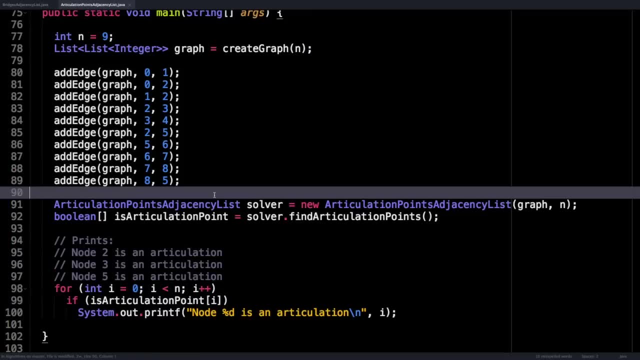 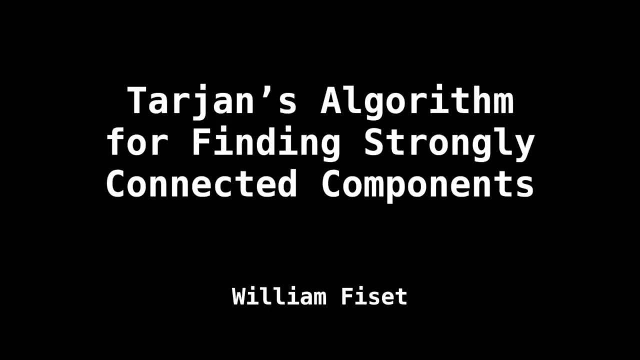 root. That's pretty important, And here's the same graph as before, But instead of printing bridges, it prints articulation points. So some very subtle differences between finding articulation points and bridges, but still very important ones. Today I want to talk about a fascinating topic, And that is 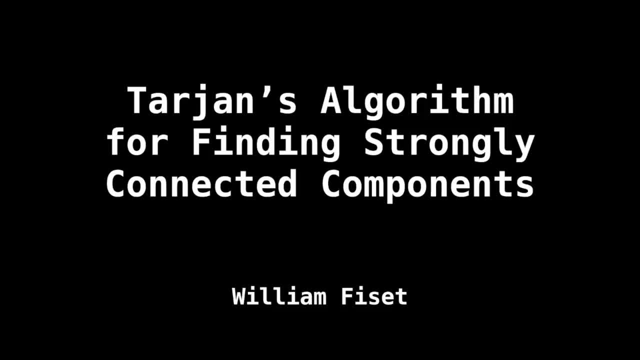 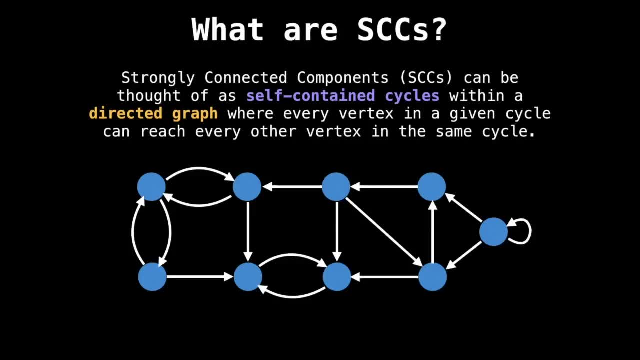 strongly connected components And how we can use Tarzan's algorithm to find them. So what are strongly connected components, or SCC? I like to think of them as self contained cycles within a directed graph where, for every vertex in a given cycle, you can reach every other. 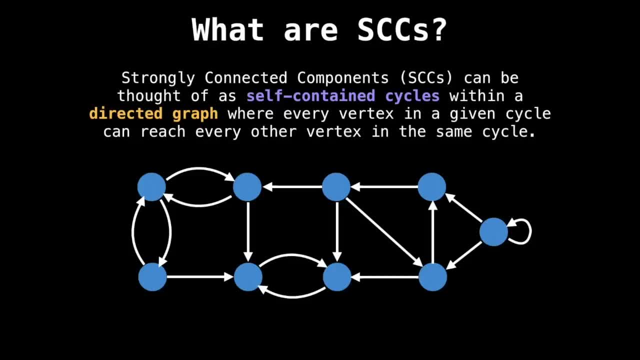 vertex in the same cycle. For example, in the graph below there are four strongly connected components. I've outlined them here in different colors. If you inspect each strongly connected component, you'll notice that each has its own self contained cycle and that for each 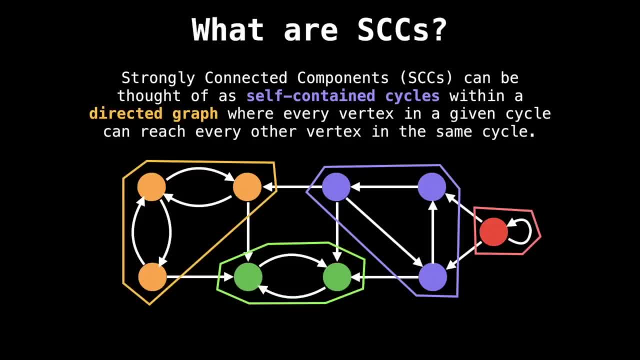 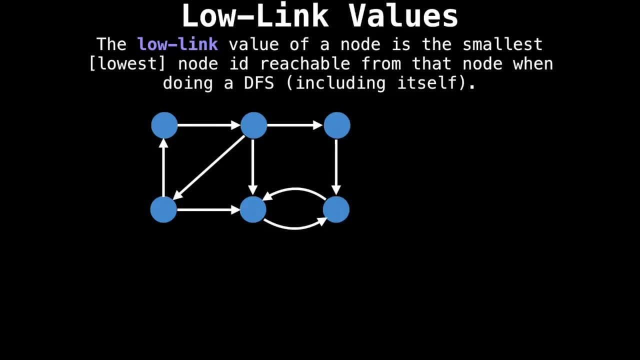 component. there's no way to find a path that leaves a component and comes back Because of that property. we can be sure that strongly connected components are unique within a directed graph. To understand Tarzan's strongly connected components algorithm, we're going to need to. 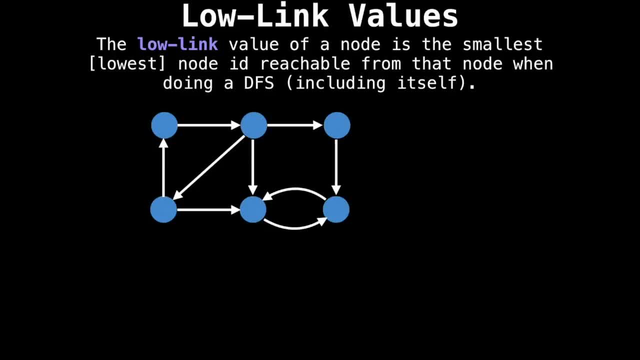 understand the context of each component. So let's start with the concept of a low link value. Simply put, a low link value is the smallest node ID reachable from that node, including itself. For that to make sense, we're going to need to label the nodes in our graph using a depth first search. Suppose we 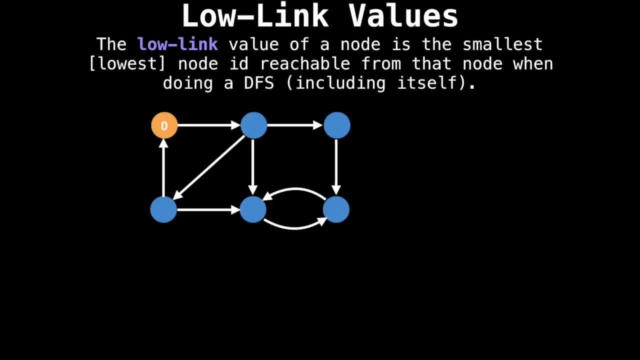 start at the top left corner and label that node with an ID of zero. Now we continue exploring that graph until we visit all the edges and have labeled a node with a low link value of zero. Alright, now that we're done labeling the nodes, inspect the graph and try and determine the low link value of each node. Again, the low. 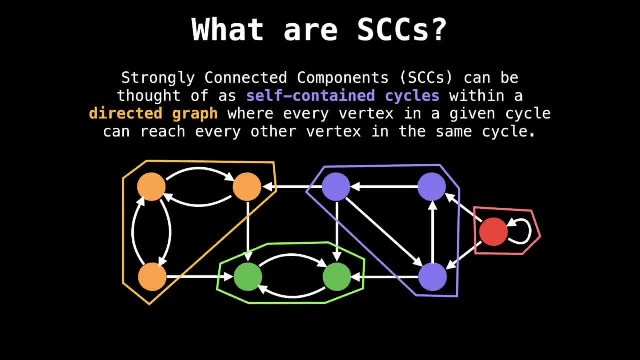 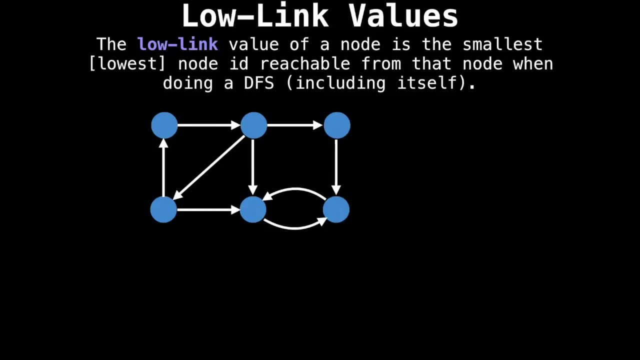 there's no way to find a path that leaves a component and comes back Because of that property. we can be sure that strongly connected components are unique within a directed graph. To understand Tarzan's strongly connected components algorithm, we're going to need to understand the concept of a low link value. Simply put, a low link value is the smallest node ID reachable from that node. 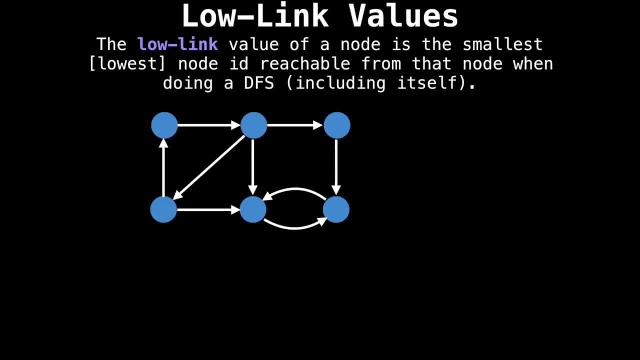 including itself, makes sense. we're going to need to label the nodes in our graph using a depth first search. Suppose we start at the top left corner and label that node with an ID of zero. Now we continue exploring that graph until we visit all the edges and have labeled all the 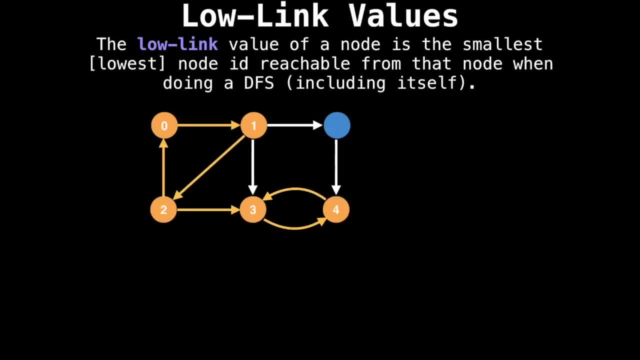 nodes. Alright, now that we're done labeling the nodes, inspect the graph and try and determine the low link value of each node. Again, the low link value of a node is the smallest node ID reachable from that node, including itself. For example, the loading value of node one. 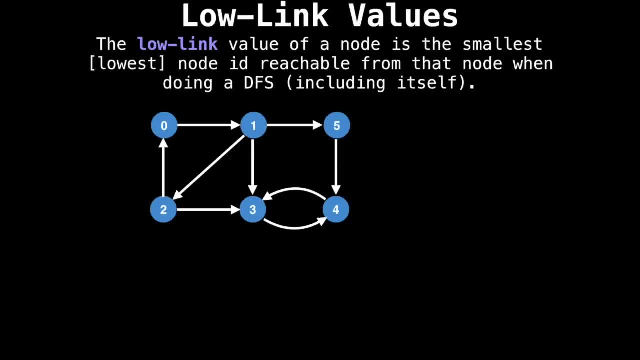 should be zero, since node zero is reachable from node one via some series of edges. Similarly, node four is loading value should be three, since node three is the lowest node that is reachable from node four. So if we assign all the loading values, we get the following setup: From this view, you realize that all nodes which have 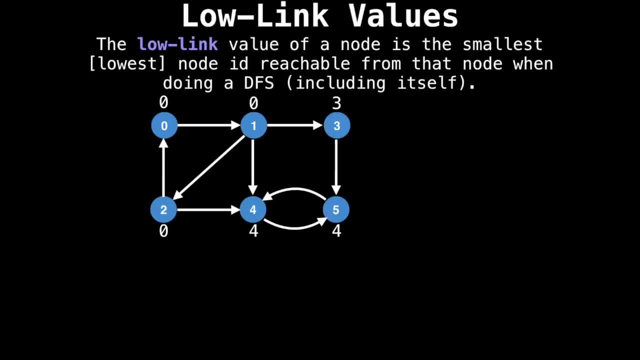 the same loading value belong to the same strongly connected component. If I now assign colors to each strongly connected component, we can clearly see that for each component all the low link values are the same. This seems too easy, right? Well, you're not wrong. there is a catch. The flaw with this technique? 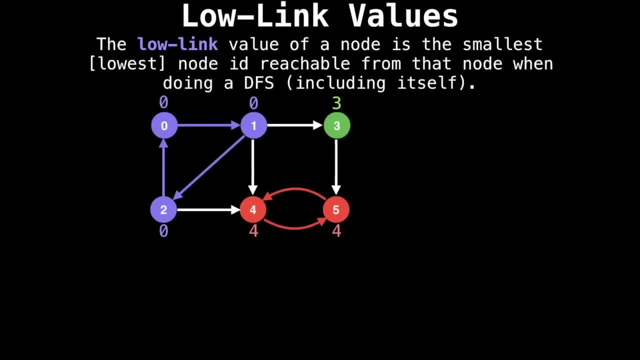 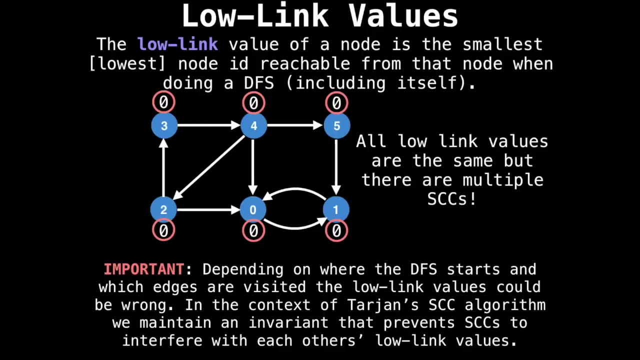 is that it is highly dependent on the traversal order of the depth first search, which for our purposes, is at random. For instance, in the same graph I rearrange the node IDs as though the Death first search started at the bottom middle node. In such an event, the low link values 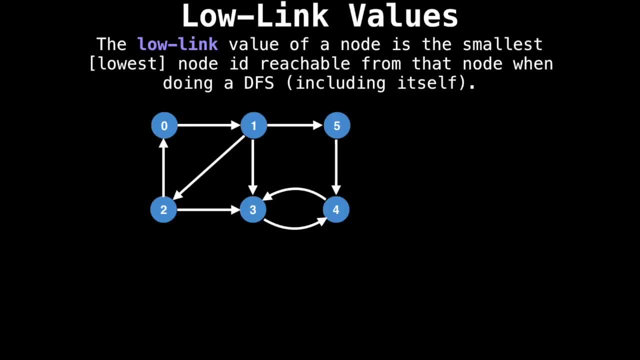 link value of a node is the smallest node ID reachable from that node, including itself. For example, the low link value of node one should be zero, since node zero is reachable from node one Via some series of edges. Similarly, node fours low link value should be three, since node three is the lowest node that is reachable from. 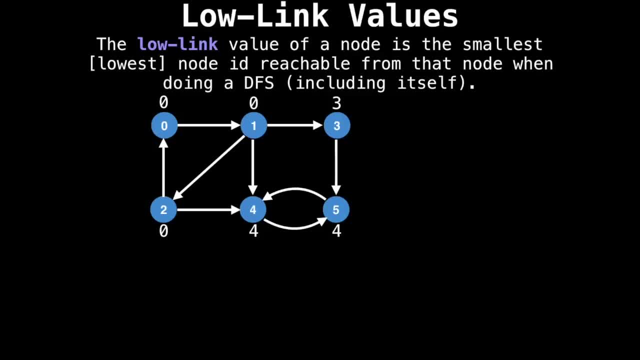 node four. So if we assign all the loading values, we get the following setup: From this view, you realize that all nodes which have the same low link value belong to the same strongly connected component. If I now assign colors to each strongly connected 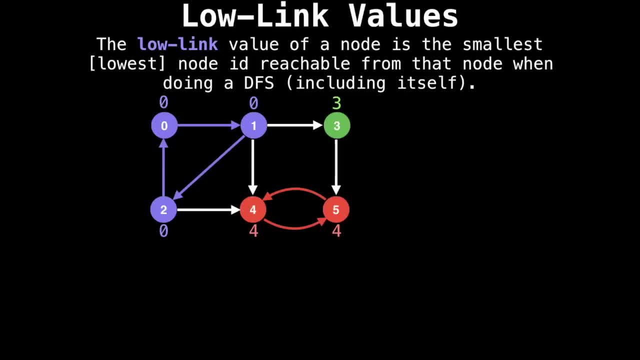 component. we can clearly see that for each component, all the low length values are the same. This seems too easy, right? Well, you're not wrong. there is a catch. The flaw with this technique is that it is highly dependent on the traversal order of the depth of search. 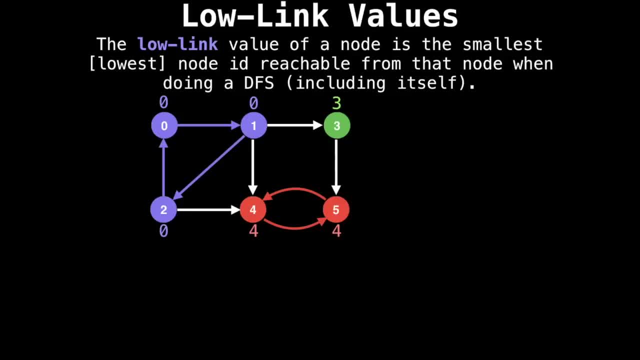 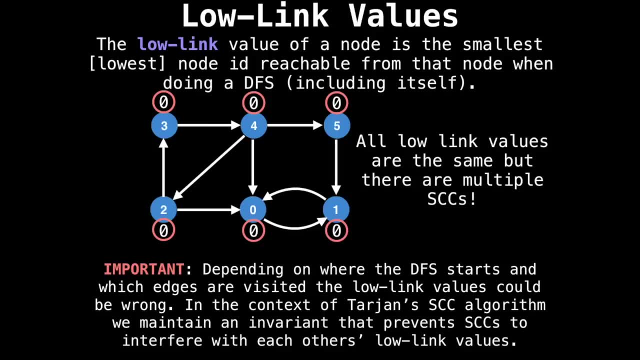 which, for our purposes, is at random. For instance, in the same graph I rearrange the node IDs as though the depth first search started at the bottom middle node And such an event, the link values will be incorrect. In this specific case, all the low link values are. 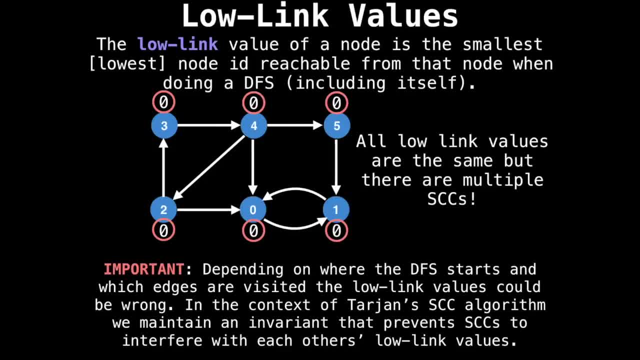 the same, But there clearly are multiple strongly connected components. So what is going on? Well, what's happening is that the low link values are highly dependent on the order in which the nodes are explored in our depth. first search, Speaker 2. So what's happening is that the low link values are highly dependent on the 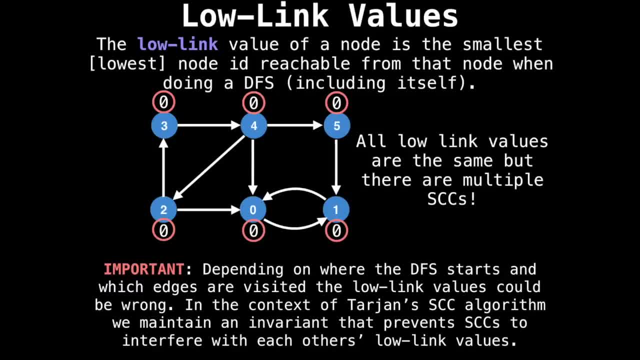 order in which the nodes are explored in our depth first search. so won't be worth asking we might not end up with a correct arrangement of node IDs for our low link values to tell us which nodes are in which strongly connected component. This is where tarjans algorithm. 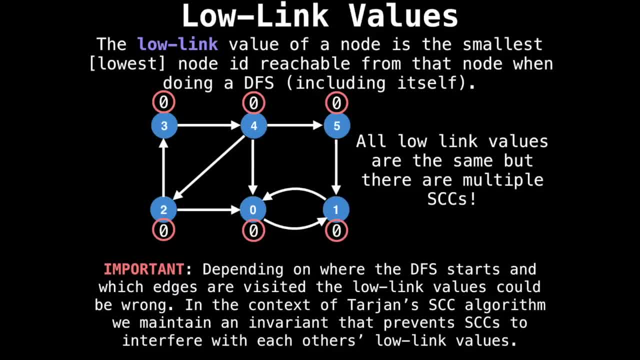 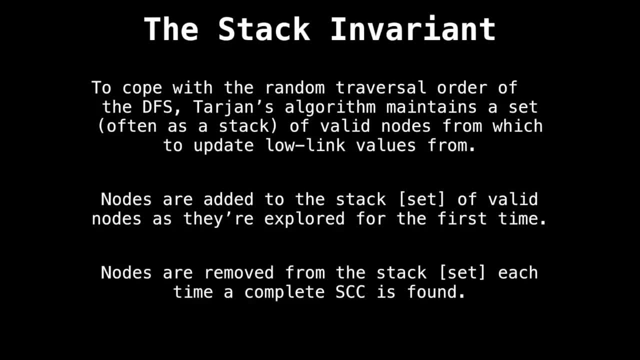 kicks in with its stack invariant to prevent strongly connected components from interfering with each other's low link values. So to cope with the random traversal order of the depth, first search tarjans algorithm maintains a set, often as a stack, of valid nodes from which to update low link values. from how the stack works is that nodes are added to the 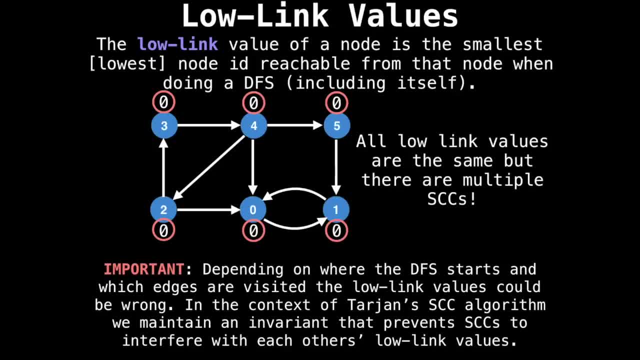 will be incorrect. In this specific case, all the low link values are the same, But there clearly are multiple strongly connected components. So what is going on? Well, what's happening is that the low link values are highly dependent on the order in which the 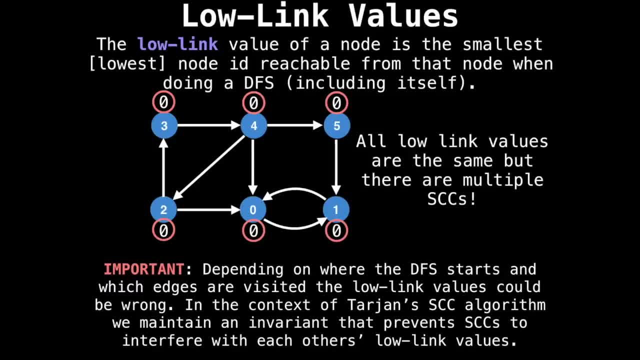 nodes are explored in our depth first search, So we might not end up with a correct arrangement of node IDs for our low link values to tell us which nodes are in which strongly connected component. This is where tarjans algorithm kicks in with its stack invariant to prevent. 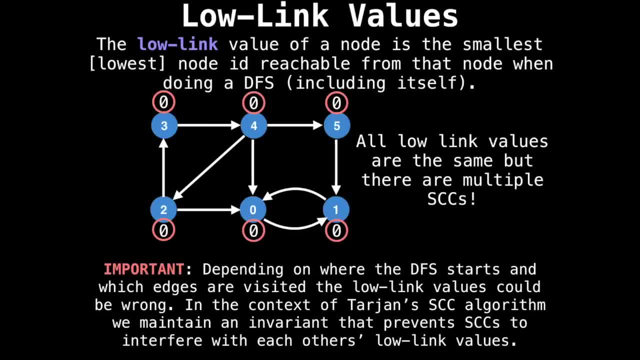 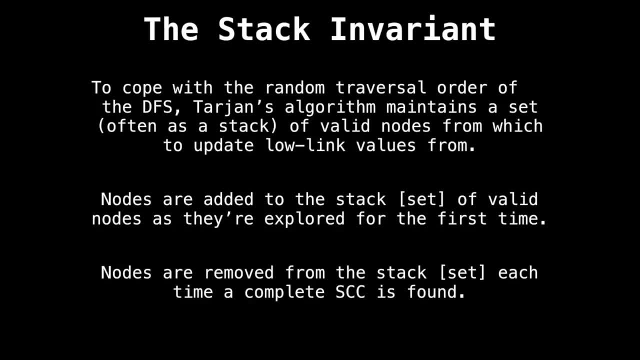 strongly connected components from interfering with each other's low link values. So, to cope with the random traversal order of the depth for search, tarjans algorithm maintains a set, often as a stack, of valid nodes from which to update low link values. from how the stack works is that nodes are: 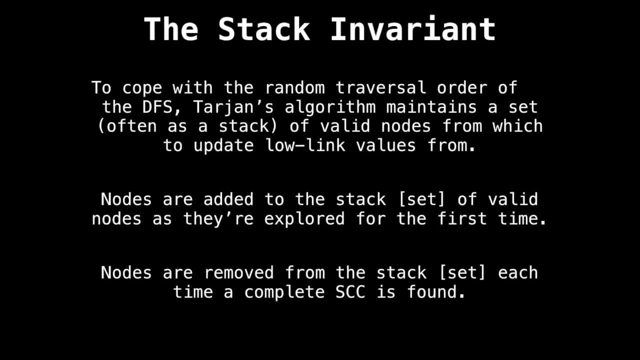 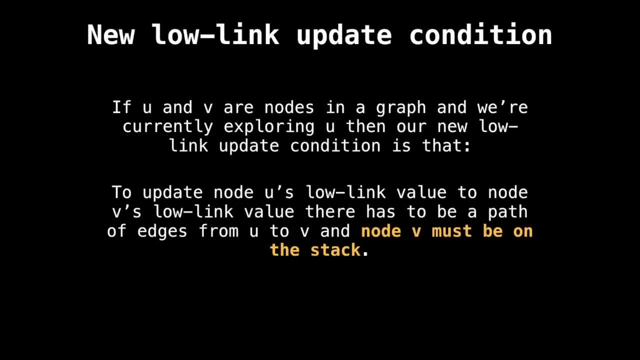 added to the stack as nodes are explored for the first time And nodes are removed from the stack each time a strongly connected component is found. Taking a step back, if the variables you find v are nodes in our graph and we are currently exploring node u, then our new low 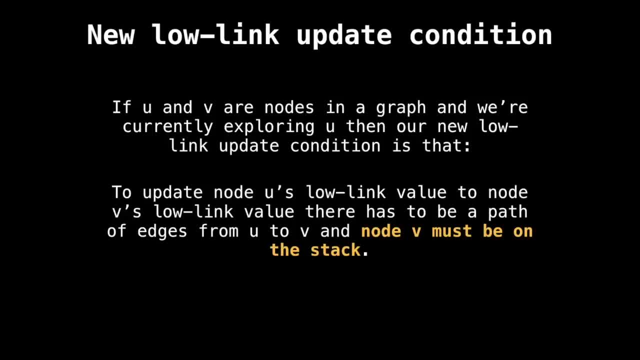 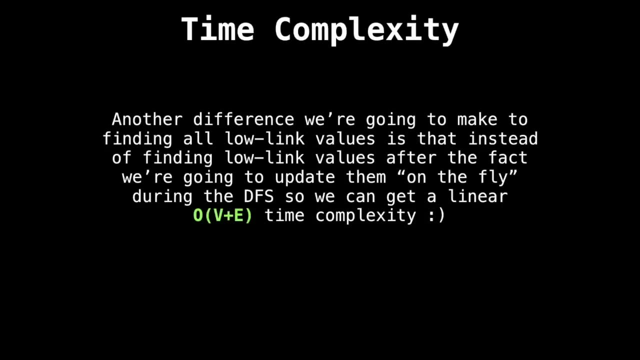 link. update condition is that to update node use loading value to node V's loading value, there has to be a path of edges from u to v and node v must be on the stack. Another small difference we're going to make to finding the correct loading values is that, instead 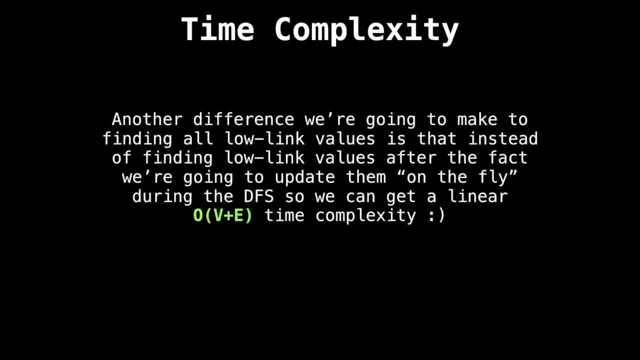 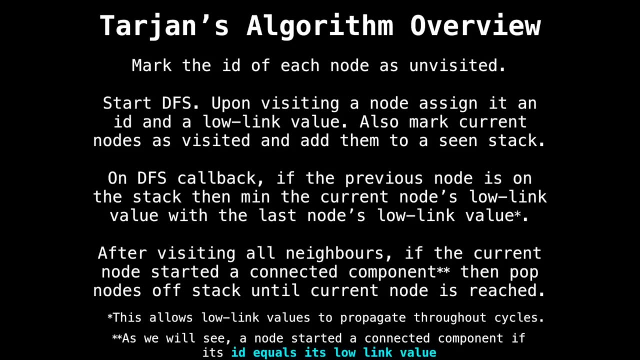 of finding all the loading values after the fact. we're going to update them as we do our depth first search on the fly, if you will. this will allow us to obtain a linear time complexity. We'll be doing an example in the following slides, But this is tarjans algorithm in a 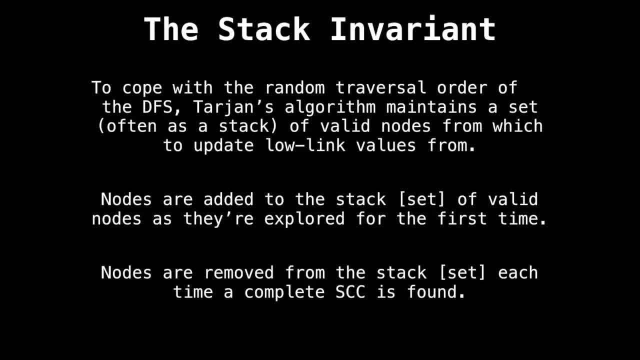 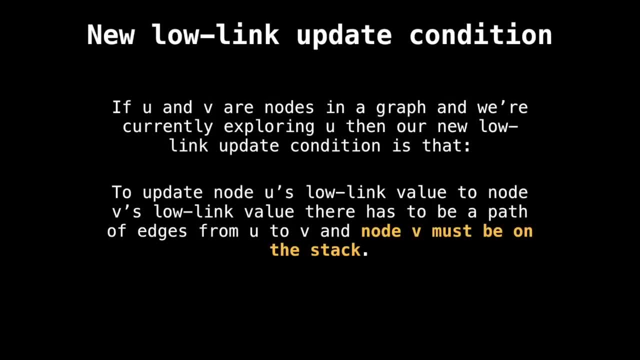 stack, as nodes are explored for the first time And nodes are removed from the stack each time a strongly connected component is found, Taking a step back. if the variables u and v are nodes In our graph and we are currently exploring node u, then our new low link update condition. 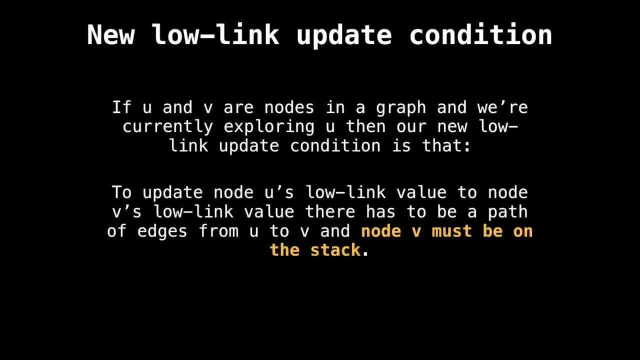 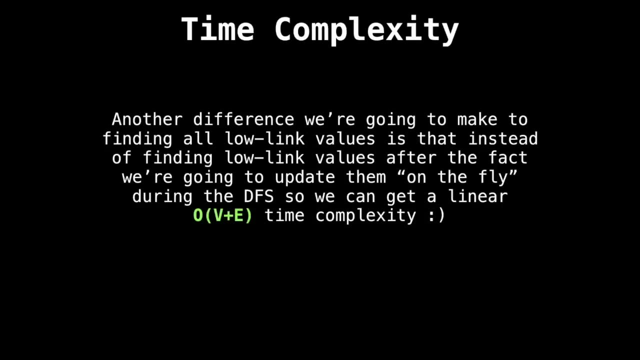 is that to update node use low link value to node V's low link value, there has to be a path of edges from u to v and node v must be on the stack. Another small difference we're going to make to finding the correct low link values is that, instead of finding 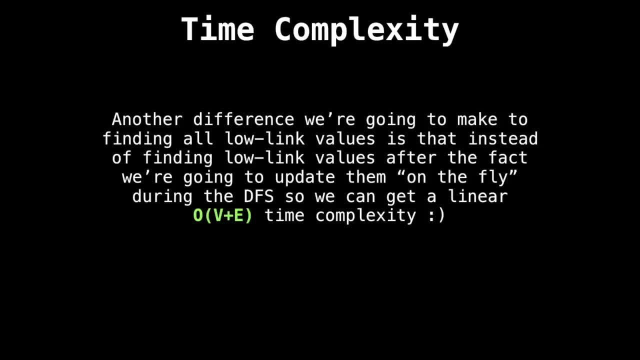 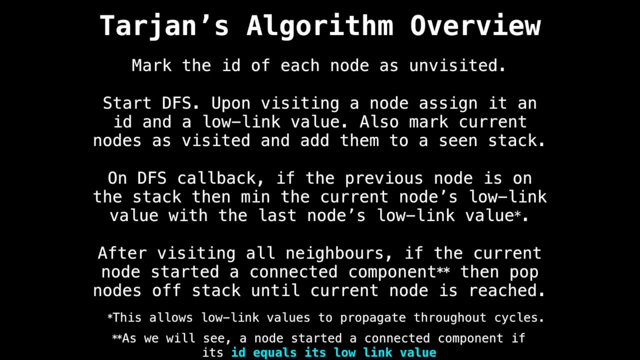 all the low link values after the fact. we're going to update them As we do our depth first search on the fly, if you will. this will allow us to obtain a linear time complexity. We'll be doing an example in the following slides, But this is tarjans algorithm in a nutshell start. 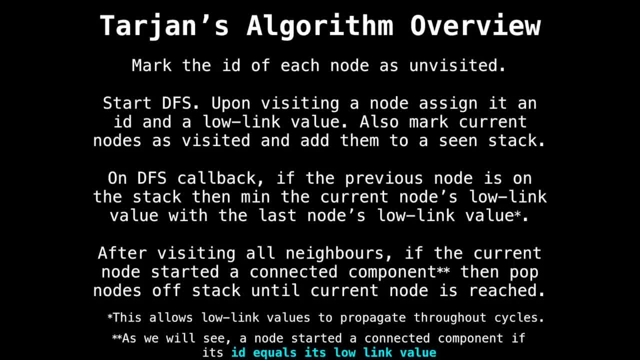 out and mark each node as unvisited. Start the depth first search somewhere and don't stop until all the nodes are visited. Upon visiting a node, you'll notice that the nodes are not visited. After visiting a node, assign it an ID and a low link value. Additionally, also mark 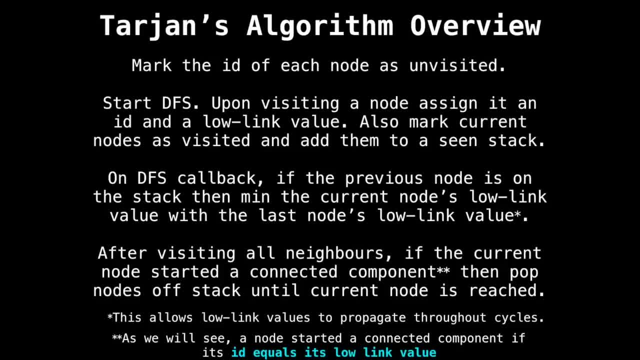 the node as visited and add it to the scene stack On the depth first search callback. after the recursion comes back. If the previous node is on the stack, then min the current nodes- low link value with the last nodes- low link value. This is essentially what will. 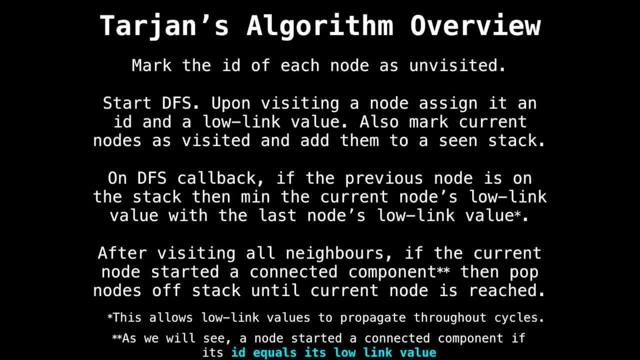 allow low link values to propagate throughout cycles. After visiting all the nodes, you'll notice that the nodes are not visited. After visiting all nodes neighbors, if the current node started the strongly connected component, then pop off all nodes from the stack which are in the strongly connected component. You know a node started a strongly connected. 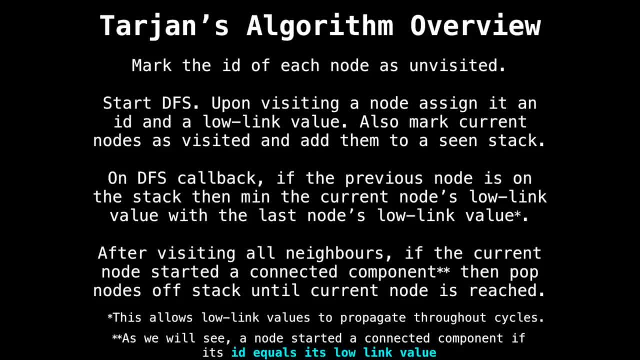 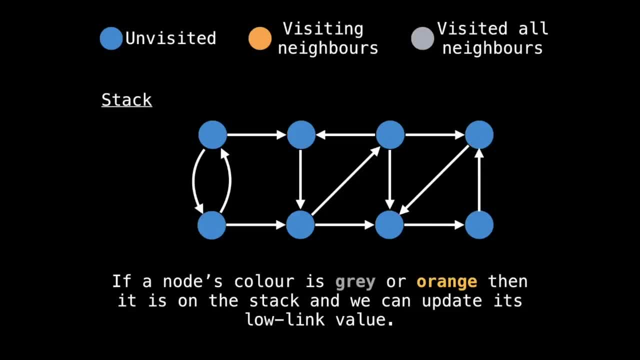 component if its ID is equal to its low link value. I'll let you think about that a bit more and it'll start making sense. Let's do an example. I'm going to mark unvisited nodes as blue nodes, for which the depth first search is unvisited. 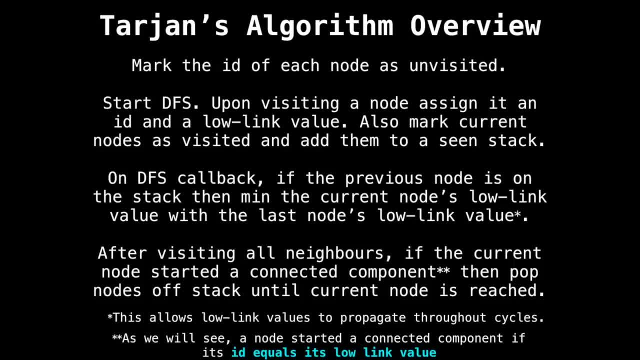 nutshell: Start out and mark each node as unvisited. Start the depth for search somewhere and don't stop until all the nodes are visited. Upon visiting a node, assign it an ID and a low link value. Additionally, also mark the node as visited and add it to the scene. stack On the depth: first search callback. 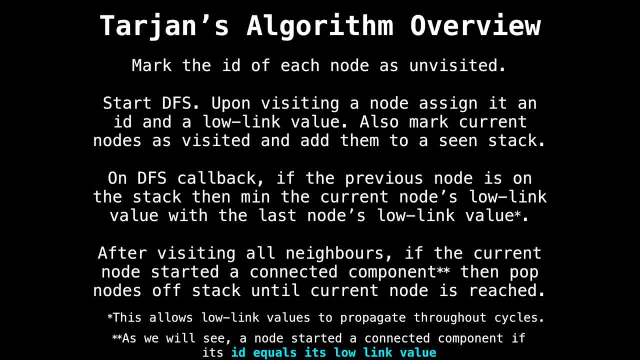 after the recursion comes back. if the previous node is on the stack, then min the current nodes- low link value with the last nodes- low value. This is essentially what will allow loading values to propagate throughout cycles. After visiting all nodes neighbors, if the current node started, the strongly connected 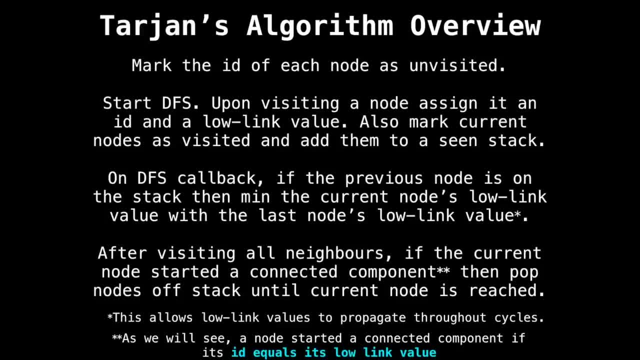 component, then pop off all nodes from the stack which are in the strongly connected component. You know a node started a strongly connected component if its ID is equal to its loading value. I'll let you think about that a bit more And it'll start making sense. 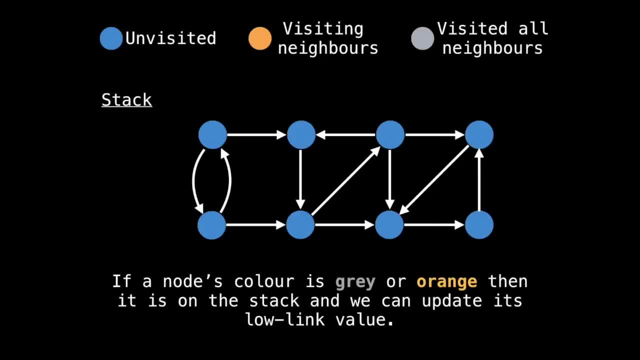 Let's do an example. I'm going to mark unvisited nodes as blue, nodes for which the depth first search is still exploring some neighbors as orange, and nodes which the depth first search has explored all of its neighbors as gray. Note that if a node is orange or gray, then 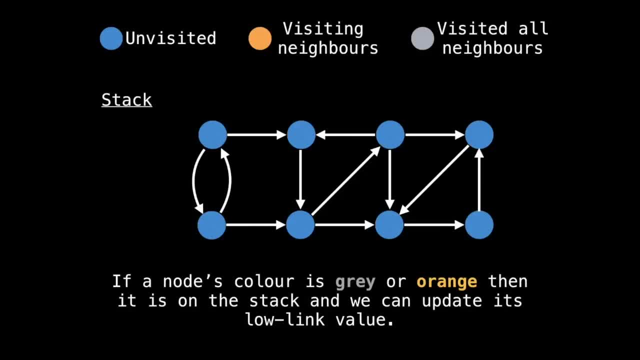 it is on the stack and we can update its loading value. I will also be tracking the nodes which are on the stack in the left column, So keep your eyes peeled on that as well. So let's start our depth first search. So just randomly pick a node. 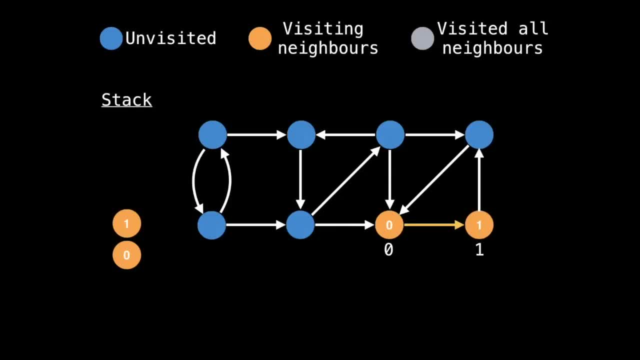 and start there. As we explore unvisited nodes, give each node an ID and a low link value equal to the ID. So now we're at node two and our only option is to now visit node zero. Since node zero is already visited, we don't want to visit it again. 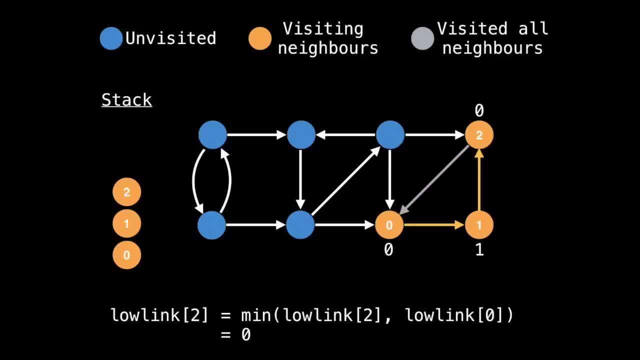 So now we backtrack on the backtracking. Since node zero is on the stack, we take the minimum of the current nodes- low link value and node zeros, low link value. Similarly, now min the low link value of the node we were just at, which is node one, with node two And also. 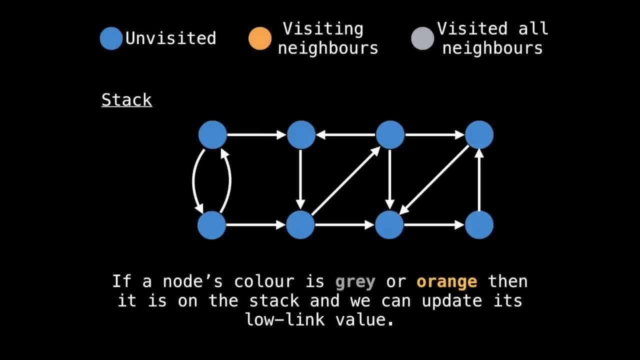 nodes for which the depth first search is still exploring some neighbors as orange, and nodes which the depth first search has explored all of its neighbors as gray. Note that if a node is orange or gray, then it is on the stack and we can update its loading value. 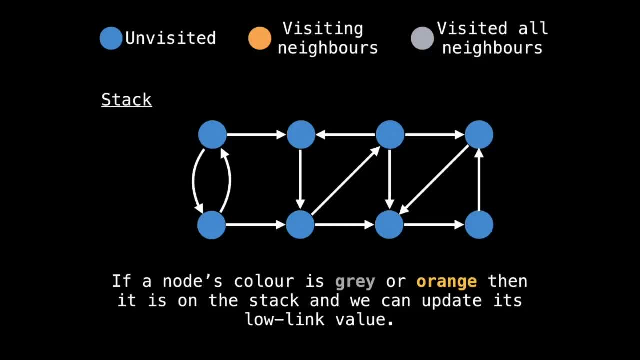 I will also be tracking the nodes which are on the stack in the left column, So keep your eyes peeled on that as well. So let's start our depth first search. So just randomly pick a node and start there As we explore unvisited nodes, give each node an ID and a low link value. 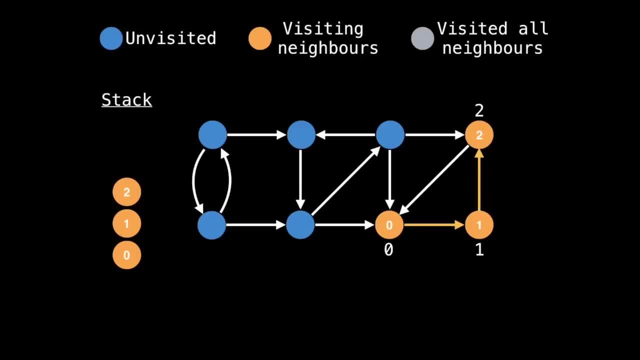 equal to the ID. So now we're at node two and our only option is to now visit node zero. Since node zero is already visited, we don't want to visit it again. So now we backtrack on the backtracking Since node zero. 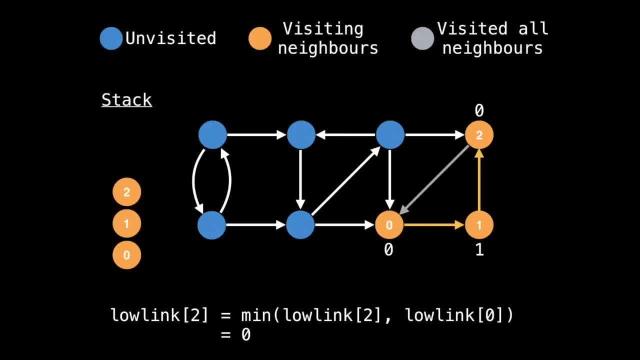 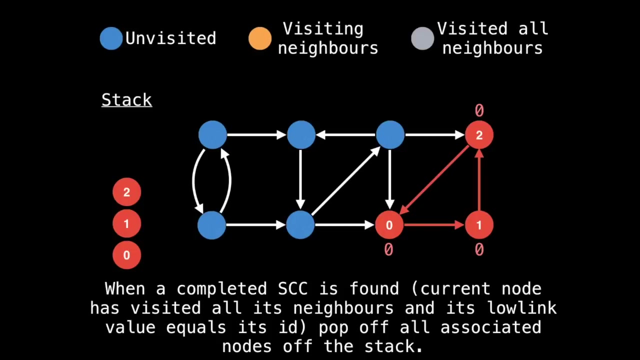 is on the stack. we take the minimum of the current nodes- low link value and node zeros, low link value. Similarly, now min the low link value of the node we were just at, which is node one, with node two, And also the same for node zero, Upon returning back to node 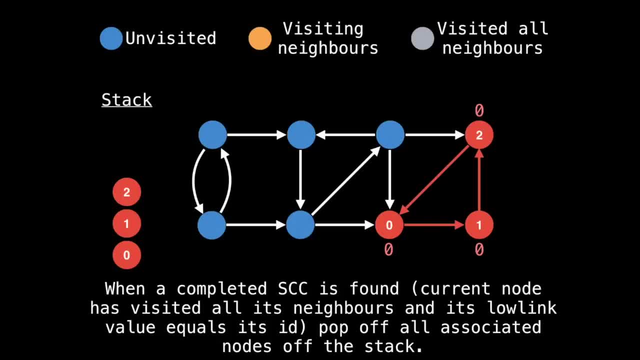 zero, we realized that we've actually finished a strongly connected component. So now we're at node two. Since we visited all the neighbors of node zero and its ID is equal to its low link value, This means we need to remove all the nodes associated with a strongly connected 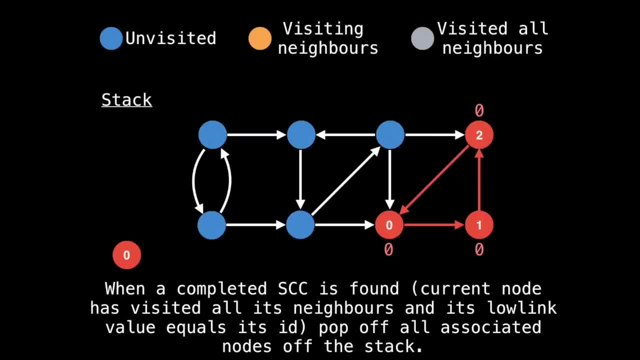 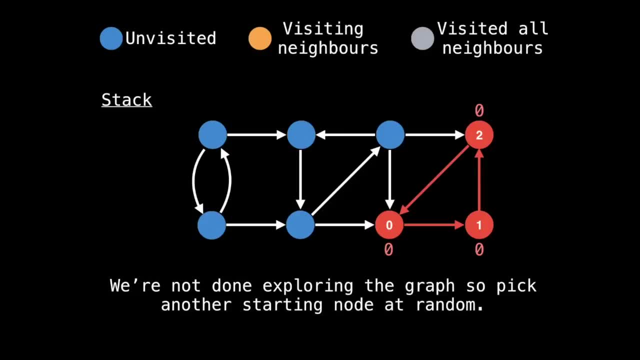 component from the stack. However, we're not done exploring the graph, So pick another node at random. Let's start at node three And go right. Now our only option is to go down. Now we're at node five. let's take the edge to node. 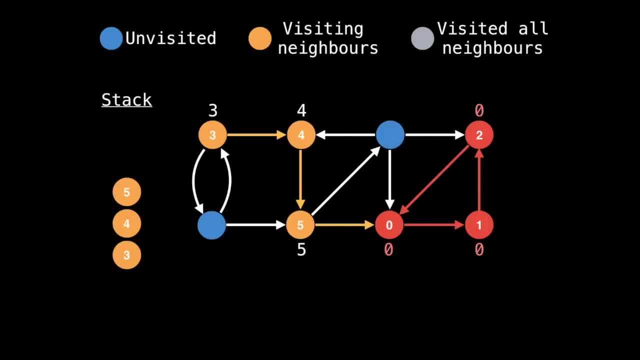 zero. So node zero is already visited So we can't go there. On the callback we noticed that node zero is not on the stack at the moment So we can't min. node five is low link value against node zero. This is actually very, very good, Because if we did, then we 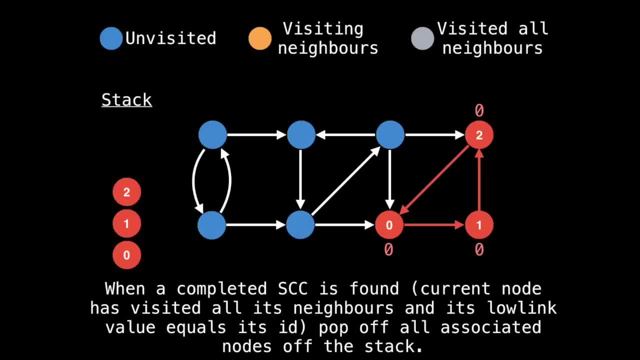 the same for node zero. Upon returning back to node zero, we realize that we've actually finished a strongly connected component, Since we visited all the neighbors of node zero and its ID is equal to its low link value. This means we need to remove all the nodes associated with a strongly connected 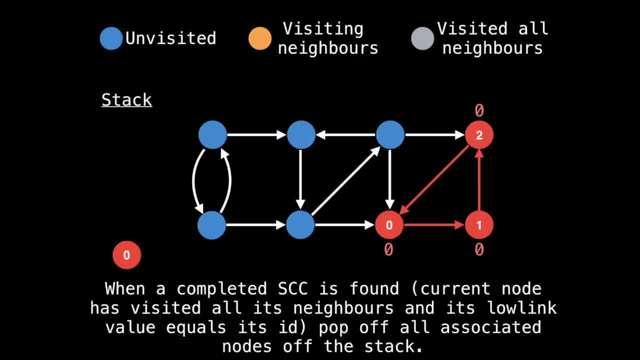 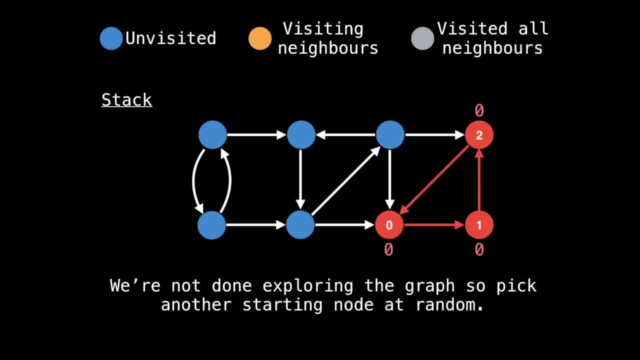 component from the stack. However, we're not done exploring the graph, So pick another node at random. Let's start at node three And go right. Now our only option is to go down. Now we're at node five. let's take the edge to node zero. So node zero is already visited, So we 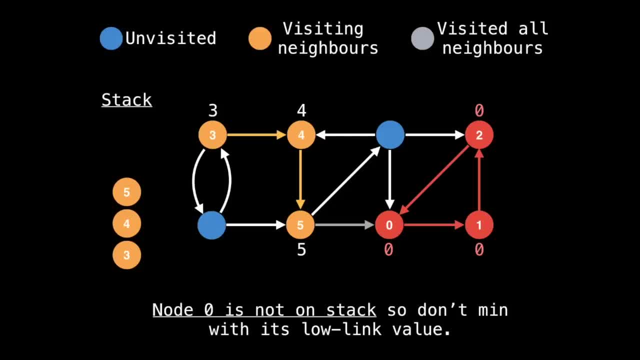 can't go there. On the callback we notice that node zero is not on the stack at the moment, So we can't min. node five is low link value against node zero. This is actually very, very good, Because if we did, then we would contaminate the strongly connected. 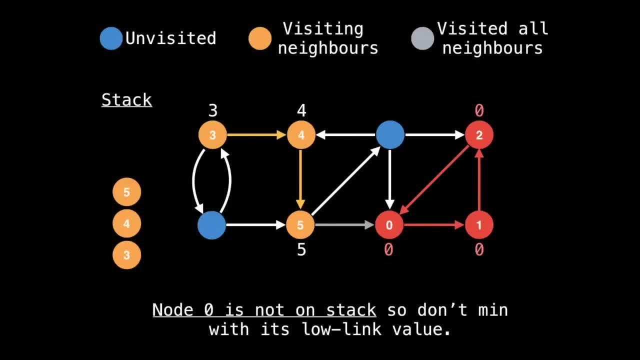 component node five as part of with a lower low link value, which node zero has to offer. So let's go to node six. So now we have three edges to choose from. Let's take the one on the right. Node two is not on the stack, So don't min with its low link value. Now let's 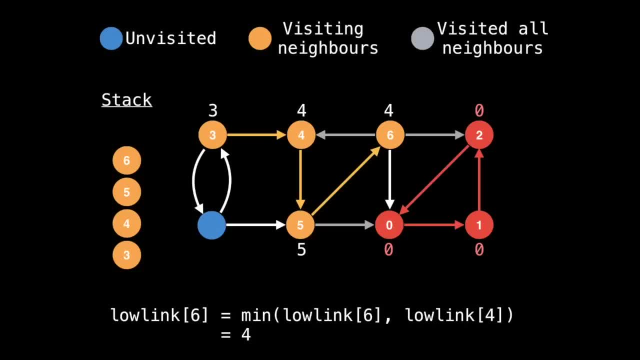 take the left edge to node five And then we're going to go to node six And then we're going to take the one on the right And then we're going to take the one on the left edge to node four. node four is on the stack So we can manage low link value giving node six also. 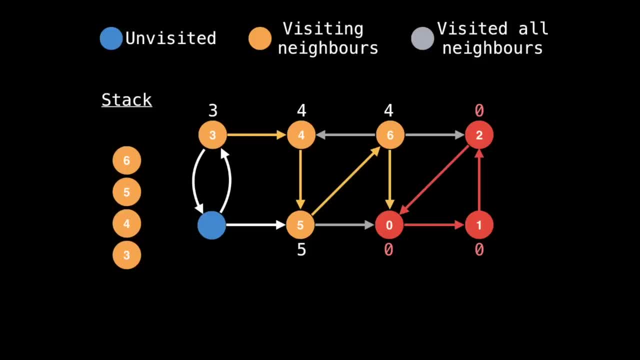 a low link value of four. The last edge we need to visit is the one going to node zero. This is a situation where node zero is not on the stack, So we can't min with its low link value. On the callback, node five can min with. node six is low link value because 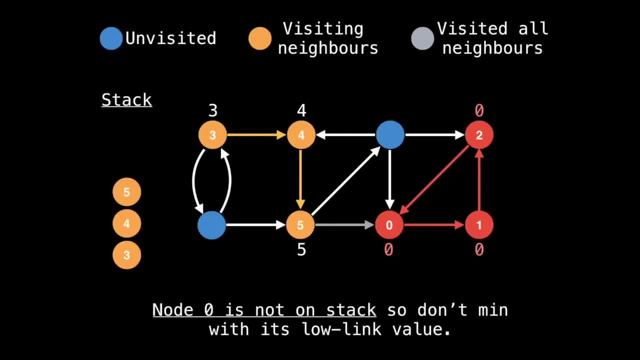 would contaminate the strong connected component, node five, as part of with a lower low link value, which node zero has to offer. So let's go to node six. So now we have three edges to choose from. Let's take the one on the right. Note two is not on the stack, So don't min with its low link. 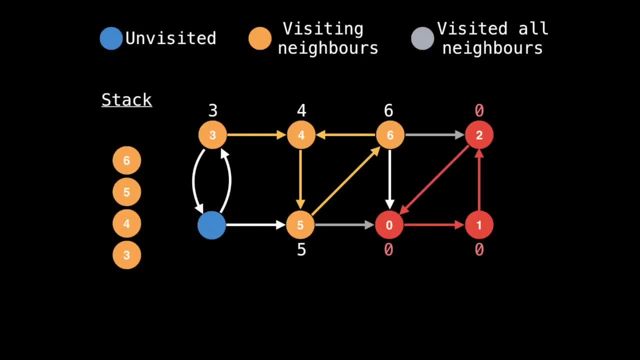 value. Now let's take the left edge to node four. Note: four is on the stack, So we can manage low link value, giving node six also a low link value of four. The last edge we need to visit is the one going to node zero. This is a situation where node zero is not on the stack, So we can't. 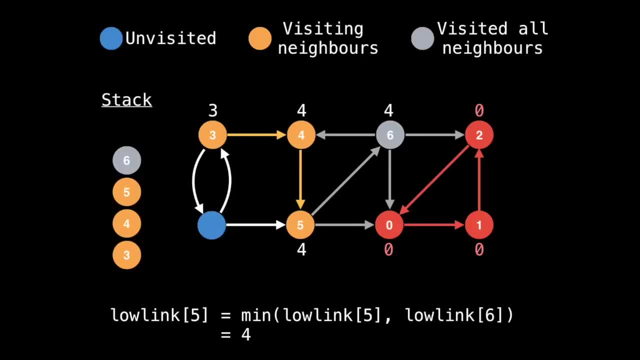 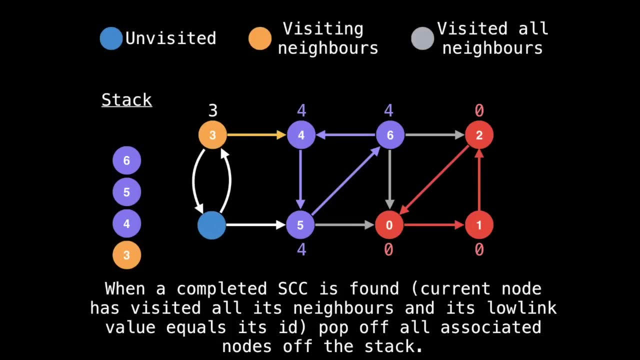 min with its low link value. On the callback, node five can min with. node six is low link value because it is on the stack. Similarly for node four. Coming back to node four, we visited all its neighbors and its IDs equal to its low link value. So it marks the start of a strongly connected component. 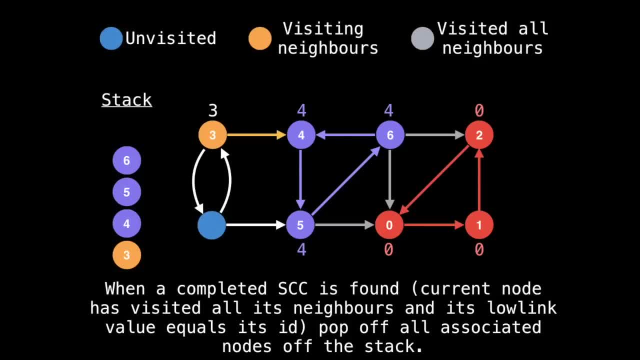 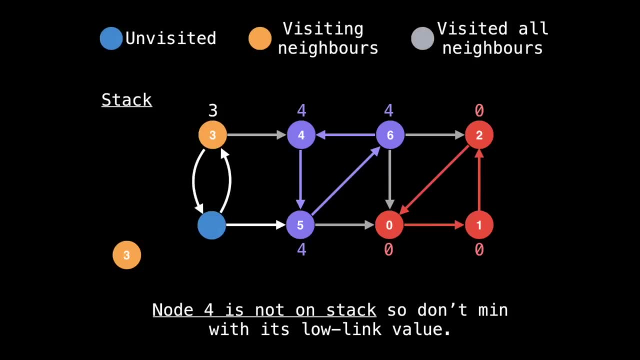 So we now have to remove all associated nodes in the strongly connected component from the stack. These would be all of the purple nodes. Now, coming back to node three, we cannot min its low link value with node four because we just removed node four from the stack. 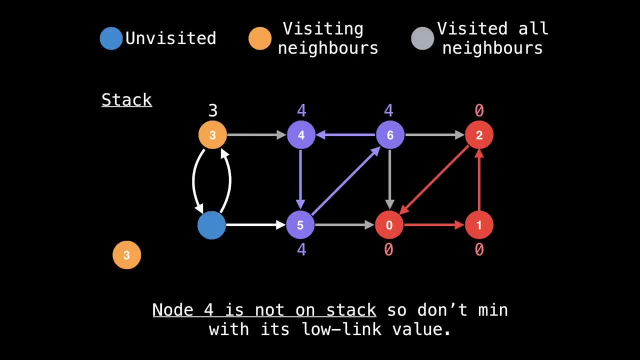 you will also notice that node three's ID is equal to its low link value, So it should be the start of a strongly connected component. However, we have not finished visiting all of node three's neighbors, So we cannot make that assessment just yet. Now see the downward. 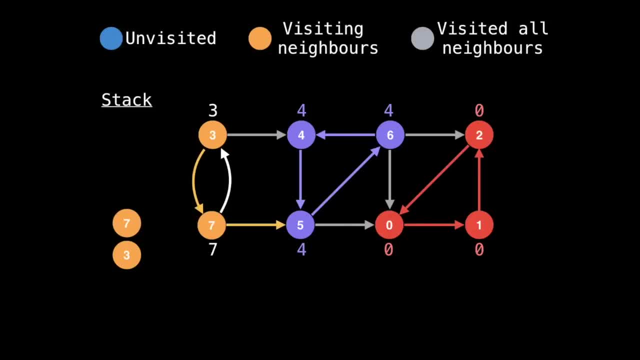 edge to visit node seven. Now take the edge to node five On the callback. notice that node five is not in the stack so we don't min with its low link value. now up to node three On the callback. we can min with node three's low link, since node three is on the 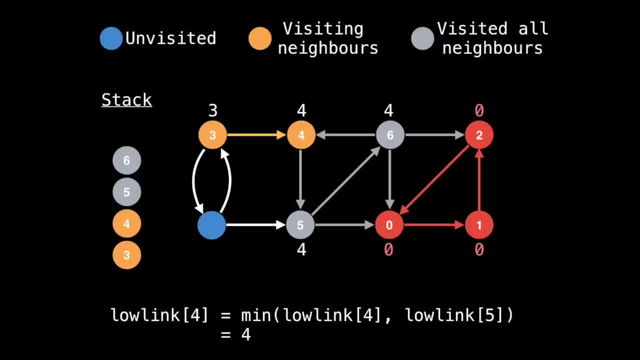 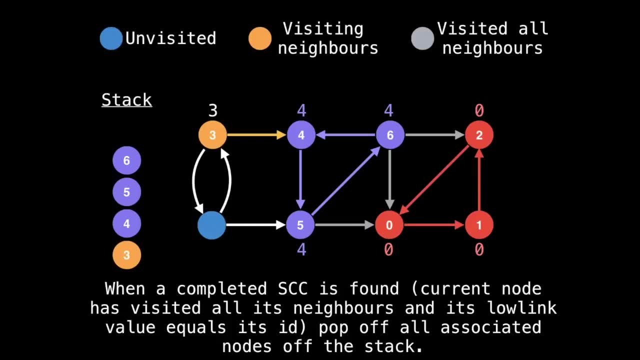 it is on the stack. Similarly for node five. Coming back to node four, we visited all its neighbors and its ID is equal to its low link value. So it marks the start of a strongly connected component. So we now have to remove all associated nodes in the strongly connected component from the stack. These would be all. 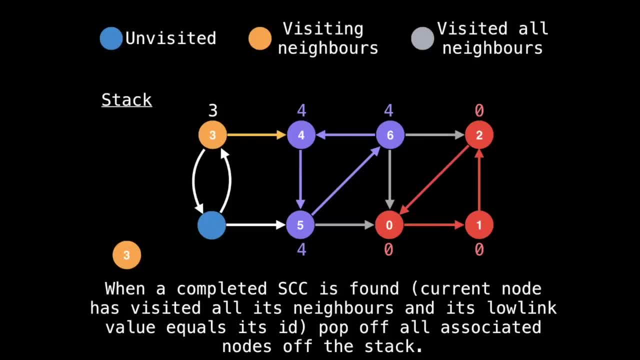 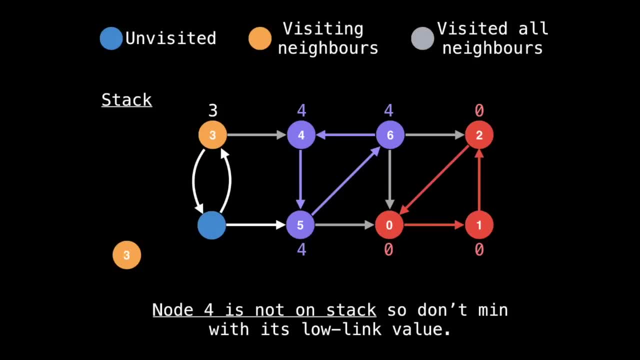 of the purple nodes. Now, coming back to node three, we cannot min its low link value. So we can't min its low link value with node four, because we just removed node four from the stack. You will also notice that node threes ID is equal to its low link value, So it should. 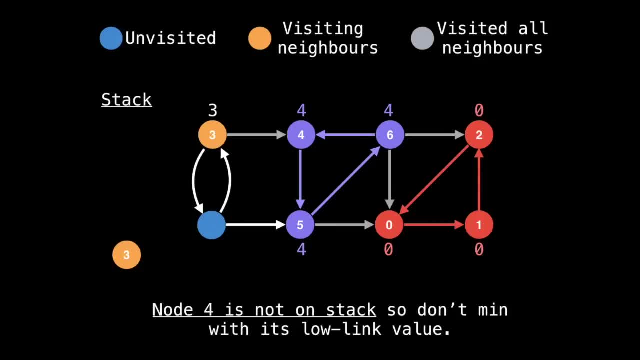 be the start of a strongly connected component. However, we have not finished visiting all of node threes neighbors So we cannot make that assessment just yet. Now see the downward edge to visit node seven. Now take the edge to node five. On the callback, notice that node five is not in the stack. 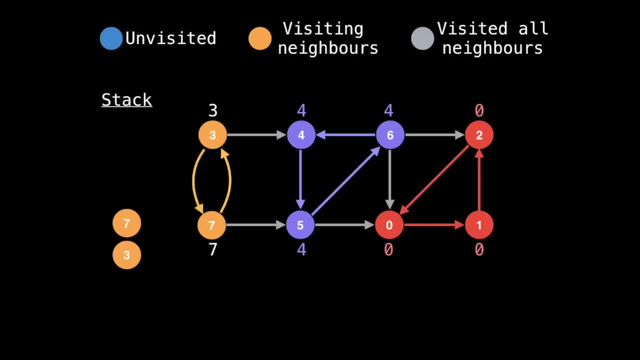 So we don't min with its low link value. Now, up to node three On the callback, we can min with node threes low link. since node three is on the stack, Also min with node seven. So now we've finished with the last strongly connected component. all we need to do is 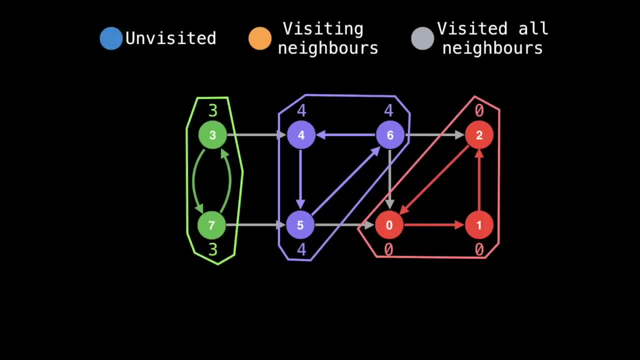 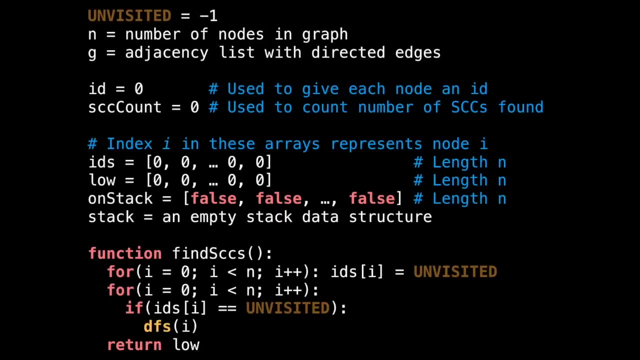 remove all associated nodes from the stack, And that's how Tarzan's algorithm works: to find strongly connected components. Very beautiful, isn't it? Let's look at some pseudocode for how this works. I think it will solidify your understanding. To get started in the global or class scope, I defined a few variables. 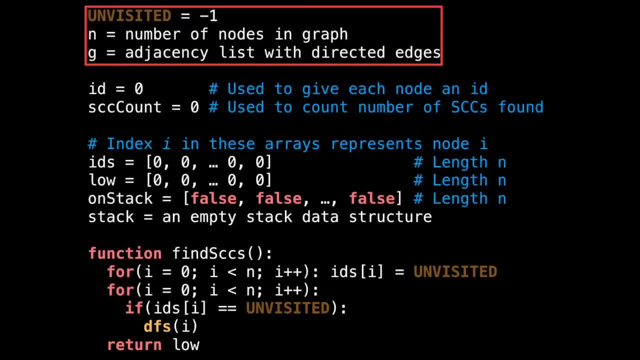 that will need. the first is a constant to represent unvisited nodes. Then comes n, the number of nodes in the graph, and G and adjacency list of directed edges. Both n and g are inputs to this algorithm. Then comes two variables: ID to give each node. 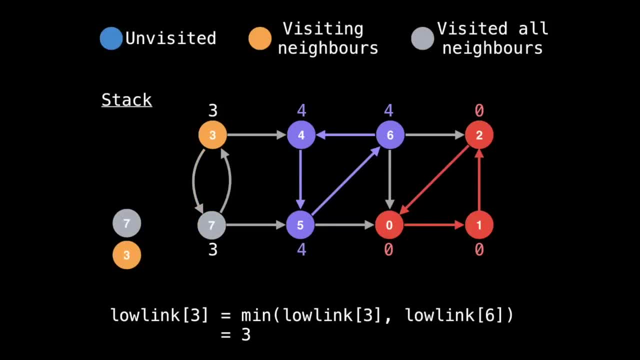 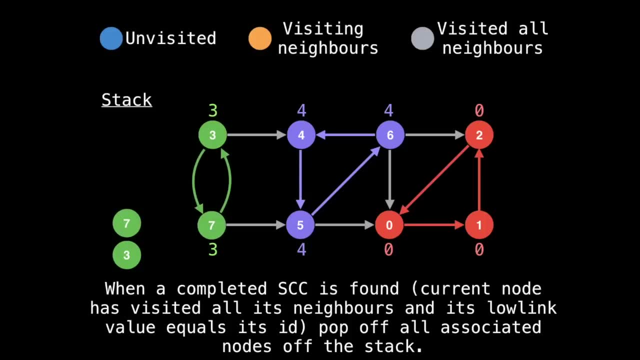 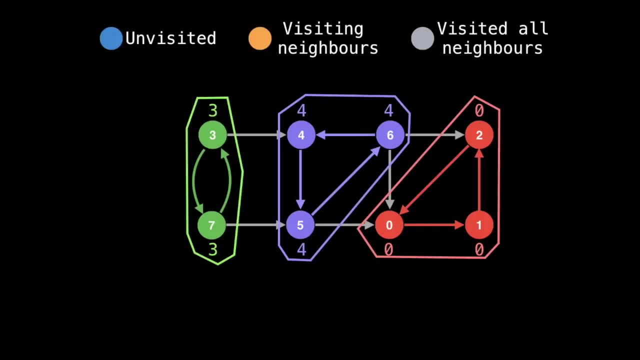 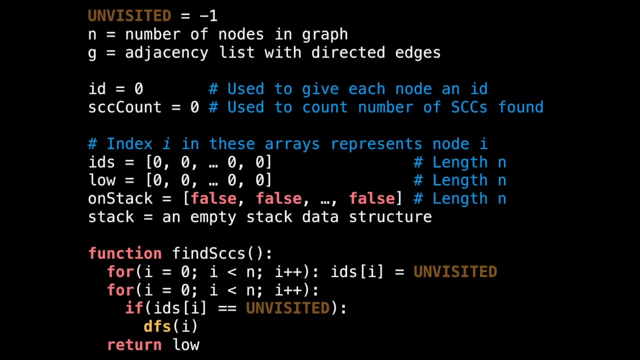 stack Also min with node seven. So now we've finished with the last strongly connected component. All we need to do is remove all associated nodes from the stack, And that's how tardians algorithm works. components- Very beautiful, isn't it? Let's look at some pseudocode for how this works. 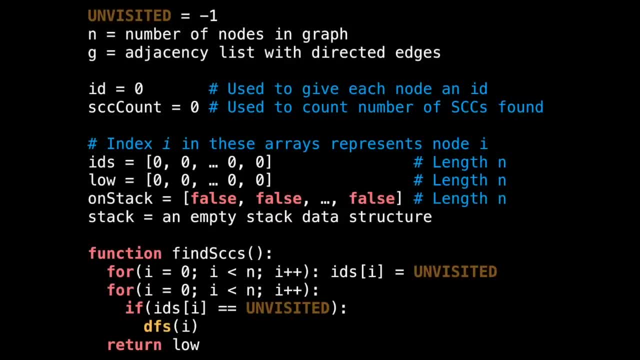 I think it will solidify your understanding. To get started in the global or class scope, I defined a few variables that we'll need. The first is a constant to represent unvisited nodes. then comes n- the number of nodes in the graph, and G and adjacency list of directed. 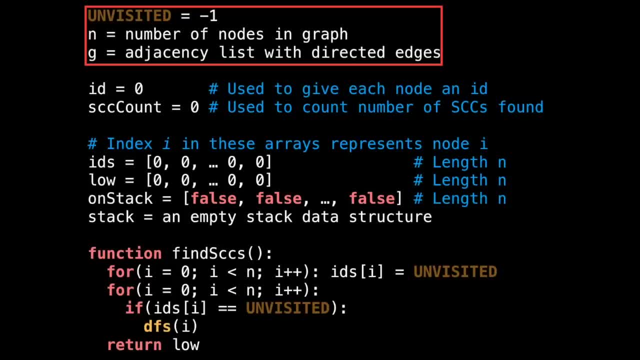 edges. Both n and G are inputs to this algorithm. then comes to variables: ID, to give each node an ID, and s CC count to track the number of strongly connected components. After I define a few arrays which store auxiliary information about the nodes, Then I define a few arrays which store auxiliary information about the 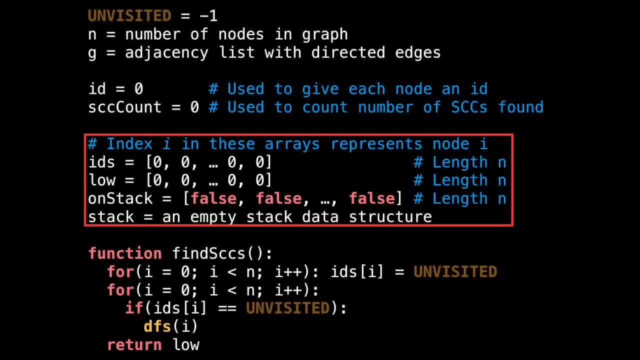 nodes. Then I define a few arrays which store auxiliary information about the nodes. Then I define a few arrays which store auxiliary information about the nodes in our graph. The first array is IDs, which stores the ID of each node. then is low to store the low link. 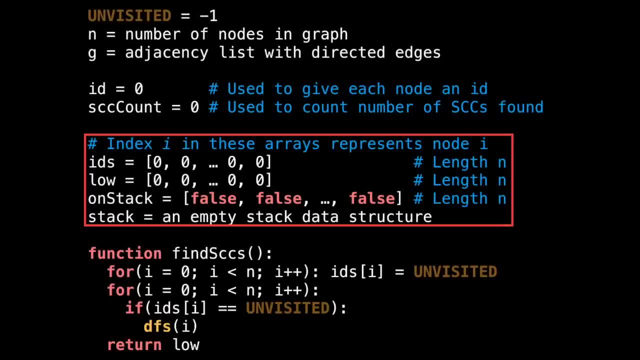 values And finally, on stack, to track whether or not a node is on the stack. Finally, is the stack data structure itself, which should, at minimum, support push and pop operations Inside the find s CCS method. The first thing I do is I'm going to do a little bit of a. 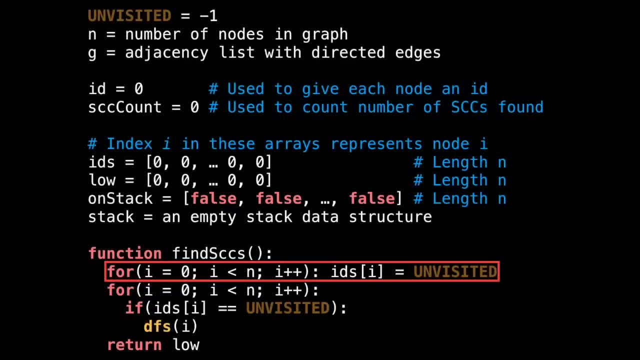 test. So I'm going to assign the ID of each node to be unvisited. The IDs array will be serving to track whether or not a node has been visited, as well as what a nodes ID is. In the following loop I iterate through all the nodes in the graph. There I start a depth first search on: 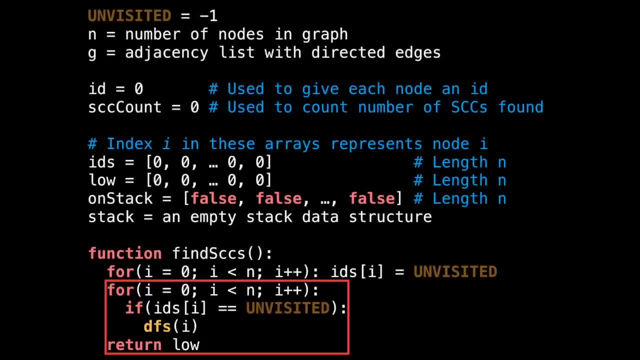 node i. if node i has not yet been visited. At the end I return the array low and array of low link values, which will be the final output of the algorithm. Now let's look at what's happening inside the depth first search method, which is really where all the magic happens. So 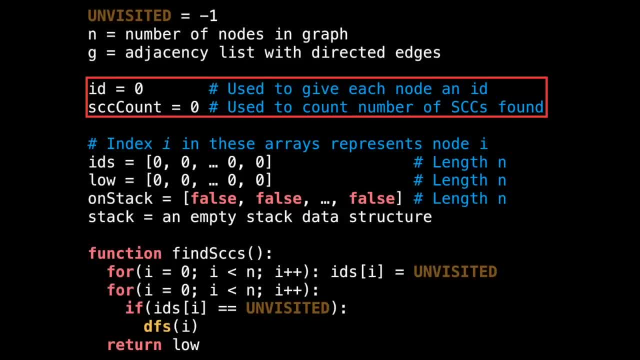 an ID and s CC count to track the number of strongly connected components. After I define a few arrays which store auxiliary information about the node nodes in our graph. the first array is IDs, which stores the ID of each node. then is low, to store the low link values. And finally, on stack, to track whether or not a node is. 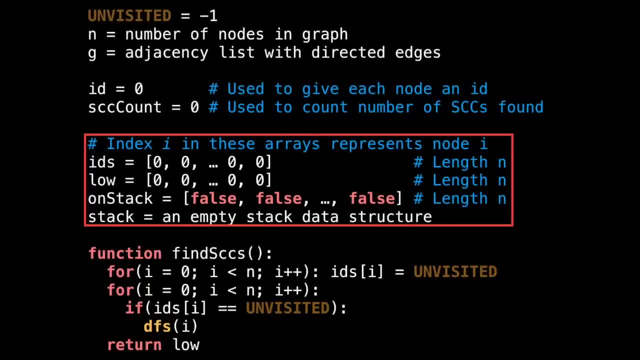 on the stack. Finally, is the stack data structure itself, which should, at minimum support push and pop operations Inside the find s CCS method. The first thing I do is assign a string array for every node, the ID of each node to be unvisited. The IDs array will be serving. 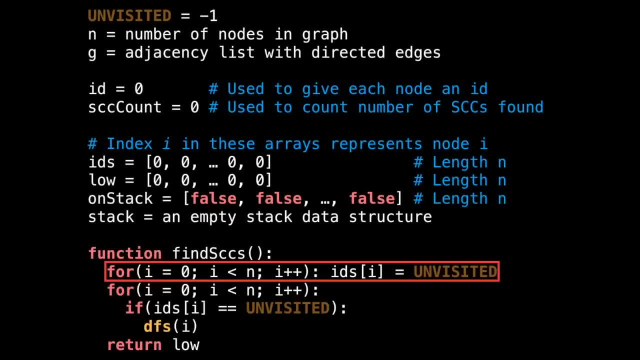 to track whether or not a node has been visited, as well as what a nodes ID is. In the following loop I iterate through all the nodes in the graph. There I start a depth first search on node i. if node i has not yet been visited, At the end I return the array low and array. 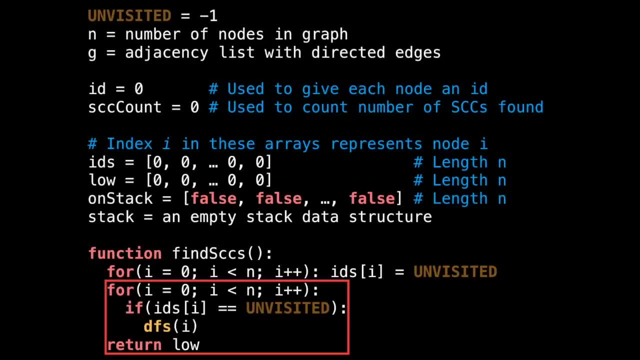 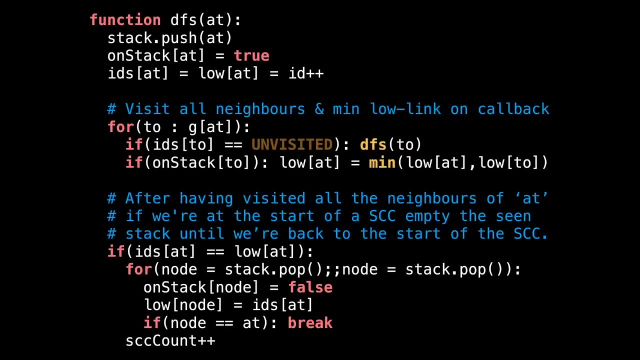 of low link values, which will be the final output of the algorithm. Now let's look at what's happening inside the depth first search method, which is really where all the magic happens. So this is the inside of the depth first search method: the input argument to the depth first search method. 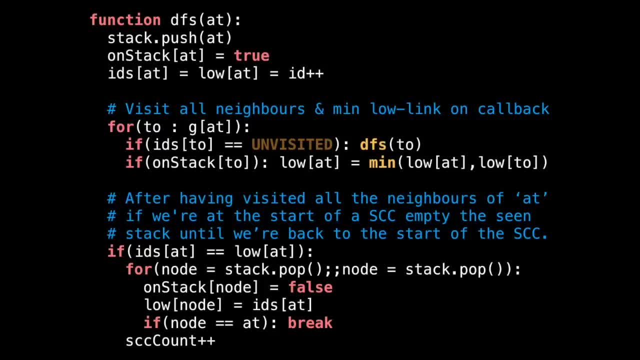 is a variable called at which I use to denote the ID of the node we are currently at. On the first three lines I do some housekeeping stuff, which is add the current node to the stack, mark the current node as being on the stack and give an ID and a low link value. 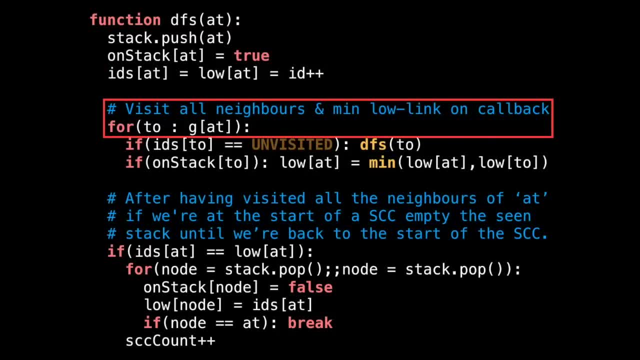 to the current node. Then comes the part where I visit all the neighbors of the current node. To do this, I reach into our graph stored as an adjacency list and loop over a variable called two, which represents the ID of the node we're going to. 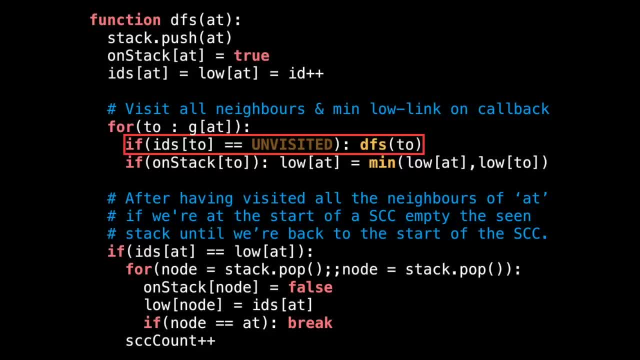 The next line says that if the node we're going to is unvisited, then visit it. Remember: the IDs array tracks the ID of node i, but also whether or not node i has been visited. This next line is very important. In fact it's probably the most important line on the 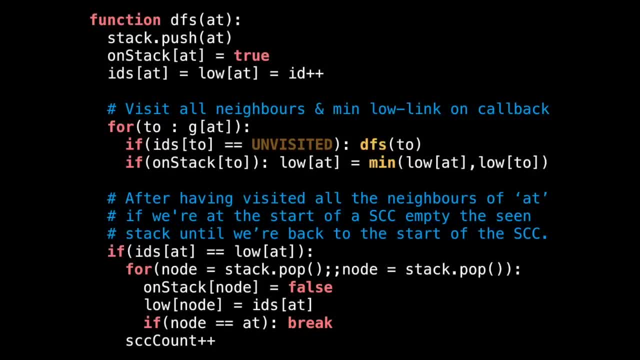 this is the inside of the depth first search method. The input argument to the depth first search method is a variable called at, which I use to denote the ID of the node we are currently at. On the first three lines I do some housekeeping stuff which is add the. 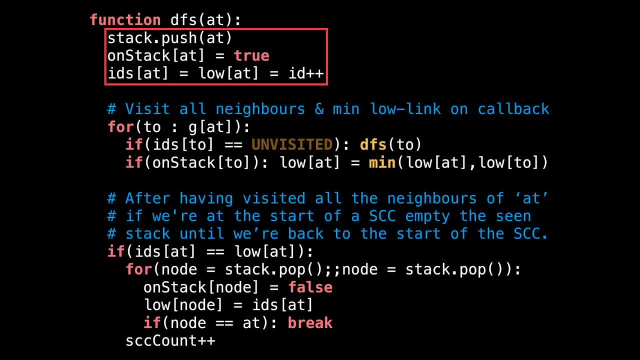 code, And then I'm going to add the code, And then I'm going to add the code, And then I'm going to add the current node to the stack, mark the current node as being on the stack and give an ID and a low link value to the current node. then comes the part where I visit all the 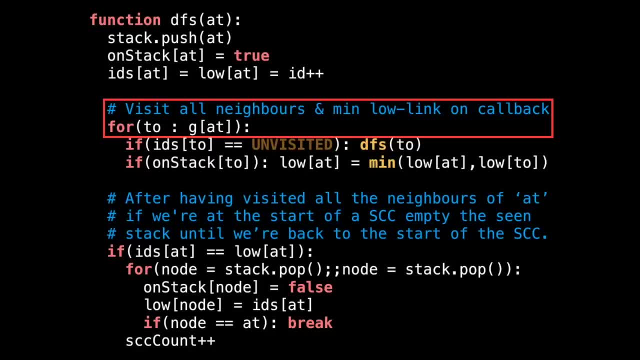 neighbors of the current node. To do this, I reach into our graph stored as an adjacency list and loop over a variable called two, which represents the ID of the node we're going to. the next line says that if the node we're going to 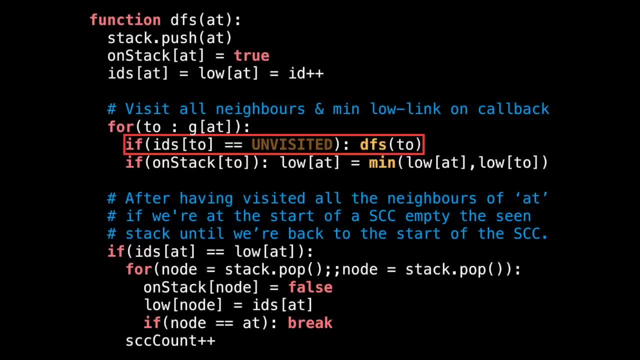 do is unvisited, then visit it. Remember, the IDs array tracks the ID of node I, but also whether or not node I has been visited. This next line is very important. In fact, it's probably the most important line on the slide. The first thing to notice is that this line happens. 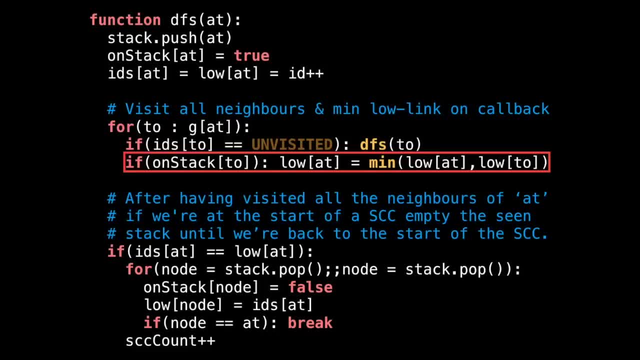 after the recursive call to the depth first search method, meaning that this line gets called on. the callback back from the depth first search line says that if the node we just came from is on stack, then min the current low link value with the node we were just at. this is what allows the 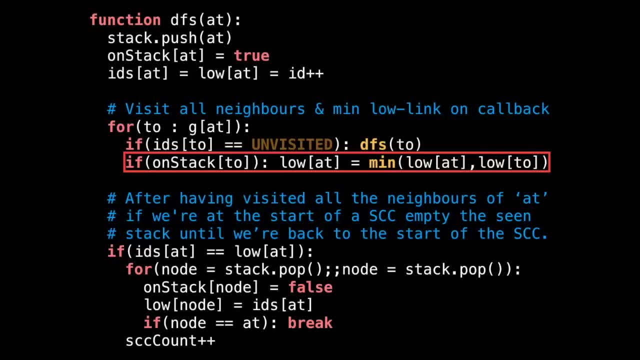 low link values to propagate throughout a cycle. So after we finish the for loop that visited all the neighbors of the current node, we need to check if we're at the start of a strongly connected component. To check if we're at the start of a strongly connected 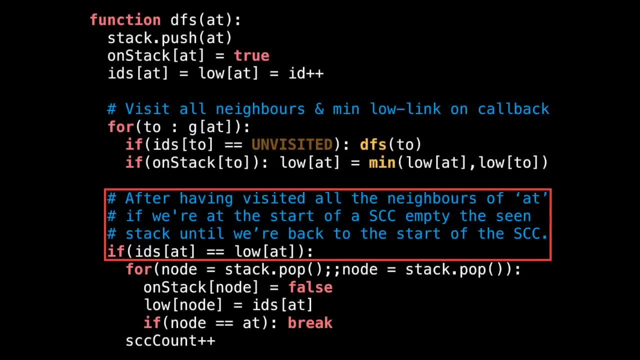 component check. the ID of the current node is equal to the low link value for that node. After we have identified that we're at the beginning of a completed strongly connected component, pop off all the nodes inside the strongly connected component from the stack, As we're. 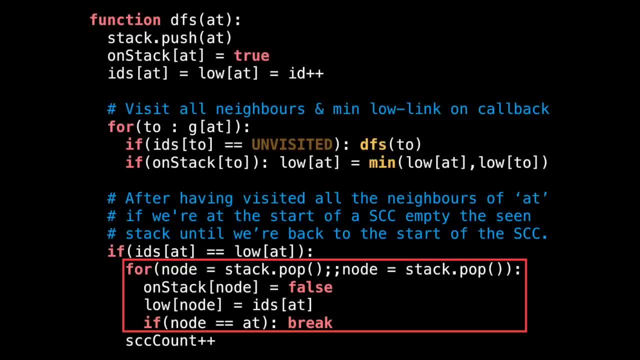 popping nodes from the stack also mark off nodes as no longer being on the stack. One more critical thing we need to do while we're removing nodes from our stack is to make sure that all nodes which are part of the same strongly connected component have the same. 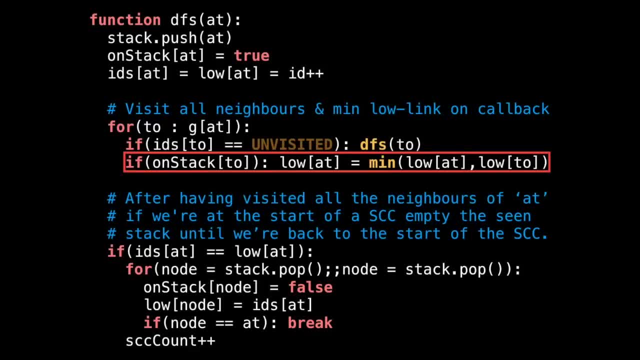 slide. The first thing to notice is that this line happens after the recursive call to the depth first search method, meaning that this line gets called on. the callback from the depth first search line says that if the node we just came from is on stack, then min the current. 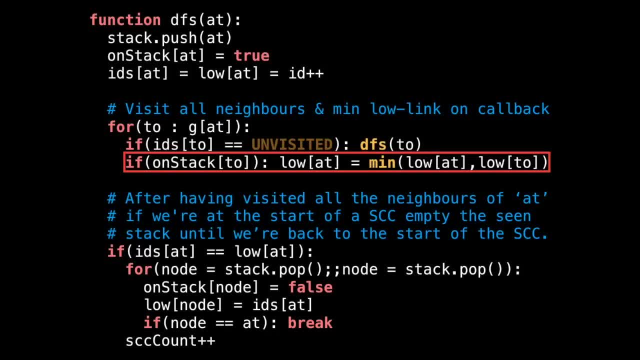 low link value with the node we were just at. This is what allows the low link values to propagate throughout a cycle. So after we finish the for loop that visited all the neighbors of the current node, we need to check if we're at the start of a strongly 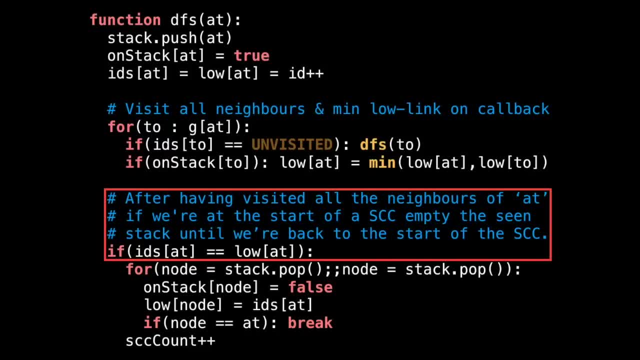 connected component. To check if we're at the start of a strongly connected component check. the ID of the current node is equal to the low link value for that node, After we have identified that we're at the beginning of a completed strongly connected component. 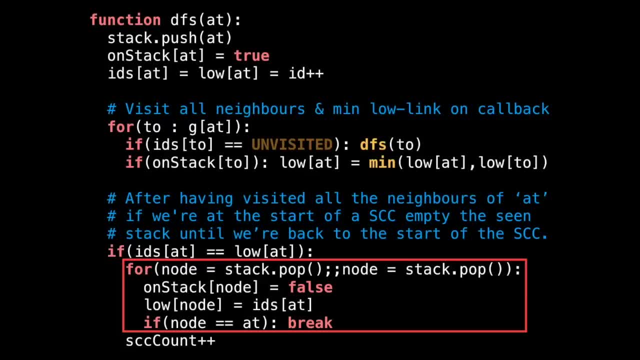 pop off all the nodes inside the strongly connected component from the stack. As we're popping nodes from the stack, also mark off nodes as no longer being on the stack. One more critical thing we need to do while we're removing nodes from our stack is to make sure 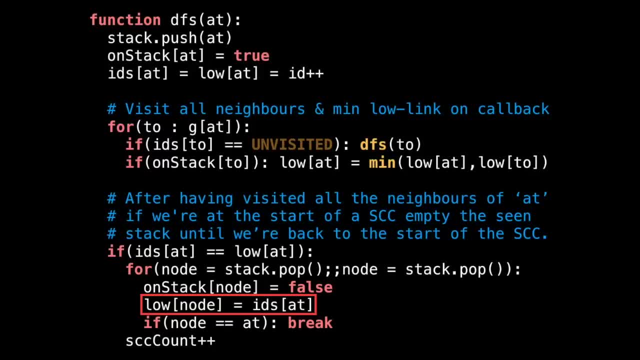 that all nodes which are part of the same strongly connected component have the same ID. So here I just assign each node to have the same ID as the ID of the node which started the strongly connected component. Last things are to stop popping off nodes from the stack. 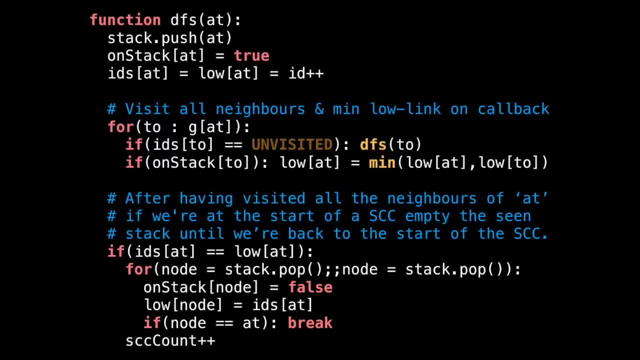 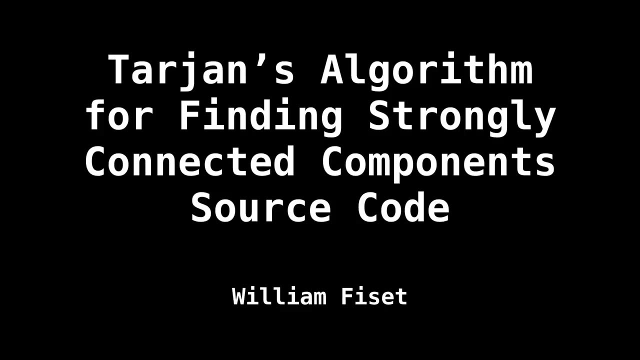 once we reach the start of the strongly connected component and also increment the strongly connected component count If you want to track the number of strongly connected components that were found. today we will be looking over some source code for Tarzan's strongly connected components algorithm. Here we are in the source code for Tarzan's algorithm. 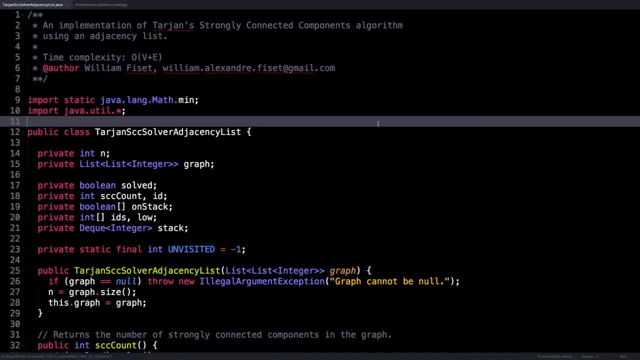 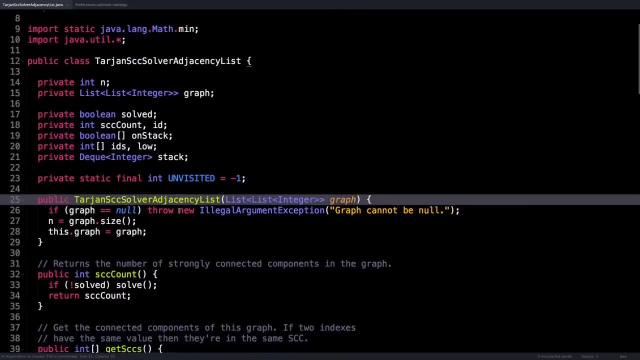 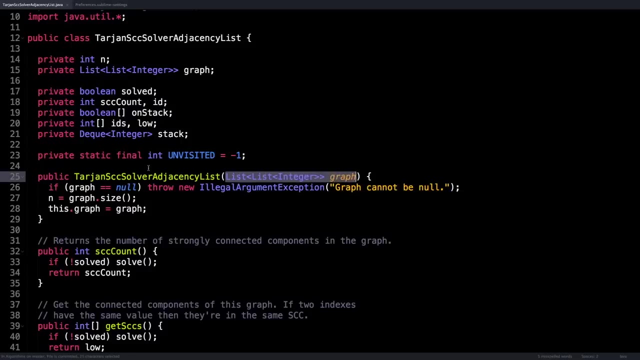 to find strongly connected components. You'll notice that this source code is written in the Java programming language. So to get started, let's have a look at the constructor for the class And you'll notice that it takes a graph as an adjacency list, as an argument. But before we get into the details, 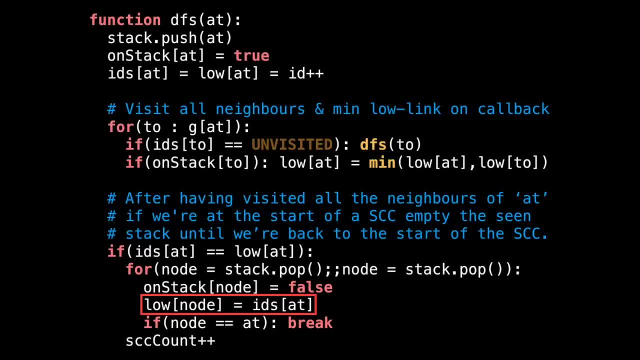 ID. So here I just assign each node to have the same ID as the ID of the node which started the strongly connected component. Last things are to stop popping off nodes from the stack once we reach the start of the strongly connected component And also increment the strongly. 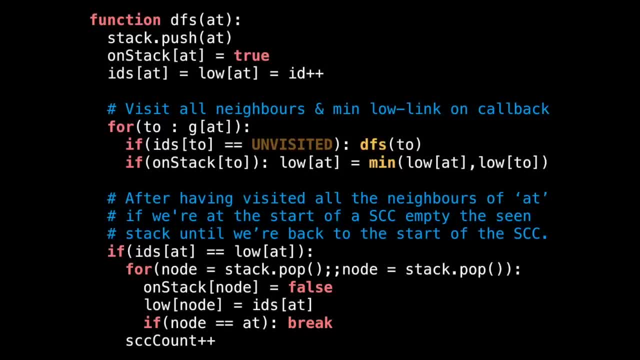 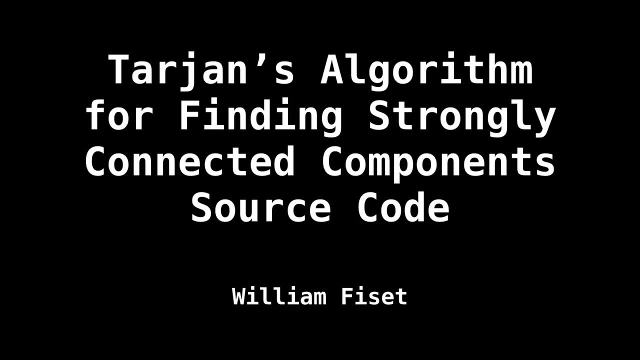 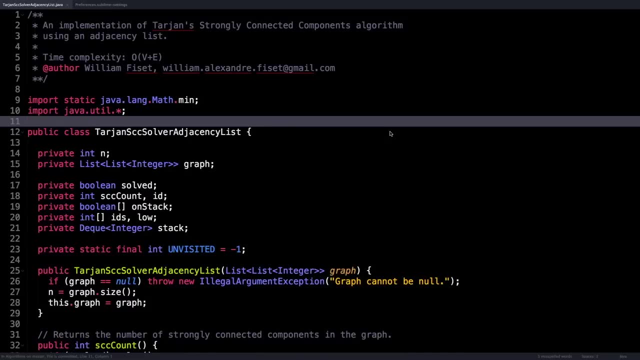 connected component count If you want to track the number of strongly connected components that were found. today we will be looking over some source code for Tarzan's strongly connected components algorithm. Here we are in the source code for Tarzan's algorithm to find strongly connected components. You'll notice that this source code is written in: 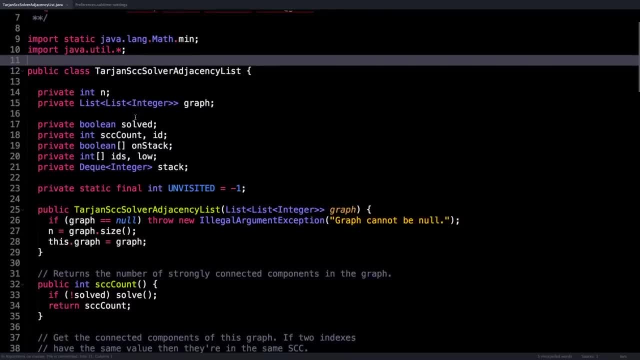 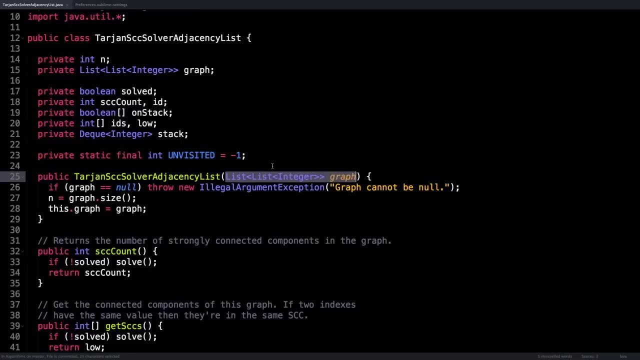 the Java programming language. So, to get started, let's have a look at the constructor for the class And you'll notice that it takes a graph as an adjacency list, as an argument. But let's start with the constructor And we'll look at the constructor and we'll see that it takes 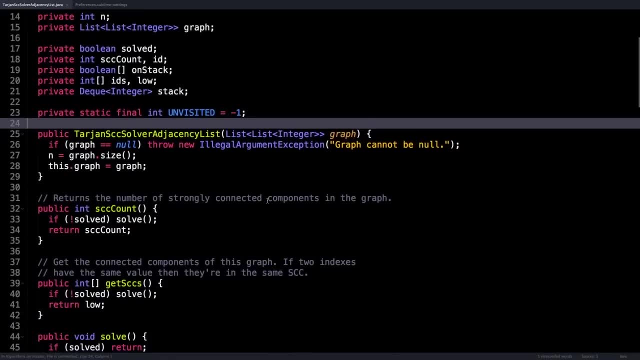 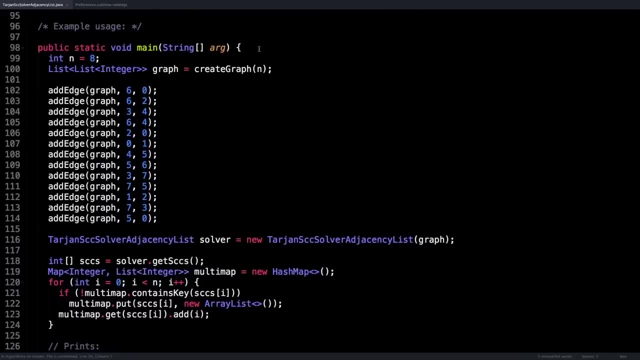 But before we get into the details of this actual algorithm, I want to show you how the algorithm actually works in practice if you're going to execute it. So if we look at the main method, you'll notice that here is how the algorithm is meant to be used. you set: 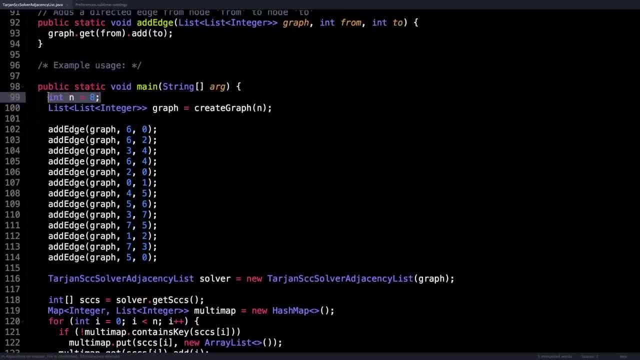 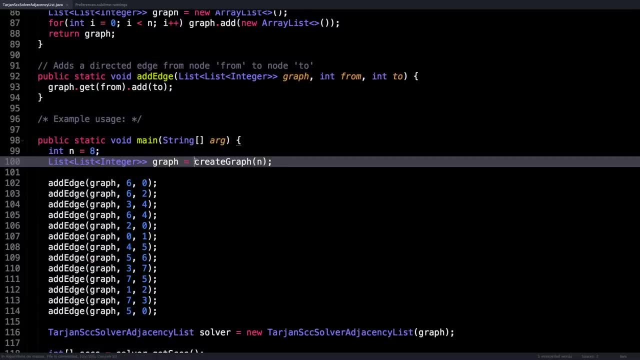 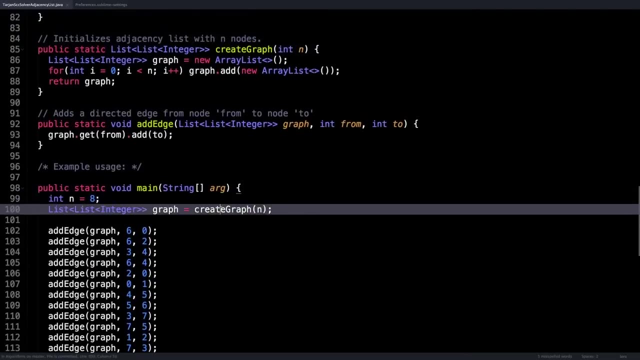 up the graph and then you run the solver. So to begin with you declare a variable called n, which is the number of nodes that are going to be in your graph. then you create the graph. So this initializes the adjacency, this list for n nodes. If we look at that, create graph. 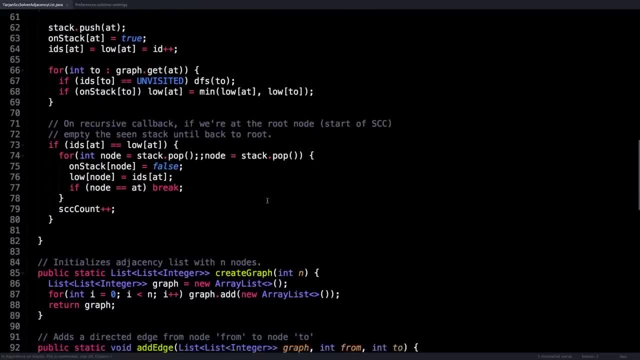 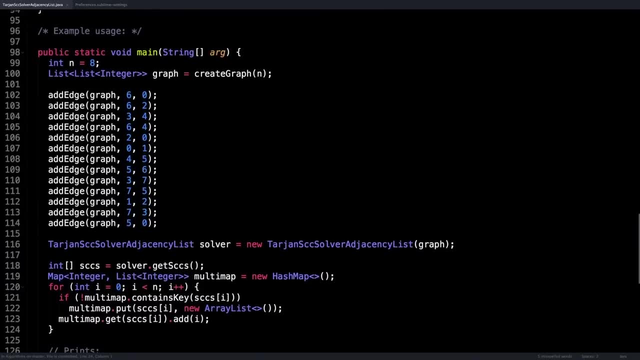 of this actual algorithm. I want to show you how the algorithm actually works in practice if you're going to execute it. So, if we look at the main method, you'll notice that here is how the algorithm is meant to be used. You set up the graph and then you run the 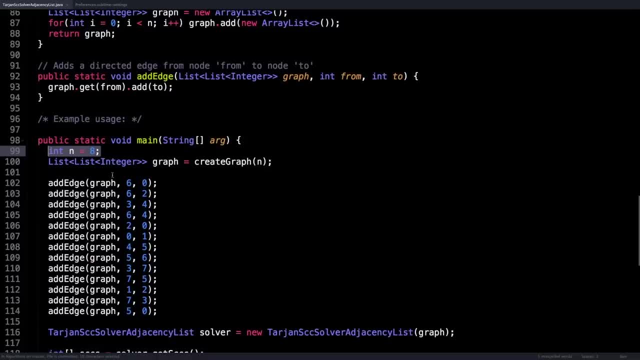 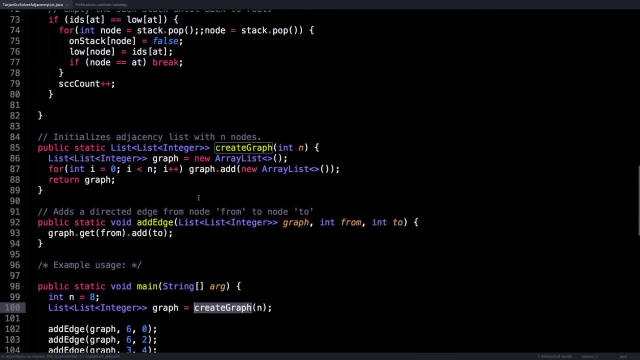 solver. So to begin with, you declare a variable called n, which is the number of nodes that are going to be in your graph. then you create the graph. So this initializes the adjacency list for n nodes And if we look at that create graph method up here, all that does is initializes. 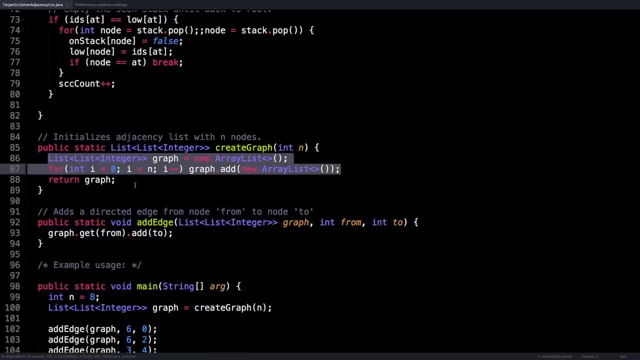 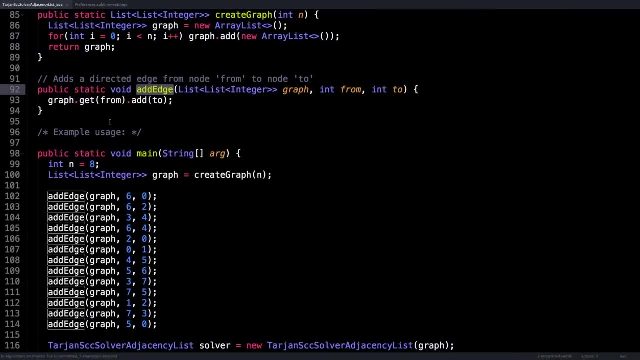 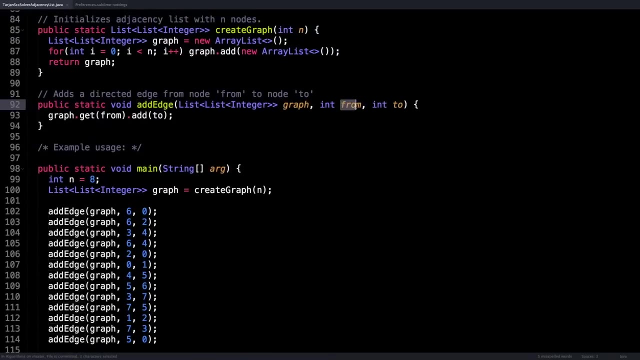 the adjacency lists and then populates that with empty lists so that we can be ready to add edges to our directed graph. So if you want to add an edge to the graph, then you would call this method: Give it the graph, give it the directed edge, So from a node to another node, and then it. 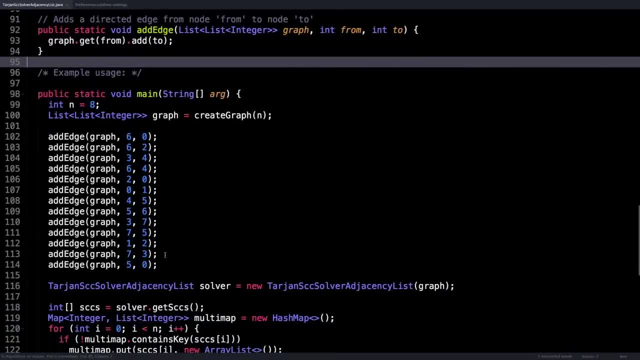 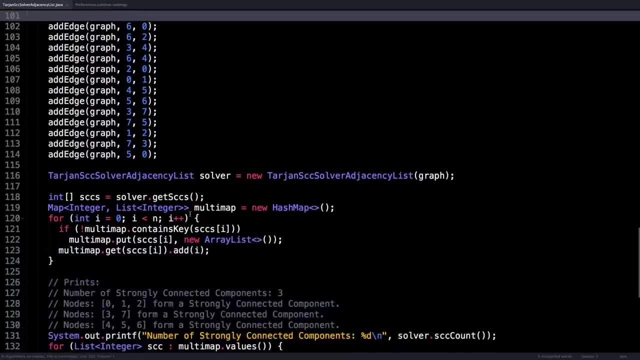 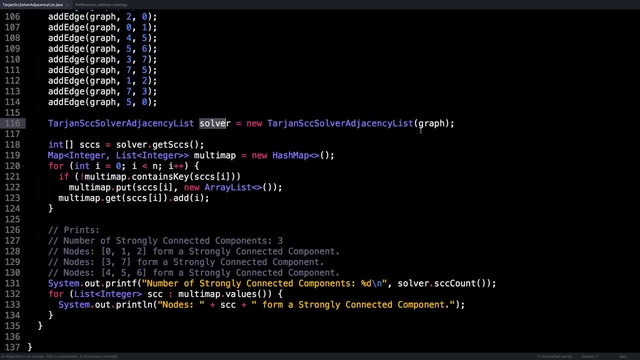 will add that edge to the graph. So I believe this graph is the one from the slides, the very last graph, if I recall correctly. So to actually find the strongly connected components, you create an object of the solver, you give it the graph and then you run the solver. 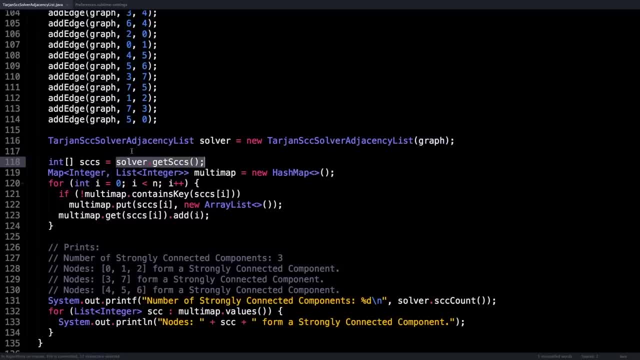 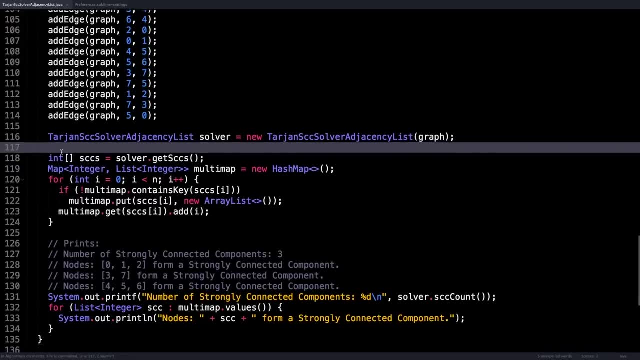 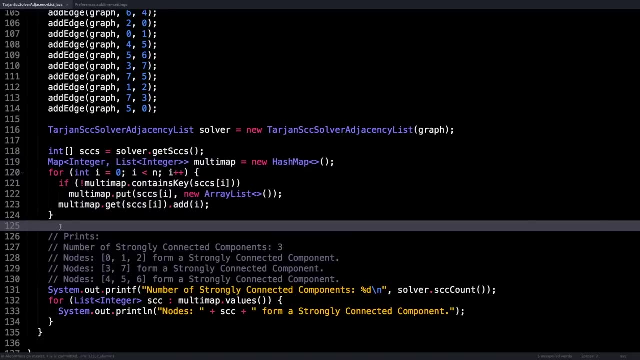 on the graph. So this is what actually finds the strongly connected components, And this will return the the array of low link values. Then what I do is I dump all of these inside a multi map So we can know for each connected component, which are the nodes associated with that connected component. 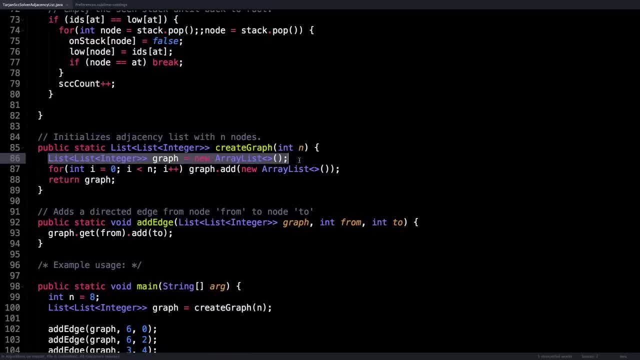 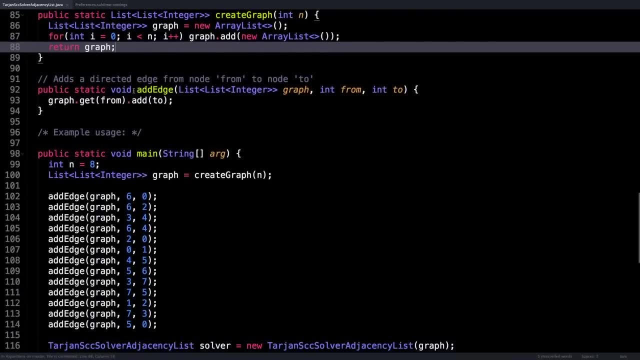 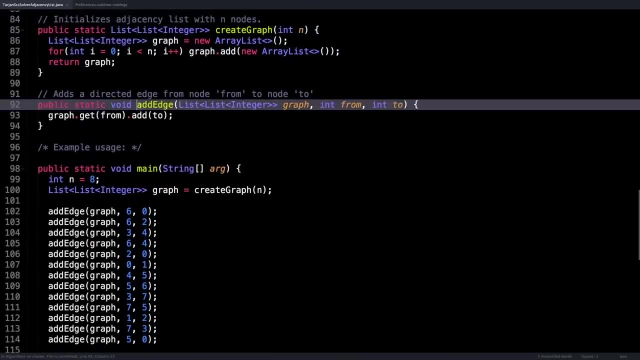 method up here all that does is initialize the adjacency lists and then populates that with empty lists so that we can be ready to add edges to our directed graph. So if you want to add an edge to the graph, then you would call this method: give it the graph. 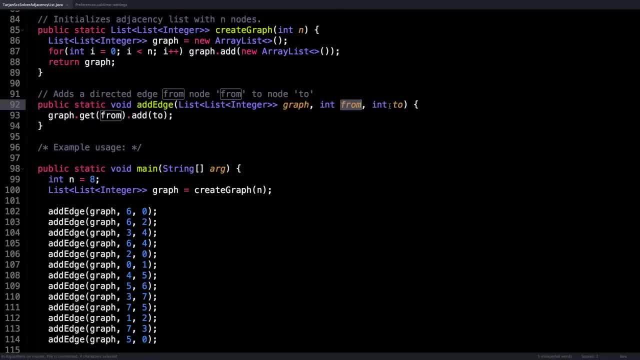 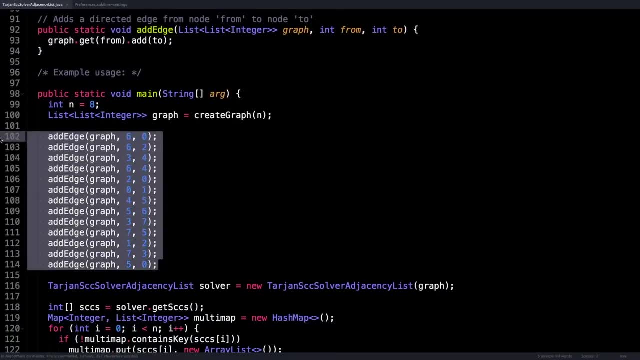 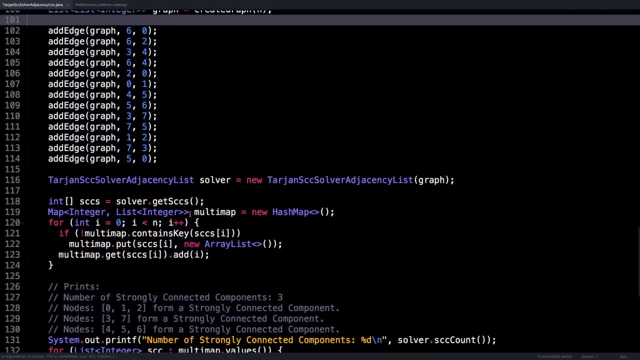 give it the directed edge, So from an node to another node, and then it will add that edge to the graph. So I believe this graph is the one from the slides, the very last graph, if I recall correctly. So to actually find the strongly connected components, you create an object of the solver, you give it. 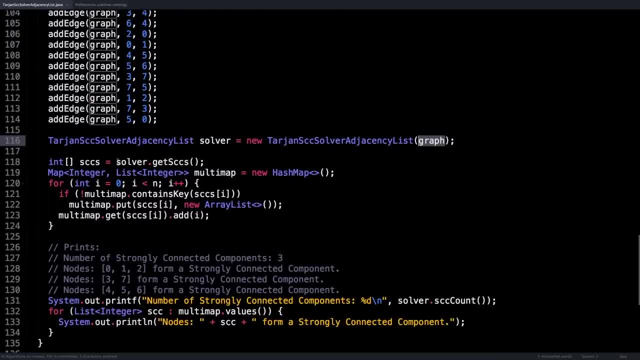 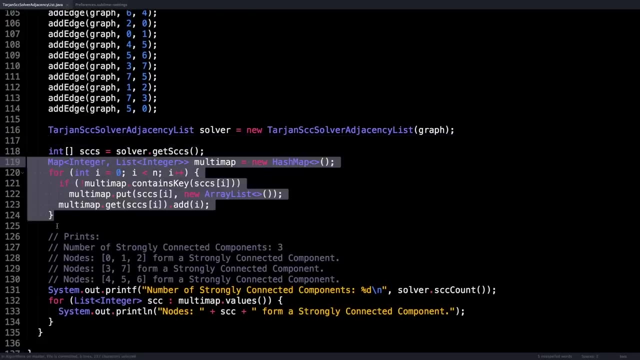 the graph and then you run the solver on the graph. So this is what actually finds the strongly connected components And this will return the the array of low link values. Then what I do is I dump all of these inside a multi map So we can know for each connected. 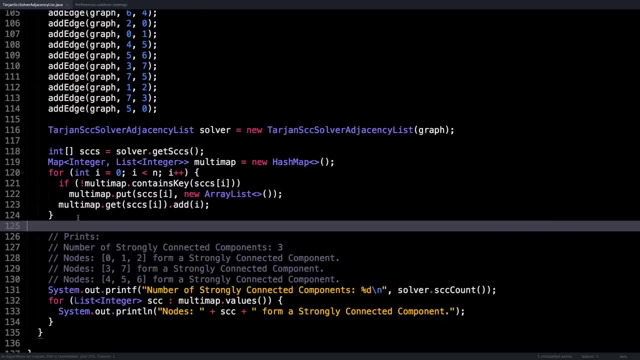 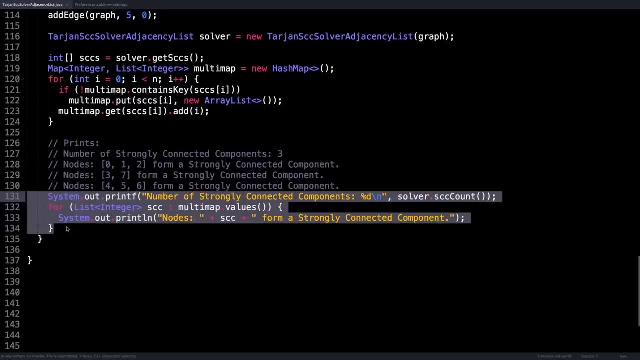 component, which are the nodes associated with that connected component. And then all I do is I print out which groups which nodes are part of. So you notice that I print out that there are three connected components And here are the nodes and what connected. 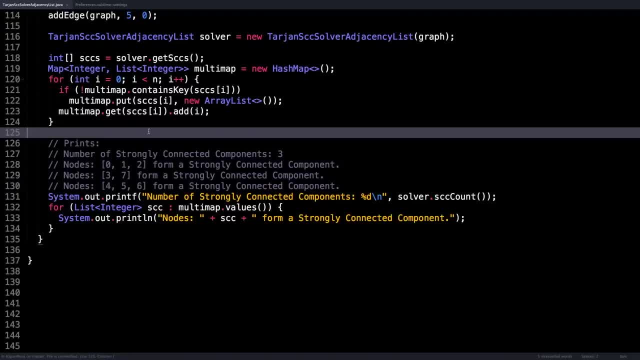 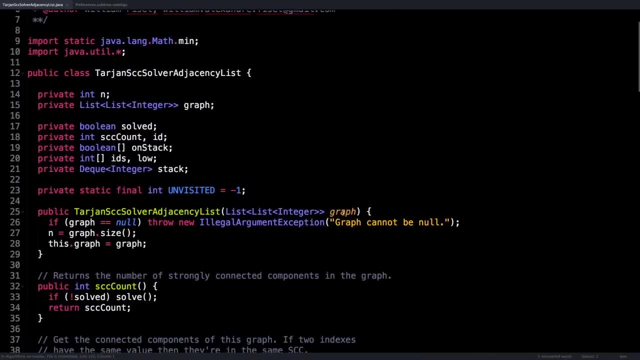 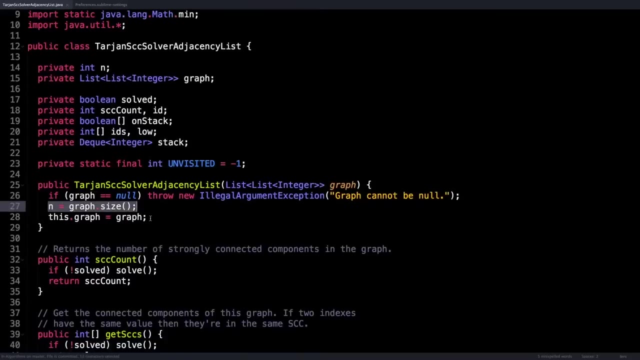 components they belong to. So that's how you use the algorithm. Let's see what it's doing. So we already ran over the constructor which passed in a graph, extracts the size of the graph and caches the adjacency list As other instance variables. we want to know what is the adjacency list, So I'm going. 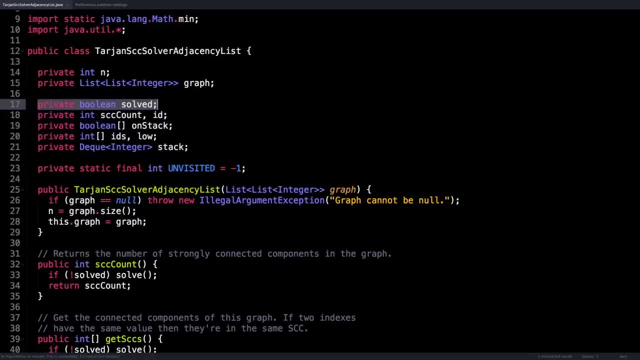 to call it the adjacency list, And then I'm going to call it the adjacency list And then I'm going to type a variable here, which is a variable that I want to call the adjacency list And variables: we have a Boolean variable with tracks whether or not we have already solved. 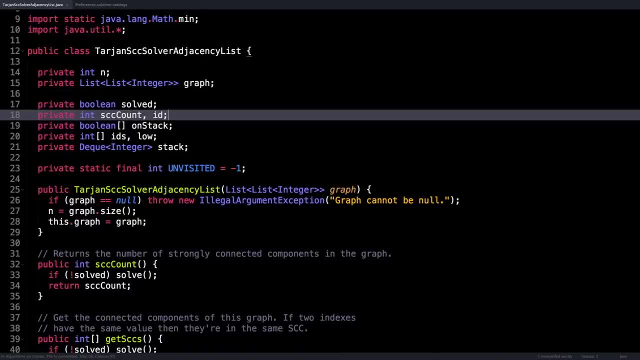 the problem. then two variables to count the number of strongly connected components and assign an ID to each node, an array to track whether or not a node is on the stack, and then two integer arrays to track the ID of each node and the loading values of each node. 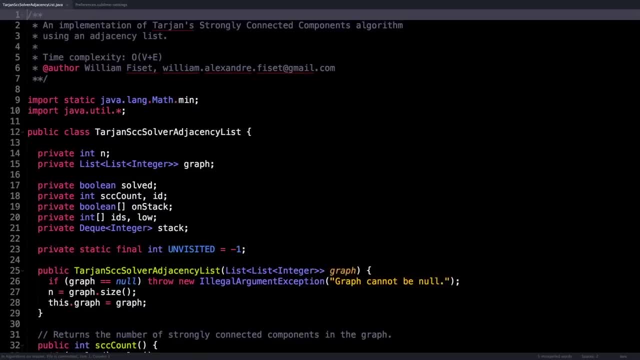 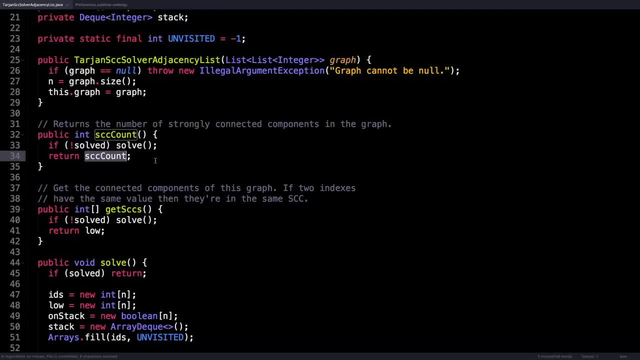 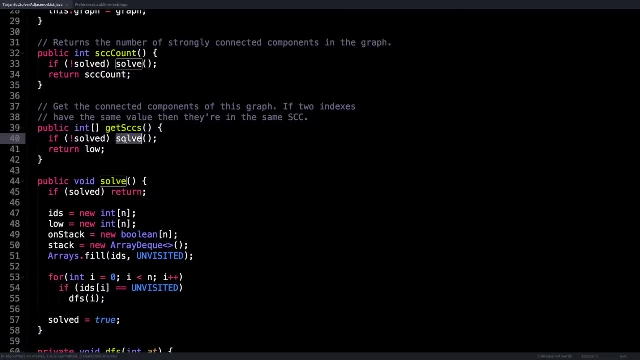 And finally a stack. So if we look at the SCC count method, it runs the solver if has not yet been solved and simply returns the number of strongly connected components. The get SCC method also simply runs the solver if it has not yet been run and returns the 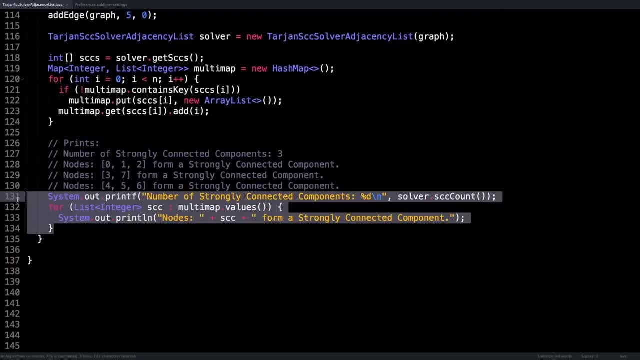 And then all I do is I print out which groups which nodes are part of. So you notice that I print that there are three connected components And here are the nodes and what connected components they belong to. So that's how you use the algorithm. Let's see what. 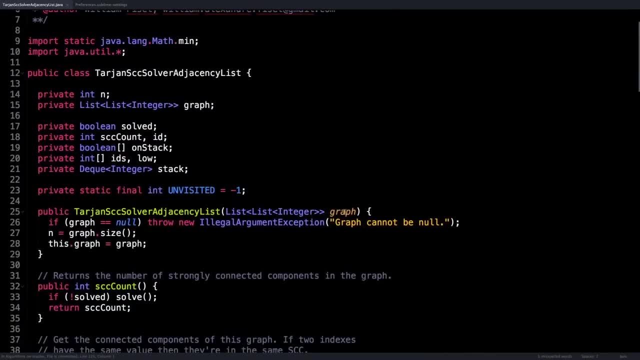 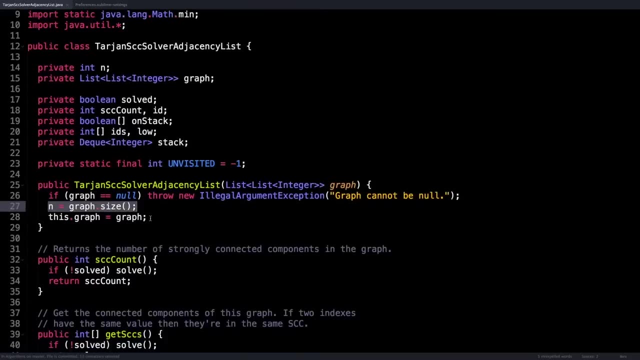 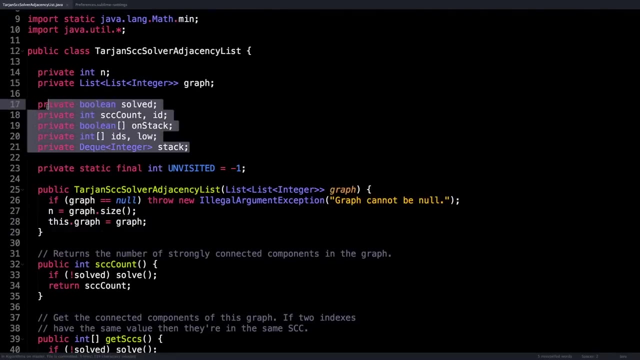 it's doing So. we already ran over the constructor which passed in a graph, extracts the size of the graph and caches the adjacency list As otherИ other instance variables. we have a Boolean variable with tracks whether or not we have already solved the problem, then two variables to count the number of strongly connected. 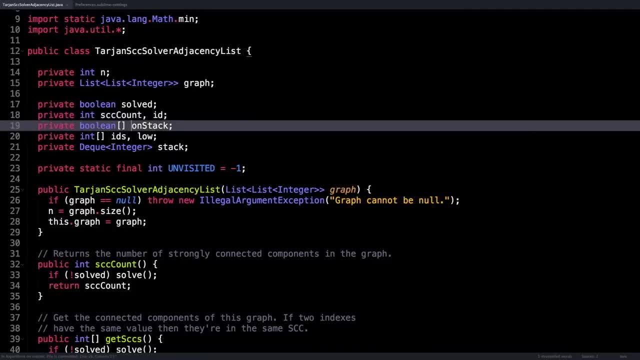 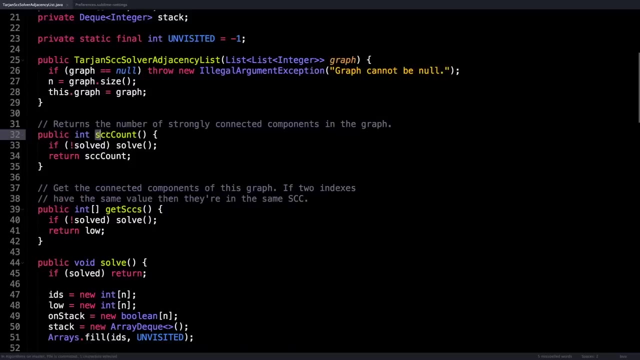 components and assign an ID to each node. an array to track whether or not a node is on the stack, and then two integer arrays to track the ID of each node and the loading values of each node, And finally a stack. So if we look at the SCC count method, it 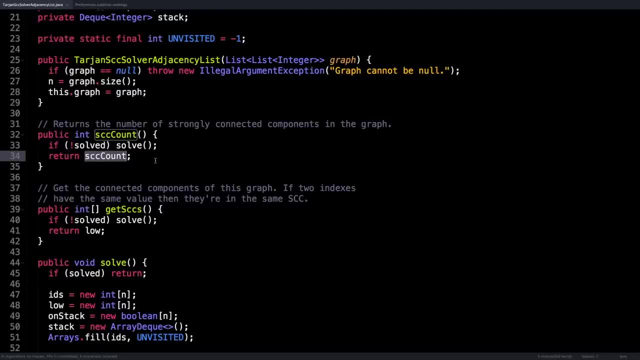 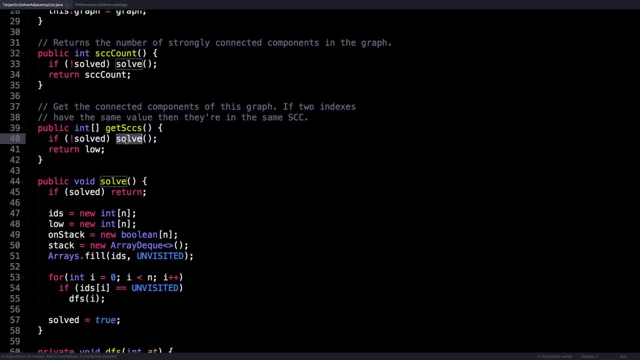 runs the solver if has not yet been solved, and simply returns the number of strongly connected components. The get SCC is method also simply runs the solver if it has not yet been run and returns the low link values array. Now let's look at the solver itself. 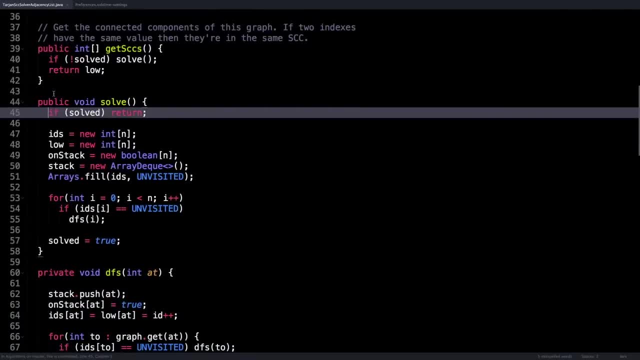 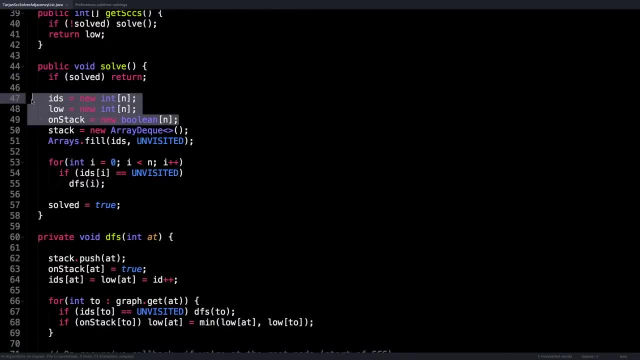 So it returns if it's already been solved, because we don't want to do more work than we need to. Inside the solve method, I initialize all our arrays. I also fill the IDs array with the unvisited token So we can know whether or not a node has been visited or not. Recall that the IDs. 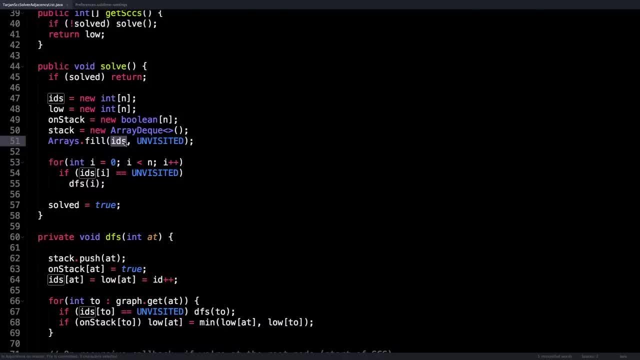 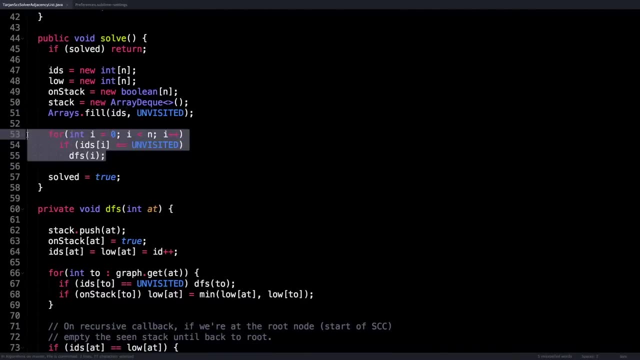 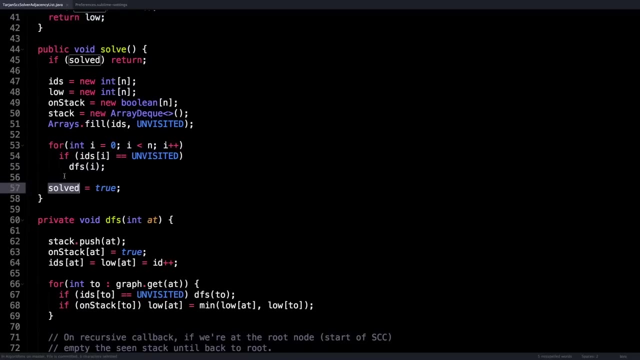 array keeps track of the ID of a node, but it also keeps track of whether or not a node has been visited. So iterate through each node And if node I is unvisited, then start a depth first search at node I. Finally, mark that we have solved. 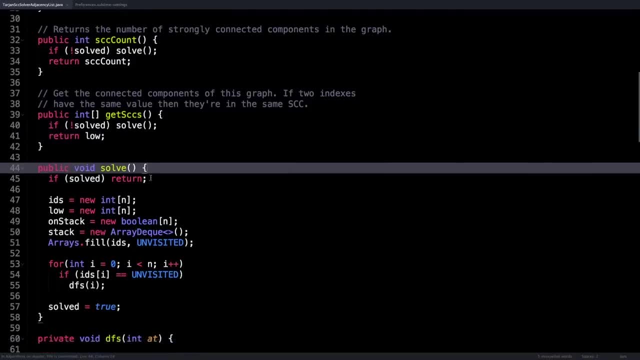 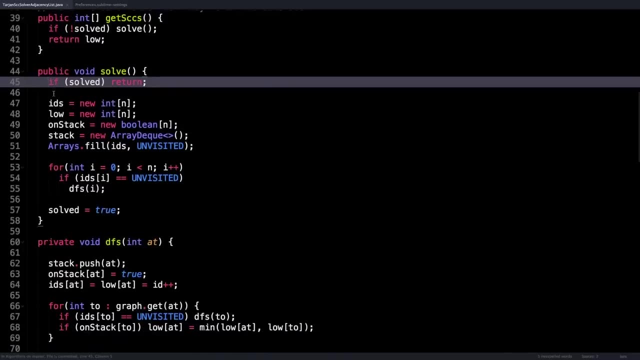 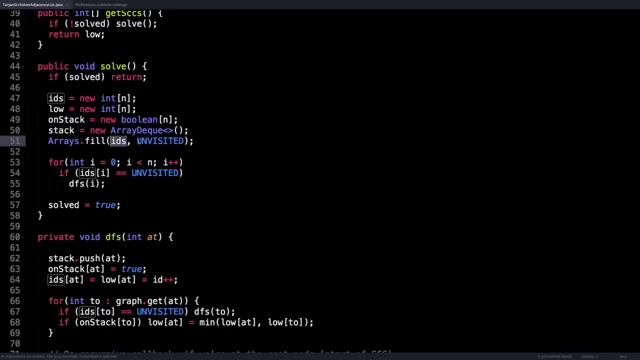 low link values array. Now let's look at the solver itself. So it returns if it's already been solved. Because we don't want to do more work than we need to Inside the solve method I initialize all our arrays. I also fill the IDs array with the unvisited token So we can know whether. 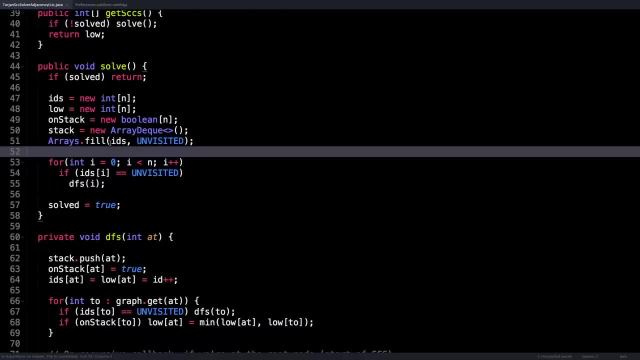 or not a node has been visited or not. Recall that. the IDs array keeps track of the ID of a node, But it also keeps track of whether or not a node has been visited, So iterate through each node And if node i is unvisited, 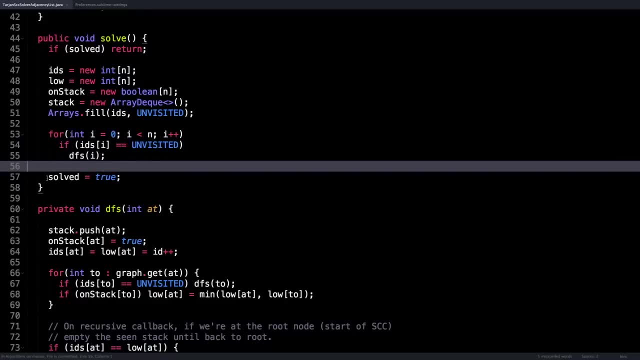 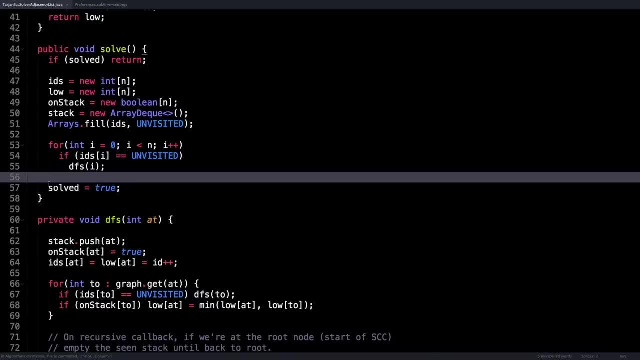 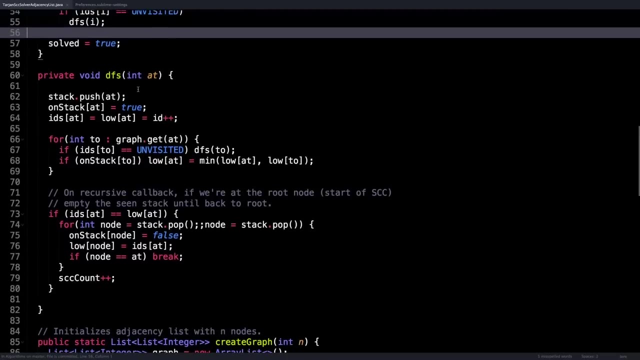 then start a depth first search at node. i Finally mark that we have solved the strongly connected components for this graph Inside the depth first search method. it's almost exactly like the slides. So do the housekeeping stuff which is like push the current node on the 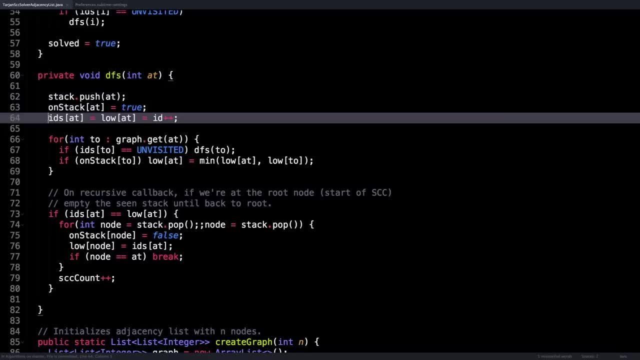 stack. mark the current node as being on the stack. give the the current node and ID and the loading value, because it's the first time we're visiting it. Then iterate over all the neighbors of this node. Do a depth first search if the node we're going to is unvisited on the callback. 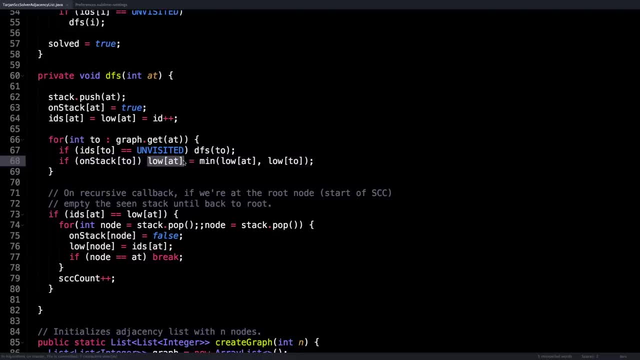 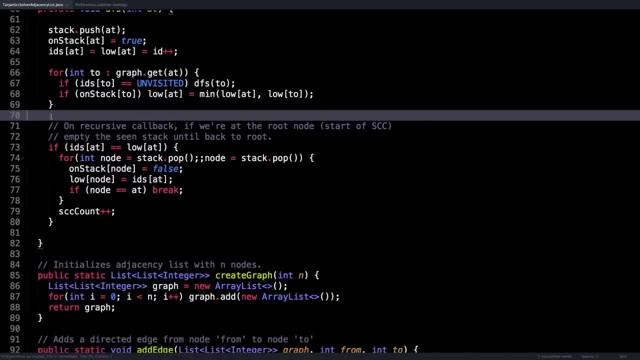 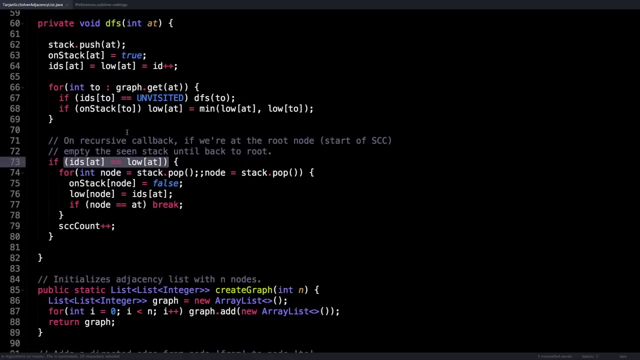 check if it's on the stack and minutes low link value with where we were just at And back here after we've visited all the neighbors of the node. Then we check if we're at the start of a strongly connected component And if we are, we want to pop off all the nodes. 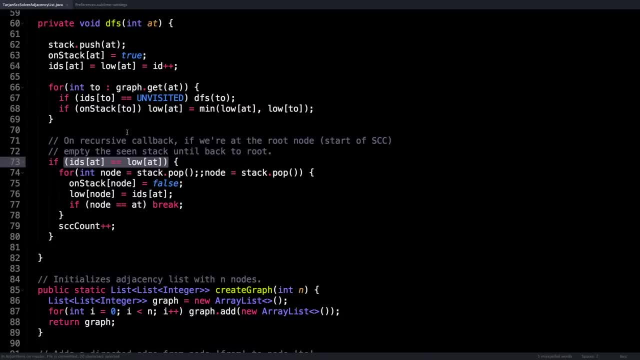 associated with astronomy connected component which are on the stack. So I start with a first node and my condition is to POP until I return back to the, the start of that strongly connected component. And as I'm popping off nodes from the stack, I mark the node as no. 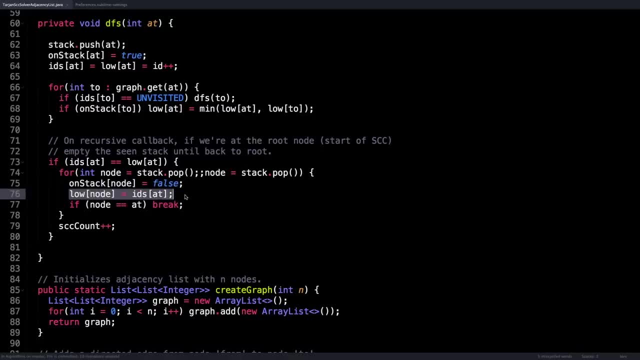 longer being on the stack, And then I'm going to go into the server and check if the node has been sold. This way, we're going to be able to see that this particular new node- And I also assign every node part of that- strongly connected components have the same. 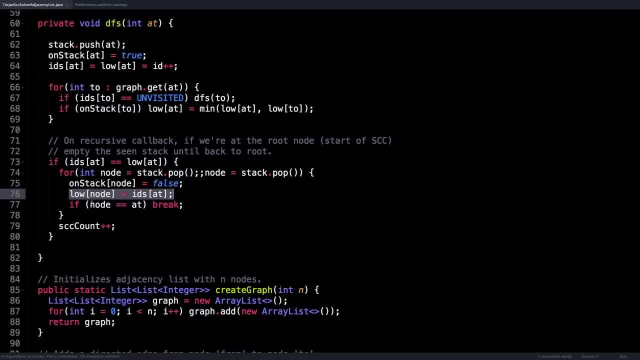 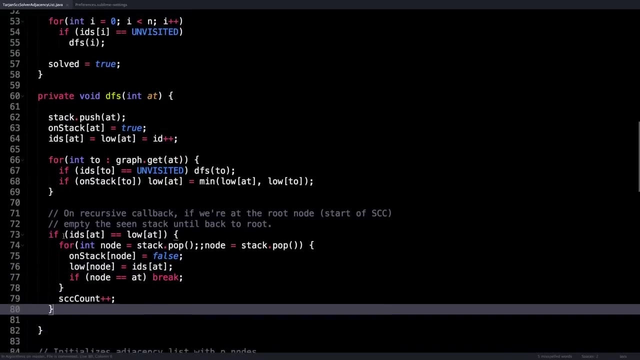 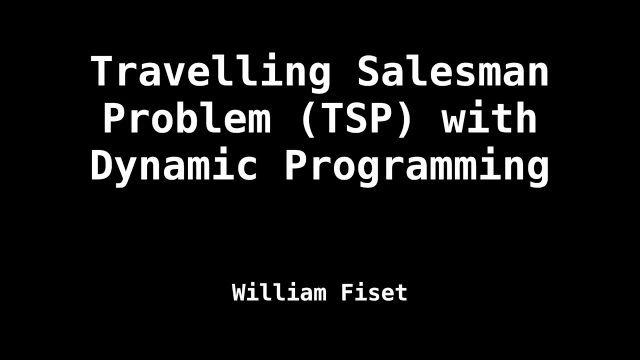 ID as the node which started the strongly connected component, Just so that we know, after the fact, which nodes belong to which strongly connected component. Finally, increment the number of strongly connected components, in case we are interested in that. And that's basically Tarzan's algorithm in a nutshell. Hello and welcome to this tutorial on how. 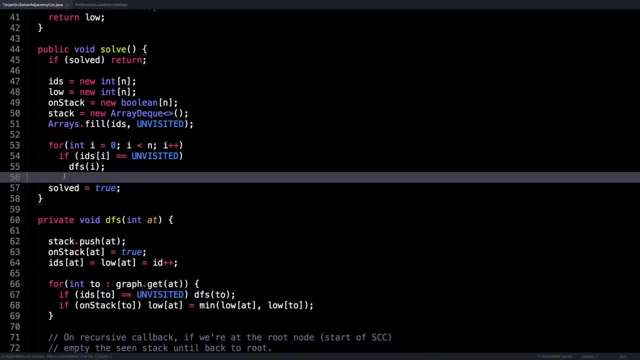 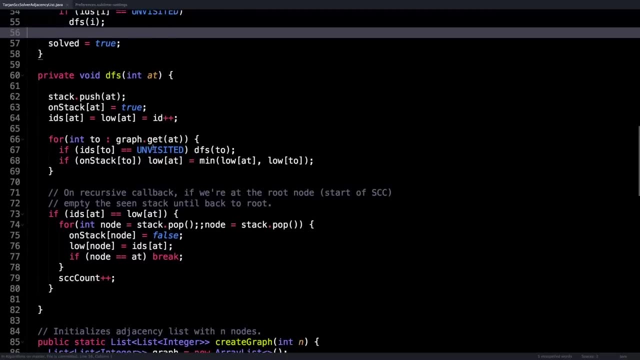 the strongly connected components for this graph Inside the depth first search method. It's almost exactly like the slides. So do the housekeeping stuff, which is like: push the current node on the stack. mark the current node as being on the stack. give the the current. 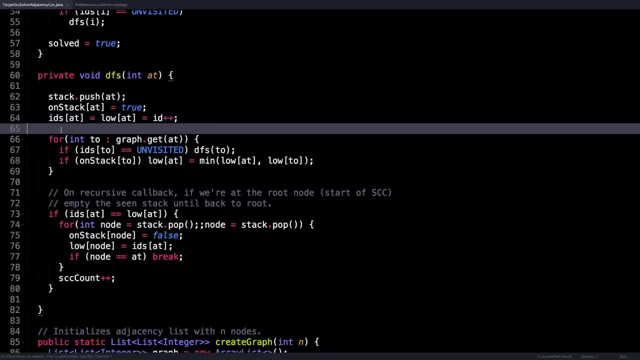 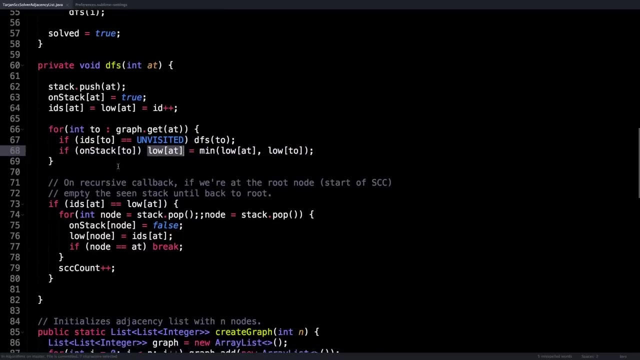 node and ID and the load Link value, because the first time we're visiting it then iterate over all the neighbors of this node. do a depth first search if the node we're going to is unvisited. on the callback check if it's on the stack and minutes low link value with where we were just at And 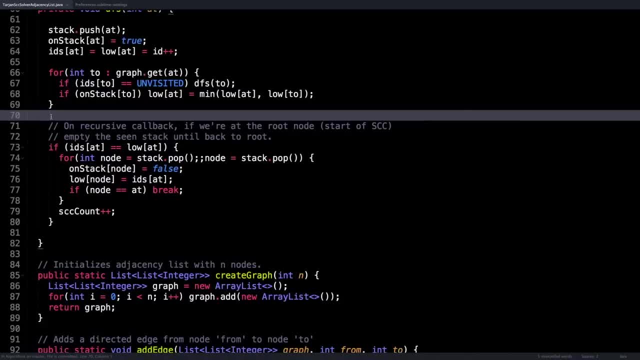 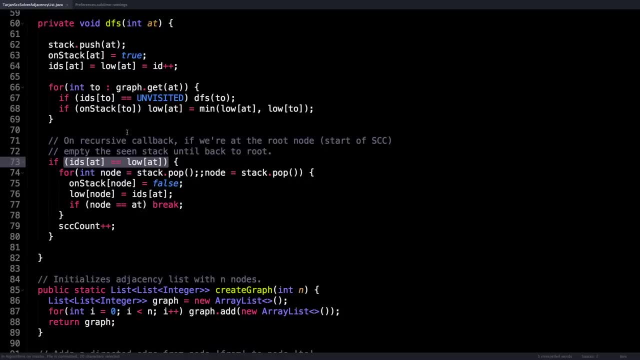 back here after we've visited all the neighbors of the node. Then we check if we're at the start of a strongly connected component And if we are, we want to pop off all the nodes associated with that strongly connected component which are on the stack. So I start with a first node and my condition is to pop until I return. 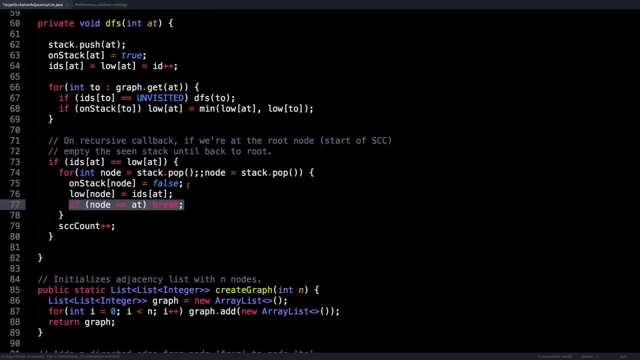 back to the the start of that strongly connected component And as I'm popping off nodes from the stack, I mark the node as no longer being on the stack And I also assign every node part of that. strongly connected components have the same ID as the node which started the strongly connected component. Just so that we know. 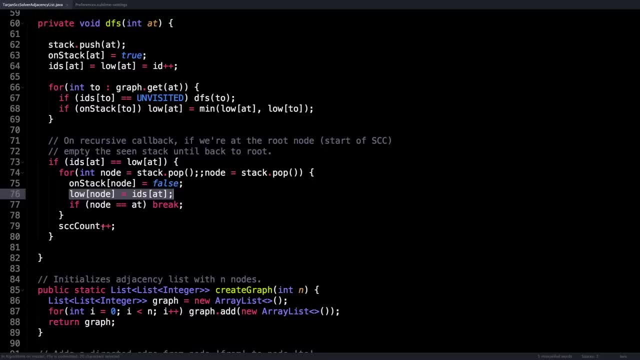 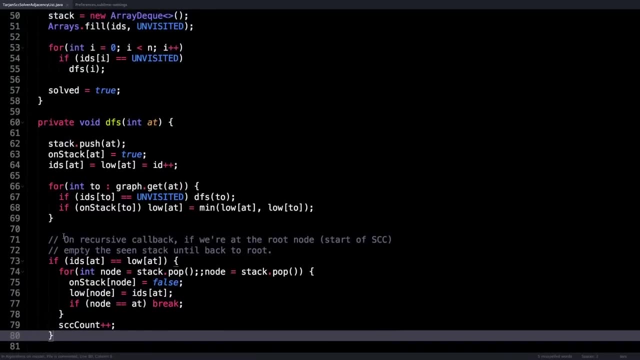 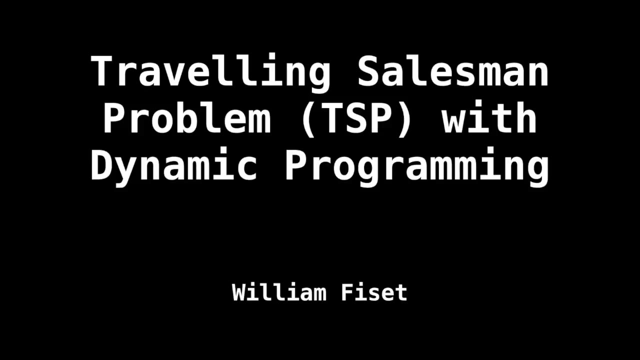 after the fact which nodes belong to which strongly connected component, Finally increment the number of strongly connected components, in case we are interested in that. And that's basically Tarzan's algorithm in a nutshell. Hello and welcome to this tutorial On how to solve the traveling salesman problem with dynamic programming. Today we're going. 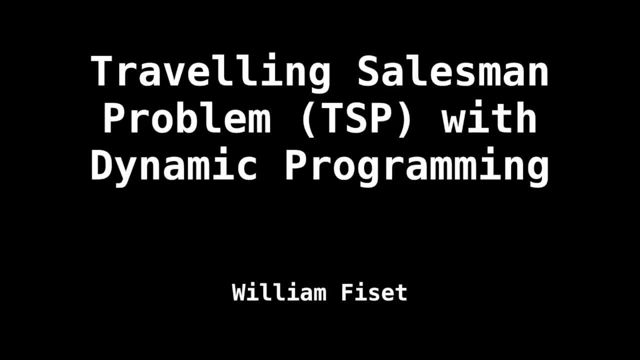 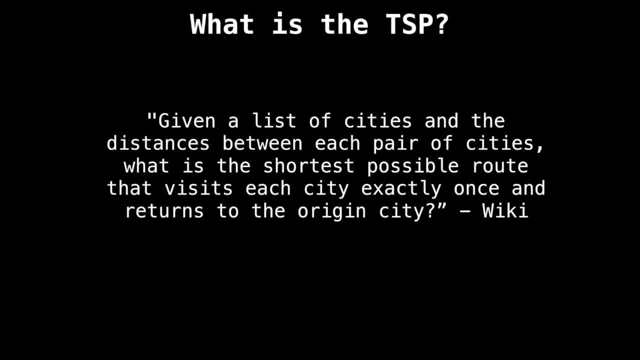 to look at two things: First is how to find the cost of the best tour, and then how to actually find that tour. Alright, so let's get started. What is the traveling salesman problem? In a nutshell, it's when you're given a list of cities and the distances between each pair of cities. 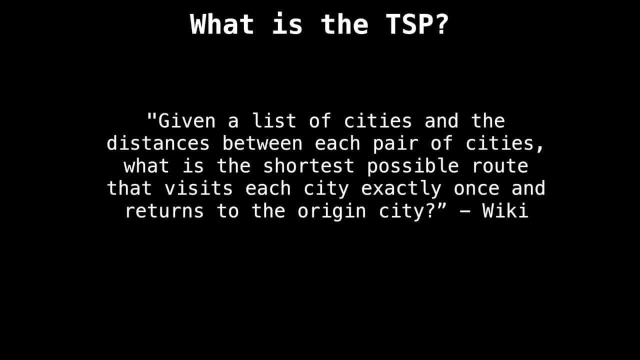 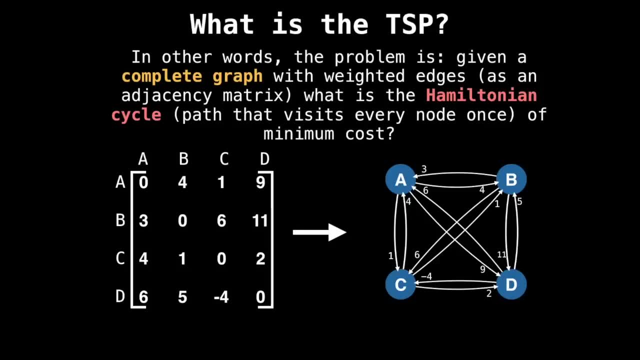 and you want to find the shortest possible route That visits each city exactly once and then it returns to the city of origin. In some other words, we can say that the problem is given a complete graph with weighted edges. What is the Hamiltonian cycle of minimum cost? A Hamiltonian cycle is simply a path which 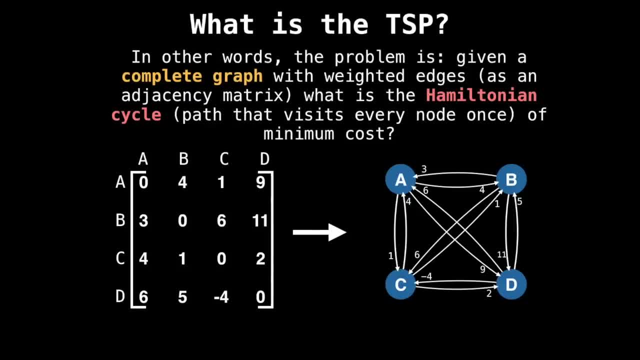 visits each node exactly once. In practice, you will probably want to represent what the node is, whatever graph you have as an adjacency matrix. for simplicity, If an edge between two nodes does not exist, simply set the edges value to be positive infinity. So in 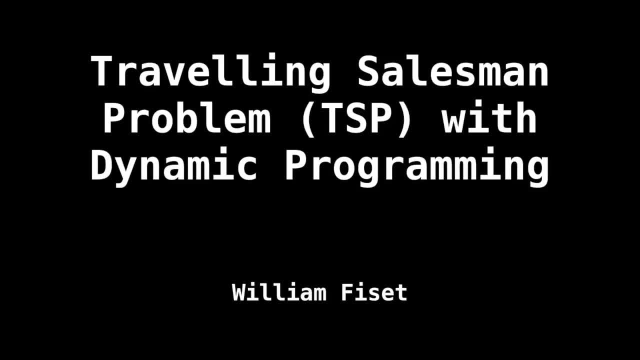 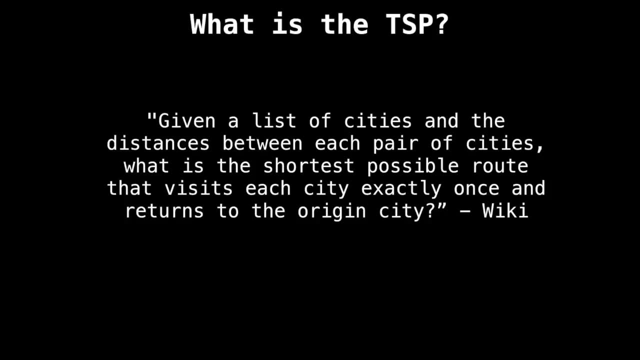 to solve the traveling salesman problem with dynamic programming. Today, we're going to look at two things. First is how to find the cost of the best tour, and then how to actually find that tour. Alright, so let's get started. What is the traveling salesman problem In? 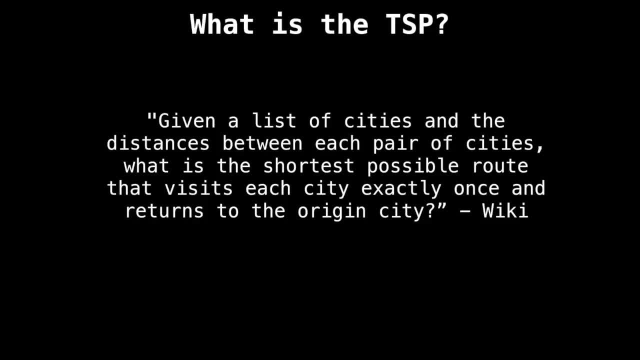 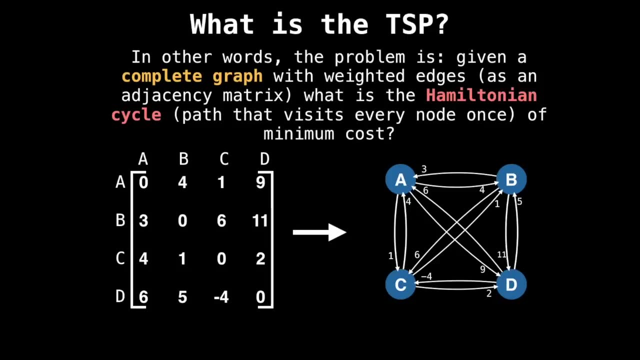 a nutshell, it's when you're given a list of cities and the distances between each pair of cities and you want to find the shortest possible route That visits each city exactly once and then returns to the city of origin. In some other words, we can say that the problem is given a complete graph with weighted edges. What 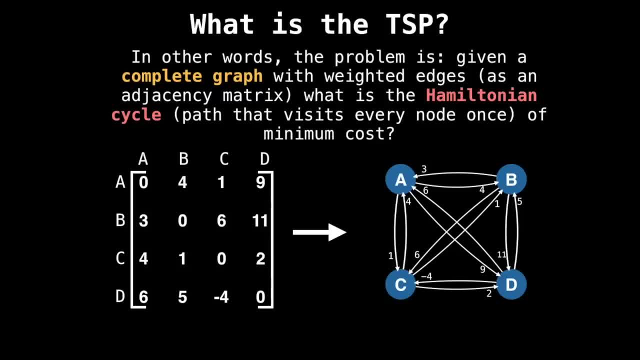 is the Hamiltonian cycle of minimum cost. A Hamiltonian cycle is simply a path which visits each node exactly once. In practice, you will probably want to represent whatever graph you have as an adjacency matrix, for simplicity, If an edge between two nodes does. 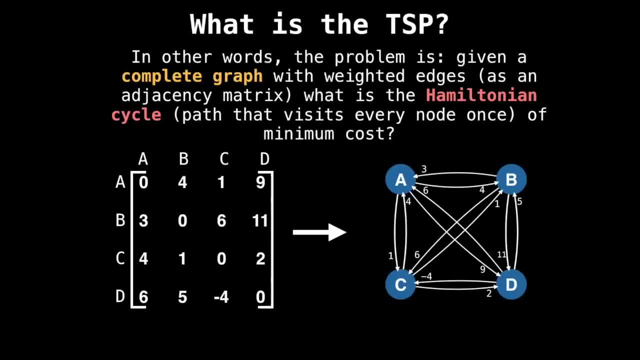 not exist. simply set the edges value to be positive infinity. So in the graph I had you can see that one optimal tour consists of going from A to D to C to B and then finally back to a, with a minimum cost of nine. Note that it is entirely possible to find the cost. 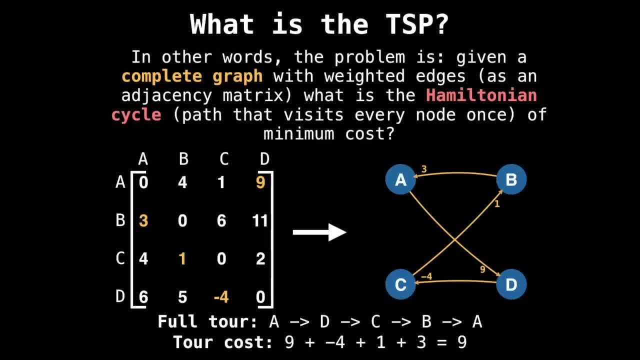 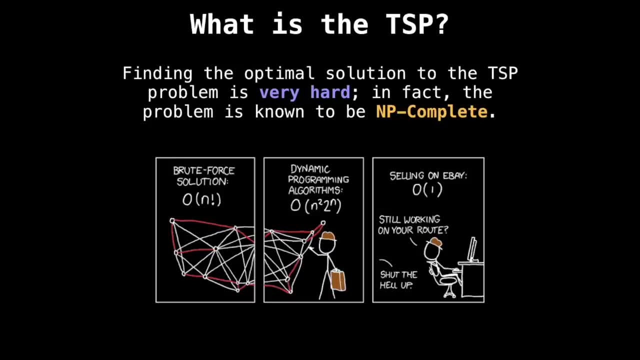 of the traveling salesman problem. So it's only possible that there are many possible valid optimal tours, but they will all have the same minimum cost. As it turns out, solving the traveling salesman problem is extremely difficult. In fact, the problem has been proven. 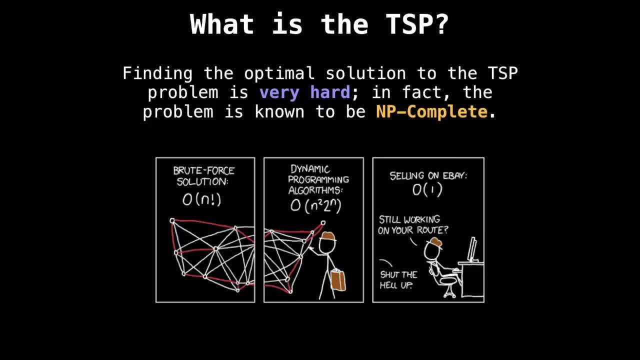 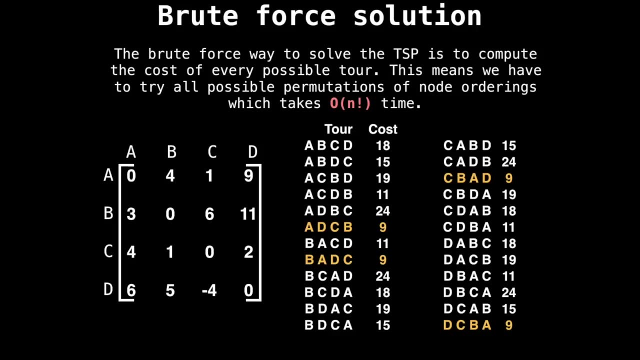 to be NP, complete meaning it's very difficult to find an optimal solution for large inputs. However, numerous approximation algorithms exist. If you want to get an optimal solution, get an algorithm that runs very quickly, even for large inputs. So the brute force way to. 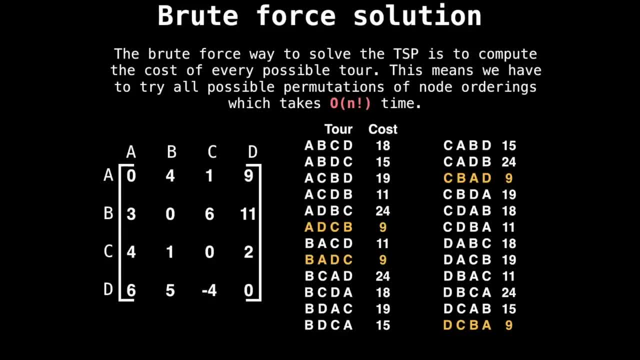 solve this problem is to actually compute all possible tours, And this means we have to try all permutation of node orderings, which will take big O of n factorial time, which is very slow. But, as you can see, I've listed all the permutation of nodes and highlighted 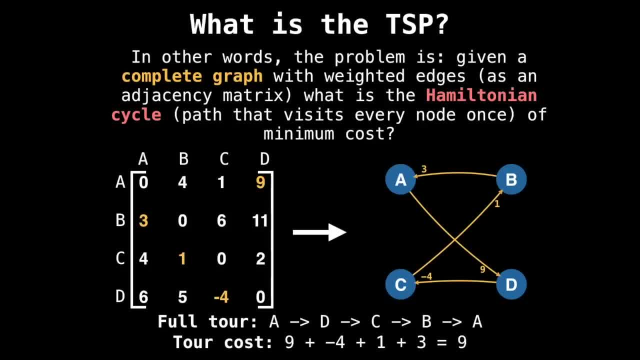 the graph I had, you can see that one optimal tour consists of going from A to D, to C to B and then finally back to A, with a minimum cost of nine. Note that it is entirely possible that there are many possible valid optimal tours, but they will. 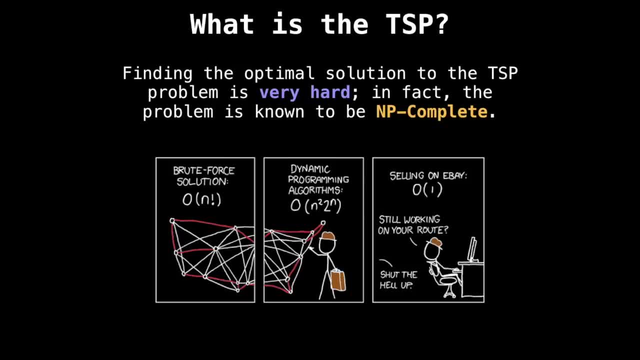 all have the same minimum cost. As it turns out, solving the traveling salesman problem is extremely difficult. In fact, the problem has been proven to be NP complete, meaning it's very difficult to find an optimal solution for large inputs, However numerous approximation. 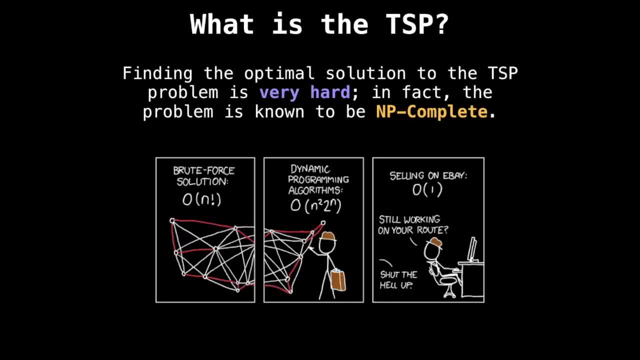 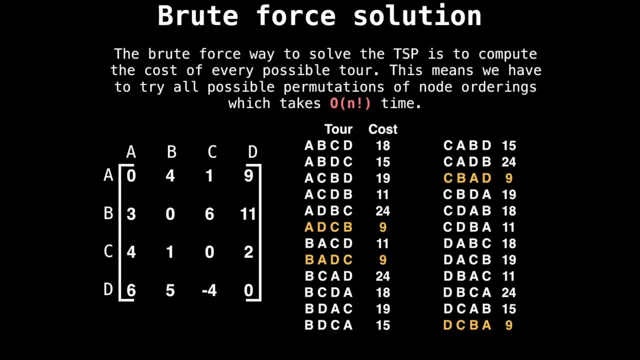 algorithms exist If you want to get an algorithm that runs very quickly, even for large inputs. So the brute force way to solve this problem is to actually compute all possible tours, And this means we have to try all permutation of node orderings, which will take big O of n factorial 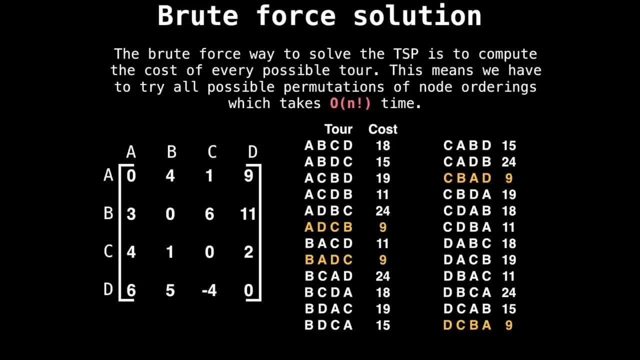 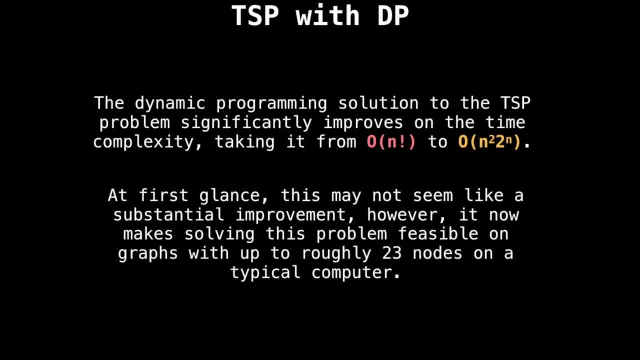 time, which is very slow, But, as you can see, I've listed all the permutation of nodes and highlighted the ones, The ones which yield the optimal solution. The dynamic programming solution we're going to develop today is able to improve on this naive approach by reducing the complexity. 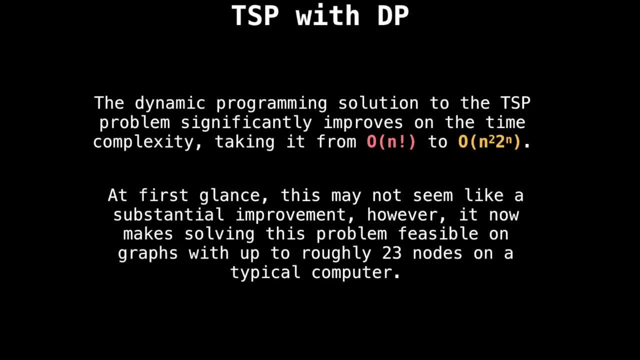 to big O of n squared times two at the end. At first glance this may not seem like a substantial improvement. However, it now makes graphs with roughly 23 nodes give or take feasible for modern home computers. Here's a table of n factorial versus n squared to the end. 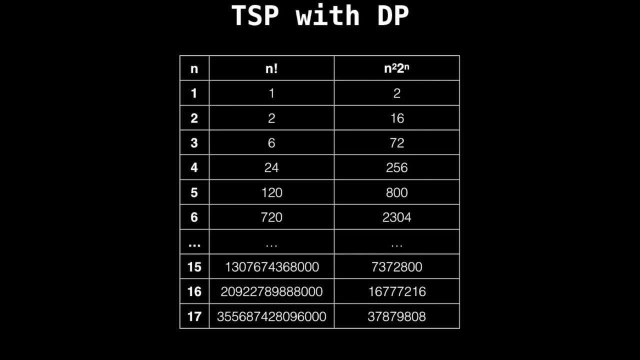 At first you notice that n factorial is optimal for small numbers. But this quickly changes favor to n squared to the end, which can give a significant improvement over n factorial. you can already see that how large the numbers get for n factorial when we hit n equals 15. 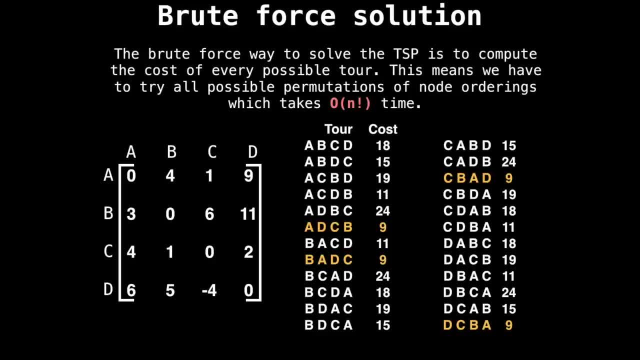 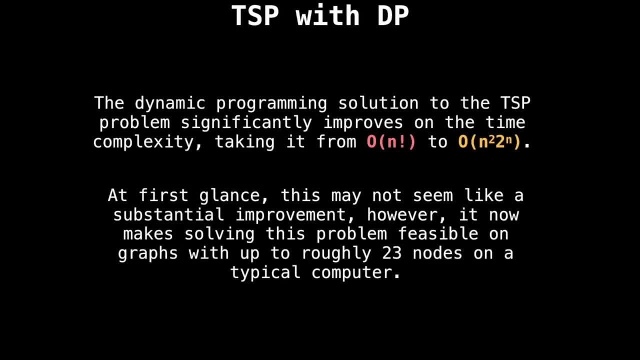 the ones which yield the optimal. The optimal solution, The dynamic programming solution we're going to develop today, is able to improve on this naive approach by reducing the complexity to big O of n squared times to the end. At first glance, this may not seem like a substantial improvement, However. 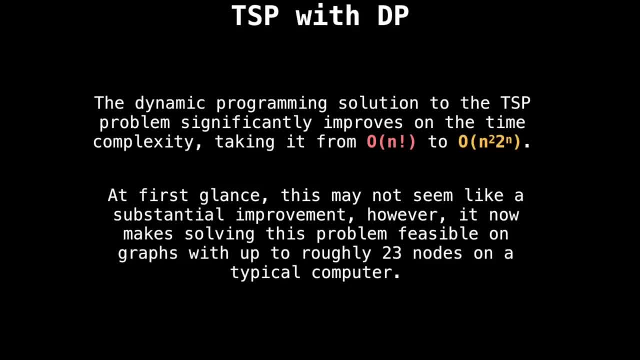 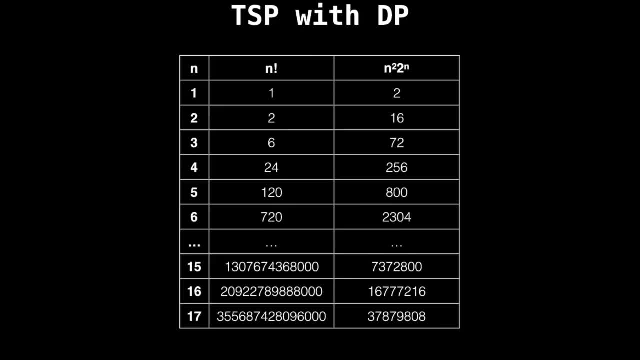 it now makes graphs with roughly 23 nodes give or take feasible for modern home computers. Here's a table of n factorial versus n squared to the n. At first you notice that n factorial is optimal for small numbers, But this quickly changes favor to n squared to the n, which 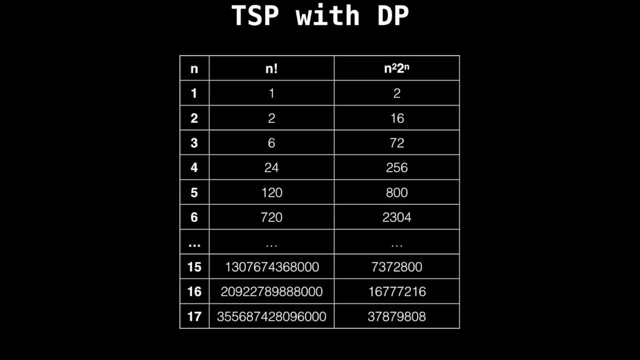 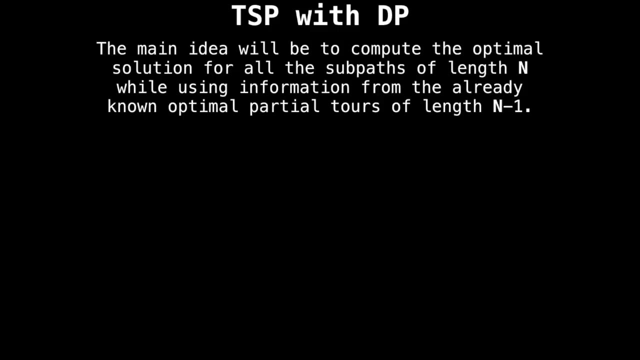 can give a significant improvement over n factorial. you can already see that how large the numbers get for n factorial when we hit n equals 15 versus the n squared to the n squared to the n. All right time to talk about how to solve this problem using dynamic. 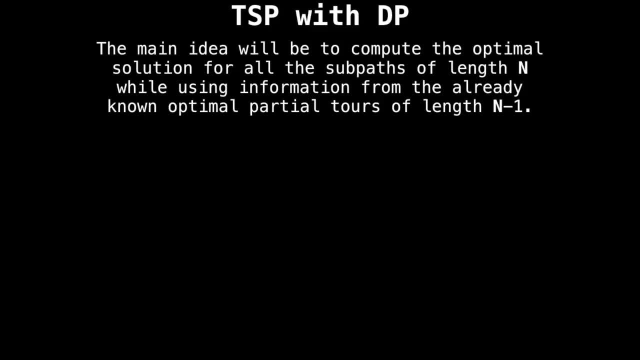 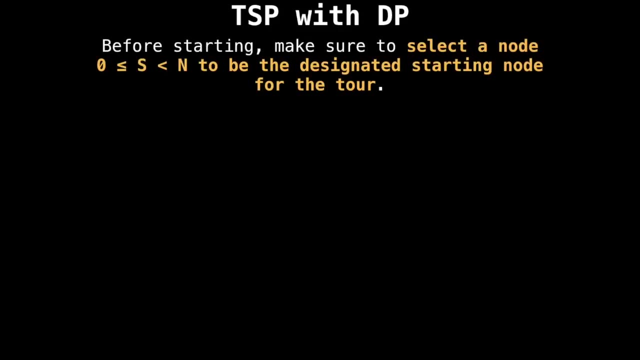 programming. The main idea is going to be to compute the optimal solution for paths of length, and we will have to reuse information from paths of length and minus one. But before we get started, there's some setup information we need to talk about. The first thing we're 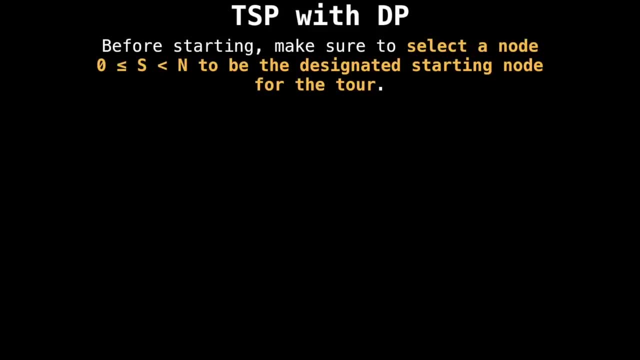 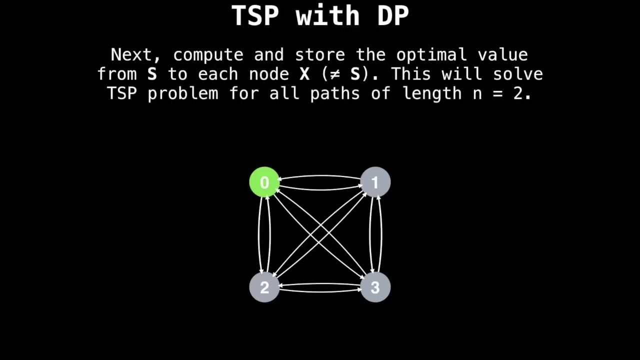 going to need to do is pick a starting node s. it doesn't matter which node is picked, just make sure that this nodes index is between zero and n, non inclusive. Suppose we have this graph with four nodes and we choose our starting node to be node zero. The next thing we need to do is store. 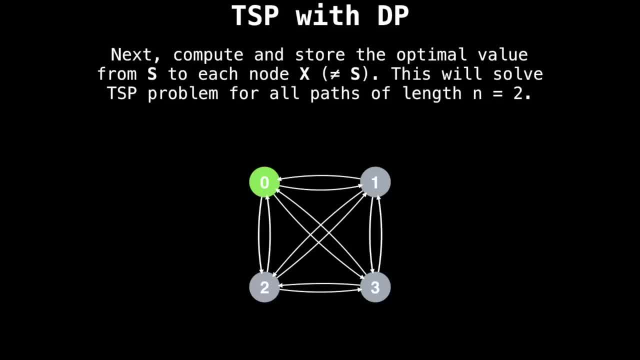 the optimal value from s, the starting node, to every other node. This will solve the traveling salesman problem for all paths with exactly two nodes. the optimal value for paths with two nodes is given in the input through the adjacency matrix, And this is all the setup we need to do. 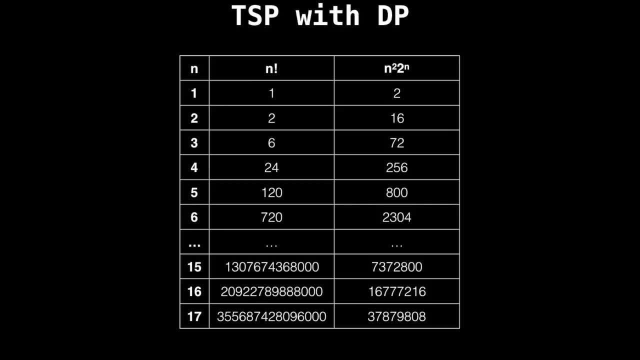 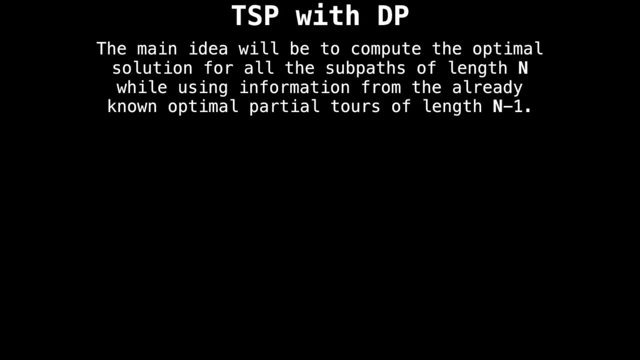 versus the n squared to the end. All right time to talk about how to solve this problem using dynamic programming. The main idea is going to be to compute the optimal solution for paths of length n. we will have to reuse information from paths of length and minus one, But before 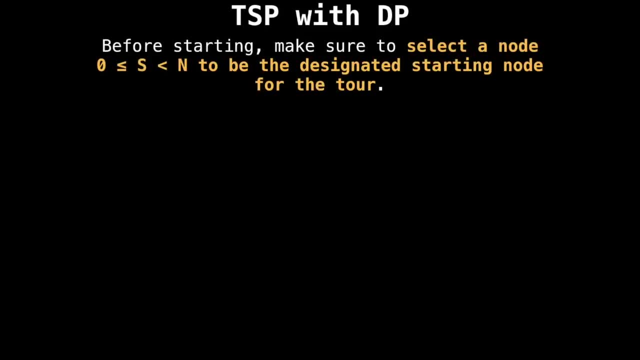 we get started, there's some setup information we need to talk about. The first thing we're going to need to do is pick a starting node s. it doesn't matter which node is picked, just make sure that this nodes index is between zero and n, non inclusive, Suppose we have. 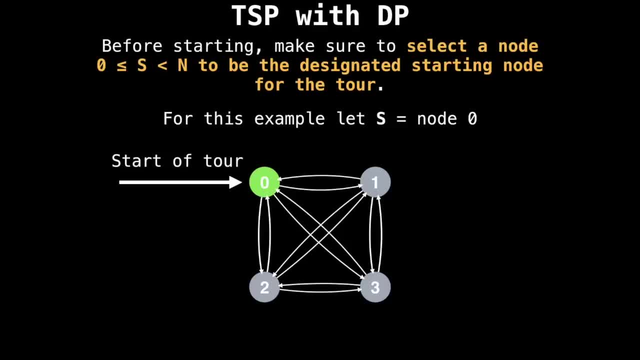 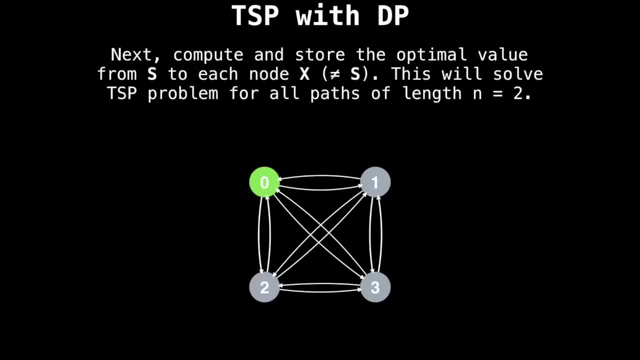 this graph with four nodes and we choose our starting node to be node zero. The next thing we need to do is store the optimal value from s, the starting node, And then we can store the value from s, the starting node, to every other node. This will solve the. 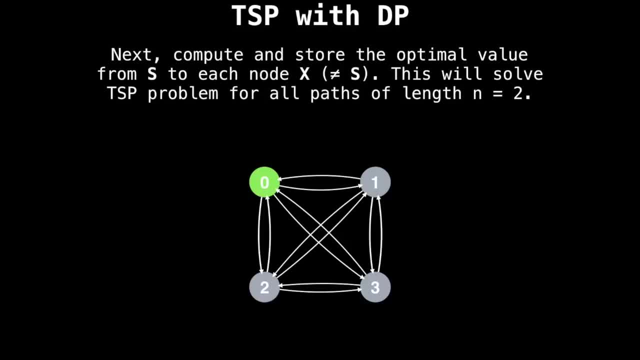 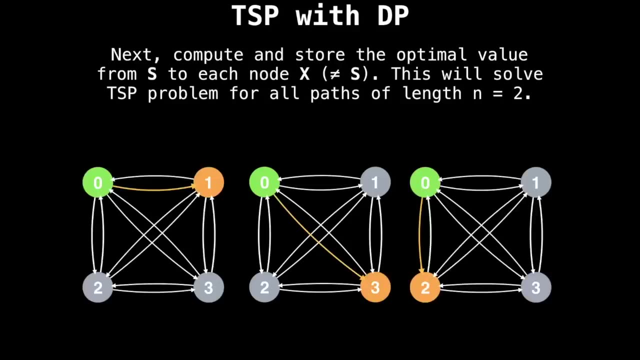 traveling salesman problem for all paths with exactly two nodes. the optimal value for paths with two nodes is given in the input through the adjacency matrix. And this is all the setup we need to do Visually, if you want to look at it, we can see that we would. we'd 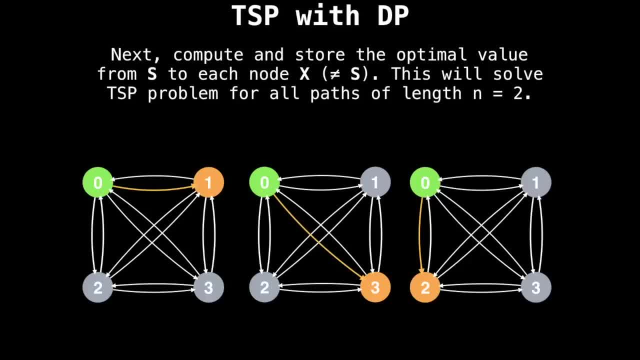 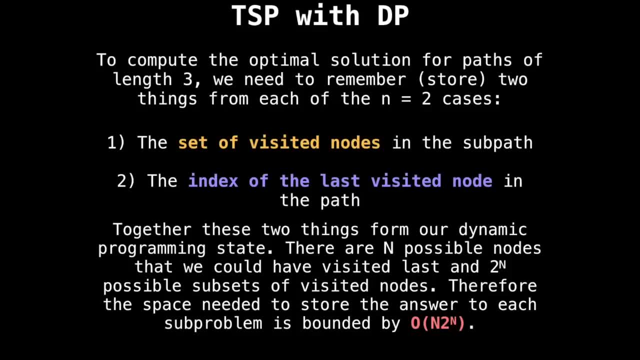 store the value from zero to n, and then we can store the value from zero to n, and then we can store the value from zero to n, and then we can store the value from zero to n, zero to one, zero to two and finally zero to three. In the last slide I talked about 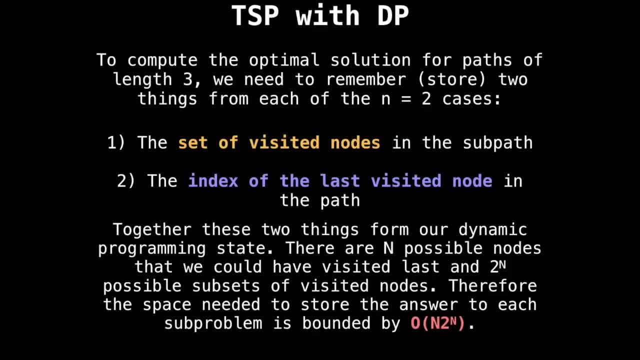 storing the solution for n equals two, But what is it we really need to store? there are two key things. The first is obvious, and that's the set of visited nodes and the partially completed tour. The other is the index of the last visited node in the path. 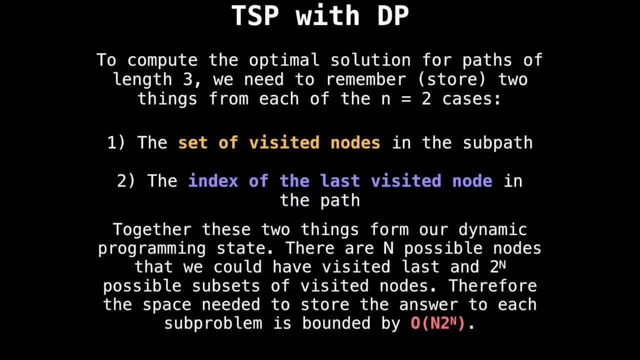 For each partially completed tour. we need to save which node was the last node we were on so that we can continue extending that partially completed tour from that node we were on and not from some other node. This is very important. So together, these two, 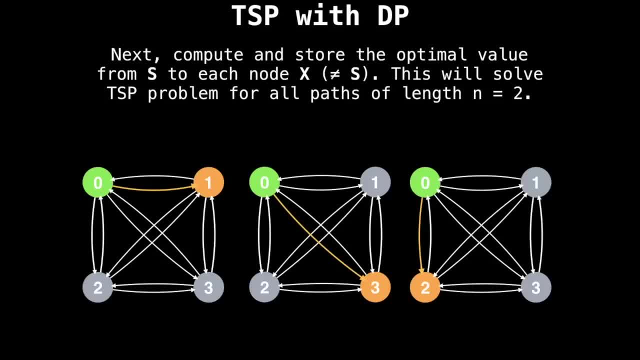 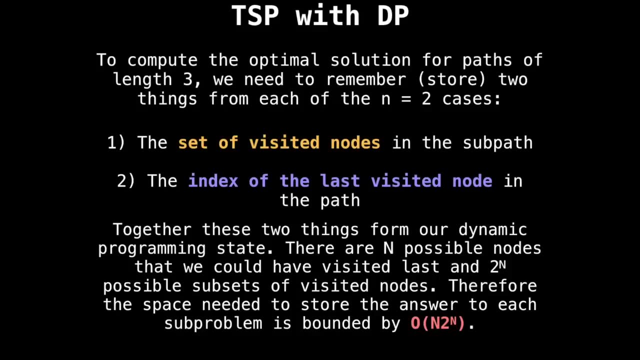 Visually, if you want to look at it, we can see that we would. we'd store the value from zero to one, zero to two And finally zero to three. In the last slide I talked about storing the solution, for n equals two. But what is? 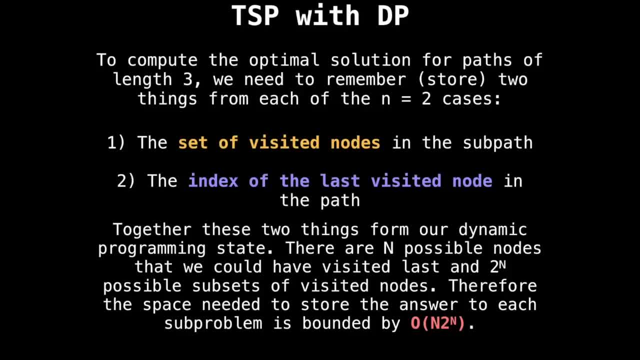 it we really need to store. there are two key things. The first is obvious, and that's the set of visited nodes and the partially completed tour. The other is the index of the last visited node in the path For each, Each partially completed tour. we need to save which node was the last node we were. 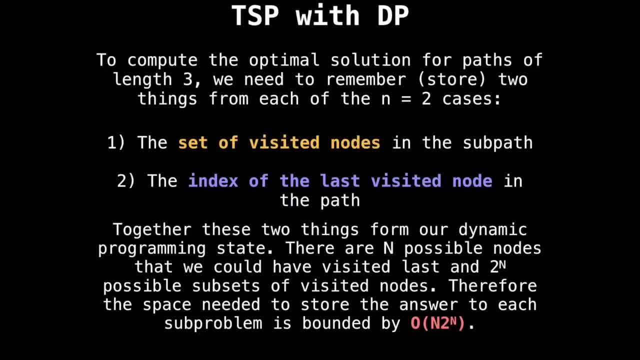 on so that we can continue extending that partially completed tour from that node we were on and not from some other node. This is very important. So together, these two things, the set of visited nodes and the index of the last visit node- form what I call. 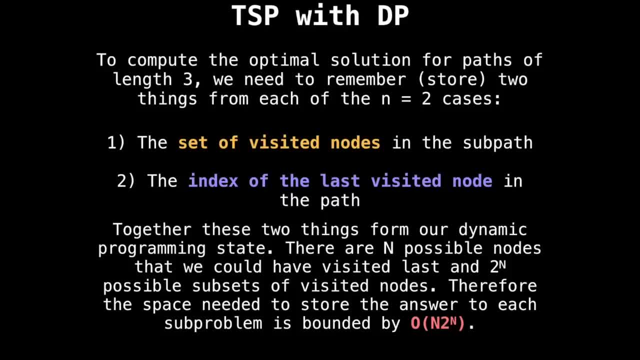 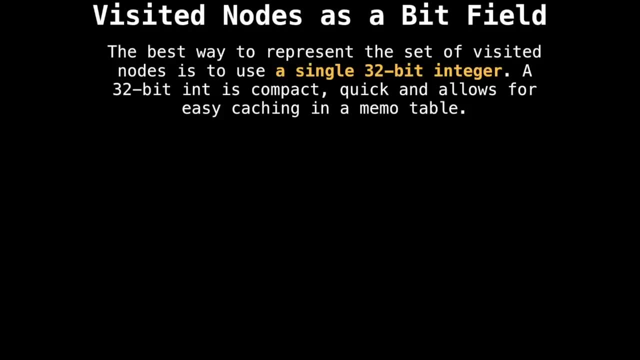 the dynamic programming State. Since there are n possible last nodes and to the power of n node subsets, our storage space is bounded by big O of n times to the end. An issue we're going to face when trying to store the DP state is representing the set of visited nodes And the way- and I mean 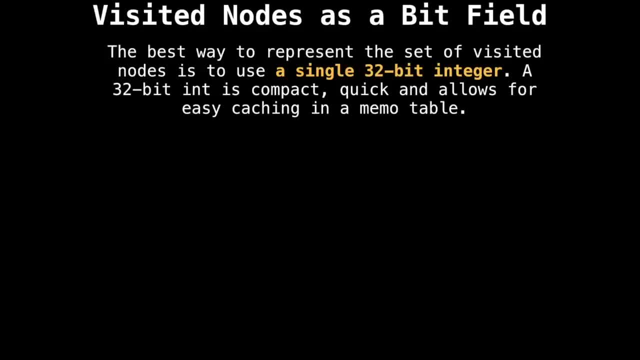 the way to do this is to use a single 32 bit integer. The main idea is that if the ID note has been visited, we flip on the bit to a one in the binary representation of the integer. The advantage to this representation is that 32 bit integer is compact, quick and allows for easy caching. 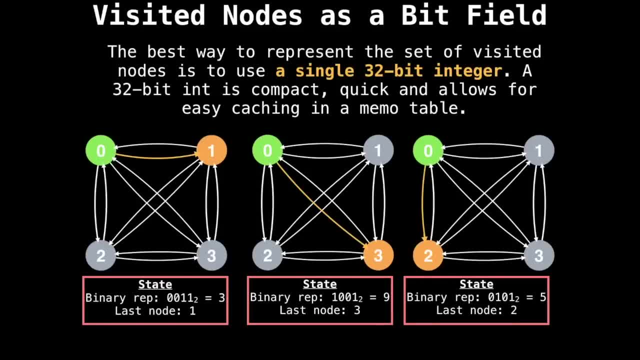 in a memo table, For example, on the left most graph we have visited the zero and first nodes. So the binary representation is 0011.. If the least significant bit is on the right, Similarly, the binary representation of the middle graph is 1001. 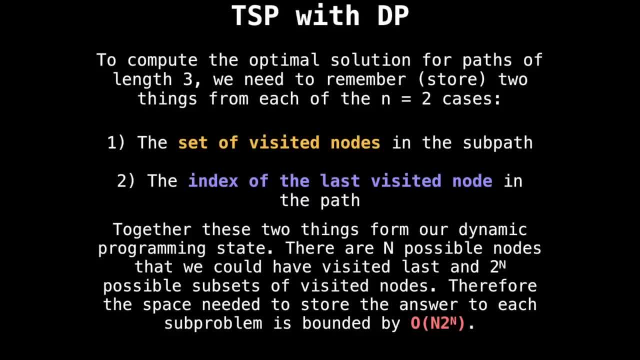 things: the set of visited nodes and the index of the last visit node form what I call the dynamic programming state. Since there are n possible last nodes and to the power of n node subsets, our storage space is bounded by big O of n times to the n, An issue we're going to face. 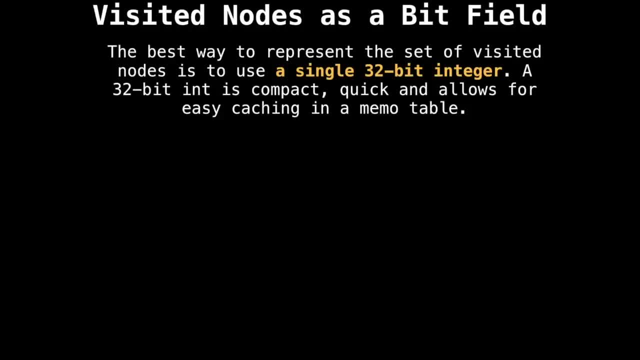 when trying to store the DP state is representing the set of visited nodes, And the way- and I mean one way- to do this is to use a single 32 bit integer. The main idea is that if the ith node has been visited, we flip on the ith bit to a one in the binary representation. 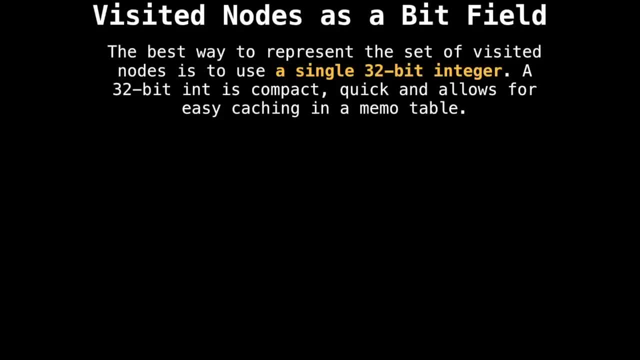 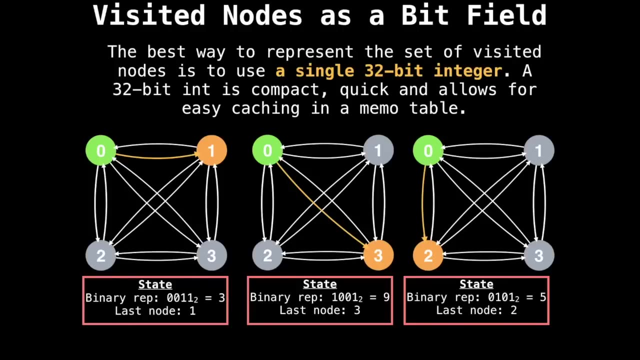 of the integer. The advantage to this representation is that a 32 bit integer is compact, quick and allows for easy caching in a memo table, For example. on the leftmost graph we have a single 32 bit integer. visited the zeroth and first nodes, So the binary representation is 0011.. If the least. 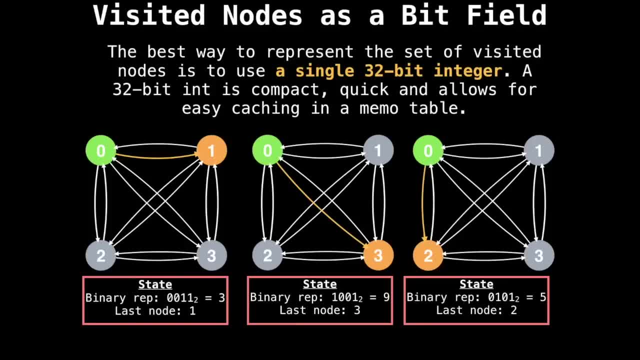 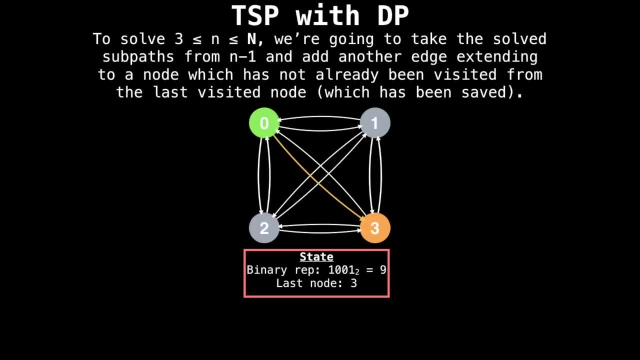 significant bit is on the right. Similarly, the binary representation of the middle graph is 1001, or just the number nine and decimal, since nodes zero and three have been visited. Now suppose we're trying to expand on our previous state. one particular instance of a two node partial: 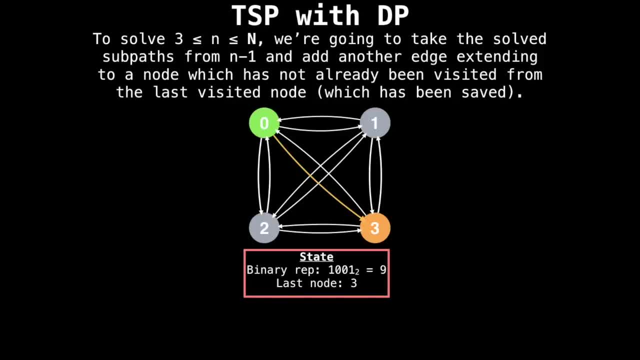 torso shown below. what we want to do from our last node, which in this graph is no three, is expand to visit all other unvisited nodes. These are the gray nodes one and two, to make our partial Tor a little longer with three nodes And if there are the two nodes that 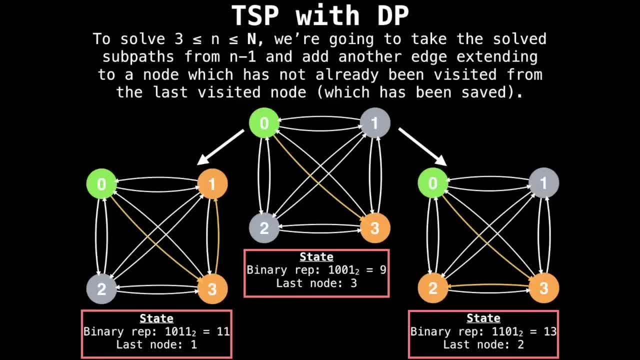 are actually visited, then we're gonna ask that jä��릴게요 and jä legislature тебя to do number three instead particular state. we were able to generate an additional two states, But we would also need to do this for all states with two nodes, not just this one with zero and three In. 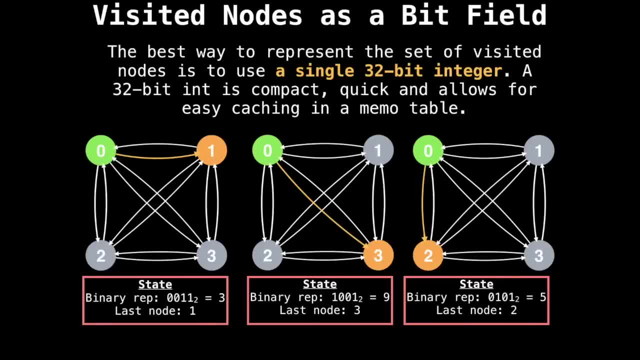 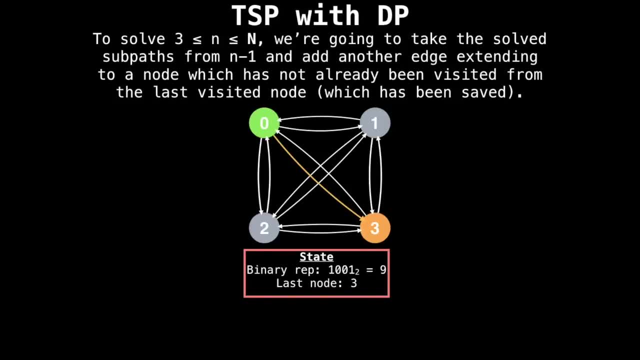 or just the number nine and decimal, since nodes zero and three have been visited. Now suppose we're trying to expand on our previous state. One particular instance of a two node partial tour is shown below: What we want to do from our last node, which in this graph, 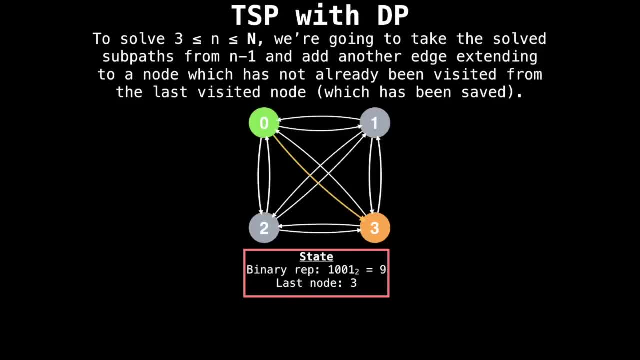 is no. three is expand to visit all other unvisited nodes. These are the gray nodes one and two. to make our partial tour a little longer with three nodes, For this part we want to expand to the left and right side. So let's say we want to expand. 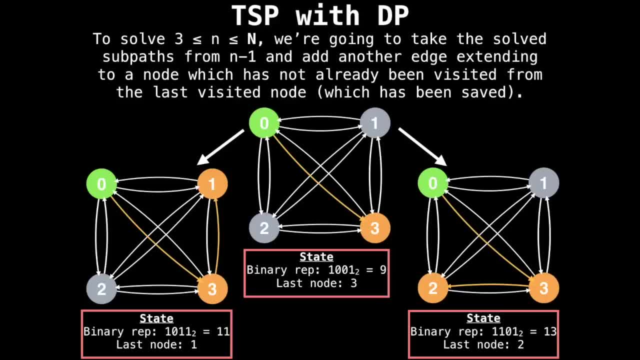 particular state, we were able to generate an additional two states, But we would also need to do this for all states with two nodes, not just this one with zero and three. In total, this process would result in six new states for partial tours with three nodes. 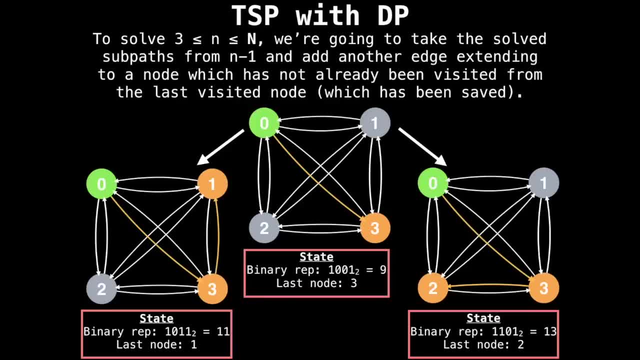 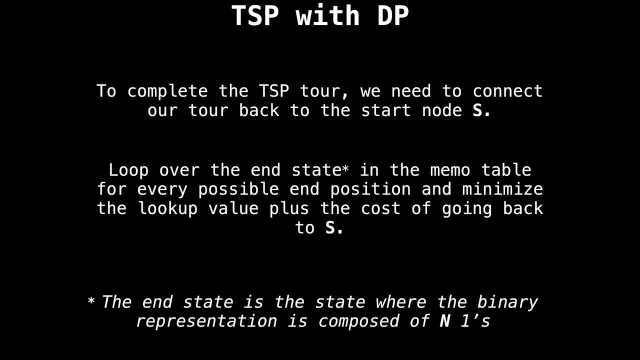 This process continues with gradually longer and longer paths until all paths are of length, and the last thing we need to do to wrap up the traveling salesman problem is to reconnect the tour to the designated starting node s. To do this loop over the end state in the 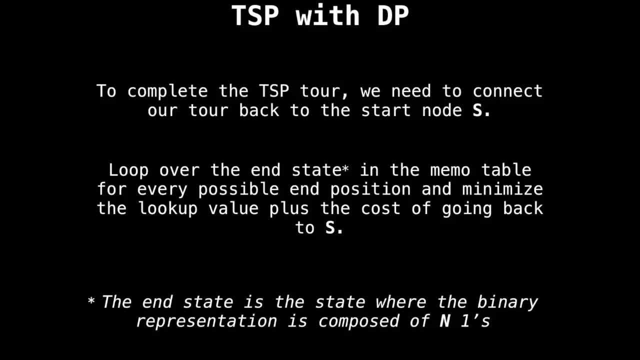 memo table for all possible end positions excluding the start node, and minimize the look up value plus the cost of going back to s. Note that the end state is the one where the binary representation is composed of all ones, meaning each node has been visited. It's finally. 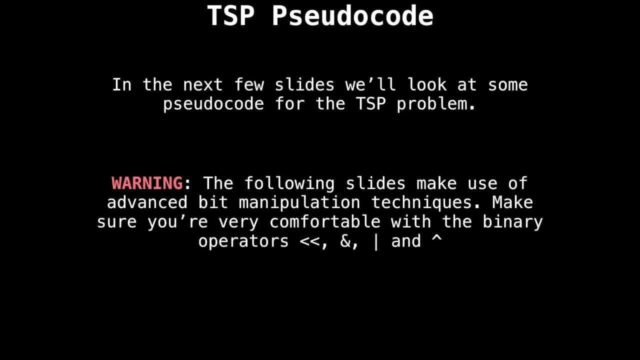 time to look at some pseudocode for the traveling salesman problem. Just a heads up to everyone who's still a beginner: the following slides make use of advanced bit manipulation techniques, So make sure you're familiar with this, Make sure you're comfortable with how binary shifts and ores and X ores work. Here's the. 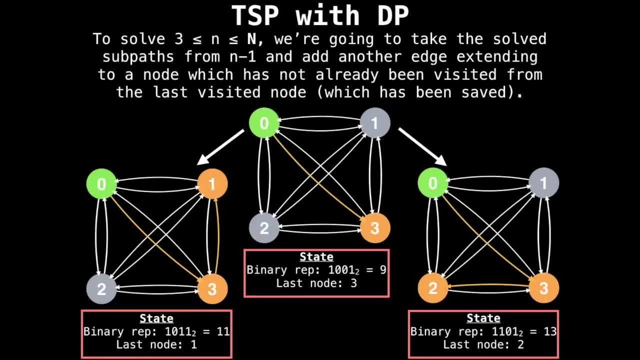 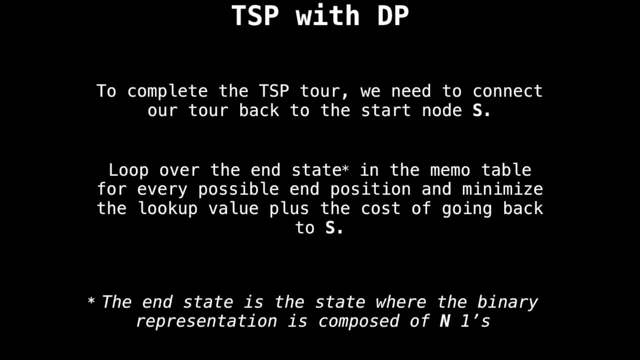 total, this process would result in six new states for partial tours with three nodes. This process continues with gradually longer and longer paths until all paths are of length, and the last thing we need to do to wrap up the traveling salesman problem is to reconnect the tour to the designated starting node s To do this loop over the end state in the 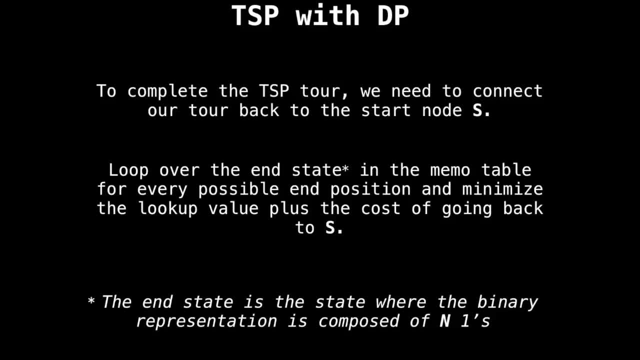 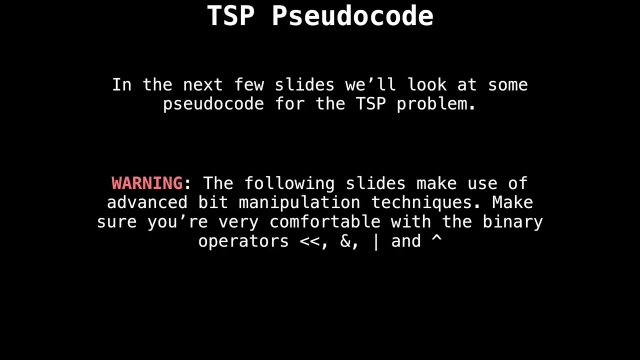 memo table for all possible end positions, excluding the start node, and minimize the look up value plus the cost of going back to s. Note that the end state is the one where the binary representation is composed of all ones, meaning each node has been visited. It's finally time to look at some pseudocode for the traveling. 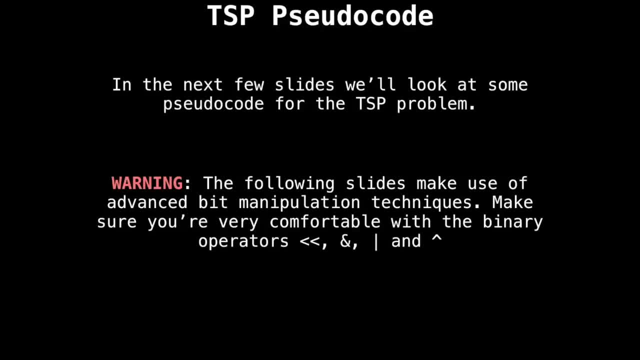 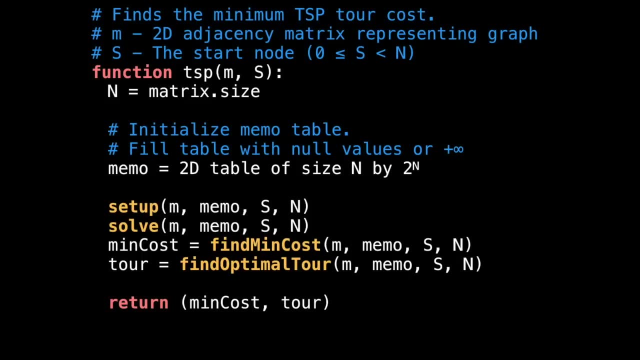 salesman problem. Just a heads up to everyone who's still a beginner: the following slides make use of advanced bit manipulation techniques. So make sure you're familiar with the advanced bit manipulation techniques and make sure you're comfortable with how binary shifts and ores and X ores work. Here's the function that solves the traveling salesman problem. 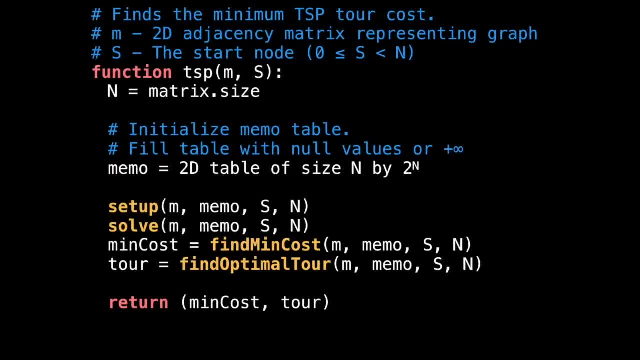 It takes two inputs. The first is m, a two dimensional adjacency matrix representing the input graph, and s, the index of the starting node. The first thing we do is get the size of the matrix and store it in a variable color called n, which tells us how many nodes there are. Then we initialize the two dimensional 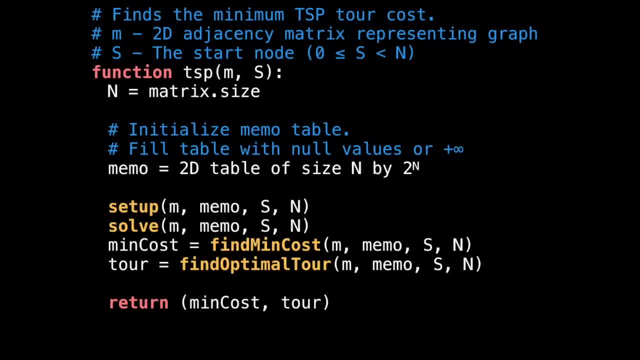 memo table. the table should have size n by to the power of n. I recommend filling the table with null values so that programmatic errors throw runtime exceptions. Then we're going to call four functions: setup, solve, find min cost and find optimal tour. 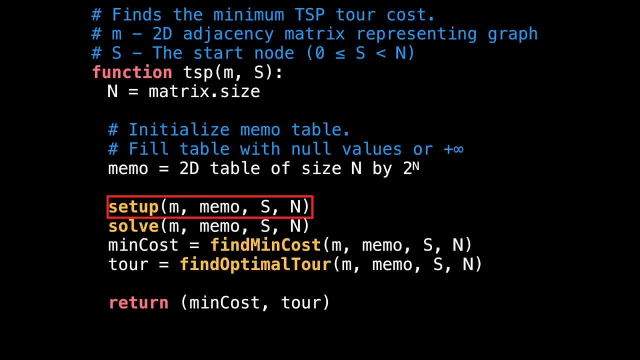 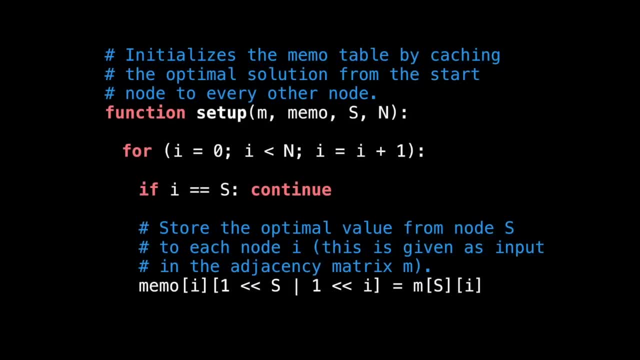 Let's begin by looking at what happens inside the setup method. The setup method is very easy. It simply does what I illustrated a few slides ago by storing the optimal value from the start node to every other node. you loop through each node, skipping over the start. 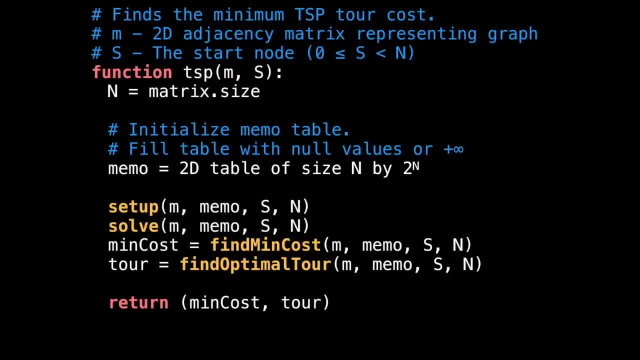 function that solves the traveling salesman problem. It takes two inputs. The first is m, a two dimensional adjacency matrix representing the input graph, and s, the index of the starting node. The first thing we do is get the size of the matrix and store it in a variable called 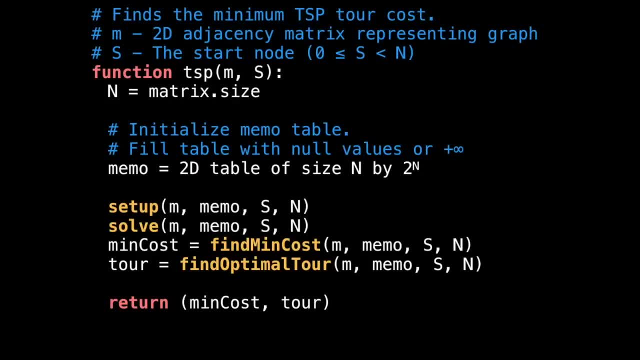 n, which tells us how many nodes there are. Then we initialize the two dimensional memo table. The table should have size n by to the power of n. I recommend filling the table with null values so that programmatic errors throw runtime exceptions. Then we're going. 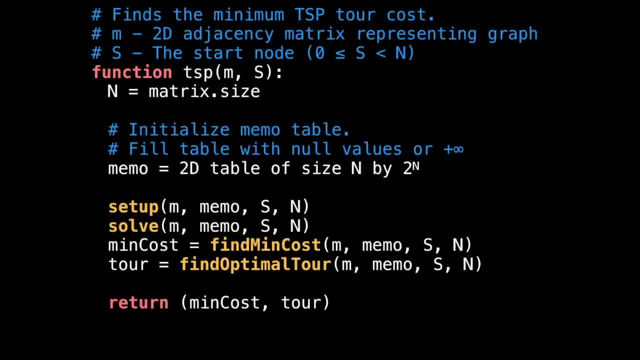 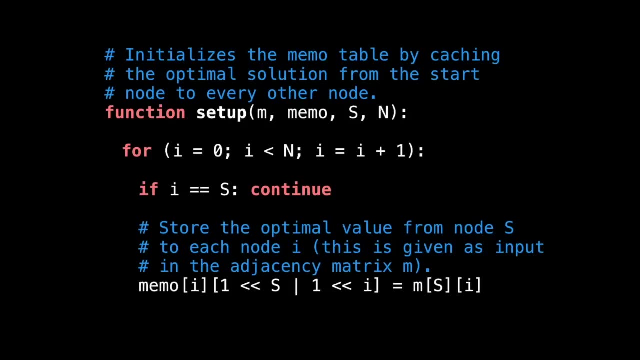 to call four functions: setup, solve, find min cost and find optimal tour. Let's begin by looking at what happens inside the setup method. The setup method is very easy. It simply does what I illustrated a few slides ago by storing the optimal value. 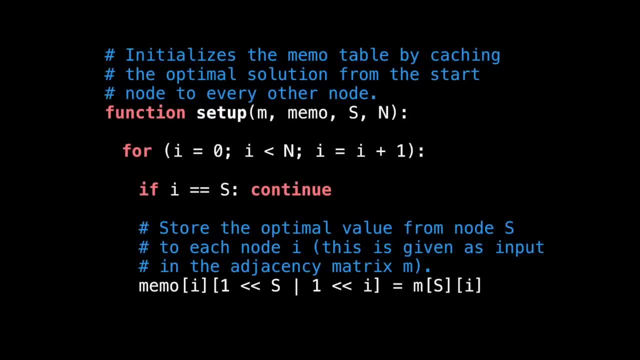 from the start node to every other node. you loop through each node, skipping over the start node, And then you cache the optimal value from s to i which can be found in the distance. So in this case, I'm going to use the start node And then I'm going to use the end node, as 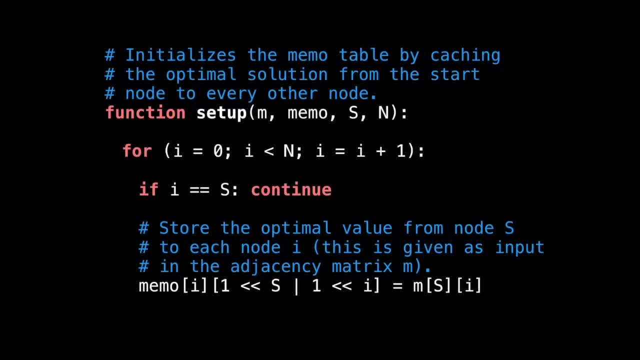 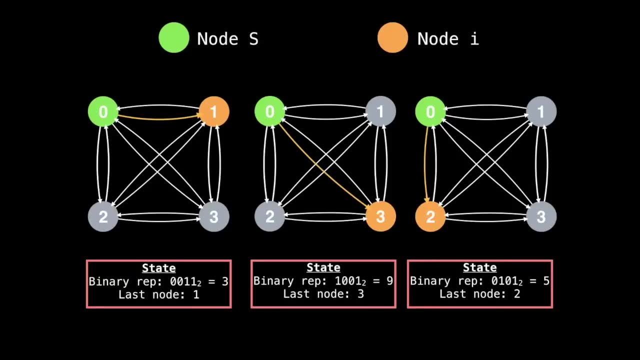 i and the mask with bits s and i set to one, hence the double bit shift. Visually, the green node is the start node and orange node is node i, which changes with every iteration. You notice now that the orange node is never on top of the green node, which is why I'm 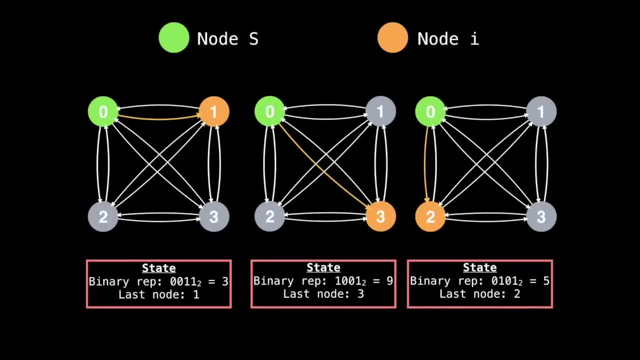 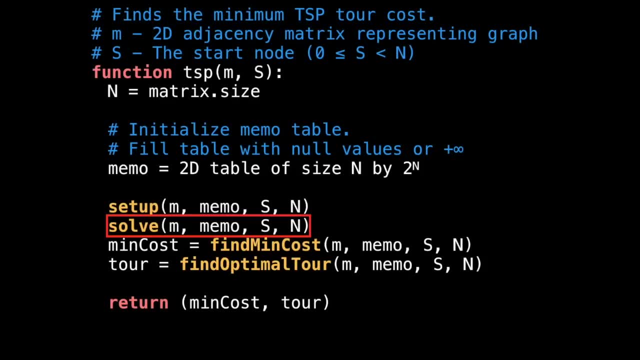 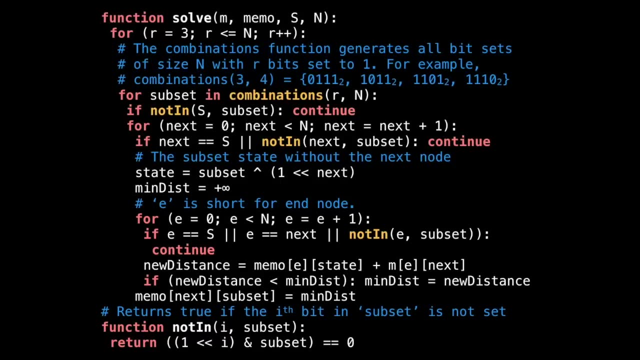 going to use the end node, which is why I had a continue statement to skip that case. Now let's look at how the solve method works. The solid method is by far the most complicated, but I've broken it down to be easy to understand. The first line in the method loops over r. 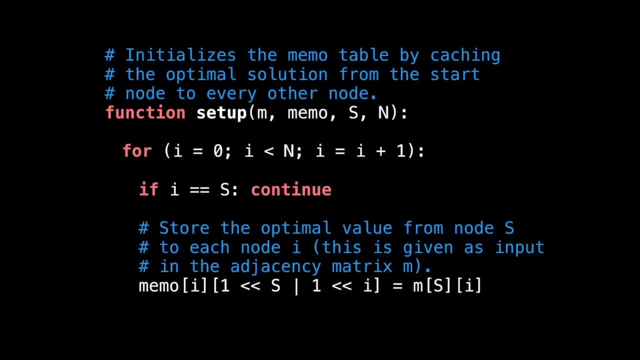 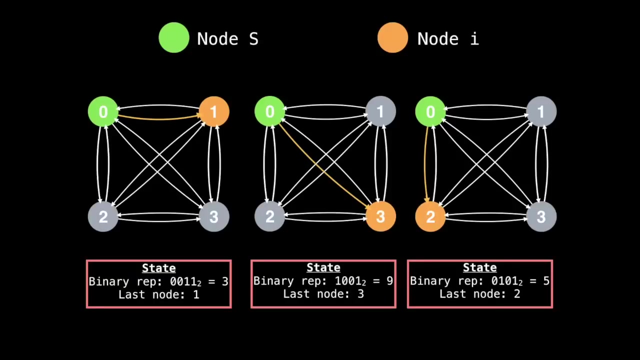 node And then you cache the optimal value from s to i which can be found in the distance matrix. The DP state you store is the end node as I, and the mask with bits s and i set to one, hence the double bit shift. Visually, the green node is the start node and orange. 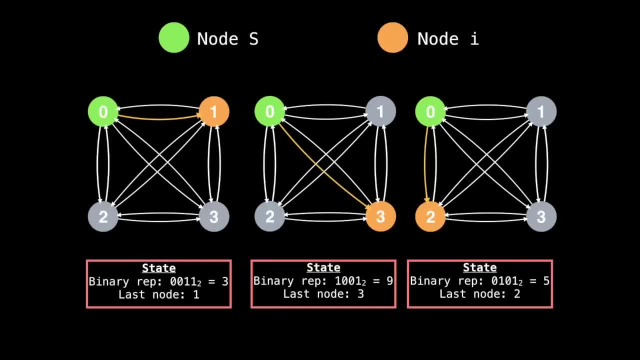 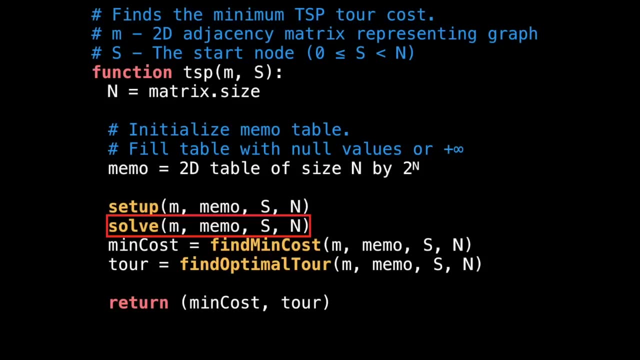 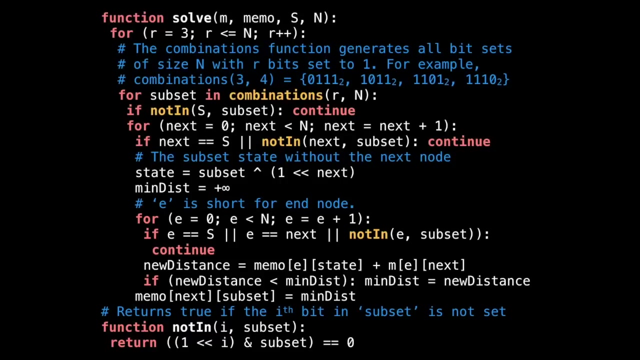 node is node i, which changes with every iteration. You notice now that the orange node is never on top of the green node, which is why I had to continue statement to skip that case. Now let's look at how the solve method works. The solid method is by far the most complicated. 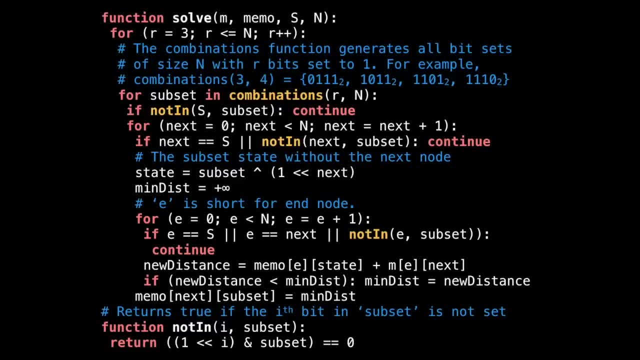 but I've broken it down to be easy to understand. The first line in the method: loops over r equals three up to an inclusive. Think of our as the number of nodes in a particular partial tour. So we're increasing this number one at a time. The next line says for subset: 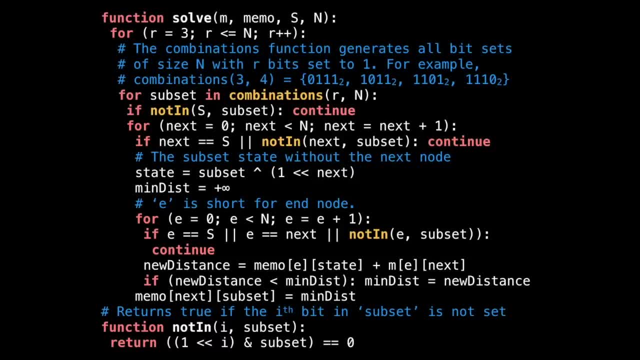 in combinations. The combinations function generates all bit sets of size and with exactly our bits set to one. For example, as seen in the comments, when calling the combinations function with r equals three and n equals four, we get four different bit sets And 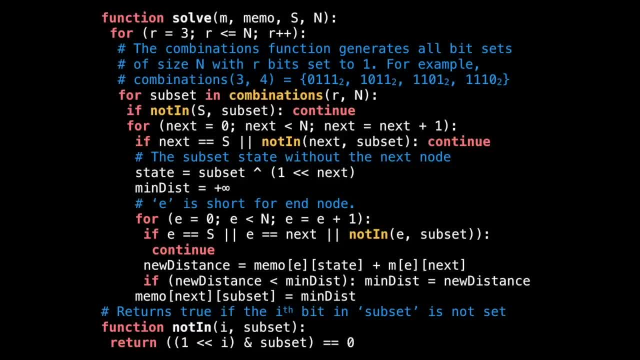 then we get a set of nodes, each distinct and with three ones turned on. These are meant to represent a subset of visited nodes. Moving on, notice that I enforce the node s to be part of the generated subset. Otherwise, the subset of nodes is not valid, since it 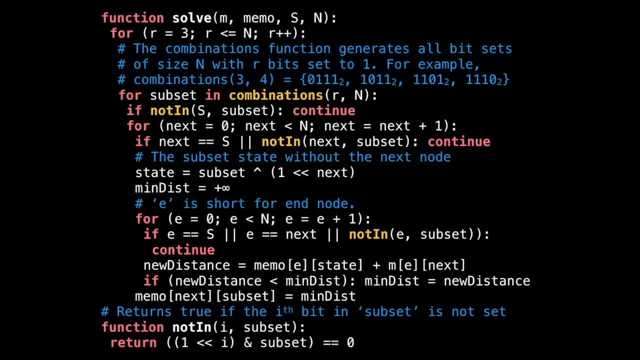 could not have started at our designated starting node. Notice that this if statement calls the not in function defined at the bottom of this slide. all it does is it checks. if the ith bit in the subset is a zero, Then we loop over a variable called next, which represents the index of the next node. 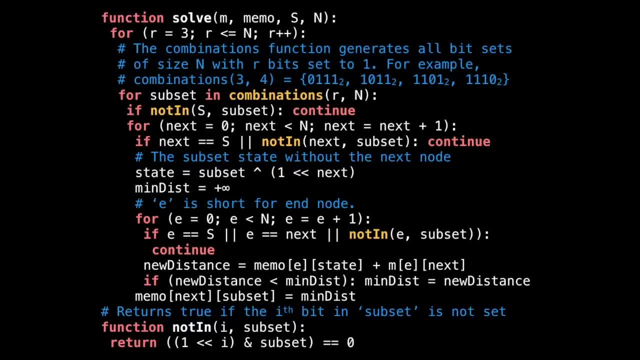 equals three up to an inclusive. Think of our as the number of nodes in a particular set of nodes in a partial tour. So we're increasing this number one at a time. The next line says four subset in combinations. The combinations function generates all bit. 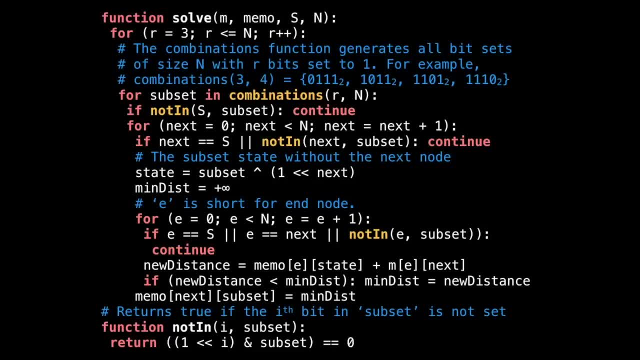 sets of size and with exactly our bits set to one. For example, as seen in the comments, when calling the combinations function with r equals three and n equals four, we get four different bits. The next line says four sets, each distinct and with three ones turned on. These are meant. 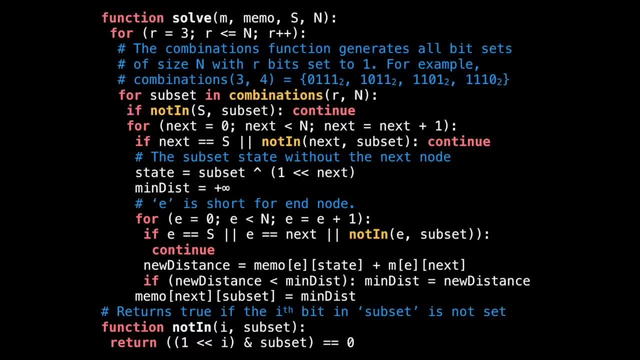 to represent a subset of visited nodes Moving on, notice that I enforce the node s to be part of the generated subset. Otherwise the subset of nodes is not valid, since it could not have started at our designated starting node. Notice that this if statement calls the not in function defined at the bottom of this slide. all it. 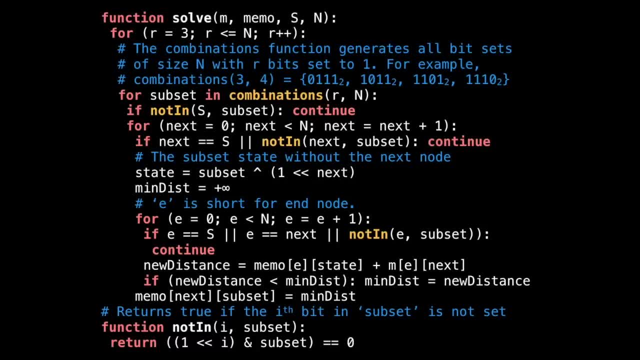 does is it checks. if the I th bit in the subset is a zero, Then we loop over a variable called Next, which represents the index of the next node. The next node must be part of the current subset. This may sound strange, but know that the 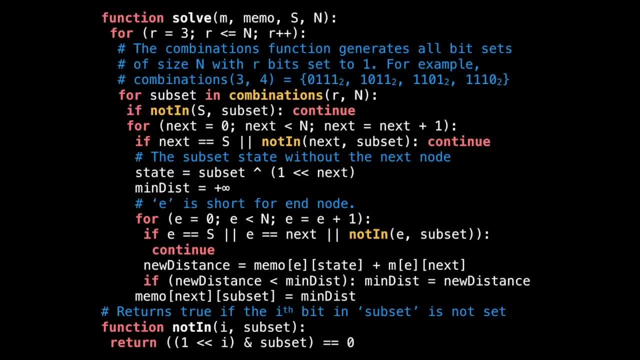 subset is part of the current subset. This may sound strange, but know that the subset subset variable generated by the combinations function has a bit which is meant for the next node. This is why the variable state on the next line represents the subset excluding the next node. This is so we can look up in our memo table to figure out what the best. 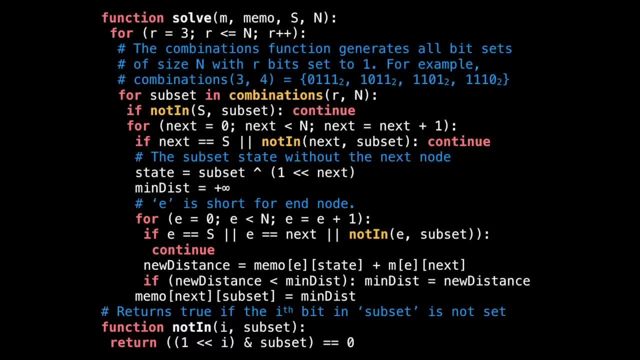 The next node must be part of the current subset. This may sound strange, but know that the subset variable generated by the combinations function has a bit which is meant for the next node. This is why the variable state on the next line represents the subset excluding. 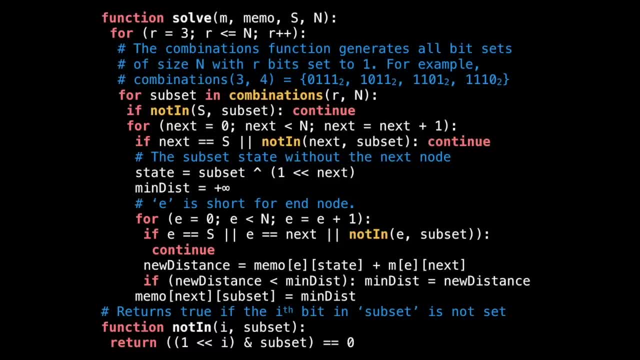 the next node. This is so we can look up in our memo table to figure out what the best partial tour value is when the next node was not yet in the subset. Being able to insulate that second value as the null value here is how you can get the best rest partial value. 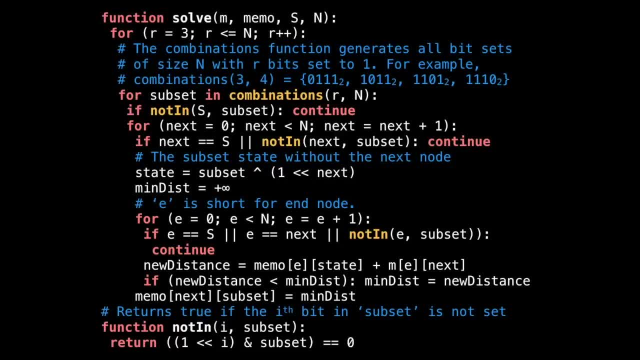 It's all done, of course, by look at your 38.1, 18 put and then you're good. After that, to look back and reuse parts of other partially completed tours is essential to the dynamic programming aspect of this algorithm. The following variable to consider is E short. 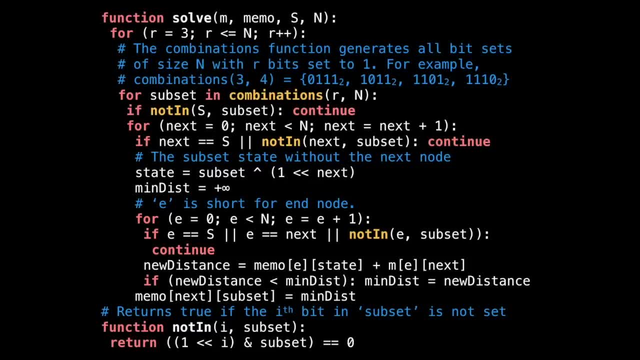 for end node Because I ran out of room. this variable is quite important Because, while the next node is temporarily fixed in the scope of the inner loop, we try all possible end nodes of the current subset and try to see which end node best optimizes this partial 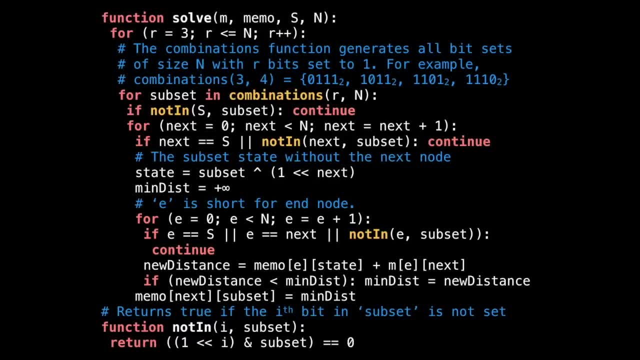 tour. Of course the end node cannot be any of the start node, the next node or not be part of the current subset that we're considering. So we skip all those possible end nodes And we're going to look at all possible end nodes. So we compute the new distance and compare. 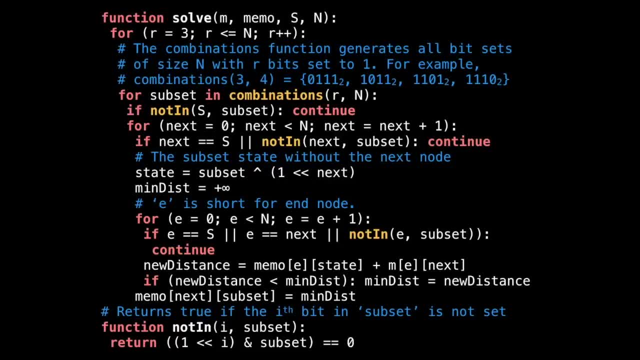 partial tour value is when the next node was not yet in a subset. Being able to look back in the reuse parts of other partially completed tours is essential to the dynamic programming aspect of this algorithm. The following variable to consider is E short for end node, because 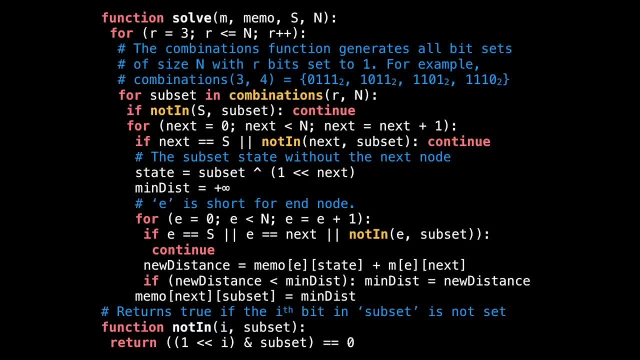 I ran out of room. this variable is quite important Because, while the variable state on the next line represents the subset excluding the combinations function, the next node is temporarily fixed in the scope of the inner loop. we try all possible end nodes of the current subset and try to see which end node best optimizes this partial. 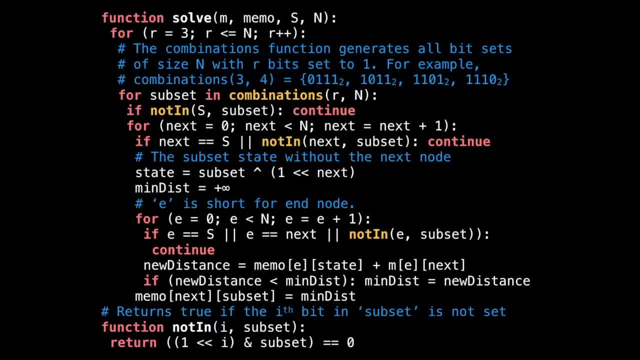 tour. Of course the end node cannot be any of the start node, the next node or not be part of the current subset that we're considering. So we skip all those possibilities. So we compute the new distance and compare it to the minimum distance. If the new distance 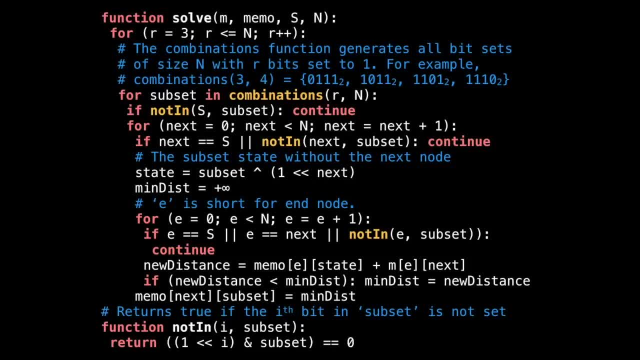 is better than the minimum distance, then we update the best minimum distance Afterwards, once we've considered all possible end nodes to connect to the next node, we store the best partial tour in the memo table And this concludes the solve method, The only unanswered. 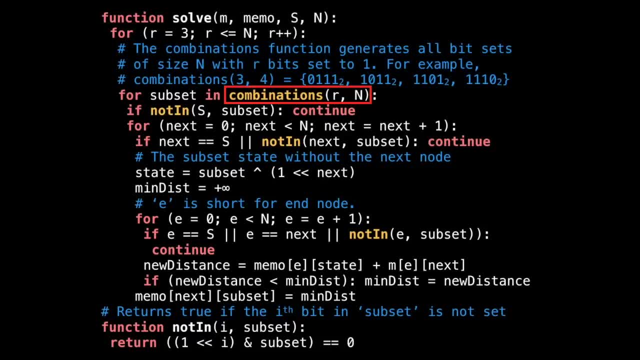 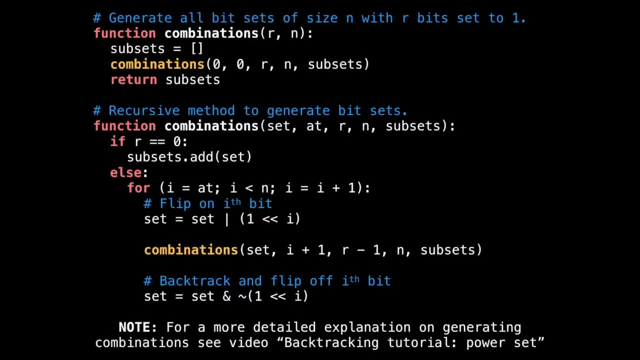 question in this slide is how the combinations method works, And I do not mean to leave this unanswered. So let's see how this gets done. This method is actually far simpler than you might imagine for what it does. What the first combinations method does is it fills up the subsets array. 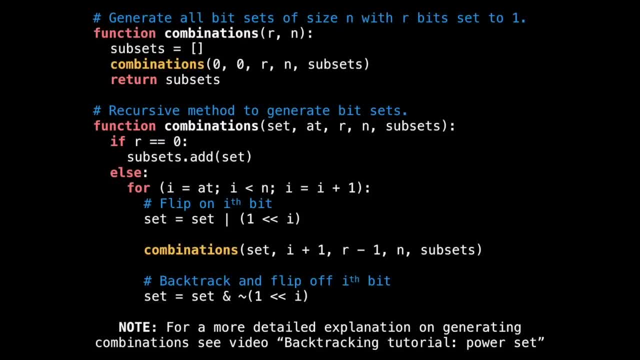 using the second combinations method and then returns that result. So what does the second combinations method do? I already covered this in more detail in my tutorial: backtracking the power set, if you want more detail, but I'll give you a quick rundown of what this. 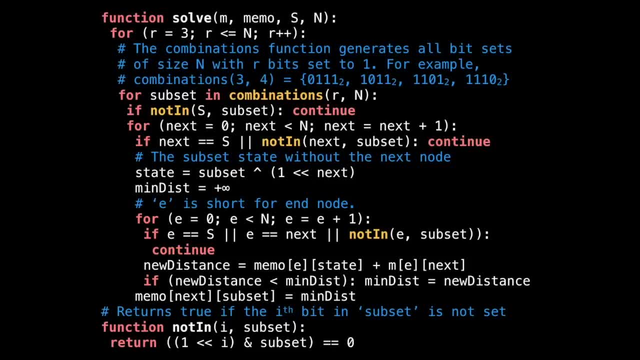 it to the minimum distance. If the new distance is better than the minimum distance, then we update the best minimum distance Afterwards, once we've considered all possible end nodes to connect to the next node. we store the best partial tour in the memo table And this 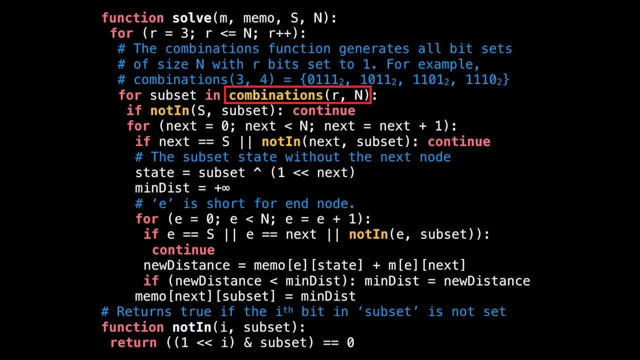 concludes the solve method. The only unanswered question in the next part of this algorithm, of this slide, is how the combinations method works, And I do not mean to leave this unanswered. So let's see how this gets done. This method is actually far simpler than you might imagine. 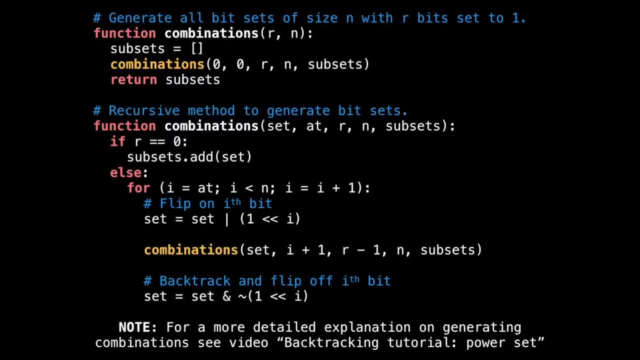 for what it does. What the first combinations method does is it fills up the subsets array using the second combinations method and then it returns that result. So what does the second combinations method do? I already covered this in more detail in my tutorial: backtracking the power set, if you want more detail, but I'll give you a quick rundown. 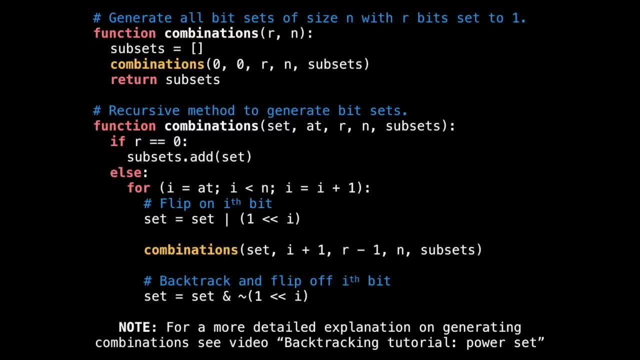 of what this recursive method does Basically, starting with the empty set, which is zero, you want to set our out of n bits to be one for all possible combinations, So you keep track of which index position you're currently at And then try and set the bit position to a one and keep moving forward, hoping that at 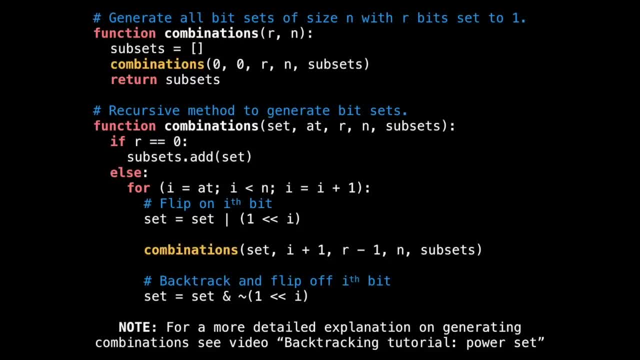 the end you have exactly our bits, But if you didn't, you backtrack, flip off the bit you flipped on and then move to the next position. This is a classic backtracking problem. you might want to research. This is how you solve it, But I don't want to focus on this in this. 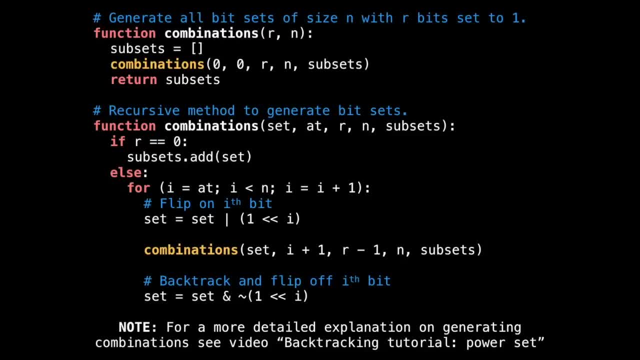 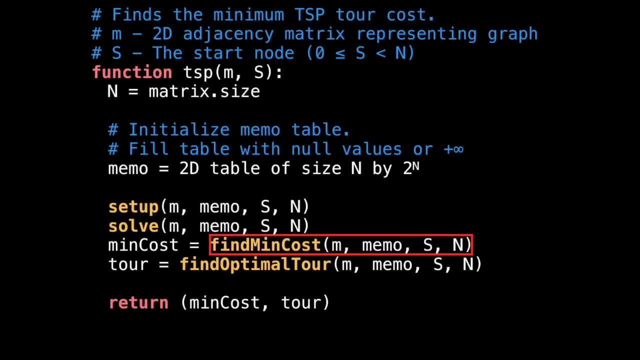 video per se. So I want to get back to the traveling salesman problem. Watch my backtracking video on the power set for more guidance. If you're lost, I'll try and remember to put a link in description. So right now in our memo table, we have optimal value for each partial tour with and nose. 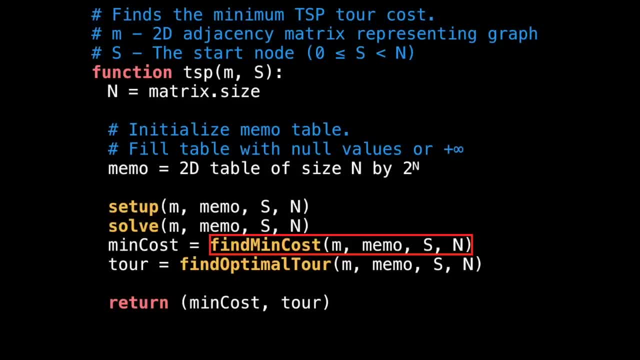 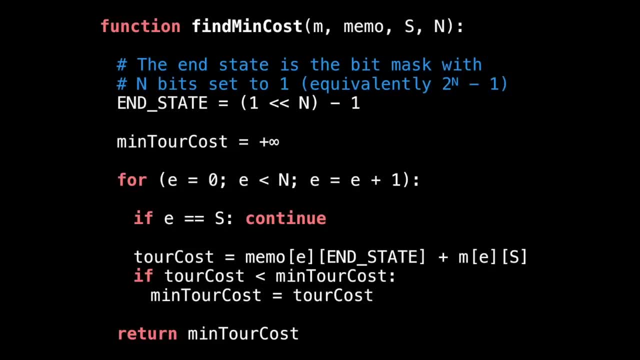 So let's see how we can reuse that information to find the minimum Torah value. The true trick is going to be to construct a bit mask for the end state and use that to do a lookup in our memo table. The end state is the bit mask with n bits set to one which we can obtain. 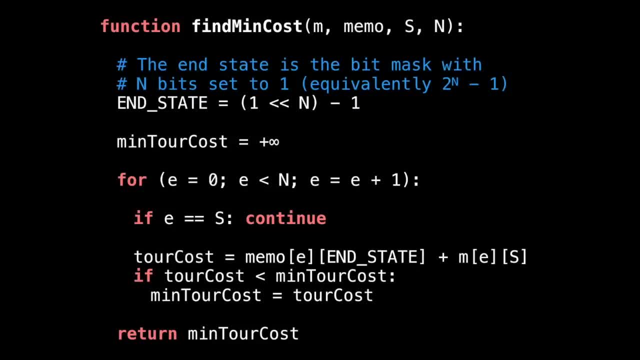 by doing a bit shift and then subtracting one. Then what we do is look at each end node candidate and minimize over the tour costs by looking at what's in our memo table and the distance From the end node back to the start node s. The last method we need to look at is the 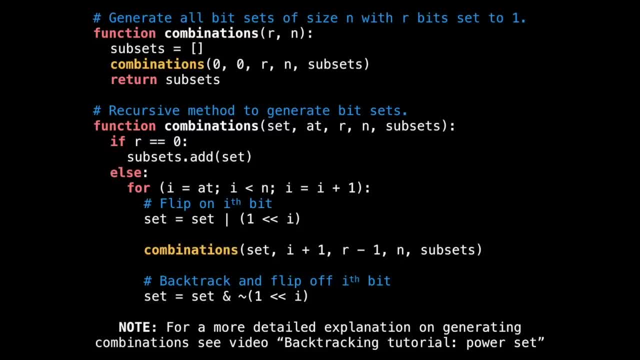 recursive method does. Basically, starting with the empty set, which is zero, you want to set our out of n bits to be one for all possible combinations. So you keep track of which index position you're currently at And then try and set the bit position to a one and keep moving forward, hoping that at 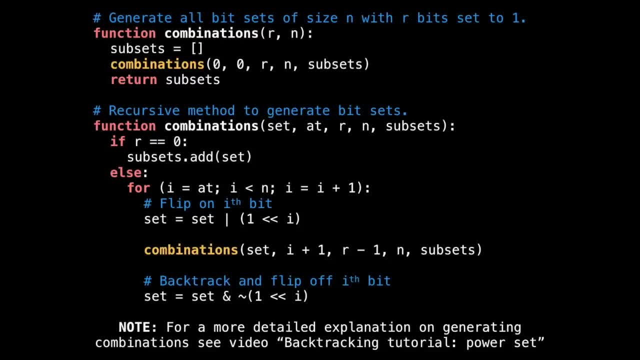 the end you have exactly our bits, But if you didn't, you backtrack, flip off the bit you flipped on and then move to the next position. This is a classic backtracking problem. you might want to research. This is how you solve it, But I don't want to focus on this in this. 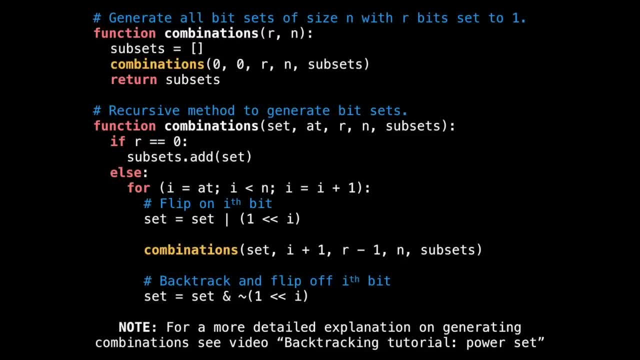 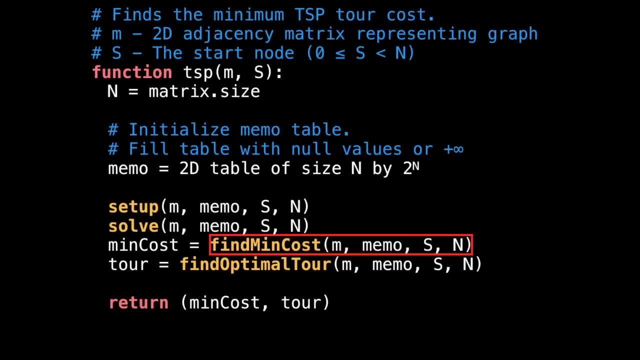 video per se. So I want to get back to the traveling salesman problem. Watch my backtracking video on the power set for more guidance. If you're lost, I'll try and remember to put a link in the description. So right now in our memo table we have optimal value for each partial tour with and nose. 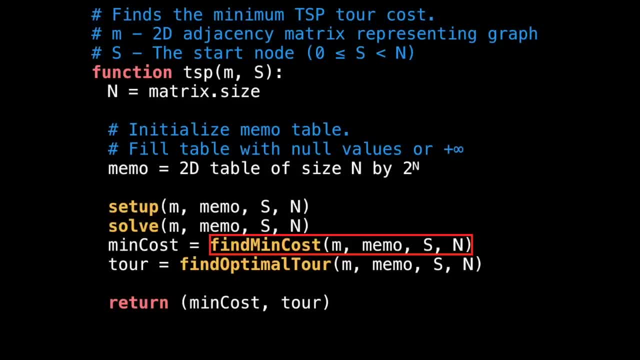 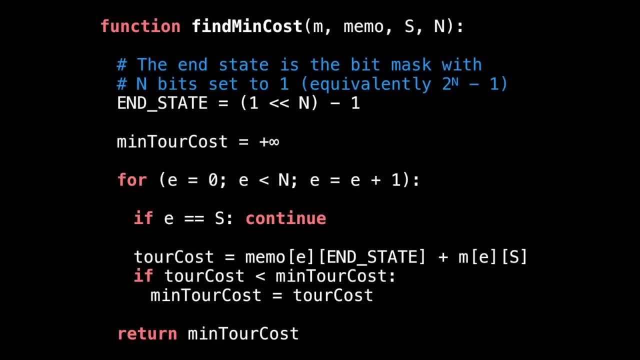 So let's see how we can reuse that information to find the minimum tour value. The trick is going to be to construct a bit mask for the end state and use that to do a lookup in our memo table. The end state is the bit mask with n bits set to one, which 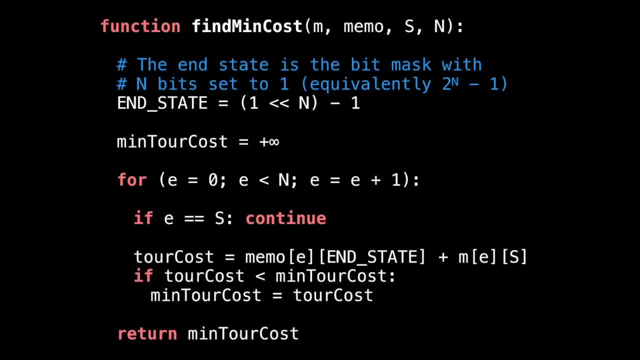 we can obtain by doing a bit shift and then subtracting one. Then what we do is look at each end node candidate and minimize over the tour cost by looking at what's in our memo table. So we're going to take the distance from the end node back to the start node s, The last. 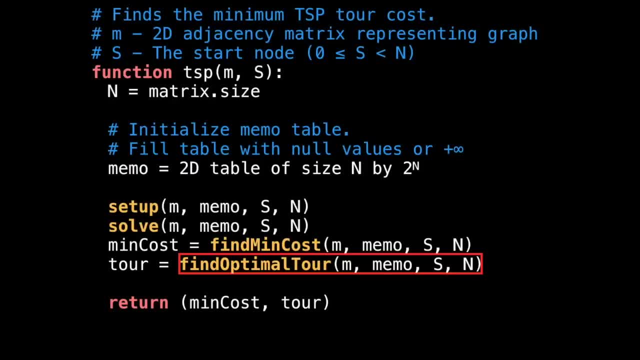 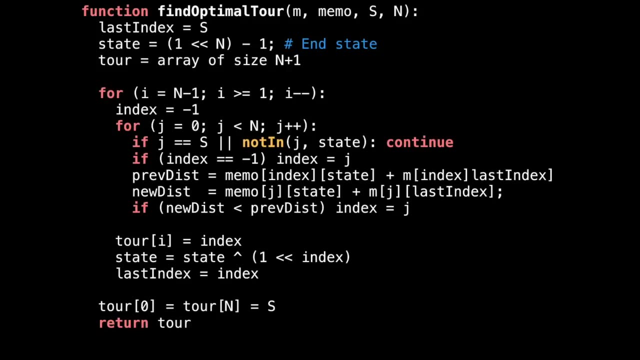 method we need to look at is the find optimal tour function, because what good is our algorithm if it cannot actually find you what the optimal tour is For this method? what we're going to do to find the actual tour is work backwards from the end state and do lookups in our memo. 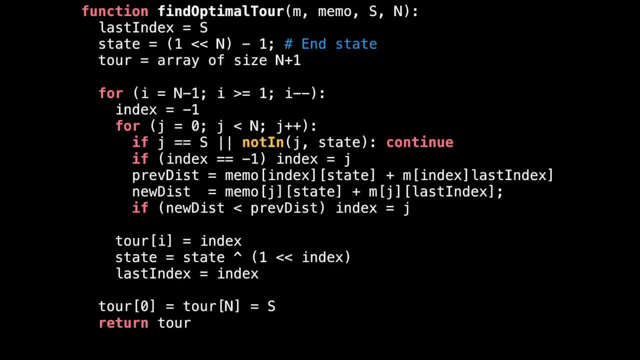 table to find the next optimal node. We will keep track of the last index we were at and the current state, which begins with all visited nodes. Then we loop over I from n minus one to one, which tracks the index position for the tour, To actually find the next optimal node. going backwards we're going. 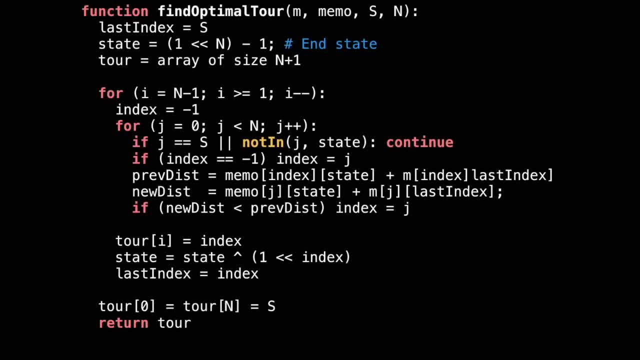 to use a variable called index, which will track the best node. The inner loop loops j, which represents all possible candidates for the next node. we must ensure that j is not the starting node and that it is part of the state, meaning it has not yet been visited. 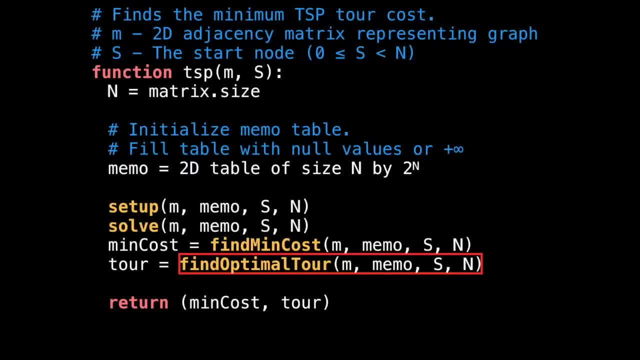 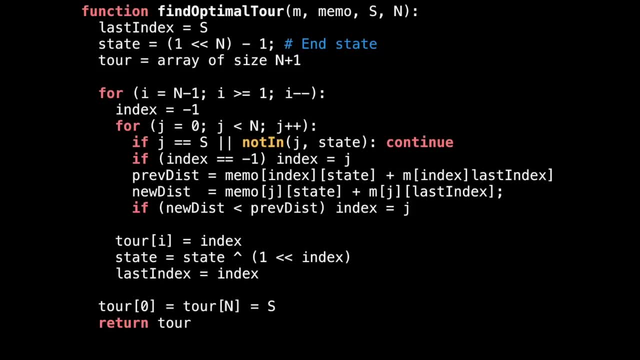 find optimal tour function, because what good is our algorithm if it cannot actually find you what the optimal tour is For this method? what we're going to do to find the actual tour is work backwards from the end state and do lookups in our memo table to find the 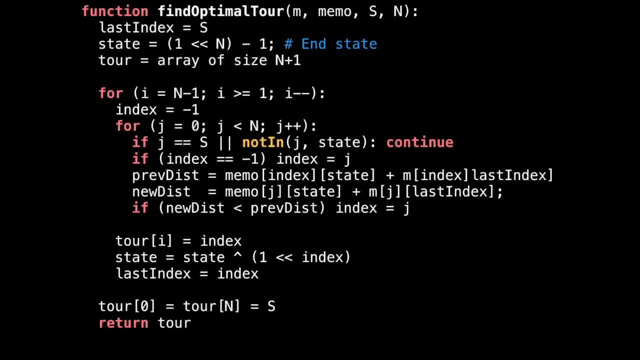 next optimal node. We will keep track of the last index we were at and the current state which begins with all visited nodes. Then we loop over I from n minus one to one which tracks the index position for the tour, To actually find the next optimal node. going backwards we're going. 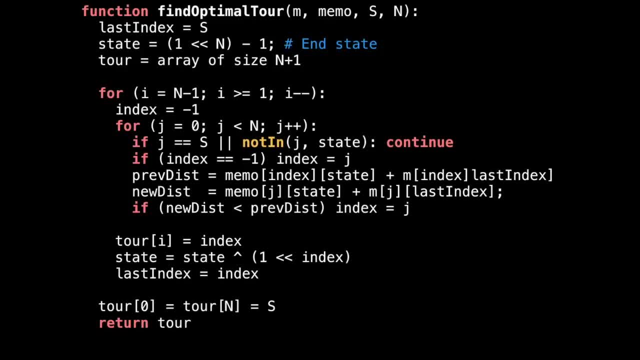 to use a variable called index, which will track the best node. The inner loop loops over j, which represents all possible candidates for the next node. we must ensure that j is not the starting node, that it is part of the state, meaning it has not yet been visited. 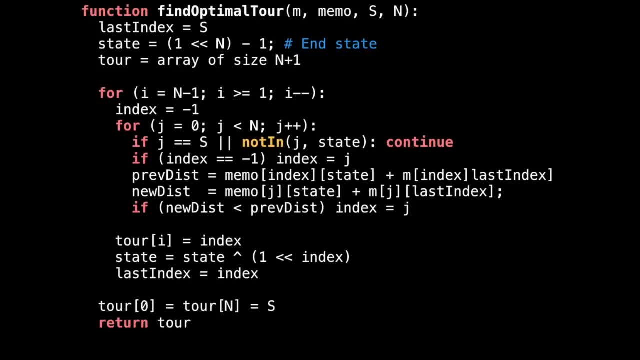 If this is the first valid iteration, the variable index will be set to minus one. So set it to j. Otherwise, compare the optimal values of the best distances between nodes: index and j. Otherwise, compare the optimal values of the best distances between nodes. 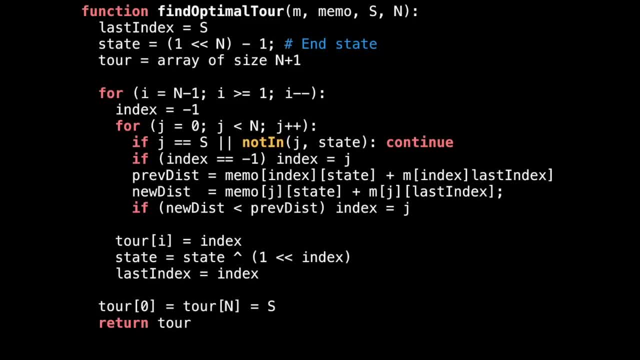 index and j and update index. if node j is better, Once the optimal index is found, store that as part of the tour and flip off the bit in the state which represents the index node. Finally, set the first and last nodes of the tour to be s the starting node. 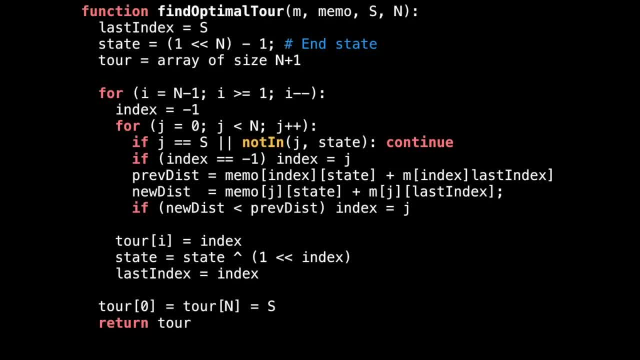 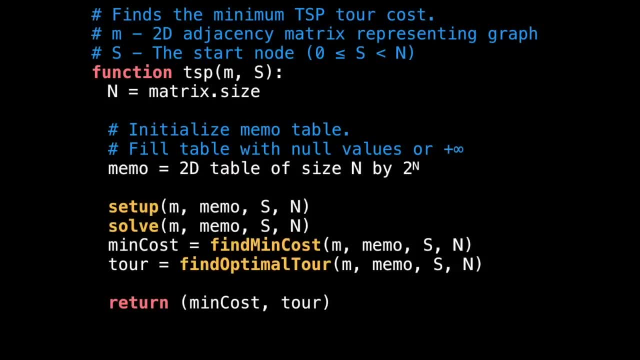 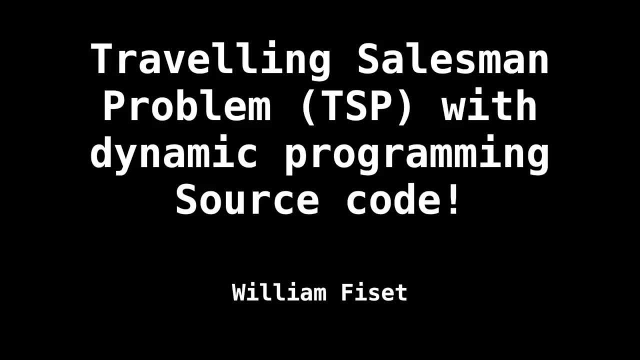 because the tour needs to start and end on that node. then simply return the tour And that is how you solve the traveling salesman problem with dynamic programming. Hello and welcome to this video on the traveling salesman problem with dynamic programming. Today we're going. 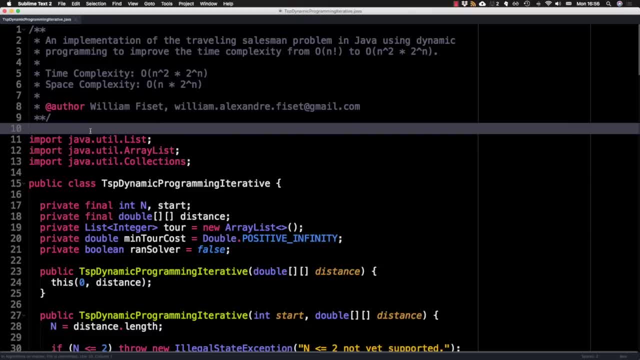 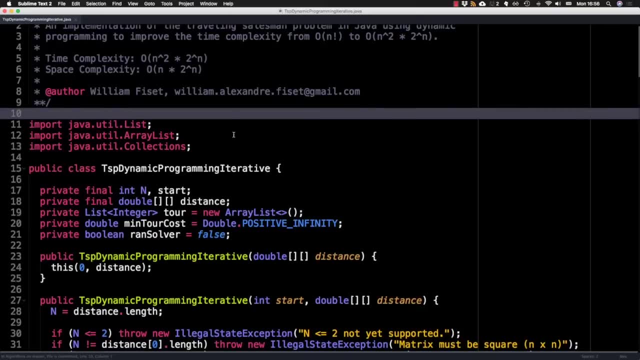 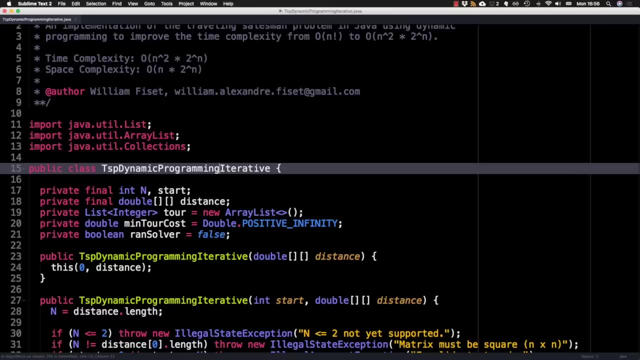 to have a look at some source code. All right, here we are in the source code for the traveling salesman problem with dynamic programming. This is the iterative implementation. If you look in the repository, you should see that there is also a recursive implementation. 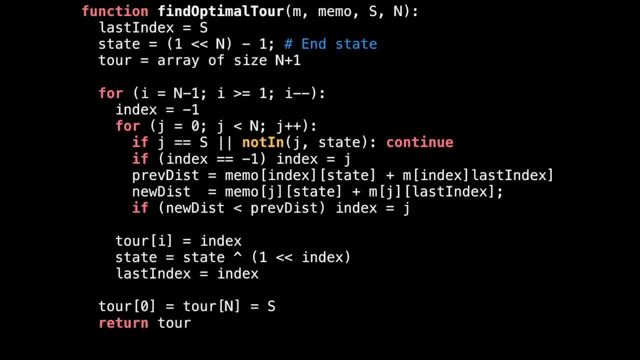 If this is the first valid iteration, the variable index will be set to minus one. So set it to j. Otherwise, compare the optimal values of the best distances between nodes index and j And update index if node j is better. Once the optimal index is found, store that as. 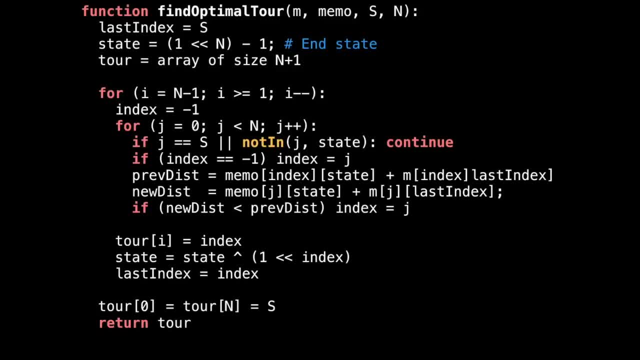 part of the tour and flip off the bit in the state which represents the index node. Finally, set the first and last nodes of the tour to be s the starting node, because the tour needs to start and end on that node. then simply return the tour, And that is how we're going. 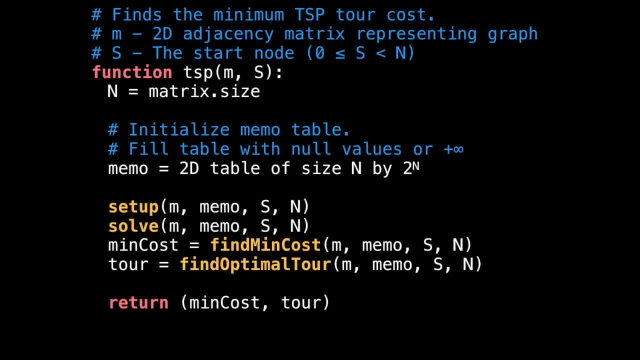 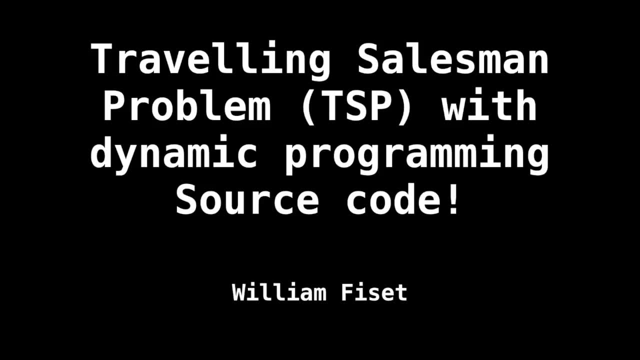 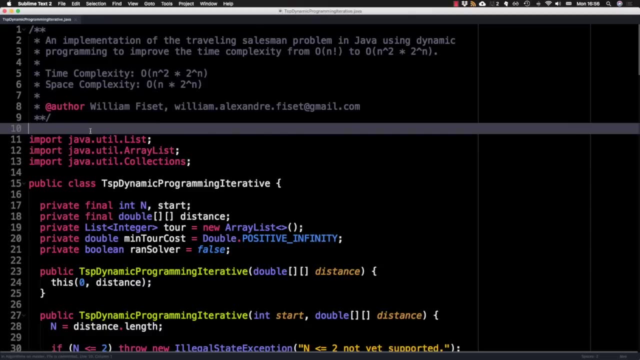 to solve the traveling salesman problem with dynamic programming. Hello and welcome to this video on the traveling salesman problem with dynamic programming. Today we're going to have a look at some source code. All right, here we are in the source code for the traveling. 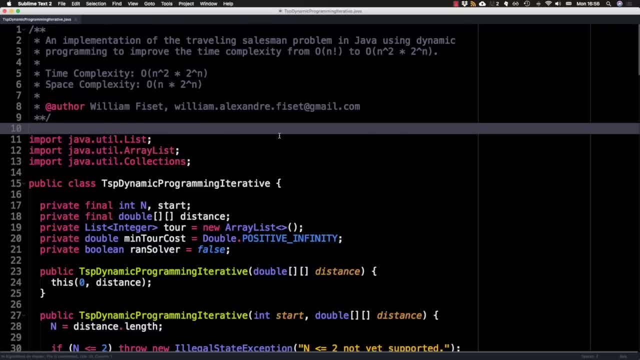 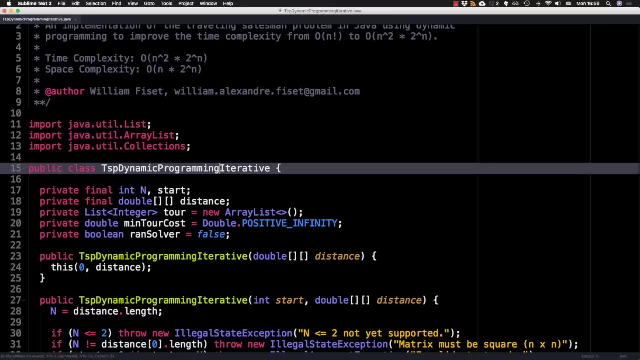 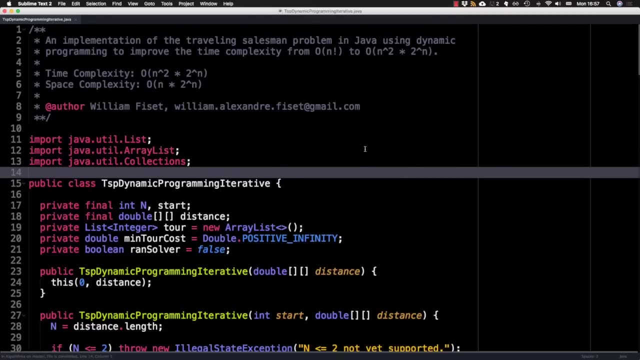 salesman problem with dynamic programming. This is the iterative implementation. If you look in the repository, you should see that there is also a recursive implementation, If you are interested in that. this implementation is in the Java programming language, but you should be able to translate it pretty easily to any programming language. So let's get. 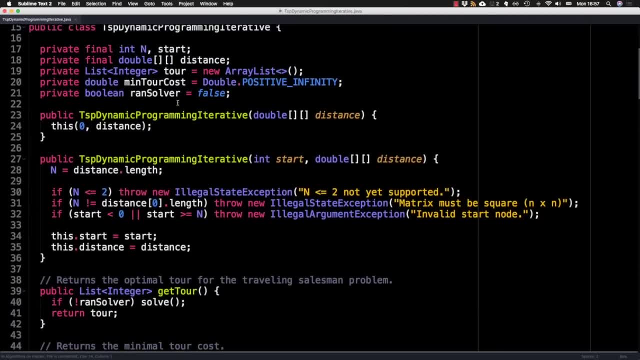 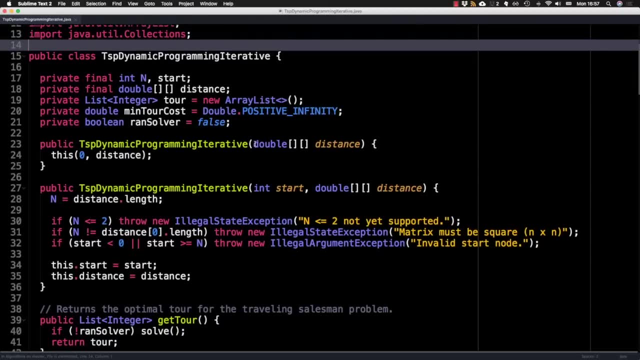 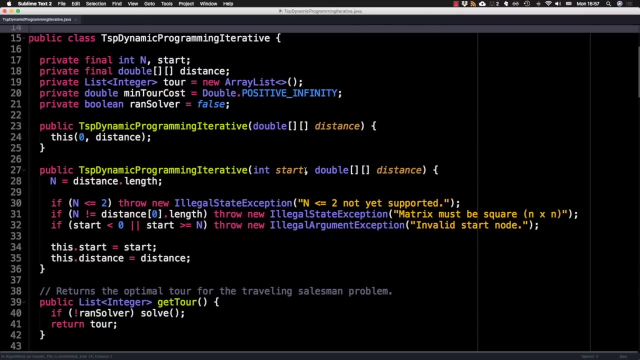 started. So if we want to solve this problem, we're going to have to create this object called TSP, dynamic programming iterative, And it has two constructors, one with a distance matrix as an input And the other optional constructor is the distance matrix, but also with a designated starting. 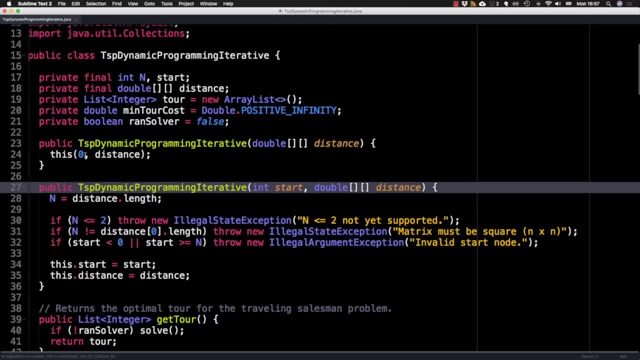 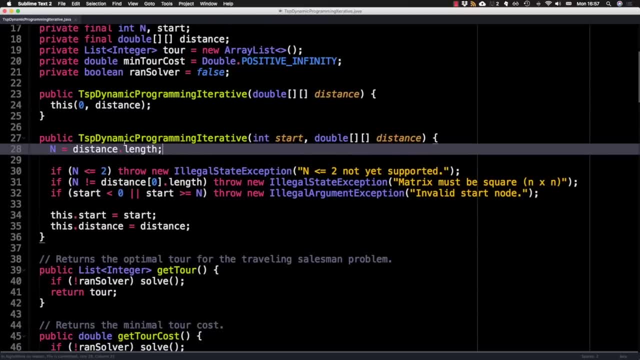 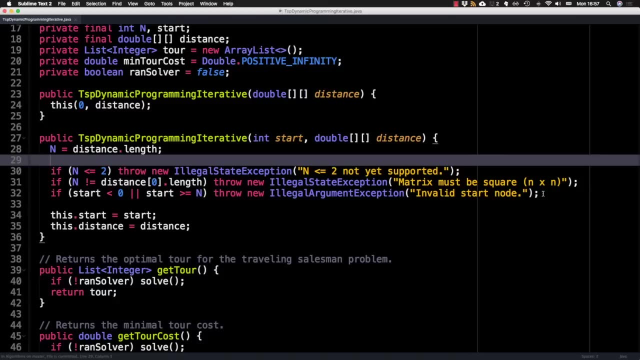 node. So by default I have the starting node to be zero, but you can set that to be whichever node you like, And then I simply store how many nodes are in the graph And then check for some edge cases. I haven't supported n equals. 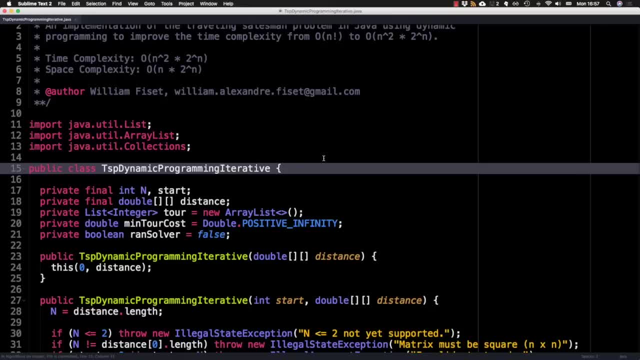 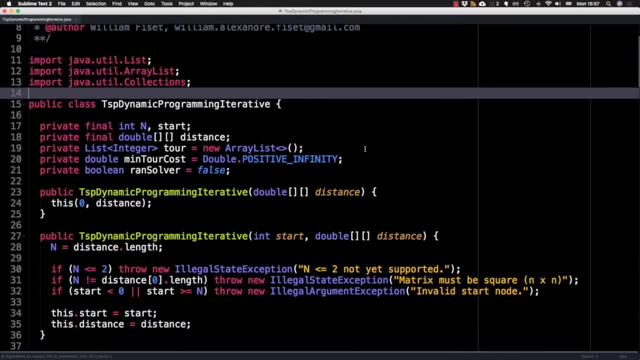 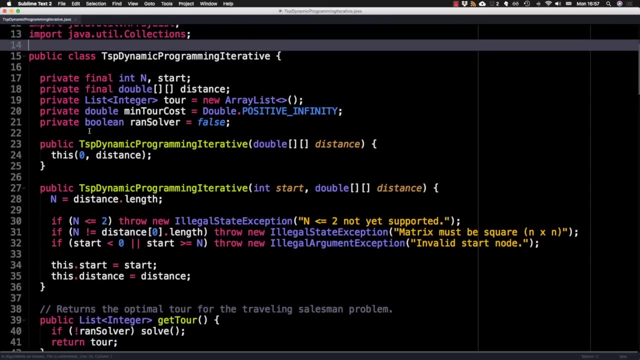 If you are interested in that. This implementation is in the Java programming language, but you should be able to translate it pretty easily to any programming language, So let's get started. So if we want to solve this problem, we're going to have to create this object. 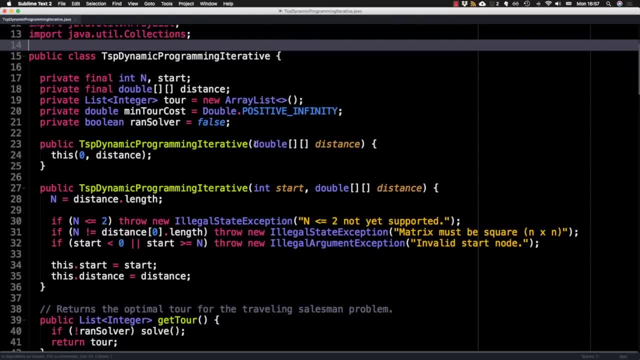 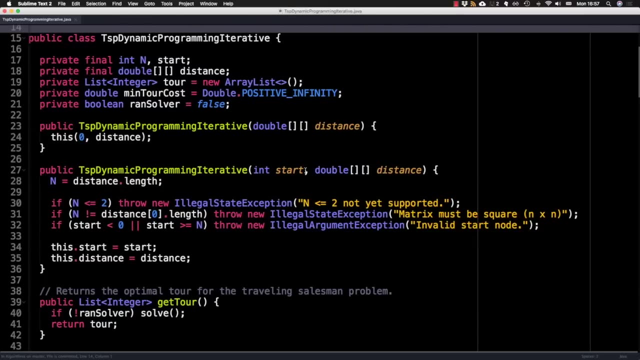 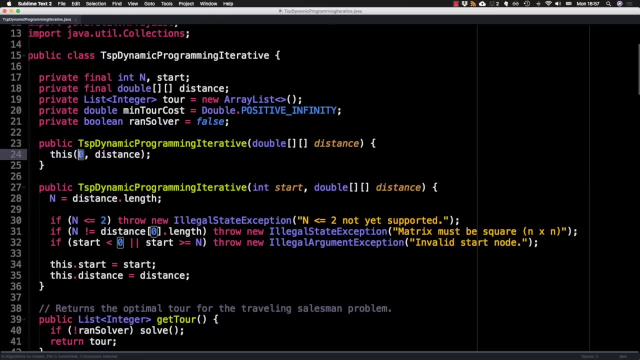 called TSP dynamic programming iterative, And it has two constructors: one with a distance matrix as an input And the other optional constructor is the distance matrix but also with a designated starting node. So by default I have the starting node to be zero, but you can set that to be whichever. 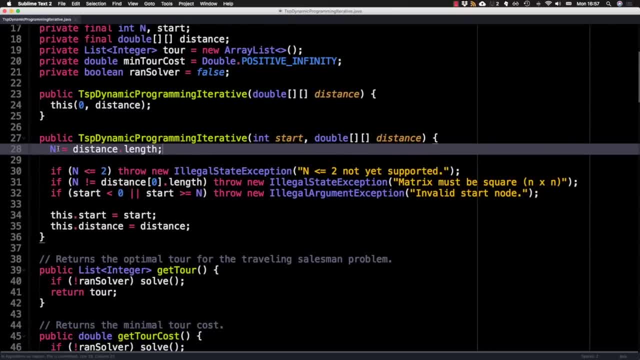 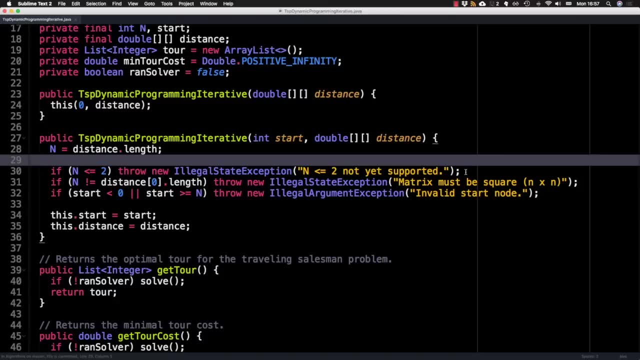 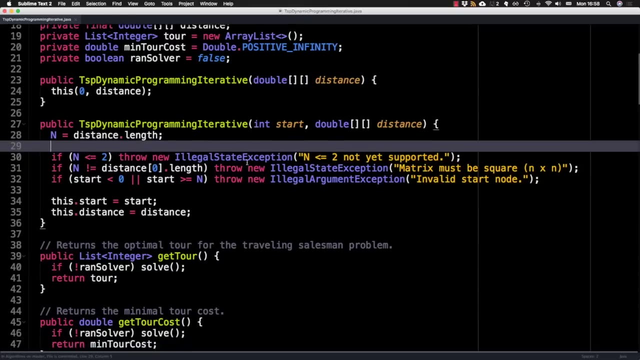 node you like, And then I simply store how many nodes are in the graph and then check for some edge cases. I haven't supported an equal n equals two yet, but that should be pretty trivial to do And then just check for some. 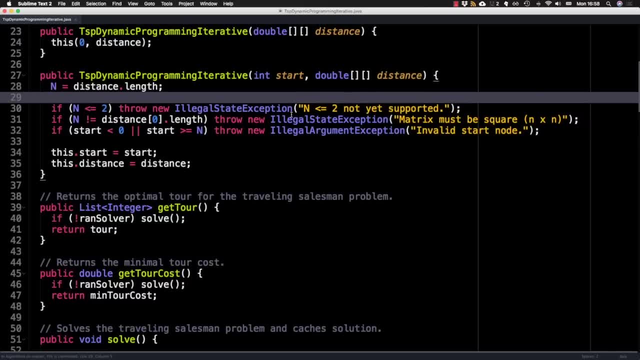 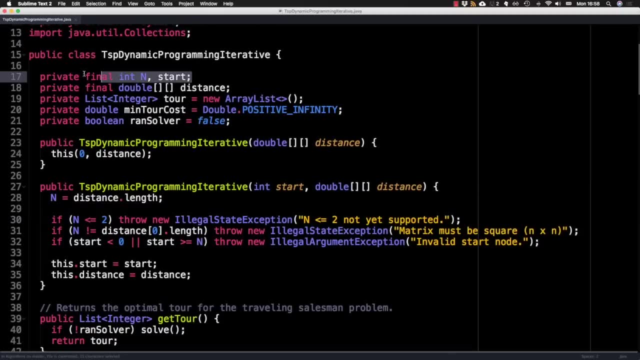 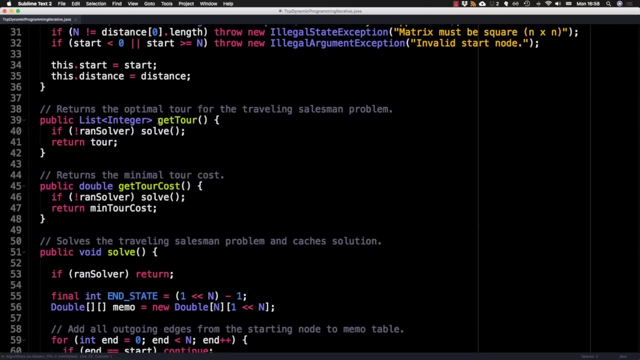 edge cases, make sure the matrix is square, you know just that kind of stuff. And then I cache the start position and the distance, in these instance variables. And then here are the two methods that you will be interested in: the first called get tour And it returns. 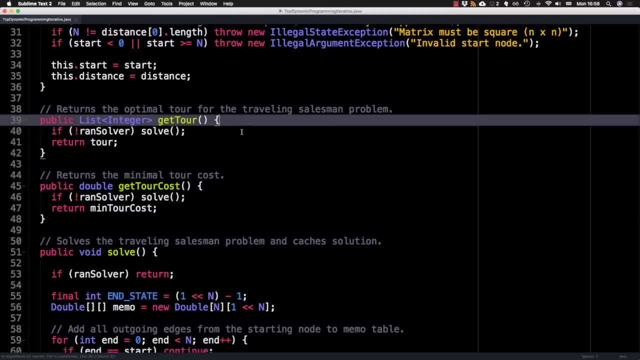 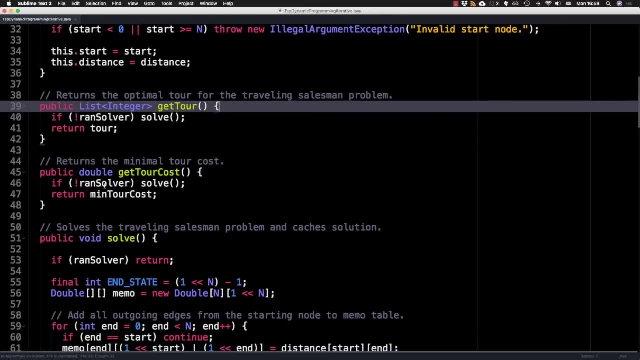 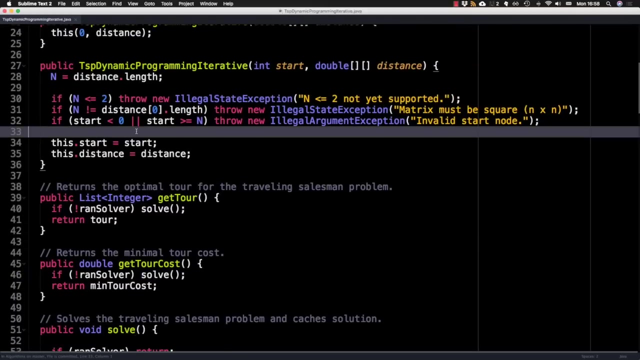 a list of integers use representing the optimal tour for the input graph. And this other method, called get tour cost, returns the minimum tour cost. And notice that they both call the solve method. if the solver has not been a run yet, I could call the solve method in the constructor. 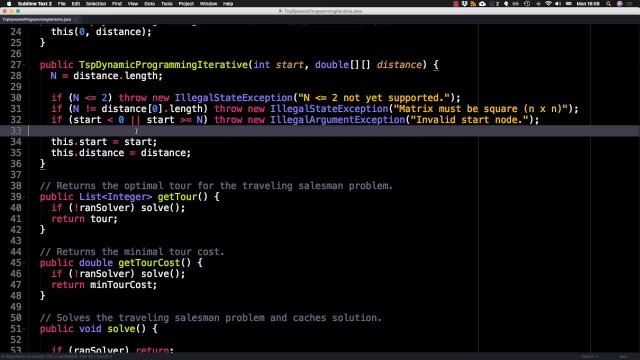 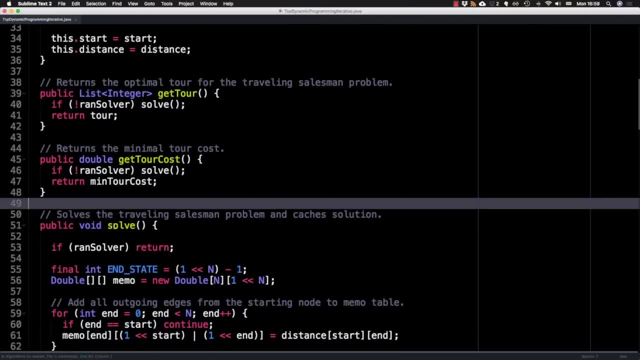 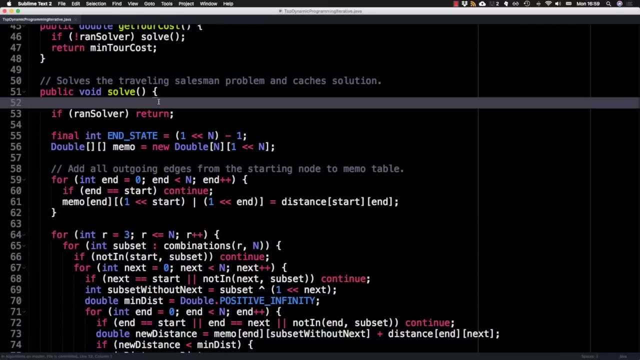 but that's generally considered bad practice to do work in the constructor. So I leave it up to the methods to call the solve method, Or you can explicitly call it yourself, doesn't matter. So the solve method is what basically solves the child and salesman person problem. 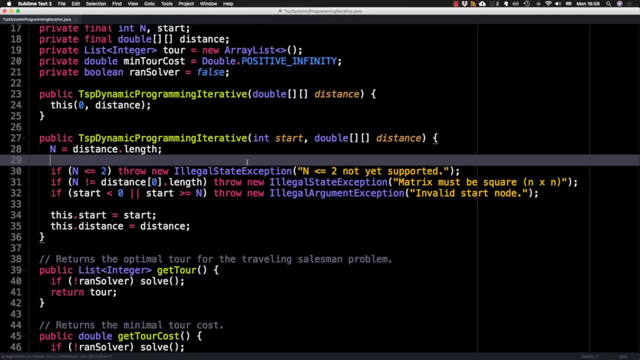 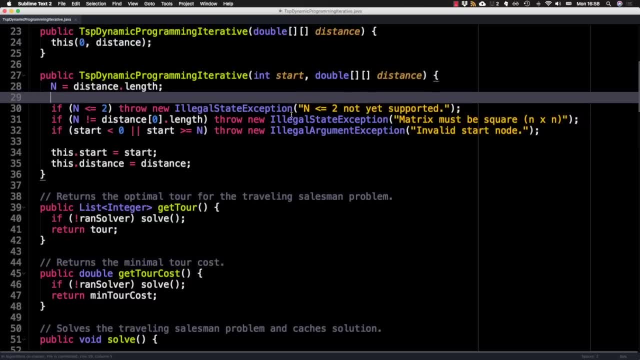 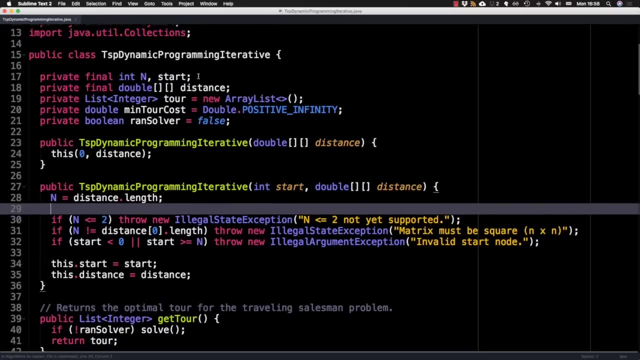 two yet, but that should be pretty trivial to do, And then just check for some edge cases, make sure the matrix is square, you know just that kind of stuff, And then I cash the start position and the distance- in these instance variables- And then here are the two methods. 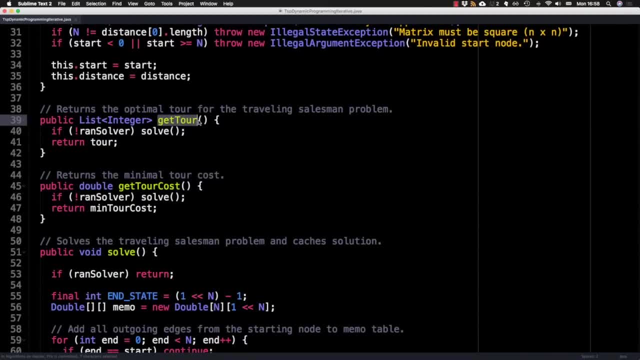 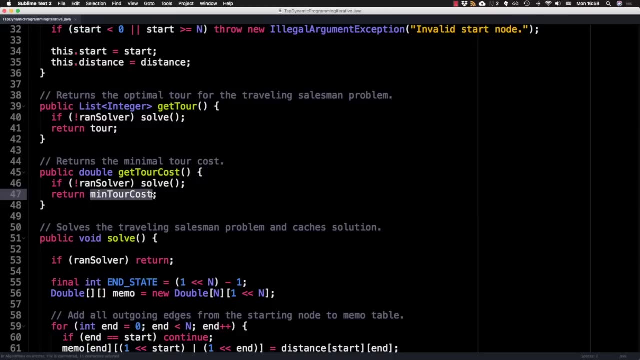 that you will be interested in. the first called get tour, And it returns a list of integers representing the optimal tour for the input graph. And this other method, called get tour costs, returns the minimum tour cost And notice that they both call the solve method. 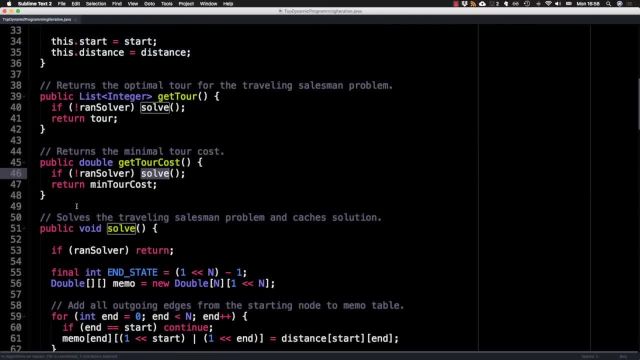 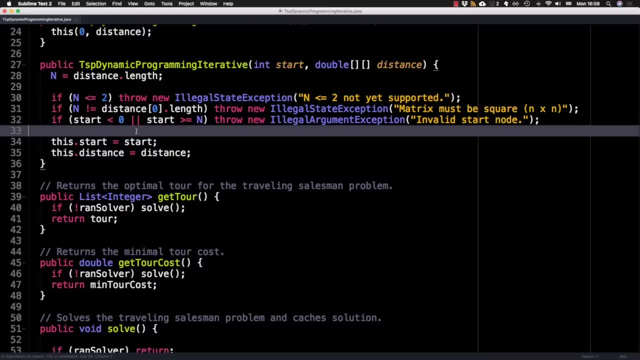 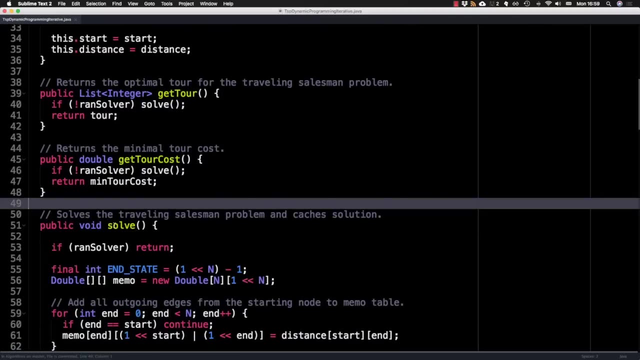 if the solver has not been a run yet, I could call the solve method in the constructor, but that's generally considered bad practice to do work in the constructor, So I leave it up to the methods to call the solve method, Or you can explicitly call it yourself, doesn't? 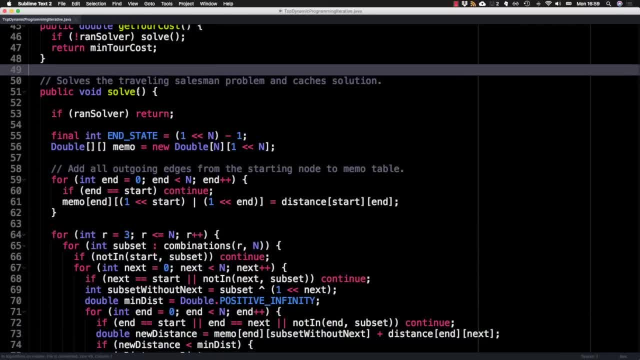 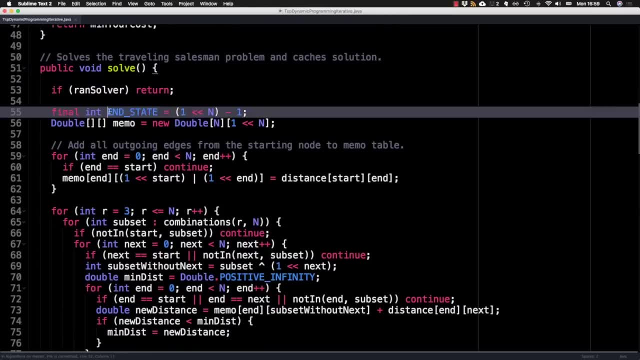 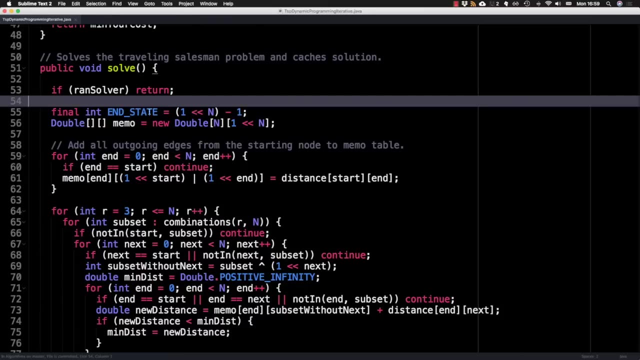 matter. So the solve method is what basically solves the traveling salesman person problem. So the first thing I do is I initialize a variable called the end state, And this is the state with all nodes visited, So all bits are set to one. then I initialize a memo table of 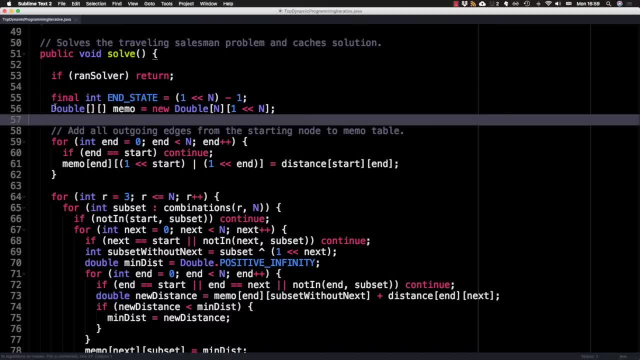 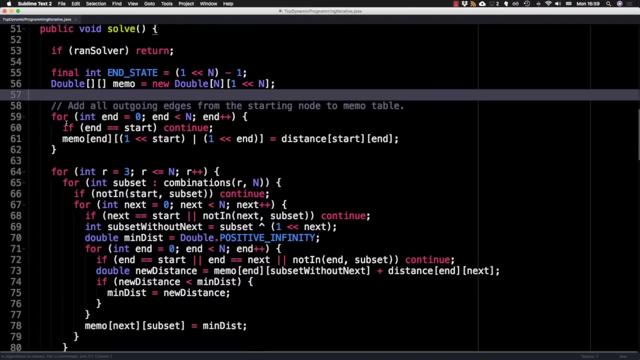 size n times to the end And it takes type double. So initially this entire table is filled with null values And then I do an initialization step where I add all edges from the starting node to every other node which is not start node. So this is like the first step in the 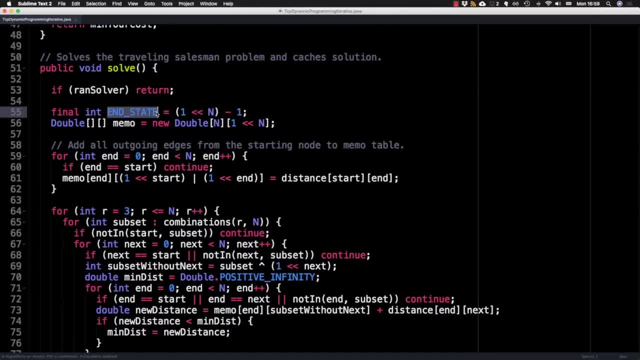 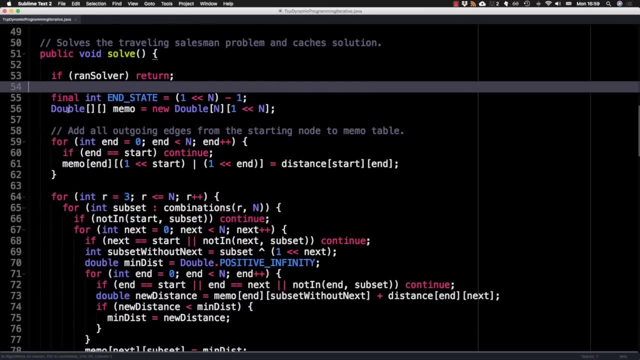 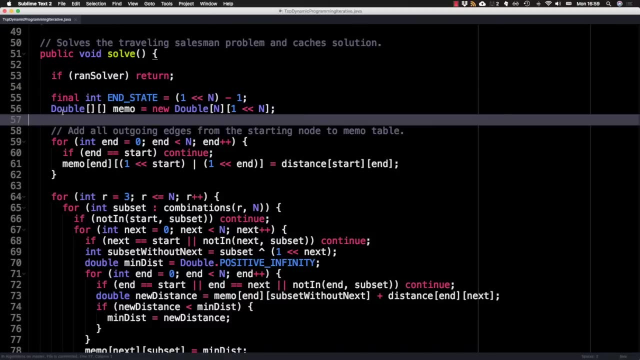 So the first thing I do is I initialize a variable called the end state, And this is the state with all nodes visited, So all bits are set to one. then I initialize a memo table of size n times 10.. To the end, and it takes type double. So initially this entire table is filled with. 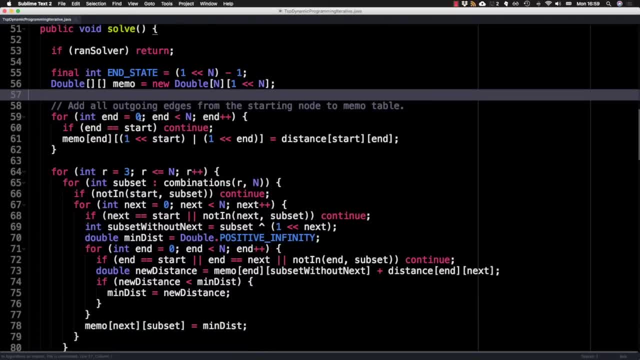 null values. And then I do an initialization step where I add all edges from the starting node to every other node which is not start node. So this is like the first step in the slides, if you remember correctly, and then you set it equal. 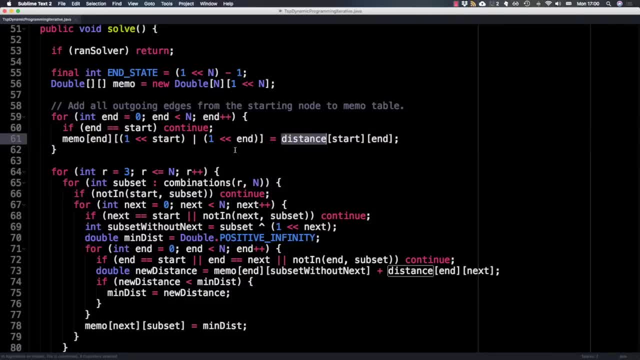 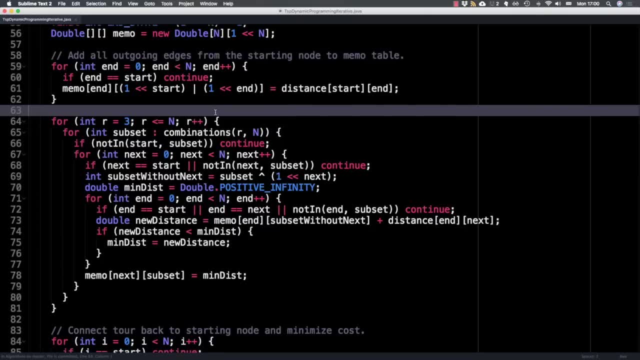 To the value in the adjacency matrix. Then we start the phase where we're trying to create tours of path that are one longer, So our is once again the number of nodes in the partially completed tour. Then we loop through all subsets with our bits set to null And 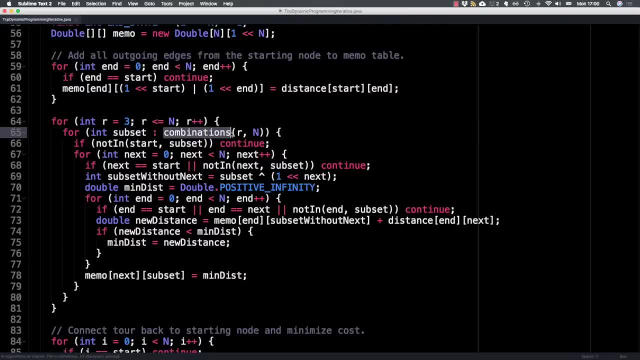 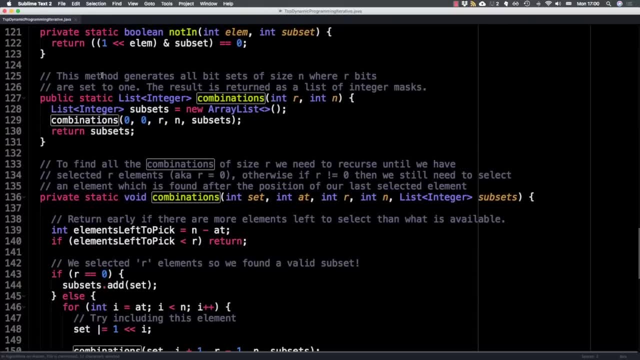 then we have our set produced from our combinations function, which is below- I guess I'll jump to that right now. So that's right here- And this method basically generates all the bit sets of size and where our bits are set to one, And then you can see that the result. 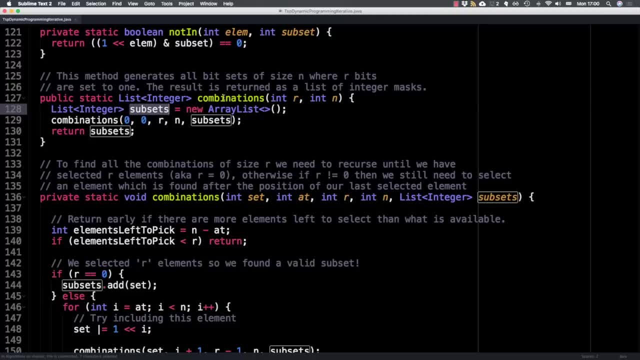 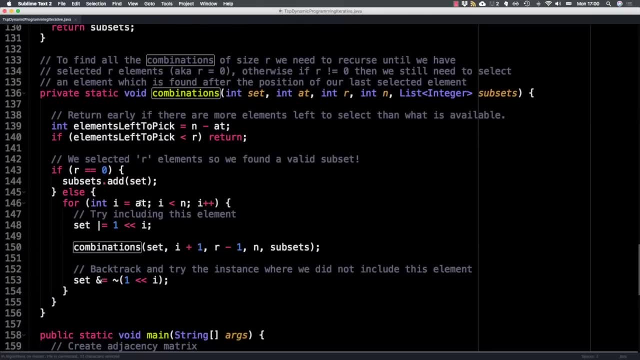 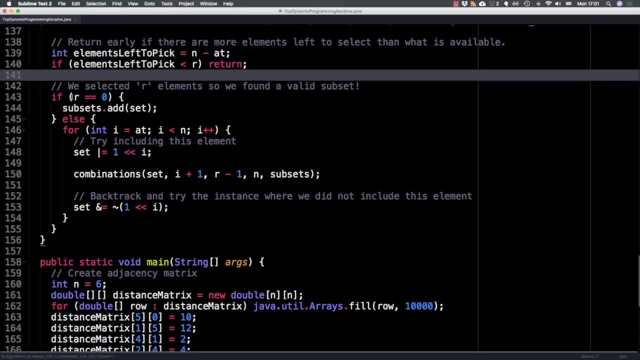 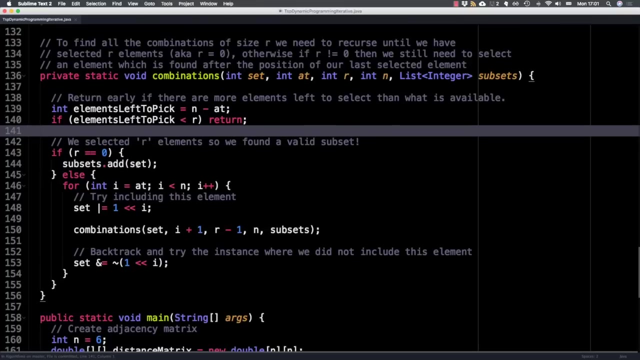 is returned in this variable called subsets. So this is the combinations method And then this calls the private combinations method down here. So ignoring this part, which is just an optimization, if r is zero, meaning we've selected exactly our elements, then we find found a valid subset and then add. 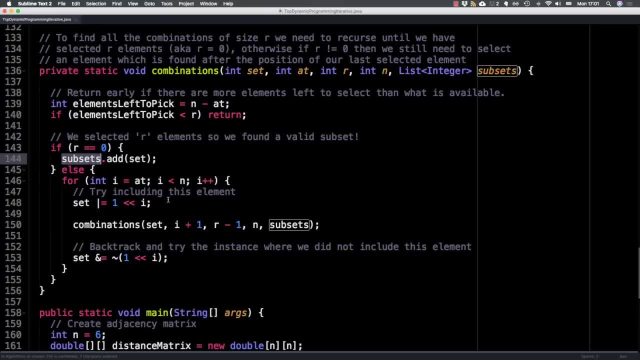 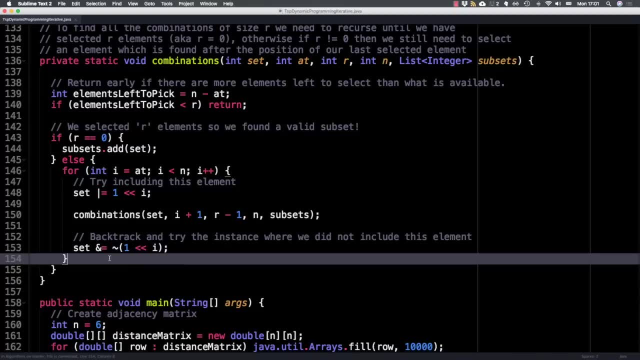 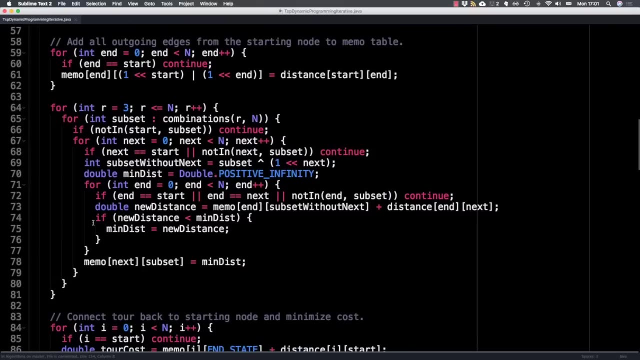 it to our subsets array, Otherwise we flip on the ith bit recursively, call the method and then backtrack and flip off the ith bit. All right, So going back over here Now, we make sure that the starting node is inside the subset. 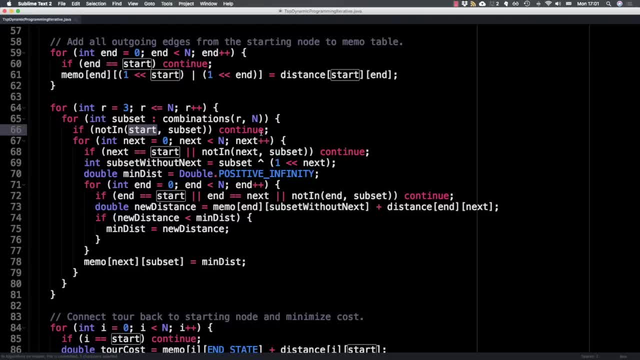 Otherwise we're not going to be able to create a valid tour Next. Next, we loop over the variable called next, from zero to n And the next node is going to be our next like target node, the one we're trying to do. 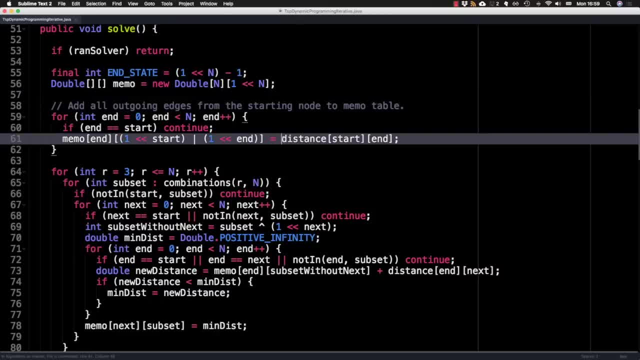 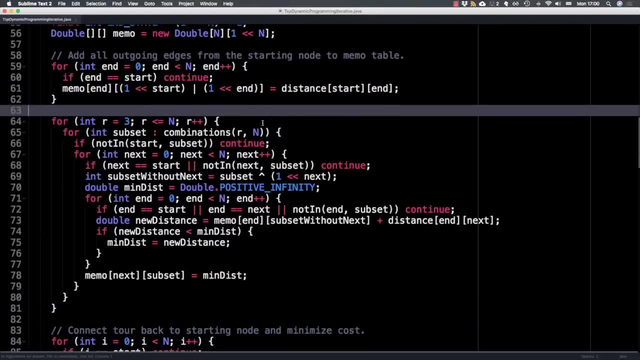 slides, if you remember correctly, and then you set it E equal to the value and the adjacency matrix, Then we start the phase where we're trying to create tours of path that are one longer. So our is once again the number of nodes. 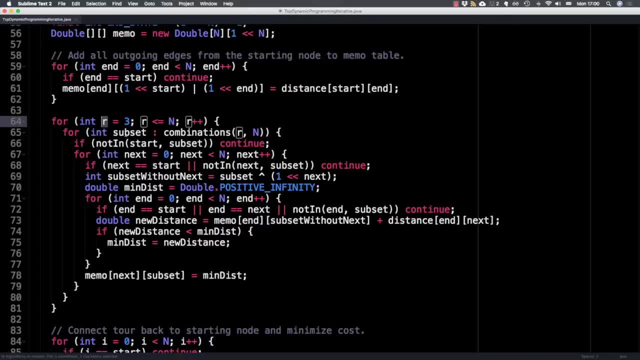 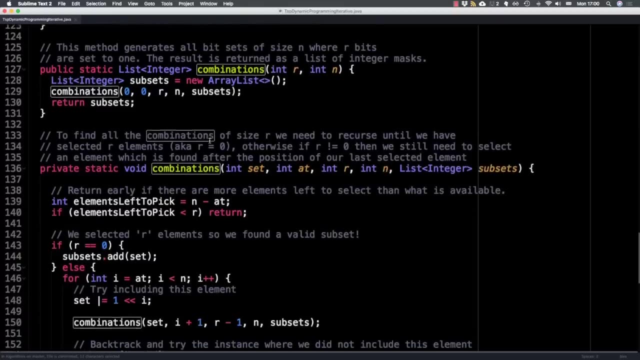 in the partially completed tour. Then we loop through all subsets with our bits set to one set produced from our combinations function, which is below- I guess I'll jump to that right now. So that's right here- And this method basically generates all the bit sets. 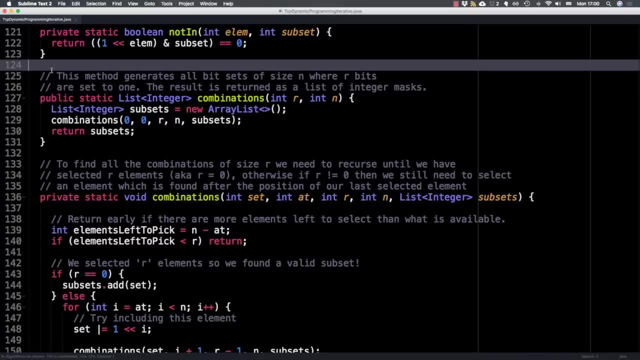 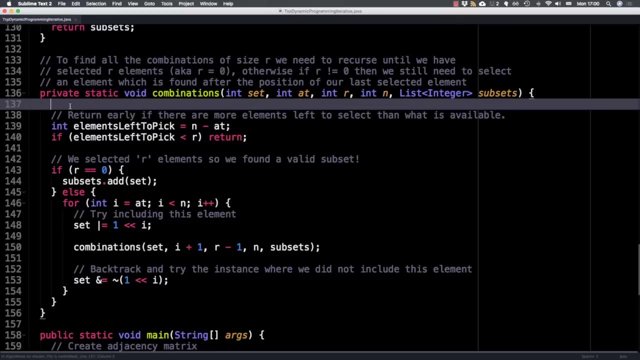 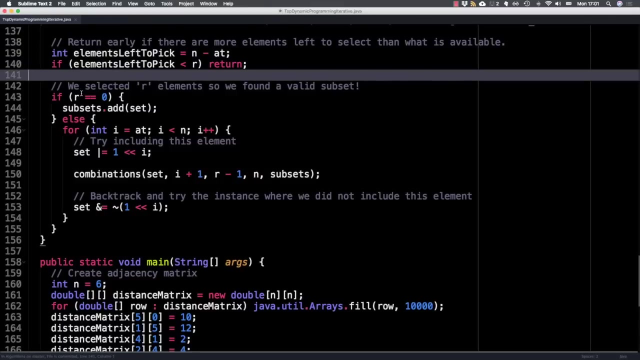 of size and where our bits are set to one, And then you can see that the result is returned in this variable called subsets. So this is the combinations method, And then this calls the private combinations method method down here. So ignoring this part, which is just an optimization, if r is zero, 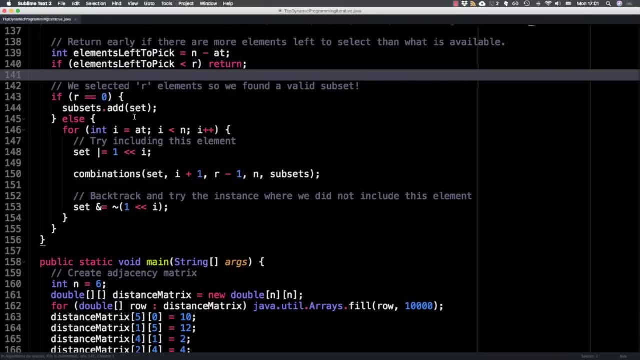 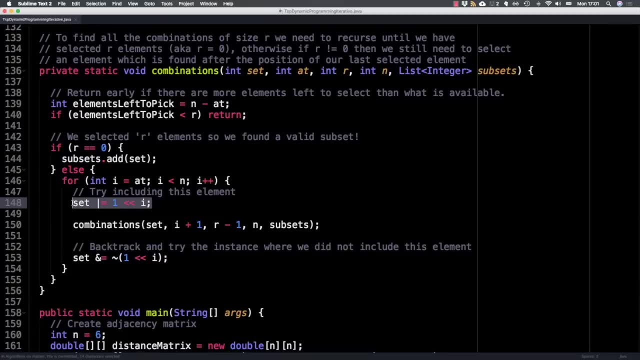 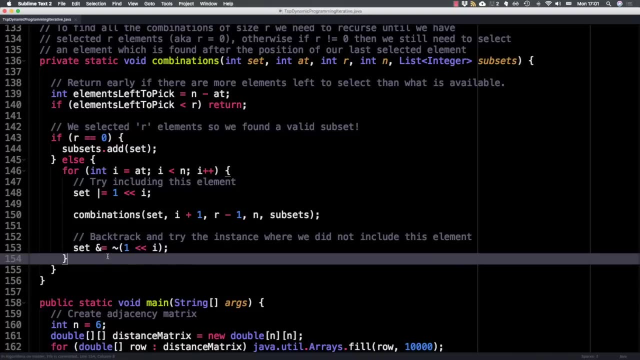 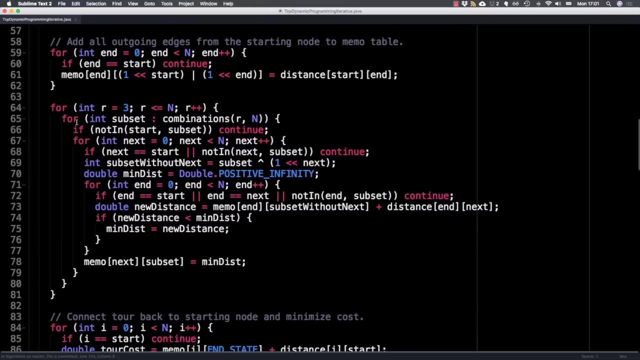 meaning we've selected exactly our elements. then we find, found a valid subset and then add it to our subsets array. Otherwise we flip on the ith bit recursively, call the method and then backtrack and flip off the ith bit. All right, So going back over here, Now we make sure that the starting node is inside. 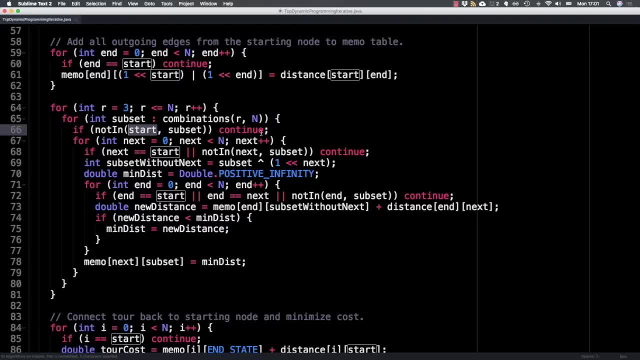 the subset, Otherwise we're not going to be able to create a valid tour Next. next we loop over the variable called next, from zero to n, And the next node is going to be our next like target node. the one we're talking about is going to be our next target node. 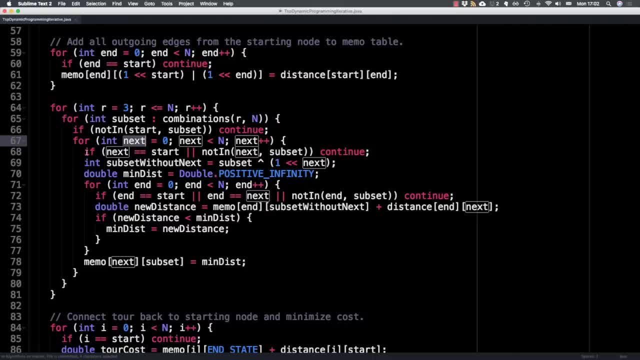 We're trying to expand to, if you will. So we make sure that the next node is not the starting node And we also make sure that it is in the subset produced by the combinations function, Otherwise we're not interested in in it. Then we generate the mask, which 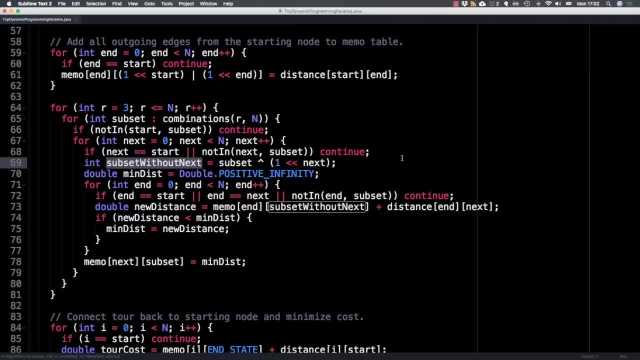 is called subset without next, And this is the, the state or the the partially completed tour without that next node. So we basically flip off the next node and set it to zero, And this allows us to do a lookup in our memo table later on So we can compute the new. 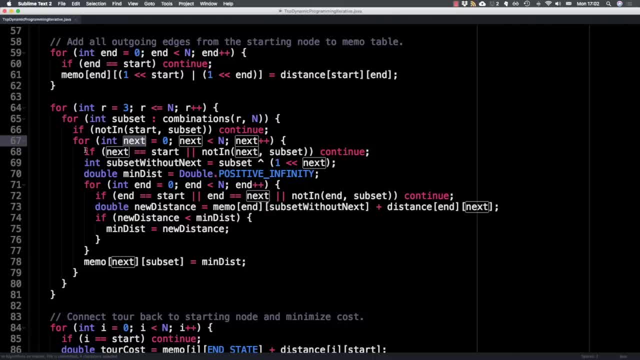 To expand to, if you will. So we make sure that the next node is not the starting node And we also make sure that it is in the subset produced by the combinations function, Otherwise we're not interested in it. Then we generate the mask, which is called subset, without next, And this is the the state. 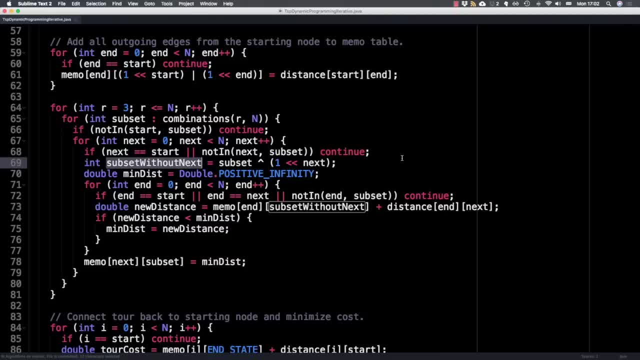 or the partially completed tour without that next node. So we basically flip off the next node and set it to zero, And this allows us to do a lookup in our memo table later on So we can compute the new distance. But before that, 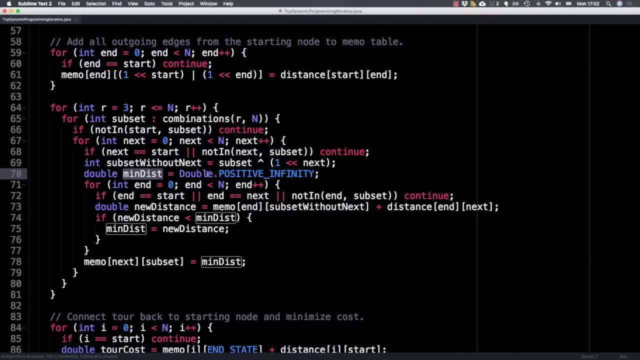 we initialize a variable called min distance, which I initialize the positive infinity, And this is the variable we're trying to compute And this is going to minimize for the next note, then for every possible end node, every possible end node which is not the start node or the end node and is part of our subset. 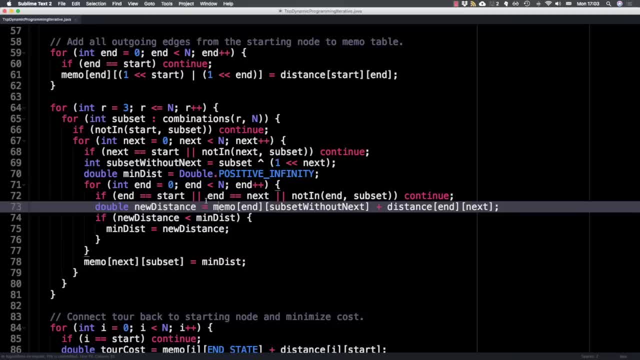 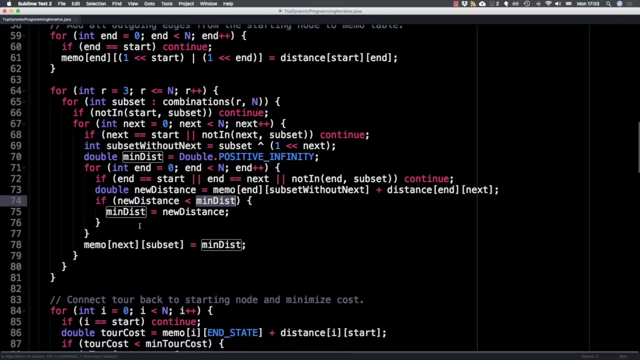 we calculate the new distance from the end node using the subset, without next, And then from the end node to the next node, And then if that new distance is less than the global or, sorry, the just the min distance we declared up here, then just update the min distance and finally cache that in the 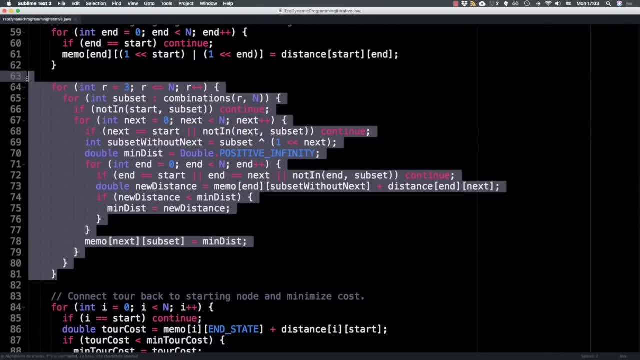 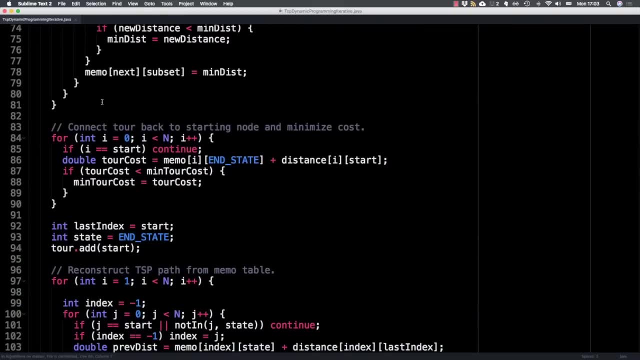 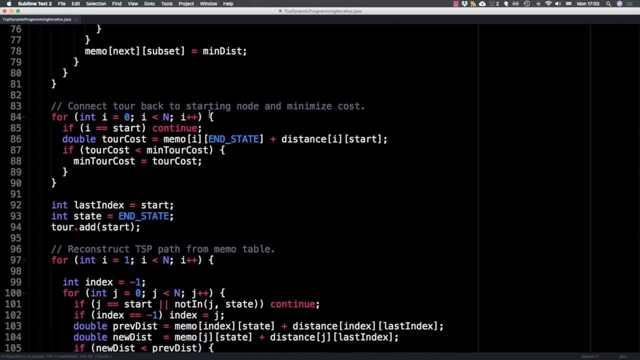 memo table. So this is the the bulk of the algorithm right here. But we're not done yet. we still want to calculate the minimum cost, like the overall minimum cost of the optimal tour, And to do that we simply loop from i zero to n, skip over the starting node and and. 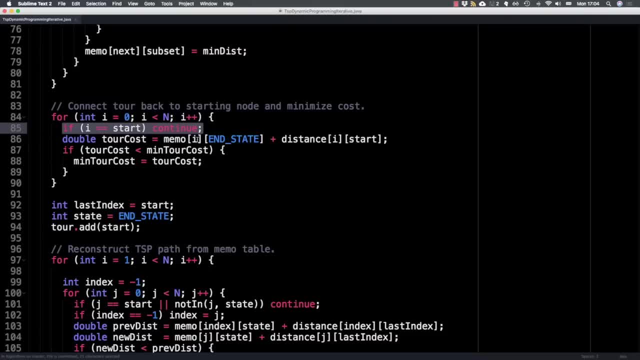 then do a lookup in our table for that end, node I and the state and state. So we finished a tour and the tour ended on node i and then go from i, which we ended on, back to the start node. So that's the tour cost. Now we just minimize over this variable and update the min tour. 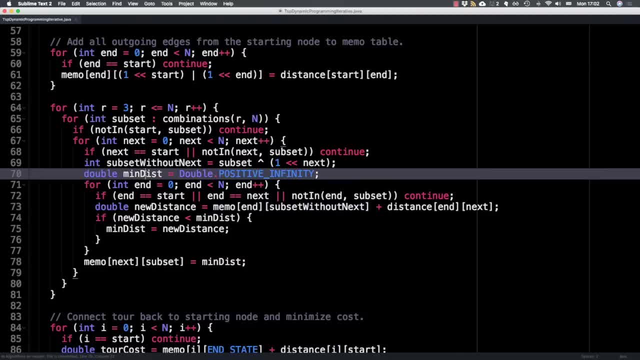 distance. But before that, we initialize a variable called min distance, which I initialized positive infinity, And this is the variable we're trying to min, minimize for the next note. Then, for every possible end node, every possible end node which is not the start node or the end node and is part of our subset, we calculate the. 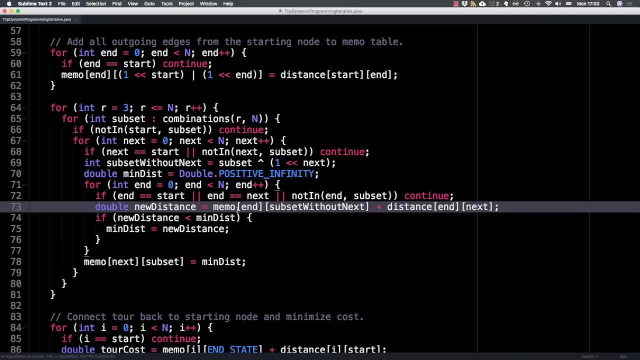 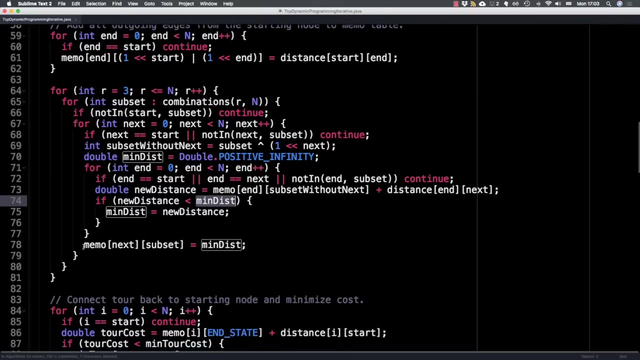 new distance from the end node using the subset, without next, and then from the end node to the next node, And then if that new distance is less than the global or, sorry, the just the min distance we declared up here, then just update the min distance and finally cache that in the memo table. 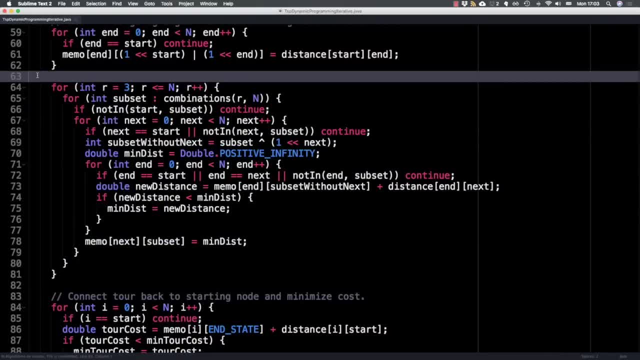 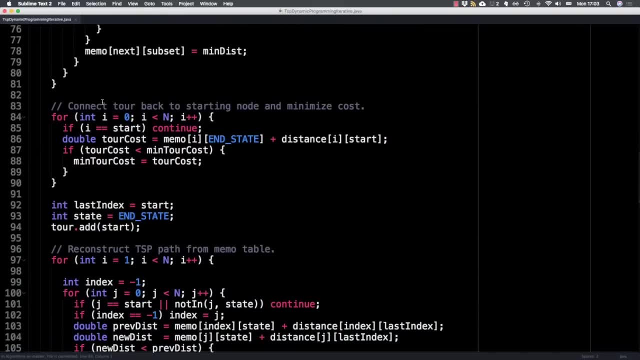 So this is the the bulk of the algorithm right here, But we're not done yet. we still want to calculate the minimum cost, like the overall minimum cost of the optimal tour, And this is what we're going to do. And to do that, we simply loop from i zero to n, skip over the 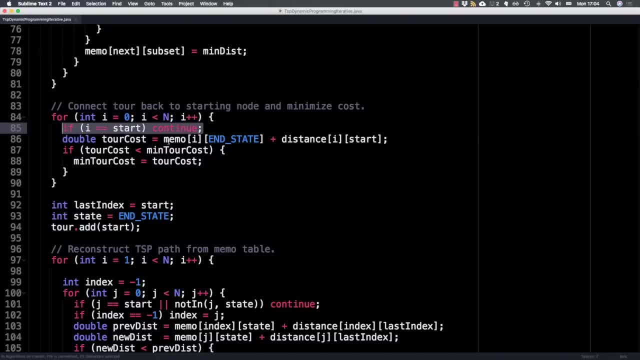 starting node and and then do a lookup in our table for that end, node I and the state and state. So we finished a tour and the tour ended on node i and then go from i, which we ended on, back to the start node. 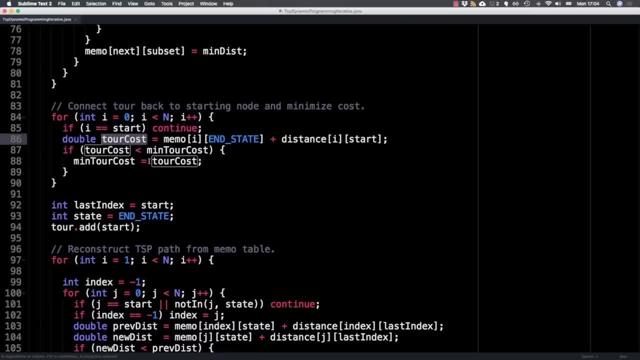 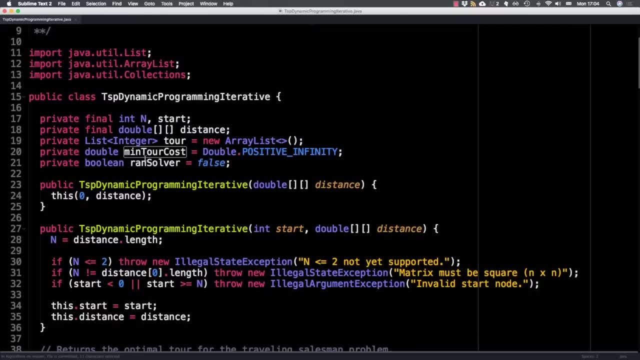 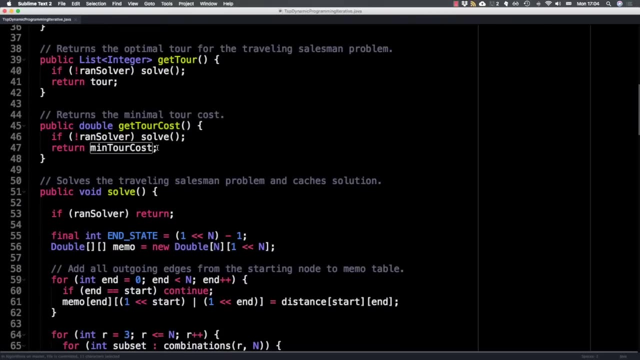 So that's the tour cost. Now we just minimize over this variable and update the mint or cost which, if we go back you can see was one of our instance variables which had set the positive infinity. So we're minimizing this And this is what gets returned on the get tour cost. 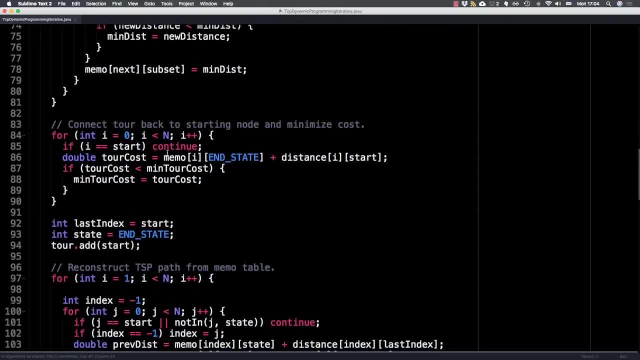 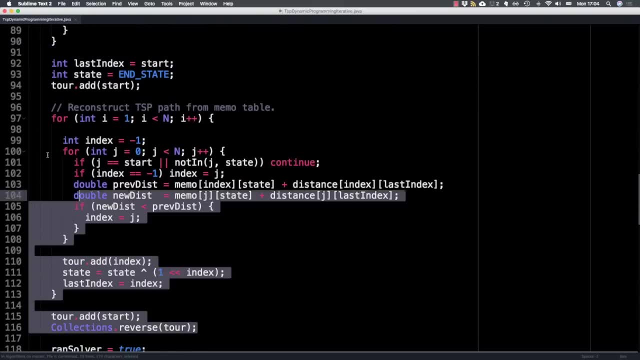 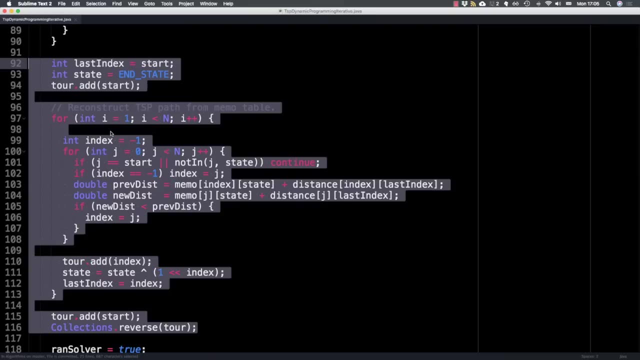 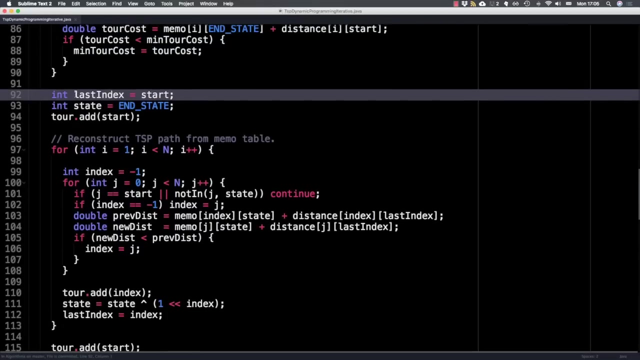 function All right. So this finds the minimum tour cost And this section you see right here finds what the actual tour is, which is really useful, And it does that by looking inside the the memo table at the values we've computed. So 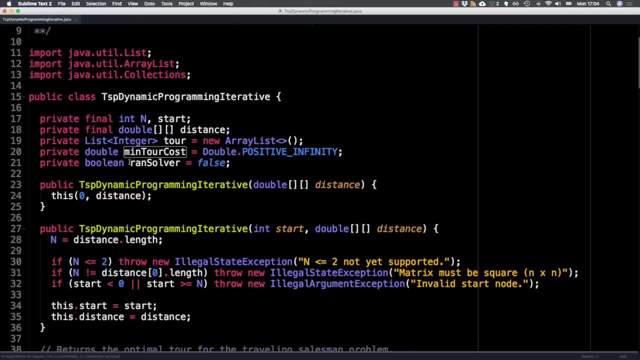 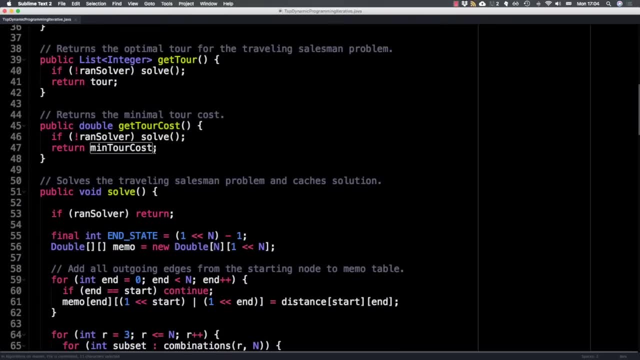 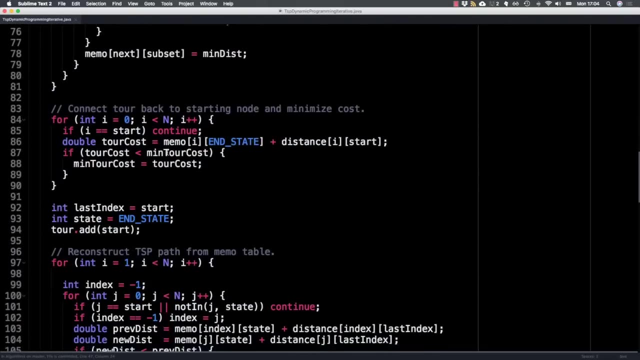 cost which, if we go back you can see, was one of our instance variables which had set the positive infinity. So we're minimizing this And this is what gets returned on the get tour cost function. All right, So this finds the minimum tour cost And this second 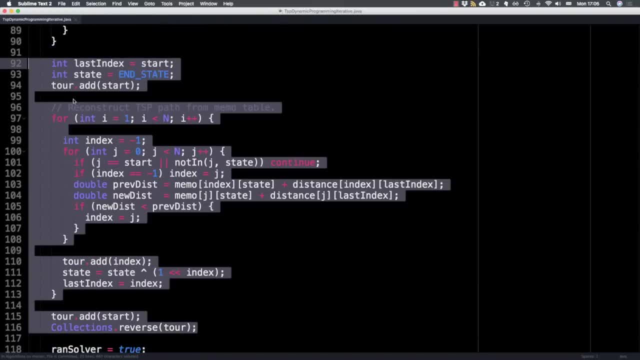 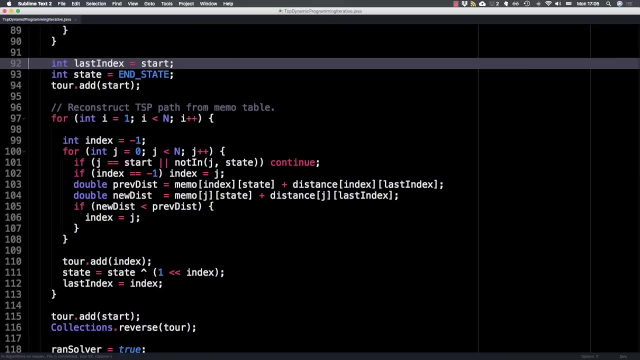 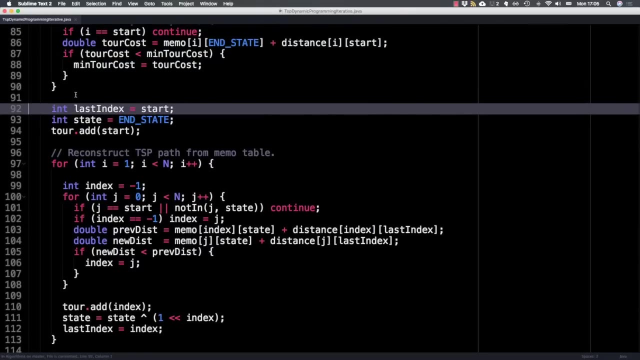 section you see right here, finds what the actual tour is which is really useful, And does that by looking inside the the memo table at the values we've computed. So we initialize a variable called the last index and it initialize the starting node, because that's essentially. 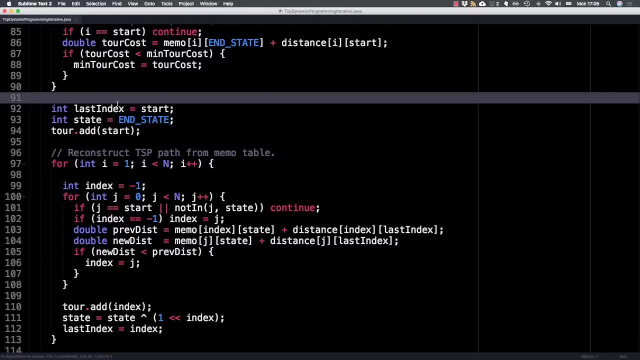 the very last node, if you want. when we do the tour, we end up at the start node again And the state It is the end state. So we're working our way backwards. So we start at the end state and then we're going to slowly, I guess, reduce our tour until we're back to the, the starting. 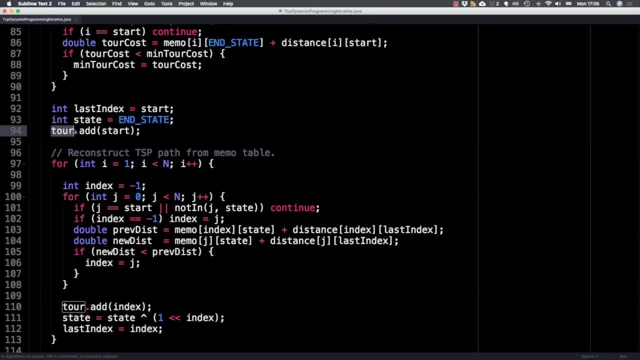 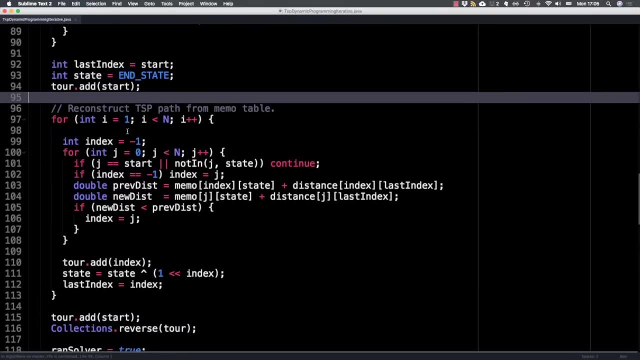 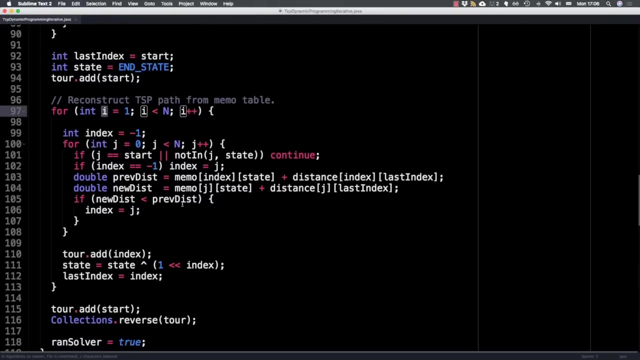 node. So. So in our tour we add that starting node And then we're going to loop n minus one times. And this variable i is just for a, for a counter, So it's not, it's not used anywhere in here. So we loop n minus one times. 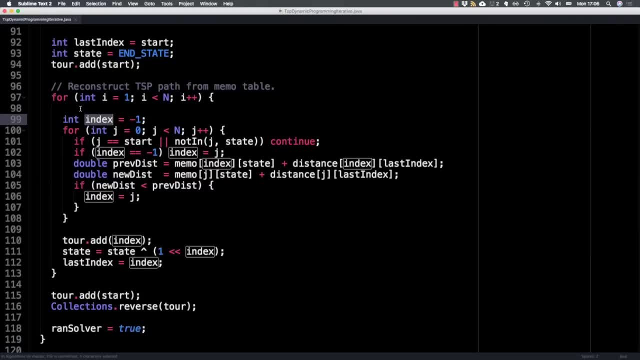 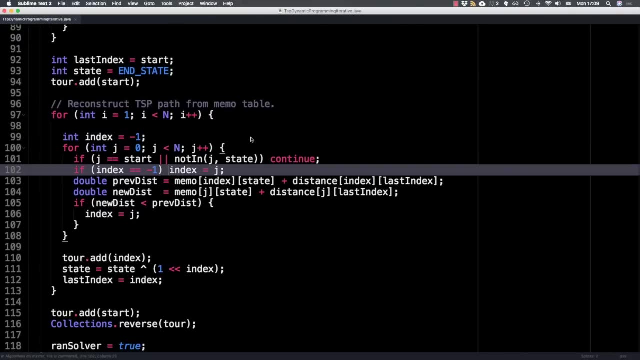 And for this index variable. so this is like the, the node we want to to go to next, So it's the best, It's the index of the best next node. But to find that next best node we need to look at where we were last, which is the last index, and go to the next best node, which? 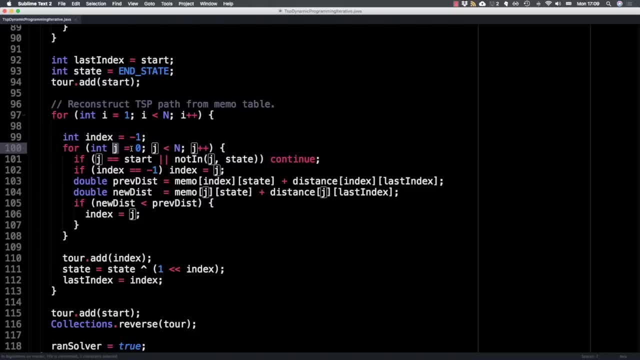 is going to be j, So we loop over all possible j nodes. if you will start j at zero and loop up to n And then skip over when j is equal to the start or is not in the state, Because we would have already visited a node. 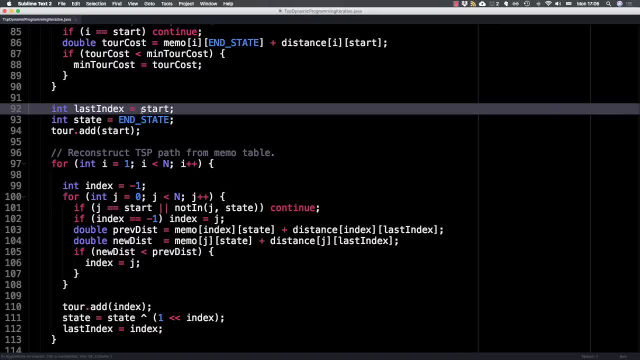 we initialize a variable called the last index and it initialize the starting node, because that's essentially the very last node. if you want, when we do the tour, we end up at the start node again And the state is the end state. So we're working our way backwards. 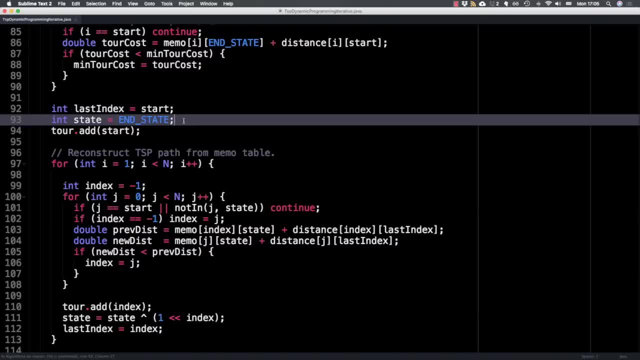 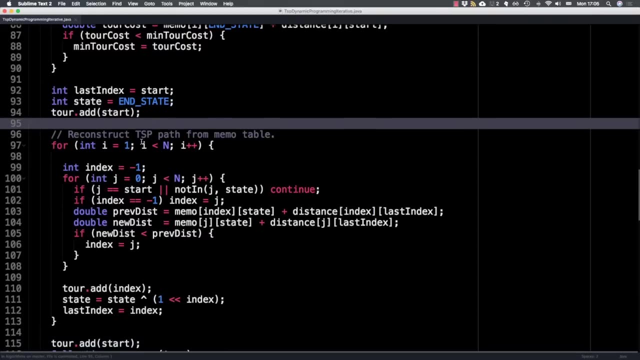 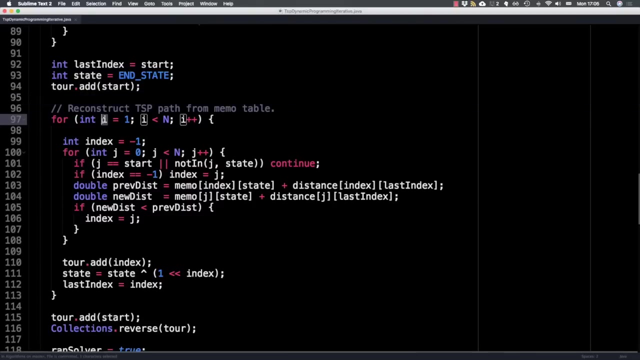 So we start at the end state and then we're going to slowly, I guess, reduce our tour until we're back to the starting node. So So in our tour we add that starting node And then we're going to loop n minus one times And this variable I 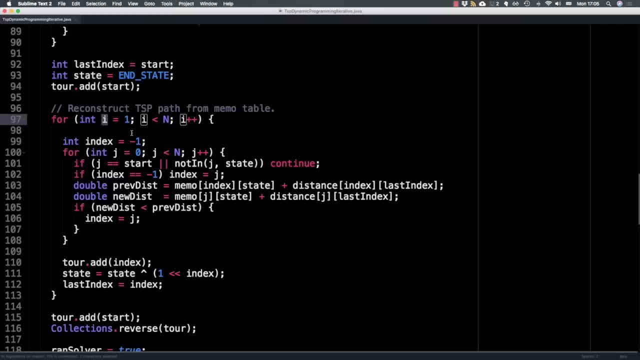 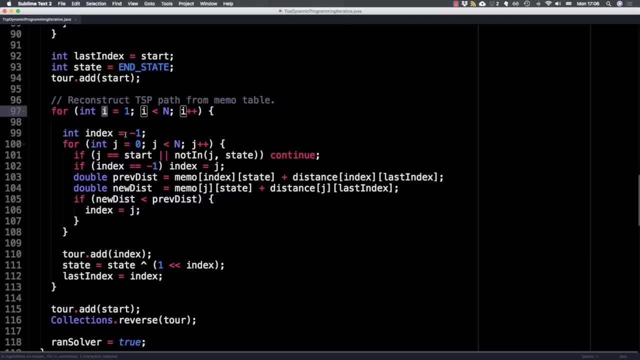 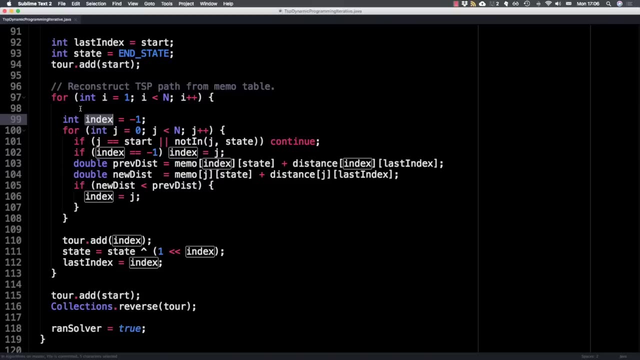 is just for for counter, So it's not, it's not used anywhere in here. So we loop n minus one times And for this index variable. so this is like the, the node we want to to go to next. So it's the best, That's the index of the best, next node, But to find that next. 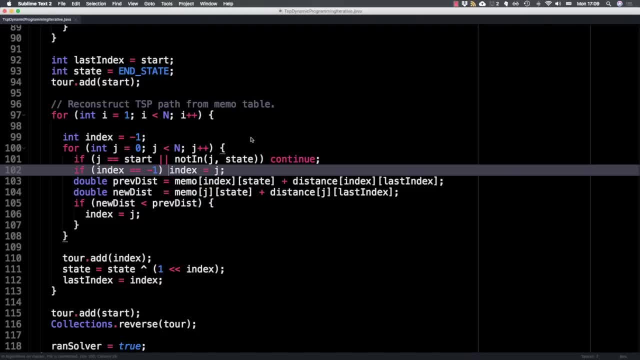 best node. we need to look at where we were last, which is the last index, and go to the next best node, which is going to be j. So we loop over all possible jth nodes. if you will start j at zero and loop up to n And then skip over when j is equal to the start or is not? 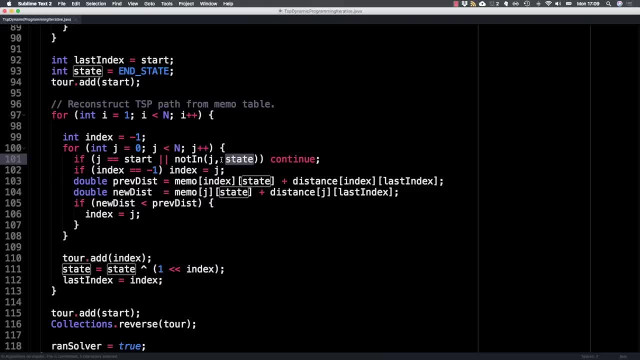 in the state, Because we would have already visited a node otherwise. And if index is minus one, then it's the first valid node we encounter. So set index equal to j. Otherwise look at the previous distance. So for the node at index. 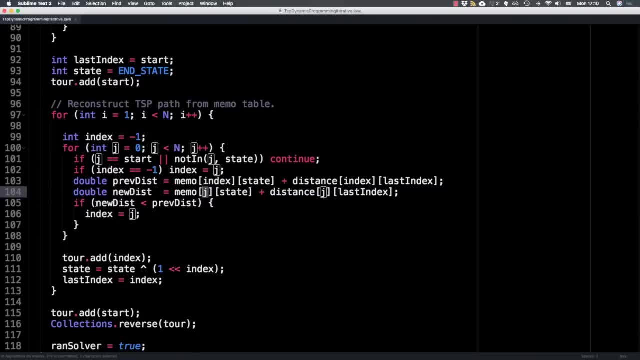 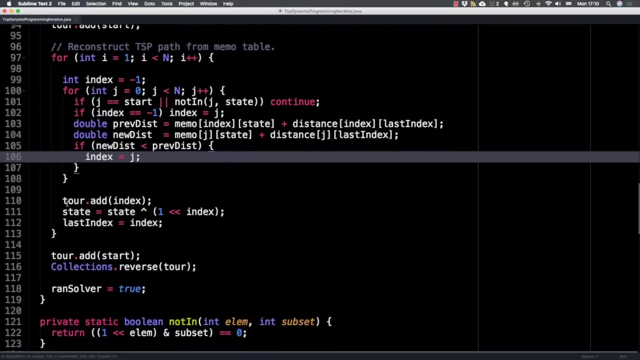 versus the node j And then if selecting node j gives us a smaller value, then we know we want to update index to be j And, and doing this for all all the nodes will find us the next best node going backwards. then we want to add that nodes index to the tour and then toggle the. 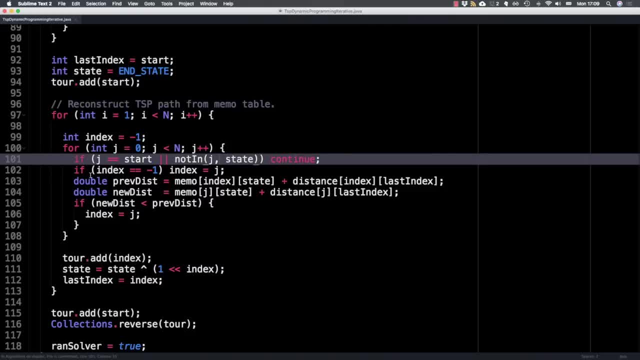 Otherwise, and if index is minus one, then it's the first valid node we encounter. So set index equal to j. Otherwise, look at the previous distance, So for the node index versus the node j, And then if selecting node j gives us a smaller value, then we know we want to. 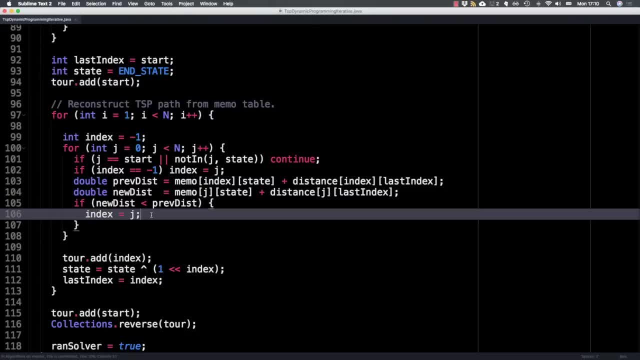 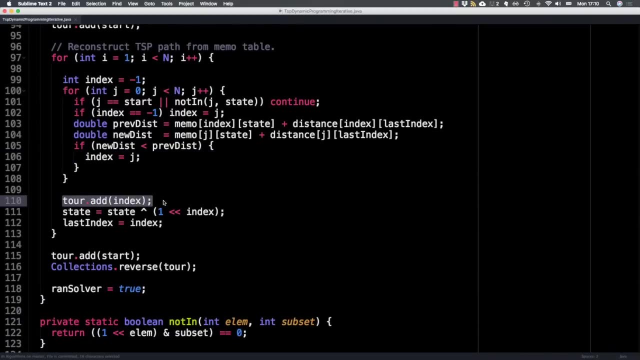 update index to be j And and doing this for all all the nodes will find us the next best node going backwards. then we want to add that nodes index to the tour and then toggle the that bit off and then set the last index to be the current index. So we're going backwards. 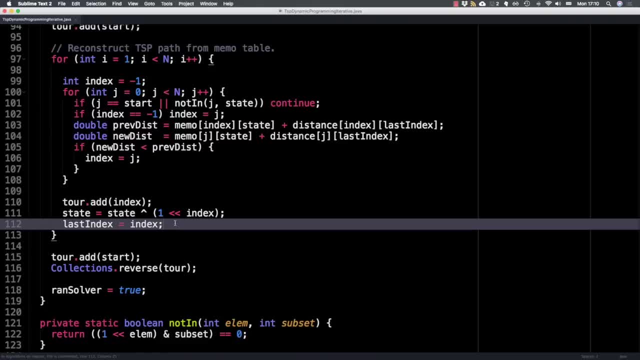 And basically starting from a fully completed tour and like shrinking the tour down to just the starting node again, And at the very end we want to add that starting node to the tour and then reverse the order of the tour. This is because we're going backwards. we're starting at the 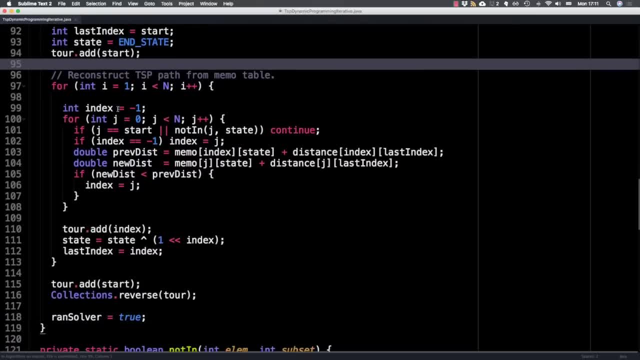 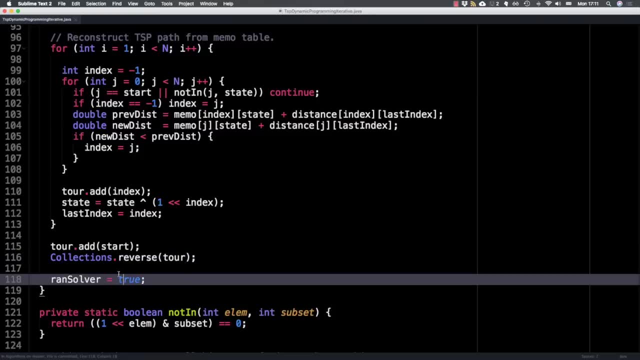 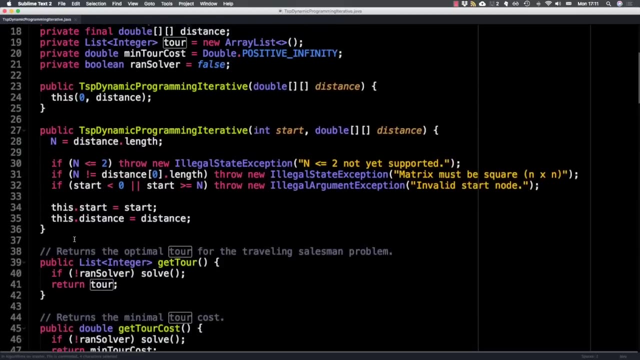 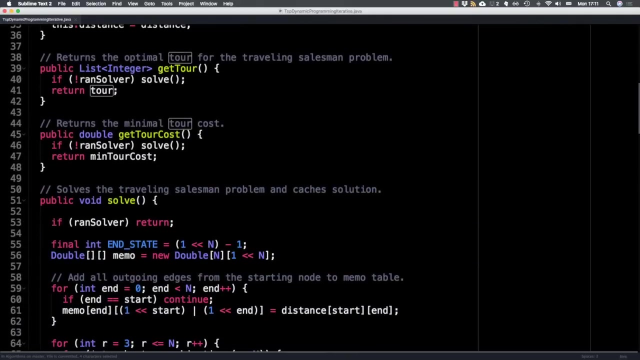 end state and then working our way backwards. So our tour is in effect in reverse order. So we want to reverse the tour order And then we can mark the solver as completed And tour, if we look up, here was just a list of integers And tour is the variable we return when we call get. 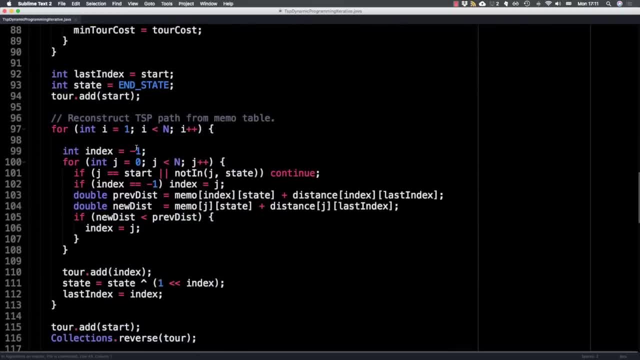 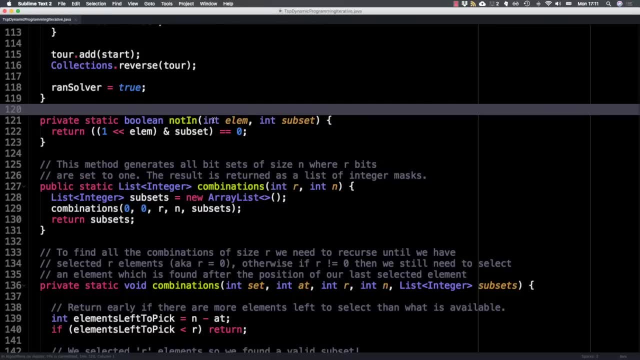 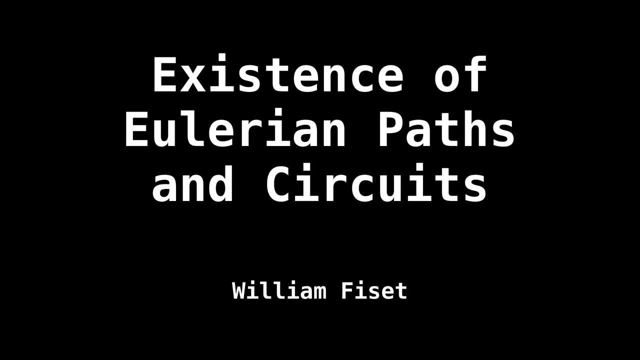 tour. The only thing I did not cover was this not in function which just checks if a bit or the element was not set in subset. So you check that bit is equal to zero. Today we're going to talk about Eulerian paths and circuits from a computer science perspective. we're going to start 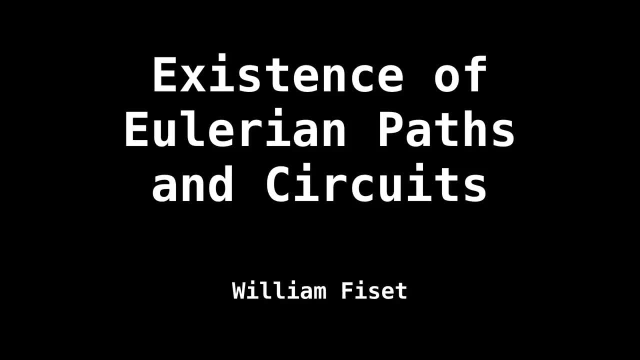 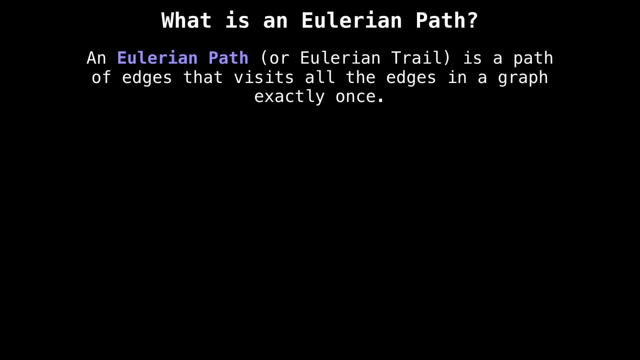 with discussing what Euler paths and circuits are, how to determine their existence, how to find them And, lastly, we're going to look at some code to wrap things up. Let's begin with what an Euler Eulerian path is, And Euler path, also called an Eulerian trail, is a path of edges in a graph that 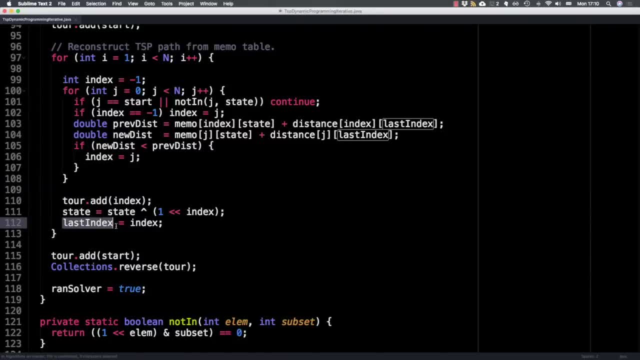 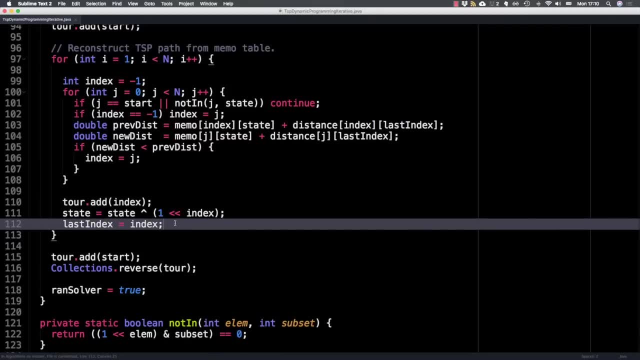 that bit off and then set the last index to be the current index. So we're going backwards and basically starting from a fully completed tour and like shrinking the tour down to just the starting node again, And at the very end we want to add that starting node to the tour and then 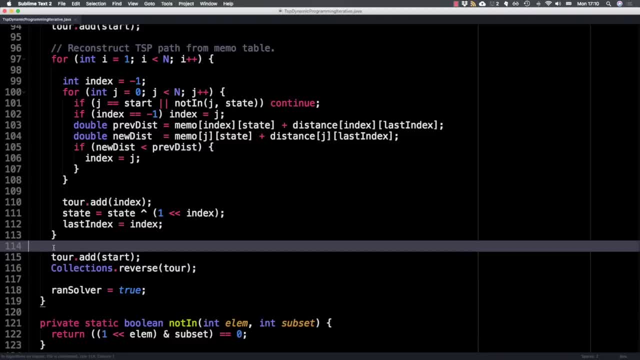 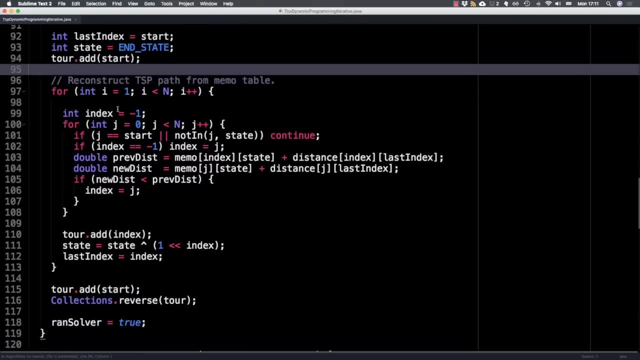 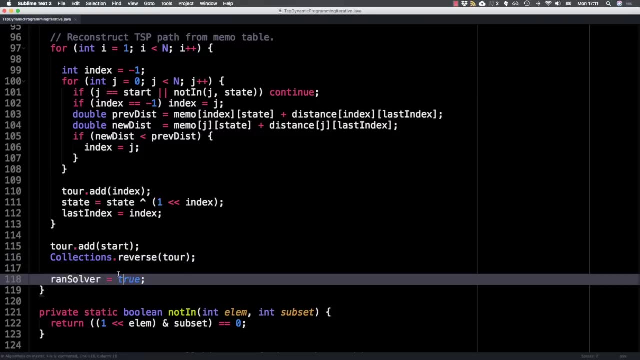 reverse the order of the tour. This is because we're going backwards. we're starting at the end state and then working our way backwards, So our tour is in effect, in reverse order. So we want to reverse the tour order And then we can mark the solver as completed And tour. 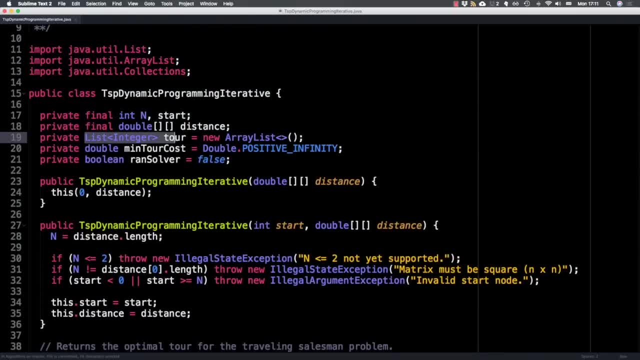 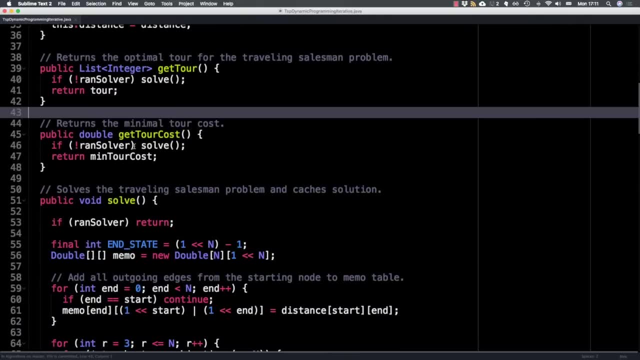 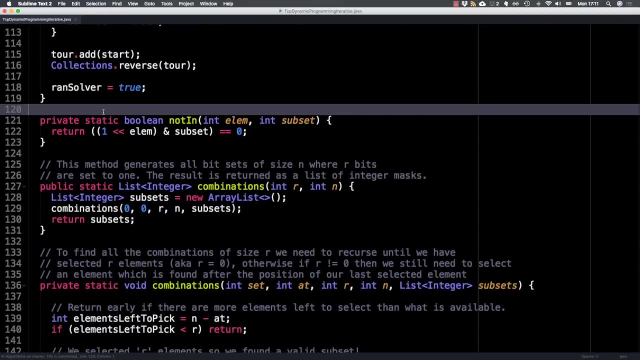 if we look up, here was just a list of integers And tour is the variable we return when we call get tour. The only thing I did not cover was this not in function, which just checks if a bit Okay Or the element was not set in subset, So you check that bit is equal to zero. Today we're 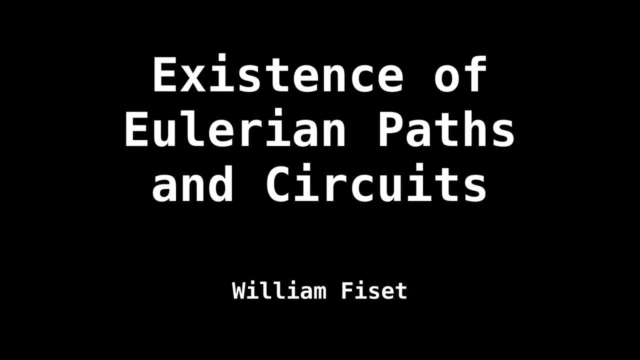 going to talk about Eulerian paths and circuits from a computer science perspective. we're going to start with discussing what Euler paths and circuits are, how to determine their existence, how to find them And, lastly, we're going to look at some code to wrap things. 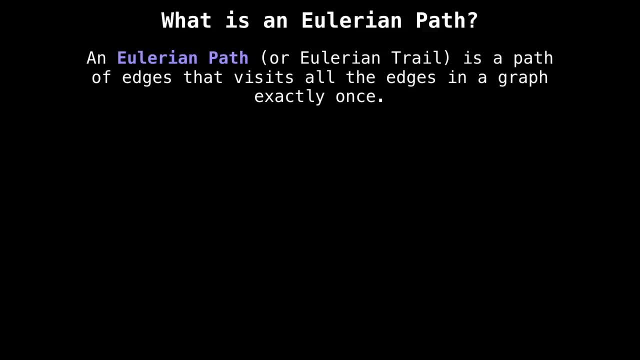 up. Let's begin with what an Eulerian path is. Okay, An Euler path, also called an Eulerian trail, is a path of edges in a graph that visits every edge exactly once. Suppose we have the undirected graph below and we want to find: 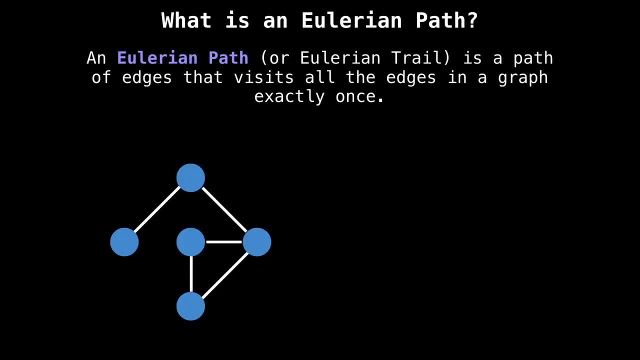 an Eulerian path. First off, not every graph has an Eulerian path. This one does, But even still, we need to be careful about which node we start our path at. Suppose we begin the path at the middle right node and decide to follow the path left down, up, up again. 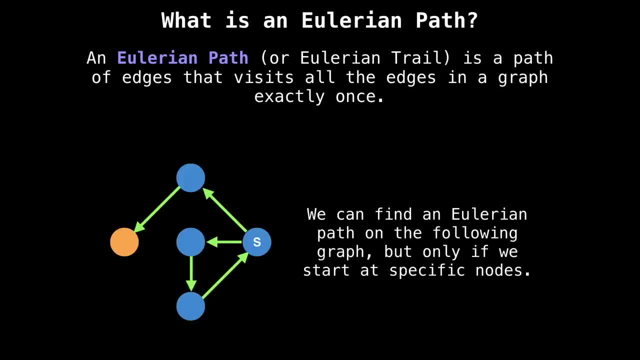 and finally left. This completes the Eulerian path. However, suppose we start at the top node. what happens if we decide to find a path from this node? If we take the edge going down, you'll notice that we are now stuck. we cannot go anywhere else from this node. 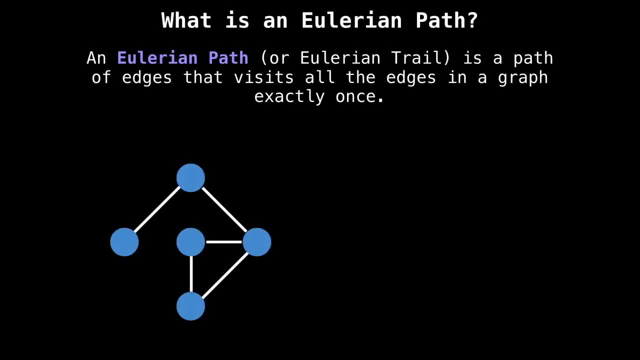 visits every edge exactly once. Suppose we have the undirected graph below and we want to find an Eulerian path First off. not every graph has an Eulerian path. This one does, But even still we need to be careful about which node we start our path at. Suppose we begin the path with a path that 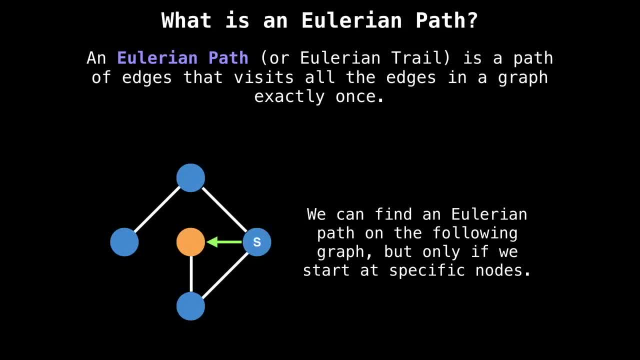 is the middle right node and decide to follow the path left, down, up, up again and finally left. this completes the Eulerian path. However, suppose we start at the top node. what happens if we decide to find a path from this node? If we take the edge going down, you'll notice that we are now stuck. 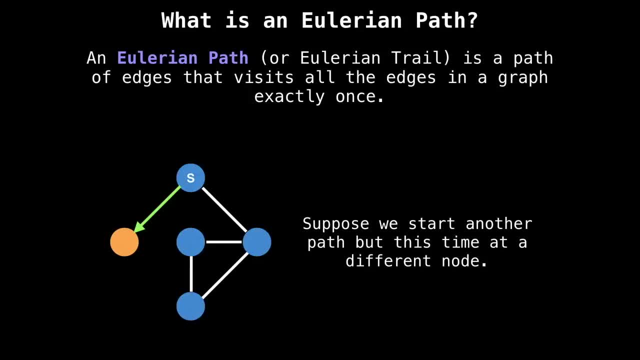 we cannot go anywhere else from this node, since there are no edges left to follow. More importantly, the issue is that we have unvisited edges that we still have not used or traversed. So we'll see how to resolve, or rather avoid, this issue altogether later, so that we always find an Eulerian. 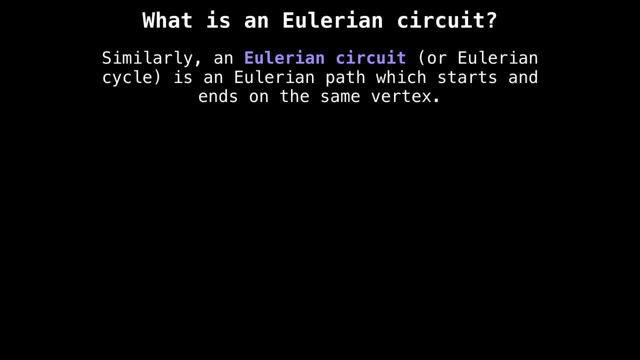 path, when we know one exists. Moving on, let's talk about Eulerian circuits, also called Eulerian cycles. And Eulerian circuit is an Eulerian path which starts at the top of the graph and ends at the same vertex, So similar to Eulerian paths. not every graph has an Eulerian circuit, but the 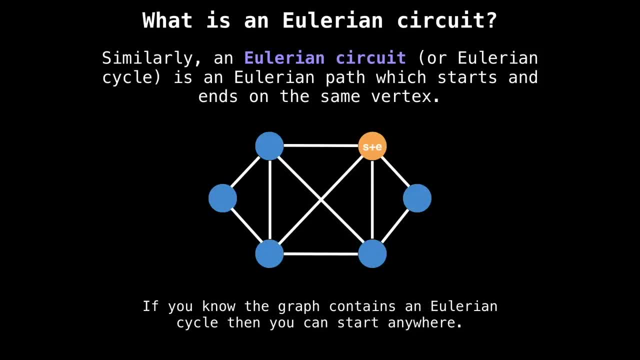 following graph does. If you know your graph has an Eulerian circuit, then you can begin the circuit at any node. I'm going to begin the circuit on the orange node and also end it on the orange node And that's the full circuit. If your graph does not contain an Eulerian circuit, you may not be able to. 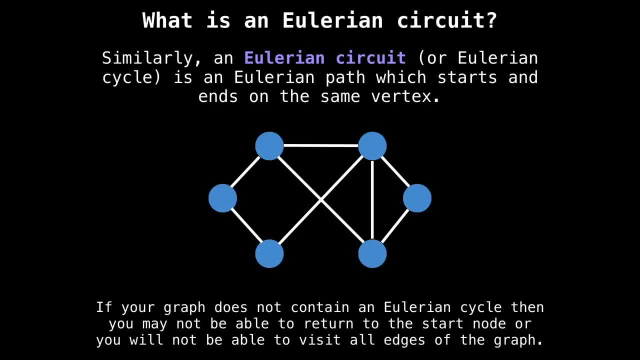 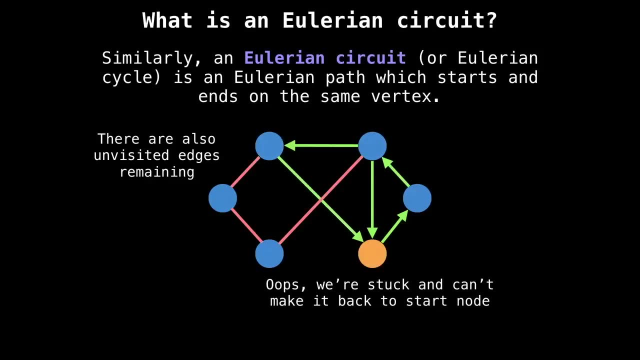 return to the start node or you will not be able to visit all the edges of the graph. For example, let's start another circuit starting from the same node on this slightly modified graph. So by randomly selecting edges to traverse, we weren't able to make it back to the starting node. 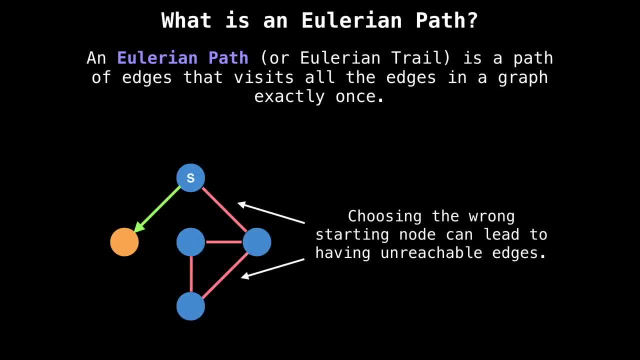 since there are no edges left to follow. More importantly, the issue is that we have unvisited edges that we still have not used or traversed. So we'll see how to resolve, or rather avoid, this issue altogether later, so that we always find an Eulerian path when we know one exists. Moving on, let's talk. 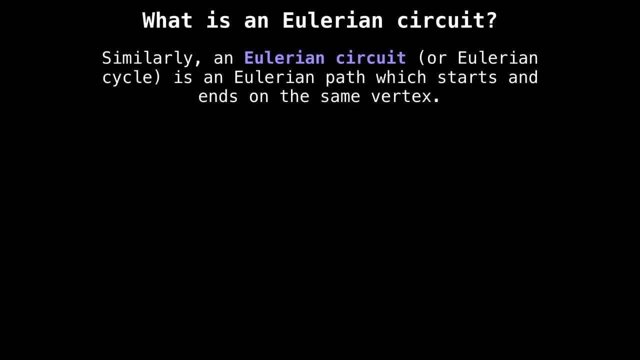 about Eulerian circuits, also called Eulerian cycles. And Eulerian circuit is an Eulerian path which starts at the top of the graph and then goes down to the bottom of the graph And ends on the same vertex, So similar to Eulerian paths. not every graph has an Eulerian. 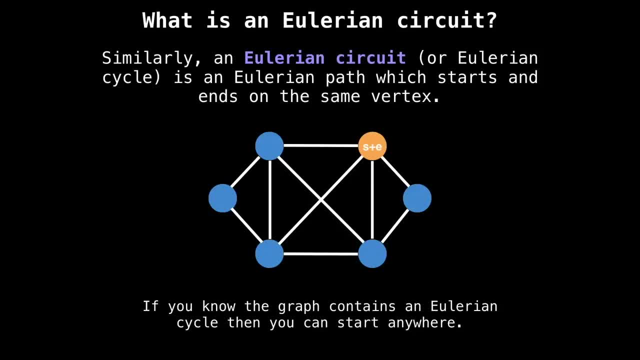 circuit, but the following graph does. If you know your graph has an Eulerian circuit, then you can begin the circuit at any node. I'm going to begin the circuit on the orange node and also end it on the orange node, Okay. 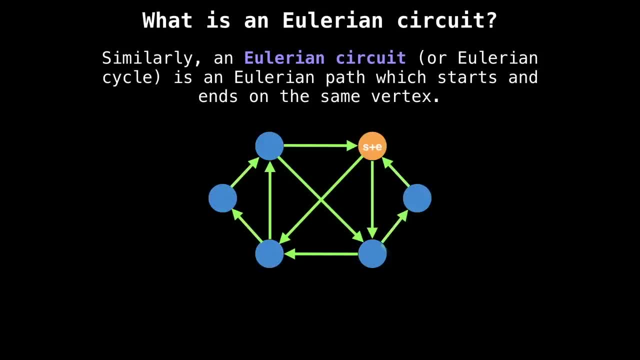 and that's the full circuit. If your graph does not contain an Eulerian circuit, you may not be able to return to the start node or you will not be able to visit all the edges of the graph. For example, let's start another circuit starting from the same node on this: 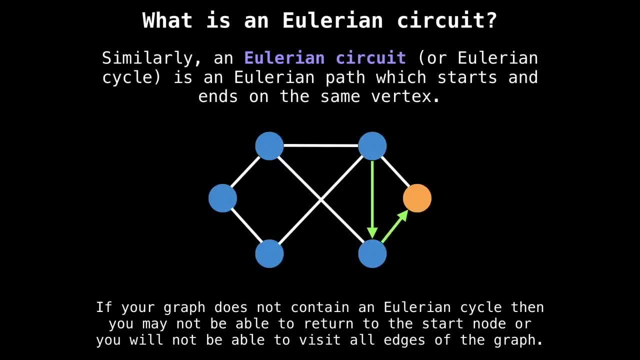 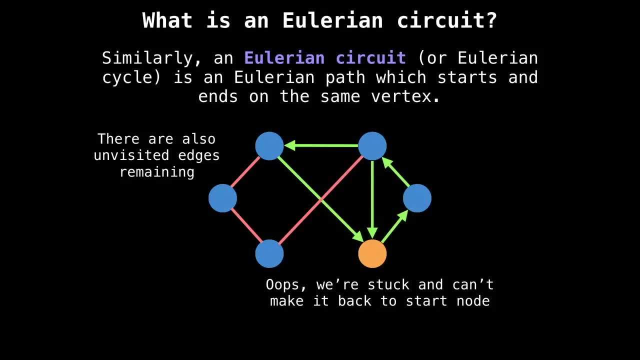 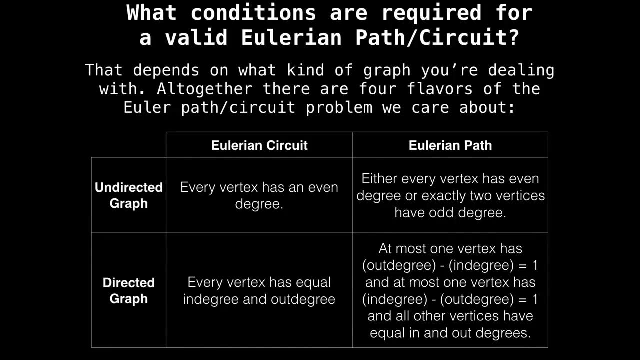 slightly modified graph, So by randomly selecting edges to traverse, we weren't able to make it back to the starting node. Furthermore, we also have unvisited edges, So that's double bad. Luckily for us, we don't have to guess whether or not a graph contains an Eulerian path or an Eulerian circuit. 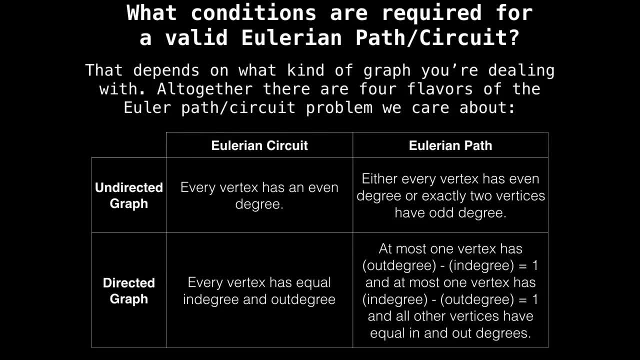 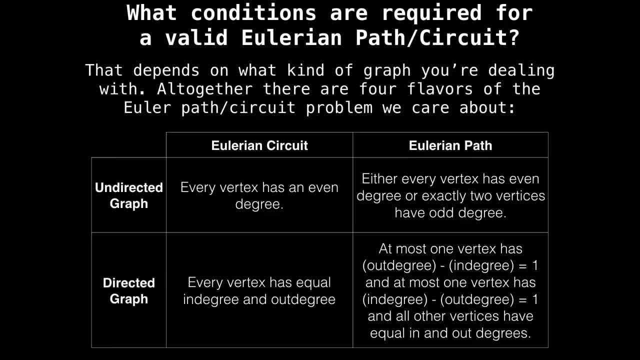 with the start node. So let's start with the start node. So let's start with the start node First up. this next graph will show us what it means. in this table, There are four flavors of Eulerian paths and circuits that we care about, And those are: whether the graph is 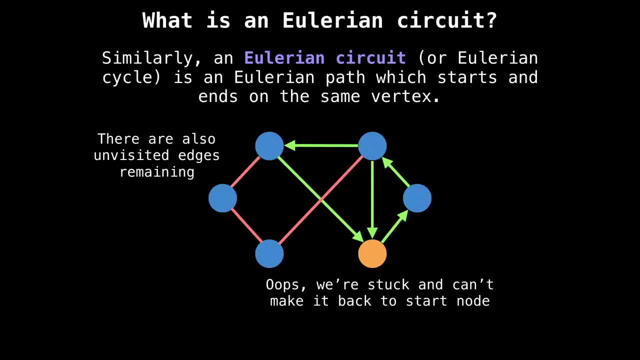 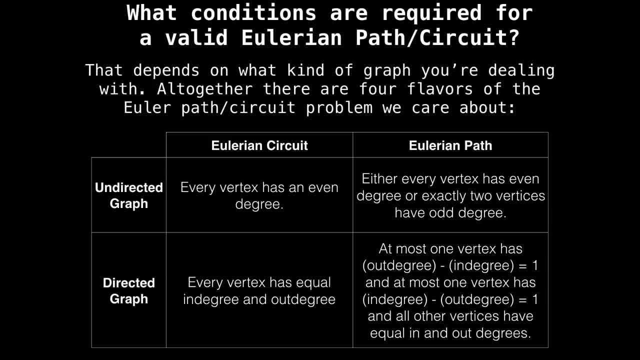 Furthermore, we also have unvisited edges, So that's double bad. Luckily for us, we don't have to guess whether or not a graph contains an Eulerian path or an Eulerian circuit. we can inspect the graph we're dealing with by counting the in and out degrees of each node to determine whether or not. 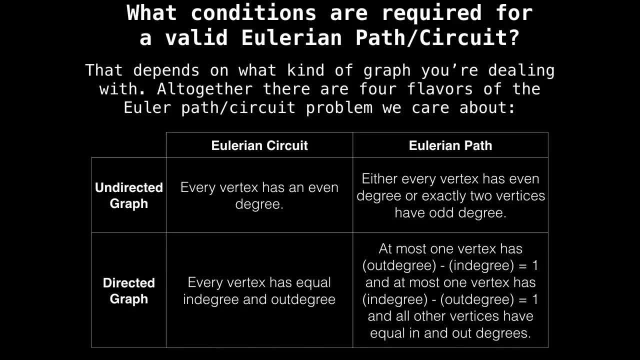 the graph meets one of the conditions. in this table, There are four flavors of Eulerian paths and circuits that we care about, And those are whether the graph is directed or undirected, and whether or not we want to find an Eulerian path or an Eulerian circuit. All 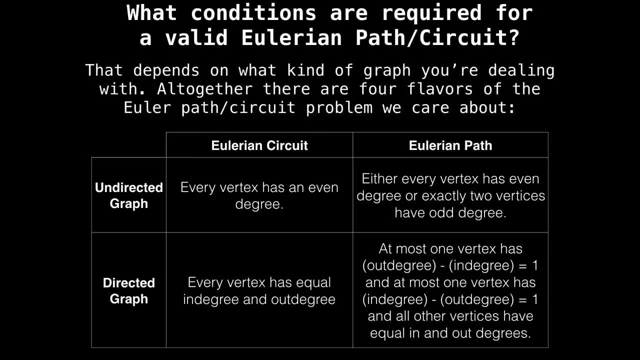 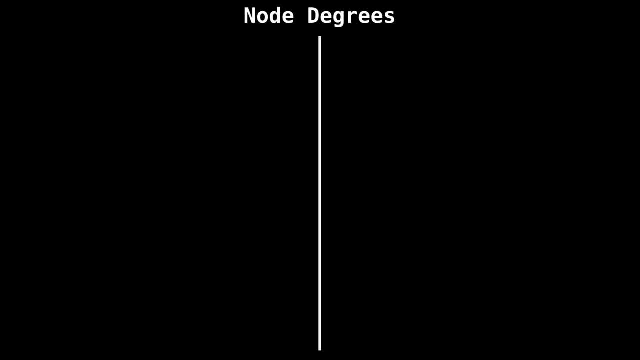 of these variants talk about node degrees, So I want to have a quick look at that before coming back to this table. The degree of a node means different things depending on whether the graph we're dealing with is directed or undirected. In an undirected graph, the node degree is simply how many edges are attached to a particular node- the blue. 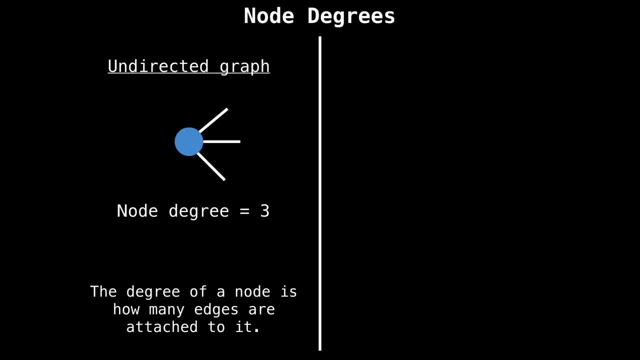 node in this picture has three edges attached to it, So it's degrees three. In a directed graph there are two forms of node degrees. there are in degrees and out degrees, because the edges are directed. The in degree is the number of incoming edges to a node and the out degree of a node is the number of outgoing edges from that. 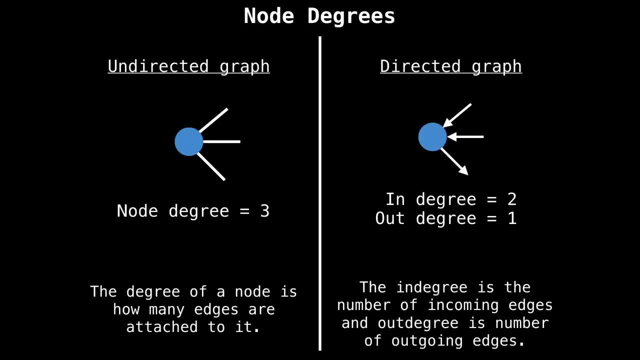 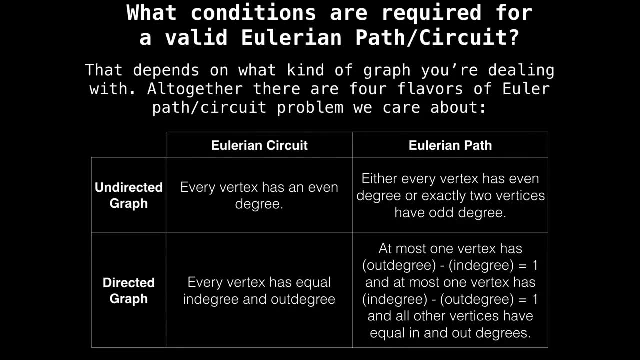 node. So in the example on the right, the in degree of the notice to, while the out degree is one pretty simple. Coming back to the table, you should be able to understand the constraints required for each variant of the Eulerian path and Eulerian circuit problem. However, let's go over them one by one. Anyways, the simplest case is when we have 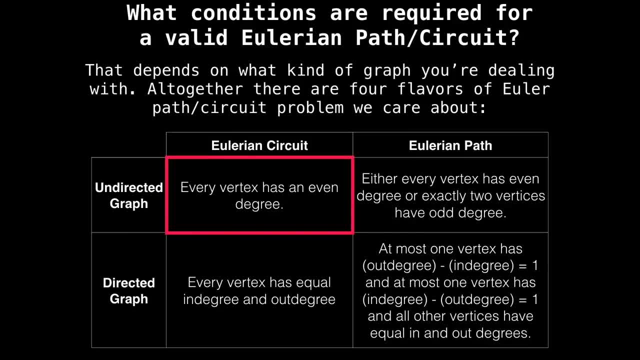 an undirected graph and we want to find an Eulerian circuit. The requirement for this is that every node in the graph has an even degree. The oily variant path problem on an undirected graph is very similar, except that, in addition that every vertex has an even degree, you can also have exactly two vertices which have an odd degree. those two vertices, if they exist, would be the start and end nodes of the Eulerian path I directed graph. you can have an oil layer circuit if every vertex has an equal in and out degree. This 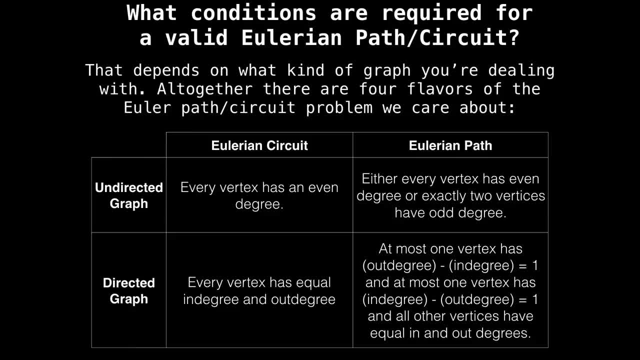 directed or undirected, And whether or not we want to find an Eulerian path or Eulerian circuit. All of these variants talk about no degrees, So I want to have a quick look at that before coming back to this table. The degree of a node means different things. 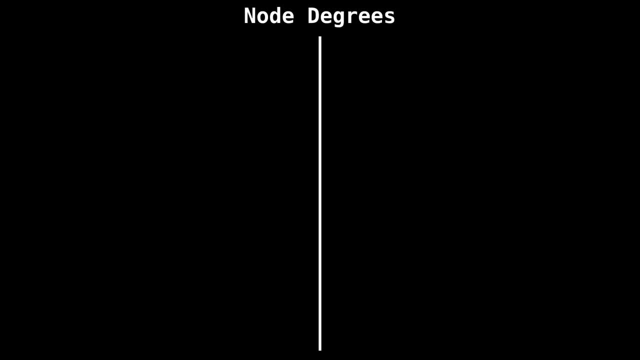 depending on whether the graph we're dealing with is directed or或 beret Abbой 공 iteration, or undirected. In an undirected graph, the node degree is simply how many edges are attached to a particular node. the blue node in this picture has three edges attached to it, So 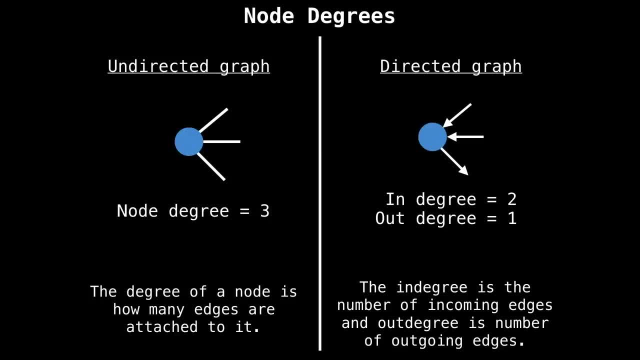 it's degrees three. In a directed graph there are two forms of no degrees. there are in degrees and out degrees, because the edges are directed. The in degree is the number of incoming edges to a node and the out degree of a node is the number of outgoing edges. 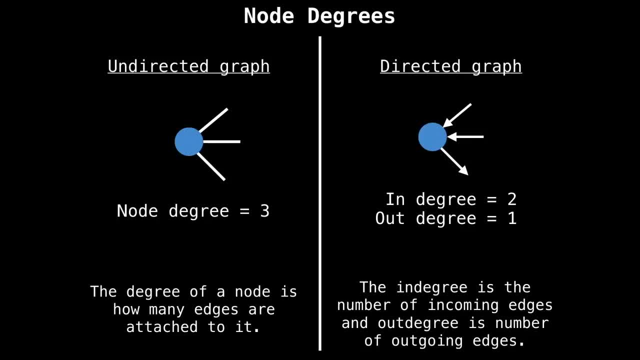 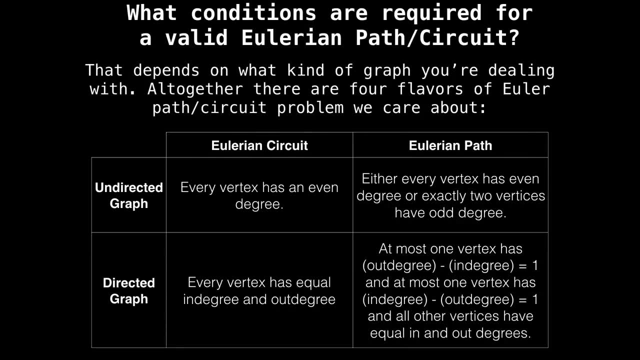 from that node. So in the example on the right, the in degree of the node is two, while the out degree is one. pretty simple, Coming back to the table, you should be able to understand the constraints required for each variant of the Eulerian path and Eulerian circuit. 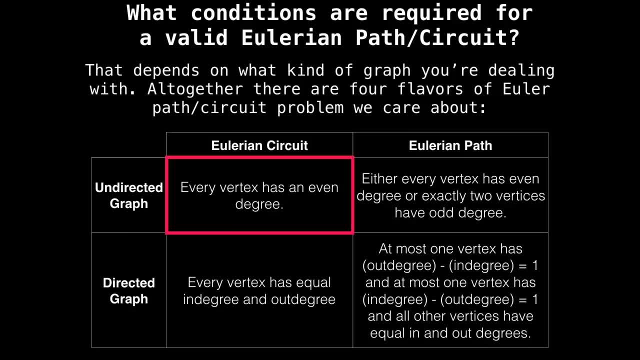 problem. However, let's go over them one by one. Anyways, the simplest case is when we have an undirected graph and we want to find an Eulerian circuit. The requirement for this is that every node in the graph graph has an even degree. the Eulerian path problem on an undirected graph is very similar. except that, in addition that every vertex has an even degree, you can also have exactly two vertices which have an odd degree. those two vertices, if they exist, would be the start and end nodes of the Eulerian path. I directed graph. you can have an Eulerian. 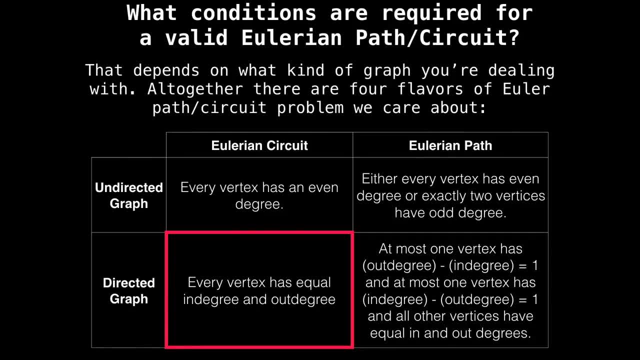 circuit if every vertex has an equal in and out degree. This is the counterpart to the undirected graph version. The last variant is finding an Eulerian path on a directed graph. for there to exist an Eulerian path on a directed graph, at most one vertex has an out degree minus an N degree which is equal to one, and at 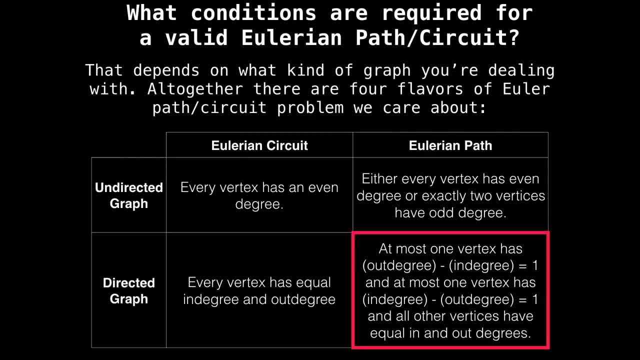 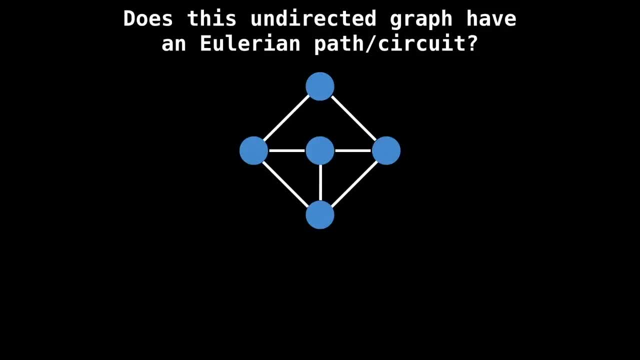 most, one vertex has an N degree minus an out degree equal to one, and all other verse vertices have equal in and out degrees. So it's now quiz time And I'm going to make sure you've been paying attention to this part of the video until the end of the video. I'll see you next time. 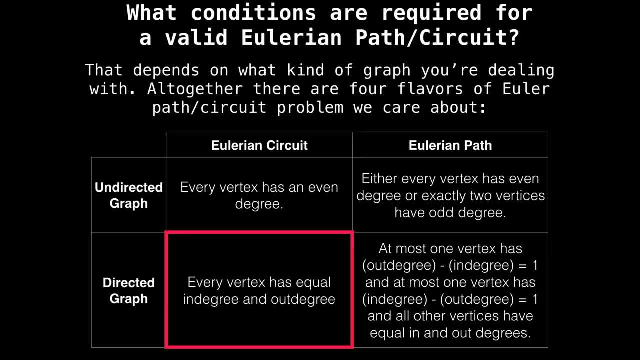 is the counterpart to the undirected graph version. The last variant is finding an Euler and path on a directed graph. for there to exist an Euler and path on a directed graph, at most one vertex has an out degree minus an N degree which is equal to one, and at most one vertex has 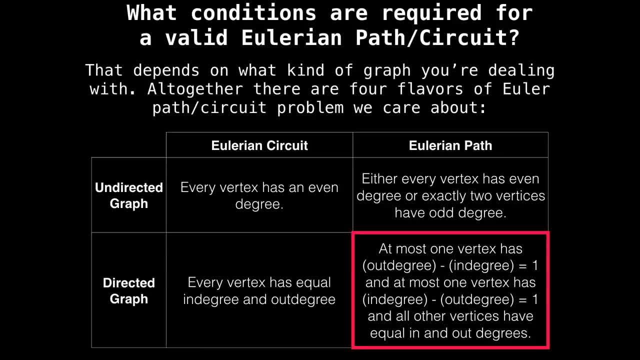 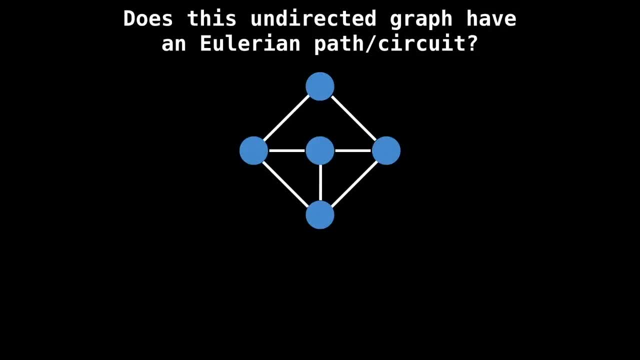 an N degree minus an out degree equal to one, and all other verse vertices have equal in and out degrees. So it's now quiz time and I'm going to make sure you've been paying attention. I'm going to present to you various graphs and you need to determine whether the 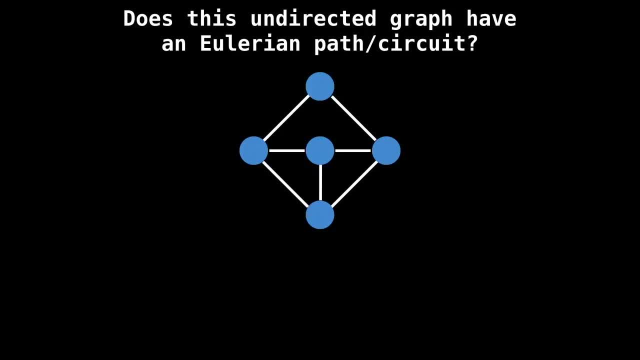 following graph has an Euler and path and Euler and circuit or both. So we'll start with undirected graphs and then later move on to directed graphs. Please feel free to pause the video to think things over. So this graph has no Euler and path or circuit. you can tell, because there are too many nodes. 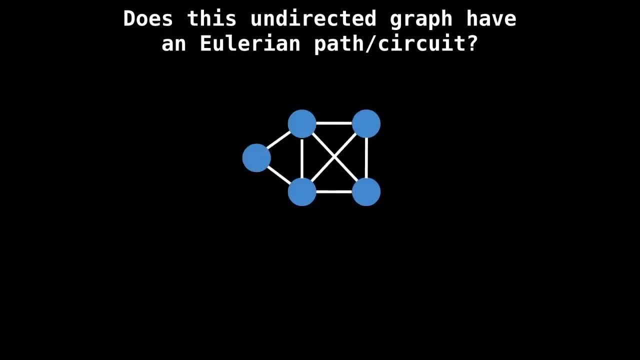 with an odd degree. How about this graph? Again, feel free to pause the video. This graph has an Euler and path and the green nodes represent the valid start and end nodes for the Euler and path. What about this graph? This graph has both an Euler and path and an 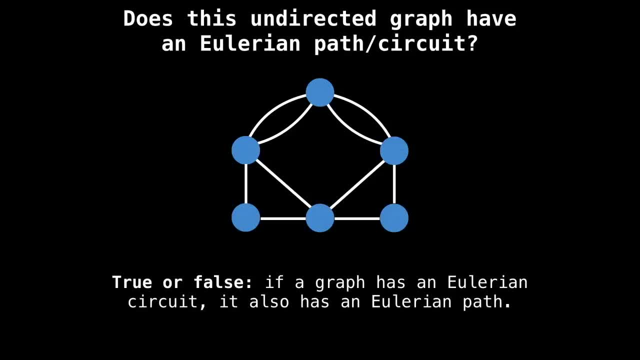 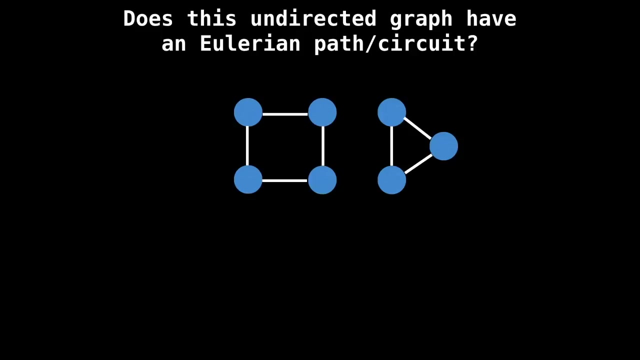 Euler and circuit As a side question: true or false? If a graph has an Euler and circuit, it also has an Euler and path. I'll give you a moment to think about it. The answer is true. Any circuit is an Euler and path. Here's another one. Are there any paths or circuits in this graph? 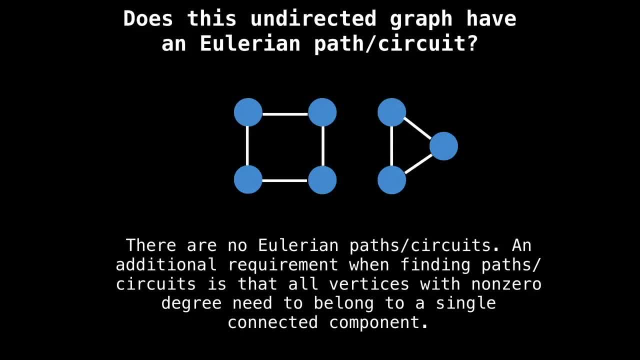 This one is a bit of a trick question, but there are no Euler and paths or circuits here. An additional requirement I have not yet mentioned is that, when finding paths and circuits, is that all vertices with nonzero degree need to belong to a single connected component. And here we have two connected components, So we cannot. 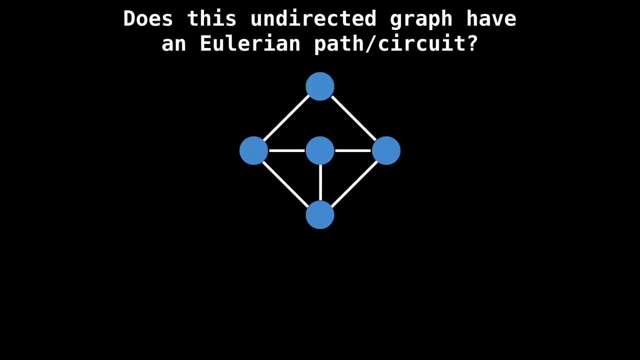 I'm going to present to you various graphs and you need to determine whether the following graph has an Eulerian path and Eulerian circuit or both. So we'll start with undirected graphs and then later move on to directed graphs. please feel free to pause the video to think. 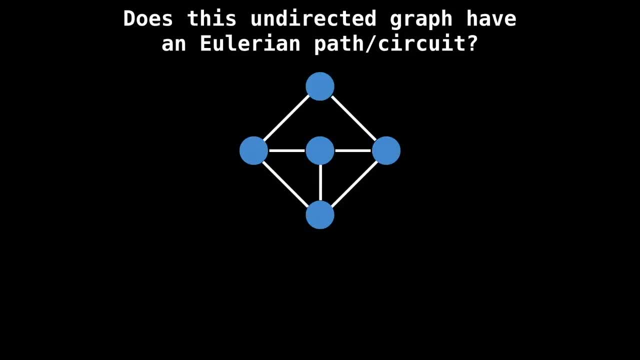 things over. So this graph has no Eulerian path or circuit, you can tell, because there are too many nodes, nodes with an odd degree. How about this graph? Again, feel free to pause the video. This graph has an Eulerian path and the green nodes represent the valid start and end nodes. 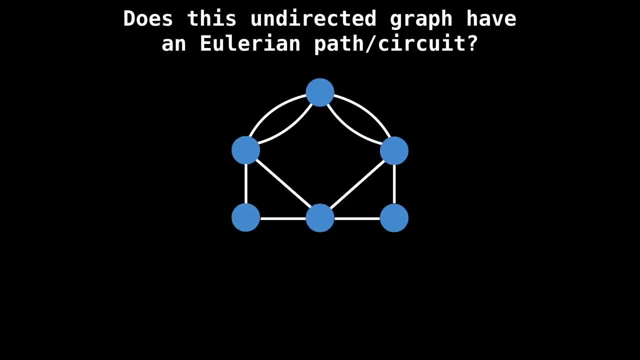 for the Eulerian path. What about this graph? This graph has both an Eulerian path and an Eulerian circuit. As a side question: true or false? if a graph has an Eulerian circuit, it also has an Eulerian path. I'll give you a moment to think about it. The answer is true. Any circuit is an. 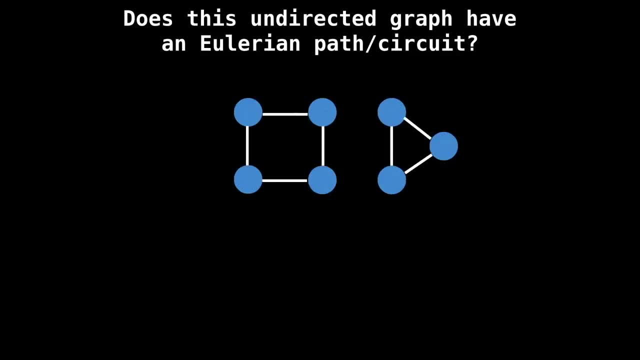 Eulerian path. Here's another one. Are there any paths or circuits in this graph? This one is a bit of a trick question, But there are no Eulerian paths or circuits here. An additional requirement I have not yet mentioned is that when finding paths and circuits, is that all vertices with nonzero degree need. 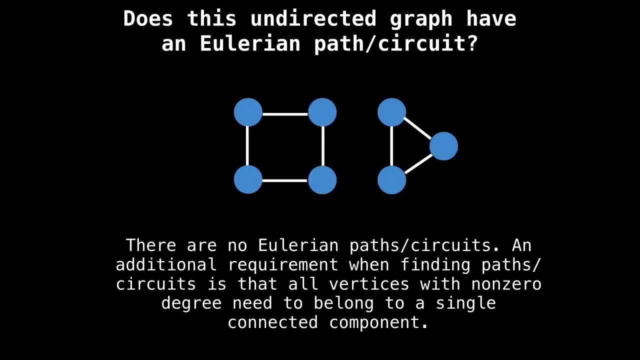 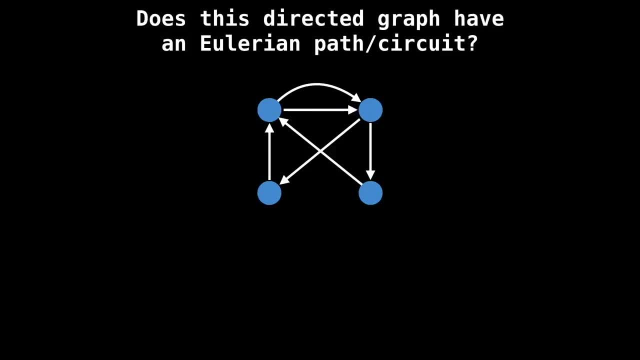 to belong to a single connected component, And here we have two connected components, So we cannot have an Eulerian path or circuit. Now let's have a look at an example with a directed graph. Does the following graph have any Eulerian paths or circuits? I'll give you a moment to think about it. Yes, this graph has both. 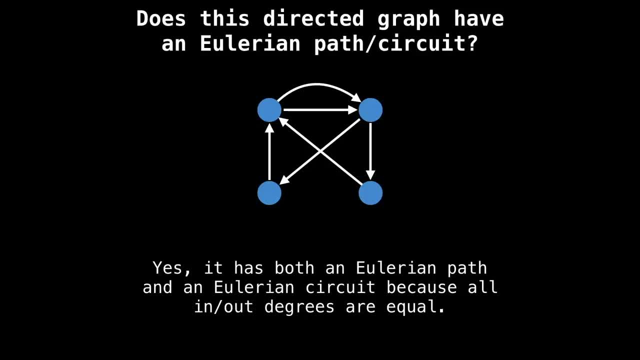 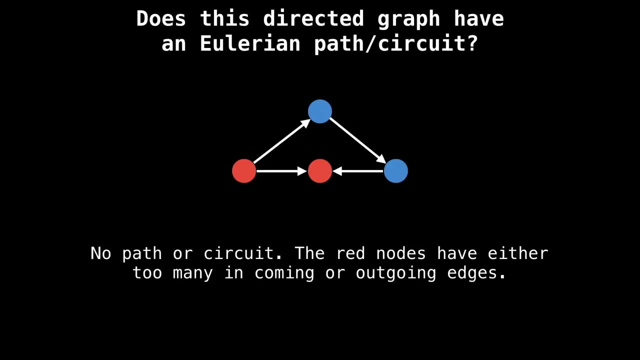 an Eulerian path and an Eulerian circuit, because all in and out degrees are equal. What about this graph? This graph has no Eulerian paths or circuits. the red nodes either have too many incoming or outgoing edges For an Eulerian path or circuit to exist. What about this graph? I'll give you a bit. 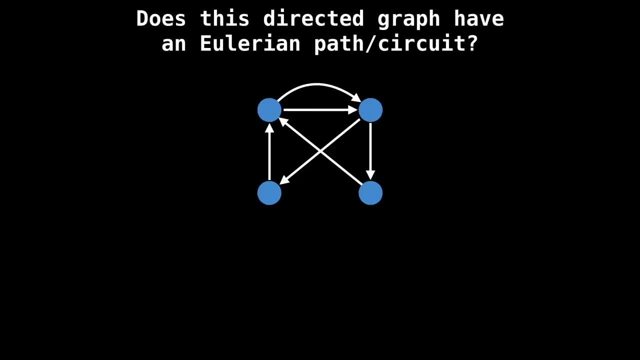 have an Euler and path or circuit. Now let's have a look at an example with a directed graph. Does the following graph have any? or they're in paths or circuits? I'll give you a moment to think about it. Yes, this graph has both an Euler and path. 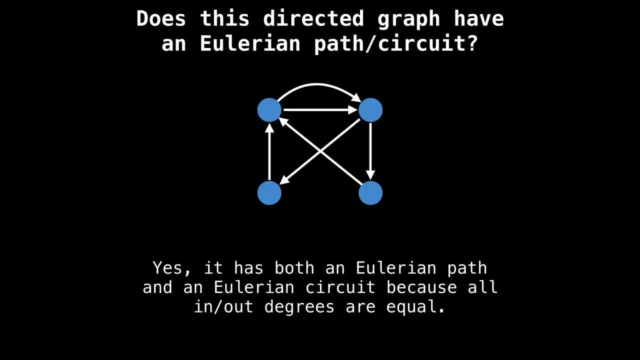 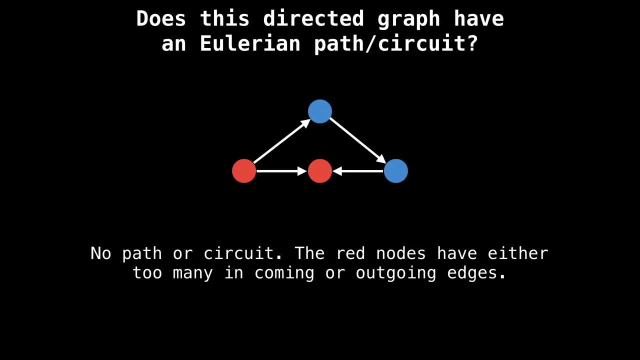 and an Euler and circuit, because all in and out degrees are equal. What about this graph? This graph has no Euler and paths or circuits. The red nodes either have too many incoming or outgoing edges for an Euler and path or circuit to exist. What about this graph I'll give you. 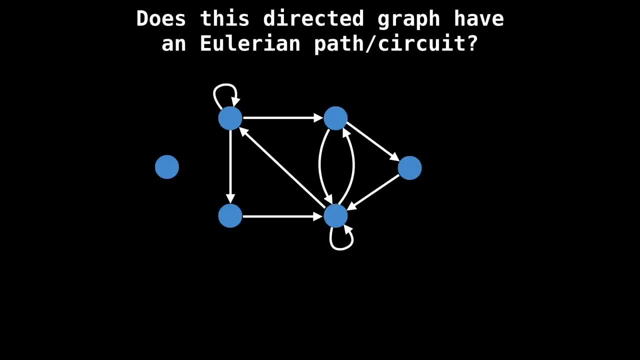 a bit more time because there are a lot of edges. This graph only has an Euler and path, but no Euler and circuit. It also has a unique start and end node for the path. Note that the singleton node has no incoming or outgoing edges, So it doesn't impact whether or not we have an Euler and path. Today we're talking. 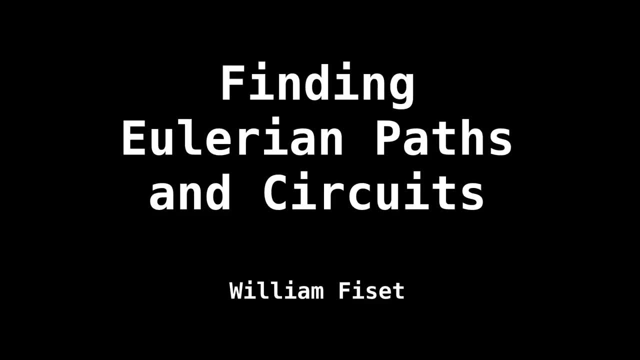 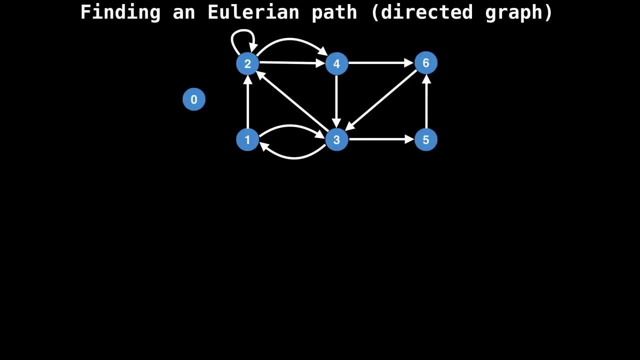 about how to algorithmically find Euler and paths and circuits on graphs. So finding Euler and paths and Euler and circuits are actually very similar problems for both directed and undirected graphs. If you have an algorithm that finds an Euler and path, finding an Euler and circuit comes for free. 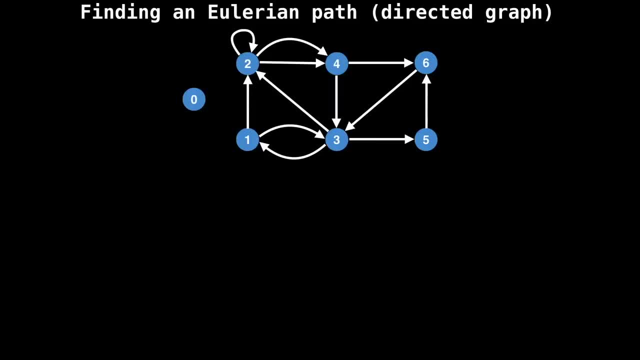 What you do is feed the graph with the Euler and circuit into the Euler and path algorithm and outcomes the Euler and circuit. For that reason, today we'll be looking at an algorithm that finds an Euler and path on a directed graph. So the first step to finding an Euler 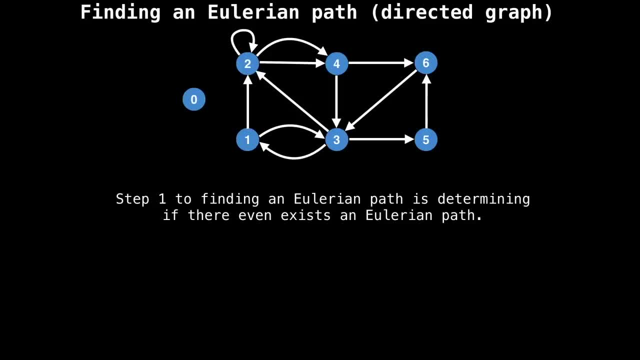 and path is to verify that one exists, because maybe it's impossible to find an Euler and path that traverses all the edges of your graph, And it's good to know that before you actually find your Euler and path. So recall that for an Euler and path to exist, at most one vertex. 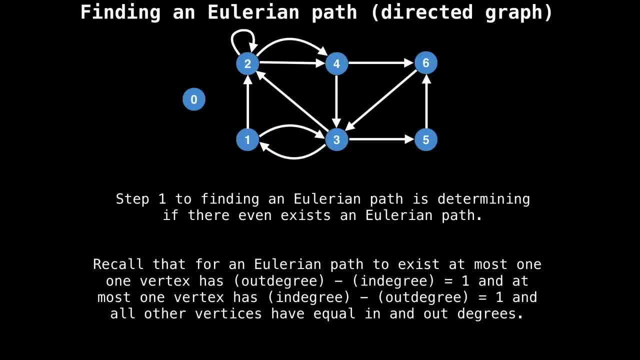 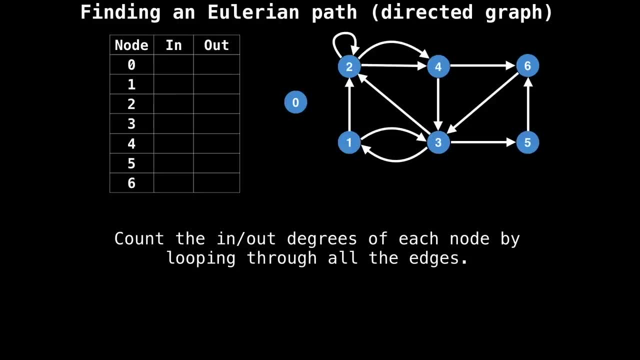 has out degree minus n degree equal to one, and at most one vertex has in degree minus out degree equal to one, and all other vertices have equal in and out degrees. we're going to count the in and out degrees of each node by looping through all the edges. we'll be 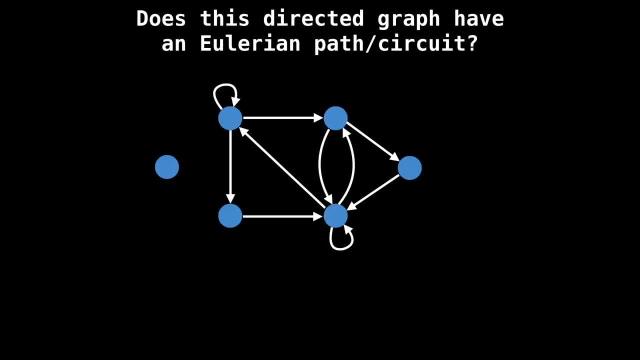 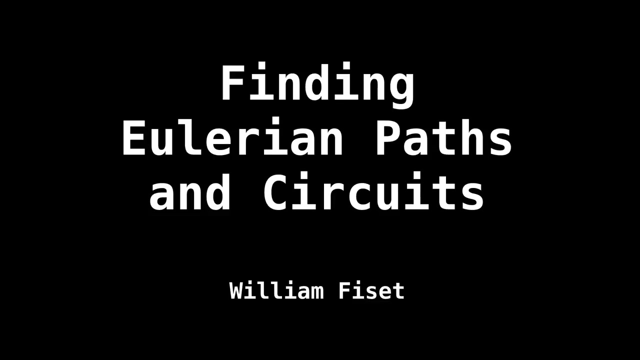 more time because there are a lot of edges. This graph only has an Eulerian path, but no Eulerian circuit. It also has a unique start and end node for the path. Note that the singleton node has no incoming or outgoing edges, So it doesn't impact whether or not we have an Eulerian path. Today we're talking about how. 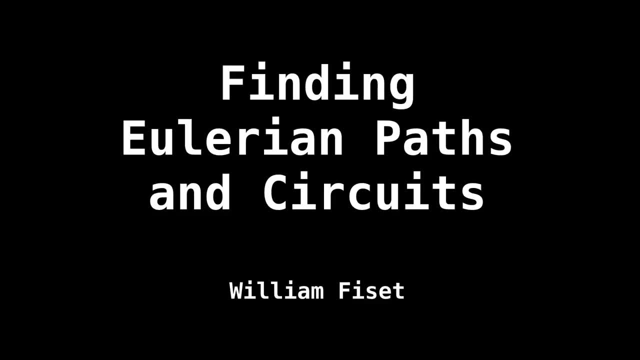 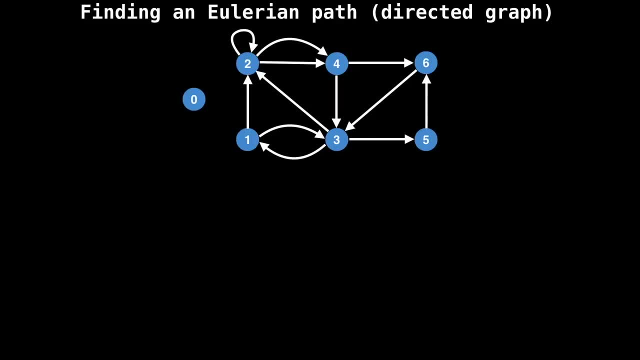 to algorithmically find Eulerian paths and circuits on graphs. So finding Eulerian paths and Eulerian circuits are actually very similar problems for both directed and undirected graphs. If you have an algorithm that finds an Eulerian path, finding an Eulerian circuit comes for free. 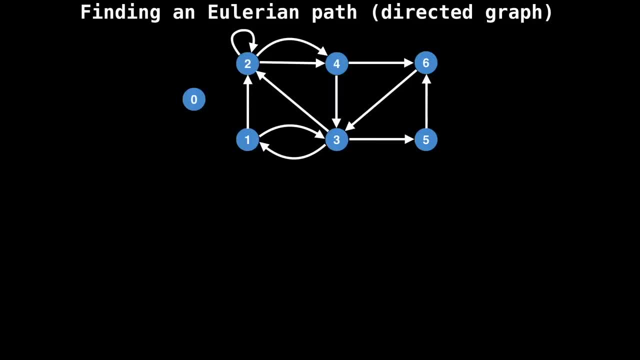 So what you do is feed the graph with the Eulerian circuit into the Eulerian path algorithm and outcomes the Eulerian circuit. For that reason, today we'll be looking at an algorithm that finds an Eulerian path on a directed graph. So the first step to finding an Eulerian path. 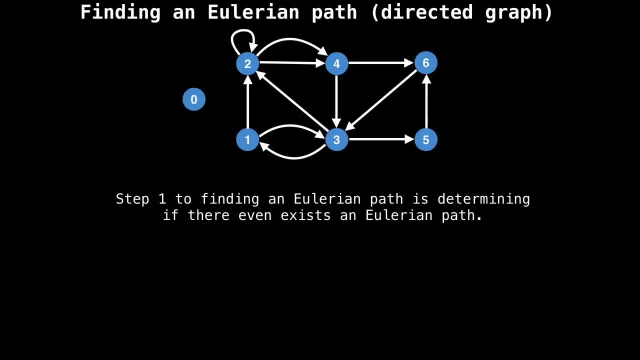 is to verify that one exists, because maybe it's impossible to find an Eulerian path that traverses all the edges of your graph, And it's good to know that before you actually find your Eulerian path. So recall that for an Eulerian path to exist, at most one vertex. 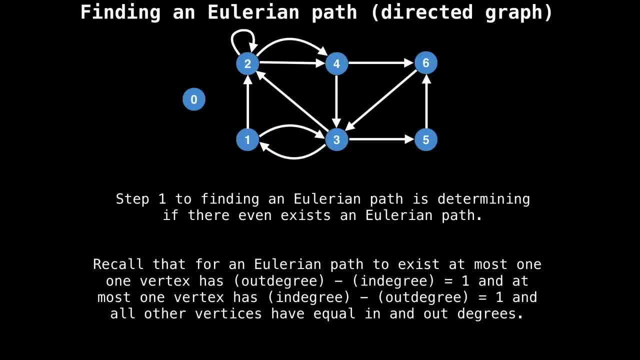 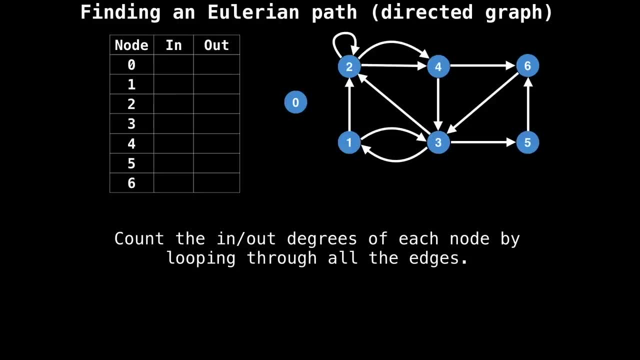 has out degree minus n degree equal to one, and at most one vertex has in degree minus out degree equal to one, and all other vertices have equal in and out degrees. we're going to count the in and out degrees of each node by looping through all the edges. we'll be 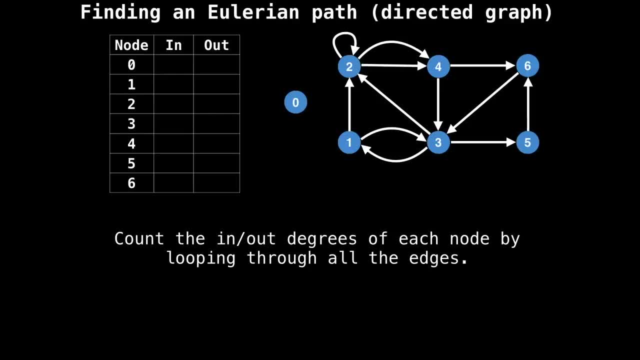 needing two arrays, which I've called in and out, to track the in and out degrees of each node. So, for each edge, increment the n degree of a node, If a node has an incoming edge, and increment the out degree if it has an outgoing edge. 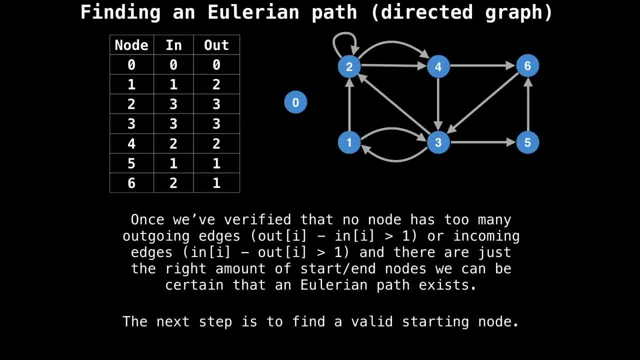 and so on for all the other edges. Once we verified that no node has too many outgoing edges or too many incoming edges, Unless the reference from that debit address looks like to have an in and out, We don't worth to check that we don't type means entry and then just paste the part double selected. 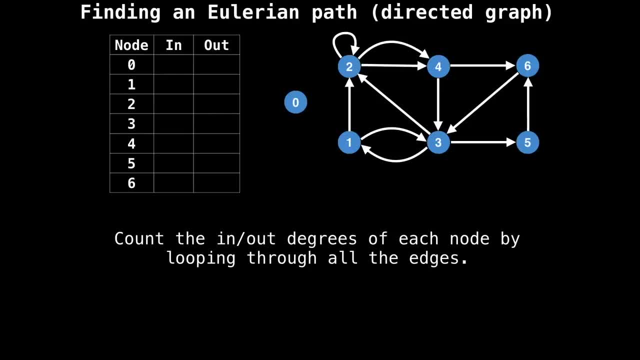 needing two arrays, which I've called in and out, to track the in and out degrees of each node. So, for each edge, increment the in degree of a node if a node has an incoming edge, and increment the out degree if it has an outgoing edge. 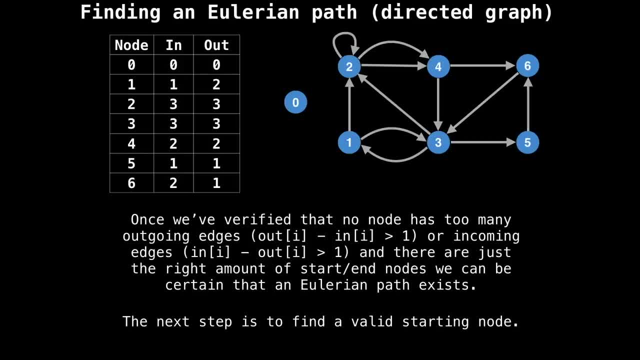 And so on for all the other edges. Once we've verified that no node has too many outgoing edges or too many In coming edges and there are just the right amount of start and end nodes, we can be certain that our Euler and path exists. The next step is to find a valid starting node, because we 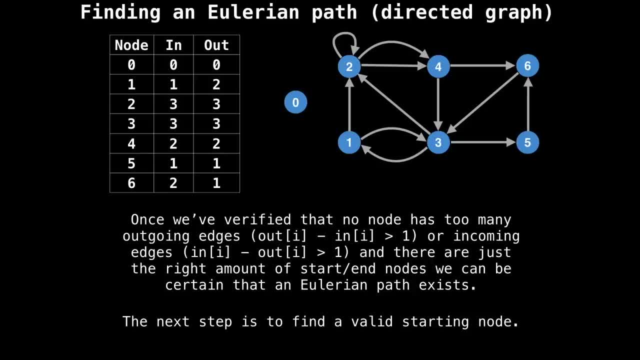 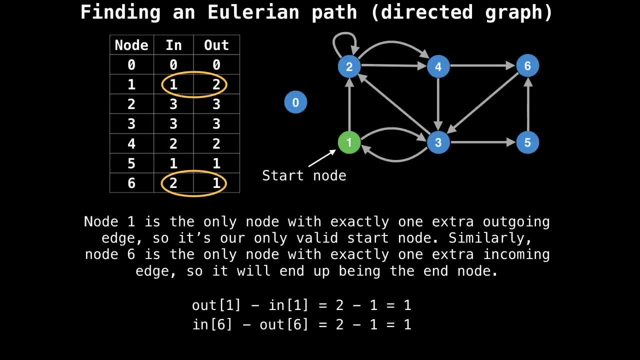 can't start the algorithm at any node we choose. necessarily, node one is the only node with exactly one extra outgoing edge, So it's our only valid start node. Similarly, node six is the only node with exactly one extra incoming edge, So it will end up being our ended node. Note that if all in and out, 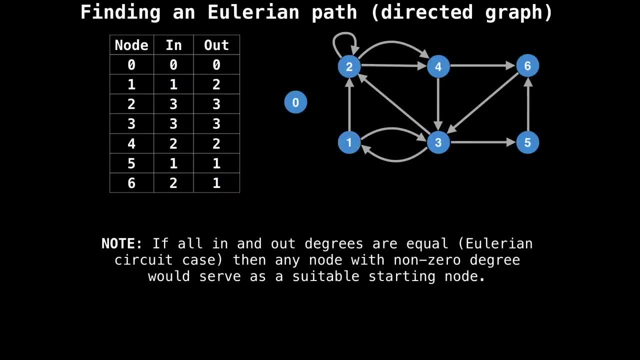 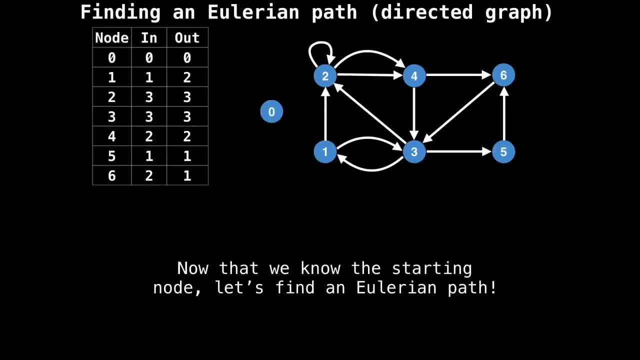 degrees are equal, then we have an Eulerian circuit And we can choose to start the algorithm at any node which has a non zero degree. So we have everything we need to find an Eulerian path. Let's see what happens if we try and do a naive depth for search to traverse as 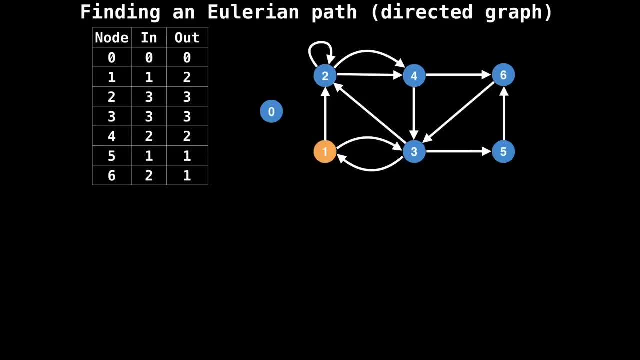 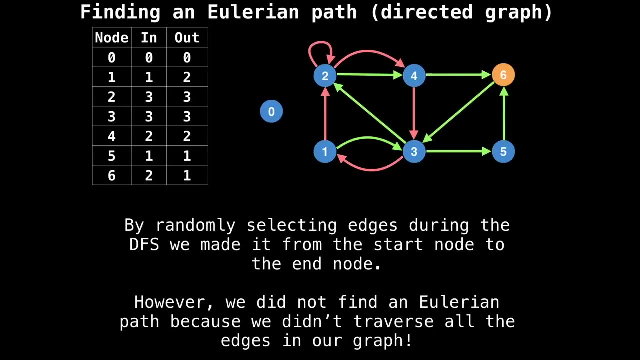 many edges as possible until we get stuck. Let's begin at our starting node and execute a random depth for search. Let's take a right, another right up, down, diagonally, up, diagonally, right and right Again. you'll notice that 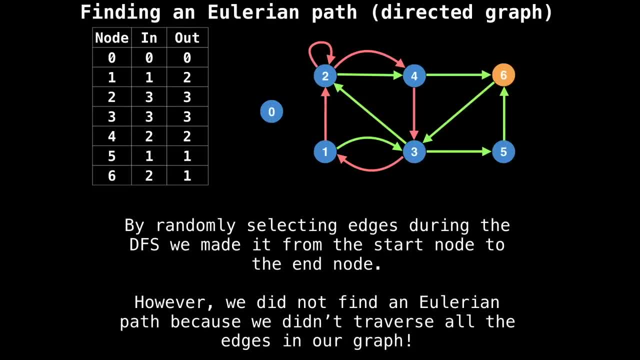 even though we started at the correct starting node and that we knew an Eulerian path existed and, furthermore, that we did end up at the correct end node, that we still did not find a valid Eulerian path Since we didn't traverse all the edges. So what's going on? Well, what's happening is: 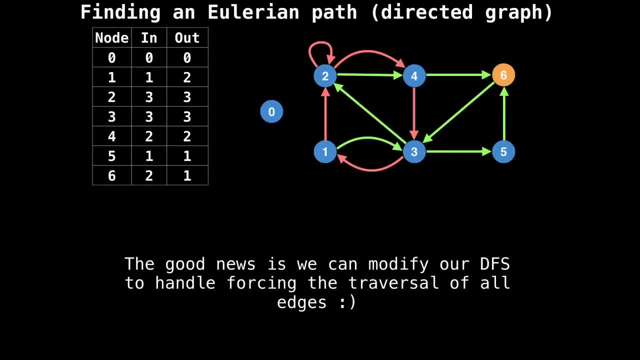 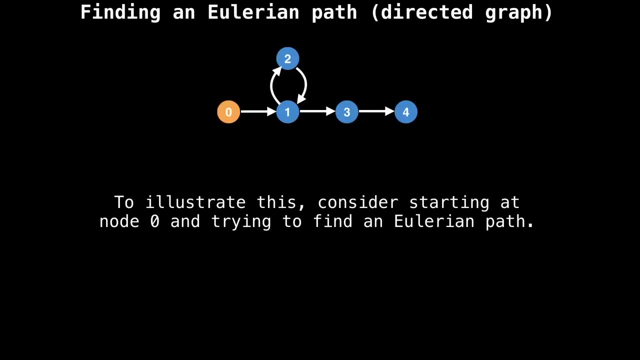 that we're doing our depth first search wrong. we need to modify the depth first search algorithm to force the depth first search to visit all the edges of our graph. To illustrate this, consider this simpler, smaller graph. Suppose we start our depth first search at node zero. 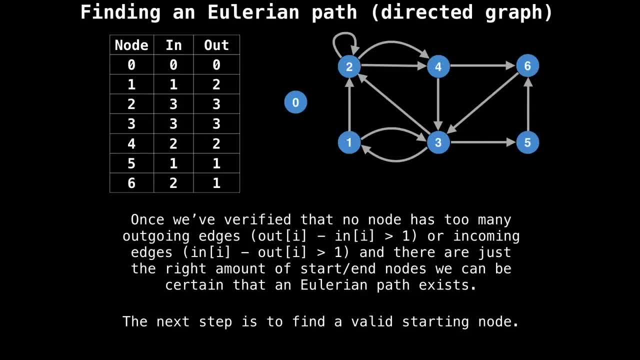 in output, So each square always has one in and out, but definitely you'll only find an нее edges and there are just the right amount of start and end nodes. we can be certain that our oilerian path exists. The next step is to find a valid starting node, because we 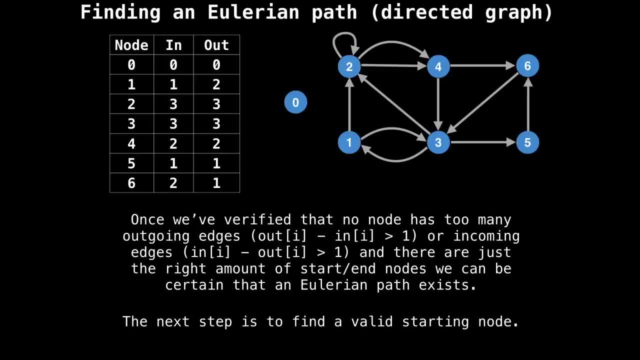 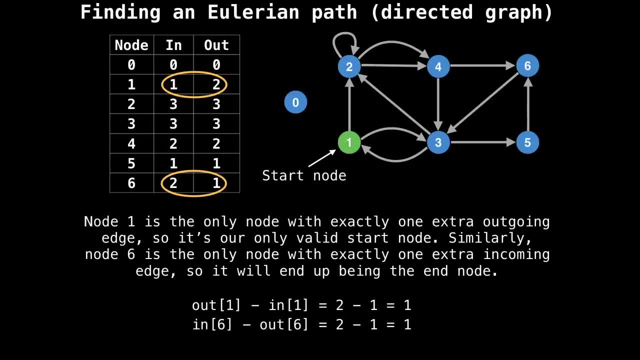 can't start the algorithm at any node we choose. necessarily, Node one is the only node with exactly one extra outgoing edge, So it's our only valid start node. Similarly, node six is the only node with exactly one extra incoming edge, So it will end up being our ended node. 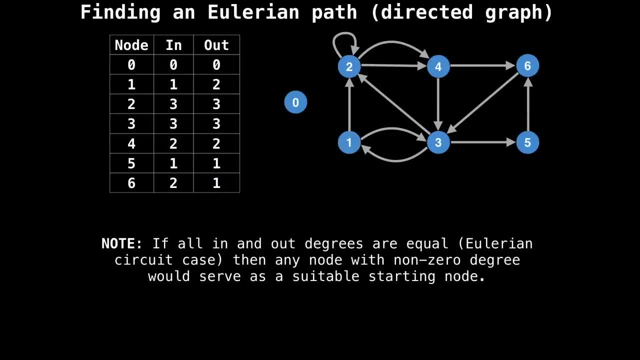 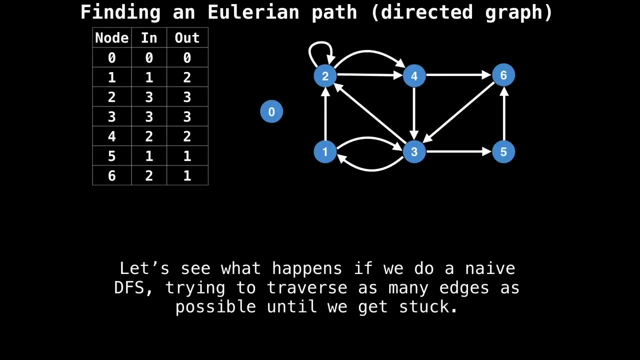 Note that if all in and out degrees are equal, then we have an oilerian circuit And we can choose to start the algorithm at any node which has a non zero degree. So we have everything we need to find an oilerian path. Let's see what happens if we try and do a naive depth. 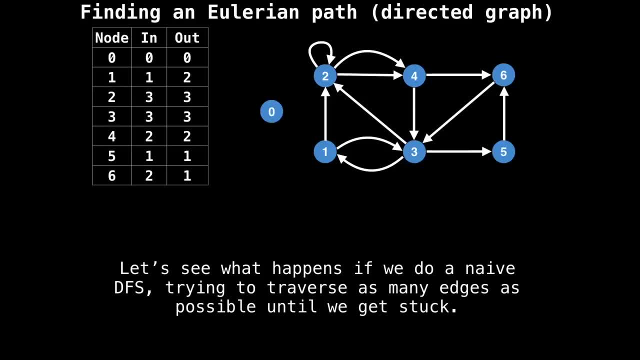 for search to traverse As many edges as possible until we get stuck. Let's begin at our starting node and execute a random depth for search. Let's take a right, another right up down, diagonally up, diagonally right and right. again, you'll notice that, even though we started at the correct starting, 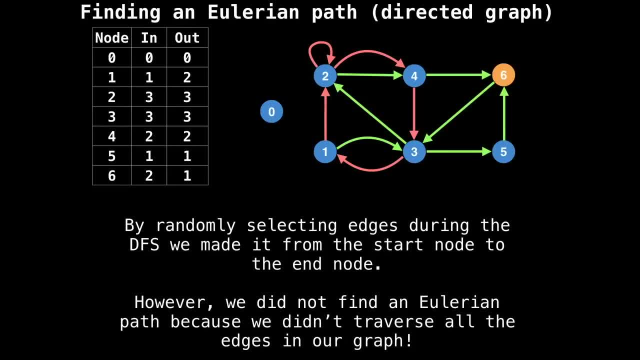 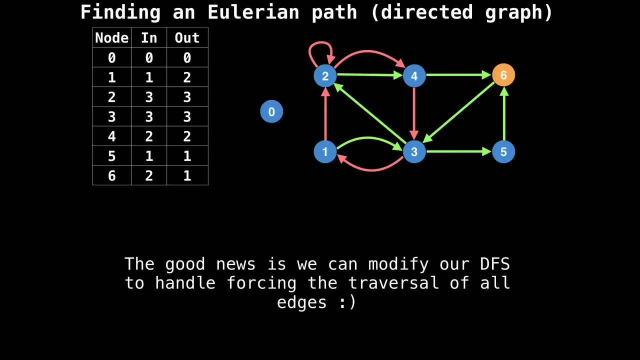 node and that we knew an oilerian path existed and, furthermore, that we did end up at the correct end node, still did not find a valid Eulerian path, since we didn't traverse all the edges. So what's going on? Well, what's happening is that we're doing our depth first search wrong. we need 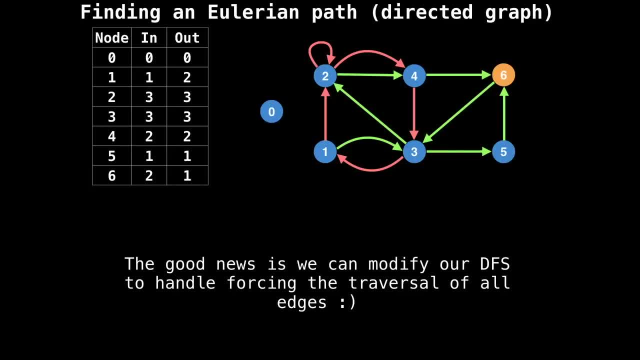 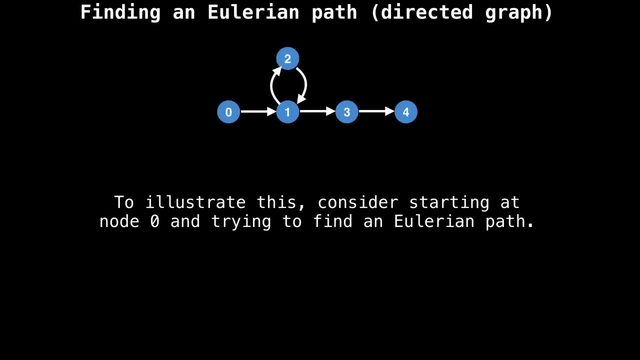 to modify the depth first search algorithm to force the depth first search to visit all the edges of our graph. To illustrate this, consider this simpler, smaller graph: Suppose we start our depth first search at node zero and try to find an Eulerian path. Suppose 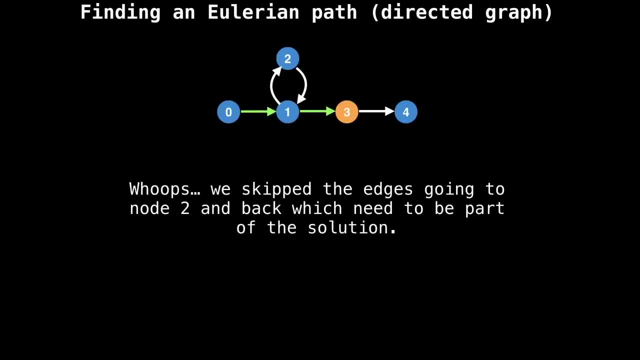 we take the edge to the right, then suppose the depth first search takes us right again. this causes us to accidentally skip the edges going to node two and back, which we know will need to be part of the Eulerian path solution. For now, let's not worry about it and keep. 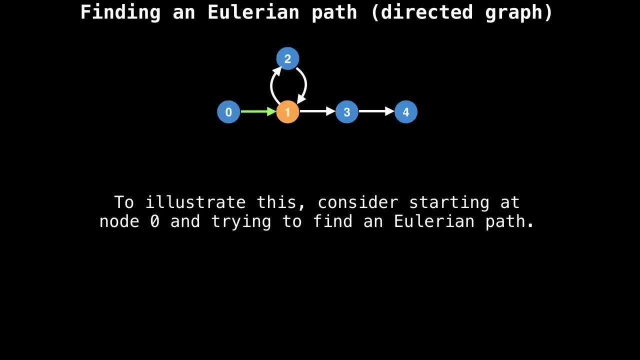 and try to find an Eulerian path. Suppose we take the edge to the right. Then suppose the depth first search takes us right again. this causes us to accidentally skip the edges, going to node two and back, which we know will need to be part of the 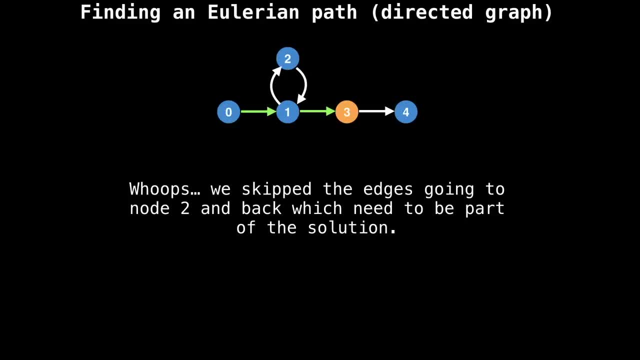 Eulerian path solution. For now let's not worry about it and keep executing our depth first search. So once we get stuck, meaning the current node has no unvisited outgoing edges, we backtrack and add the current node to the solution. So four gets added to the 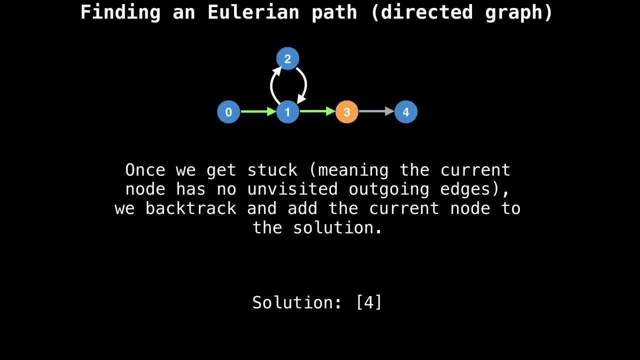 solution And we get backtracked to the solution. And we get backtracked to the solution And we return to the node we were just at. we are stuck again because node three has no outgoing edges that are unvisited. So we add three to the front of the solution and backtrack. 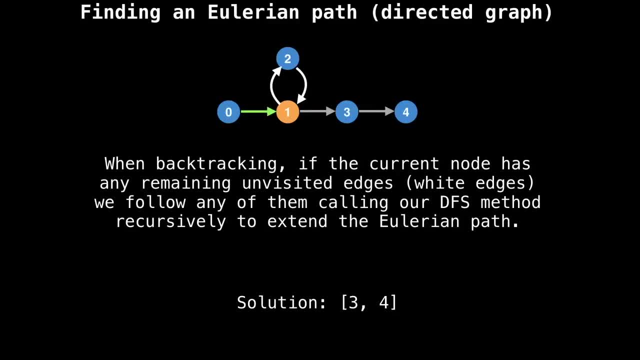 When backtracking, if the current node has any remaining unvisited edges, that is white edges, we follow any of them, calling our depth first search method recursively to extend the Eulerian path. So we follow the edge up to node two, and then there's still another. 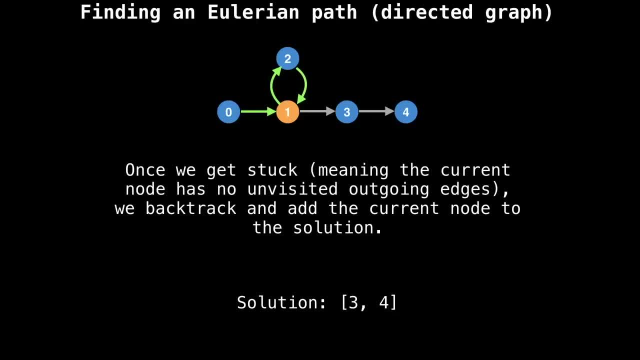 edge going downward. So we take that one too. Now we're stuck again because there aren't any unvisited edges anymore. What we do is we backtrack and add the current node to the front of the solution. Effectively, we do this until we return to the start node and the recursion unwinds. So in summary, 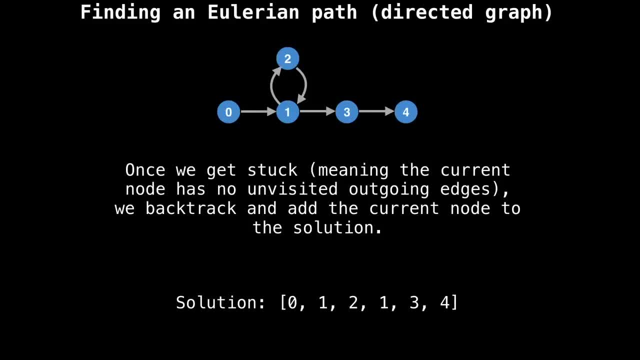 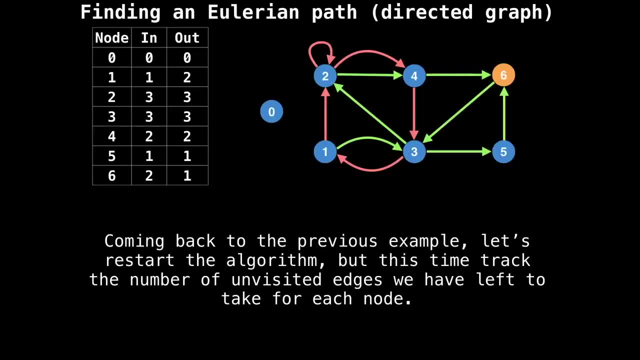 how we force the depth first search to take all the edges is to keep taking unvisited edges on the recursive callback until no unvisited edges Remain. coming back to the previous example, Let's restart the algorithm, But this time let's track the number of unvisited edges we still have left to take at each node In. 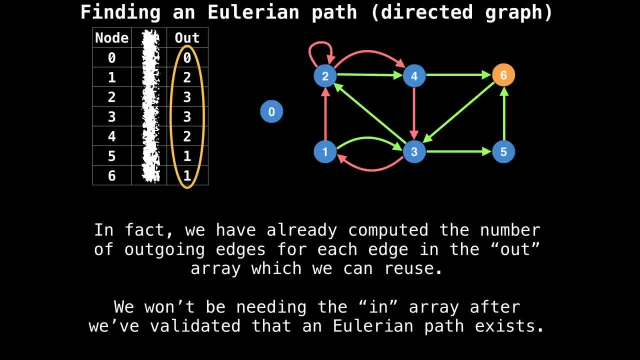 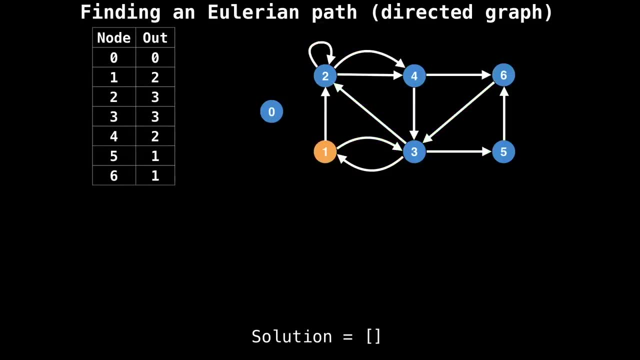 fact, we have already computed the number of outgoing edges for each node in the out array, which we can reuse. we won't be needing the inner array anymore once we validated that an Eulerian path exists, so we can ignore it. Let's begin at the starting node. 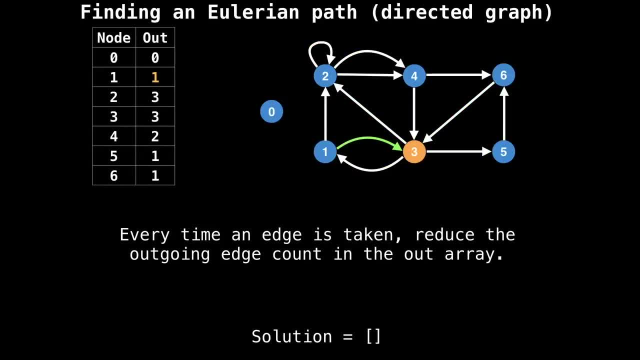 Once again. now, one thing we're going to do slightly differently is that every time an edge is taken, we'll reduce the outgoing edge count for that node. Doing this will enable us to know when a certain node has no more unvisited edges. So let's just follow. 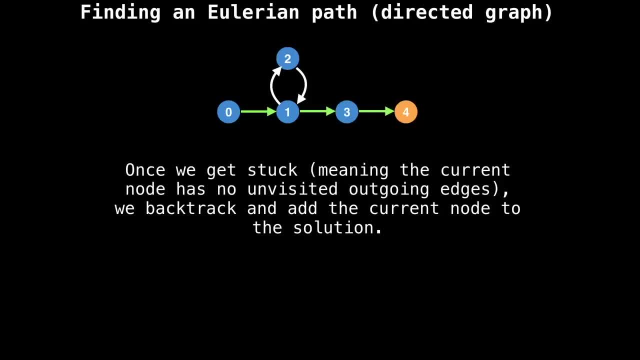 executing our depth first search. So once we get stuck- meaning the current node has no unveiling visited outgoing edges- we backtrack and add the current node to the solution. So four gets added to the solution and we return to the node we were just at. we are stuck again. 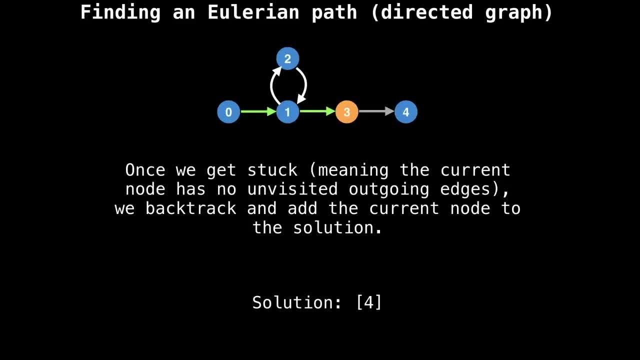 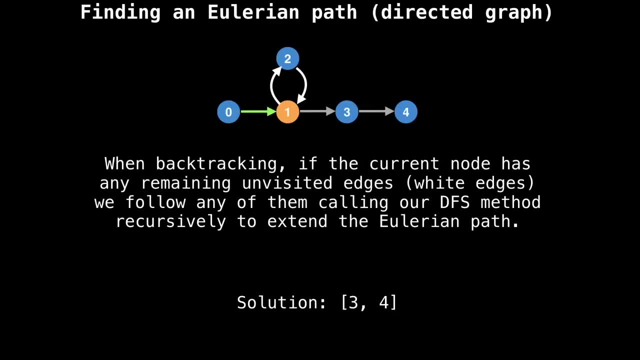 because node three has no outgoing edges that are unvisited. So we add three to the front of the solution and backtrack. When backtracking, if the current node has any remaining unvisited edges- that is, white edges- we follow any of them, calling our depth first search method. 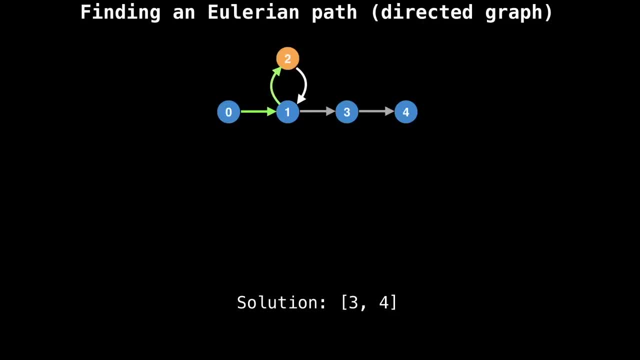 recursively to extend the Eulerian path. So we follow the edge up to node two, and then there's still another edge going downwards, So we take that one too. Now we're stuck again because there aren't any unvisited edges anymore. What we do is we backtrack and add the current. 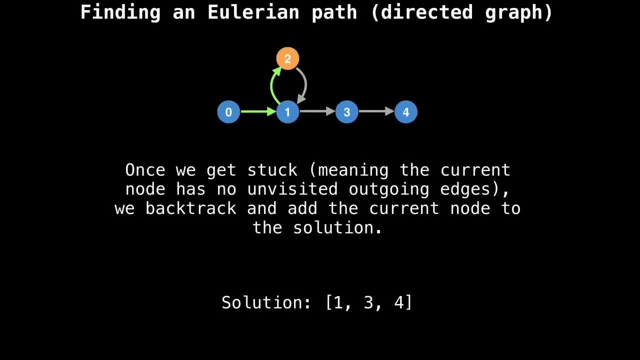 node to the front of the solution. Effectively, we do this until we return to the start node and the recursion unwinds. So, in summary, how we force the depth first search method- depth first search- to take all the edges is to keep taking unvisited edges on the recursive. 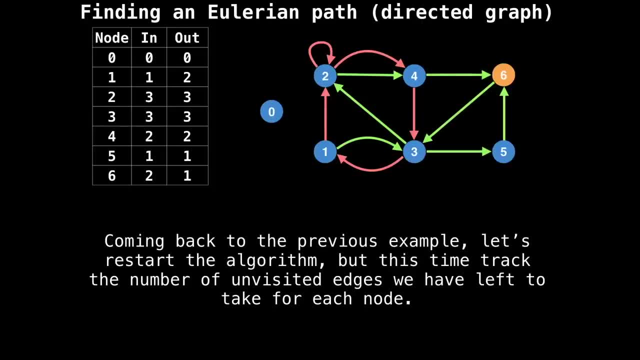 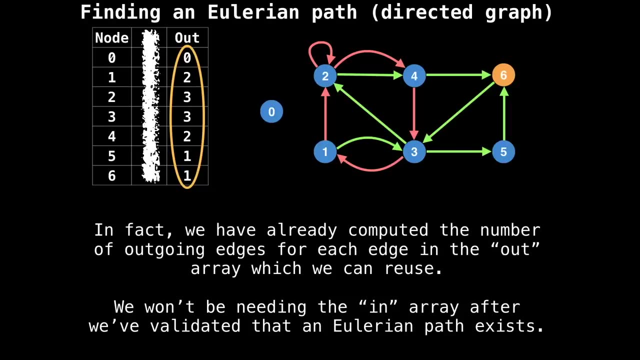 callback until no unvisited edges remain. Coming back to the previous example, let's restart the algorithm, But this time let's track the number of unvisited edges we still have left to take at each node. In fact, we have already computed the number of outgoing. 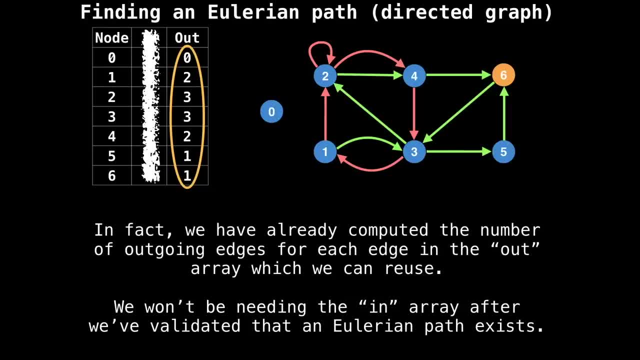 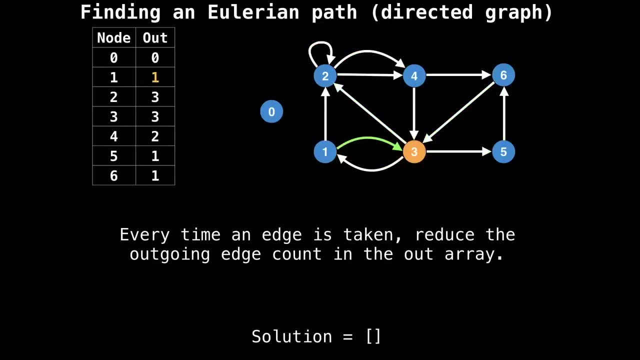 edges for each node in the out array, which we can reuse. we won't be needing the in array anymore once we validated that an Eulerian path exists, so we can ignore it. Let's begin at the starting node once again. Now one thing we're going to do slightly differently. 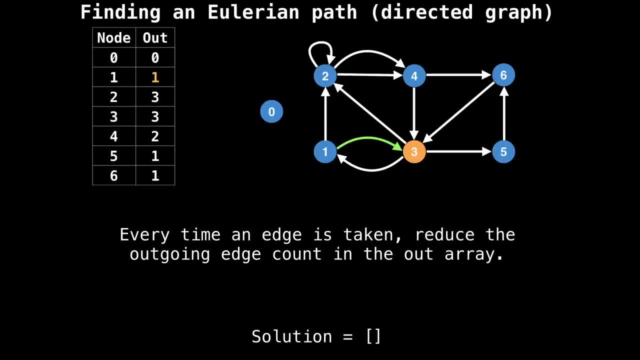 is that every time an edge is taken, we'll reduce the outgoing edge count for that node. Doing this will enable us to know when a certain node has no more unvisited edges. So let's just follow the same path we had last time until we get stuck. 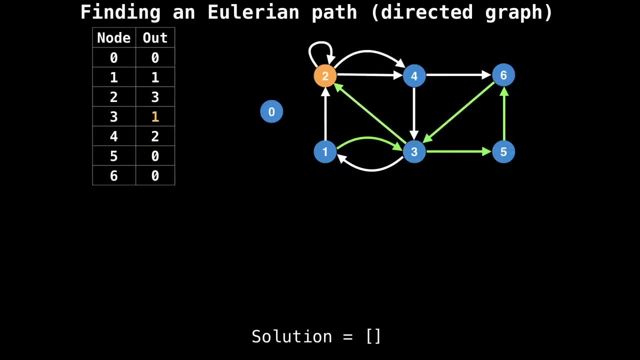 So let's just follow the same path we had last time until we get stuck. So let's just follow the same path we had last time until we get stuck. So now we are where we were last time, but we're not going to terminate the algorithm. 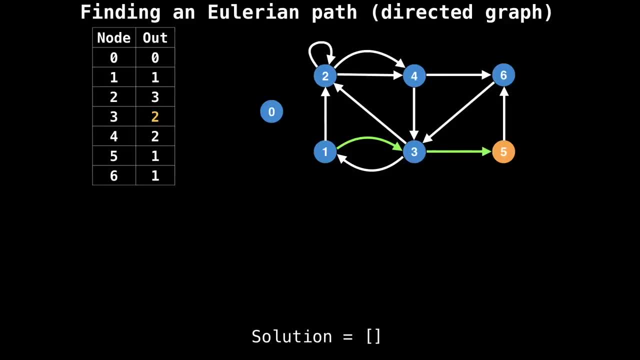 the same path we had last time until we get stuck. So now we are where we we were last time, but we're not going to terminate the algorithm just yet. Instead, we're going to backtrack because we're stuck and there are no more outgoing edges to take. 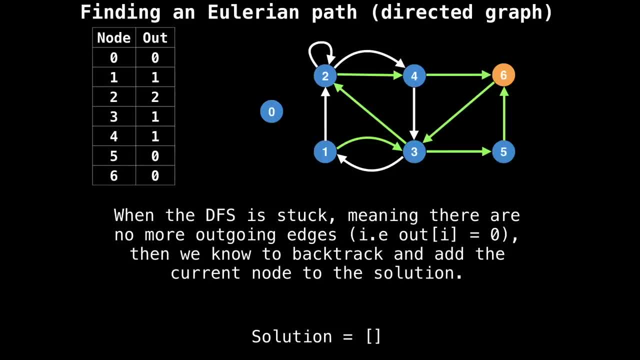 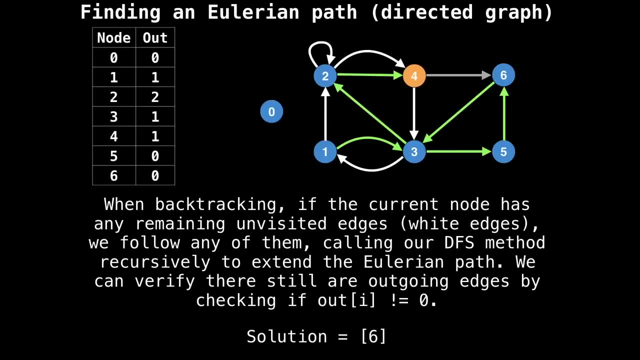 from node six. One way to know this without looking at the graph, is to check whether the out array at index six has a value of zero, and it does, So let's backtrack and add six to the front of our solution. Now we are at node four, and node four has remaining unvisited. 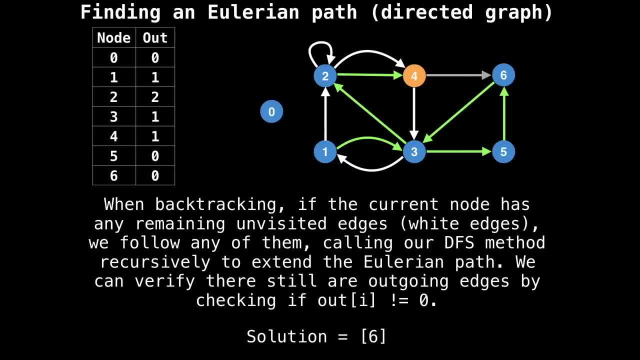 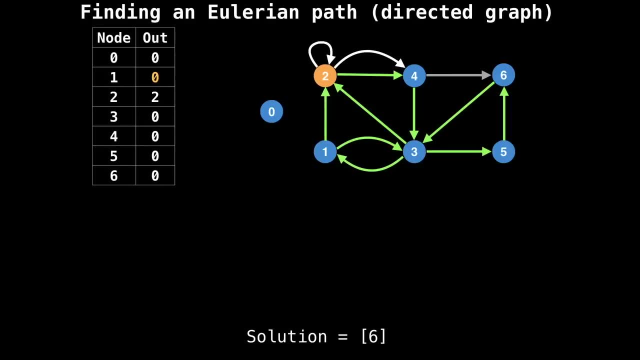 edges. those are the white edges which we still need to take. So we call our depth first search method recursively and follow all the unvisited edges. for node four, similar situation at node three and node one and node two. for node two we're going to take the edge. 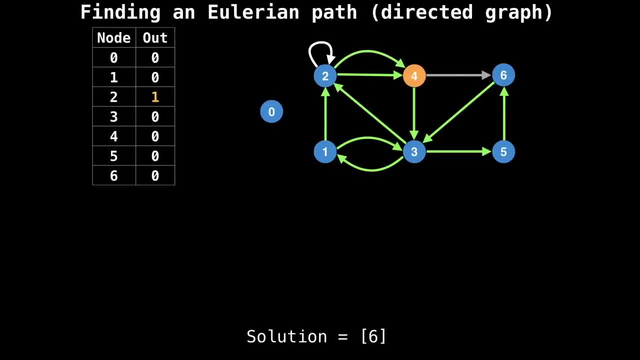 going to the right, which brings us back to node four, But this time there are no more unvisited edges at node four. So what do we do? we backtrack and add four to the front of our solution. Now we're at node two and no two still has. 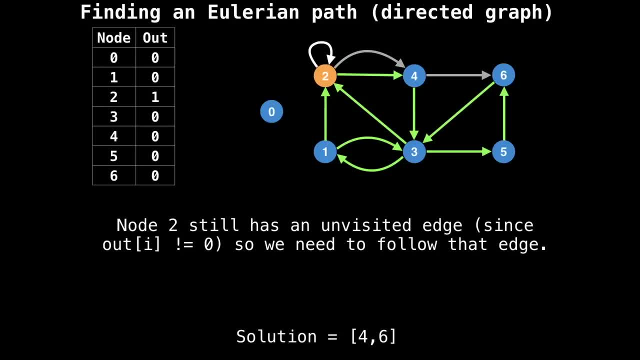 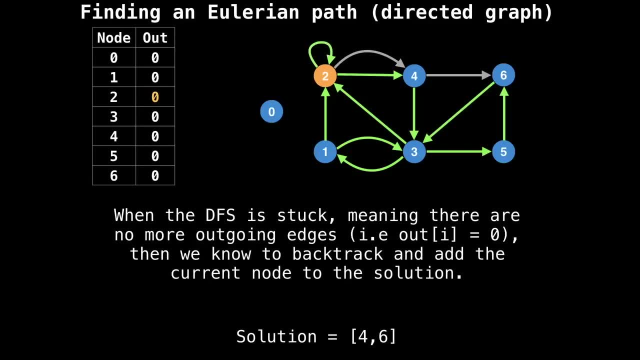 an unvisited edge, since the out array at index two is not equal to zero. So what we do is we follow that unvisited edge, which brings us back to node two, and node two now has no more unvisited edges. So we backtrack and add to the solution. 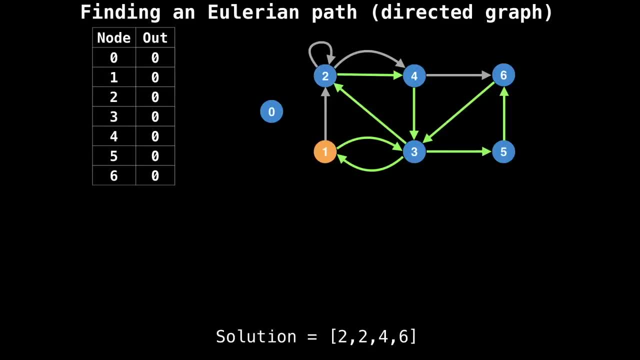 And we're back at node two and we backtrack- Now we're at node one, and backtrack from node one, Now we're at node three, and so on, since all the edges have been visited, And at this point we're just going to unwind the stack and add the current node to the 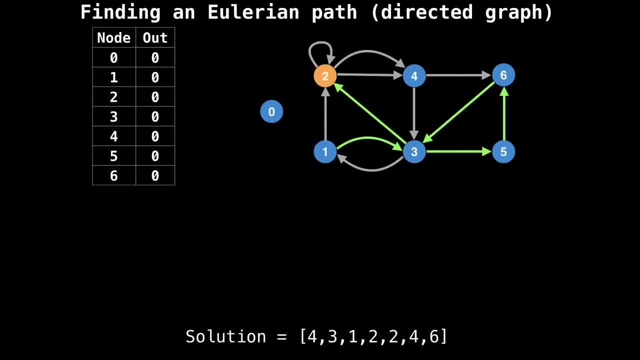 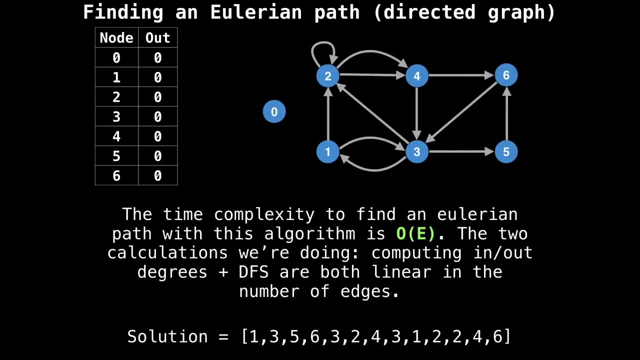 front of the solution. I'll let the animation play. And that's how you find an Eulerian path on a graph. In terms of the time complexity required to find an Eulerian path, we know that it has to be big O of E. The reason is that the calculations we're doing to compute the Eulerian path are 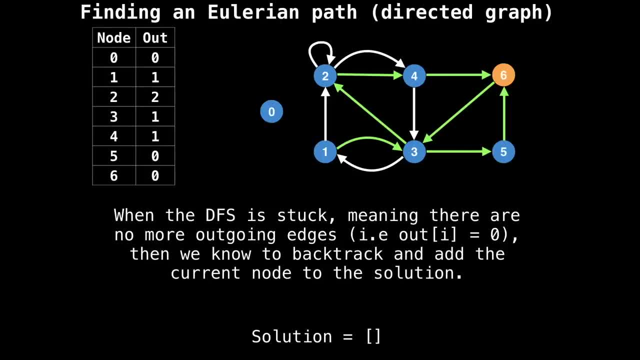 just yet. Instead, we're going to backtrack because we're stuck and there are no more outgoing edges to take from node six. One way to know this, without looking at the graph, is to check whether the out array at index six has a value of zero, and it does. So let's 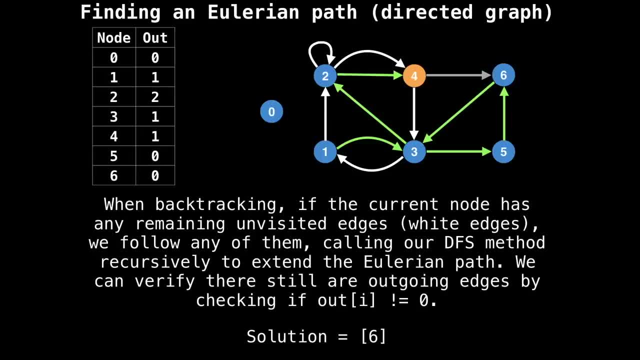 let's backtrack and add six to the front of our solution. Now we are at node four and node four has remaining on visited edges. Those are the white edges which we still need to take. So we call our depth first search method recursively and follow all the unvisited. 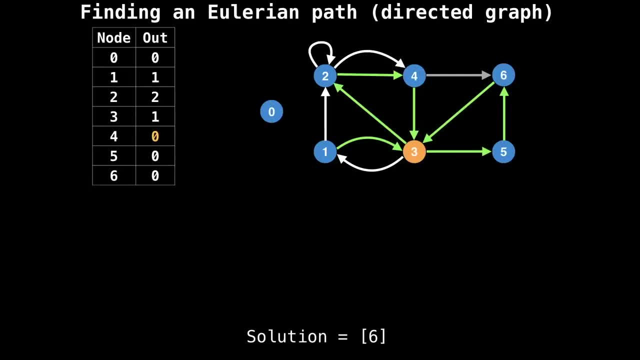 edges for node for similar situation at node three and node one And no two for node two. we're going to take the edge going to the right. living on the right will be myft for ria end. It's either on or over. on this example, people lot will notice that it's on when we're. 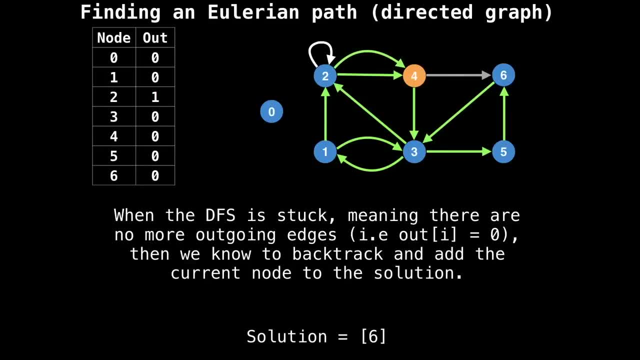 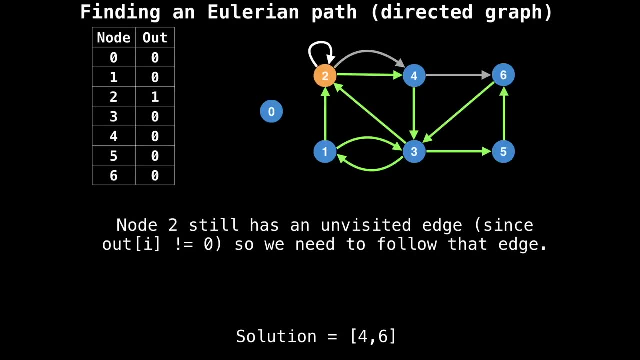 brings us back to node four, But this time there are no more unvisited edges at node four. So what do we do? we backtrack and add four to the front of our solution. Now we're at node two, and node two still has an unvisited edge, since the out array at index two is not. 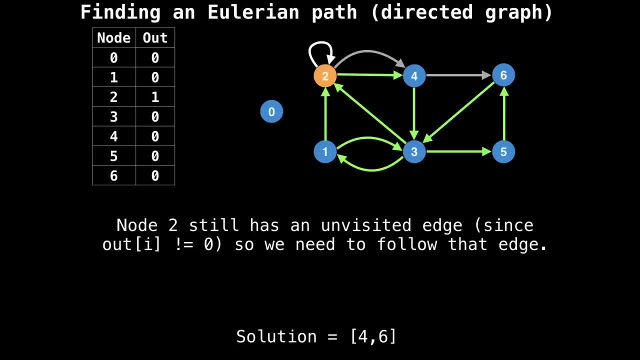 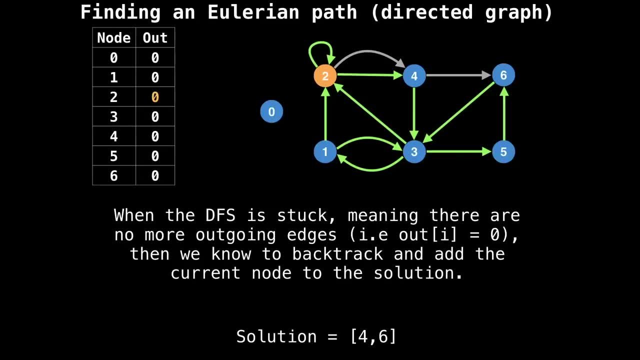 equal to zero. So what we do is we follow that unvisited edge which brings us back to node two, and node two now has no more unvisited edges. So we backtrack and add to the solution And we're back at node two and we backtrack. Now we're at node one and 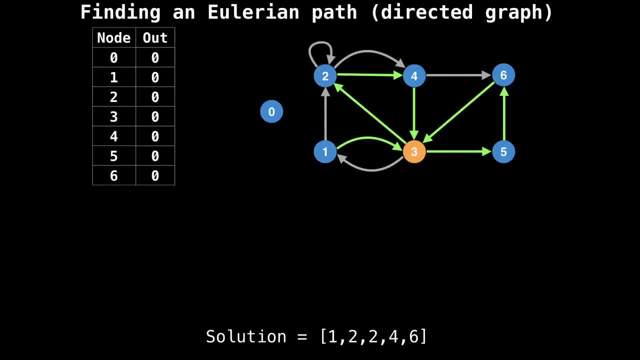 backtrack from node one, Now we're at node three and so on, since all the edges have been visited, And at this point we're just going to unwind the stack and add the current node to the front of the solution. I'll let the animation play. 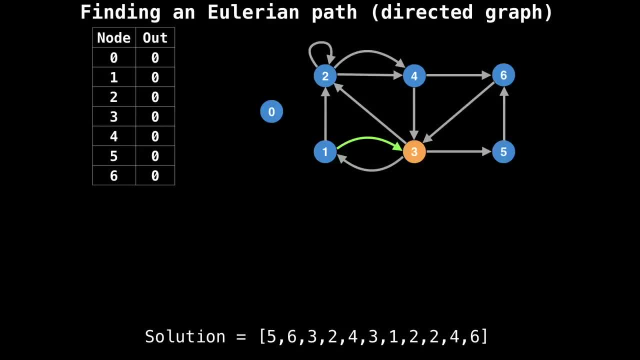 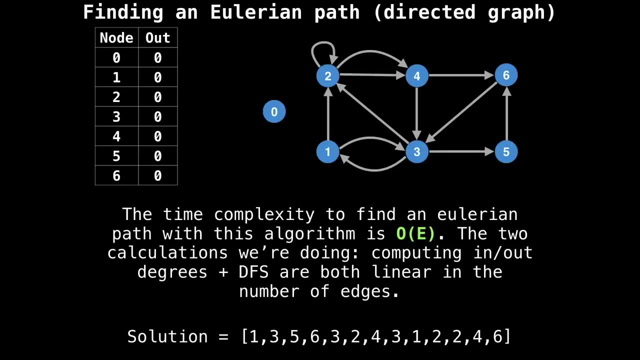 Okay, okay, and that's how you find an Eulerian path on a graph. In terms of the time complexity required to find an Eulerian path, we know that it has to be big O of E. The reason is that the calculations we're doing to compute the Eulerian path are all linear in the number. 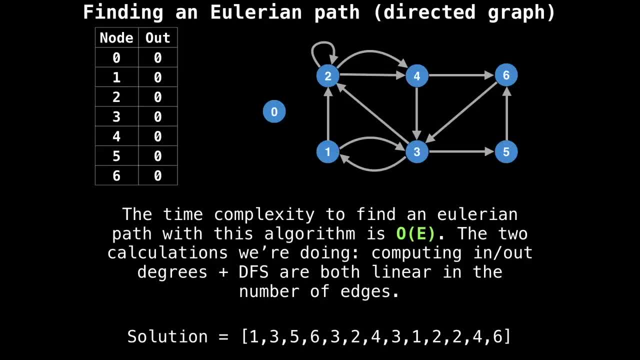 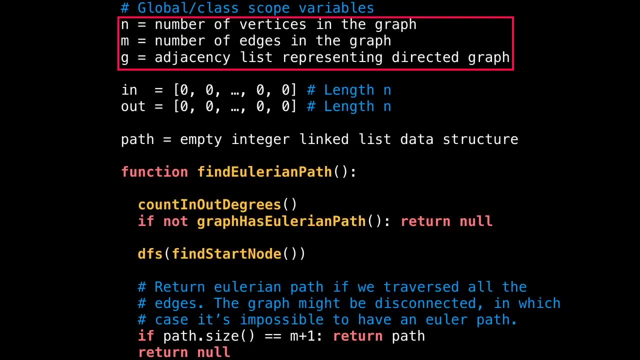 of edges. Think about computing the in and out degrees or the depth first search. both of those only take big O of E time. So the whole thing is linear in the number of edges. And now let's have a look at some pseudocode to find an Eulerian path. Let's have a look at some of the variables we're 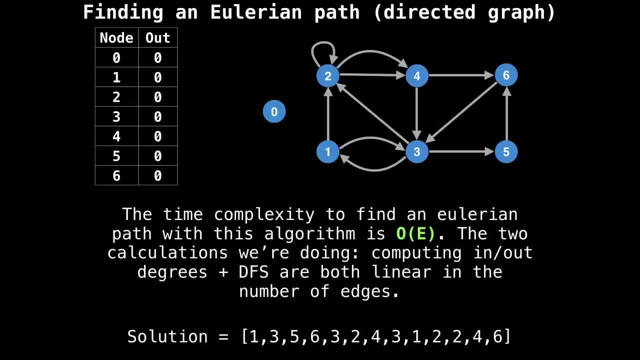 all linear in the number of edges. Think about computing the in and out degrees or the depth. first search. both of those only take big O of E time. So the whole thing is linear in the number of edges. And now let's have a look at some pseudocode. 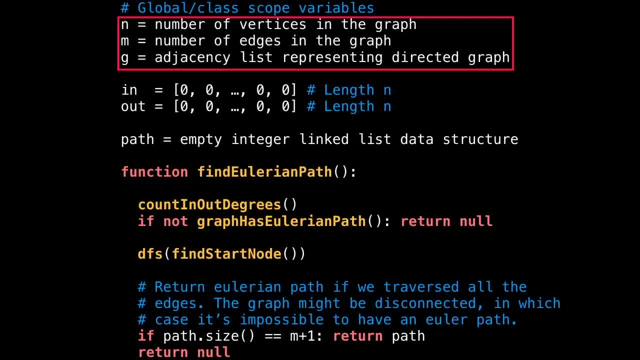 to find the Eulerian path. Let's have a look at some of the variables we're going to need. The first three here are inputs to the algorithm, which are: n- the number of nodes in the graph, m- the number of edges in the graph And, lastly, G, the graph itself stored as an adjacency list. 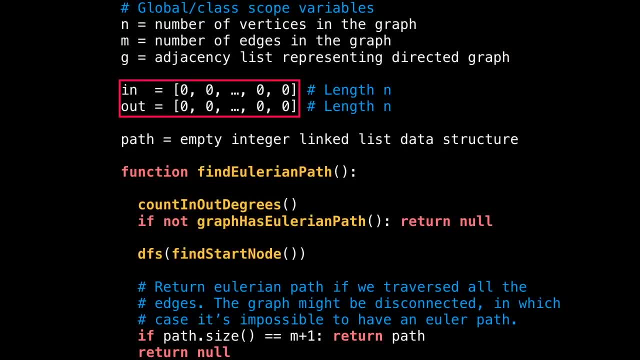 Then there's the in and out arrays I talked about earlier to track the in and out degrees of every node. Lastly, there's a variable called path, which is a linked list which is going to store the Eulerian path solution. You can also use an array or some other data structure to store. 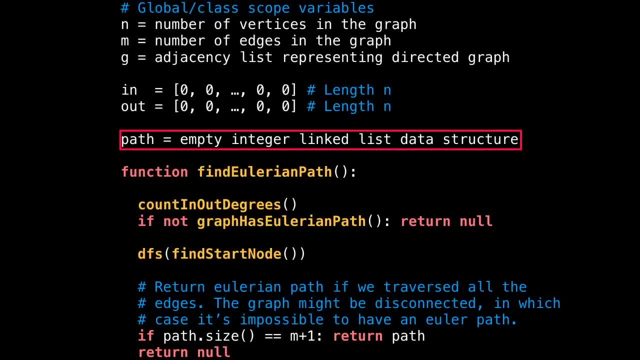 the solution, But I find that a linked list simplifies the code. to actually find an Eulerian path on our graph G, we're going to call the find Eulerian path method. The first thing we want to do is verify that the path is actually linked to the Eulerian path. So we're going. 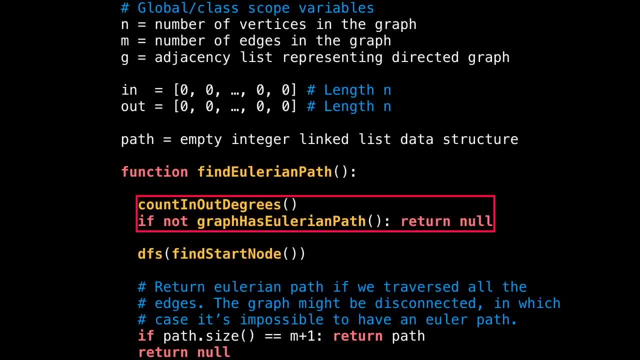 to verify that an Eulerian path exists. To do that, we first need to count the in and out degree of each node, And once we know that, we can verify that the graph is a good candidate for an Eulerian path. So here we are looking at the methods which count the 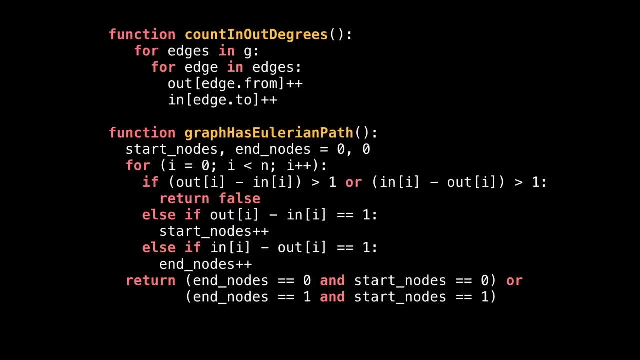 in and out degrees of each node and verifies that an Eulerian path can exist. The count in and out degrees method is very simple: simply loop over all the edges in the graph and increment the in and out degree arrays for incoming and outgoing edges. The graph has 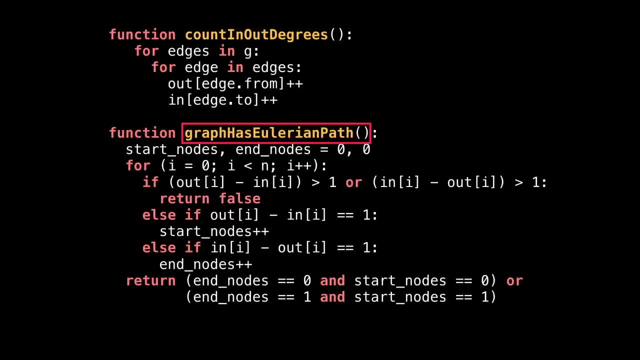 Eulerian path method checks all the preconditions for an Eulerian path. we're going to keep track of the number of start nodes and end nodes that we encounter. A start node is a node with one extra outgoing edge and an end node is a node with one extra incoming edge. 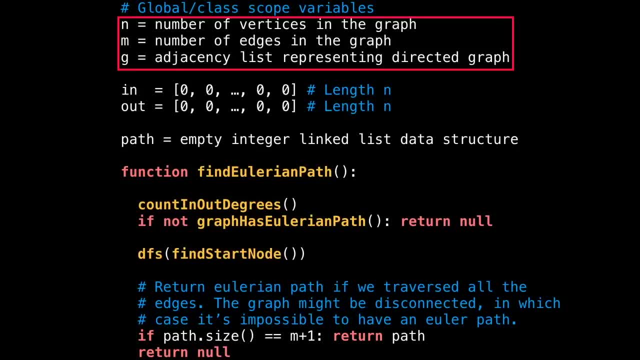 going to need The first three. here are inputs to the algorithm, which are: n- the number of nodes in the graph, m- the number of edges in the graph And, lastly, G- the graph itself stored as an adjacency list. 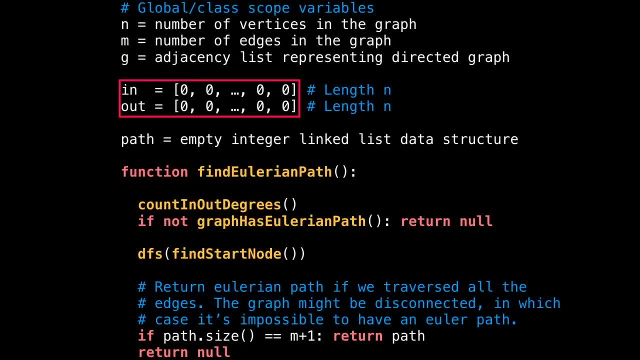 Then there's the in and out arrays I talked about earlier to track the in and out degrees of every node. Lastly, there's a variable called path, which is a linked list which is going to store the Eulerian path solution. You can also use an array or some other data. 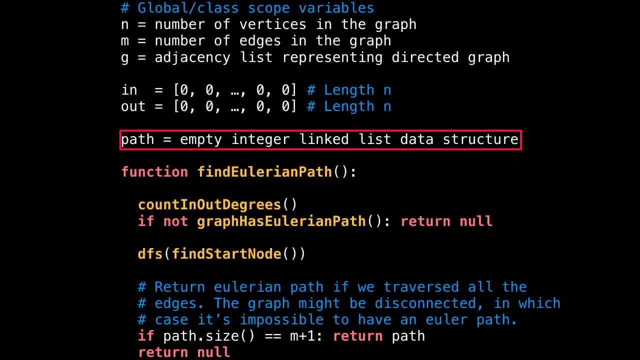 structure to store the solution. But I find that a linked list simplifies the code. to actually find an Eulerian path on our graph G, We're going to call the find Eulerian path method. The first thing we want to do is verify that an Eulerian path exists. To do that we first need to count the in and out degree. 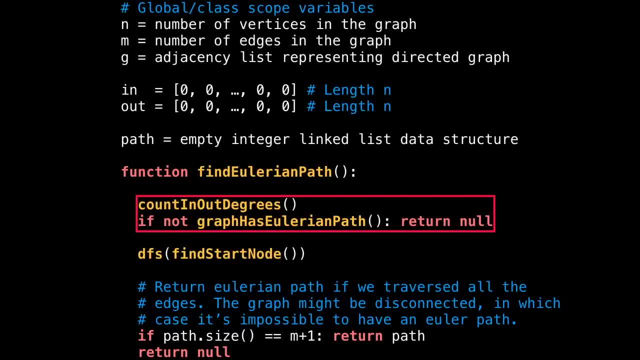 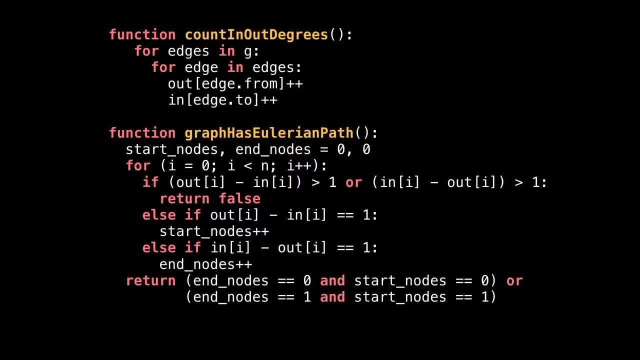 of each node And once we know that, we can verify that the graph is a good candidate for an Eulerian path. So here we are, looking at the methods which count the in and out degrees of each node and verifies that an Eulerian path can exist. The count in and 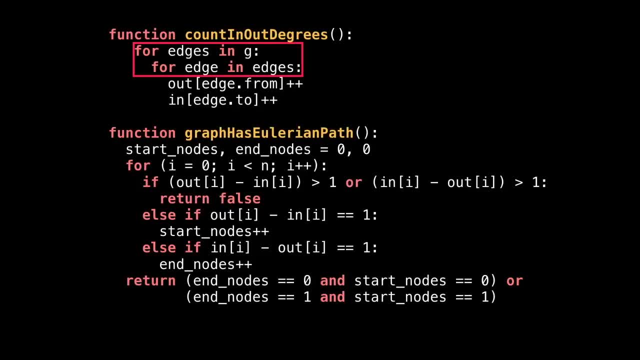 out degrees method is very simple. simply loop over all the edges in the graph and increment the in and out degree arrays for incoming and outgoing edges. The graph has Eulerian path method checks all the preconditions for an Eulerian path. we're going to keep track. 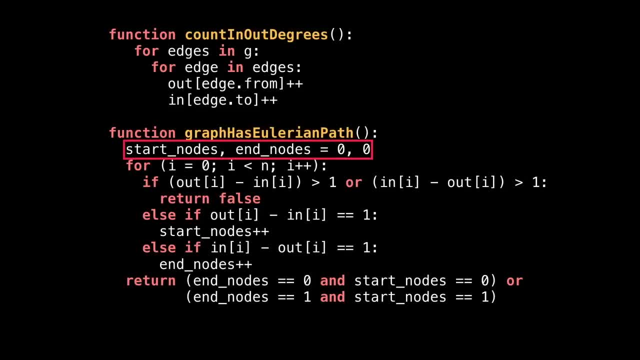 of the number of start nodes and end nodes that we encounter. A start node is a node with one extra outgoing edge and end nodes- An end node- is a node with one extra incoming edge. If, at any point, we encounter a node which either has more than one extra outgoing edge or more than one extra incoming edge, 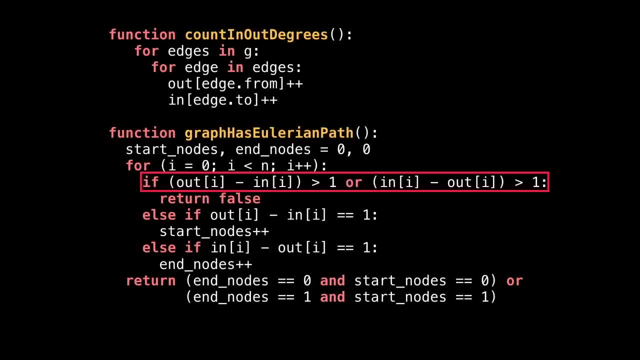 we know that this graph is not Eulerian And we can return false immediately Because of symmetry. I believe you only need one of these checks. But to be explicit, I put both conditions there. Next up, I check if the current node 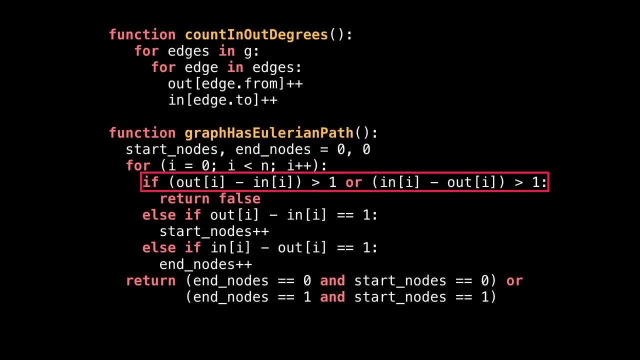 If at any point, we encounter an incoming edge, we're going to have to do the same thing with a counter node which either has more than one extra outgoing edge or more than one extra incoming edge. we know that this graph is not Eulerian And we can return false immediately. 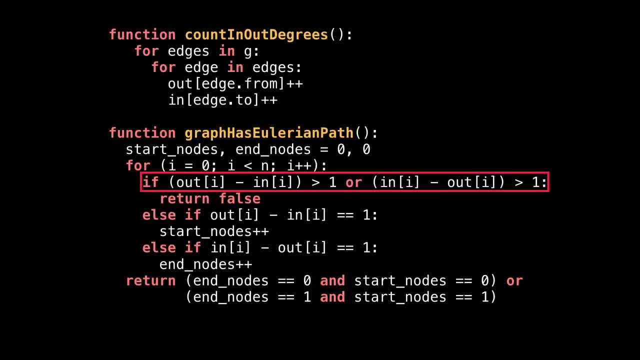 Because of symmetry, I believe you only need one of these checks. But to be explicit, I put both conditions there. Next up, I check if the current node is a start node or an end node. you cannot be a start node and an end node. 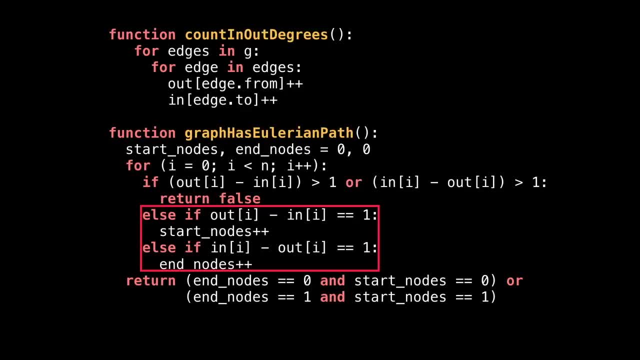 Which is why this is an else if clause. the last thing to do is check if we have a valid number of start nodes and end nodes for our path. Either there are no designated start and end nodes- that is the Eulerian circuit case, which is also an Eulerian path- or there 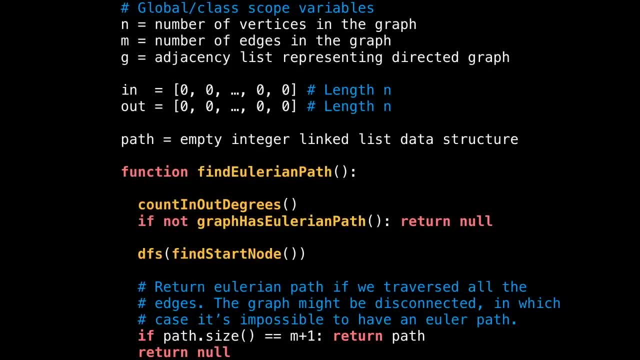 are exactly one start node and one end nodes. Coming back to the main method, the next step is to find that starting node and perform a depth first search To actually find the Eulerian path. Let's begin with finding the starting node. we're 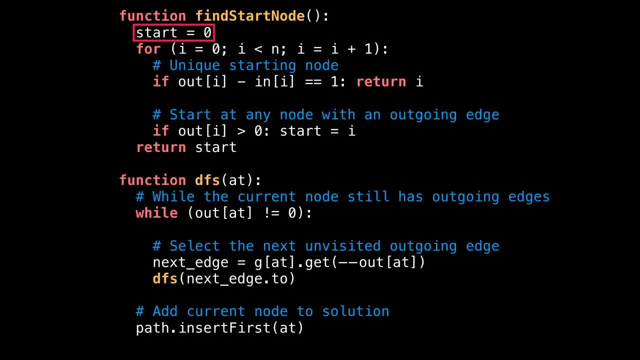 going to start by assuming that the start node is node zero, although this will likely change in the future, Since we know that at this point our graph is an Eulerian graph. This means that if we encounter a node with one extra outgoing edge, that this node must. 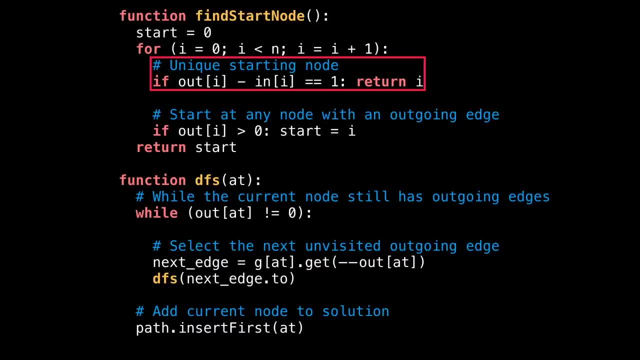 be the unique starting node and we can return that nodes index immediately. Otherwise, we just want to ensure that we begin on a node with an outgoing edge. our default node, node zero, might not have an outgoing edge. In fact, this check prevents us from starting. 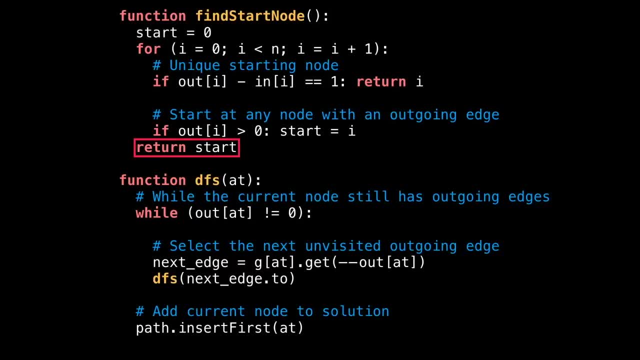 the depth first search on a singleton node, then return the start node after the loop. the depth first search method is where things start to get interesting. This depth first search method takes one argument, and that is the current node. we're at the while loop. 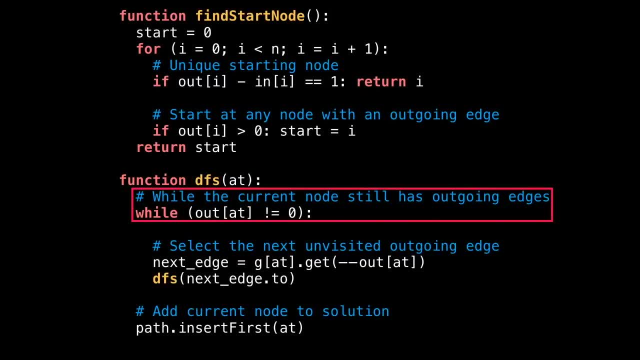 in the depth- The depth first search loops, while the current node still has outgoing unvisited edges. It does this by looking in the outer array at the current node and checking if there are still outgoing edges. The next line selects the next unvisited outgoing edge from the 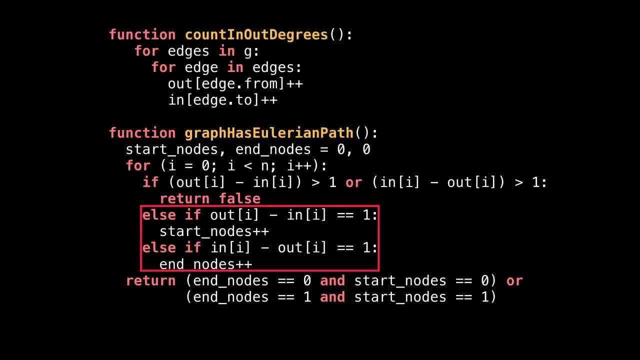 is a start node or an end node. you cannot be a start node and an end node, which is why this is an else if clause. The last thing to do is check if we have a valid number of start nodes and end nodes for our path. Either there are no designated start and end nodes. 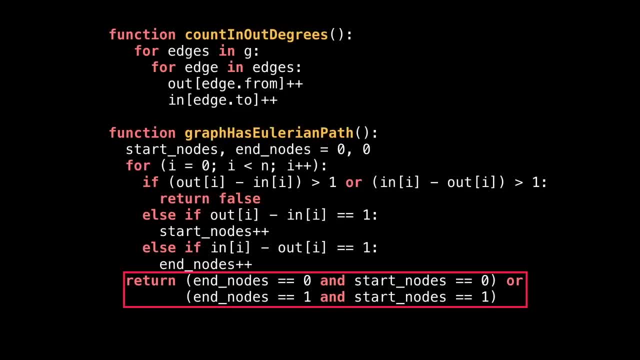 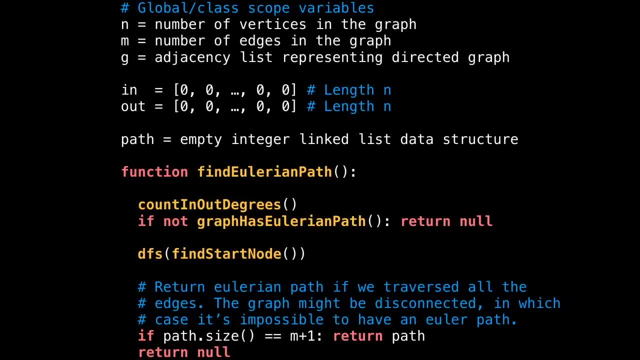 that is the Eulerian circuit case, which is also an Eulerian path, or there are exactly one start node and one end nodes. Coming back to the main method, the next step is to find that starting node and perform a depth first search to actually find the Eulerian path. Let's begin with finding the starting node. we're 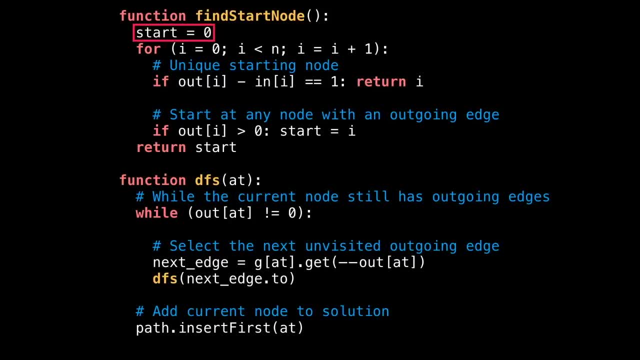 going to start by assuming that the start node is node zero, although this will likely change in the future, Since we know that at this point our graph is an Eulerian graph. This means that if we encounter a node with one extra outgoing edge, that this node must. 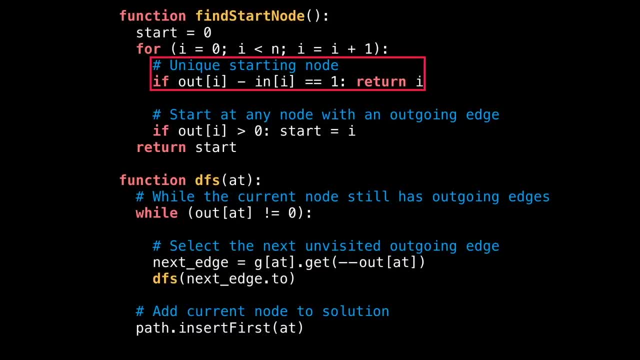 be the unique starting node and we can return that nodes index immediately. Otherwise, we just want to ensure that we begin on a node with an outgoing edge. our default node, node zero, might not have an outgoing edge. In fact, this check prevents us from starting the depth. 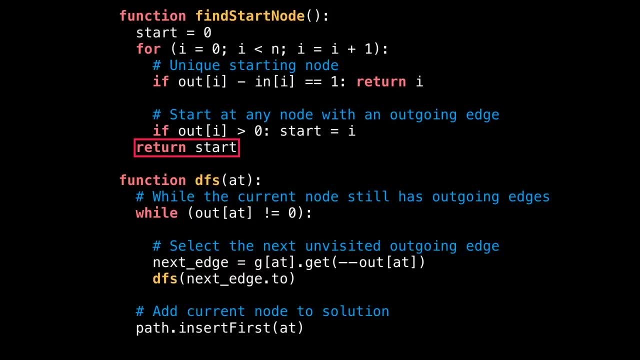 first search on a singleton node, then return the start node after the loop. the depth first search method is where things start to get interesting. This depth first search method takes one argument, and that is the current node. we're at the while loop in the depth. 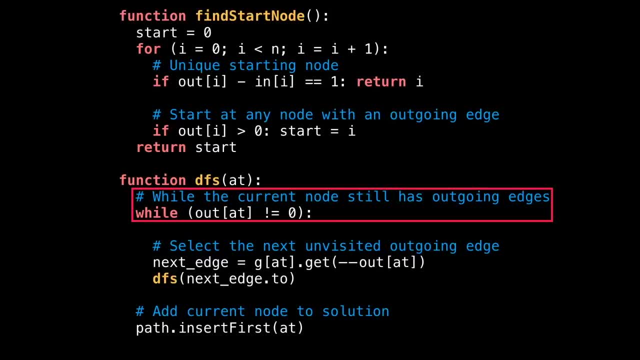 first search loops while the current node still has outgoing unvisited edges. It does this by looking in the outer array at the current node and checking if there are still outgoing edges. The next line selects the next unvisited outgoing edge from the current node from our adjacency list. It also decrements the number of outgoing unvisited edges from: 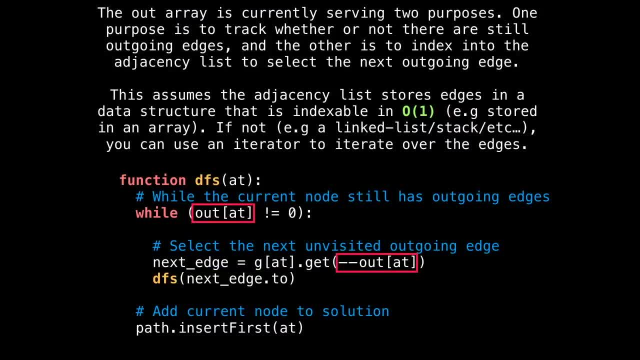 the current node. So if you haven't caught on already, the out array is currently serving two purposes. One purpose is to track whether or not there are still outgoing edges and the other is to index into the adjacency list to select the next outgoing edge. This assumes 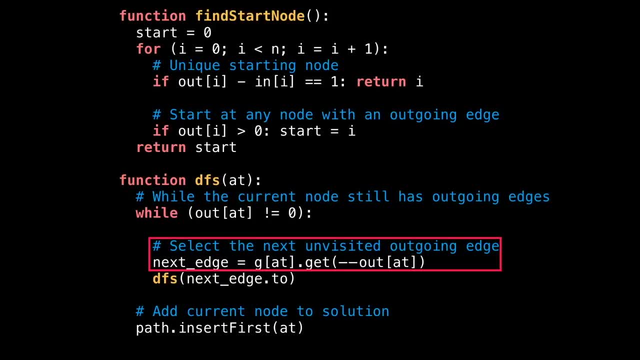 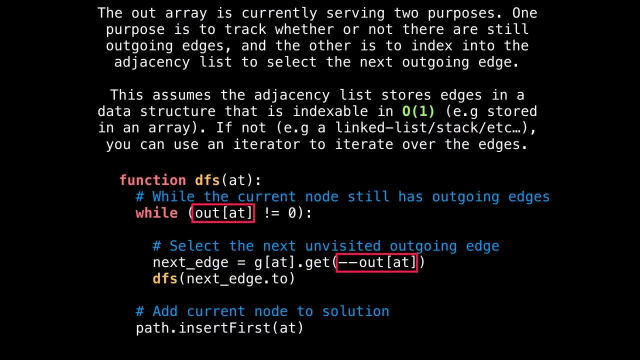 current node from our adjacency list. It also decrements the number of outgoing unvisited edges from the current node. So if you haven't caught on already, the out array is currently serving two purposes. One purpose is to track whether or not there are still outgoing edges. 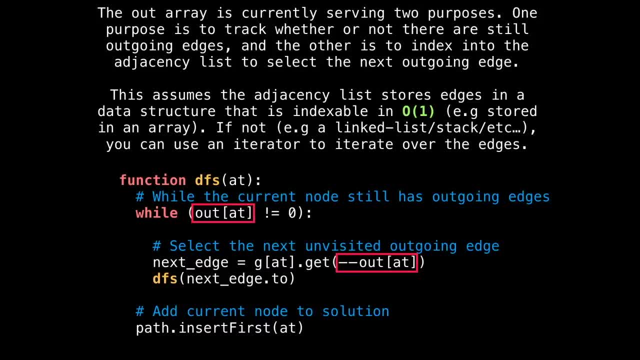 and the other is to index into the adjacency list to select the next outgoing edge. This assumes the adjacency list stores edges in a data structure that is indexable in constant time, just like an array. If not, say you're using an adjacency list composed of linked 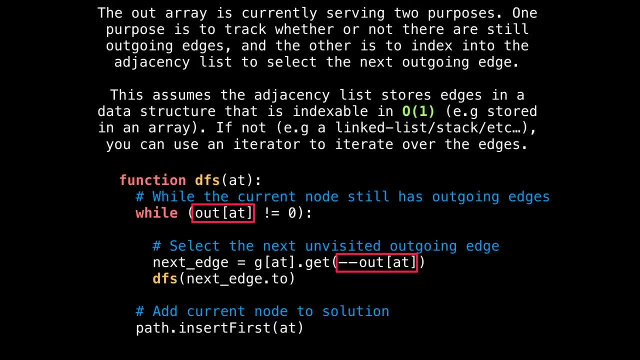 lists, then you can use an iterator to iterate over all the edges. Once we've selected an array, then we can use an iterator to iterate over all the edges. Once we've selected an array, then we can use an iterator to iterate over all the edges Once we've selected the next. 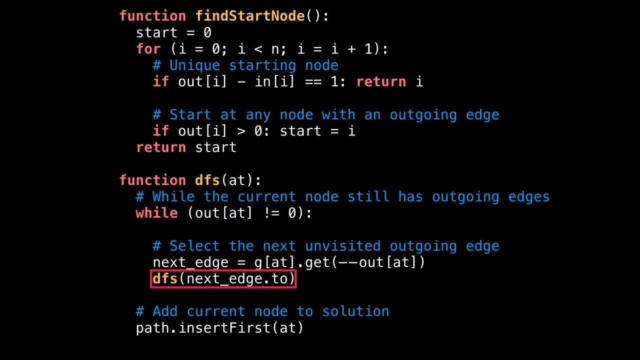 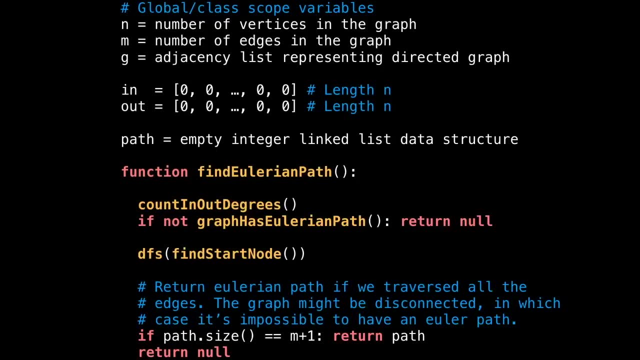 unvisited edge. we visit that edge by calling the depth first search method recursively. Once we exit the loop, append the current node to the front of the solution. Returning back to the main method, the last thing we need to do is check that we have actually found the correct number of 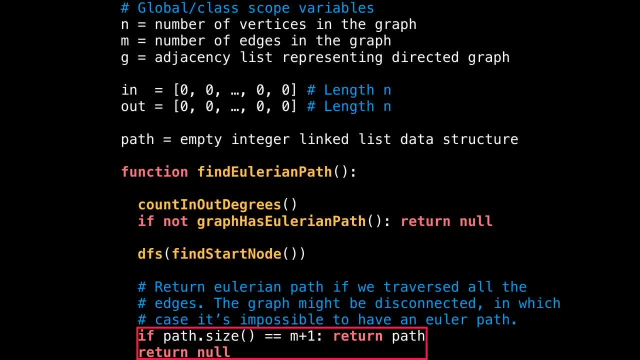 edges for an Eulerian path. it might be the case that our graph is disconnected and we found an Eulerian path On one of the many connected components of our graph, in which case it's impossible to actually have an Eulerian path. So we return null in that case. Otherwise, we simply return our path Today. 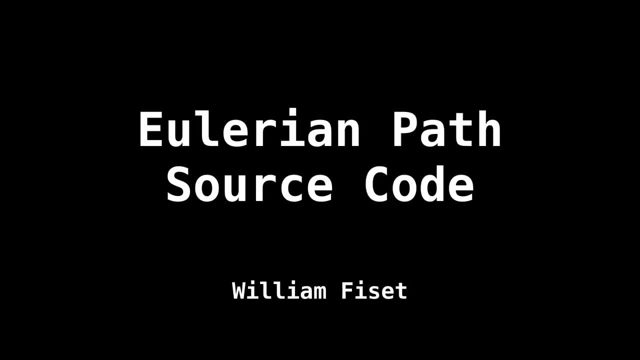 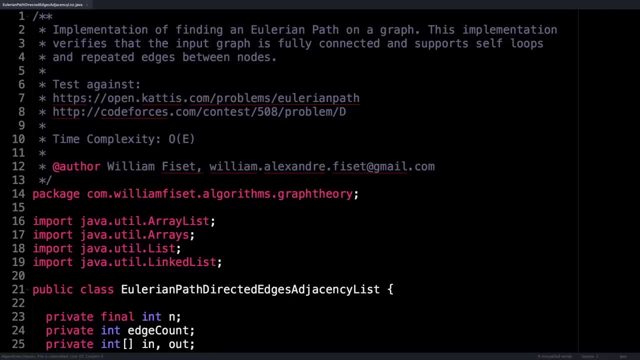 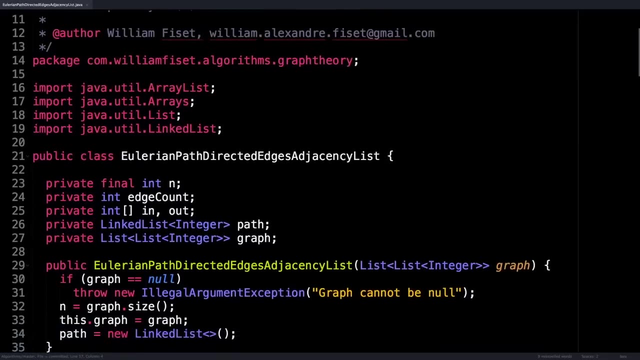 we're going to look at some source code for the Eulerian path algorithm. Awesome, here we are in the source code for the Eulerian path algorithm. This code works by first instantiating this Eulerian path solver class and then calling a method to fetch the Eulerian path itself, should it exist. 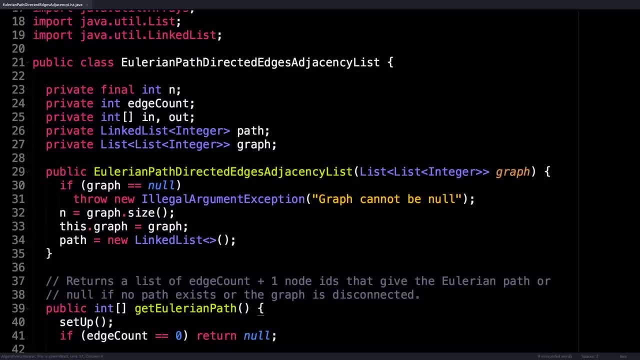 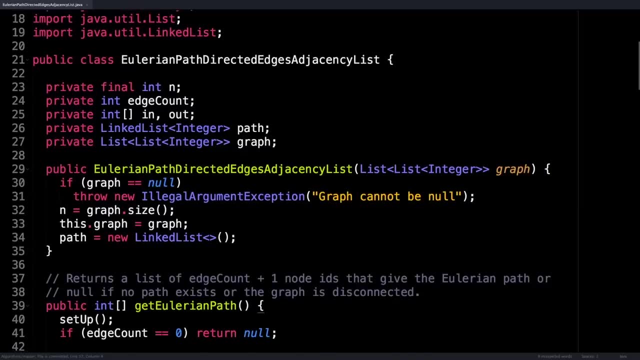 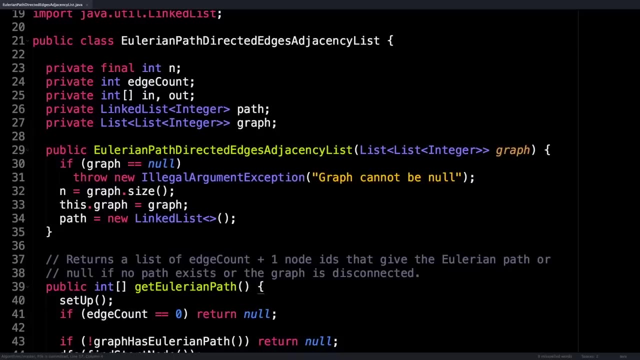 Let's begin by taking a look at the class constructor. in the constructor, what you do is you pass in a directed graph to the algorithm as input, And then the constructor verifies that you actually passed in a graph that's not null, And it also initializes a few variables, including n. 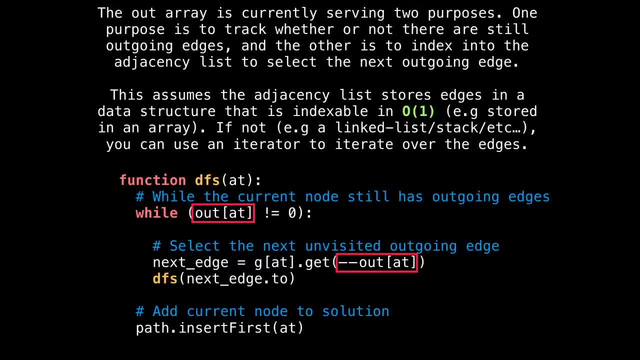 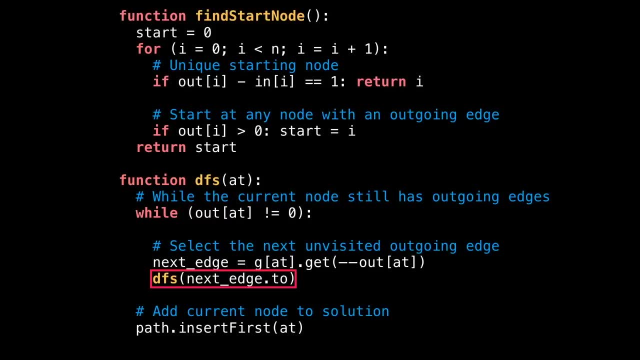 the adjacency list stores edges in a data structure that is indexable in constant time, just like an array. If not, say, you're using an adjacency list composed of a linked list lists, then you can use an iterator to iterate over all the edges. Once we've selected the 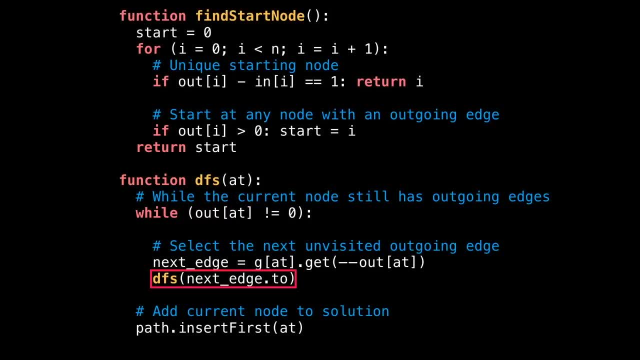 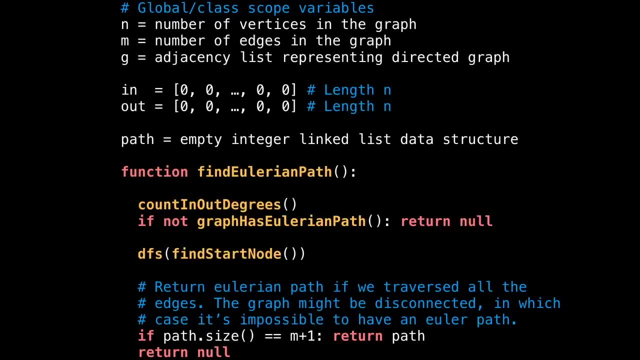 next unvisited edge. we visit that edge by calling the depth first search method recursively. Once we exit the loop, append the current node to the front of the solution. Returning back to the main method, the last thing we need to do is check that we have actually. 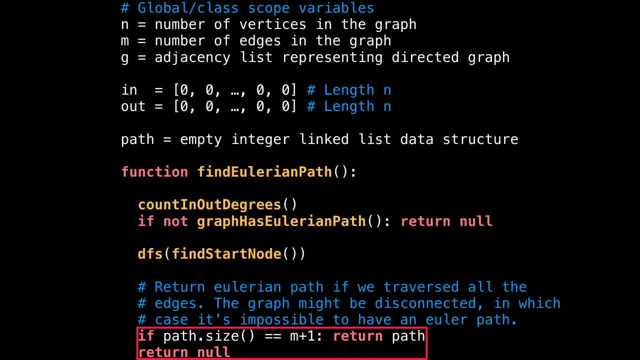 found the correct number of edges for an Eulerian path. It might be the case that our graph is disconnected And we found an Eulerian path on one of the many connected components of our graph, in which case it's impossible to actually have. 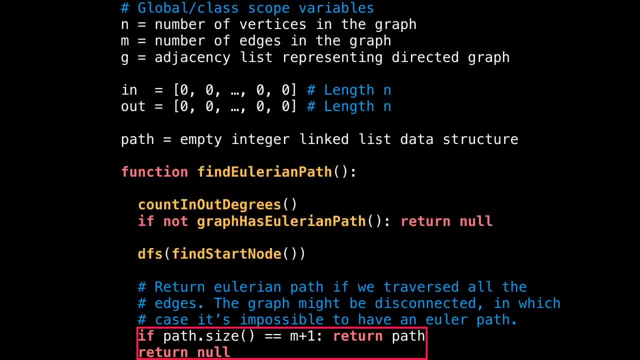 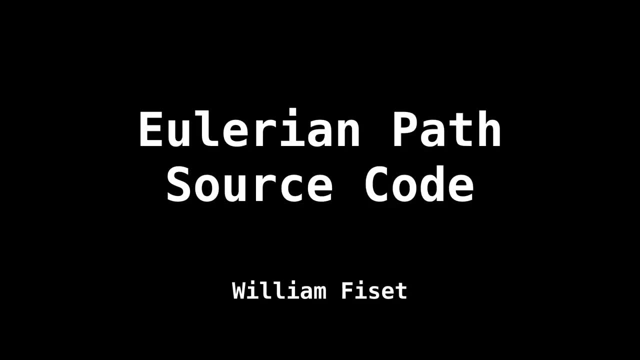 an Eulerian path, So we return null in that case. Otherwise, we simply return our path. Today, we're going to look at some source code for the Eulerian path algorithm. Awesome, Here we are in the source code for the Eulerian path algorithm. 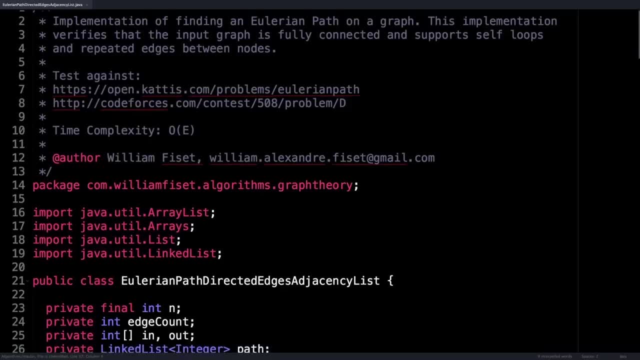 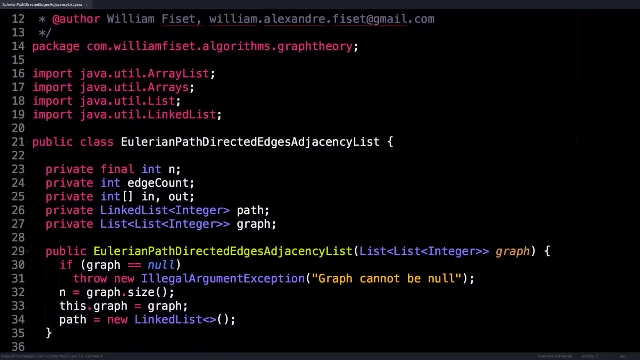 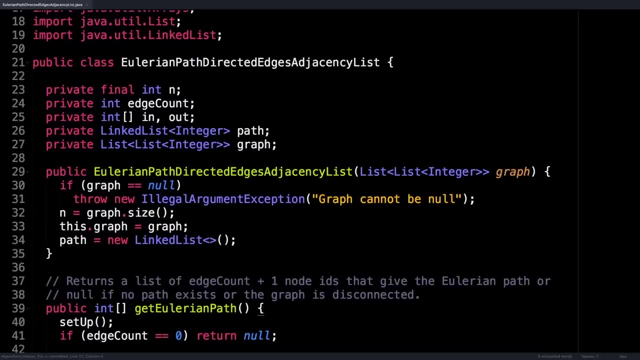 Okay, this code works by first instantiating this Eulerian path solver class and then calling a method to fetch the Eulerian path itself, should it exist. Let's begin by taking a look at the class constructor In the constructor. what you do is you pass in a directed graph. 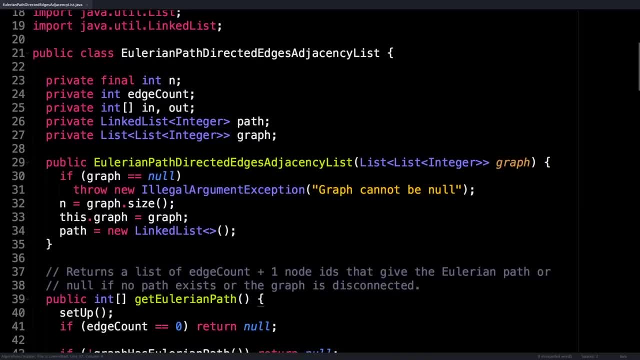 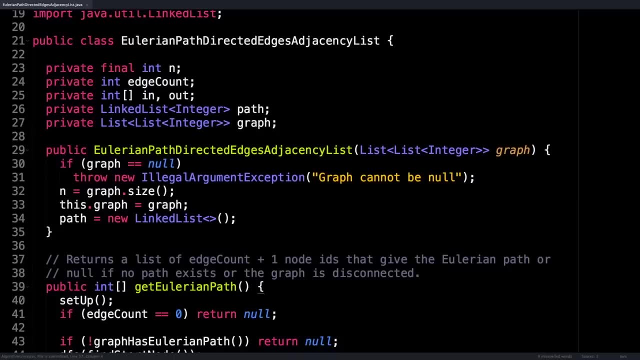 to the algorithm as input, And then the constructor verifies that you actually passed in a graph that's not null, And it also initializes a few variables, Including n, the number of nodes in the graph and the path linked to list. Before we go, 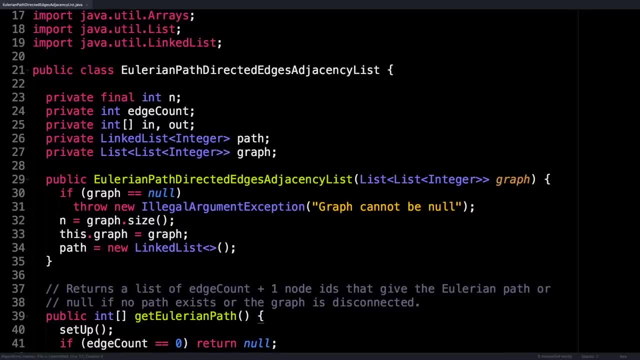 too far. let's have a look at some of the instance variables for this class. We already talked about n, the number of nodes in the graph. Next, we have edge count, which we will compute dynamically from the input graph, followed by in and out, which are integer. 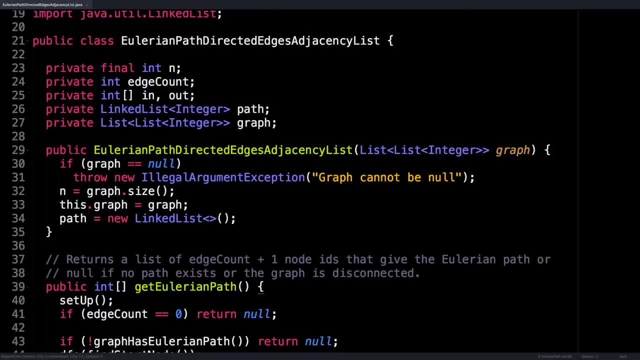 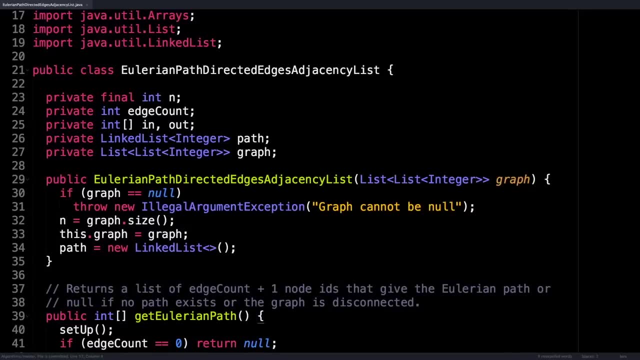 the number of nodes in the graph and the path linked to list. Before we go too far, let's have a look at some of the instance variables for this class. we already talked about n, the number of nodes in the graph. Next we have edge count, which we will compute. 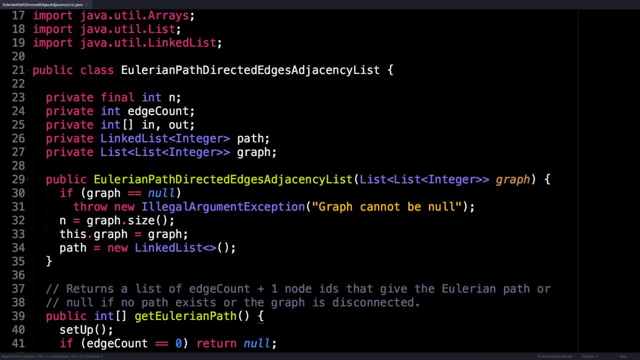 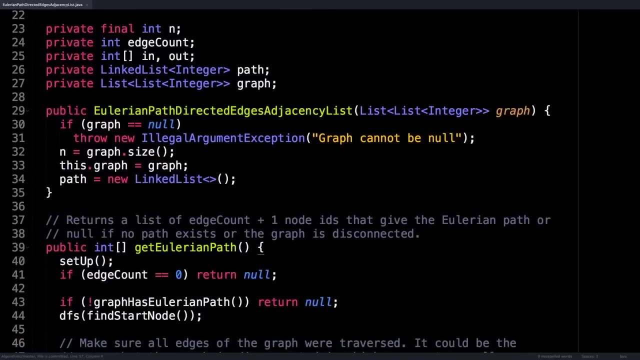 dynamically from the input graph, followed by in and out, which are integer arrays to track the in and out degree of each node. then we have path, which is the Eulerian path solution, as well as a reference to the input graph. So once you create an instance of this class, the Eulerian path solution. 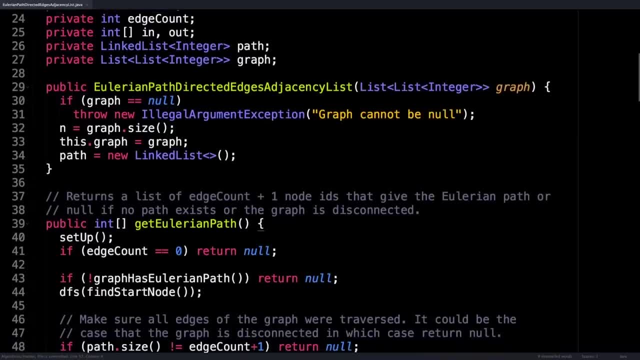 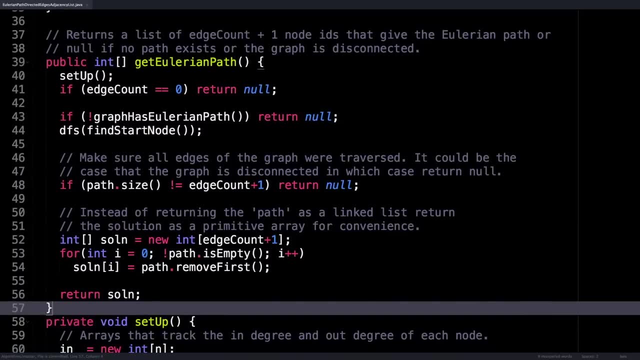 will be able to run in the Eulerian path, And once you create an instance of this class, there's only one public method, And that's get Eulerian path, which does exactly what it says. it will return to you an integer path consisting of the nodes you need to traverse to get a valid Eulerian. 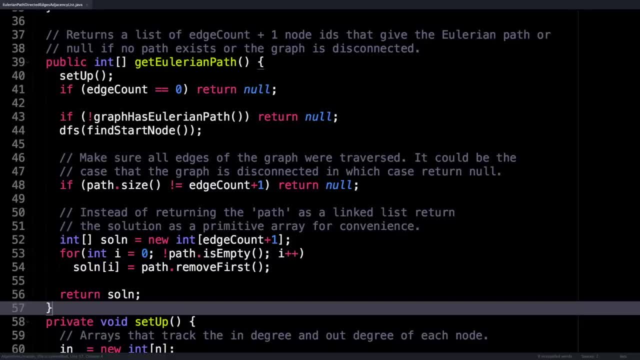 path, or null if no path exists. So there's a few things that get Eulerian path does which will cover step by step. The first thing in the get Eulerian path method is the setup method, So let's have a look at that first. 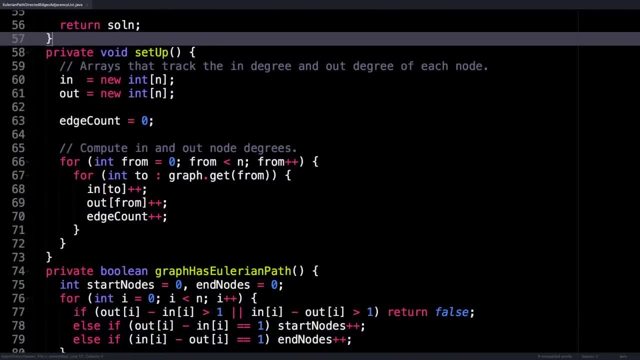 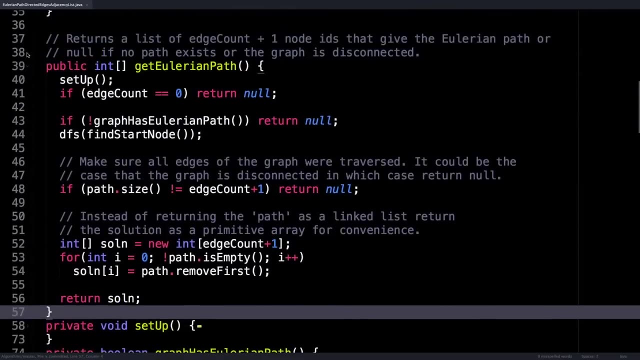 All the setup method does is loop through all the edges and increment the in and out array degrees, as well as compute the number of edges in the graph which is being tracked by the edge count variable. Back to the get Eulerian path method. the next thing is to check if the edge count is. 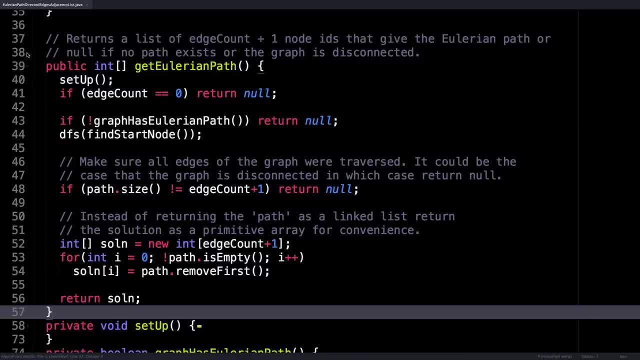 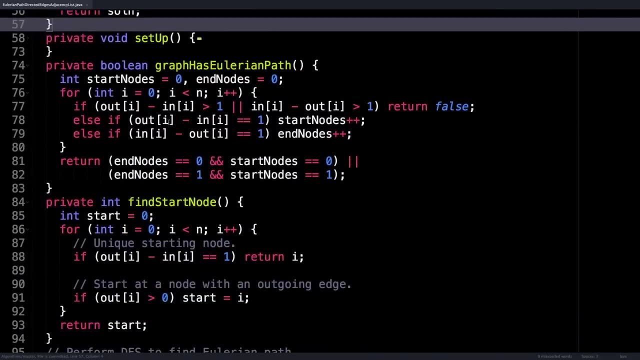 zero and return null if we don't have any edges to work with. Following this, I call the graph has Eulerian path method, which verifies that our graph actually has an Eulerian path, because most graphs don't. The graph has Eulerian path method is also fairly simple. What we want to. 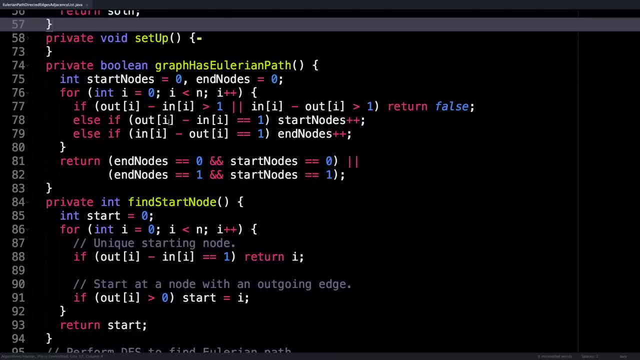 do is make sure that no node has too many outgoing edges or too many incoming edges, as well as ensure that there's the correct amount of start and end nodes for an Eulerian path to exist. the variables- start nodes and end nodes- nodes- keep track of how many nodes have either exactly one extra outgoing edge or one extra. 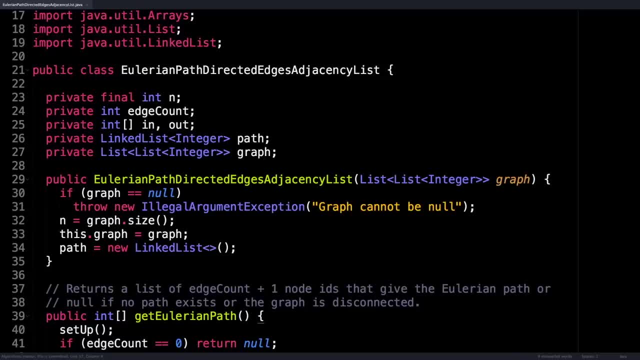 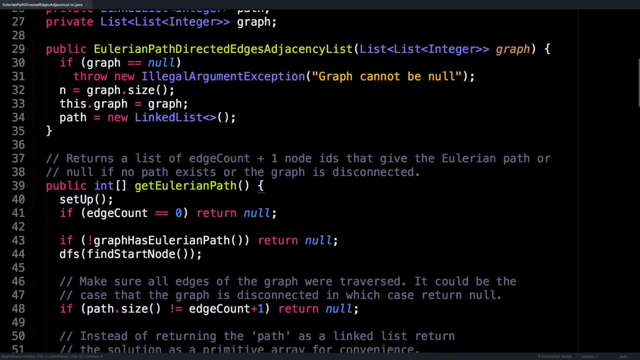 arrays to track the in and out degree of each node. then we have path, which is the Eulerian path solution, as well as a reference to the input graph. So once you create an instance of this class, there's only one public method And that's get Eulerian path, which does exactly what it says it'll. 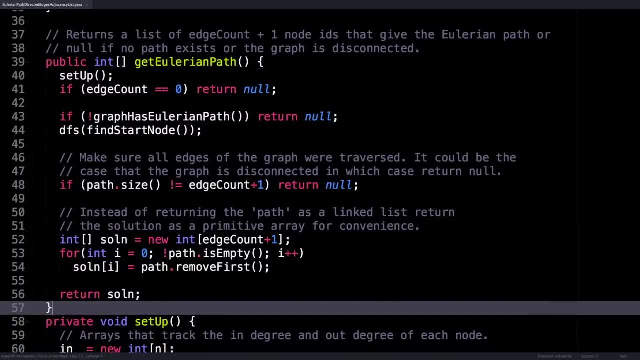 return to you an integer path consisting of the nodes you need to traverse to get a valid Eulerian path, or null if no path exists. So there's a few things that get Eulerian path does, which will cover step by step. The first thing. 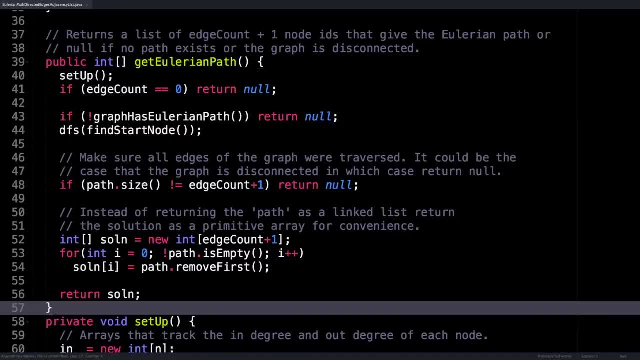 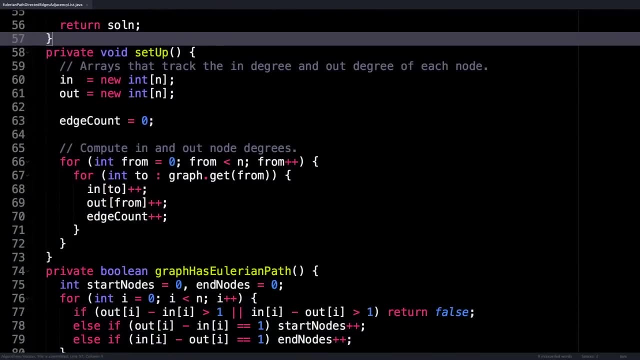 in the get Eulerian path method is the setup method. So let's have a look at that first. All the setup method does is loop through all the edges and increment the in and out array degrees, as well as compute the number of edges in the graph which is being tracked. 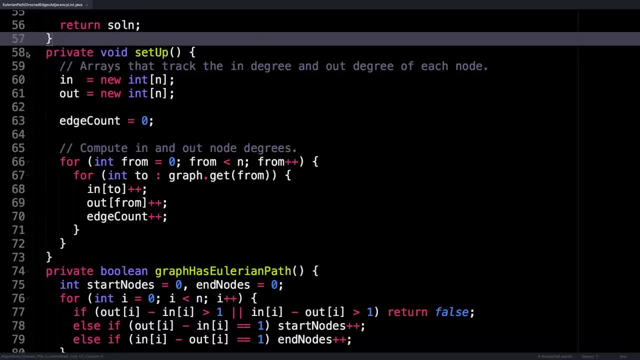 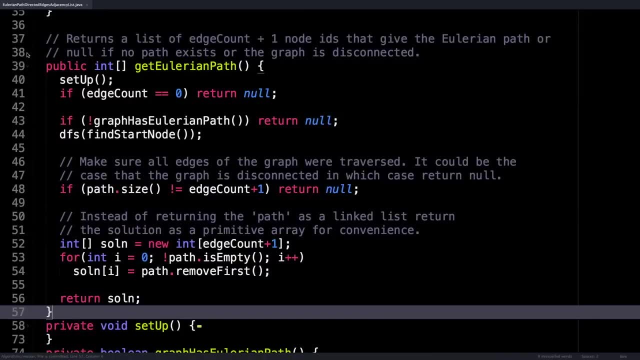 by the edge count variable. Back to the get Eulerian path method. the next thing is to check if the edge count is zero and return null If we don't have any edges to work with. Following this, I call: the graph has Eulerian path method, which verifies that our graph actually has an Eulerian path. 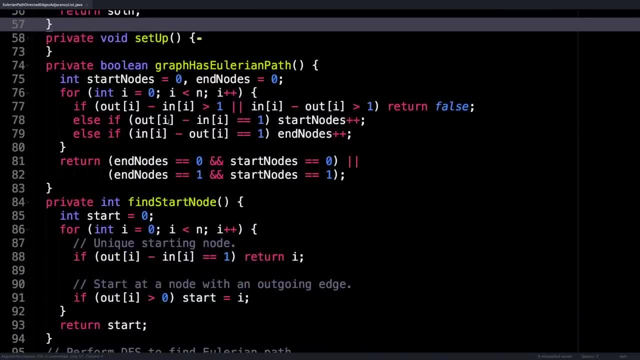 because most graphs don't. The graph has Eulerian path. method is also fairly simple. What we want to do is make sure that no node has too many outgoing edges or too many incoming edges, as well as ensure that there's the correct amount of start. 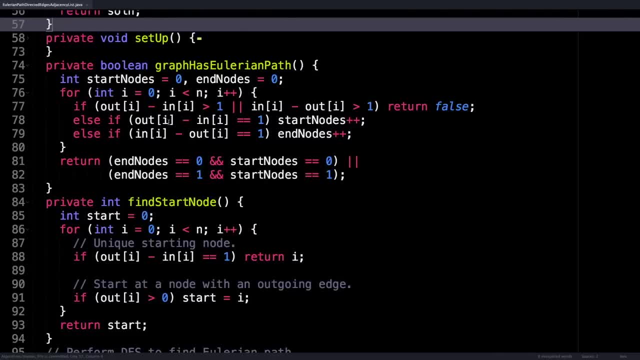 and end nodes for an Eulerian path to exist. The variables start nodes and end nodes keep track of how many nodes have either exactly one extra outgoing edge or one extra incoming edge. for an Eulerian path to exist, there has to be at most one start and end node. 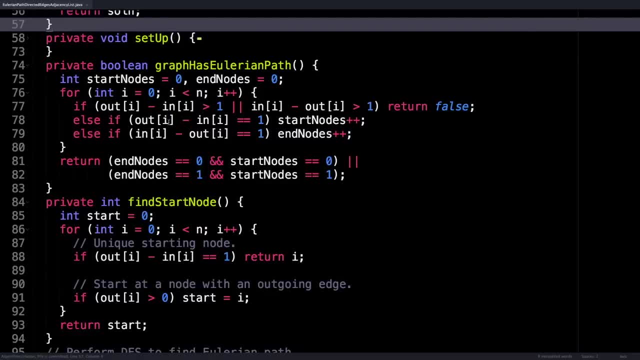 So when we're inside the for loop, we have three conditions. The first is to identify if the current node has too many incoming or outgoing edges, which mathematically means that the different conditions between the in and out degree, or vice versa, is greater than one. In this. 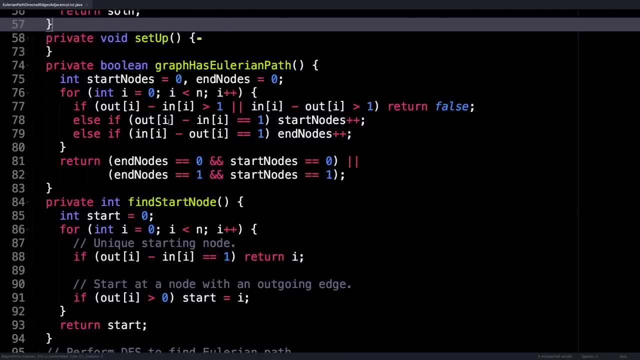 incoming edge. for an or layer and path to exist, there has to be at most one start and end node. So when we're inside the for loop, we have three conditions. The first is to identify if the current node has too many incoming or outgoing edges which mathematically 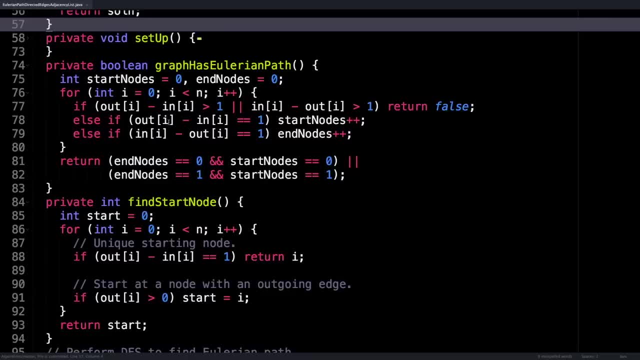 means that the difference between the in and out degree, or vice versa, is greater than one. In this case, return false because the path is impossible. there will be no or there in path in such an event. The other conditions we care about are whether the current node 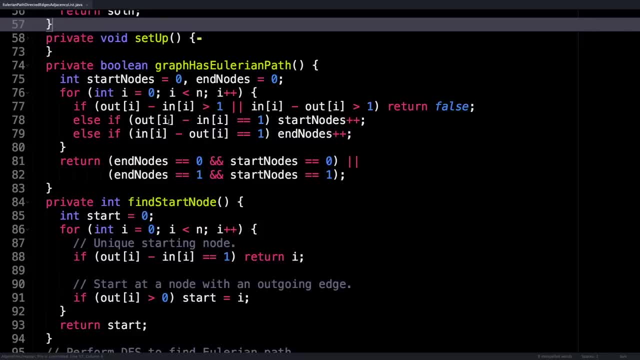 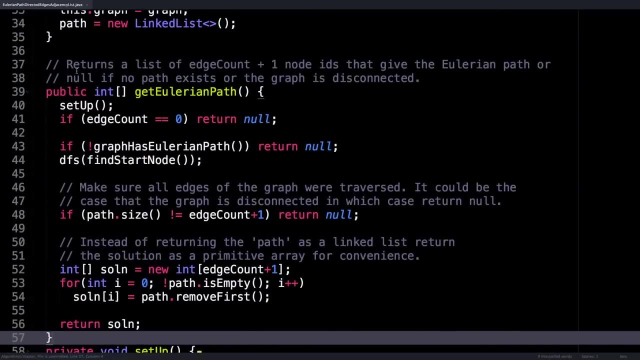 might be a start node or an end node, And if it is, then we increment the start node and end node counters respectively. The last step is to actually check that we have the correct number of certain nodes and end nodes and return the Boolean value Returning back. 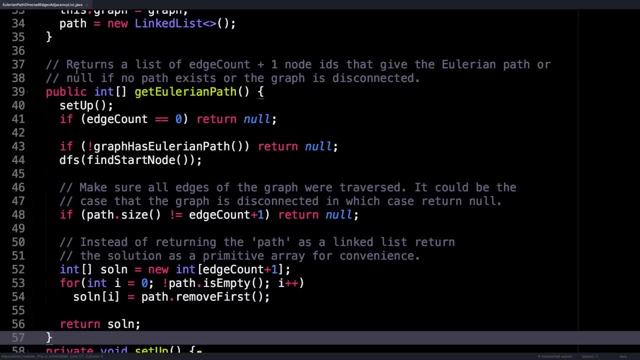 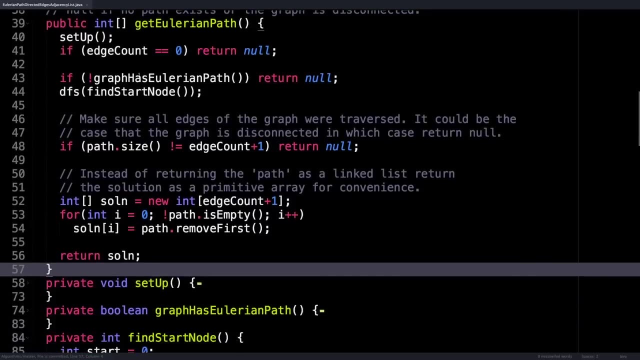 to the get or layer and path method. The next thing in the algorithm is to actually find the or layer and path. now that we know one exists to do this, we find a valid starting node and feed that as the first node to the depth for search method. So let's have a look at both of those. We don't want to start our. 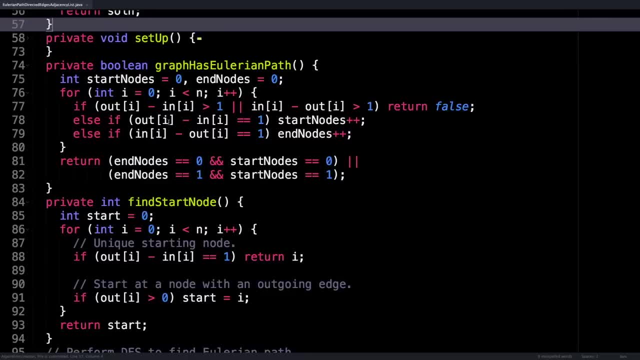 case return false, because the path is impossible. there will be no Eulerian path in such an event. The other conditions we care about are whether the current node might be a start node or an end node, And if it is, then we increment the start node and end node counters respectively. 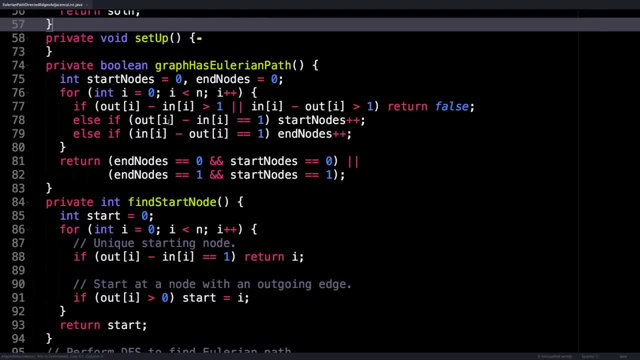 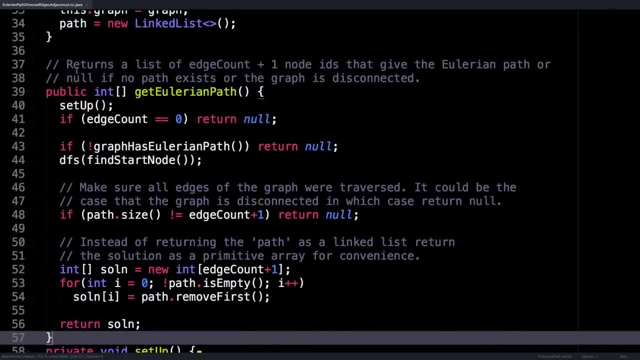 The last step is to actually check that we have the correct number of start nodes and end nodes and return the Boolean value. Returning back to the get Eulerian path method, the next thing in the algorithm is to actually find the Eulerian path. now that we know one exists. To do this, we find a valid starting. 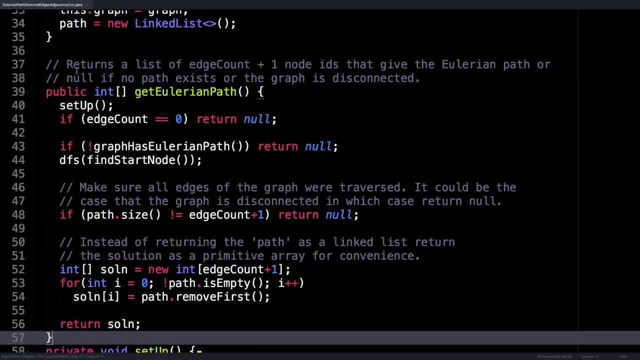 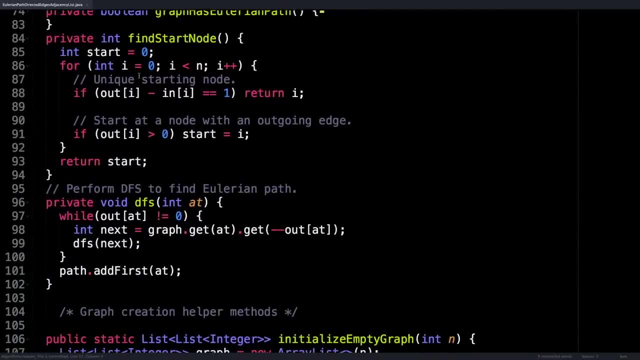 node and feed that as the first node to the depth first search method. So let's have a look at both of those. We don't want to start our Eulerian path anywhere, as we saw in the first video, because this doesn't ensure that we find an Eulerian path even though we know. 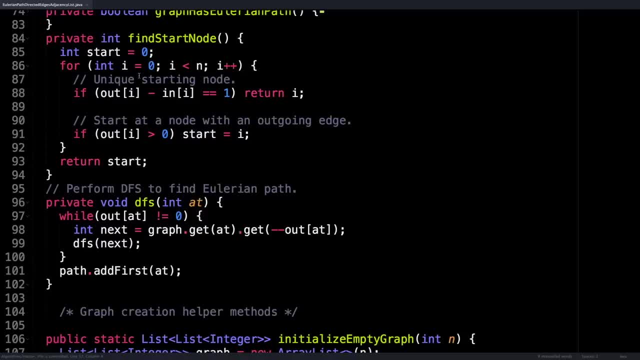 one exists. The fine start node method does exactly what it sounds like. it looks for a node which is a valid starting node, meaning a node with exactly one extra outgoing edge or, in the case of an Eulerian circuit, just any node with an outgoing edge. it's important. 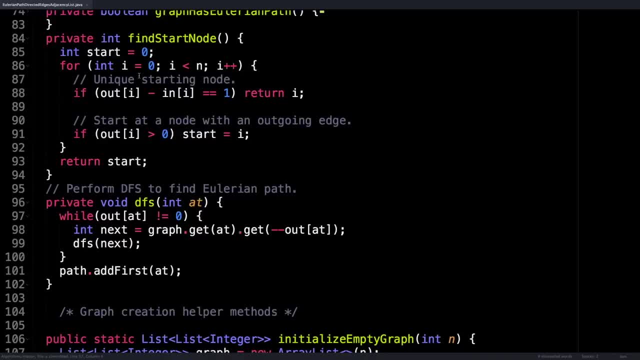 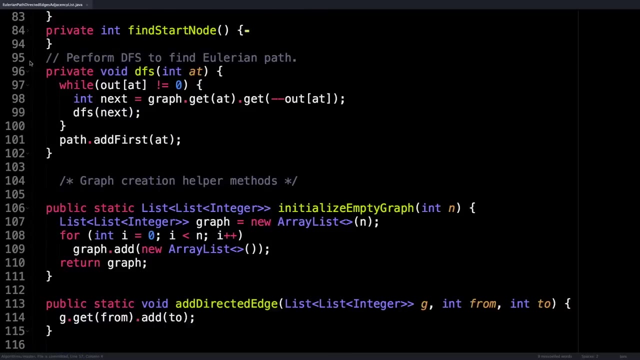 that we start at a node with an outgoing edge, because our graph might contain singleton nodes that have no outgoing edges, but another component in the graph might have outgoing edges, which is where we really want to start If we are to find an Eulerian path. Next up is the depth first search method, where things 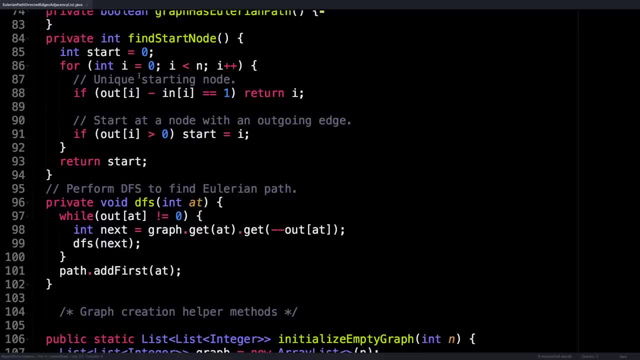 or layer and path anywhere, as we saw in the first video, because this doesn't ensure that we find an oil layer and path, even though we know one exists. the fine start node method does exactly what it sounds like: It looks for a node which is a valid starting node, meaning a node with exactly one extra. 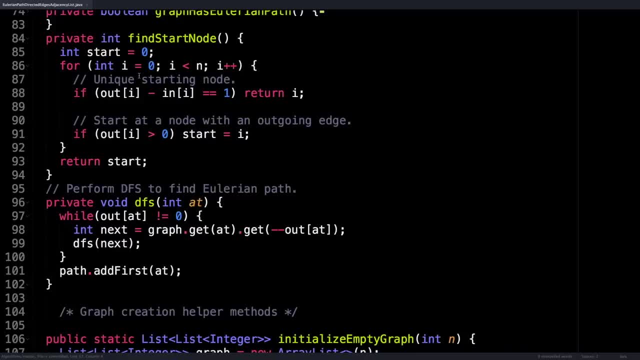 outgoing edge or, in the case of an or layer in circuit, just any node with an outgoing edge. it's important that we start at a node with an outgoing edge, because our graph might contain singleton nodes that have no outgoing edges, but another component in the graph might 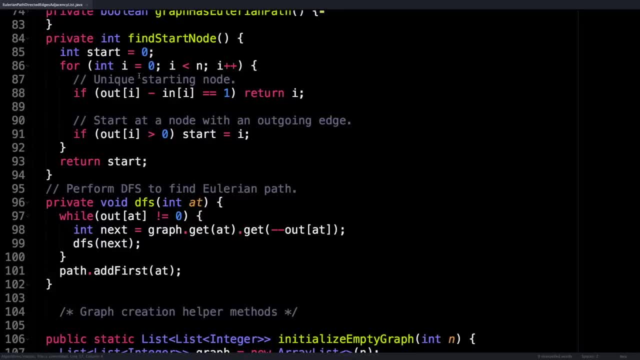 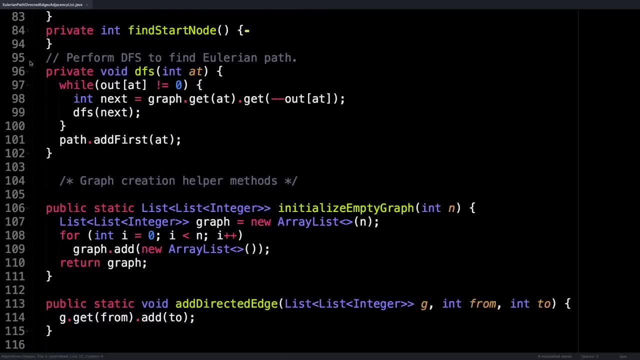 have outgoing edges, which is where we really want to start if we are to find an or layer and path. Next up is the depth first search method, where things get interesting. It turns out the depth first search method is really short and could even be shorter, but at the expense of readability. 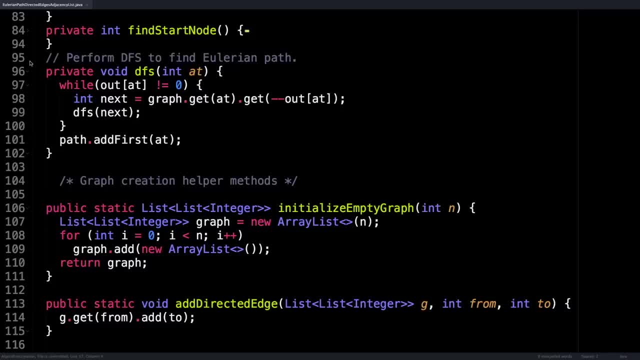 remember that, when calling this method, the first node is the starting node, which is the at variable in this method which, if you haven't guessed it yet, is the current node index we're currently at. in essence, what's happening in this method is that, while the 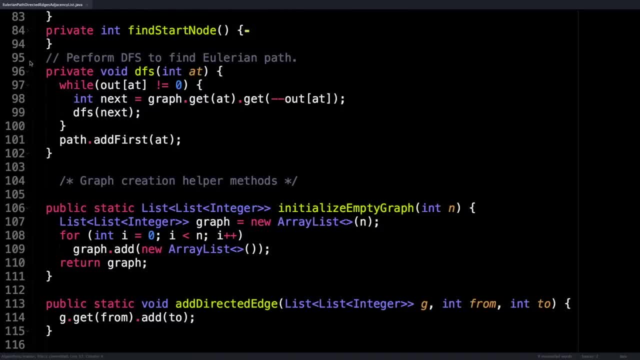 get interesting, It turns out the depth first search method is really short and could even be shorter, but at the expense of readability. Remember that when calling this method, the first node is the starting node, which is the at variable in this method which, if you, 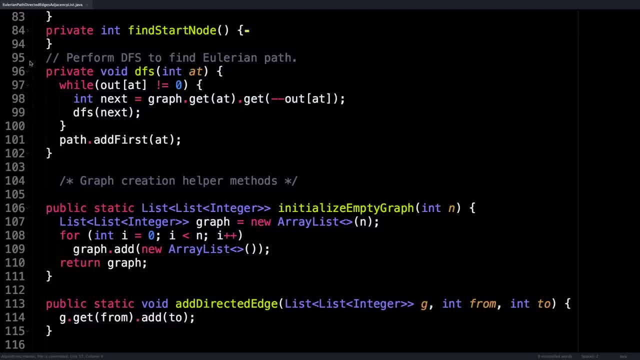 haven't guessed it yet, is the current node index we're currently at. In essence, what's happening in this method Is that, while the current node still has unvisited edges, we're going to select the next node to explore and call the depth first search method recursively Each time we take an edge. 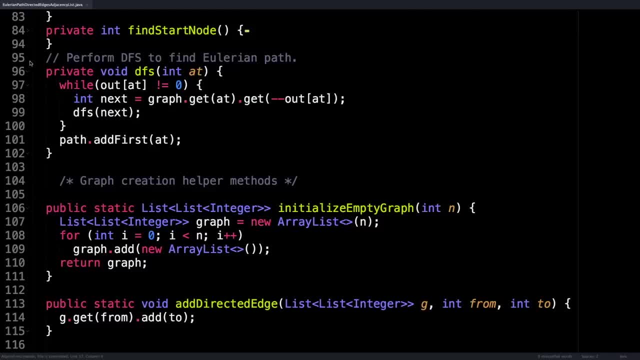 we decrease the number of outgoing edges for that note, which means that eventually there will be no more outgoing edges for the current node and the loop will terminate. Once this happens, we can add the current node to the front of the solution, The key realization. 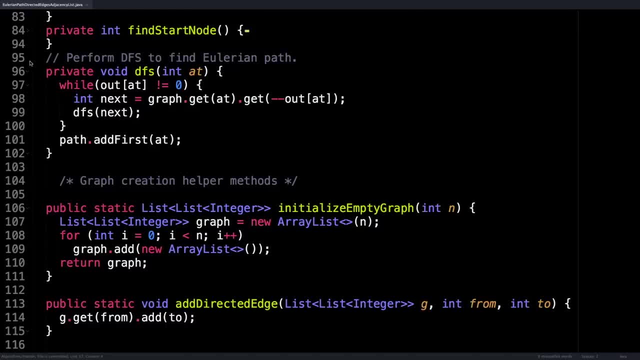 current node still has unvisited edges. we're going to select the next node to explore and call the depth first search method recursively. Each time we take an edge, we decrease the number of outgoing edges for that note, which means that eventually there will be no more outgoing edges for the current node and the loop will. 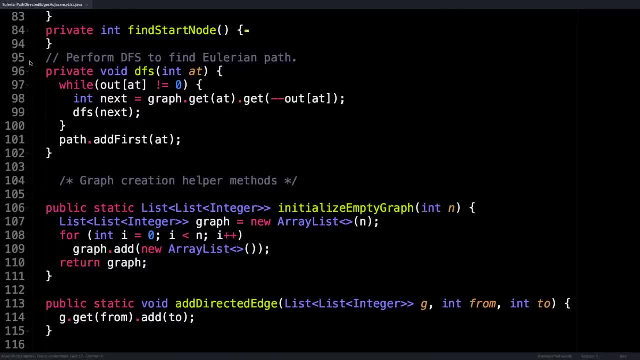 terminate. Once this happens, we can add the current node to the front of the solution. The key realization in this method, I think, is that you have to notice that the out array is being used As both a way of determining if there are any unvisited edges left at the current node. 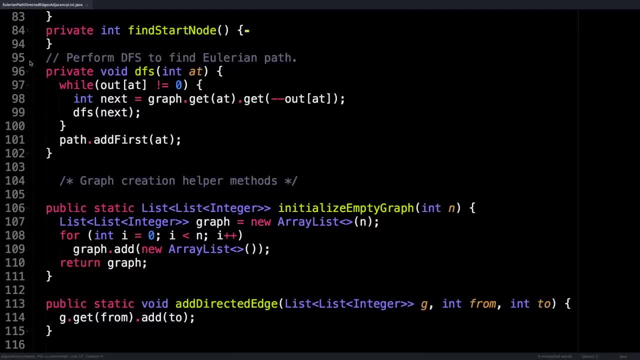 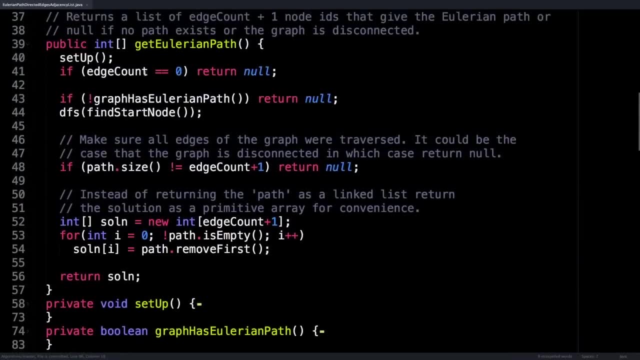 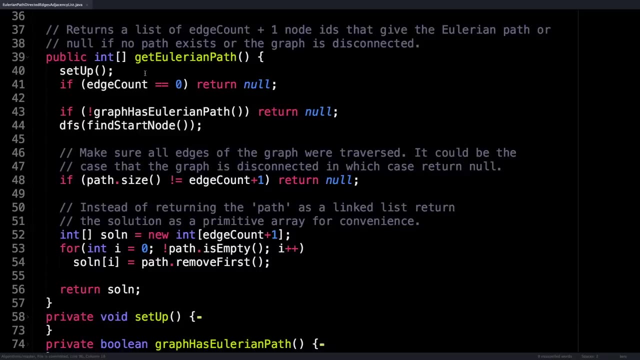 as well as an index for reaching into the adjacency list to grab the next note to visit. Let's go back up to the get Eulerian path method. Once we've finished executing the depth first search, the next thing to do is ensure that we found an Eulerian path. it. 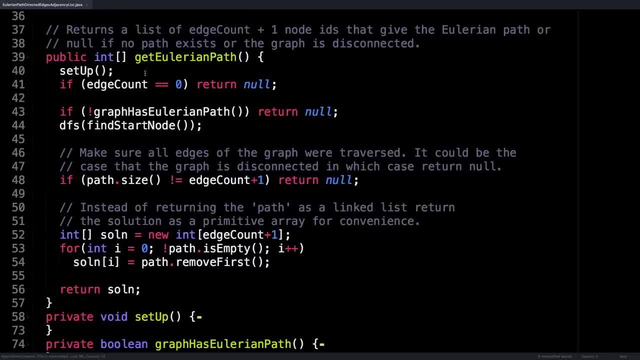 could be the case that the graph is disconnected into multiple components, in which case we have to return null because no Eulerian path exists. Checking that the graph is disconnected is not something the graph has. Eulerian path method verifies, And this is intentional. 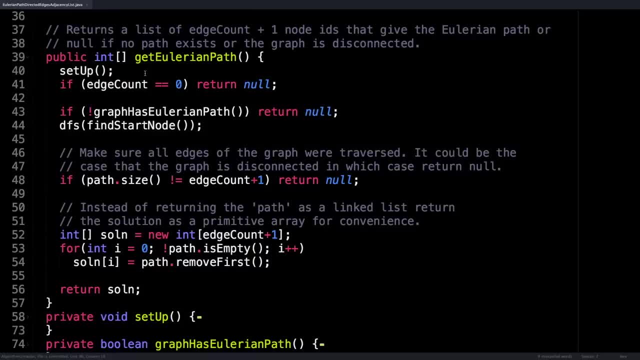 because it's easier to do. after running the depth first search, by ensuring that the solution actually has a size equal to edge count plus one, The next thing I do before returning the solution, which is optional, is simply to empty the depth first search method. So 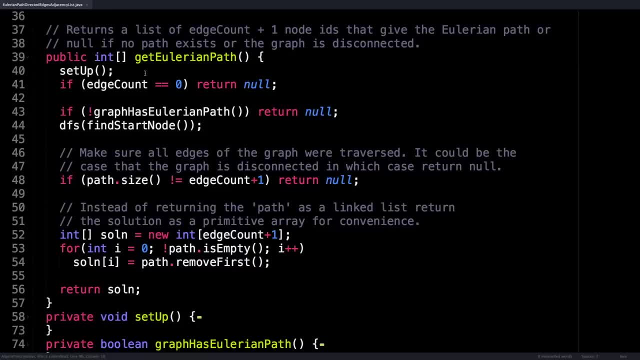 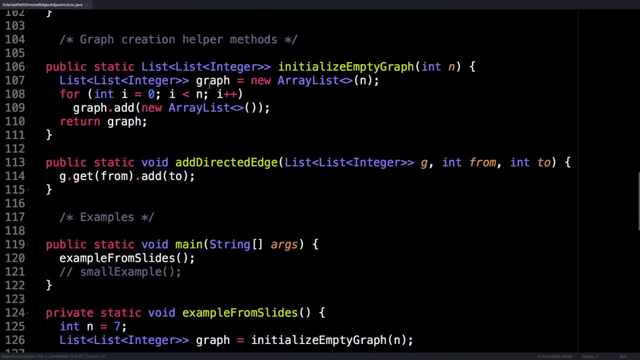 I'm going to empty the contents of the linked list into a primitive integer array just for convenience. I do this because it's easier for the caller to index an array than it is a linked list. The rest of this file are just helper methods for creating a directed graph. 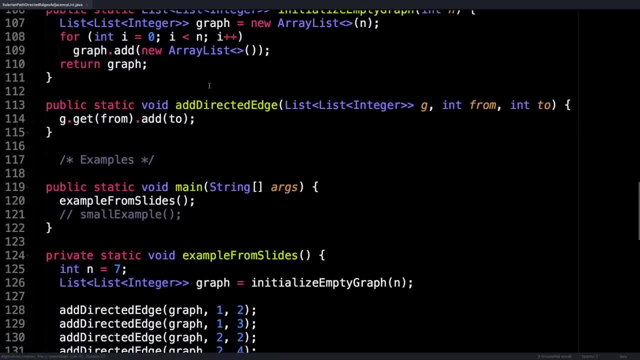 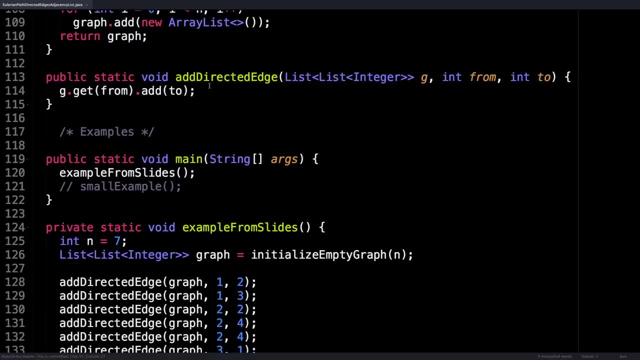 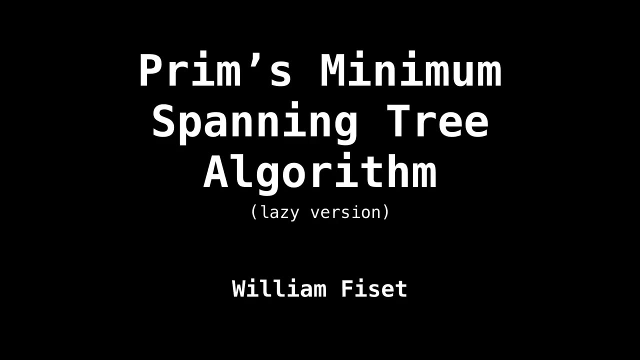 and adding directed edges to the graph. I also provide two examples, one from the previous slides and another that I made up. I encourage you to look them over to understand how this program works. Today, we're talking about minimum spanning trees And, in particular, we're talking about 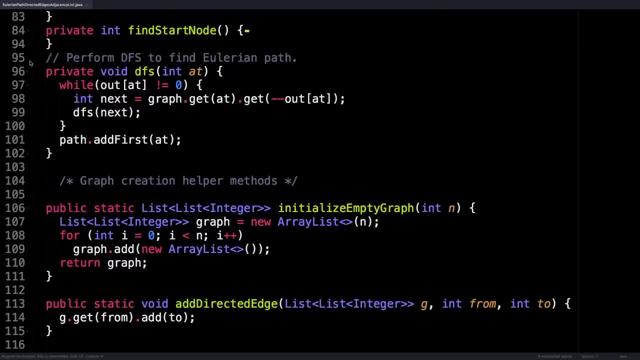 in this method, I think, is that you have to notice that the out array is being used as both a way of determining if there are any unvisited edges left at the current node, as well as an index for reaching into the adjacency list. to grab the next note to visit, Let's go back. 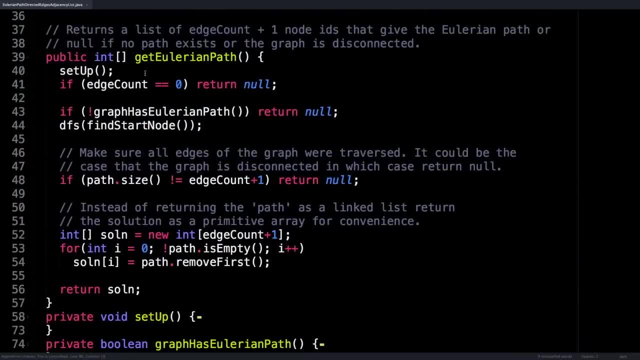 up to the get Eulerian path method. Once we finished executing the depth first search, the next thing to do is ensure that we found an Eulerian path. It could be the case that the graph is disconnected into multiple components, in which case the 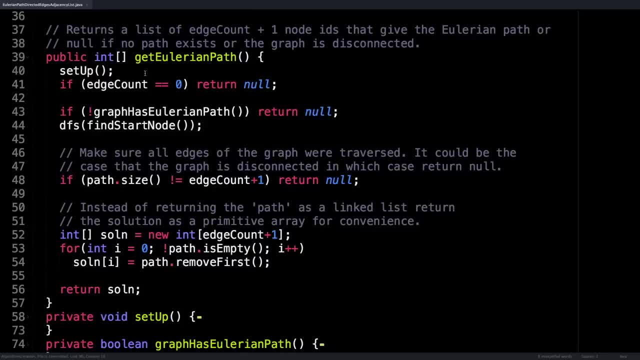 correct thing to do is to return null because no Eulerian path exists. Checking that the graph is disconnected is not something the graph has Eulerian path method verifies, And this is intentional because it's easier to do after running the depth. first search by 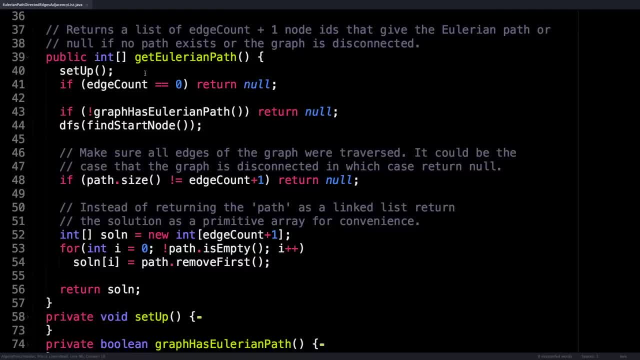 ensuring that the solution actually has a size equal to edge count plus one. The next thing I do before returning the solution, which is optional, is simply to empty the contents of the linked list into a primitive integer array, just for convenience. I do this because it's easier. 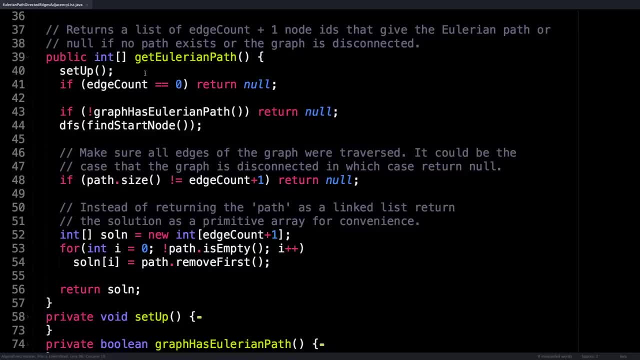 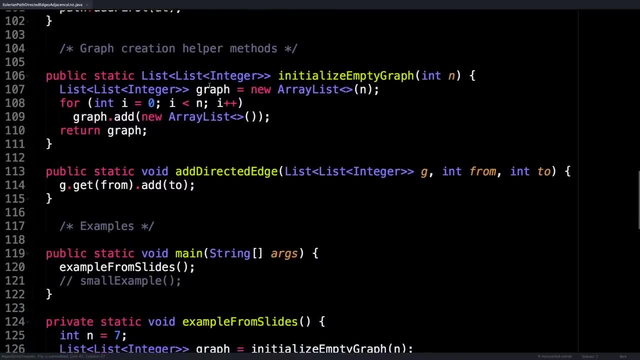 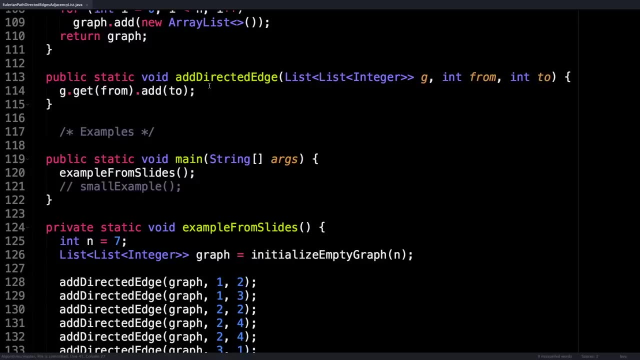 for the color to index an array than it is a linked list. The rest of this file are just helper methods for creating a directed graph and adding directed edges to the graph. I also provide two examples, one from the previous slides and another that I made up. I encourage 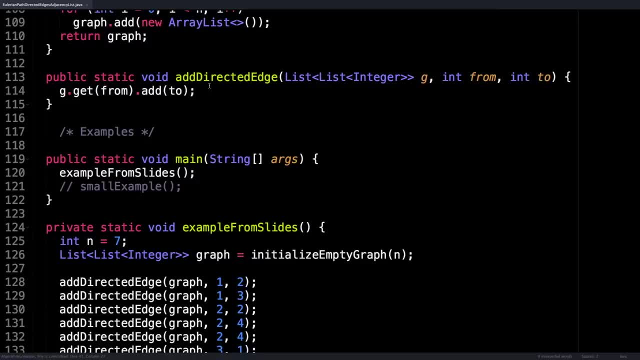 you to check out the previous slides for more information on how to create a directed graph. I also provide two examples, one from the previous slides and another that I made up. I encourage you to look them over to understand how this program works. Today, we're talking about minimum spanning. 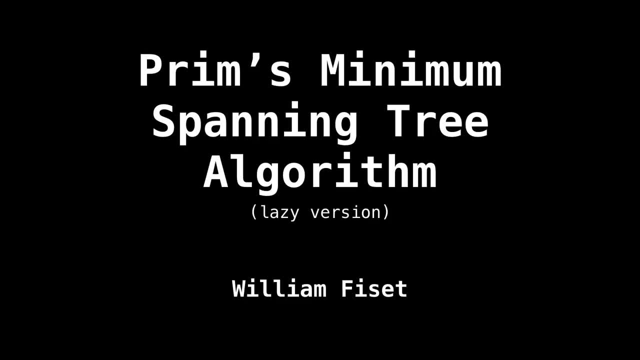 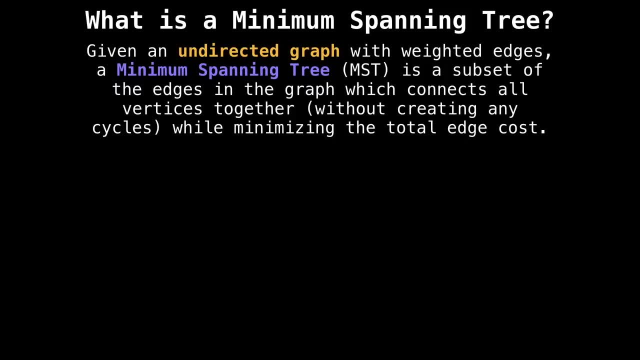 trees And in particular, we're talking about prims algorithm and how it is used to find minimum spanning trees. So what is a minimum spanning tree on a weighted graph? a minimum spanning tree, or just MST for short, is a tree which spans the whole graph, connecting all nodes together, while 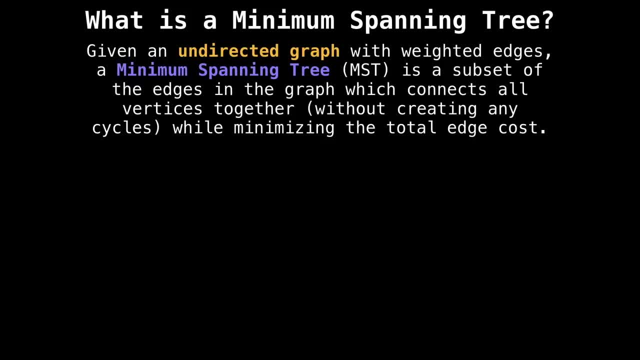 minimizing the number of nodes that are connected to each other. So what is a minimum spanning tree on a weighted graph, or just MST for short? And while minimizing the total edge cost is so important to know that your spanning tree cannot contain cycles, Otherwise it's not a tree. Here's a weighted 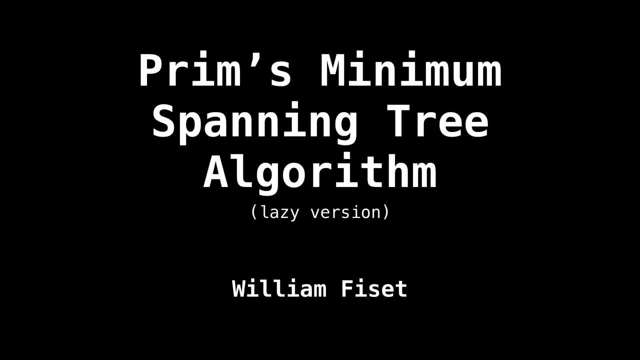 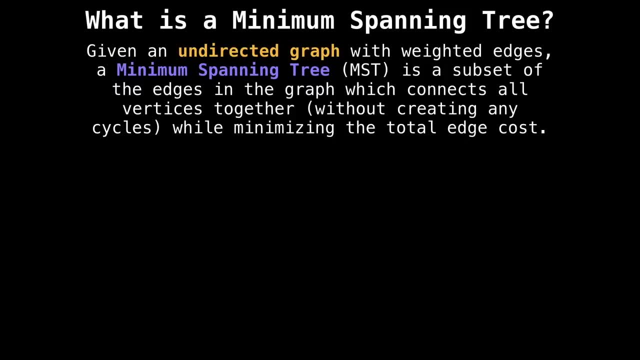 prims algorithm and how it is used to find minimum spanning trees. So what is a minimum spanning tree on a weighted graph? a minimum spanning tree, or just MST for short, is a tree which spans the whole graph, connecting all nodes together while minimizing the total. 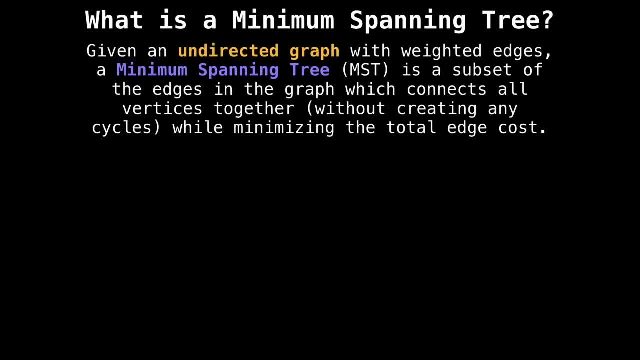 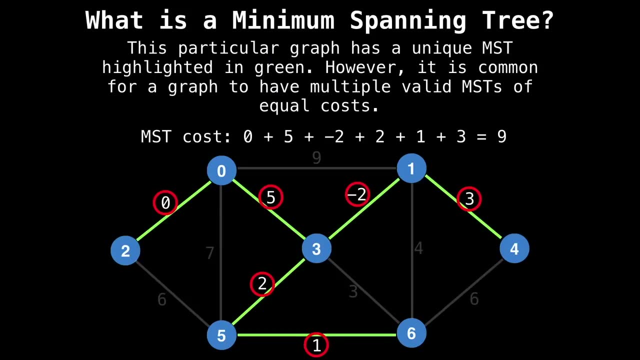 edge cost. It's important to note that your spanning tree cannot contain cycles, Otherwise it's not a tree. Here's a weighted graph with nodes labeled zero through six, with various edges of different costs. One possible minimum spanning tree is the following edges highlighted in green, whose edge costs some to nine. there's 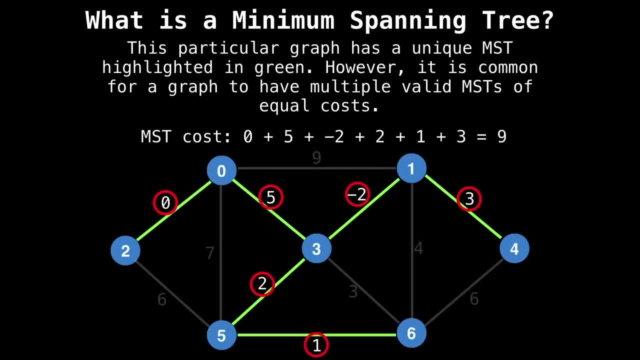 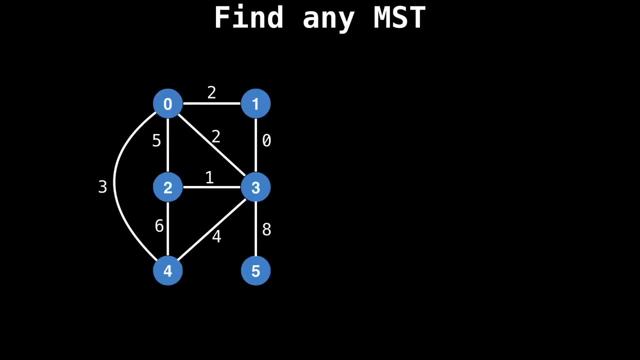 no way to connect all the nodes together and get a lower cost than this. Note that even though the minimum spanning tree in this graph is unique, in general it's possible for a graph to have multiple MSTs of equal costs. All right, hopefully you've been paying attention, because now it's your. 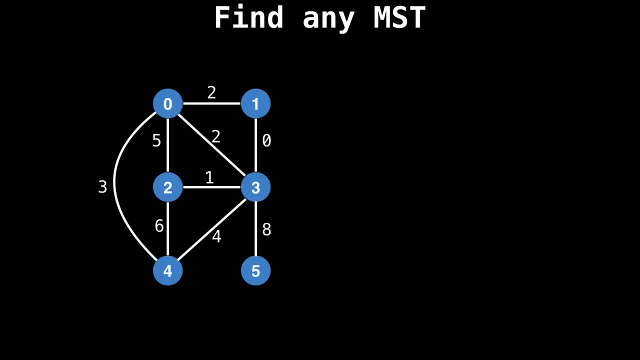 turn. I'm going to present to you some weighted graphs And your job is to identify any possible minimum spanning tree you can find. Let's begin with this graph. Take a moment, pause the video and find any minimum spanning tree you can. 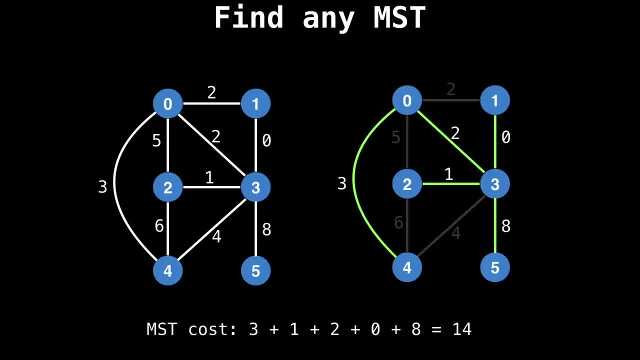 So one possible minimum spanning tree is the following, with a cost of 14.. Again, minimum spanning trees are not unique, So there could be another valid minimum spanning tree here, But they'll all have a cost of 14.. Let's do another one. Can you find a minimum spanning? 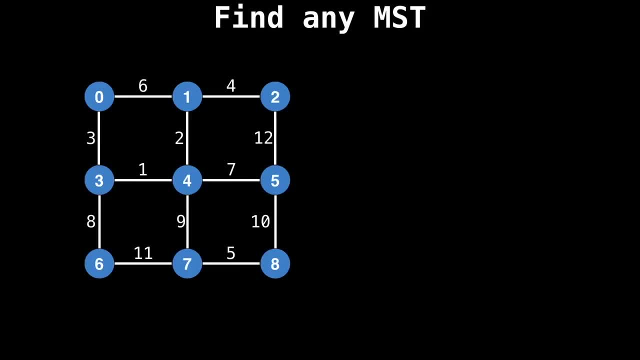 tree here I'll give you a moment. Here's one possible answer with the minimum spanning tree highlighted in green, with a cost of 39.. All right, one last graph. I promise This one is a bit of a trick question, because there is no minimum spanning tree. all the 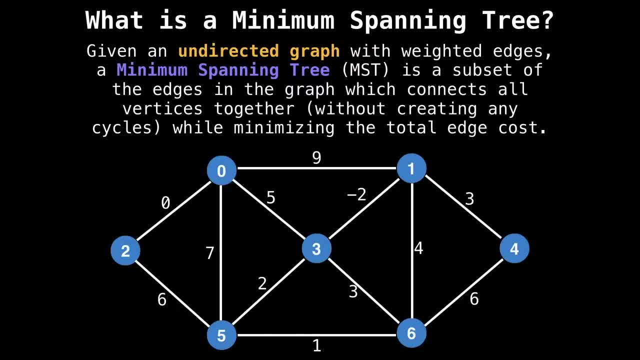 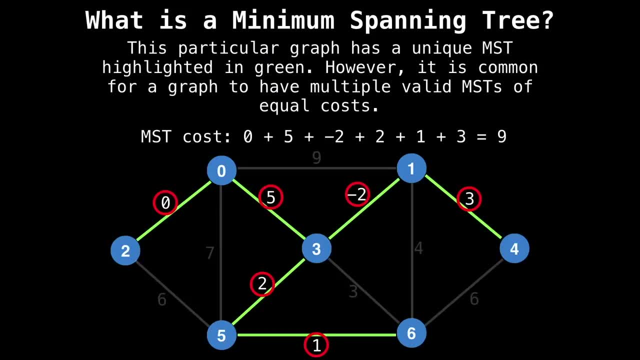 graph with nodes labeled 0 through six with various edges of different costs. One possible minimum spanning tree is the following edges highlighted in green, whose edge costs up some to nine. there's no way to connect all the nodes together and get a lower cost or budget. 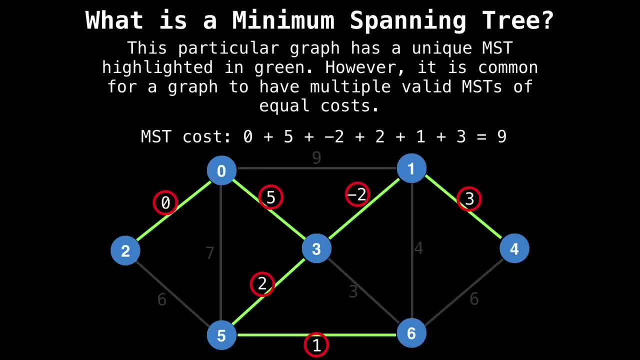 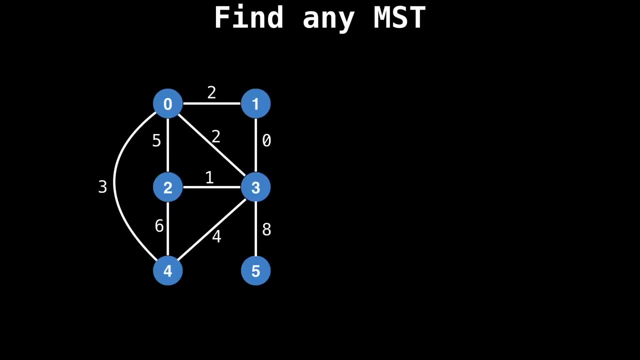 cost than this. Note that even though the minimum spanning tree in this graph is unique, in general it's possible for a graph to have multiple MSTs of equal costs. All right, hopefully you've been paying attention, because now it's your turn. I'm going to present to you some 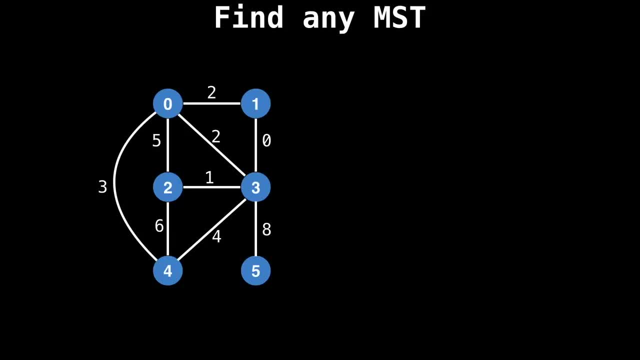 weighted graphs And your job is to identify any possible minimum spanning tree you can find. Let's begin with this graph. Take a moment, pause the video and find any minimum spanning tree you can. So one possible minimum spanning tree is the following, with a cost: 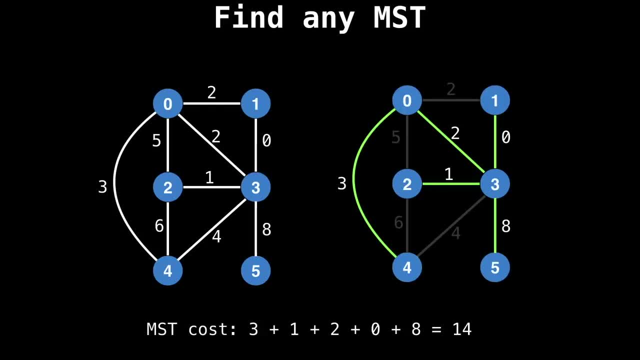 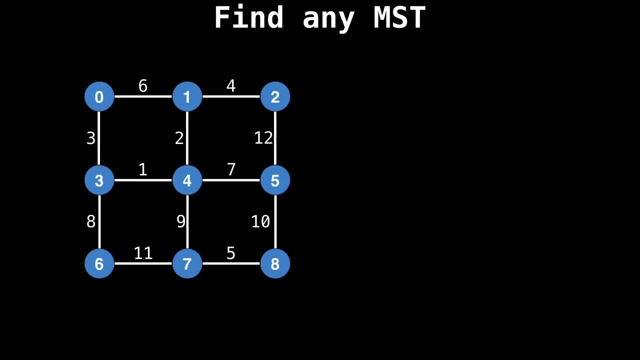 of 14.. Again, minimum spanning trees are not unique, So there could be another valid minimum spanning tree here, But they'll all have a cost of 14.. Let's do another one. Can you find a minimum spanning tree Here? I'll give you a moment. Here's one possible answer with the minimum spanning. 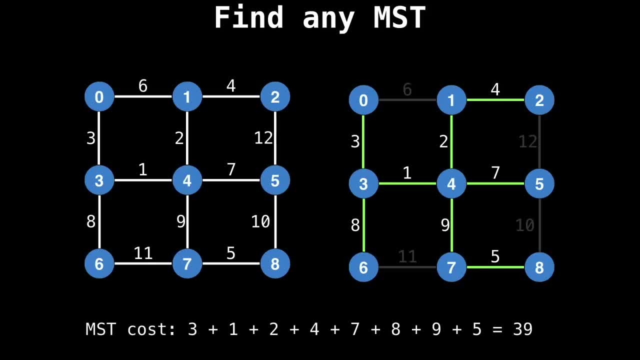 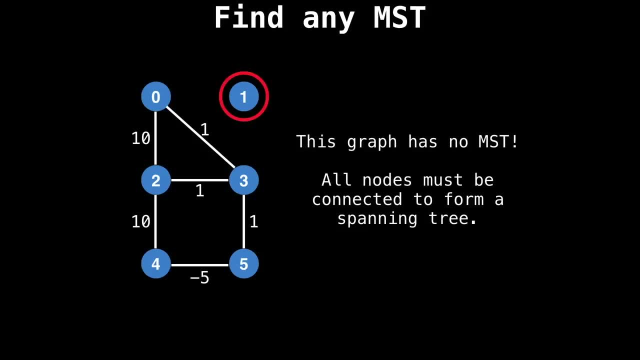 tree highlighted in green, with a cost of 39.. All right, one last graph. I promise This one is a bit of a trick question, because there is no minimum spanning tree. all the nodes must be connected on a single component for a spanning tree to exist. 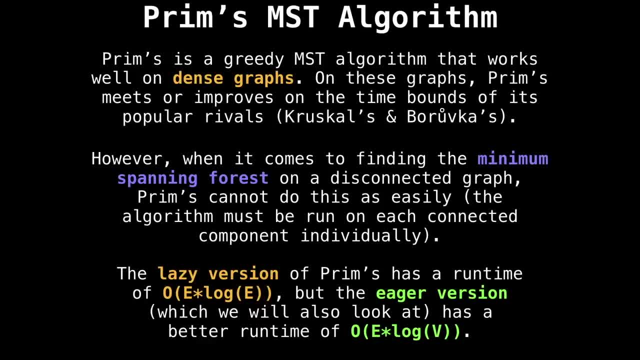 Let's change focus and start talking about Prim's algorithm. Prim's is one of my favorite minimum spanning tree algorithms because of how simple and how intuitive it is. By nature, it's a greedy algorithm which always selects the next best edge and adds it to the minimum. 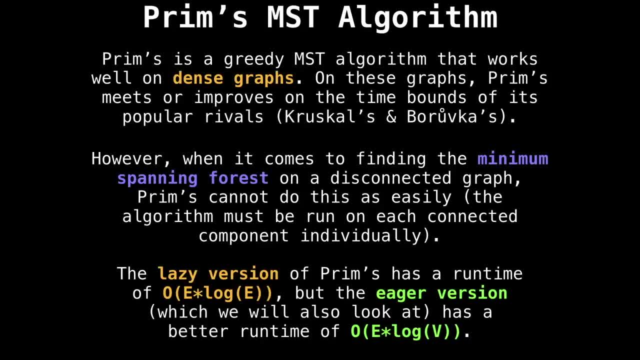 spanning tree, So it works very well on dense graphs which have a lot of edges. However, a few downsides to Prim's is that it's not easily parallelized, So it's not going to be as parallelizable, or at least not as parallelizable as other well known minimum. 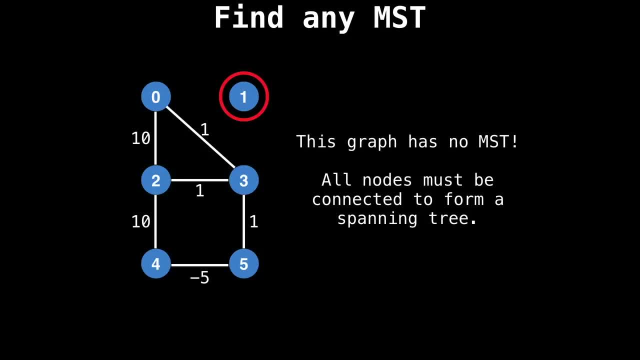 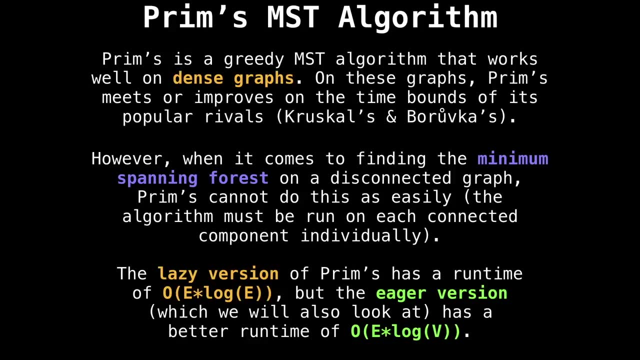 nodes must be connected on a single component for a spanning tree to exist. Let's change focus and start talking about prims algorithm. prims is one of my favorite minimum spanning tree algorithms Because of how simple and how intuitive it is. By nature, it's a greedy algorithm which 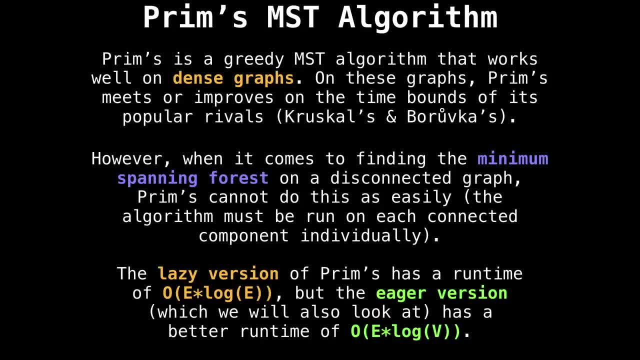 always selects the next best edge and adds it to the minimum spanning tree. So it works very well on dense graphs which have a lot of edges. However, a few downsides to prims is that it's not easily parallelizable, or at least not as parallelizable as other well. 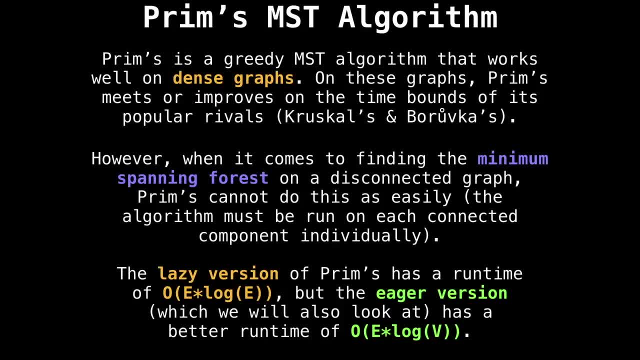 known minimum spanning tree algorithms And it's slightly harder but not impossible to find the minimum spanning forest of a graph. There are two well known versions of prims I want to discuss. The first is the common lazy version, which runs in big O, of E log. 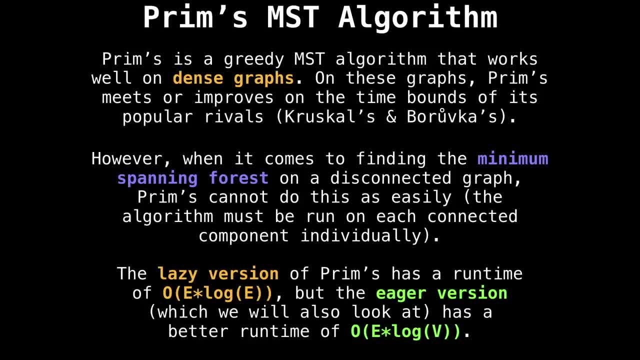 E. And then there's the improved eager version, which runs in big O, of E log V but requires a slightly different data structure. We're going to have a look at both, but this video is primarily going to focus on the lazy version. Let's start by looking at the lazy version. 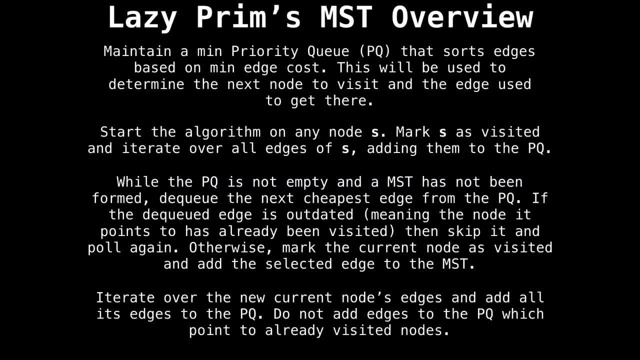 Just because it's slightly easier to implement. Here's the general idea: maintain a priority queue that sorts edges based on minimum edge cost. This product queue is used to tell you which node to go to next and what edge was used to get there. Then the algorithm begins. 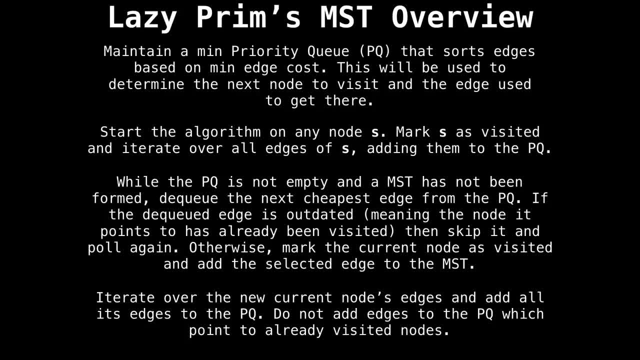 and we start on any starting node s and Mark as visited and iterate over all the edges of s and add them to the priority priority queue. From this point on, while the priority queue is not empty and a minimum spanning tree has not been formed, dequeue the next best edge from the priority queue. 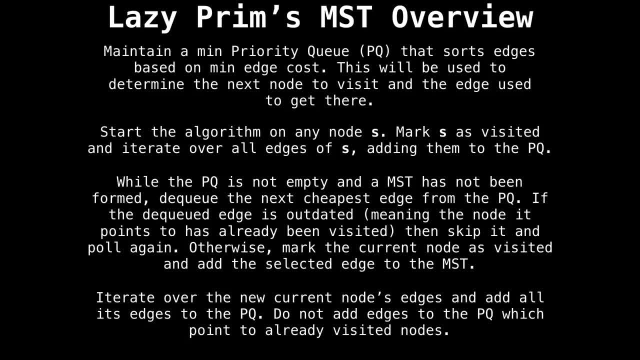 If the dequeued edge is not outdated, which it could be. if we visit the node that edge points to via another path before getting to the edge we just pulled, then we want to mark the current node as visited and add the selected edge to the priority queue, If you. 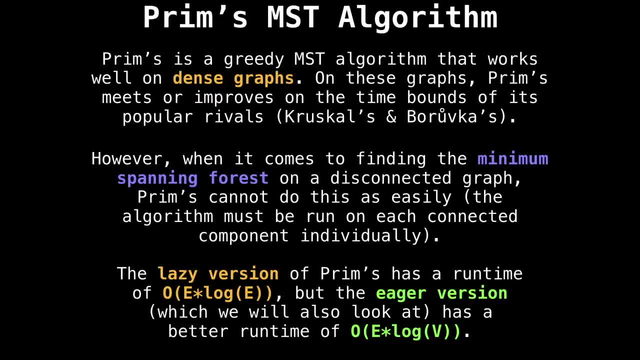 spanning tree algorithms And it's slightly harder but not impossible to find the minimum spanning forest of a graph. There are two well known versions of prims I want to discuss. The first is the common lazy version, which runs in big O, of e, log, e, And then there's 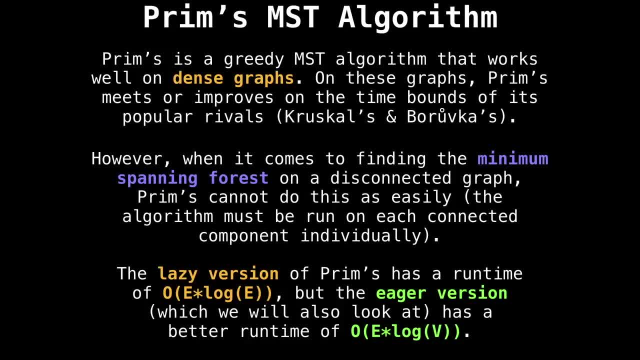 the improved eager version, which runs in big O of e log v But requires a slightly different data structure. We're going to have a look at both, but this video is primarily going to focus on the lazy version. Let's start by looking at the lazy version. 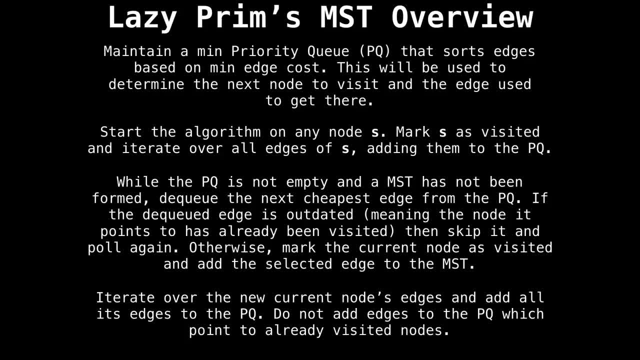 just because it's slightly easier to implement. Here's the general idea: maintain a priority queue that sorts edges based on minimum edge cost. This particular queue is used to tell you which node to go to next and what edge would use use to get there. Then the algorithm. 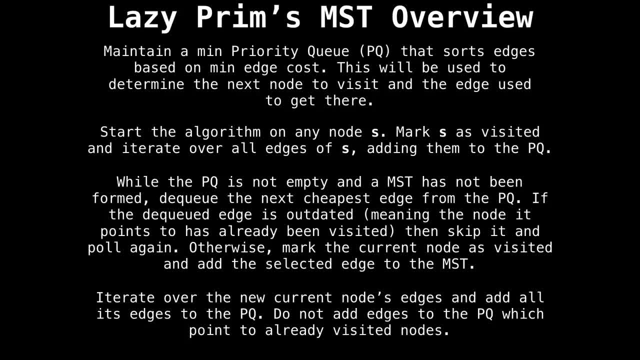 begins and we start on any starting node, s and Mark s as visited, and iterate over all the edges of s and add them to the priority queue. From this point on, while the priority queue is not empty and a minimum spanning tree has not been formed, dequeue the next best edge. 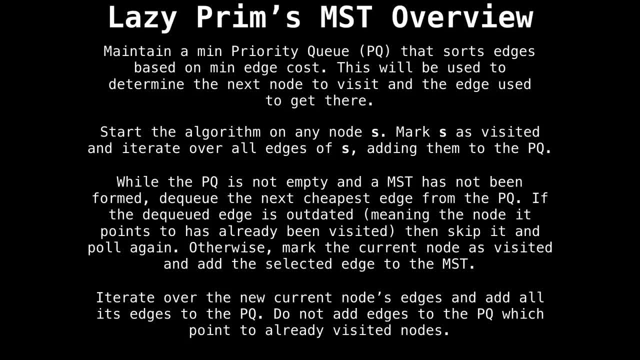 from the priority queue If the dequeued edge is not outdated, which it could be. if we visit the node that edge points to via another path. Before getting to the edge we just pulled, then we want to mark the current node as visited and add the selected edge to the priority queue. If you selected a stale, outdated edge, 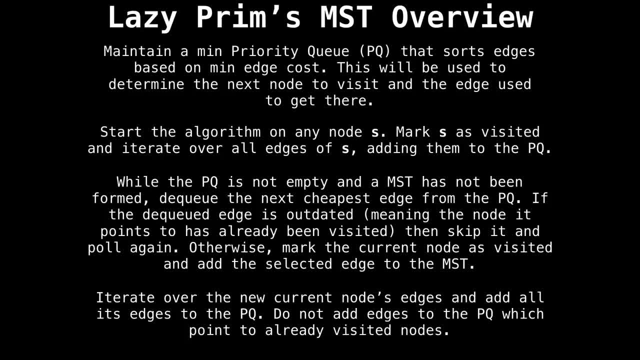 then you can simply pull again, then repeat the process of iterating over the current nodes, edges, adding them to the party queue, And while doing all this, take care not to add edges which already point to visited nodes. This will reduce the number of outdated edges. 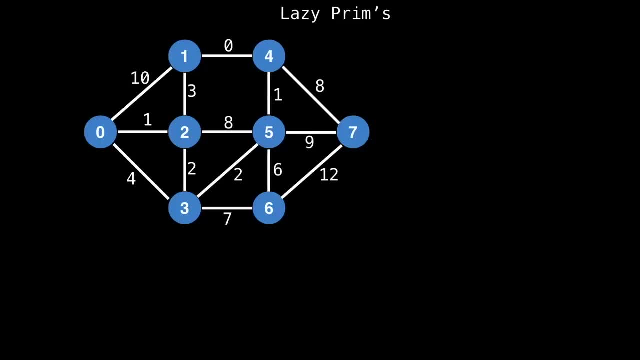 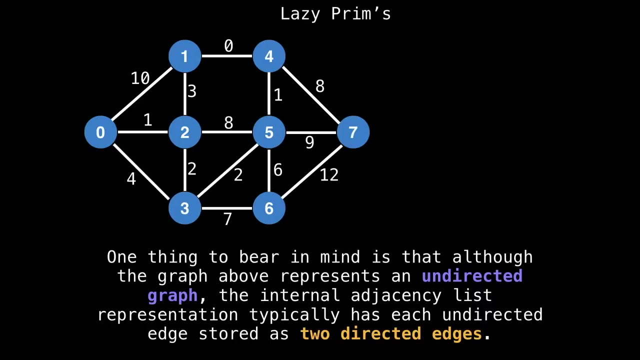 in the priority queue. Let's look at the priority queue. Let's have a look at an example. Suppose we have this weighted undirected graph and we want to find any minimum spanning tree. An important thing to keep in mind is that, while the graph above represents an undirected graph, our internal adjacency list representation. 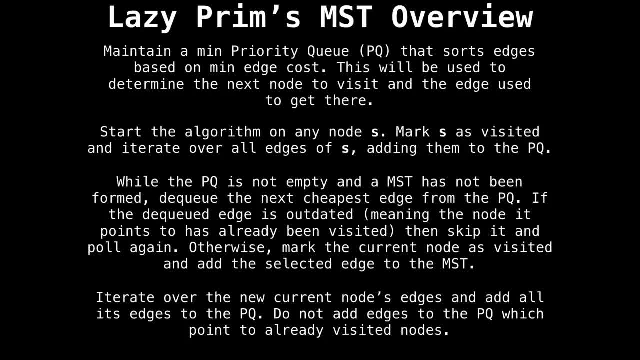 selected a stale, outdated edge, then you can simply pull again, then repeat the process of iterating over the current nodes, edges, adding them to the party queue, And while doing all this, take care not to add edges which already point to visited nodes. This 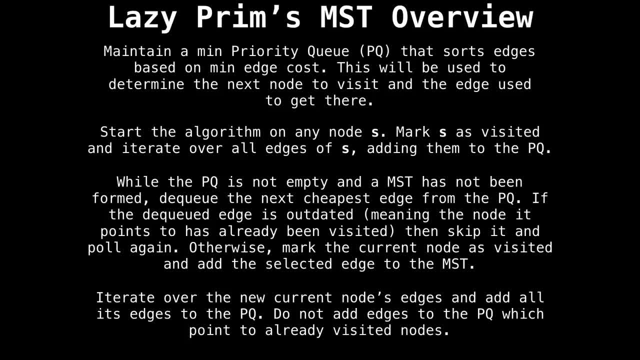 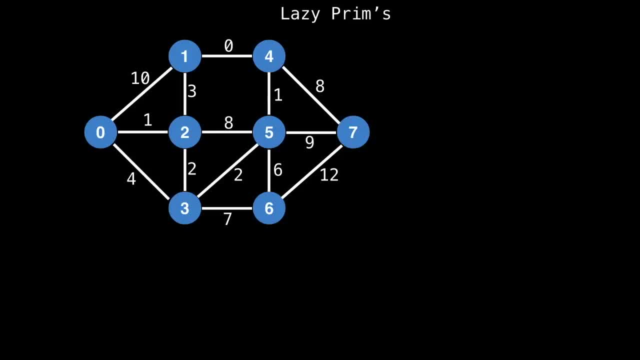 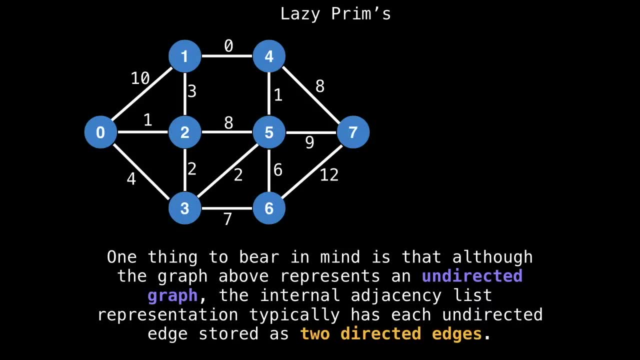 will reduce the number of outdated edges in the priority queue. Let's have a look at an example. Suppose we have this weighted undirected graph and we want to find any minimum spanning tree. Okay, An important thing to keep in mind is that, while the graph above represents an 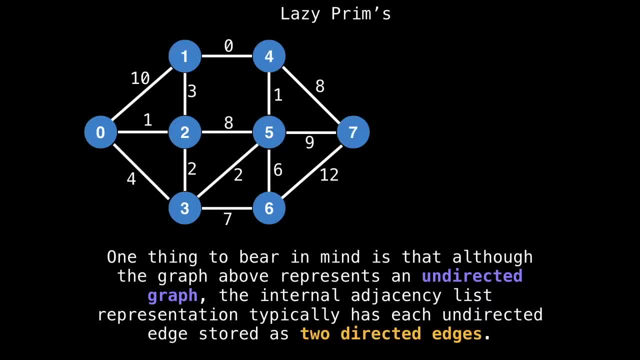 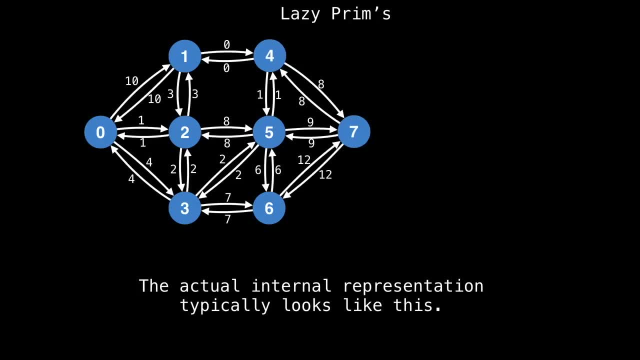 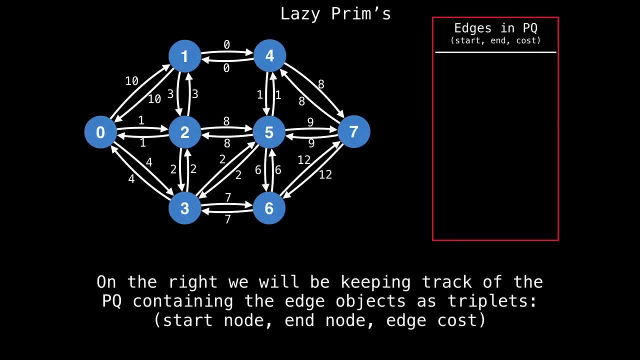 undirected graph. our internal adjacency list representation has each undirected edge stored as two directed edges, So the actual internal representation typically looks something like this, which is a lot easier to work with. Along with the graph, I will also be keeping track of the edges currently in the priority queue on the right. 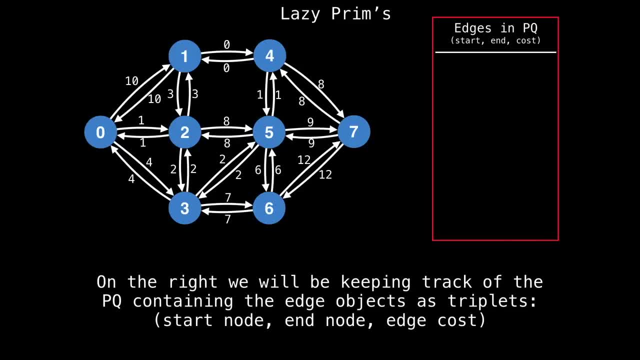 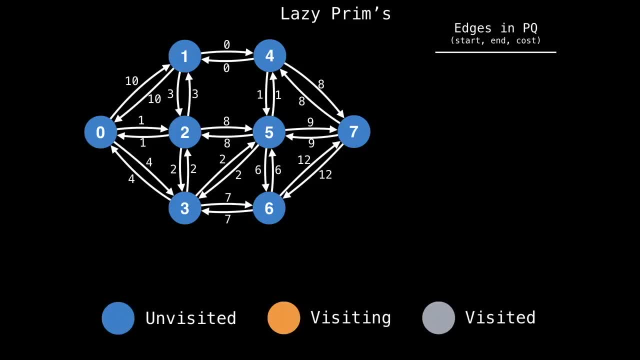 I will be representing edges as triplets containing the start node of the edge, the end node of the edge and the edge cost. Lastly, I will be coloring nodes as either blue for unvisited, orange for visiting or gray for visited. So let's begin prims on node zero, Iterate over 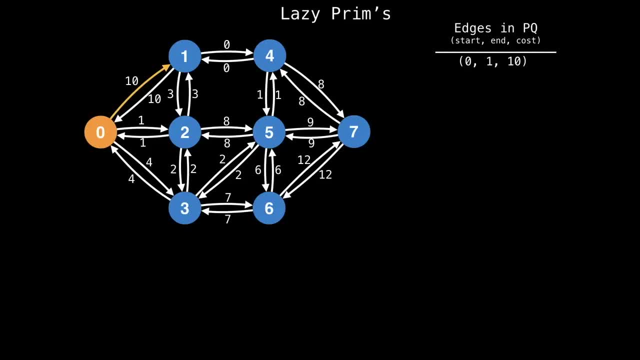 all the outgoing edges and add them to the priority. The first edge will be the one that we're going to add to the priority queue, is the edge from zero to one with a cost of 10.. Then the edge from zero to two with a cost of one, And finally the edge from zero to three with a cost. 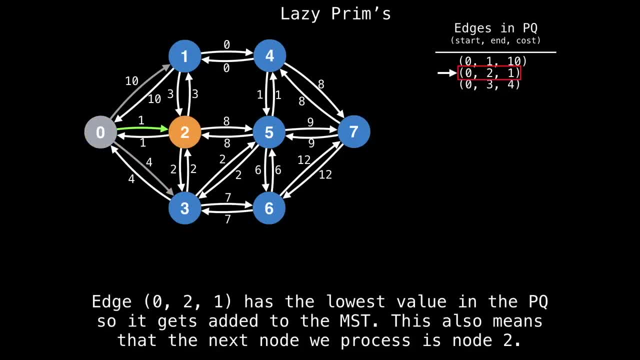 of four. Now we look inside our priority queue and we pull the next most promising edge and add it to the minimum spanning tree. the edge from zero to two with a cost of one has the lowest value in the priority queue, So it gets added to the minimum spanning tree. This also means that the next node we process is node two. 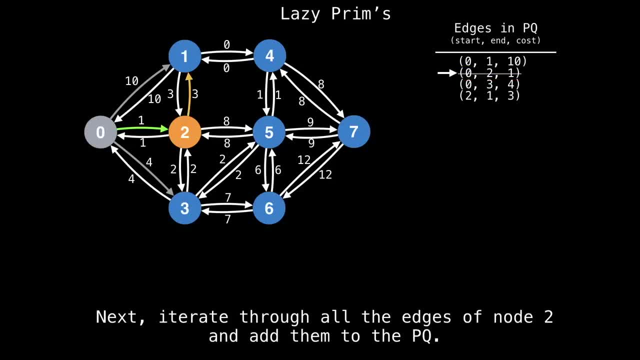 So next, we iterate through all the edges of node two and add them to the priority queue. While entering over the outgoing edges of node two realize that we may encounter edges which point to already visited nodes. we do not want to add these to the priority queue because they 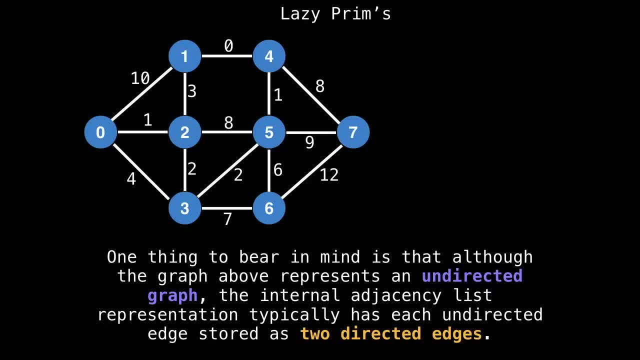 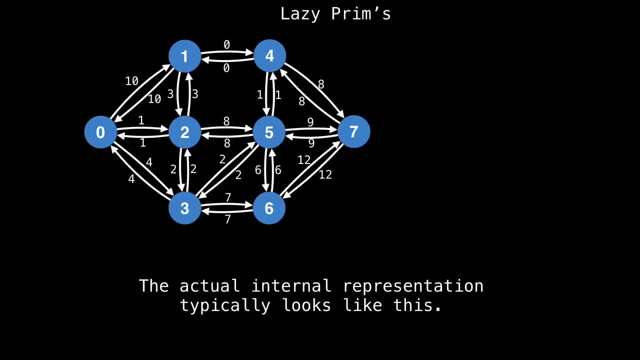 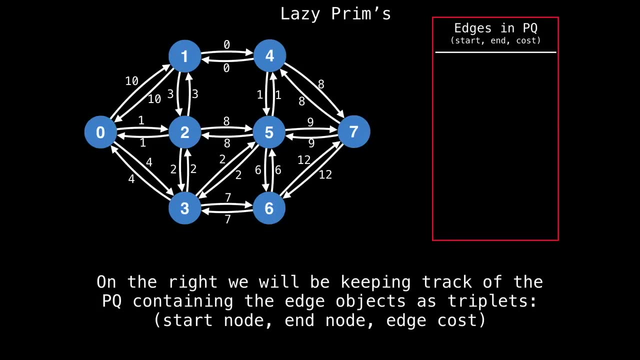 has each undirected edge stored as two directed edges, So the actual internal representation typically looks something like this, which is a lot easier to work with. Along with the graph, I will also be keeping track of the edges currently in the priority queue. on the right, I will be representing edges as triplets containing the start node. 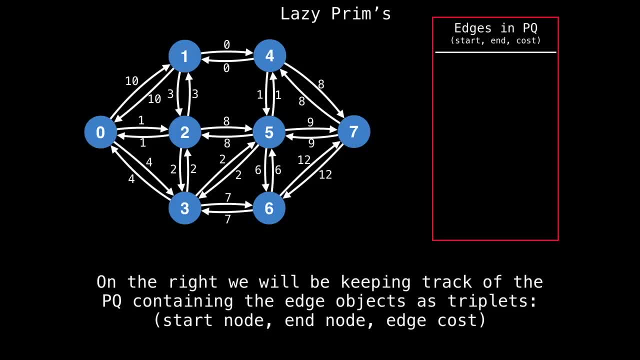 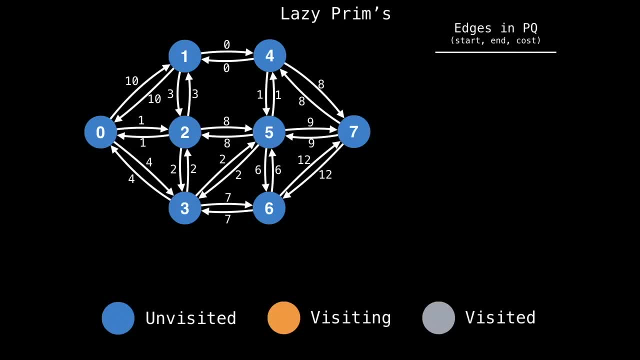 of the edge, the end node of the edge and the edge cost. Lastly, I will be coloring nodes as either blue for unvisited, orange for visiting or gray for visited. So let's begin, prims, on node zero, iterate over all the outgoing edges and add them to the priority, The first edge. we're. 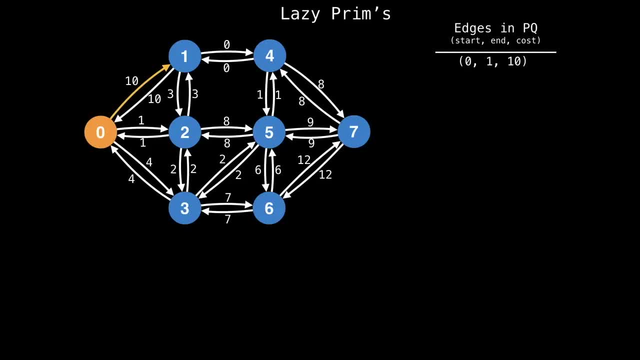 going to add to the priority queue is the edge from zero to one, with a cost of 10.. Then the edge from zero to two with a cost of one, And finally the edge from zero to three with a cost of four. Now we look inside our priority queue and we pull the next most promising. 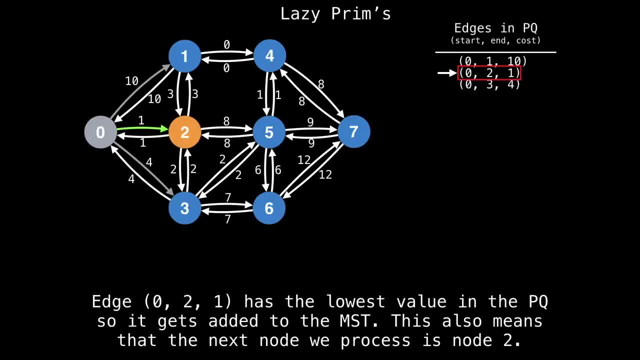 edge and add it to the minimum spanning tree. The edge from zero to two with a cost of one has the lowest value in the priority queue, So it gets added to the minimum spanning tree. This also means that the next node we process is node two. 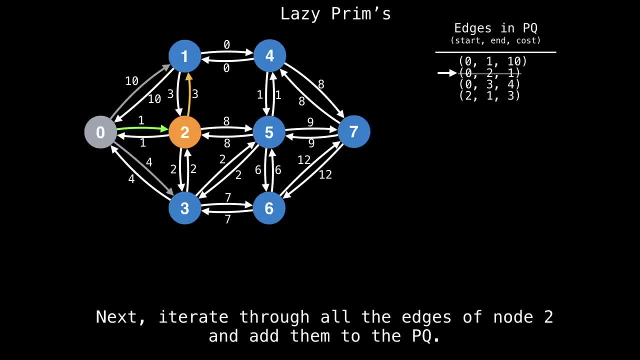 So next we iterate through all the edges of node two and add them to the priority queue. While entering over the outgoing edges of node two realize that we need to add them to the priority queue. We can see that we may encounter edges which point to already visited nodes. we do not. 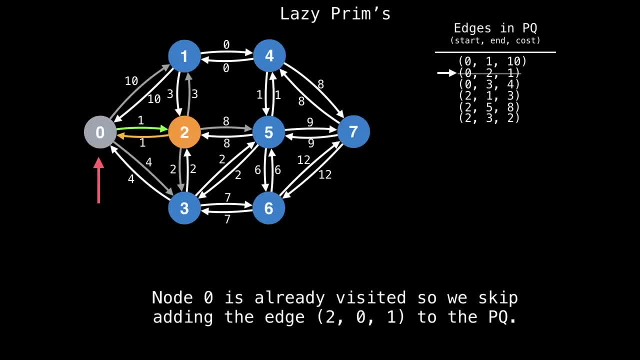 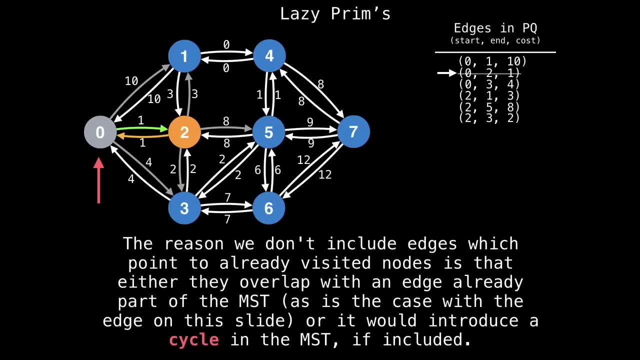 want to add these to the priority queue, because they are of no use. The reason we don't include edges which already point to visited nodes is that either they overlap with an edge already part of the minimum spanning tree, as is the case with the edge on the slide, or they would 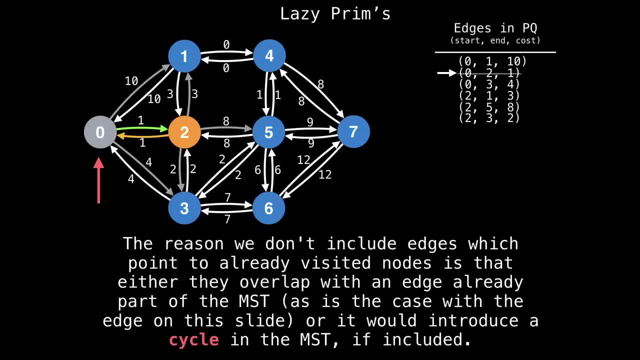 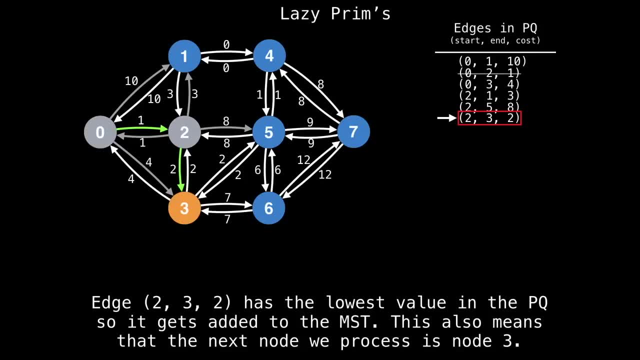 introduce a cycle in the minimum spanning tree, if included, which is forbidden, So we can add edges to the priority queue. So the next best edge in the priority queue is the edge from two to three with a cost of two, So it gets added to the minimum spanning tree. This also means that the next node we 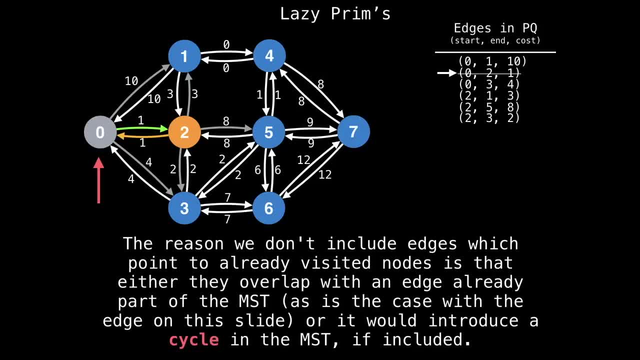 are of no use. The reason we don't include edges which already point to visited nodes is that either they overlap with an edge already part of the minimum spanning tree, as is the case with the edge on the slide, or they would introduce a cycle in the minimum spanning tree if included, which is 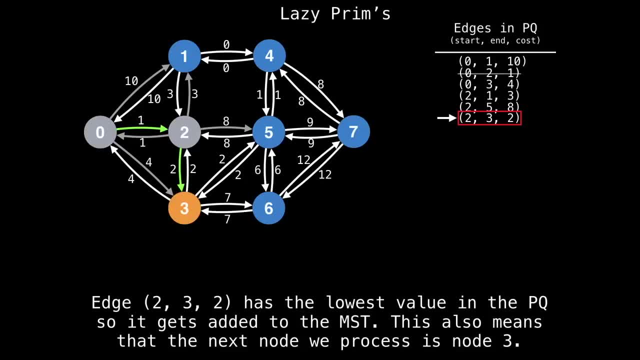 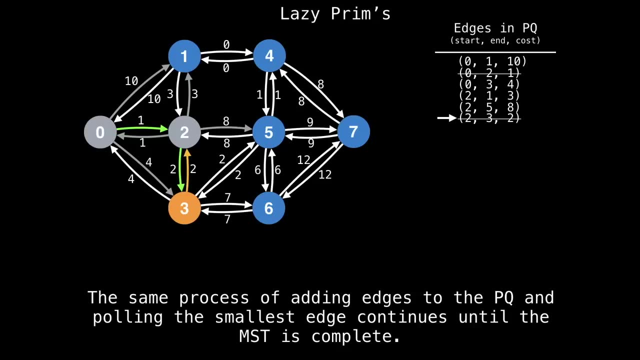 forbidden. So the next best edge in the priority queue is the edge from two to three with a cost of two. So it gets added to the minimum spanning tree. This also means that the next node we process is node three, The same process of adding edges to the. 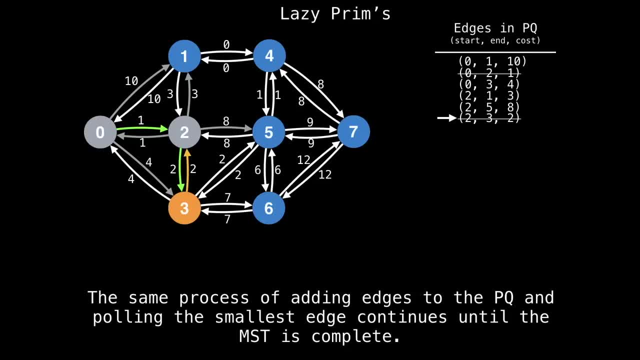 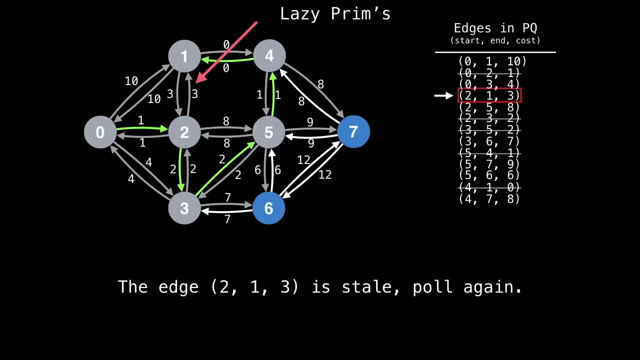 priority queue and pulling the smallest edge continues until the minimum spanning tree is complete. I'll let the animation play until something interesting happens. All right, notice that the next best edge we pull from the priority queue is an edge which already points to a visited node, node one. This means that the edge is outdated and stale because we 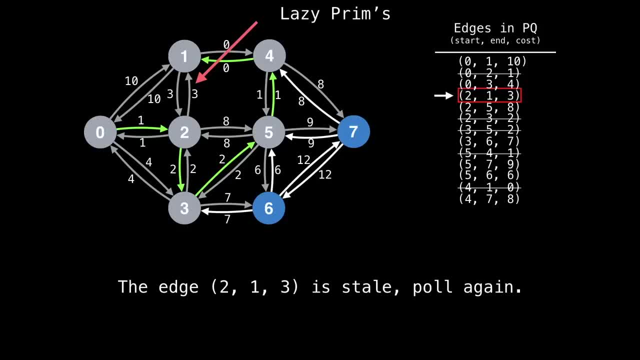 find that the edge from the priority queue is already out of the priority queue. So we can't find a cheaper path to node one. So we can safely ignore this edge and pull again. The next edge is also stale, So let's keep pulling. 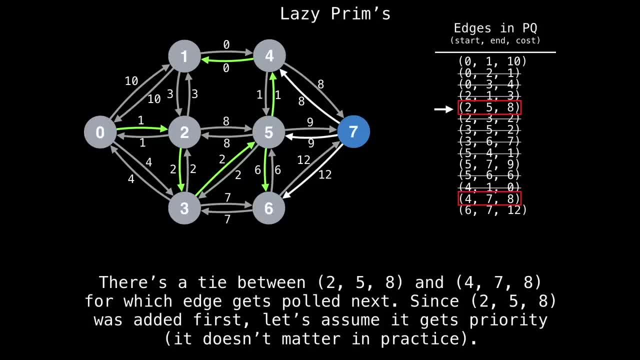 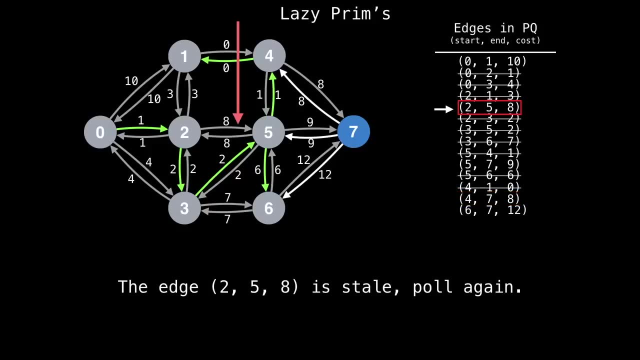 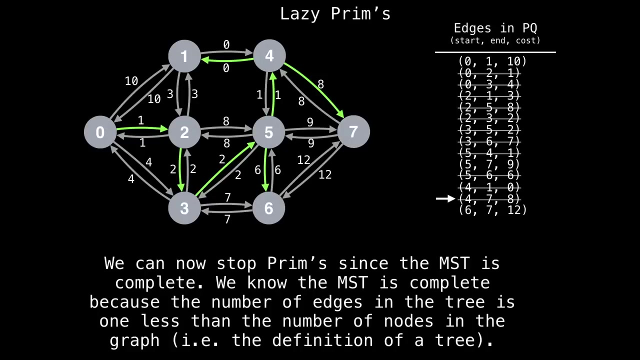 So what happens when we have two edges with the same cost in the priority queue? Which one gets pulled first? In practice this this doesn't matter. So we can assume that edge 258 gets pulled first because it was added first. We can now stop prisms because the minimum spanning tree is complete. We know the minimum. 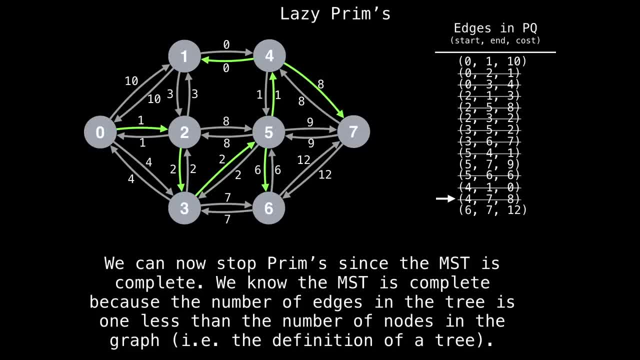 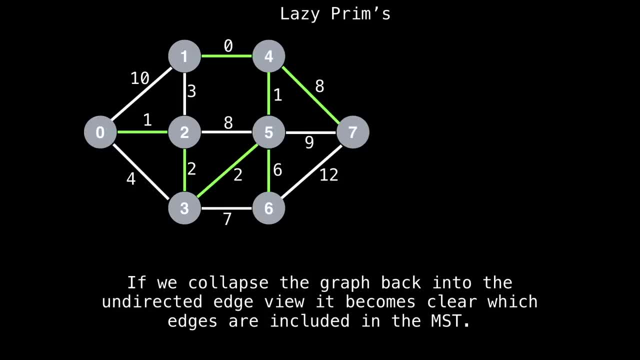 spanning tree is complete because the number of edges in the tree is one less than the number of, less than the number of nodes in the graph. This is precisely the definition of a tree. If we collapse the graph back into the undirected edge view, it becomes clear which edges are. 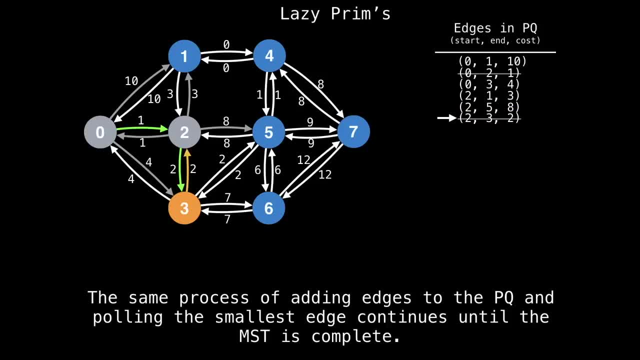 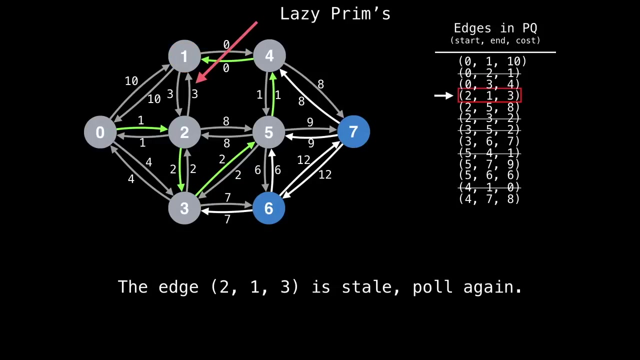 process is node three. The same process of adding edges to the priority queue and pulling the smallest edge continues until the minimum spanning tree is complete. I'll let the animation play until something interesting happens. All right, notice that the next best edge we pull from the priority queue is an edge. 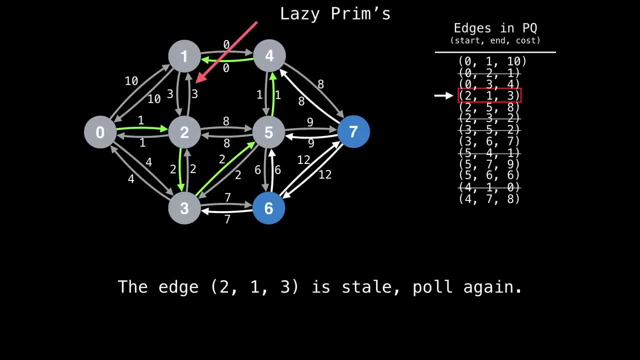 which already points to the priority queue. All right, notice that the next best edge we pull from the priority queue is an edge which already points to a visited node, node one. This means that the edge is outdated and stale because we found a cheaper path to node one, So we can safely ignore this. 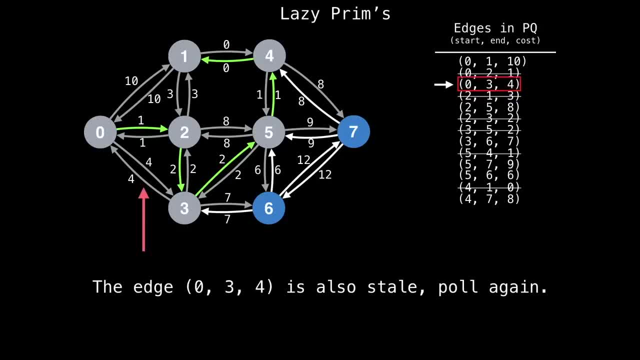 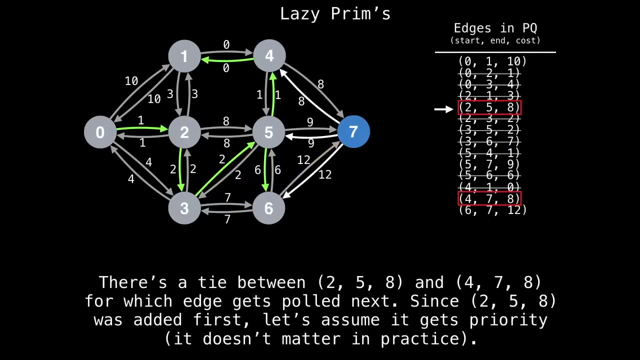 edge and pull again. The next edge is also stale, So let's keep pulling. So what happens here? This happens when we have two edges with the same cost in the priority queue. which one gets pulled first? In practice this doesn't matter, So we can assume that edge 258 gets. 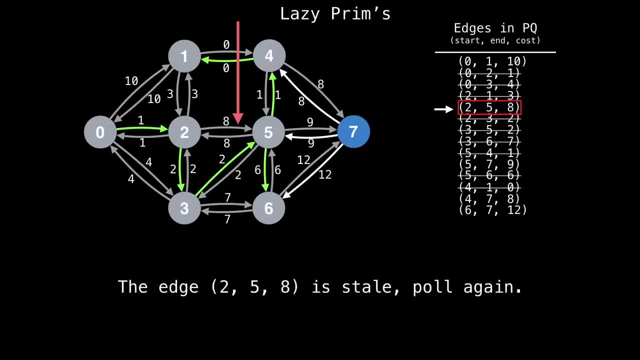 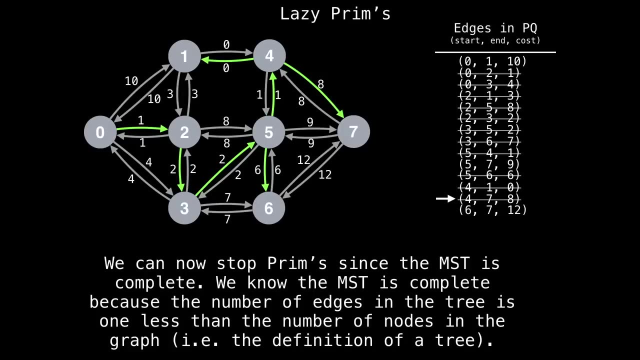 pulled first because it was added first. We can now stop prims because the minimum spanning tree is complete. We know the minimum spanning tree is complete because the number of edges in the tree is one less than the number of nodes in the graph. This is precisely the. 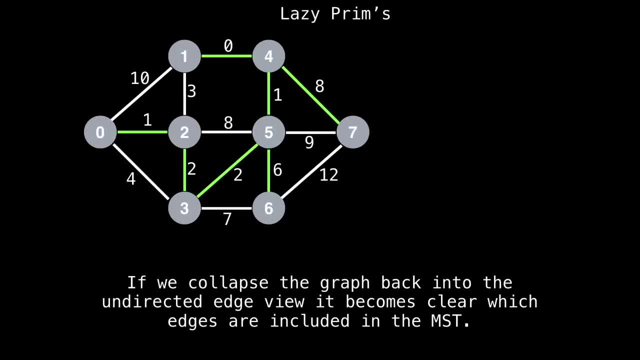 definition of a tree. If we collapse the graph back into the undirected edge view, it becomes clear which edges are included in the minimum spanning tree. To find the cost of the minimum spanning tree is simply sum up the cost of all the edges which were selected to be put. 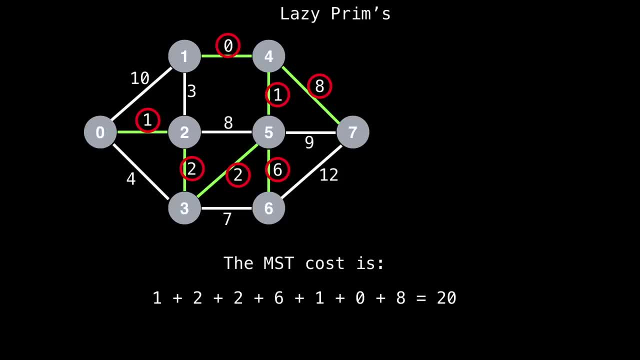 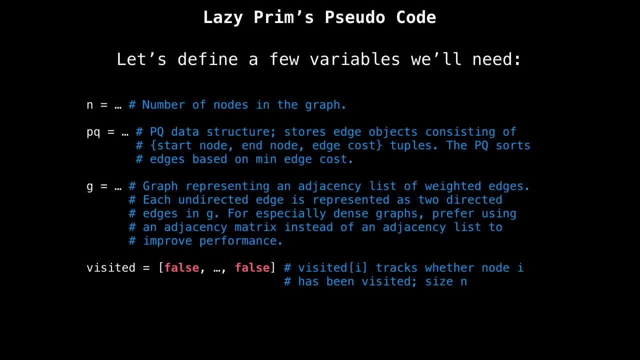 in part of the minimum spanning tree, And this totals to 20.. Great, we now understand the gist of the lazy implementation of prims. Let's have a look at some pseudocode. Let me first define a few variables that we will need. First is n the number of nodes and graph. 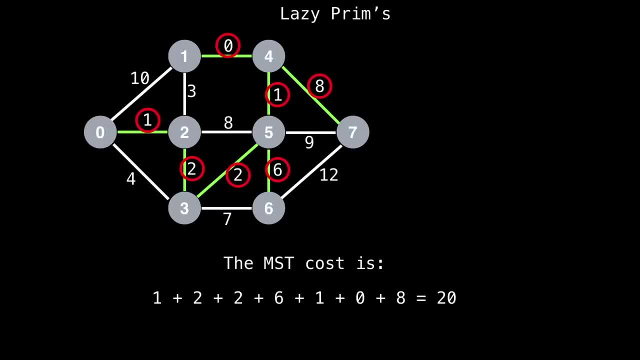 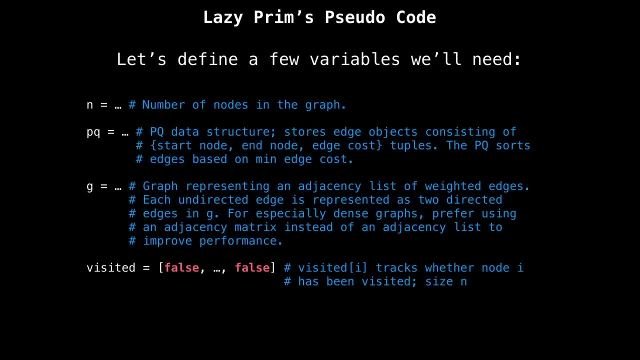 included in the minimum spanning tree. To find the cost of the minimum spanning tree is simply sum up the cost of all the edges which were selected to be part of the minimum spanning tree, and this totals to 20.. Great, we now understand the gist of the lazy implementation. 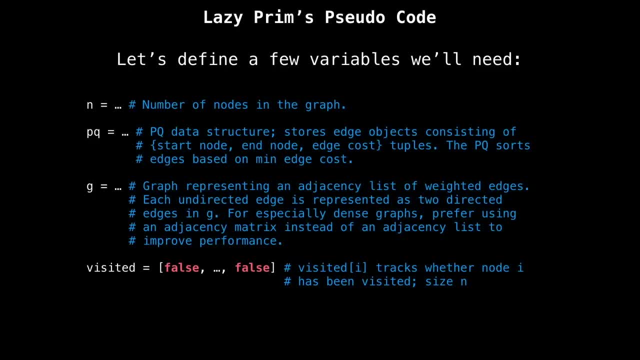 of prims. Let's have a look at some pseudocode. Let me first define a few variables that we will need. First is n the number of nodes in the graph. The variable pq represents the priority queue data structure. it stores the edge objects based on minimum edge cost And 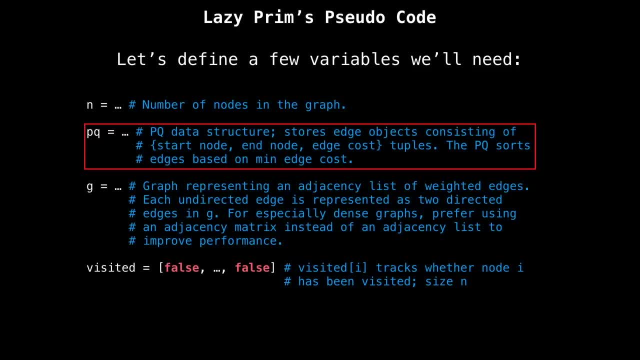 cost. Again, each edge object consists of a start node, an end node and an edge cost. Next is G, which represents the graph we're working with. G represents an adjacency list of weighted edges. In G, every undirected edge is represented as two directed edges. 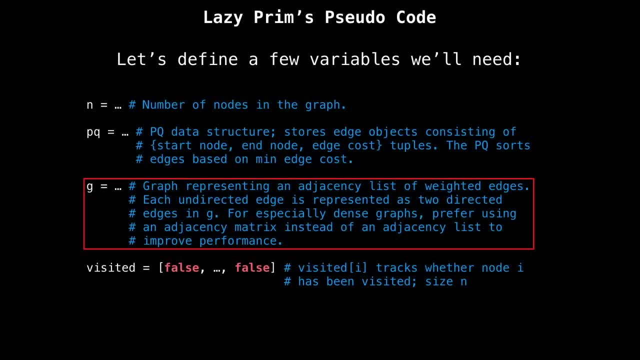 As a side note, if your graph is extremely dense, meaning it has numerous edges, you should probably prefer using an adjacency matrix instead of an adjacency list for efficiency and space gains. And lastly, a visited Boolean array of size n which keeps track of whether 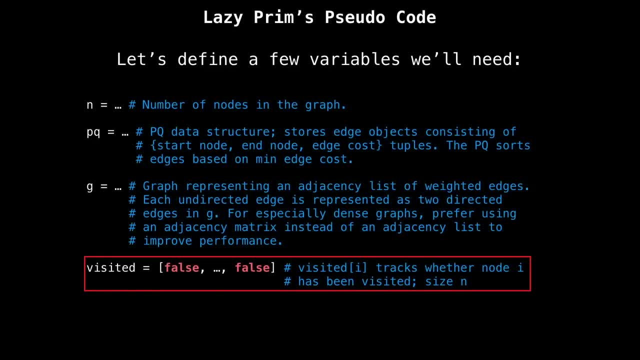 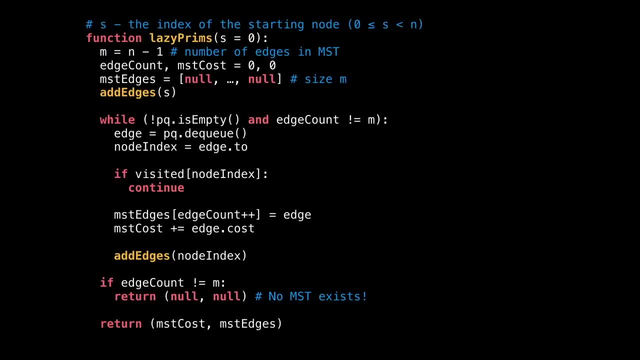 node i has been visited or not. So on this slide is the whole algorithm for the lazy implementation of prims. Let's go over it one step at a time. The function takes one argument, s, which is the start node index, And by default s is set to node zero. 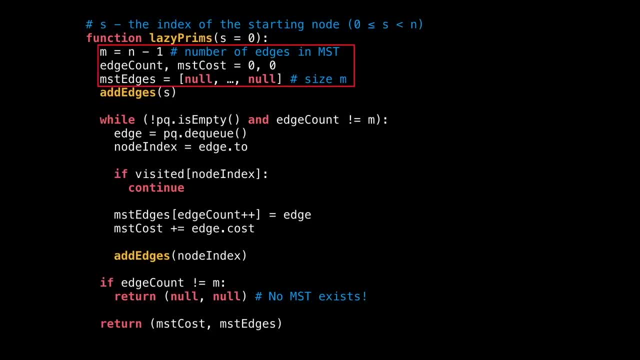 Then I define a few more variables that we'll need just inside this function. M is a constant representing the number of expected edges in the minimum spanning tree. edge count is the number of edges we currently have included in the minimum spanning tree. This variable. 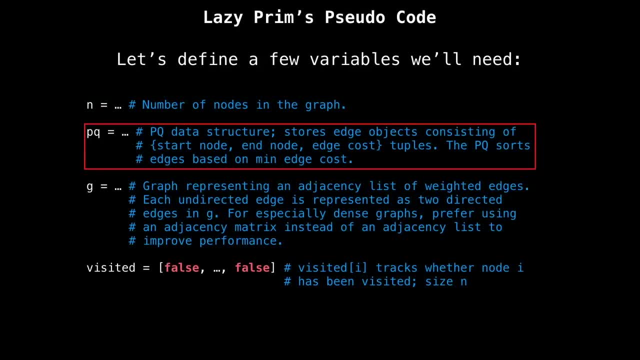 The variable PQ represents the priority queue data structure. it stores the edge objects based on min minimum edge cost. Again, each edge object consists of a start node and end node and an edge cost. Next is G, which represents the graph we're working with. G represents 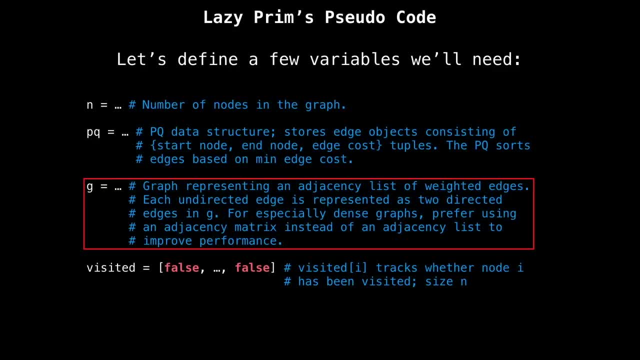 an adjacency list of weighted edges. In G, every undirected edge is represented as two directed edges. As a side note, if your graph is extremely dense, meaning it has numerous edges, you should probably prefer using an adjacency matrix instead of an adjacency. 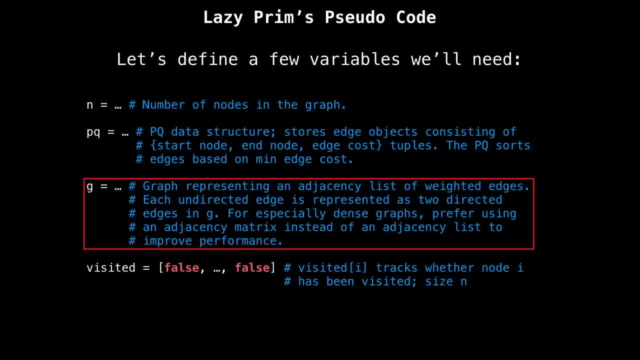 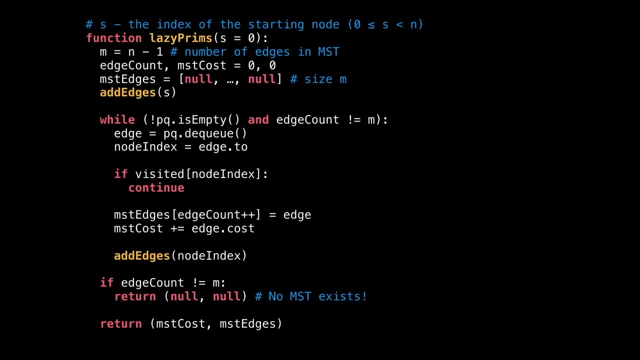 list for efficiency and space gains. And lastly, a visited Boolean array of size n which keeps track of whether node i has been visited or not. So on this slide is the whole algorithm for the lazy implementation of prims. Let's go over it one step at a time. 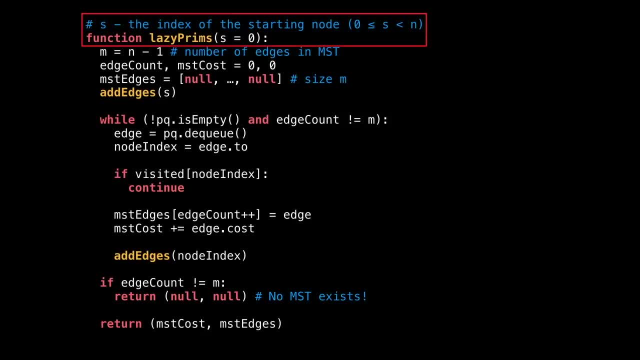 The function takes one argument, s, which is the start node index, And by default s is set to node zero. Then I define a few more variables that will need just inside this function. M is a constant representing the number of expected edges in the minimum spanning. 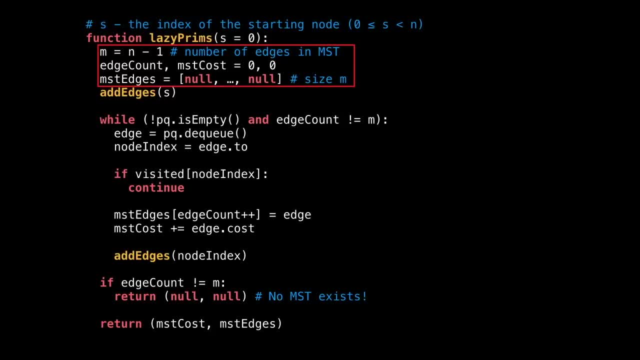 tree edge count is the number of edges we currently have included in the minimum spanning tree. This variable is to make sure that the tree spans the whole graph. MST cost tracks the total cost of the minimum spanning tree And finally, MST edges is an. 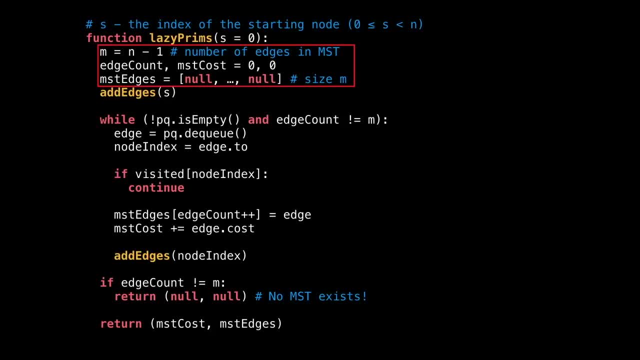 array which holds edges which we have included in the minimum spanning tree. The first actual bit of logic we do is add all the outgoing edges from s to the priority queue with the add edges method. So let's look at this method and see what's going on in there. 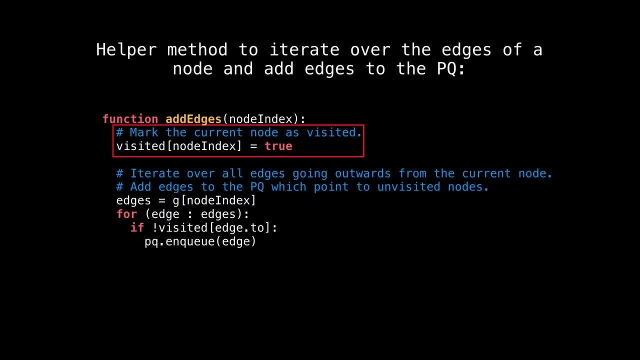 Alright, here we are at the add edges function. The first thing I do is mark the current node as visited. Next I iterate through all the outgoing edges of the current node And, if the destination node is unvisited, add the edge to the priority queue. So that's all. 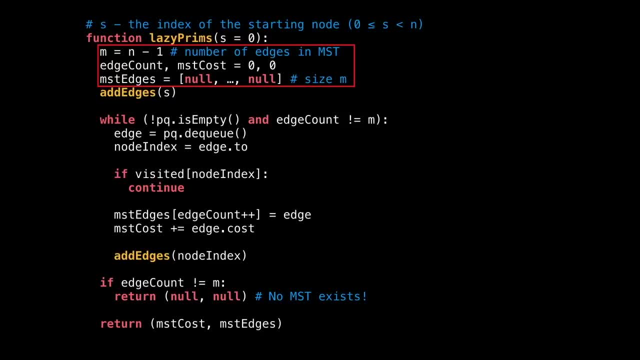 is to make sure that the tree spans the whole graph. MST cost tracks the total cost of the minimum spanning tree And, finally, MST edges is an array which holds edges which we have included in the minimum spanning tree. The first actual bit of logic we do is add all the outgoing edges from s to the priority queue with the. 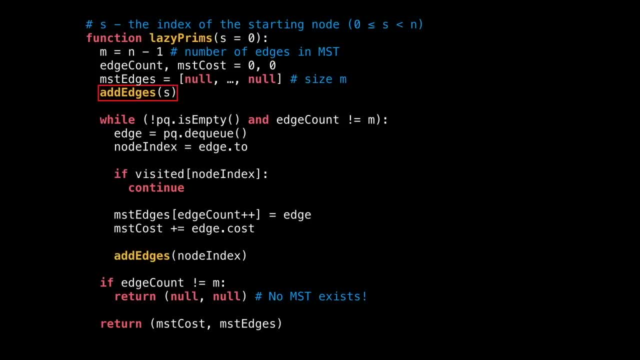 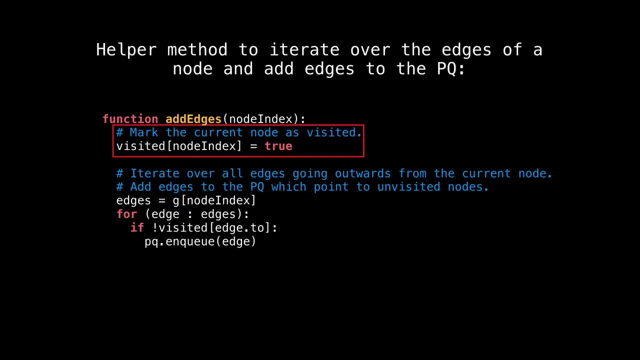 add edges method. So let's look at this method and see what's going on in there. All right, here we are In the add edges function. the first thing I do is mark the current node as visited. Next I iterate through all the outgoing edges of the current node And if the destination 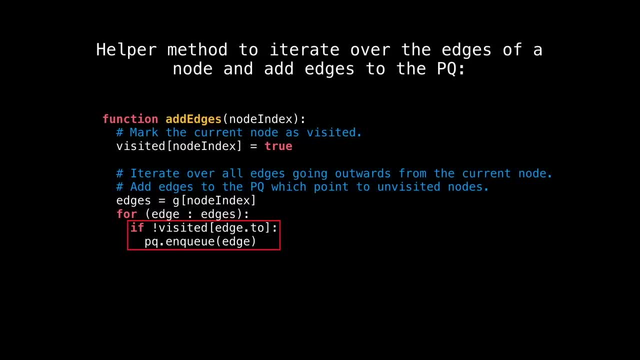 node is unvisited. add the edge to the priority queue. So that's all this method does, is it goes through all the edges of a node and adds them to the priority queue, if appropriate. Once we've added the first set of edges to the priority queue, the algorithm really begins. 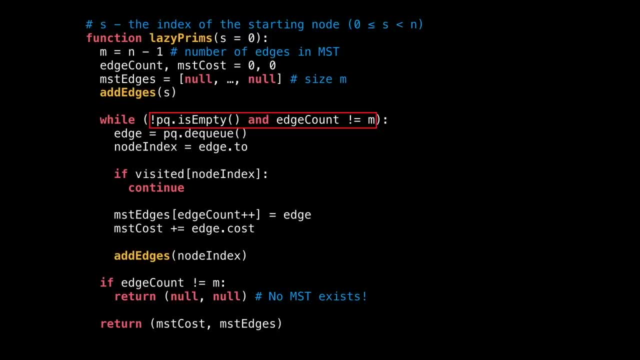 and we enter a while loop. While the priority queue is not empty and the minimum spanning tree is not complete, keep iterating. then, inside the loop, we pull the next best edge out of the priority queue and grab a reference to the destination node index. This is the node the edge is pointing. 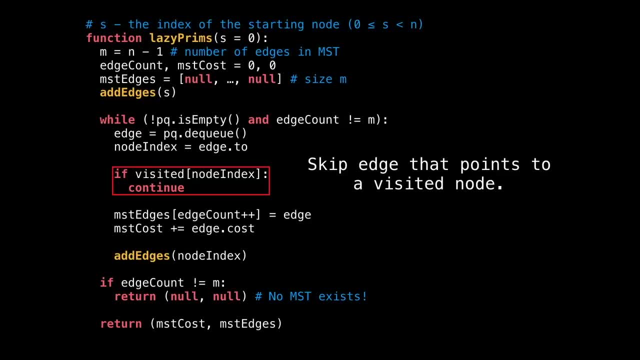 at This. next line is very important. It's the logic that skips adding an edge to the priority queue If that edge points to an already visited node. Again, edges can be become stale or outdated in the priority queue if the node they're pointing at becomes. 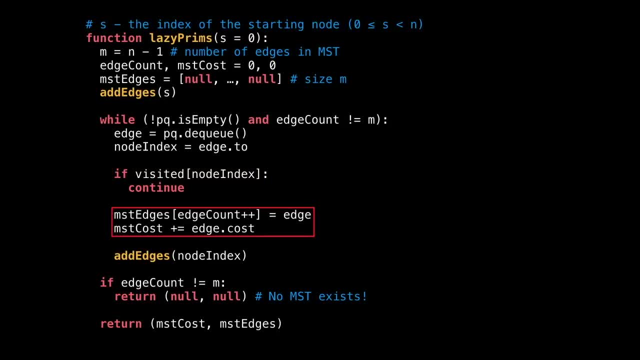 visited via another path. Next, actually add the edge to the minimum spanning tree by adding it to the amnesty edges array And, while adding the edge to the tree, also sum over the edge costs. The last thing we want to do is call the add edges method with the new current. 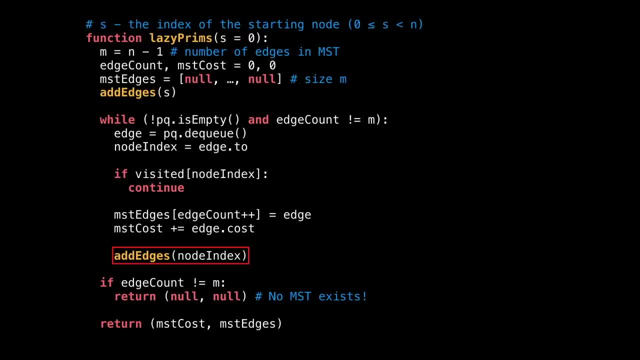 node Recall that this will add all the outgoing edges Pointing to unvisited nodes to the priority queue. And the very last thing is we make sure that we have actually found a minimum spanning tree that spans the entire graph And we return the edges along with the MST costs. Today we're talking about finding minimum. 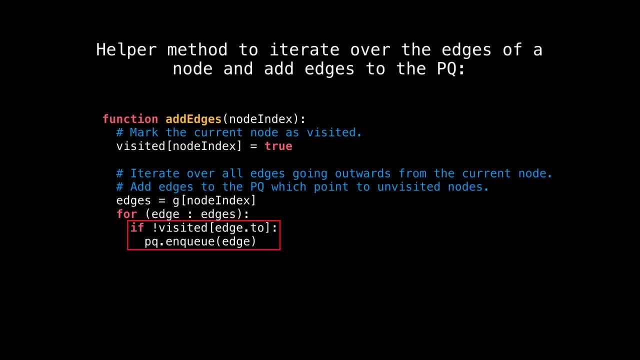 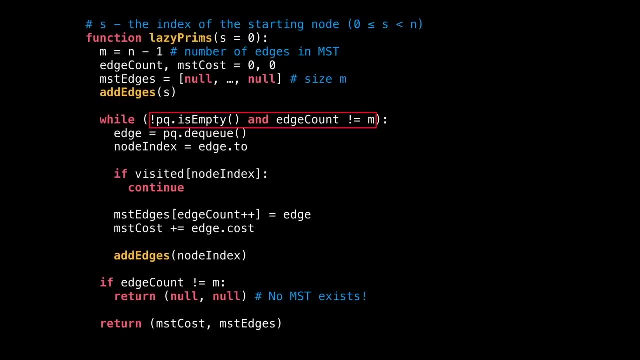 this method does is it goes through all the edges of a node and adds them to the priority queue, if appropriate. Once we've added the first set of edges to the priority queue, the algorithm really begins And we enter a while loop, While the priority queue is not empty and the minimum spanning. 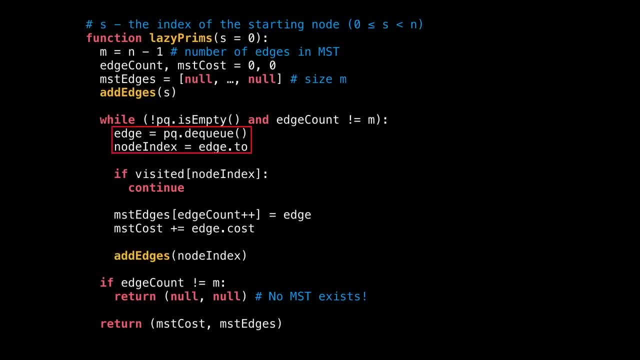 tree is not complete. keep iterating. Then inside the loop, we pull the next best edge out of the priority queue and grab a reference to the destination node index. This is the node the edge is pointing at. This next line is very important. It's the logic that skips. 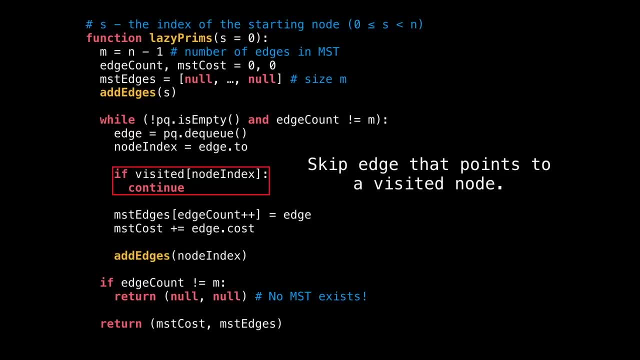 adding an edge to the priority queue If that edge points to an already visited node. again, edges can become stale or outdated in the priority queue if the node they're pointing at becomes visited via another path. Next, actually add the edge to the minimum spanning. 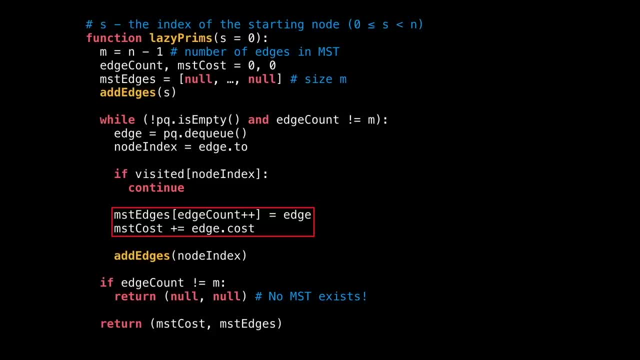 tree by adding it to the MST edges array And, while adding the edge to the tree, also sum over the edge costs. The last thing we want to do is call the add edges method with the new current node. So we have all the outgoing edges pointing to unvisited nodes to the priority queue. 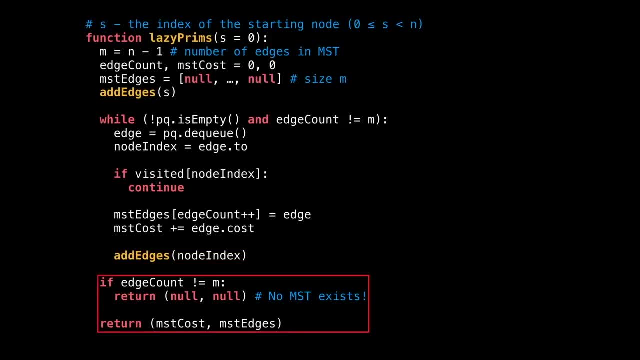 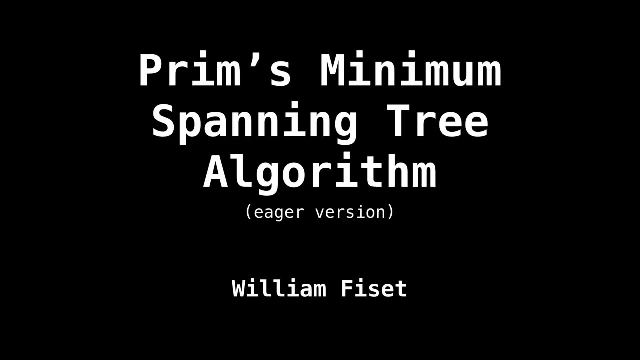 And the very last thing is, we make sure that we have actually found a minimum spanning tree that spans the entire graph And we return the edges along with the MST costs. Today, we're talking about finding minimum spanning trees with prims algorithm, The lazy implementation. 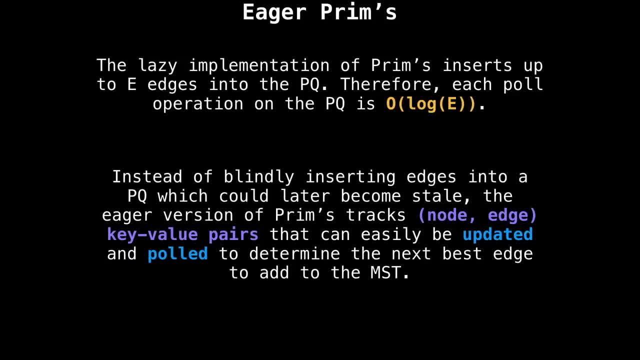 of prims inserts, he edges into a priority queue. This results in each pole operation on the priority queue to be big O of log e in the eager version. we maintain the idea that instead of adding edges to the priority queue, which can later become stale, 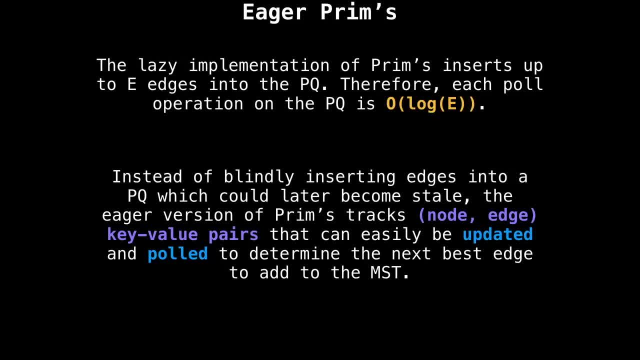 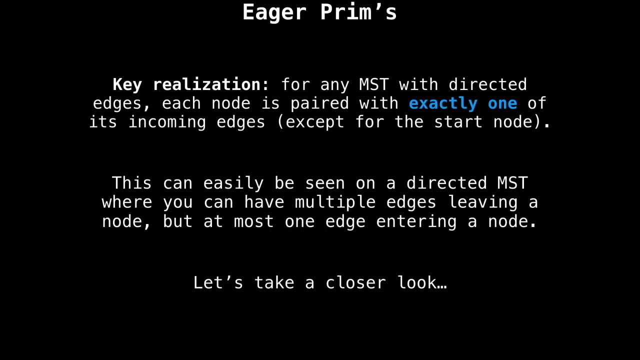 that instead we should track node edge key value pairs that can easily be updated and pulled to determine the next best edge. we should add to the minimum spanning tree. For this all to make sense, there's a key realization that needs to happen, And that is for any MST with directed edges. each node is paired with exactly one of its 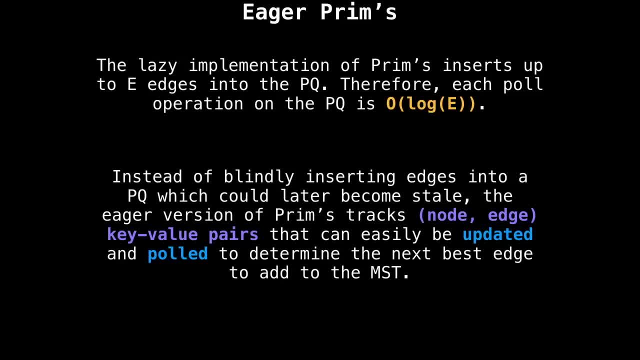 spanning trees with prims algorithm. The lazy implementation of prims inserts E edges into a priority queue. This results in each pole operation on the priority queue to be big O of log E In the eager version. we maintain the idea that instead of adding edges to the priority queue, which can later become stale, that instead we should: 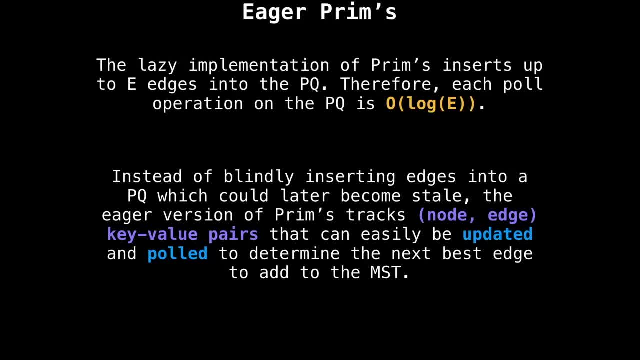 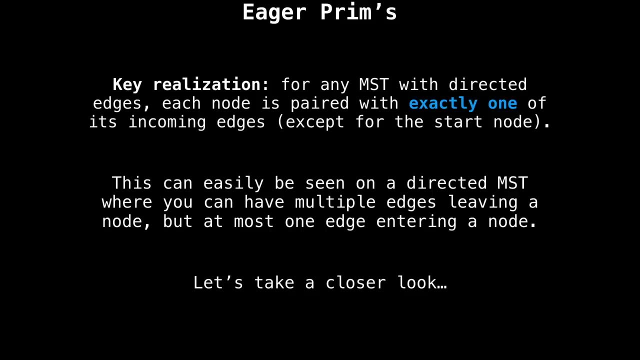 track node edge key value pairs that can easily be updated and pulled to determine the next best edge. we should add to the minimum spanning tree. For this all to make sense, there's a key realization that needs to happen, And that is for any MST with directed edges: each node is paired with exactly one of its incoming edges. 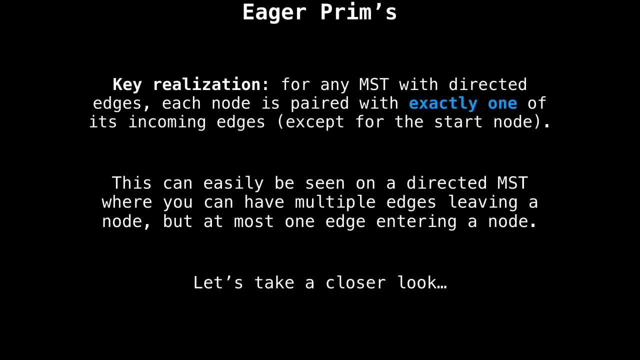 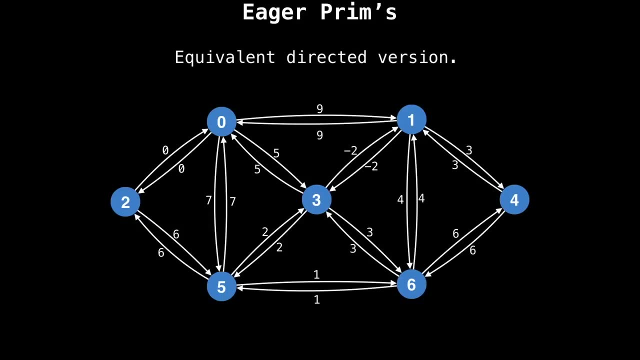 That is, except for the start node. One way to see this is on a minimum spanning tree with multiple edges leaving a node, but only ever one edge entering a node. Let's have a closer look at what I mean. Suppose we have this undirected graph, The equivalent directed. 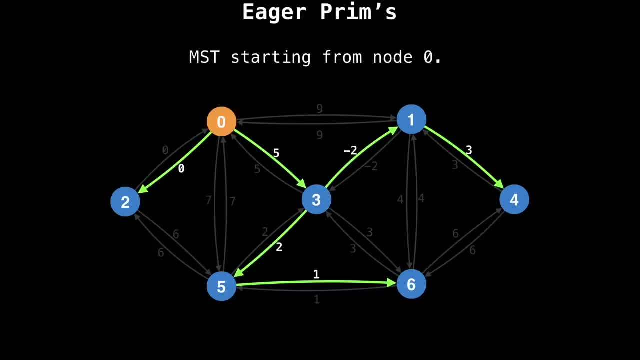 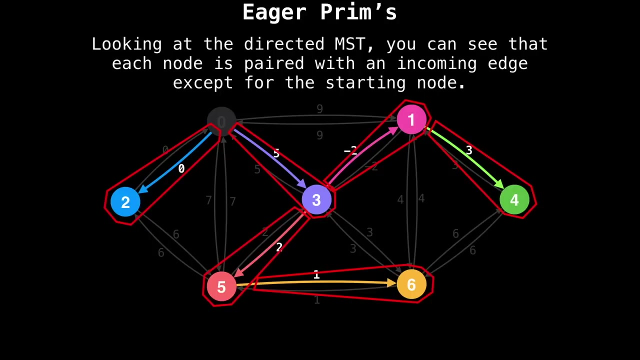 version of this graph looks like this: A possible minimum spanning tree starting at node zero might be the following, highlighted in green. Now notice that on this directed MST each node is paired with exactly one edge except for the starting node, So in a sense there seems to be a relationship. we 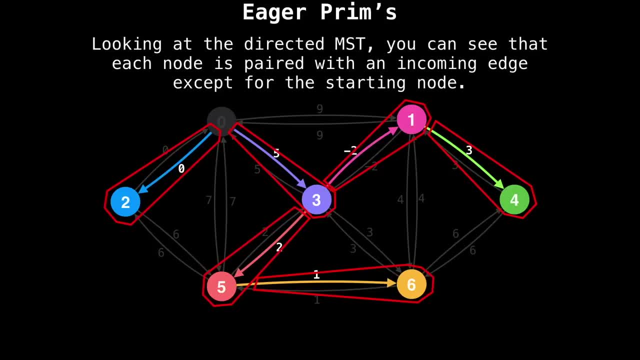 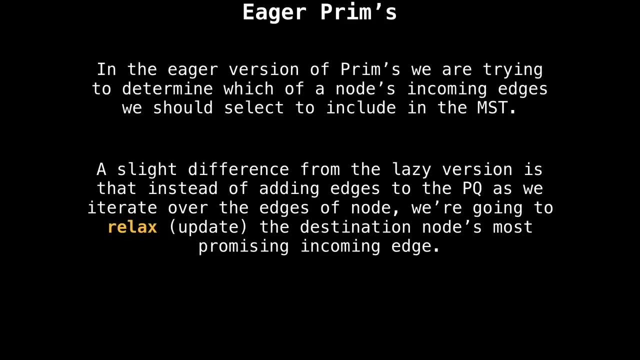 can take advantage of here, which is that each node is paired with exactly one incoming edge. In the eager version we are trying to determine which of a nodes incoming edges we should select to include in the MST. The main difference, coming from the lazy version, is that instead, 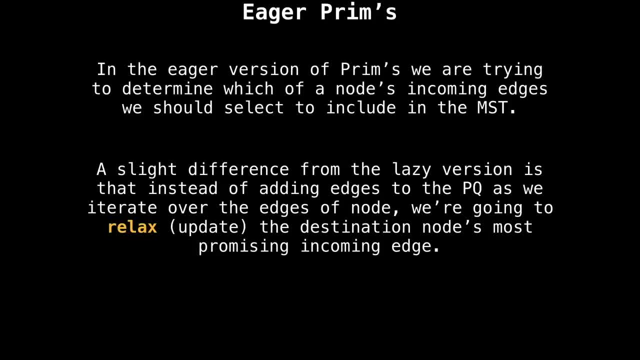 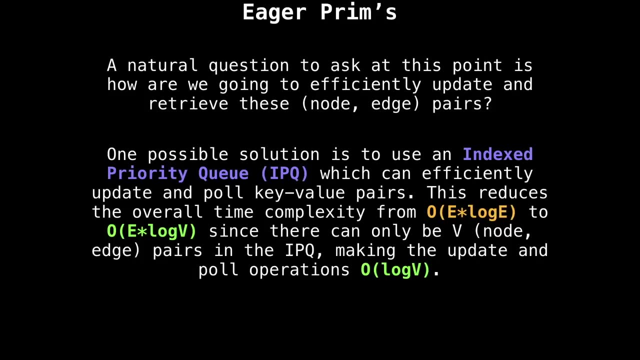 of adding edges to a priority queue. as we iterate over the edges of a node, we're going to relax, that is, to update the destination nodes most promising incoming edge. So you might be asking yourself the question: how are we going to efficiently update and retrieve these node edge pairs? Well, one 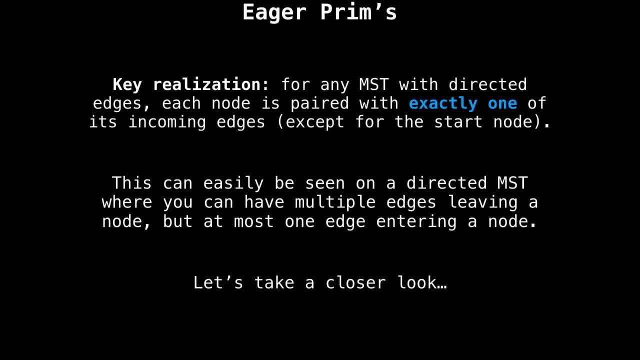 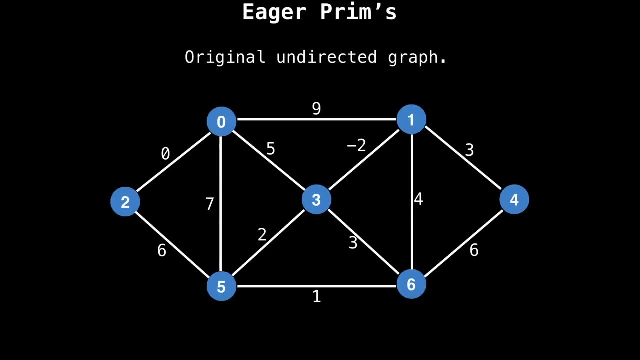 incoming edges, That is, except for the start node. One way to see this is on a minimum spanning tree with multiple edges leaving a node but only ever one edge entering a node. Let's have a closer look at what I mean. Suppose we have this undirected graph, the equivalent. 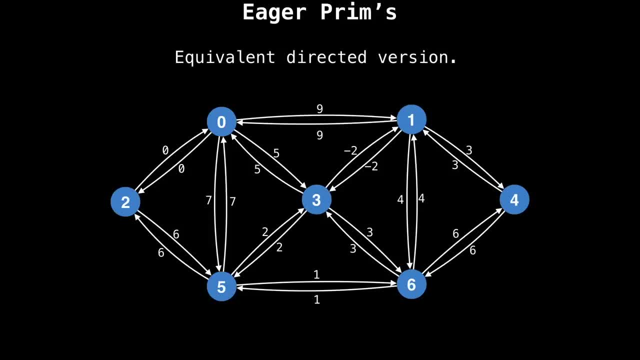 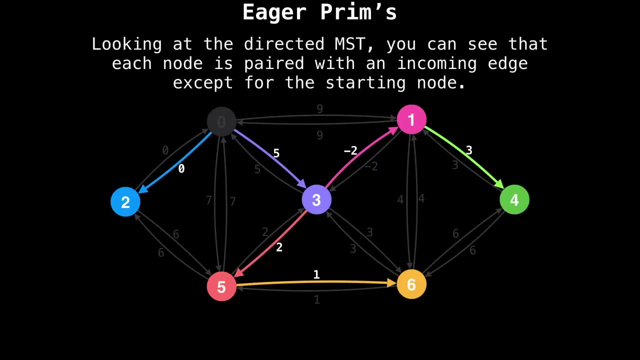 directed version of this graph looks like this. A possible minimum spanning tree, starting at node zero, might be the following, highlighted in green: Now notice that on this directed MST each node is paired with exactly one edge except for the starting node, So in a sense there seems to be a relationship. 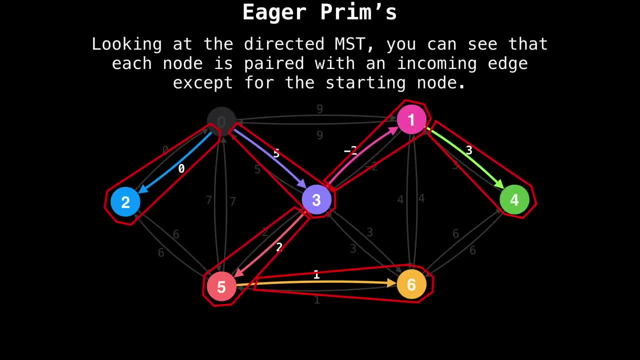 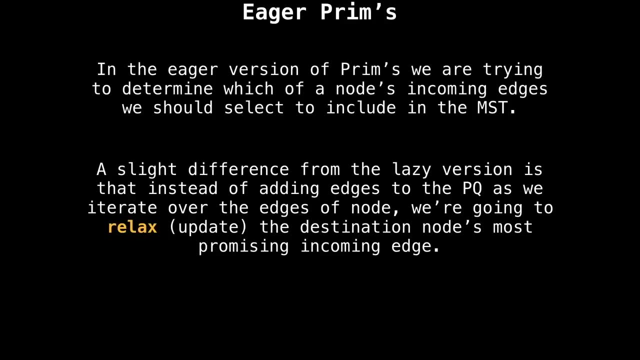 we can take advantage of here, which is that each node is paired with exactly one incoming edge. In the eager version, we are trying to determine which of a nodes incoming edges we should select to include in the MST. The main difference, coming from the lazy version, is that, instead, 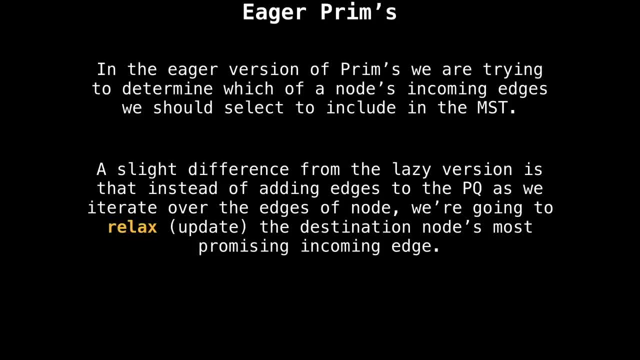 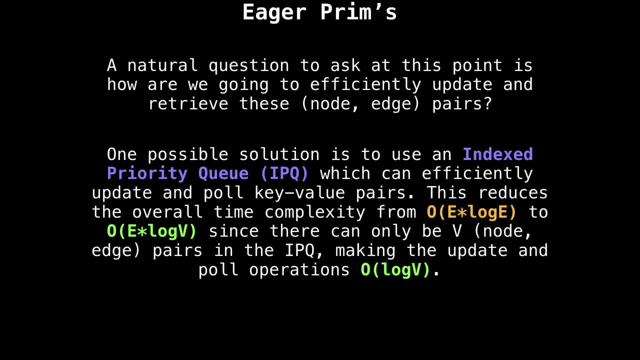 of adding edges to a priority queue. as we iterate over the edges of a node, we're going to relax, that is, to update the destination nodes most promising incoming edge. So you might be asking How are we going to efficiently update and retrieve these node edge pairs? Well, one: 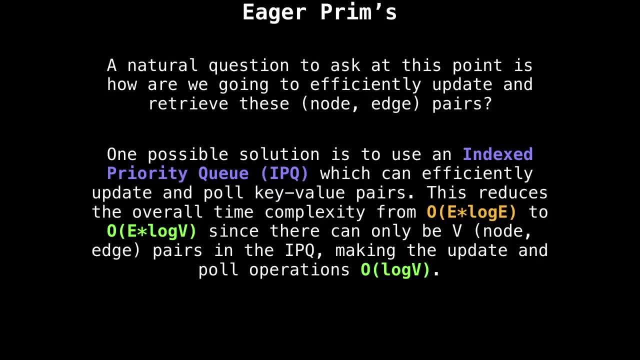 solution is to use an index priority queue, or simply IP queue for short, which can efficiently update and pull key value pairs. you can think of an IP queue as the data structure you would get if a hash table and a priority queue had a baby together. it supports sorted key value. 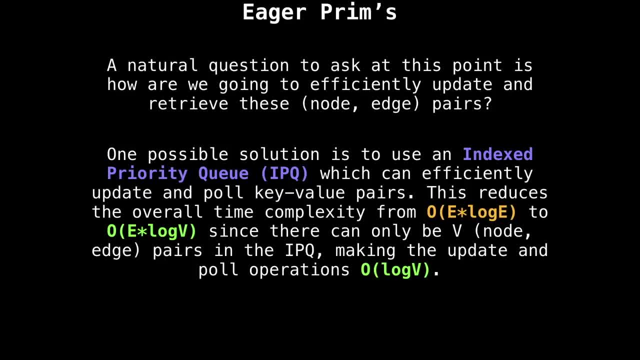 pair updates And pull operations in a logarithmic time. Using this new approach would reduce the overall time complexity from big O of e log e to big O of e log v, Since there can only be V node edge pairs in the IP queue. If you're interested in learning more about the index priority, 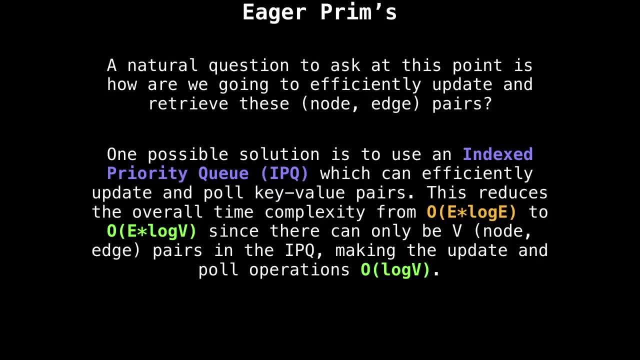 solution is to use an index priority queue, or simply IP queue for short, which can efficiently update and pull key value pairs. you can think of an IP queue as the data structure you would get if a hash table and a priority queue had a baby together. it supports sorted key value. 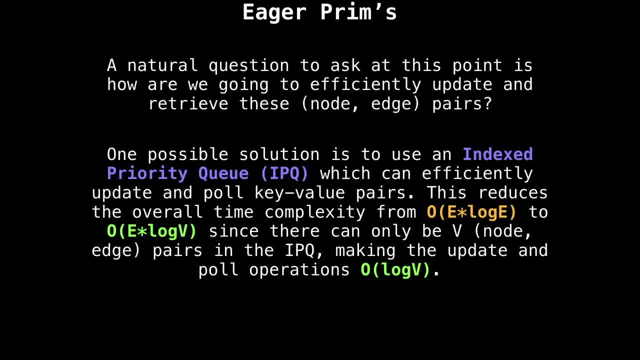 pair updates and pull operations In logarithmic time. using this new approach would reduce the overall time complexity from big O of e log e to big O of e log v, since there can only be v node edge pairs in the IP queue. If you're interested in learning more about the index priority queue data structure, 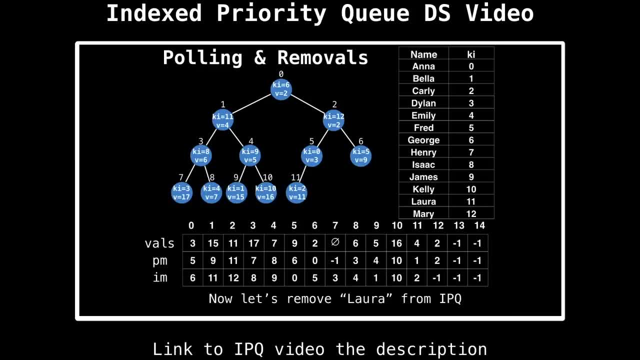 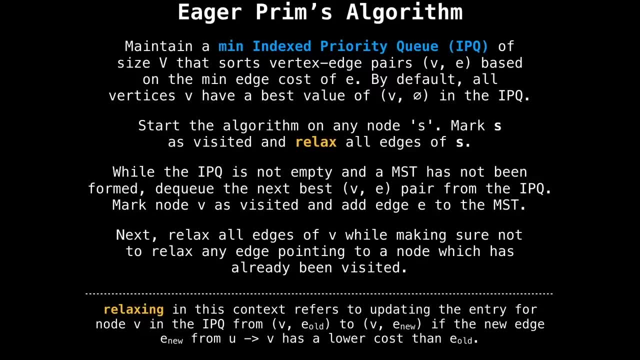 and how it's implemented. I would highly recommend my data structures video on the subject. I will link it in the description below if you need to catch up. The implementation for the eager version is slightly different and the algorithm goes as follows: Maintain an IP queue of size v that sorts vertex edge pairs v, e, based on. 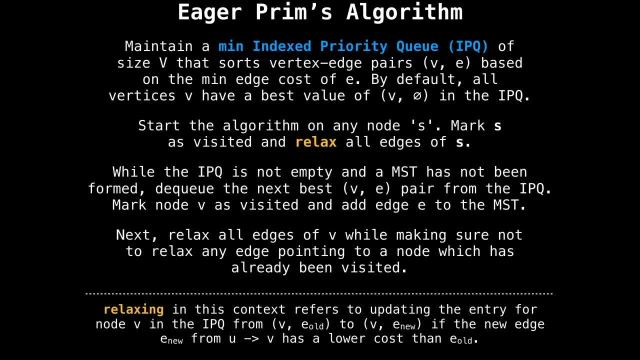 minimum edge cost of e. Start the algorithm on any node s mark s as visited and relax all the edges of s. Relaxing this context refers to updating the entry for node v to the IP queue from v old edge to v new edge If the new edge has a better cost than the. 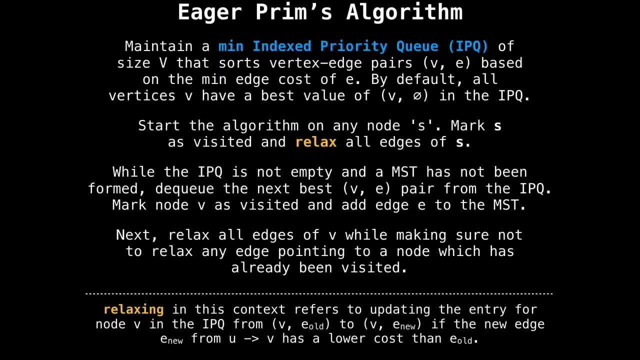 old edge, then, while the index priority queue is not empty and a minimum spanning tree has not been formed, DQ, the next best vertex: edge, pair v e from the IP queue. mark node v as visited and add edge e to the MST. 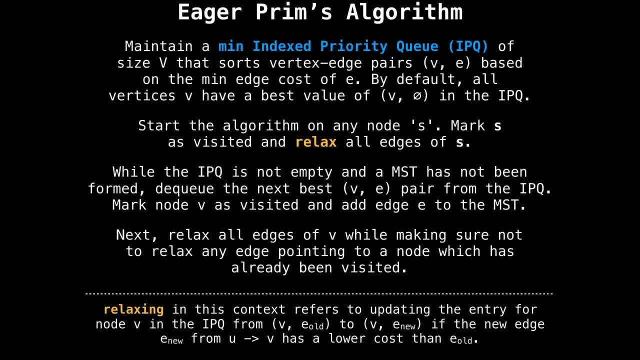 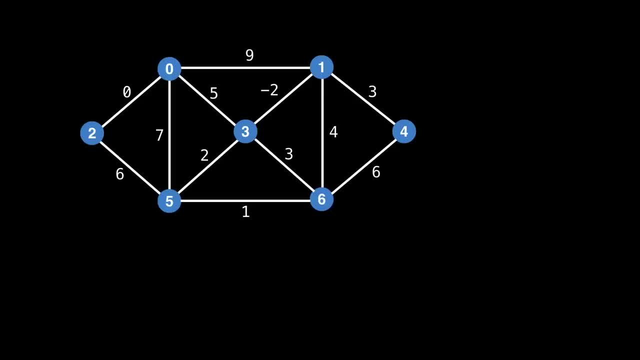 Lastly, relax all edges of v, while making sure not to relax any edge pointing to a node which has already been visited. Alright, I think it's time to see an example. Suppose we have the following weighted, undirected graph and we want to find any minimum spanning tree: 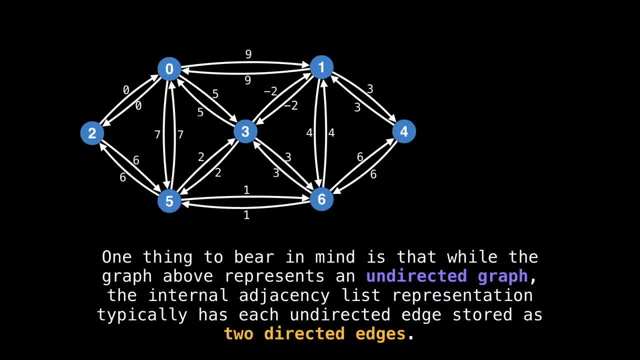 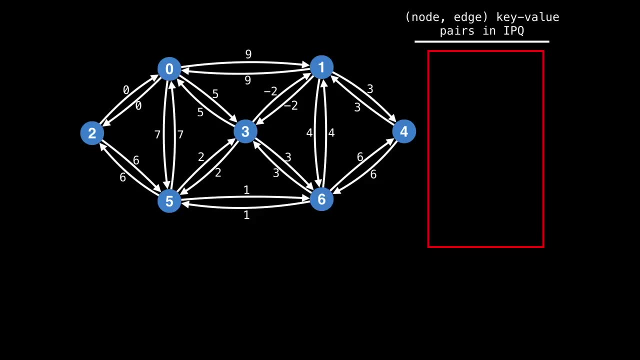 One thing to remember is that while we're dealing with an undirected graph, we will be internally representing it as a directed graph, where each undirected edge is still stored as two directed edges. I will be keeping track of all node edge key value pairs on. 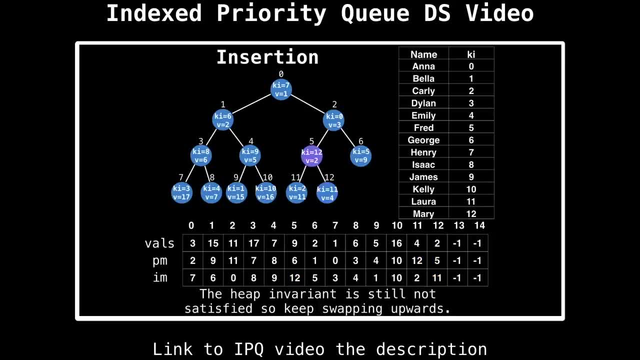 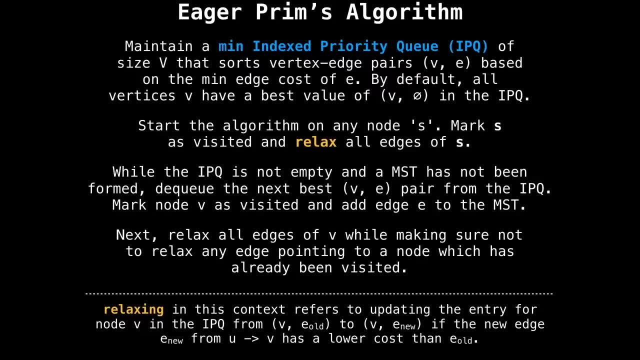 queue data structure and how it's implemented. I would highly recommend my data structures video on the subject. I will link it in the description below. The implementation for the eager version is slightly different And the algorithm goes as follows: Maintain an IP queue of size v that sorts vertex edge pairs v, e, based on. 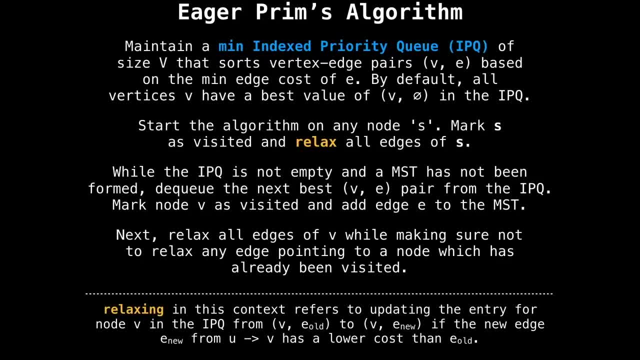 minimum edge cost of e. Start the algorithm on any node s mark s as visited and relax all the edges of s. Relaxing this context refers to updating the entry tree for node v in the IP queue from v old edge to v new edge if the new edge has a better 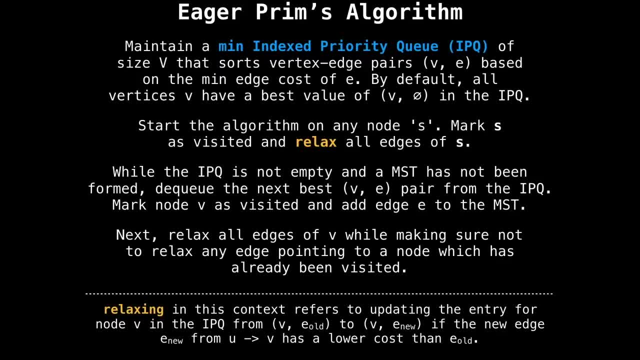 cost than the old edge, then, while the index priority queue is not empty and a minimum spanning tree has not been formed, DQ, the next best vertex, edge pair v e from the IP queue. mark node v as visited and add edge e to the MST. 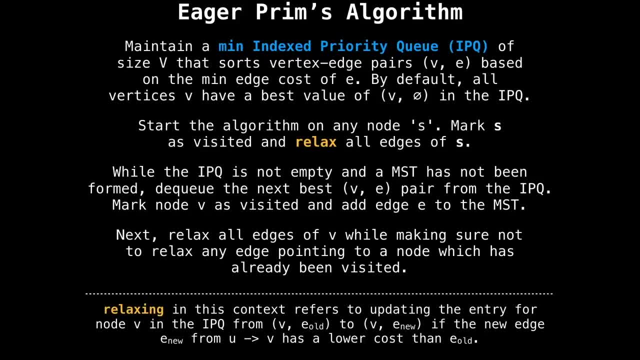 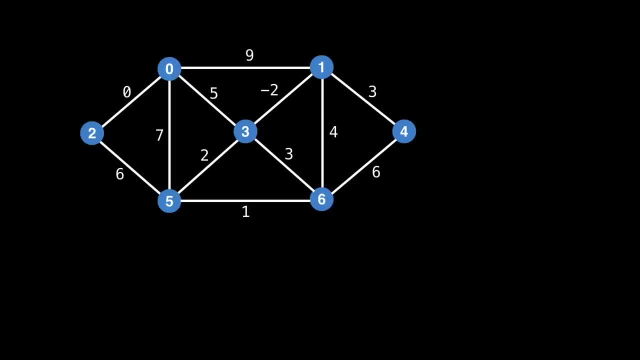 Lastly, relax all edges of v, while making sure not to relax any edge pointing to a node which has already been visited. All right, I think it's time to see an example. Suppose we have the following weighted, undirected graph And we want to find any minimum spanning: 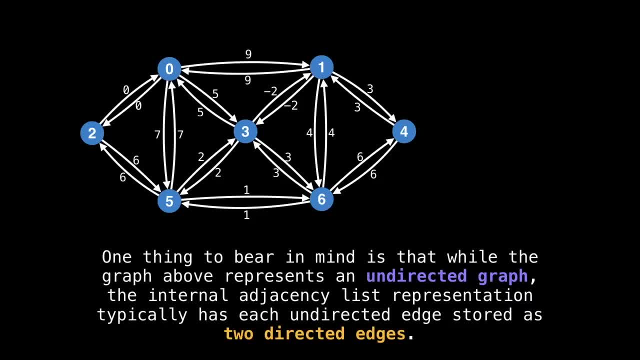 tree. One thing to remember is that, while we're dealing with an undirected graph, we will be internally representing it as a directed graph, where each undirected graph is represented. The undirected Graph is the source for any value in the string, for which the value of 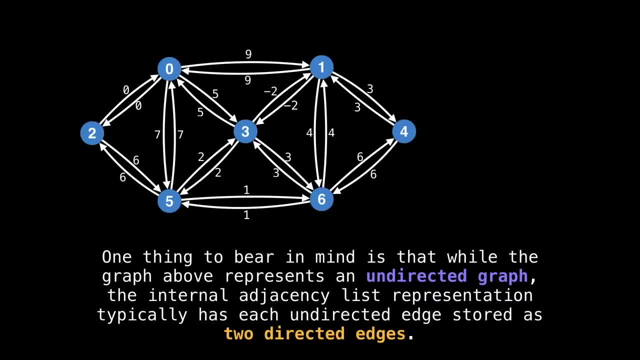 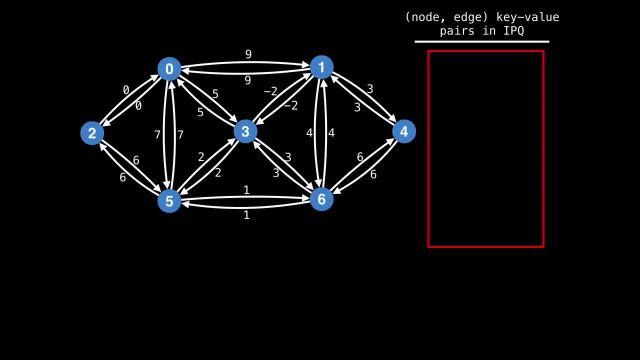 or at a fixed value, is set to 0.. Now we need to make sure that we remember that we're dealing with an undirected graph. we will be internally representing it as a directed graph, where each undirected edge is stored as two directed edges. I will be keeping track of all node. 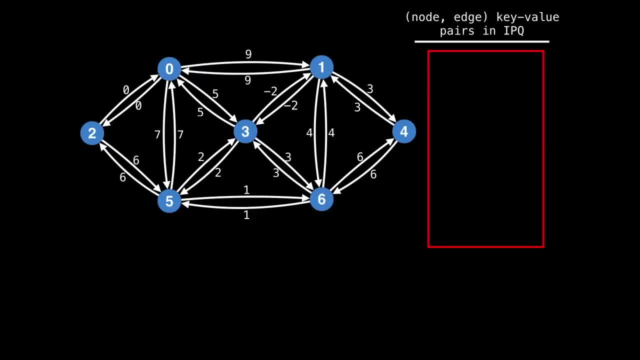 edge key value pairs on the right and update them accordingly as the algorithm executes. So you can think of the red box as the contents of the indexed priority queue. Let's begin the algorithm on node zero. start by iterating over all the edges of zero and relax them. 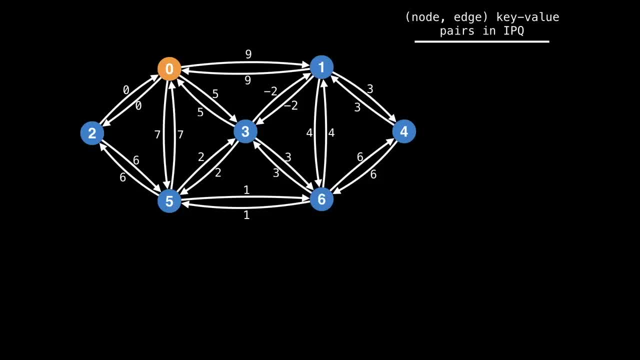 during the relaxing process. add a node edge pair to the indexed priority queue if it does not exist yet. Otherwise, update the value if the new edge has a better cost than what already exists. The first node edge pair we add is node two, with the incoming edge from: 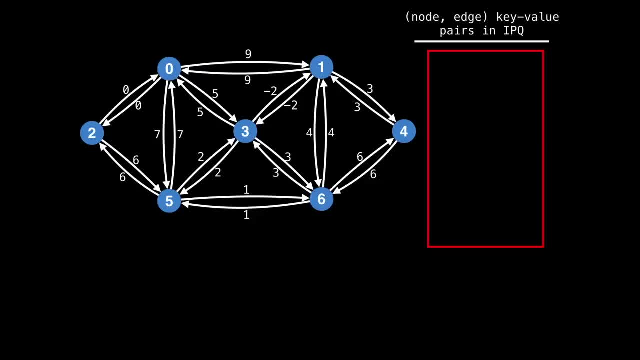 the right and update them accordingly as the algorithm executes. So you can think of the red box as the contents of the index priority queue. Let's begin the algorithm on node zero. start by iterating over all the edges of zero and relax them During the relaxing process. 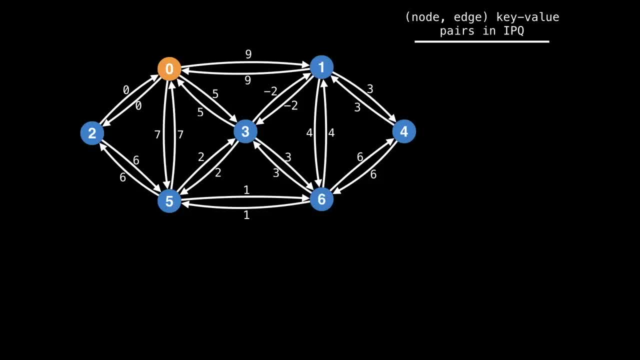 add a node edge pair to the index priority queue if it does not exist yet. Otherwise, update the value if the new edge has a better cost than what already exists. The first node edge pair we add is node two, with the incoming edge from zero to two, with a cost of zero. 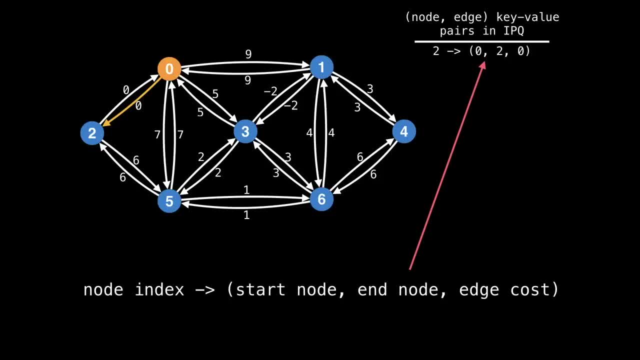 And similarly for the rest of zeros edges. The next best node edge pair is node two. The next best node edge pair is node two. The next best node edge pair is node two. Theさぁ No, iterate through all the edges of node two and relax all edges character. 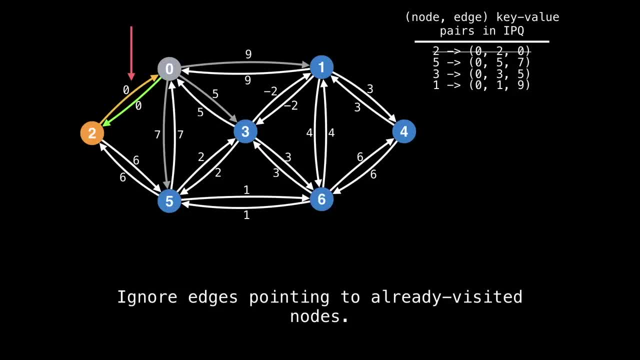 ignore edges pointing to already visited nodes like the one on this slide. The edge 256 has a better cost going to node five than the edge from node zero to node five with a cost of seven. update the index party queue with this new edge. I will denote IP queue updates with. 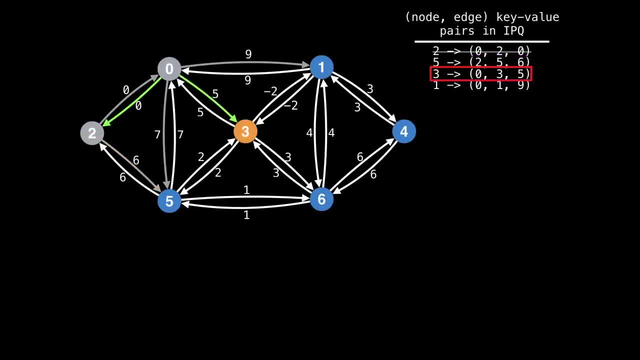 a purple box around the edge being updated. The next best node edge pair is no three, with the edge coming from node zero, with a cost of five. Now iterate through all the edges of node three and relax all edges. The edge coming from node three offers a better value. 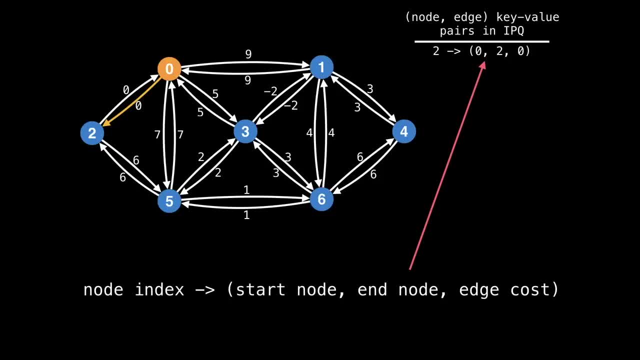 zero to two with a cost of zero, and similarly for the rest of zeros edges. Okay, so the next best node edge pair based on the minimum edge cost is node two with the incoming edge from node zero. Now iterate through all the edges of node two and relax all edges. 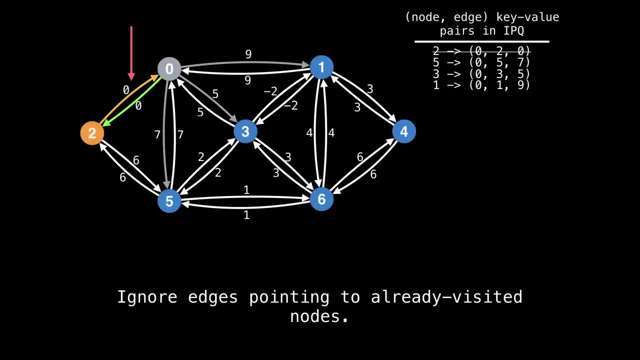 character. ignore edges pointing to already visited nodes like the one on this slide. The edge to five six has a better cost, going to node five, then the edge from node zero to node five with a cost of seven. So update the indexed priority queue with: 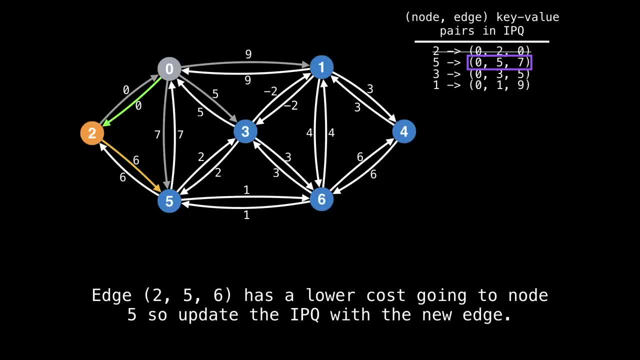 this new edge. I will denote IP queue updates with a purple box around the edge being updated. The next best node edge pair is no three, with the edge coming from node zero with a cost of five. Now iterate through all the edges of node three and relax all edges. The 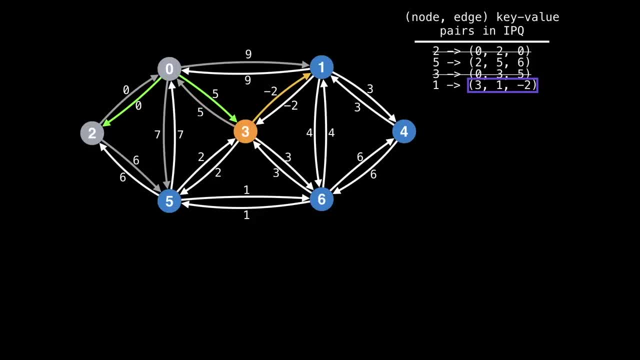 edge coming from node 3 offers a better value. So I update the value for node one in the index party queue with the new edge. Add a new key value: pair entry for node six. since node six is not yet inside the index party queue, Update the value for node five with the new better edge we just 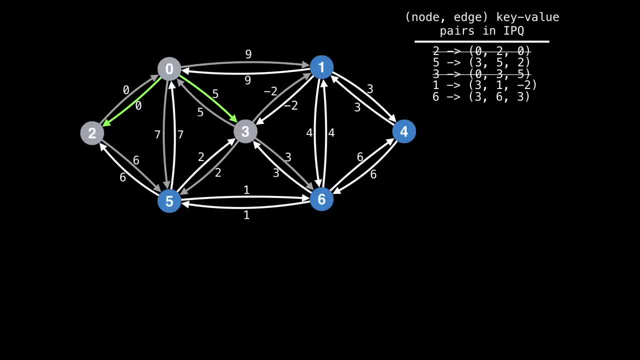 found And from this point on I will let the animation play. Please try and follow along. All right, and that's the algorithm. you can see that the minimum spanning tree we found consists of the edges highlighted in green. If we collapse, the graph back into its undirected 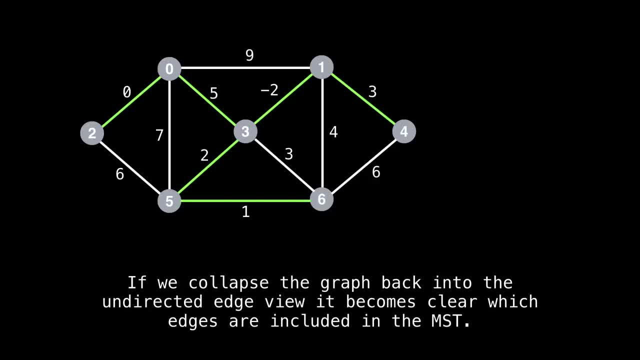 edge view, it becomes clear which edges are included in the minimum spanning tree. You can also get the MST cost by adding the minimum spanning tree value to the minimum spanning tree, The values of all the edges in the spanning tree. for a cost of nine Let's have 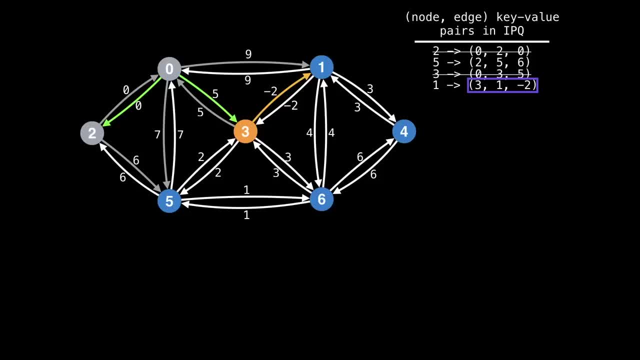 So I update the value for node one in the index party queue with the new edge. Add a new key value: pair entry for node six. since node six is not yet inside the index party queue, Update the value for node five with the new, better edge we just found, And from: 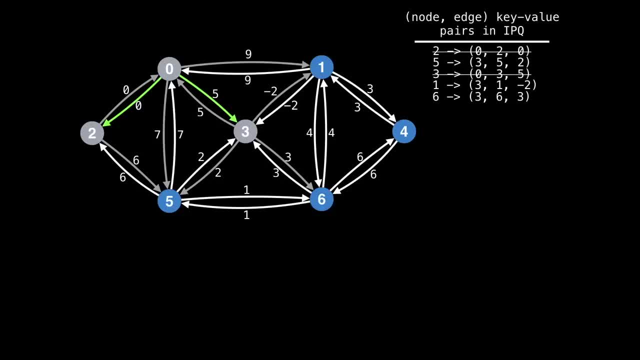 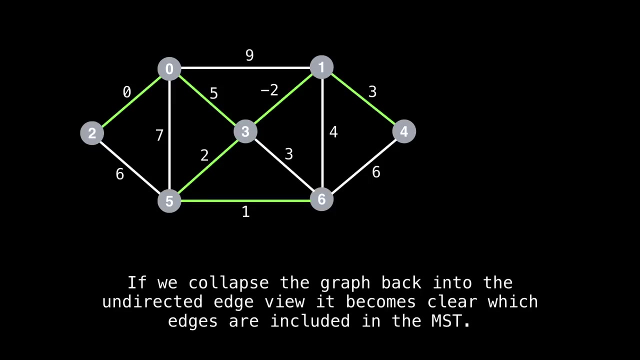 this point on, I will let the animation play. Please try and follow along. Okay, All the right, and that's the route algorithm. you can see that the minimum spanning tree we found consists of the edges highlighted in green. If we collapse the graph back into its undirected edge view, it becomes clear. 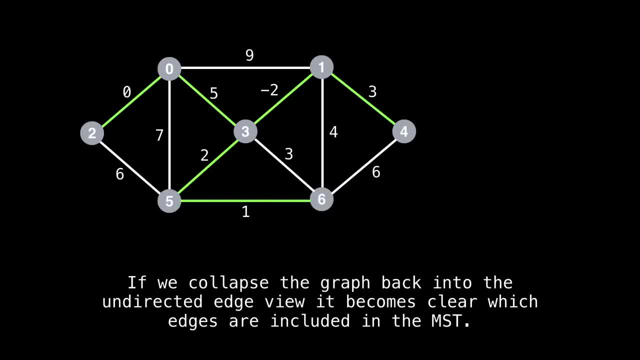 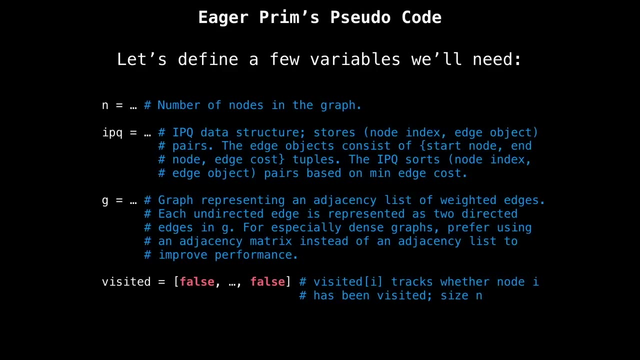 which edges are included in the minimum spanning tree. You can also get the MST cost by adding the values of all the edges in the spanning tree for a cost of nine. Let's have a look at some pseudocode for the eager implementation of prims. you'll notice that it's almost identical. 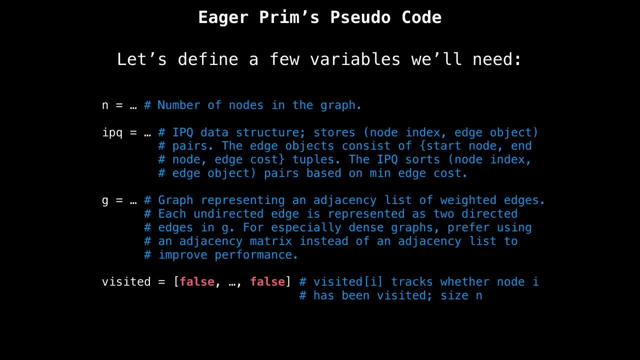 to the lazy version, except for a few key details which I will highlight. First is n, which is still the number of nodes in the graph, followed by the variable IP queue, which represents the index priority queue, instead of a traditional priority queue which stores node index edge. 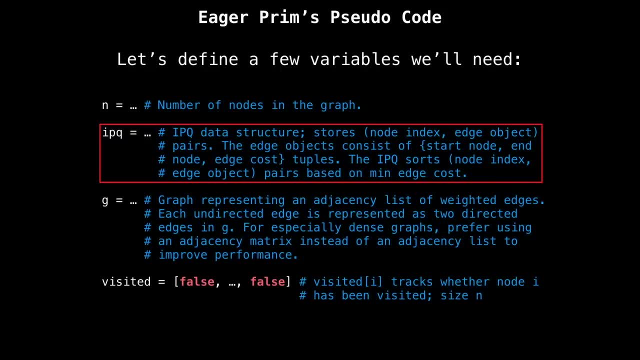 object pairs. edge objects are still represented as start node And node edge cost triplets, with the node index being an integer. g is once again our graph adjacency list of weighted edges. Remember that in G every undirected edge is represented as two directed edges. There's also the whole story about whether we should be using an. 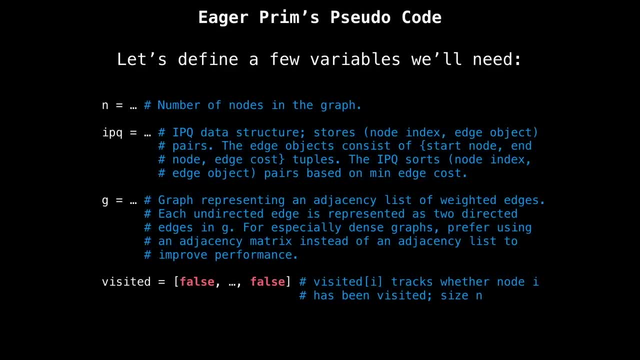 a look at some pseudocode for the eager implementation of prims, You'll notice that it's almost identical to the lazy version, except for a few key details which I will highlight. First is n, which is still the number of nodes in the graph, followed by the variable IP queue, which represents 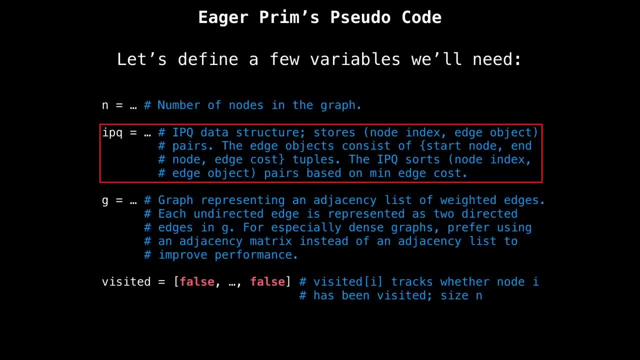 the index party queue instead of a traditional priority queue which stores node index, edge object pairs. edge objects are still represented as start node and node edge cost triplets, with the node index being an integer. G is once again our graph adjacency list of weighted edges. Remember that in G every undirected edge is represented as two. 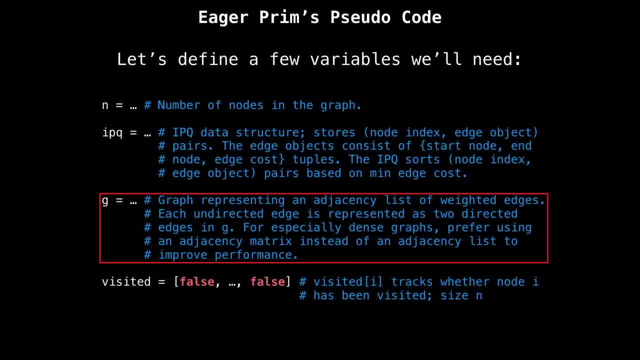 directed edges. There's also the whole story about whether we should be using an adjacency list. We're using an adjacency matrix to represent our graph when running prims because we know that this can greatly impact performance. I was curious and did some analysis comparing. 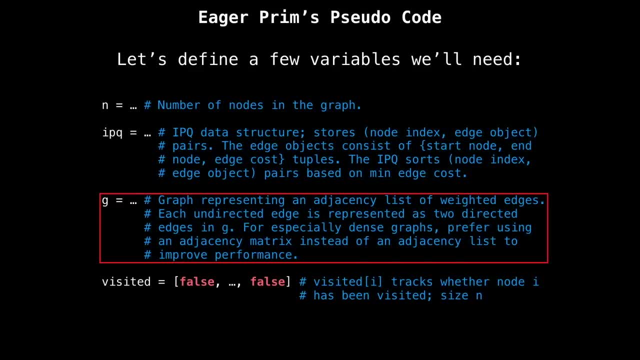 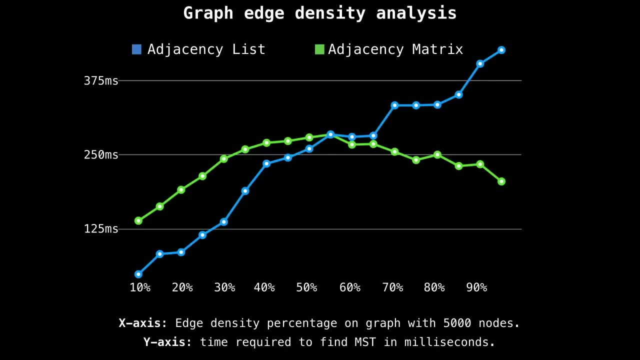 the adjacency list versus the adjacency matrix, And the results I got were interesting. This dotted line graph shows the performance of using an adjacency list in blue versus an adjacency matrix in green, And the x axis represents the graph edge density percentage And the y axis indicates performance measured in milliseconds. As you can see for graphs, 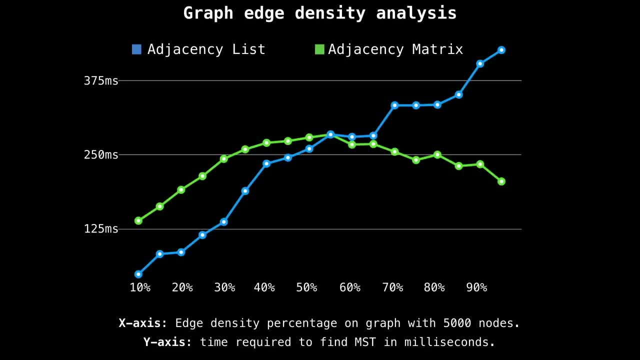 with fewer edges, the adjacency list outperforms the adjacency matrix, But as the edge density increases, the adjacency matrix becomes the obvious choice. You may be wondering why the adjacency matrix is. performance starts to increase after the middle point, where the graph starts to become more and more dense. 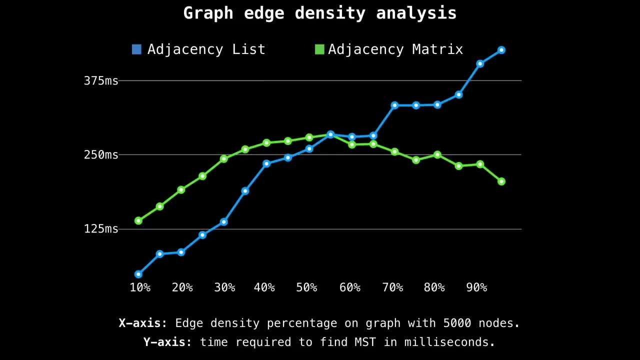 So let's take a look at the adjacency matrix. The adjacency matrix is a graph that is more dense than the adjacency matrix. The adjacency matrix is a graph that is more dense than the graph. This is an excellent question, And my guess is that the denser the graph, the 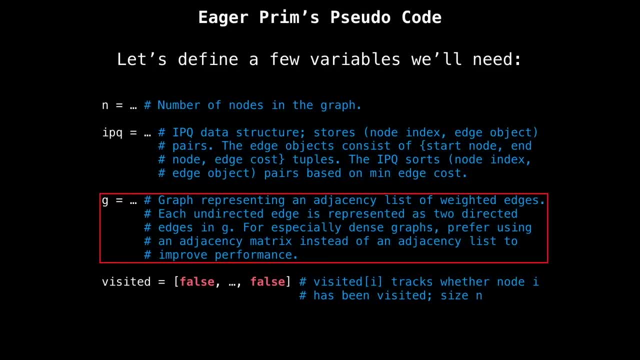 adjacency list or using an adjacency matrix to represent our graph when running prims, because we know that this can greatly impact performance. I was curious and did some analysis comparing the adjacency list versus the adjacency matrix, And the results I got were interesting. This dotted 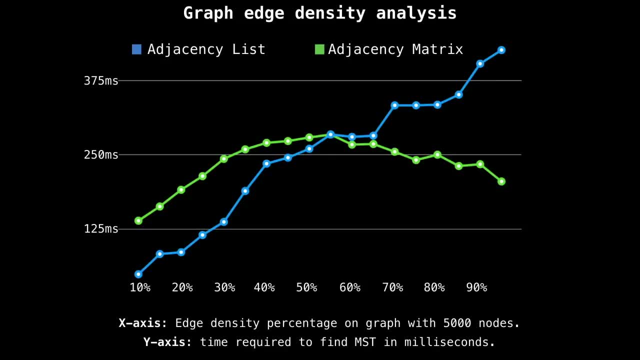 line graph shows the performance of using an adjacency list and blue versus an adjacency matrix. in green, The x axis represents the graph edge density percentage And the y axis indicates performance measured in milliseconds. As you can see, the graph is not the same as the dot line graph, But it's still a good example of the performance of the dot line. 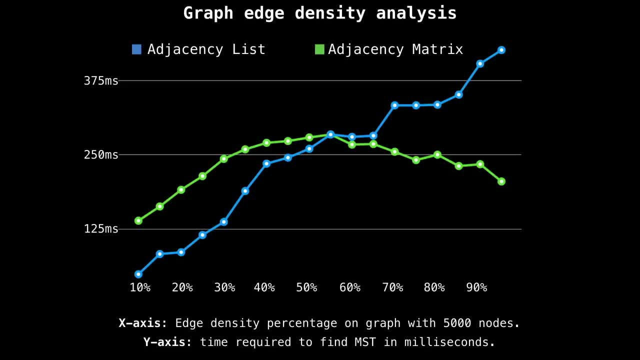 graph In addition to the adjacency. for graphs with fewer edges, the adjacency list outperforms the adjacency matrix, But as the edge density increases, the adjacency matrix becomes the obvious choice. You may be wondering why the adjacency matrix is. performance starts to. 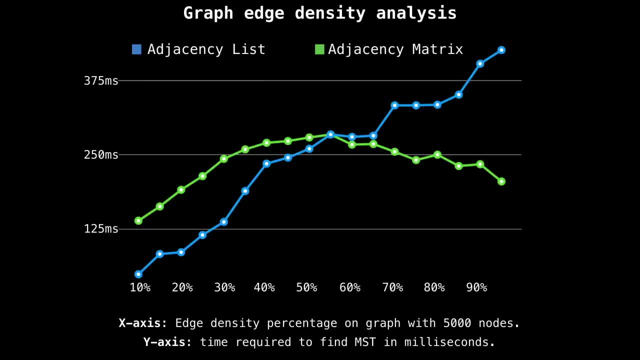 increase after the middle point, where the graph starts to become more and more dense. This is an excellent question, And my guess is that the denser the graph, the fewer relative relaxation operations need to be performed, which is an expensive part of prims algorithm. 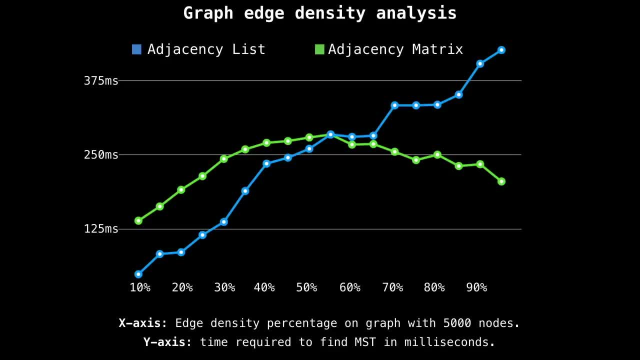 Since the time to iterate over all the edges of a node is constant, but fewer relaxation operations are needed. performance should increase as a result, but I may be wrong. Even still, the results are interesting And the takeaway is that the graph representation you choose. 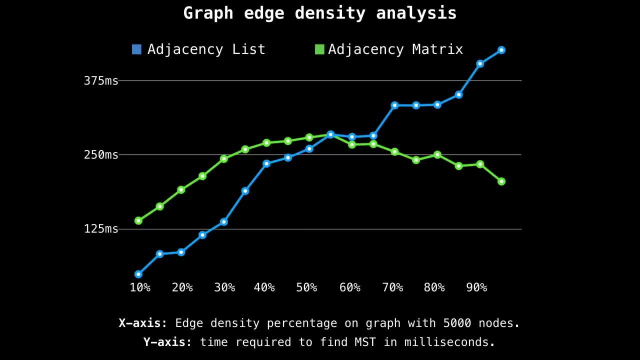 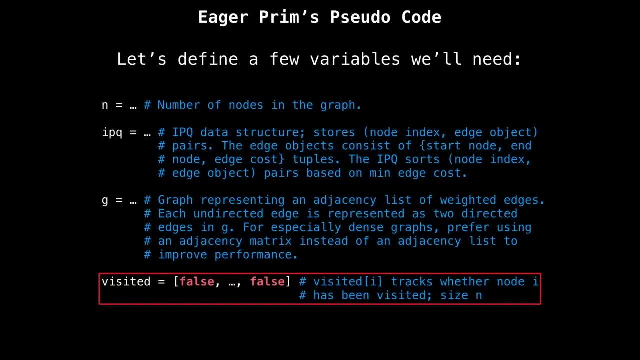 can greatly impact the performance of your algorithm, depending on whether your graph is sparse or dense. All right back to the pseudocode. The last variable is the visited Boolean array of size n, which tracks whether node i has been visited or not. Now let's. 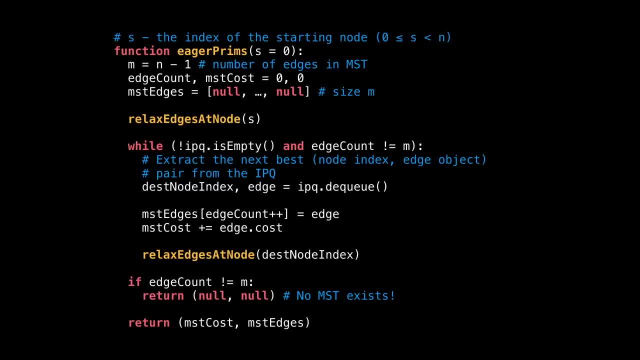 have a look at the actual algorithm for eager prims. In the first block I define a few more variables that will need M, the number of expected edges in the MST. edge count, the number of edges we currently have included in the MST. This variable is used to make sure the tree spans. the whole graph then is MST cost, which. 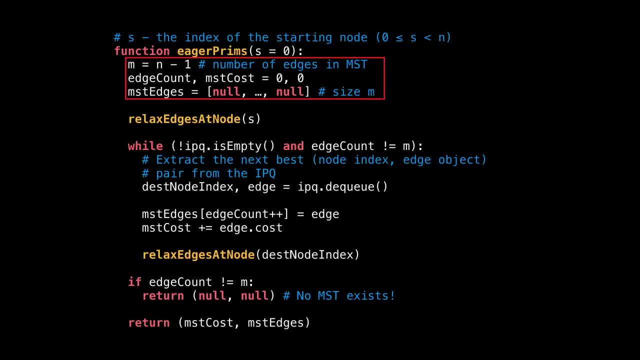 tracks the total cost of our minimum spending tree. And finally MST edges, which is an array that holds the edges we have included in the MST. After this I call the relaxed edges at node method, passing in the start node as an argument Let's have a look at. 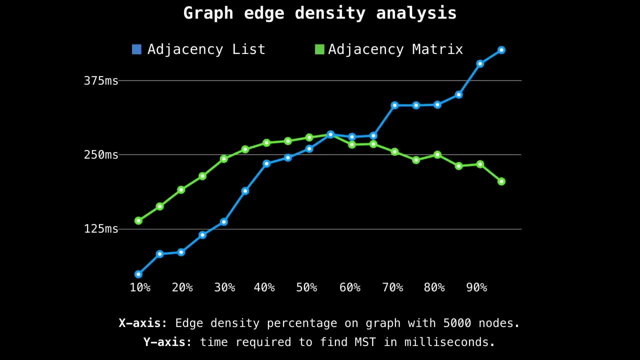 fewer relaxation operations need to be performed, which is an expensive part of prims algorithm, Since the time to iterate over all the edges of a node is constant, but fewer relaxation operations are needed. performance should increase as a result, but I may be wrong. 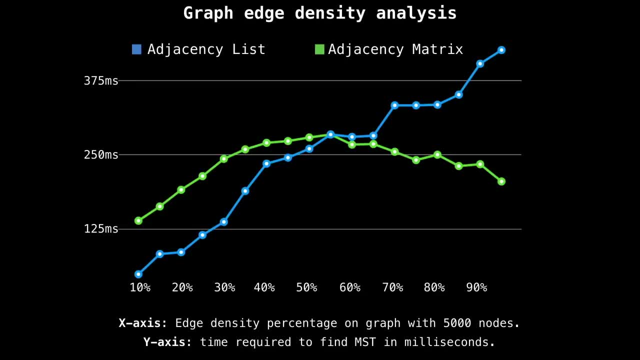 Even still, the results are interesting And the takeaway is that the graph representation you choose is less than the adjacency matrix, And that's because the adjacency matrix is more dense than the adjacency matrix. So the more relaxation operations you choose, the more relaxation operations you choose can greatly impact the performance of your algorithm. 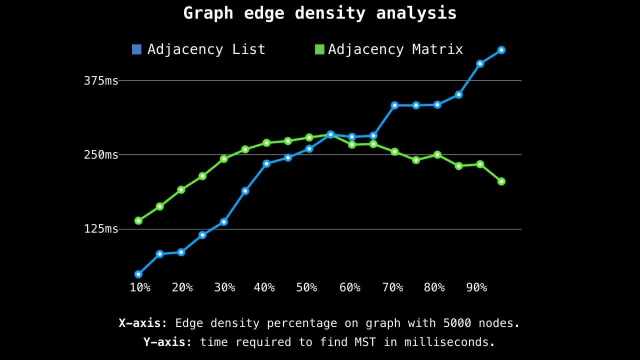 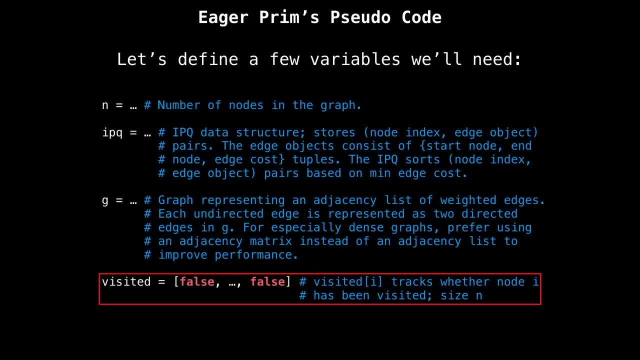 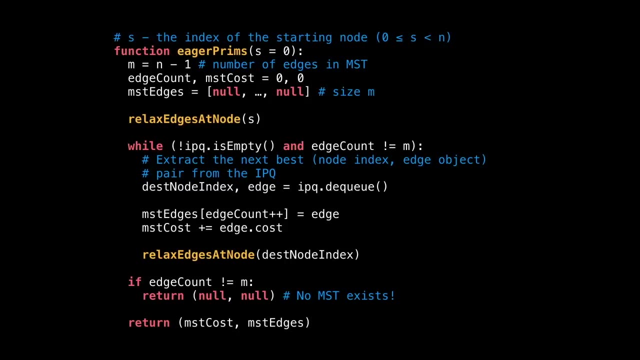 depending on whether your graph is sparse or dense. All right back to the pseudocode. The last variable is the visited Boolean array of size n, which tracks whether node i has been visited or not. Now let's have a look at the actual algorithm for eager prims In. 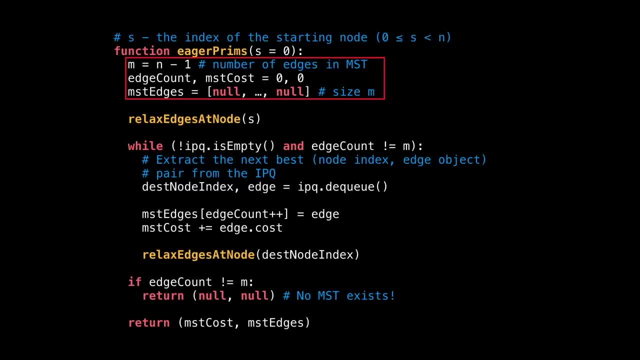 the first block, I define a few more variables that will need m, the number of expected edges in the MN St edge count, the number of edges we currently have included in the MST. This variable is used to make sure the tree spans the whole graph. then is MST cost, which tracks the 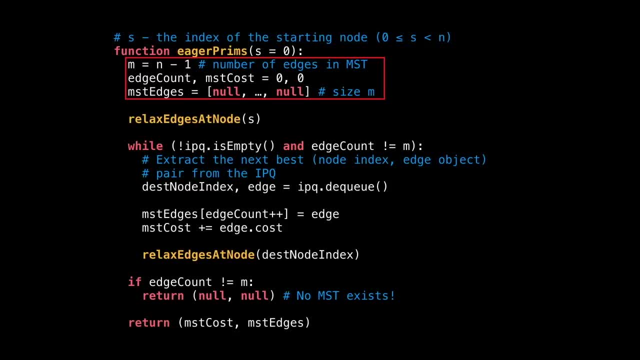 total cost of our minimum spanning tree. And finally MST edges, which is an array that holds the edges we have included in the MST. After this I call the relaxed edges at node method, pressing in the start node as an argument. Let's have a look at the relaxed edges at. 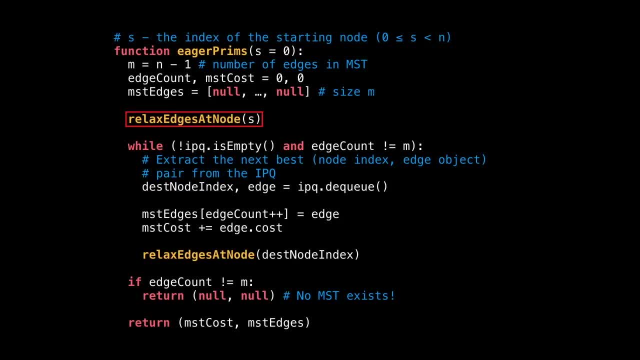 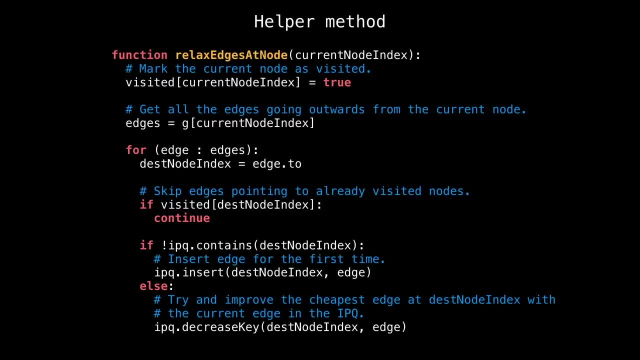 node method to understand what's happening in there. All right, here we are. you'll notice that this method takes a single argument, which is the current node we care about. The first thing we do is mark the current node as visited, So we don't visit it again in the future. 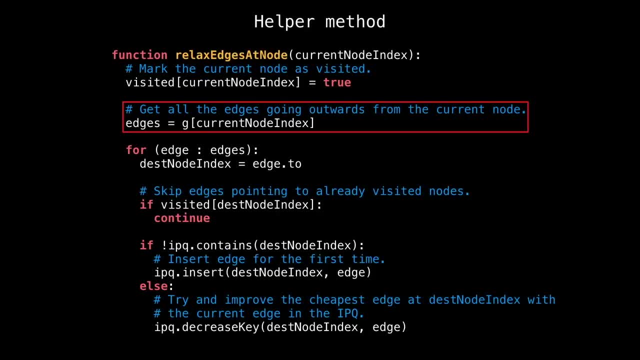 Then I'll reach into our graph adjacency list and get all the edges going outwards from the current node. As we enter the loop and start iterating over all the outgoing edges, the first thing I do inside the loop is grab a reference to the destination node index. This is the node. 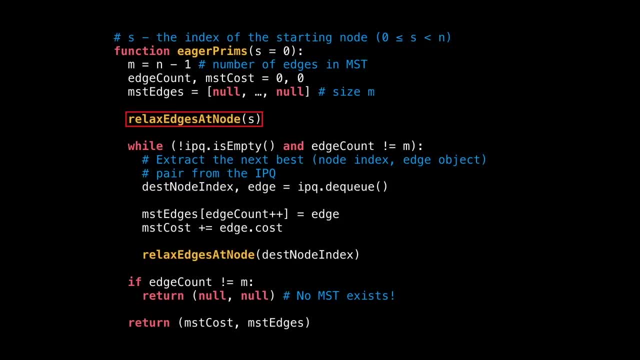 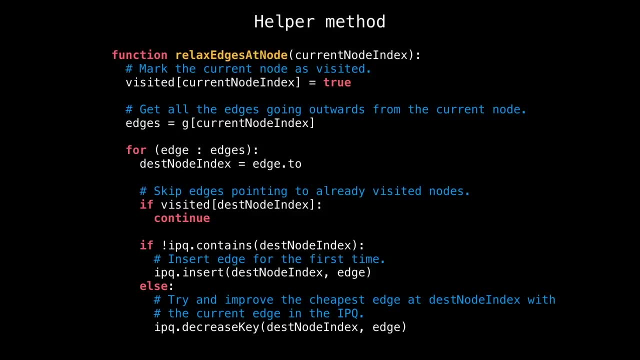 the relaxed edges at node method to understand the MST cost. Alright, here we are. you'll notice that this method takes a single argument, which is the current node we care about. The first thing we do is mark the current node as visited. 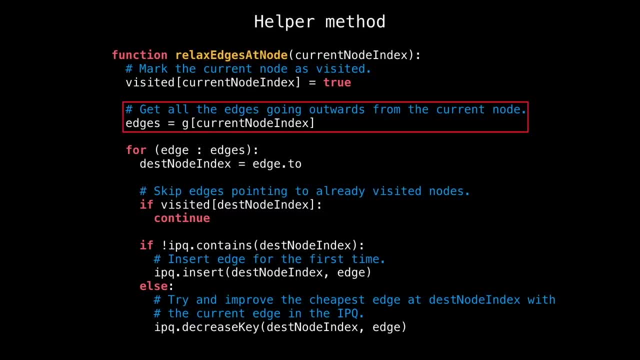 so we don't visit it again in the future. Then I reach into our graph adjacency list and get all the edges going outwards from the current node. As we enter the loop and start iterating over all the outgoing edges, The first thing I do inside the loop is grab. 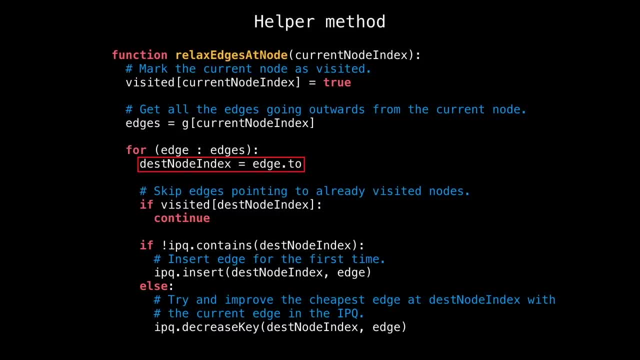 a reference to the destination node index. This is the node the edges pointing at. Next skip edges which point at already visited nodes. Now here's the bit where we actually relax the edge. First check if the IP queue contains the key with the value of the destination. 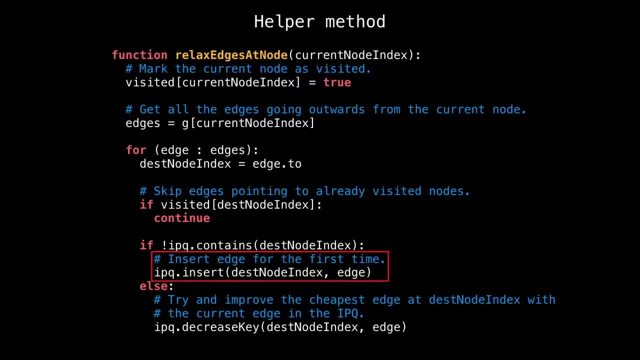 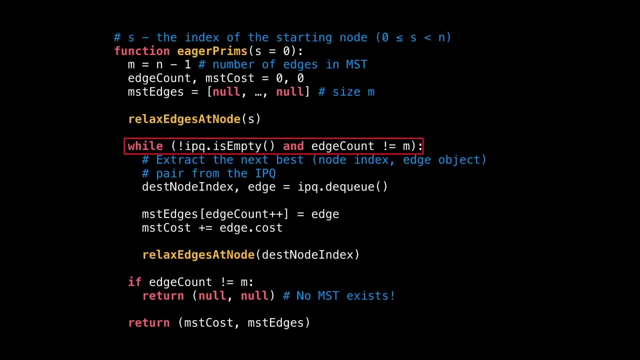 node. If it doesn't, then add the edge to the IP queue for the first time. Otherwise, try and improve the cheapest edge at destination node index with the current edge in the priority queue Back inside the main method. Next up: 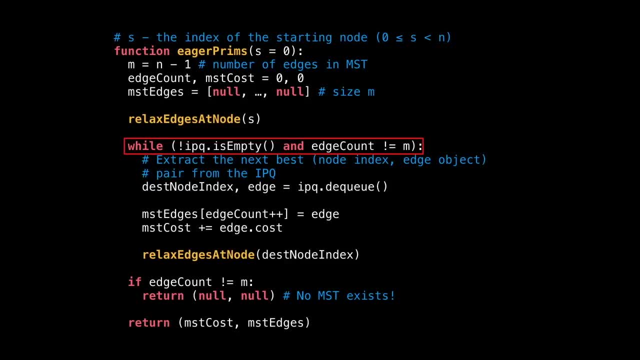 keep looping while the IP queue is not empty And we have not yet completed the MST. After extract the next best node index edge object pair from the IP queue based on minimum edge cost, Include the selected edge as part of the MST and sum over the edge costs. Lastly, 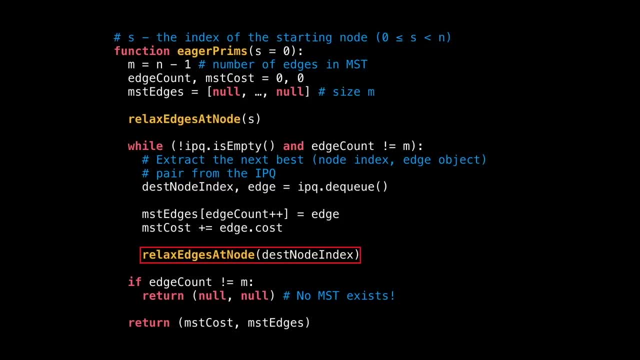 relax all edges of the current node and repeat until the loop breaks Outside the main loop. check if we have successfully created a spanning tree. This might not be the case if some of the nodes are unreachable. But assuming that that is not the case, return the MST cost. 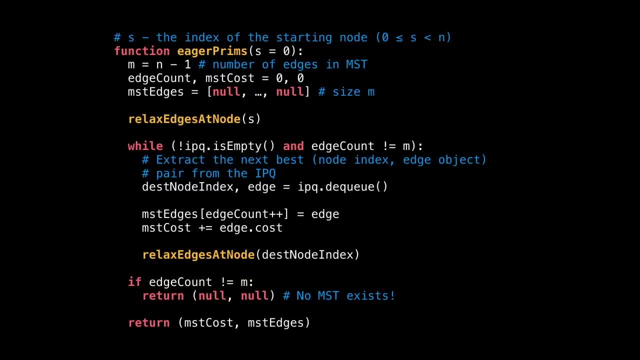 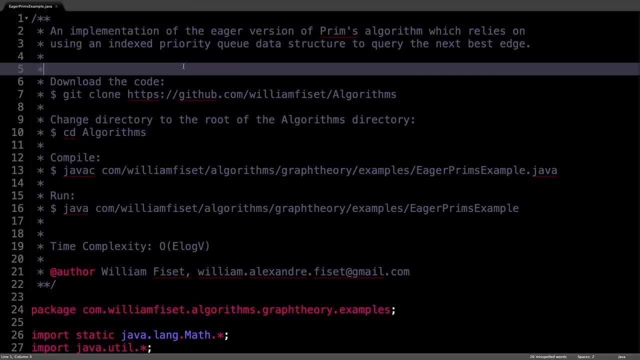 and the edges which make up the spanning tree. And that concludes the pseudocode for prims algorithm. All right, here we are in the source code for prims. Let's take a look at some of the methods implemented in Java. At the top here I posted some instructions. 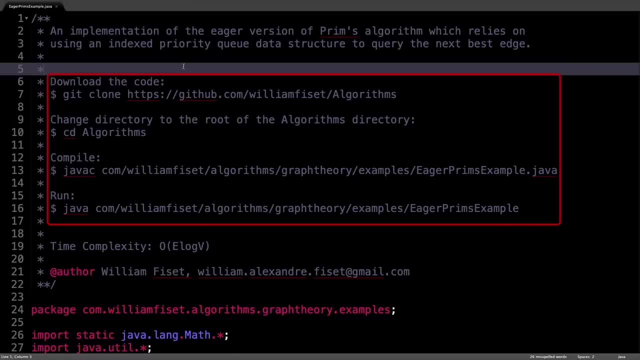 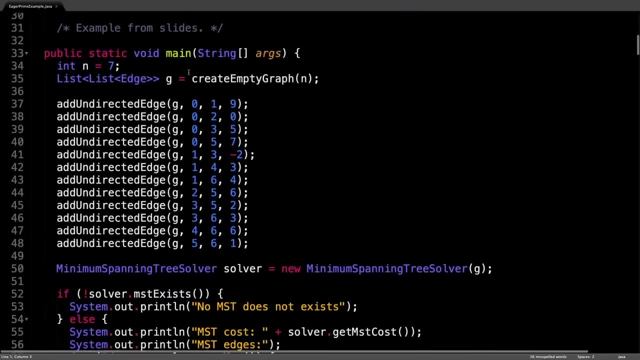 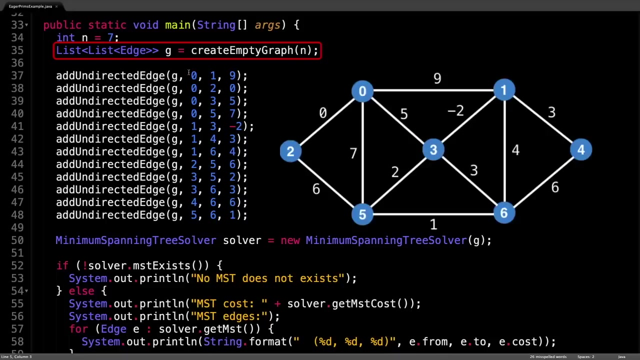 on how to download and run the script. in case you want to play around with it a little bit, Let's begin by taking a look at the main method right over here. The first thing I do is set up a graph. we want to find the minimum spanning tree of. In fact, it's the same graph we had. 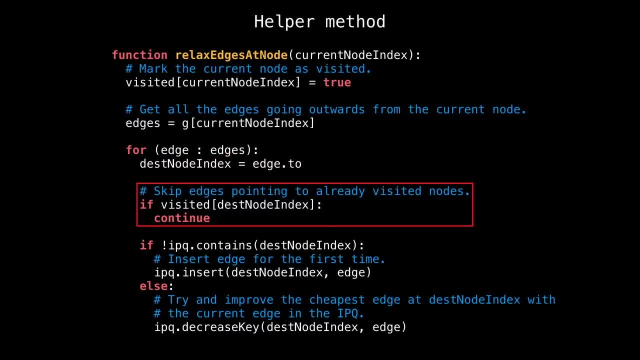 the edges pointing at Next skip edges which point at already visited nodes. Now here's the bit where we actually relax the edge. First, check if the IP queue contains the key with the value of the destination node. If it doesn't, then add the edge to the IP. 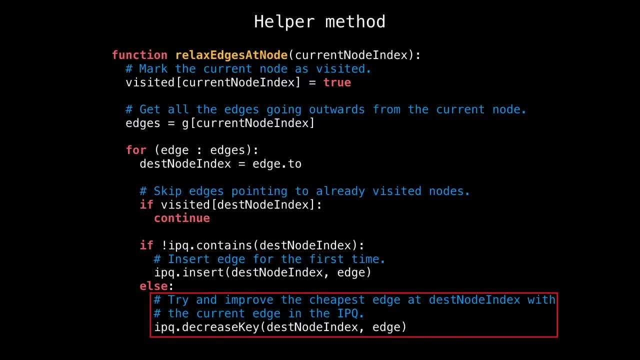 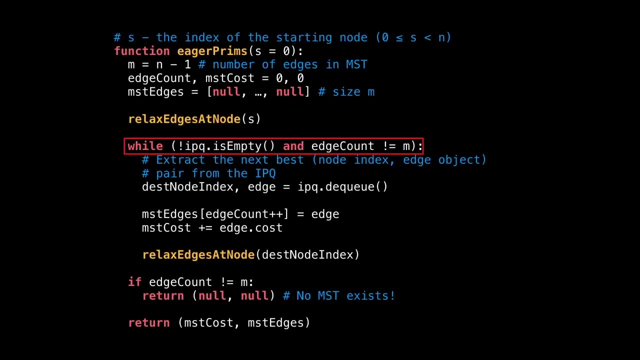 queue for the first time. Otherwise, try and improve the cheapest edge at dest node index with the current edge in the priority queue Back inside the main method Next up. keep looping while the IP queue is not empty And we have not yet completed the MST After. 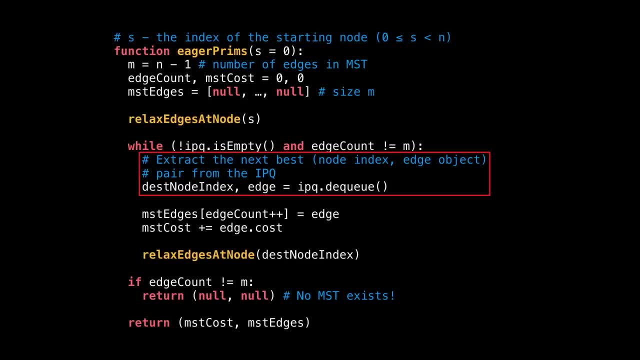 extract the next best node index edge object pair from the IP queue based on minimum edge cost. Include the selected edge as part of the MST and sum over the edge costs. Lastly, relax all edges of the current node and repeat until the loop breaks Outside the main loop. check. 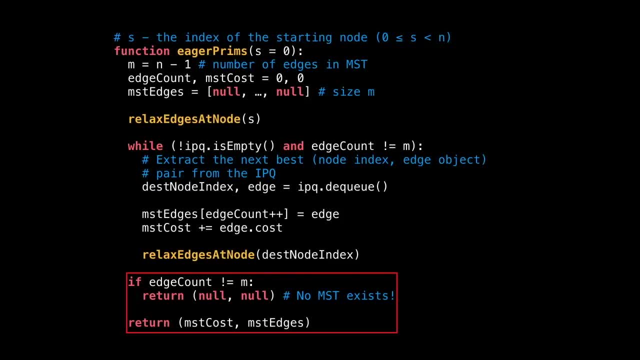 if we have successfully created a spanning tree. This might not be the case if some of the nodes are unreachable. But assuming that that is not the case, return the MST cost and the edges which make up the spanning tree. And that concludes the pseudo. 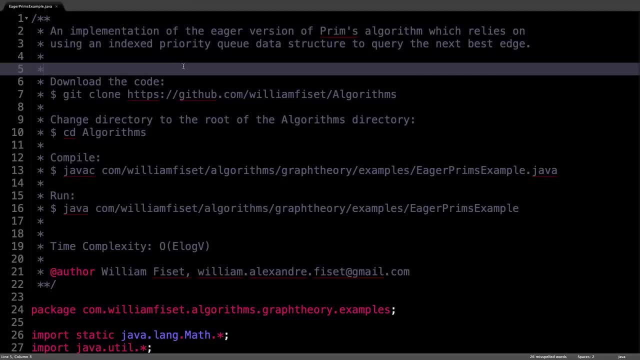 code for prims algorithm. All right, here we are in the source code for prims implemented in Java. At the top here I posted some instructions on how to download and run the script, in case you wanted to play around with it a little bit. Let's begin by taking a look at the main. 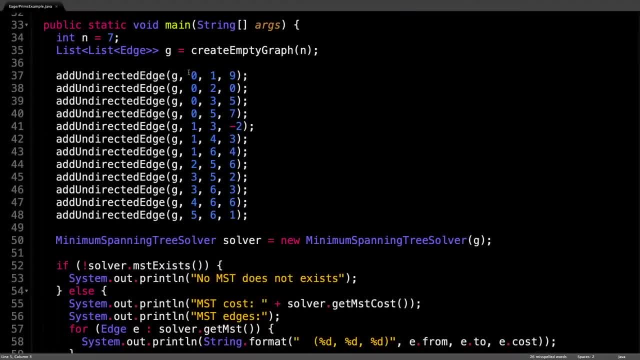 method right over here. The first thing I do is set up a graph. we want to find the minimum spanning tree of. In fact, it's the same graph we had in the slide slides in the previous video. To create the graph, I call the helper method: create empty. 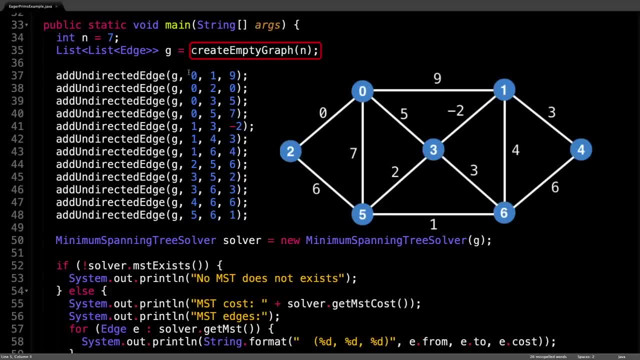 graph and initialize an adjacency list of size n And afterwards add various undirected edges of different weights to the graph. Once the graph is set up, I create a minimum spanning tree solver and pass in the graph we just created. The solver is able to tell us whether 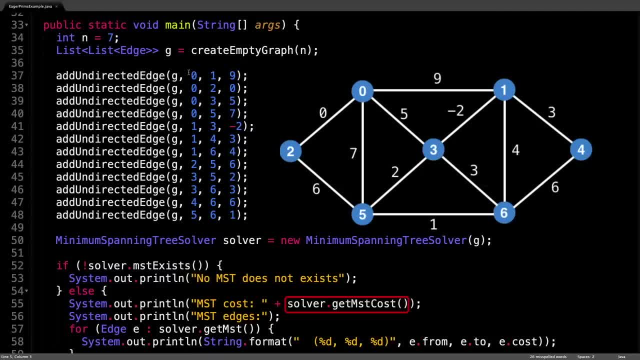 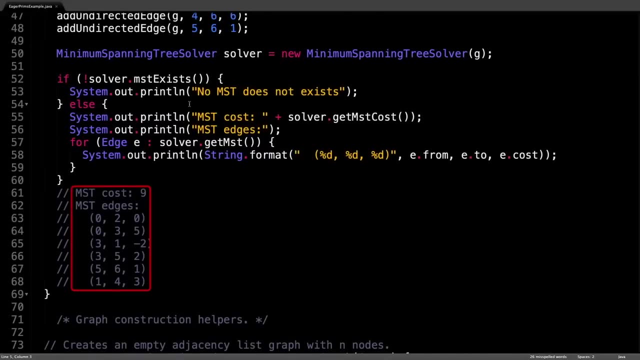 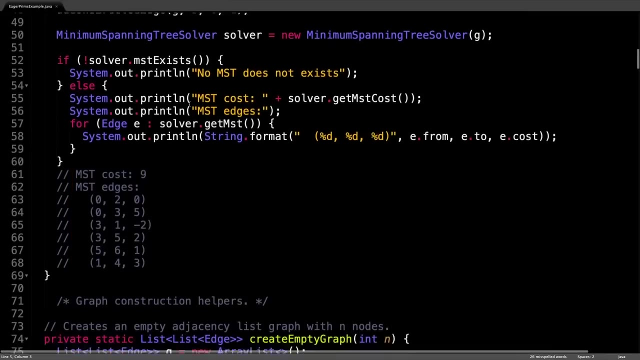 a minimum spanning tree exists, what the cost of the MST is, as well as get all the edges which make up the MST. The output of running the script is illustrated below right here you can see that this particular minimum spanning tree has a cost of nine and it has these six edges. If you were curious as to how the adjacency 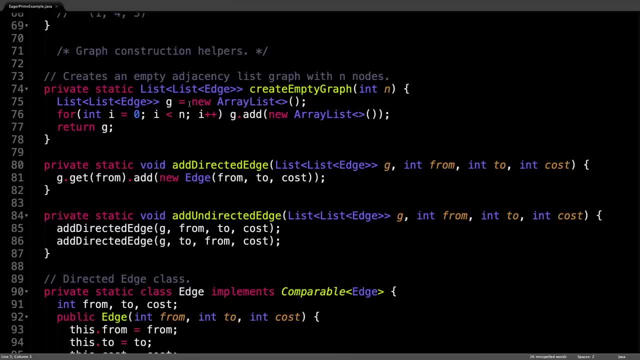 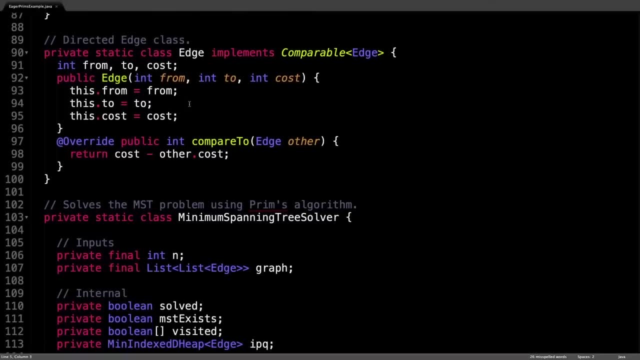 list gets initialized and how I add edges to the graph. here's the code that does it. It does exactly that. Next up is a class struct which represents a directed edge used in the graph. One important thing to note about this class is that it implements the comparable interface and overrides 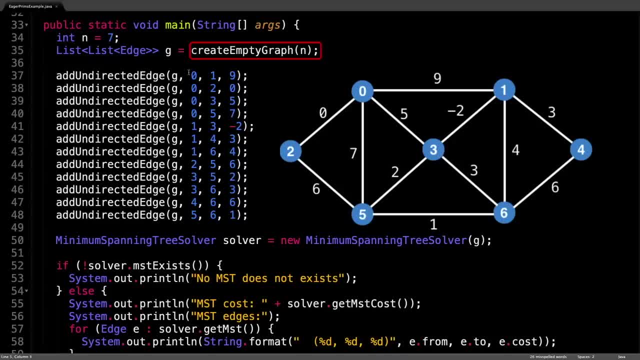 in the slides in the previous video To create the graph. I call the helper method. I'm going to create empty graph and initialize an adjacency list of size n And afterwards add various undirected edges of different weights to the graph. Once the graph is set up, I create 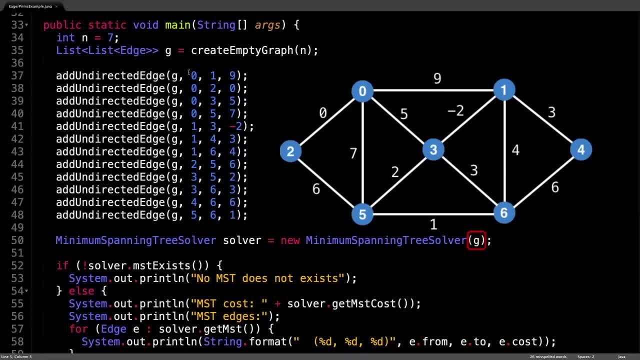 a minimum spanning tree solver and pass in the graph we just created. The solver is able to tell us whether a minimum spanning tree exists, what the cost of the MST is, as well as get all the edges which make up the MST. So the first step of running the script is illustrated below right here you can see. 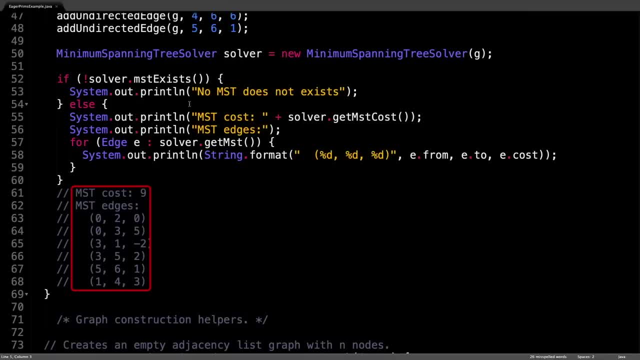 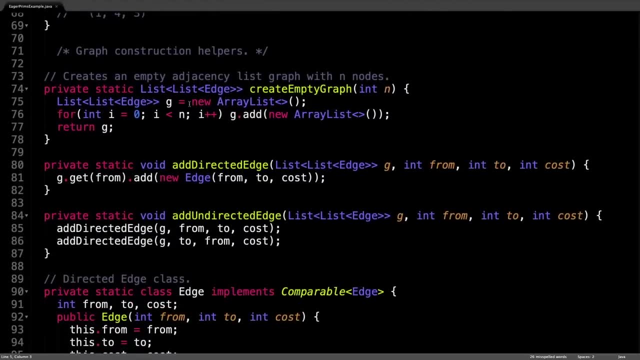 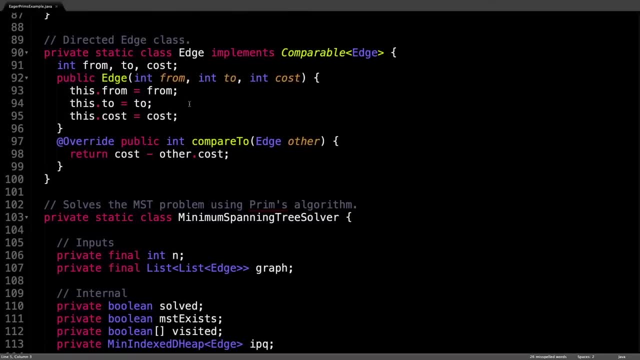 Next up is a class struct which represents a directed edge used in the graph. One important thing to note about this class is that it implements the comparable interface and overrides the compare to method. This simply means that edges are able to be sorted in reference to. 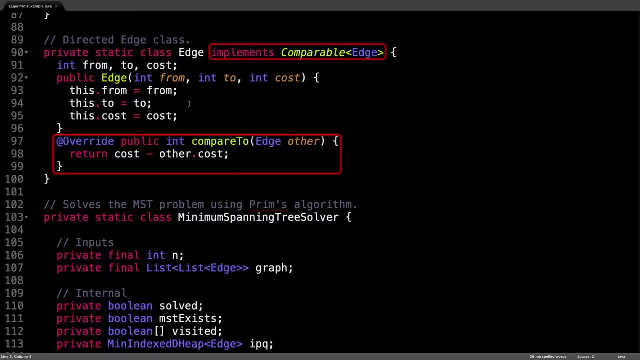 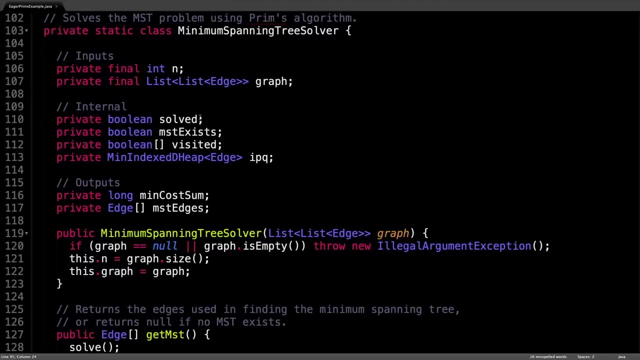 one another based on the minimum edge cost. This is important for the index priority queue because it needs to know how to compare edge objects with one another. to sort them After the edge class is the minimum spanning tree solver, where all the interesting logic. 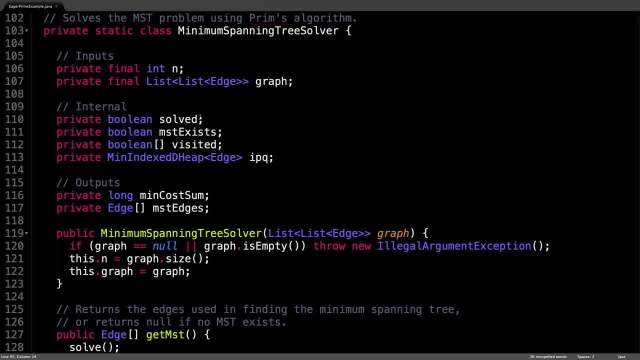 happens In this class. I store a whole bunch of variables to help us out. The first two inputs are n, the number of nodes in the graph which I get from the constructor, and the graph adjacency list itself. Internally I store a Boolean solved variable to track whether 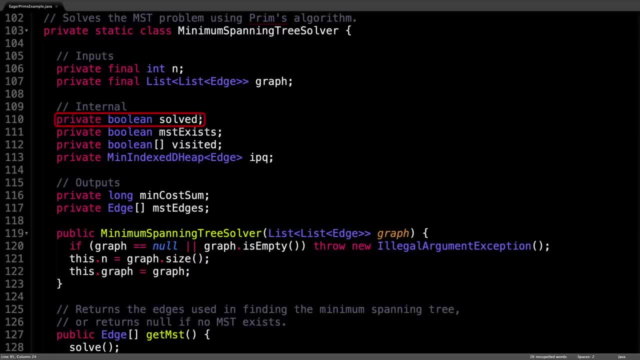 we have already computed the minimum spanning tree so that we don't need to do it again Once we've already solved the problem. the MST exists variable tells you whether a minimum spanning tree was found in the input graph. it's important to note that, by default, this 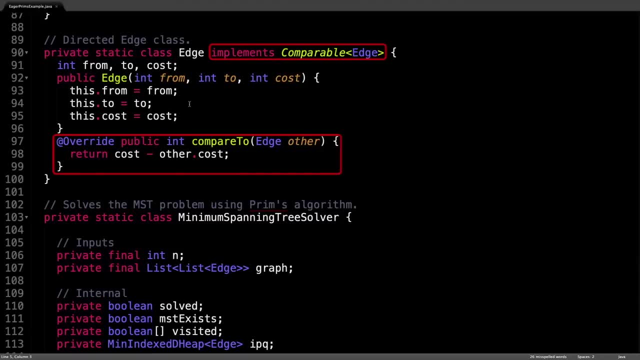 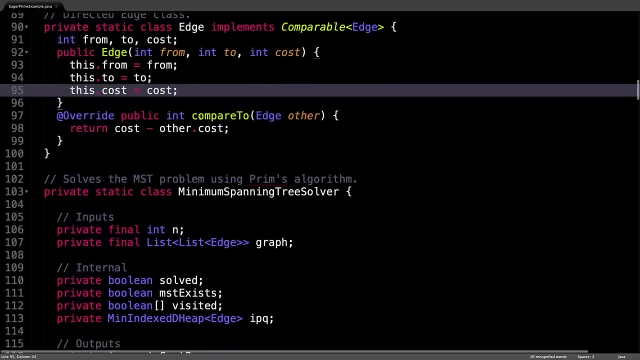 the compare to method. This simply means that edges are able to be sorted in reference to one another based on the minimum edge cost. This is important for the index priority queue because it needs to know how to compare edge objects with one another to sort them After the edge. 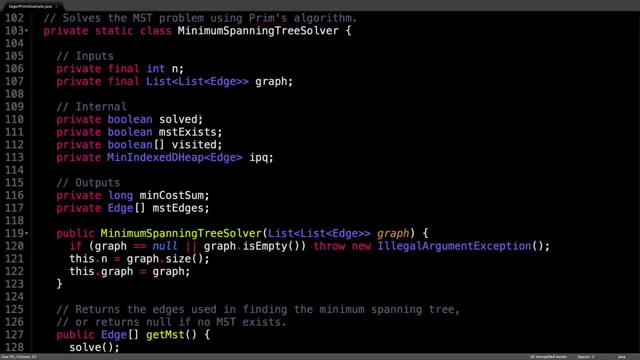 class is the minimum spanning tree solver, where all the interesting logic happens. In this class I store a whole bunch of variables to help us out. The first two inputs are n, the number of nodes in the graph which I get from the constructor, and the graph adjacency. 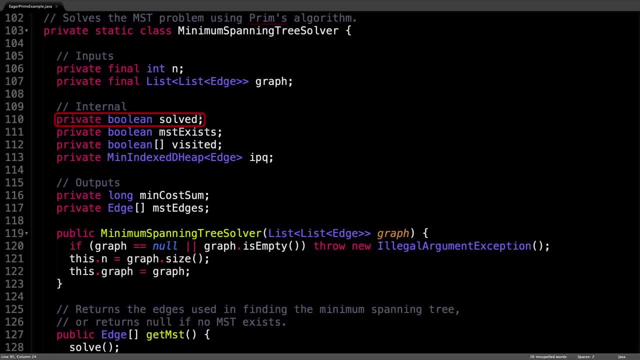 list itself. Internally, I store a Boolean solved variable to track whether we have already computed the minimum spanning tree, so that we don't need to do it again Once we've already solved the problem. the MST exists variable tells you whether a minimum spanning tree was found. 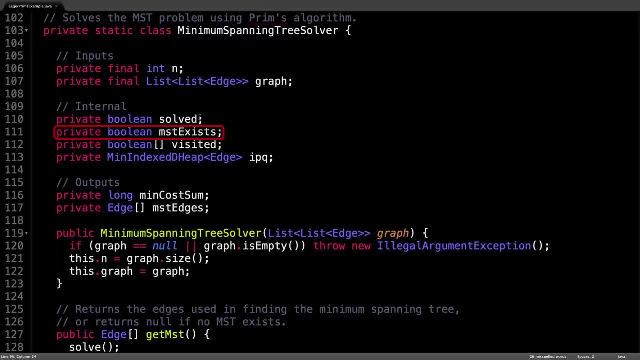 in the input graph. It's important to note that, by default, this value is false. The Boolean visited array is used to keep track of whether node I has been visited or not, And it's important to note that the Boolean visited array is used to keep track of whether. 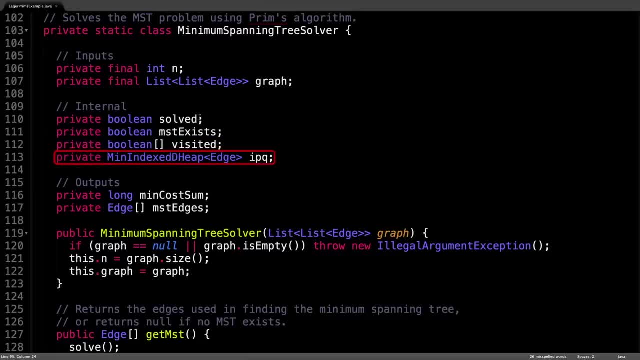 node I has been visited or not. The Boolean visited array is used to keep track of whether node I has been visited or not. And, lastly, is the variable IP queue, which is short for indexed priority queue, which is a data structure I have defined below The outputs to this: 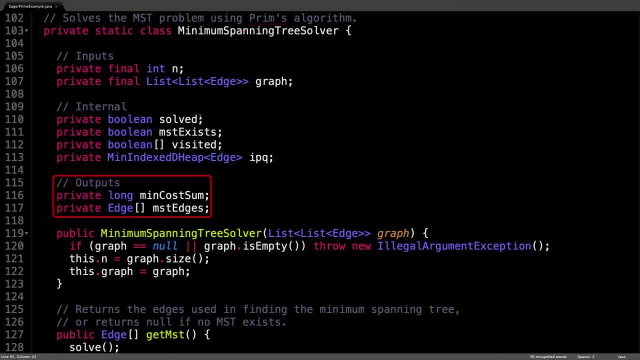 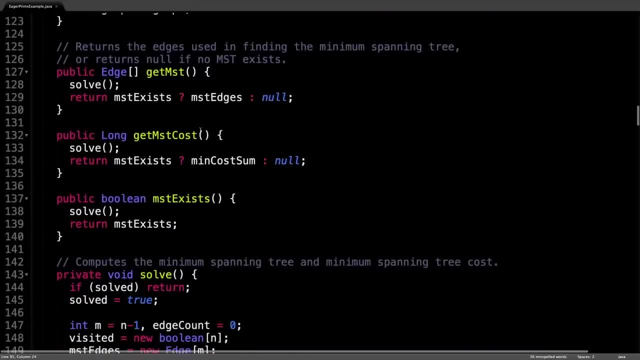 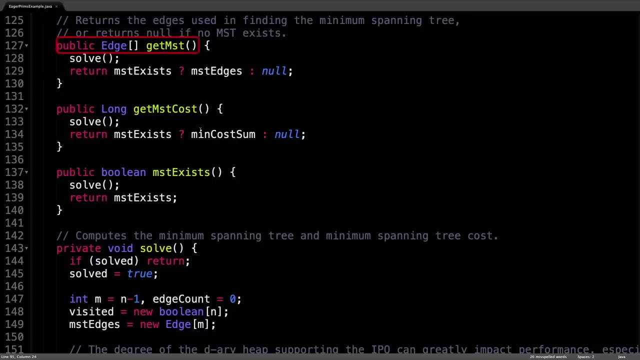 class include the minimum spanning tree costs and the edges which make up the minimum spanning tree if one exists, After the constructor and initialization. there are two important methods to know about. there is the constructor initialization And the constructor initialization is the get MST method for retrieving the MST edges and get MST cost which gets the spanning. 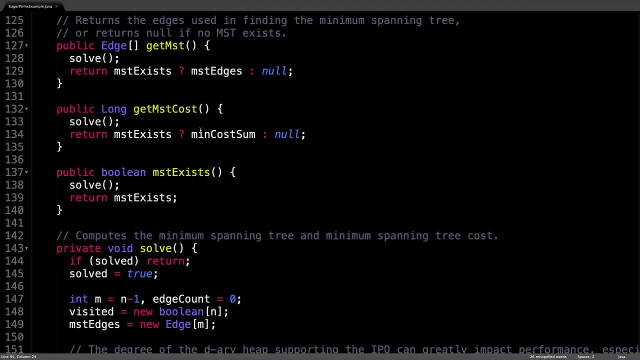 tree cost. Both of these methods work in the same manner. they both call the solve method and then check whether the minimum spanning tree exists and returns a value or no. Therefore, the real method we care about is the solve method. So let's have a look at that. 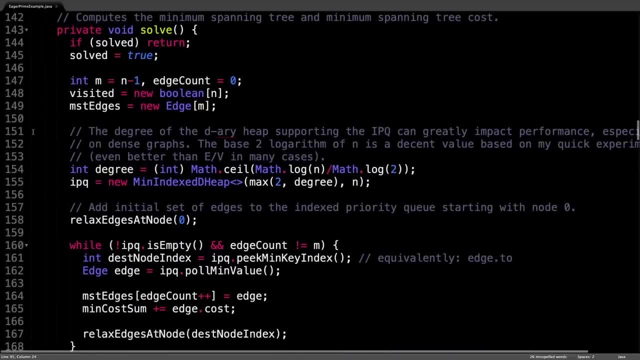 Okay, so the solve method is only ever executed once, because we mark the solve, the Boolean value, as true the first time solve is called And the other times the method returns early. The first thing I do in the solve method is initialize some more variables and allocate. 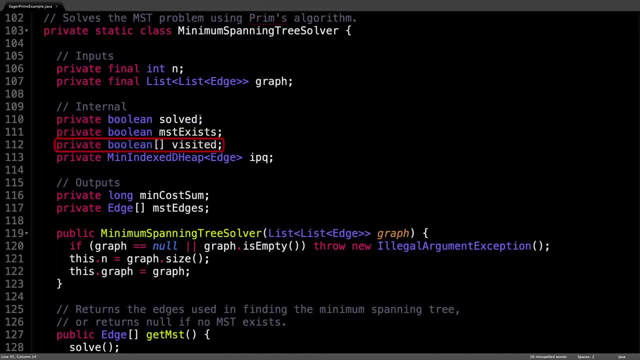 value is false. The Boolean visited array is used to keep track of whether node i has been visited or not. And, lastly, is the variable Ipq queue, which is short for indexed priority queue, which is a data structure I have defined below. The outputs to this class include the minimum spanning tree costs and the edges. 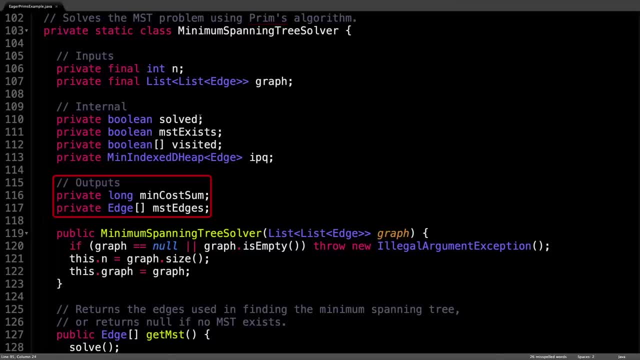 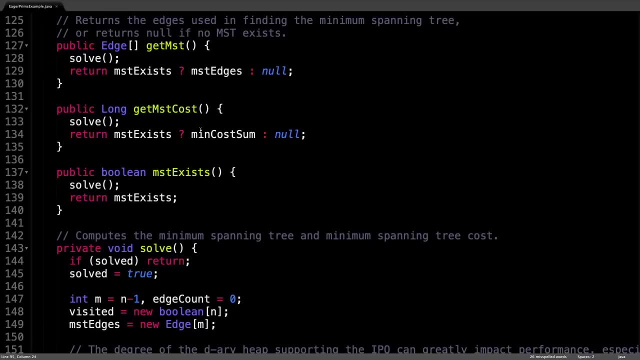 which make up the minimum spanning tree, if one exists After the constructor initialization. there are two important methods to know about. there is the get MST method for retrieving the MST edges, and get MST cost, which gets the spanning tree cost. Both of these methods work in the same manner. they both call the solve method. 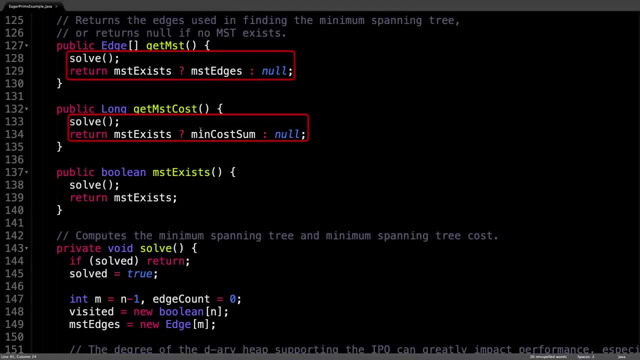 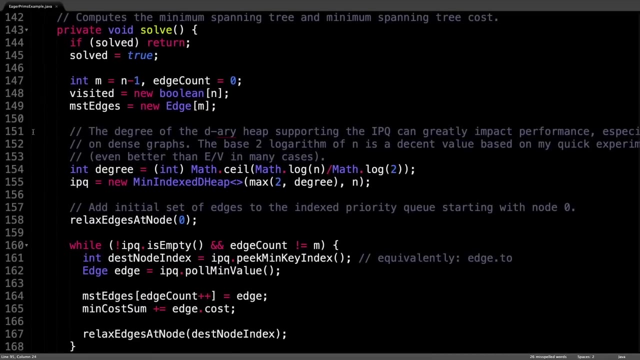 and then check whether the minimum spanning tree exists and returns a value or no. Therefore, the real method we care about is the solve method. So let's have a look at that. Okay, so let's have a look at that. The solve method is only ever executed once, because we mark the solve Boolean value as 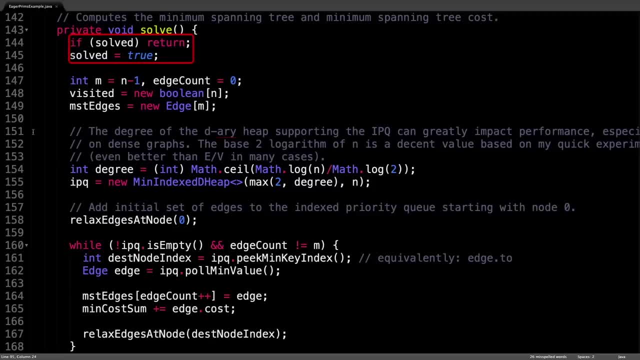 true, the first time solve is called And the other times the method returns early. The first thing I do in the solve method is initialize some more variables and allocate some memory for the arrays we will be using. M is the expected number of edges in a minimum spanning. 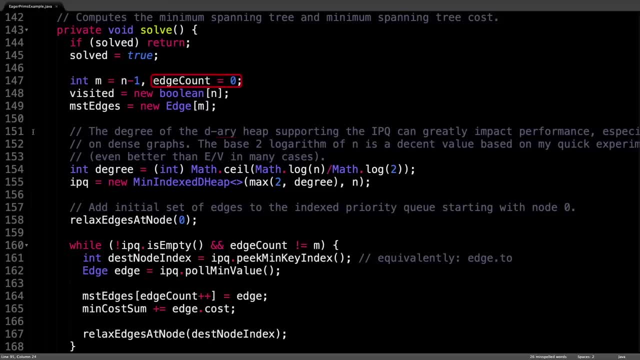 tree And edge count is the number of edges we have And edge count is the number of plants we have, And the empty value gets calculated for the array by the query And then after that, the query is parsley used in the function of an arrow that can be used to assign the value that we are going to be using today. 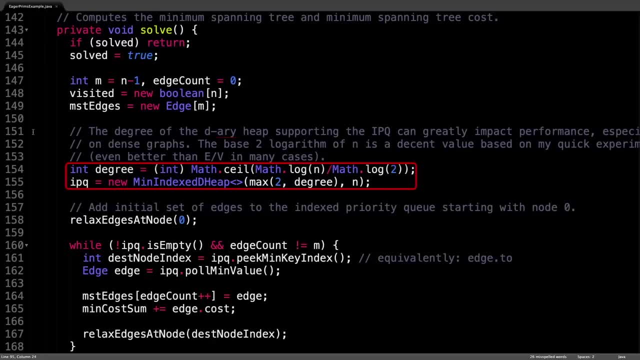 So that is a pretty simple example of reading an array that we know. So now that the query we just did with a query, let's turn it over to our radiator And we're going to try and see how this works. So let's go back to our base two source And let's do a test. So 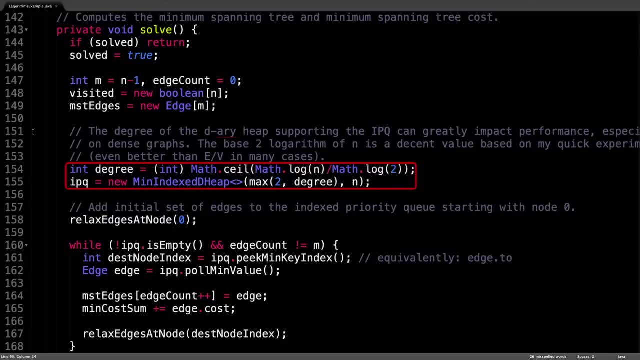 in our case, let's first do a test. So here we've got the base two source and we're going to use a nice base two node to get that value. So we're going to choose the base two. but you can also choose a base two node without the base two node. So what that'll do is 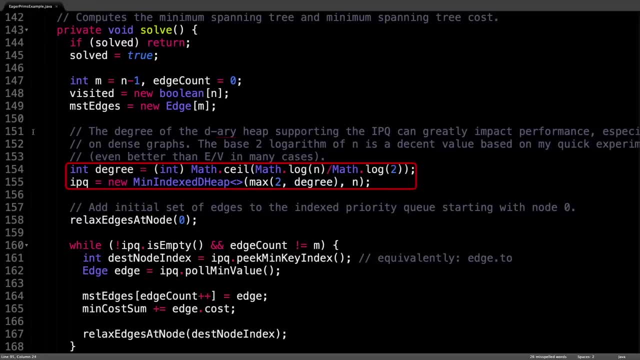 pretty good performance, Although typically this is an implementation detail that you do not need to worry about. The first actual bit of logic we're going to do is call relax edges at node for node zero. This adds the initial set of edges to the priority queue. 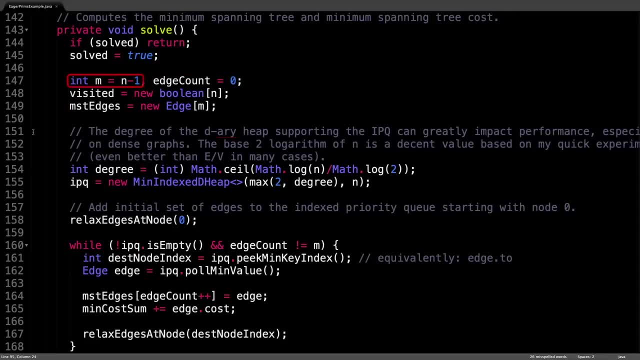 some memory for the arrays we will be using. M is the expected number of edges in a minimum spanning tree And edge count is the number of edges we have currently used. So the number of edges we have currently included in the minimum spanning tree so far. Next, I initialize. 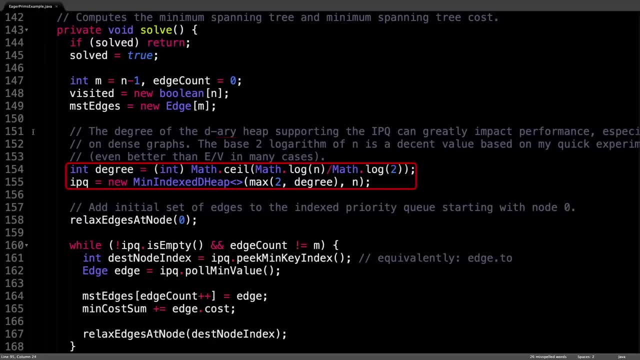 an indexed priority queue of size n. this particular indexed priority queue is implemented using a dairy heap, So we need to provide a node degree for the underlying supporting heap structure. I arbitrarily choose the base two logarithm of the number of nodes, which actually seems to give a pretty good performance, Although typically this is an implementation. 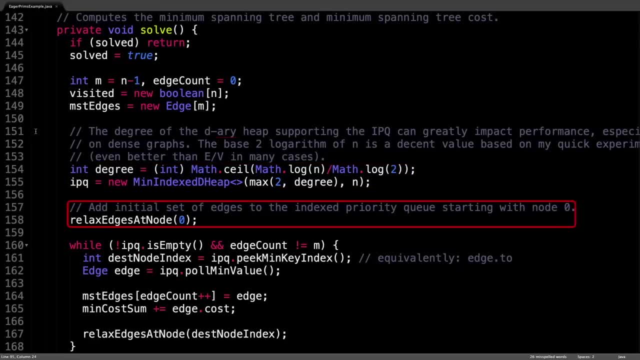 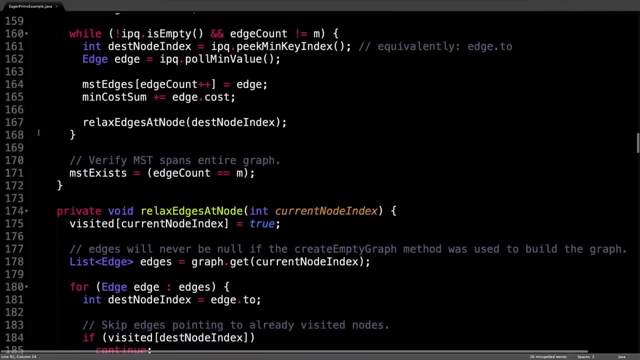 detail that you do not need to worry about. The first actual bit of logic we're going to do is call relax edges at node for node zero. this adds the initial set of edges to the priority queue. Let's scroll down and take a closer look at that method, which is: 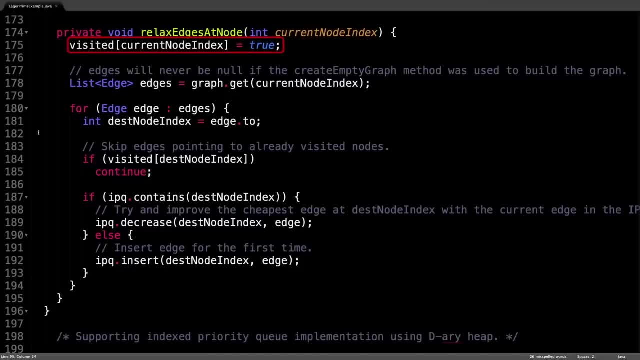 right here. The first thing we do is mark the current node as visited so that we don't visit it again in the future. then I reach into the adjacency list and get all the outgoing edges from the current node. As we enter the loop and start iterating over all the outgoing edges, the first thing 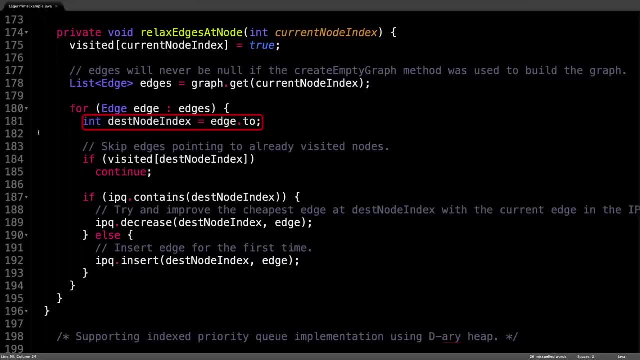 I do inside the loop is grab a reference to the destination node index. This is the node the edge is pointing at. Next skip edges which point to already visited nodes, because we know that we don't want to process those Now. here's the bit where we actually relax. 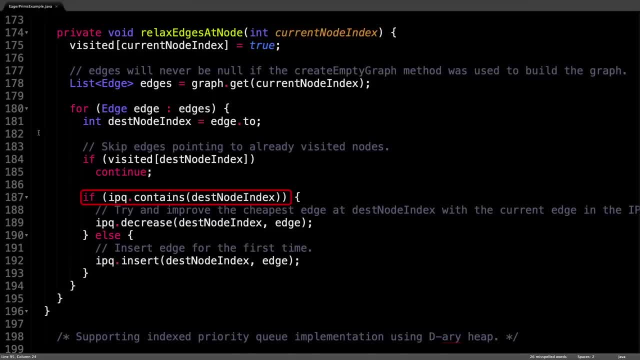 the edge. First check if the index priority queue contains the key with the value of the destination node. If it doesn't, then add the edge to the index priority queue for the first time. Otherwise try and improve the cheapest edge at the destination node index. 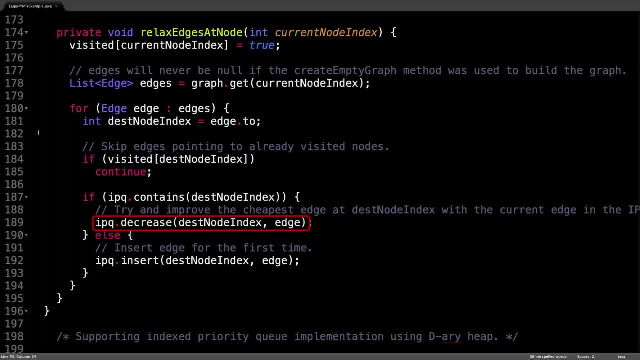 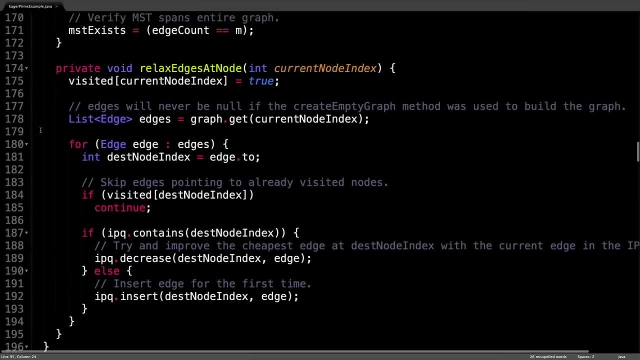 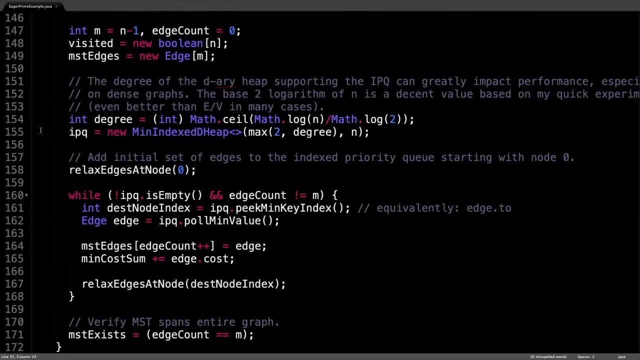 with the current edge in the priority queue by calling the decrease function. So that's all for the relax edges at node method. Let's scroll back up to the main implementation right here. So after we add the initial set of edges to the index priority queue, we enter: 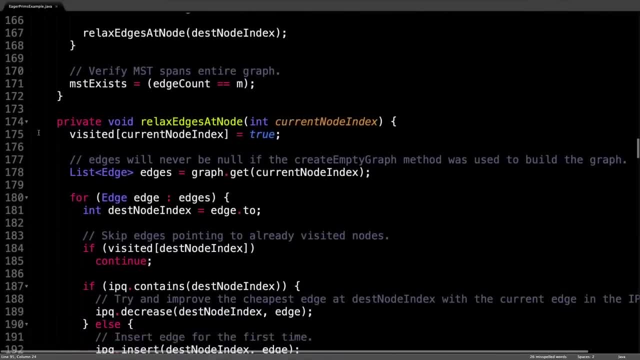 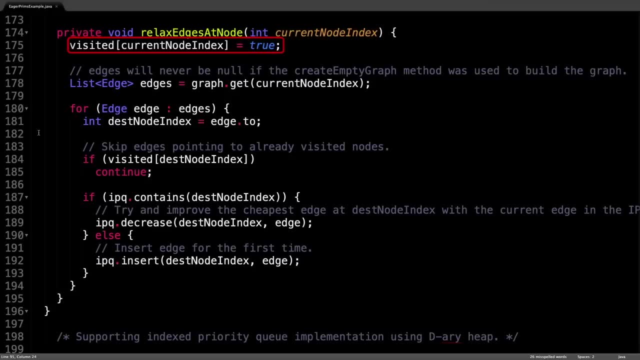 Let's scroll down and take a closer look at that method, which is right here. The first thing we do is mark the current node as visited so that we don't visit it again in the future. Then I reach into the adjacency list and get all the outgoing edges from the current node. 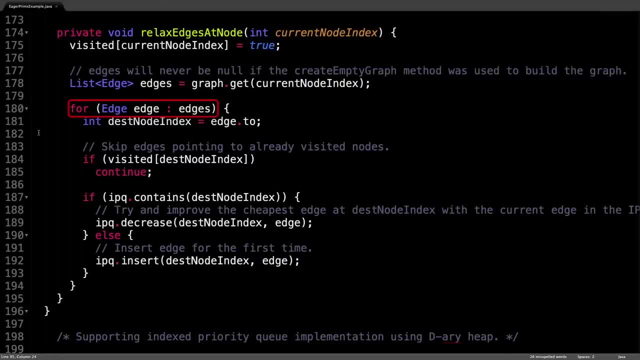 As we enter the loop and start iterating over all the outgoing edges, the first thing I do inside the loop is grab a reference to the destination node index. This is the node that edge is pointing at. Next skip edges which point to already visited nodes, because 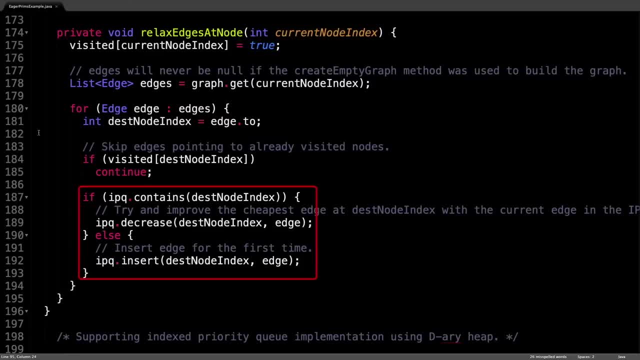 we know that we don't want to process those. Now here's the bit where we actually relax the edge. First we're going to go to the destination node index, And then we're going to go to the destination node index, And then we're going to go to the destination node index, And 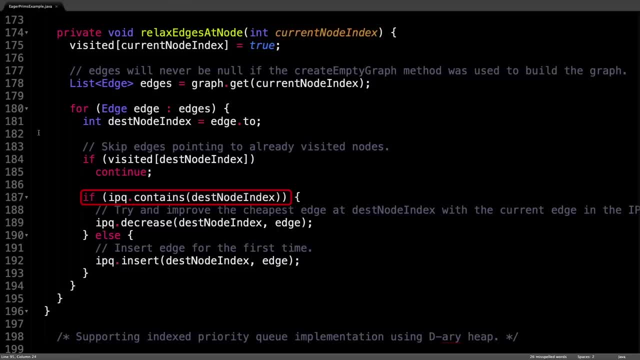 first check if the index priority queue contains the key with the value of the destination node. If it doesn't, then add the edge to the index priority queue for the first time. Otherwise, try and improve the cheapest edge at the destination node index with the current 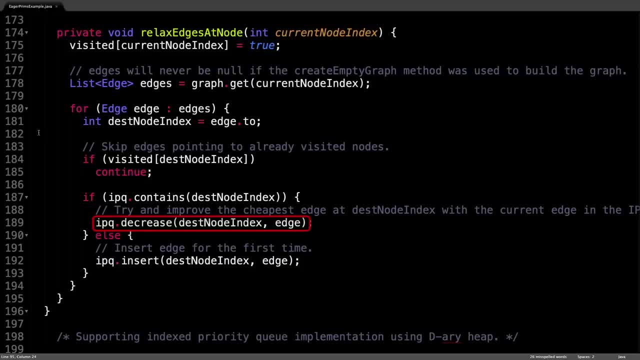 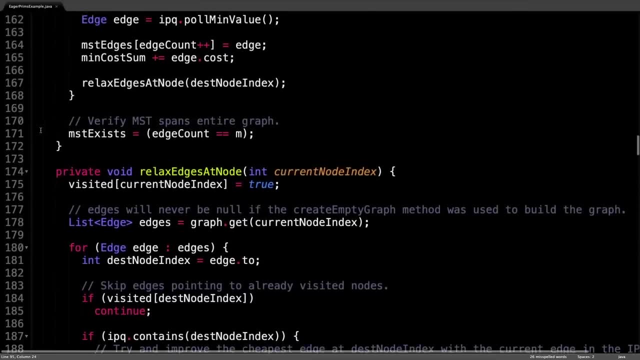 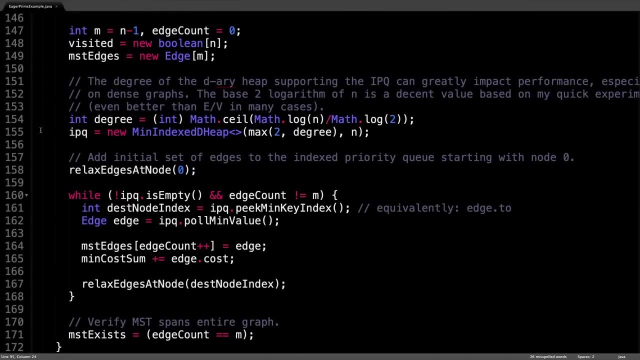 edge in the priority queue by calling the decrease function. So that's all for the relax edges at node method. Let's scroll back up to the main implementation right here. So after we add the initial set of edges to the index priority queue, we enter a while loop and loop while. 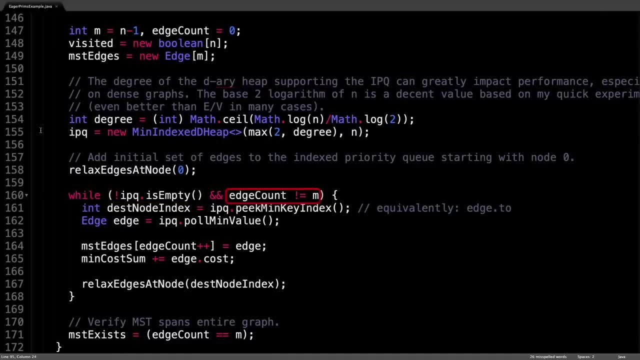 the index priority queue is not empty and a minimum spanning tree has not been formed inside the loop. pull out the next best node index edge pair. the destination node can also be found by checking which node the directed edge we just pulled out of the queue is pointing. 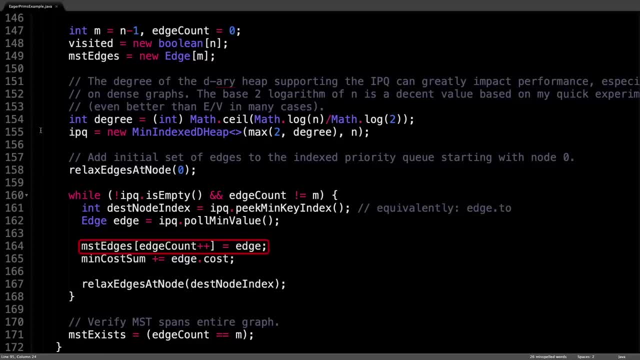 at. After that, add the pulled edge to the minimum spanning tree by placing it inside the MST edges array and sum over the edge costs. Finally, relax all the edges of the new current node. this process continues And we keep pulling the next best edge and 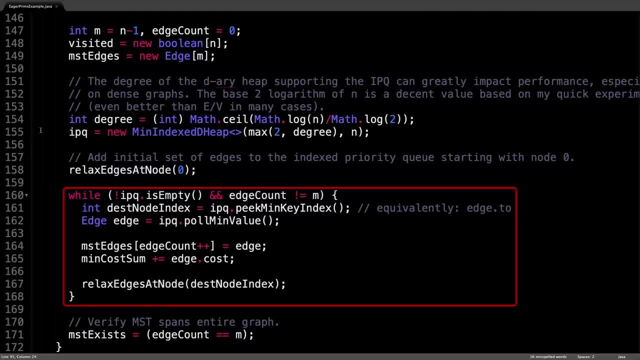 slowly start building our minimum spanning tree until eventually the loop breaks. The last thing we need to do is set the MST exists variable to check if we have actually found a minimum spanning tree. If the F count is equal to m, then M equals the minimum spanning. 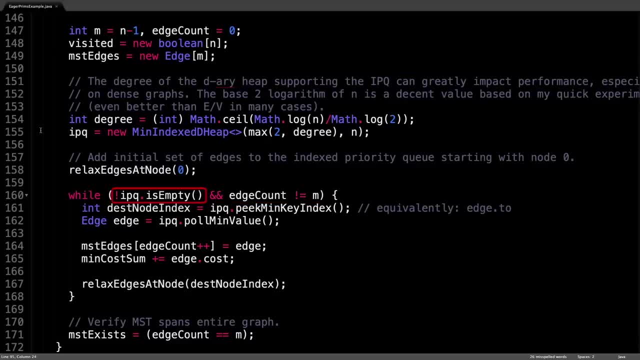 a while loop and loop. while the index priority queue is not empty and a minimum sin banning tree has not been formed Inside the loop, pull out the next best node index edge pair. the destination node can also be found by checking which node the directed edge we just pulled. 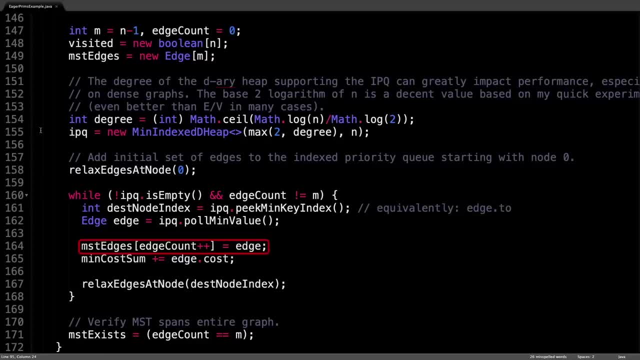 out of the queue is pointing at: After that, add the pulled edge to the minimum spanning tree by placing it inside the MST edges array and sum over the edge costs. Finally, relax all the edges of the new current node. this process continues and we keep. 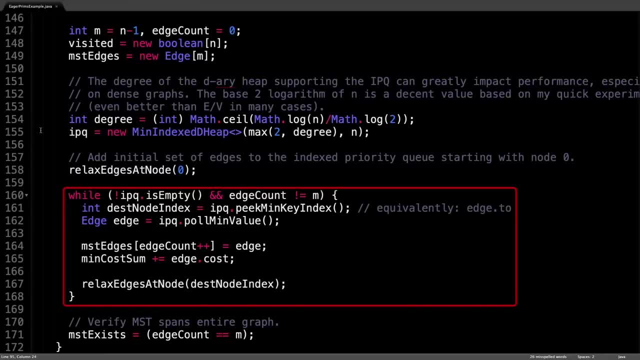 pulling the next best edge and slowly start building our minimum spanning tree until eventually the loop breaks. The last thing we need to do is set the MST exists variable to check if we have actually found a minimum spanning tree. If the edge count is equal to M, then 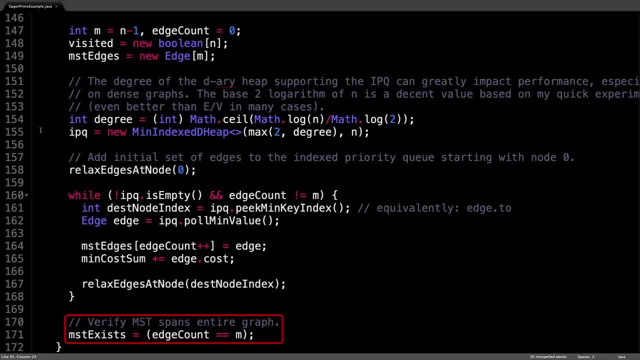 we have successfully computed a minimum spanning tree. Otherwise, the minimum spanning tree should be set to the minimum spanning tree. If the edge count is equal to M, then we have successfully computed a minimum spanning tree. Otherwise, the minimum spanning tree should be set to the minimum spanning tree. Otherwise, the graph is disconnected in some way and 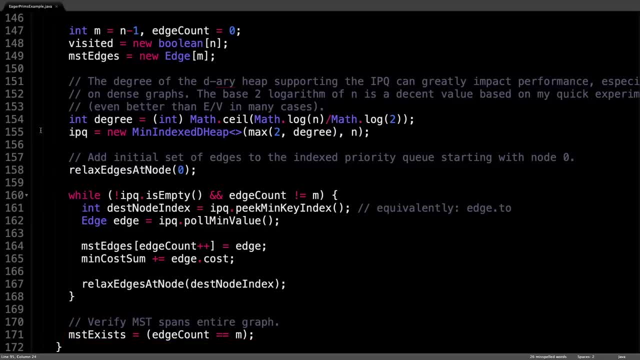 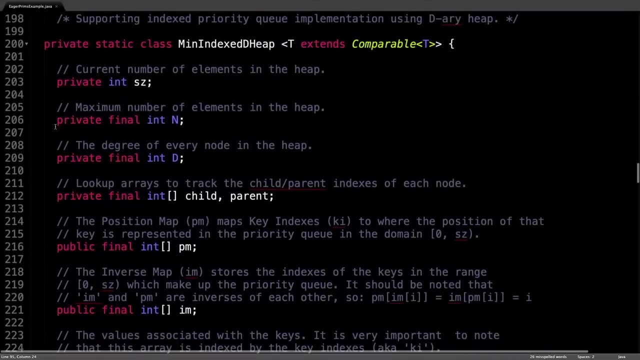 no spanning tree exists. So that's all for the eager implementation of prims. The only piece of the puzzle that might still be unclear is how the index party queue implementation works. Here's the index party queue implementation. However, this data structure merits a video. 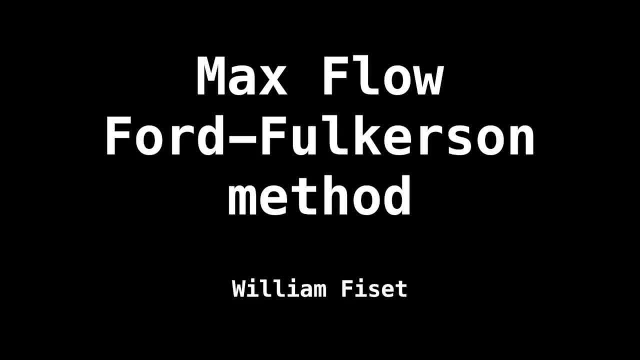 on its own. Today, we're going to start tackling the field of nets network flow by understanding what max flow is and, in particular, how we can use the Ford Fulkerson method to find it. Finding the maximum flow begins with having what's. 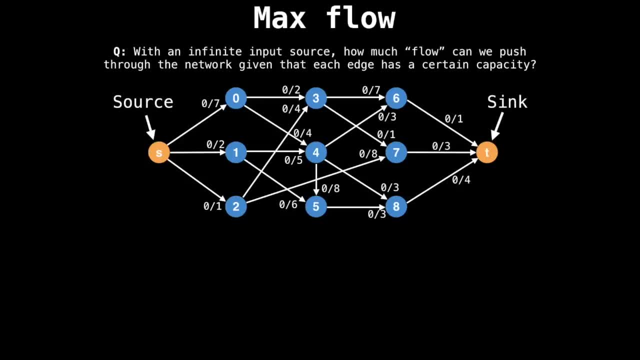 called a flow graph. This is a graph where edges have a certain maximum capacity which cannot be exceeded. Edges also have a flow value, which is how many units of flow are passing through that edge. Initially, the flow is zero for all edges everywhere, until we run a max flow algorithm. 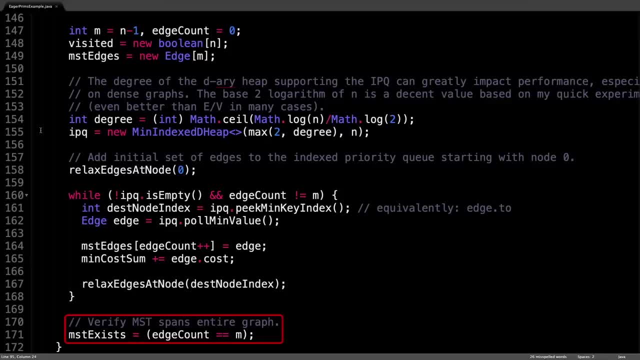 tree. the next best edge is the minimum spanning tree. If the H count is equal to m, then the M and the index priority queue is equal to M, So we'll use this variable to set the mst. then we have successfully computed a minimum spanning tree. Otherwise the graph is disconnected. 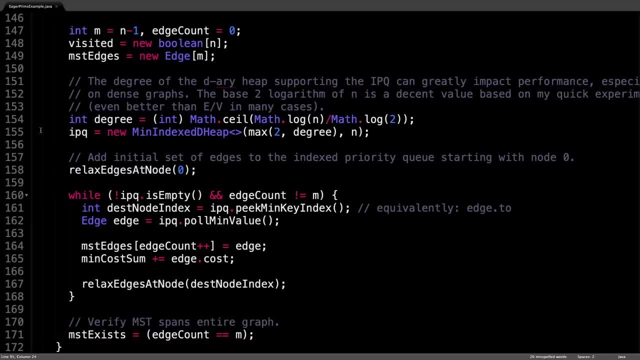 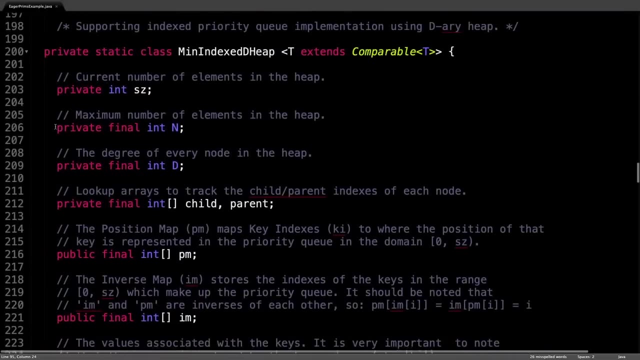 in some way, and no spanning tree exists. So that's all for the eager implementation of prims. The only piece of the puzzle that might still be unclear is how the index party queue implementation works. Here's the index party queue implementation. However, this data structure. 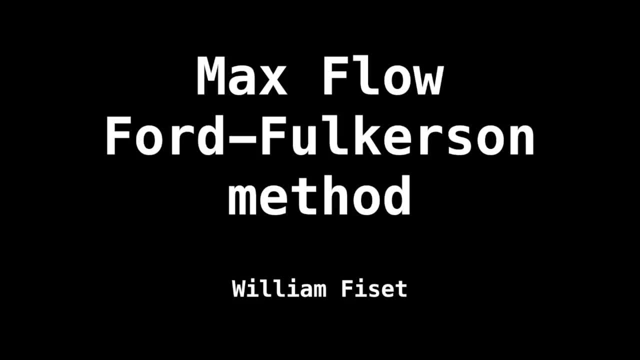 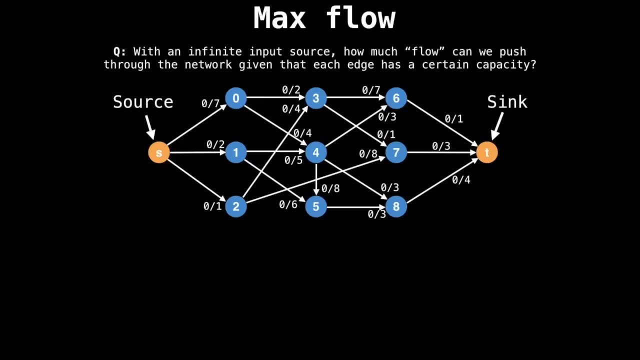 merits a video on its own. Today we're going to start tackling the field of network flow by understanding what max flow is and, in particular, how we can use the Ford Fulkerson method to find it. Finding the maximum flow begins with having what's called a flow graph. 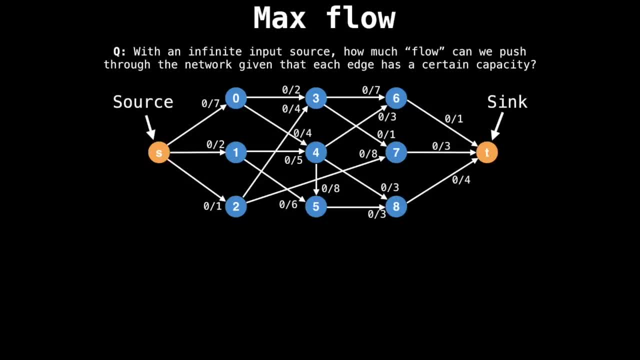 This is a graph where edges have a certain maximum capacity which cannot be exceeded. Edges also have a flow value, Which is how many units of flow are passing through that edge. Initially, the flow is zero for all edges everywhere, until we run a max flow algorithm on it. There are also 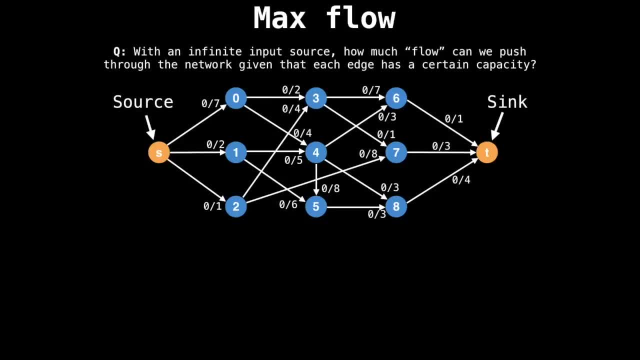 two special types of nodes in the flow graph: the source node and the sink node, usually denoted as s and t respectively. The maximum flow problem asks, with an infinite input source, how much flow can we push through Through the network without exceeding the capacity of any edge? And it's not obvious. 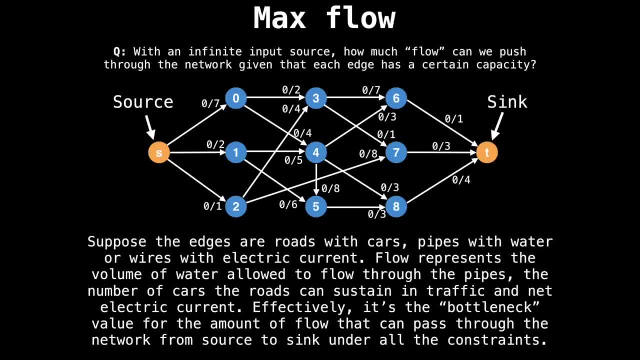 how one should figure that out. Maximum flow can be used in numerous situations where edges and nodes can represent any number of things. For instance, suppose the edges or roads, cars or pipes with water wires, with electric current, and so on. Each of those has a certain. 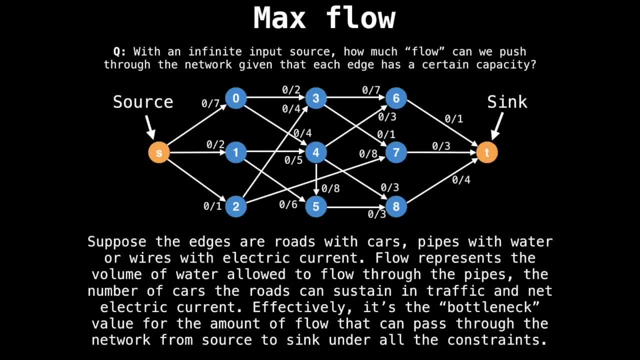 capacity value we can associate with The maximum, on the other hand, would represent the volume of water that can flow through the pipe, So the number of cars the roads can sustain and traffic or the net electric current that your system can sustain Effectively. the maximum flow is a bottleneck value for the amount. 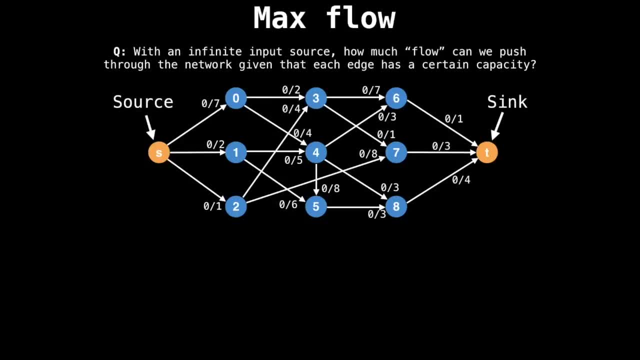 on it. There are also two special types of nodes in the flow graph: the source node and the sink node, usually denoted as s and t respectively. The maximum flow problem asks, with an infinite input source, how much flow can we push through the network without exceeding the capacity? 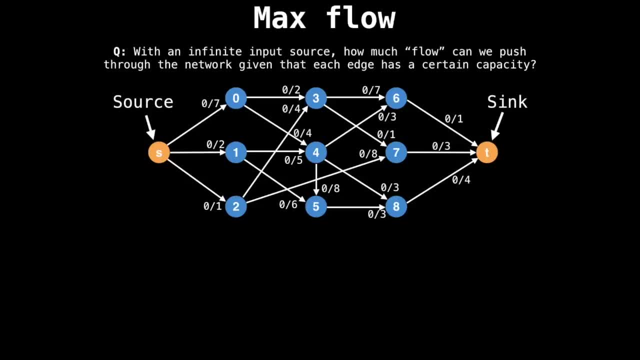 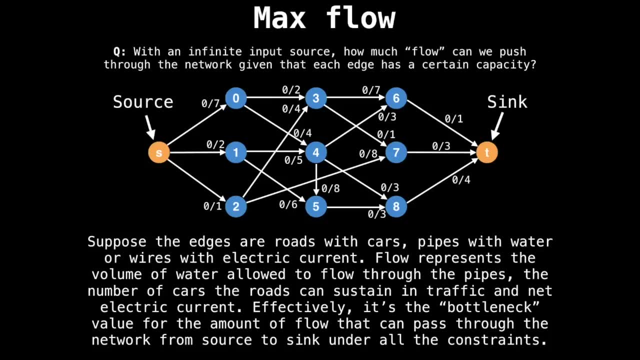 of any edge, And it's not at all obvious how one should figure that out. Maximum flow can be used in numerous situations where edges and nodes can represent any number of things. For instance, suppose the edges are roads with cars or pipes with water, wires with electric current and 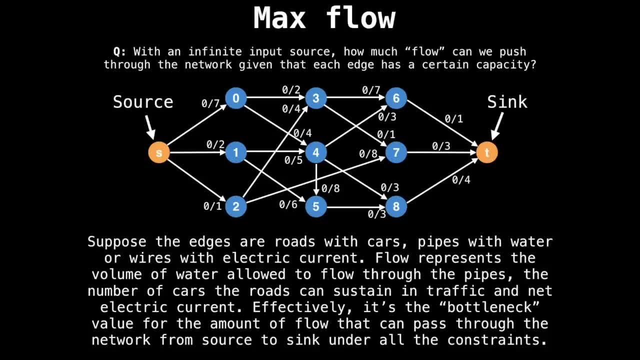 so on. Each of those has a certain capacity value we can associate with the maximum flow, on the other hand, would represent the volume of water that can flow through the pipe, And so the number of cars the roads can sustain and traffic, or the net electric current that. 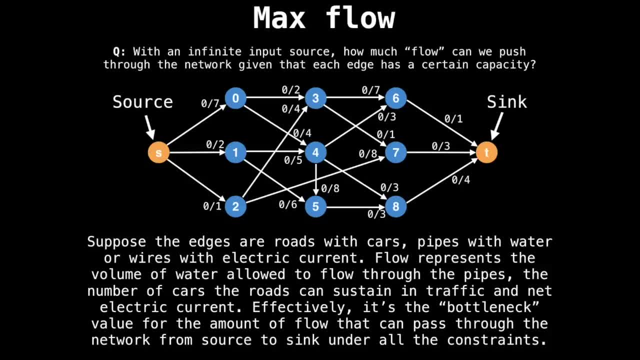 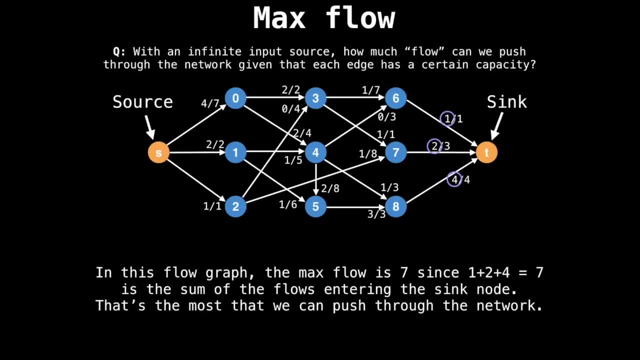 your system can sustain Effectively. the maximum flow is a bottleneck value for the amount of traffic your network can handle, And that is going from the source to the sink. under all those constraints, The maximum flow for this particular network is seven And. 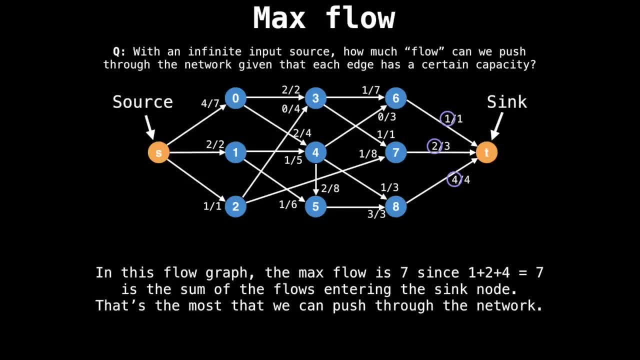 you can tell because, after running the maximum flow algorithm, the sum of the flows attached to the sink node is seven. running a maximum flow algorithm is used to determine how much flow each edge should receive to achieve the overall maximum flow. Note that there might 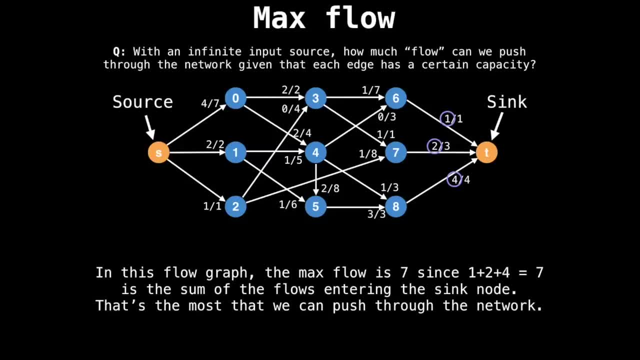 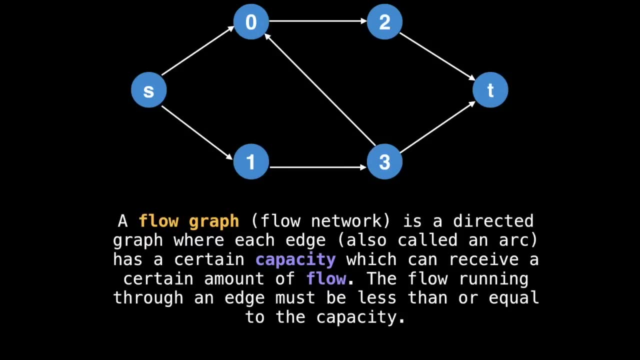 be multiple ways of achieving the maximum flow, by giving each edge different flow values, but overall solutions will have the same maximum flow. Let's dig deeper into how to find the maximum flow. To begin with, you will need a flow graph which consists of directed edges, which are also called arcs. Each directed edge has 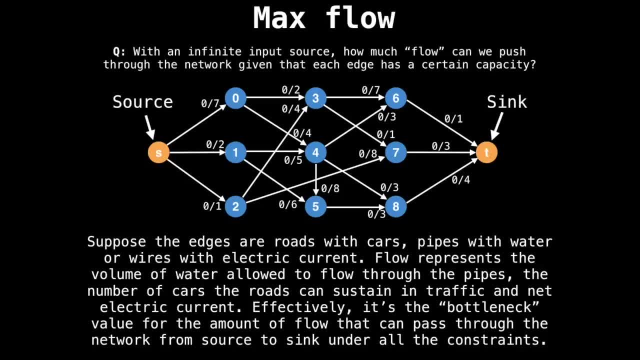 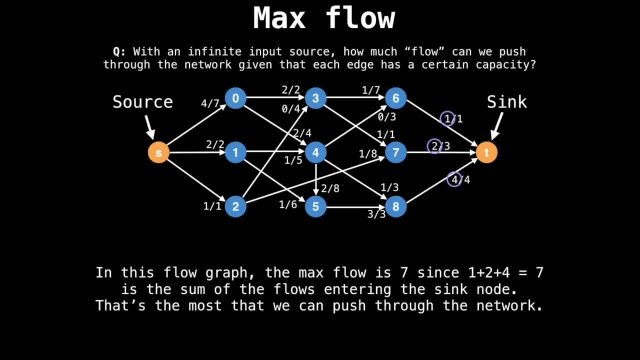 of traffic your network can handle And that is going from the source to the sink. under all those constraints, The maximum flow for this particular network is seven. And you can tell because, after running the maximum flow algorithm, the sum of the flows attached to the sink node is seven. Running a maximum flow algorithm is used to determine how much. 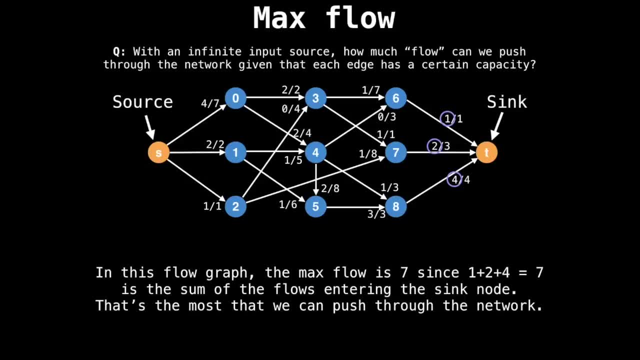 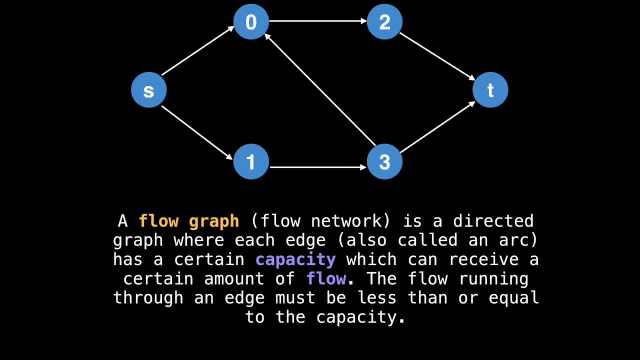 flow each edge should receive to achieve the overall maximum flow. Note that there might be multiple ways of achieving the maximum flow by giving each edge a maximum flow, of edge different flow values, but overall solutions will have the same maximum flow value. Let's dig deeper into how to find the maximum flow. To begin with, you will need a flow graph. 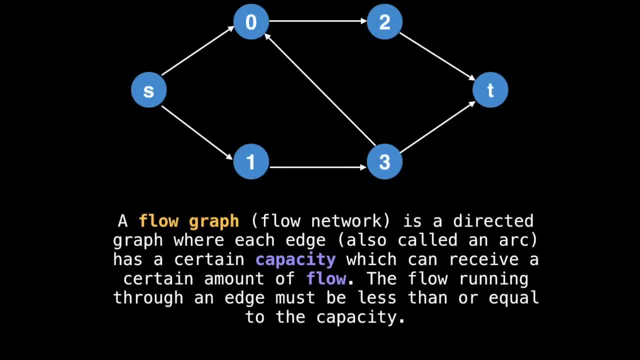 which consists of directed edges, which are also called arcs. Each directed edge has a certain capacity which can receive a certain amount of flow. At all times, the flow running through an edge must be less than or equal to the capacity. This intuitive way of running an edge must be less than or equal to the capacity. This 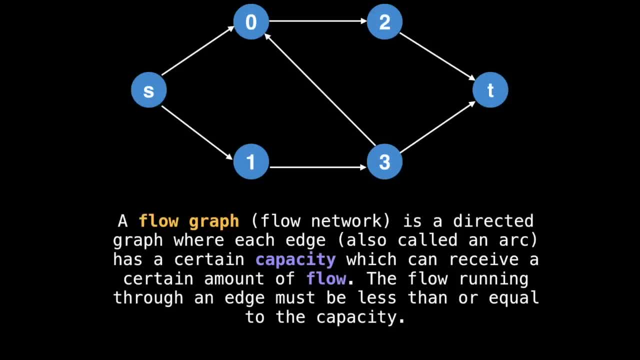 intuitive way of running an edge must be less than or equal to the capacity. This intuitive way of running an edge must be less than or equal to the capacity. This intuitive way makes sense because if we allow more flow than what the capacity permits, it means something. 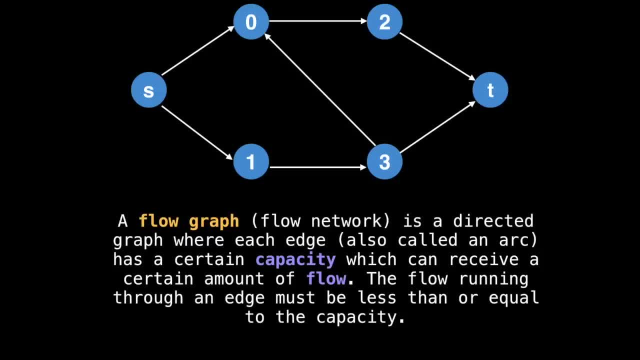 has to go wrong. When an edge becomes over capacitated in some manner, It means that we've pushed the system past its limit. In the context of edges representing pipes with water, It means your pipe broke or it leaked. if your edges a wire with electric current, 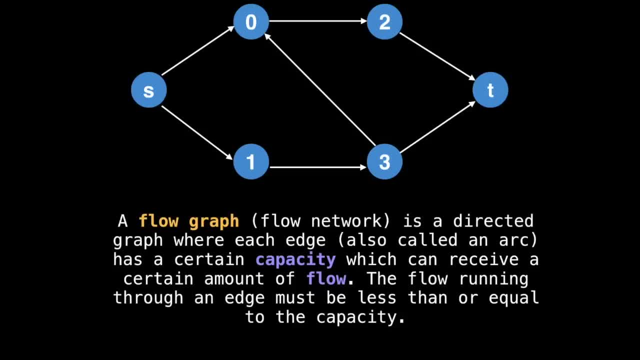 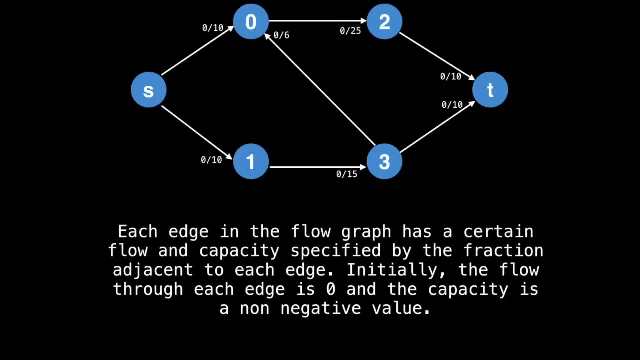 It means or wire, literally fried, or melted, exploded or something bad happened to it because there was too much electric current current. This is not good, So this is why we don't allow more flow than capacity. Each edge in the flow graph has a certain flow and capacity specified by the two values separated. 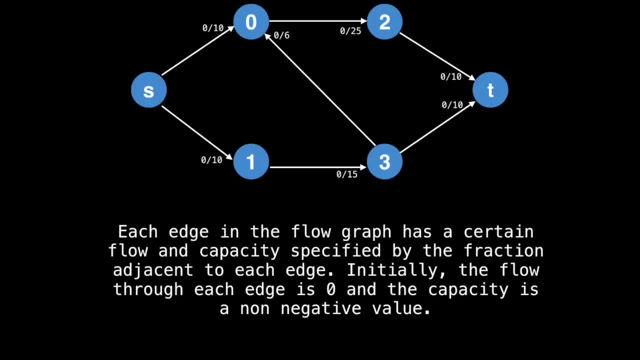 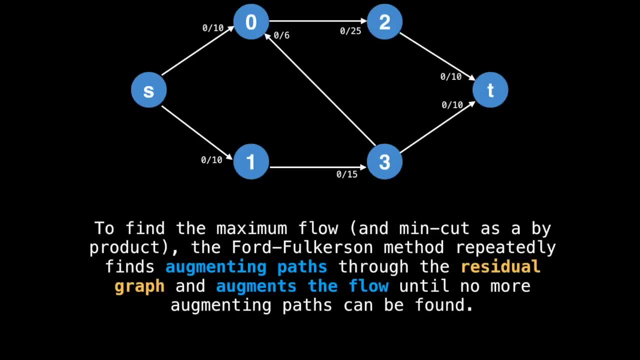 by a slash adjacent to each edge. Originally, the flow through each edge is zero and the capacity is a non negative value to find the maximum flow and also the min cut. as a byproduct, The Ford Fulkerson method repeatedly finds augmenting paths through the residual graph. 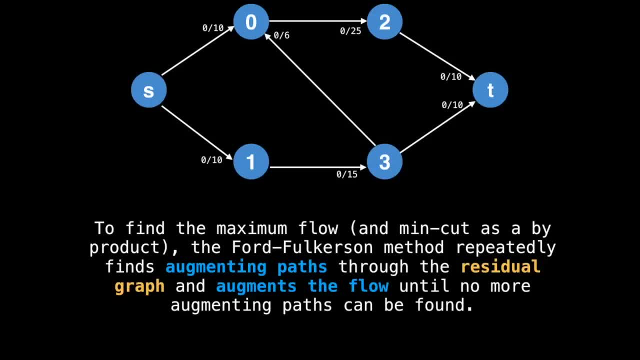 and augments the flow until no more augmenting paths can be found. So you're probably asking yourself at this moment: what is an augmenting path? What the heck is a residual graph, And what do you mean by augment the flow? All right, let me explain. We'll do them one by 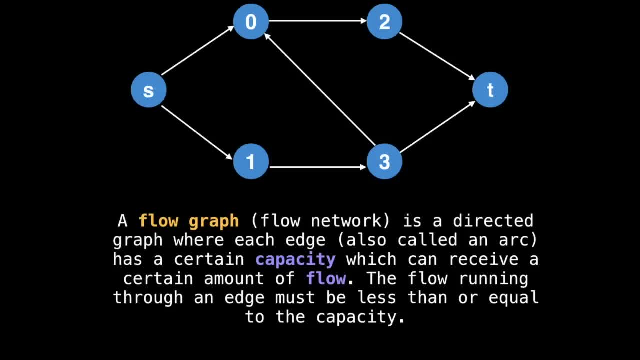 a certain capacity which can receive a certain amount of flow. At all times, the flow running through an edge must be less than or equal to the capacity. This intuitively makes sense because if we allow more flow than what the capacity permits, it means something has to go wrong When an edge becomes overcapacitated in some manner. 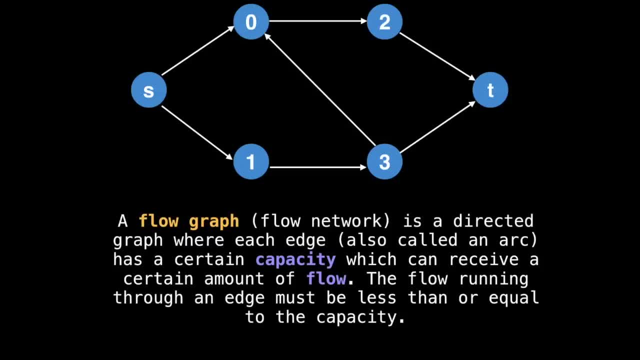 it means that we've pushed the system past its limit. In the context of edges representing pipes with water, it means your pipe broke or it leaked. If your edge is a wire with electric current, it means your wire literally fried or melted, exploded or something bad. 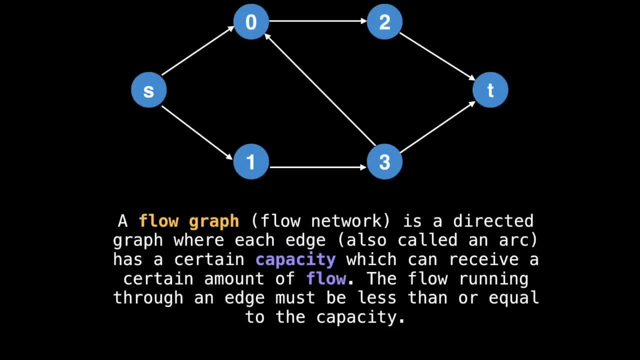 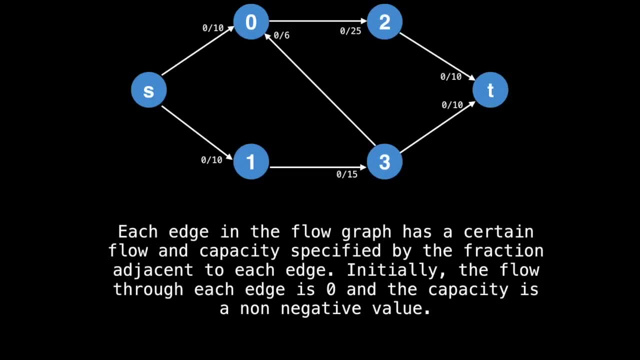 happened to it because there was too much electric current. This is not good, So this is why we don't allow more flow than capacity. Each edge in the flow graph has a certain flow and capacity specified by the two values, separated by a slash adjacent to each edge. 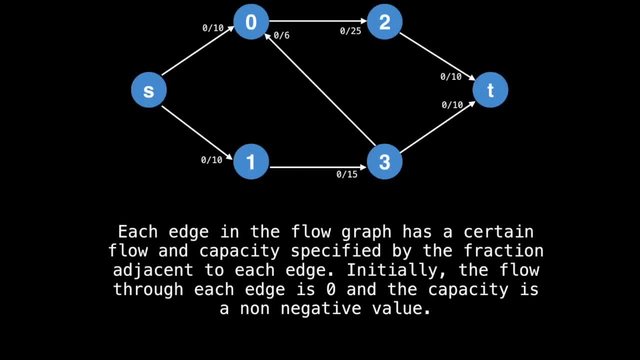 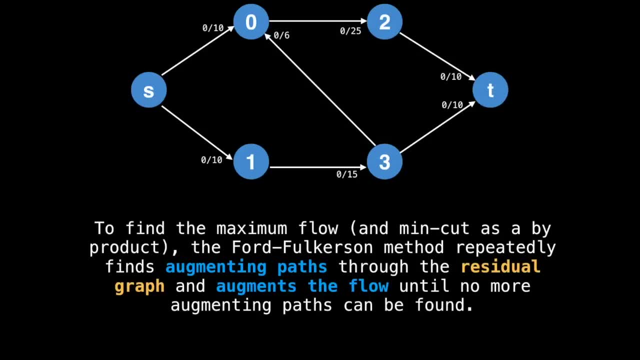 Originally, the flow through each edge is zero and the capacity is a non negative value to find the maximum flow and also the min cut. as a byproduct, The Ford Fulkerson method repeatedly finds augmenting paths Through the residual graph and augments the flow until no more augmenting paths can be found. So 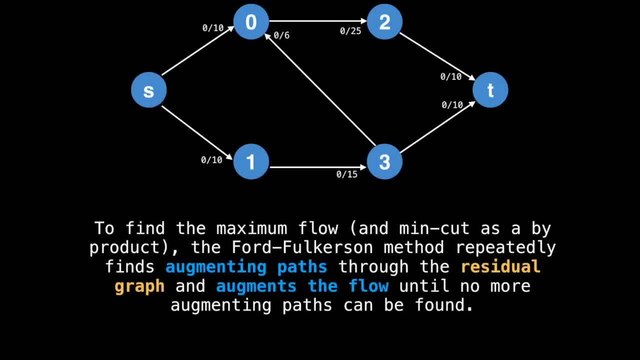 you're probably asking yourself at this moment: what is an augmenting path? What the heck is a residual graph, And what do you mean by augment the flow? Alright, let me explain. We'll do them one by one. An augmenting path is a path of edges in the residual graph, with 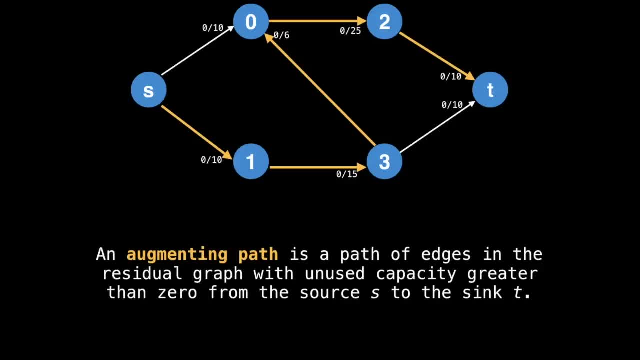 capacity greater than zero from the source s to the sink t In orange. here I have highlighted a possible augmenting path. The key thing to remember about an augmenting path is that they can only flow through edges which aren't fully saturated. yet. In fact, you know, you've. 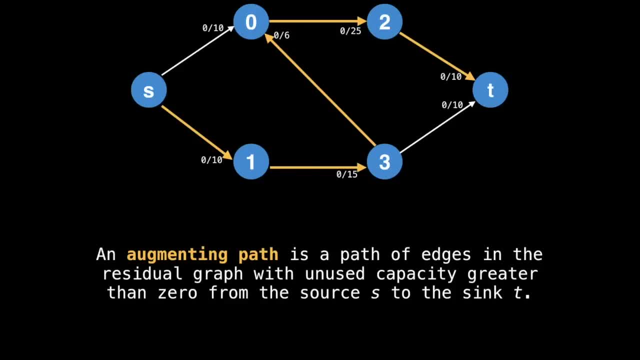 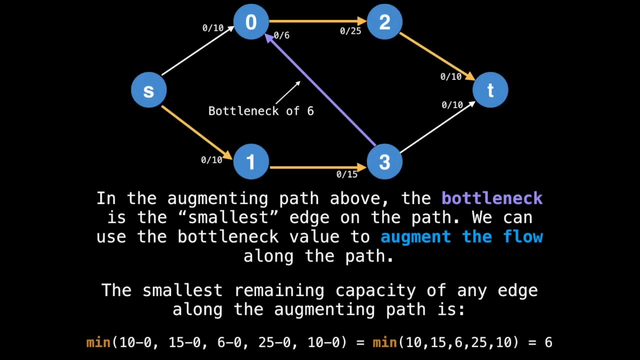 achieved the maximum flow when there are no more augmenting paths left to be found. How to actually find an augmenting path is a detail left unspecified by the Ford Fulkerson method for flexibility. For now, let's assume that we're using a depth for search Something. 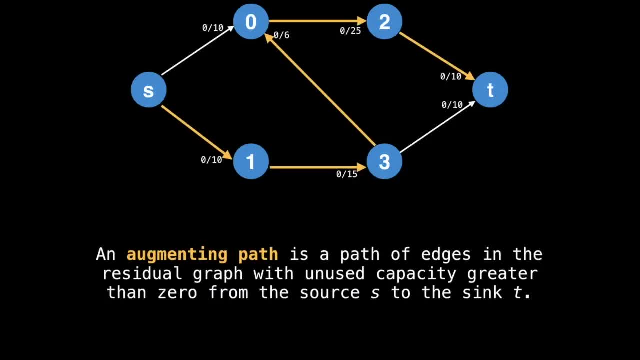 one And augmenting path is a path of edges in the residual graph with capacity greater than zero, from the source s to the sink t In orange. here I have highlighted a possible augmenting path. The key thing to remember about an augmenting path is that 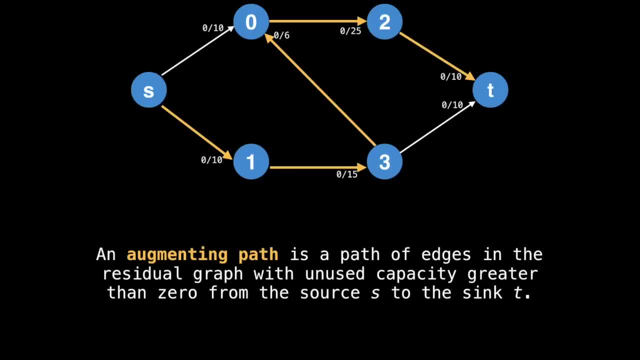 it can only flow through edges which aren't fully saturated yet. In fact, you know you've achieved the maximum flow when there are no more augmenting paths left to be found. How to actually find an augmenting path is a detail left unspecified by the Ford Fulker. 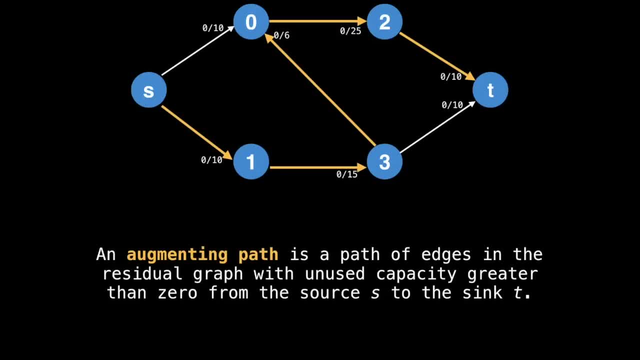 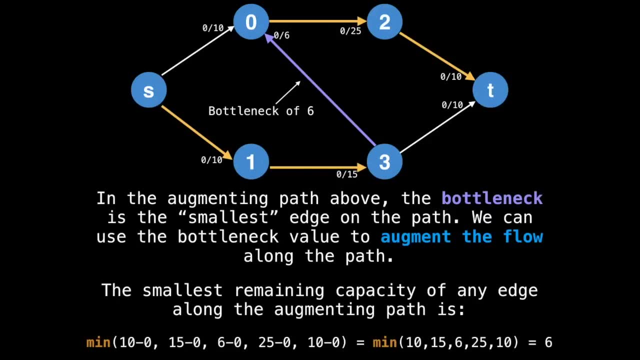 Fulkerson method for flexibility. For now, let's assume that we're using a depth for search. Something else to know is that every augmenting path will have what I call a bottleneck value, which is the smallest edge along the path you can find the value of the bottleneck. 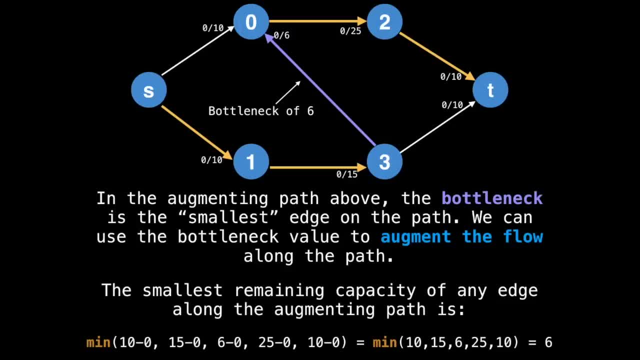 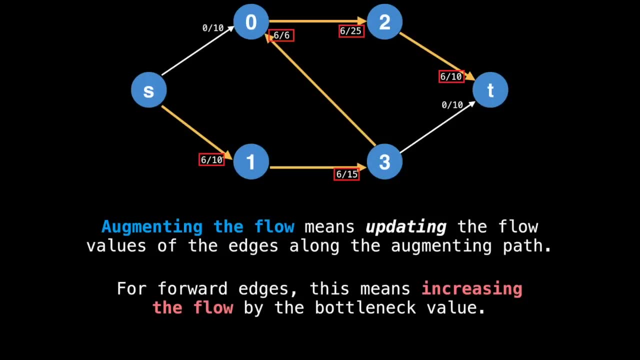 by taking the difference between the capacity and the current flow of an edge For this augmenting path, the bottleneck value is six. we can use the bottleneck value to argument the flow along the path. augmenting the flow simply means to update the flow values of the edges along the augmenting 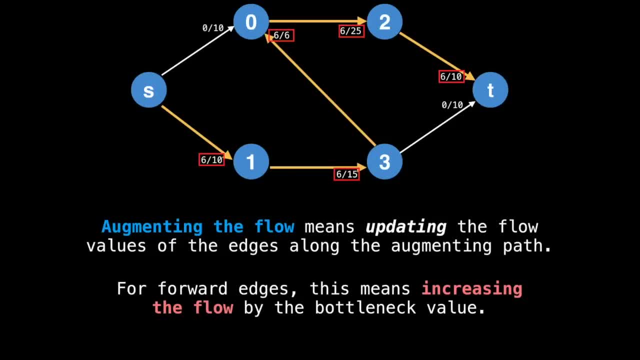 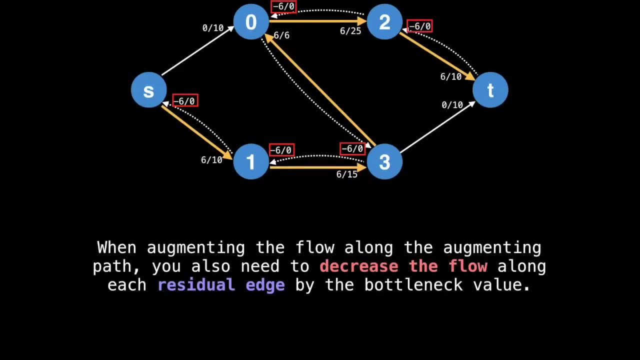 path. Here you can see that I've increased the flow of each edge along the augmenting path by exactly six units. However, we're not done augmenting the flow. we not only need to increase the flow along the forward edges, but also decrease the flow along the. 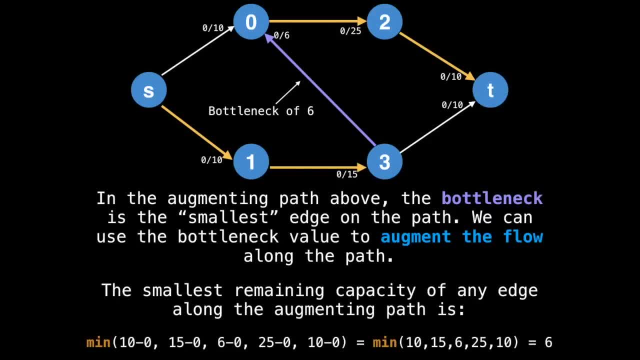 else to note is that the depth of the search is not equal to the depth of the structural. to know is that every augmenting path will have what I call a bottleneck value, which is the smallest edge along the path. you can find the value of the bottleneck by taking 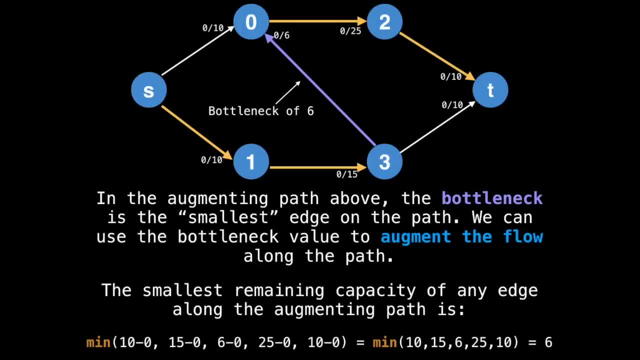 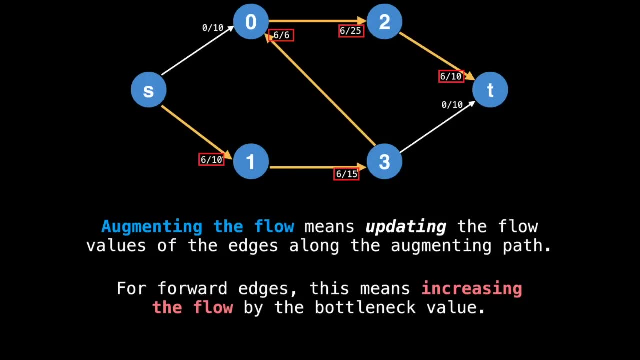 the difference between the capacity and the current flow of an edge. For this augmenting path, the bottleneck value is six. we can use the bottleneck value to argument the flow along the path. augmenting the flow simply means to update the flow values of the edges. 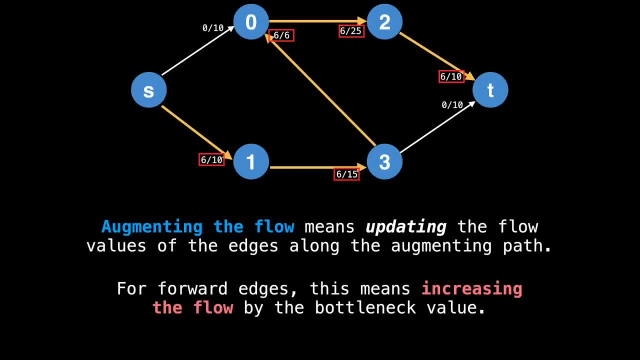 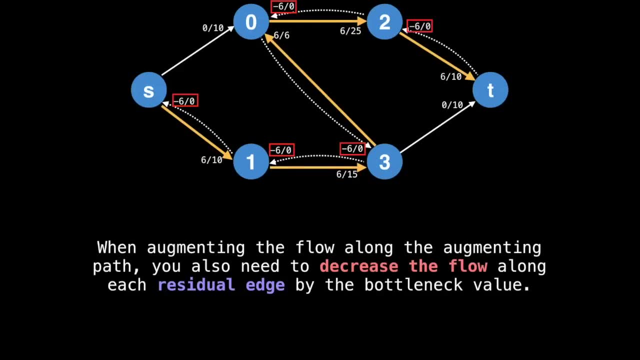 along the augmenting path. Here you can see that I've increased the flow of each edge along the augmenting path by exactly six units. However, we're not done augmenting the flow. we not only need to increase the flow along the forward edges, but also decrease the flow. 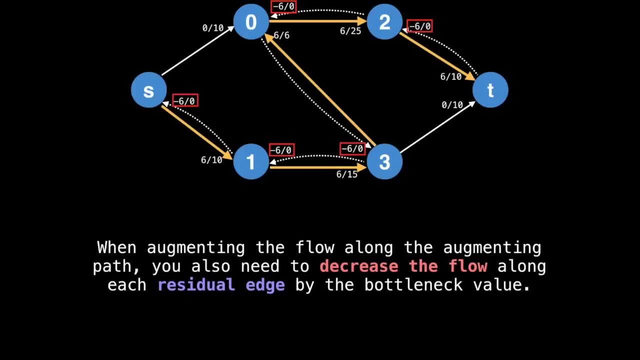 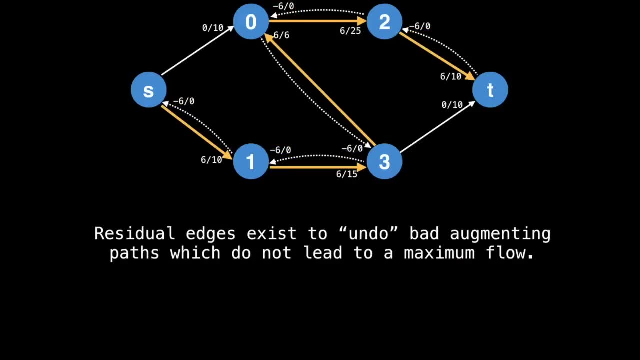 along the backwards edges, which are called residual edges. The residual edges are the dotted edges going backwards in the reverse order of the augmenting path. The logic behind having residual edges is to undo bad choices of augmenting paths which do not lead to. 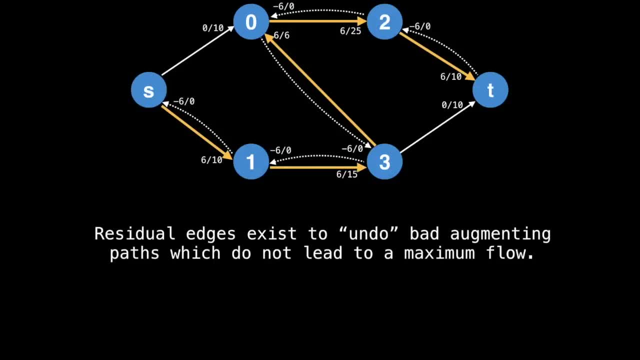 a maximum flow Effectively. we don't know which are the best, or even correct augmenting paths to take, So this mechanism enables us to freely find any augmenting paths without having to worry about whether or not we'll be able to achieve the maximum flow it should. 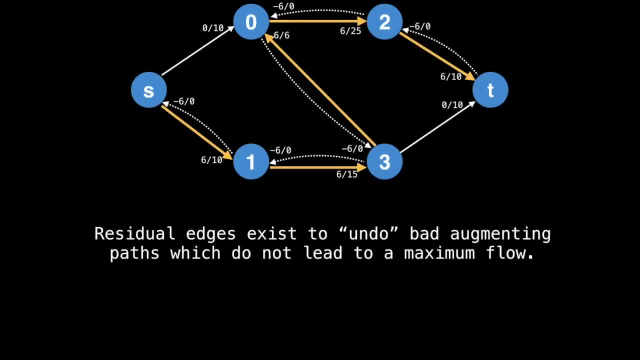 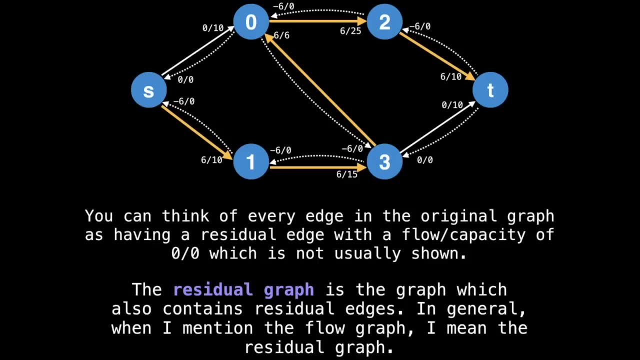 be mentioned that residual edges become valid edges to take, finding an augmenting path in later iterations. So if we take a step back, you can think of every edge in the original graph as having a residual edge with a flow and capacity of zero, which is not usually shown. Now that we know what residual edges are, the term 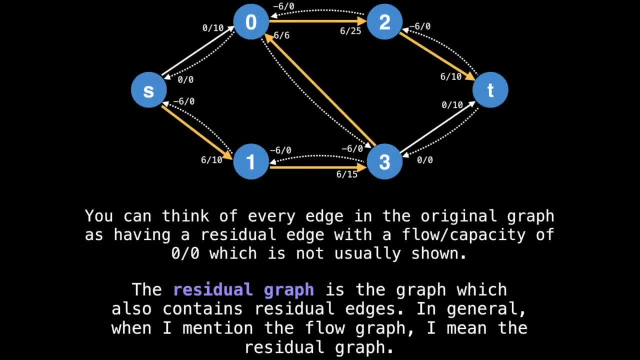 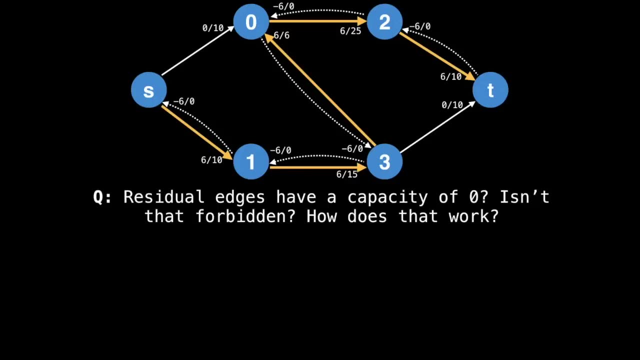 residual graph simply means the graph which also contains residual edges, not just the original edges given in the flow graph. So, generally speaking, when I mentioned the flow graph, I usually mean the residual graph. So here's a good question you might have at this point. the residual edges shown have 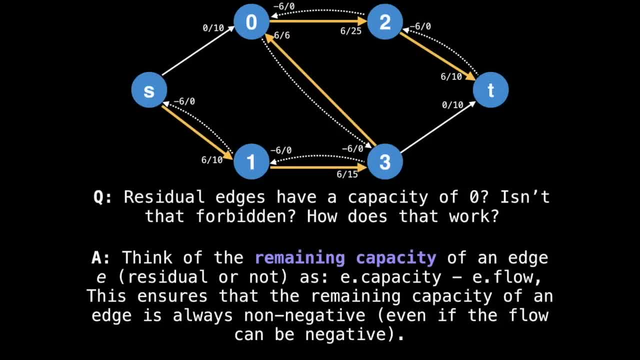 a capacity of zero. aren't those forbidden? How does that work? So here's the thing: With this method of augmenting the flow, you have to think of the remaining capacity of an edge E, residual or not, as the difference between the capacity and the flow. 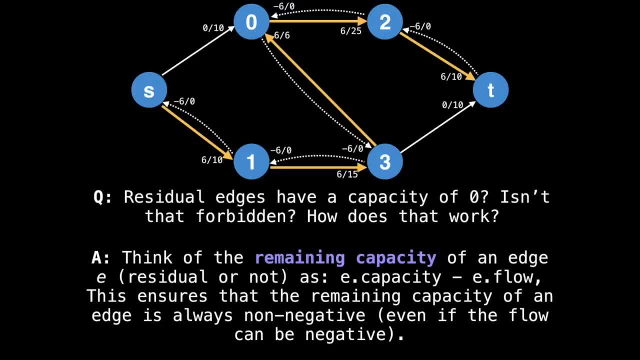 flow of that edge- that is, the difference between the capacity and the flow- is the true remaining capacity for that edge. This ensures that the remaining capacity of an edge is always non negative, even if the flow can be negative, For example in the residual. 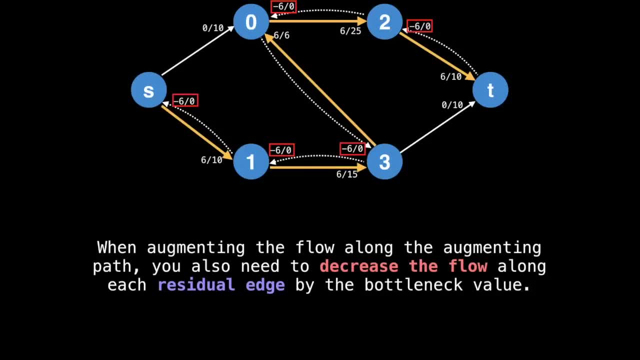 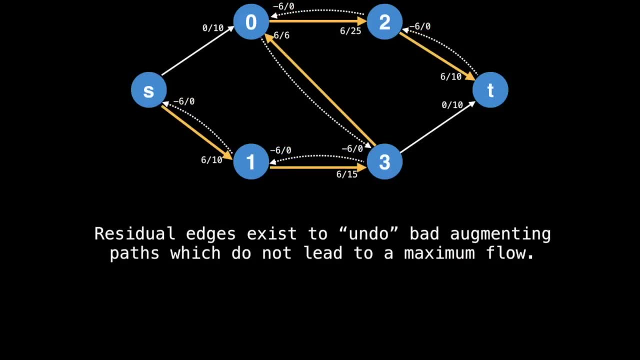 backwards edges, which are called residual edges. The residual edges are the dotted edges going backwards in the reverse order of the augmenting path. The logic behind having residual edges is to undo bad choices of augmenting paths which do not lead to a maximum flow. 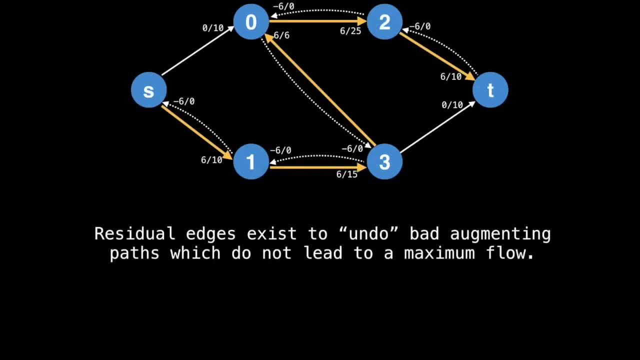 Effectively. we don't know which are the best, or even correct augmenting paths to take, So this mechanism enables us to freely find any augmenting paths without having to worry about whether or not we'll be able to achieve the maximum flow. It should be mentioned that residual edges become valid edges to take when finding an. 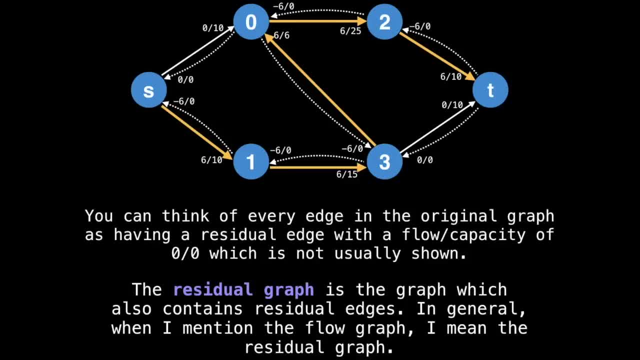 augmenting path in later iterations. So if we take a step back, you can think of every edge in the original graph as having a residual edge with a flow and capacity of zero which is not usually shown. Now that we know what residual edges are, the term residual graph. 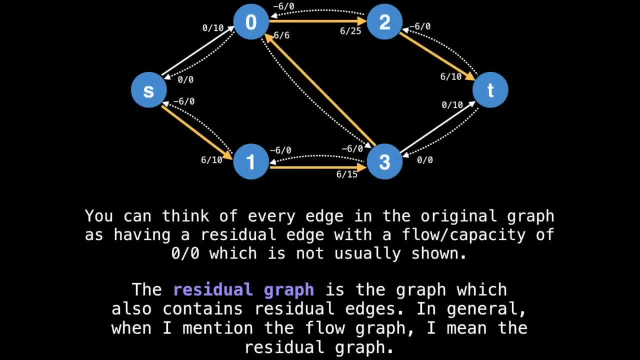 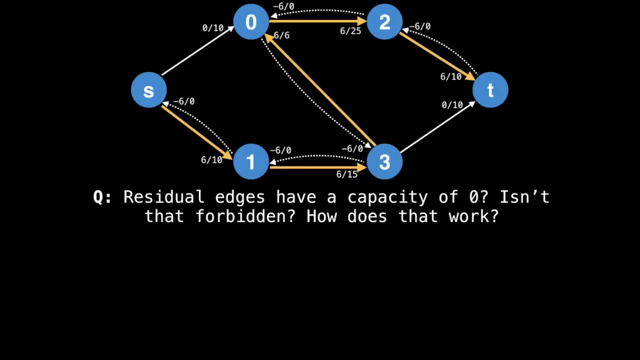 simply means the graph which also contains a residual edge. Residual edges not just the original edges given in the flow graph. So, generally speaking, when I mentioned the flow graph, I usually mean the residual graph. So here's a good question you might have at this point. the residual edges shown have a capacity of zero. 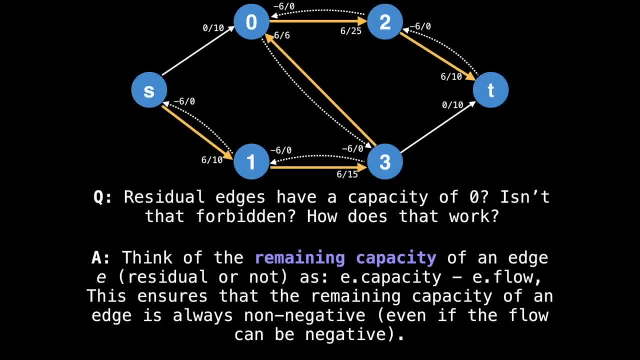 aren't those forbidden? How does that work? So here's the thing: With this method of augmenting the flow, you have to think of the remaining capacity of an edge- E residual or not- as the difference between the capacity and the flow of that edge. That 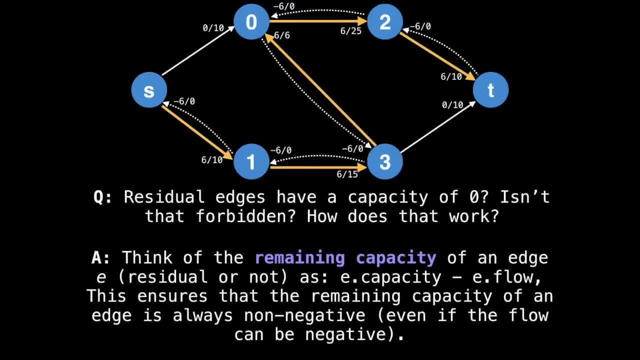 is the difference between the capacity and the flow is the true remaining capacity for that edge. This ensures that the remaining capacity of an edge is always non negative, even if the flow can be negative, For example, in the residual edges we have right now zero. 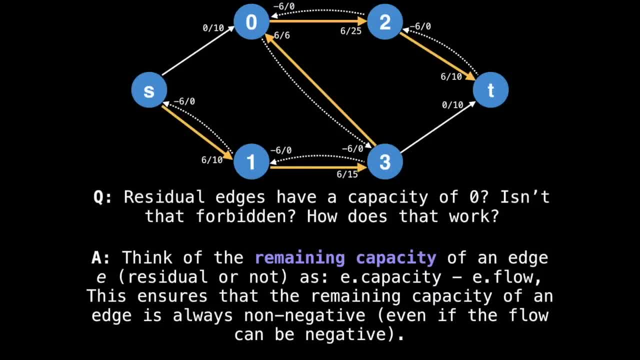 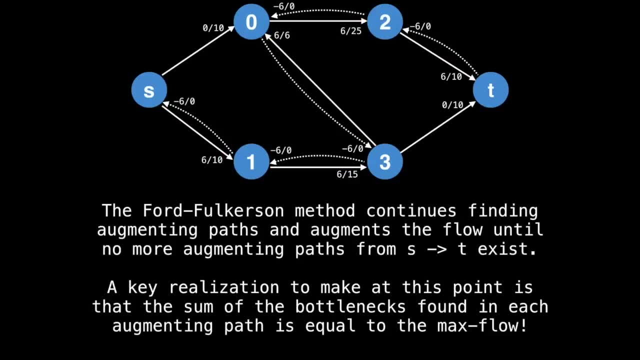 minus minus six is six. So we know that all our residual edges actually have a residual edge: the remaining capacity of six. So the algorithm proceeds and the Ford Fulkerson method continues to repeatedly find augmenting path after augmenting path and to augment. 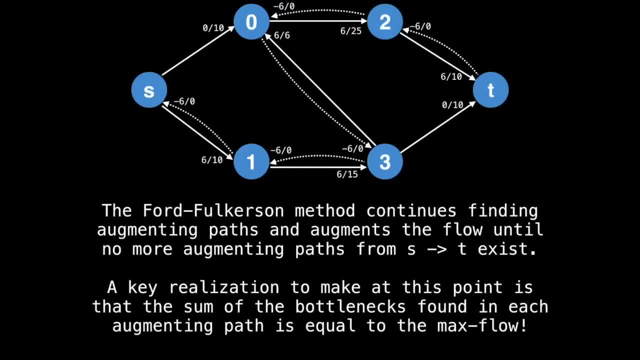 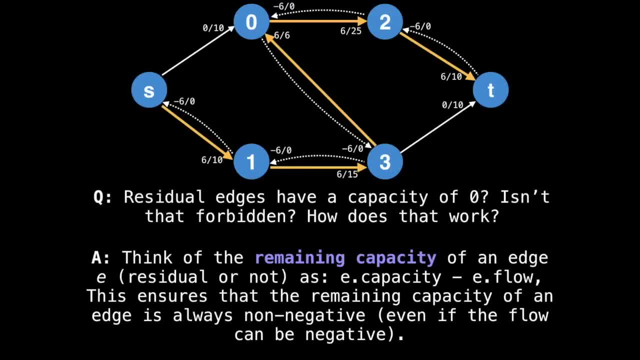 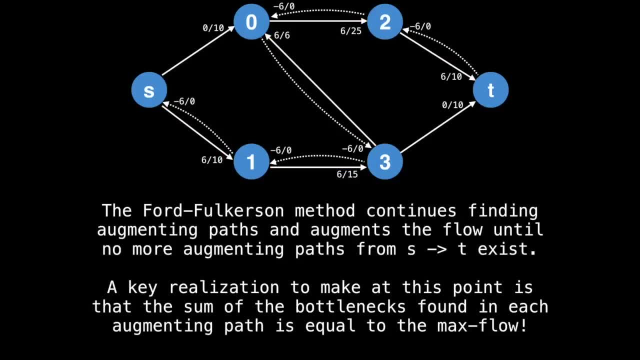 edges we have right now. zero minus minus six is six. So we know that all our residual edges actually have a remaining capacity of six. So the algorithm proceeds and the Ford Fulkerson method continues to repeatedly find augmenting path after augmenting path and to augment. 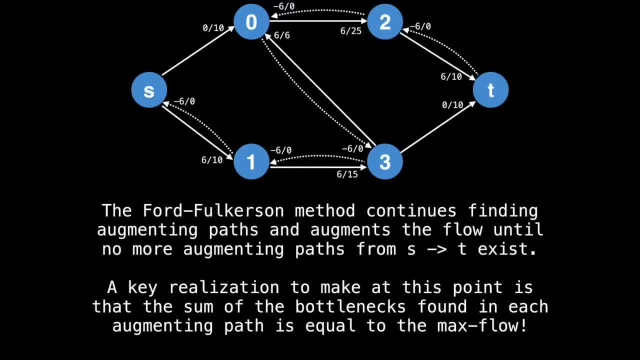 the flow until no more augmenting paths from s to t can be found. The key realization to make at this point is that the sum of the bottleneck values that we acquire with each augmenting paths will result in the maximum flow, And that's the whole premise of this. 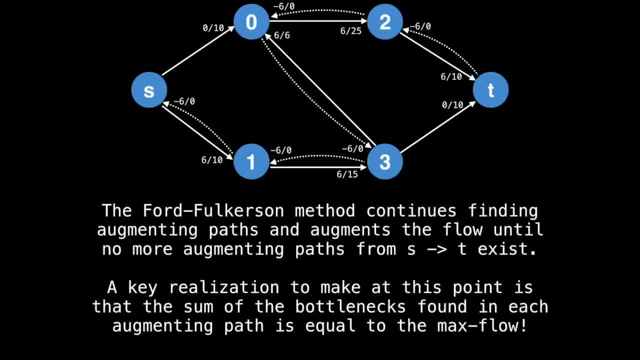 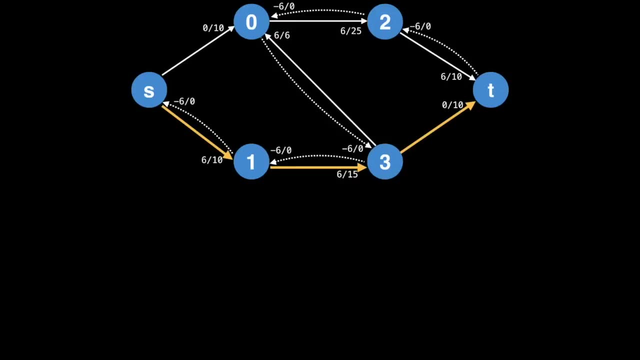 algorithm. It doesn't matter so much how you find augmenting paths, but so long as you keep finding the bottleneck values which they produce, you'll find the maximum flow. So let's keep finding augmenting paths. Remember that we can only select edges whose remaining capacity 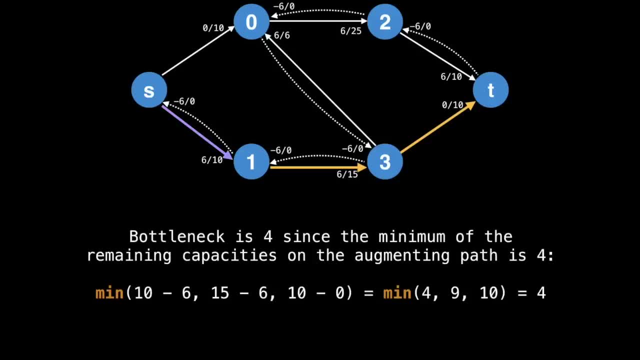 is greater than zero to be part of the augmenting path. So the bottleneck for this augmenting path is four, since four is the minimum of all the remaining capacities along this augmenting path. Here's another augmenting path, from the source to the sink. 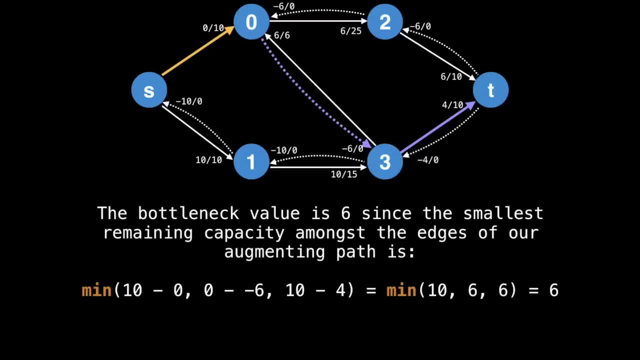 You'll notice that we're actually using one of the residual edges we created earlier in this path. you'll also notice that there are two purple edges in the slide. This is just a coincidence, since both of those edges have the same bottleneck value of six. then we 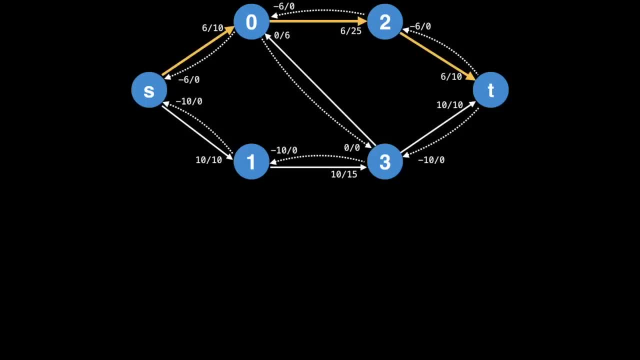 augment the flow as we do. I'll let the animation play for this next one. Okay, so we're going to go ahead and do a search for the augmenting path And at the end we can see that if we sum all our bottleneck values, 646 and four, we're able to achieve. 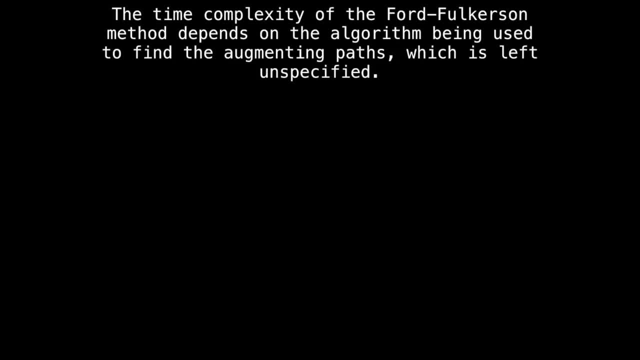 the maximum flow, which is 20.. In terms of the time complexity, the Ford Fulkerson method derives its complexity from how we actually find those augmenting paths which, as we know, is left as an unspecified detail, If you assume that finding augmenting paths are found by 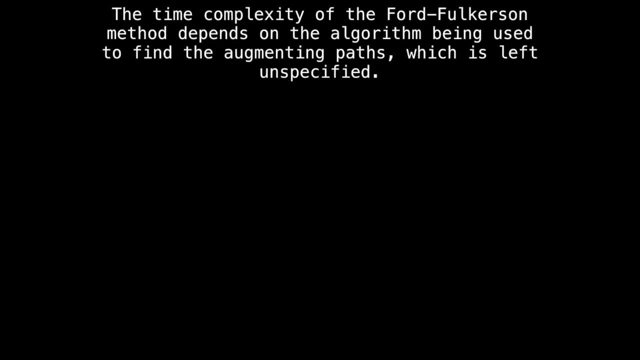 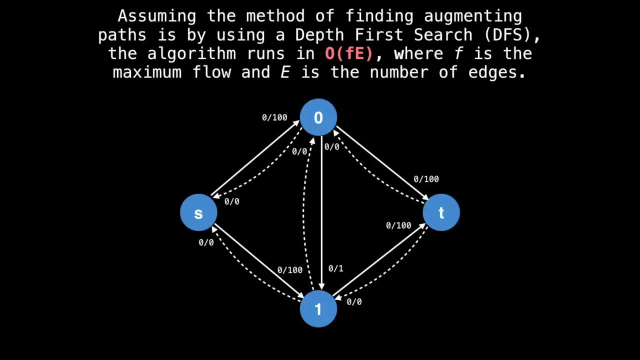 doing a search. then the algorithm runs in a time complexity of a big O of F being the maximum flow times, E the number of edges in the graph. Here's a graph where we can derive the time complexity. suppose that the side edges have very high capacity values of 100.. And the 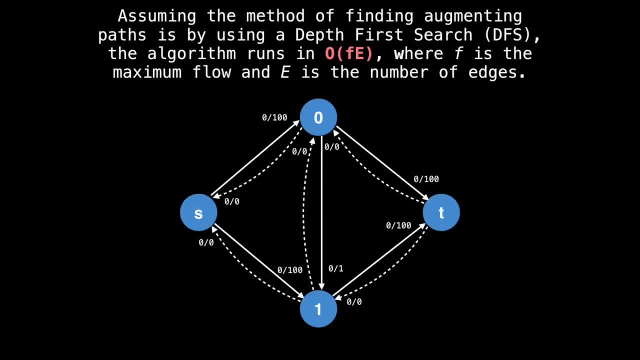 middle edge has a capacity of one, you can clearly tell that the maximum flow should be 200. Because you can run two augmenting paths at the same time. you can run two augmenting paths with flow values of 100 on the top and the bottom of the graph, from the source to. 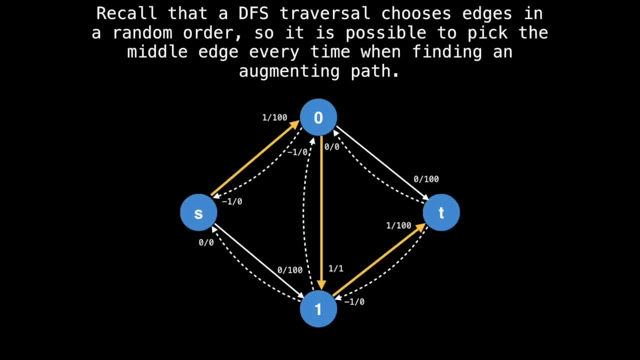 the sink. However, recall that a depth first search traversal is essentially random. So it's possible for you to pick that middle edge with a capacity of one every single time, And what that will do is it'll limit flow. you can push from the source the sink to be. 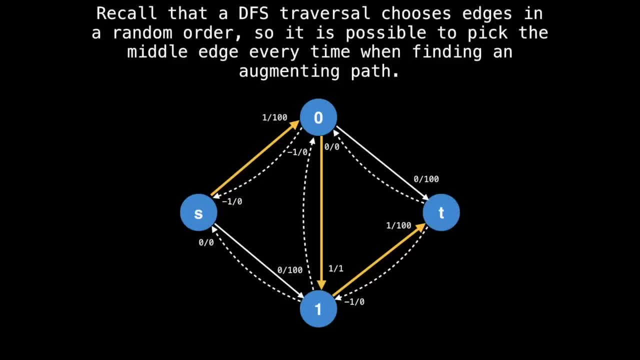 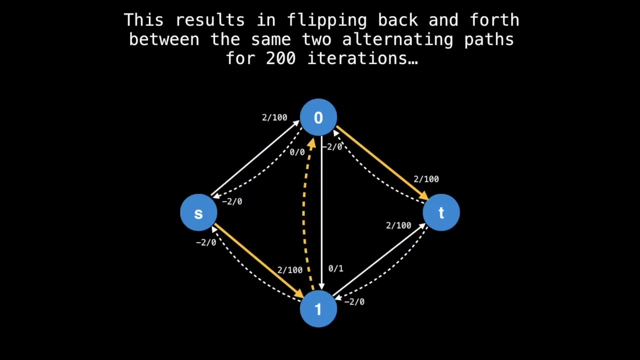 one, So one is always going to be your bottleneck value, So you're never going to be able to augment the flow by more than one unit. This results in flipping back and forth between the same two alternating paths for 200 iterations, which really kills your time- complexity- Luckily, 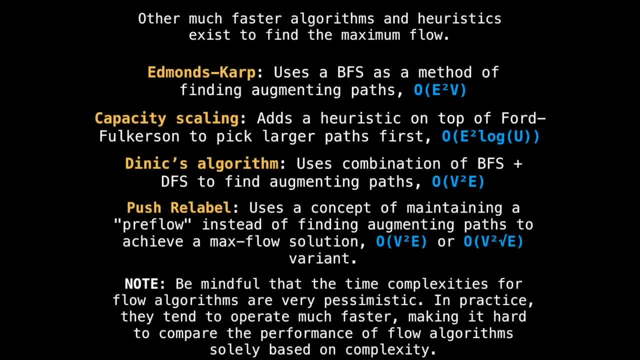 much faster algorithms and better heuristics exist to find the maximum flow value. One example is Edmonds Karp, which is Ford Fulkerson. But instead of using a depth first search, use a breath first search To find the shortest augmenting path from the source to the sink In every iteration. 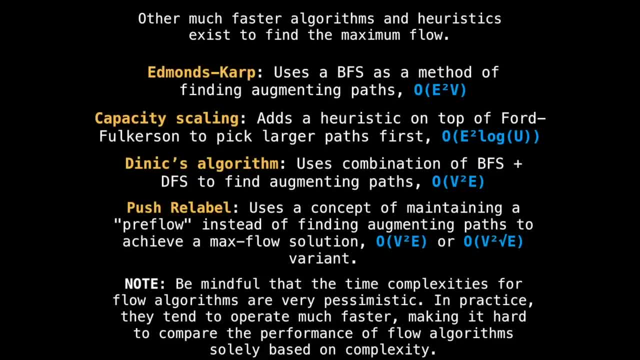 there's also capacity scaling, which is the idea of picking larger paths first to reduce the number of paths you need to find overall, And this turns out to work really well, at least from my empirical tests. then there's Dynix, which uses a combination of a breadth. 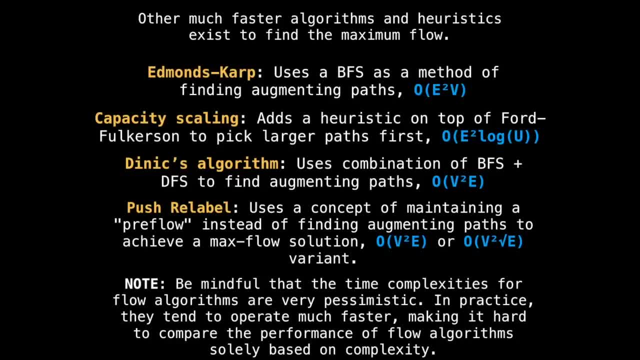 first search to first find a layered graph that guides edges towards the sink, which you then find the shortest augmenting path from the source to the sink. in every iteration There's also capacity scaling, which is the idea of picking larger paths first to reduce. 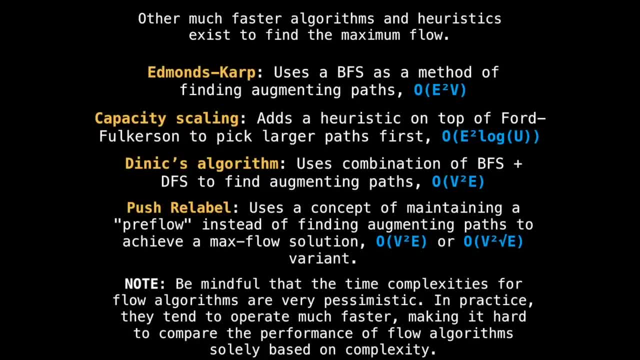 the number of paths you need to find overall And then use a depth first search to actually find the augmenting paths. There's also this idea of push relable algorithms, which work differently than the algorithms we've discussed here, which try and find augmenting paths. 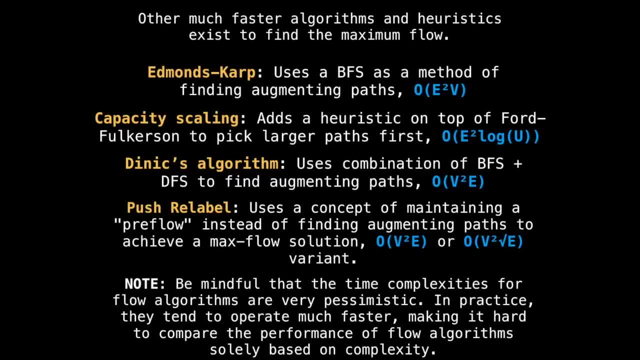 Instead push relable algorithms. maintain this concept of a pre flow, if you will, to find the maximum flow of a network. please be mindful that the time complexities posted here are very pessimistic In practice running maximum flow with any of these algorithms. 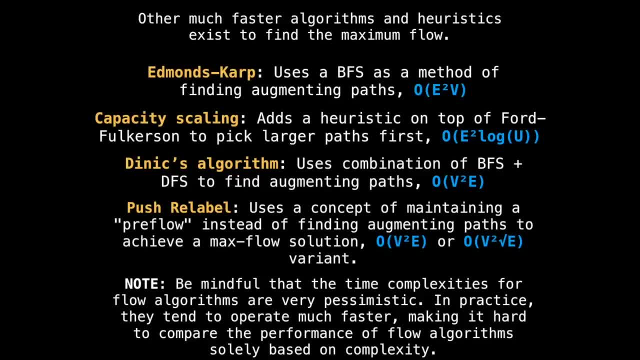 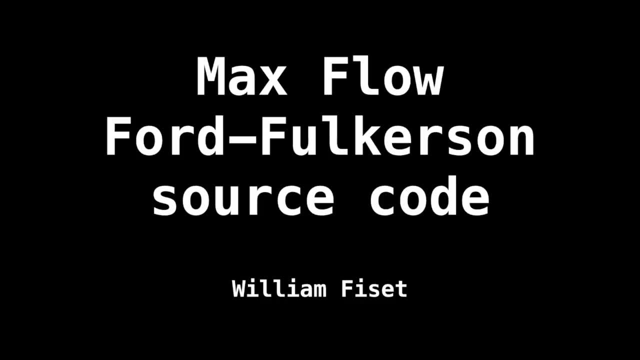 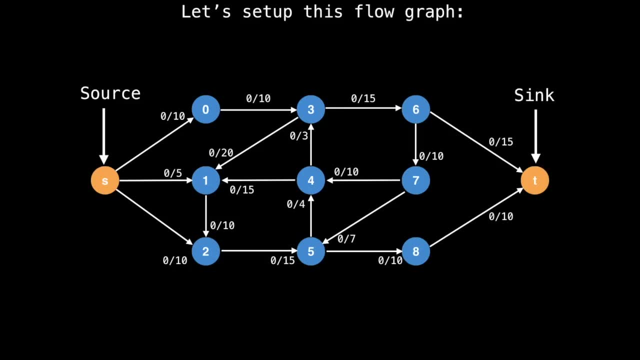 operates much faster. So it's very hard to compare the performance of two flow algorithms solely based on the complexity. Today we're taking a look at the source code for the Ford Fulkerson method implemented with a depth first search. The goal of this video is to 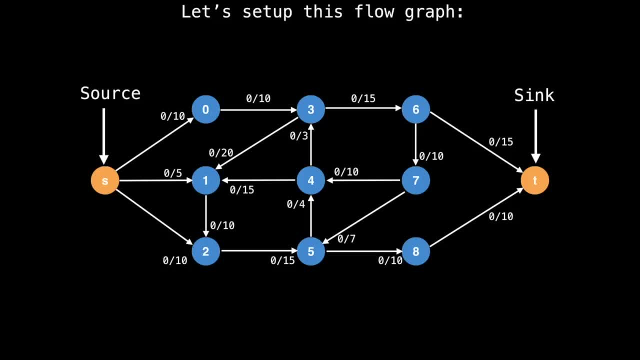 show you how to set up the following flow graph and find the maximum flow through it. So after we run the maximum flow algorithm, we should get a graph similar to this one, with flow running through some, but not all of the edges and achieving the maximum flow. 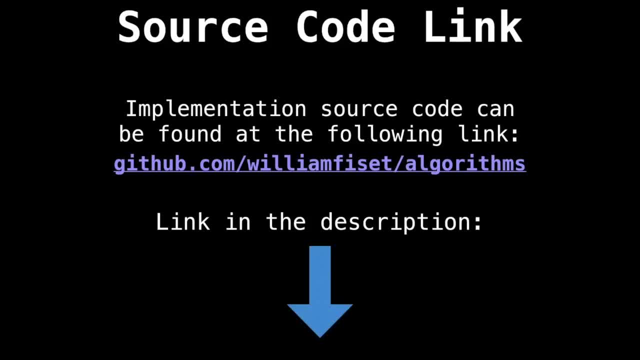 of 23.. The source code and the example I have lined up for you today can both be found on GitHub. There's a link in the description for today. I encourage you to check that out and also play along, as we're going over the source code. Alright, here we are in the source. 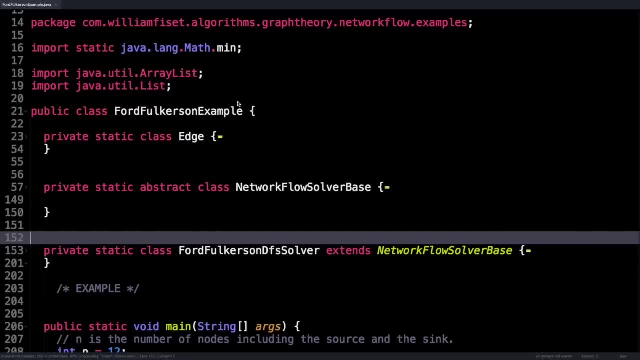 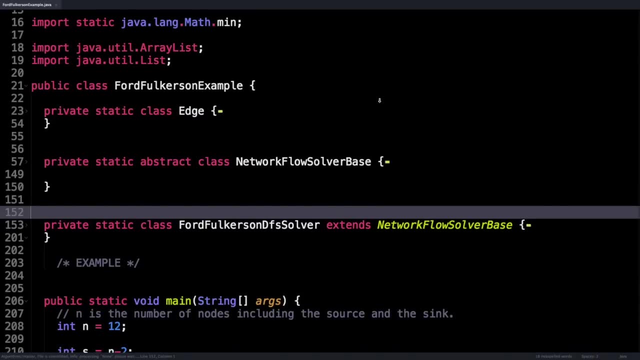 code written in Java. This program has three main supporting classes: an edge class, a network flow solver base and the Ford Fulkerson depth first search solver. However, before we get into any of those, I want to take a look at the main method where I actually use the classes. 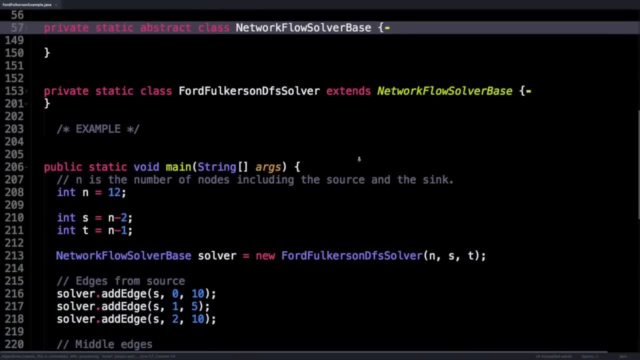 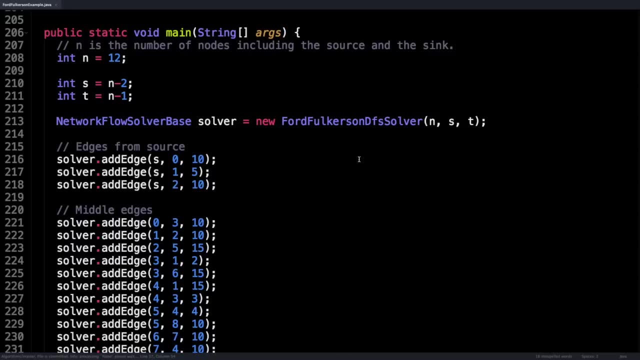 above to solve the flow problem we just saw. I know a lot of people struggle setting up the flow graph, which is usually somewhat of a mystery, So I want to clear that up. The first thing I recommend you do every time you set up a flow problem is initialize three. 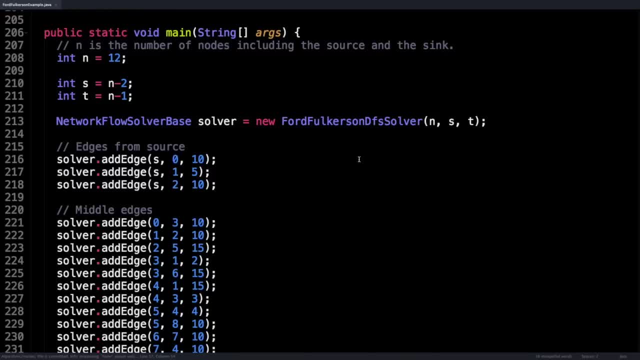 variables. One is n, the number of nodes in your graph. that is including the source and the sink nodes. And then what I recommend you do is you actually label the source in the sink nodes and assign them indices. And what I usually end up doing is I say the source. 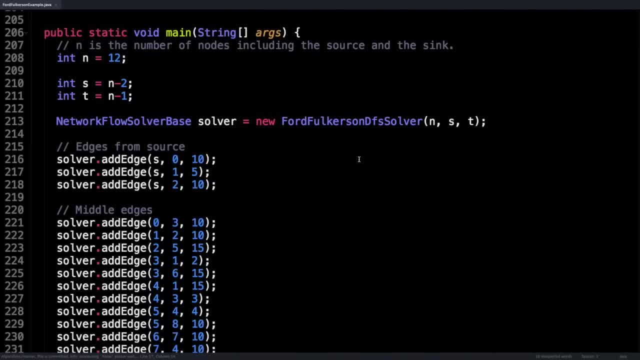 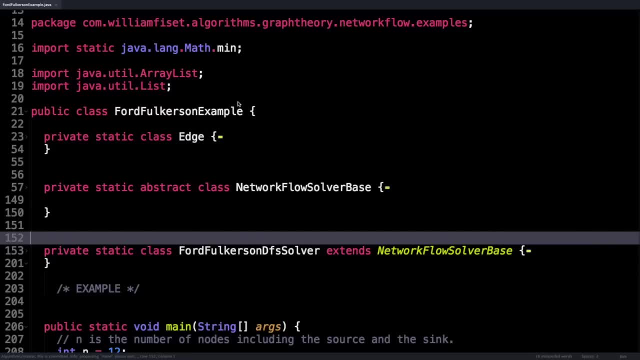 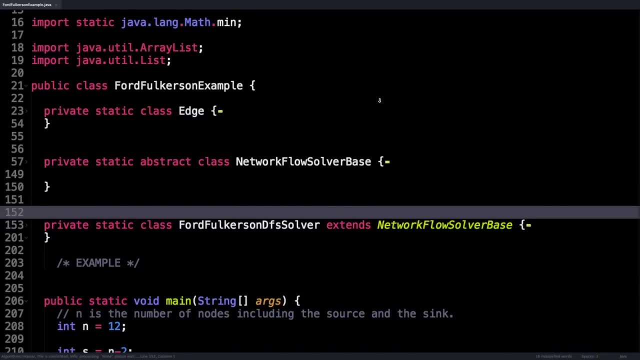 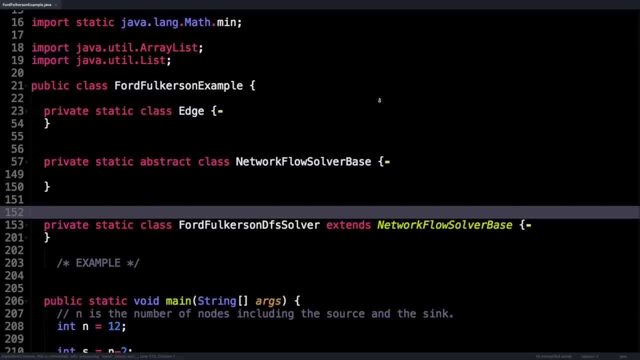 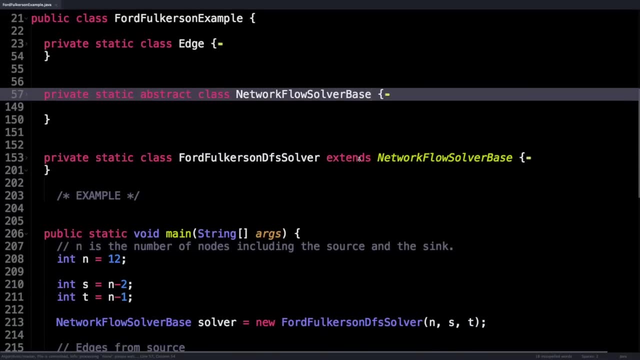 first search solver. However, before we get into any of those, I want to take a look at the main method where I actually use the classes above to solve the flow problem we just saw. I know a lot of people struggle setting up the flow graph, which is usually somewhat 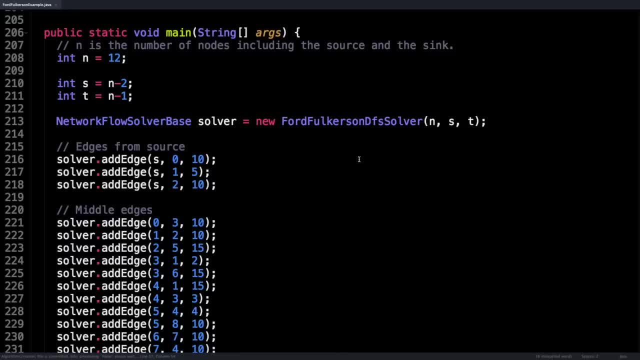 of a mystery, So I want to clear that up. The first thing I recommend you do every time you set up a flow problem is initialize three variables And the number of nodes in your graph- that is, including the source and the sync nodes- And then what I recommend you. 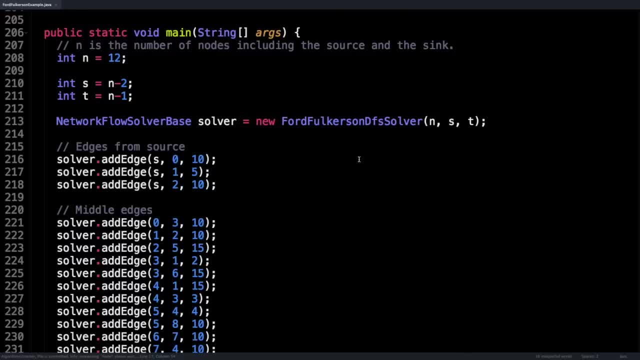 do is you actually label the source and the sync nodes and assign them indices. And what I usually end up doing is I say the source node equals, equals index n minus one and the sink equals n minus two. the rest of the nodes in your 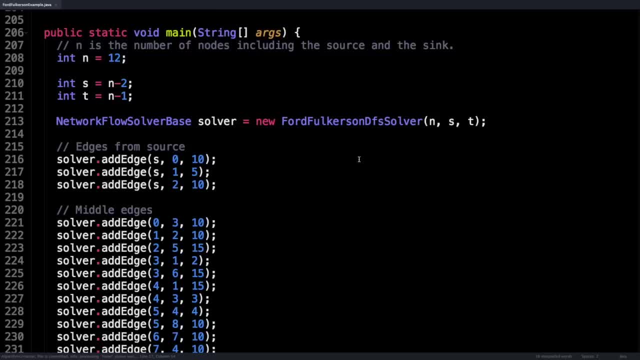 graph should then have indices between zero and n minus three inclusive. I've always found this to be the easiest way to set up your flow graph. Next, I create the flow solver by providing the three variables n, s and t as inputs to the solver, So it knows how. 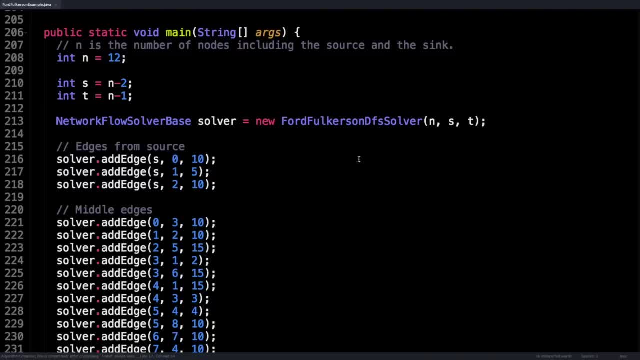 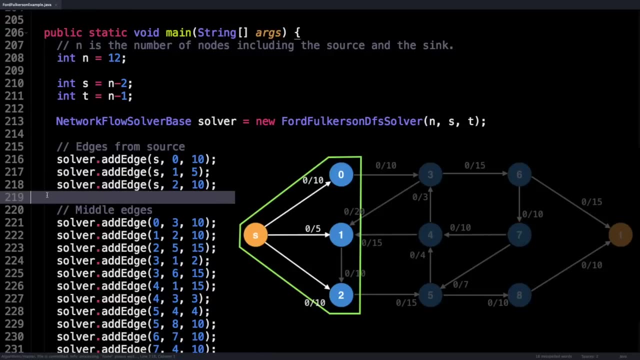 many nodes there are and which nodes are labeled- the source and the sink. Then I use the solver to actually create the flow graph by adding edges with different capacities. The next step is to hook up the edges to the source. Those would be the ones shown in this picture. 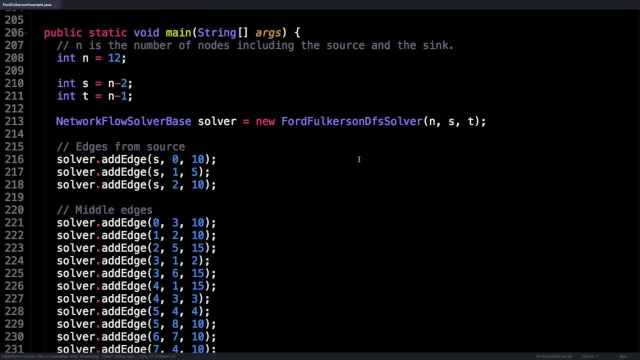 with the rest of the nodes in your graph. First, I'm going to set the index to zero and the. I've always found this to be the easiest way to set up your flow graph. Next, I create the flow solver by providing the three variables n, s and t as inputs to the solver. So it knows. 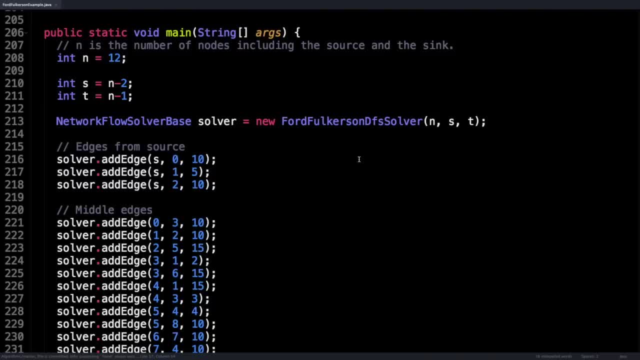 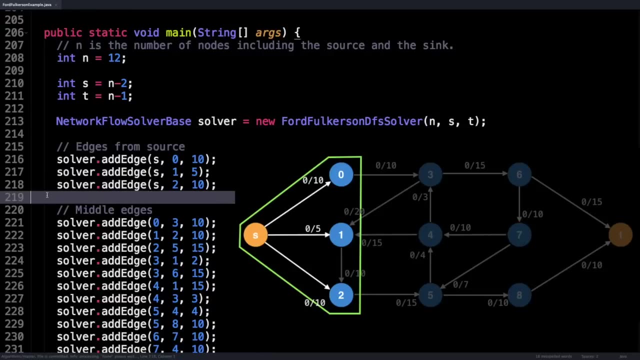 how many nodes there are and which nodes are labeled: the source and the sink. Then I use the solver to actually create the flow graph by adding edges with different capacities. The next step is to hook up the edges to the source. Those would be the ones shown in the 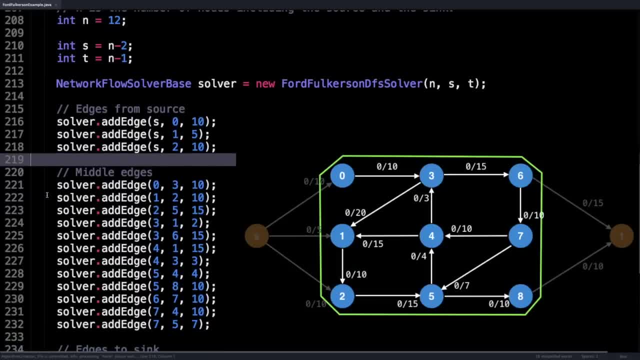 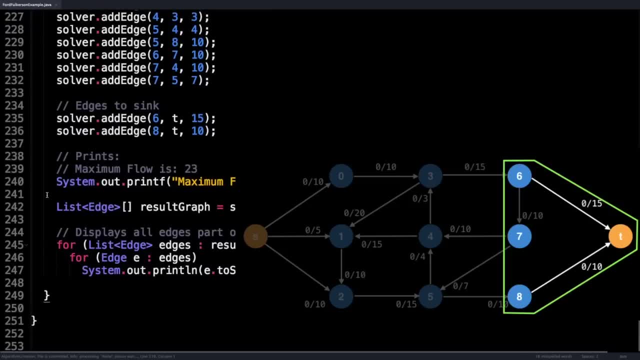 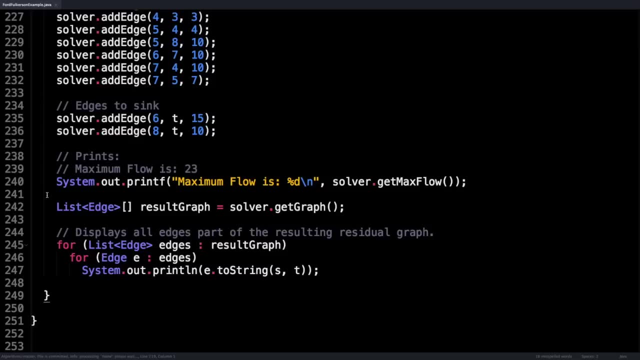 picture. Then I carefully hook up all the middle edges And lastly, the edges leading into the sink. It's usually always these three steps And for most of the time your graph is bipartite, So the middle edges are even simpler to set up. After this, I call the. 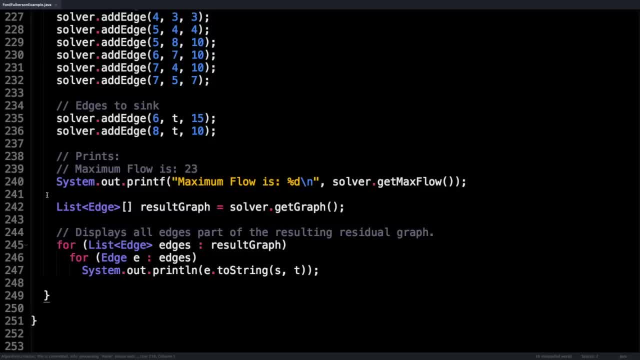 get max flow method on the solver which actually runs the Ford Fulkerson max flow depth first. search Then returns an integer value for this graph. we're expecting a max of 23.. Followed by printing the max flow. I also display all the interesting edges of the residual graph. First I get 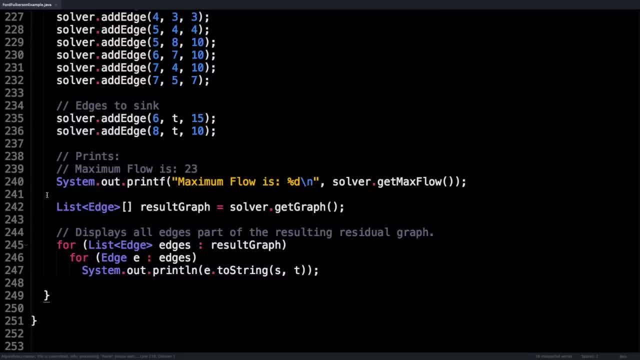 the residual graph from the solver after executing the max flow and iterate over all the edges and just display the flow on each edge. Let's actually run this program and see what the output looks like. So I just popped open a terminal And for those of you who also have, a terminal open and want to run this program, you can do that by clicking on the top right corner. So I'm going to use my back end right now, but since we're just going to run this program, I'll just hit the etc button. Once you click on the wrong button, your file will. 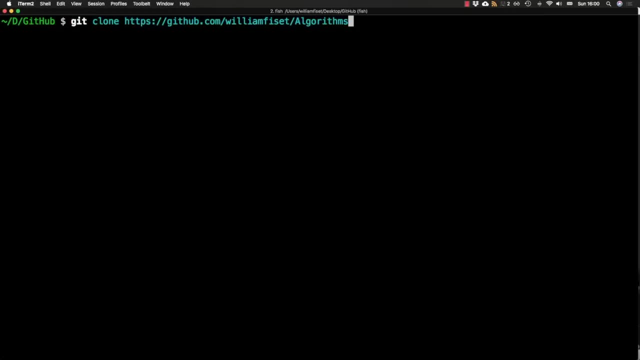 go to the left of the system. you'll see like this: I'll justneo at the right left corner to the left, and then the Alt key And I'll right click on the button. Now you can see that the file will go to the left of the system, because I already did the math on the right side. And if you click on that, you'll see that it's going to go to the left of the system, And once you click on the right side, you'll see a new folder that's called the Incident Example dot Java file And it's in the graph that I just created. it's going to be using. 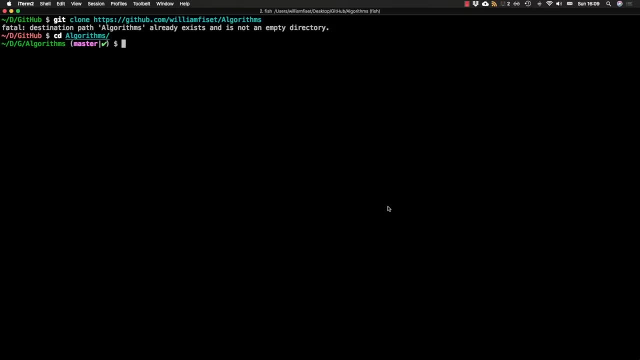 an argument for the example dot Java file. and it is in the proper authentic file folder file And it's in the graph theory network flow examples package. And luckily for us it doesn't have any dependencies yet So we can just compile it on its own with Javac. 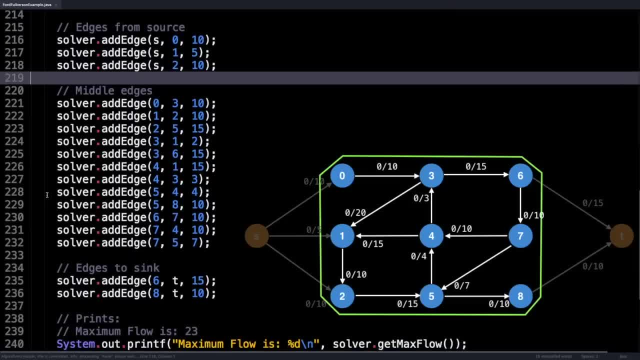 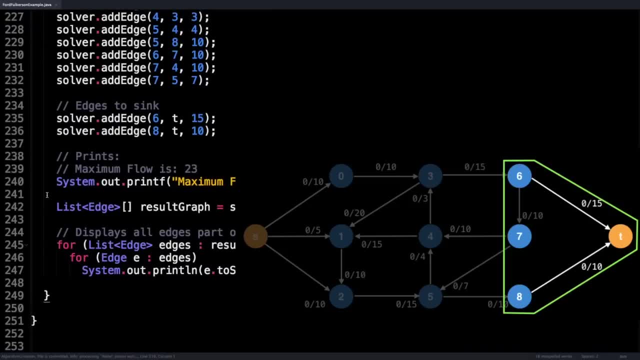 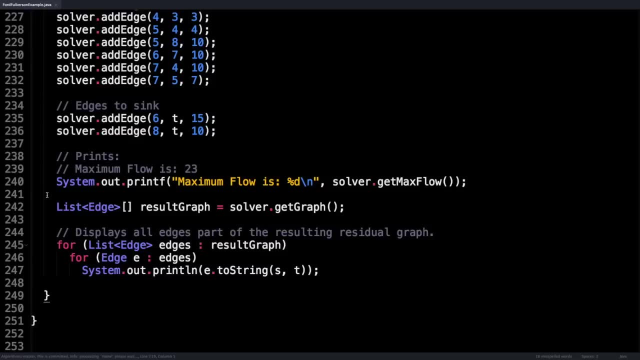 Then I carefully hook up all the middle edges And lastly, the edges leading into the sink. Okay, it's usually always these three steps And for most of the time your graph is bipartite, So the middle edges are even simpler to set up. After this, I call the get max flow method. 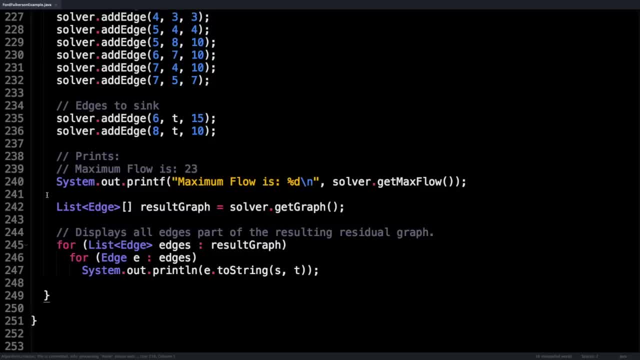 on the solver which actually runs the Ford Fulkerson max flow depth first search and returns an integer value for this graph. we're expecting a max of 23, followed by printing the max flow. I also display all the interesting edges of the residual graph. 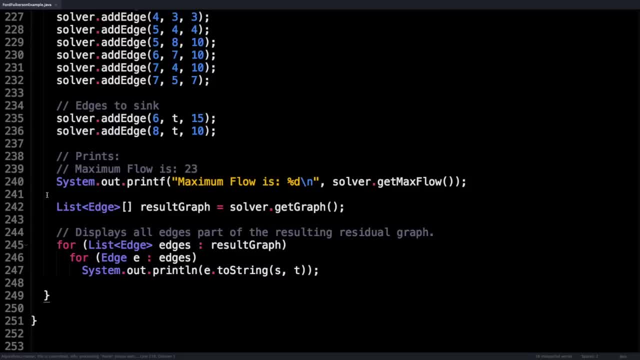 First I get the residual graph from the solver after executing the max flow and iterate over all the edges and just display the flow on each edge. Let's actually run this program and see what the output looks like. So I just popped open a terminal And, for those of you, 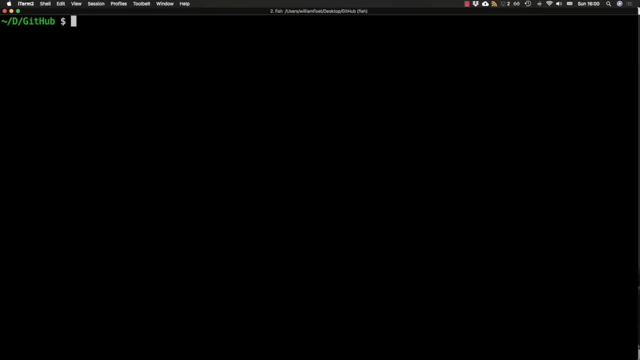 who also have a terminal open and want to play along. First, you can just clone the GitHub repo by typing git clone, followed by the repo URL, which is githubcom slash William Fuse, And then just change algorithms. you see that I've already cloned the repo, so I don't need 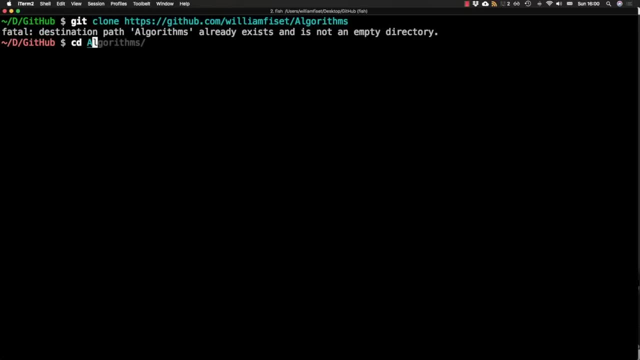 to do it again, then just change directory into the algorithms folder. So the file we're working with is called the Ford Fulkerson example dot Java file And it's in the graph theory network flow examples package And luckily for us, it doesn't have any dependencies. 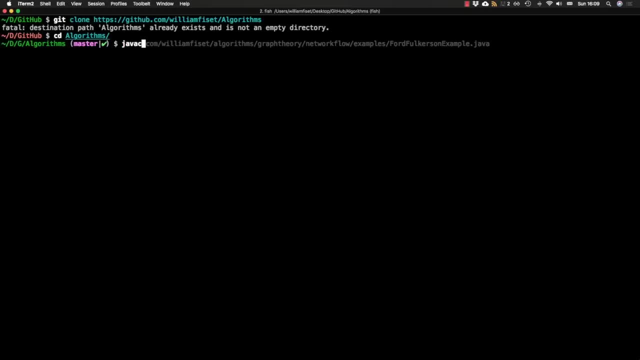 yet. So we can just compile it on its own with Javac. So if you type Java C, followed by from Williams algorithms, graph theory, network flow, examples, and then you find that file Ford Fulkerson example, dot Java, you compile it, it'll produce a dot class file. 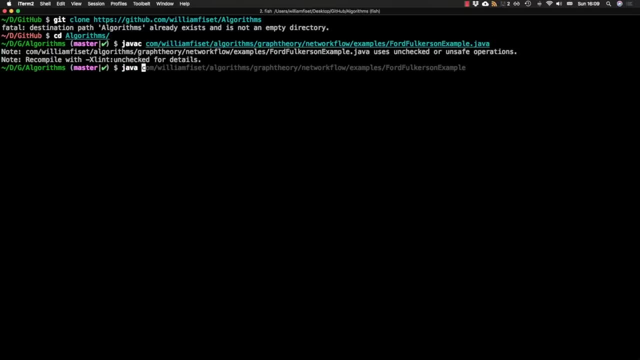 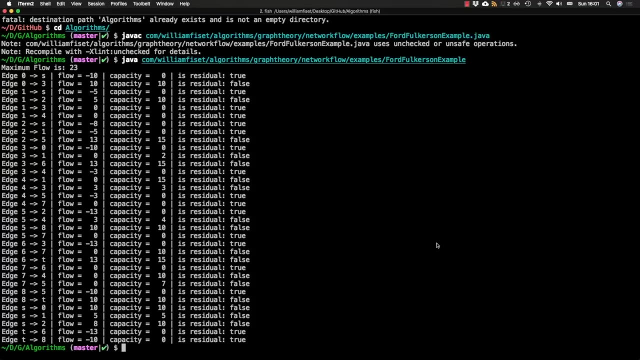 in that directory. So you can execute it by typing Java and then the name of the class and then pressing Enter, and then you get this beautiful output. So this prints a lot of interesting information. Notably it prints the max flow of 23 and all of the edges plus. 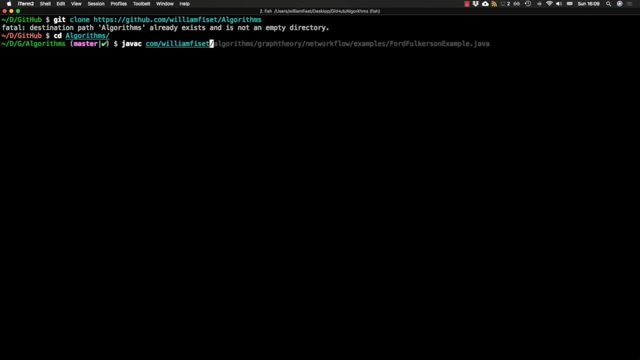 So if you type Java C, followed by calm Williams algorithms, graph theory, network flow examples, and then you find that file for Fulkerson example, dot Java, you compile it. it'll produce a dot class file in that directory So you can execute it by typing Java and then the 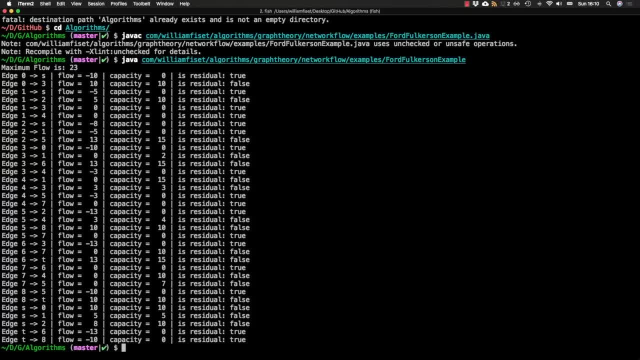 name of the class and then pressing Enter and then you get this beautiful output. So this prints a lot of interesting information. Notably it prints the max flow of 23. And all of the edges plus four columns. The first column represents the start and end nodes. 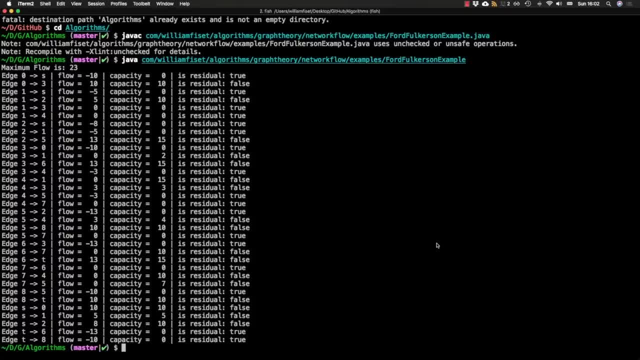 of the directed edge, then the amount of flow running through the edge, the capacity of the edge And, lastly, a Boolean value indicating whether the edge is a residual edge or not, Which is quite handy for debugging. So let's go back to the code. So let's scroll back. 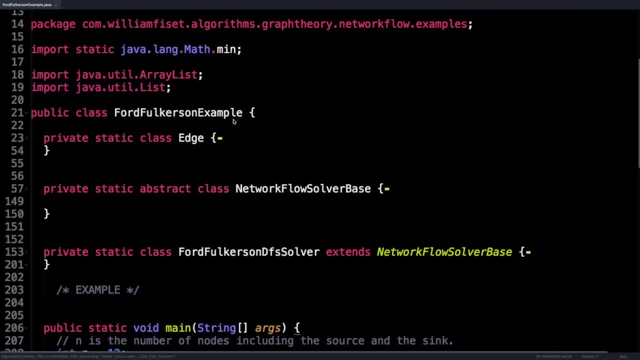 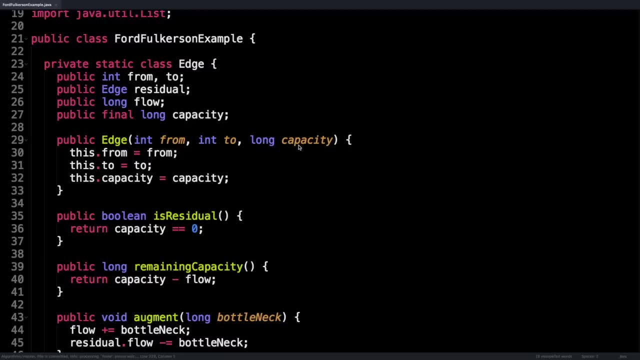 up the code and take a look at the first of the three classes, which is the edge class. The edge class is composed of a few instance variables. In particular, every edge has a start node called from and an end node called to. each edge in the flow graph has a certain 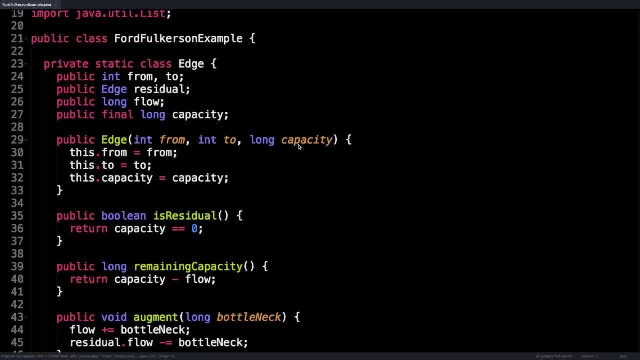 amount of flow and capacity. The capacity of the edge is a certain amount of flow and capacity. The capacity of the edge is constant and does not change. The flow is dynamic and adjusts as we augment the flow. When you create a new edge, it should have a start and an end node plus an initial. 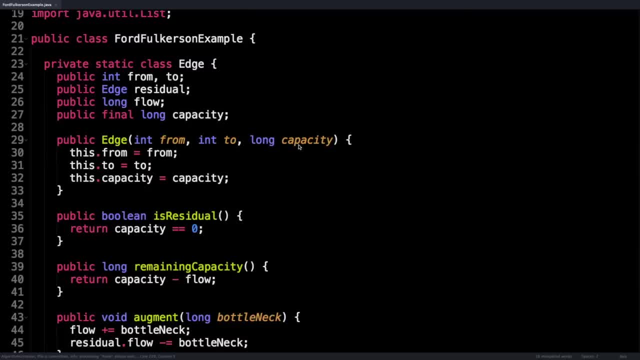 capacity, the flow defaults to zero. you might notice that the residual edge instance variable does not get initialized here or through the constructor. The reason is that I initialize the residual edge together with the forward edge and hook them up together in a helper method. 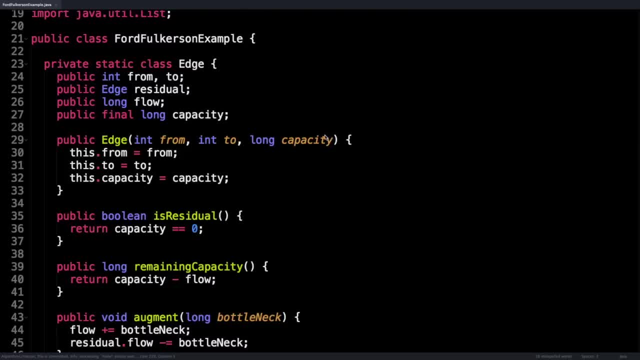 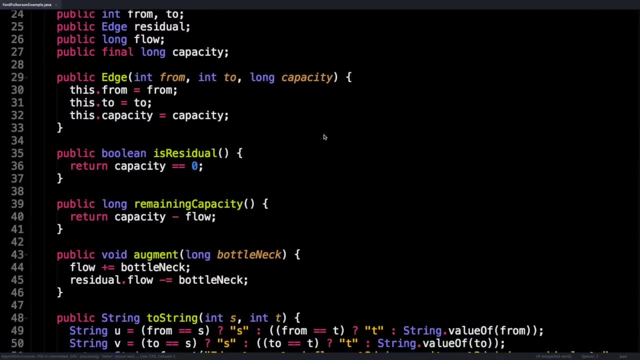 Which we'll see later. The next method is the is residual method, which determines whether an edge is a residual edge or not, because forward edges are not permitted to have a capacity of zero. you know, an edge is residual if the capacity is zero. pretty. 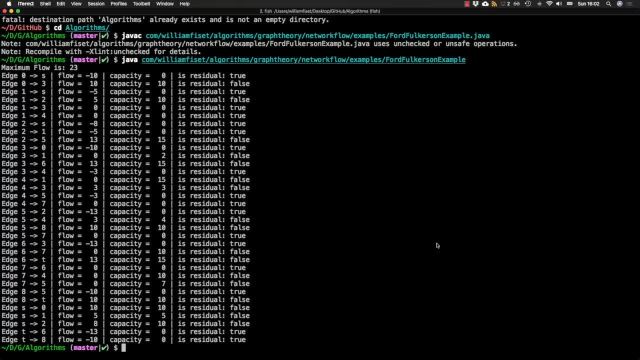 four columns. The first column represents the start and end nodes of the directed edge, then the amount of flow running through the edge, the capacity of the edge and lastly, a Boolean value indicating whether the edge is a residual edge or not, which is quite handy for debugging. So let's 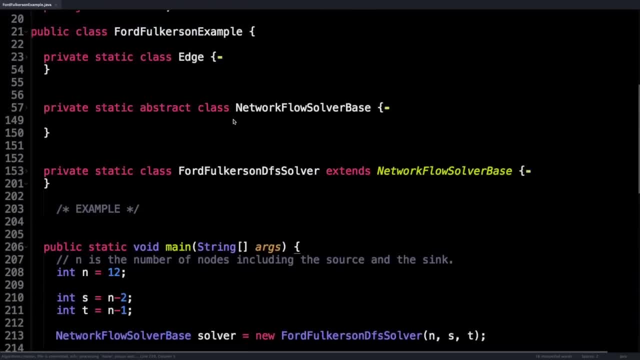 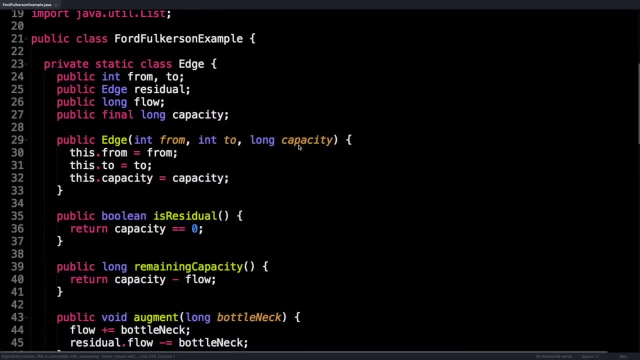 go back to the code. So let's scroll back up the code and take a look at the first of the three classes, which is the edge class. The edge class is composed of a few instances, variables. In particular, every edge has a start node called from and an end node called. 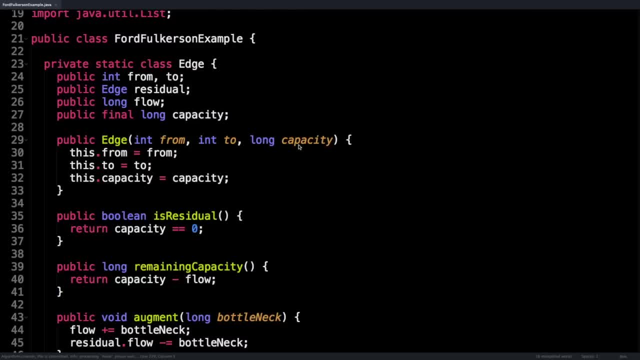 to each edge in the flow graph has a certain amount of flow and capacity. the capacity of the edge is constant and does not change. the flow is dynamic and adjusts as we augment the flow. When you create a new edge, it should have a start and an end node plus an initial. 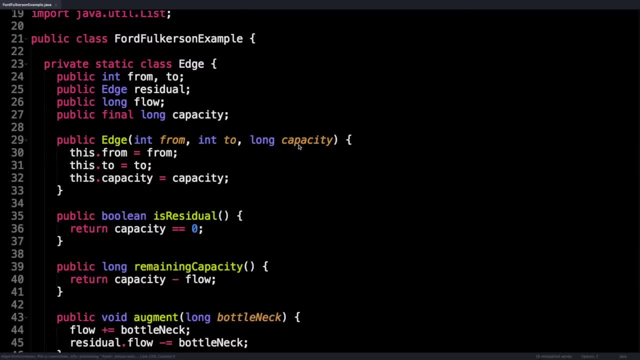 capacity, the flow defaults to zero. You might notice that the residual edge instance variable does not get initialized here or through the constructor. The reason is that I initialize the residual edge together with the forward edge and hook them up together in a helper method which we'll see later. 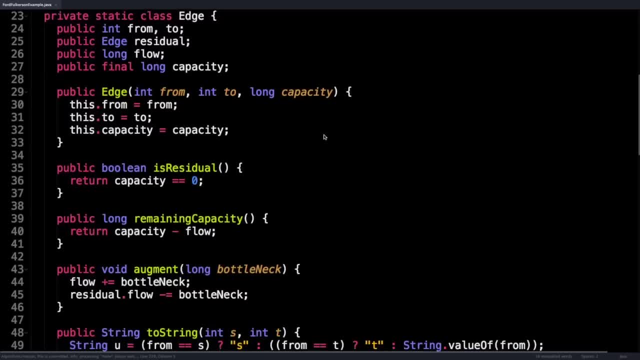 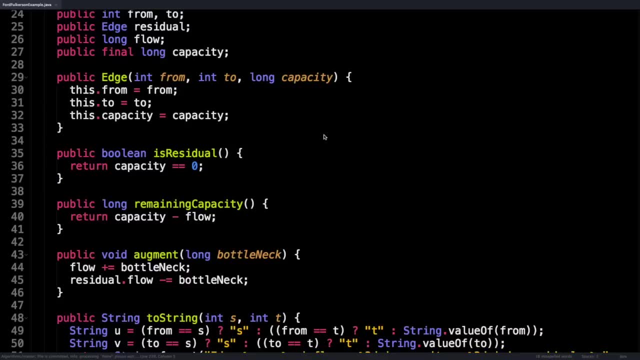 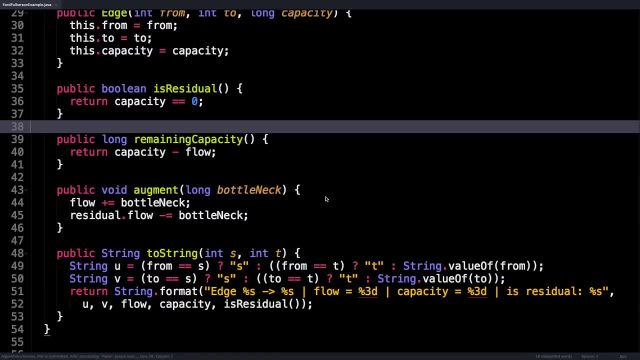 The next method is the is residual method, which determines whether an edge is a residual edge or not, Because forward edges are not permitted to have a capacity of zero. you know, an edge is residual if the capacity is zero, pretty easy. There's also the remaining capacity method. 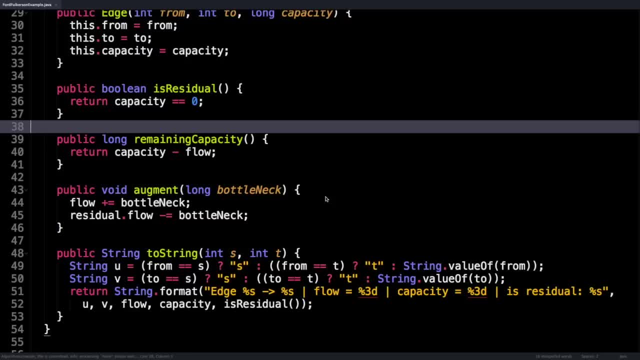 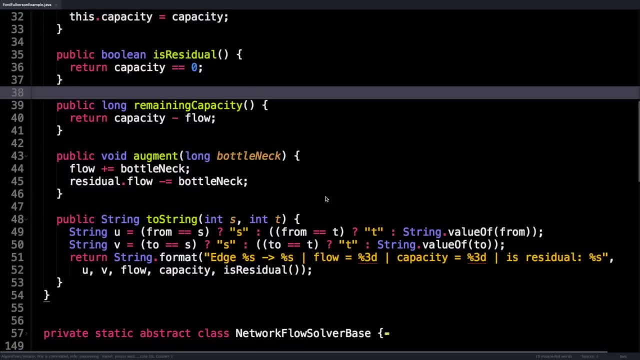 which can be used to determine the maximum amount of flow that we can push through this edge. This method works whether the flow is positive or negative. Next is the augment method, which augments the flow for this edge alone. all it does is it increases the flow. 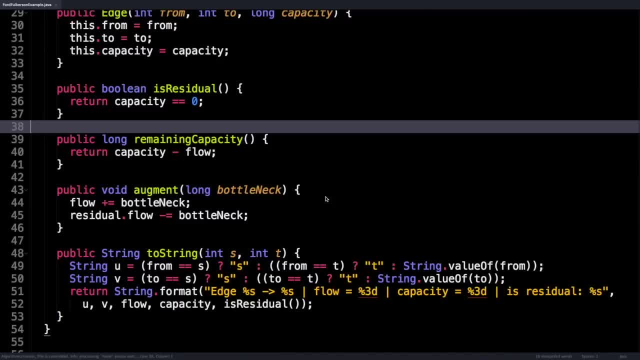 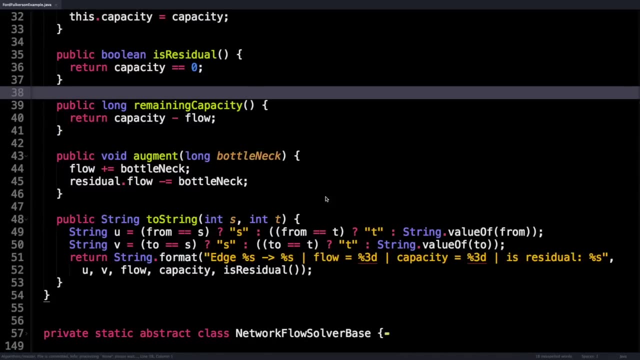 easy. There's also the remaining capacity method, which can be used to determine the maximum amount of flow that we can push through this edge. This method works whether the flow is positive or negative. Next is the augment method, which augments the flow. for this edge alone, all it does. 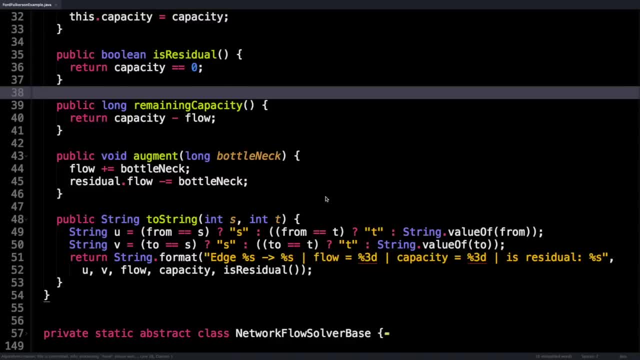 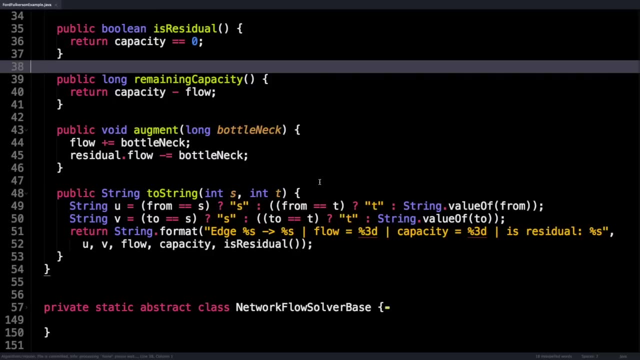 is. it increases the flow on the forward edge by the bottleneck value we found along the augmenting path And it also decreases the flow along the residual edge. Last is the to string method, which is responsible for displaying those nice columns we saw in the. 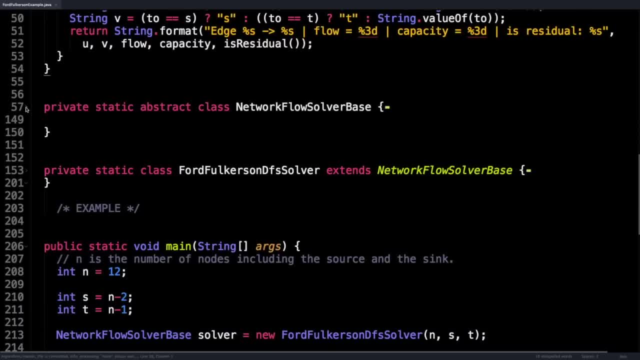 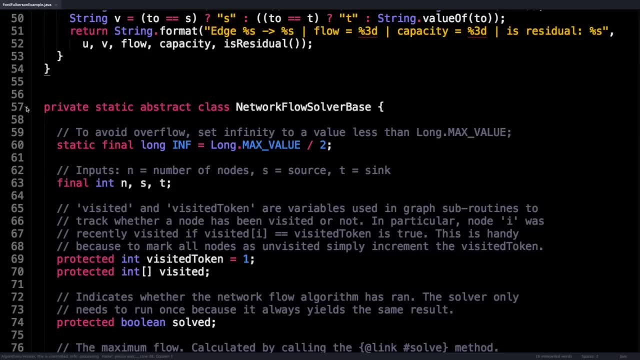 terminal. The next class we're going to take a look at is the terminal class. This class is a generic base for max flow solvers, which all solvers should extend to gain access to reused variables and setup methods and so on. For example, a simple task like adding: 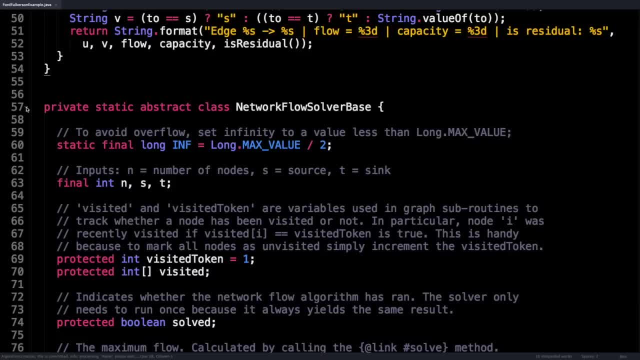 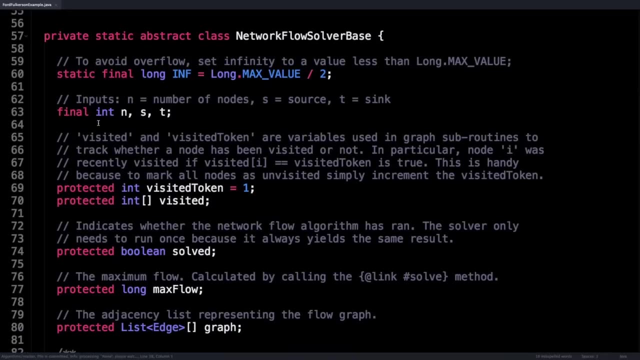 an edge to a flow graph should be the same. whether the max flow algorithm is Edmonds Karp didn't x some capacity scaling algorithm, it shouldn't matter. Therefore, it makes sense to abstract. So we're going to connect that behavior and capture it in a base class. So there are many. 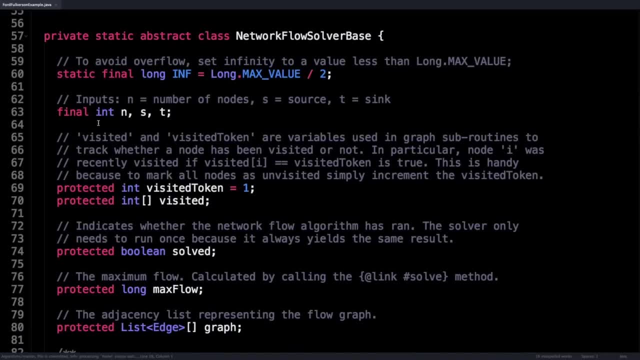 variables in this class. The first one is, in short, for infinity, which is just a handy large constant that doesn't overflow if you add numbers to it, or at least it can handle having large numbers added to it. Then there are the three input variables and the number. 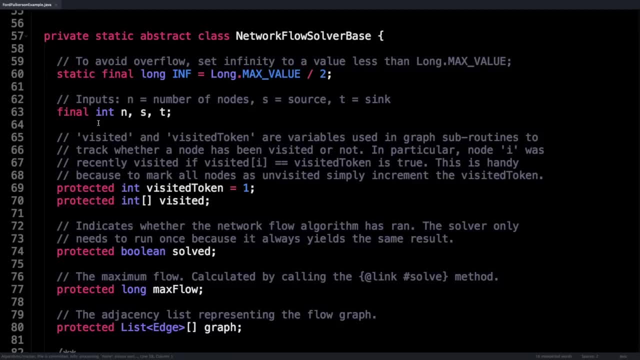 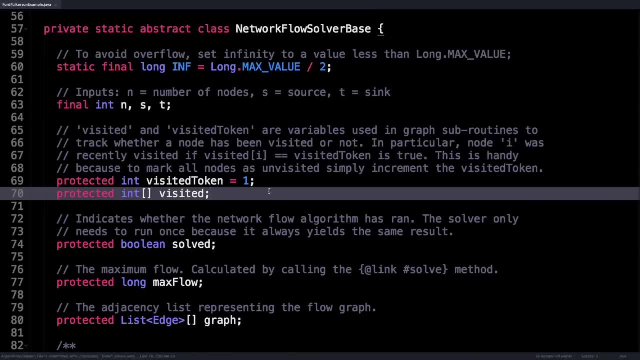 of nodes in the graph s, the index of the source node and T the index of the sink, followed by this. And then there are two special variables I usually end up using because they greatly help boost performance. So the rationale behind using the visited token and combination with 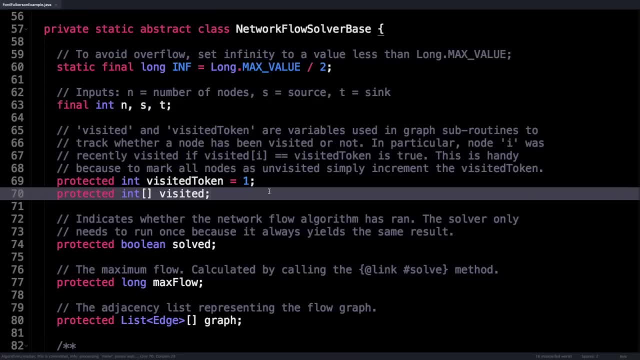 an integer array that tracks the visited state of a node is that when we're finding augmenting paths, whether via depth first search or breadth first search or whatever graph traversal method you want to use- you generally want to ensure that your augmenting path does. 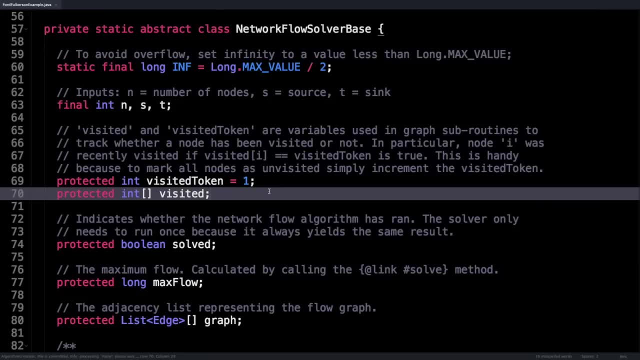 not visit the same node twice. Otherwise that could result in a cycle which we don't want. The way to check if node i is visited is to check if the state in the visited array at index i is equal to the visited token. This is super handy because in the next iteration 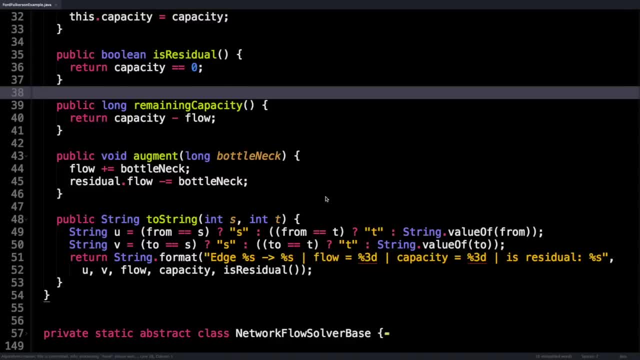 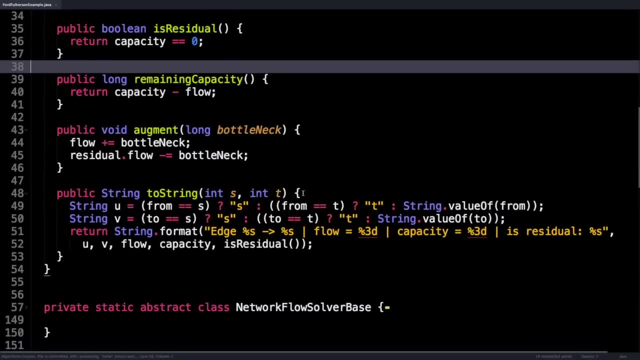 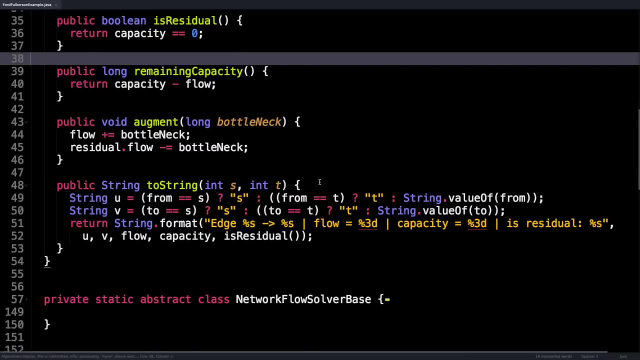 on the forward edge by the bottleneck value we found along the augmenting path, And it also decreases the flow along the residual edge. Last is the two string method, which is responsible for displaying those nice columns we saw in the terminal. The next class we're. 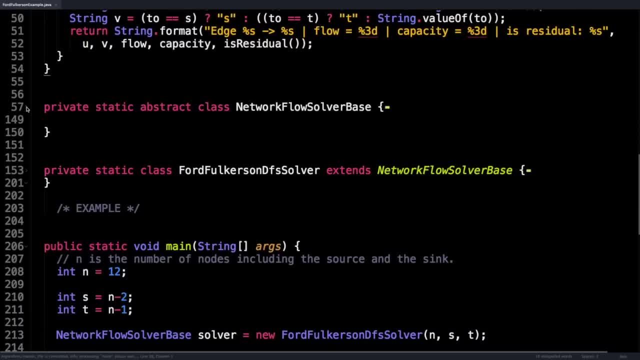 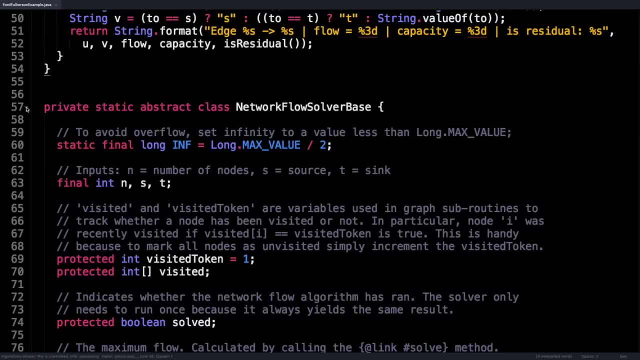 going to take a look at is the network flow solver base. This class is a generic base for max flow solvers, which all solvers should extend to gain access to reused variables and setup methods and so on. For example, a simple task like adding an edge to a flow graph should be the same whether the max flow 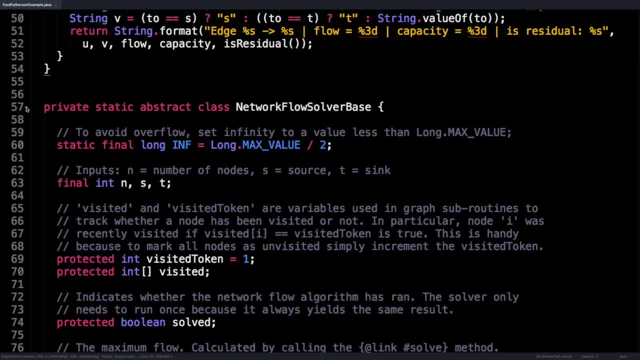 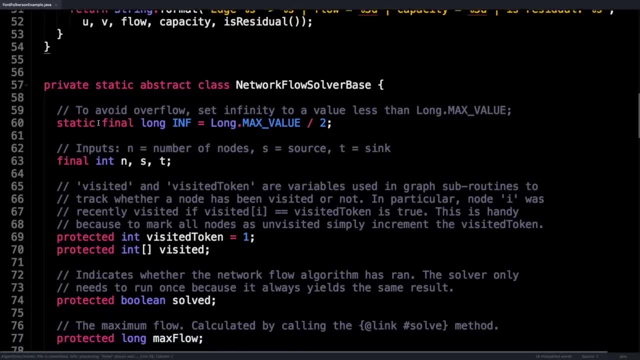 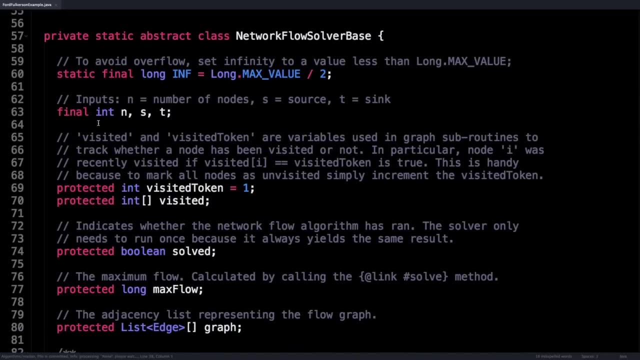 algorithm is Edmonds Karp didn't x some capacity scaling algorithm? it shouldn't matter. Therefore, it makes sense to abstract that behavior and capture it in a base class. So there are many variables in this class. The first one is, in short, for infinity, which is just a handy. 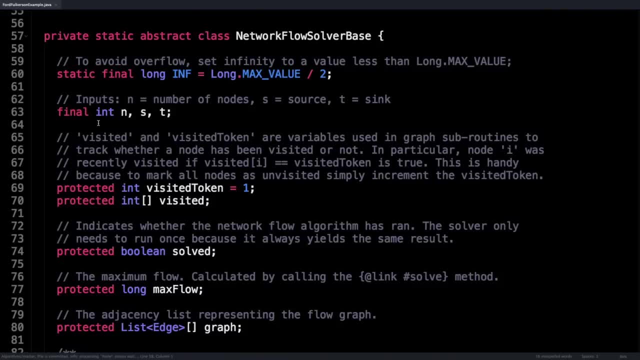 large constant that doesn't overflow If you add numbers to it, or at least it can handle having large numbers added to it. then there are the three input variables and the number of nodes in the graph s, the index of the source node, and T, the index of the sink. followed by this, are two special variables. 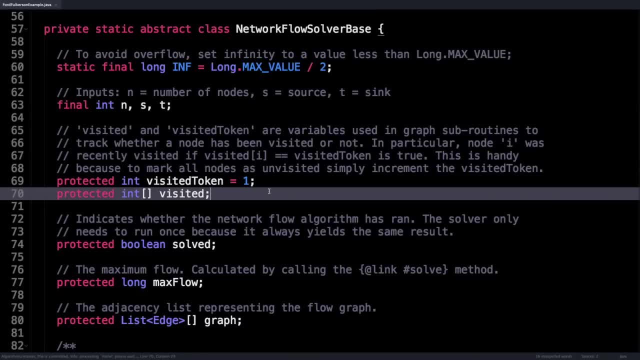 I usually end up using because they greatly help boost performance. So the rationale behind using the visited token in combination with an integer array that tracks the visited state of a Node is that when we're finding augmenting paths, whether via depth for search or breadth, 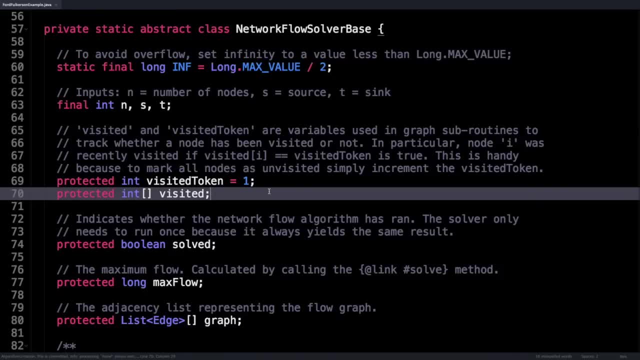 for search or whatever graph traversal method you want to use. you generally want to ensure that your augmenting path doesn't visit the same node twice. Otherwise that could result in the cycle which we don't want. the way to check if node is visited is to check if the 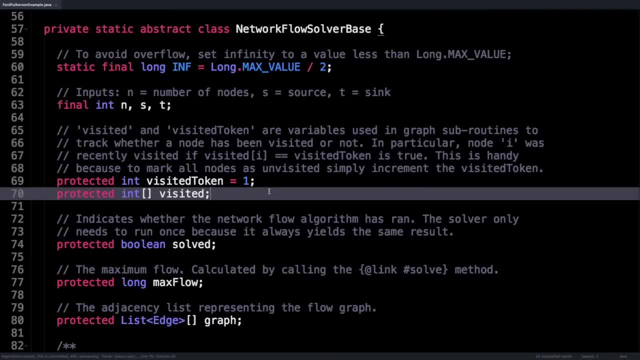 state in the visited array at index is equal to and weighted Tha. and then this is another verb to the visited token. This is super handy because in the next iteration, when we yet again want to find another augmenting path, we can simply reset all the visited states. 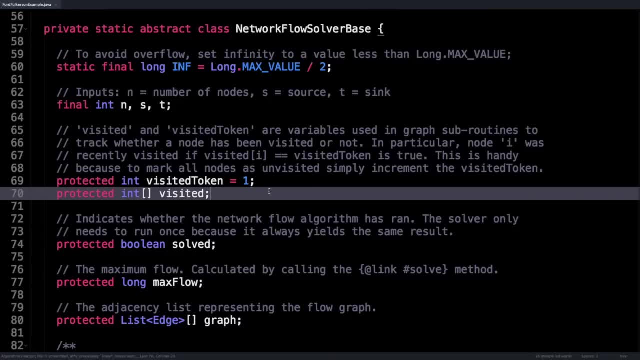 of every node simultaneously by simply incrementing the visited token. I know it's kind of hacky, but it's super efficient and really handy to have. the alternative is actually to maintain a Boolean visited array And you fill that with false values every time just before you. 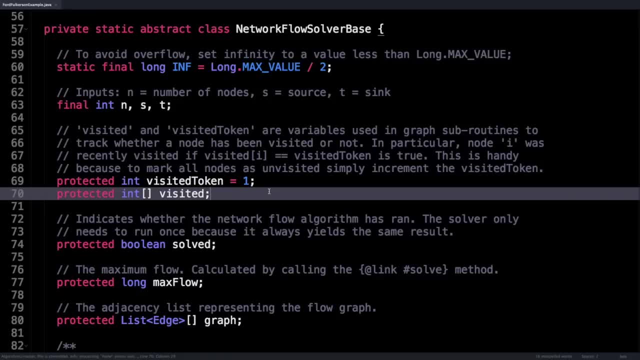 when we yet again want to find another augmenting path, we can simply reset all the visited states of every node simultaneously By simply incrementing the visited token. I know it's kind of hacky, but it's super efficient and really handy to have. The alternative is actually to maintain a Boolean visitor. 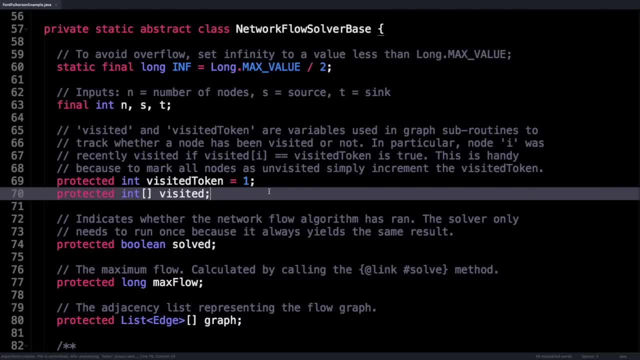 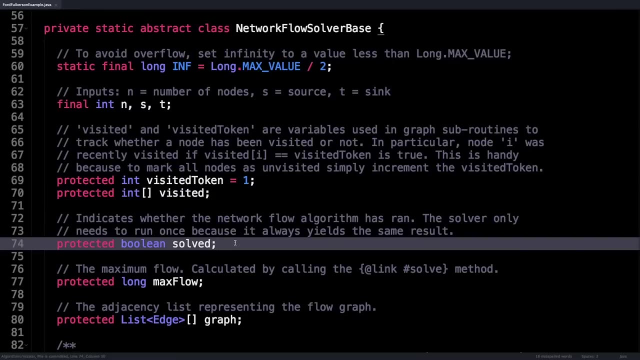 array And you fill that with false values every time, just before you find an augmenting path. That's not great because it requires an additional order and work every time you want to find an augmenting path. Next is a Boolean variable called solved, which indicates: 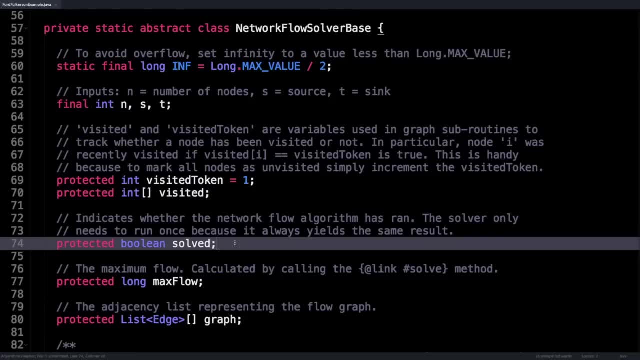 whether or not we have an augmenting path. In this example, we have actually run the network flow solver. the solver only needs to run once because it always yields the same result. So, for example, if the user calls the get max flow method multiple times, the solver only needs to run once. The next value: 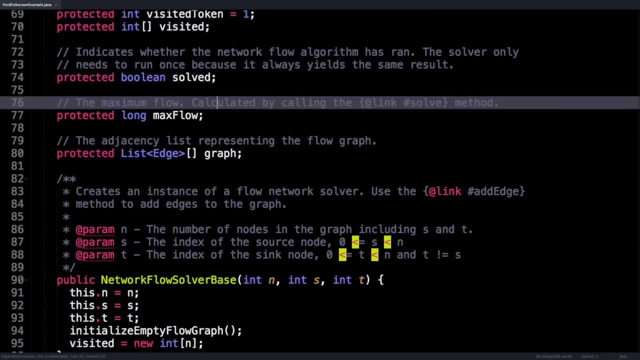 that we have right here is the max flow variable, which is the value we're actually trying to calculate, And finally is the adjacency limit. So the initial value of the max flow method depends on the limit in the method, which is super easy to do. Let's now see a better example of how to increase lung green units. So this is going to be using the max flow method. For my example, I'm going to have a max piping method And I'm going to use this method called the v1.. We're going to see that with my flow graph method. Instead of that, we're going to need to define a max flow method with the index of the index of the index. we're going to have a max flow method with the index of the index of the index of the index. So we create a graph. So this is going to be a graph. I can see that. 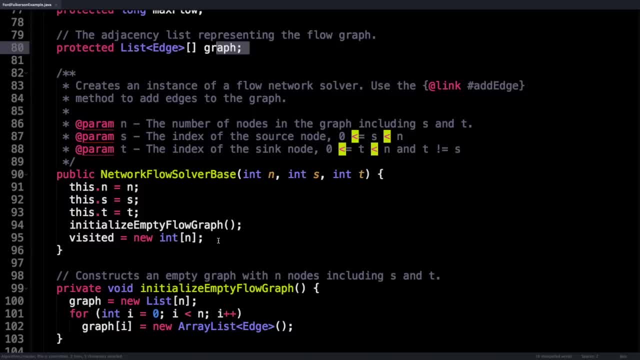 the symbol and the number of nodes in the index are equal to the number of nodes. When our flow graph is in the index, we're going to see that I'm going to have a blank, and then, inside this method, I also take the opportunity to initialize the flow graph and, as well, allocate. 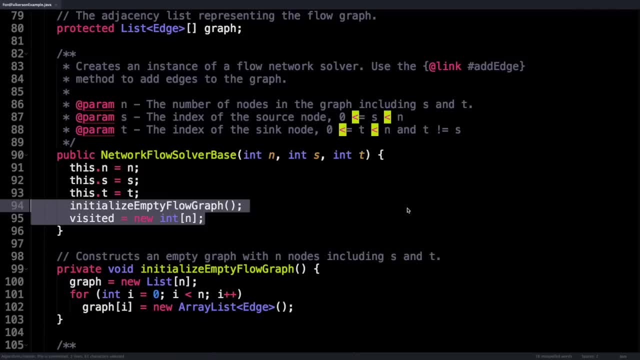 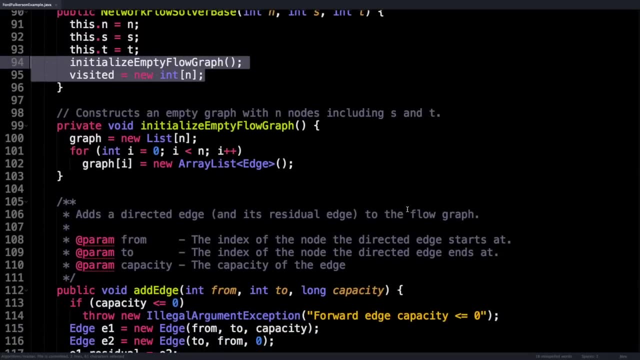 some memory for the visited array we'll be making use of later In the initialize empty flow graph method. all I do is initialize an empty array list of edges for each node index so that we don't get a null pointer exception when we try and add an edge to the 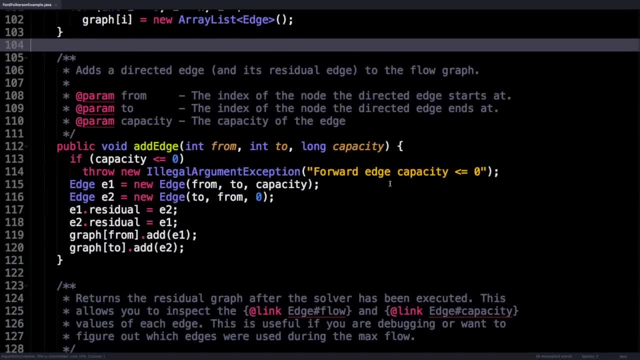 graph, Talking about adding edges to the graph as having a look at the add edge method. here we need to provide the start node and the N node of the directed edge and also provide a positive capacity for that edge. If the capacity is negative or a zero, we throw an. 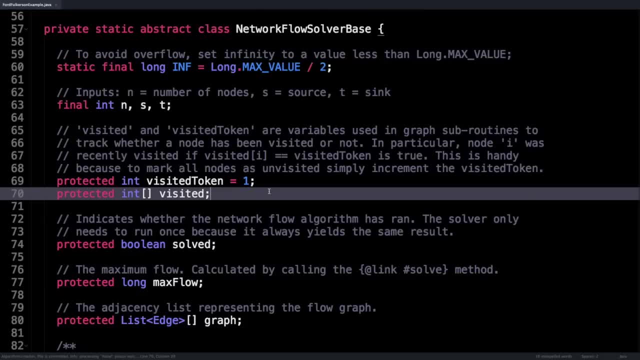 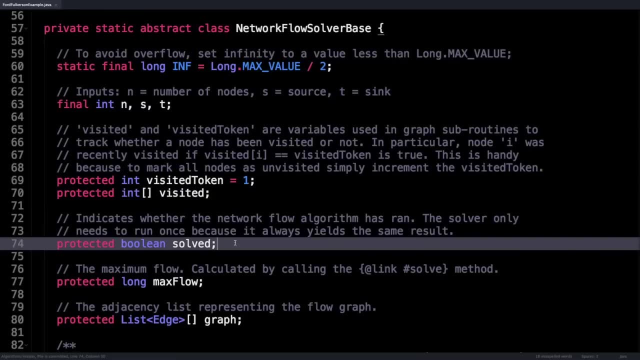 find an augmenting path. That's not great, because it requires an additional order and work every time you want to find an augmenting path. Next is a Boolean variable called solved, which indicates whether or not we have actually run the network flow solver- the solver only. 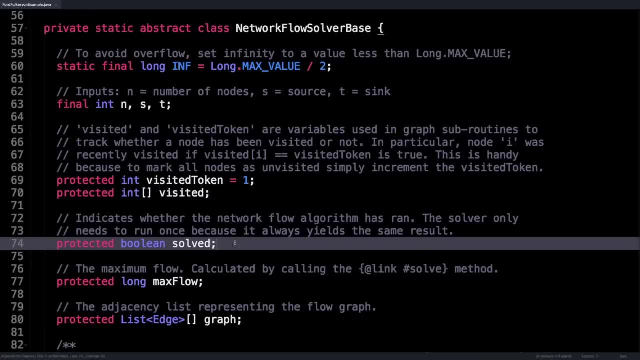 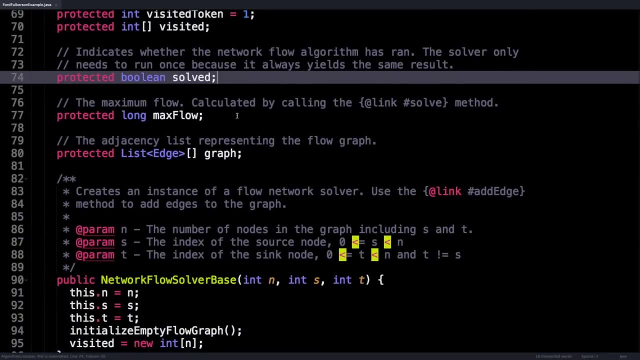 needs to run once, because it always yields the same result. So, for example, if the user calls the get max flow method multiple times, the solver only needs to run once. The next value that we have right here is the max flow variable, which is the. 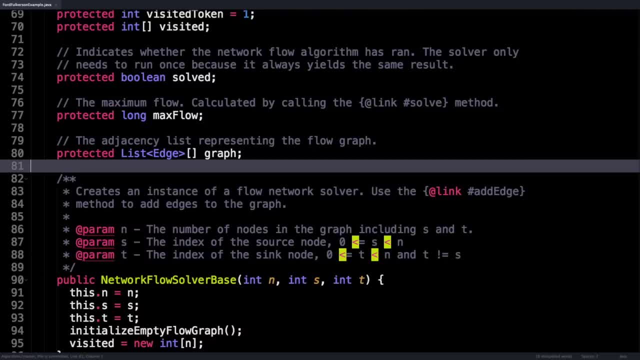 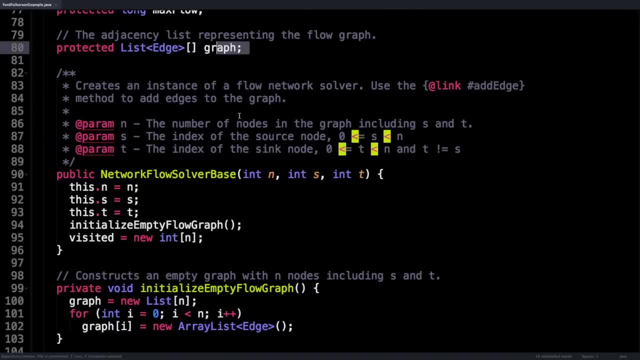 value we're actually trying to calculate. And finally, is the adjacency list representing the flow graph itself. Looking at the constructor, we require the user to specify the number of nodes, along with the index Of the source and the sink nodes. Then, inside this method, I also take the opportunity to 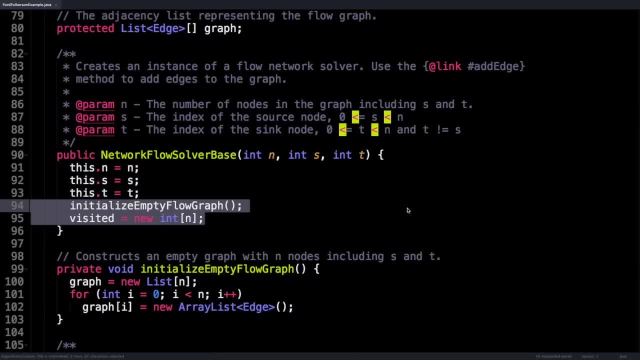 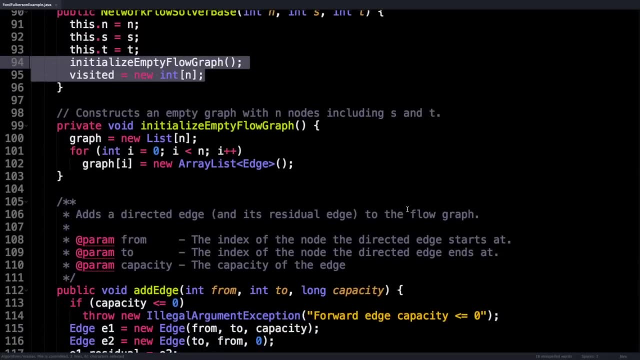 initialize the flow graph and, as well, allocate some memory for the visited array we'll be making use of later In the initialize empty flow graph method. all I do is initialize an empty array list of edges for each node index, so that we don't get a null pointer. 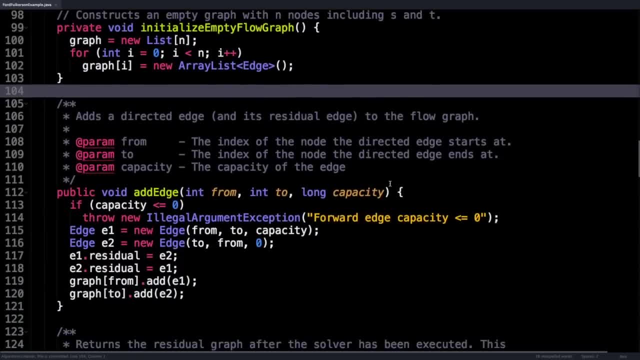 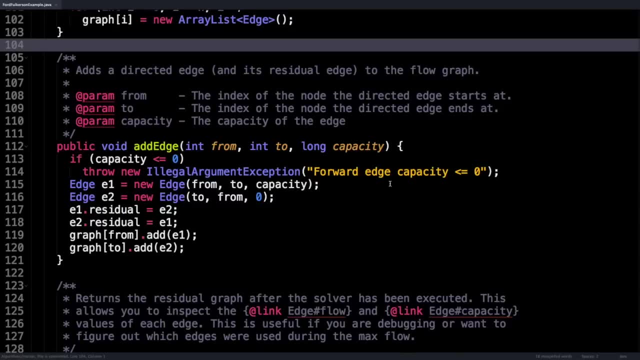 exception when we try and add an edge to the graph. Talking about edge, we're going to talk about adding edges to the graph. Let's have a look at the add edge method. Here we need to provide the start node and the end node of the directed edge and also provide 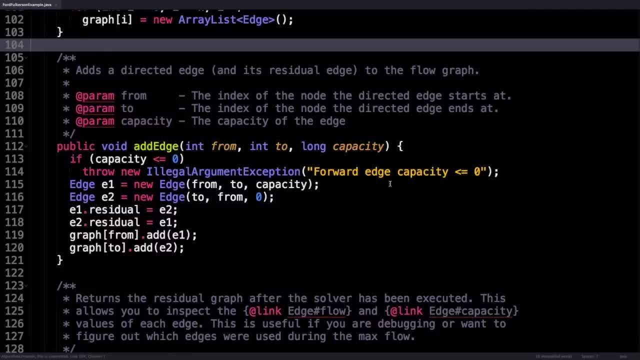 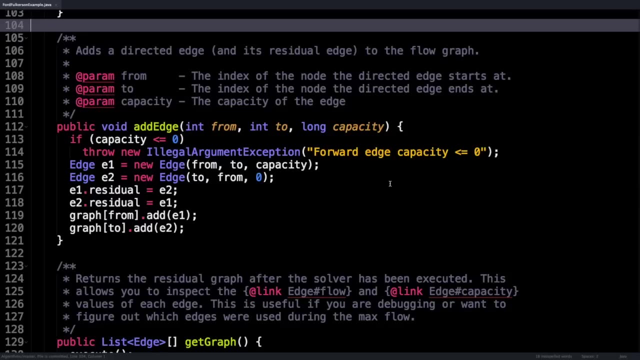 a positive capacity for that edge. If the capacity is negative or zero, we throw an exception because that is an illegal argument. Then what we do is we actually create the forward edge and the residual edge. you'll notice that the residual edge actually has. 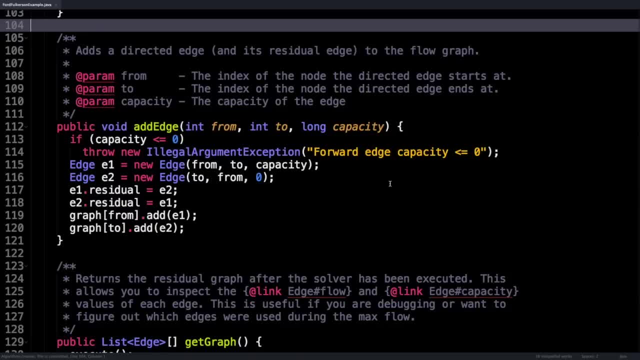 a capacity of zero, then what we do is we make the forward edges residual edge, the residual edge, and the residual edges residual edge, the forward edge, And finally we add them both to the flow graph. So, in effect, each edge is each other's inverse, And this: 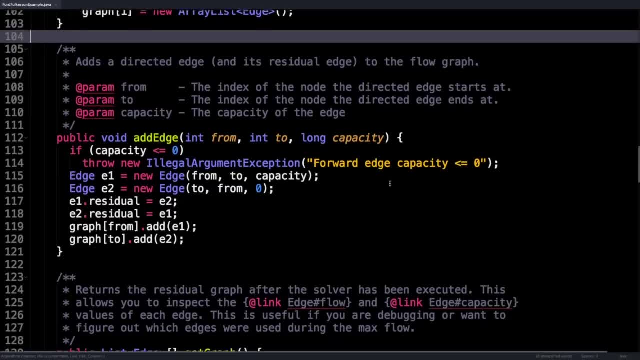 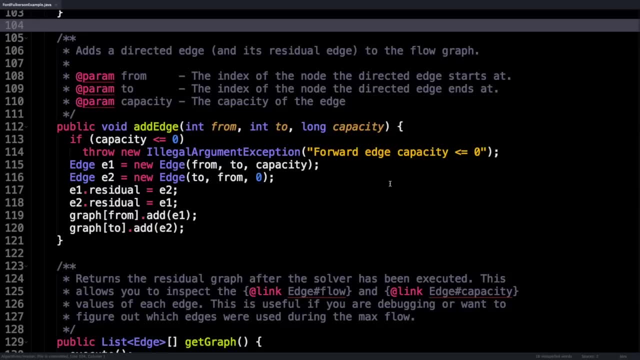 exception, because that is an illegal argument. Then what we do is we actually create the forward edge and the residual edge. you'll notice that the ace residual edge actually has a capacity of zero. then what we do is we make the forward edges residual edge, the residual edge and the residual edges residual edge, the forward edge, And 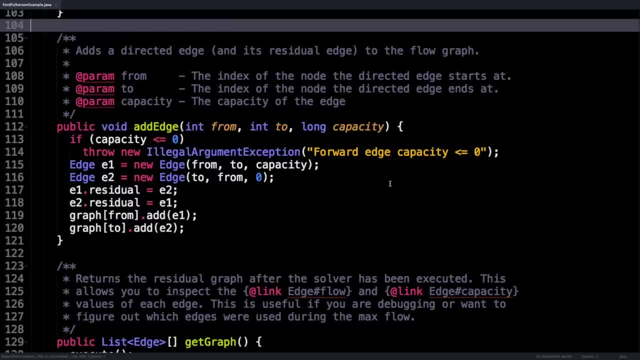 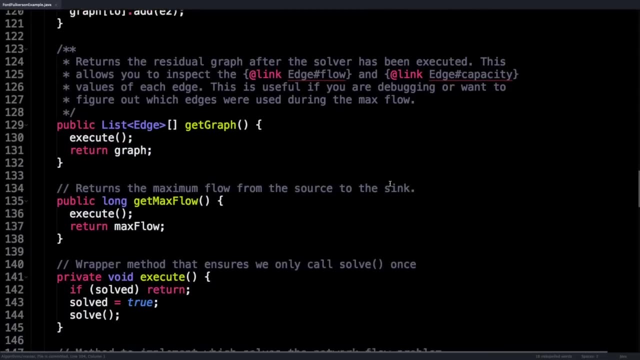 finally, we add them both to the flow graph. So, in effect, each edge is each other's inverse, And this is exactly what we want. we want a pointer that we can simply access when we need to access an edges- residual edge. The remaining methods here are simply client facing. 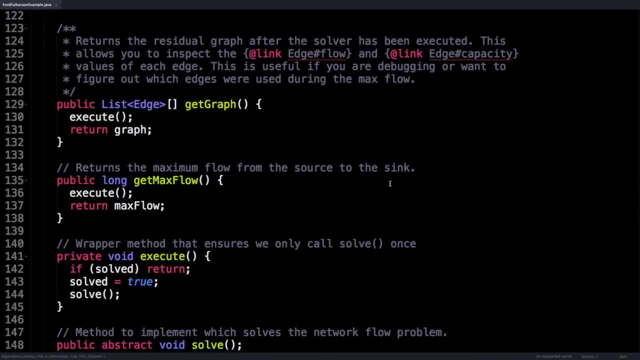 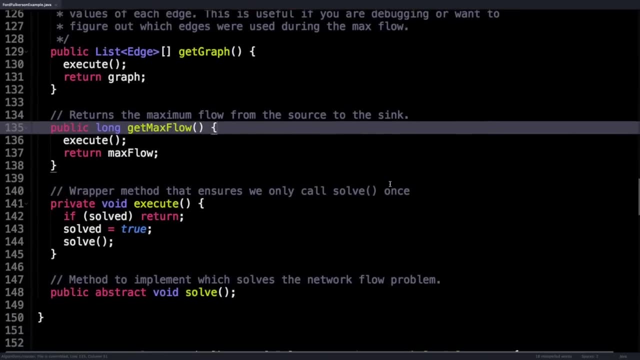 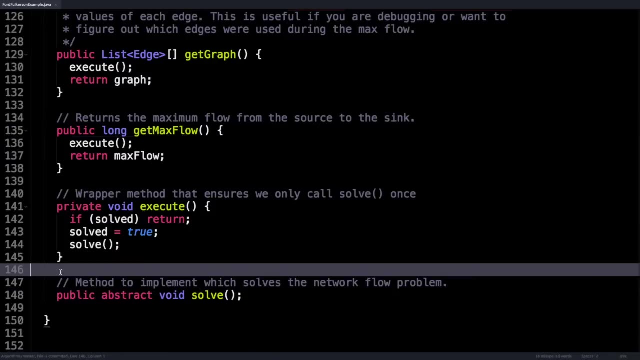 methods. they can be used to get the residual graph after the solver has been executed And to obtain the maximum flow of the graph. you'll notice that there's also this one special method down here, which is the solve method, And this is the method that the subclass needs. 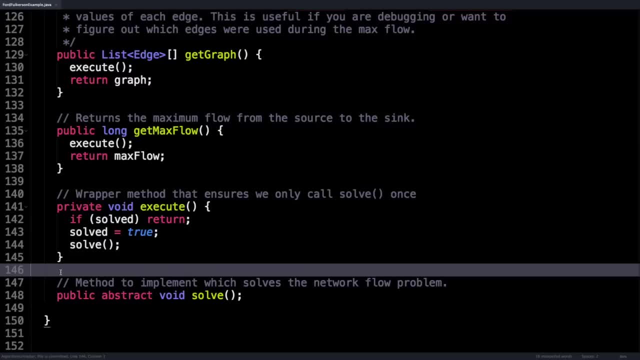 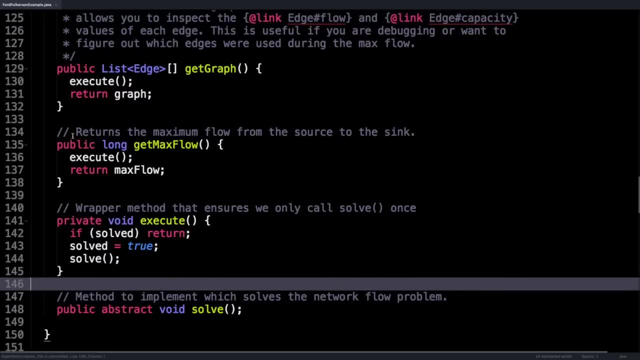 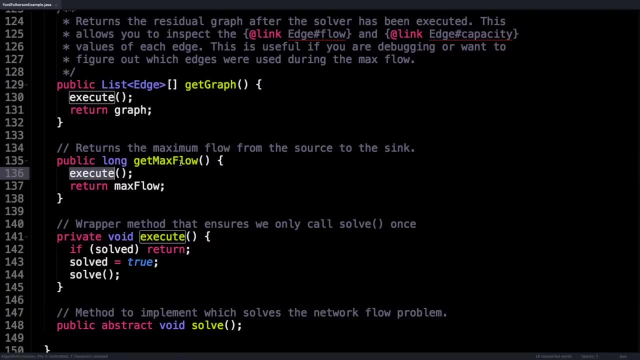 to override. This is the method which actually is solves the network flow problem and actually pushes the flow through the network. And you can see that every time the client goes and calls one of these methods, like get graph or get max flow, it calls the execute method and the execute method will run the solver. 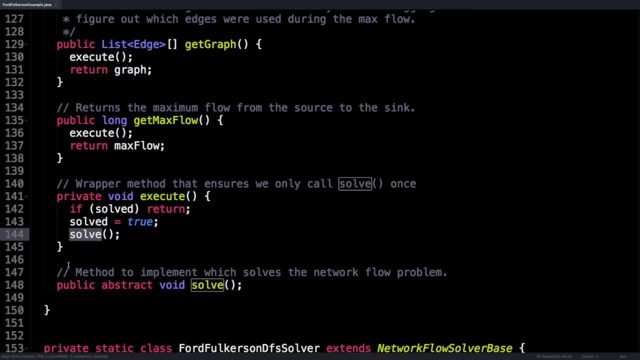 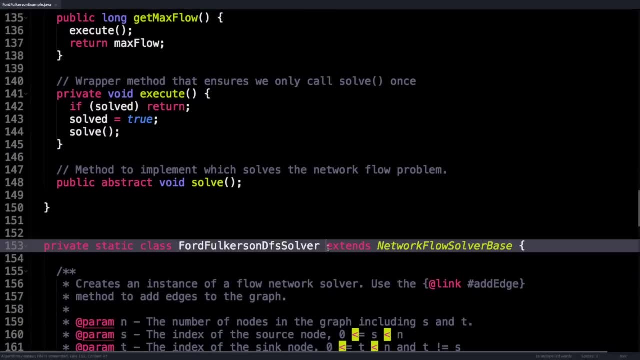 So we will call this method if it hasn't been executed already. So it's got that smart logic built in. Now let's take a look at the Ford Fulkerson depth first search solver which you can see actually extends the network flow based solver. So we know it actually implements the solve method. 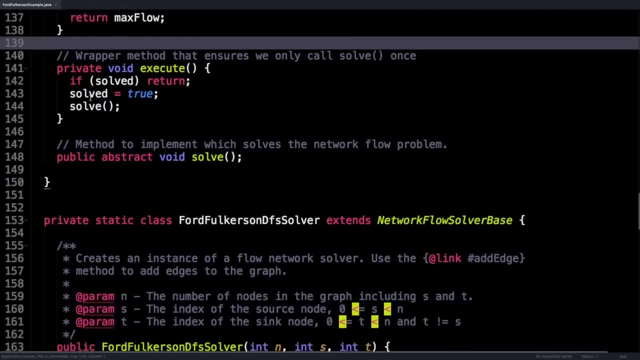 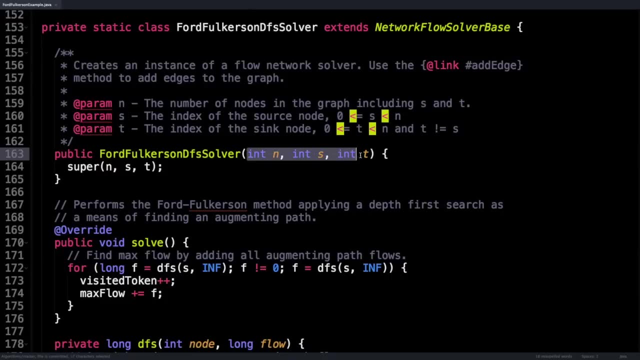 that we need for the get max flow method. Awesome, Let's, let's have a look at this. So the first thing you'll notice is that this method also takes the inputs and s&t, And all we do here is we call the superclass constructor in the network flow based solver, which does. 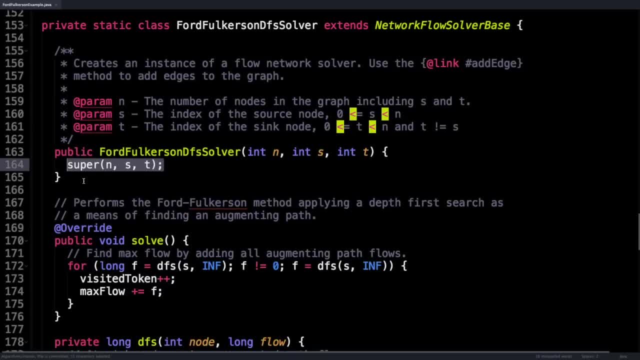 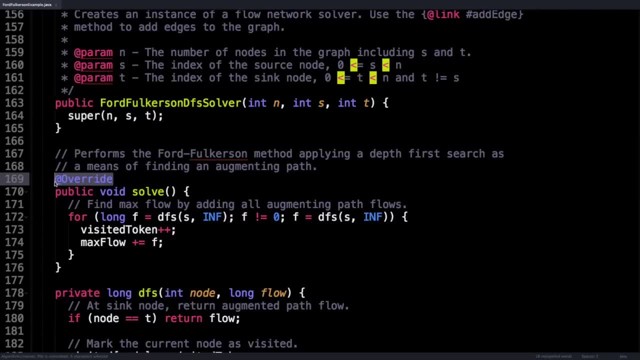 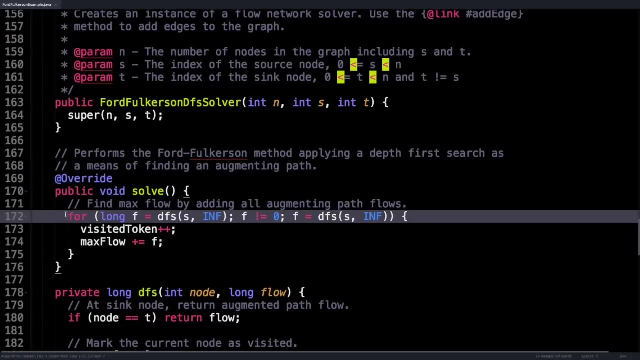 all that nice initialization that we know about. Next is the most important method, which is that solve method I was talking to you about And you can see that actually overrides the method in the superclass. So in this method you can see that I'm repeatedly calling the depth. first search method returns as output. 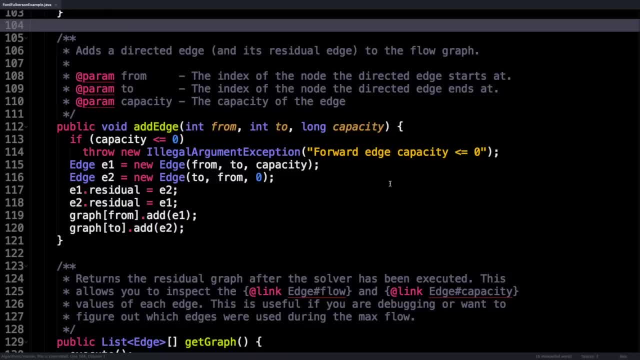 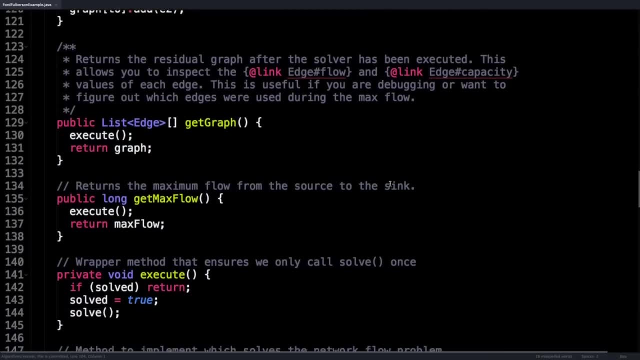 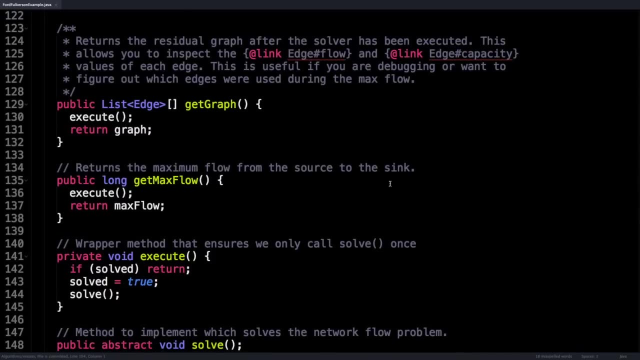 is exactly what we want. We want a pointer that we can simply access when we need to access an edges residual edge. The remaining methods here are simply client fields Basing methods. they can be used to get the residual graph after the solver has been executed. 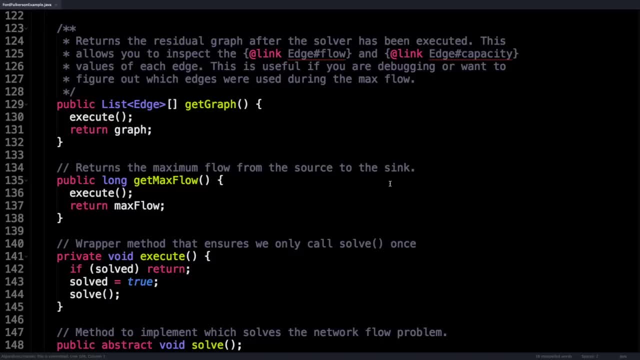 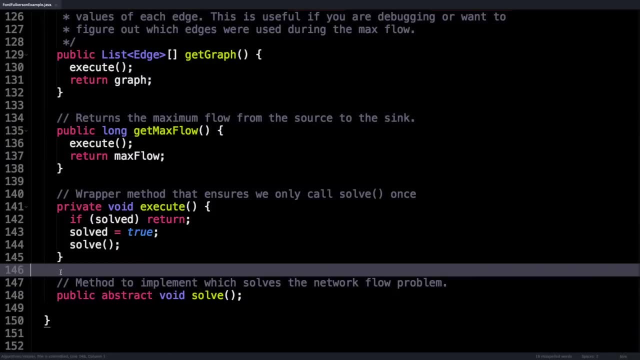 and to obtain the maximum flow of the graph. you'll notice that there's also this one special method down here, which is the solve method, And this is the method that the subclass needs to override. This is the method which actually solves the network flow problem and actually 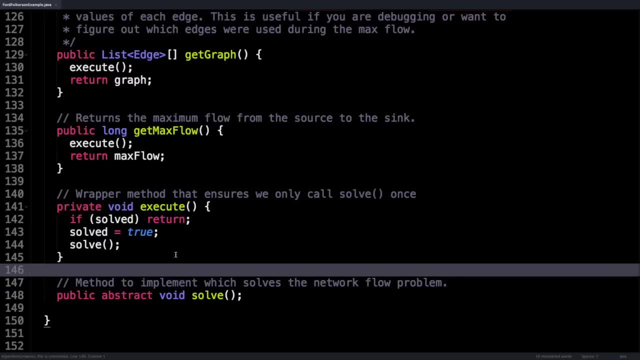 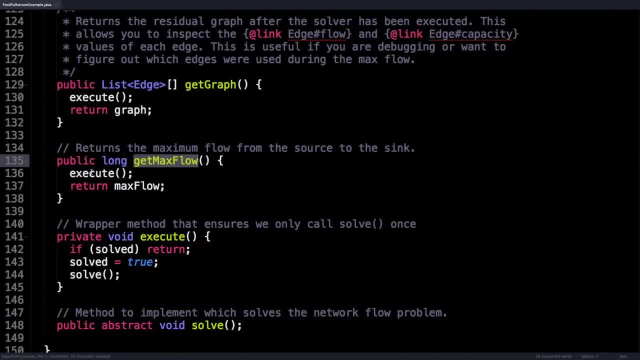 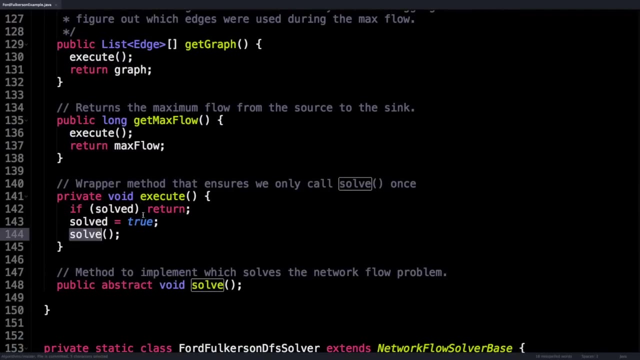 pushes the flow through the network. And you can see that every time the client goes and calls one of these methods, like get graph or get max flow, it calls the execute method and the execute method will run the solver. so we will call this method if it hasn't been executed already. So it's got that smart logic built in Now. 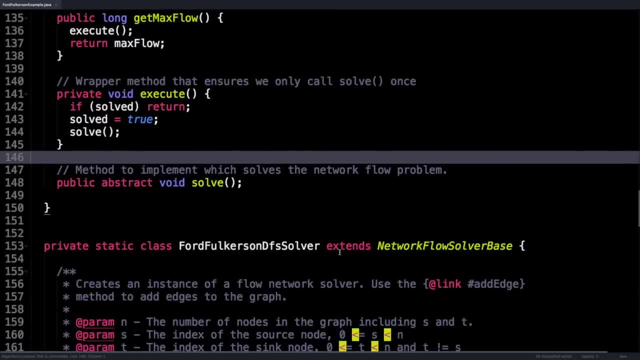 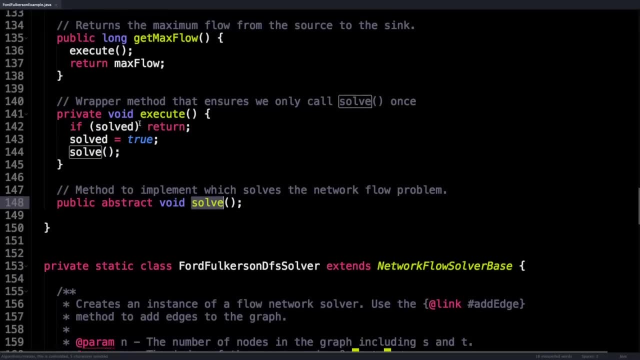 let's take a look at the Ford Fulkerson depth first search solver, which, you can see, actually extends the network flow based solver, So we know it actually implements the solve method that we need for the get max flow method. Awesome, Let's, let's have a look at this. So the first thing you'll notice: 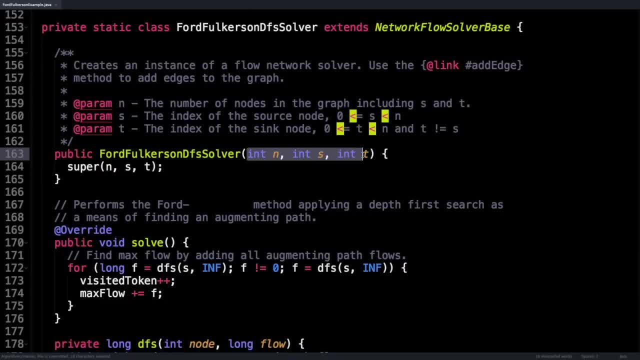 is that this method also takes the inputs and s and t, And all we do here is we call the superclass constructor in the network flow based solver, which does all that nice initialization that we know about. Next is the most important method, which is that solve. 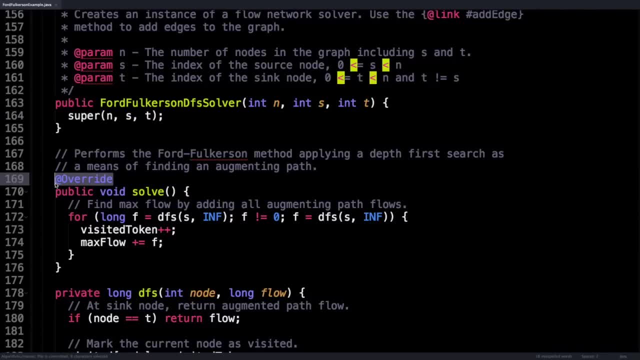 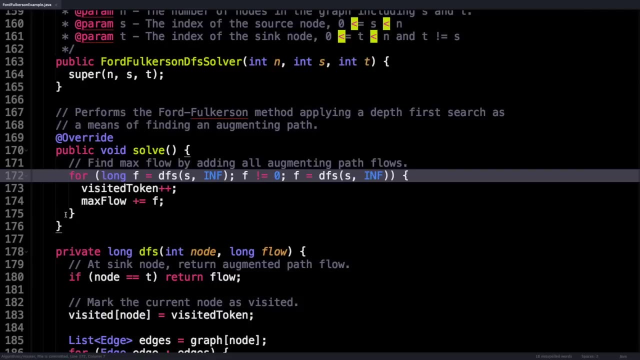 method I was talking to you about And you can see that actually overrides the method in the superclass. So in this method you can see that I'm repeatedly calling the depth. first search method returns as output the bottleneck value found along the augmenting path. I store that value as F and increase the max flow by F in each iteration because 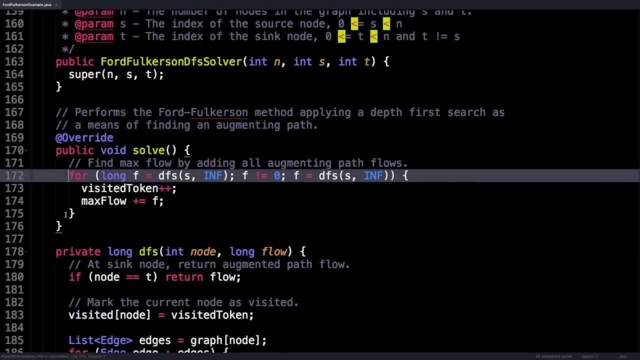 we know that the sum of the bottleneck values equals the max flow. we do this until the bottleneck value is zero, at which point we know that no more augmenting paths exist And the algorithm can terminate in between finding each augmenting path. you can see that increment the visited 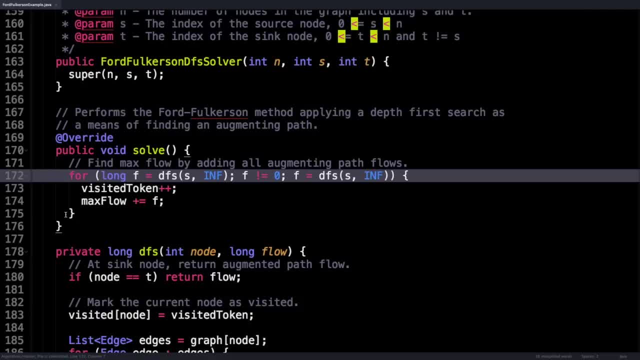 the bottleneck value found along the augmenting path. I store that value as F and increase the max flow by F in each iteration, because we know that the sum of the bottleneck values equals the max flow. we do this until the bottleneck value is zero, at which point we 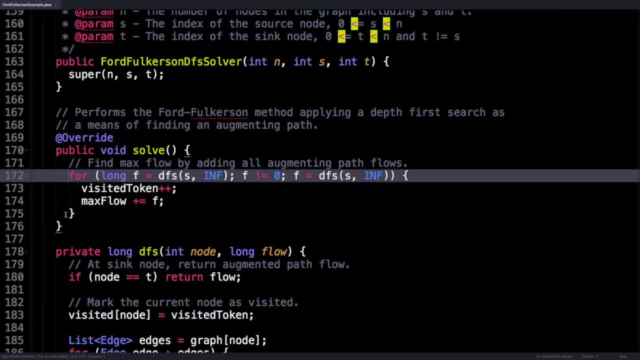 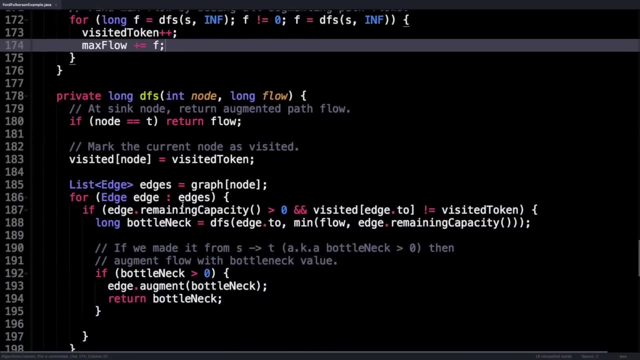 know that no more augmenting paths exist and the algorithm can terminate In between finding each augmenting path. you can see that increment the visited token. this is used to make the state of every node on visited. The depth for search method itself takes two arguments: the node ID and 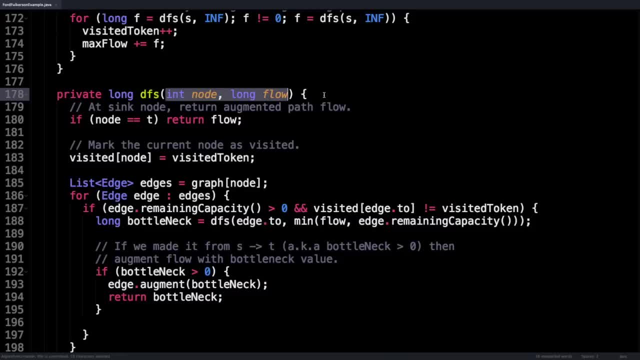 the flow. Initially the starting node is passed in as the node index and the flow is set to be infinity. As we progress through the flow graph, the flow value eventually becomes the bottleneck value as we find smaller and smaller edges with more restricting capacities, And we stop the algorithm once the node index. 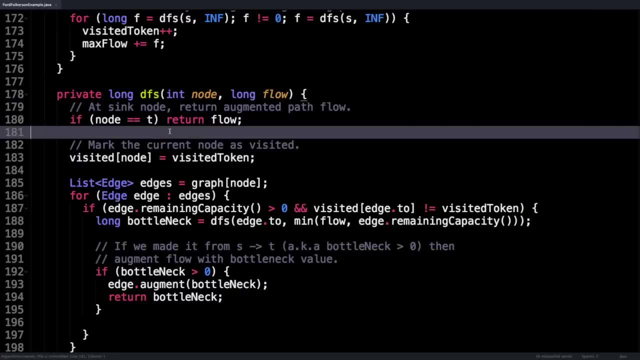 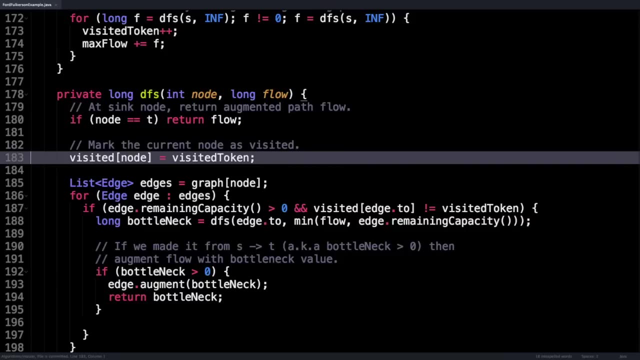 equals the sink. So that's actually our base case right here. Afterwards, since we know that the current node is not the sink, what we do is we explore it by marking the current node as visited. We do this by assigning the current index or the current node index to 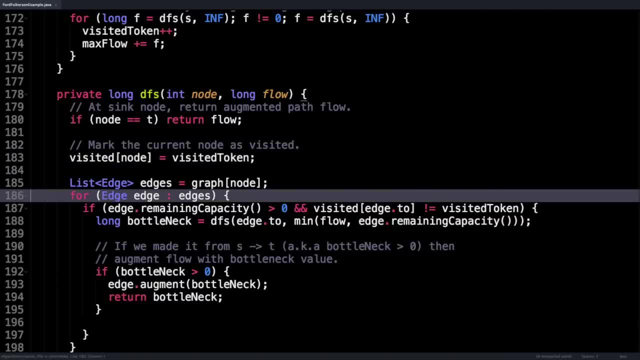 be equal to the visited token. then comes the interesting part. First, we get all the outgoing edges of this node- residual otherwise- and then loop over them If the remaining capacity is greater than zero, meaning we can push flow through that edge. And the next: 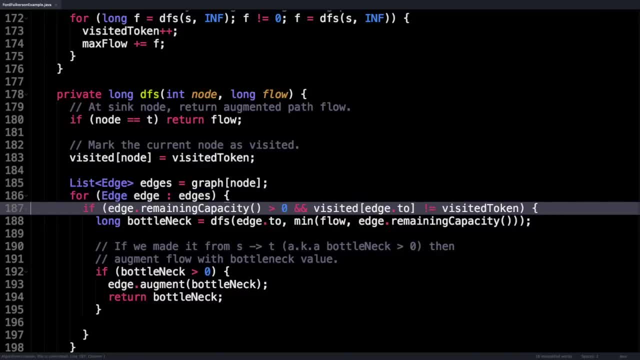 node that we're going to is unvisited, meaning we don't risk creating a cycle. then we're going toеля Marketing, clamcom and we're also going to create the cycle designer and we will give the visibility node: the Canadians of the Alaska system this time. 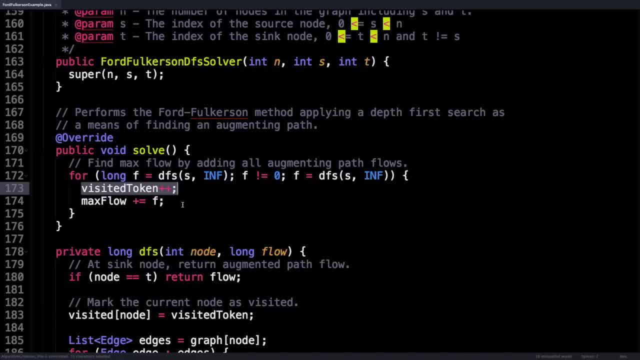 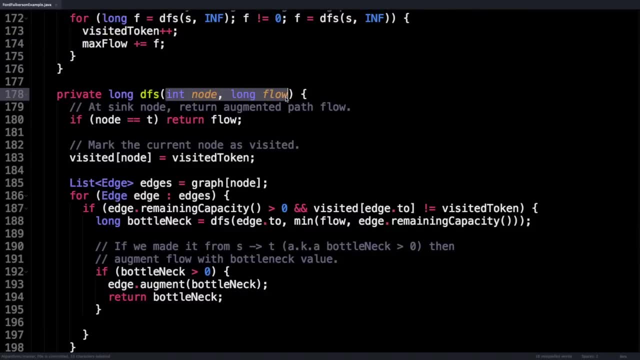 token. this is used to make the state of every node on visited the depth first. search method itself takes two arguments: the node ID and the flow. Initially, the starting node is passed in as the node index and the flow is set to be infinity. As we progress through, 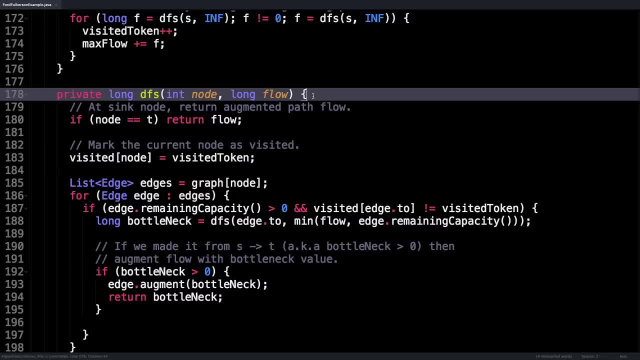 the flow graph. the flow value eventually becomes the value after the flow graph. So when we do the flow graph we actually see comes the bottleneck value as we find smaller and smaller edges with more restricting capacities. And we stopped the algorithm once the node index equals the sink. So that's actually. 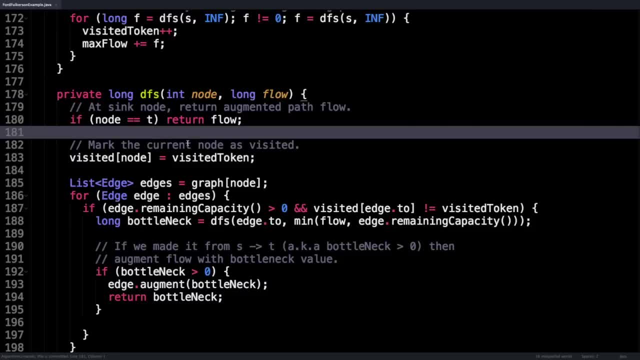 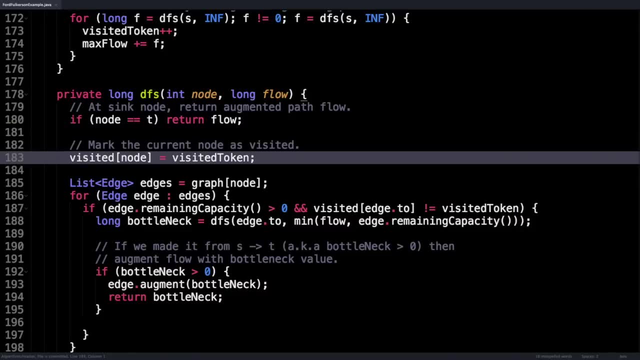 our base case right here Afterwards, since we know that the current node is not the sink, what we do is we explore it by marking the current node as visited. we do this by assigning the current index, or the current node index, to be equal to the visited token. then comes 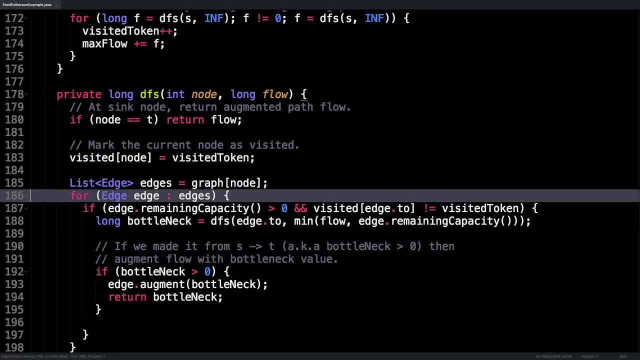 the interesting part: First we get all the outgoing edges of this node, residual or otherwise, and then loop over them. If the remaining capacity is greater than zero meaning, we can push flow through that edge. and the next node that we're going to is unvisited meaning. 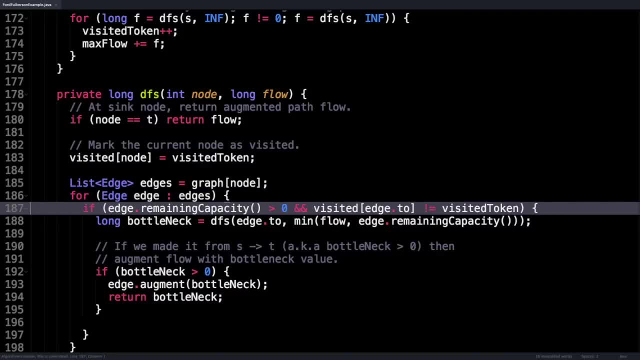 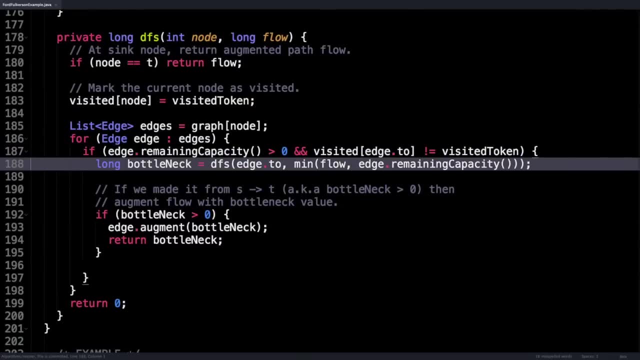 we don't risk creating a cycle, then we can enter this inner if block right here And inside the if block. the first thing I do is call the depth first search method recursively. what I do is I pass in the index of the next node where we want to go to and the new flow. 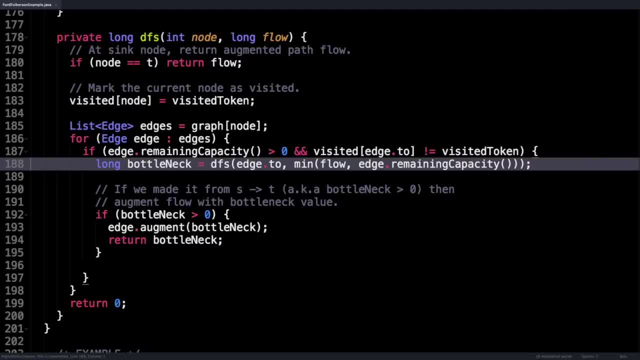 value which should equal the minimum of the current flow, or the current edges remain in capacity. Remember that that flow parameter is trying to capture the bottleneck value. that intuitively makes sense. It's saying: either keep the previously found bottleneck bottleneck value Or, if this new edge is even smaller than it should be the new bottleneck. 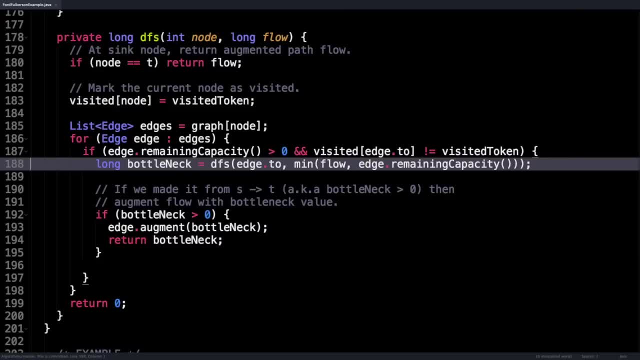 value. This process continues recursively until the base cases hit and the sink was reached. This returns the bottleneck of the augmenting path. we can then use that value to augment the flow of our augmenting path. However, first check that the bottleneck value. 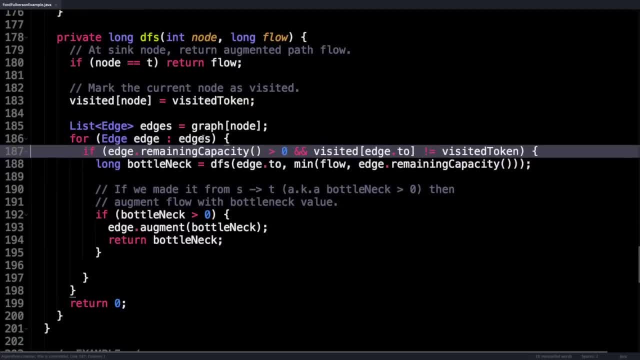 we can enter this inner if block right here Inside the if block. the first thing I do is call the depth for search method recursively. What I do is I pass in the index of the next node we want to go to and the new flow value, which should equal the minimum of the current. 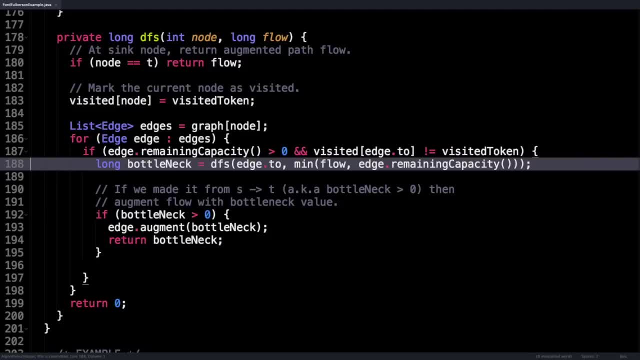 flow or the current edges, remaining capacity. Remember that that flow parameter is trying to capture the bottleneck value. that intuitively makes sense. It's saying: either keep the previously found bottleneck value or, if this new edge is even smaller than it should be, the new. 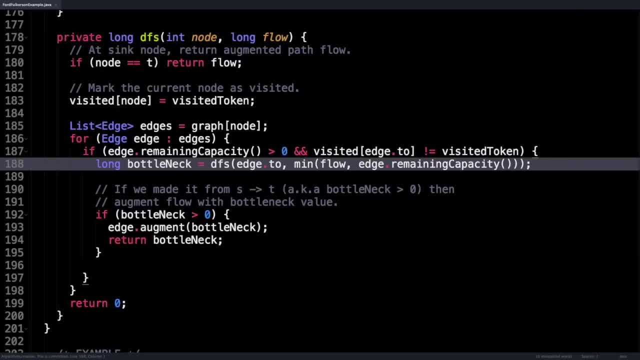 bottleneck value. This process continues recursively until the base cases hit and the sink was reached. This returns the bottleneck of the augmenting path. we can then use that value to augment the flow of our augmenting path. However, first check the that the bottleneck value is greater than zero. it could be the case that we never actually 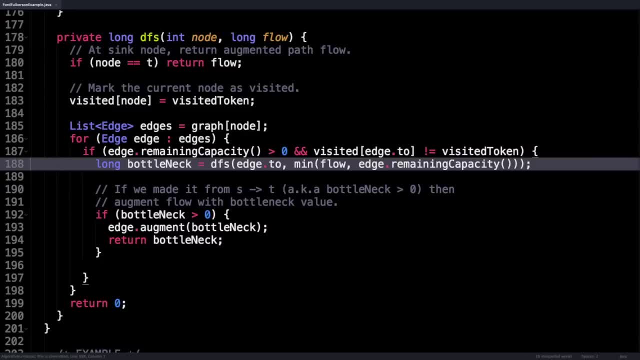 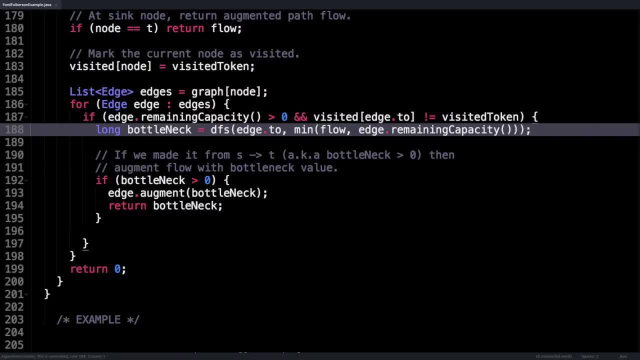 made it to the sink And we hit a dead end. Assuming that's not the case, simply argument the flow by increasing the flow in the forward edge by the bottleneck value and decreasing the flow in the residual edge by the bottleneck value. After that, simply return the bottleneck. 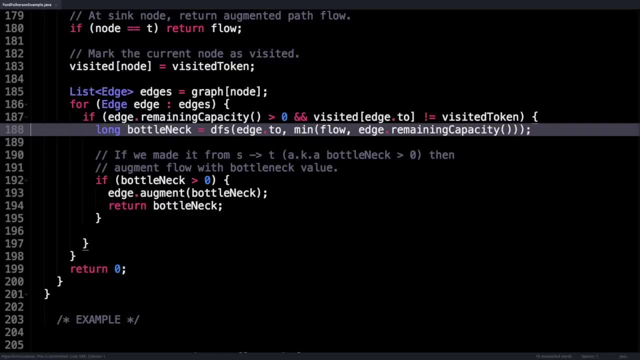 value. This propagates it up the stack so that all the other edges along the augmenting path can also be augmented. This also ensures that the bottleneck value is returned to the solve method, where the max flow is actually calculated. So that's about everything I want. 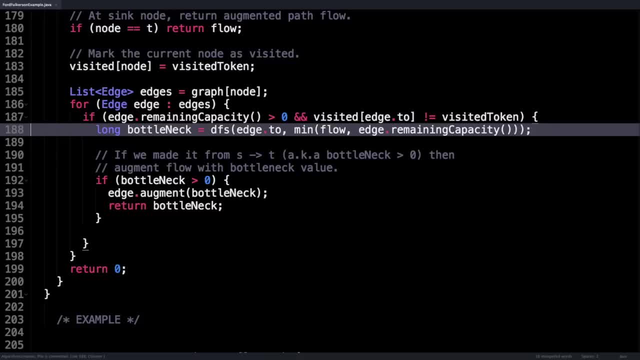 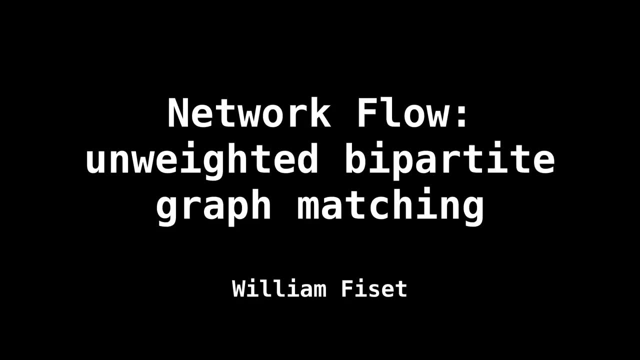 to cover for the Ford Fulkerson method implemented with a depth first search. Today we're going to start diving a little deeper into network flow. we're going to talk about unweighted bipartite graph matching and specifically, how we can use max flow to find a matching. 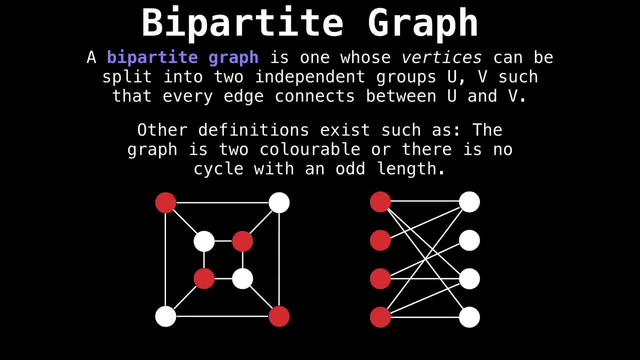 for us. Before we get started, though, I should mention what a bipartite graph is. A bipartite graph is one whose vertices can be split into two independent groups, u and v, such that every edge connects between u and v. Other definitions exists, such as the graph is too. 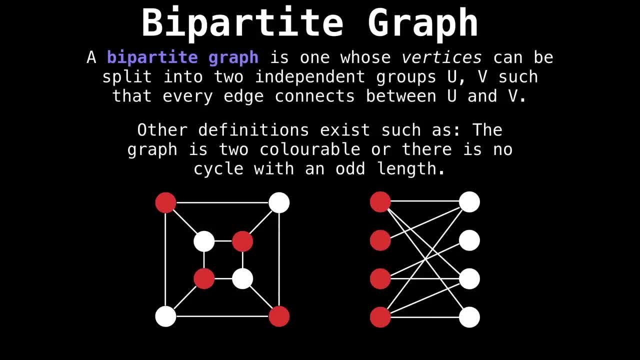 colorable or there is a cycle with an odd line. bipartite graphs often arise when we're trying to match one group of items to another in some way. Think of situations such as matching suitable candidates to jobs. there could be multiple jobs and multiple candidates, but not every. 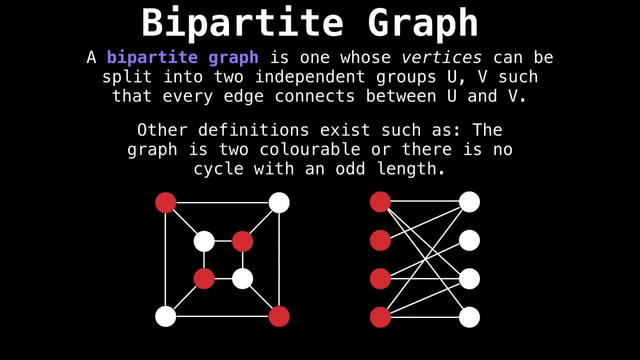 candidate is suitable for each job. If jobs are red nodes and candidates are white nodes, then there would be an edge between the two if the candidate is good fit. Another situation could be matching surfers to surfboards. Suppose there are multiple surfers. 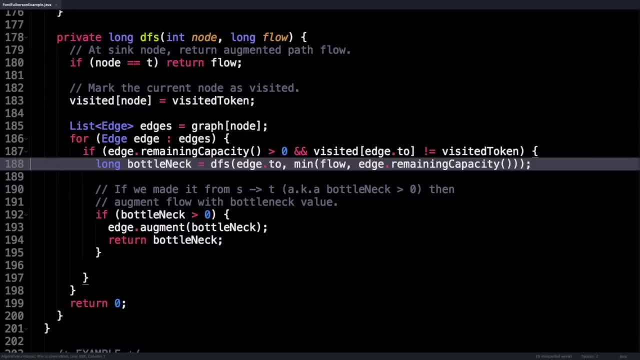 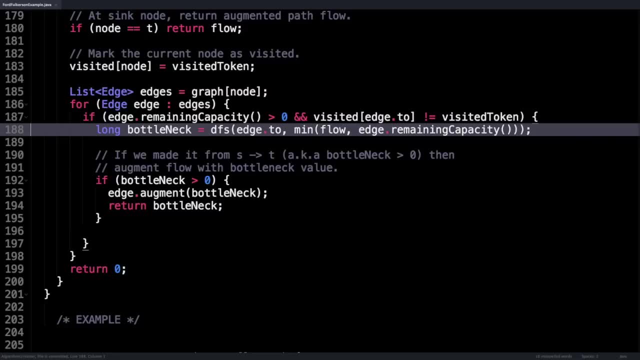 is greater than zero. it could be the case that we never actually made it to the sink And we hit a dead end. Assuming that's not the case, simply argument the flow by increasing the flow in the forward edge by the bottleneck value and decreasing the flow in the residual. 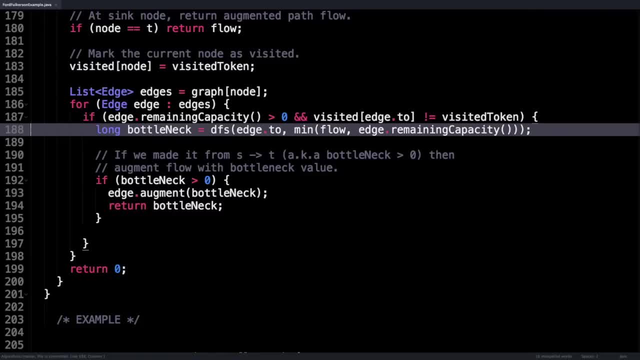 edge by the bottleneck value. After that, simply return the bottleneck value. This propagates it up the stack so that all the other edges along the augmenting path can also be augmented. This also ensures that the bottleneck value is returned to the solve method where the 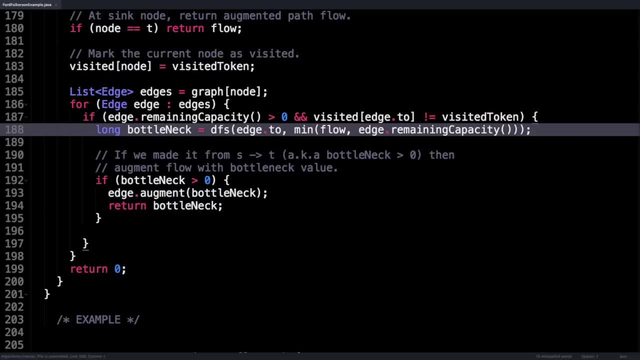 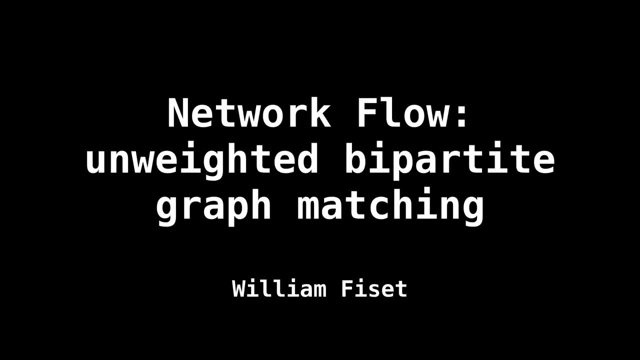 max flow is actually calculated. So that's about everything I want to cover for the Ford Fulkerson method implemented with a depth first search. Today we're going to start diving a little deeper into network flow. we're going to talk about unweighted bipartite. 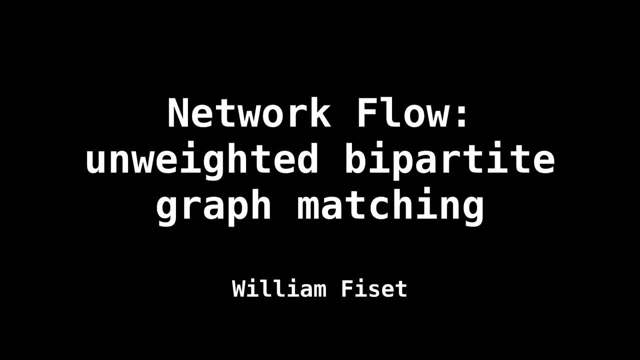 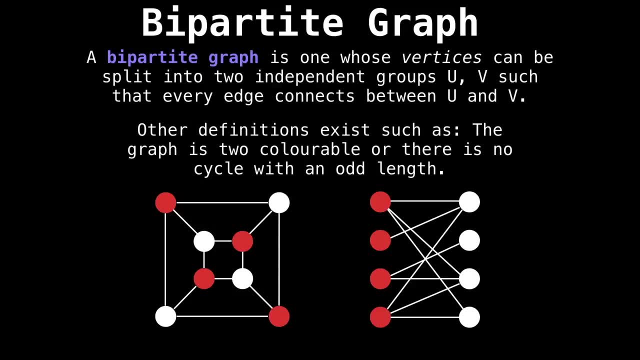 graph matching and specifically, how we can use max flow to find a matching for us. Before we get started, though, I should mention what a bipartite graph is. A bipartite graph is one whose vertices can be split into two independent groups, u and v, such that every edge connects. 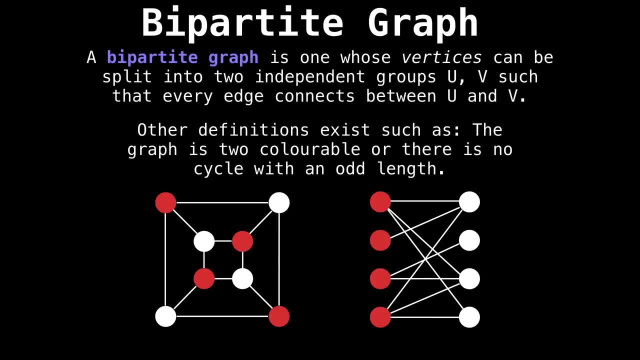 between u and v. Other definitions exists, such as the graph is too colourable or there is a cycle with an odd line. bipartite graphs often arise when we're trying to match one group of items to another in some way. Think of situations such as matching suitable candidates. 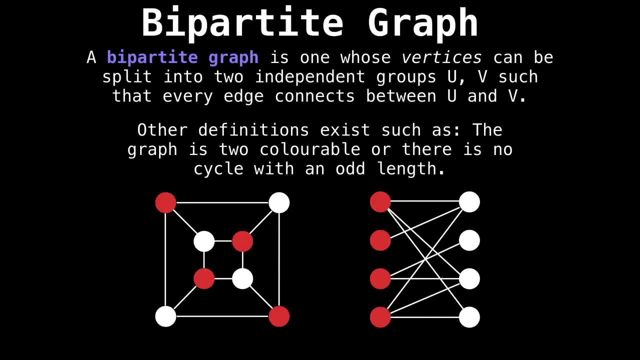 to jobs. There could be multiple jobs and multiple candidates, but not every candidate is suitable for each job. If jobs are red nodes and candidates are white nodes, then there would be an edge between the two if the candidate is a good fit. Another situation could be matching surfers. 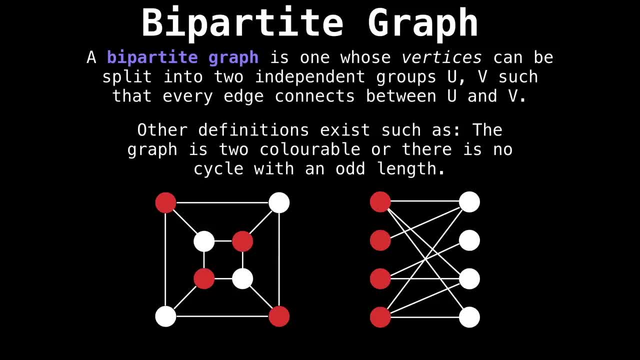 to surfboards. Suppose there are multiple servers and multiple surfboards, But the surfers have preferences and requirements for their boards, such as colour, size and size And so on. then the same thing happens. we place an edge between the surfer and the surfboard. 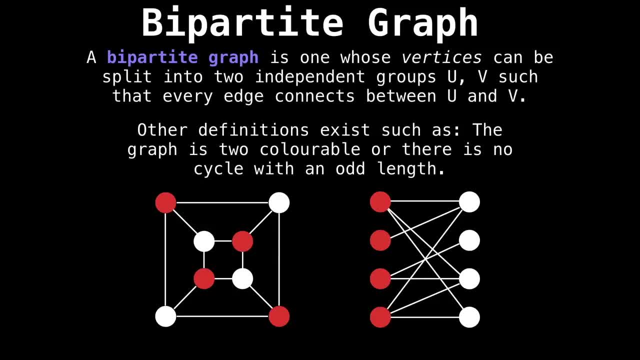 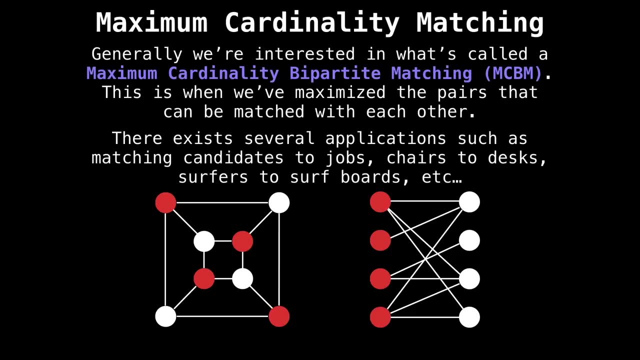 and multiple surfboards, but the surfers have preferences and requirements for their boards, such as color, size and so on, then the same thing happens. we place an edge between the surfer and the surfboard to indicate that they are able to be matched. Generally, when 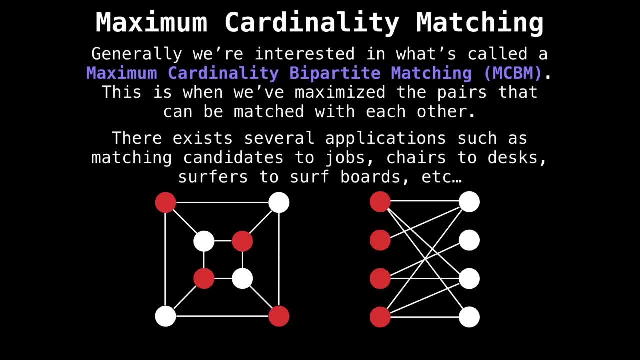 we're setting up a bipartite graph. we're interested in what's called a maximum cardinality bipartite matching. This is when we've maximized the pairs that can be matched. So we're going to be matching the pairs that can be matched with each other. For example, we've maximized 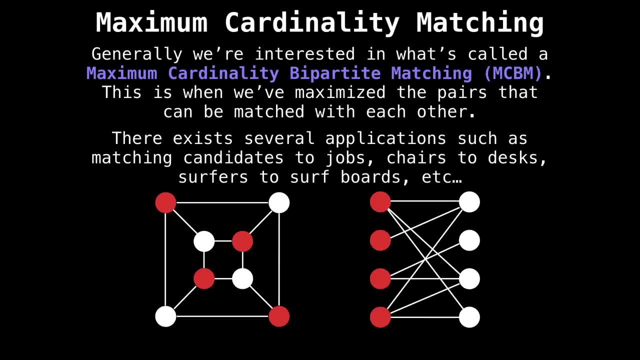 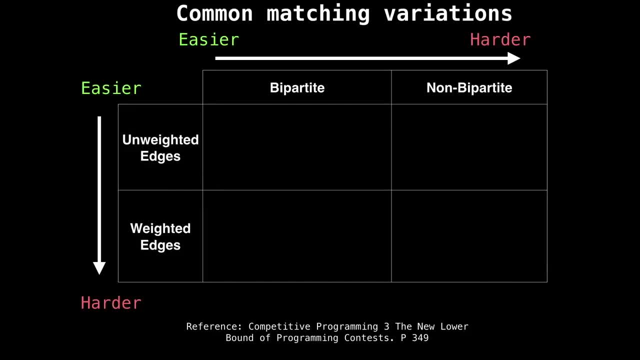 the number of candidates that can be matched to jobs or the number of surfers to surfboards. Finding a matching is not unique to bipartite graphs, However. you can also have a matching on a non bipartite graph. This variant is a lot harder to solve and also much less common. 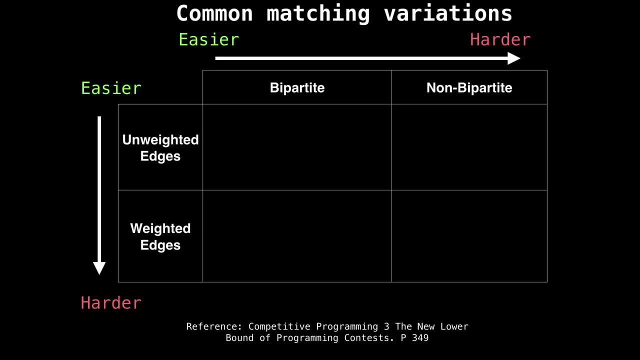 Another variant is finding a maximum matching on a weighted graph where you can either match or maximize or minimize the cost of the matching. This variant is also much harder to solve than the unweighted version. In the unweighted version, no edge is better in any sense than 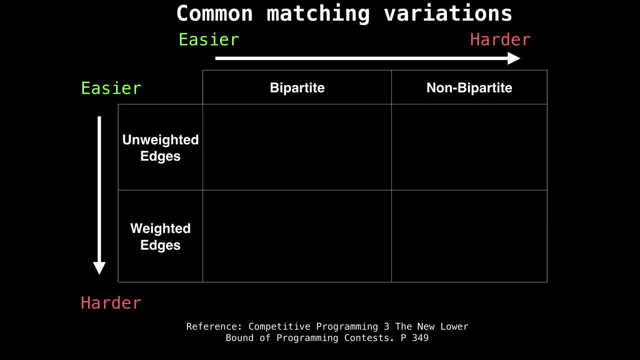 any other edge, So it makes finding a matching much, much easier. We're mostly going to focus on the top left box, which is the easiest of the four variants, But hopefully we'll get to poke around in some of the other boxes as well. So if you want to find a maximum 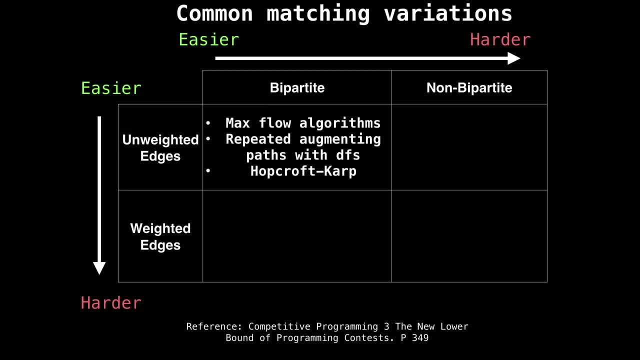 matching on an unweighted bipartite graph. you have lots of options. You can either set up the graph as a flow problem and push flow through it, which is what we'll look at in this video, But you can also repeatedly find augmenting paths which maximize the matching. 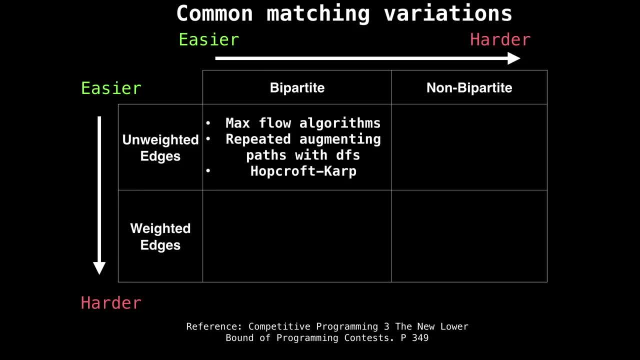 using a depth first search, Or we can use the specialized Hopcroft CARP algorithm to do the same thing a lot faster If your edges are weighted and your graph is still bipartite. you also have a lot of options. You can use a min cost, max flow algorithm, or you can run the Hungarian algorithm And 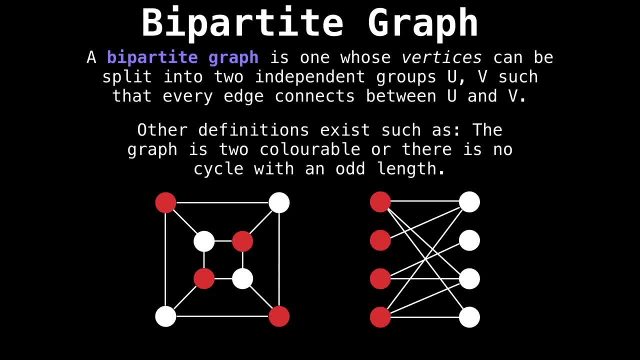 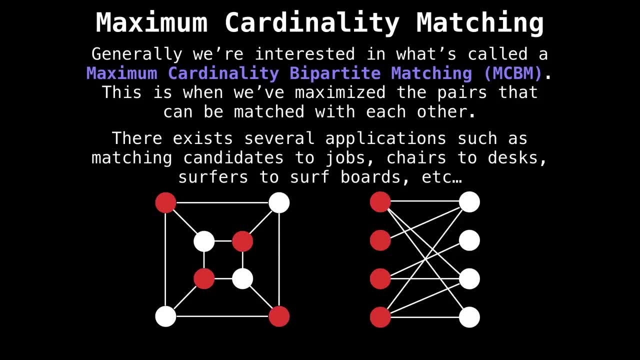 to indicate that they are able to be matched. Generally, when we're setting up a bipartite graph, we're interested in what's called a maximum cardinality bipartite matching. This is when we've maximized the pairs that can be matched with each other. For example, 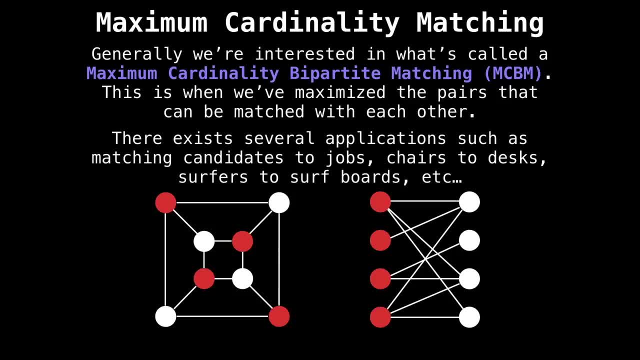 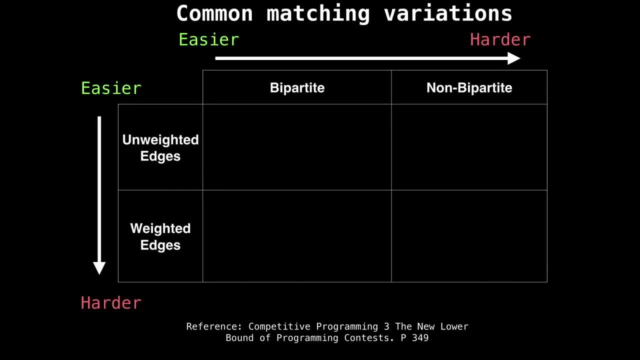 we've maximized the number of candidates that can be matched to jobs or the number of surfers to surfboards. Finding a matching is not unique to bipartite graphs, however. you can also have a matching on a non bipartite graph. This variant is a lot harder to solve and 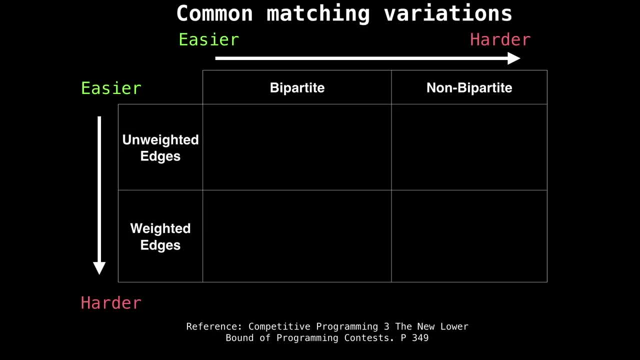 also much less common. Another variant is finding a maximum matching on a weighted graph, where you can either maximise- minimise the cost of the matching. This variant is also much harder to solve than the unweighted graph. It's also so much harder to solve than the unweighted. 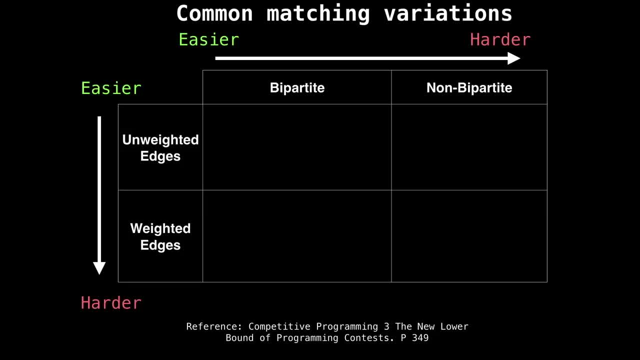 version. In the unweighted version, no edge is better in any sense than any other edge, So it makes finding a matching much, much easier. We're mostly going to focus on the top left box, which is the easiest of the four variants, but hopefully we'll get to poke around and 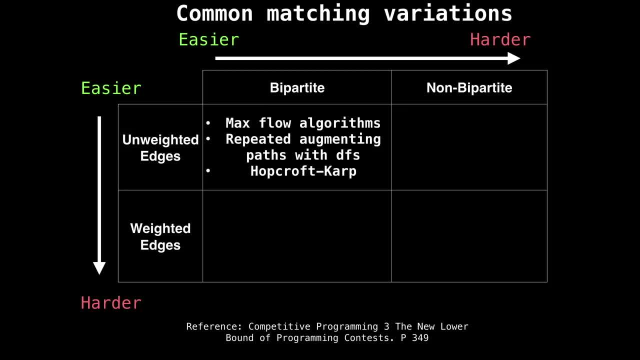 some of the other boxes as well. So if you want to find a maximum matching on an unweighted bipartite graph, you have lots of options. You can either set up the graph as a flow problem and push flow through it, which is what we'll look at in this video, But you 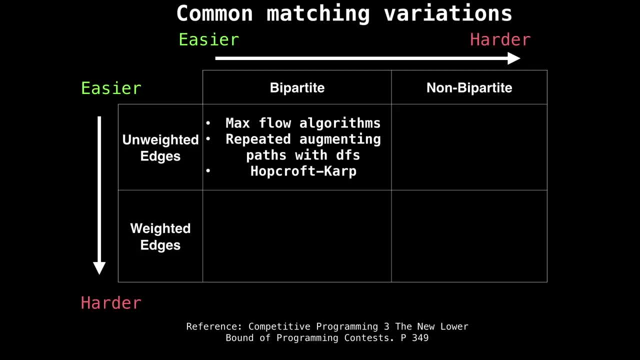 can also repeatedly find augmenting paths which maximize the matching using a depth first search, Or we can use the specialized Hopcroft CARP algorithm to do the same thing a lot faster. If your edges are weighted and your graph is still bipartite, you also 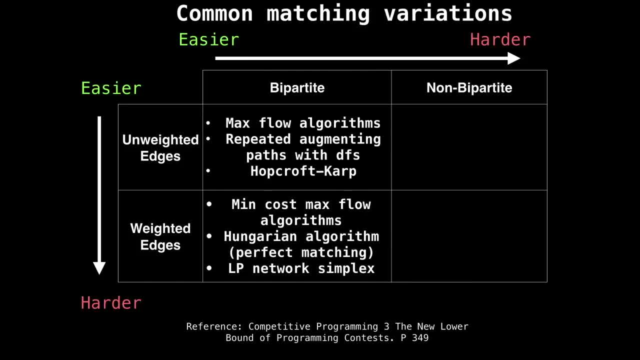 have a lot of options. You can use a min cost max flow algorithm, or you can run the Hungarian algorithm And lastly, there's the more sophisticated network simplex algorithm, which uses linear programming. If, however, your graph is not bipartite but your edges are unweighted, you can use admins blossom. 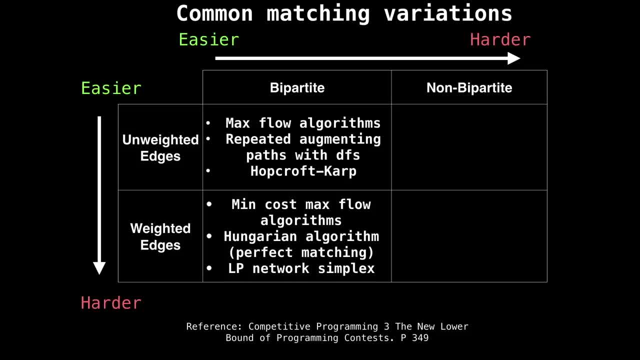 lastly, there's the more sophisticated network simplex algorithm, which uses linear programming. If, however, your graph is not bipartite but your edges are unweighted, you can use admins blossom algorithm. And lastly, the hardest of the four variants is when your graph is 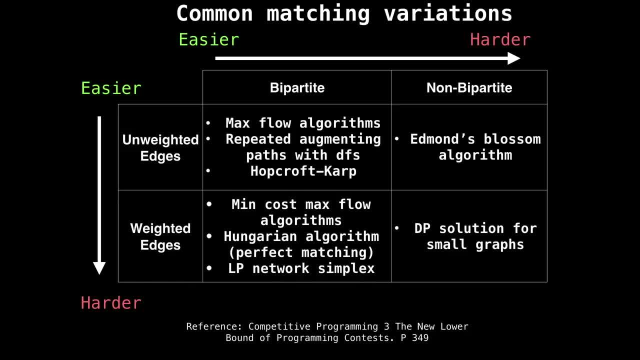 non bipartite and the edges are weighted. I didn't find much information about this one online, But the recommendation seems to be to use dynamic programming on small graphs. Now let's look at an example. This is going to be, for the unweighted bipartite case, the easiest of the four variants, So I want you. 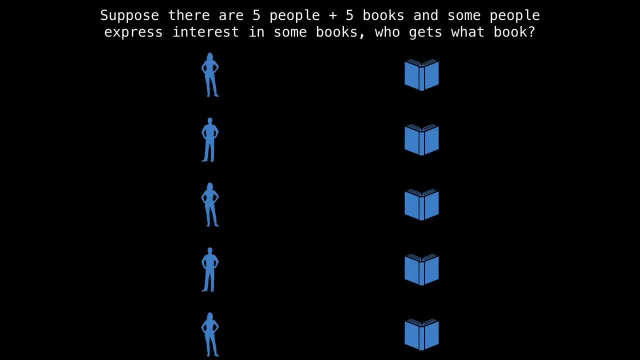 to imagine that there are five people and five books in the library and that some people express interest in some of the books. This results in a bipartite graph with people on one side and five books on the other, And then you can see that there are five people. 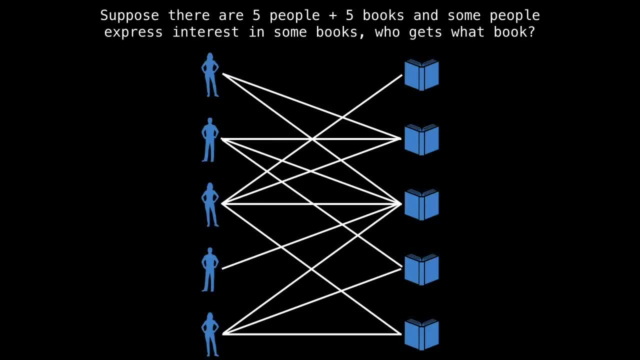 and books on the other. So far, so good. Now suppose we want to find the maximum cardinality bipartite matching, Or in other words, we want to match as many people with as many books as we can. Let's try the greedy approach to this matching problem. Let's start with. 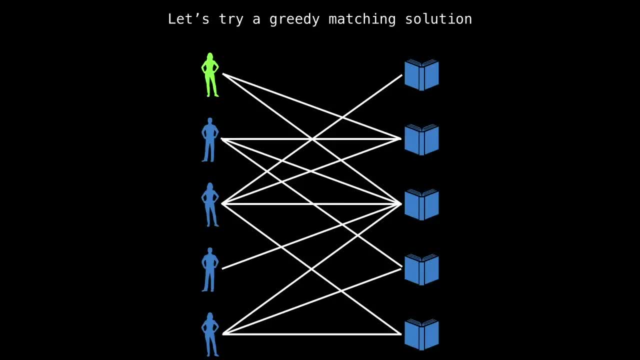 person green. Their first edge connects to the second book on the right side. The second book is unallocated, So person green is matched with what is now book green. Next up is person orange. The first book they want is the same book as person. 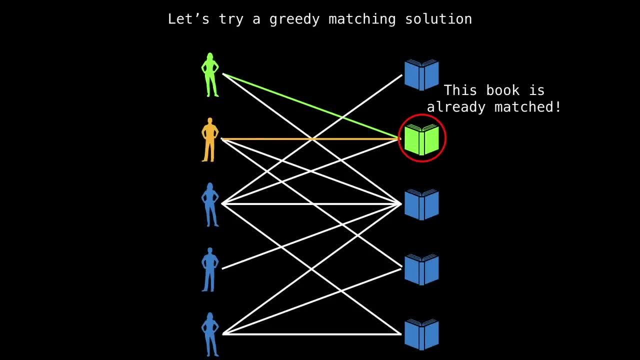 green, which is already matched, So we cannot select person greens book. Their next choice is the third book, which is unallocated, So they get matched to that one. Next up is person purple. they instantly matched to an unallocated book on the right hand side. Now person green. 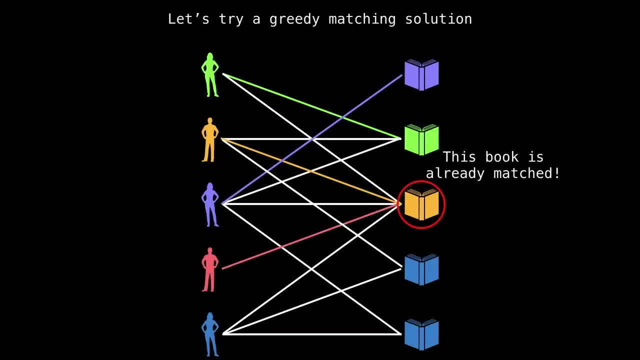 person red. red only has one edge, meaning that they're only willing to read that one book. However, that book has already been allocated to person orange, So person red cannot have it. Next up is person brown. They also want person oranges book, but they also 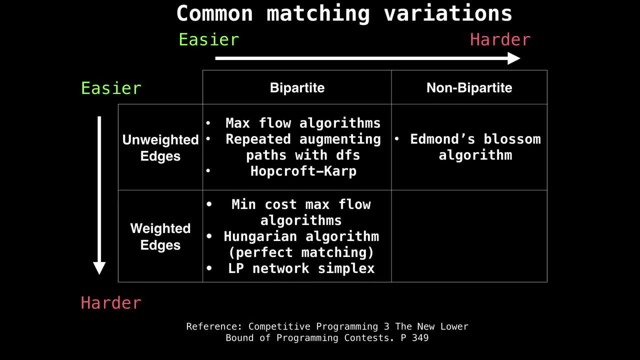 algorithm. And lastly, the hardest of the four variants is when your graph is non bipartite and the edges are weighted. I didn't find much information about this one online, But the recommendation seems to be to use dynamic programming on small graphs. Now let's look at an example. This is going to be for the unweighted bipartite. 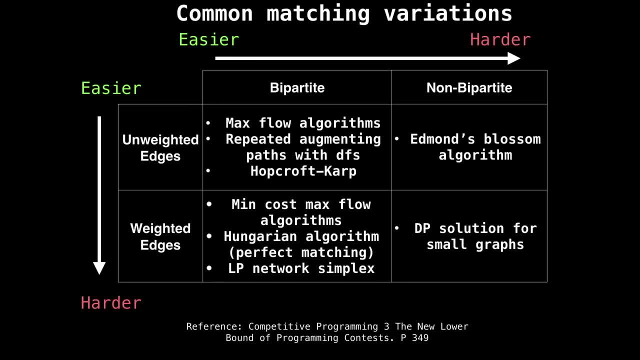 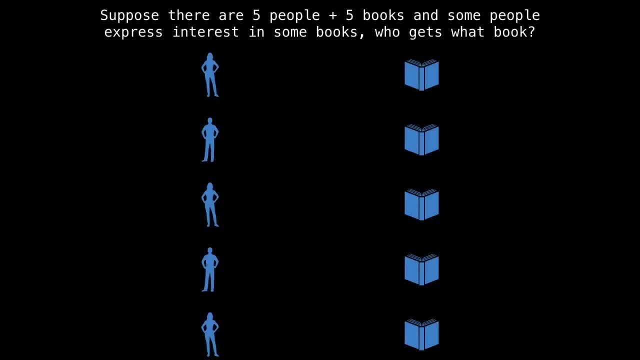 case the easiest of the four variants. So I want you to imagine that there are five people and five books in the library and that some people express interest in some of the books. This results in a bipartite graph, with people on one side and books on the other. 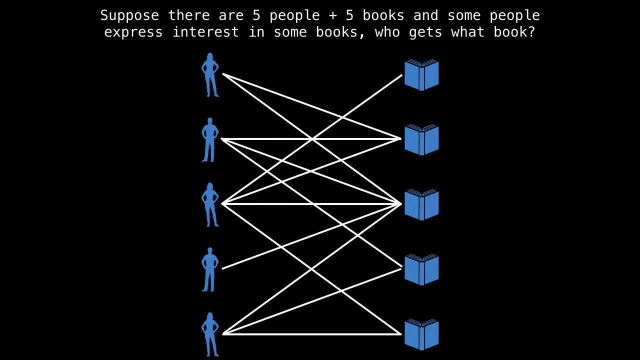 So far, so good. Now suppose we want to find the maximum cardinality bipartite matching, Or in other words, we want to match as many people with as many books as we can. Let's try the greedy approach to this matching problem. Let's start with person green Their first. 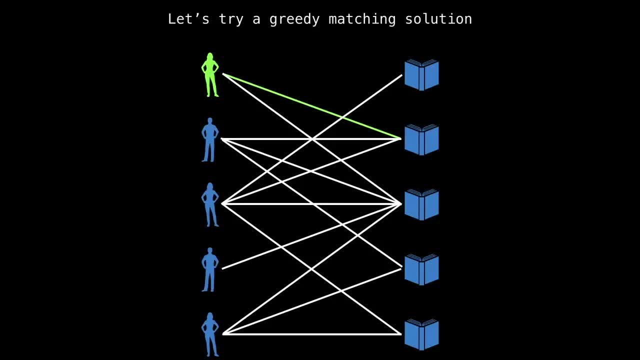 edge connects to the second book on the right side. The second book is unallocated, So person green is matched with what is now book green. So next up is person orange. The first book they want is the same book as person green, which. 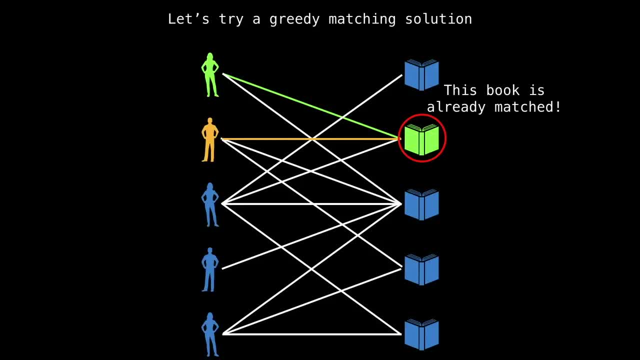 is already matched, So we cannot select person greens book. Their next choice is the third book, which is unallocated, So they get matched to that one. Next up is person purple. They instantly match to an unallocated book on the right hand side. Now person read: read only. 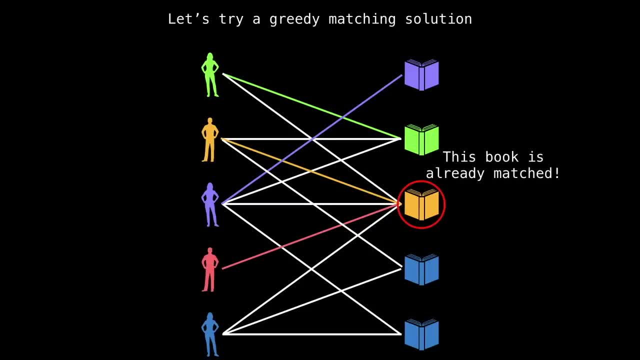 has one edge, meaning that they're only willing to read that one book. However, that book has already been allocated to person orange, so person red cannot have it. Next up is person brown. they also want person oranges book, but they also cannot have it. Fortunately. 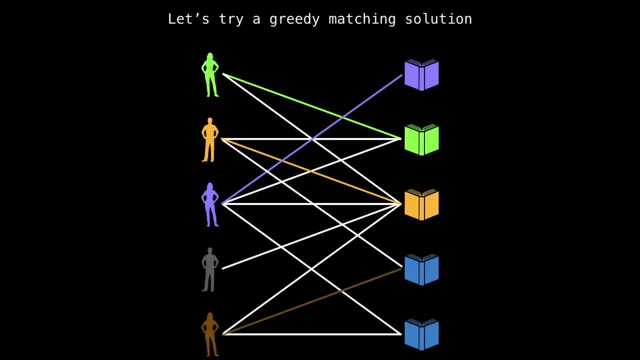 they have other options of books that are willing to read, So person brown gets one of those. So in the end, the greedy approach only found a matching of four. only four people were able to be matched with books. but can we do any better? Is this the true maximum cardinality matching? Turns out that it's not a greedy. 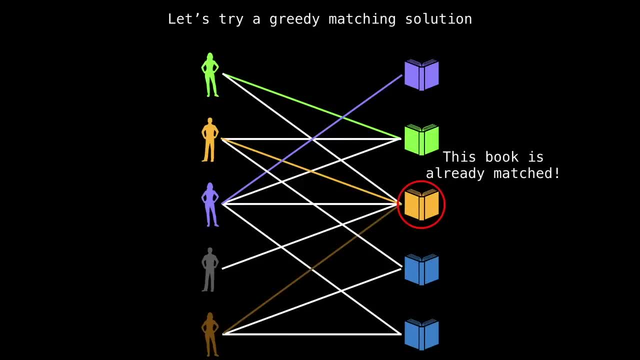 cannot have it. Fortunately they have other options of books they're willing to read, So person brown gets one of those. So in the end, the greedy approach only found a matching of four. only four people were able to be matched with books. But can we do any better? Is this the true maximum cardinality? matching Turns out. 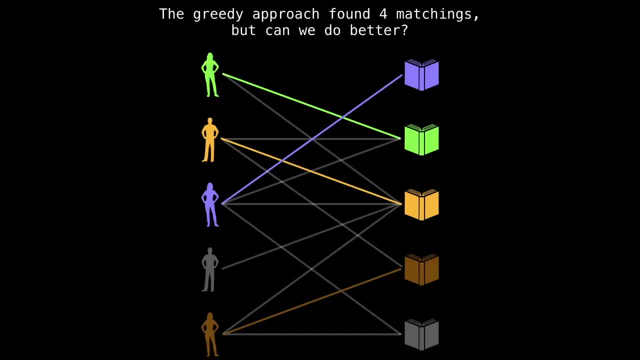 that it's not a greedy approach to the maximum matching problem will not work, as we just saw. we need a more sophisticated approach to ensure that we are able to get that maximum matching. So we're going to solve this problem, This maximum matching problem, by turning our problem into a network flow problem and finding 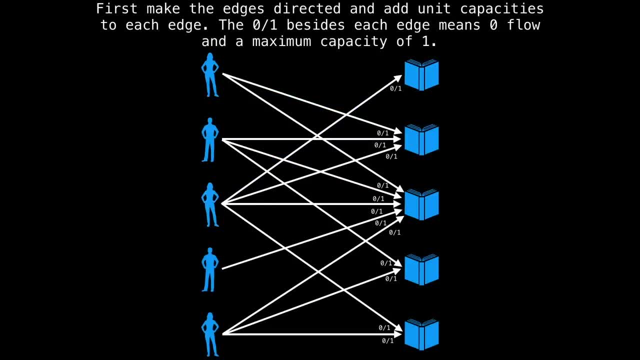 the max flow. The first thing we're going to do is make every edge directed and add one unit capacity to each edge. The zero slash one besides each edge means zero flow and a maximum capacity of one. Next, we're going to introduce two new nodes. 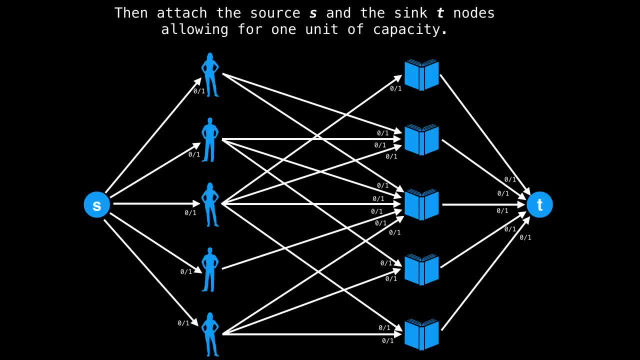 We're going to call them the source and the sink- and hook up edges outwards, from the source to the people, with a capacity of one, and hook up edges from books to the sink, Also with a capacity of one. Once that's all set up, use any max flow algorithm to push flow through the network. What? 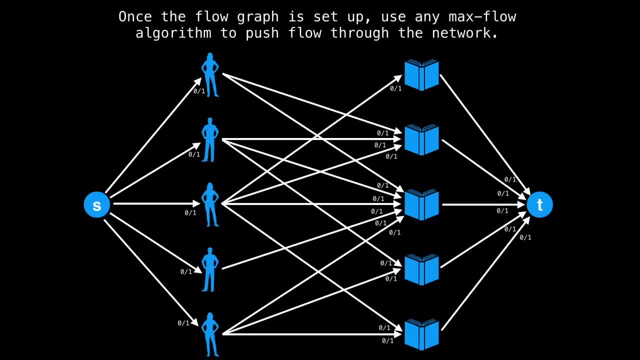 this will do is show us what edges get populated with flow. with that information, we will be able to reconstruct the maximum matching. So we're going to create a new node, and we're going to create a new node, which is going to be. Here's a graph after the flow algorithm has ran. you can see that some of the edges have. 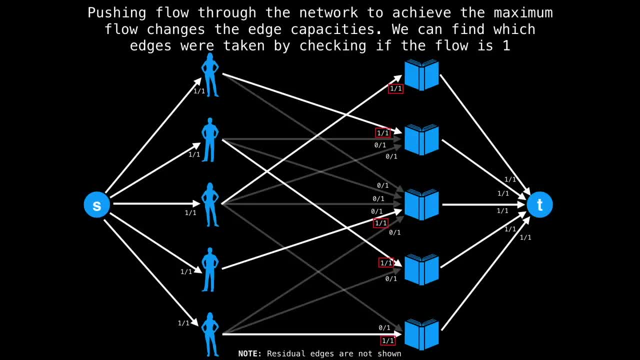 one unit of flow. Those were the edges selected by the max flow algorithm. The most interesting edges are the middle edges with one unit of flow. These are the edges which form the maximum cardinality matching. If we color in the middle edges, which have one unit of flow, you can: 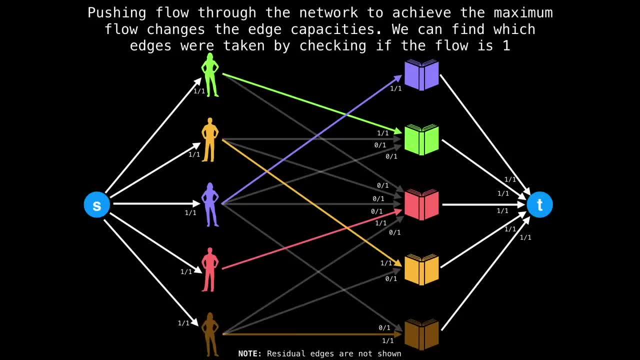 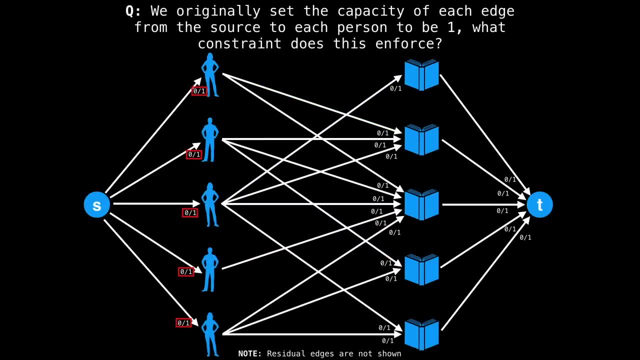 see that this time everybody goes home with a book and no one is left empty handed. Okay, so now we understand how this basic setup works and how it leads to a matching. Let's play around with this model a little bit to truly understand what all the weights here. 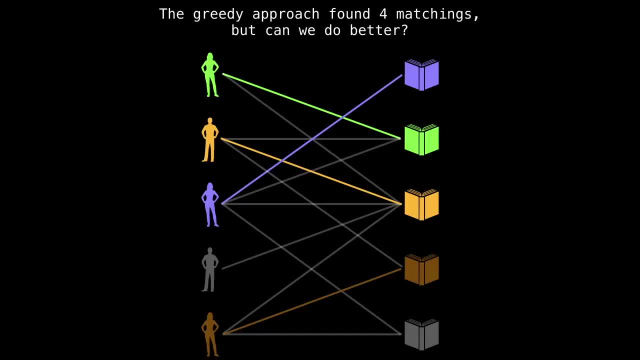 approach to the maximum matching problem will not work, As we just saw. we need a more sophisticated approach to ensure that we are able to get that maximum matching. So we're going to solve this maximum matching problem by turning our problem into a network flow problem and finding 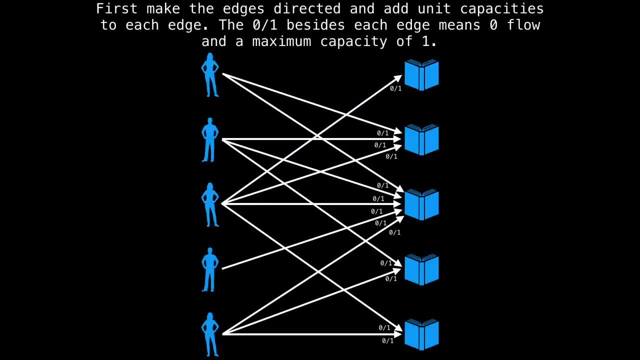 the max flow. The first thing we're going to do is make every edge directed and add one unit capacity to each edge. The zero slash one besides each edge means zero flow and a maximum capacity of one. Next, we're going to introduce two new nodes. 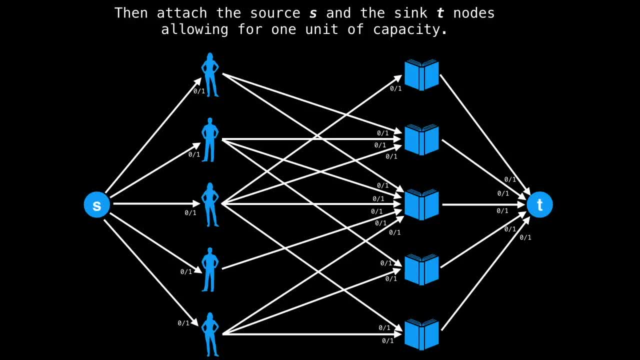 So we're going to call them the zero slash one and the maximum matching problem And we're going to call them the source and the sink and hook up edges outwards from the source to the people with a capacity of one, and hook up edges from books to the sink, also with 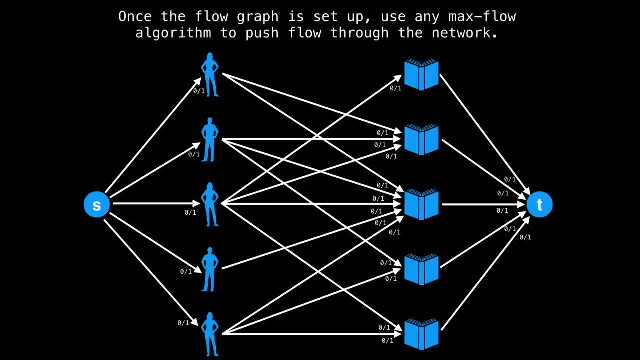 a capacity of one. Once that's all set up, use any max flow algorithm to push flow through the network. What this will do is show us what edges get populated with flow. With that information, we will be able to reconstruct the maximum matching problem. 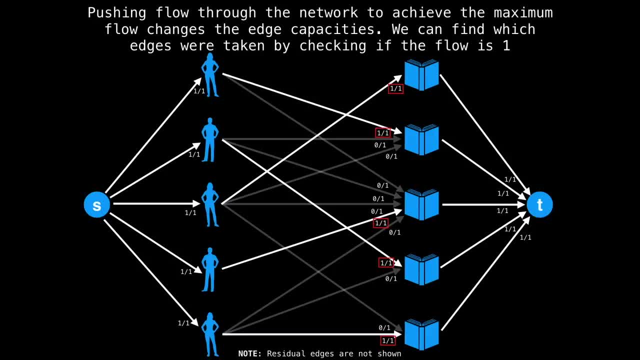 Here's a graph after the flow algorithm has ran. you can see that some of the edges have one unit of flow. Those were the edges selected by the max flow algorithm. The most interesting edges are the middle edges with one unit of flow. These are the edges which form the maximum. 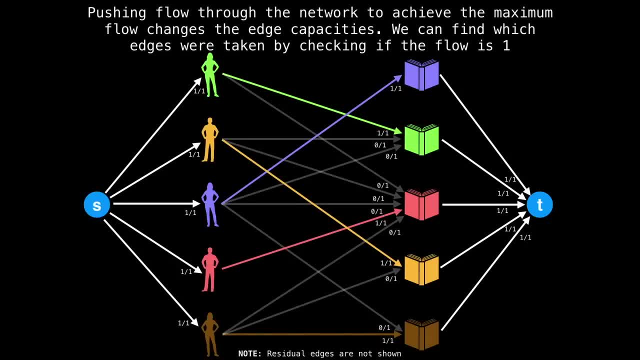 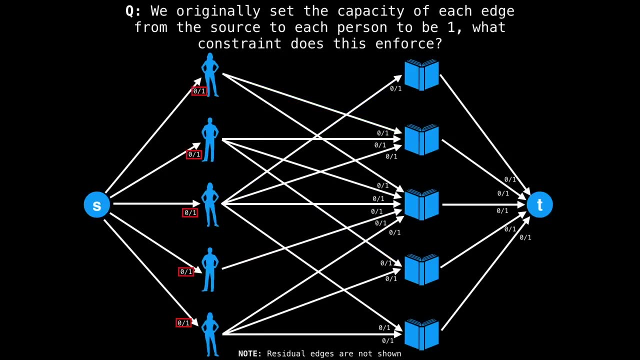 cardinality matching. If we color in the middle edges, which have one unit of flow, you can see that this time everybody goes home With a book and no one is left empty handed. Okay, so now we understand how this basic setup works and how it leads to a matching. Let's play around with this model a little. 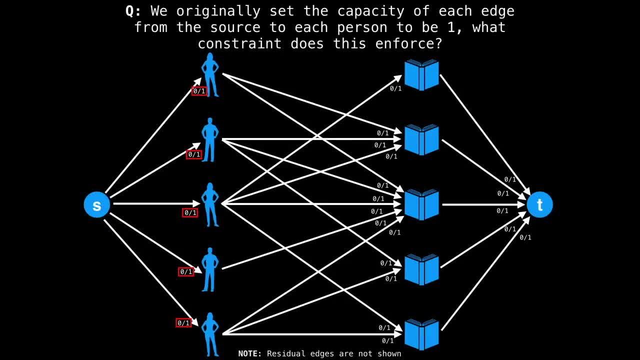 bit to truly understand what all the weights here mean. We originally set the capacity of each edge from the source to each person to be one, But what constraint is that really enforcing? I'll let you pause the video and think about that for a second, because it's 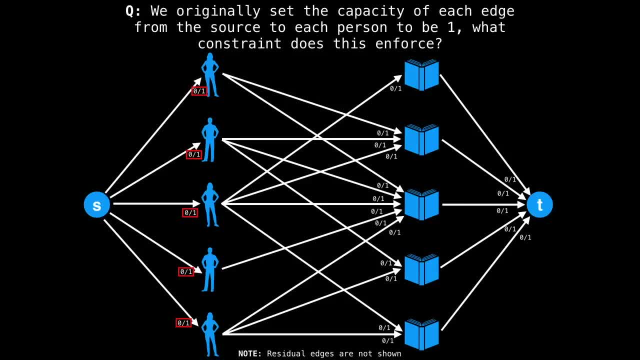 mean We originally set the capacity of each edge from the source to each person to be one, But what constraint is that really enforcing? I'll let you pause the video for a moment and think about that for a second, because it's so important. The answer is that that. 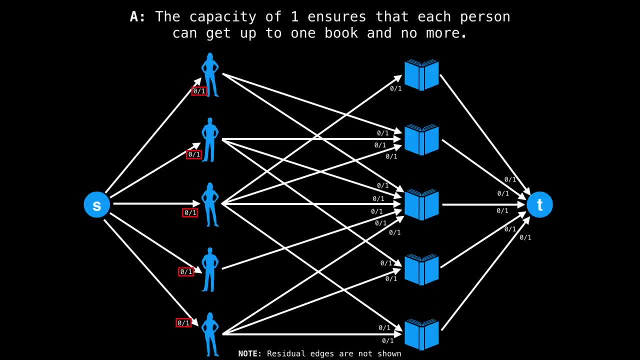 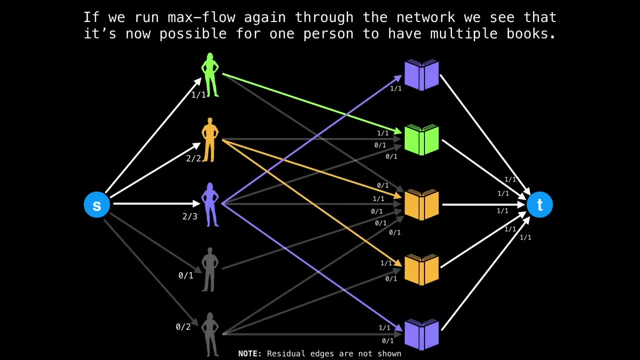 capacity of one ensures that each person can get up to one book and no more. if we increase this number for some people, we can allow them to possibly pick up more than one book. If we rerun the max flow algorithm through this network, we see that it's now possible. 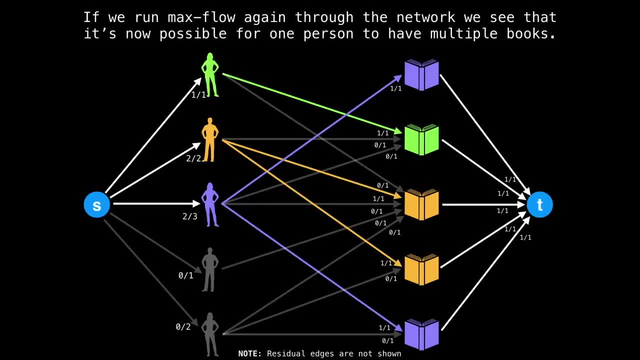 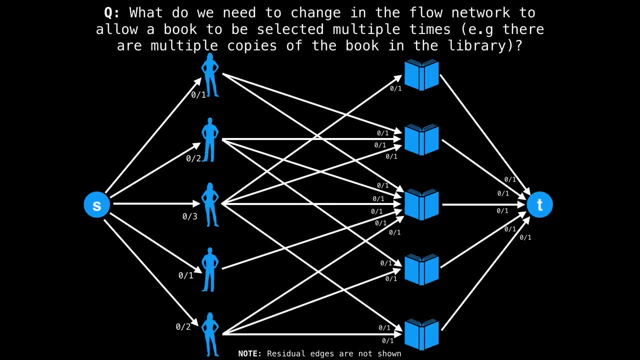 for max diversions to be transferred to the other side of the exists, as well as flow for one person to be matched with multiple books. The next thing we want to do is change the flow network to allow a book to be selected multiple times. pause the video and think. 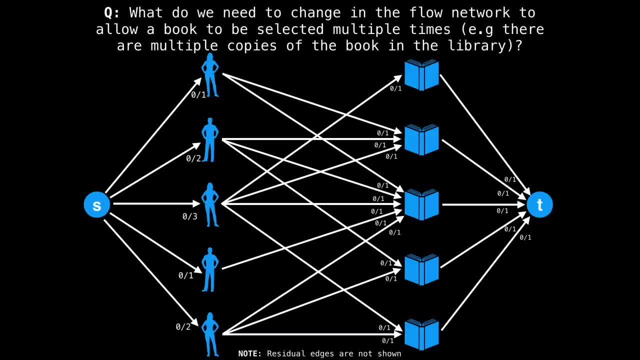 about how we can modify this flow graph to support having multiple copies of the same book in the library. I'll give you a short moment. The number of copies of a book is controlled by the capacity of the edges leading to the sink t. Increasing this value will. 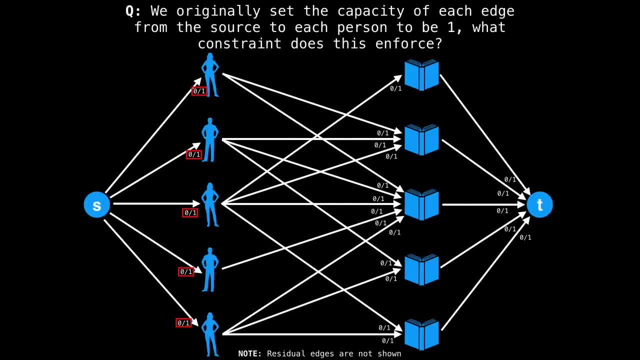 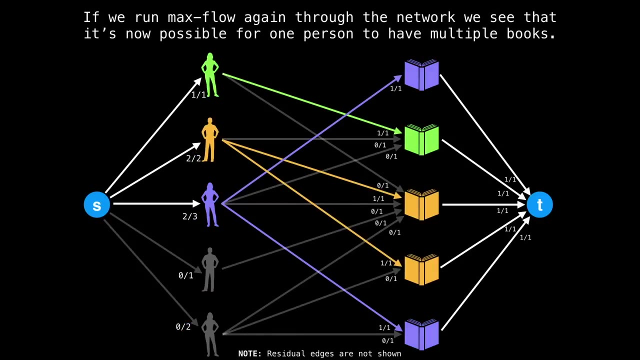 so important? The answer is that that capacity of one ensures that each person can get up to one book and no more. If we increase this number for some people, we can allow them to possibly pick up more than one book. If we rerun the max flow algorithm through this network, we see. 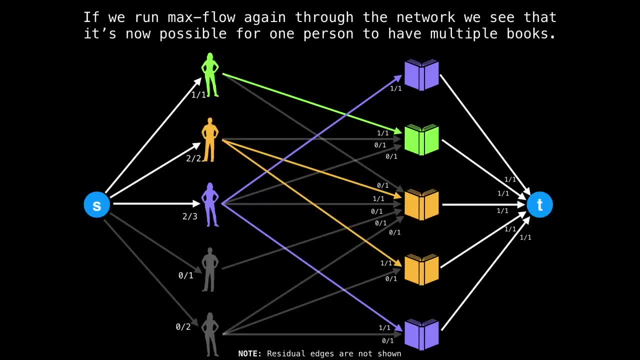 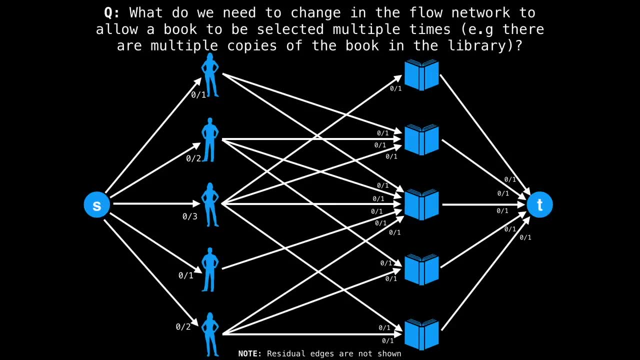 that it's now possible for one person to be matched with multiple books. The next thing we want to do is change the flow network to allow a book to be selected multiple times. pause the video and think about how we can modify this flow graph to. 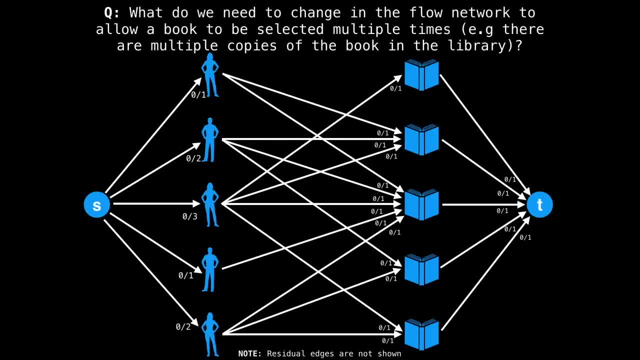 support having multiple copies of the same book in the library. I'll give you a short moment. The number of copies of a book is controlled by the capacity of each person to pick up one book. The next thing we want to do is change the flow network to allow a book to be selected. 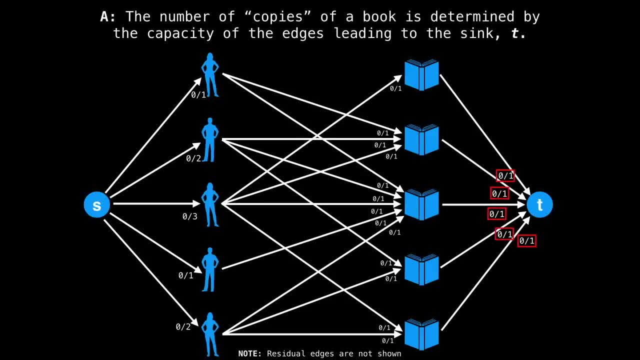 multiple times. Pause the video and think about how we can modify this flow graph to support having multiple copies of the same book, because currying pullback to the book is really important. What we're doing is we're allowing the urc that. oh right, there are three characters. 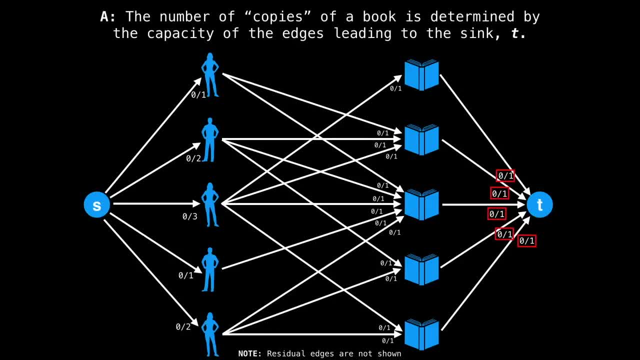 called the text. there mean reads the text. it in continuous paper in there, in there, and it's been horrifying. anddadえば read the text little higher. finally we have that paper that the text is display certain characters. The third thing we want to get rid of is the capacity of the edges leading to the sink. 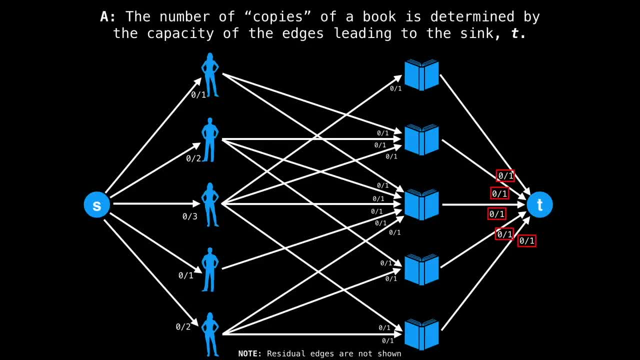 t. increasing This value will allow more flow to run through those designated edges. This effectively limits or controls the number of copies of a book. let's change the capacity of those edges leading into the sink to allow having multiple copies of the same book and 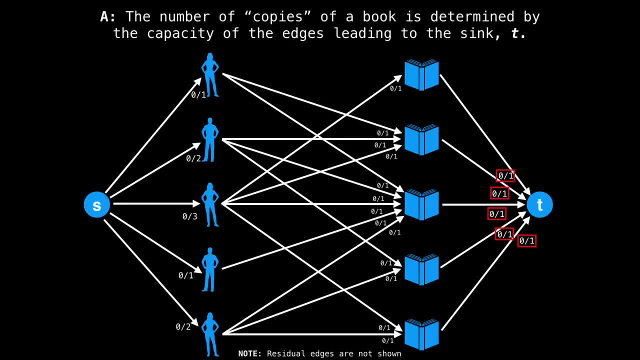 allow more flow to run through those designated edges. This effectively limits or controls the number of copies of a book. let's change the capacity of those edges leading into the sink. The number of copies of a book is controlled by the capacity of the edges leading to the 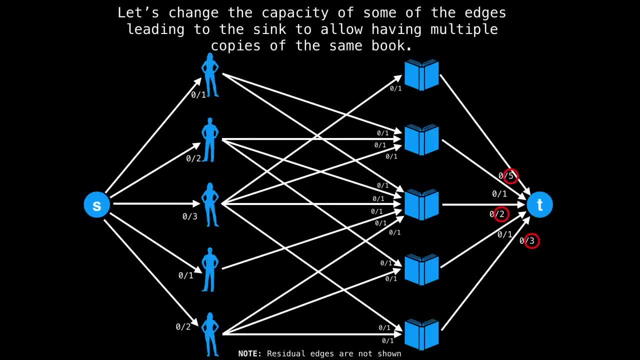 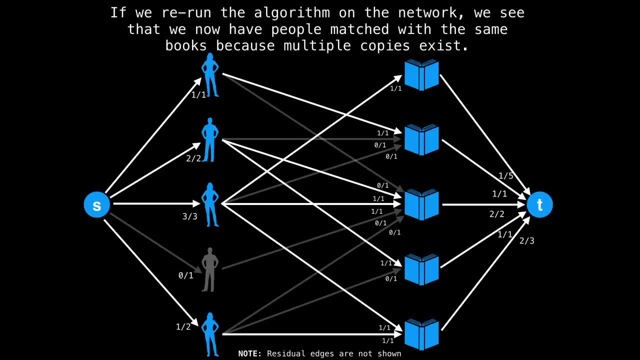 sink to allow having multiple copies of the same book and see what happens. If we rerun the max flow algorithm once again through the network, we see that we now have people matched with the same book multiple times because multiple copies exist, For example. 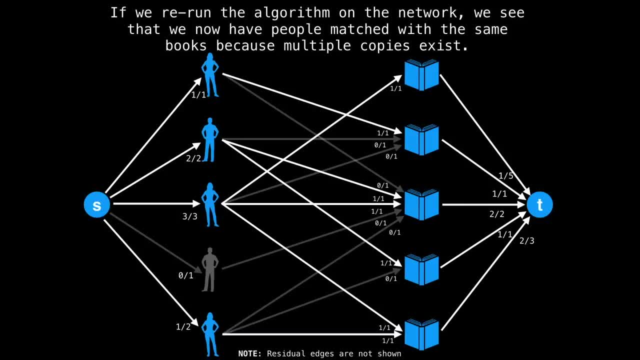 book three and book five both have two people grabbing a copy of them. the actual assignment of people to books would be as follows. I'll let the animation play After the flow algorithm has ran, if you want to know how many copies of each book were. 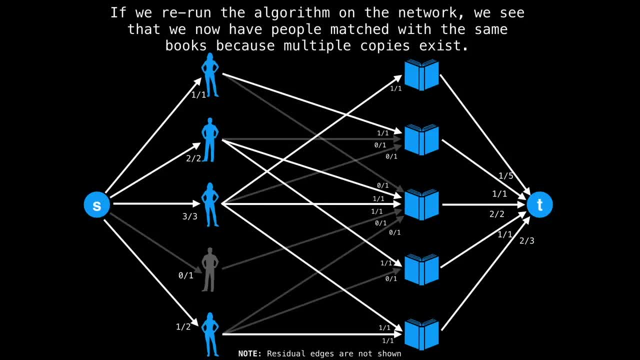 see what happens If we rerun the max flow algorithm once again. through the network work, we see that we now have people matched with the same book multiple times because multiple copies exist. For example, book three and book five. both have two people grabbing. 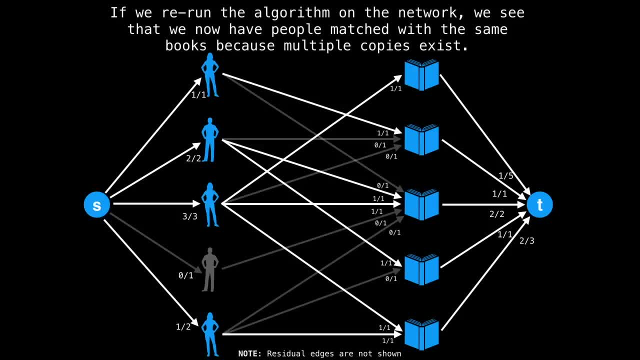 a copy of them. the actual assignment of people to books would be as follows. I'll let the animation play After the flow algorithm has ran. if you want to know how many copies of each book were actually given out, you can inspect the flow value on the edge leading. 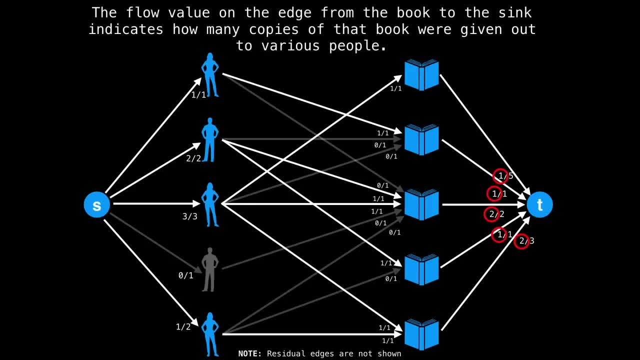 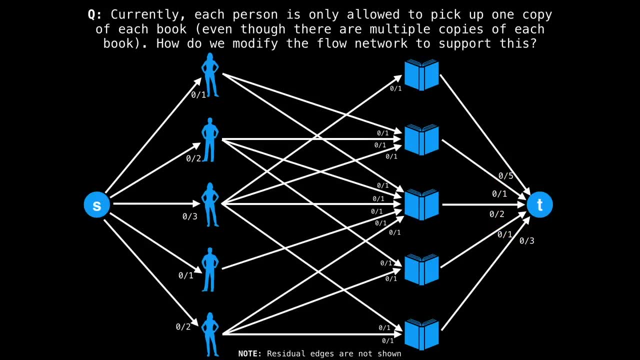 actually given out. you can inspect the flow value on the edge leading to the sink. Currently, each person is only allowed to pick up one copy of each book, even though there are multiple copies of each book, how can we modify the flow network to support this? Let's first 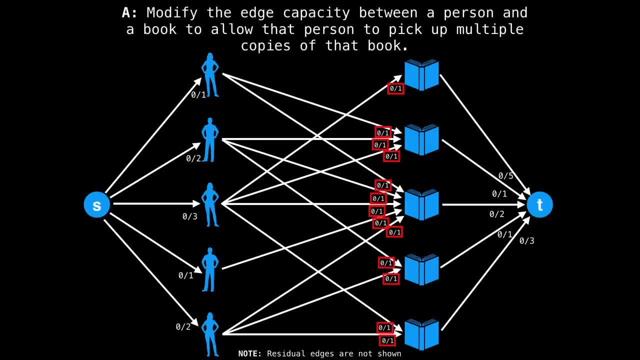 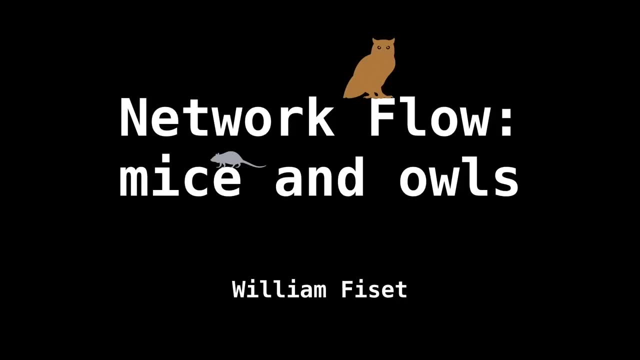 look at this. You've guessed it. we need to modify the edge capacity between a person and the book to allow that person to pick up multiple copies of that book. Today we're going to look at how to use network flow to actually solve a useful problem- The problem. 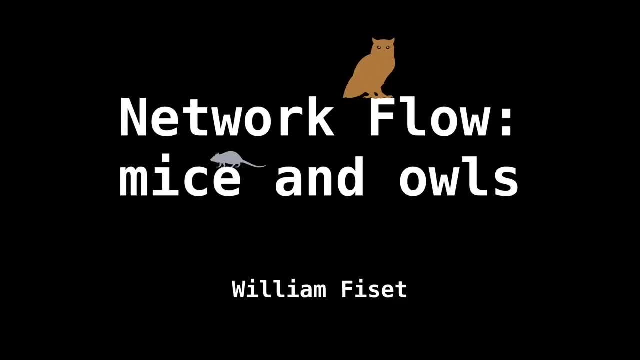 we're going to tackle is what I call the mice and owls problem, which is a slightly harder variation of another competitive programming problem Which I'll link in the description. I love this problem because of its simple and elegant solution, but also its realistic real world application. Let's have a look, Suppose, there. 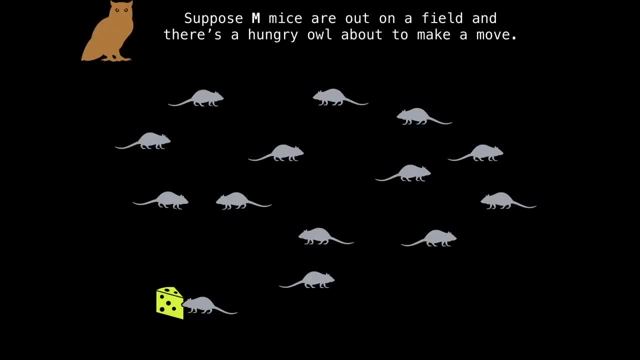 are m mice out on a field and there's a hungry owl about to make a move. Assume that the owl can reach every single one of these mice. Further, suppose that there are H holes scattered across the ground and that each hole has a certain capacity for the number of mice. 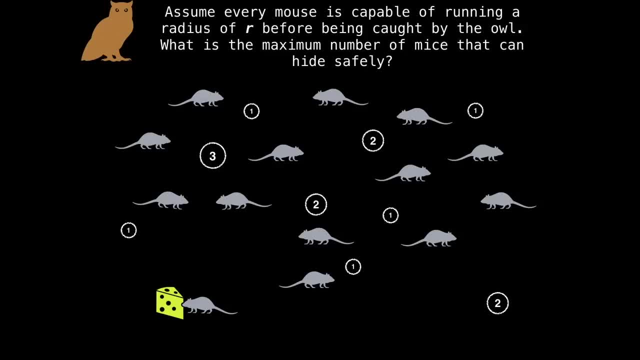 that can hide in it. We also happen to know that every mouse is capable of running a distance of R in any direction before being caught by the owl. The question asks: what is the maximum number of mice that can hide safely before being caught? If you want to give this, 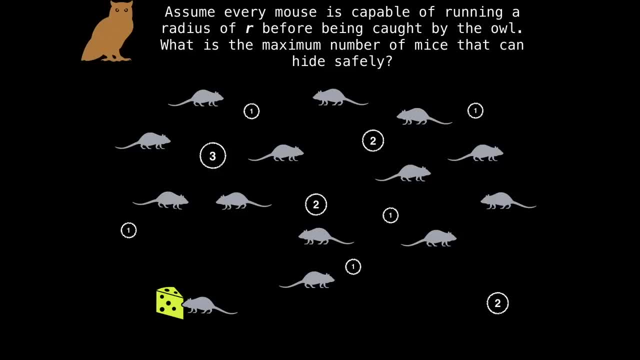 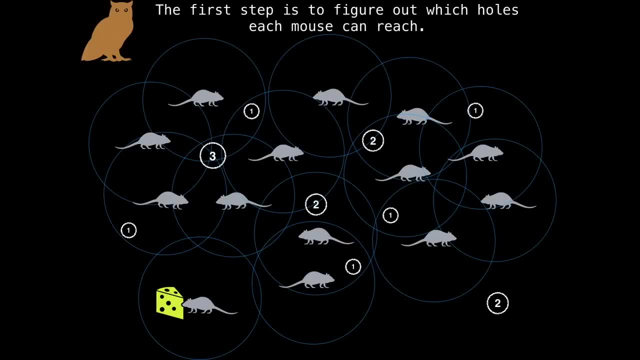 problem a try. now's a good time to pause the video and try and write some code. The first step is to figure out which holes each mouse can reach. Visualize this by drawing a radius of R around each mouse And if inside the radius there's. 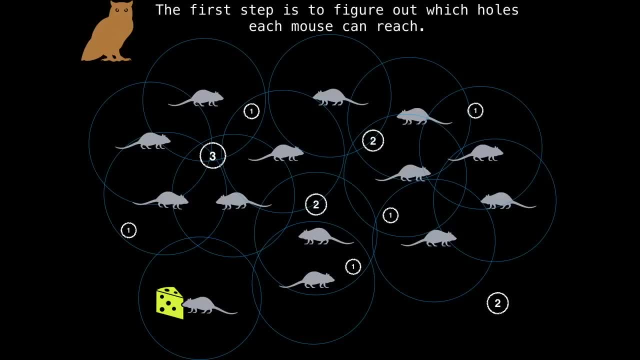 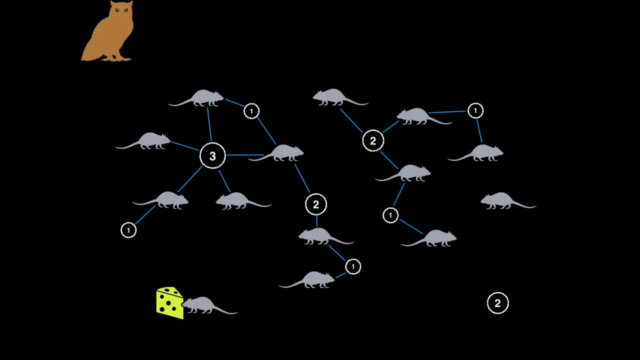 a hole or the circle touches a hole, we'll assume that the mouse can make it to the hole safely. So if we draw an edge between a mouse and a hole, if the mouse can make it to that hole, we get the following graph: The next step is to actually match mice to holes, to 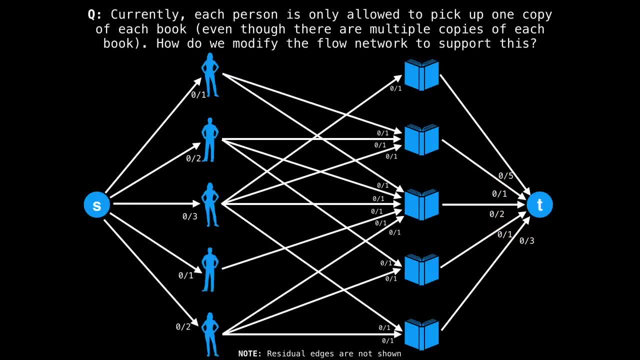 to the sink. Currently, each person is only allowed to pick up one copy of each book. even though there are multiple copies of each book, how can we modify the flow network to support this? You've guessed it: we need to modify the edge capacity between a person. 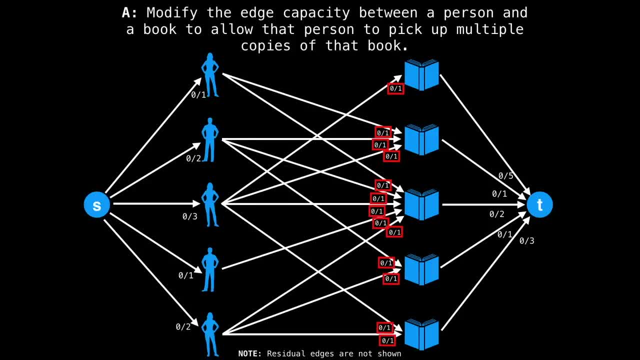 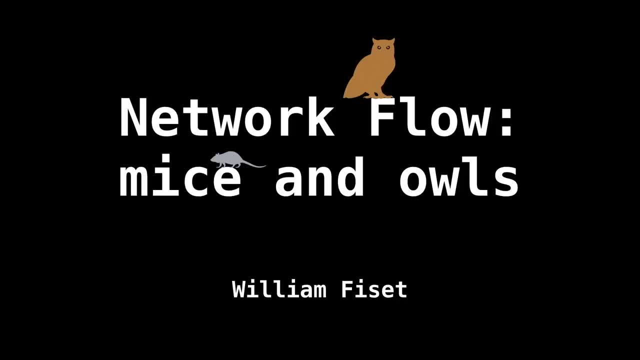 and the book to allow that person to pick up multiple copies of that book. Today we're going to look at how to use network flow to actually solve a useful problem. The problem we're going to tackle is what I call the mice and owls problem, which is a slightly harder 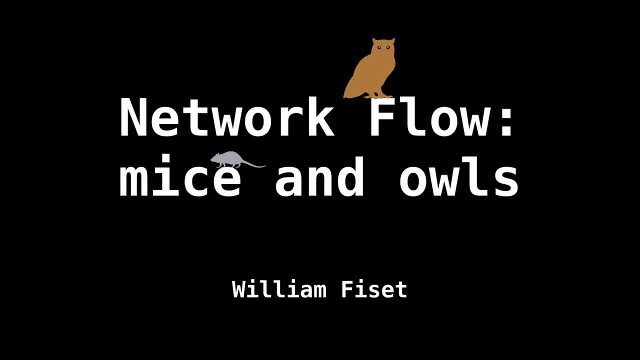 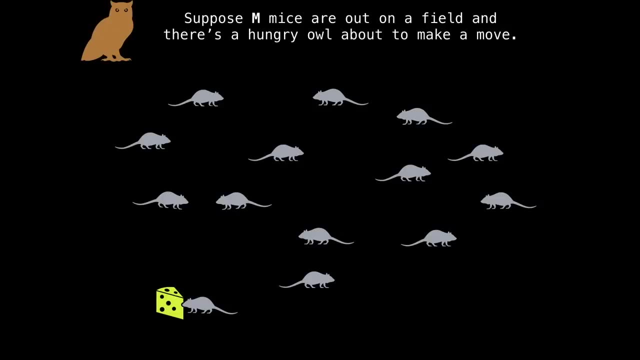 variation of another competitive program. I love this problem because of its simple and elegant solution, but also its realistic real world application. Let's have a look. Suppose there are M mice out on a field and there's a hungry owl about to make a move. Assume that the owl can reach every single. 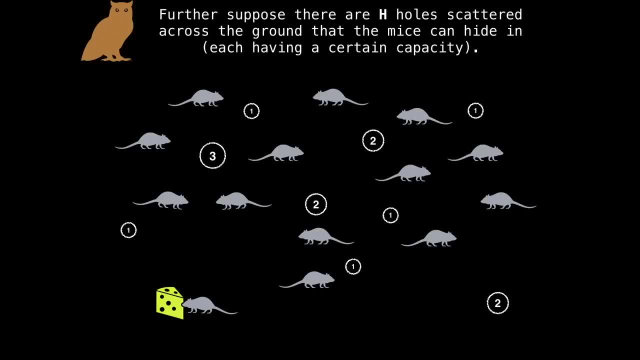 one of these mice Further suppose that there are H holes scattered across the ground and that each hole has a certain capacity for the mouse to reach. If the mouse reaches the mouse, the number of mice that can hide in it. We also happen to know that every mouse 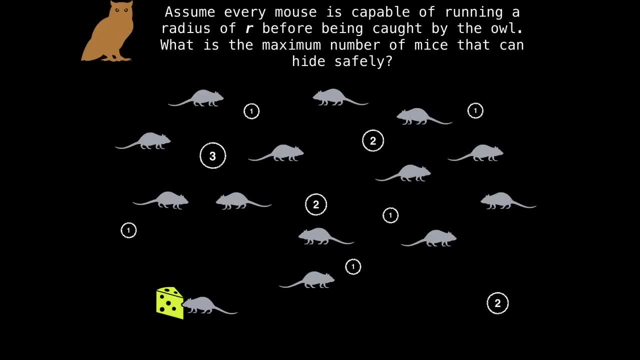 is capable of running a distance of R in any direction before being caught by the owl. The question asks: what is the maximum number of mice that can hide safely before being caught? If you want to give this problem a try, now's a good time to pause the video. 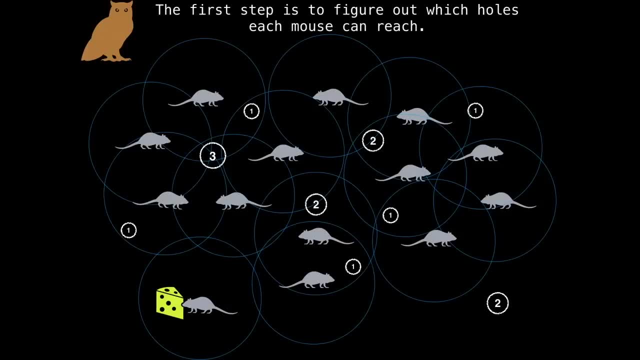 and try and write some code. The first step is to figure out which holes each mouse can reach. visualize this by drawing a radius of R around each mouse And if inside the radius there's a hole or the circle touches a hole, we'll assume that the mouse can make. 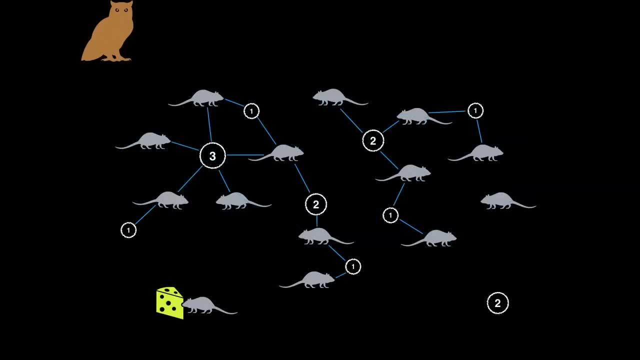 it to the hole safely. So if we draw an edge between a mouse and a hole, if the mouse can make it to that hole, we get the following graph: The next step is to actually match mice to holes to maximize the overall safety of the group. 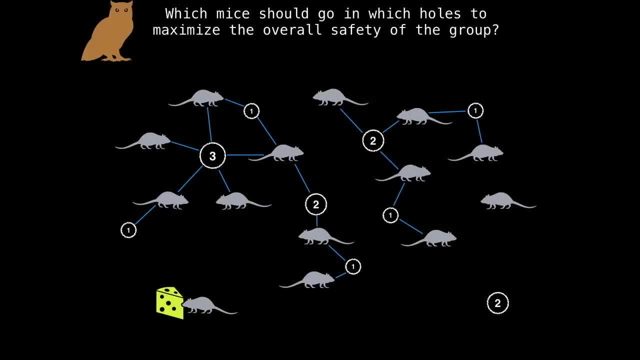 By doing this, we can actually make the mouse safe. By doing this, we can actually make the mouse safe. By doing a simple, quick inspection. it's clear that not every mouse should be matched to any hole. For example, this orange mouse should probably not try and run to the. 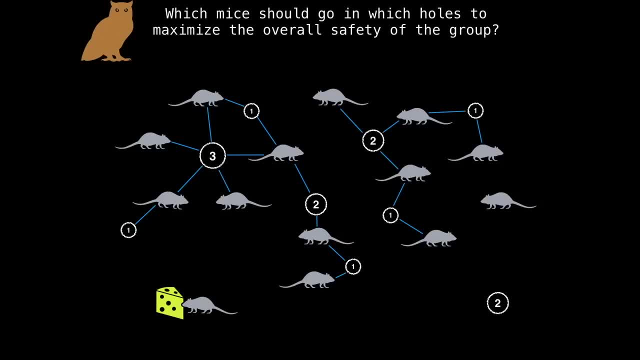 maximize the overall safety of the group By doing a simple, quick inspection. it's clear that not every mouse should be matched to any hole. For example, this orange mouse should probably not try and run to the hole with a capacity of three because it's the only mouse that can reach the hole behind it with a capacity. 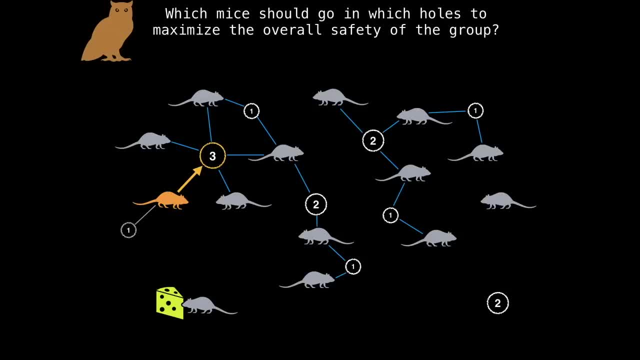 of one. Making any bad decision like this has the chance to jeopardize the maximum number of overall mice that can hide safely. The key realization with this problem is that the mouse should not be able to run to the hole with a capacity of three, because it's 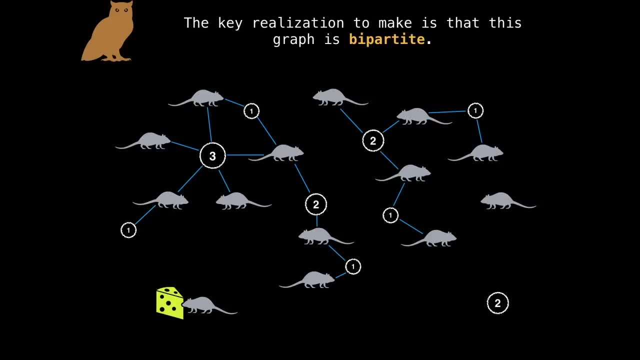 unnecessary to maximize the overall safety of the group, Because it needs to have the maximum number of overall numbers to be stimulated. In other words, thegiess 이거를vote. step t comes first, The mouse over liberté comes next, And then the mouse over liberté is. 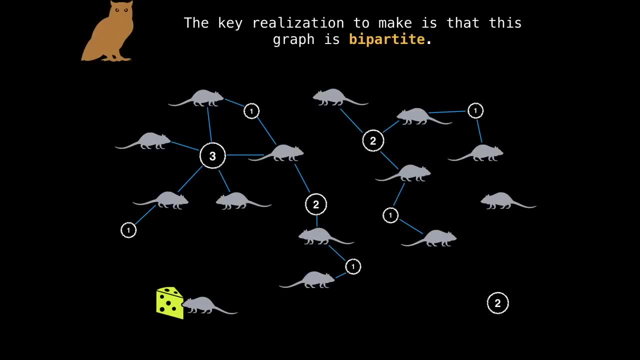 actaully called the mouse over liberté, is that the Architect is actually bipartite, And once we know that, it actually becomes a much simpler problem because we can set up a flow graph and run a maximum flow algorithm to maximize the overall number of mice which 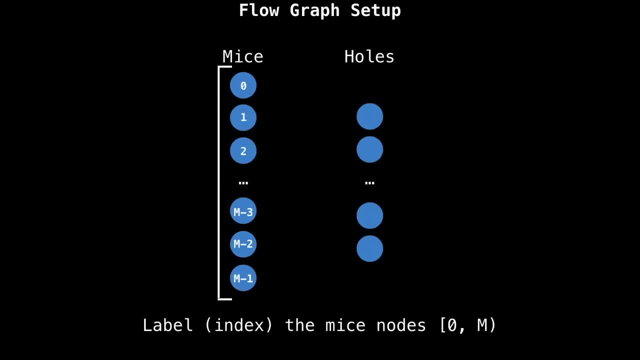 can hide safely. Here's the steps I would do to set up the flow graph and run a max flow. First I would create M mice nodes labeled zero through m minus one inclusive, then on. On the other side, I would create h nodes, each representing a hole. I would label or. 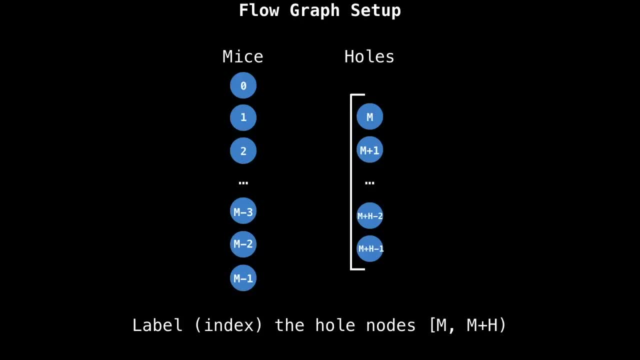 index these nodes from m to m plus h minus one inclusive, to give them a different ID than the mouse nodes. then I would place an edge with a capacity of one between the mouse and the hole, If the mouse can reach that particular hole in time. After that I would. 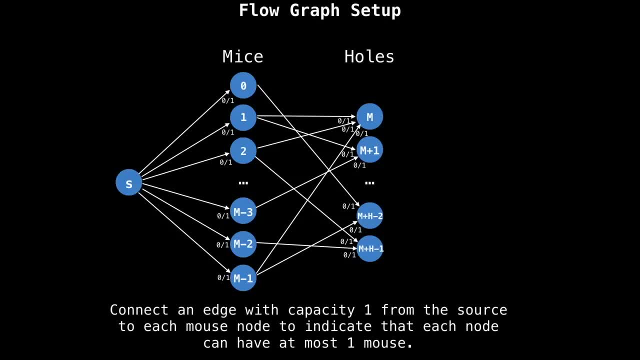 connect an edge with a capacity of one from the source to each mouse, to indicate that each node can have at most one mouse, and lastly, connect an edge from each hole node to the sink node with the capacity of the hole. The problem has now been transformed into a maximum. 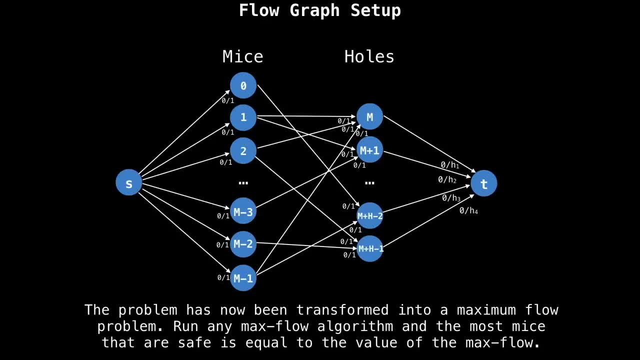 flow problem. we can run any maximum flow algorithm to get the maximum number of mice that can be safe. This is really neat And it's worth looking at some source code to really understand how to run this. Now this setup works Alright. here we are in the source code I've laid out some instructions. 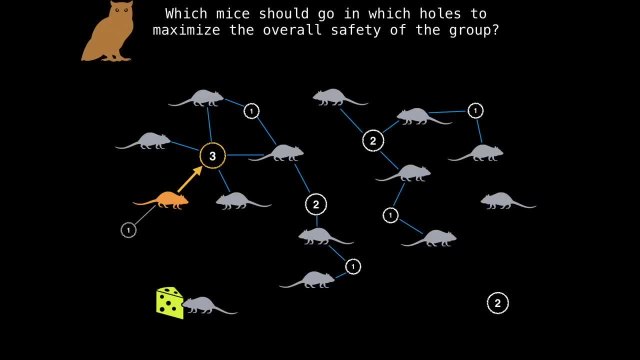 hole with a capacity of three, because it's the only mouse that can reach the hole behind it with a capacity of one. Making any bad decision like this has the chance to jeopardize the maximum number of overall mice that can hide safely The key realization with this. 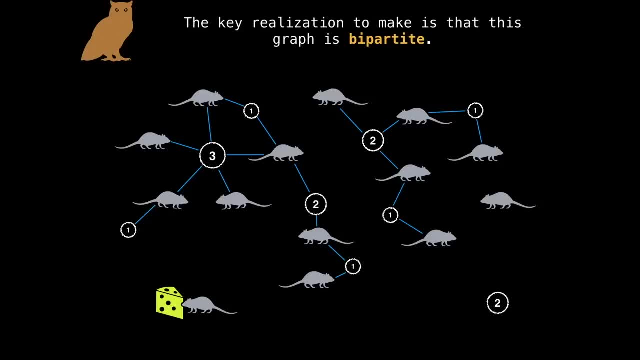 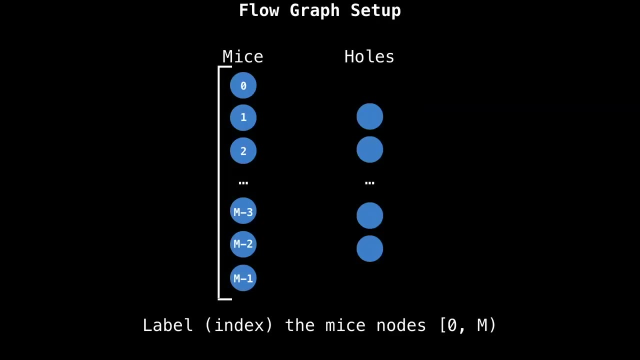 problem is that the graph is actually bipartite, And once we know that, it actually becomes a much simpler problem because we can set up a flow graph and run a maximum flow algorithm to maximize the overall number of mice which can hide safely. Here are the steps I would. 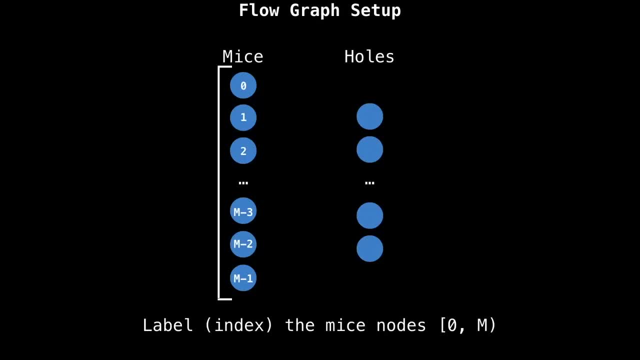 do to set up the flow graph and run a max flow. First I would create m mice nodes labeled zero through m minus one inclusive. Then, on the other side, I would set up a flow graph and I would create h nodes, each representing a hole. I would label or index these nodes. 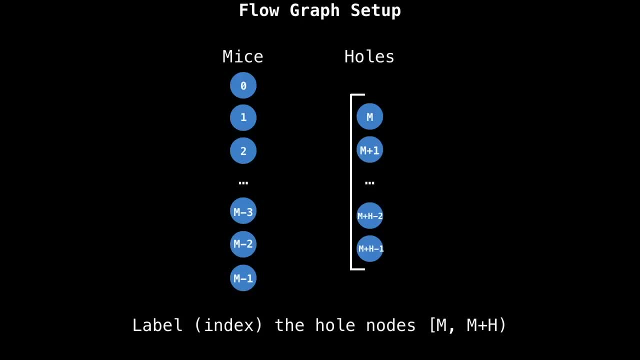 from m to m plus h, minus one inclusive, to give them a different ID than the mouse nodes. Then I would place an edge with a capacity of one between the mouse and the hole, If the mouse can reach that particular hole in time. After that I would connect an edge. 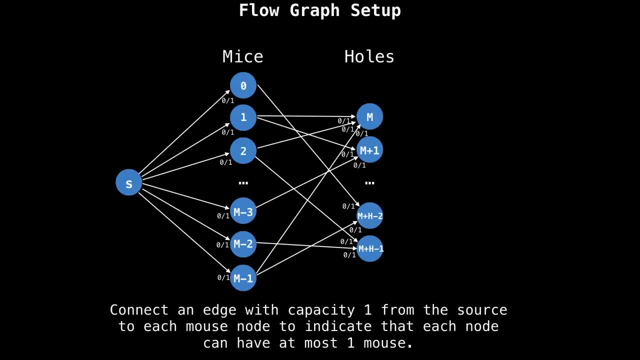 with a capacity of one from the source to each mouse To indicate that the mouse is able to reach that particular hole in time. After that, I would connect an edge with a capacity of one from the source to each mouse to indicate that each node can have at most one mouse And, lastly, connect an edge from each hole node. 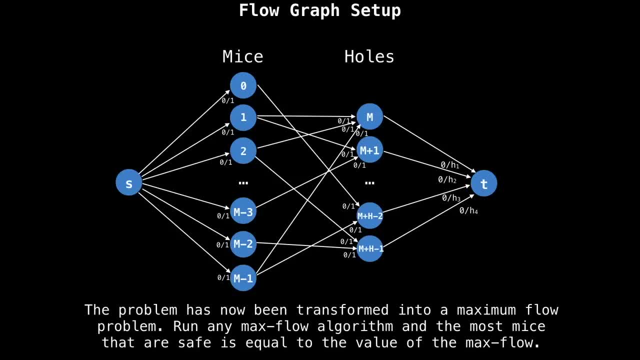 to the sink node with the capacity of the hole. The problem has now been transformed into a maximum flow problem. we can run any maximum flow algorithm to get the maximum number of mice that can be safe. This is really neat And it's worth looking at some source. 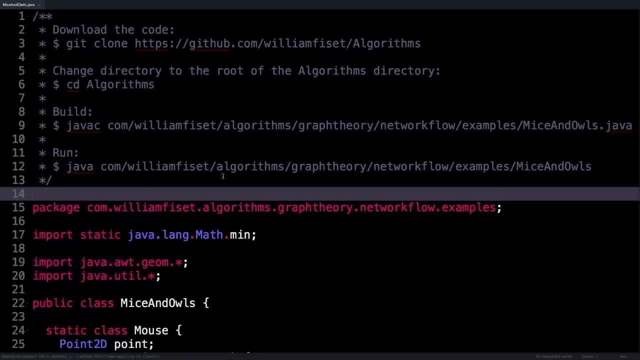 code to really understand how this setup works. Alright, here we are. in the source code, I've laid out some instructions for how to set up a maximum flow algorithm. First, I'm going to show you some instructions on the top here, in case you wanted to download the code and 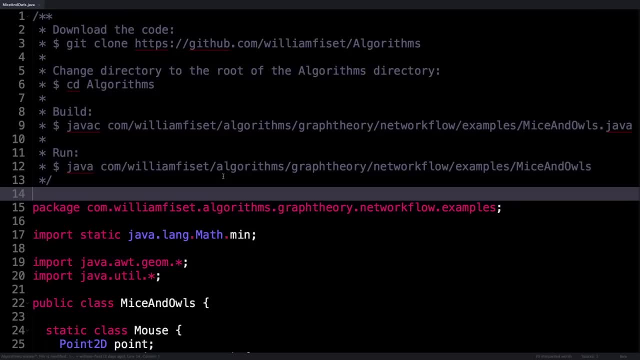 actually play around with it on your machine. This program also uses the Ford Fulkerson flow solver we saw two videos ago, So I highly recommend you go and watch that video before continuing. I'll link to it in the description below just in case you haven't seen it So. 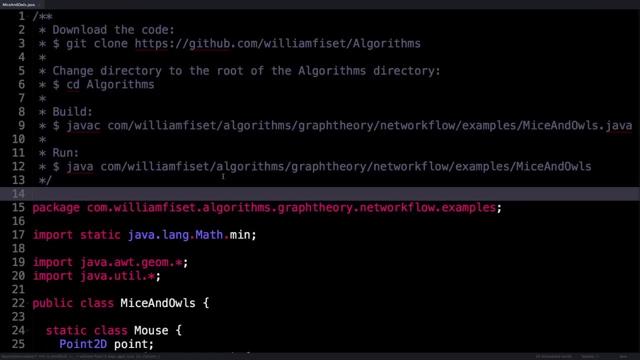 on the top here in case you wanted to download the code and actually play around with it on your machine. This program also uses the Ford Fulkerson flow solver. we saw two videos ago, So I highly recommend you go and watch that video before continuing a link to it. 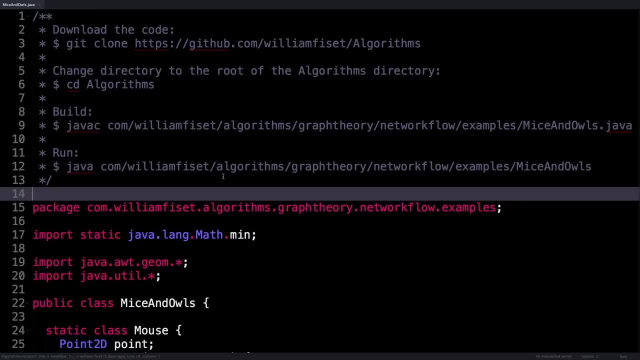 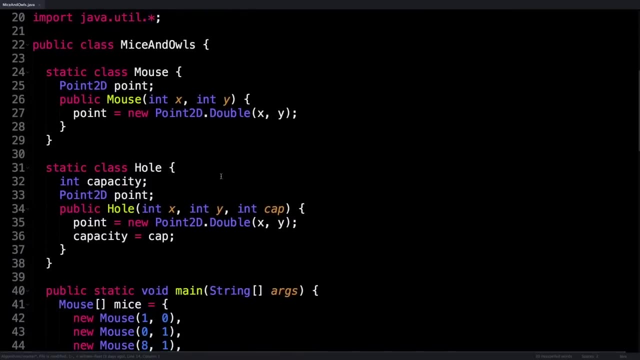 in the description below, just in case you haven't seen it. So let's get started. The first thing I do here is I create a mouse class Which is essentially a wrapper around a point object. Effectively, a mouse is just the point. 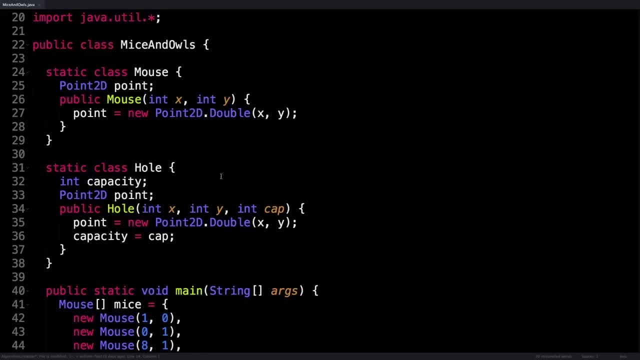 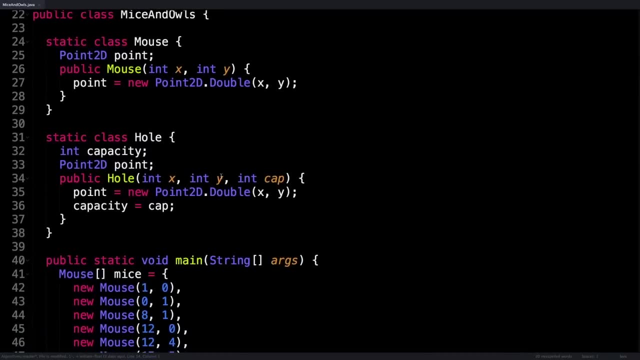 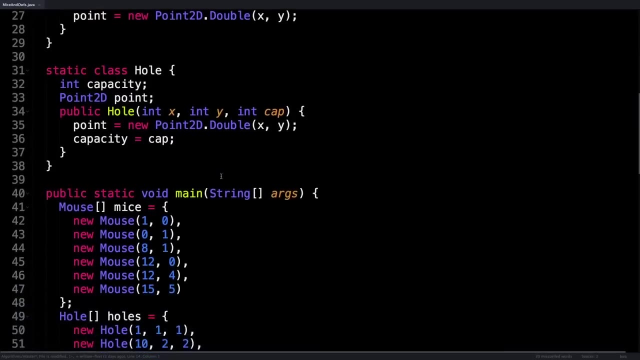 on a plane. I also do the same thing with the whole class, except that the whole class, with addition to having a 2d point object, it also has a certain capacity, because we know that holes can only contain a certain number of mice Next up in the main method. 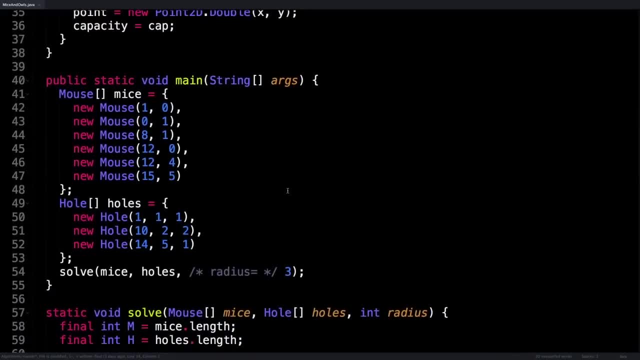 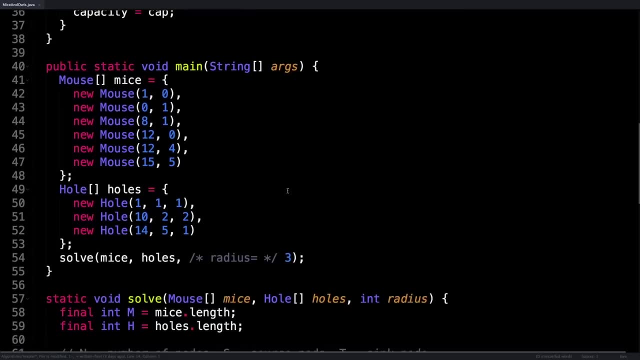 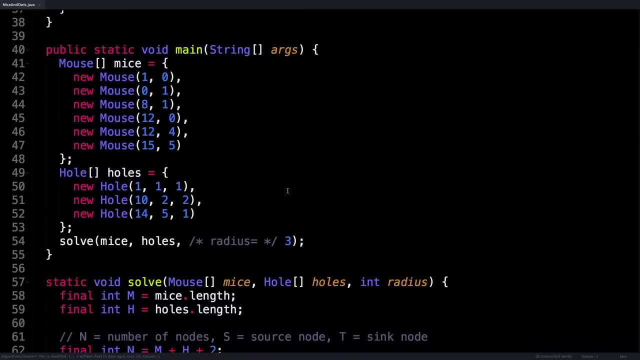 I create a bunch of mouse objects And place them in an array. I scour the mice more or less randomly across the field And then I do the same thing with holes. The last thing I do in the main method is called the solve method, which actually takes as input the two arrays we just created and a radius. 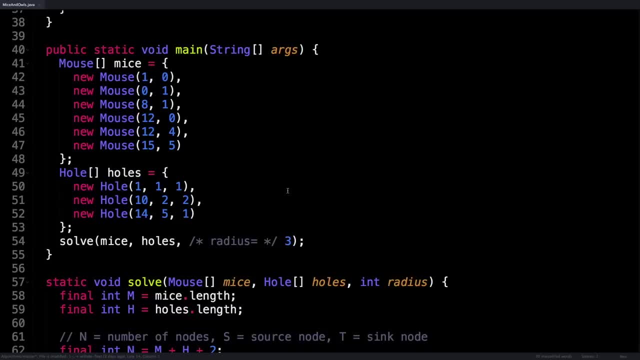 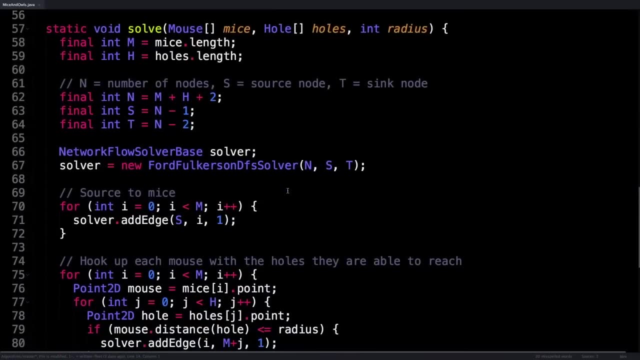 The radius is how far a mouse can run from its current position before being caught by the owl. The solve method is where things really start to get interesting. Let's define some constants that will make our lives a lot easier. First is m, which is just the number of mice. 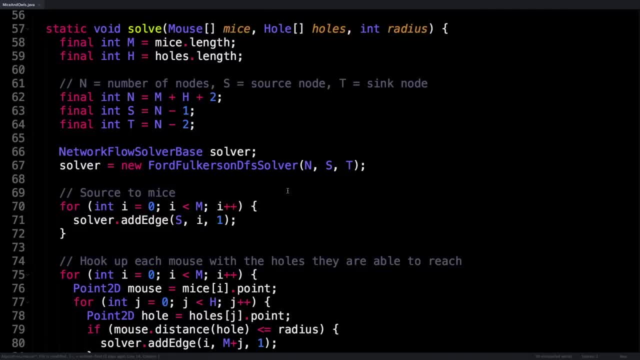 then is h the number of holes we have. Following that, I compute n the number of nodes, which is the number of mice plus the number of holes, plus two. the plus two is to account for the source and the sink node And, as per convention, I always index s and t, the source and the. 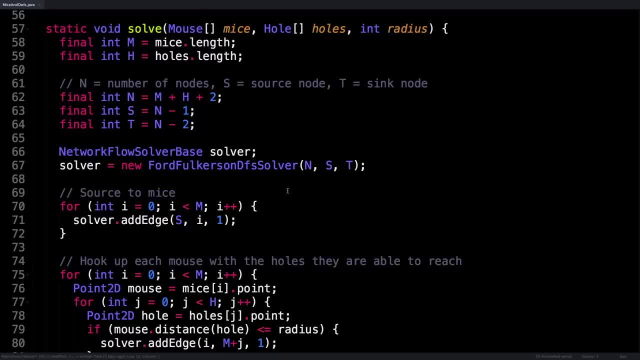 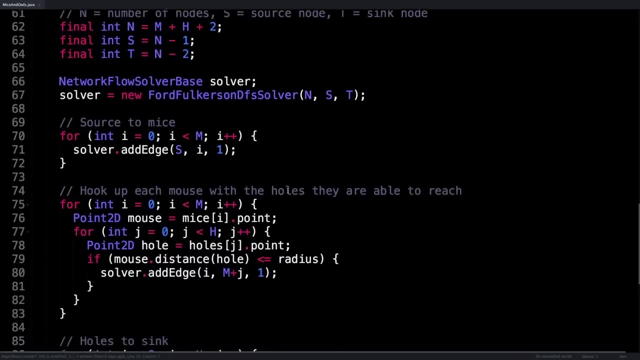 sink to indices and minus one and minus two To ensure that they are unique. After that, I initialize the network flow solver base by providing n, s and t. the solver class is defined below. It's the exact same one from the Ford Fulkerson source code video. In short, the solver lets you add edges with various 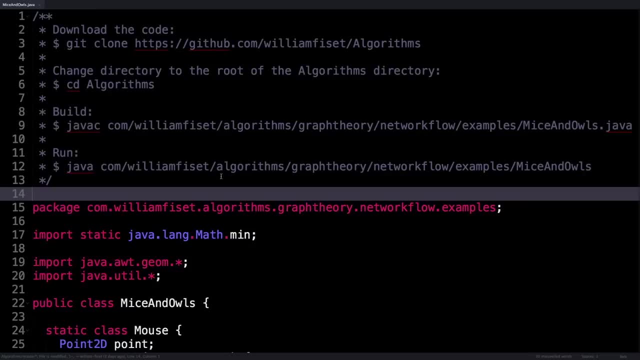 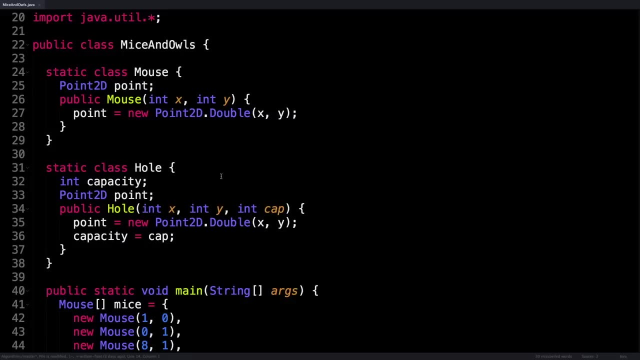 let's get started. The first thing I do here is I create a mouse class which is essentially a wrapper around a point object. Effectively, a mouse is just a point on a plane. I also do the same thing with the whole class, except that the whole class, with addition to having a 2d point object, it also has a 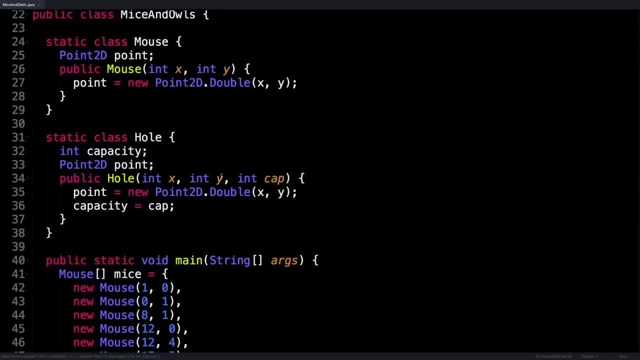 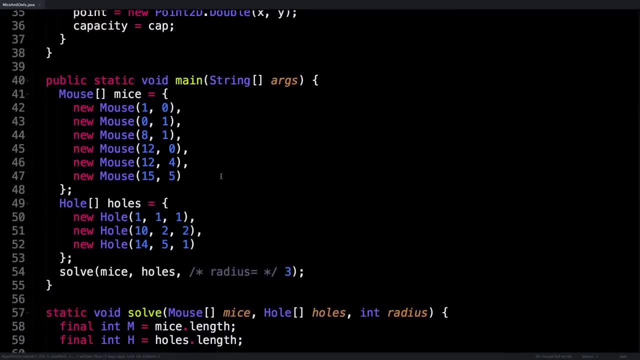 certain capacity, because we know that holes can only contain a certain number of mice. Next up in the main method, I create a bunch of mouse objects and place them in an array. I scatter the mice more or less randomly across the the field And then I do the same thing with holes- The last thing I do in the main method. 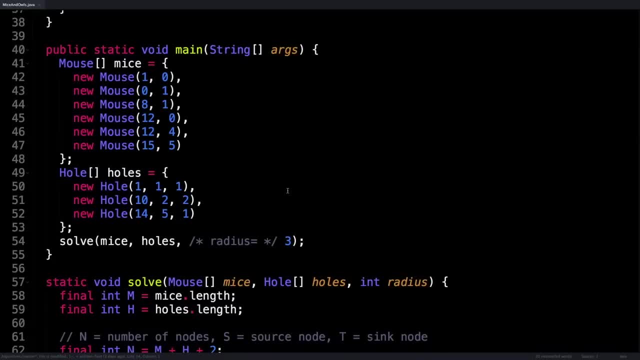 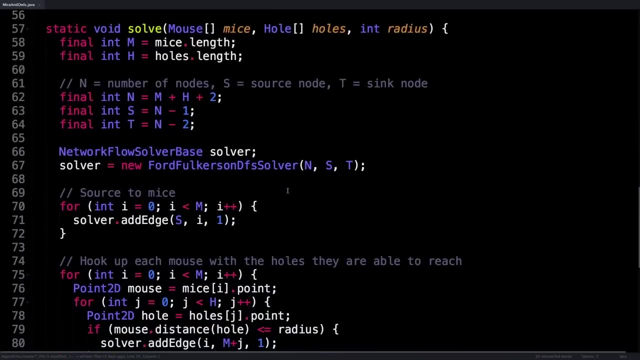 is called the solve method, which actually takes as input the two arrays we just created and a radius. The radius is how far a mouse can run from its current position before being caught by the owl. The solve method is where things really start to get interesting. Let's 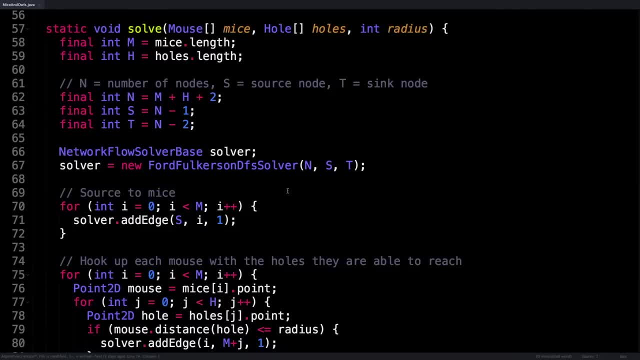 define some constants that will make our lives a lot easier. First is m, which is just the number of mice. then is h, the number of holes we have. Following that, I compute n the number of nodes, which is the number of mice plus the number of holes, plus two, the 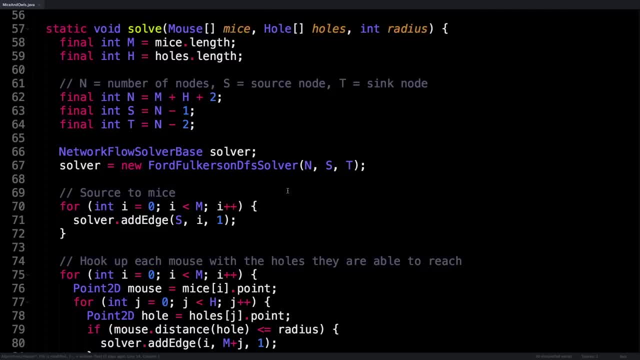 plus two is to account for the source and the sink node And, as per convention, I always index s and t- the source and the sink- to indices, and minus one and minus two to ensure that they are unique. After that I initialize the number of nodes and the number of holes. 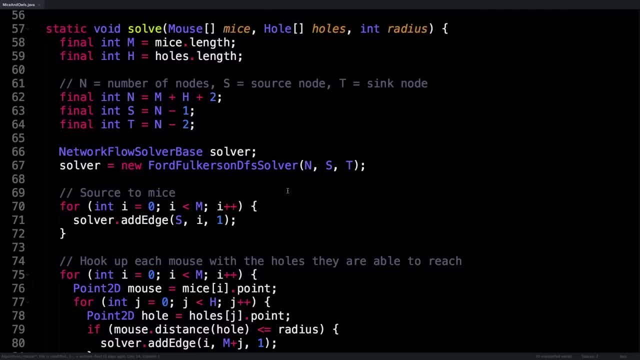 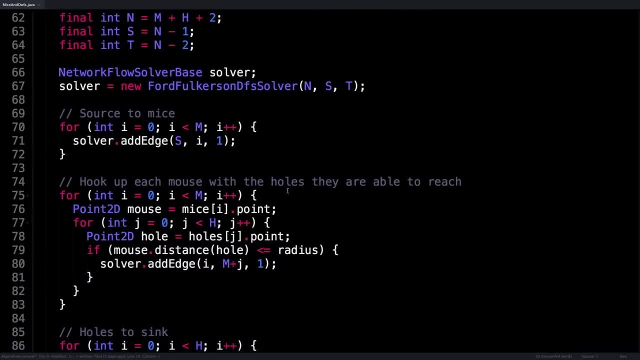 and the sink node. After that, I initialize the network flow solver base by providing n, s and t. the solver class is defined below. It's the exact same one from the Ford Fulkerson source code video. In short, the solver lets you add edges with various capacities to the 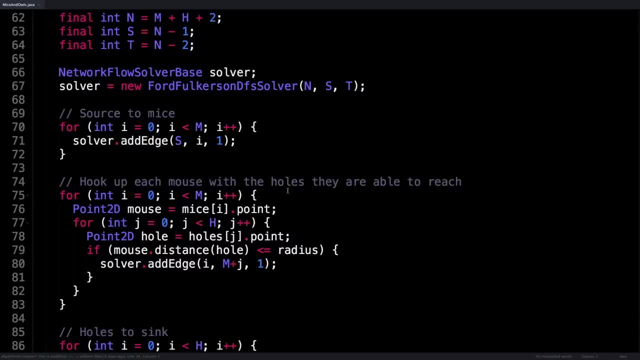 flow graph and then find the max flow once it's all set up. The goal of this video is not to explain to you how the max flow itself is found or how the solver works. I already discussed that previously. What I really want to find out about the max flow is that it's 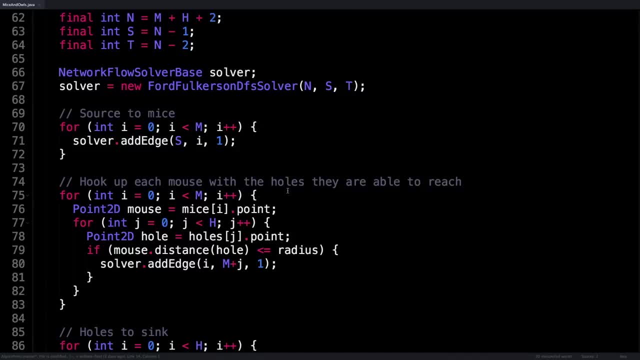 based on the flow graph, And what I want to focus on in this video is how to set up the flow graph for this problem and push some flow through it. When the graph is bipartite, like it is in this problem, the setup is actually pretty straightforward. The first step is 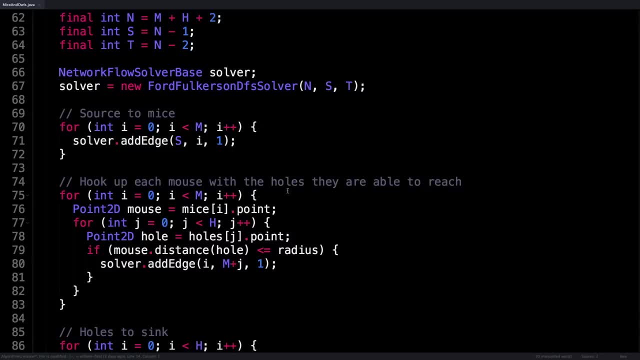 capacities to the flow graph and then find the max flow once it's all set up. The goal of this video is not to explain to you how the max flow itself is found or how the solver works. I already discussed that previously. What I really want to focus on in this video, 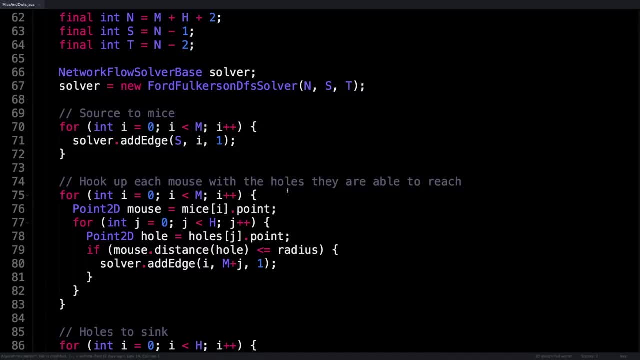 is how to set up the flow graph for this problem and push some flow through it. When the graph is bipartite, like it is in this problem, the setup is actually pretty straightforward. The first step is to hook up edges from the source s to each mouse with a capacity of 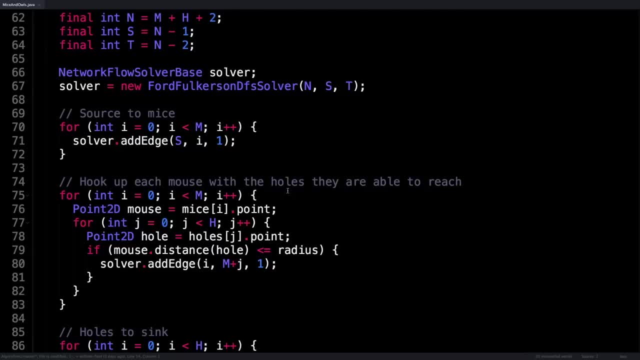 one. Intuitively, this limits each mouse node to represent at most one mouse. Now let's say we want to represent one mouse. this is necessary because we don't want a mouse node to represent more than one mouse. that doesn't really make sense. The next part is to hook. 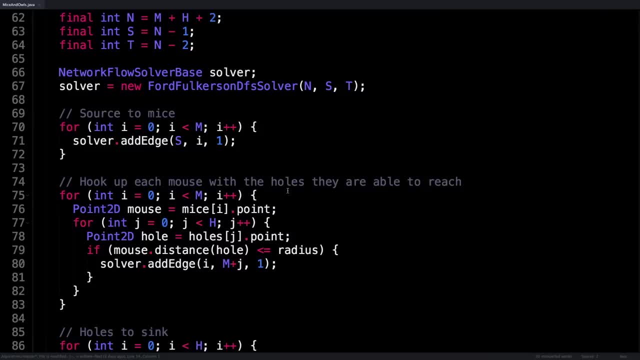 up mouse nodes with whole nodes in the flow graph. This is the middle section of the flow graph where we add an edge between a mouse node and a hole if the distance from a mouse to the hole is less than the radius, In other words, if the mouse can make it to the hole. 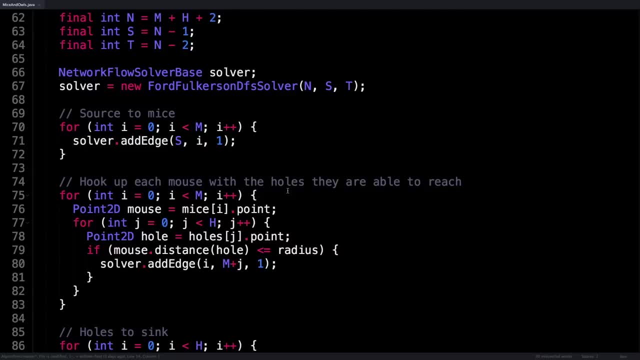 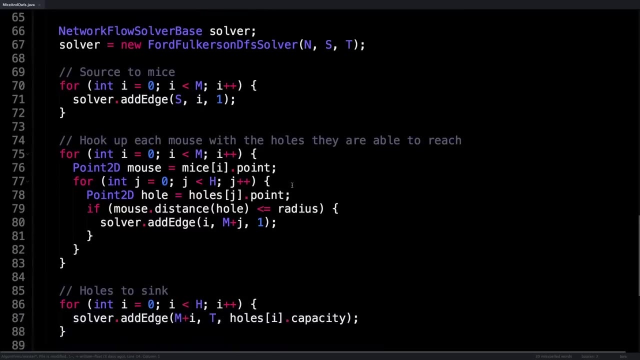 on time, add an edge connecting the mouse and the hole. The last step is also important. you need to remember to hook up the edges between the holes and the sink. These edges are slightly different because their capacity represents the number of mice which can fit into each. 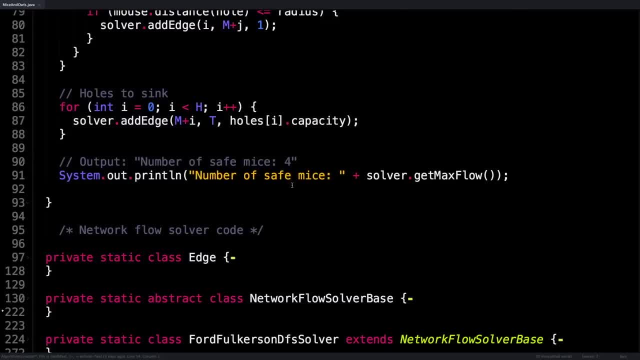 particular hole. Say, a hole has a capacity of three, but there are five mice which can make it to that hole. Well, we cannot allow more than three of those mice to fit in the hole. So we need to make sure that we have enough space between the holes and the sink to be. 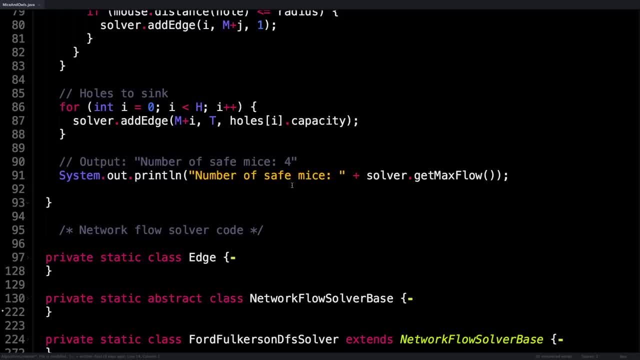 three. Those two leftover mice will need to find another hole or get scooped up by the owl. The very last thing we need to do to actually get the max flow is to run the solver, which will return the number of safe mice which, for this configuration, happens to be. 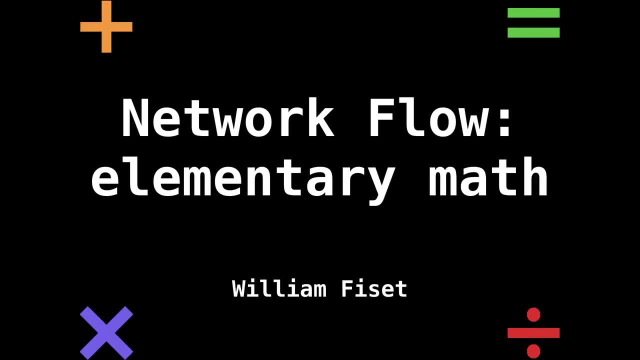 four, we're still talking about network flow, And today's topic is one of my all time favorite flow problems, which is the elementary map problem. This problem is so interesting because its solution uses flow, but it really doesn't hit you as a flow problem to begin with. One of the hardest things about network flow: 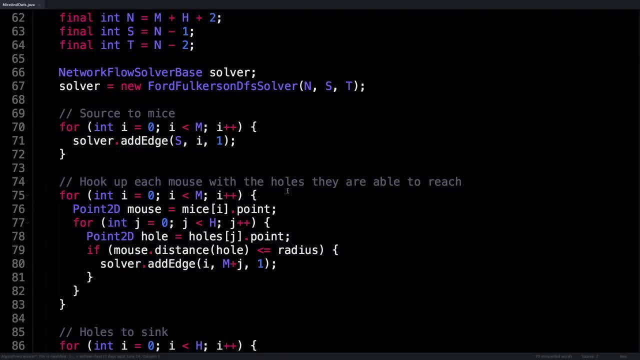 to hook up edges from the source s to each mouse with a capacity of one. Intuitively, this limits each mouse node to represent at most one mouse. This is necessary because we don't want a mouse node to represent more than one The mouse. that doesn't really make sense. The next part is to hook up mouse nodes with: 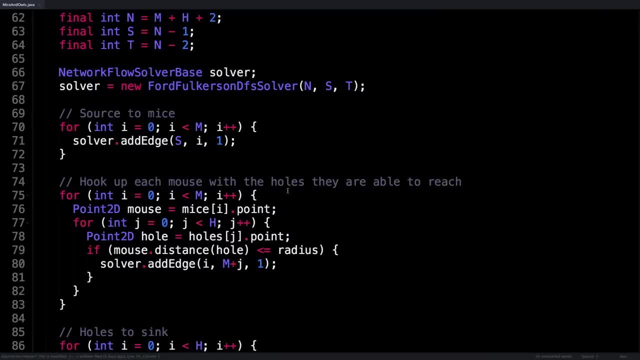 whole nodes in the flow graph. This is the middle section of the flow graph where we add an edge between a mouse node and a hole if the distance from a mouse to the hole is less than the radius, In other words, if the mouse can make it to the hole on time. add. 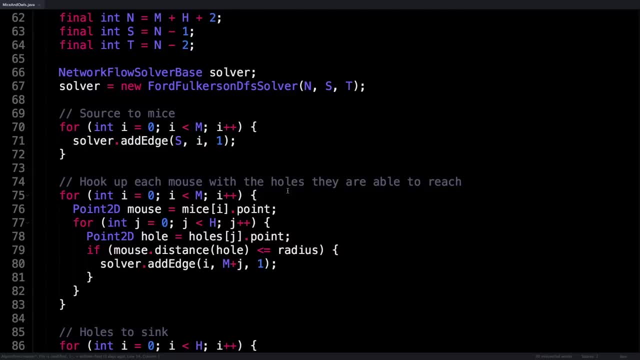 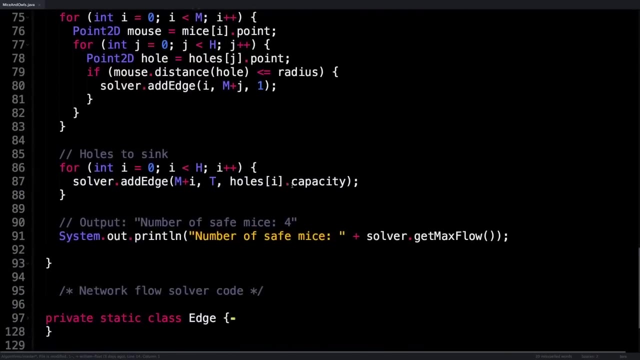 an edge connecting the mouse and the hole. The last step is also important. you need to remember to hook up the edges between the holes and the sink. These edges are slightly different because their capacity represents the number of mice which can fit into each particular hole. Say, a hole has a capacity of three, but there 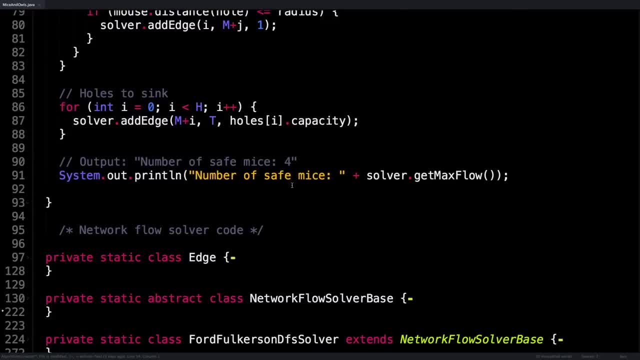 are five mice which can make it to that hole. Well, we cannot allow more than three of those mice to fit in the hole, So we set the capacity of the edge to the sink to be three. Those two leftover mice will need to find another hole or get scooped up by the owl, The very last thing we need to do to 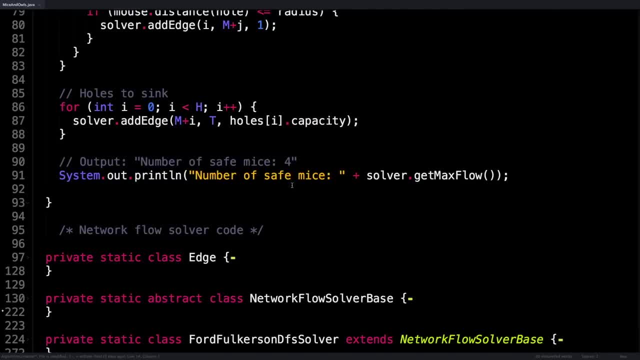 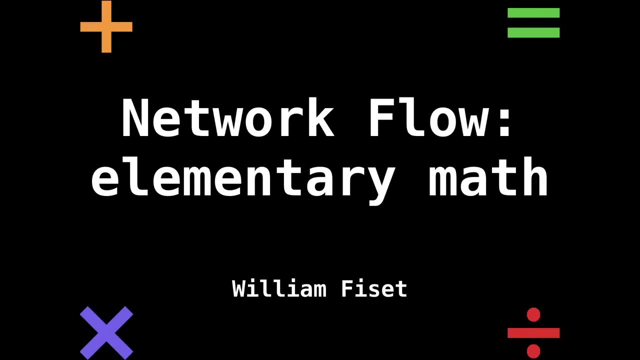 actually get the max flow is to run the solver, which will return the number of safe mice, which, for this configuration, happens to be four. we're still talking about network flow, And today's topic is one of my all time favorite flow problems, which is the elementary math. 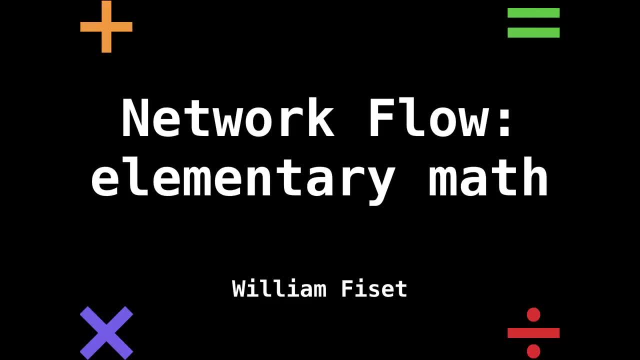 problem. This problem is so interesting because its solution uses flow, but it really doesn't hit you as a flow problem to begin with. One of the hardest things about network flow, I believe, is actually identifying that a problem is a flow problem and then setting it up as so. this is why I'm spending so many videos. 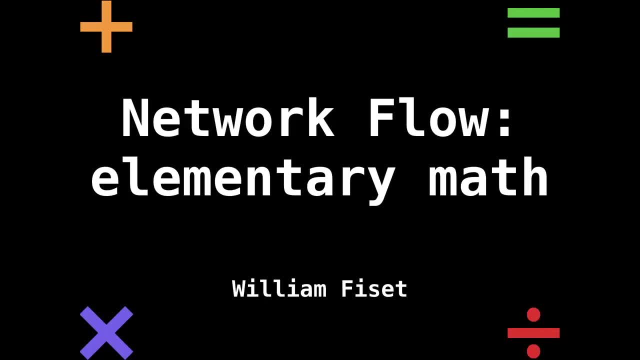 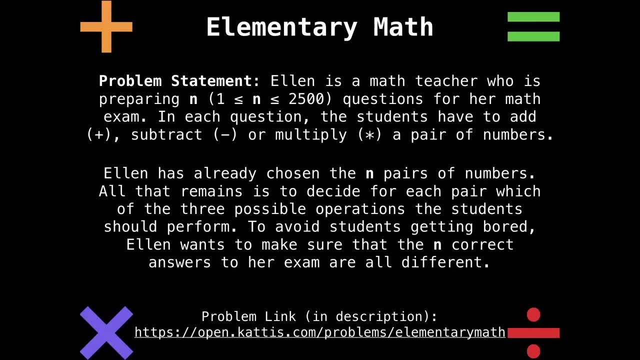 solving some flow problems. So you really start understanding how to approach them and how they are solved. So let's dive into the elementary math problem. This problem is actually on caddis, Should you want to attempt it. the link is at the. 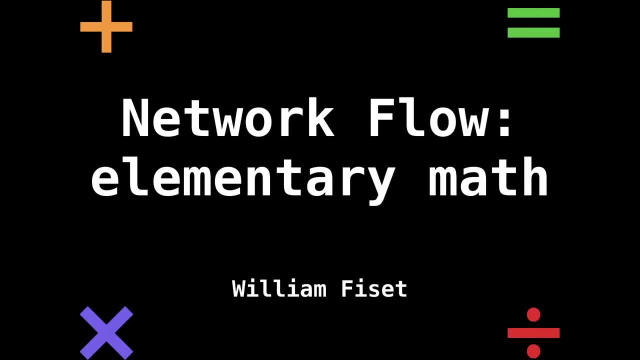 I believe, is actually identifying that a problem is a flow problem and then setting it up as so. this is why I'm spending so many videos solving some flow problems, So you really start understanding how to approach them. So let's get started And how they are solved. So let's dive into the elementary math problem, This problem. 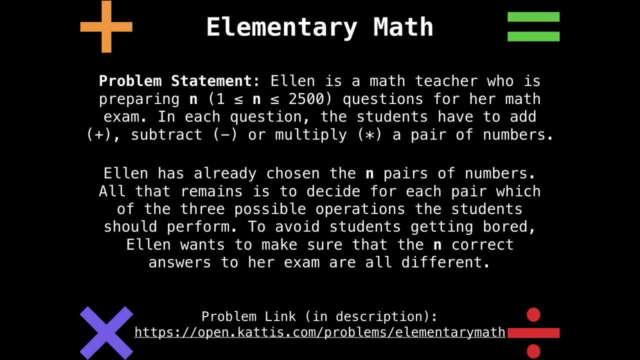 is actually on caddis, Should you want to attempt it. the link is at the bottom of the slide and also in the description. Here's the problem statement. Ellen is a math teacher who is preparing n questions for her exam. In each question the students have to add: 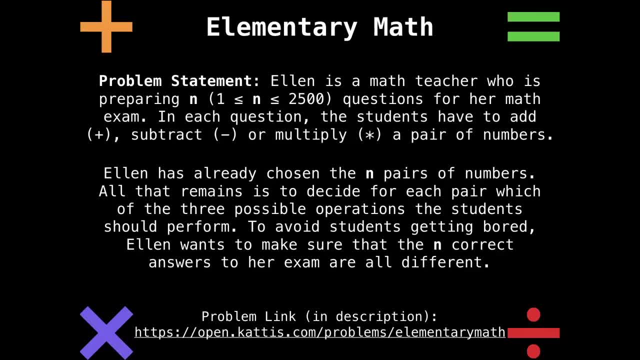 subtract or multiply a pair of numbers. Ellen has already chosen the n pairs of numbers. All that remains is to decide, for each pair, which of the following three possible operations the students should perform. To avoid students getting bored, Ellen wants to make sure that. 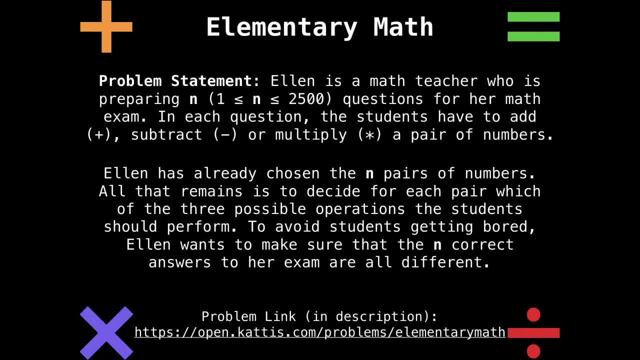 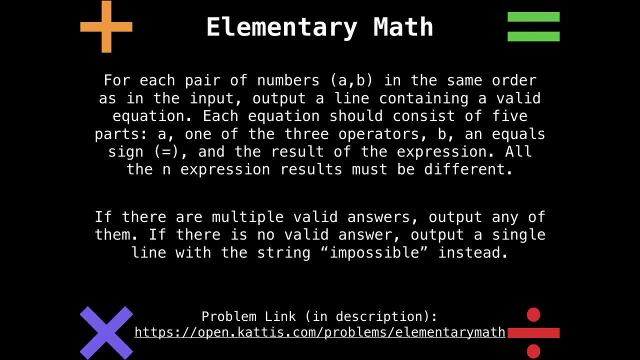 the n correct answers on her exam are all different. For each pair of numbers- a, B- in the same order as the input, output a line containing a valid equation. Each equation should consist of five parts: A- one of the three operators. B- an equal sign and the result of the expression all. 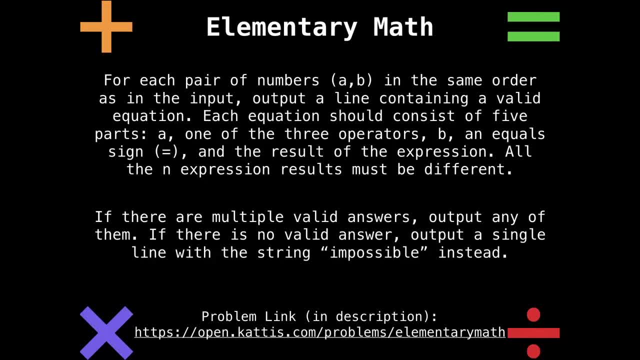 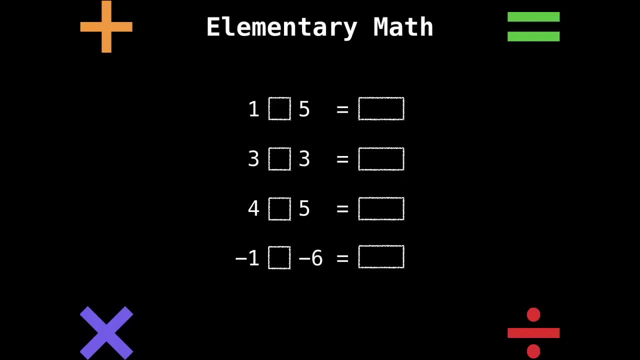 the n expression. results must be different. If there are multiple valid solutions, output any of them. If there are no valid answers, output a single line with the string impossible. instead, Let's have a look at an example. So Ellen goes and picks four pairs of numbers. 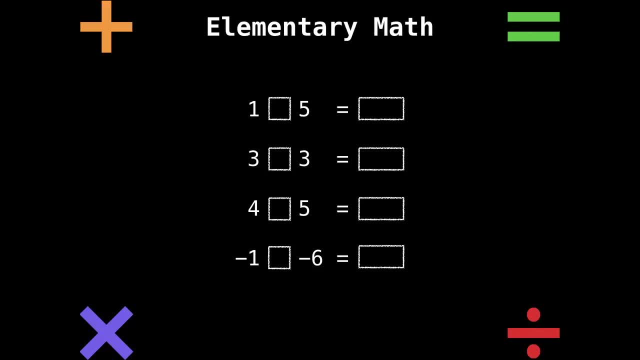 say one and five, Three and three, four and five and lastly, minus one and minus six, She wants to assign operators either plus, minus or multiply to yield the unique answers on the right hand side of the equation. One assignment of operators might be the following: However, this assignment 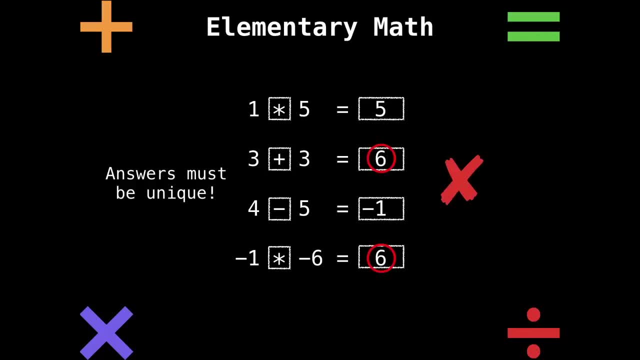 of operators doesn't quite work because the answers are not unique on the right hand side. Here's another way of assigning operators to the pairs of numbers. This assignment, however, does work because the answers are unique on the right hand side, which is one. 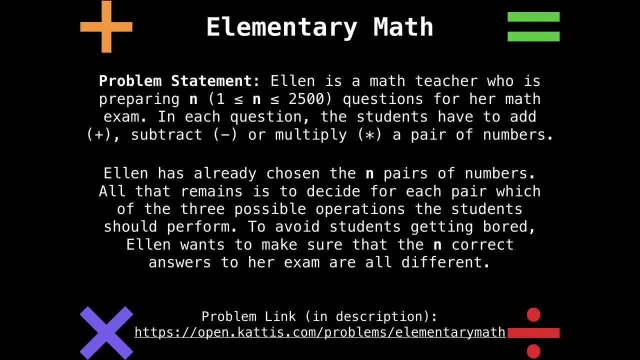 bottom of the slide and also in the description. Here's the problem statement. Ellen is a math teacher who is preparing and questions for her exam. In each question the students have to add, subtract or multiply a pair of numbers. Ellen has already chosen the end pairs of. 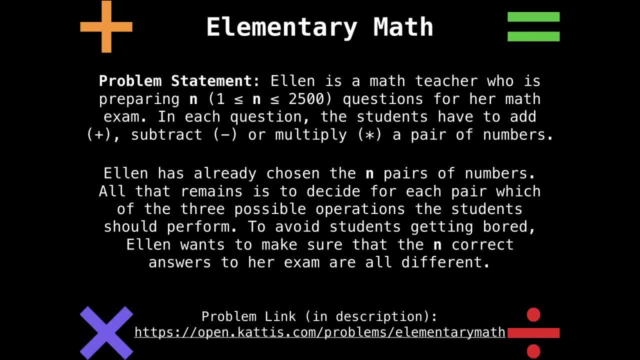 numbers. All that remains is to decide, for each pair, which of the following numbers should be added or subtracted. For each pair, which of the following numbers should be added in the following three possible operations the students should perform. to avoid students getting bored, Ellen wants to make sure that the end correct answers on her exam are all. 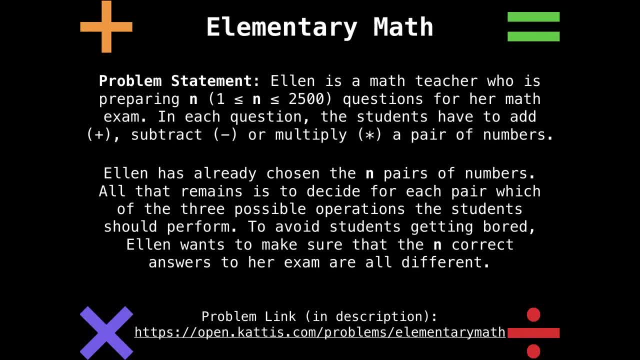 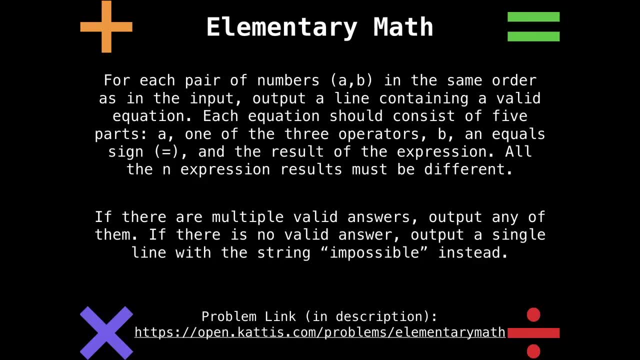 different for each pair of numbers, a, B, in the same order as the input output, a line containing a valid equation. Each equation should consist of five parts: A, one of the three operators, B and equals SUN sign and the result of the expression. All the n expression results must be different. 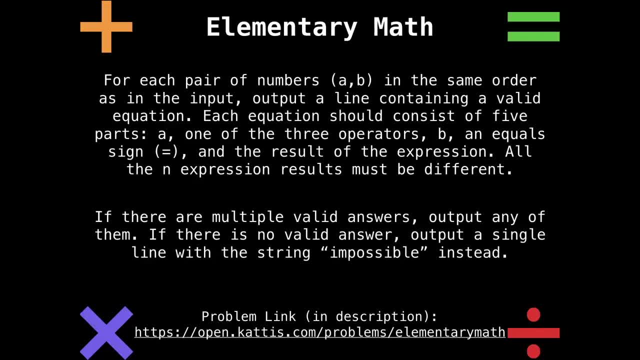 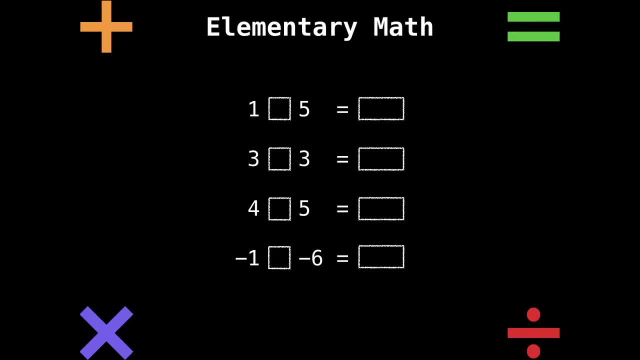 If there are multiple valid solutions, output any of them. If there are no valid answers, output a single line with the string impossible. instead, Let's have a look at an example. So Ellen goes and picks four pairs of numbers, say one and five, three and three, four and. 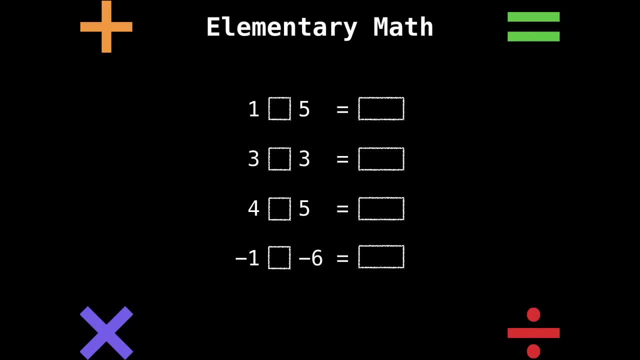 five and lastly, minus one and minus six. She wants to assign operators either plus, minus or multiply to yield the unique answers on the right hand side of the equation. One assignment of operators might be the following: However, this assignment of operators doesn't 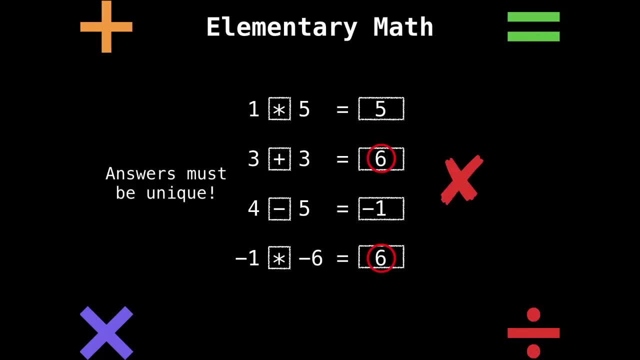 quite work because the answers are not unique on the right hand side. Here's another way of assigning operators to the pairs of numbers. This assignment does work because the answer answers are unique on the right hand side, which is one of the requirements for the problem. 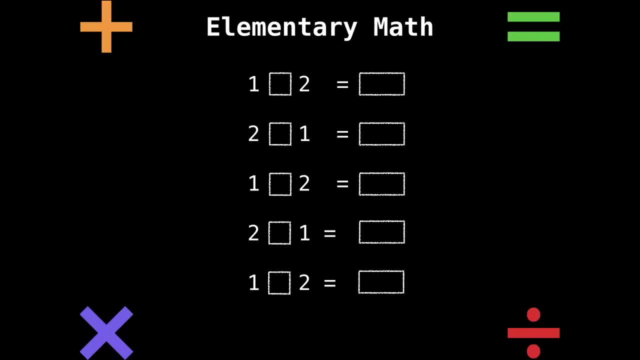 So we just saw that not any arbitrary assignment of operators yields a valid solution. But it's also possible for no answer to exist. Consider the following pairs of numbers: In this case there can be no solution because there are not enough unique answers that can. 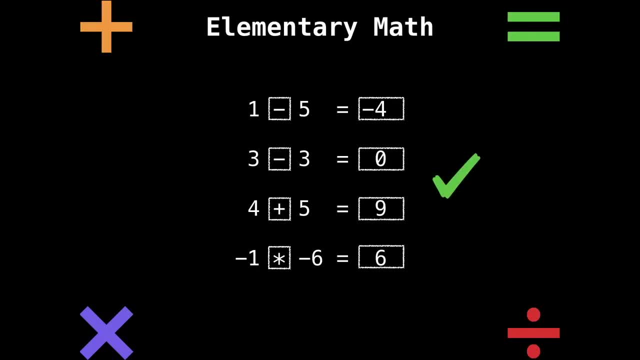 of the requirements for the problem. So we just saw that not any arbitrary assignment of operators yields a valid solution, But it's also possible for no answer to exist. Consider the following pairs of numbers: In this case, there can be no solution because 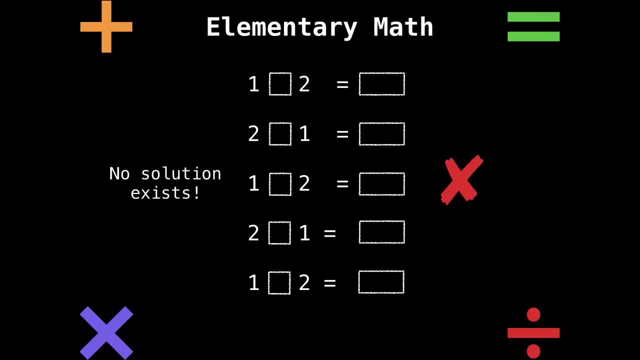 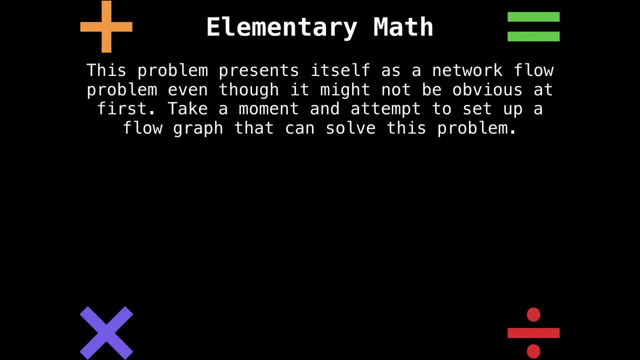 there are not enough unique answers that can be produced using the operators plus, minus and multiply. As it happens, this problem presents itself as a network flow problem, even though that might not be obvious at first. So take a moment and attempt to set up a flow graph that can. 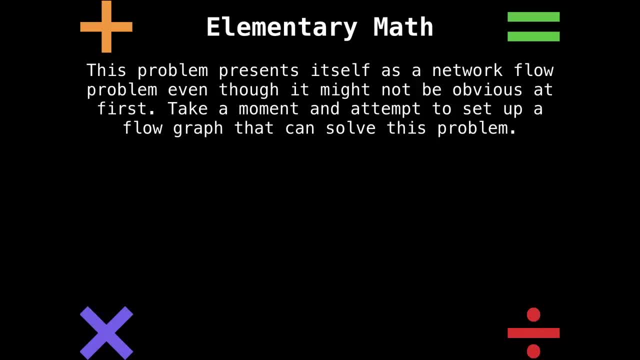 actually solve this problem. It's actually a really great exercise. Along the way, While you're doing this, there are a few questions you should ask yourself, or at least that I asked myself when I first did this. The first: is there a way that this problem can? 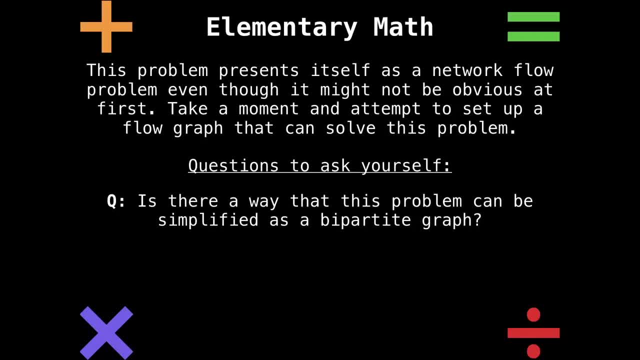 be simplified into a bipartite graph. I asked myself this because I know that solving a flow problem when it's a bipartite graph can be done very efficiently, And also because bipartite graphs are very easy to set up. Then I asked myself: how am I going to detect? 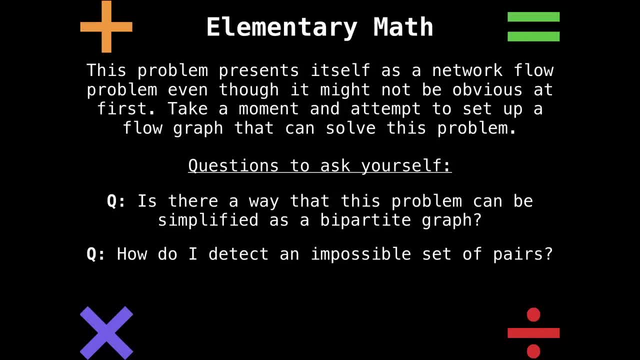 impossible sets of pairs. Will my flow graph be able to handle that, Or do I need to do some pre or post processing to actually figure that out? And lastly, I'm thinking about the edge cases, So like: how do I handle multiple repeated input pairs And how is I going to 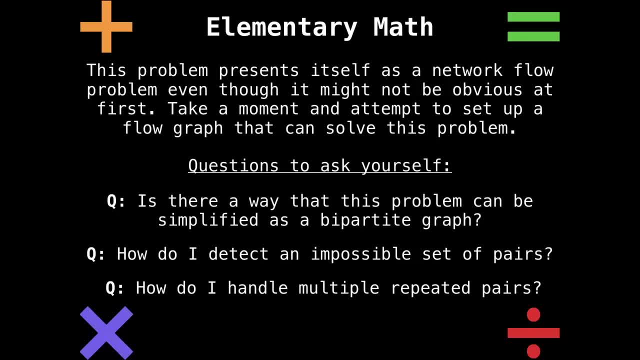 change the flow graph? these are all super important questions you need to ask yourself when solving this problem. This slide deck explains the first two and the third is somewhat left as an exercise. I don't want to give away the full solution to this. really awesome. 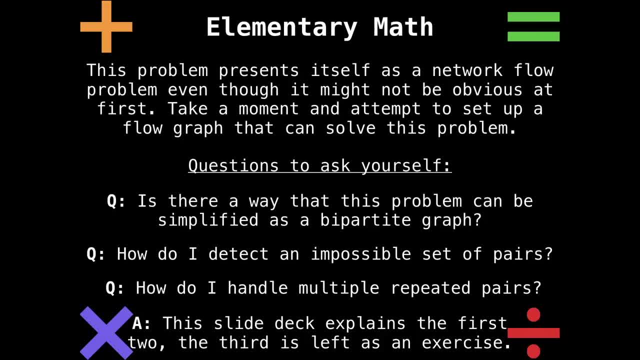 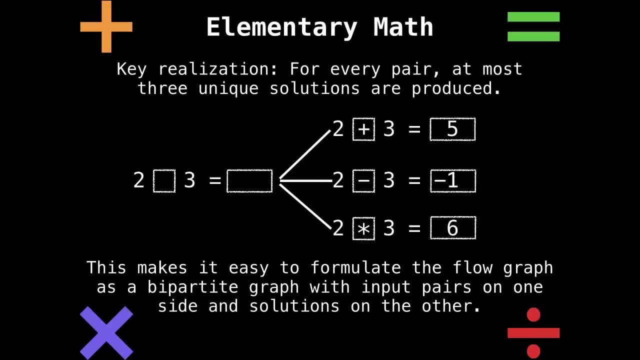 problem. So, thinking about how we're going to solve this problem a little more, a key realization to make is that for every input pair- at most three times- you're going to have three unique solutions are produced. Think of the input pair two and three. Well, 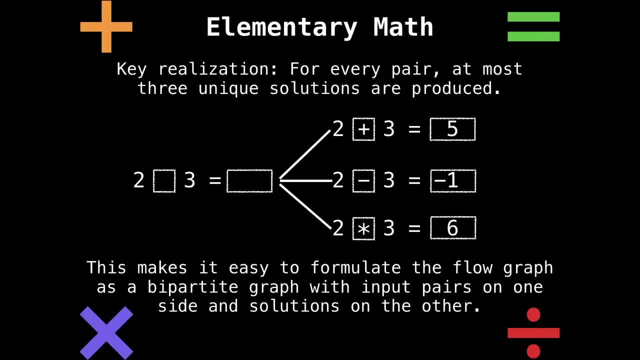 for that pair. we can either add two and three, subtract two and three or multiply two and three, So there can be at most three unique results. there may be last, if there are collisions, think of the input pair: 00, zero plus 00, zero multiplied by 00. And zero subtracted. 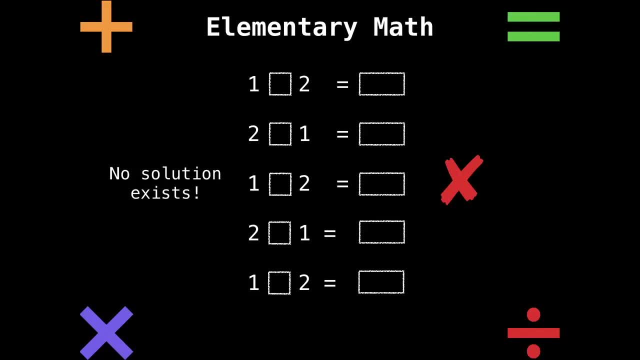 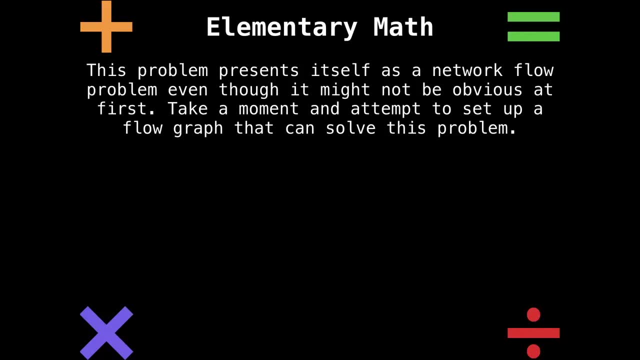 be produced using the operators plus, minus and multiply. As it happens, there are no solutions. This problem presents itself as a network flow problem, even though that might not be obvious at first. So take a moment and attempt to set up a flow graph that can. 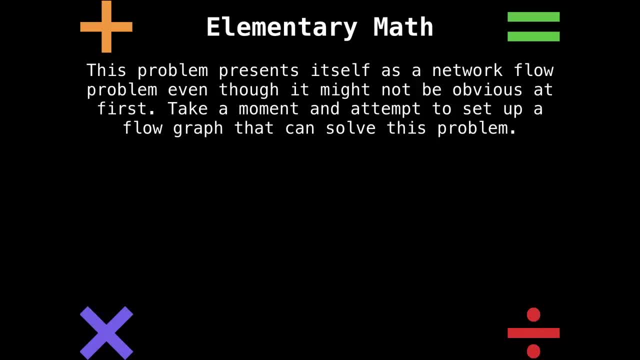 actually solve this problem. It's actually a really great exercise. Along the way, while you're doing this, there are a few questions you should ask yourself, or at least that I asked myself when I first did this. The first: is there a way that this problem can? 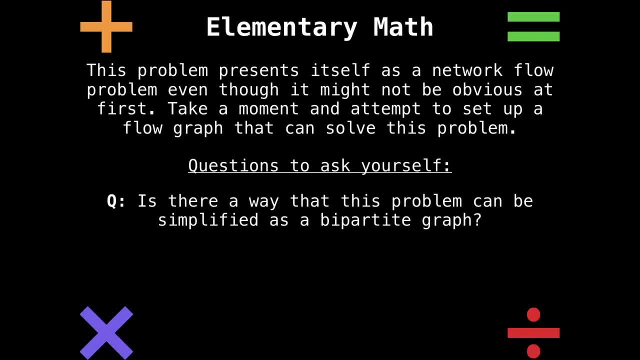 be simplified into a bipartite graph. I asked myself this because I know that solving a flow problem when it's a bipartite graph can be done very efficiently, And also because bipartite graphs are very easy to set up. then I asked myself: how am I going to detect impossible sets of pairs? 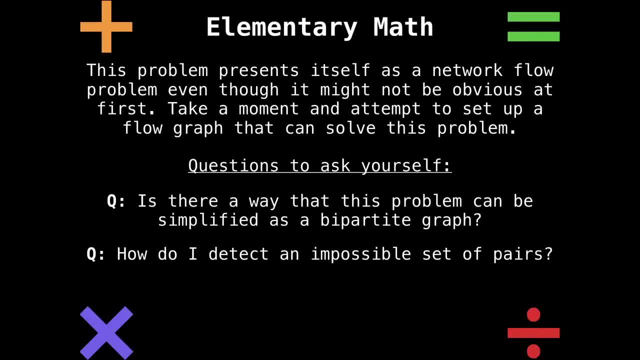 Will my flow graph be able to handle that, Or do I need to do some pre or post processing to actually figure that out? And lastly, I'm thinking about edge cases. So like: how do I handle multiple repeated input pairs And how is that going to change the flow graph? 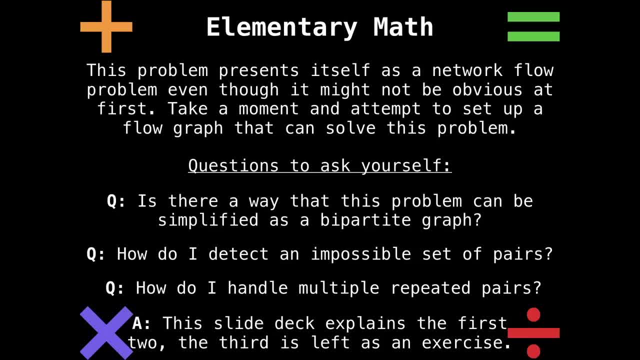 These are all super important questions you need to ask yourself when solving this problem. This slide deck explains the first two, And the third is somewhat left as an exercise. I don't want to give away the full solution to this really awesome problem, So thinking: 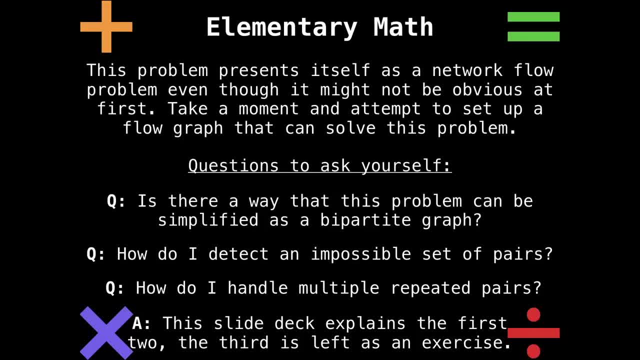 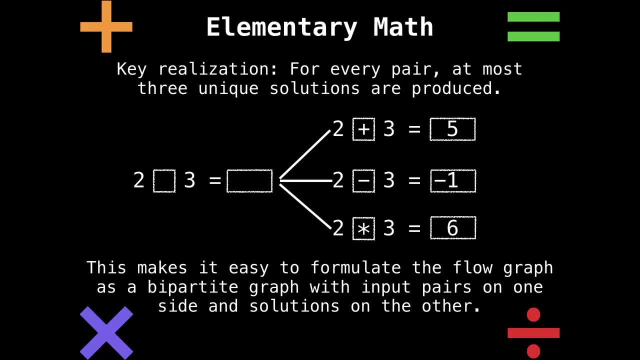 about how we're going to solve this problem a little more. a key realization to make is that for every input pair, at most three unique solutions solutions are produced. think of the input pair two and three. well, for that pair. 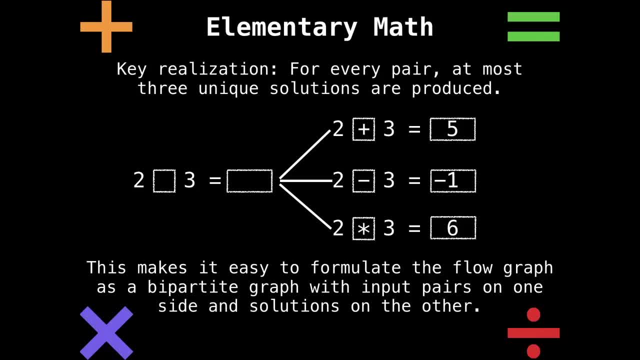 we can either add two and three, subtract two and three or multiply two and three, So there can be at most three unique results. there may be the last if there are collisions. think of the input pair: 00, zero plus 00, zero multiplied by 00. And zero subtracted. 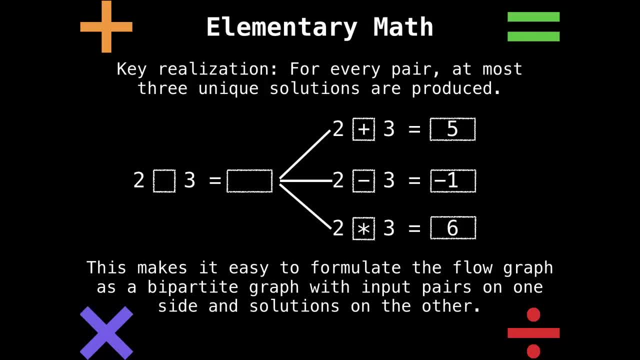 by zero is also zero, So we may end up with less than three unique solutions, And that's fine. The great thing about this is that we can easily set up a bipartite flow graph from this, because we can have input pairs on one side and solutions on the other side. Let's 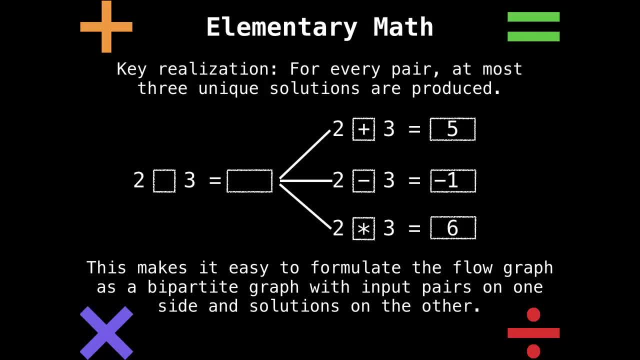 by zero is also zero, So we may end up with less than three unique solutions, And that's fine. The great thing about this is that we can easily set up a bipartite flow graph from this, because we can have input pairs on one side and solutions. 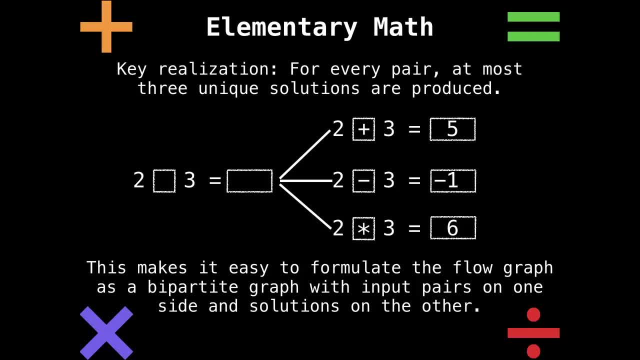 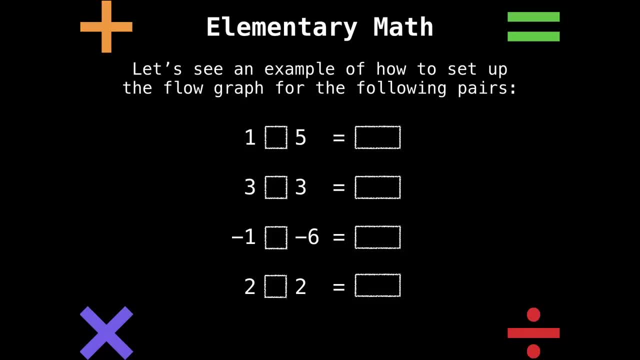 on the other side. Let's see if we can set the flow graph and solve the set of input pairs. we have the pairs 1533 minus one, minus six and finally to two. So how we're going to set up this bipartite graph is we're going to have input nodes on the left side and 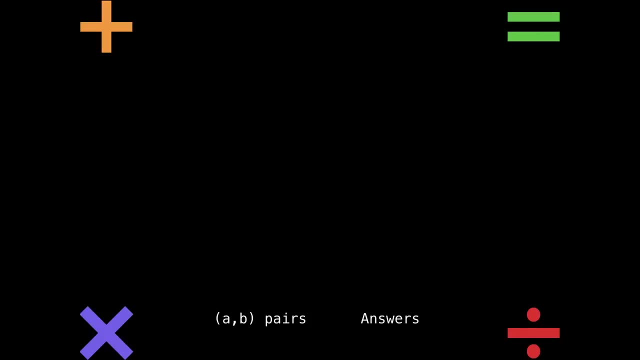 answer nodes on the right side For our first input, pair 15.. If we compute one minus five, one plus five and one multiplied by five, we get minus four, six and five, which become answer nodes on the right hand side. then we want to attach an edge between that input. 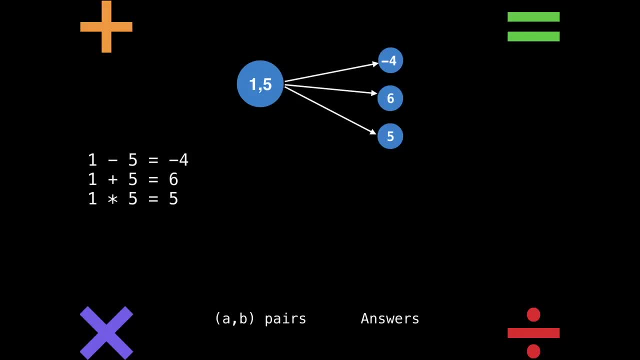 pair and the answer. Do the same thing for the next input pair. make an input pair node and attach edges to the answer nodes. However, don't create another answer node if there already exists one with the value we need. In this example, you'll see that three plus three equals six, and we already. 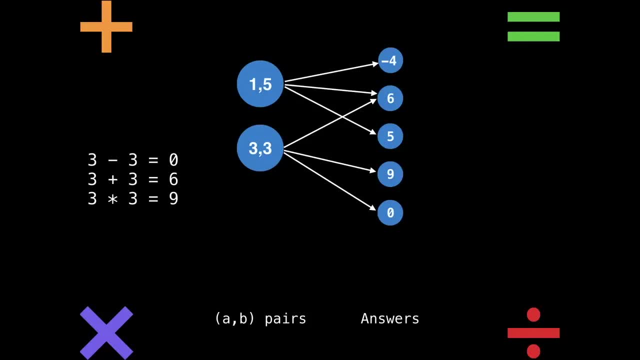 have an answer node for six, So simply attach an edge from three, three to six. do not create another answer node. This is to ensure that our answers remain unique And do the same thing for the other two remaining input pairs. You'll notice that the last input pair is 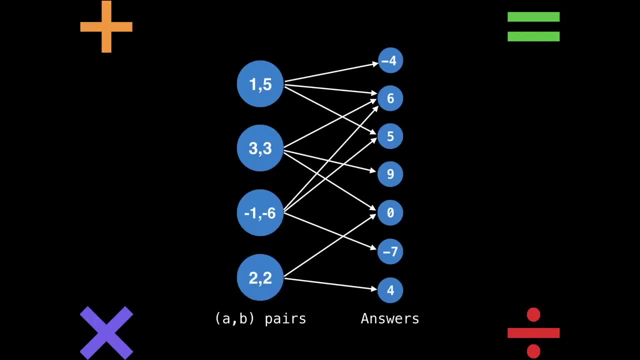 only produced two outgoing edges and not three. This is because there was a collision, in particular, two plus two equals four, but also two multiplied by two equals four. And this is fine. Just put one edge, don't put two edges. then, like every bipartite graph you're trying to find, 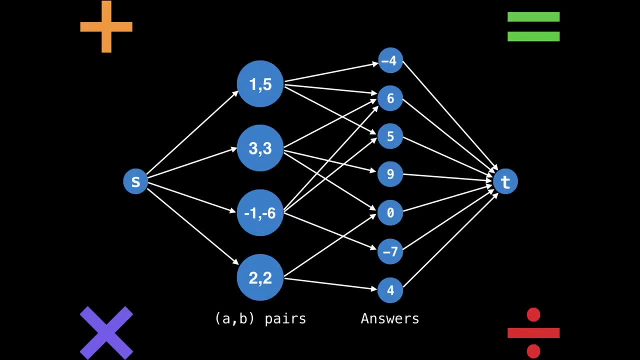 a matching, for you'll want to add the source s and the sink t, And the matching is really what we're after here. we want to match input pairs to answers, And then we've actually solved the problem. The next step, after adding the source in the 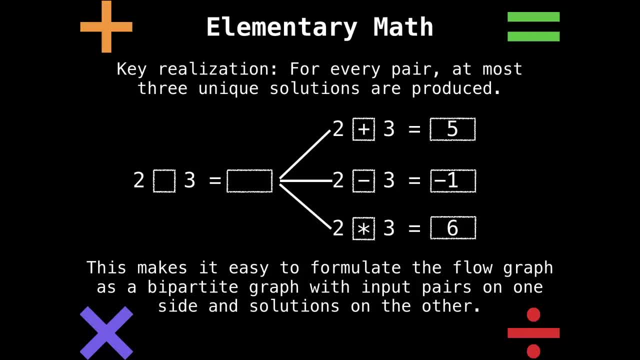 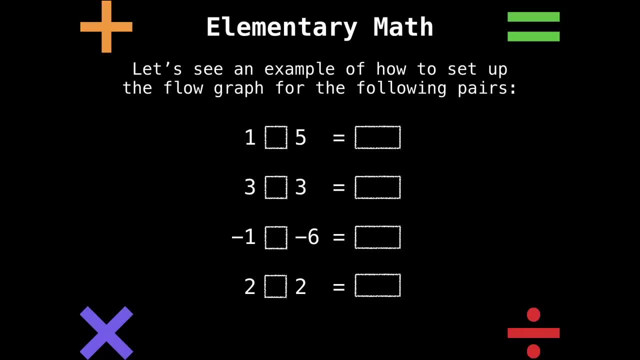 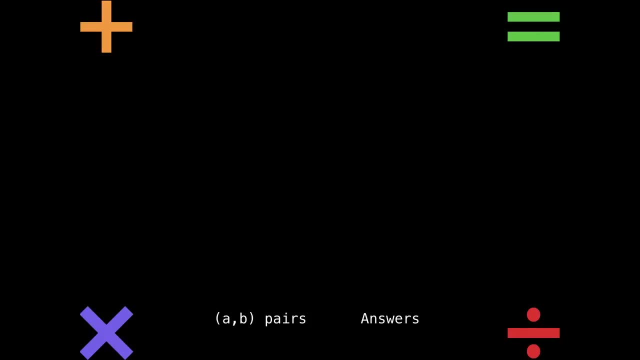 see if we can set the flow graph and solve the set of input pairs. we have the pairs 1533, minus one, minus six and finally to two. So how we're going to set up this bipartite graph is we're going to have input nodes on the left side and answer nodes on the right. 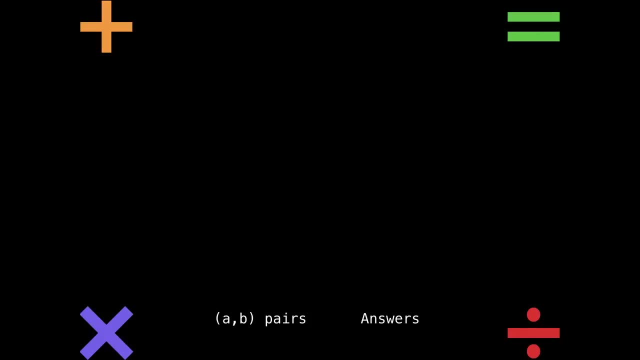 side For our first input pair 15.. If we compute one minus five, one plus five and one multiplied by five, we get minus four, six and five which become answer nodes on the right hand side. then we want to attach an edge between that input pair and the answer Do the same. 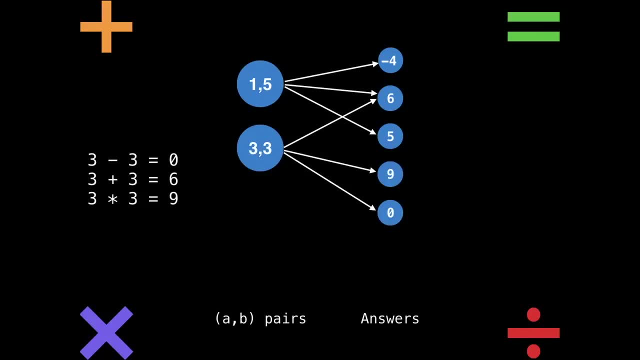 thing for the next input pair. make an input pair node and attach edges to the answer nodes. However, do not create another answer node if there already exists one with the value we need. In this example, you'll see that three plus three equals six and we already have an answer. 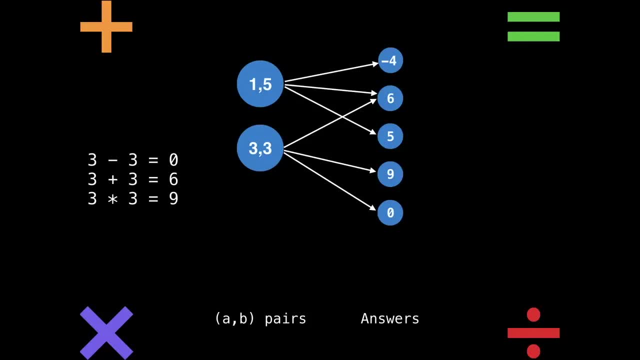 node for six. So simply attach an edge from three, three to six. do not create another answer node. This is to ensure that our answers remain unique. And do the same thing for the other two remaining input pairs. you'll notice that the last input pair only produced two. 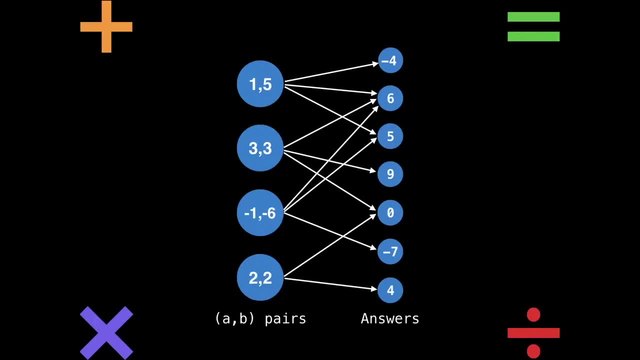 outgoing edges and not three. This is because there was a collision, in particular: two plus two equals four, but also two multiplied by two equals four. And this is fine. Just put one edge, don't put two edges. then, like every bipartite graph, you're trying to find a matching. 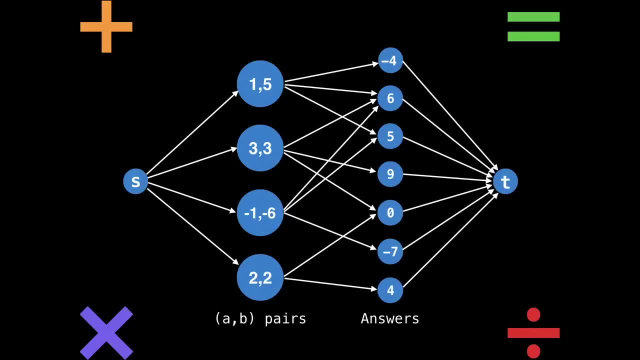 for you'll want to add the source s and the sink t, And the matching is really what we're after here. we want to match input pairs to answers And then we've actually solved the problem. The next step, after adding the source in the sink, is to actually assign capacities. 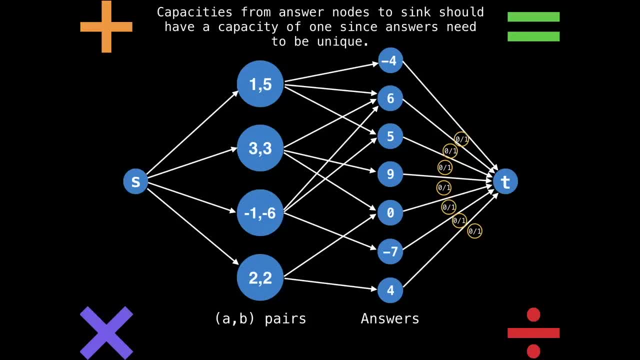 to the edges of the flow graph. Let's start on the right side. the capacities from the answer nodes to the sink should all have a capacity of one, since the answers need to be unique, and limiting the edge capacity to one ensures that capacities for the input. 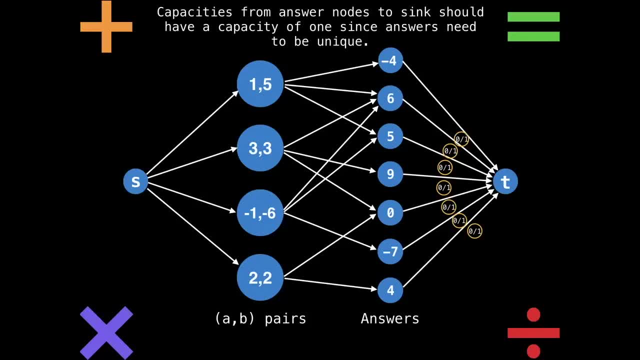 sink is to actually assign capacities to the edges of the flow graph. Let's start on the right side. the capacities from the answer nodes to the sink should all have a capacity of one, since the answers need to be unique, and limiting the edge capacity to one ensures 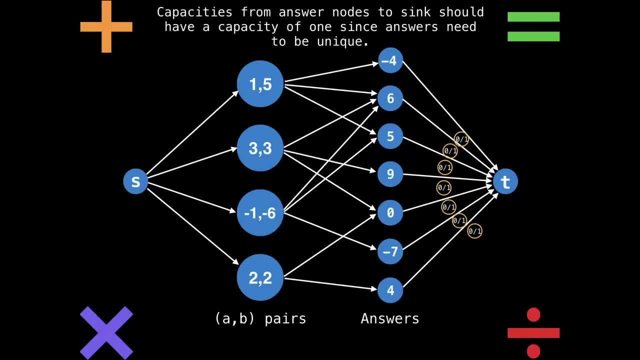 that capacities for the input pairs to answers should also have a capacity of one, since only one of the answers should be unique. In this example, all frequencies are one, but, as we know, that's not always the case. Now the flow graph is set up, let's run a max flow algorithm on it. The flow algorithm. 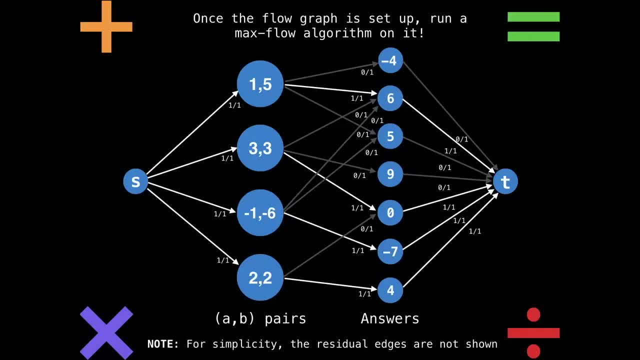 does its thing and some edges are filled with flow. These are the edges that were selected to be part of the maximum flow. From this we can derive what the matching was. More specifically, we're interested in the middle edges. those are the edges which give us information. 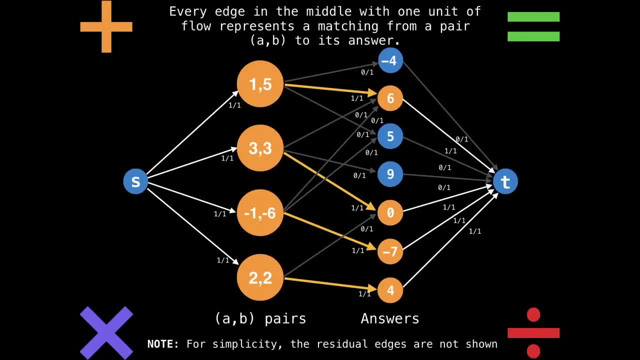 about the matching. Every edge in the middle with one unit of flow represents a matching from an input pair a, B to its answer. For example, the input pair one, five was matched to the answer node six because there's one unit of flow going through that edge. 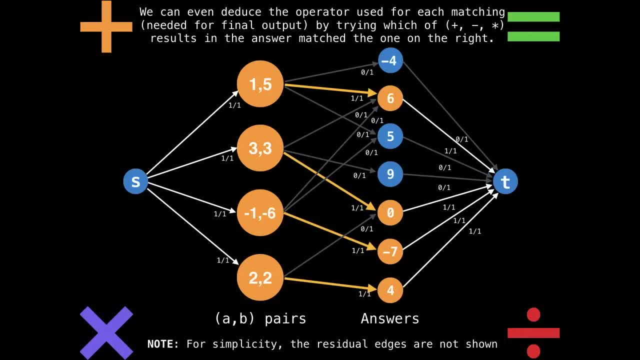 From this we can even deduce the operator used for each matching, which is actually needed for the final output. This can be done by trying which of the plus, minus or multiply operator results in the found matching. Basically, we first solve the problem by figuring out. 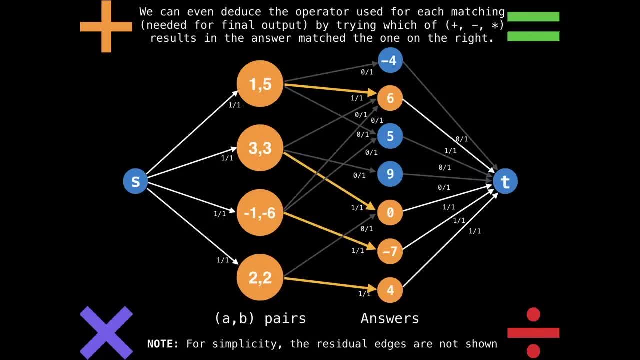 which answers we get and then work backwards to figure out which operator was used. In theory, we could tag each middle edge with what operator was used, But I didn't bother doing that It's it's more work. Let's wrap up this problem. The 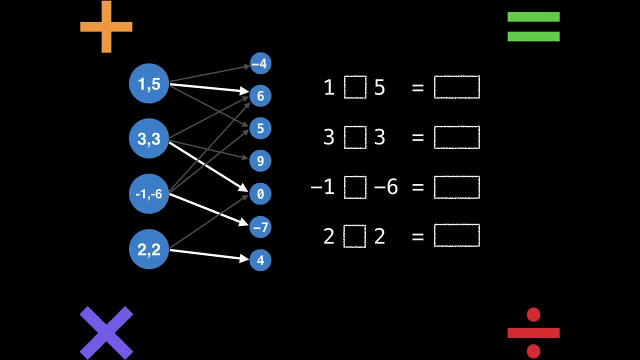 last thing we need to do is look at the matchings and figure out what operators were used. The first matching is the input pair: one five matched to six. So we ask ourselves which of the three operators- plus, minus or multiply- results in one five equaling six. So we try. 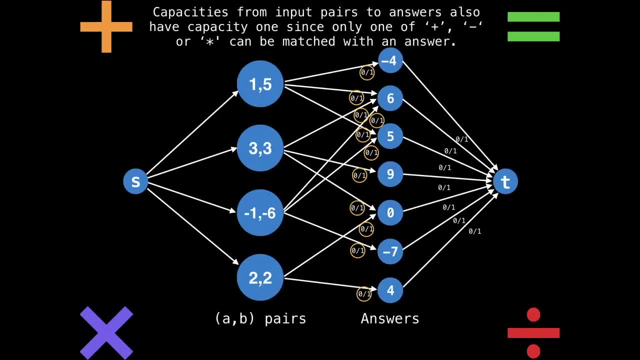 pairs to answers should also have a capacity of one, since only one of plus minus two is unique, or multiply should actually be matched to an answer. capacities from the source to the input pairs should reflect the frequency of the input pair. In this example, all frequencies. 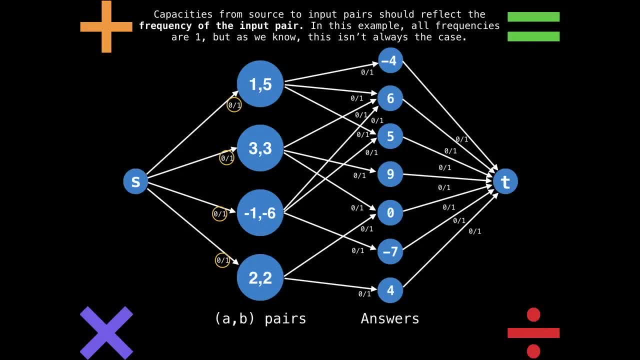 are one, But, as we know, that's not always the case. Now the flow graph is set up, let's run a max flow algorithm on it. The flow algorithm does its thing and some edges are filled with flow. These are the edges that were selected to be part of the maximum flow From this. 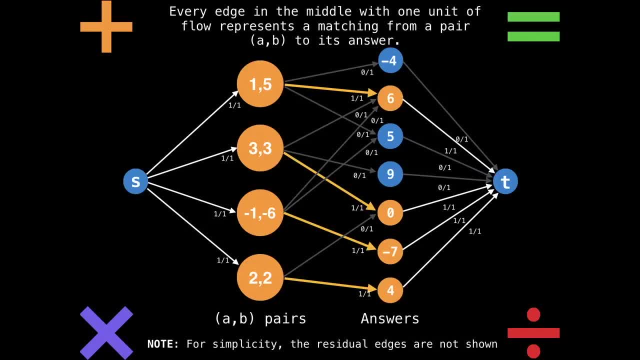 we can derive what the matching was. More specifically, we're interested in the middle edges. Those are the edges which give us information about the matching. Every edge in the middle with one unit of flow represents a matching from an input pair a, B to its answer For. 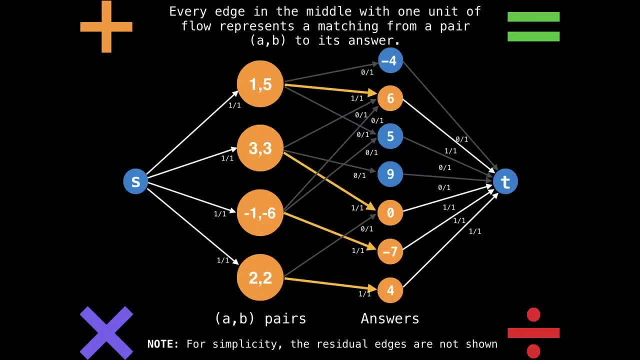 example, the input pair one, five was matched to the answer, node six, Because there's one unit of flow going through that edge. From this we can even deduce the operator used for each matching, which is actually needed for the final output. This: 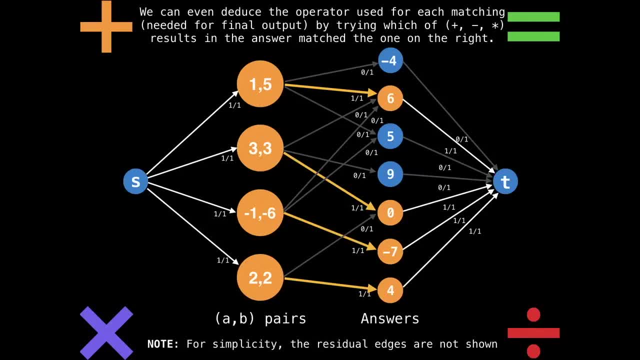 can be done by trying which of the plus, minus or multiply operators results in the found matching. Basically, we first solve the problem by figuring out which answers we get and then work backwards to figure out which operator was used. In theory, we could tag each of. 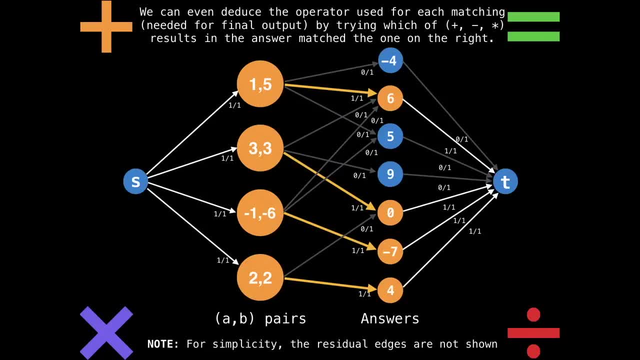 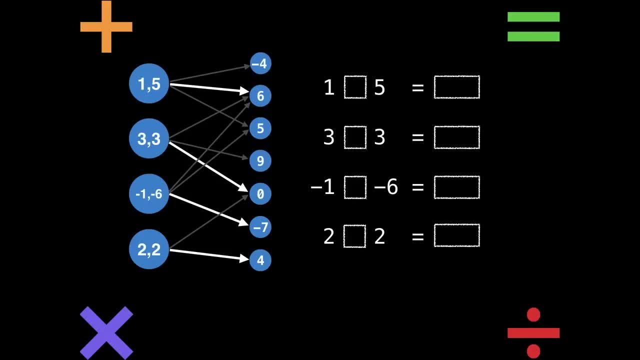 each middle edge with what operator was used. but I didn't bother doing that. It's a. it's more work. Let's wrap up this problem. The last thing we need to do is look at the matchings and figure out what operators were used. The first matching is the input pair, one five. 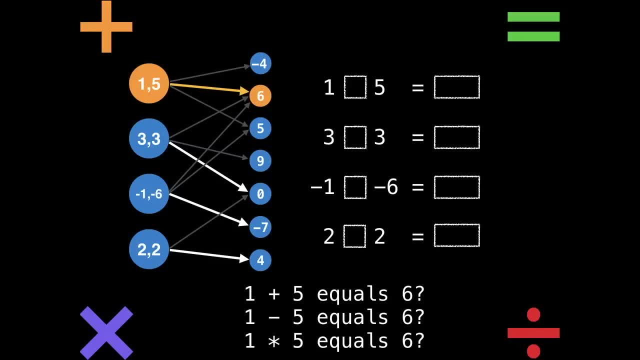 matched to six. So we ask ourselves which of the three operators- plus, minus or multiply- results in one five equaling six. So we try all three options and we figure out that, hey, one plus five is six, So the operator is the plus. then we move on to the next pair And 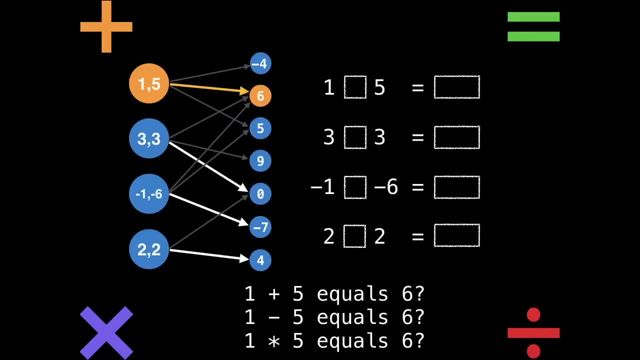 all three options and we figure out that hey, one plus five is six, So the operator is the plus. then we move on to the next pair And then we do the same thing. If there are multiple operators that result in the right answer, pick any of them And that's basically it. 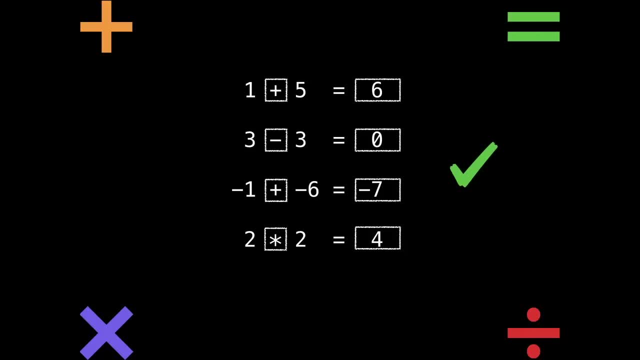 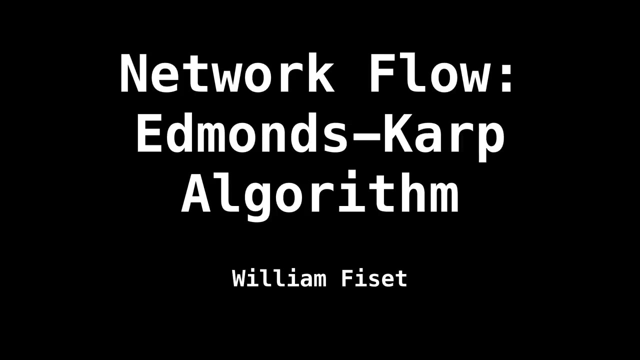 we can verify that all our operators yield the correct result and that all our answers are unique. I didn't go into great detail on how to support multiple repeated pairs, But I'll leave that as an exercise to the future For the listener. Today we're going to probe even further into network flow. we're going 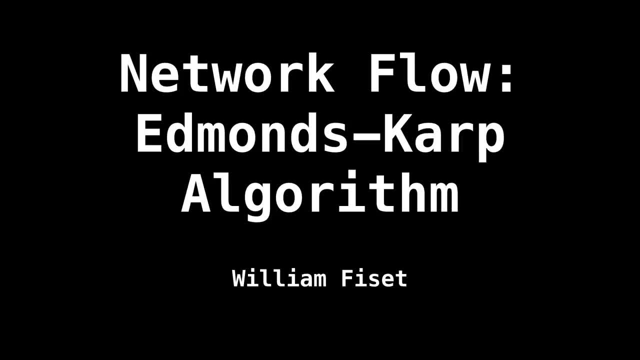 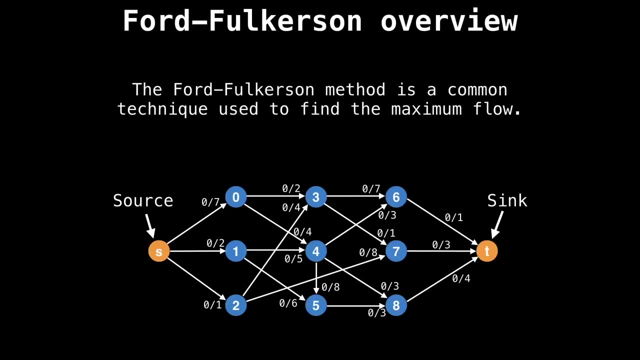 to be talking about a specific implementation of the Ford Fulkerson method, which is the Edmonds Karp algorithm. Edmonds Karp is another maximum flow algorithm which uses a different technique to find augmenting paths through the flow graph. Before we get started, let 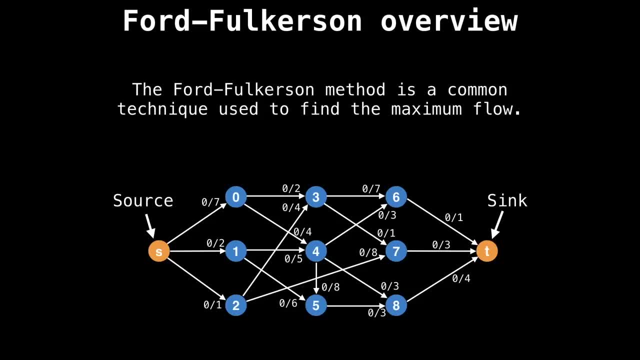 me give you a refresher on what we're trying to do. We are trying to find the maximum flow graph, And by finding the maximum flow on a flow graph, because we know that finding the maximum flow is really useful for finding bipartite matchings and also to solve a whole. 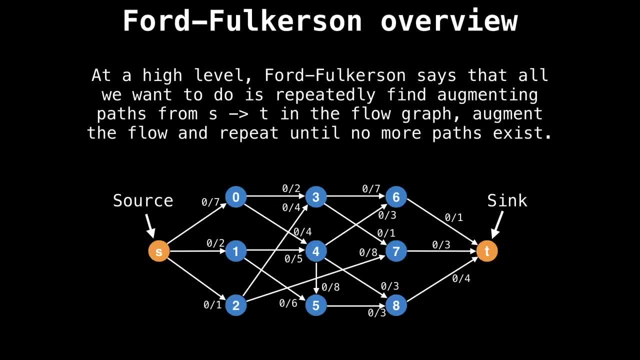 host of problems So far. we've looked at one other technique to find the maximum flow, which is to use the Ford Fulkerson method with a depth first search At a high level. it says that all we want to do is repeatedly find augmenting paths from the source to the 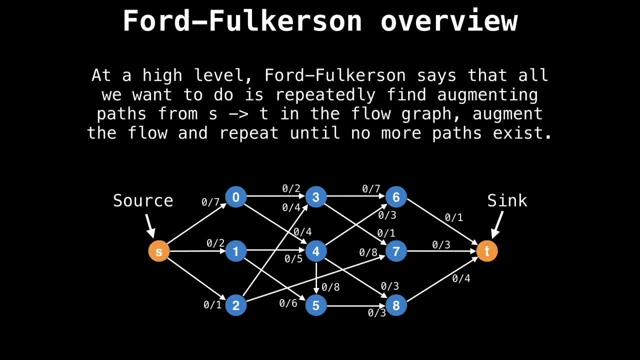 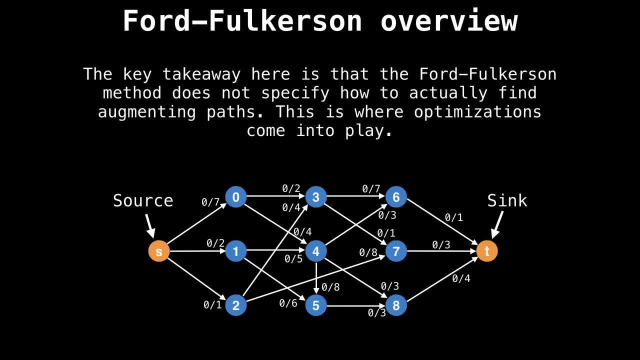 sink the flow and then repeat this process until no more paths exist. The key takeaway here is that the Ford Fulkerson method does not specify how to actually find these augmenting paths, So this is where we can optimize the algorithm. A few videos ago, we saw that the 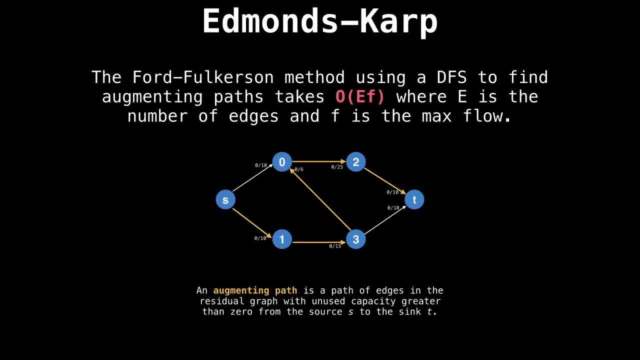 Ford Fulkerson method can be implemented with a depth first search to find the maximum flow. However, the pitfall with that technique was that the time complexity depended on the capacity values of the edges in the graph. This is because the depth first search picks. 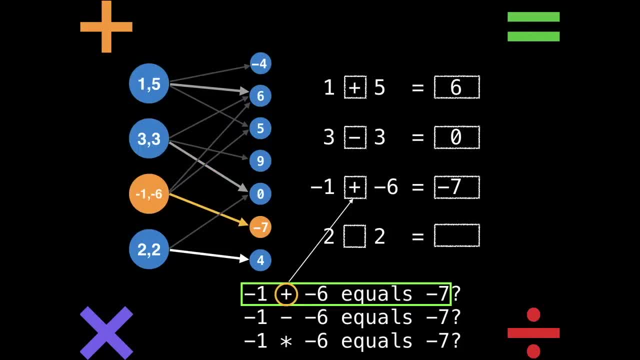 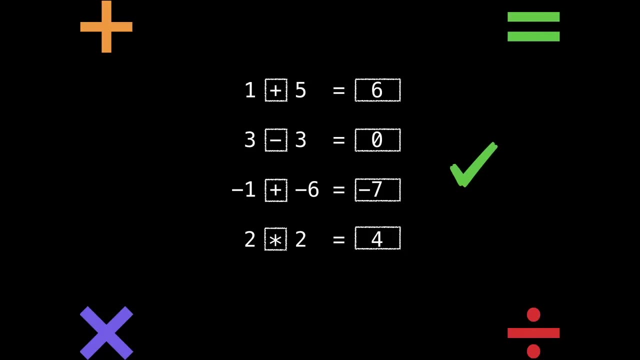 then we do the same thing. If there are multiple operators that result in the right answer, pick any of them And that's basically it. we can verify that all our operators yield the correct result and that all our answers are unique. I didn't go into great detail. 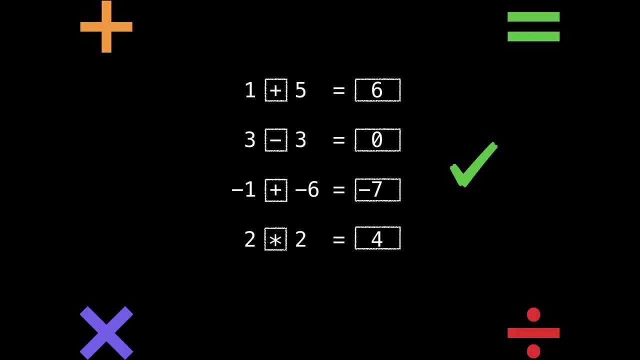 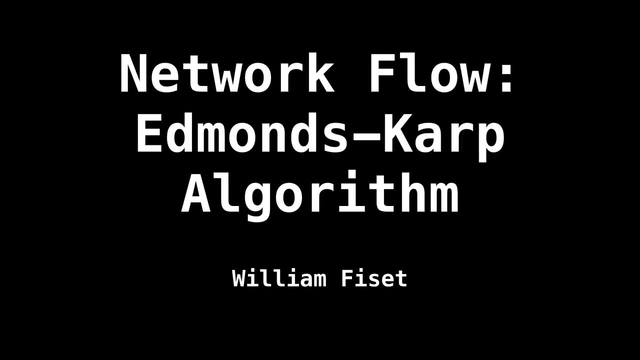 on how to support multiple repeated matches pairs, but I'll leave that as an exercise to the listener. Today we're going to probe even further into network flow. we're going to be talking about a specific implementation of the Ford Fulkerson method, which is the Edmonds Karp algorithm. Edmonds Karp is another. 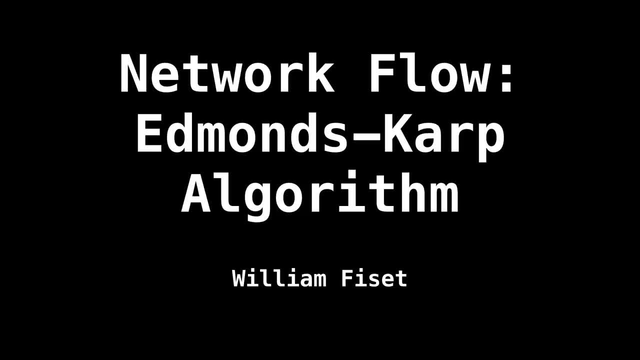 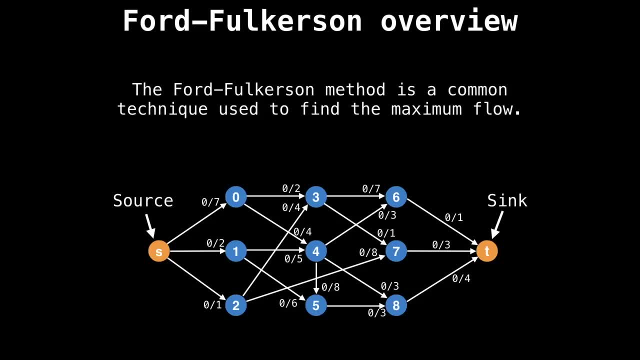 maximum flow algorithm, which uses a different technique to find augmenting paths through the flow graph. Before we get started, let me give you a refresher on what we're trying to do. We are trying to find the maximum flow on a flow graph because we know that finding. 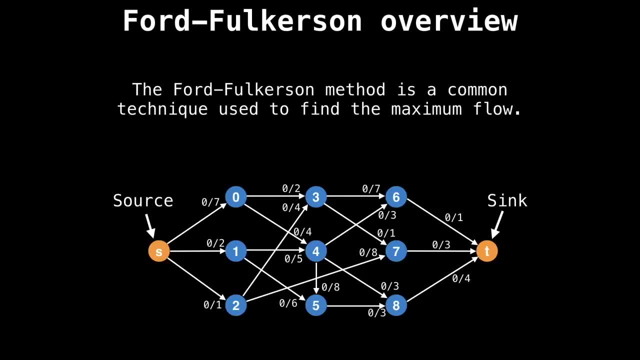 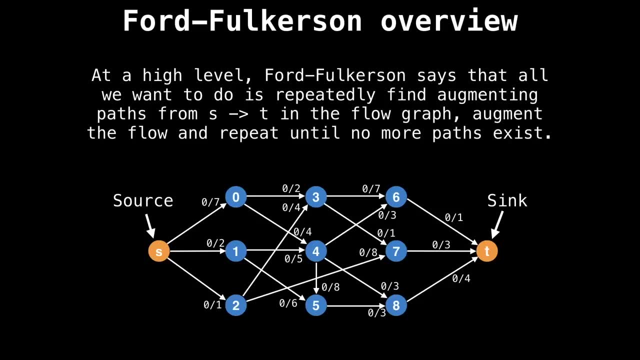 the maximum flow is really useful for finding bipartite matchings and also to solve a whole host of problems. So far, we've looked at one other technique to find the maximum flow, which is to use the Ford Fulkerson method with a depth first search At a high level. 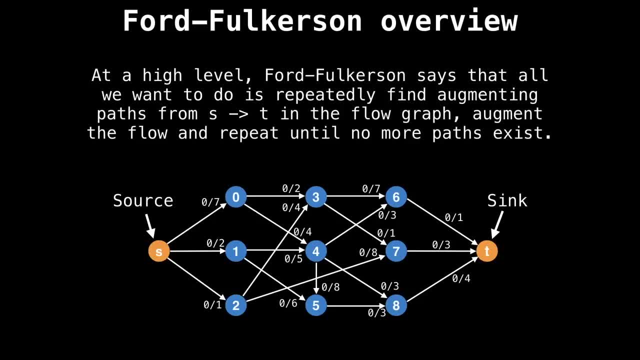 it says that all we want to do is repeatedly find augmenting paths From the source to the sink, augment the flow and then repeat this process until no more paths exist. The key takeaway here is that the Ford Fulkerson method does not specify. 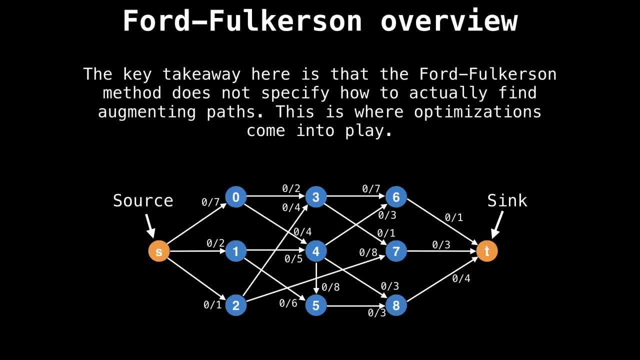 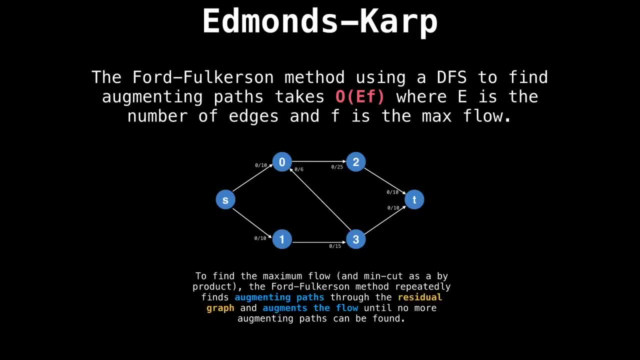 how to actually find these augmenting paths. So this is where we can optimize the algorithm. A few videos ago, we saw that the Ford Fulkerson method can be implemented with a depth first search to find the maximum flow. However, the pitfall is that we can't find the maximum. 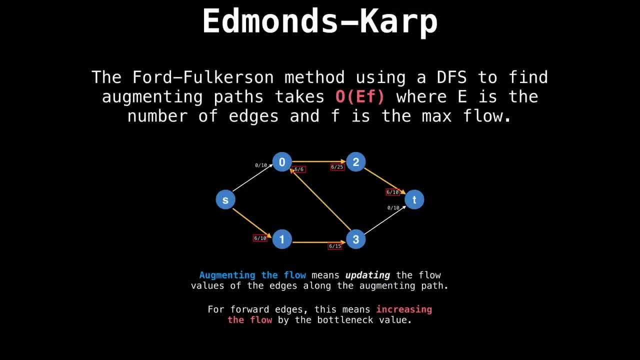 flow. The pitfall with that technique was that the time complexity depended on the capacity values of the edges in the graph. This is because the depth first search picks edges to traverse in such a way that we might only ever be able to push one unit of flow in each iteration. 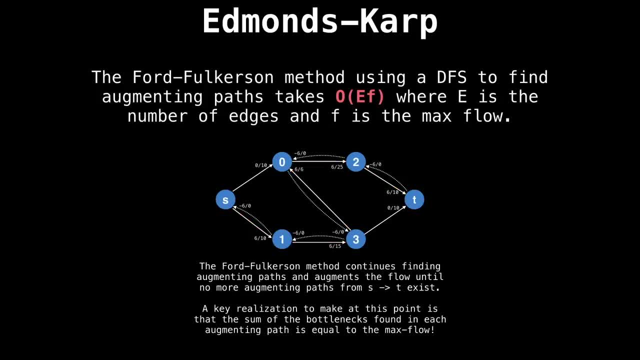 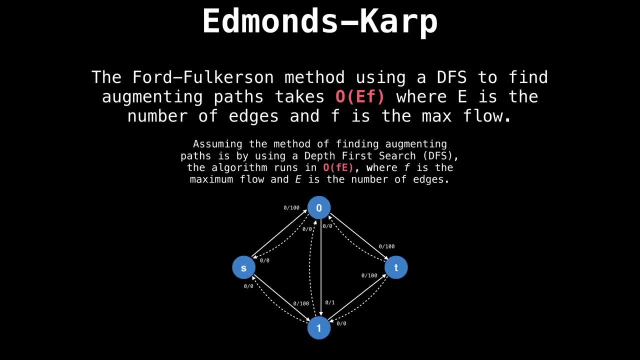 edges to traverse in such a way that we might only ever be able to push one unit of flow in each iteration. This is really bad and can kill the time complexity, even though it's highly unlikely to happen in practice, But it's absolutely something that we can do. 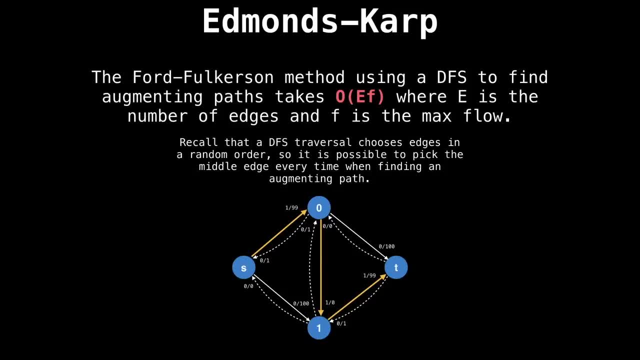 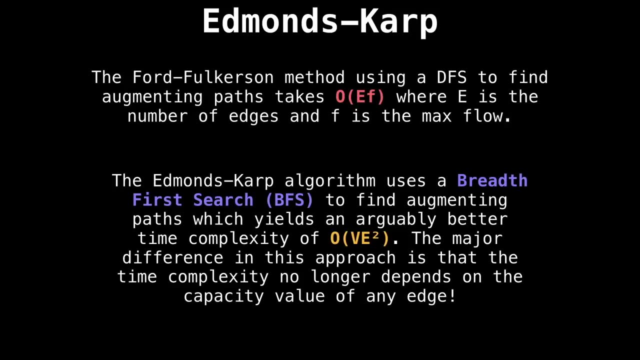 It's something we want to avoid, should it happen Right now. the time complexity of Ford Fulkerson with a depth first search is big. O of E times F, where E is the number of edges and F is the maximum flow. The idea behind Edmonds Karp says that instead of using a 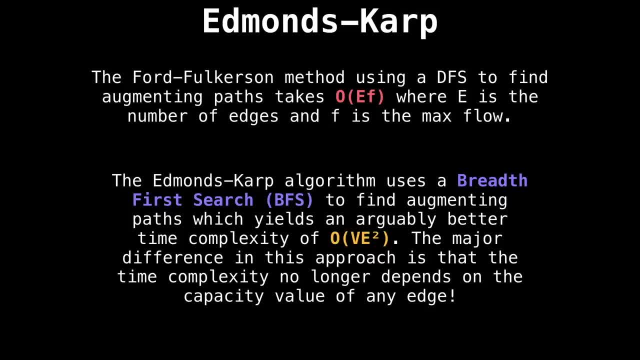 depth first search to find augmenting paths. we should use a breadth first search instead to get a better time complexity. big O of V times e squared. It may not look like a better time complexity, but it actually is. What's different is that. 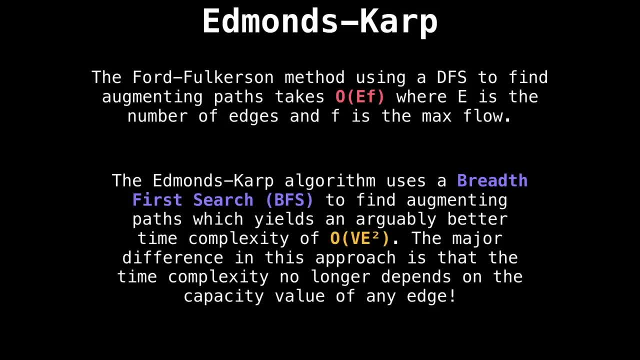 the time. complexity, while it might not look great, does not depend on the capacity value of any edge in the flow graph, which is crucial. We call such an algorithm that doesn't depend on the actual input values a strongly polynomial algorithm, And that's exactly what Edmonds. 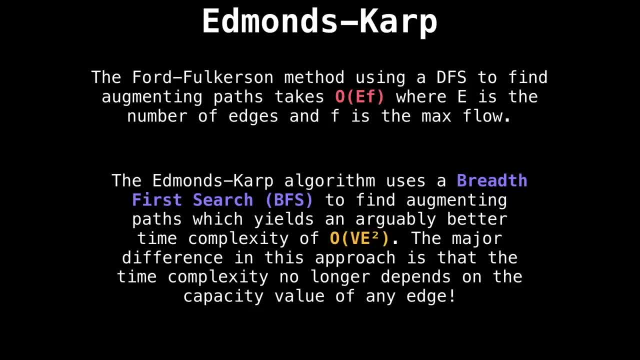 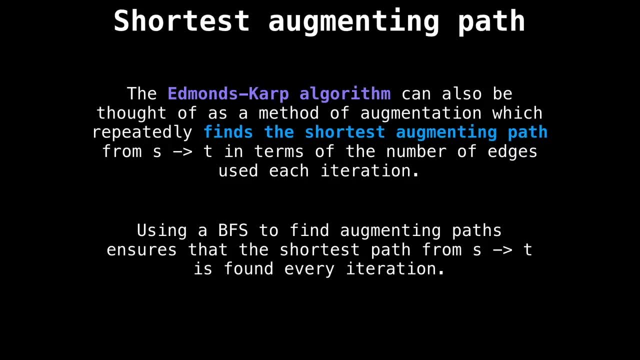 Karp is and why it was so revolutionary at the time. Edmonds Karp can also be thought of as an algorithm which finds the shortest augmenting path from s to t, that is, in terms of the number of edges used in each iteration, Using a breadth first. 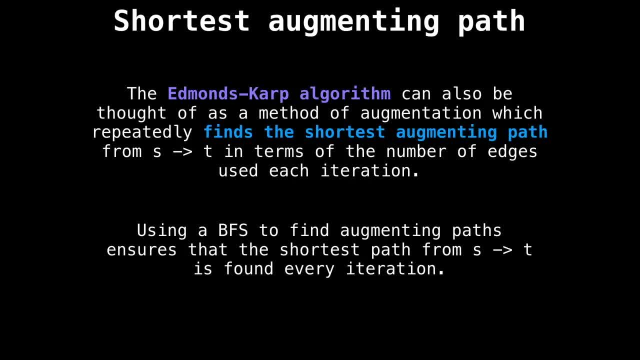 search during Edmonds Karp ensures that we find the shortest path. This is a consequence of each edge being unweighted. When I say unweighted, I mean that as long as the edge has a positive capacity, we don't distinguish it between one edge being any better or worse. 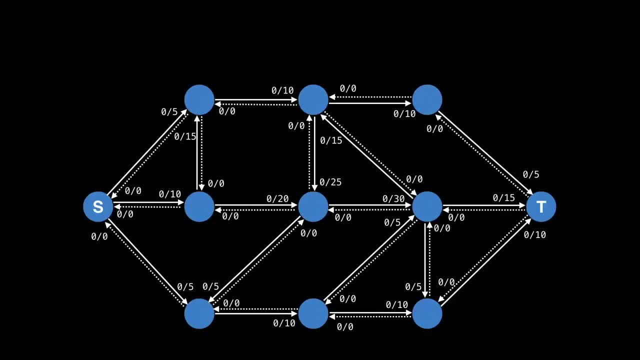 worse than any other edge. Now let's look at why we might care about using Edmonds Karp. Suppose we have this flow graph and we want to find what the maximum flow is. If we're using a depth first search, we might do something like this: Start at the source and do a random. 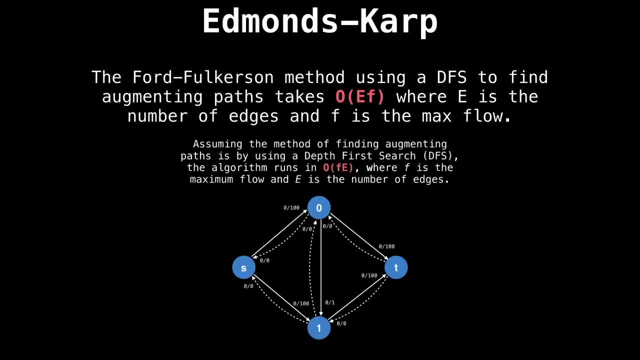 This is really bad and can kill the time complexity, even though it's highly unlikely to happen in practice, But it's absolutely something we want To avoid should it happen right now. the time complexity of Ford Fulkerson with a depth first search is big O of E times F, where E is the number of edges and F is the maximum. 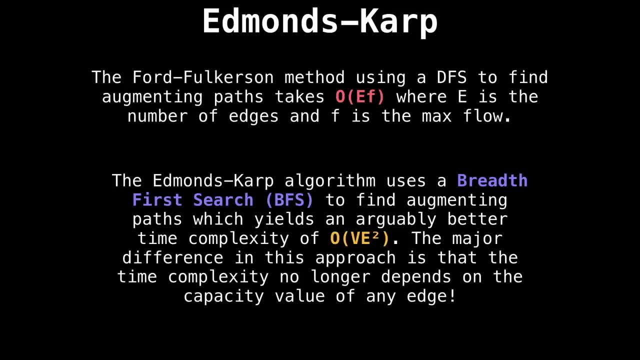 flow. The idea behind Edmonds Karp says that instead of using a depth first search to find augmenting paths, we should use a breadth first search instead to get a better time complexity. big O of V times e squared Main. It may not look like a better time complexity, but it actually is. What's different is that. 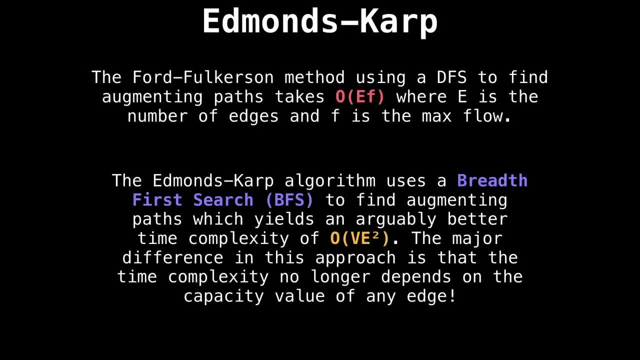 the time. complexity, while it might not look great, does not depend on the capacity value of any edge in the flow graph, which is crucial. We call such an algorithm that doesn't depend on the actual input values a strongly polynomial algorithm, And that's exactly what Edmonds. 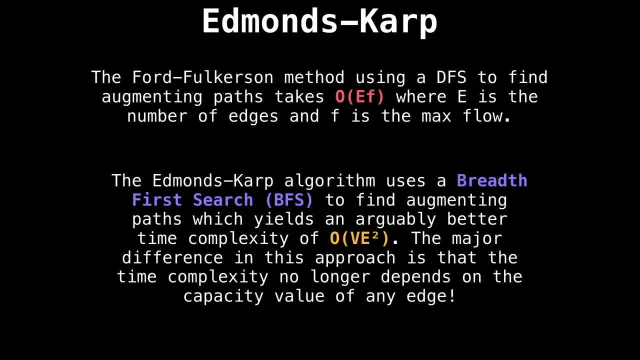 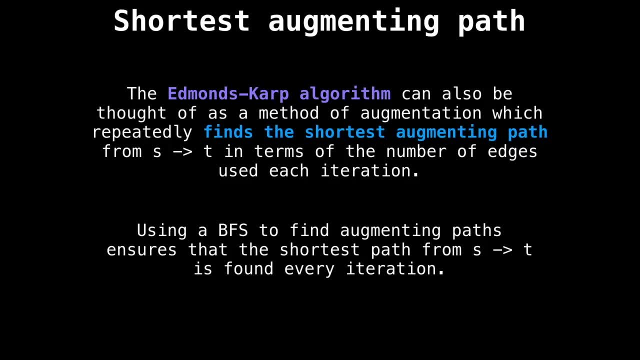 Karp is and why it was so revolutionary at the time. Edmonds Karp can also be thought of as an algorithm which finds the shortest augmenting path from s to t, that is, in terms of the number of edges used in each iteration Using a breadth. first search during Edmonds. 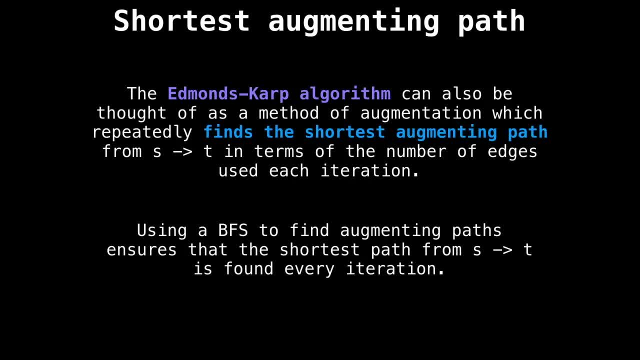 Karp ensures that we find the shortest path. This is a consequence of each edge being unweighted. When I say unweighted, I mean that, as long as the edge has a positive capacity, we don't distinguish it between one edge being any better or worse than the other edge, And that's. 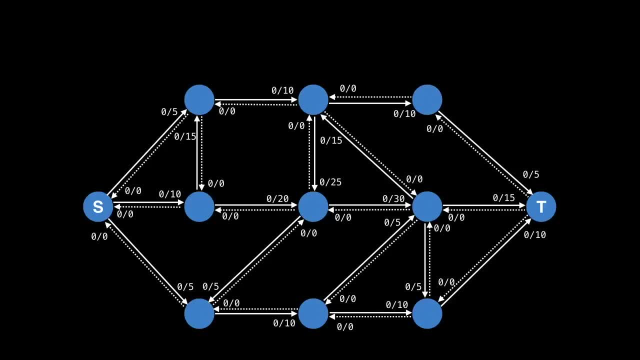 a lot less than any other edge. Now let's look at why we might care about using Edmonds Karp. suppose we have this flow graph and we want to find what the maximum flow is. If we're using a depth first search, we might do something like this: Start at the source. 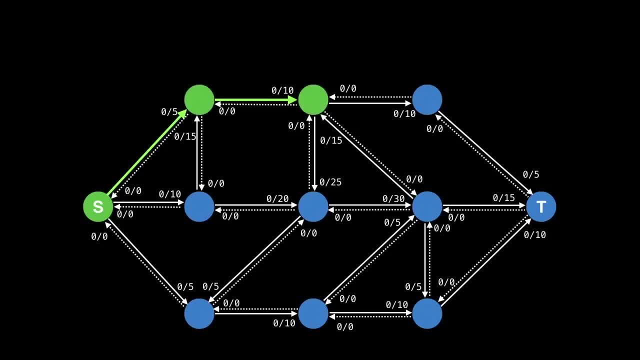 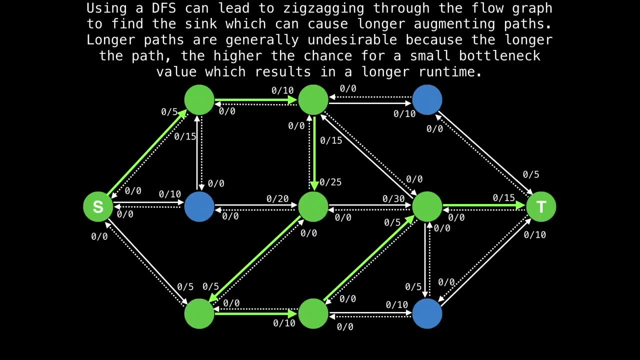 and do a random depth first search forwards. So after a lot of zigzagging through the search, through the flow graph, we are able to find the sink. As we just saw, a depth first search has the chance to cause long augmenting paths And longer paths are generally undesirable. 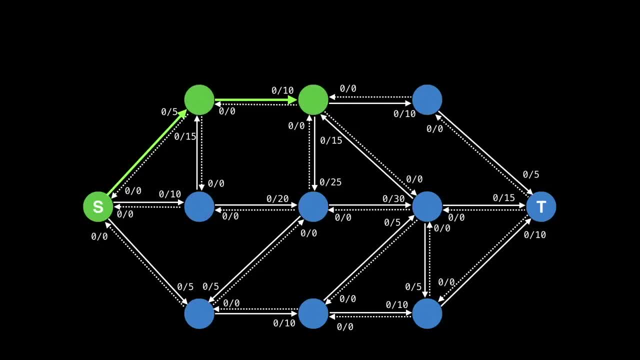 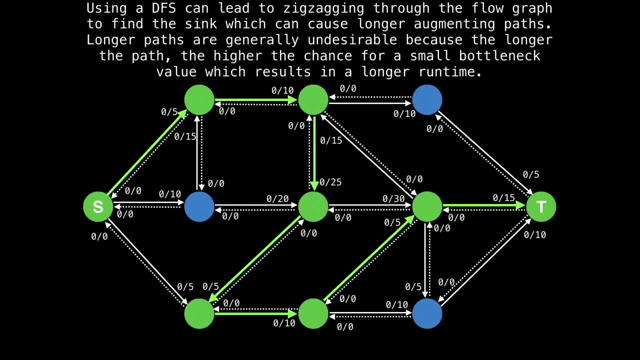 depth first search forwards, So by zigzagging through the flow graph we are able to find the sink. As we just saw, a depth first search has the chance to cause long, augmenting paths, And longer paths are generally undesirable because the longer the path, the higher the chance for a small bottleneck value. 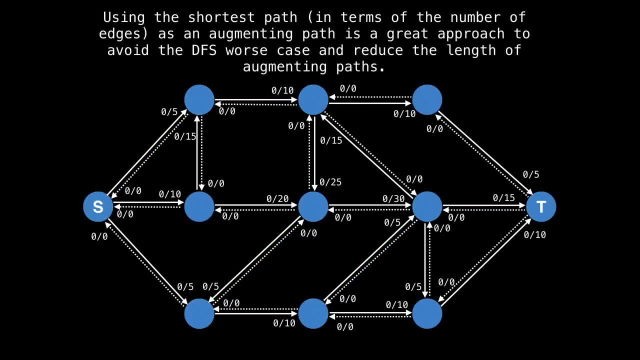 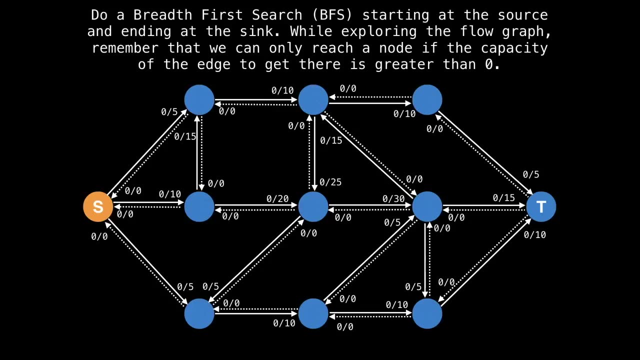 which results in a longer runtime. Finding the shortest path from s to t, again in terms of number of edges, is a great approach to avoid the depth first search worst case scenario and reduce the length of augmenting paths. To find the shortest path from s to t, do a. 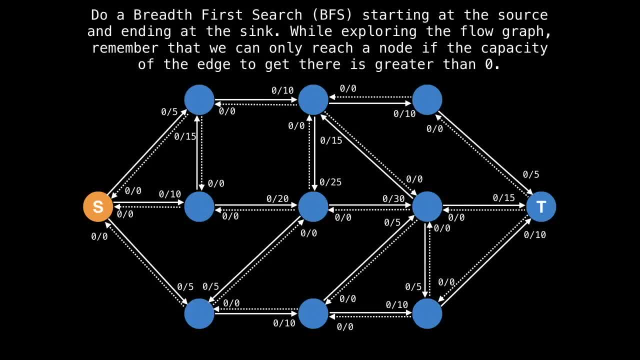 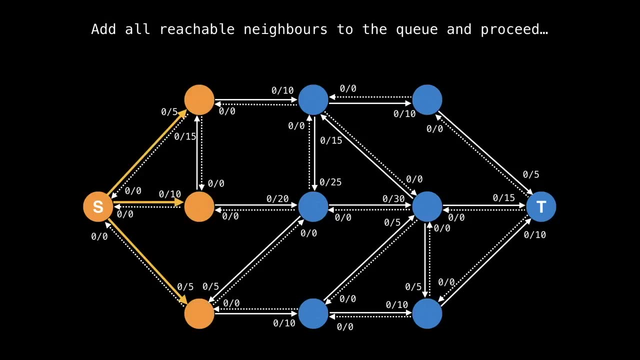 breath first search, starting at the source and ending at the sink. While exploring the flow graph, remember that we can only take an edge if the remaining capacity of that edge is greater than zero. In this example, all edges outwards from s have a remaining. 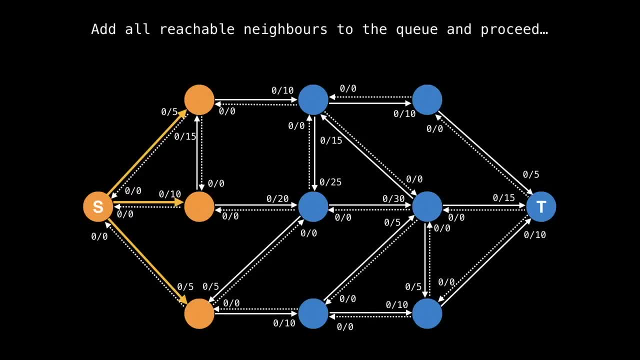 capacity greater than zero. So we can add all the neighbors to the queue when we're doing the breath first search. So we can only take an edge if the remaining capacity of the breath first search step And then we keep going forwards. So add all reachable. 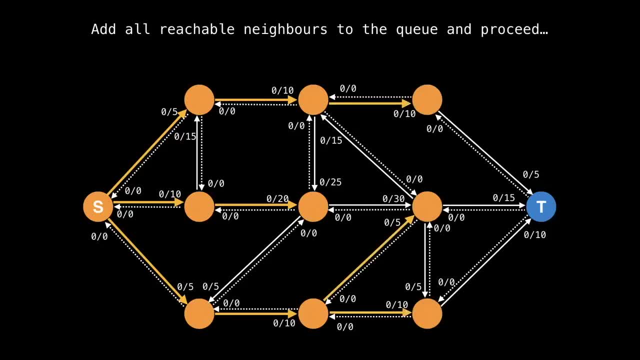 neighbors to the queue and continue. And now the breadth first search has reached the sink, so we can stop. In the real algorithm we would stop as soon as any of the edges reach the sink. But just for symmetry I show three edges here entering the sink, While in reality 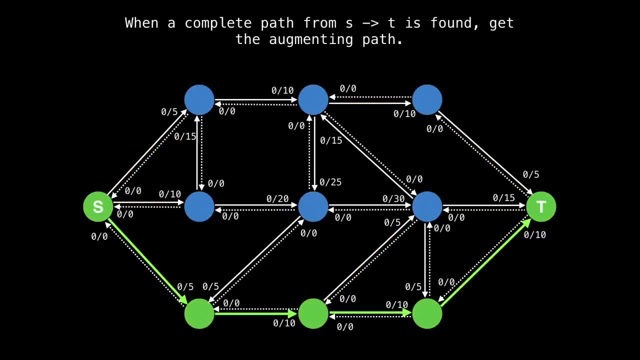 we would stop as soon as one of them reaches the sink. If we assume that the bottom edge made it to the sink first and we retrace the path, we get the following augmenting path. But we didn't just find any augmenting path, we found a shortest length augmenting path. So to augment the flow, do. 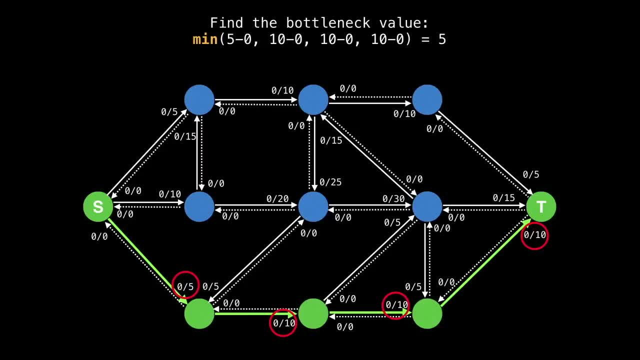 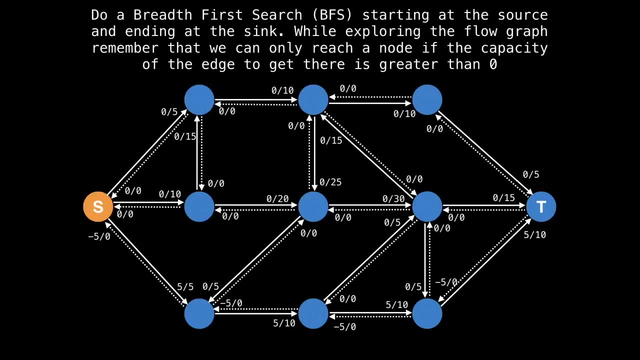 the usual: find the bottleneck value by finding the smallest remaining capacity of all the edges along the path, then augment the flow values along the path by the bottleneck. So that was the first path. However, we're not done yet. Let's continue finding paths until the entire graph is saturated. Recall that. 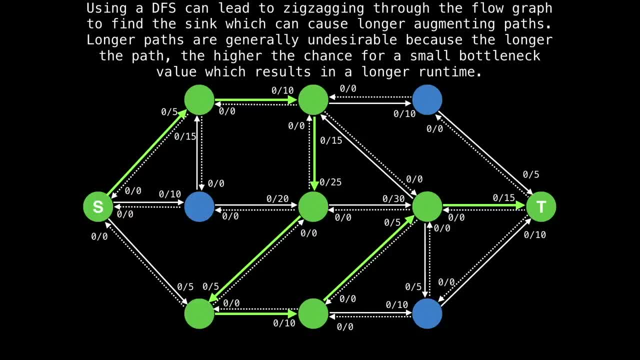 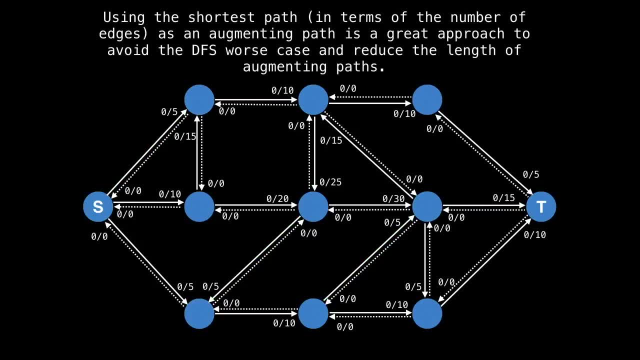 because the longer the path, the higher the chance for a small bottleneck value which results in a longer runtime. Finding the shortest path from s to t, again in terms of number of edges, is a great approach to avoid the depth first search worst case scenario and 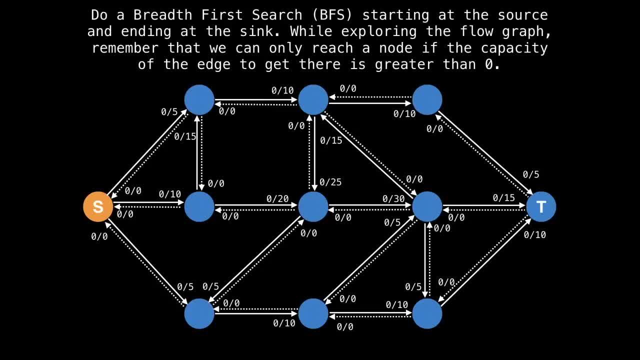 reduce the length of the search, length of augmenting paths to find the shortest path from s to t, do a breadth first search, starting at the source and ending at the sink. While exploring the flow graph, remember that we can only take an edge if the remaining capacity of that edge is greater than zero. 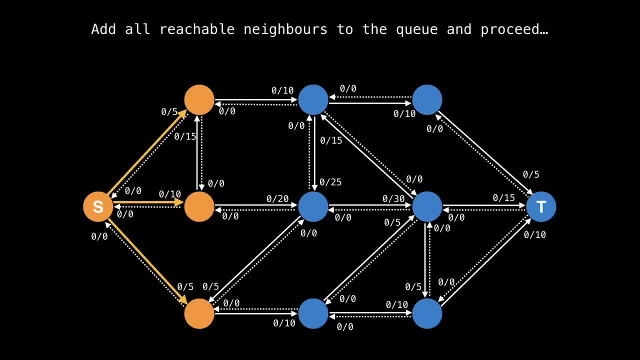 In this example, all edges outwards from s have a remaining capacity greater than zero, So we can add all the neighbors to the queue when we're doing the breadth first search step And then we keep going forwards. So add all reachable neighbors to the queue and continue. 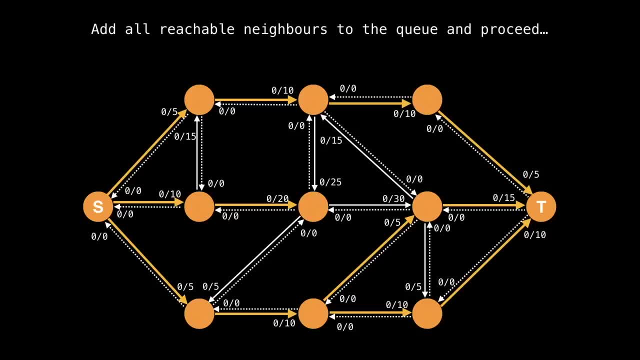 And now the breadth first search has reached the sink, So we can stop. In the real algorithm we would stop as soon as any of the edges reach the sink. But just for symmetry I show three edges here entering the sink, While in reality we would stop as soon as one of 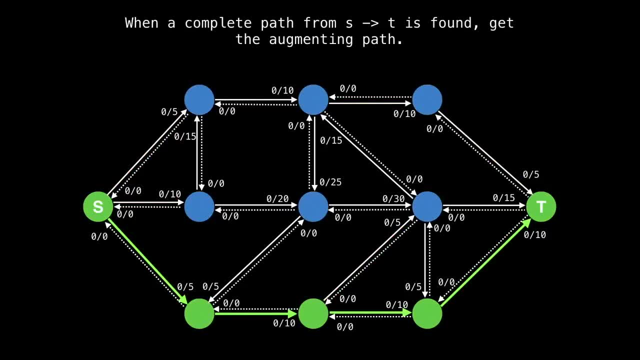 them reaches the sink. So we can stop as soon as one of the edges reaches the sink. If we assume that the bottom edge made it to the sink first and we retrace the path, we get the following augmenting path. But we didn't just find any augmenting path, we found a shortest length augmenting. 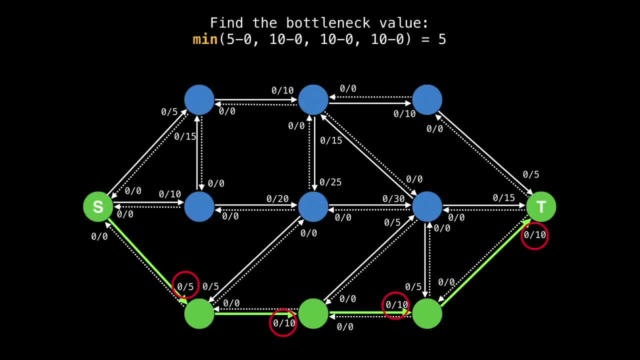 path. So to augment the flow, do the usual: find the bottleneck value by finding the smallest remaining capacity of all the edges along the path, then augment the flow values along the path by the bottleneck. So that was the first path. However, we're not done yet. Let's 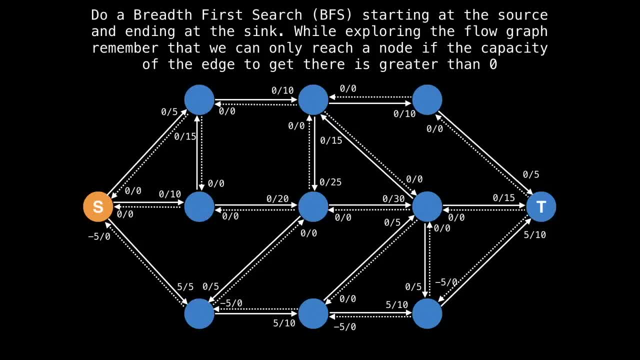 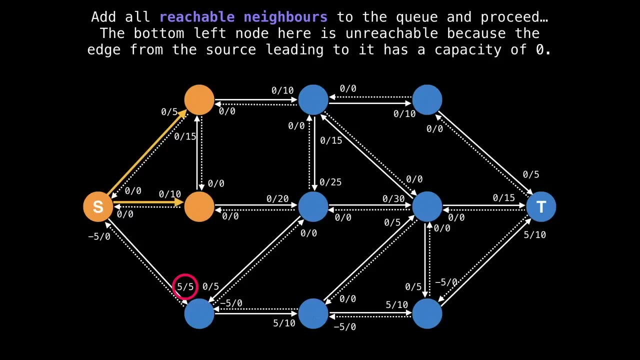 continue finding paths until the entire graph is saturated. Recall that while exploring the flow graph, we can only reach a node if the remaining capacity of the edge to get to that node is greater than zero. For instance, all the reachable neighbors of the source node. 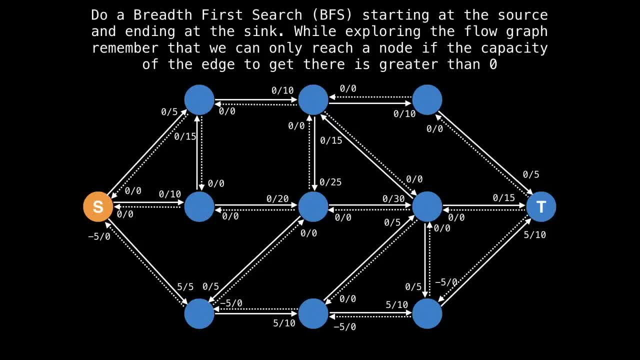 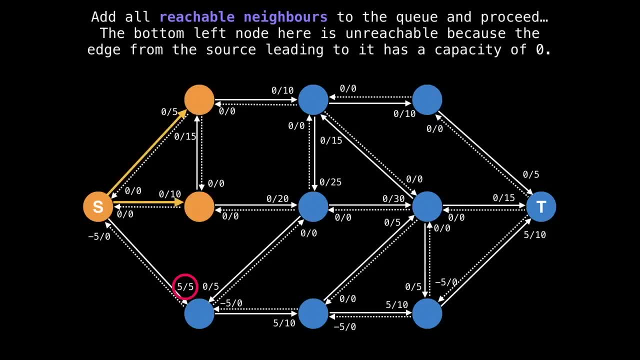 while exploring the flow graph, we can only reach a node if the remaining capacity of the edge to get to that node is greater than zero. For instance, all the reachable neighbors of the source node. in this case does not include the bottom left node, because the edge from 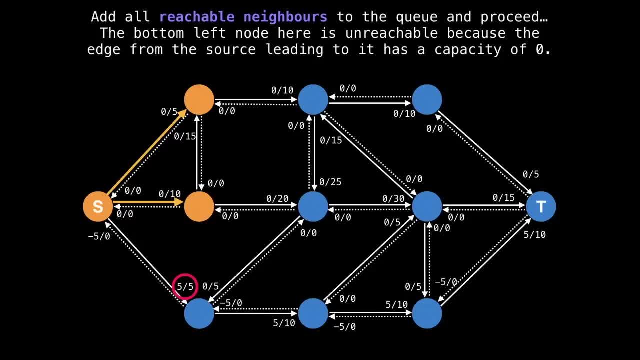 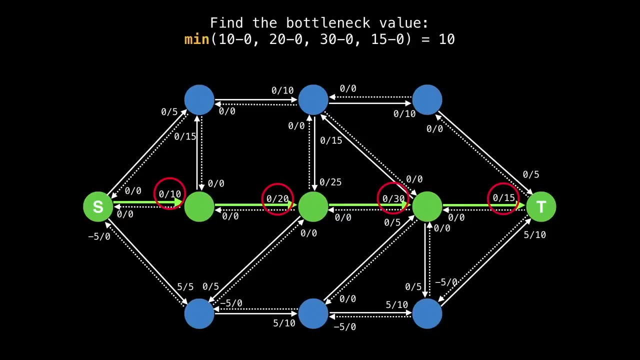 the source to the bottom left node has a remaining capacity of zero. All right, keep exploring until the sink is reached. And now we've reached the sink once more. So find the bottleneck value along this path. Then use the bottleneck value to update. 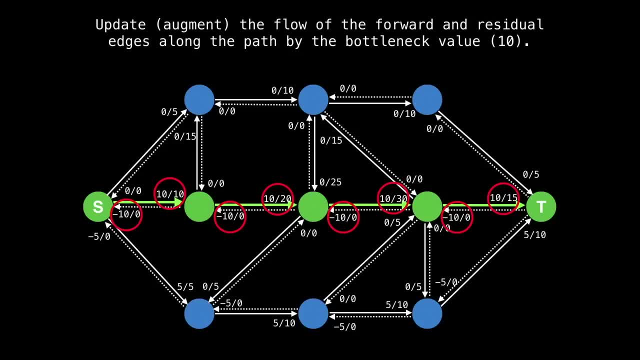 the flow along the augmenting path, Don't forget to update the residual edges. And we're still not done because there still exists Another augmenting path. So now there only exists one edge outwards from the source with a capacity greater than zero, So it's the only edge we can take. So we follow it. There's. 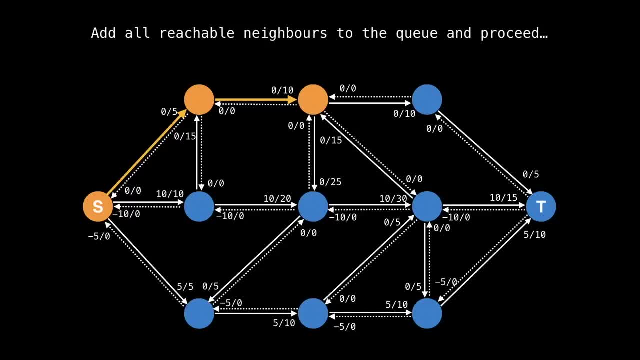 also only one edge to follow from the second node, because the other edges have a remaining capacity of zero. And now the breadth first search has reached the sink. we can trace back the edges that were used. we can find the bottleneck by finding the minimum capacity along the path and also augment. 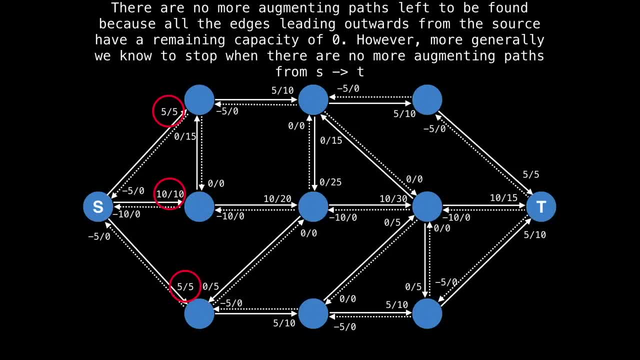 the flow, And now you can see that there are no more augmenting paths left to be found, because all the edges leading outwards from the source have a remaining capacity of zero. However, more generally, we know to stop Edmonds Karp when there are no more augmenting paths. 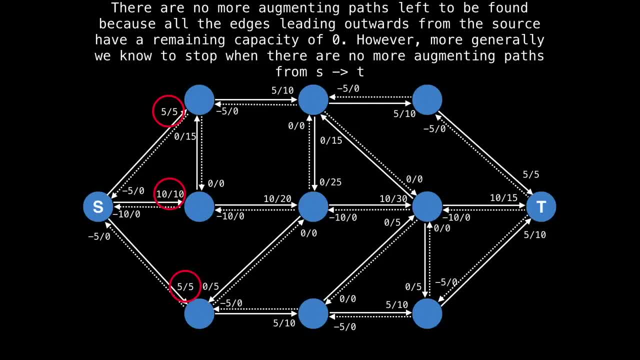 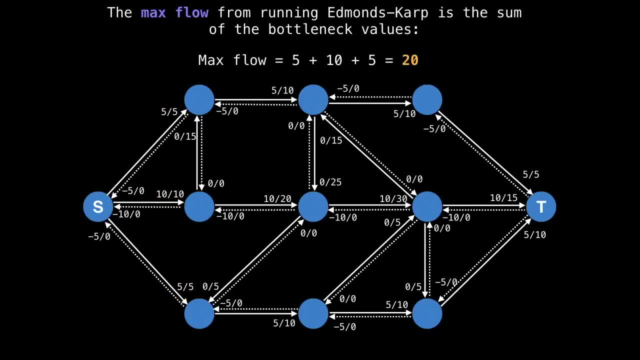 from s to t because we know we cannot increase the flow anymore. If this is the case, the maximum flow we get from running Edmonds Karp is the sum of the bottleneck values. If you recall, in the first iteration we were able to push five units of flow and the second. 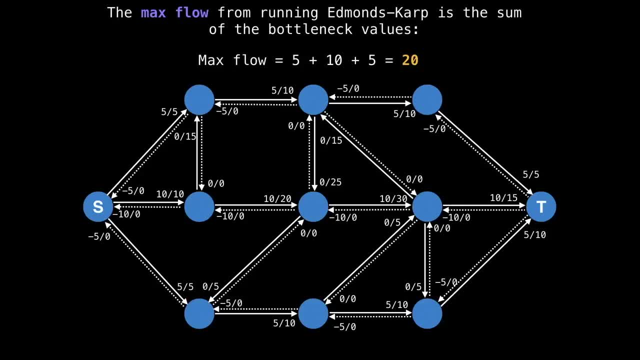 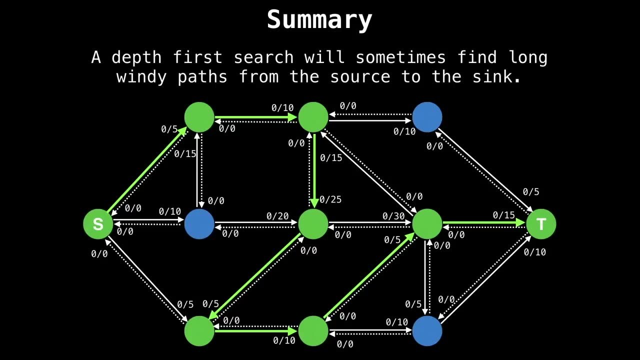 iteration, 10 units and then the last iteration, five units, for a total of 20 units of flow. Another way to find the maximum flow is to sum the capacity values going into the sink, which I have circled in red. In summary, this is what we learned using depth first. 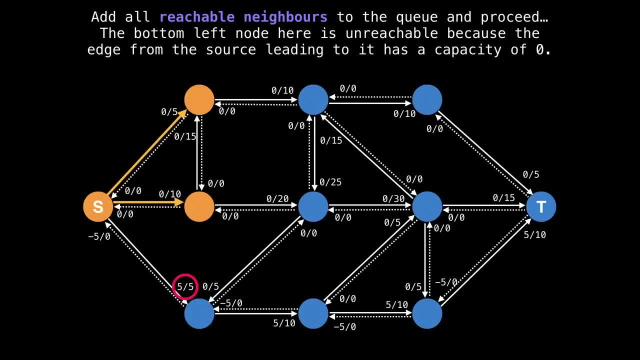 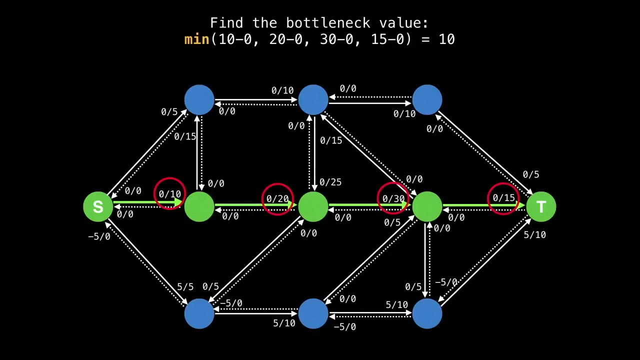 in this case does not include the bottom left node, because the edge from the source to the bottom left node has a remaining capacity of zero. Alright, keep exploring until the sink is reached. And now we've reached the sink once more, So find the bottleneck value along this path. 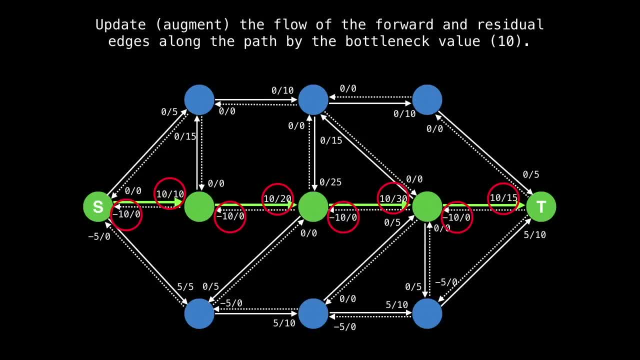 Then use the bottleneck value to update the flow along the augmenting path. Don't forget to update the residual edges, And we're still not done because there still exists another augmenting path. So now there only exists one edge outwards from the source with a capacity greater than 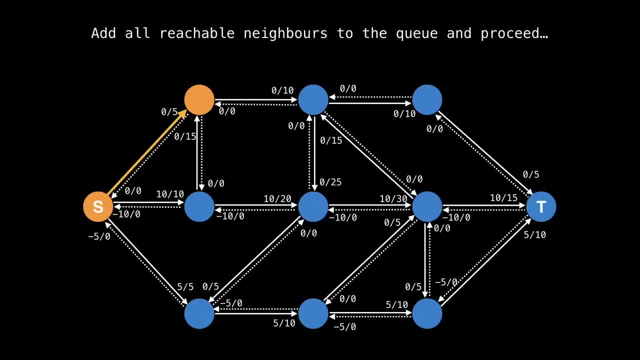 zero. So it's the only edge we can take, So we follow it. There's also only one edge to follow from the second node, because the other edges have a remaining capacity of zero. And now the breadth first search has reached the sink. we can trace back the edges that were. 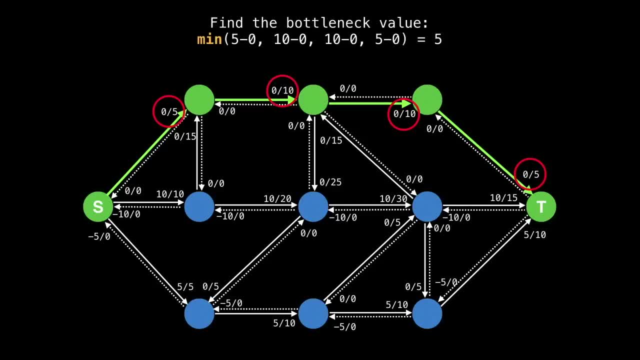 used. We can find the bottleneck by finding the minimum capacity of the sink, And now we can trace back the edges that were used. We can find the bottleneck by finding the decrease in thepod sust graves not being inspire by our use, And now we can see that. 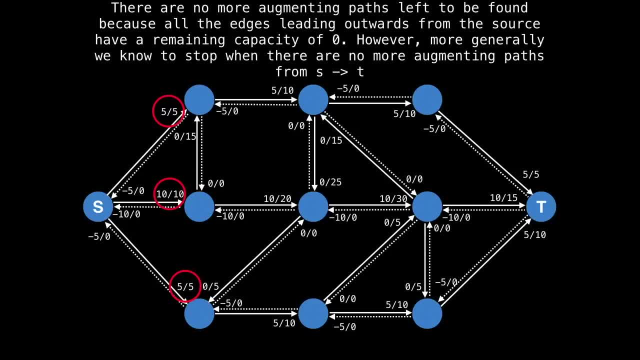 the path is no more augmenting paths left to be found, because all the edges leading outwards from the source have a remaining capacity of zero. However, more generally, we know to stop Edmonds carp when there are no more augmenting paths from s to t, because we know 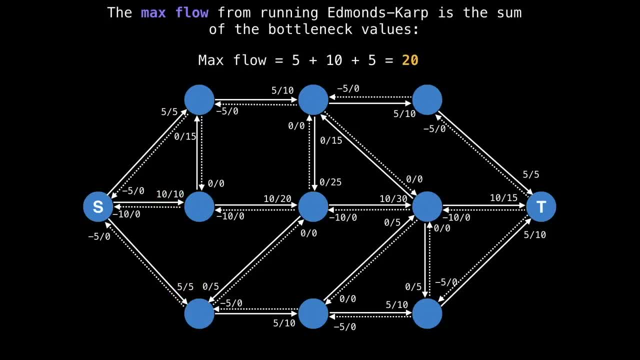 we cannot increase the flow anymore. If this is the case, the maximum flow we get from running Edmonds carp is the sum of the bottleneck values. If you recall, in the first iteration we were able to push five units of flow, in the second iteration 10 units and in the last iteration five units for a total. 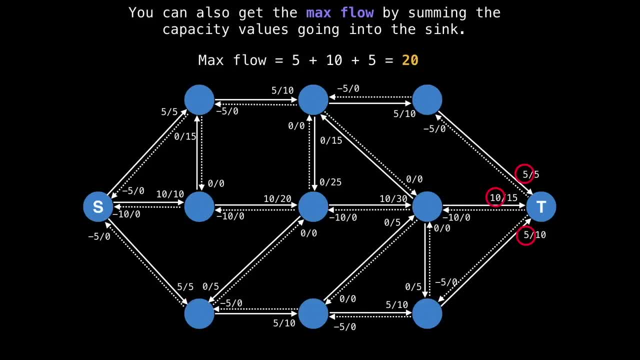 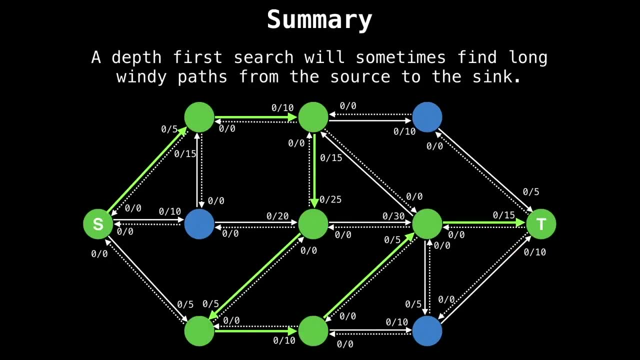 of 20 units of flow. Another way to find the maximum flow is to sum the capacity values going into the sink which I have circled in red. In summary, this is what we learned using depth. first search on a flow graph can sometimes find long, windy paths from the source. 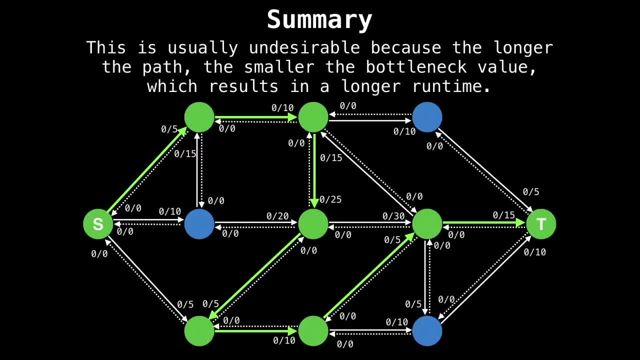 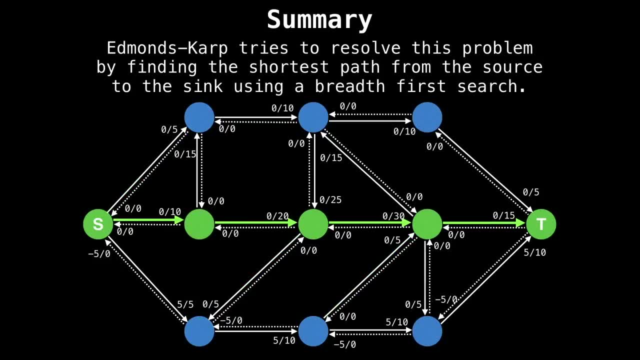 to the sink. This is usually undesirable because the longer the path, the smaller the bottleneck value and the longer the runtime. Edmonds Karp tries to resolve this problem by finding the shortest length, augmenting paths from the source to the sink using a breadth first. 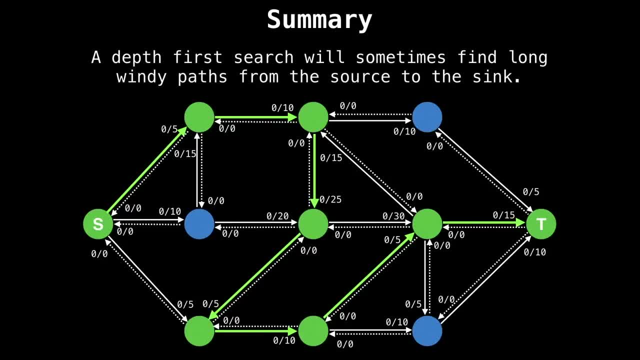 search on a flow graph can sometimes find long, windy paths from the source to the sink. This is usually undesirable because the longer the path, the smaller the bottleneck value and the longer the runtime. Edmonds Karp tries to resolve this problem by finding the shortest. 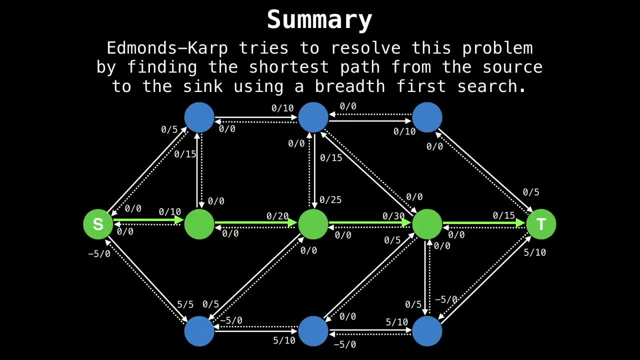 length, augmenting paths from the source to the sink using a breadth first search. However, more importantly, the big achievement of Edmonds Karp is that the length of the path is less than or equal to the length of the flow graph. And that's Edmonds Karp in a nutshell Today. 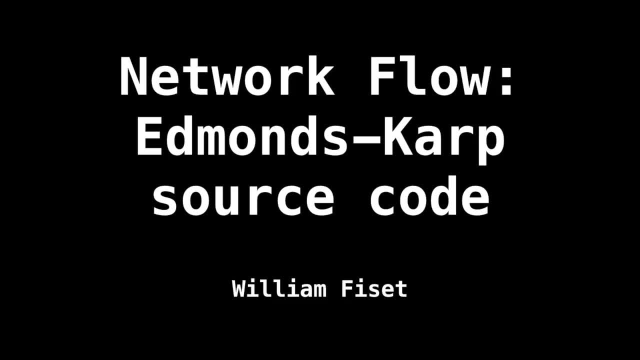 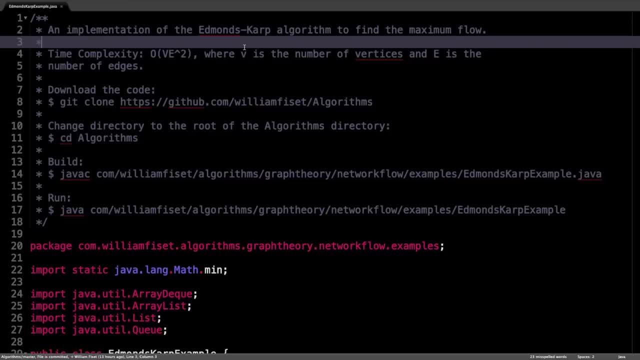 we're going to have a look at some source code for the Edmonds Karp algorithm. All right, here we are in the source code, written in Java. I've laid out some instructions here in the header in case you wanted to download the code, play around with it and run it yourself. 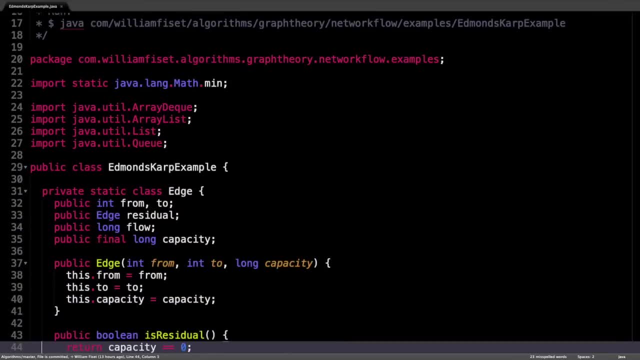 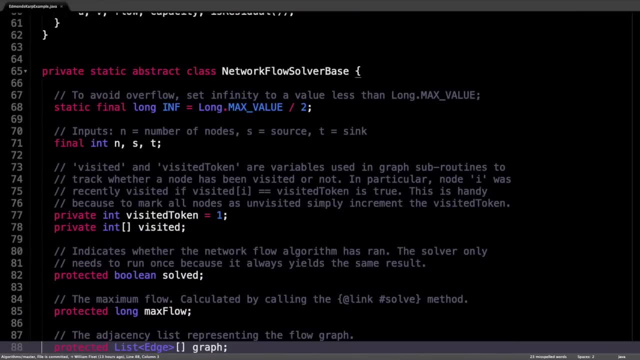 If I scroll down, you can see that we still have the same setup as before, with the edge class right here and the network flow base solver. But there is one important change I have made since the Ford fulkerson video, And that is I have added three new methods. 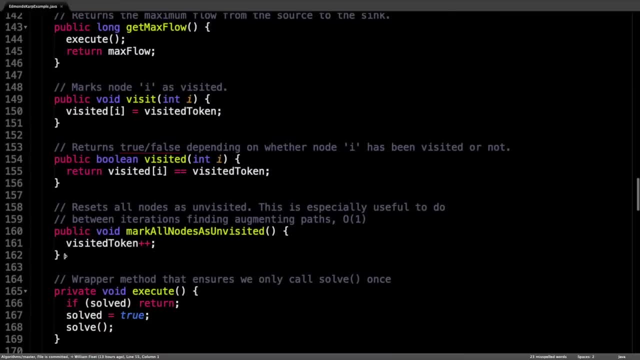 If we scroll down you can see that the three new methods are right here. The three methods I added abstract away visiting nodes and marking all of them. So if you have a look at this, nodes as unvisited. Now this is all done efficiently internally through the network flow based. 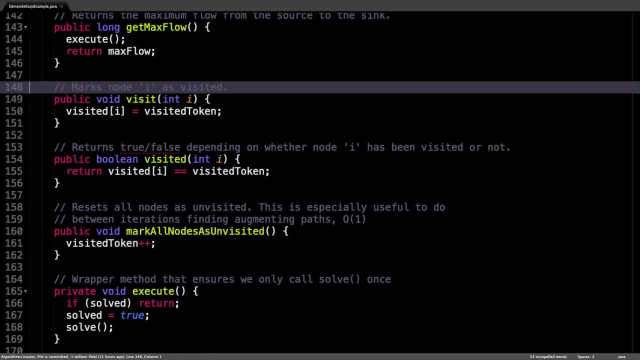 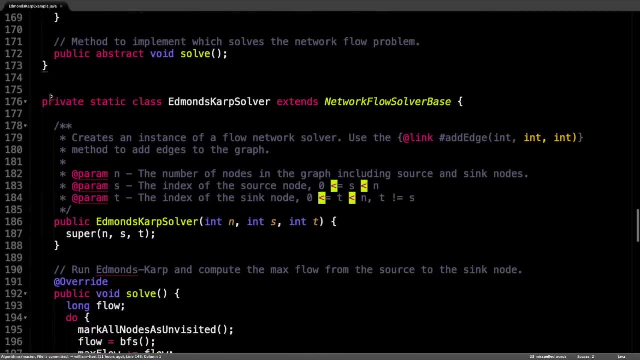 solver class using a visited token. you don't have to worry about It. also helps readability for anybody who's new to the code. Alright, now let's have a look at the Edmonds carp solver, which is the only thing different in this file. First, notice that the Edmonds 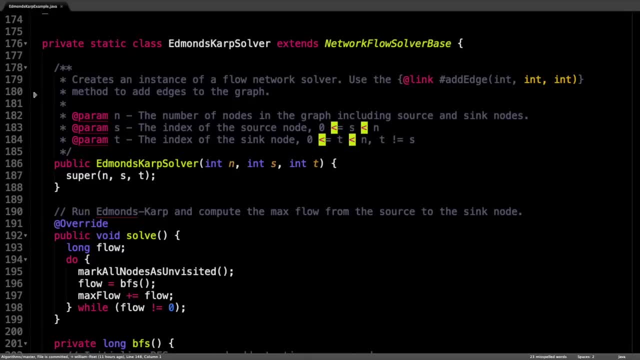 carp solver extends the network flow solver base. In doing so, we get a whole bunch of things for free, including the ability to construct a flow graph before we push flow through it In the constructor for the Edmonds carp solver. all I do is call the superclasses. 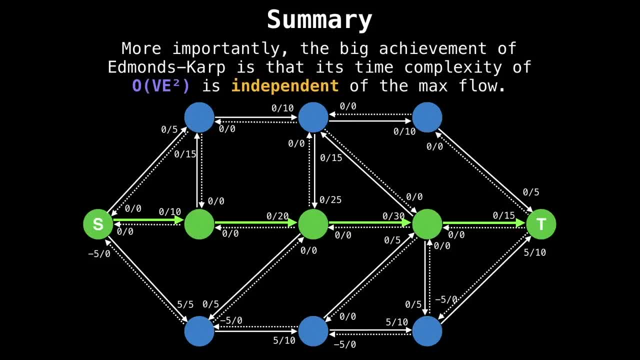 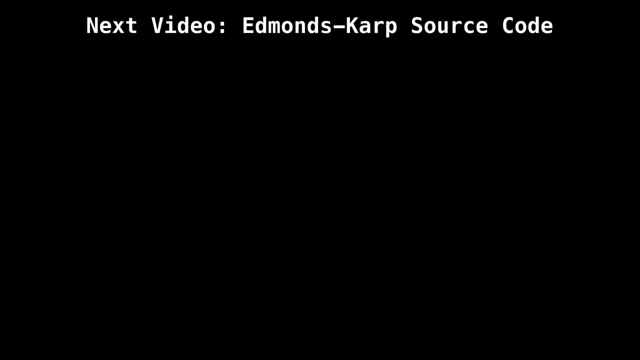 search. However, more importantly, the big achievement of Edmonds Karp is that it's time complexity of big O, of v times. E search squared is independent of the max flow, So it doesn't depend on the capacity values of the flow graph. And that's Edmonds Karp in a nutshell. Today we're going to have a look. 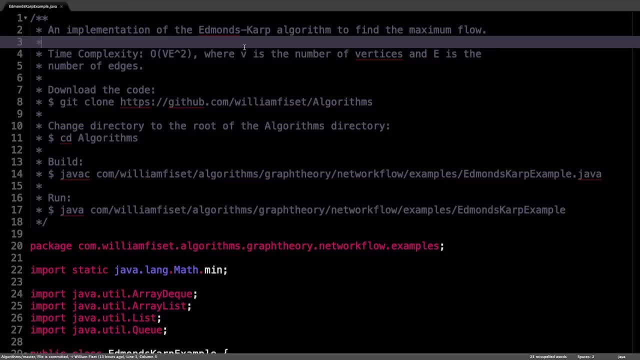 at some source code for the Edmonds Karp algorithm. All right, here we are in the source code, written in Java. I've laid out some instructions here in the header in case you wanted to download the code, play around with it and run it yourself. If I scroll down, you can see that we still 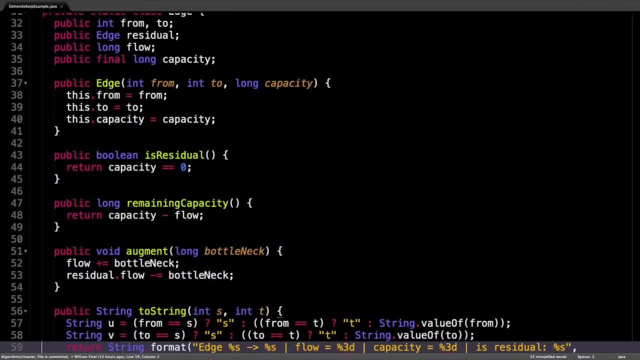 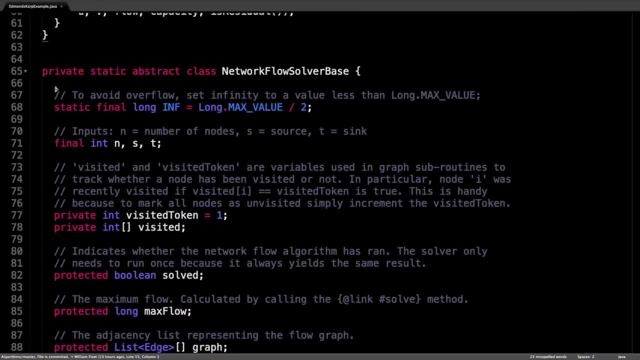 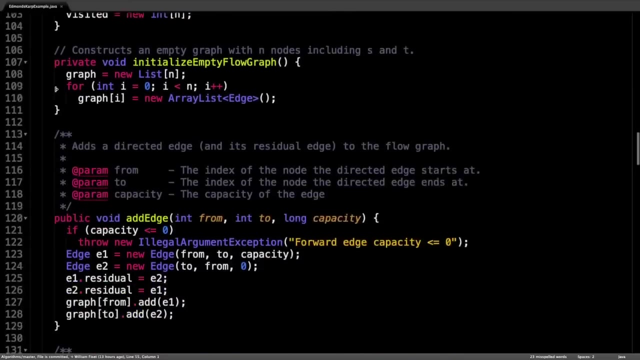 have the same setup as before, With the edge class right here and the network flow base solver. But there is one important change I have made since the Ford Fulkerson video, And that is I have added three new methods. If we scroll down you can see that the three new methods are right here: The 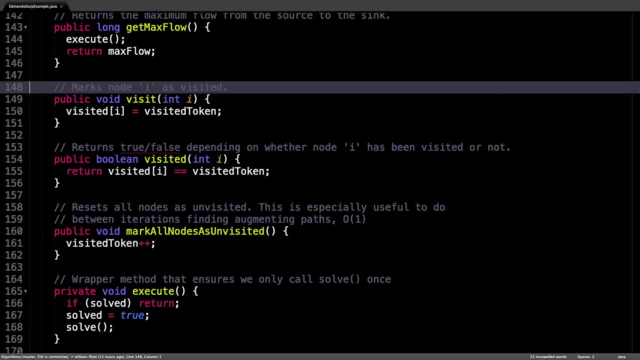 three methods. I added abstract away, visiting nodes and marking all nodes as unvisited. Now this is all done efficiently Internally through the network flow base solver class using a visited token. you don't have to worry about It. also helps readability for anybody who's new to the code. All right. 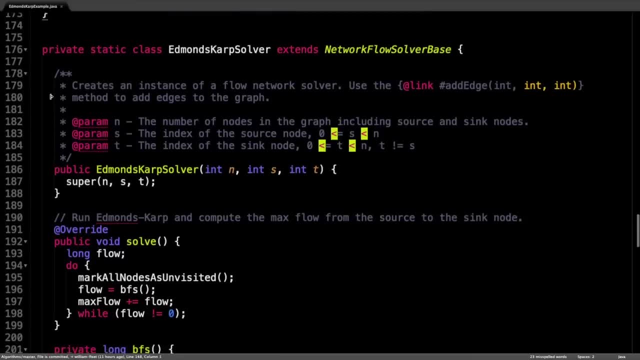 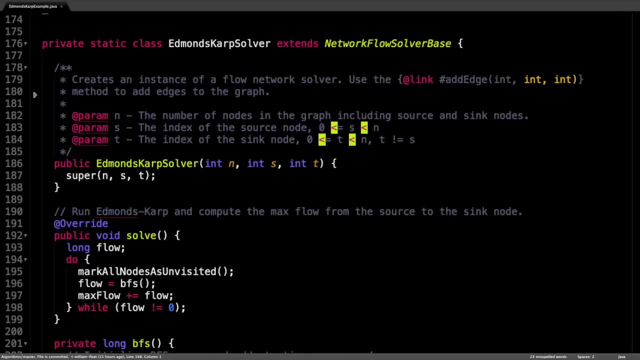 now let's have a look at the Edmonds Karp solver, which is the only thing different in this file. First, notice that the Edmonds Karp solver extends the network flow solver base. In doing so, we get a whole bunch of things for free, including the ability to 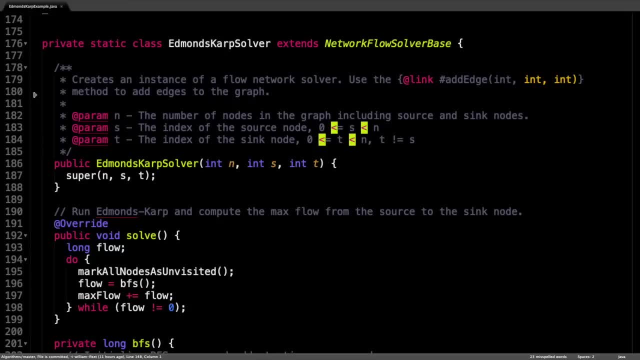 construct a flow graph Before we push flow through it. In the constructor for the Edmonds Karp solver, all I do is call the superclasses constructor. This performs various initializations, including allocating memory for the flow graph and registering which nodes are the source and the sink. The 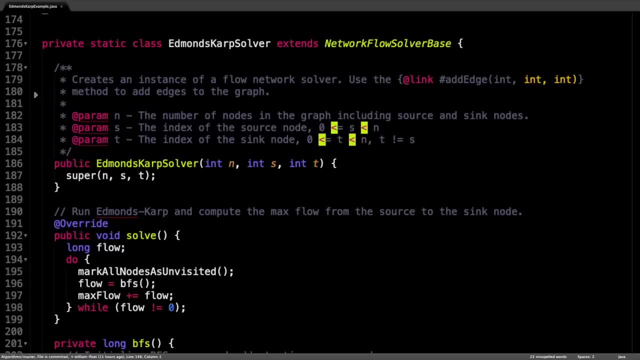 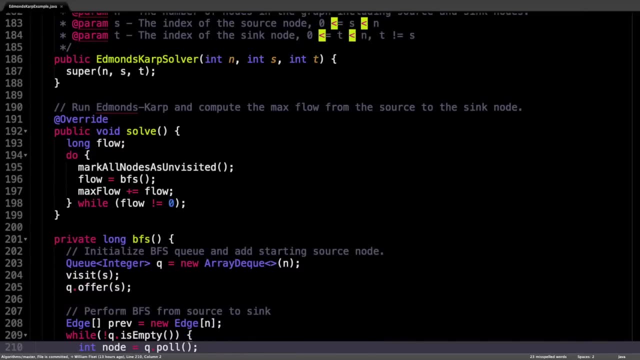 most important method in the Edmonds Karp solver is the solve method. right here The solve method is called just before we get the maximum flow. This method is really short. all we do is repeatedly find augmenting paths from the source of the sink until the flow. 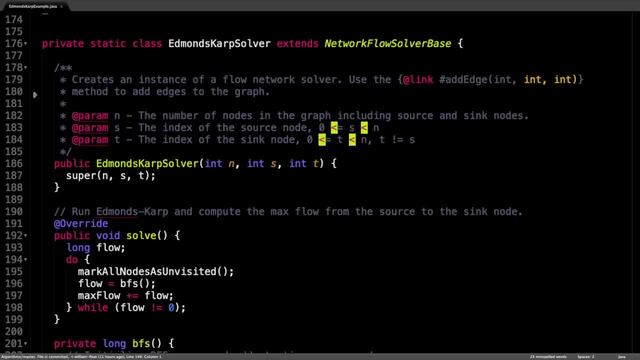 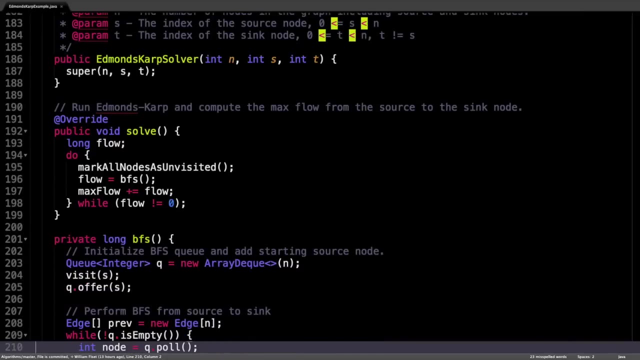 constructor. This performs various initializations, including allocating memory for the flow graph and registering which nodes are the source and the sink. The most important method in the Edmonds carp solver is the solve method. right here The solve method is called the just before we get the maximum flow. This method is really short. all we do is repeatedly. 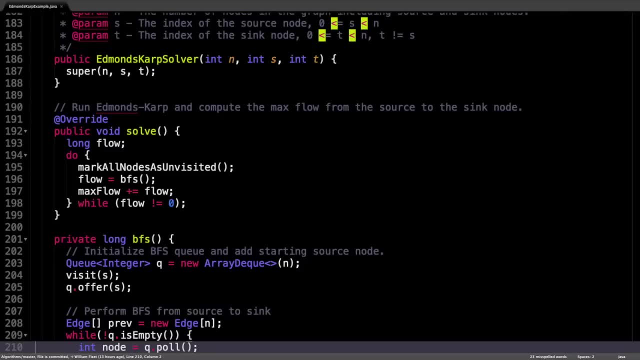 find augmenting paths from the source of the sink until the flow we get is zero, at which point we know that the graph is fully saturated and no more augmenting paths can be found Line by line. what we do is mark all nodes as unvisited. before each iteration run a. 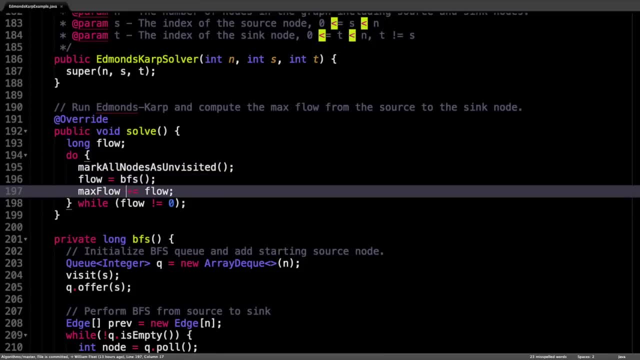 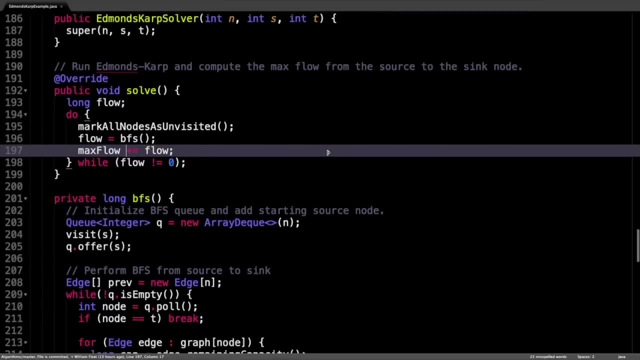 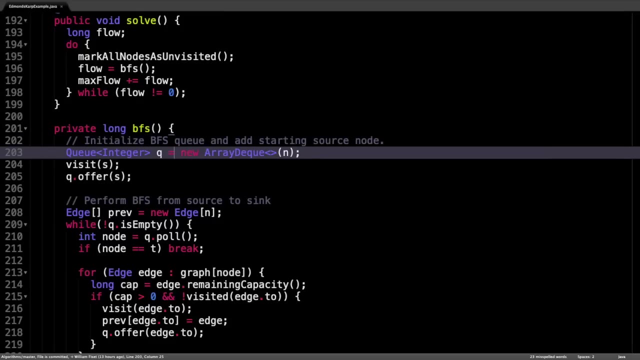 breadth first search and get the bottleneck value And then for all bottleneck values to calculate the maximum flow. Now let's take a closer look at the breadth first search method. The first thing I do is initialize an empty queue data structure, because I know that we're going to need one to do a breadth first search after. 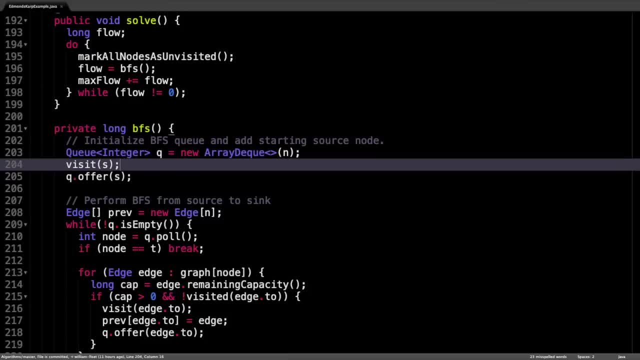 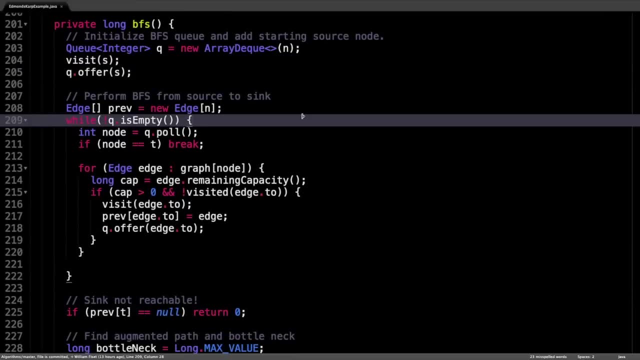 the creation of the queue. What I do is I visit the source node and add it to the queue so that the breadth first search starts at the source. Then do your standard breadth first search method. I hope, while there are still nodes in the queue, remove the first node found. 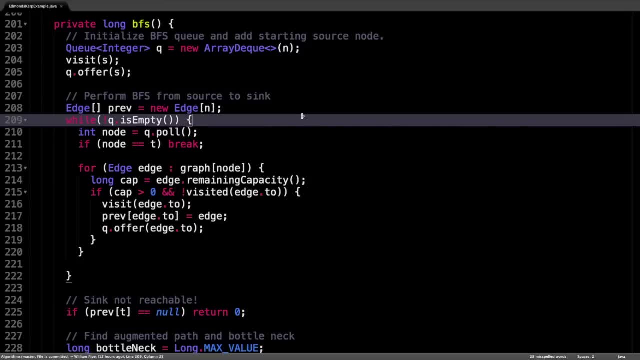 in the queue. If it's the sink, stop, otherwise iterate through all valid adjacent neighbors. we can add a node to the queue if it is not already visited and the edge leading to the node has a capacity greater than zero. However, before we add the node to the queue, we visit. 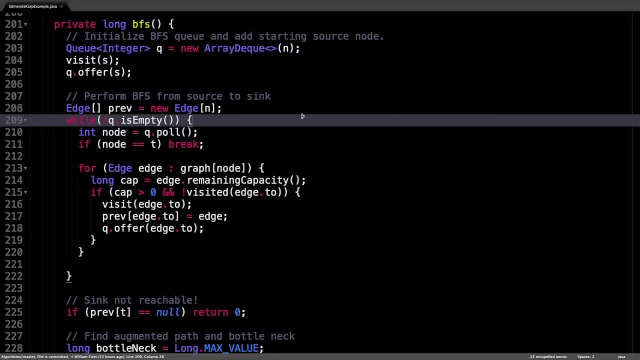 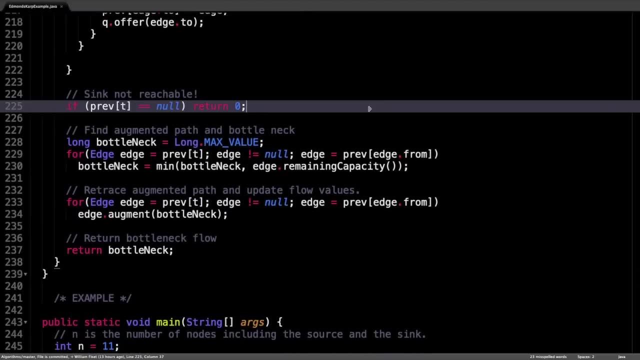 it and track where it came from by placing an edge in the prev array to rebuild the augmenting path later on. Alright, so moving on, we know that the breadth first search did not actually make it to the sink if we have no entry at the index of the sink in the prev array, So we can return early. 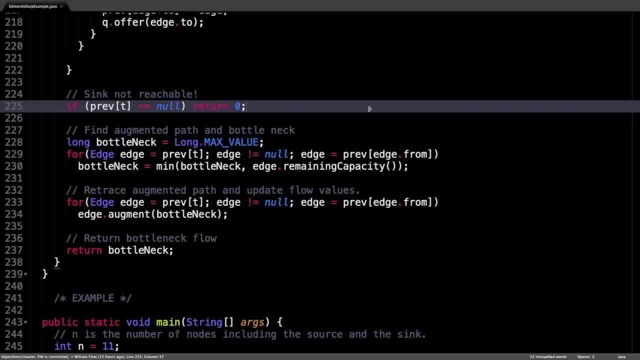 after this point, we know that there exists an augmenting path. Since we know an augmenting path exists, we can find the bottleneck value, that is, the smallest remaining edge capacity along the path. We do that by starting at the sink and reconstructing the augmenting 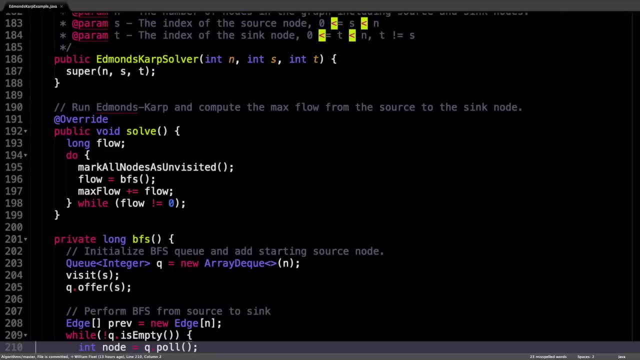 we get is zero, at which point we know that the graph is fully saturated and no more augmenting paths can be found Line by line. what we do is mark all nodes as unvisited. before each iteration, run a breadth first, search and get the bottleneck value, and then 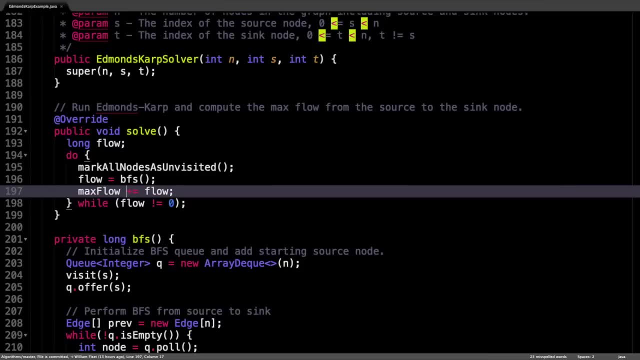 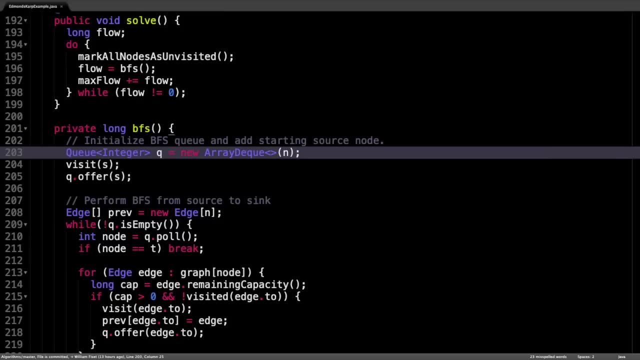 some overall bottleneck values to calculate the maximum flow. Let's take a closer look at the breadth first search method. The first thing I do is initialize an empty queue data structure, because I know that we're going to need one to do a breadth first search. after the creation of the queue, What I do is I visit the source node and add. 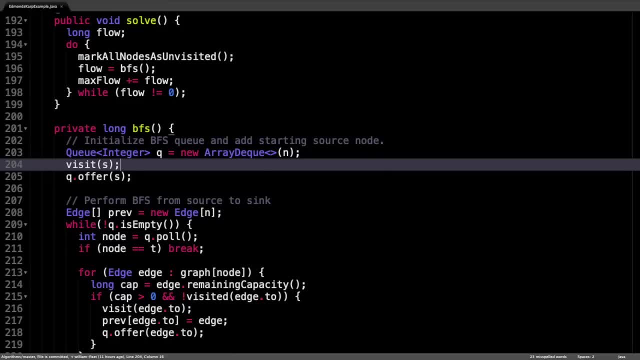 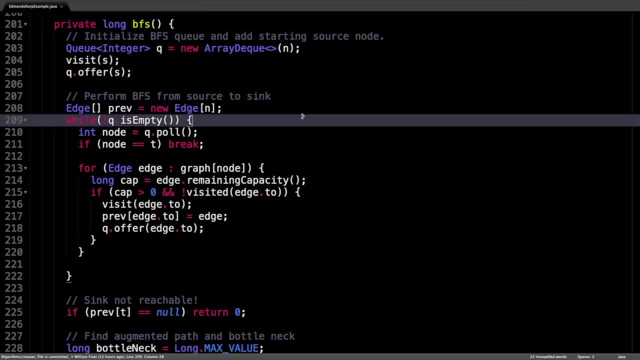 it to the queue so that the breadth first search starts at the source. Then do your standard breadth first search loop. while there are still nodes in the queue, remove the first node found in the queue. If it's the sink, stop, otherwise iterate through all valid adjacent neighbors. we can 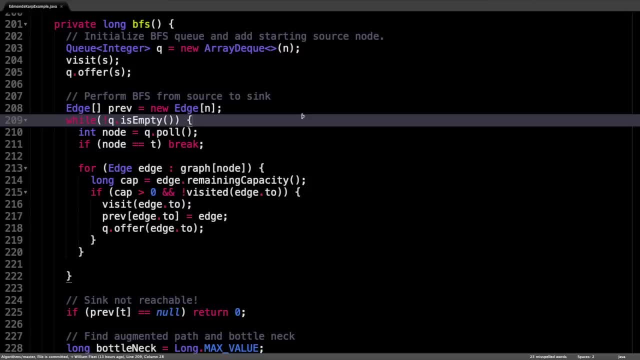 add a node to the queue if it is not already visited and the edge leading to the node has a capacity greater than zero. However, before we add the node to the queue, we visit it and track where it came from by placing an edge in the prev array to rebuild the augmenting 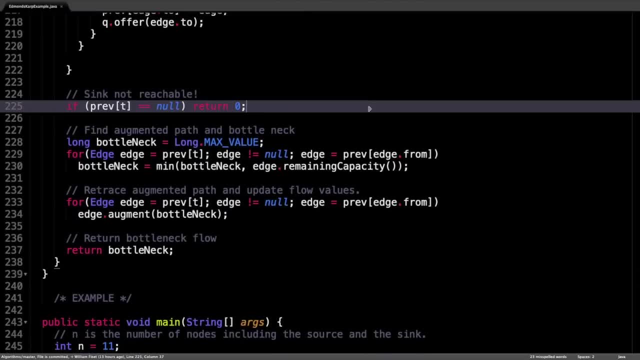 path later on. Alright, so moving on. we know that the breadth first search did not actually make it to the sink. If we have no entry at the index of the sink in the prev array, So we can return early after this point, we know that there exists. 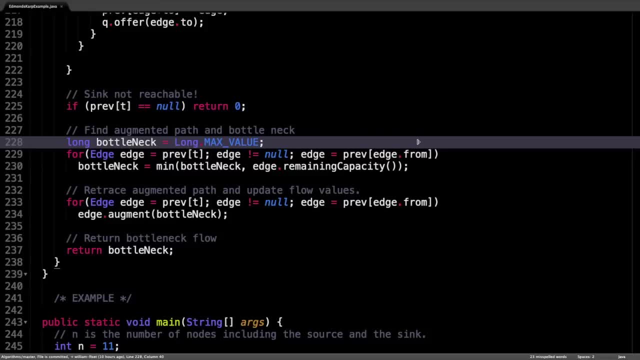 an augmenting path. Since we know an augmenting path exists, we can find the bottleneck value, that is, the smallest remaining edge capacity along the path. We do that by starting at the sink and reconstructing the augmenting path, going backwards by repeatedly reaching 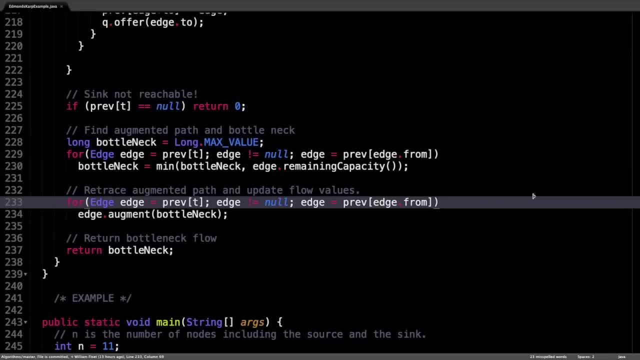 into the prev array until we are back at the sink, the source. then we need to update the flow along the augmenting path to adjust the flow values, So once again loop through the edges forming the argument path. then the augment method takes care of increasing the flow along the forward edges and decreasing the flow. 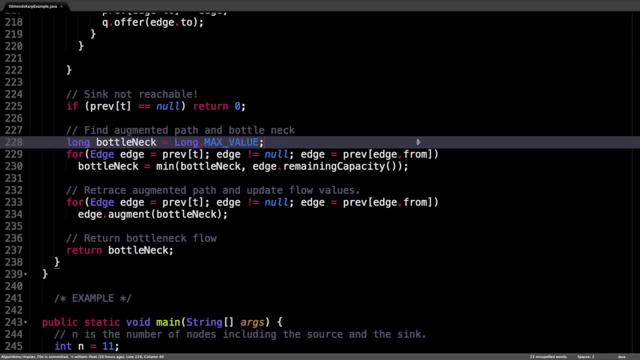 path going backwards By repeatedly reaching into the prev array until we are back at the source. then we need to update the flow along the augmenting path to adjust the flow values. So once again loop through the edges forming the augmenting path. then the augment method takes care of. 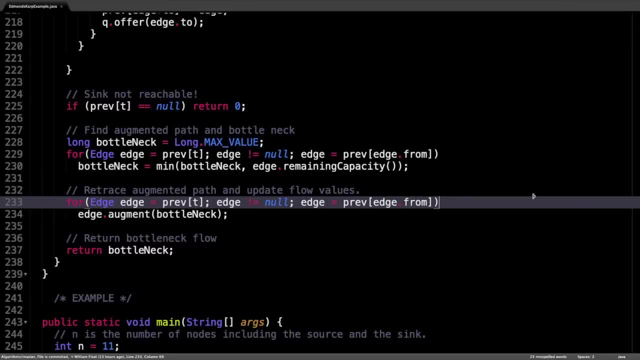 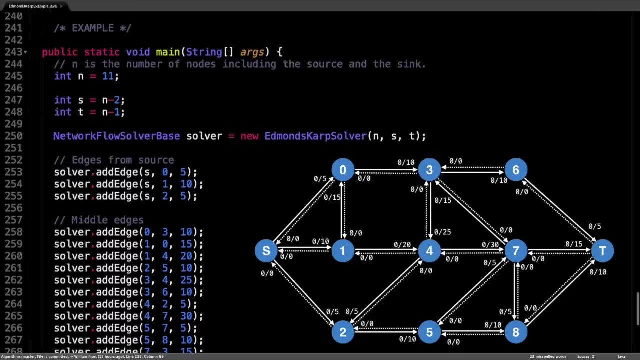 increasing the flow along the forward edges and decreasing the flow along the residual edges. The very last thing to do is to return the bottleneck value so that we can sum the max flow and the solve method, And that's basically it for Edmonds carp To actually build a flow graph. have a look. 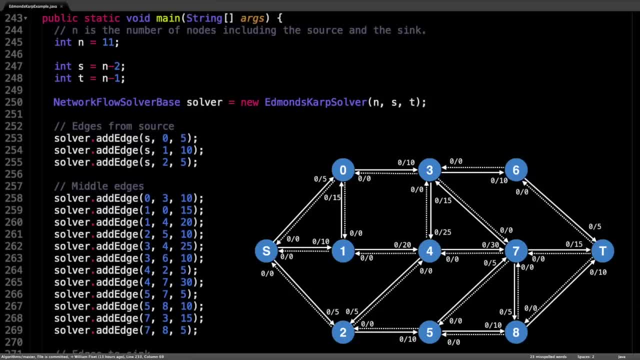 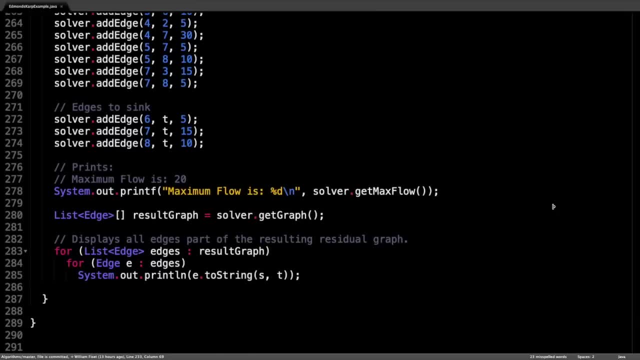 at the example right here in the main class. It sets up the flow graph from the previous video and pushes flow through it. You can see down here where we actually create the solver and run the solver to get the maximum flow and then finally display the resulting. 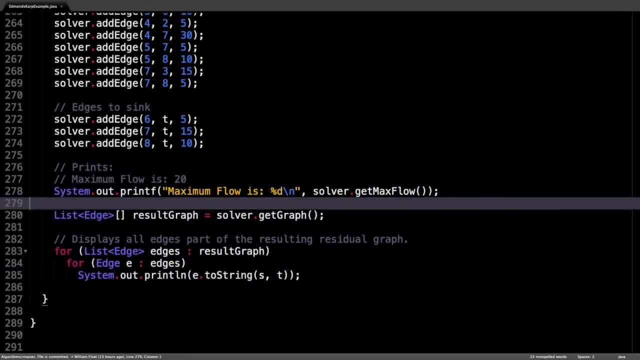 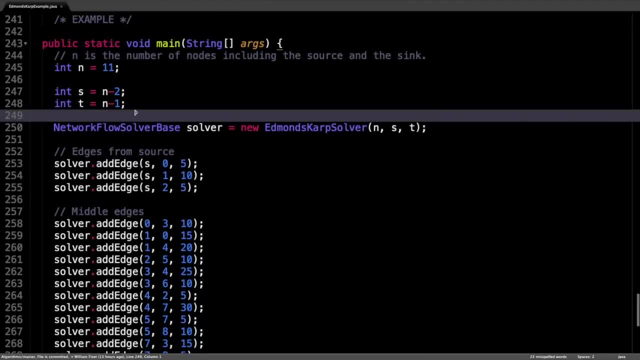 graph after the maximum flow has been pushed through it. So this is really handy to understand. So please have a look at this in more detail if you're struggling to understand Edmonds carp. Today we're still talking about network flow And, in particular, we're going to cover 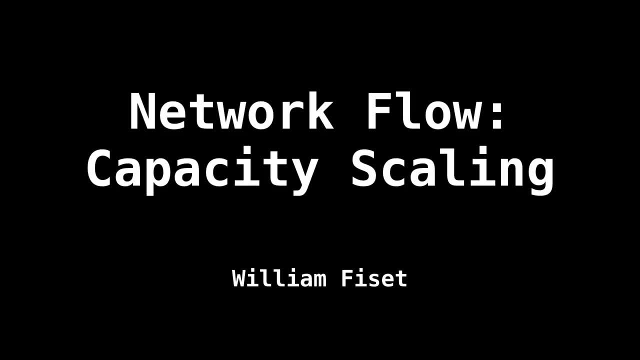 something called capacity scaling, which is really more of a heuristic than it is an algorithm. Capacity scaling is a heuristic, which says that we should attempt to push flow only through the largest edges first, and then allow using edges which have smaller capacities, and do this to achieve the maximum flow. 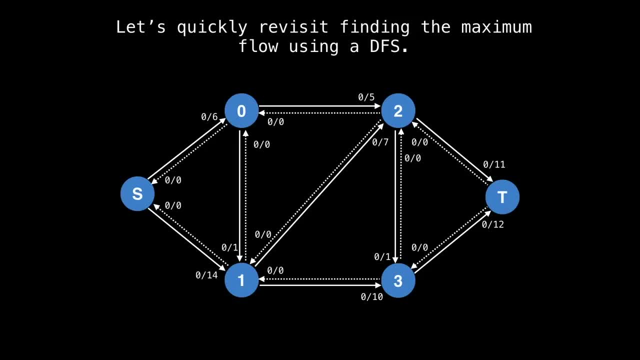 So let's take a look at this in more detail. if you're struggling to understand Edmonds carp, Today we're still talking about network flow And, in particular, we're going to cover maximum flow more rapidly, Just before we dive into capacity scaling. I want to quickly. 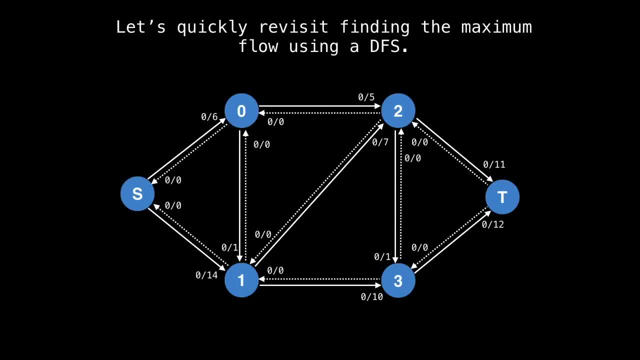 revisit finding the max flow using a depth first search and the issues surrounding that. I keep coming back to this because I think it's important that we understand the intuition behind why all these new max flow algorithms were developed and why they came about. When we're looking at finding augmenting paths, the worst case is when we can only augment. 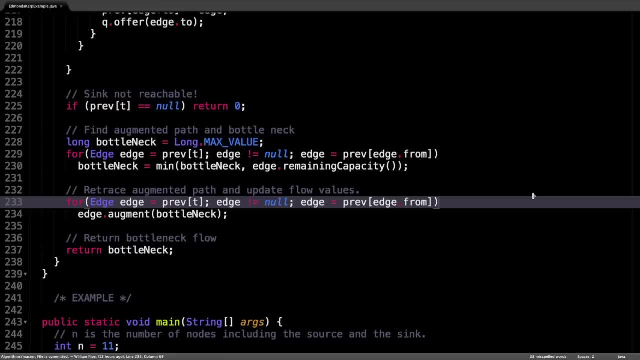 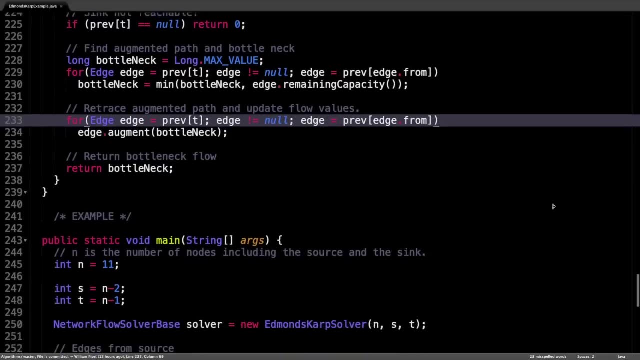 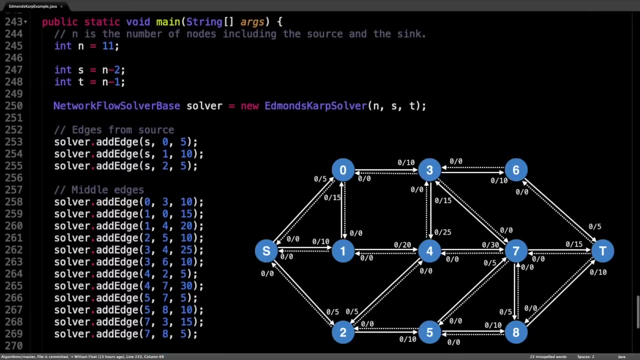 along the residual edges. The very last thing to do is to return the bottleneck value so that we can sum the max flow and the solve method, And that's basically it for admins carp To actually build a flow graph. have a look at the example right here in the main. 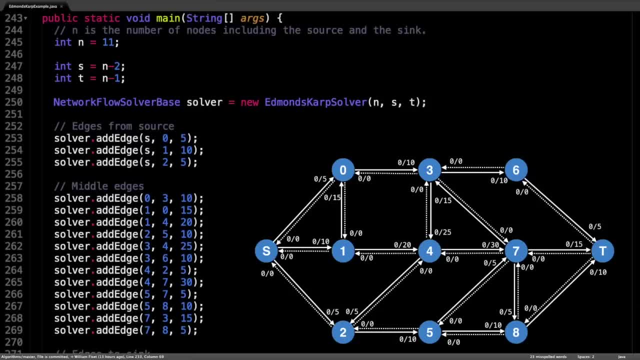 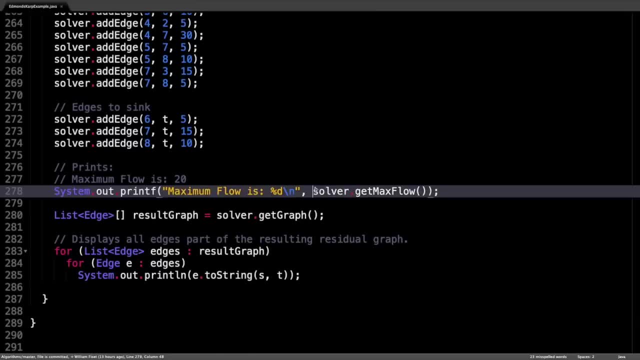 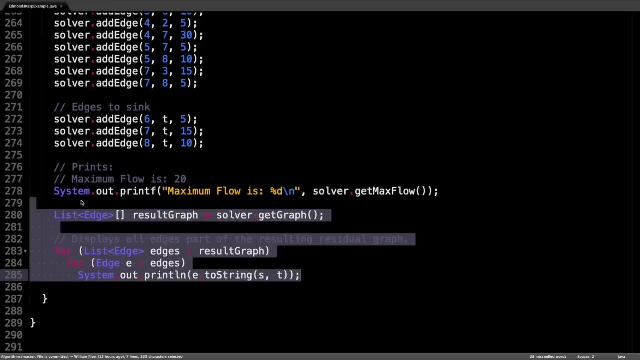 class. It sets up the flow graph from the previous video and pushes flow through it. You can see down here where we actually create the solver and run the solver to get the maximum flow and then finally display the resulting graph after the maximum flow has been pushed. 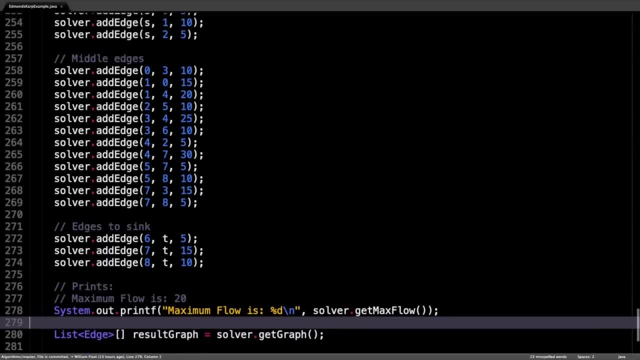 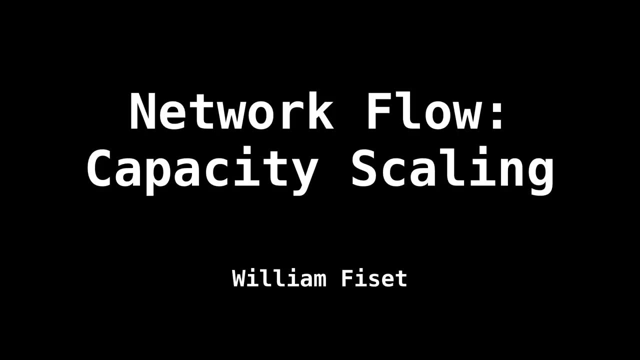 through it, So this is really handy to understand. So please have a look at this in more detail if you're starting to build a flow graph. struggling to understand admins, carp. Today we're still talking about network flow And, in particular, we're going to cover something called capacity scaling, which is really more 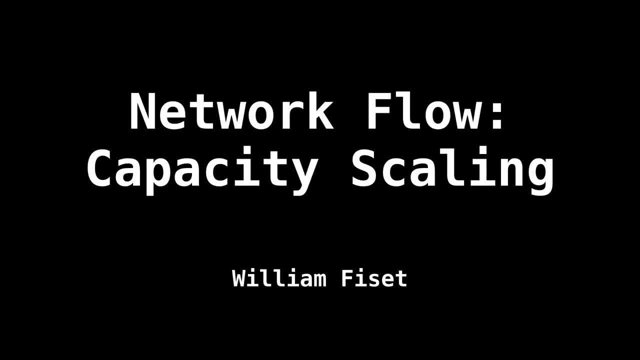 of a heuristic than it is an algorithm. Capacity scaling is a heuristic which says that we should attempt to push flow only through the largest edges first and then allow using edges which have smaller capacities, and do this to achieve the maximum flow more rapidly. Just before. 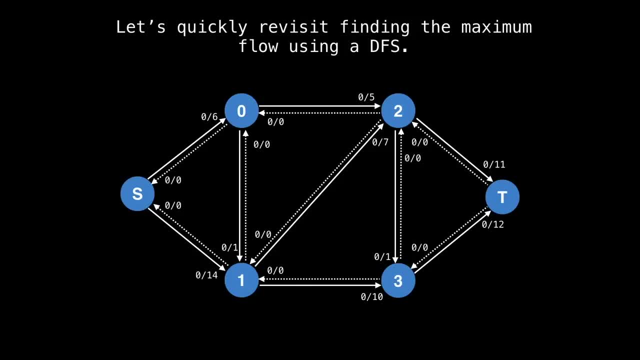 we dive in To capacity scaling, I want to quickly revisit finding the max flow using a depth first search and the issues surrounding that. I keep coming back to this because I think it's important that we understand the intuition behind why all these new max flow algorithms were developed. 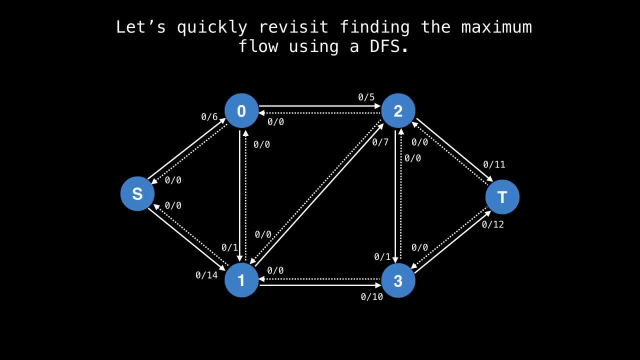 and why they came about. When we're looking at finding augmenting paths, the worst case is when we can only augment the flow by one unit, And it goes something like this: When we start at the source node, we take any edge with a remaining capacity greater than zero. 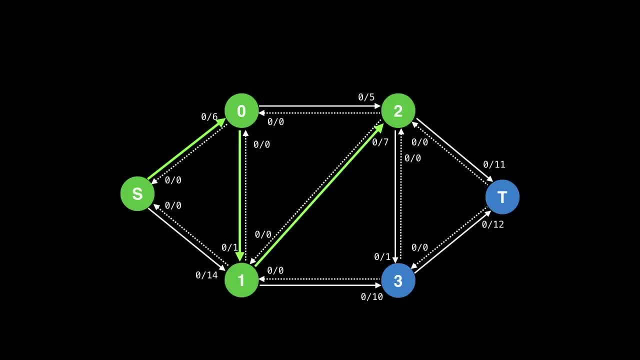 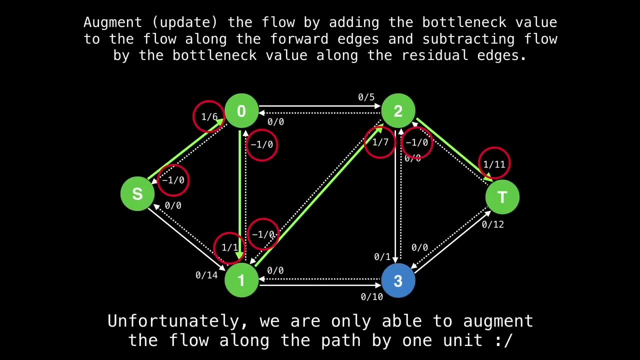 And we just keep going until we reach the sink. And once we've reached the sink we find the bottleneck value, that is, the edge with the smallest remaining capacity, along our augmenting path, which in this case happens to be one. Then we augment or update the 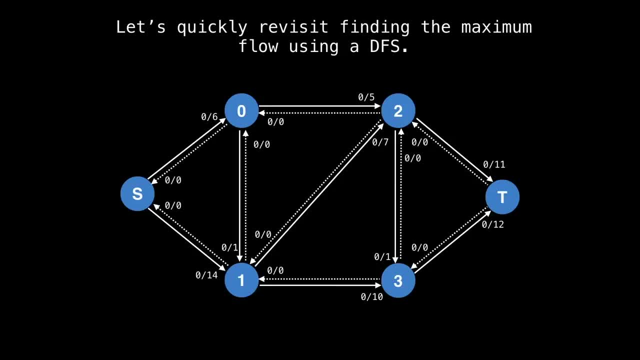 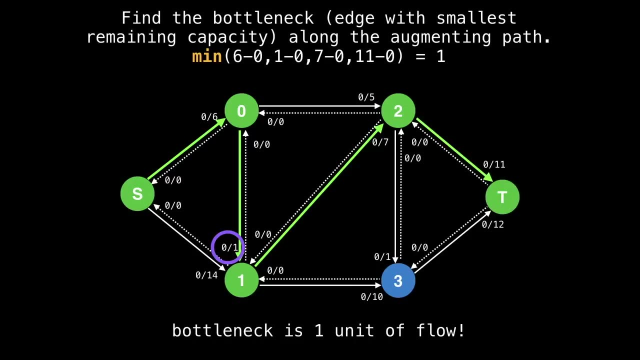 the flow by one unit. And it goes something like this: We start at the source node, we take any edge with a remaining capacity greater than zero And we just keep going until we reach the sink. And once we've reached the sink, we find the bottleneck value. that is the edge with the 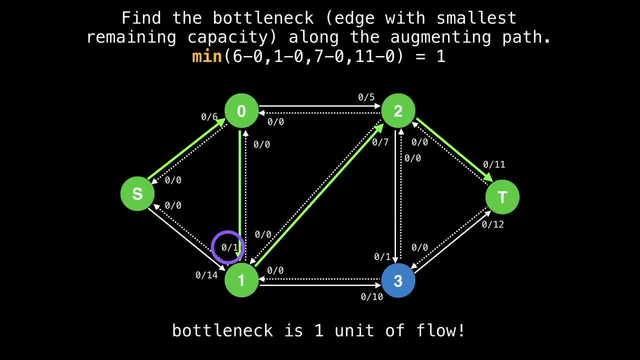 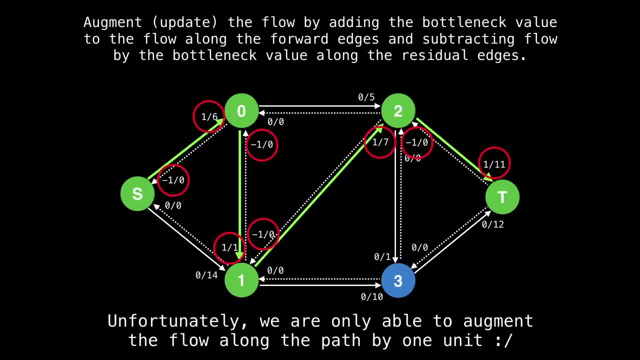 smallest remaining capacity along our augmenting path, which in this case happens to be one. Then we augment or update the flow by adding a new value. So we're going to go ahead and start by adding the bottleneck value to the flow along the forward edges and subtracting 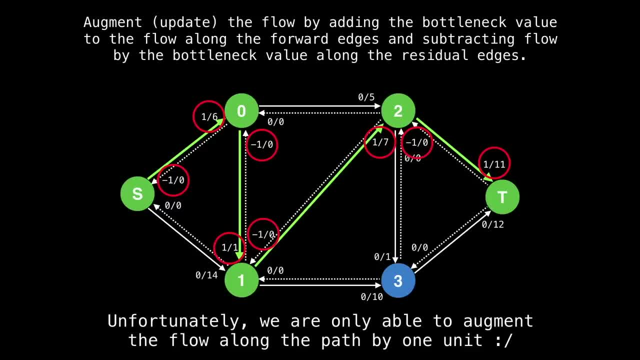 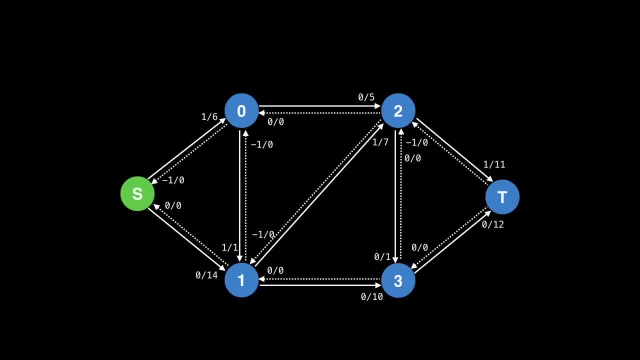 flow by the bottleneck value along the residual edges. However, we're not done, So we're going to start once again at the source and start finding another path. Suppose, this time we take the edge going down, then take the residual edge going up and sideways and then down. 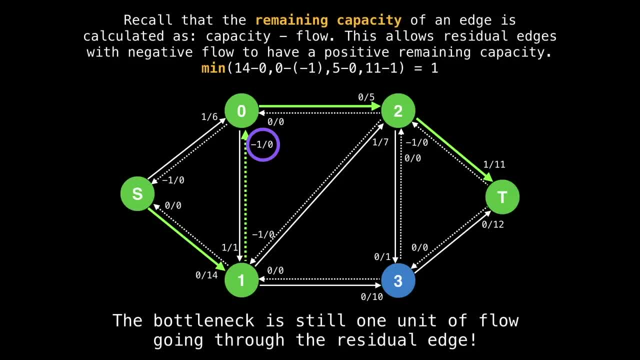 again. And now we have found another augmenting path And we can find its bottleneck value. recall that the remaining capacity of an edge is calculated as the capacity minus the flow. This allows residual edges with a negative flow to have a positive remaining capacity. 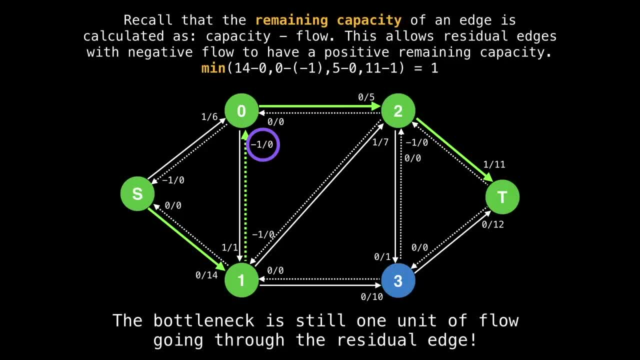 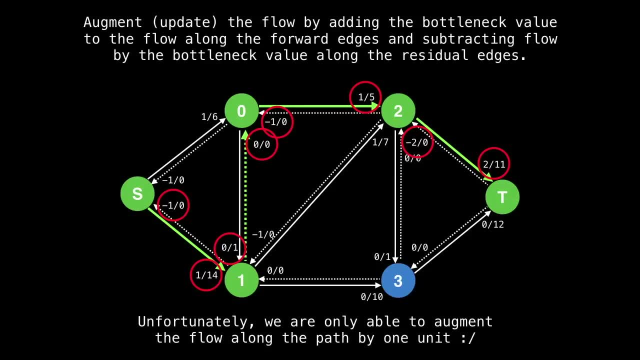 Notice that, yet again, the bottleneck value for this path is only one unit of flow. Now update or augment the flow. Do this by adding the bottleneck value to the flow along the forward edges And subtracting the flow by the bottleneck value along the residual edges. 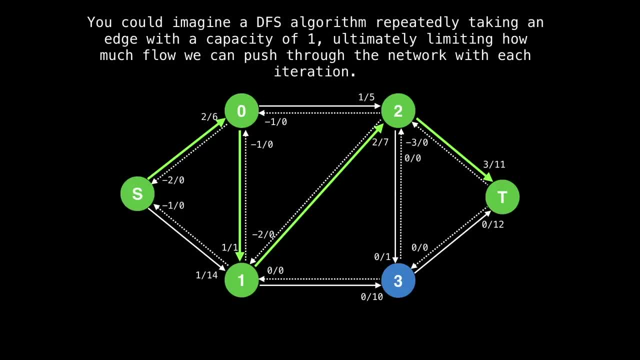 You could imagine the depth first search algorithm repeatedly taking an edge with a capacity value of one each time, which would ultimately limit how much flow we can push through the network in each iteration, as shown in the next few slides. So it would look like this: 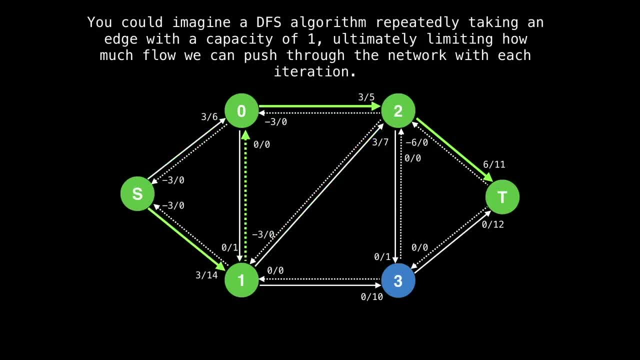 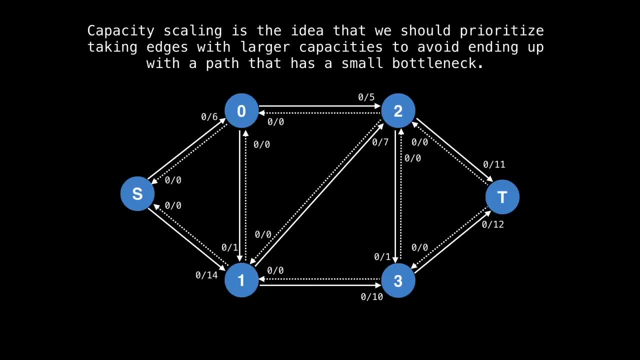 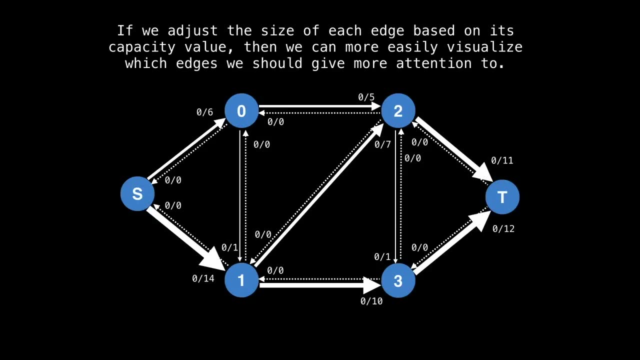 we just keep alternating between the forward and the residual edge with a capacity of one Capacity. scaling is the idea that we should prioritize taking edges with larger capacities first to avoid ending up with a path, the small bottleneck. if we adjust the size of each edge based on its capacity value, then we can more easily visualize which edges we should. 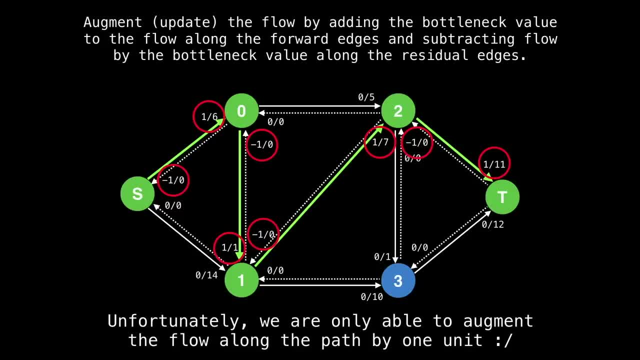 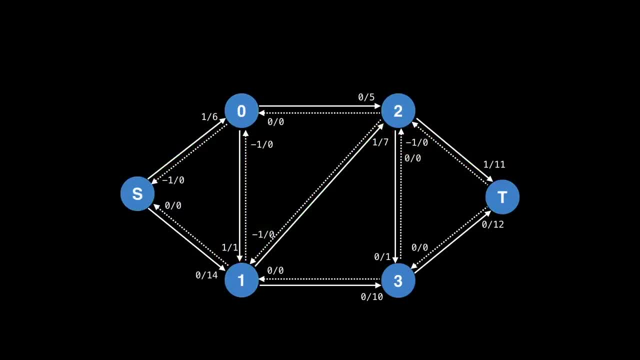 flow by adding the bottleneck value to the flow along the path. So we can see that the flow along forward edges and subtracting flow by the bottleneck value along the residual edges. However, we're not done, So we're going to start once again at the source and 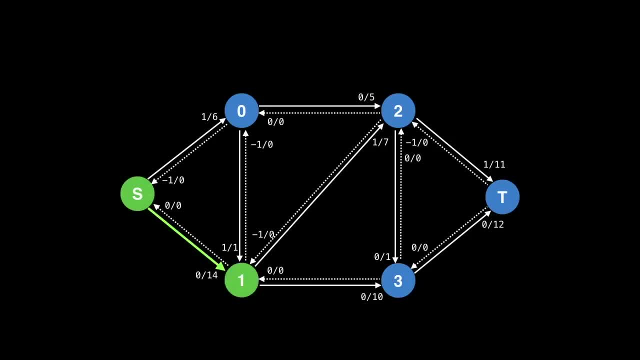 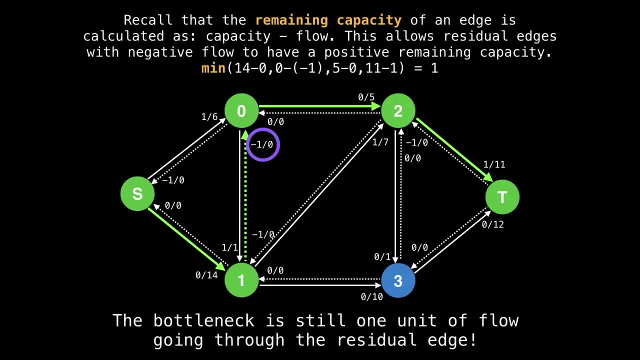 start finding another path. Suppose this time we take the edge going down, then take the residual edge going up and sideways and then down again, And now we have found another augmenting path and we can find its bottleneck value. Recall that the remaining capacity of an edge is calculated as the capacity minus the flow. This allows. 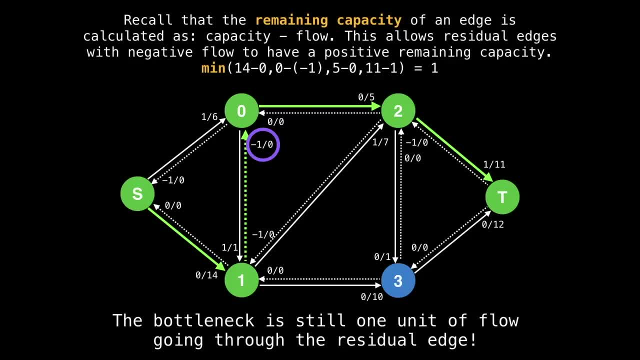 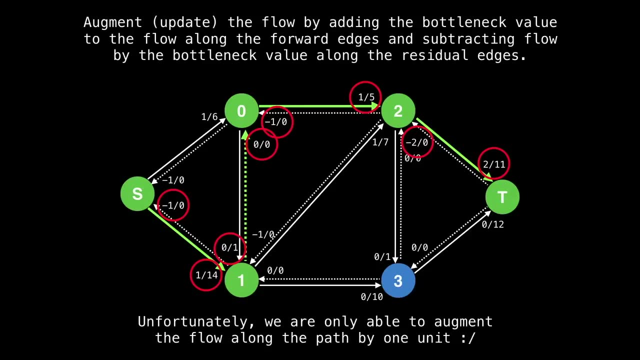 residual edges with a negative flow to have a positive remaining capacity. Notice that, yet again, the bottleneck value for this path is only one unit of flow. Now update or augment the flow. Do this by adding the bottleneck value to the flow along the forward edges. 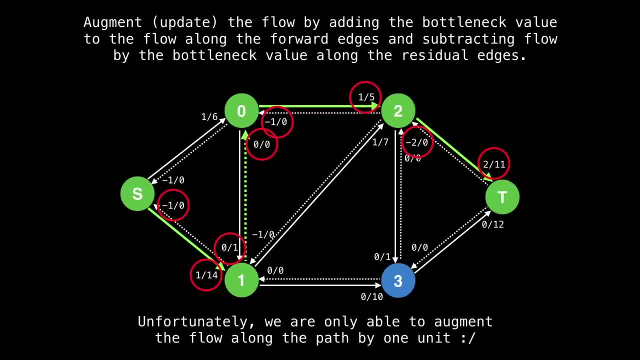 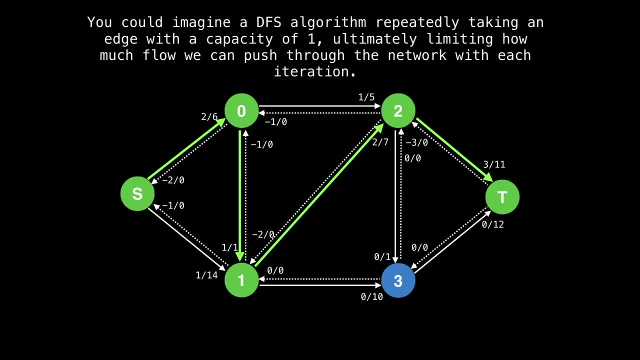 and subtracting the flow by the bottleneck value, You could imagine the depth first search algorithm repeatedly taking an edge, with a capacity value of one each time, which would ultimately limit how much flow we can push through the network in each iteration, as shown in the next few slides. So it would look like: 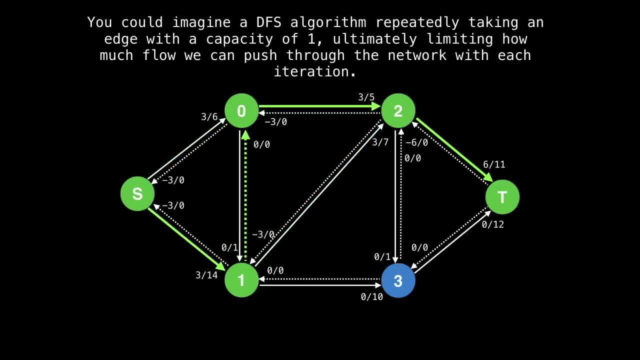 this. we just keep alternating between the forward and the residual edge with a capacity of one Capacity. scaling is a very important part of this algorithm because it allows us to see how much flow we can push through the network in each iteration. So it would. 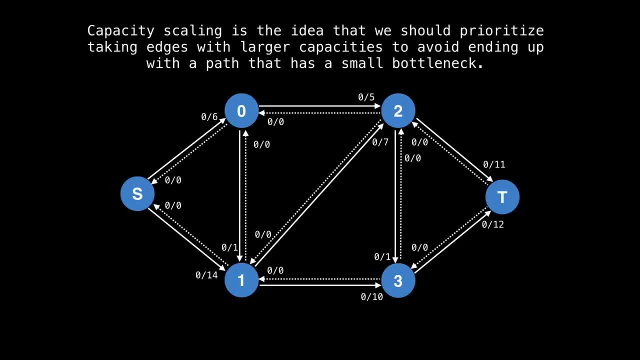 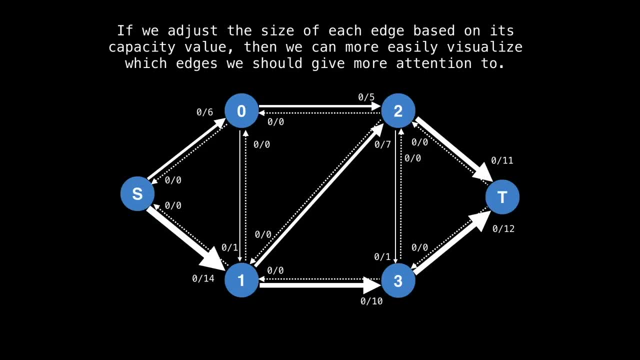 look like this: we just keep alternating between the forward and the residual edge with a capacity of one. this time, looking at the flow, Notice that each edge has to have a worthy level in order to actually eliminate that peak, in order to start a loop in the batch. This: 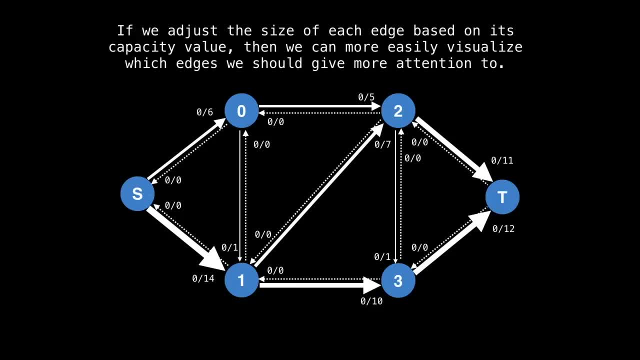 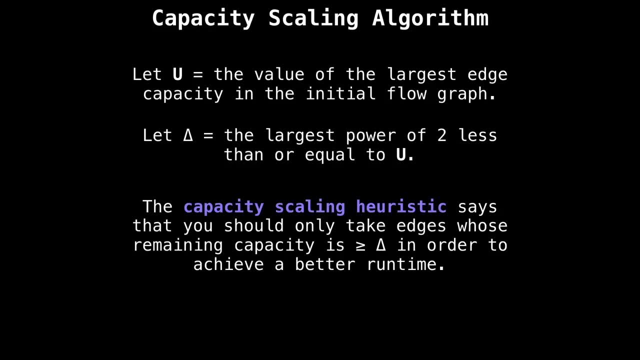 algorithm also uses the idea that we should prioritize taking edges with larger capacities first, to avoid ending up with a path, the small bottleneck. if we adjust the size of each edge based on its capacity value, then we can more easily visualize which edges we should give more attention to. The capacity scaling algorithm is pretty straightforward, But first. 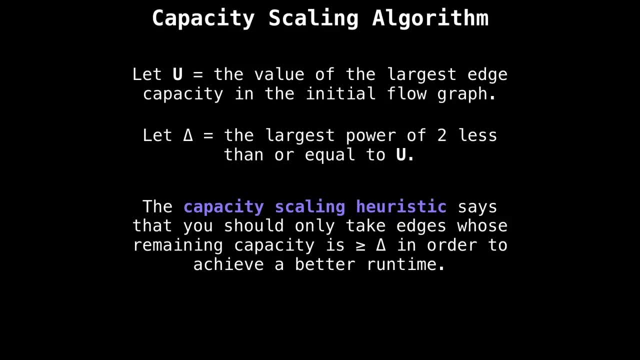 equal the value of the largest edge capacity in the initial flow graph. And also let delta be the largest power of two, which is less than or equal to the value of u. The capacity scaling heuristic says that we should always take edges whose remaining capacity is greater. 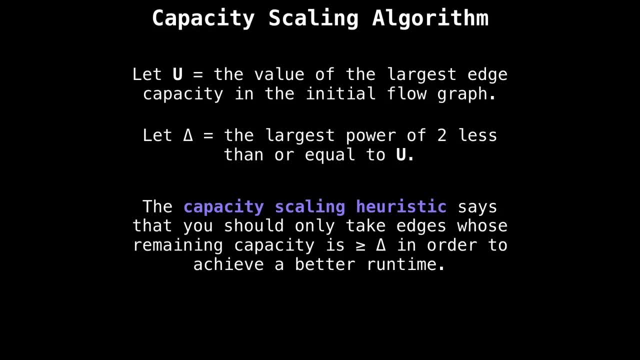 give more attention to. The capacity scaling algorithm is pretty straightforward, But first we need to define two variables that we will explain later need Let you equal the value of the largest edge capacity in the initial flow graph And also let delta be the largest power of two, which is less than or equal to the value of 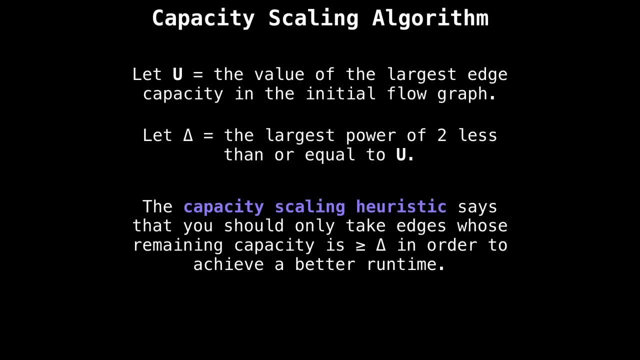 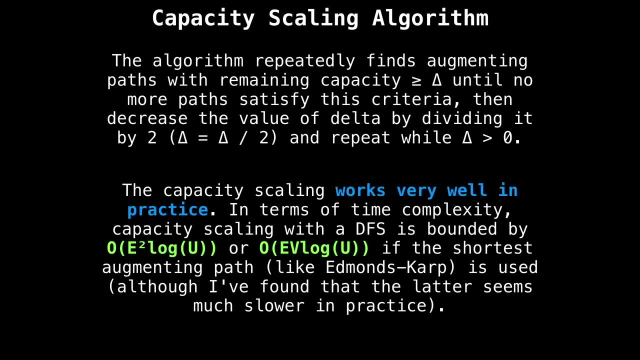 you. The capacity scaling heuristic says that we should always take edges whose remaining capacity is greater than or equal to delta in order to achieve a better runtime. But that's not everything to the algorithm. The algorithm will repeatedly find augmenting paths through the flow graph which have a remaining capacity greater than or equal to. 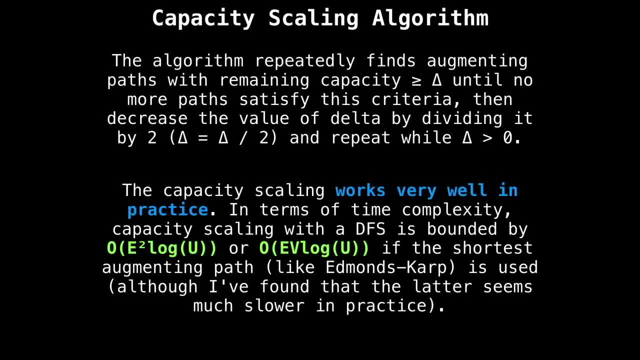 delta until no more paths satisfy this criteria. Once this criteria is no longer met, what we do is decrease the value of delta by dividing it by two, And we repeat this process while delta is greater than zero. So the reason you would want to implement capacity scaling is because it's very easy to code up and it works very. 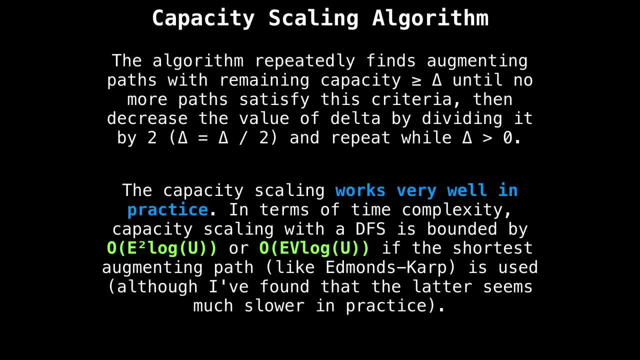 very well in practice In terms of time complexity, capacity scaling with a depth first search runs in big O of E squared log u and in big O of E times v log u if the shortest augmenting path is found, which is basically Edmonds car, but with capacity scaling, although I 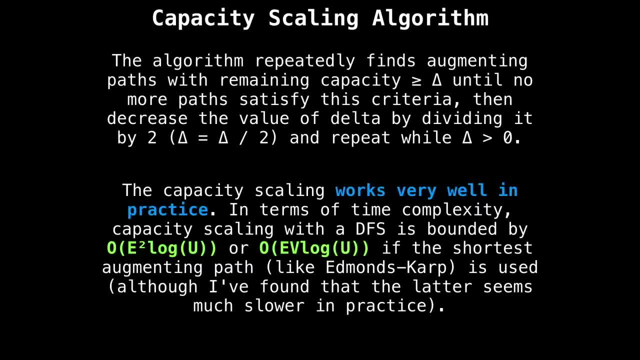 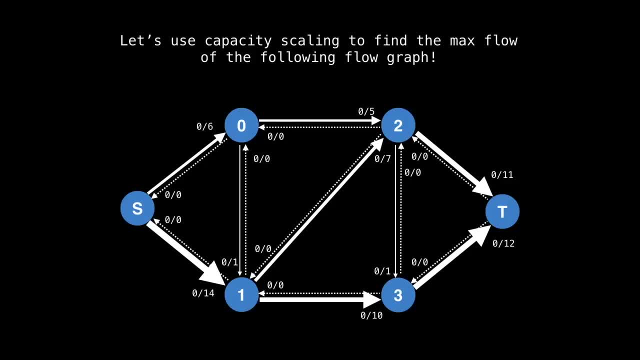 have found that to be much slower, so I would recommend the depth for search. if you are going to implement this, Let's do an example. Let's find the maximum flow of the following flow graph using capacity scaling. First, compute u as the maximum of all initial capacity values And this example. 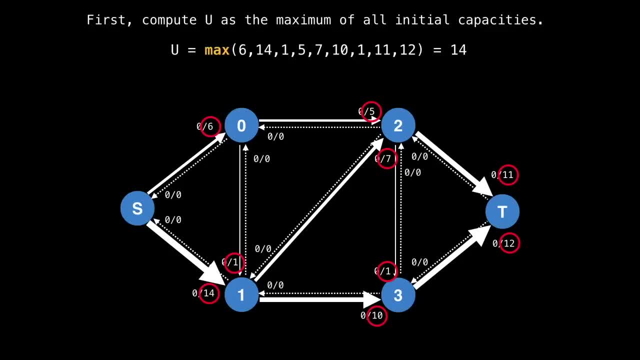 u is the maximum of 614, 157, 1011 and 12,, which happens to be 14.. Next compute the starting value for delta, which is the smallest power of two less than or equal to u, which we know is 14.. Therefore, the starting value of delta is eight, since the next power of 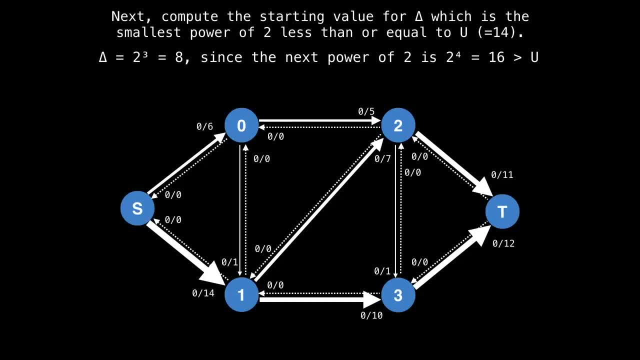 two after eight is 16.. But 16 is larger than 14.. Now that we have Delta, we can start finding paths from s to t which have a remaining capacity greater than or equal to eight. start our search at the source. From the source there's only one n. 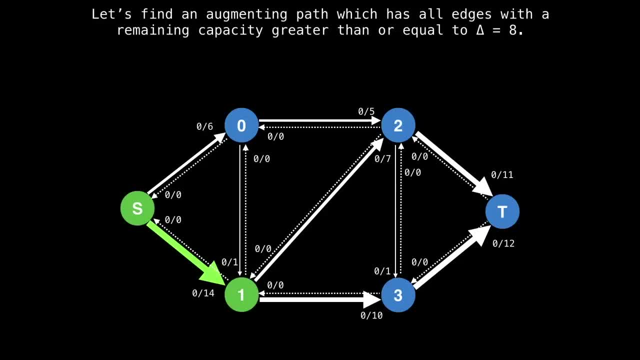 So let's say we have an edge which has a remaining capacity of eight or more, which is the edge with the capacity of 14 going downwards. then there's the edge sideways with a remaining capacity of 10 we can take And finally an edge with the remaining capacity. 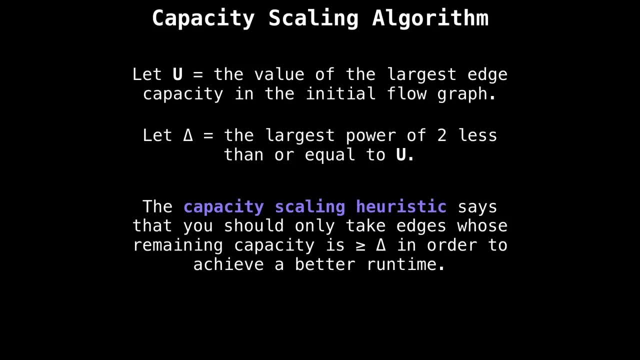 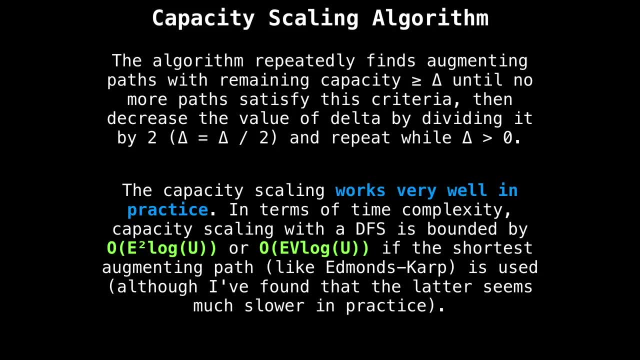 than or equal to delta in order to achieve a better runtime. But that's not everything to the algorithm. The algorithm will repeatedly find augmenting paths through the flow graph which have a remaining capacity greater than or equal to delta, until no more paths satisfy this criteria. Once this criteria is no longer met, what we do is decrease the value of delta. 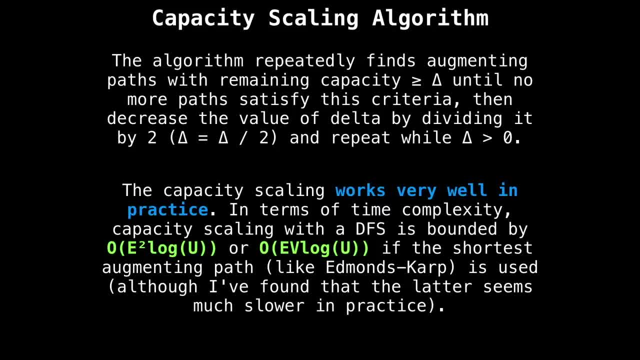 by dividing it by two, And we repeat this process while delta is greater than zero. So the reason you would want to implement this method is because you want to reduce the value of delta by dividing it by two, And we repeat this process while delta is. 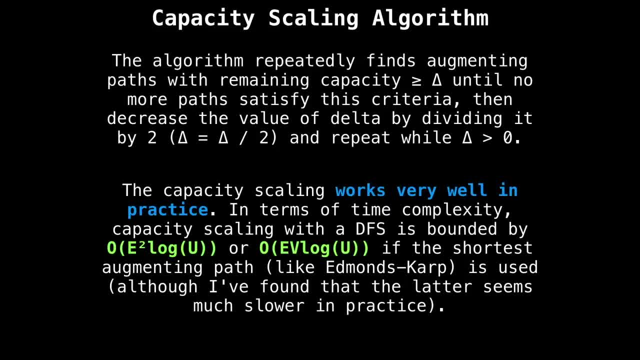 greater than zero. So the reason you would want to implement this method is because it's very easy to code up and it works very, very well in practice In terms of time, complexity, capacity scaling with a depth first search runs in big O of E squared log u and in Big 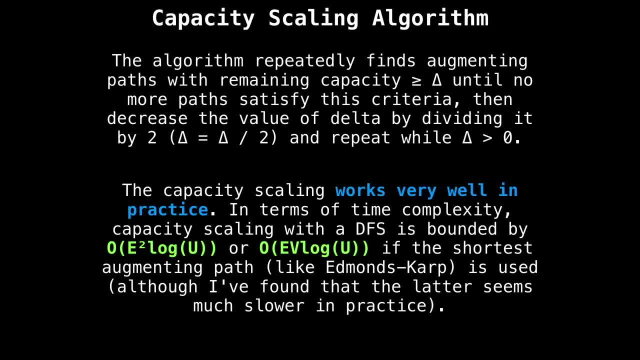 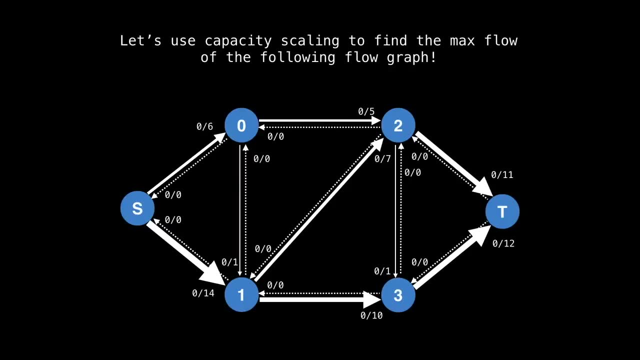 O of E times v log u if the shortest augmenting path is found, which is basically Edmonds car, but with capacity scaling, although I have found that to be much slower. So I would recommend the depth first search. if you are going to implement this, Let's. 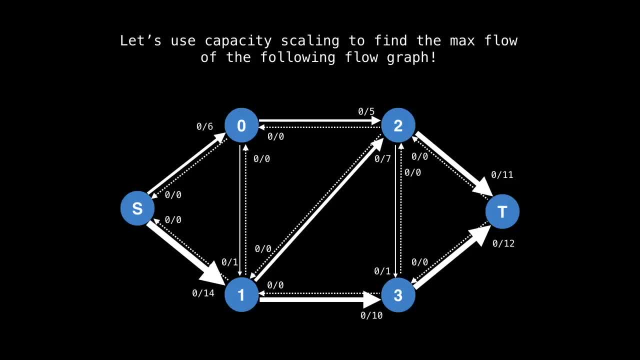 do an example. Let's find the maximum flow of the following flow graph using capacity scaling. First, compute you as the maximum of all initial capacity values And this example you is the maximum of 614, 157, 1011 and 12,, which happens to be 14.. Next, compute the starting. 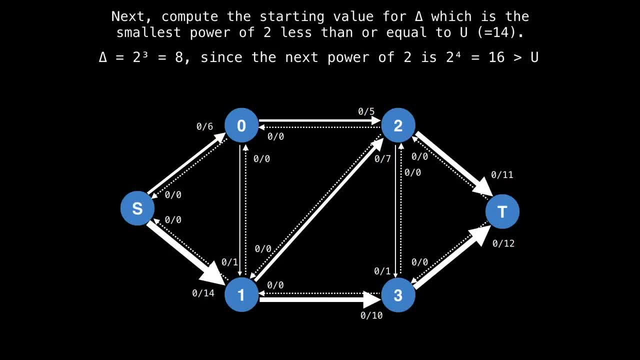 value for delta, which is the smallest power of two less than or equal to u, which we know is 14.. Therefore, the starting value of delta is eight, since the next power of two after eight is 16.. But 16 is larger than 14.. Now that we have delta, we can start finding paths. 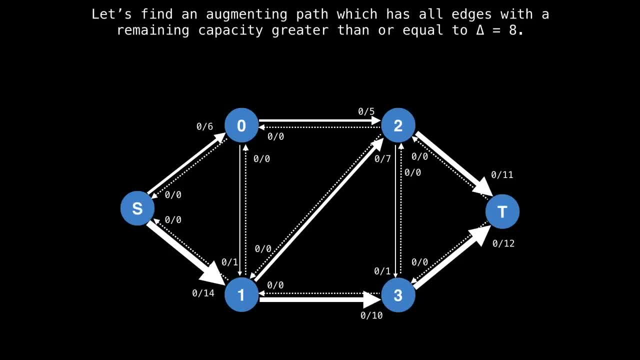 from s to t, which have a remaining capacity greater than or equal to eight. Start our search at the source. from the source, there's only one edge which has a remaining capacity of eight or more, which is the edge with the capacity of 14 going downwards. then there's 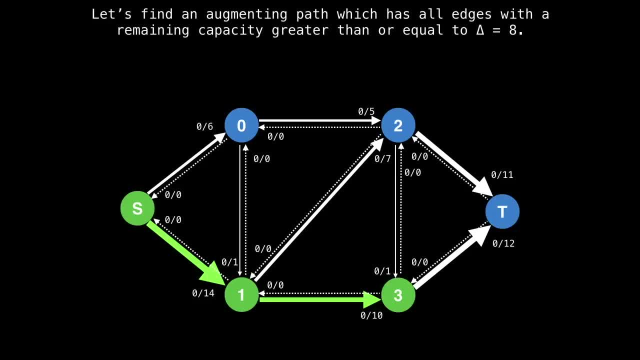 the edge sideways, with the remaining capacity of 10 we can take, And finally, an edge with the remaining capacity of 12 going upwards, which we can also take. Now we've reached the sink, So we can find the bottleneck value, which is 10, because 10 is the smallest remaining. 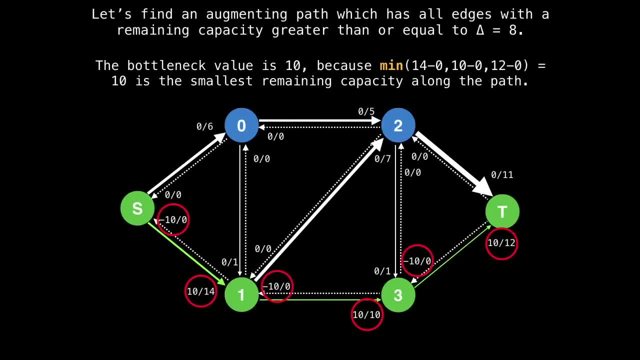 capacity along the found path. Next, augment the flow along the path. Next, we're going to scale down the size of each edge to reflect how much remaining capacity they have left. you can analyze the flow graph, but there are no more augmenting paths from s to t. 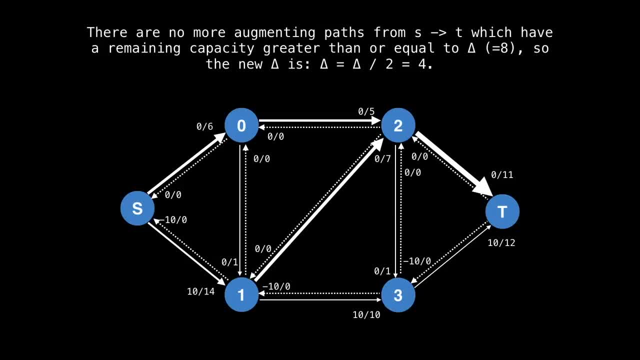 which have a remaining capacity greater than or equal to eight. So the new delta is halved in two and is now equal to four. One path we can take with all remaining capacities of four or more is the following: Start at the source, go up sideways and then go down. 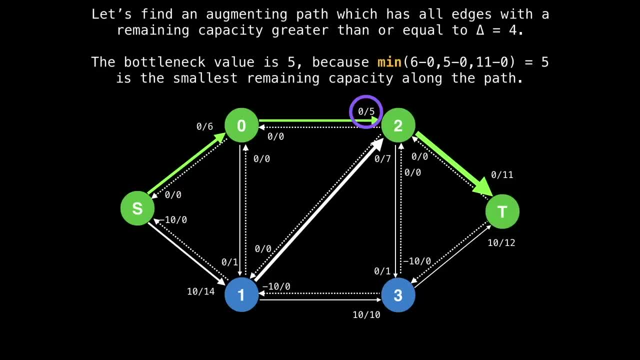 So we're going to start at the source, go up, sideways and then go down and then go sideways and sideways again, then do the usual, find the bottleneck and augment the flow. There's also another path, with all remaining capacities greater than four which we can. 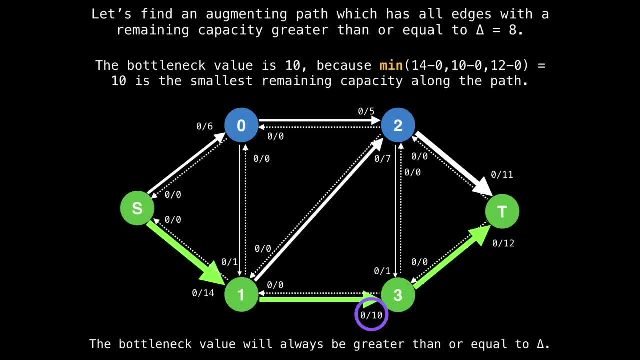 of 12 going upwards, which we can also take. Now we've reached the sink so we can find the bottleneck value, which is 10, because 10 is the smallest remaining capacity along the found path. Next, augment along the path. I scaled down the size of each edge to reflect how much remaining capacity. 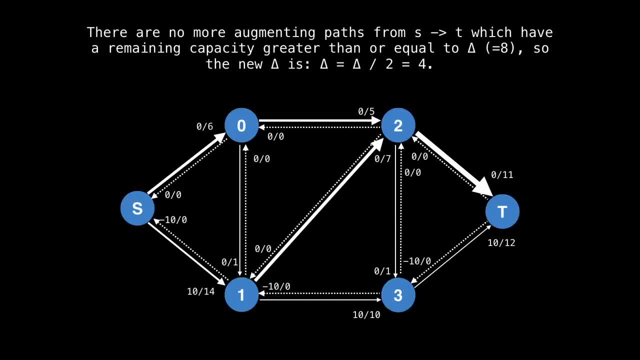 they have left. you can analyze the flow graph, but there are no more augmenting paths from s to t which have a remaining capacity greater than or equal to eight. So the new delta is halved in two and is now equal to four. One path we can take with all remaining capacities. 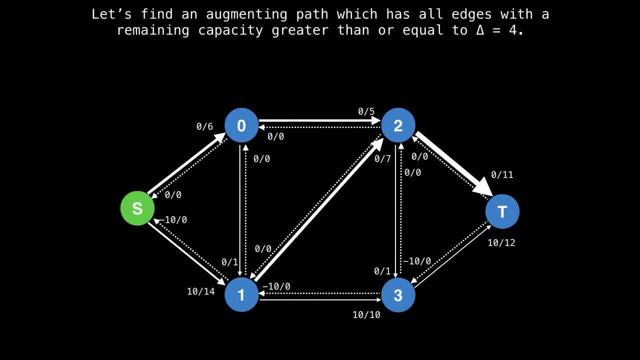 of four or more is the following: Start at the source, go up Sideways and sideways again, then do the usual, find the bottleneck and augment the flow. There's also another path, with all remaining capacities greater than four, which we can take from s to t, which is down to one, diagonally up to node two and to the sink Again find. 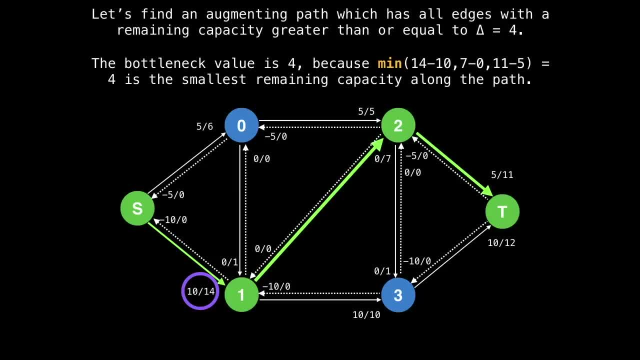 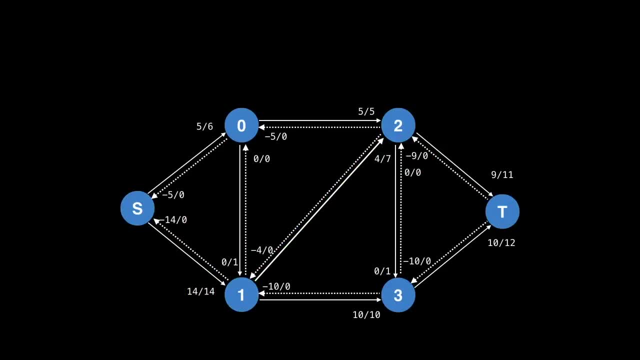 the bottleneck value, which we know to be four, because four is the smallest remaining capacity. If you now inspect the flow graph, there are no more paths with a remaining capacity, with all values greater than or equal to four, from s to t. So half the value of delta and two. 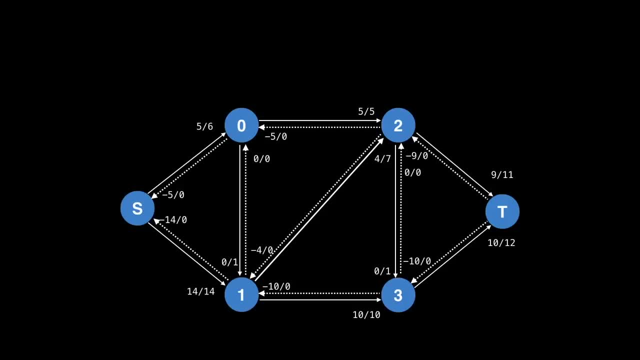 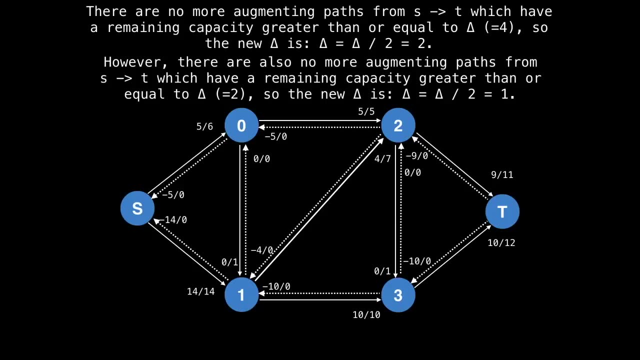 However, there are also no paths with a remaining capacity of all two or more, So we need to have the value of delta again, So now delta is equal to one. I believe there's one remaining path we can take before the graph is full. 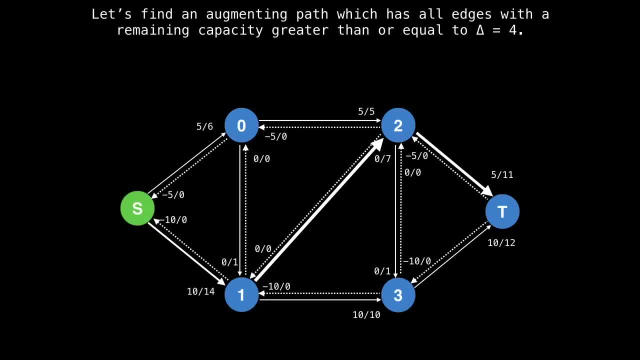 take from s to t, which is down to one, diagonally up to node two and to the sink Again, find the bottleneck value, which we know to be four, because four is the smallest remaining capacity along the path. Then we can augment the flow. If you now inspect the flow graph, there are no more paths with. 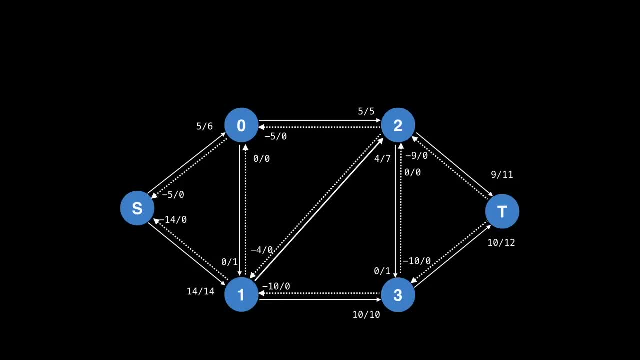 a remaining capacity with all values greater than or equal to four, from s to t. So half the value of delta and two. However, there are also no paths with a remaining capacity of all two or more, So we need to have the value of delta again. So now delta is equal. 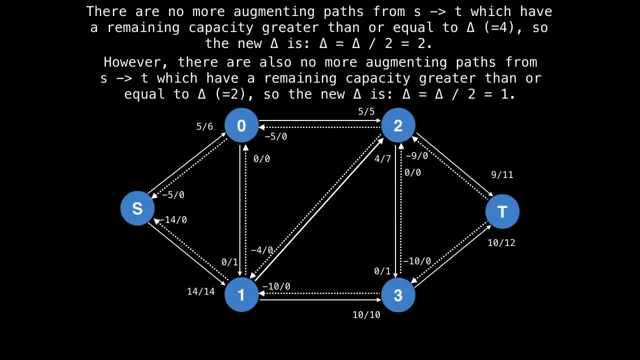 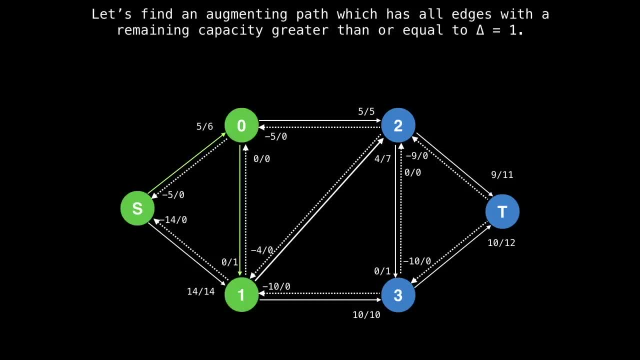 to one. I believe there's one remaining path we can take before the graph is fully set. Let's start at the source and find it All right now. we found the path, And we can also find the bottleneck, which has a value of one, And now the last step is to augment the. 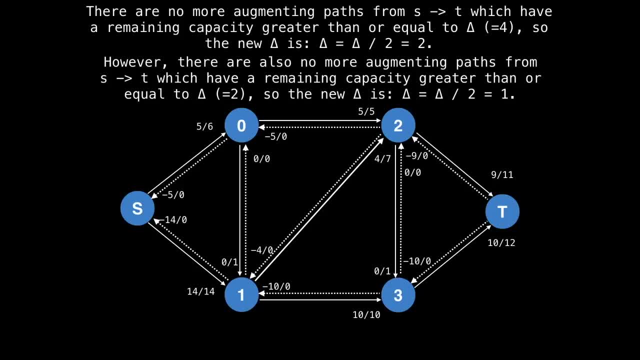 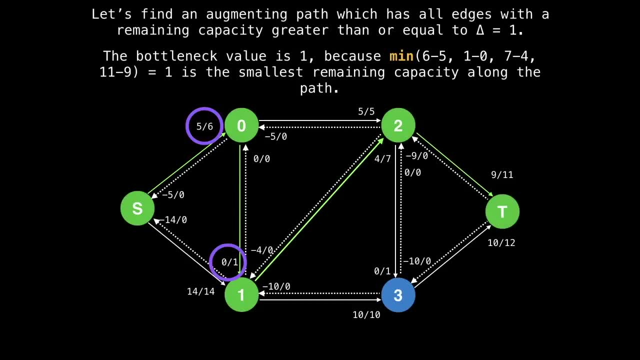 Saturated. let's start at the source and find it. Alright, now we found the path, And we can also find the bottleneck, which has a value of one. And now the last step is to augment the flow, And now there are no more paths. 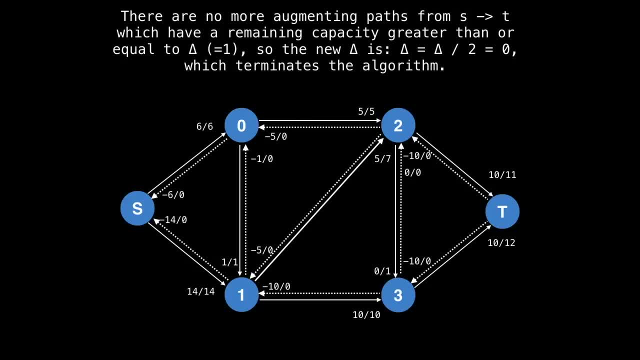 from s to t which have a remaining capacity greater than or equal to one. So the new value of delta is zero, which terminates the algorithm. We can compute the maximum flow by summing up all the bottleneck values we found in each iteration, which we know to be 1054 and one for a total of 20.. We can also compute the 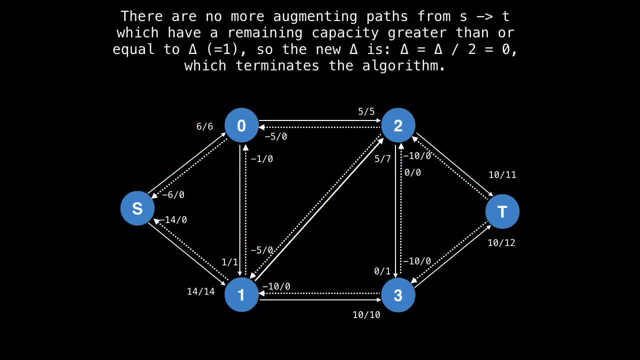 flow, And now there are no more paths from s to t which have a remaining capacity greater than or equal to one. So the new value of delta is zero, which terminates the algorithm. we can compute the maximum flow by summing up all the bottleneck values we found in each iteration which we 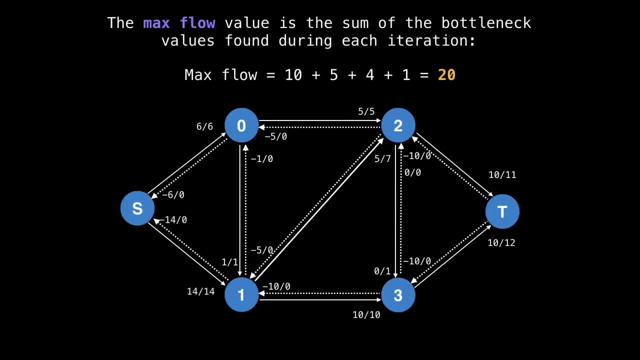 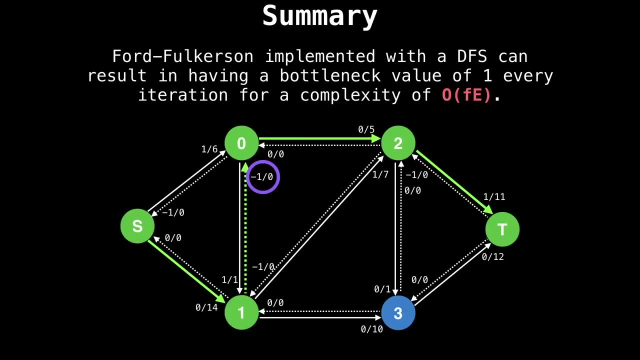 know to be 10, five, four and one, for a total of 20.. We can also compute the maximum flow by summing the flow values going into the sink highlighted in red. So, in summary of what we have learned about, we know that Ford Fulkerson implemented with a depth first search. 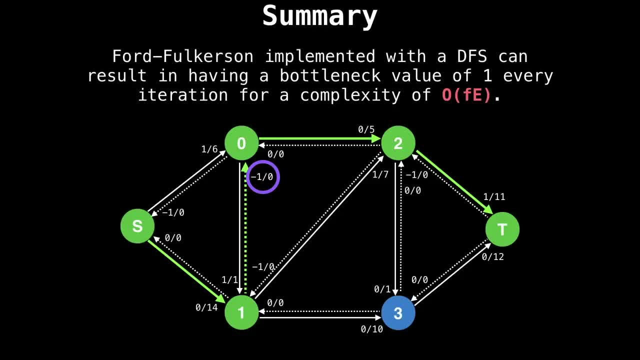 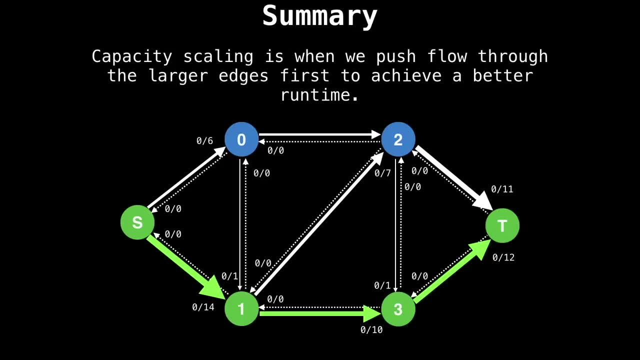 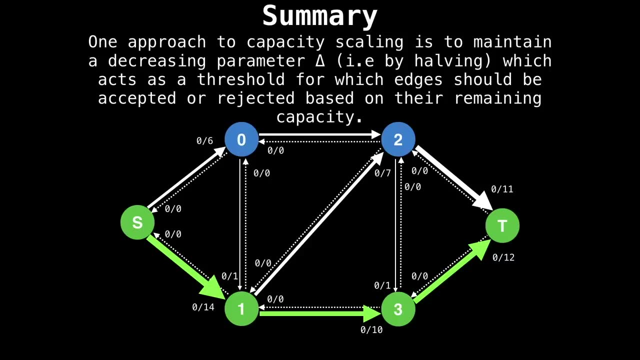 can result in having a bottleneck value of one in each iteration which kills the time. complexity Capacity scaling is when we push flow only through larger edges first to try and achieve a better runtime. One approach to capacity scaling is to maintain the decreasing parameter delta, which acts as a threshold for which edges should be accepted. 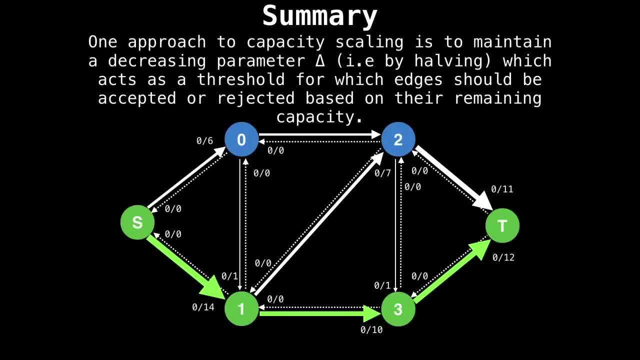 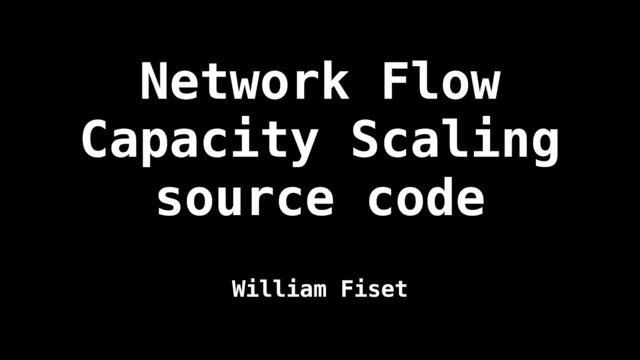 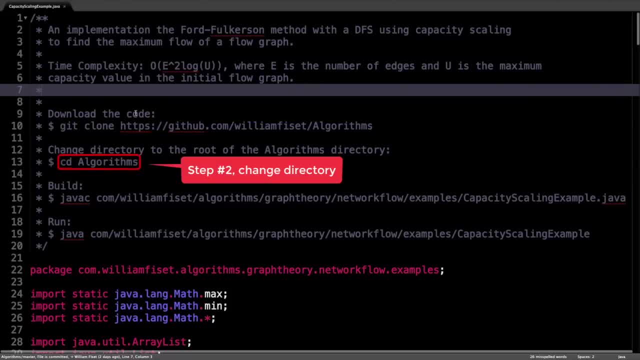 Today we're going to have a look at some source code for the capacity scaling algorithm. OK, here we are on the source code written in Java. I've laid out some instructions here in the header in case you actually want to get the code, play around with it and run it. 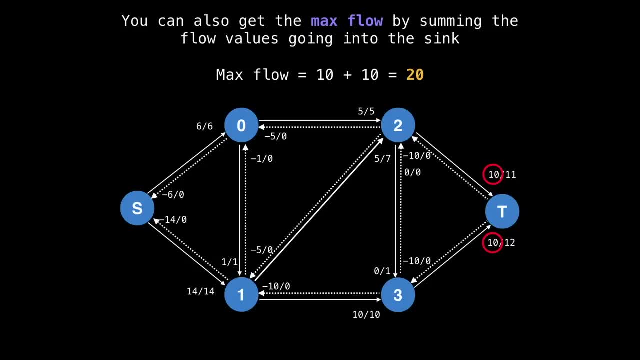 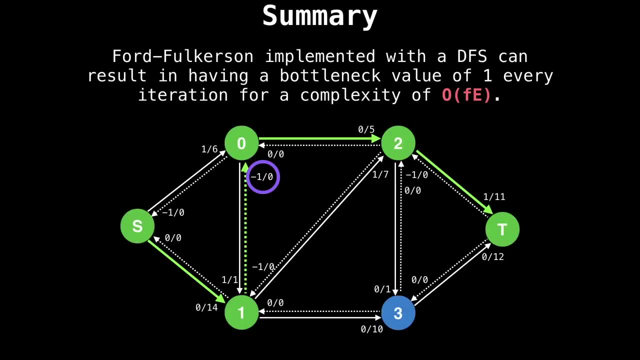 maximum flow by summing the flow values going into the sink highlighted in red. So in summary of what we have learned about, we know that Ford Fulkerson, implemented with a depth first search, can result in having a bottleneck value of one In each iteration, which kills the time. complexity capacity scaling is when we push flow only. 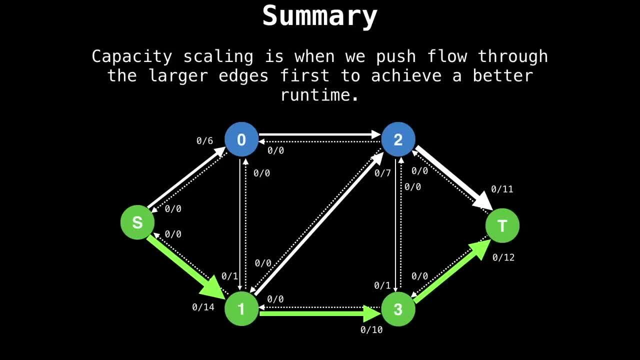 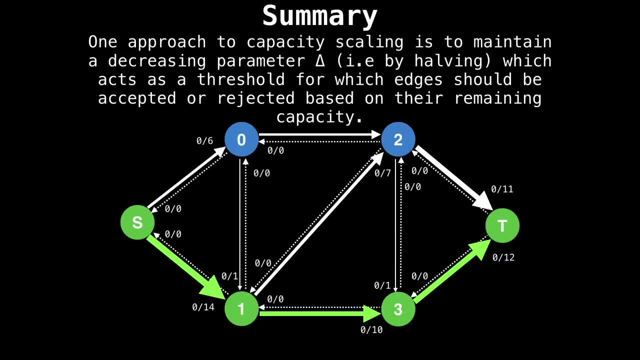 through larger edges first to try and achieve a better runtime. One approach to capacity scaling is to maintain the decreasing parameter delta, which acts as a threshold for which edges should be accepted and which should be rejected, based on their remaining capacity. This is a pretty simple but extremely powerful idea. 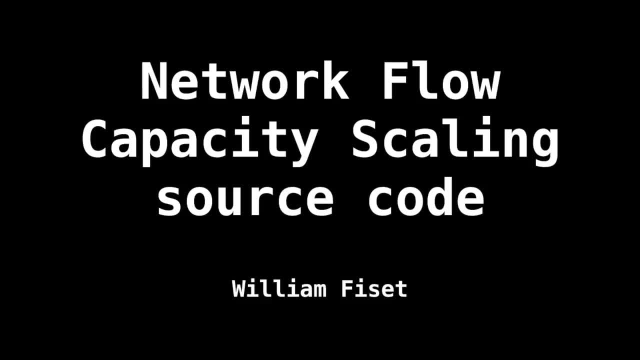 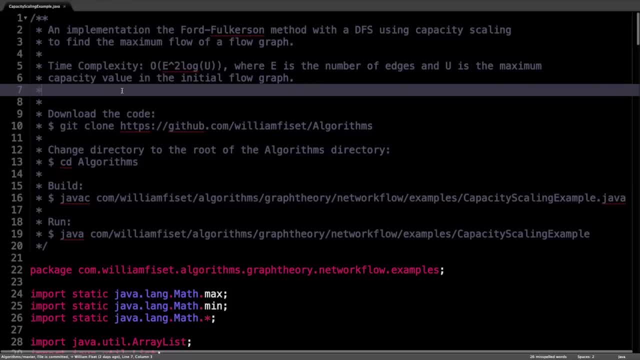 That greatly speeds up finding the maximum flow. Today we're going to have a look at some source code for the capacity scaling algorithm. Okay, here we are on the source code written in Java. I've laid out some instructions here in the header in case you actually want. 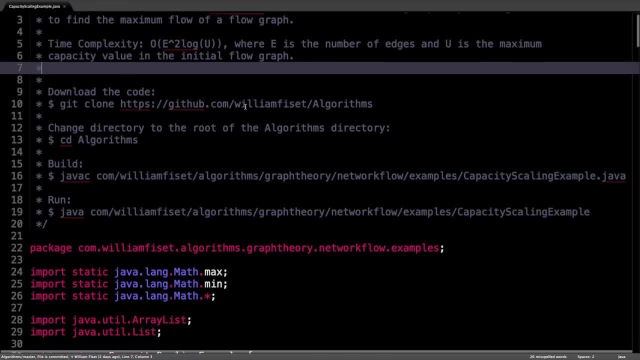 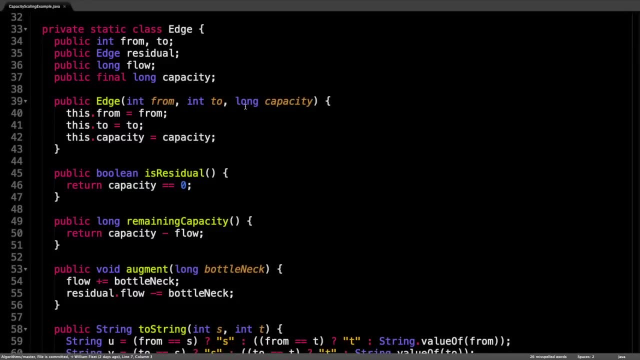 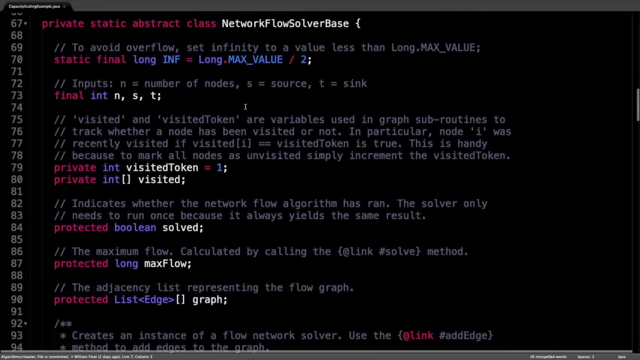 to get the code, play around with it and run it yourself. Scrolling down, you can see we have the familiar edge class here. This is the class used to represent an edge that connects two nodes with a certain capacity. If I scroll a little further down, We have the network flow solver base, which 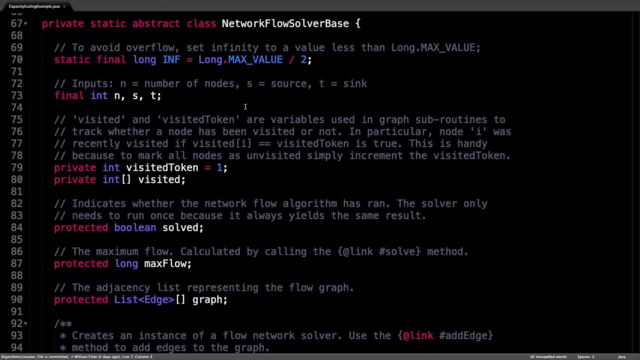 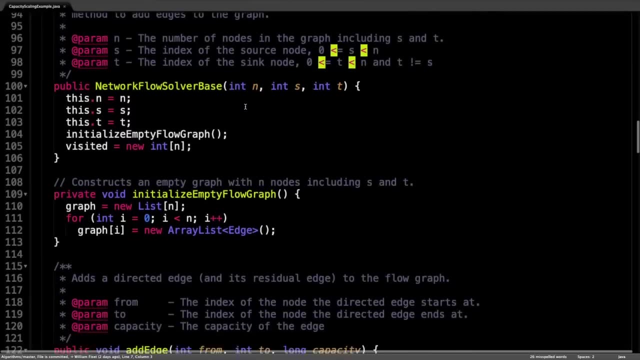 acts as a template for all the different flow algorithms we have been implementing. I have already covered how these two classes work in the previous videos linked below, So please have a look at those before continuing. However, the class we're really interested in is the. 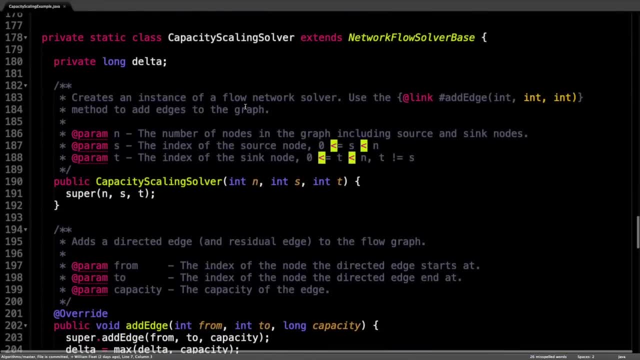 capacity scaling solver. Right here. The capacity scaling solver is an implementation of the network flow solver, our base, which uses capacity scaling to find the maximum flow. you will notice that I have defined one new instance variable in this class, which is called delta. This is the. 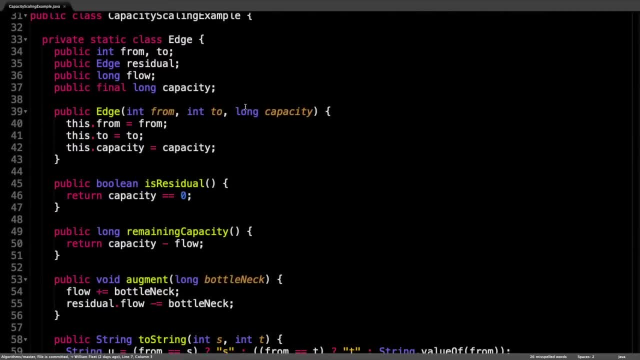 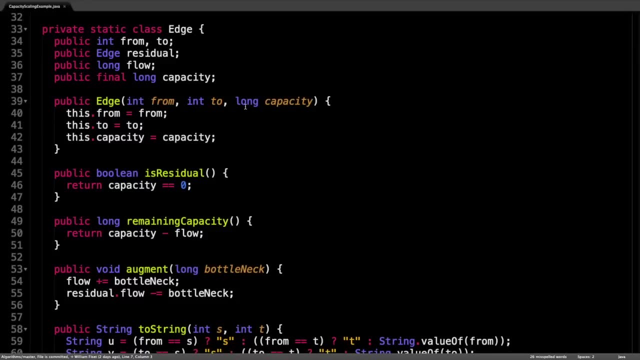 yourself. Scrolling down, you can see we have the familiar edge class here. this is the class used to represent an edge that connects two nodes with a certain capacity. If I hanging, If I scroll a little further down, we have the network flow solver base, which acts as 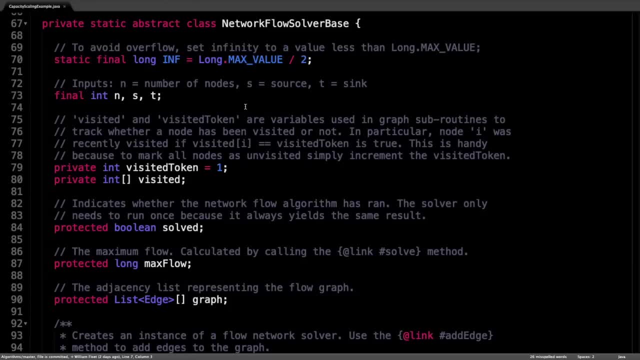 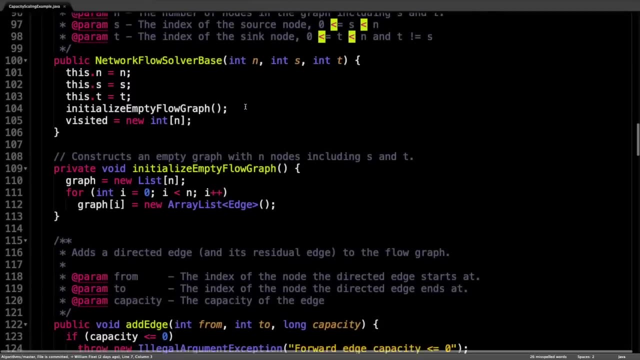 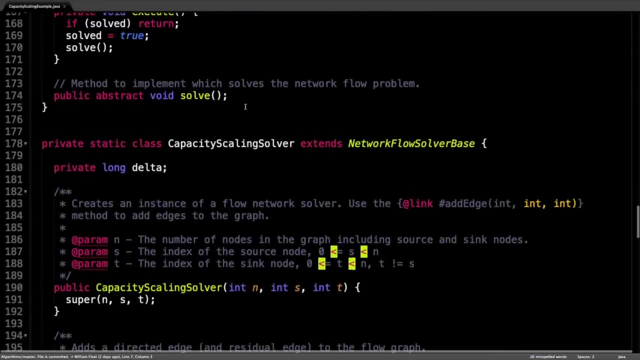 a template for all the different flow algorithms we have been implementing. I have already covered how these two classes work in the previous videos linked below, So please have a look at those before continuing. However, the class we're really interested in is the capacity scaling solver. Right here, The capacity scaling solver is an implementation of the 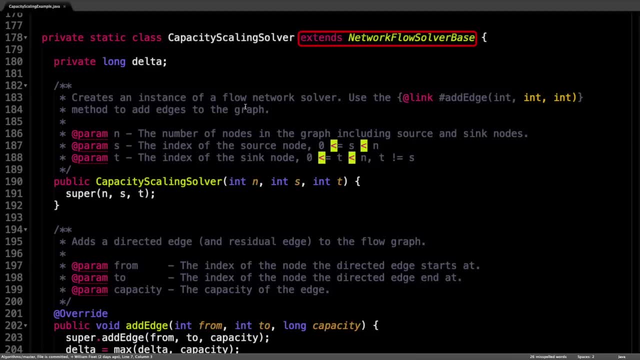 network flow solver base, which uses capacity scaling to find the maximum flow. you will notice that I have defined one new instance variable in this class, which is called delta. This is the same delta that we saw from the slides. It's the parameter we use to determine. 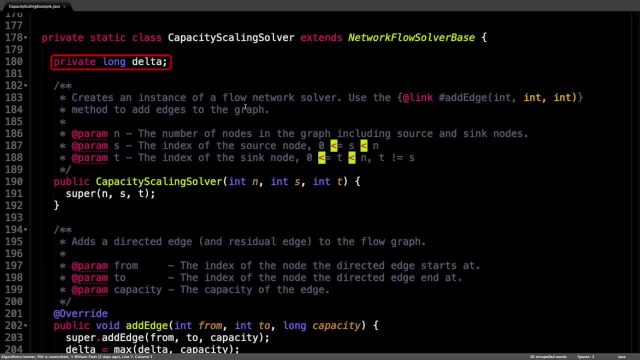 whether an edge should be accepted or rejected based on the remaining capacity relative to the value of delta. The constructor for this class simply calls the superclasses constructor to initialize the flow graph and allocate some memory that we'll need to actually push flow through the network. 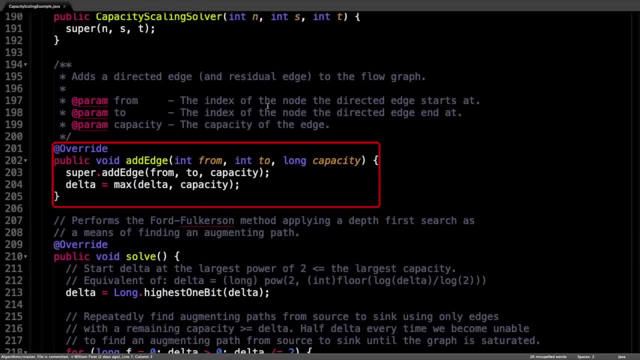 Just below is the add edge method. The add edge method is particularly interesting. for capacity scaling to work, we need to know the value of the edge with the largest capacity in our flow graph, Since we also need to construct the flow graph to actually do anything interesting. 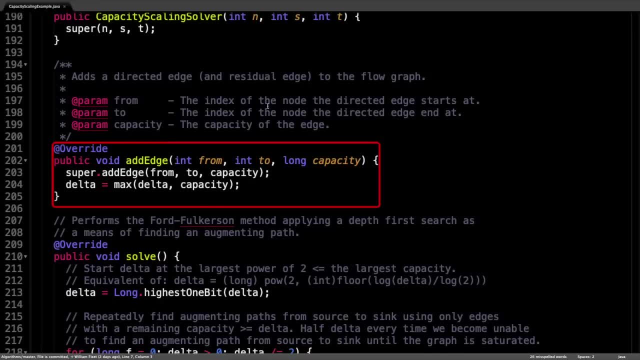 we can capture the largest capacity value as we build the graph. The implementation of the add edge method is defined in the network flow graph. To do this, we need to use the add edge method. This method is called the superclasses add edge method and I also initialize delta to be the largest capacity we encounter as edges. 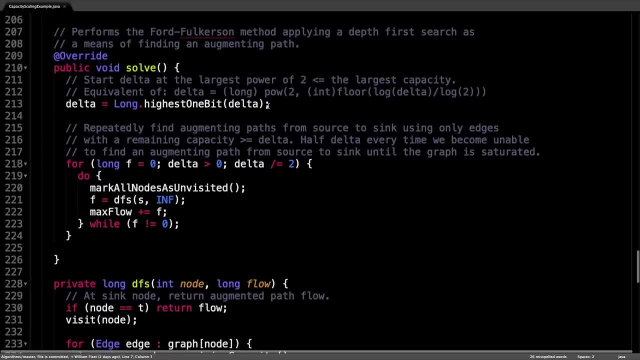 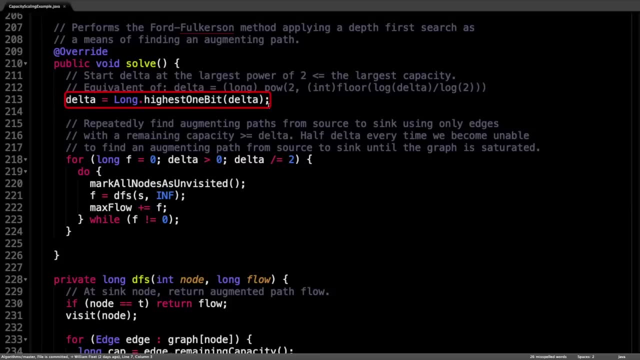 come through simple enough. Inside the solve method, which gets called to compute the maximum flow, the first thing we do is initialize delta to be the largest value of two, And then we get the maximum value of delta, And then we get the maximum value of delta, And. 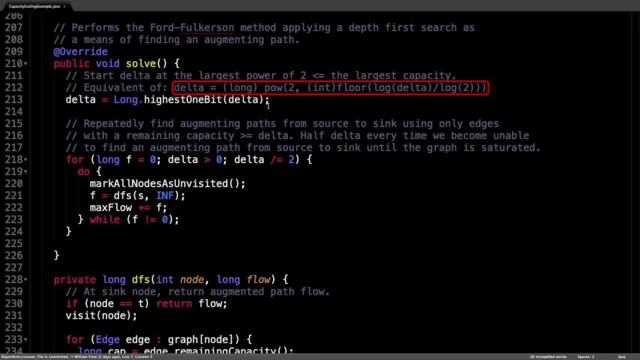 we get the maximum value of delta, And then we get the maximum value of delta, And then we get the maximum value of delta And then the maximum value of delta. just in case we don't have enough layer of delta, we get two less than or equal to the largest capacity. 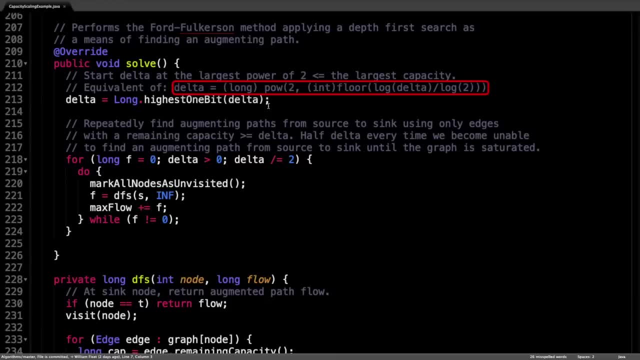 One way to do this is to find the floor of the base to logarithm and then raise that value to a power of two, or in Java, you can simply use the built in function highest one bit to do that for you more efficiently. Following that, we repeatedly find augmenting paths from 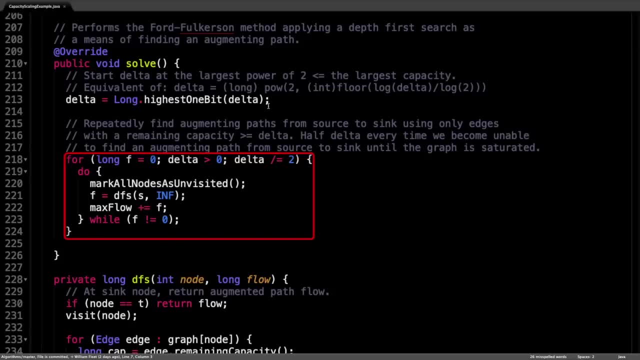 the source to the sink using only edges with a remaining capacity greater than or equal to delta. After each iteration we have the value of delta to allow takinguss CP week smaller edges and being able to find more augmenting paths from the source to the sink. 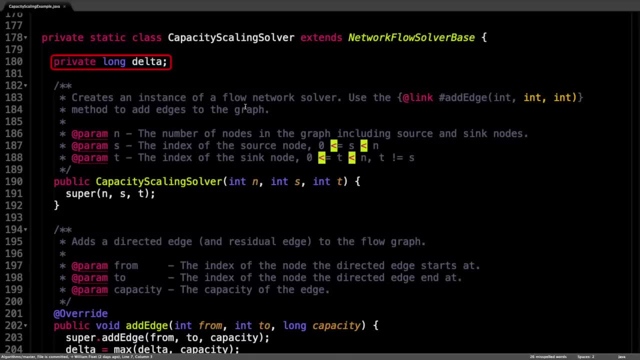 same delta that we saw from the slides. It's the parameter we use to determine whether an edge should be accepted or rejected, based on the remaining capacity relative to the value of delta. The constructor for this class simply calls the superclasses constructor to initialize the flow graph and allocate some memory that we'll need to actually push. 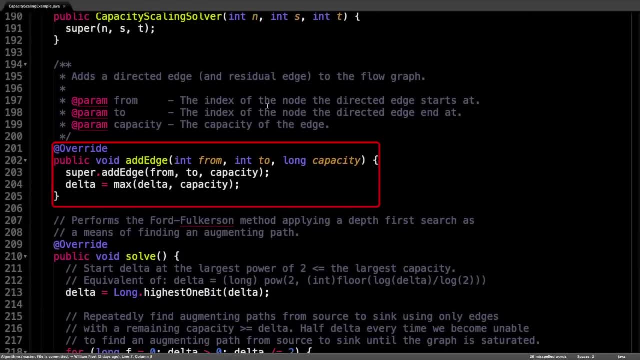 flow through the network. Just below is the add edge method. The add edge method is particularly interesting. For capacity scaling to work, we need to know the value of the edge with the largest capacity in our flow graph, Since we also need to construct the flow graph to. 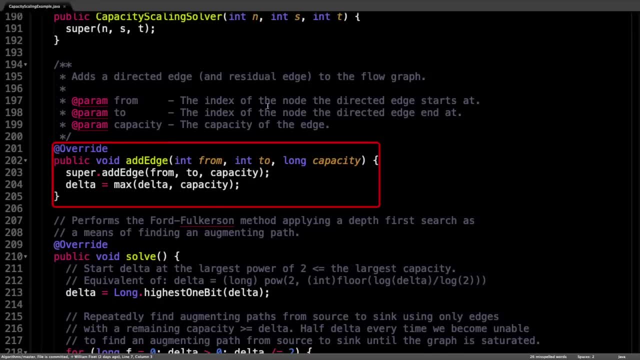 actually do anything interesting. we can capture the largest capacity value as we build the graph. The implementation of the add edge method is defined in the network. We can also work flow solver base, which we don't actually want to change the functionality of, So inside. 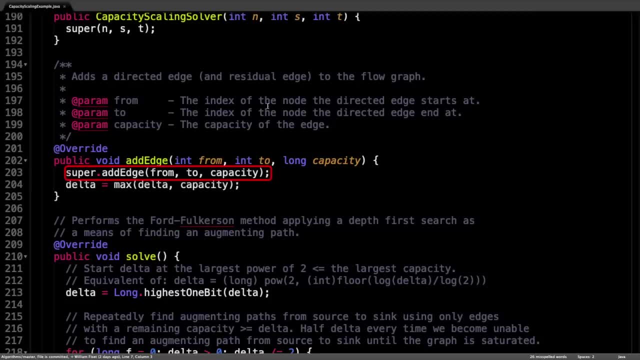 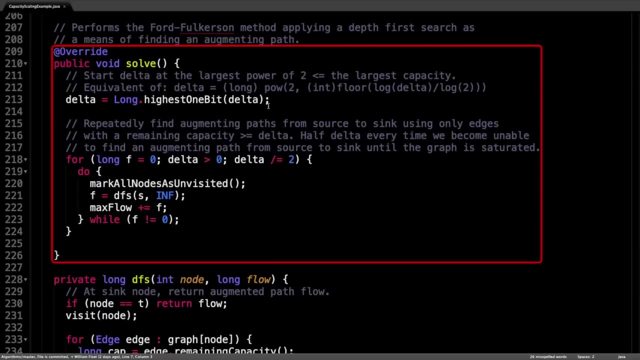 this add edge method which I'm overriding here. all I do is I call the superclasses add edge method And I also initialize delta to be the largest capacity we encounter as edges come through simple enough Inside the solve method which gets called to compute. 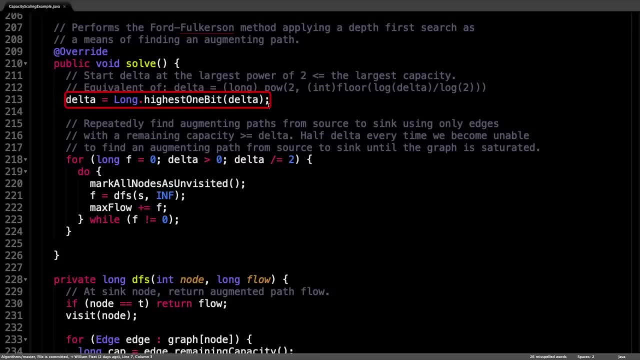 the maximum flow. the first thing we do is initialize delta to be the largest capacity value of delta, And that's just the value of two less than or equal to the largest capacity. One way to do this is to find the floor of the base two logarithm and then raise that. 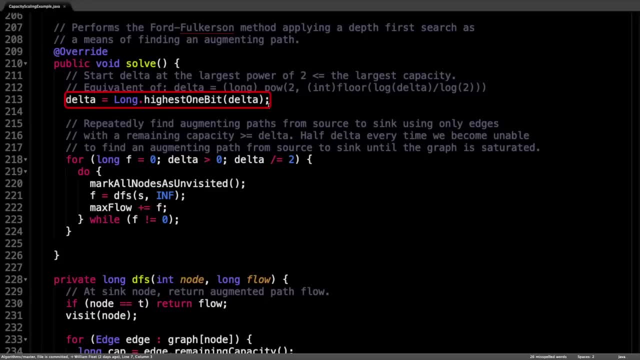 value to a power of two. Or in Java you can simply use the built in function highest one bit to do that for you more efficiently. Following that, we repeatedly find augmenting paths from the source to the sink using only edges, with the remaining capacity greater than or equal. 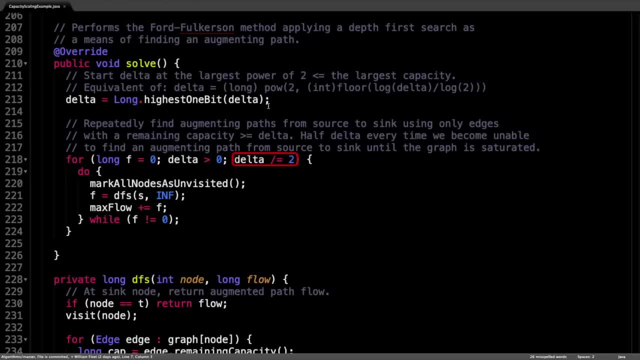 to delta. After each iteration we have the value of delta. to allow us to use the value of delta to compute the maximum flow of the base two logarithm. So we can do that in this case. we can also do that in this case. we can also do that in. 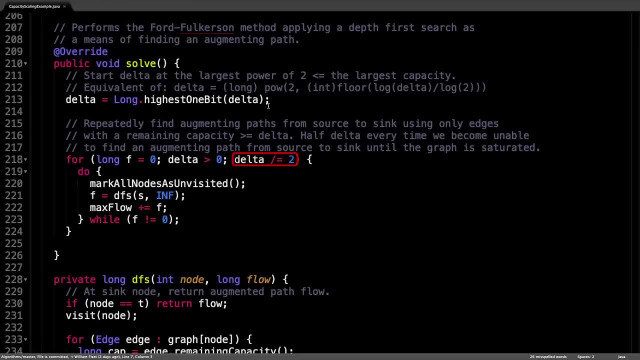 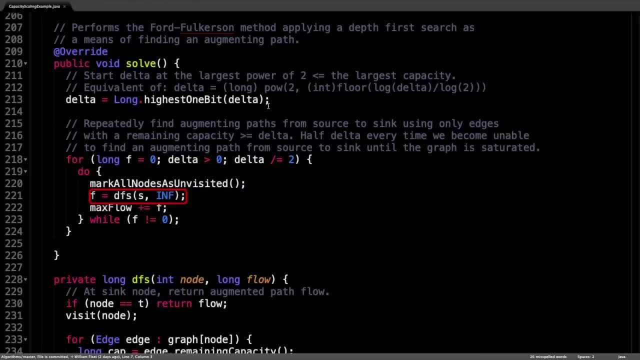 loop. we mark all the nodes as unvisited. Then we do a depth first search, and some over the bottleneck values to calculate the maximum flow. we repeatedly do this until delta is equal to zero. Now let's have a look at the depth first search method. the depth first. 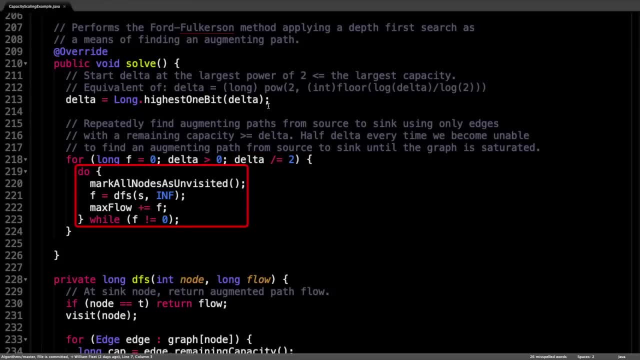 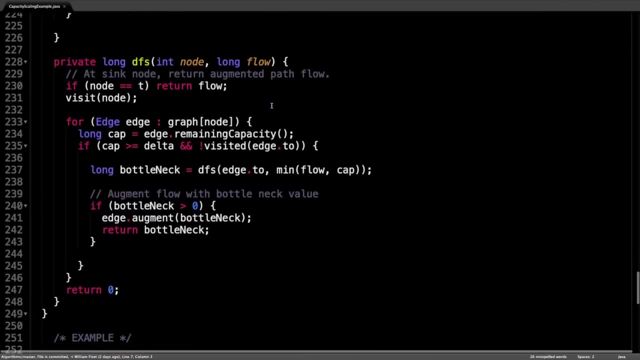 until the graph is fully saturated Inside the inner loop we mark all the nodes as unvisited. then we do a depth first search and some over the bottleneck values to calculate the maximum flow. We repeatedly do this until delta is equal to zero. Now let's have a look at the 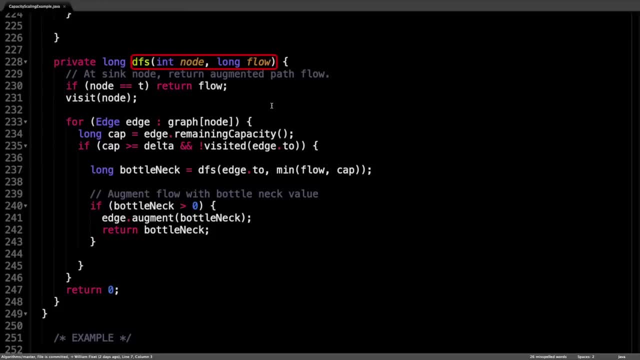 depth first search method. The depth first search method takes two arguments: the current node and the minimum flow found along the path so far. When we initially call this method, the source node is the current node and the flow is set to positive infinity. This method 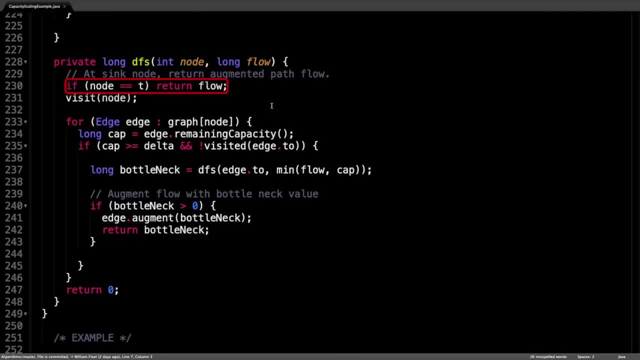 performs the depth first search recursively And we know we can stop searching when we have reached the sink node T. If the current node is not the sink node, then visit the current node and iterate through all the neighbors of the current node. However, here's the 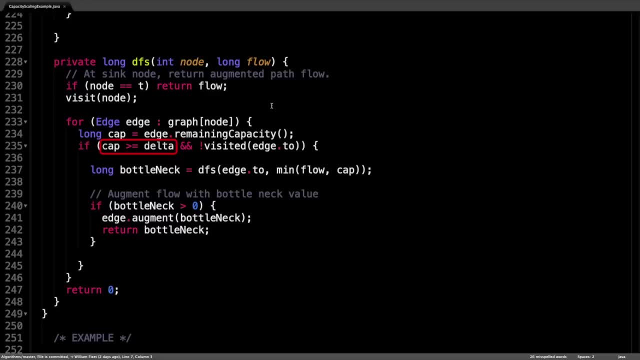 case To catch, though. we cannot take an edge going to a neighboring node if the remaining capacity of that edge is smaller than delta, because this violates the capacity scaling heuristic. We must also ensure that the node we're going to has not already been visited. We do this. 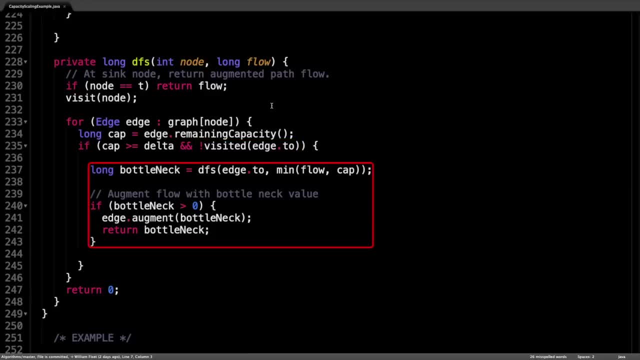 to avoid cycles in the flow graph Inside the inner if statement, we call the depth first search method recursively passing the node we're going to as the current node and the new flow as the minimum of the current flow, and this edges remaining capacity. We 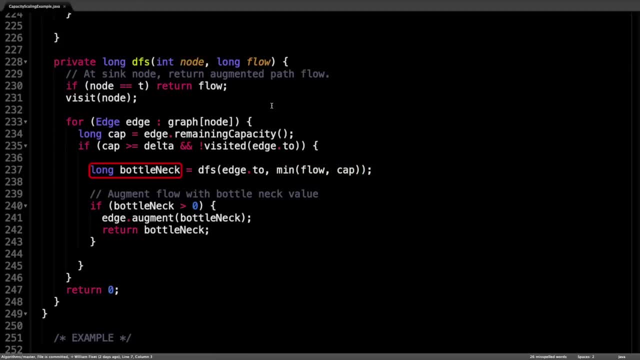 can see that the depth first search returns the bottleneck value along the augmenting path. So after the depth first search call, we are unwinding the call stack from the sink back to the source. This is a perfect time to augment the flow of each edge along the 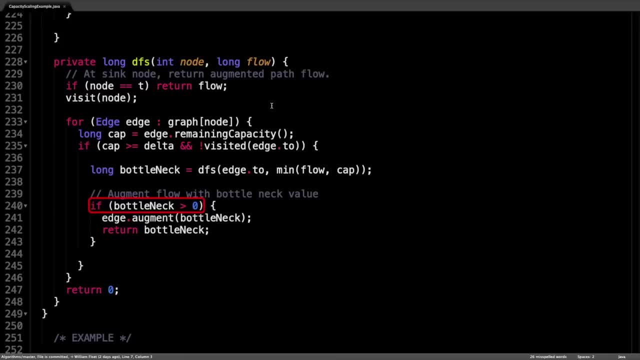 augmenting path, since we have the bottleneck value right there. So if the bottleneck value is greater than zero, this means we have found a valid augmenting path and we want to augment the flow, which is, remember, adding flow along forward edges and subtracting the flow along 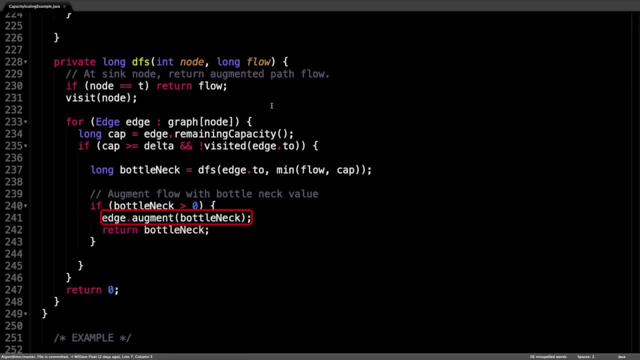 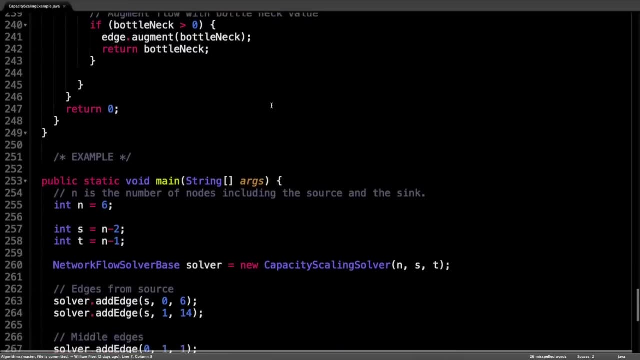 residual edges. This is all done through the argument method in the edge class and finally return the bottleneck value. If we scroll down even more, you can see that this is the main method right here In here I set up an example of how to set up a flow. 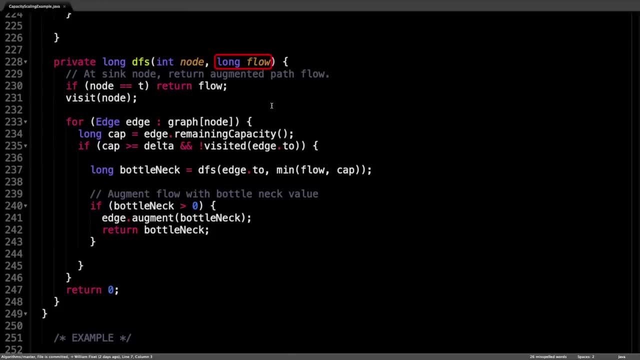 search method takes two arguments: the current node and theiatric, As drawn to alpha and the minimum value. the search method means that this survive a further 12 minutes after your code runs or, if you want, you can collect some binary data which 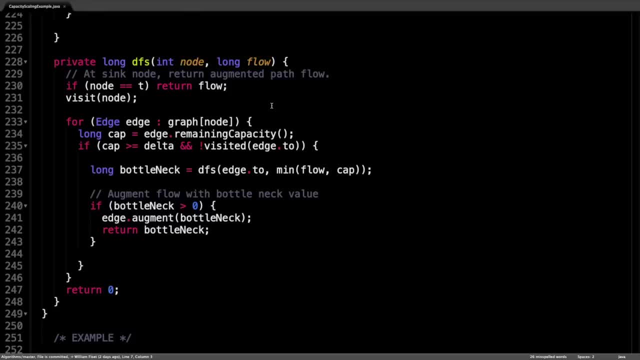 minimum flow found along the path so far. When we initially call this method, the source node is the current node and the flow is set to positive infinity. This method performs the depth first search recursively And we know we can stop searching when we have reached. 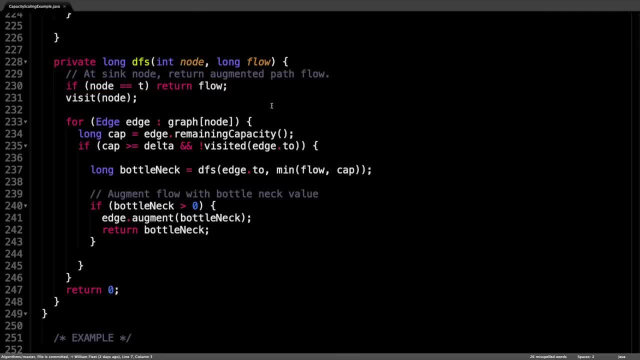 the sink node T. If the current node is not the sink node, then visit the current node and iterate through all the neighbors of the current node. However, here's the catch, though: we cannot take an edge going to a neighboring node if the remaining capacity of that edge 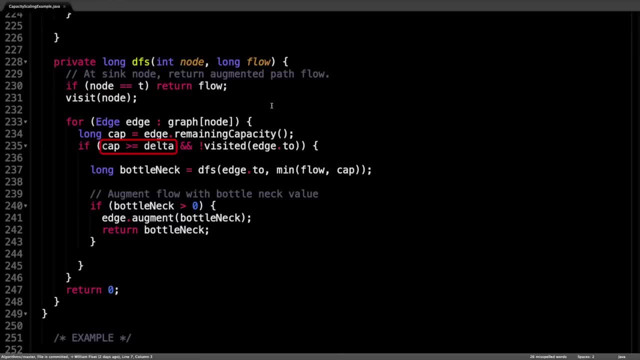 is smaller than delta, Because this violates the capacity scaling heuristic. We must also ensure that the node we're going to has not already been visited. We do this to avoid cycles in the flow graph. Inside the inner if statement, we call the depth for search. 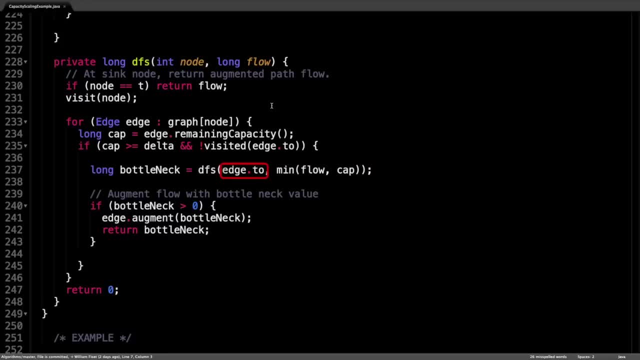 method: recursively passing the node we're going to as the current node and the new flow as the minimum of the current flow. and this edges remaining capacity. the depth for search returns the bottleneck value along the augmenting path. So after the depth for search call, we are unwinding the call stack from the sink back to the source. 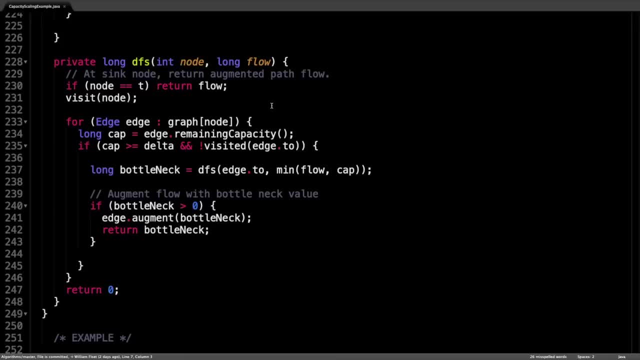 this is a perfect time to augment the flow of each edge along the augmenting path, since we have the bottleneck value right there. So if the bottleneck value is greater than zero, this means we have found a valid augmenting path and we want to augment the flow, which 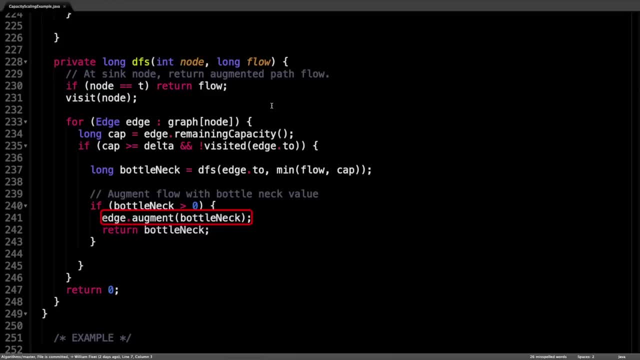 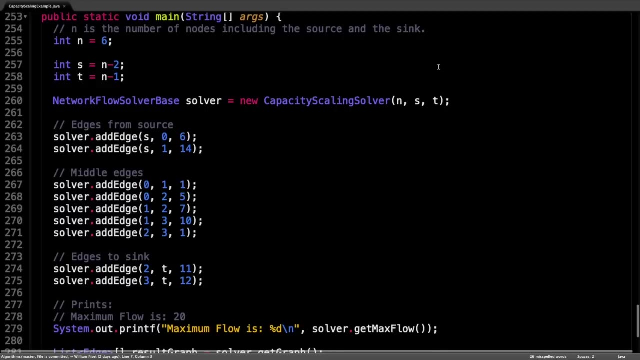 is, remember adding flow along forward edges and subtracting flow along residual edges. This is all done through the argument method in the edge class And finally return the bottleneck value. If we scroll down even more, you can see that this is the main method, right? 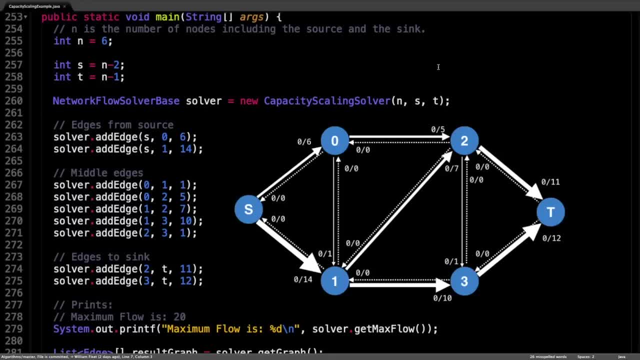 here In. here I set up an example of how to set up a flow graph. Specifically, this is the flow graph from the slides. So I create a flow solver, I add all the edges and then I push some flow graph. So I create a flow solver, I add all the edges and then I push some flow. 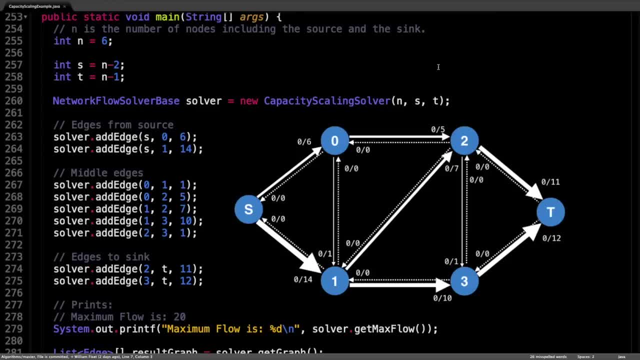 graph. So I create a flow graph. So I create a flow graph, So I go through it and get the maximum flow. I also display the resulting flow graph after the flow algorithm has been executed, So you can see what happened. Awesome, That's all I wanted to cover for capacity. 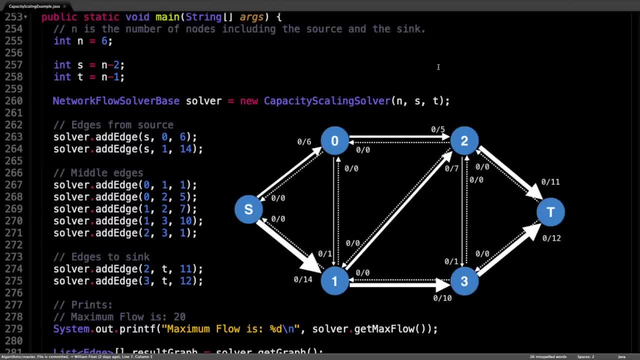 graph. Specifically, this is the flow graph from the slides. So I create a flow solver, I add all the edges and then I push some flow through it and get the maximum flow. I also display the resulting flow flow graph after the flow algorithm has been executed, So you can see what happened- Awesome. 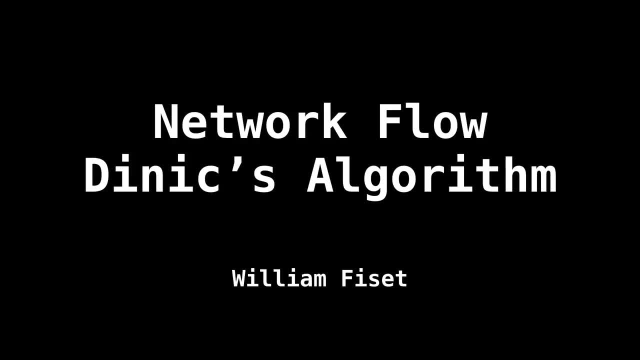 That's all I wanted to cover for capacity scaling. Today we're still talking about network flow And, in particular, we're looking at finding the maximum flow and a new, very efficient method of solving the unweighted bipartite matching problem. The next algorithm: 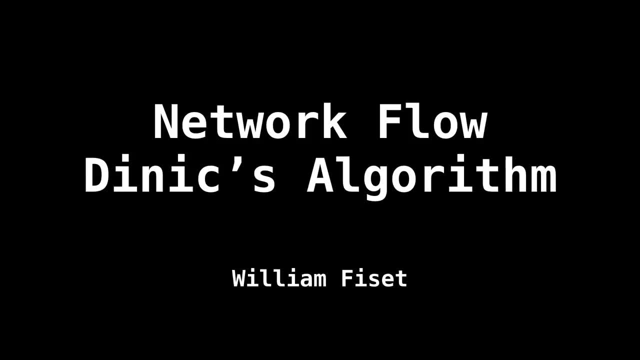 is one of those extremely fast and revolutionary algorithms which really push the field of network flow forwards. It was one, if not the first algorithm to introduce a bunch of new concepts like building a level graph, combining multiple graph traversal techniques together and the concept of a blocking flow, all of which we'll 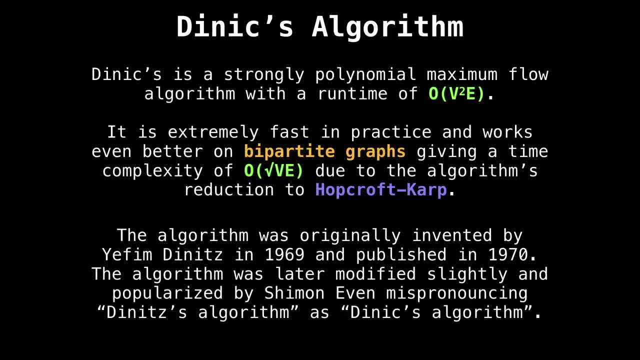 get into. So what is the next algorithm? It's a fast, strongly polynomial maximum flow algorithm. The fact that it's strongly polynomial is important. It means that the runtime doesn't depend on the capacity values of the flow graph, for which all we know could be very 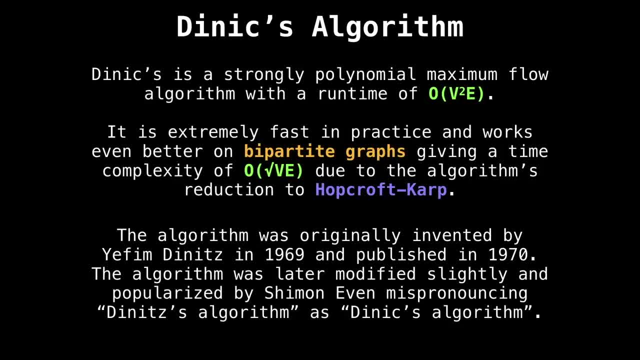 large. What's remarkable about denix is that not only is it fast in practice for general graphs, but it boasts performance on bipartite graphs running in a time complexity of big O, of square root, v, times, e. The importance of this cannot be overstated. It makes it possible to handle 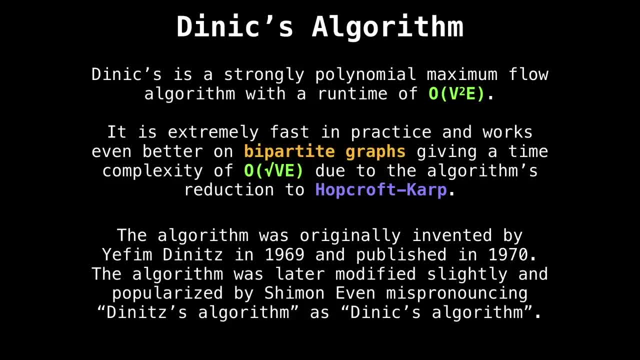 bipartite graphs of a ridiculous size If you're doing competitive programming. denix is the de facto standard algorithm to solve maximum flow algorithms. The algorithm will be conceived in 69 by Ephraim Dennett's and published in 1970.. The algorithm was later. 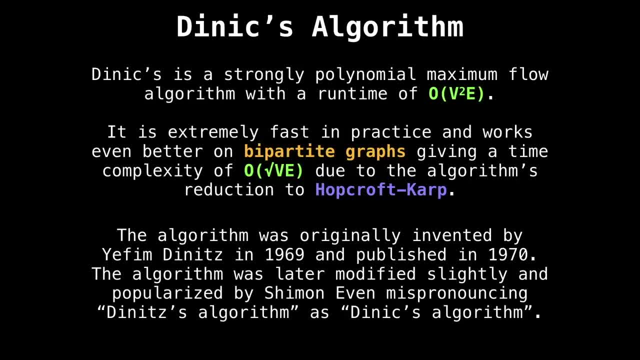 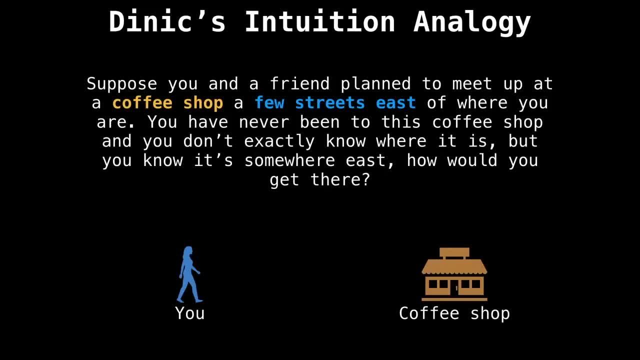 modified slightly and popularized by Shimon Evan, mispronouncing Dennett's algorithm as denix algorithm. Let's start by talking about the algorithm itself, But first beginning with an analogy. Suppose you and a friend are planning to meet up at the coffee shop. 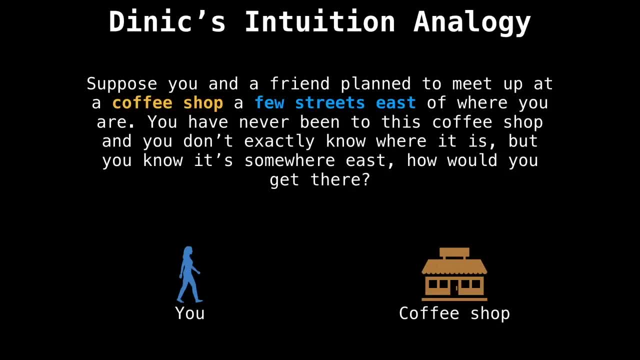 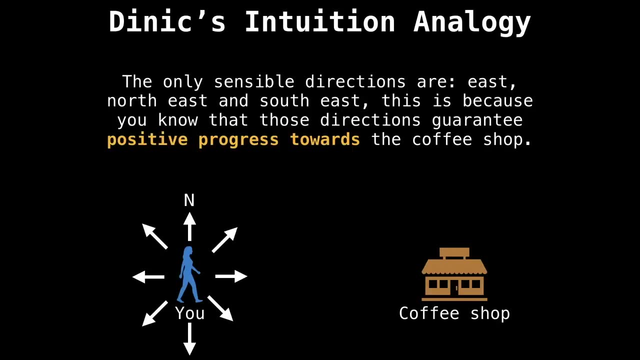 a few streets east of where you are. You've never been to this coffee shop and you don't exactly know where it is, but you know it's somewhere east. So how would you get there With the information you have? would it make sense to head south? What about Northwest? 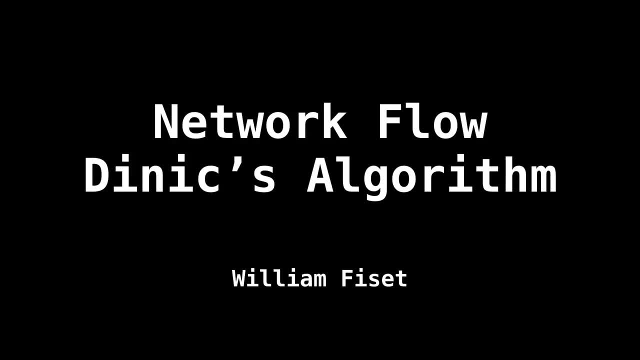 scaling. Today we're still talking about network flow And, in particular, we're looking at finding the maximum flow and a new, very efficient method of solving the unweighted bipartite matching problem. The next algorithm is one of those extremely fast and revolutionary. 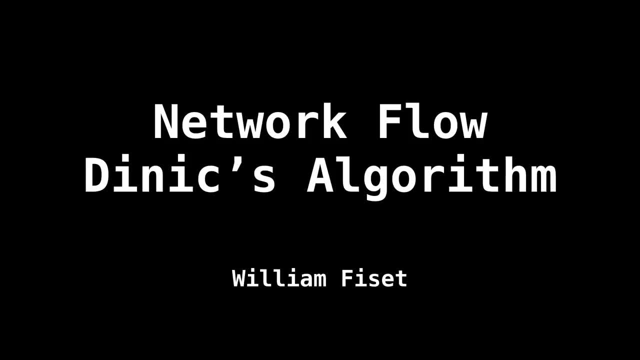 algorithms which really pushed the field of network flow forwards. It was one, if not the first algorithm to introduce a bunch of new concepts like building a level graph, combining multiple graph traversal techniques together and the concept of a blocking flow, all of which we'll get into. So what is the next? 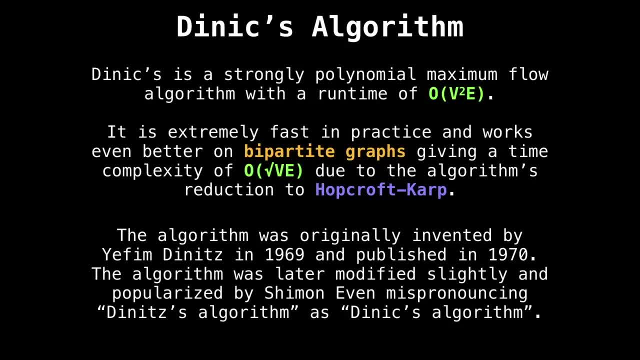 algorithm. It's a fast, strongly polynomial maximum flow algorithm. The fact that it's strongly polynomial is important. It means that the runtime doesn't depend on the capacity values of the flow graph, For which all we know could be very large. What's remarkable about Dynix is that not only is 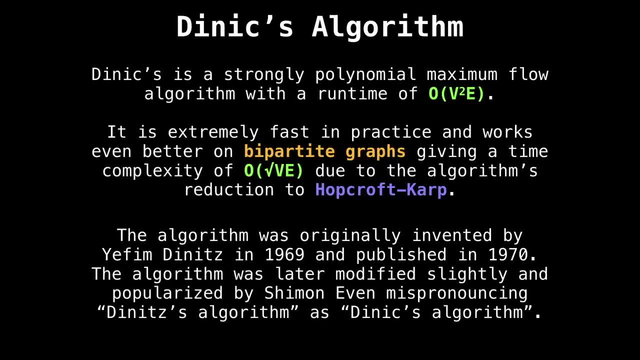 it fast in practice for general graphs, but it boasts performance on bipartite graphs running in a time complexity of big O, of square root, v times e. the importance of this cannot be overstated. It makes it possible to handle bipartite graphs of a ridiculous size If 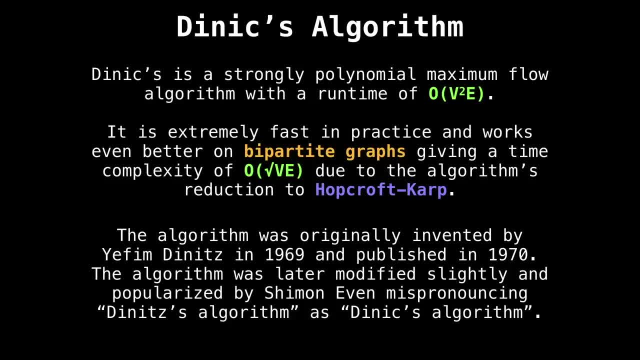 you're doing competitive programming. Dynix is the de facto standard algorithm to solve maximum flow algorithms. The algorithm was conceived in 69 by Ephraim Dennett's and published in 1970. The algorithm was later modified slightly and popularized by Shimon Evan, mispronouncing Dennett's algorithm as Dynix algorithm. Let's start by talking. 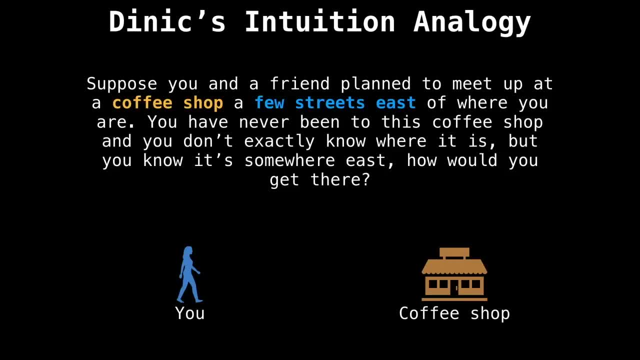 about the algorithm itself. But first, beginning with an analogy, suppose you and a friend are planning to meet up at the coffee shop a few streets east East of where you are. you've never been to this coffee shop and you don't exactly know. 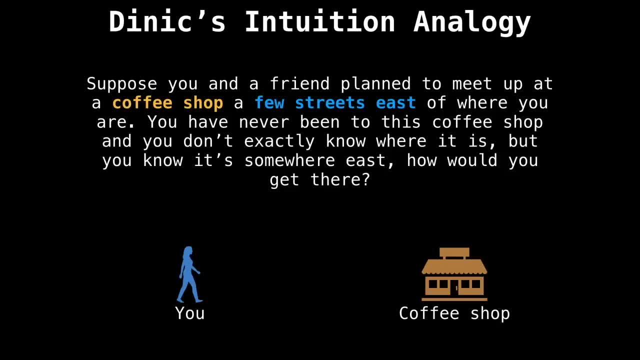 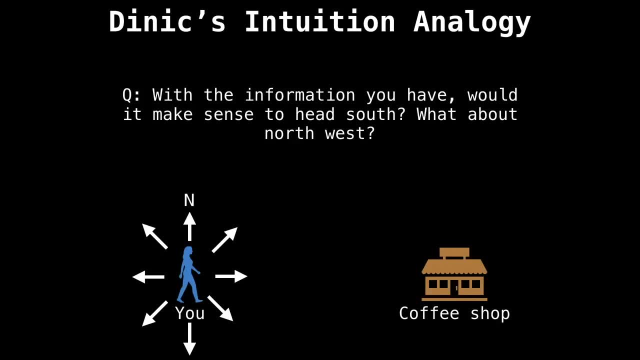 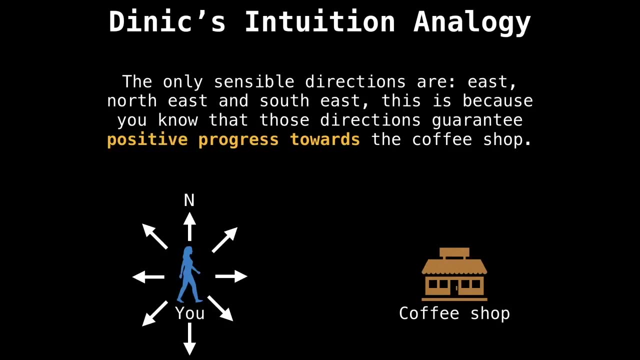 where it is, But you know it's somewhere east. So how would you get there With the information you have? would it make sense to head south? What about Northwest? The only sensible directions are east, northeast and southeast. This is because you know that those 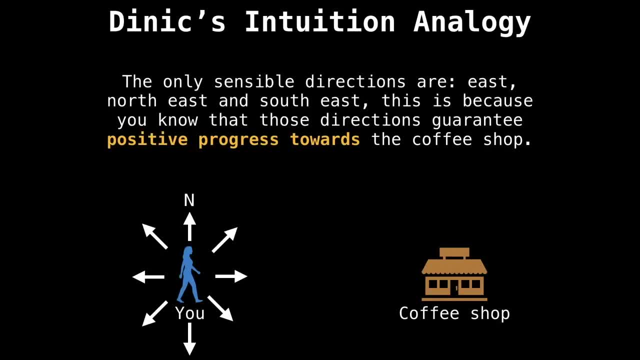 the only sensible directions are east, north east and south east. This is because you know that those directions guarantee that you make a positive progress towards the coffee shop. This form of heuristic ensures that we continuously make progress, progress towards whatever place of interest we desire to go. So how can we apply this? 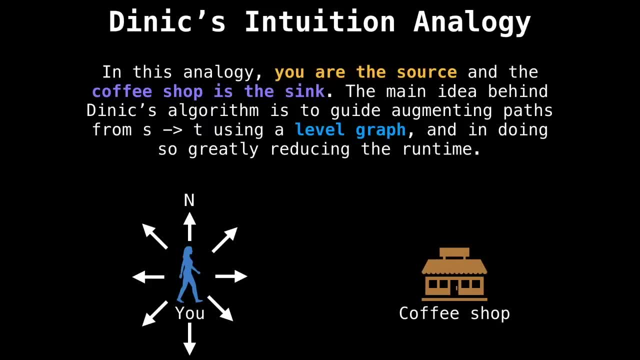 concept to solving the maximum flow. In this analogy, you are the source node and the coffee shop is the sink. The main idea behind Dynx algorithm is to guide augmenting paths from the source to the sink using a level graph and, in doing so, greatly reducing the runtime. 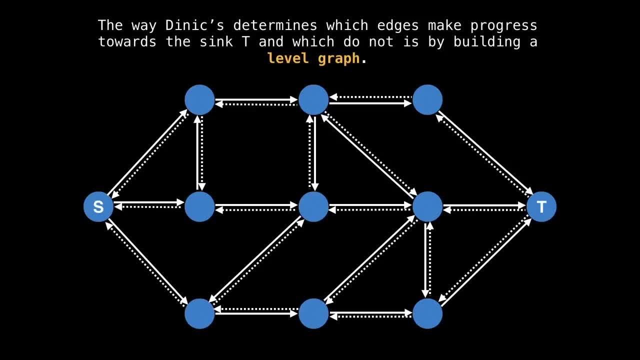 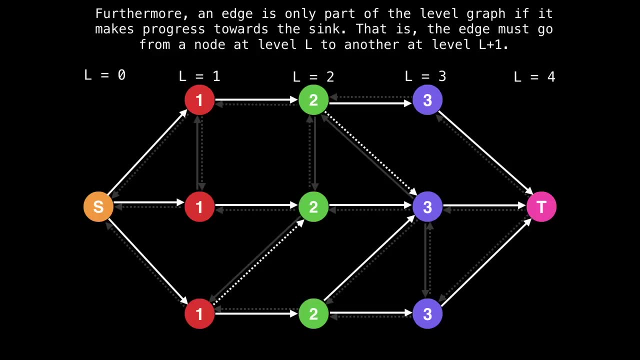 The way Dynx determines what edges make progress towards the sink T and which do not is by building what's called a level graph. The levels of a graph are those obtained by doing a breadth first search from the source. Furthermore, an edge is only part of the level graph if 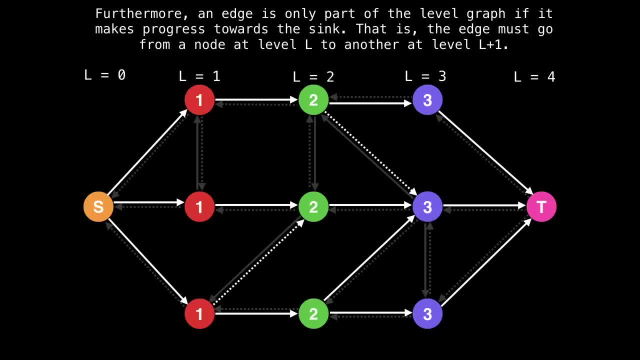 it makes progress towards the sink. That is, an edge must go from a node at level l to another node at level l plus one. the requirement that edges must go from l to l plus one prunes backwards, or what I call sideways edges. Those are all. 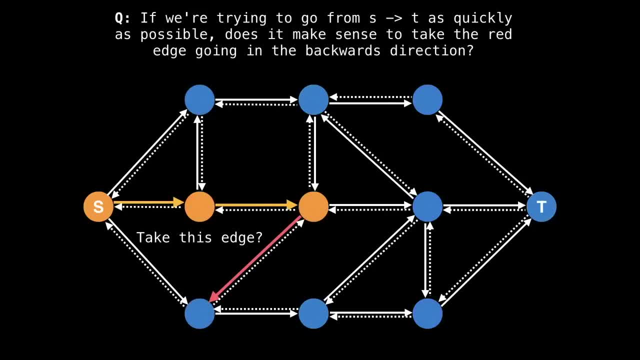 the gray edges in the slide. So ask yourself, if you're trying to get from s to t as quickly as possible, Does it make sense to take the red edge going in the backwards direction on the slide? No, taking the red edge doesn't bring you any closer to the sink, So it should. 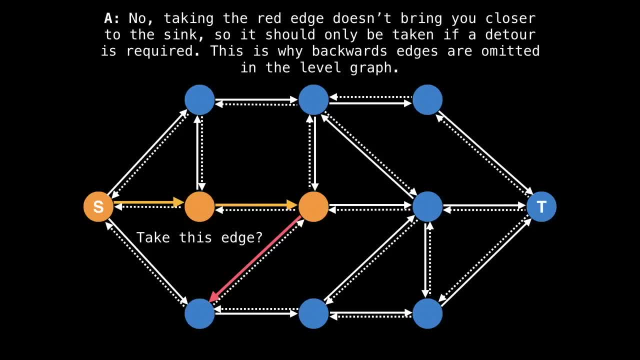 only be taken if a detour is required. This is why we're going to use the red edge: to get the red edge to go from l to l plus one. This is why backwards edges are omitted from the level graph. The same thing can be said. 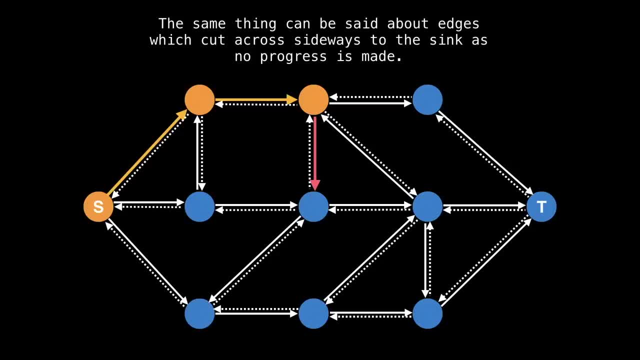 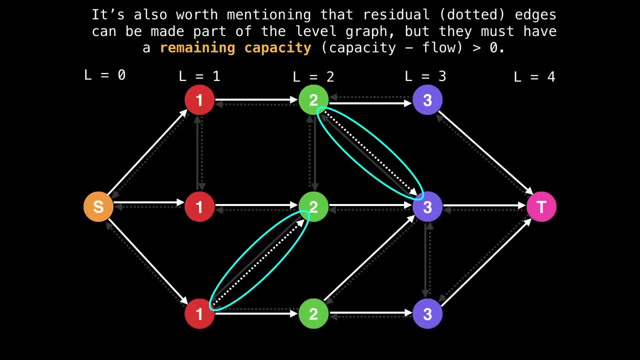 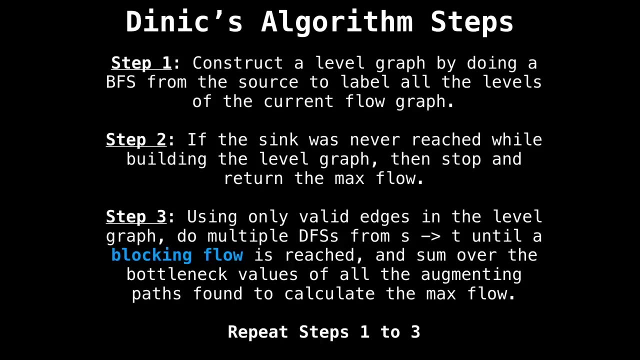 about edges which cut across sideways, across the same level, since no progress is made. It's also worth mentioning that residual edges can be made part of the level graph, but they must have a remaining capacity greater than zero. So that's the level graph, The actual. 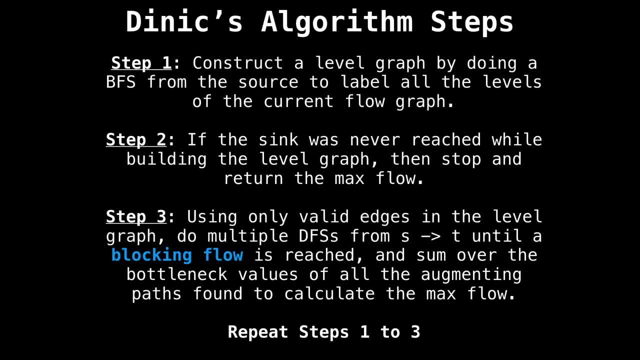 steps to executing Dynics are as follows: First, construct a level graph by using the Анvisa flow graph, So allow Dynica to be made. I will be using a cost run from the level graph. If you want to use a cost run, you need to create a functional flow graph, which is the one you use in this. 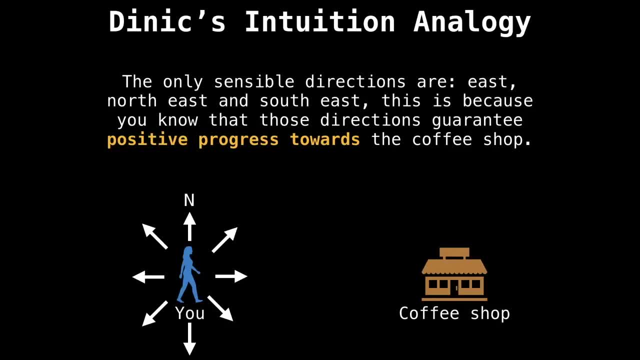 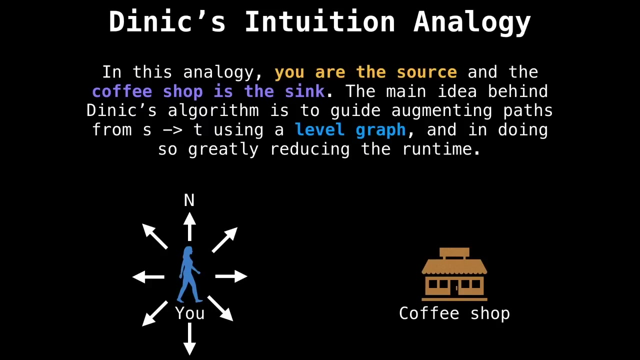 directions guarantee that you make a positive progress towards the coffee shop. This form of heuristic ensures that we continuously make progress towards whatever place of interest we desire to go. So how can we apply this concept of solving the maximum flow? In this analogy, you were the source node and the coffee shop is the sink, The main idea behind 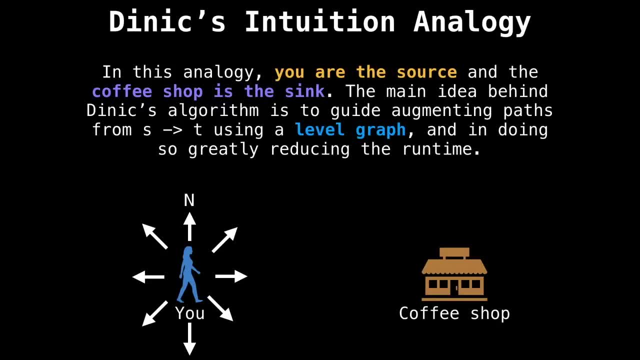 Dynix algorithm is to guide augmenting paths from the source to the sink using the level graph And, in doing so, greatly reducing the runtime. The logic behind this path is to keep the coffee shop on a safe path and therefore all the different scenarios that exist where 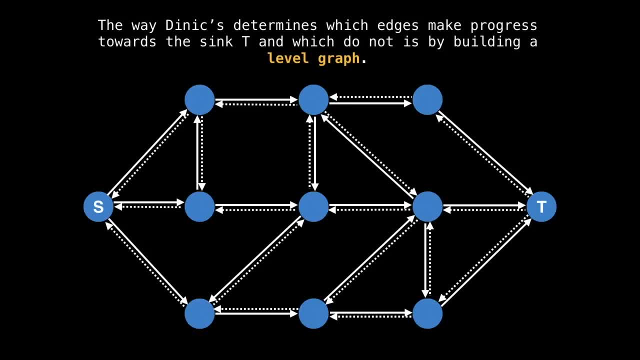 we're having to go are looped in the same path. So the sort of linearization of it is. The way Denix determines what edges make progress towards the sink T and which do not is by building what's called a level graph. The levels of a graph are those obtained by doing. 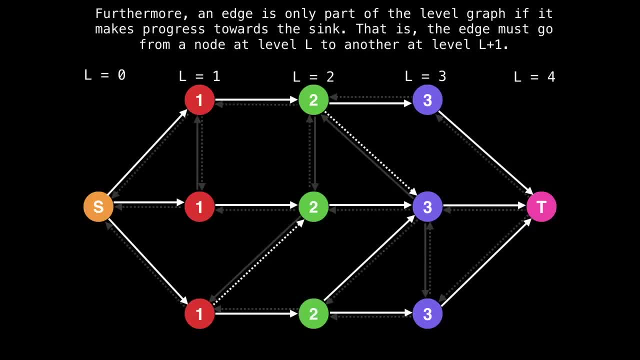 a breadth. first search from the source. Furthermore, an edge is only part of the level graph if it makes progress towards the sink. That is, an edge must go from a node at level L to another node at level L plus one. the requirement that edges must go from L to L plus one prunes. 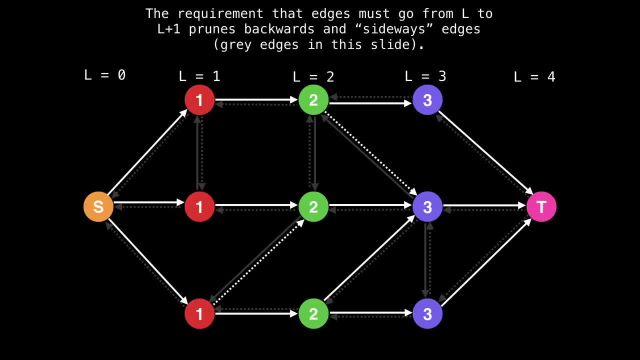 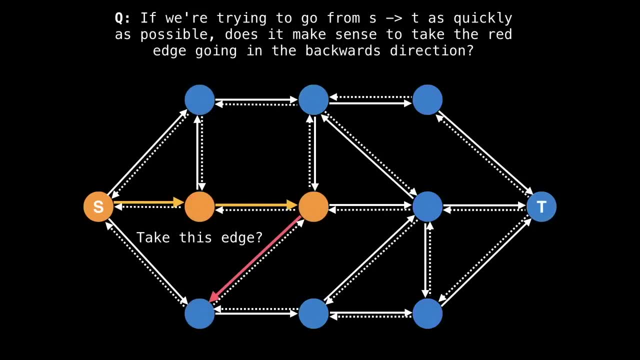 backwards, or what I call sideways edges. Those are all the gray edges in the slide. So ask yourself, if you're trying to get from s to t as quickly as possible, does it make sense to take the red edge going in the backwards direction on the slide? No, taking the red. 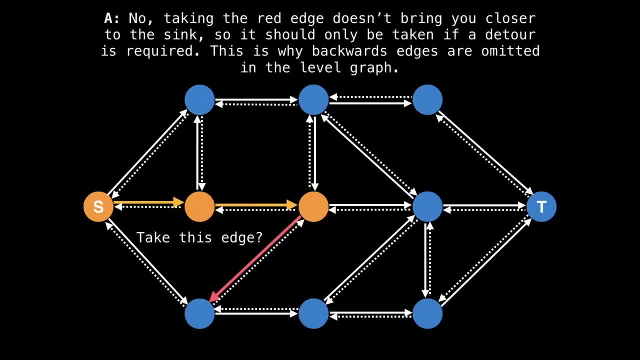 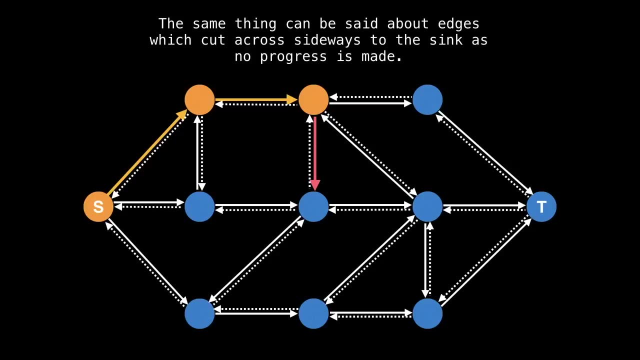 edge doesn't bring you any closer to the sink, So it should only be taken if a detour is required. This is why backwards edges are omitted from the level graph. The same thing can be said about edges which cut across sideways across the same level, since no progress is made. It's also worth mentioning that residual 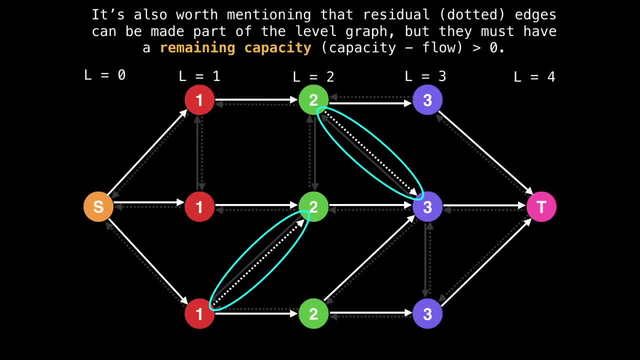 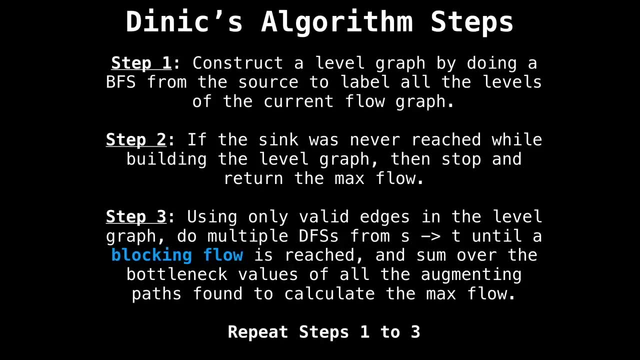 edges can be made part of the level graph, but they must have a remaining capacity greater than zero. So that's the level graph. the actual steps to executing dynamics are as follows: First, construct a level graph by doing a breadth. first, search from the source to label all the levels of the current flow graph. Then particular case. we'll be doing that in just a few slides. The only things that you need is the post run, which is the tag method for in the original Dynix. So we need to create a real wealth level graph And then we need to make the second level graph And the last. 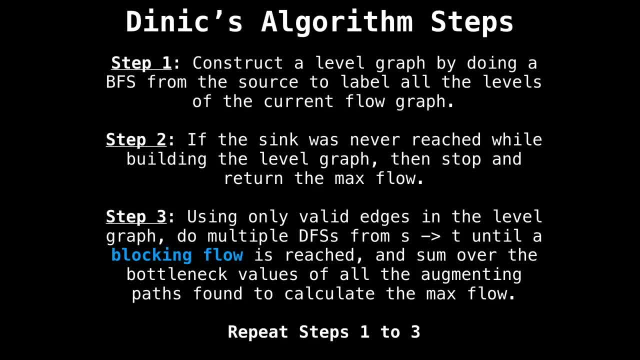 step is to use the flow graph by doing a breadth first search from the source to label all the levels of the current flow graph. Then if the sink was never reached while building the level graph, you know you can stop and return the value of the maximum flow. then 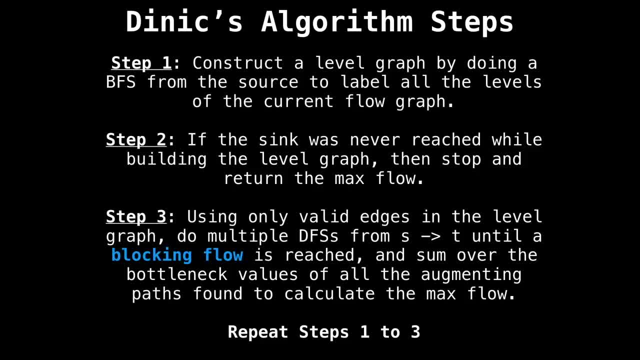 using only valid edges in the level graph. do multiple depth first searches from the source to the sink until a blocking flow is reached and some over the bottleneck values of all augmenting paths. calculate the maximum flow. as you do this, Repeat steps 123.. A blocking 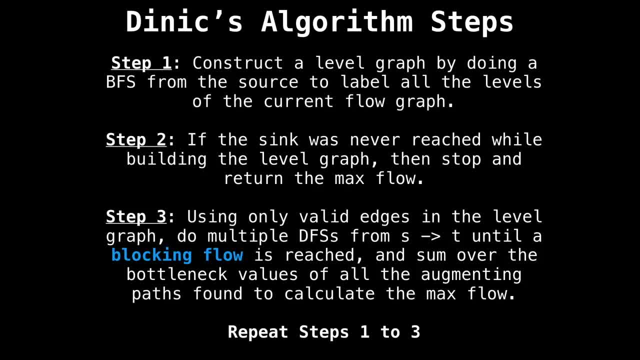 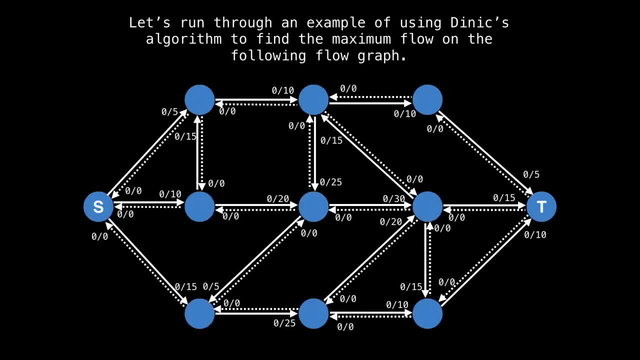 flow is when we cannot find any more paths from the source to the sink because too many edges in the level graph have been saturated. This will all become clear with an example. Let's use Denix algorithm to find the maximum flow of this flow graph If this were a bipartite. 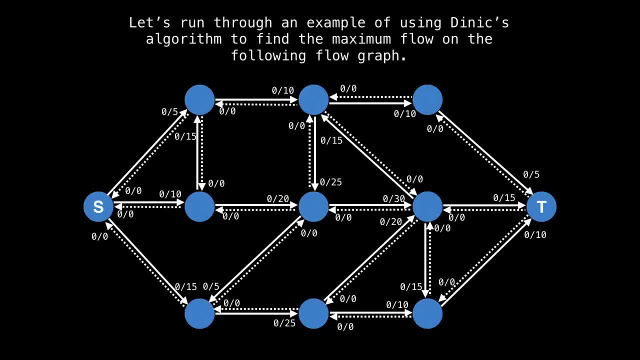 graph. we would also be able to get a maximum matching as a result. All right, step one is to figure out which edges are part of the current level graph. you don't need to think of the level graph as a totally separate graph. You can think of it rather as a subset of 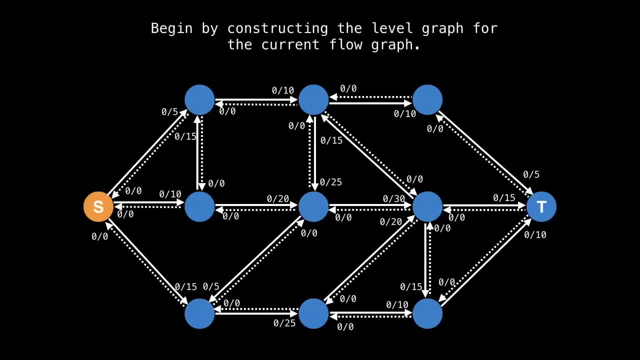 the edges. So we start at the source and do a breadth first, search outwards. The first layer includes all the red nodes, Then this is the second layer, and so on until we reach the sink. Now, if we focus on the edges, which 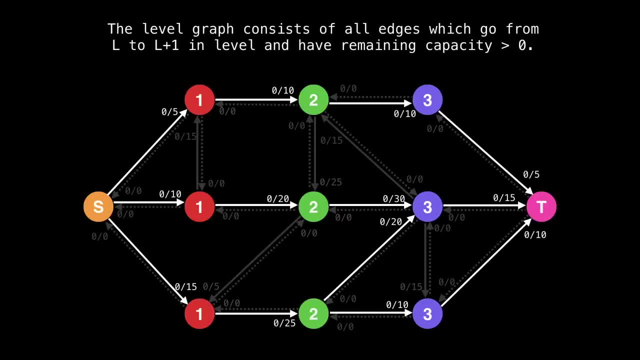 form the level graph. we can see that they are all edges which go from L to L, plus one and level, and have a remaining capacity greater than zero. Step two of the algorithm is to find paths from s to t until a blocking flow is reached, That is, we cannot find any more. 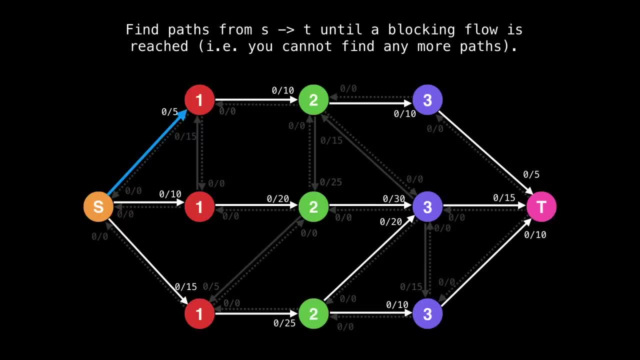 paths through the level graph. So we start at the source and do a depth first search on the edges of level graph until the sink is reached. So we found our first augmenting path and the bottleneck value along this path is five, since five is the smallest remaining. 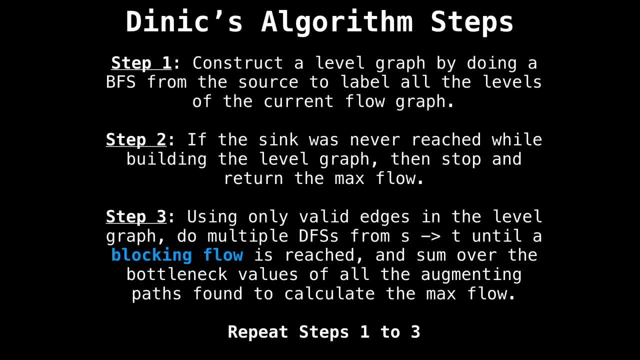 if the sink was never reached. while building the level graph, you know you can stop and return the value of the maximum flow. then, using only valid edges in the level graph, do multiple depth first searches from the source to the sink until a blocking flow is. 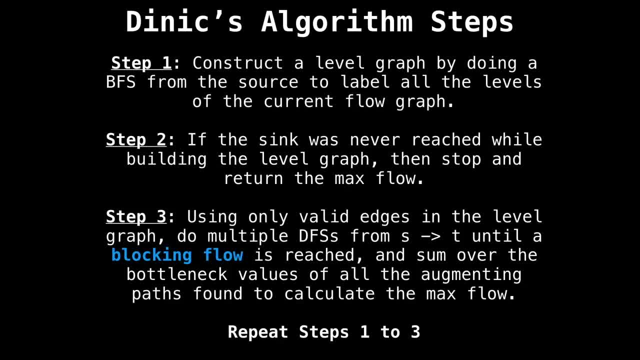 reached And some over the bottleneck values of all augmenting paths. calculate the maximum flow. as you do this, repeat steps 123. a blocking flow is when we cannot find any more paths from the source to the sink because too many edges in the level graph have been saturated. This will all become clear with. 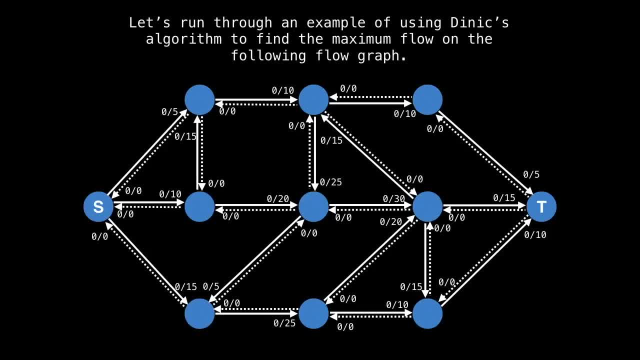 an example, Let's use the next algorithm to find the maximum flow of this flow graph. If this were a bipartite graph, we would also be able to get a maximum matching as a result. All right, step one is to figure out which edges are part of the current level graph. 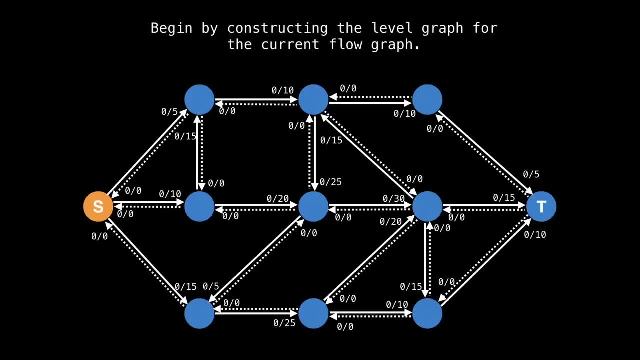 you don't need to think of the level graph as a totally separate graph. you can think of it rather as a subset of the edges. So we start at the source and do a breadth first, search outwards. The first layer includes all the red nodes, then this is the second. 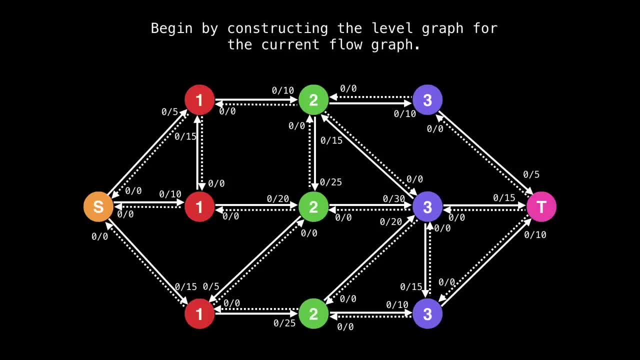 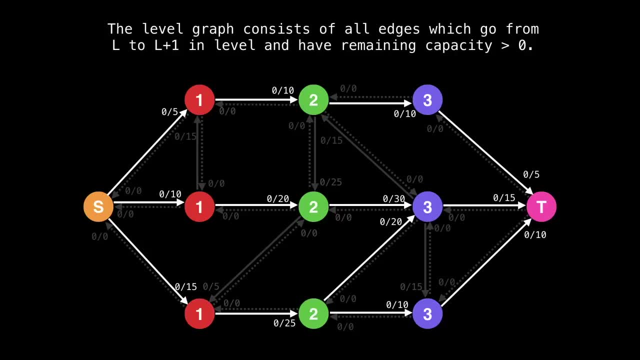 layer and so on until we reach the sink. Now, if we focus on the edges which form the level graph, we'll see that they are all edges which go from L to l plus one and level and have a remaining capacity greater than zero. Step two of the algorithm is to find paths from. 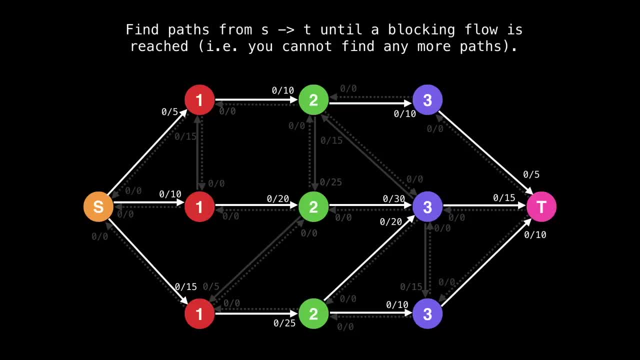 s to t until a blocking flow is reached, That is, we cannot find any more paths through the level graph. So we start at the source and do a depth first search on the edges of level graph until the sink is reached. So we found our first. 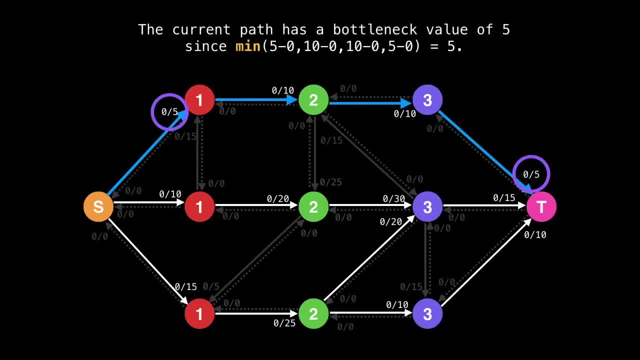 augmenting path and the bottleneck value along this path is five, since five is the smallest remaining capacity. So update the flow values along the path by five. If you inspect the graph, the blocking flow has not yet been reached, Since there still exists paths from. 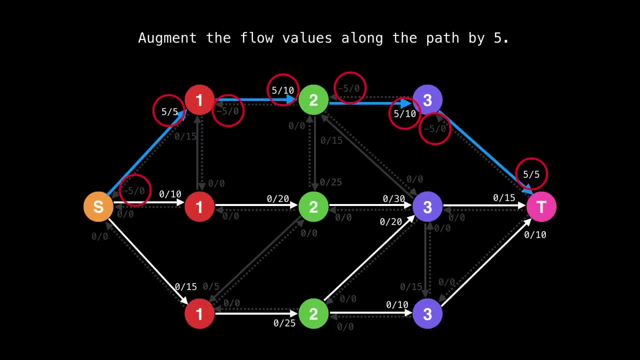 capacity. So update the flow values along the path by five. If you inspect the graph, the blocking flow has not yet been reached. Since there still exists paths. It's from s to t. Start once again at the source and do a depth for search forwards. 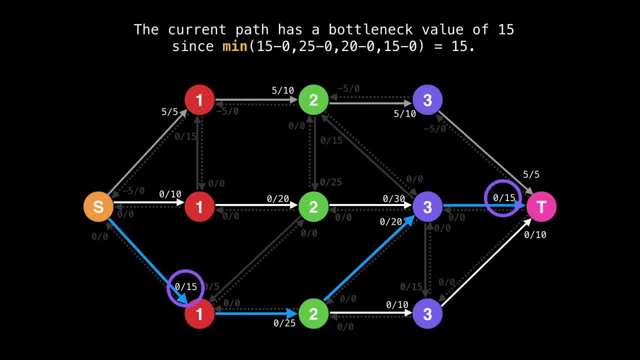 Now we found another path. This one has a bottleneck value of 15. So augment the flow along the path by 15 units. Now let's try and find another path from s to t. What happens now is that we get stuck performing the. 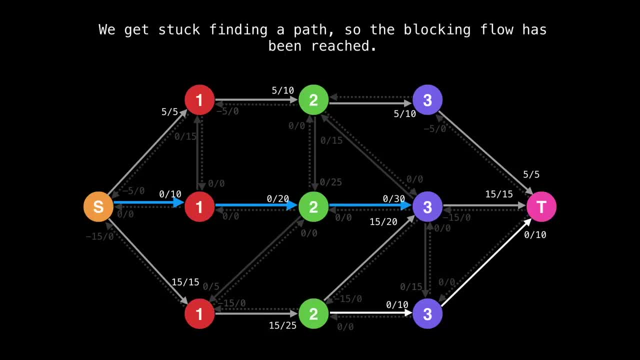 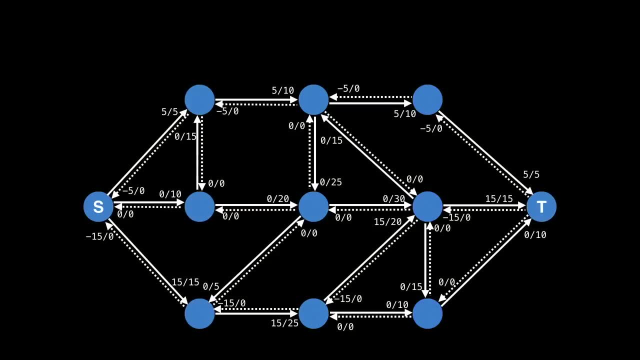 depth first search. there are no edges in the level graph with a remaining capacity greater than zero which can lead us to the sink. So the blocking flow has been reached. We just finished the first blocking flow iteration. Now we reset and rebuild the level graph. 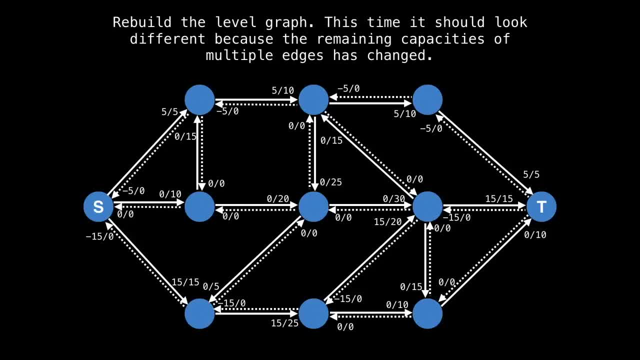 This time it should look different because the remaining capacities of multiple edges has changed. Start the source, expand outwards, taking all edges with a remaining capacity greater than zero, which in this case is zero. So we can see that the remaining capacity 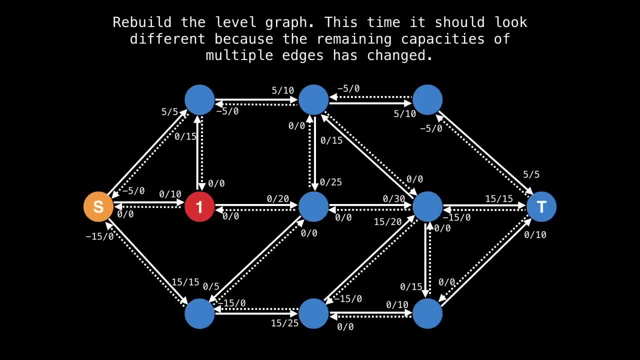 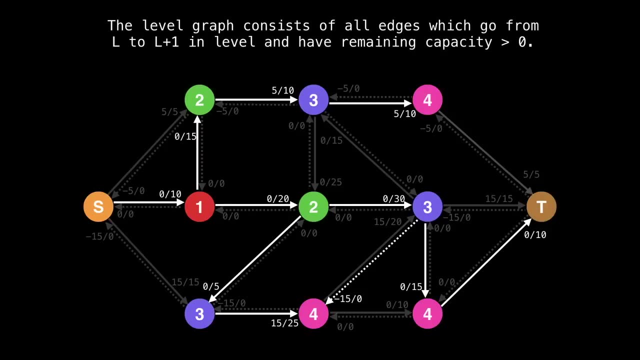 in this case, is only the middle edge leading us to the red node, the top edge going outwards from the source of saturated, and so is the one going downwards. We keep doing this and building the level graph layer by layer. Awesome. So this is our new level graph. you can see that this time we have one extra layer. 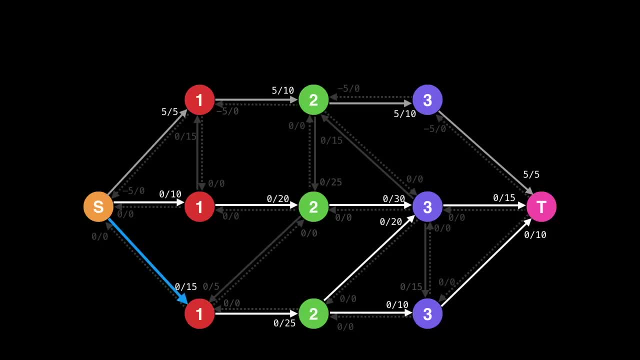 s to t, Start once again the source and do a depth for search forwards. Now we found another path. This one has a bottleneck value of 15. So augment the flow along the path by 15 units. Now let's try and find another path from s to t. What happens now is that 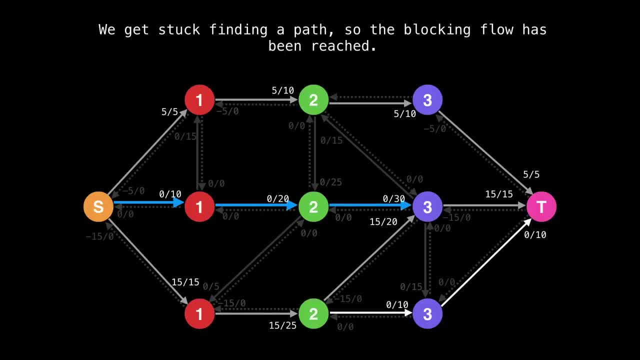 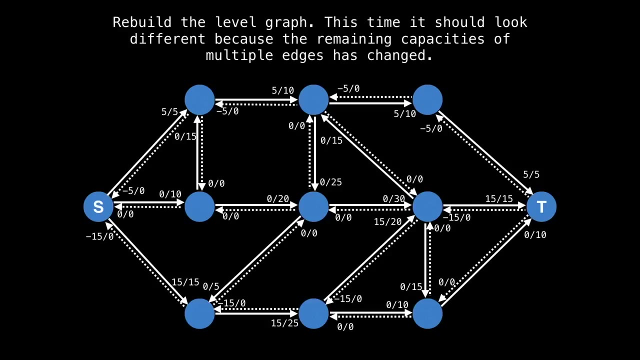 we get stuck performing the depth first search. there are no edges in the level graph with a remaining capacity greater than zero which can lead us to the sink. So the blocking flow has been reached. We just finished the first blocking flow iteration. Now we reset and rebuild the level graph. This time 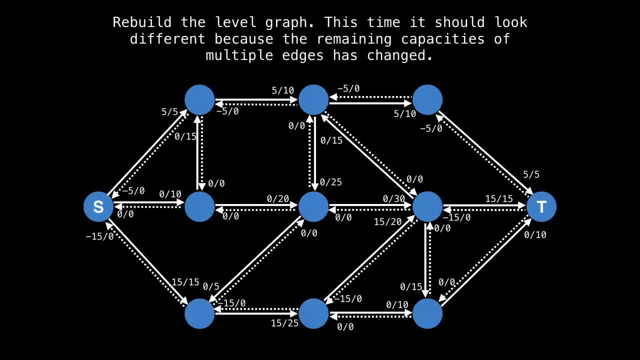 it should look different because the remaining capacities of multiple edges has changed. Start the source, expand outwards, taking all edges with a remaining capacity greater than zero, which in this case is only the middle edge, leading us to the red node, the top edge. going outwards from the sources saturated and so is the one going downwards. We keep. 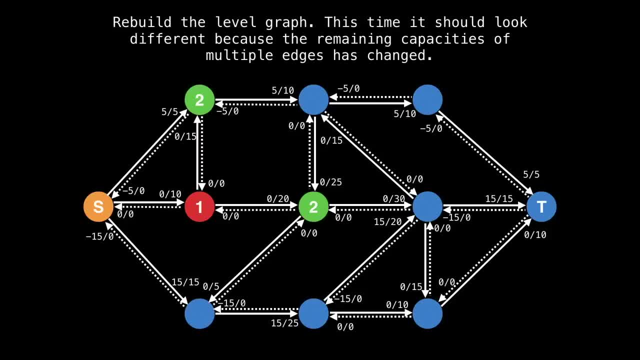 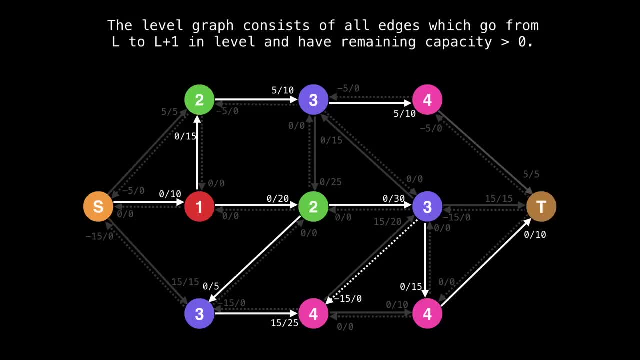 doing this and building the level graph layer by here layer- Awesome. So this is our new level graph. you can see that this time we have one extra layer to play with. Let's try and find a path from s to t. Once again, we started the source. 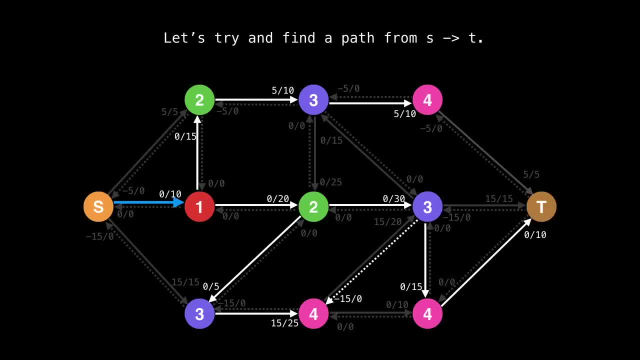 and probe forwards using only edges part of the level graph. Oops, we have now reached a dead end in our depth first search, because we can no longer go forwards. What we need to do is backtrack and keep going until we reach the sink. Perfect, we made it to the sink. the current path has a bottleneck value of 10.. Now augment. 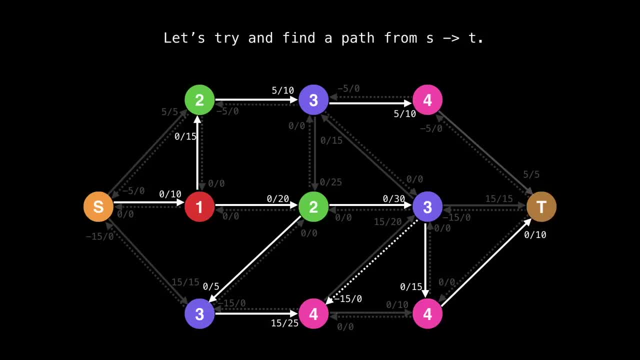 to play with. Let's try and find a path from s to t. Once again. we started the source and probe forward Using only edges part of the level graph. Oops, we have now reached a dead end in our depth first search, because we can no longer go forwards. What we need to do is backtrack. 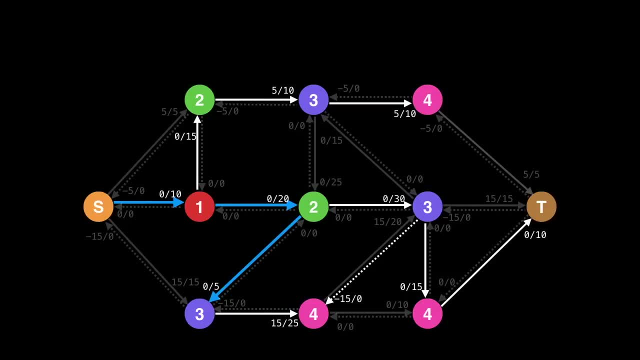 and keep going until we reach the sink. Perfect, we made it to the sink. The current path has a bottleneck value of 10.. Now augment the flow by 10 units And now, if you inspect the flow graph, you will notice that the blocking flow has once again been reached. Now no more. 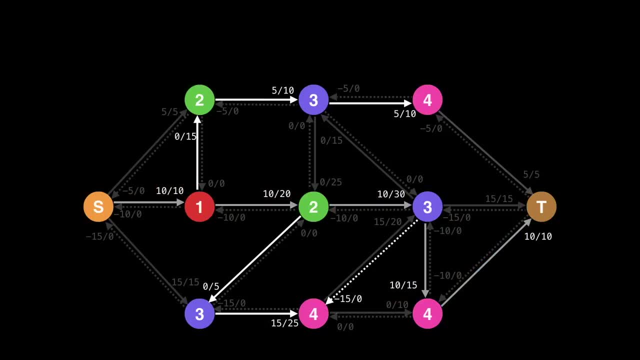 the flow by 10 units. And now, if you inspect the flow graph, you will notice that the blocking flow is not the same as the previous flow graph. So you can see that the flow graph has once again been reached. Now no more flow can be pushed through the network when we 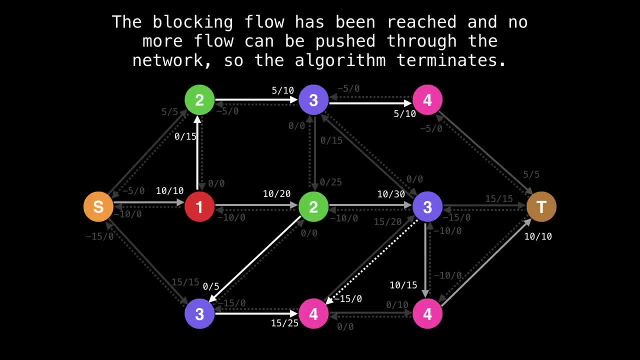 build a level graph, which means the algorithm terminates. The maximum flow is the sum of all the bottleneck values which, if you recall, were 515 and 10, for a maximum flow of 30. Maximum flow can also be calculated by looking at the flow values of the edges leading into. 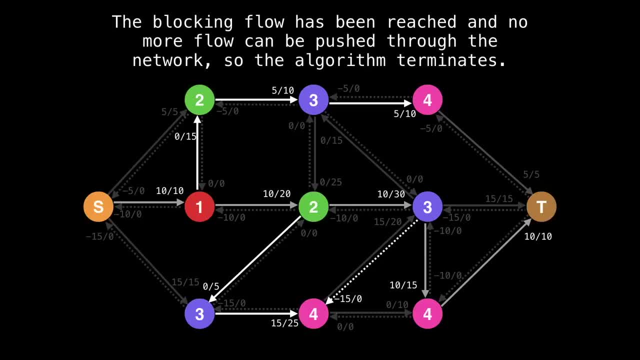 flow can be pushed through the network when we build a level graph, which means the algorithm terminates. The maximum flow is the sum of all the bottleneck values which, if you recall, were 515 and 10.. For a maximum flow of 11.. 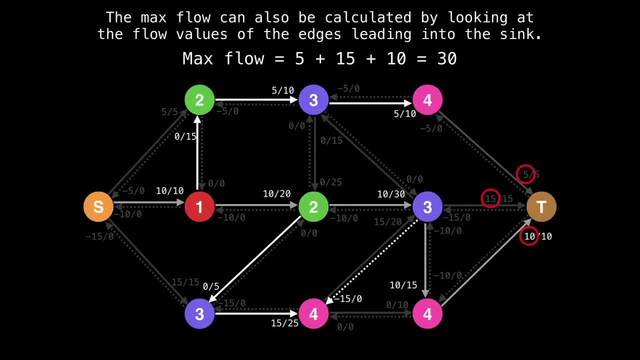 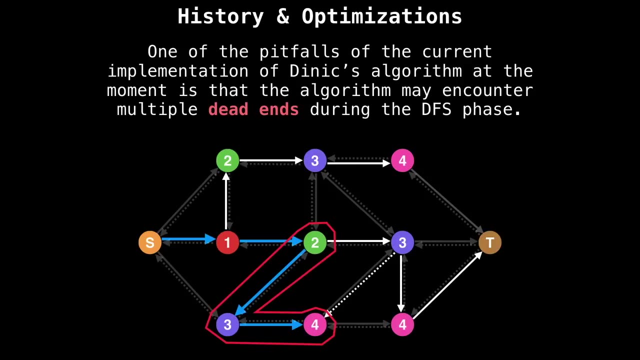 30. Maximum flow can also be calculated by looking at the flow values of the edges leading into the sink highlighted in red on the slide. However, one of the pitfalls of the current implementation of Linux algorithm at the moment is that it may encounter multiple dead ends. 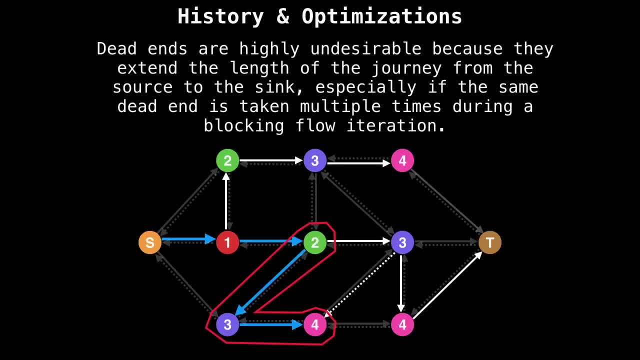 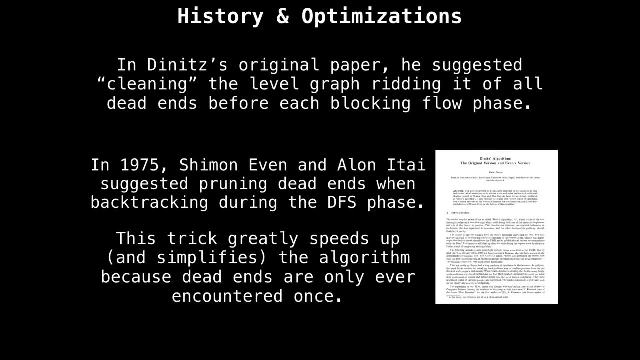 during a depth first search phase. This is especially bad if the same dead end is taken multiple times during a blocking flow iteration. To resolve this issue in his original paper didn't suggested cleaning the level graph and getting rid of all the dead ends before. 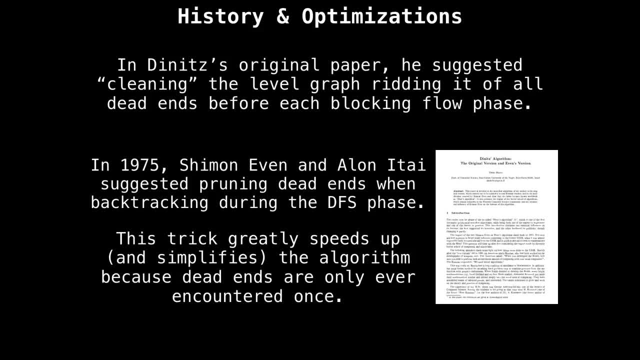 each blocking flow phase. Then later in 1975, Simon Evan suggested pruning dead ends when backtracking during the depth first search phase. effectively getting rid of dead ends on the fly As the algorithm executes this trick greatly speeds up and simplifies the algorithm because 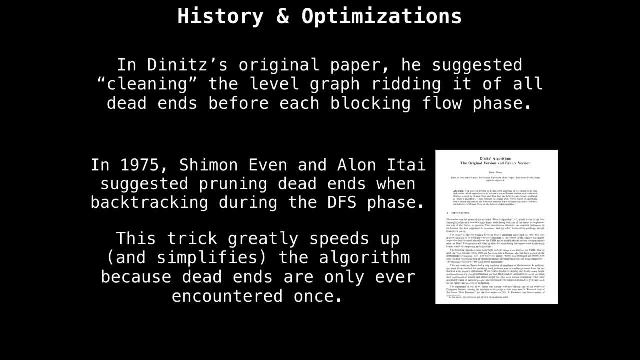 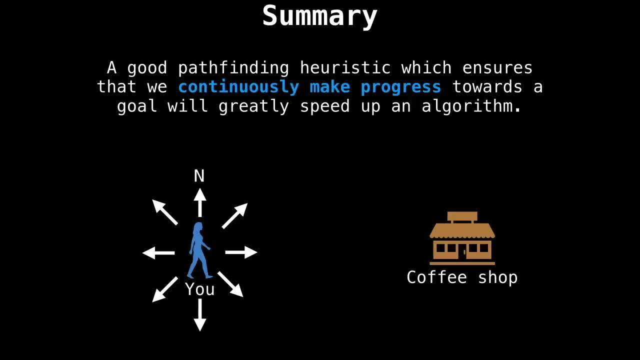 dead ends are only ever encountered once. Awesome, So that's basically everything you need to know about Linux. So let's summarize everything that we've learned. First, we talked about the motivation behind Linux and why having a guiding heuristic can greatly speed. 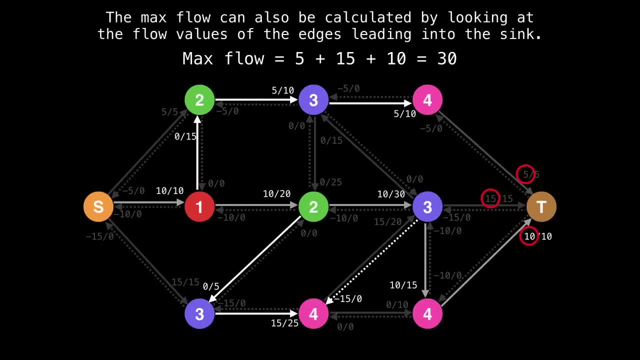 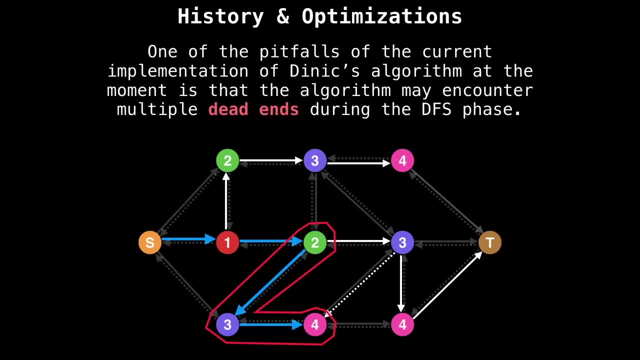 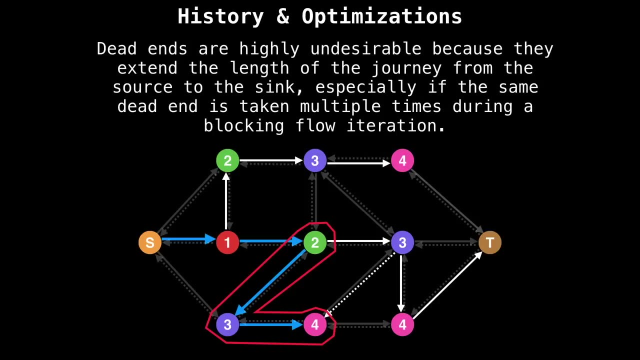 the sink. However, one of the pitfalls of the current implementation of the next algorithm at the moment is that it may encounter multiple dead ends during a depth first search phase. This is especially bad if the same dead end is taken multiple times during a blocking flow. 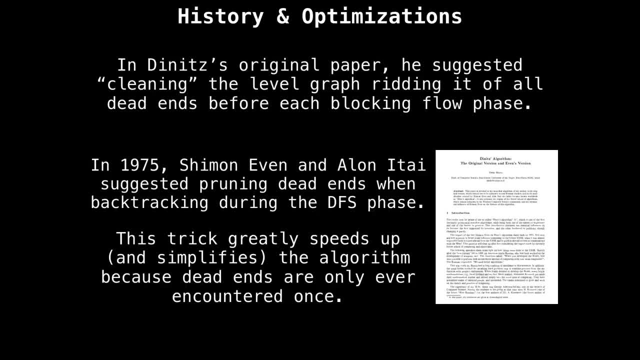 iteration To resolve this issue. in his original paper didn't suggested cleaning the level graph and getting rid of all the dead ends before each blocking flow phase. Then later in 1975, Simon Evan suggested pruning dead ends when backtracking during the depth first search phase, effectively getting rid of dead ends on the fly as the 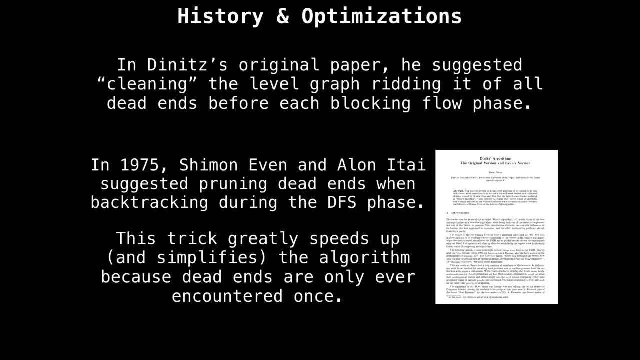 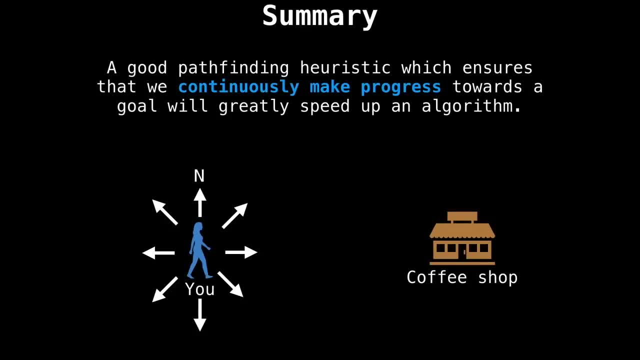 algorithm executes. This trick greatly speeds up and simplifies the algorithm, because dead ends are only ever encountered once. Awesome, So that's basically everything you need to know about Dynx. So let's summarize everything that we've learned. First, we talked about the motivation behind Dynx and why having 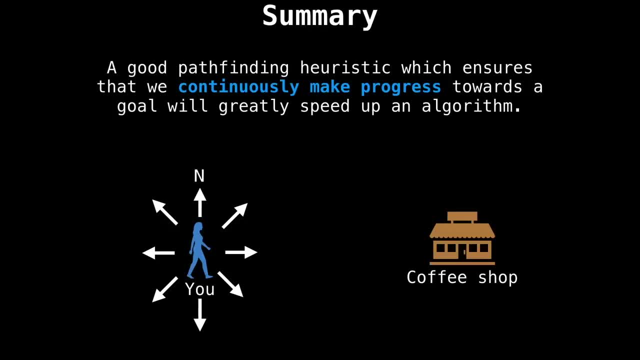 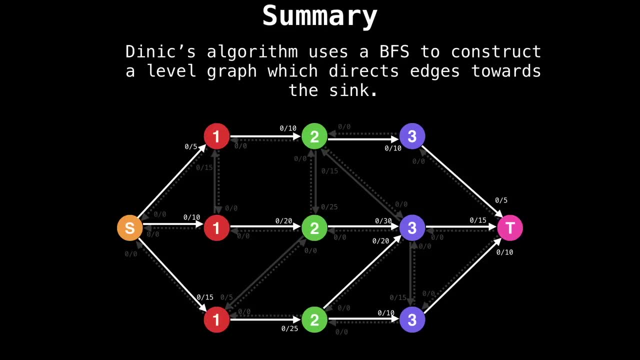 a guiding heuristic can greatly speed up our algorithm. Then we talked about the intuition and practicality behind having a level graph that directs edges towards the sink. Then we talked about the concept of a blocking flow, which is achieved by doing multiple depth searches on the level graph until the graph is saturated. Afterwards we looked at the 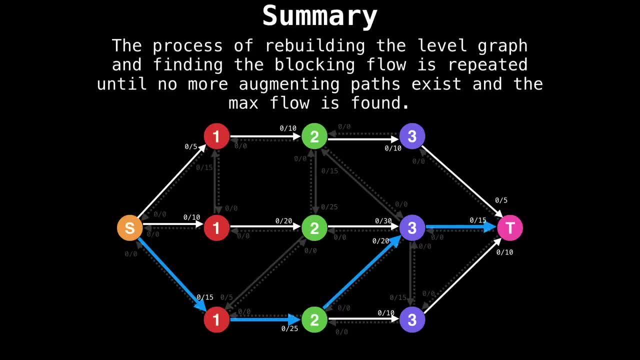 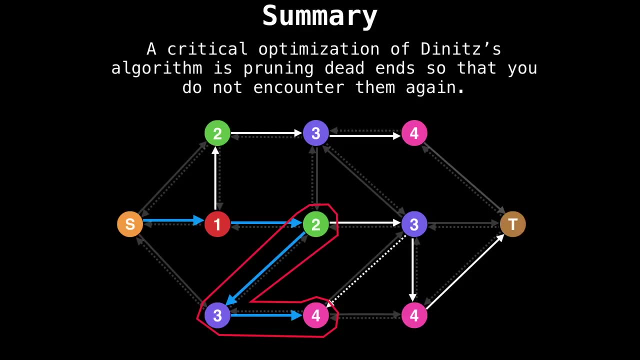 process of rebuilding the level graph and finding the blocking flow, and doing this process repeatedly until no more augmenting paths exist and the maximum flow is found. And lastly, we talked about a critical optimization of dinnits algorithm, which is pruning dead ends. 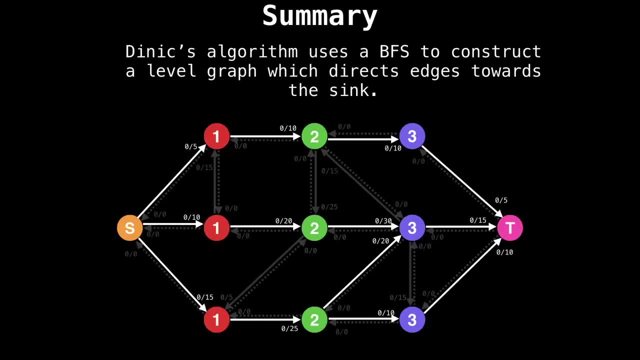 up our algorithm. Then we talked about the intuition and practicality behind having a level graph That directs edges towards the sink. Then we talked about the concept of a blocking flow, which is achieved by doing multiple depth first searches on the level graph, until the 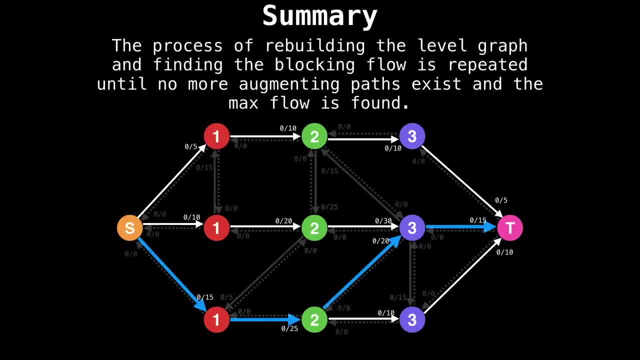 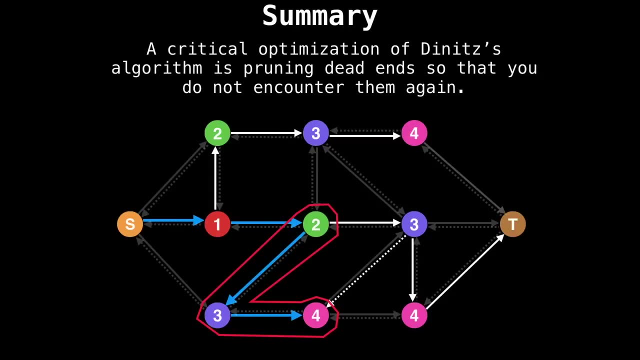 graph is saturated. Afterwards we looked at the process of rebuilding the level graph and finding the blocking flow and doing this process repeatedly until no more augmenting paths exist and the maximum flow is found. And lastly, we talked about a critical optimization. 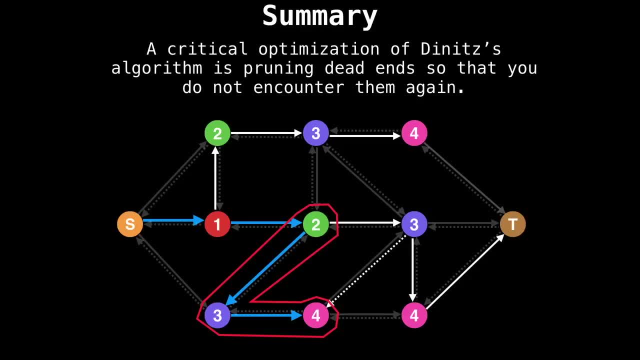 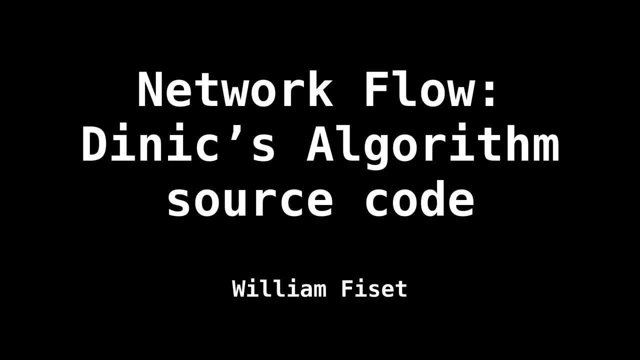 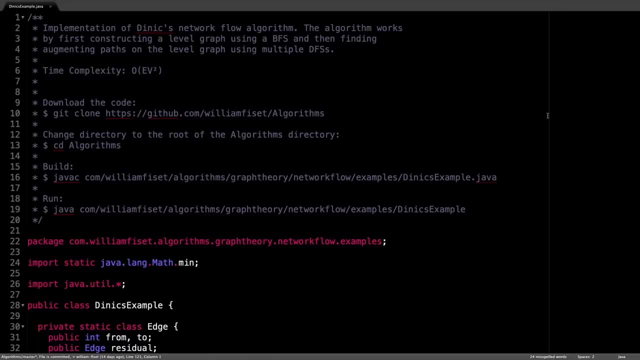 which is pruning dead ends so that we do not encounter them again. Today we're going to have a look at some source code for Dynix algorithm. Okay, let's get started. Here we are in the source code, written in Java. I laid out some instructions here in the header. 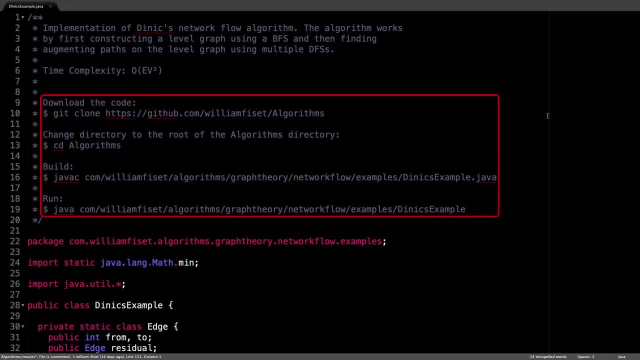 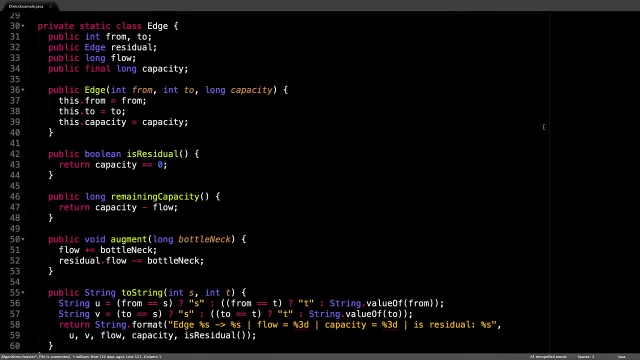 in case you wanted to get the code, play around with it and run it yourself. Scrolling down, as before, you can see the familiar edge here. This class is used to represent an edge that connects two nodes with a certain capacity. It also has two important methods: remaining capacity, which returns the true remaining 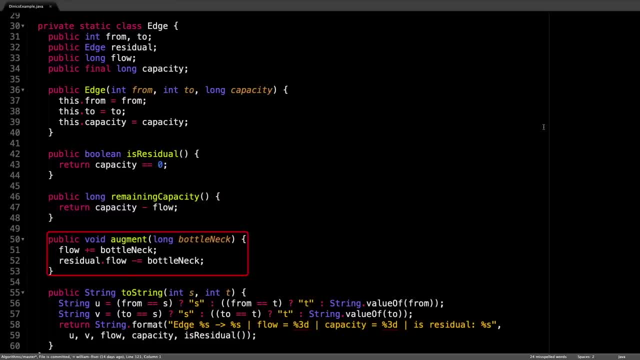 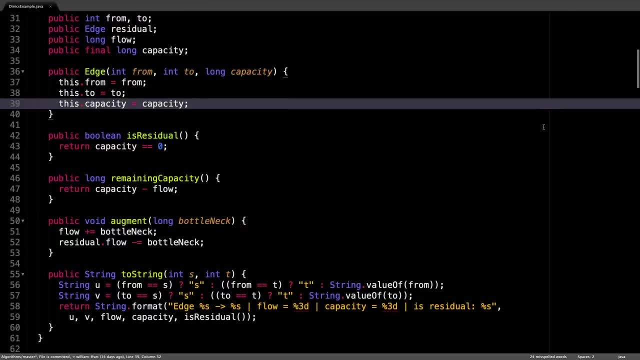 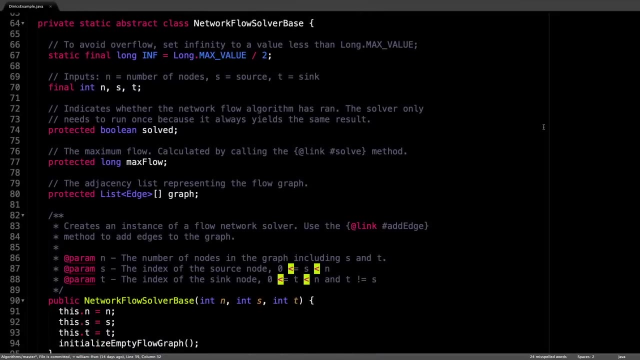 capacity of an edge, along with the augment method, which updates the flow along this edge and also the residual edge by a certain amount. A little further down is also the network flow solver base, which acts as a template For all the different flow algorithms we have been implemented. I already covered how 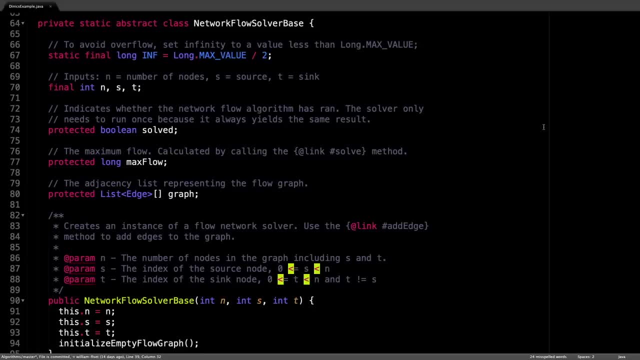 this class and the edge class work in the previous videos linked below, So I won't spend too much time here. But what you need to know is that this class initializes the flow graph, it allows edges to be added to the flow graph and it lets you call the get max flow method. 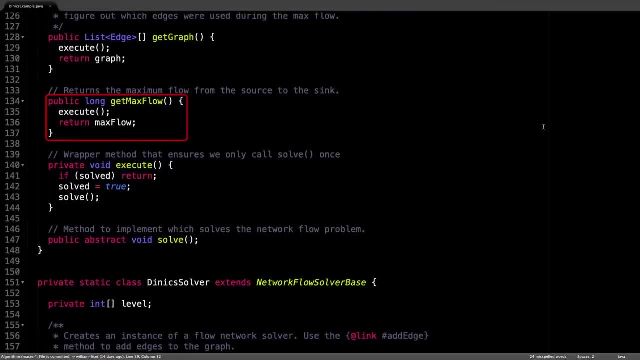 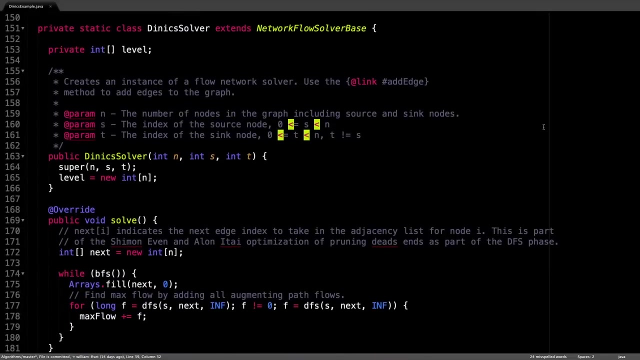 which is somewhere down here. right here, Internally, the get max flow method calls the abstract solve method which we need to implement By subclassing the network flow solver base. So the part we are really interested in is this dinnix solver. right here you will notice that the dinnix solver class extends the network. 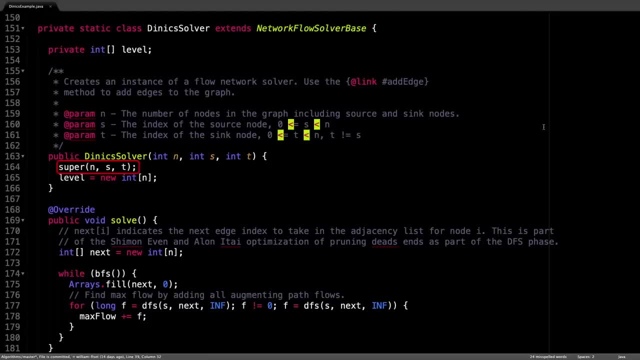 flow solver base. network flow solver base gets initialized. So when we call super by feeding it the three inputs n, s and t, and is the number of nodes in our graph. s is the index of the source node and t is the index of the sink node. 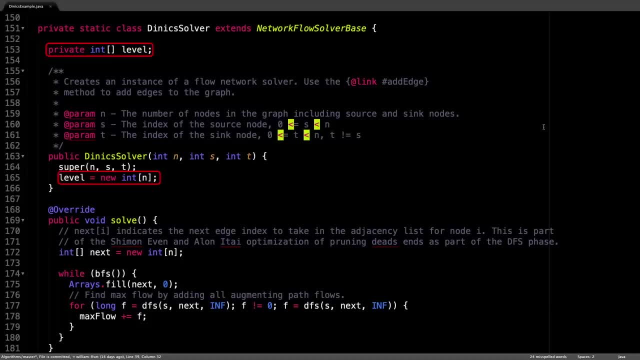 Just after that we'll have a little bit more detail about the index and the index of the sink node. We'll talk about that in a bit. But before we do that let's go ahead and I initialize an array instance variable called level to be a size and the level instance. 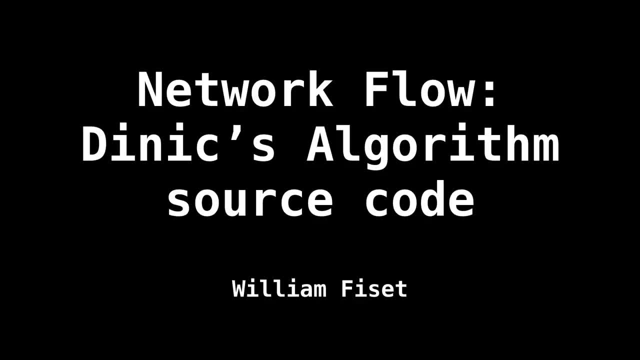 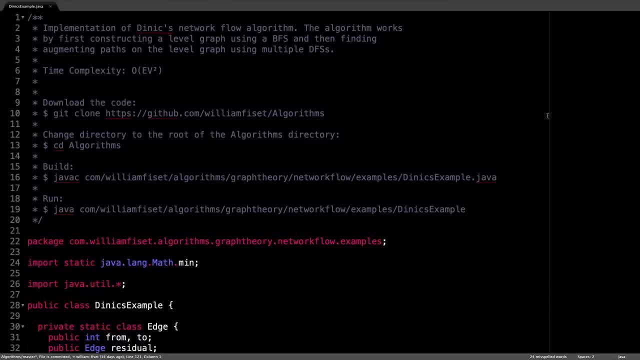 so that we do not encounter them again. Today we're going to have a look at some source code for dinnits algorithm. Okay, let's get started. Here we are in the source code written in Java. I laid out some instructions here in the header in case you wanted to get the. 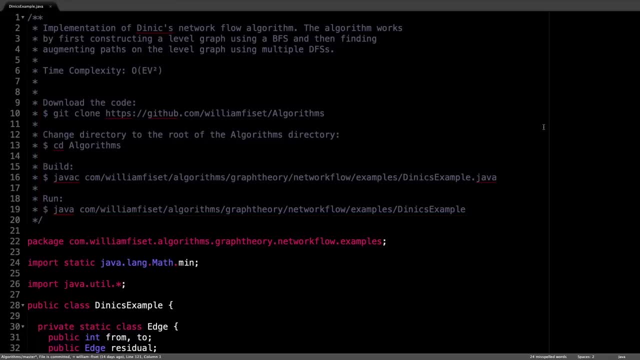 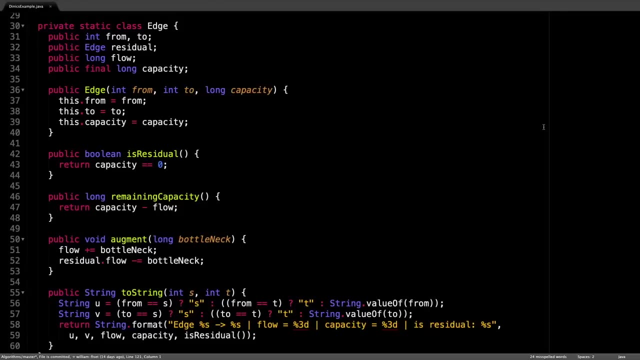 code, play around with it and run it yourself. Scrolling down as before, you can see the familiar edge class. This class is used to represent an edge that connects two nodes with a a certain capacity. It also has two important methods: remaining capacity, which returns. 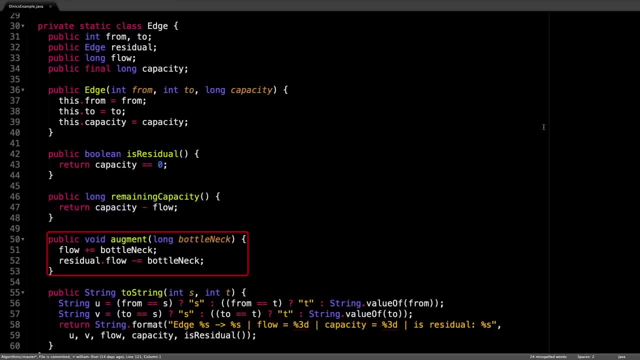 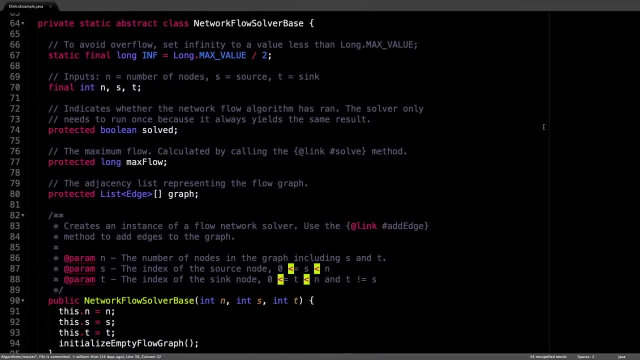 the true remaining capacity of an edge, along with the augment method which updates the flow along this edge and also the residual edge by a certain amount. A little further down is also the network flow solver base, which acts as a template for all the different flow algorithms we have been implemented. I already covered how this class 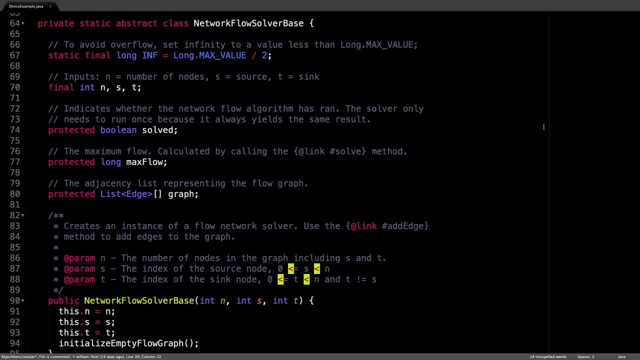 and the edge class work in the previous videos linked below, So I won't spend too much time here. But what you need to know is that this class initializes the flow graph, it allows edges to be added to the flow graph And it lets you call the get max flow method, which 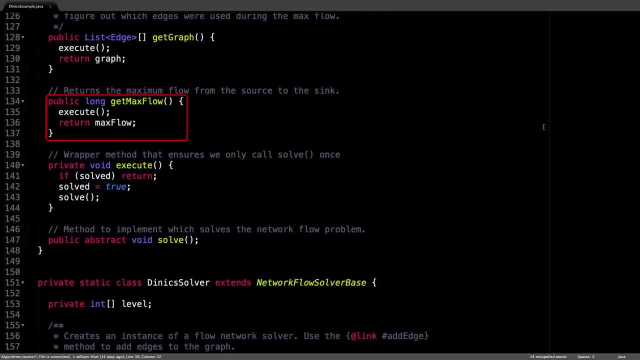 is somewhere down here, right here Internally, the get max flow method calls the abstract solid method which we need to implement by subclassing the network flow solver base. So the part that we are really interested in is the flow method. So the flow method is: 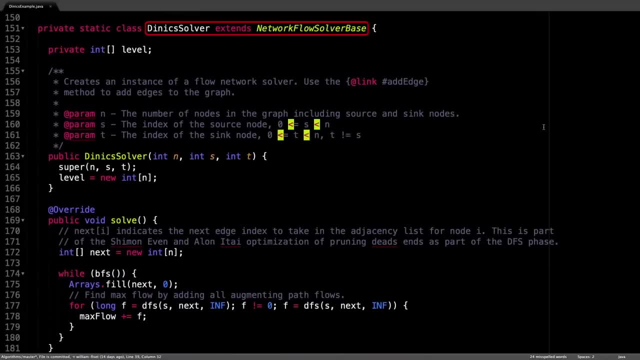 this index solver. right here you will notice that the index solver class extends the network flow solver base. network flow solver base gets initialized. So when we call super by feeding it the three inputs n, s and t, and is the number of nodes. narrow graph s is: 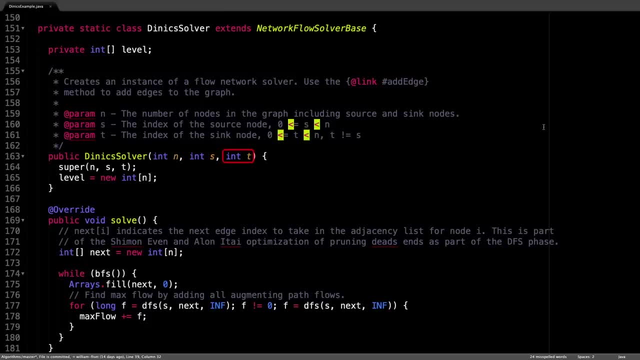 the index of the source node and t is the index of the sync node. Just after that, I initialize an array instance variable called level to be a size n. Then I initialize another instance variable called level to be a size n, and then I initialize: 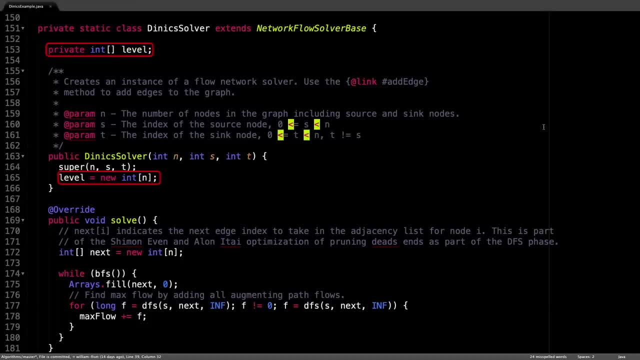 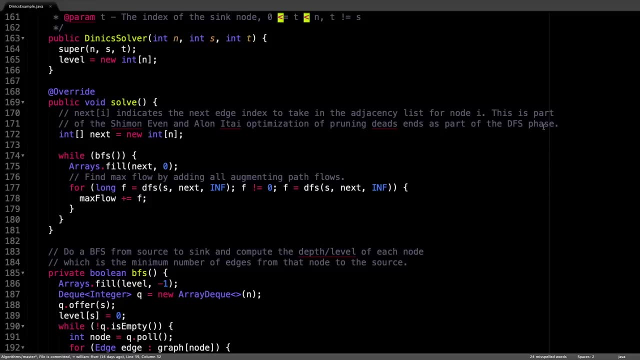 an array instance variable called level to be a size n and then I initialize another instance. the level instance variable keeps track of the level of each note. Now we're a level graph. Moving on. the following method is the solve method. Recall that this is the. 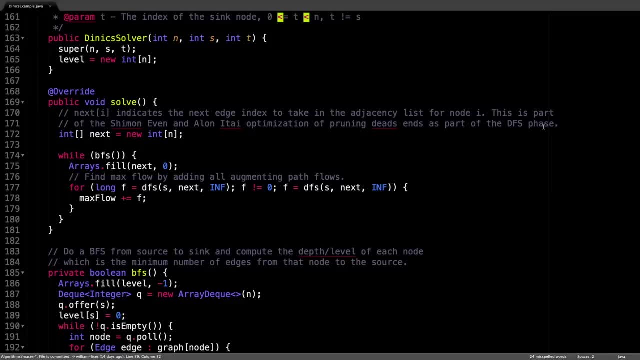 method that we need to override and compute the maximum flow in. Remember what we're trying to do. the next algorithm begins by building a level graph using a breadth first search. that is the outer loop, And for each level graph we need to find the blocking flow by. 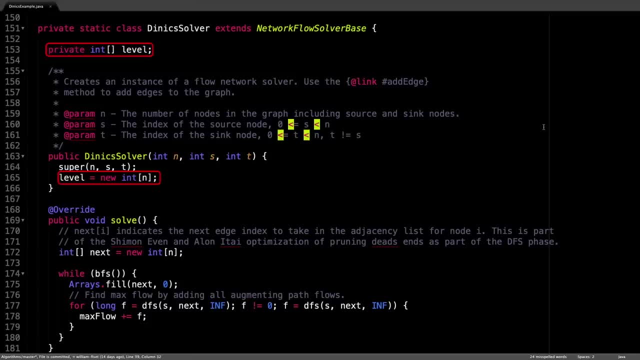 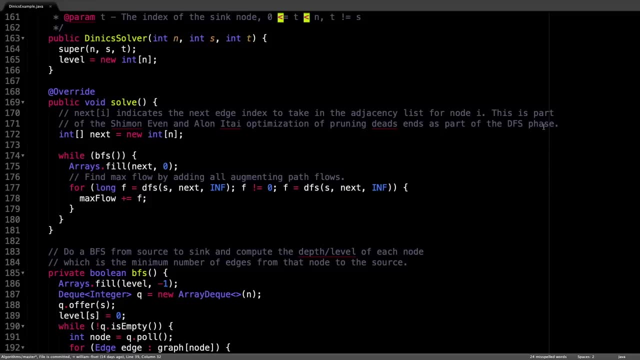 variable keeps track of the level of each node. Now we're a level graph. Moving on, the following method is the solve method. Recall that this is the method that we need to override and compute the maximum flow in. Remember what we're trying to do, didn't algorithm? 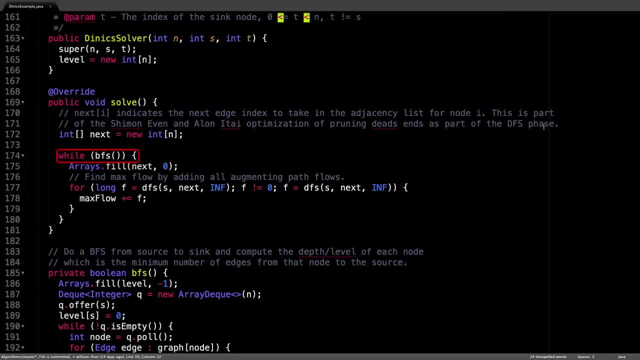 begins by building a level graph using a breadth first search. that is the outer loop And for each level graph we need to find the blocking flow by repeatedly doing multiple depth first searches from the source of the sink until the level graph is saturated and 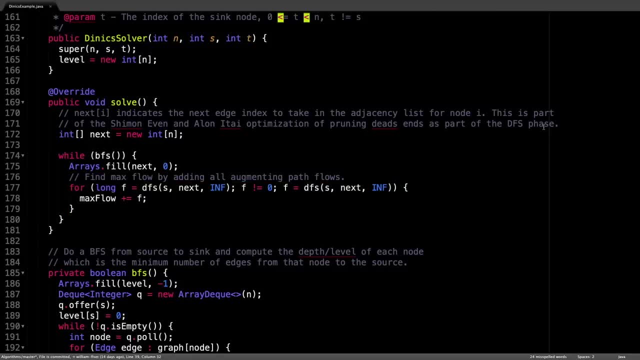 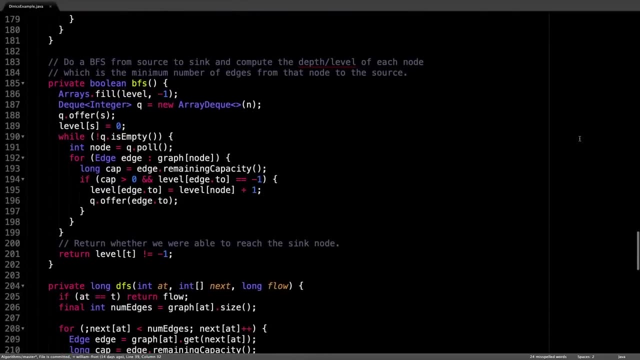 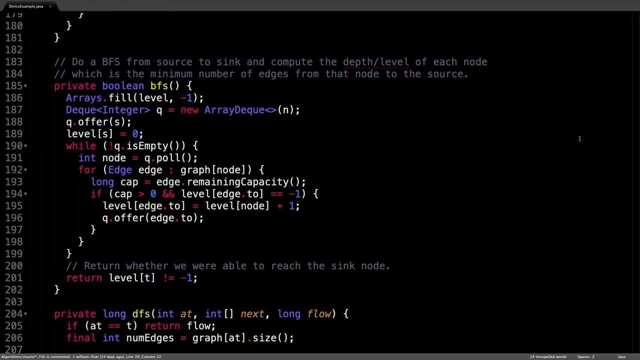 the blocking flow is reached. Once that happens, rebuild the level graph and repeat the process until the graph is truly saturated. Let's have a look at the breadth first search method. So the breadth first search method really serves two purposes. One is to build the level. 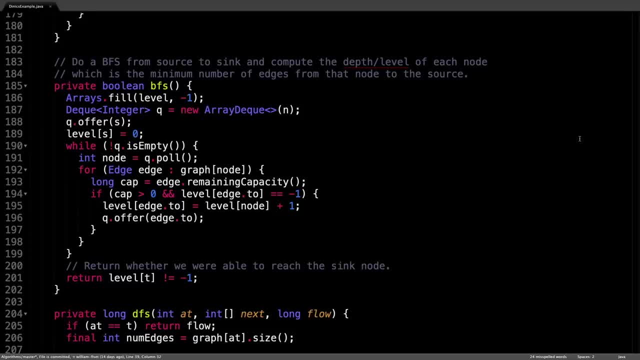 graph and assign a level to each level graph. Next, we'll create a new method called the to each node in the level array, And the other purpose is captured by the return value of the function, And that is to determine if we are able to reach the sink during the breadth. 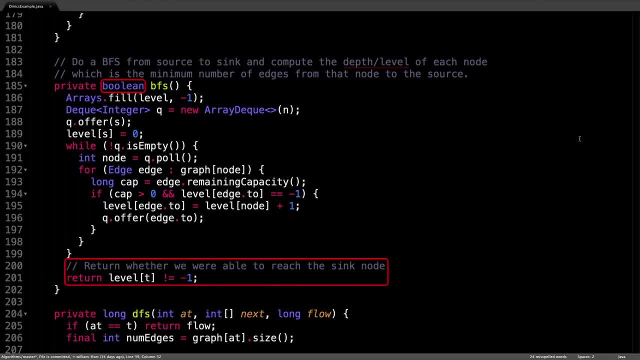 for search phase And if not, this means that the graph is fully saturated and the algorithm can stop. The first thing I do in this method is mark each note as unvisited by setting each entry in the level array to be minus one. then I initialize a queue data structure. 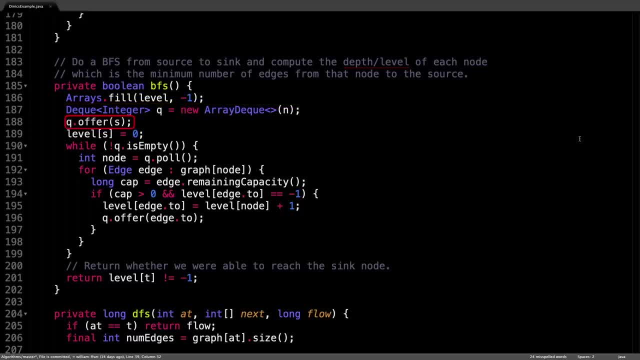 that we will need when performing the breadth first search. After that, I immediately add the source node to the queue. That's because we're starting the breadth first search at the source node. Since we're already at the source node, we can mark the distance to the 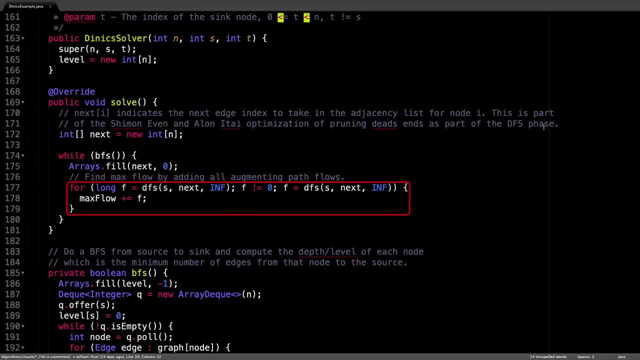 repeatedly doing multiple depth first searches from the source to the sink until the level graph is saturated and the blocking flow is reached. Once that happens, rebuild the level graph and repeat the process until the graph is truly saturated. Let's have a look at the 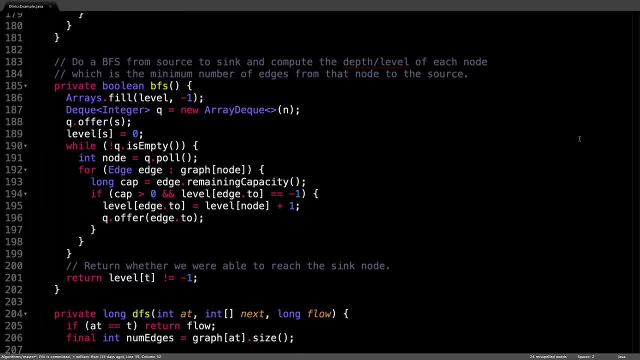 breadth first search method. So the breadth first search method really serves two purposes: One is to build the level graph and assign a level to each node in the level array, And the other purpose is to is captured by the return value of the function, And that is to determine if we are able to. 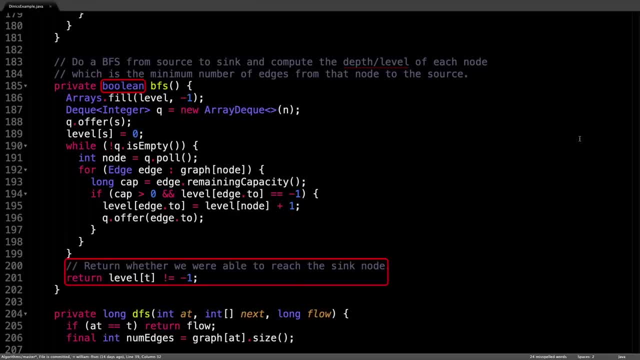 reach the sink during the breadth first search phase And if not, this means that the graph is fully saturated and the algorithm can stop. The first thing I do in this method is mark each note as unvisited by setting each entry in the level array to be minus one. then I 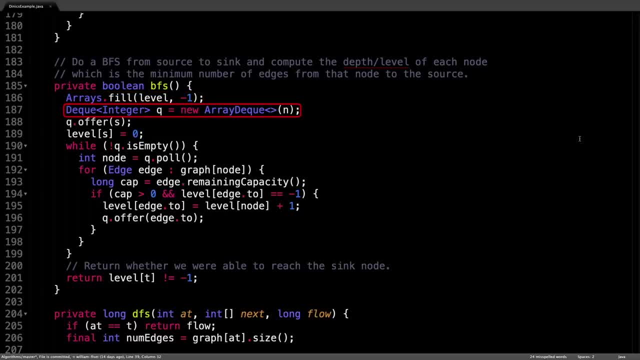 initialize a queue data structure that we will need when performing the breadth first search. After that, I immediately add the source node to the queue. That's because we're starting the breadth first search at the source node. Since we're already at the source node, we can mark the distance to the source node to be zero Once. 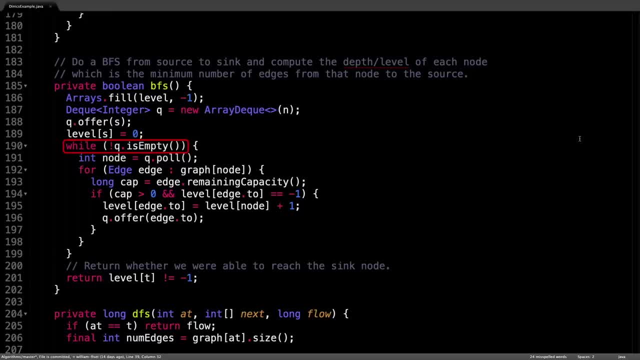 we start the breadth first search loop while the queue is not empty. Each iteration we remove the first node index we find in the queue and iterate through all the adjacent edges of that node. When building a level graph we want to ensure two things. First, 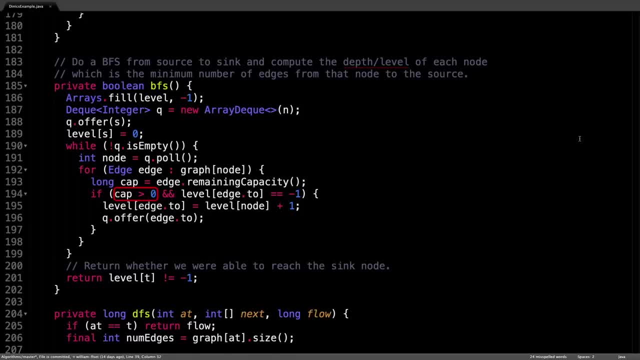 that the remaining capacity of the edges we take are greater than zero and that we are selecting Unvisited nodes. If both those cases hold, then we can compute the level for that node we're about to visit and add it to the queue. This process continues until the queue is. 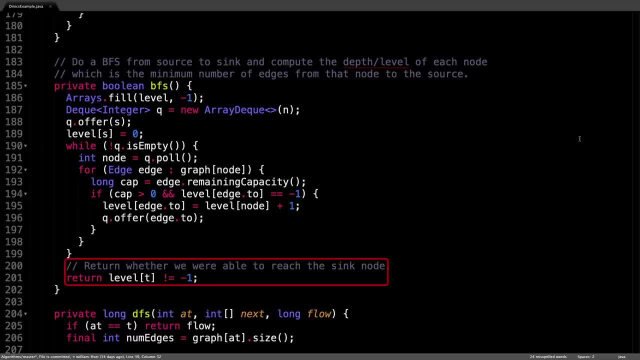 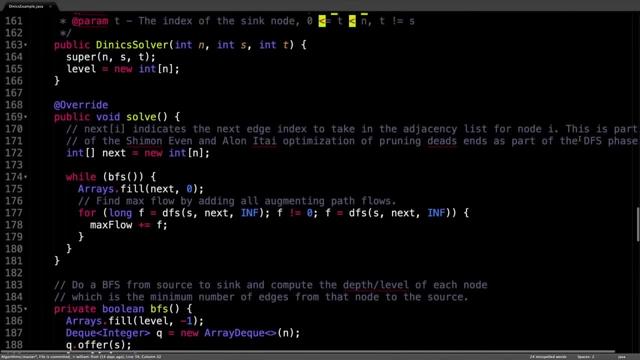 empty and the entire level graph is built. The last thing we do is return if we were able to reach the sink node during the breadth first search phase. Okay, coming back to the solve method, Now we understand how the breadth first search method works and how the level. 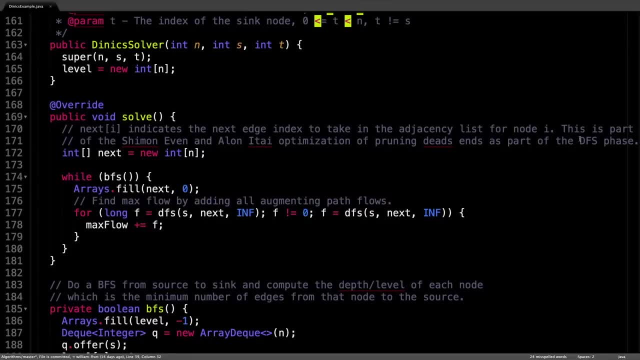 graph is constructed. Now let's have a look at the depth first search method. However, before we do that, there's a key piece of information you need to know about, And that is the next array in this method. The next array is part of the Scheinman Evan. 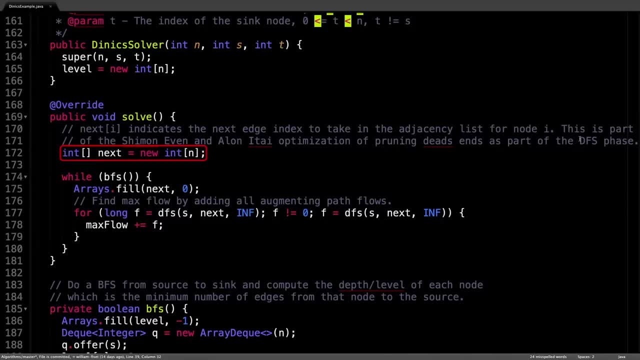 optimization, And it is how we are able to prune dead ends efficiently. The idea is that, since our graph is stored as an adjacency list, the list of edges going outwards from each node is indexed, And we can use this to our advantage to get the next edge to traverse. 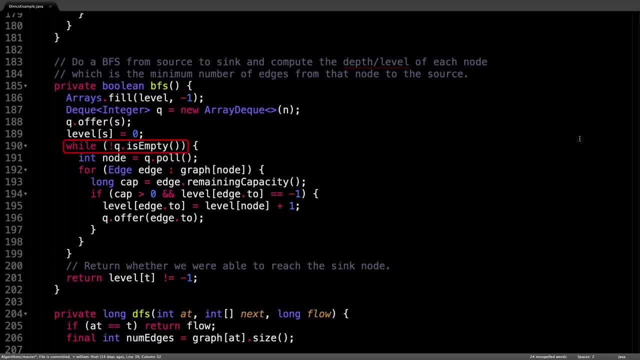 source node to be zero. Once we start the breadth first search loop while the queue is not empty, Each iteration we remove the first node index we find in the queue and iterate through all the adjacent edges of that node. When building a level graph, we 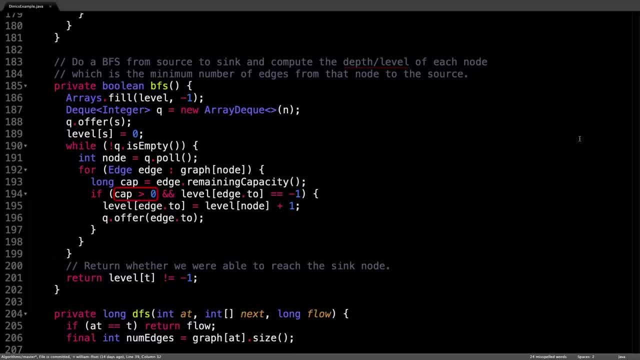 want to ensure two things: First, that the remaining capacity of the edges we take are greater than zero and that we are selecting unvisited nodes. If both those cases hold, then we can compute the level for that node we're about to visit and add it to the queue. This process continues. 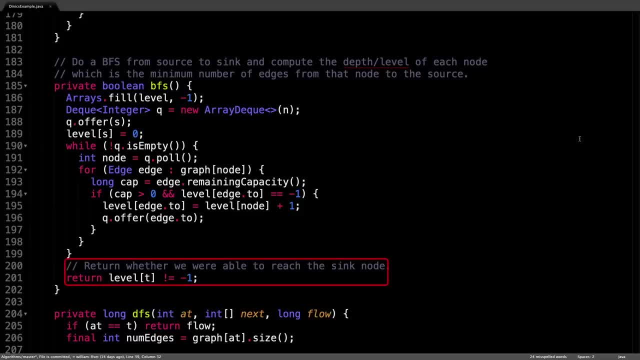 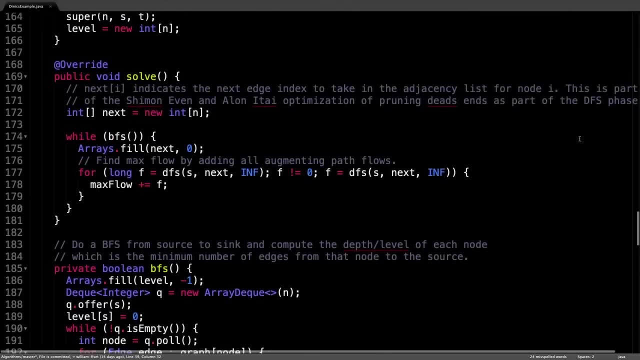 until the queue is empty and the entire level graph is built, The last thing we do is return, if we were able to reach the sink node during the breadth first search phase. Okay, coming back to the solve method. Now we understand how the breadth first search. 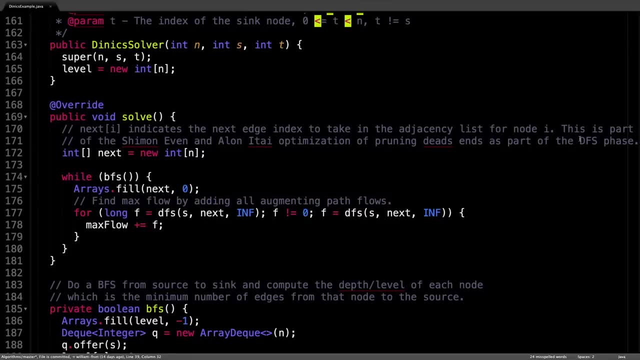 method works and how the level graph is constructed. Now let's have a look at the depth first search method. However, before we do that, there's a key piece of information you need to know about, And that is the next array in this method. The next array is part of the Scheinman. 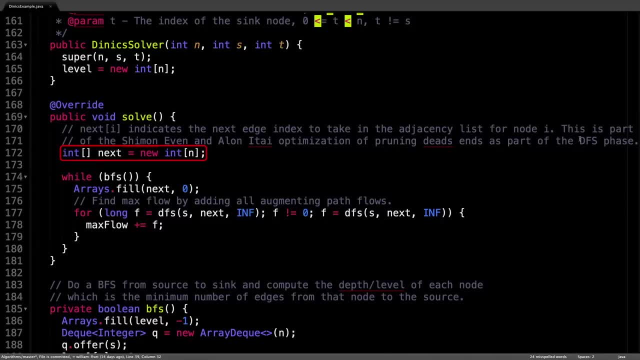 Evan, optimization, And it is how we are able to prune dead ends efficiently. The idea is that, since our graph is stored as an adjacency list, the list of edges going outwards from each node is indexed, And we can use this to our advantage to get the next edge to traverse and skip all the edges which we 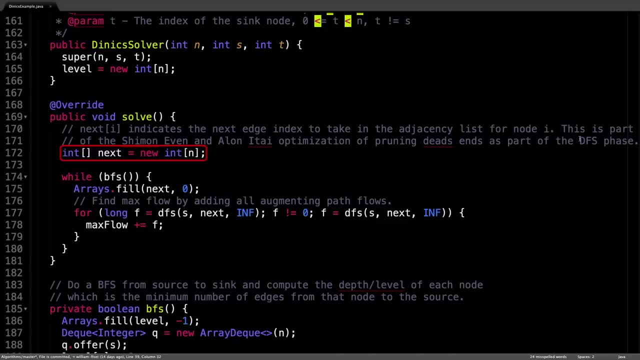 know, lead to dead ends. Say, we're at node I and we take the first edge in our adjacency list for node. I suppose that this turns out to lead us to a dead end. Well, next time, as in the next step, the first search in which we encounter the same node, we should not. 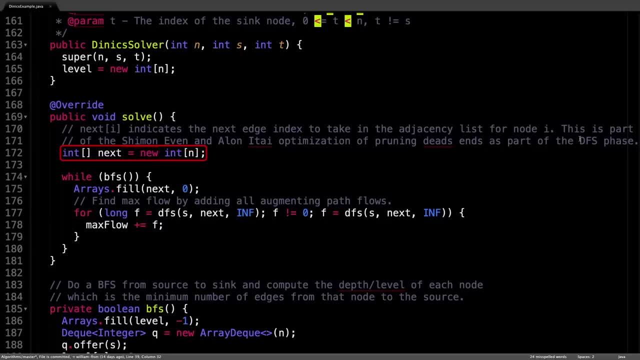 take the first edge in the adjacency list for that node, because we know it will lead us to a dead end. The next array is a way of tracking for each node which edge we should take next each iteration. you want to reset the next. 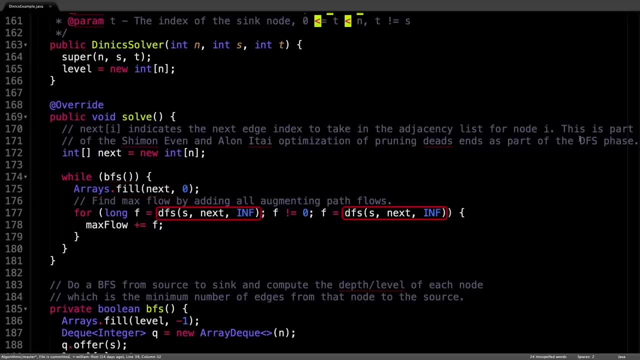 array to allow taking previously forbidden edges. Alright. so we call the depth research method and we pass in three argument: the current node being the source, the next array and the minimum flow along the path which starts at positive infinity. then, for each, 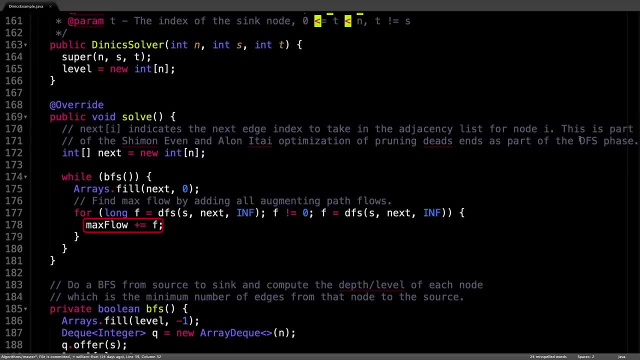 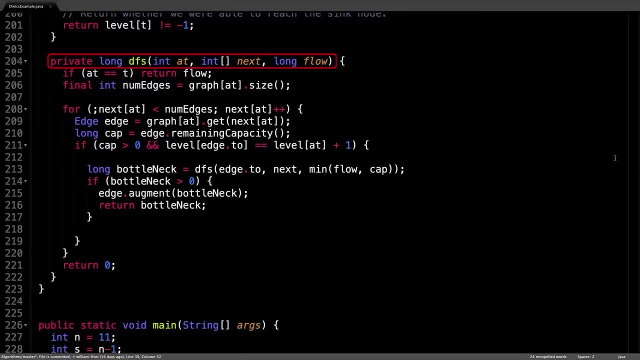 augmenting path that we find some over the bottleneck values to compute the maximum flow. Alright, let's have a look at the depth First search method itself. the depth first search method takes three arguments: the current node, the next array and the minimum flow along the path. So far, this method performs. 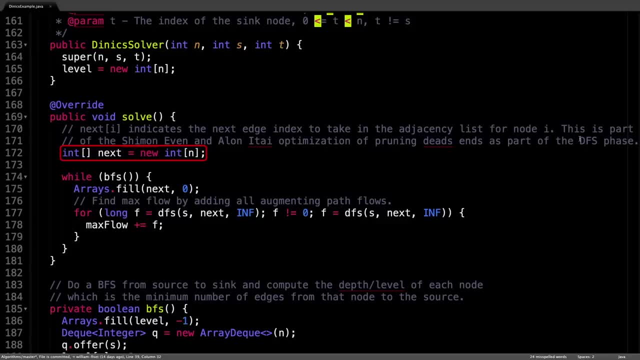 and skip all the edges, which we know are the edges that are going to the next node, And we can use this to our advantage to get the next edge to traverse and skip all the edges which we know are the edges that are going to the next node. So let's see how. 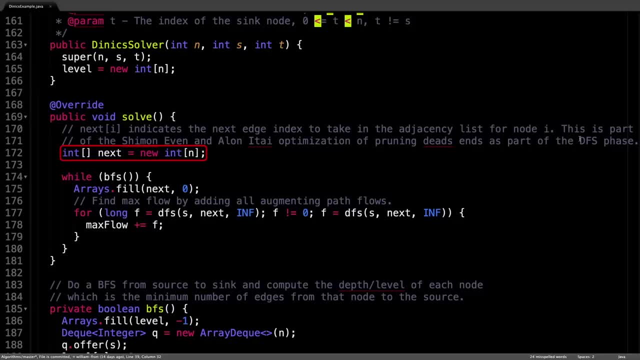 this works. Let's say we're at node i and we take the first edge. now our adjacency list for node. I suppose that this turns out to lead us to a dead end. Well, next time, as in the next step, the first search in which we encounter the same node, we should not. 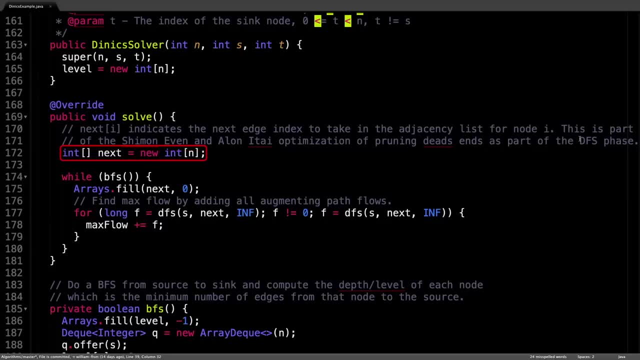 take the first edge in the adjacency list for that node, because we know it will lead us to a dead end. the next array is a way of tracking for each node which edge we should take next each iteration. you want to reset the next array. 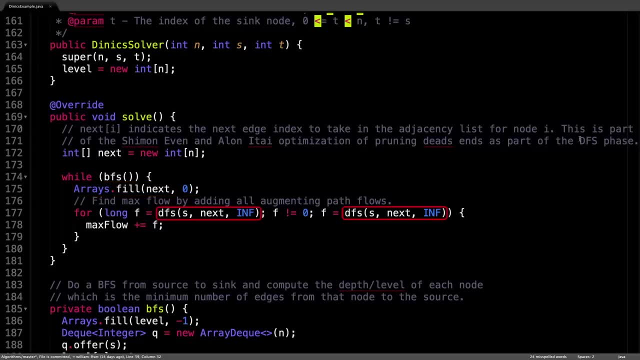 To allow taking previously forbidden edges. Alright. so we call the depth first search method and we pass in three argument: the current node being the source, the next array and the minimum flow along the path which starts at positive infinity. then, for each augmenting path, that 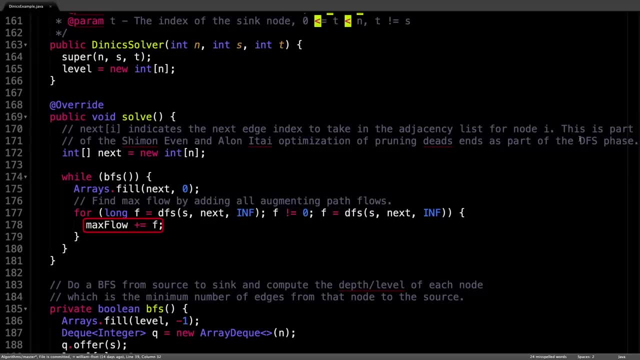 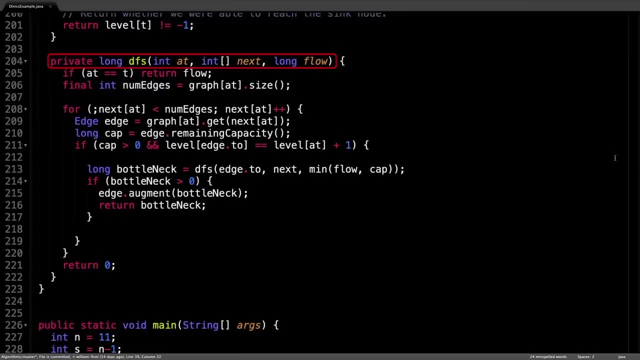 we find some over the bottleneck values to compute the maximum flow. Alright, let's have a look at the depth first search method itself. The depth first search method takes three arguments: the current node, the next array and the minimum flow along the path So far. 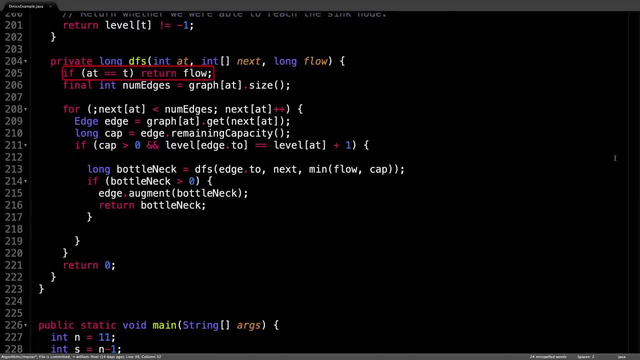 this method performs a breadth first search recursively And we know we can stop searching when we have reached the sink, node t. then I captured the number of edges going out of this node. the for loop loops through all the edges, while we have not tried taking each. 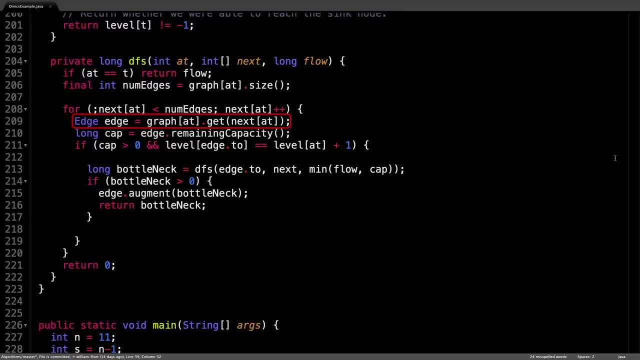 edge or the current node. the next edge to take is the next outgoing edge from this node at the index in the next array. The thing we have to watch out for is that we must ensure that the selected edge has a remaining capacity greater than zero and that it goes up a level. Remember that we're 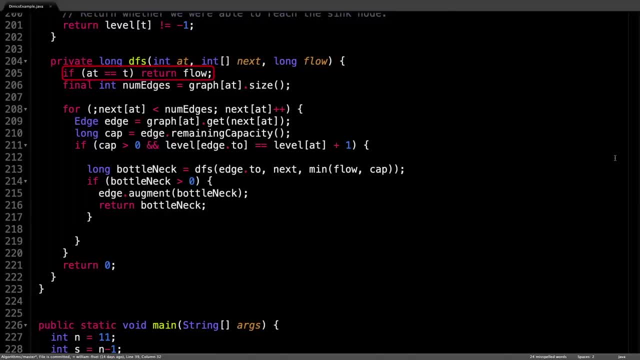 a breadth, first search recursively And we know we can stop searching when we have reached the sink, node t. then I captured the number of edges going out of this node. the four loop loops through all the edges, while we have not tried taking each edge or the current. 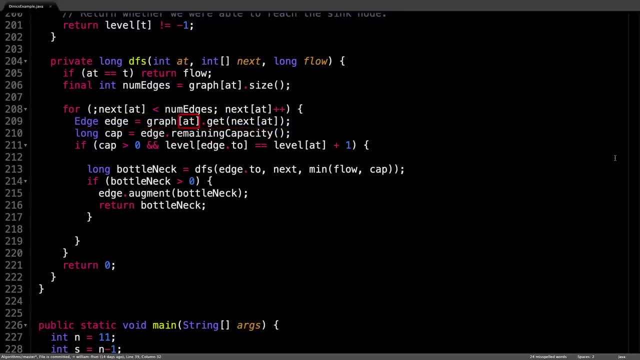 node. the next edge to take is the next outgoing edge from this node at the index in the next array. The thing we have to watch out for is that we must ensure that the selected edge has a remaining capacity greater than zero and that it goes up a level. Remember that we're always trying to make progress. 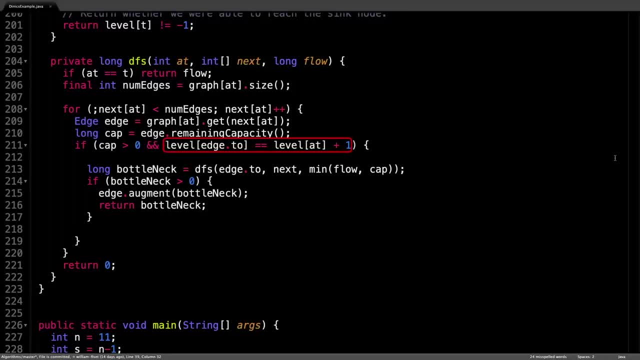 towards the sink and taking an edge at the next level guarantees that, unless of course it leads to a dead end. but we end up pruning those, so it doesn't really matter. So if all goes well, we get to enter the inner if statement. Inside the inner if statement we call the. 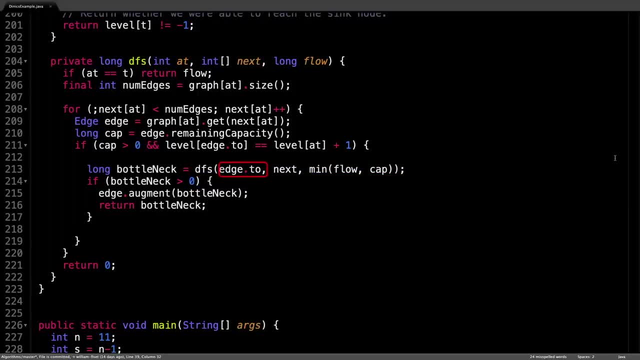 depth first search method, recursively passing in the node we're going to as the current node and the next array and the flow as the minimum of the current flow and edges remaining capacity. the depth first search returns the bottleneck value along the augmenting path. 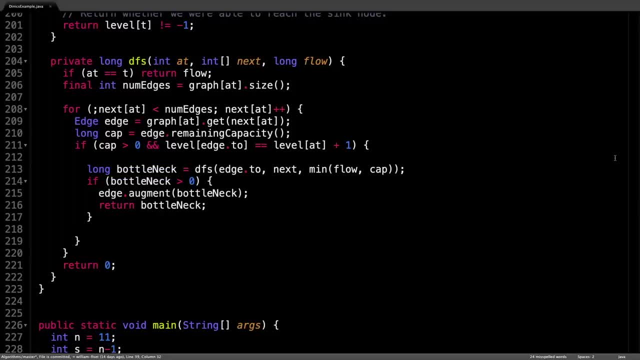 After the this depth first search call, we are unwinding the call stack, if you will, And we're going from the sink back to the wall towards the source. This is a perfect time to augment the flow for each edge along the augmenting path, since we already know what the bottleneck value is. So if the bottleneck 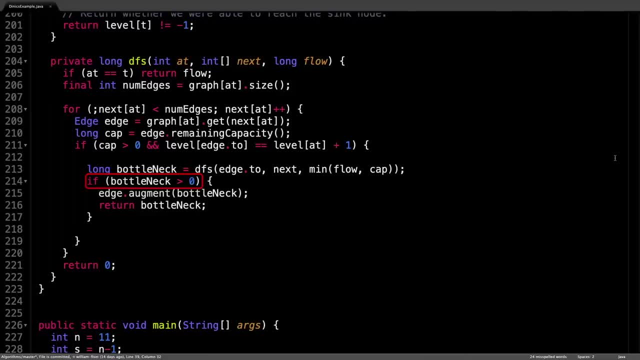 value is greater than zero, meaning we actually found an augmenting path. augment the flow, which means to add flow along the forward edge and subtract flow along the residual edge, And, once all that is done, simply return the bottleneck value. So, assuming we were, 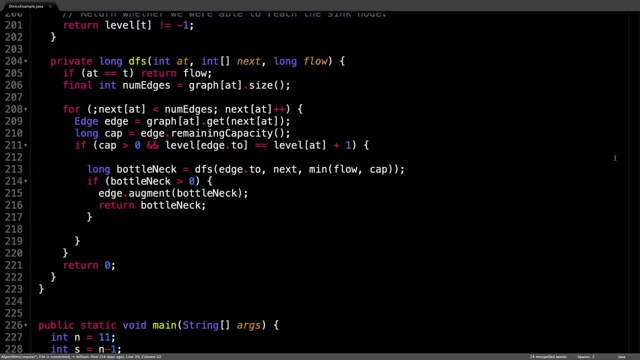 not able to take the selected edge from the current node Because it did not have enough remaining capacity or didn't increase in level, or we hit a dead end, or whatever reason. we need to mark the selected edge as invalid so we can prune it. 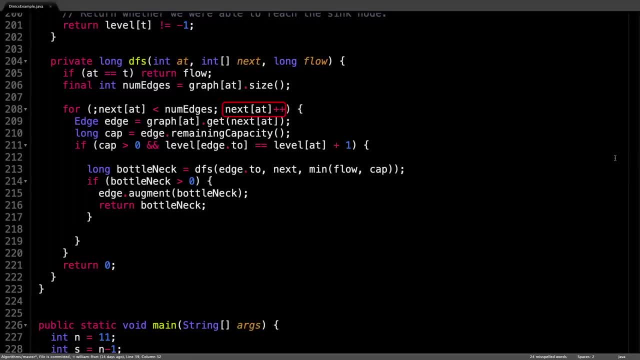 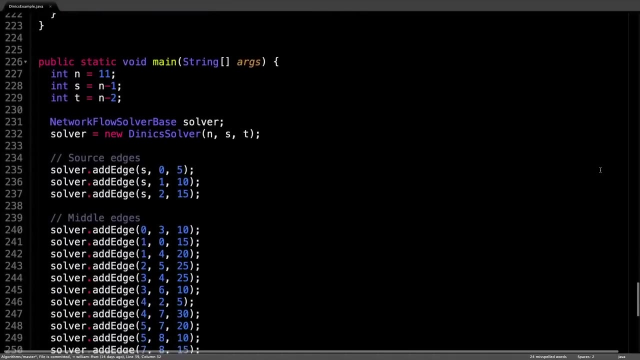 in future iterations. This is exactly what the next plus plus line does, which gets executed after the iteration of the loop. it increments the index of the edge. take at the current node. If we scroll down to the main method, you see that I show you how to set up a flow graph by initializing the flow solver and pushing some. 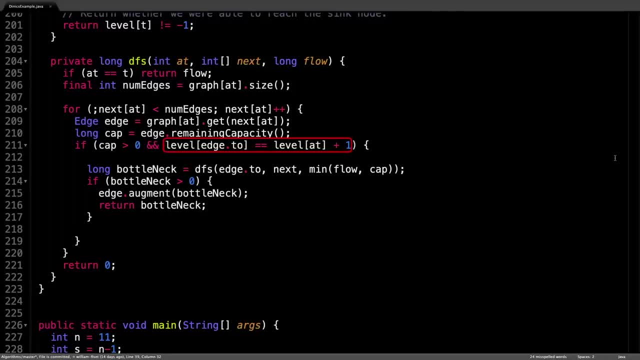 always trying to make progress towards the sink and taking an edge at the next level guarantees that, unless of course it leads to a dead end. but we end up pruning those, so it doesn't really matter. So if all goes well, we get to enter the inner if statement. 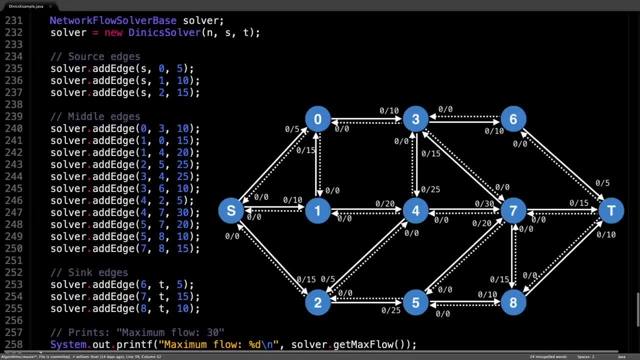 flow through the graph. In particular, this is the flow graph from the slides last video, So you can verify that the maximum flow we get should be 30..